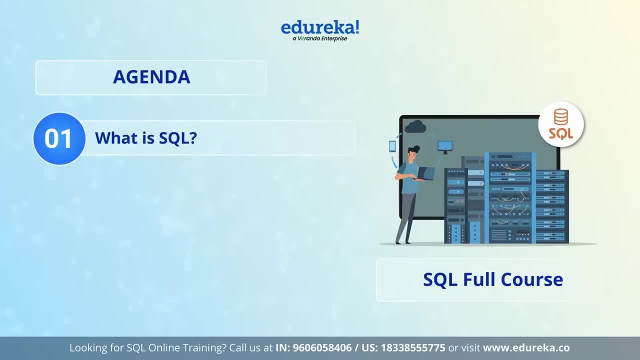 in this full-course video, We'll start by seeing what is SQL. Next we have SQL basics, followed by SQL operators. Now is the time to study deeply into SQL's technical components. We'll start with understanding what is normalization and triggers in SQL. 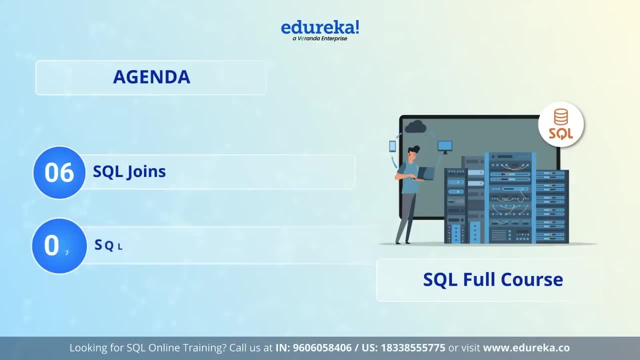 Now, once this is done, we'll understand what are joins and functions in SQL. We will then compare SQL to MySQL and, subsequently, SQL to Toolbox. We hope that this session assists you in getting jobs in the industry. In order to accomplish this, we will look at how a career in SQL works, followed by some 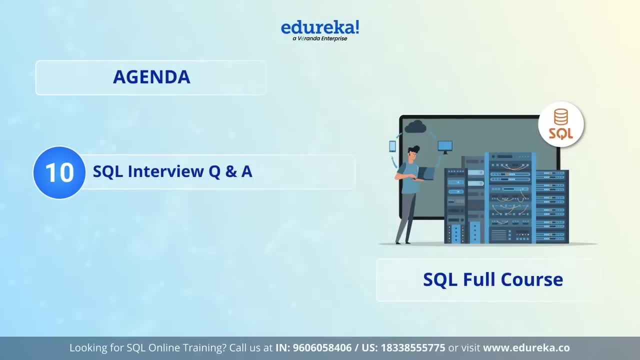 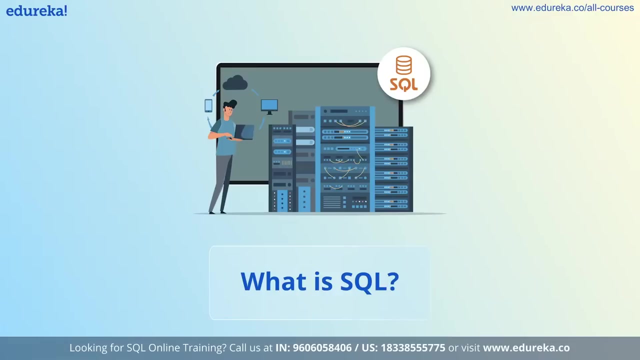 essential SQL interview questions. Now, after all this, we'll head over to how SQL is required in data science, followed by PostgreSQL and SQL Server. At last, we'll look at some SQL Server interview questions with answers. Now let's start with our first topic, that is, what is SQL? 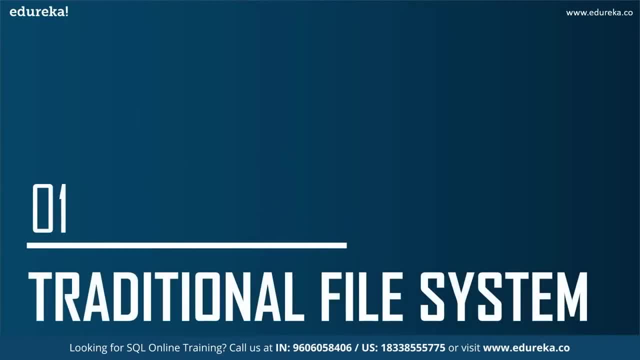 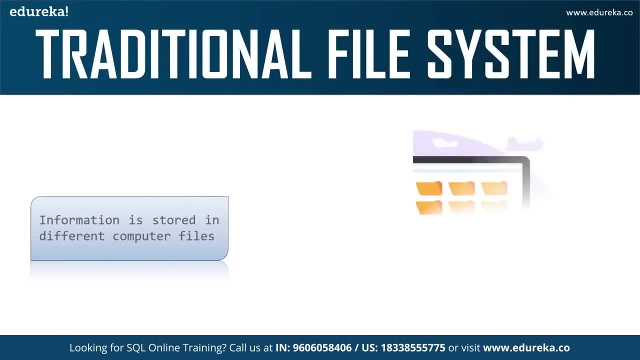 The first topic is traditional file system. in today's computing world, Managing data is a huge task. for our convenience, We store the data and documents in different location, and this is called file system. without a file system, information placed in the storage medium would be one large body of data. 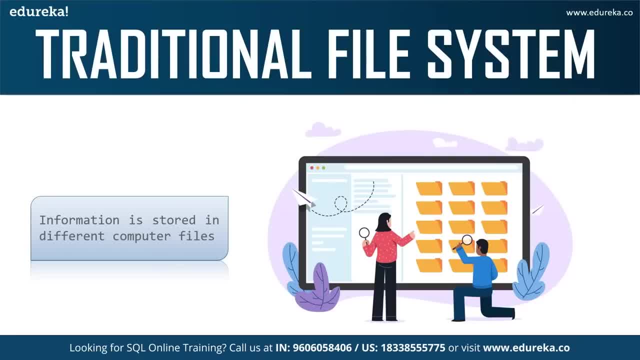 We won't be able to tell where information stops and where it begins. Let's look at the formal definition. file system is one which controls how the data is stored and retrieved. It is nothing but information stored in different computer files, Usually while storing a small amount of data, the file system is effective. but when it 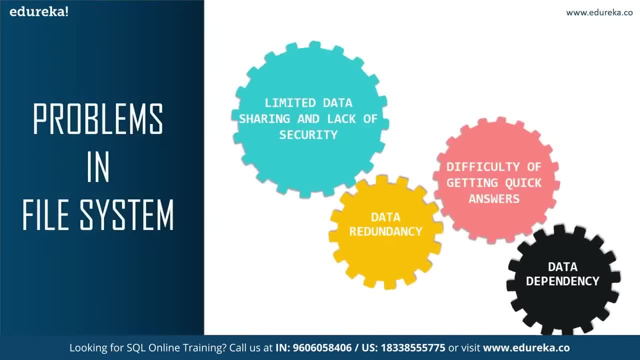 comes to storing the enormous amount of data, the file system fails. Let's look at some of the problems of file system. The first problem is data redundancy. when we store similar data, When we store similar data in different location of a computer, data gets duplicated and this 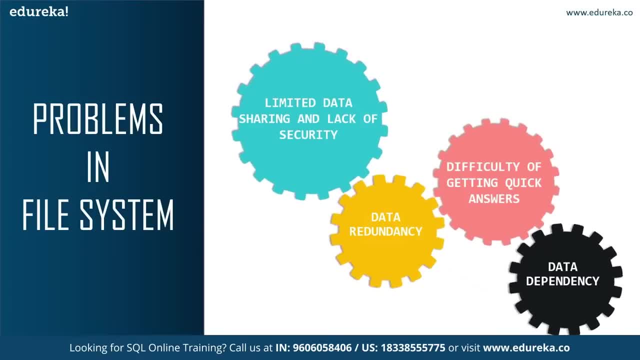 will lead to data redundancy. This will increase the storage size and also leads to failure of security features. because of this, the file system is highly vulnerable in nature. data redundancy will cause the user not only in terms of security, but also economically. the second problem is limited data sharing. 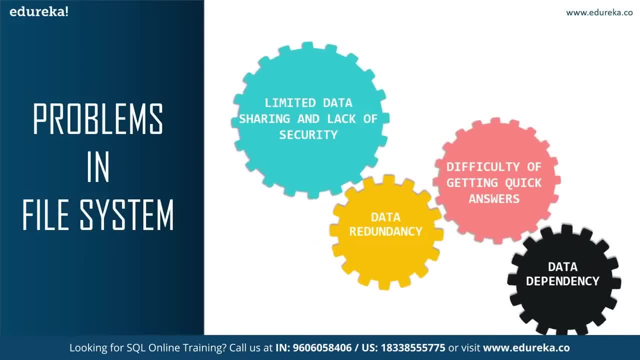 and lack of security. data sharing and security are closely related. sharing data Among multiple users introduces a lot of security risk in terms of spreadsheet data and other documents. the inbuilt file system programs provides only the basic security option, but they are not used most of the time because of this negligence. 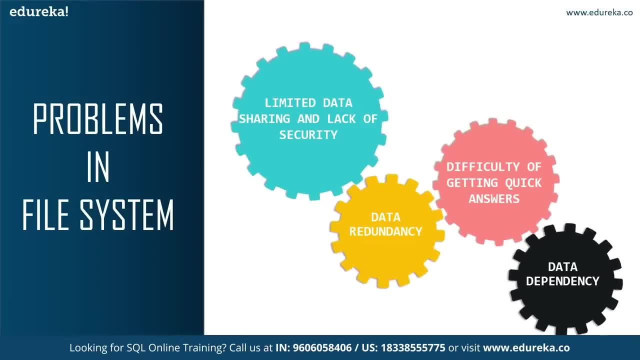 We might face some bigger problems in the near future. The third problem is the difficulty of getting quick answers. This is one of the major problems in file system, because file system doesn't allow multiple users to access the same data at a given point of time. 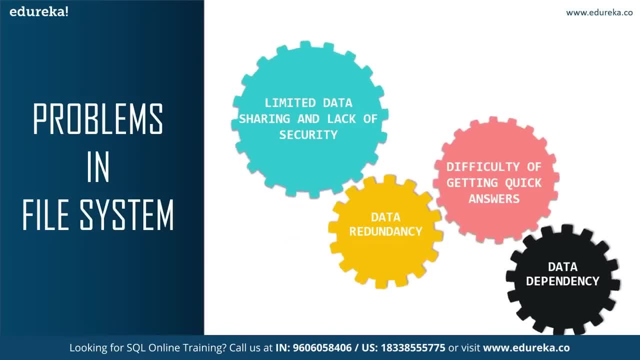 This means that multiple users at different work location cannot access the same data simultaneously. This will limit the access to important data if multiple users search for the same data at a given point of time. The next problem is data dependence. in the file system, files and records are described. 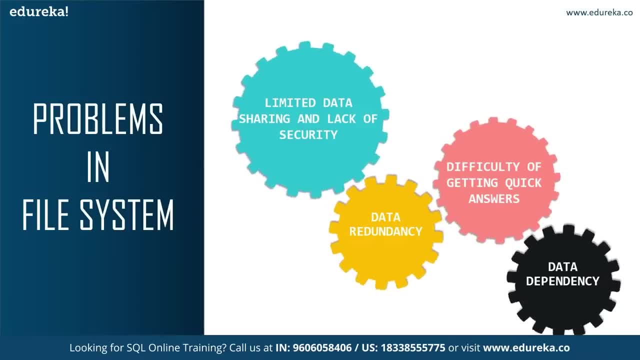 by a specific physical format that is coded into the application by the programmers. If the format of any one record was changed, then we need to make sure that all the remaining records format That is updated. This information has to be updated in the system also any changes in storage structure. 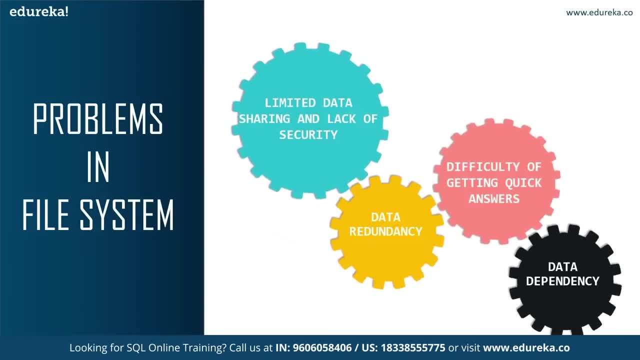 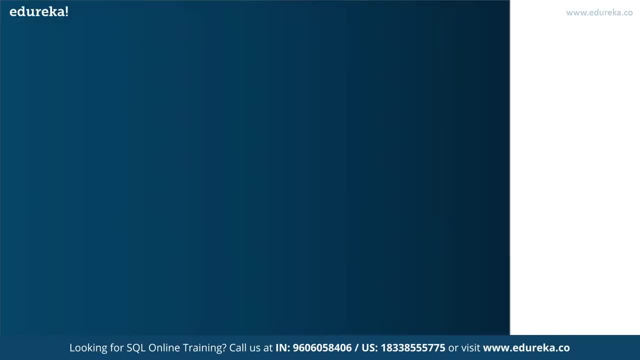 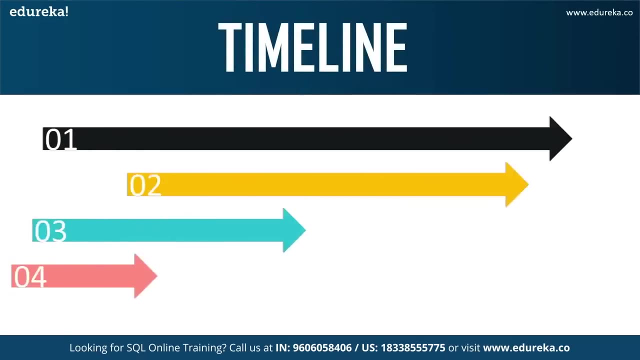 or access methods could greatly affect the process. This might result in failure of that particular application. So these were a few problems that were faced using the file system, and the solution for this is SQL and database. Let's now look at the evolution of SQL. SQL was developed at IBM by Donald e Chamberlain. 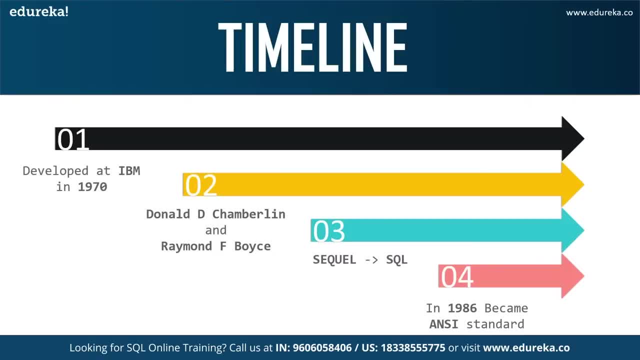 and Raymond EF boys in the early 1970s. It was initially called as sequel, that is, structured English query language, But later it was chained to SQL because SQL was a trademark of UK based engineering company in the year 1986, American National Standard Institute, that is, ANSI and the International 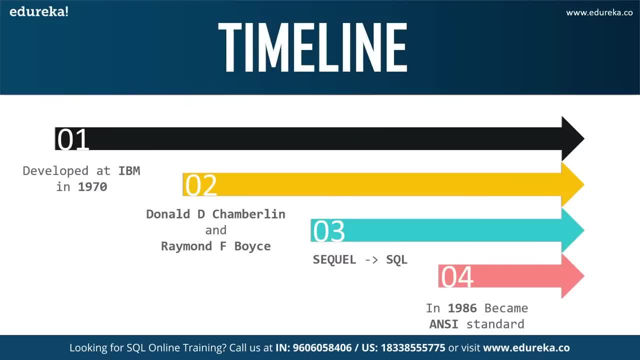 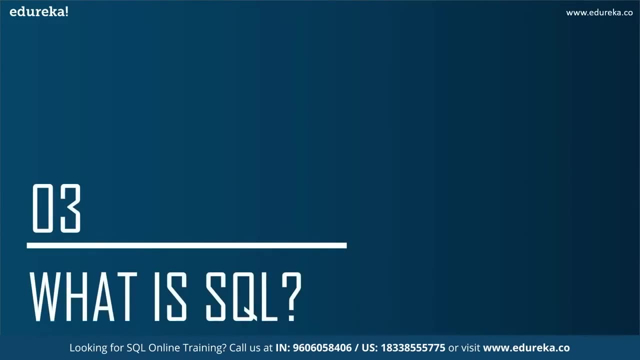 Standards Organization, that is, ISO, have deemed the SQL language as a standard language in relational database communication. This is how SQL evolved. Since we have understood the evolution of SQL, that's head to the next topic, that is, what is SQL? people from technical background may find this silly, but for a beginner it. 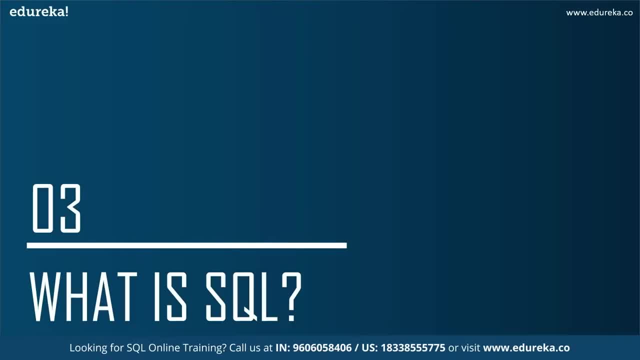 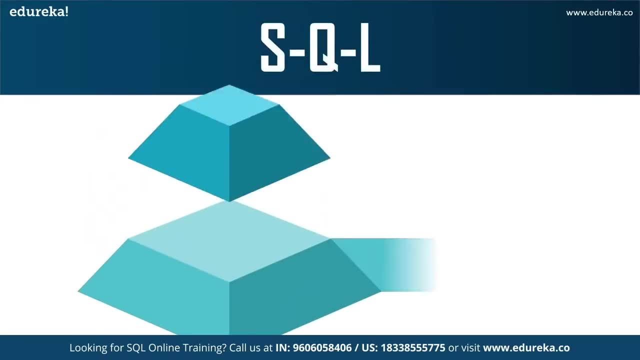 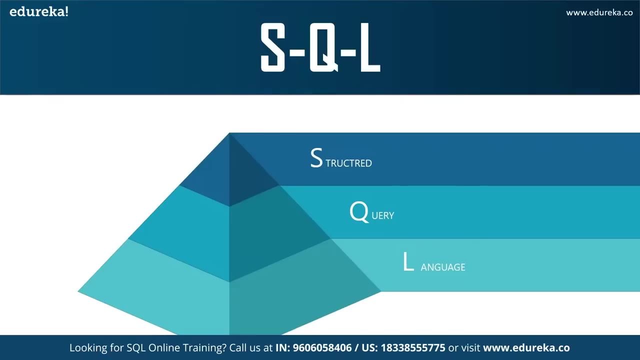 is really important to understand each and every aspect of this topic. the main focus of this entire session will be on this part. So now let's understand what is SQL. SQL is an abbreviation for structured query language, which also goes by the name sequel. even today, 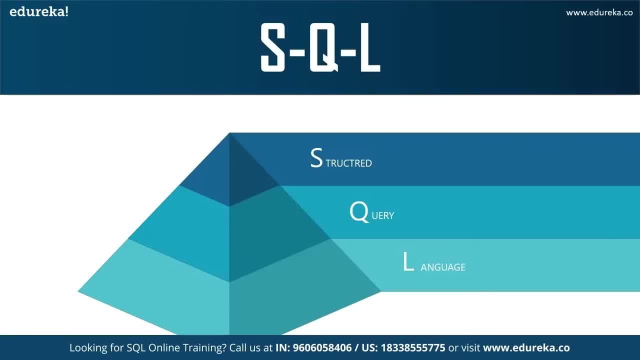 It is a language used by the database domain. SQL can be used only for relational type database and not for the others. relational database is a database which has the tabular method of storing data. Usually it consists of rows and columns. Let's now see what SQL can do. SQL is a core of relational database. 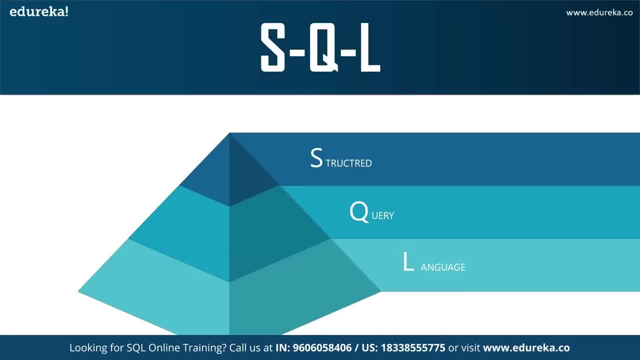 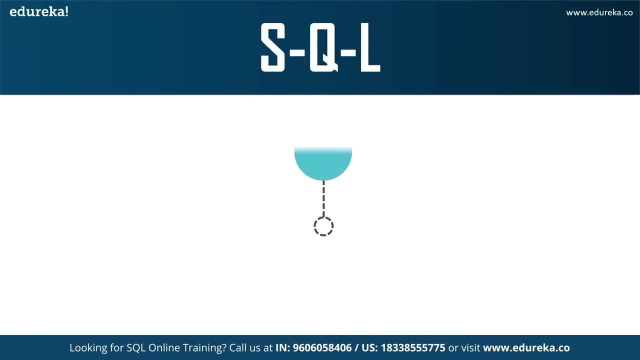 which is used for accessing and managing the database. with the help of SQL statements, You can add columns, update or delete rows of data. We can also retrieve information, modify database and perform many more actions. the different subsets of SQL commands are as follows: DDL, that is, data definition language. 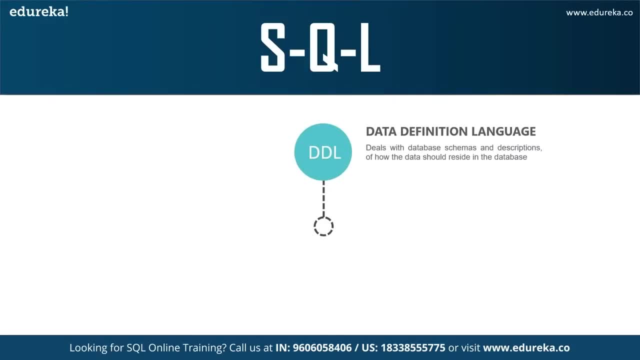 It simply deals with the description of the database schema and used to create and modify the structure of database objects in the database. It allows you to perform various operation on the database, such as create, alter and delete objects. DDL is very popular and extensively used when compared to other commands. 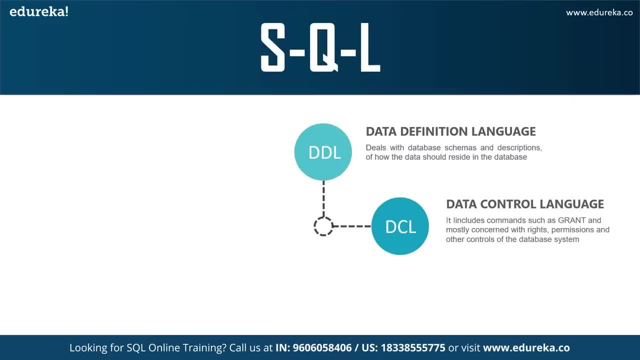 Moving on to the next command, DCL, that is data control language. It allows you to control access to the database, grant or revoke other DCL commands. grant gives user access privileges to the database, while revoke withdraws user access privileges given to the user with the help of grant command. 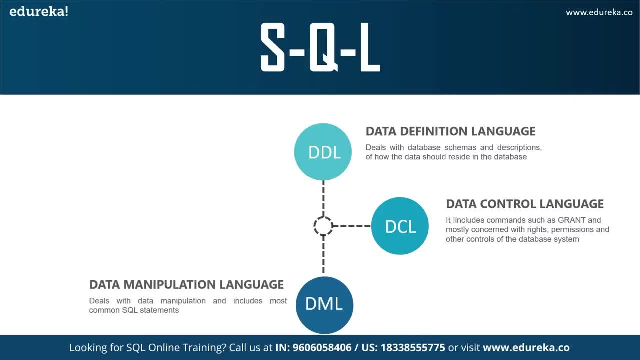 So the next command is DML, that is, data manipulation language. It allows you to access and manipulate data. It helps you to insert, update, delete and retrieve data from the database. So what does each of this command do? So the insert command is used to insert data into the table. 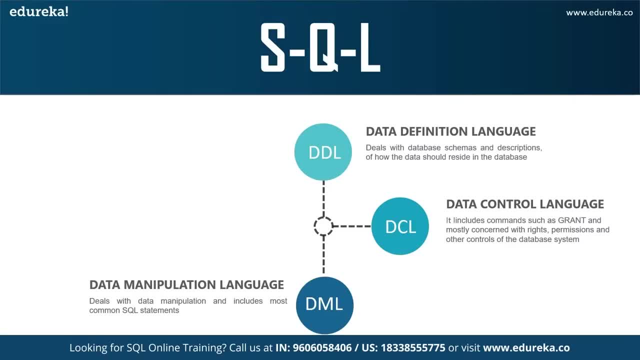 while update is used to update existing data within the table and at last, delete is used to delete records from the database. The final command is TCL, that is, transaction control language. It allows you to deal with the transaction of the database. few of the TCL commands are commit. 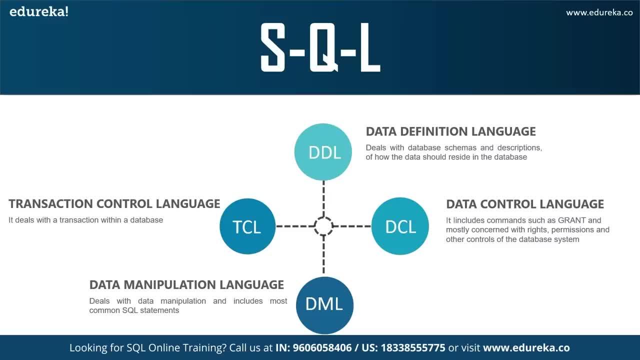 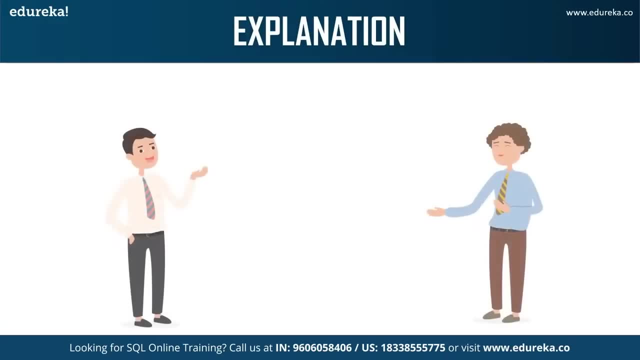 rollback, save point and set transaction. So these were the SQL commands. to understand SQL in a better way, Let's use an analogy: if two people wants to communicate with each other, then they have to use a language that is understood by both of them here. 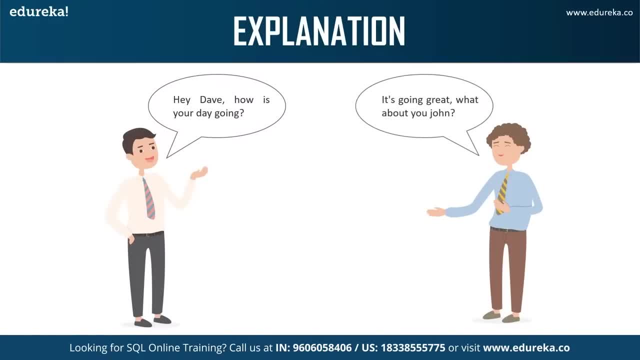 John wants to start a conversation with Dave and he uses English language to start his conversation. This language is known to Dave as well, So they will continue their conversation. But what if one of them didn't understand what the other person spoke? There won't be any conversation at all. relating this analogy. 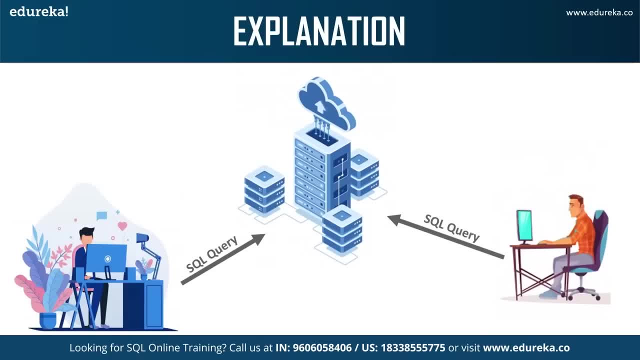 If we consider these two people, one as user and the other as database, then that language which is used to communicate between these two is called SQL. Similarly, how a language has the grammar and various rule on how it should be used, even the SQL has its own directives. 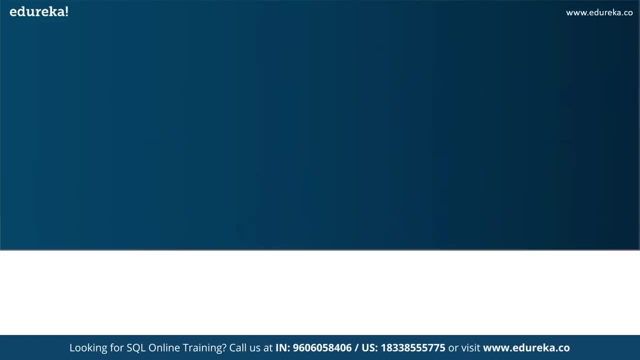 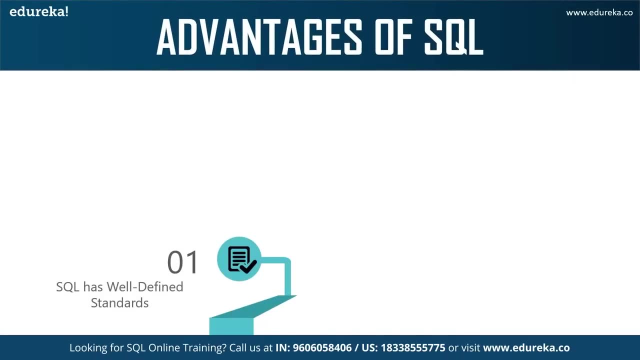 I hope you have clearly understood what exactly SQL is. Let's now head to the next topic, that is, advantages of SQL. So the first feature is: SQL has well-defined standards, as it says. developers of SQL has clearly mentioned how exactly each and every query has to be written. 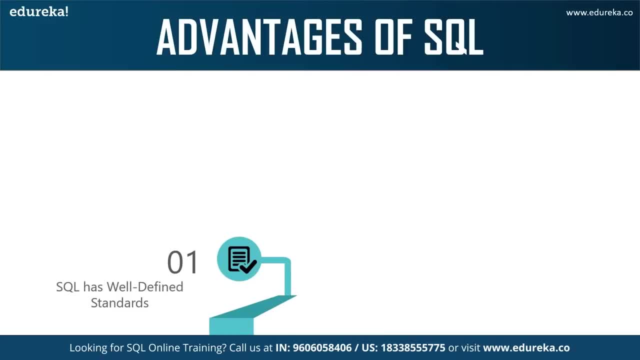 There is no room for ambiguity when it comes to writing a query. The standards have to be followed. The second advantage is SQL is easy to learn. Yes, SQL is a language that is used to work with a database, since SQL has a large user base as well as well-defined standard. 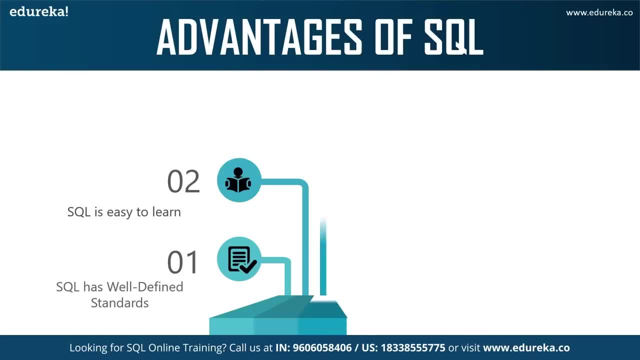 for a beginner It is really Easy to learn. the next one is in SQL, We can create multiple views. This is one of the unique and early feature that SQL came up with. view is nothing but creating a virtual table, a virtual table as a temporary table for certain use. by doing this, 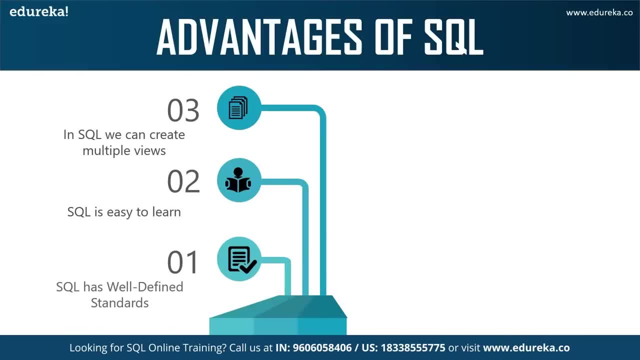 We can protect the integrity of the data. SQL has the ability to not only create a single view, but can create multiple views. The fourth one is SQL queries are portable in nature. It means we can execute the SQL query in one system and execute the same query. 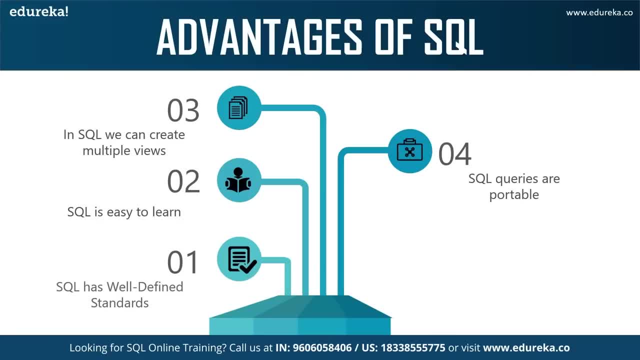 in an another system without changing the format. But the condition is that the environment setup of these two system has to be same, else The query won't be executed. the next advantages: interactive. The main purpose of SQL is to communicate with the database. We can write complex queries to fit the results. 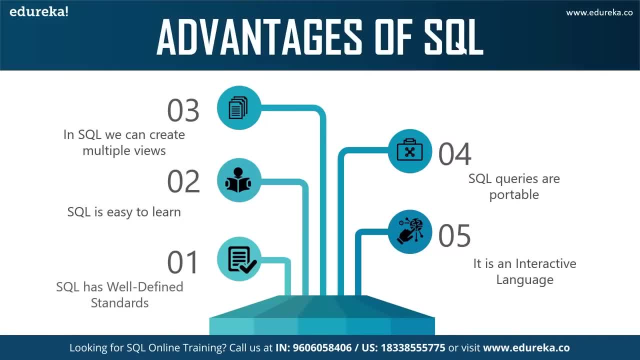 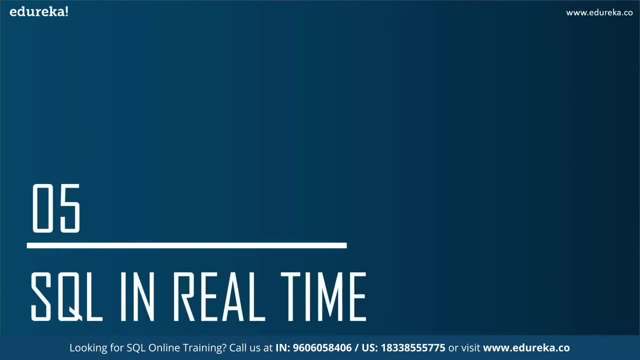 from the database, and these queries can be easily understood by anyone. So these are some of the advantages of SQL. Let's head to the next topic, That is, SQL in real time, since SQL is a language that is used to operate on the database. 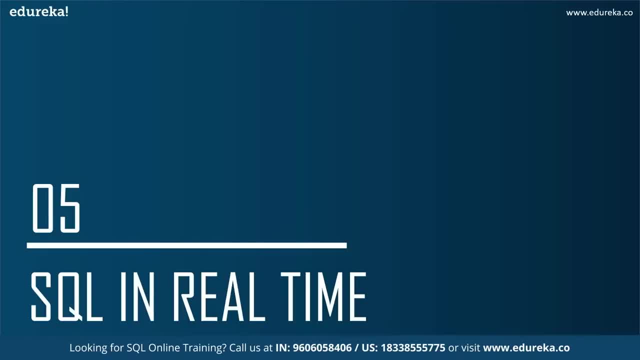 We need to look at the bigger picture of the data management industry here. If I say database, it includes SQL language as well. The database is used in different verticals, like online stores, healthcare providers, libraries, financial industry, retail industry, government agencies and many more now. 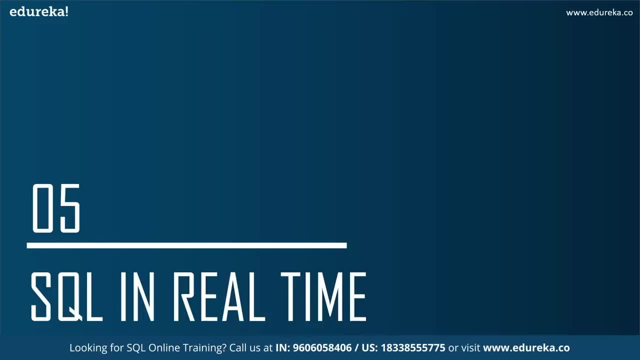 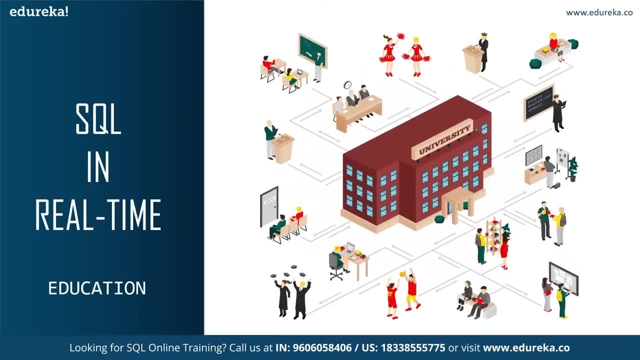 let's consider some real-time examples of the use of SQL and database. The first one is education sector. database systems are frequently used in schools, colleges and universities to store and retrieve the data. This data may be regarding students, staff details, course detail, exam details, attendance details and fees details. 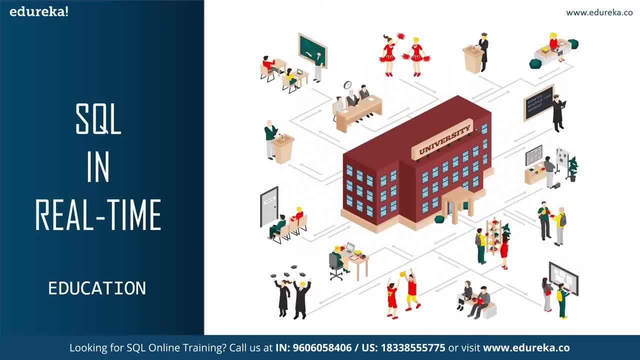 There's a lot of interrelated data that needs to be stored and retrieved efficiently. to understand the magnitude of impact that the database has made in this field, Try to imagine the days when the results were only declared on the school notice board. isn't it easier now? 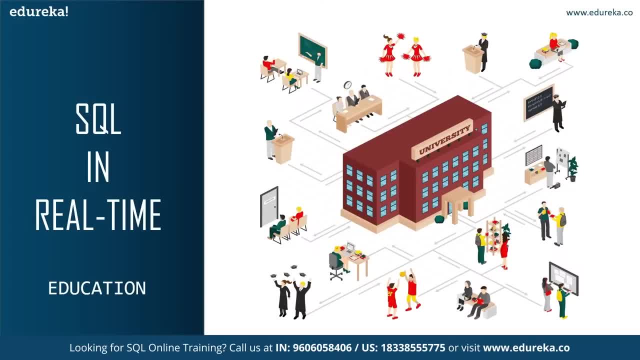 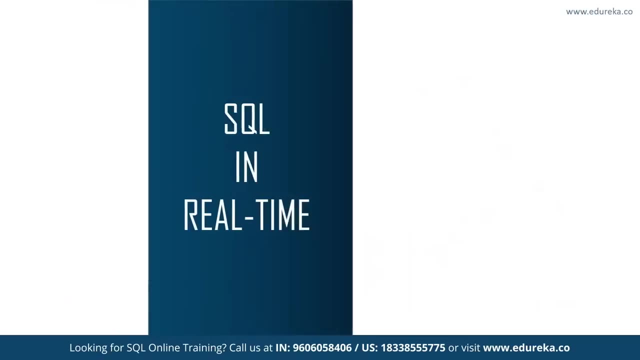 to access your exam results with just one click. who wouldn't say no to such a drastic change? also, nowadays, the online exams have increased significantly. This has increased the speed of assessment when compared to the olden days. all these are possible because of SQL and database technology. 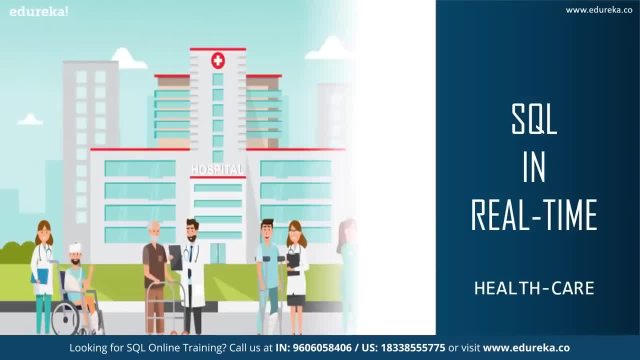 The next sector is healthcare sector. There were days when people used to stand in front of clinics and hospitals to get an appointment with a doctor, But now the time has changed. in hospitals and medical institution, maintaining data related to doctors, patients and staff is a huge task, effectively coordinating among 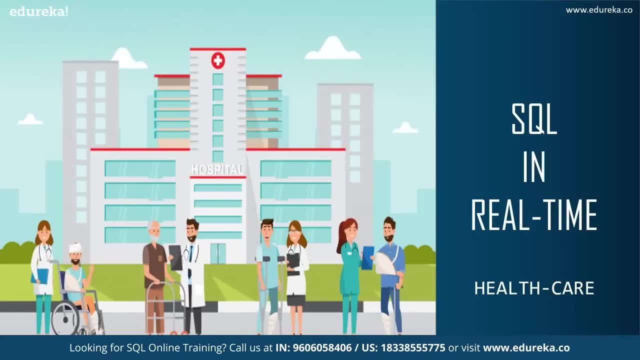 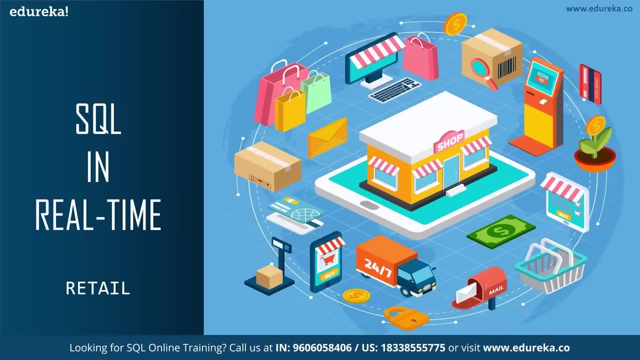 these three has to be handled seamlessly with the help of SQL and database. This industry has gained a lot with the introduction of SQL and database. inventory management has been effective. The next one is retail industry. Every year, leading e-commerce Gents come up with great offers, discounts based. 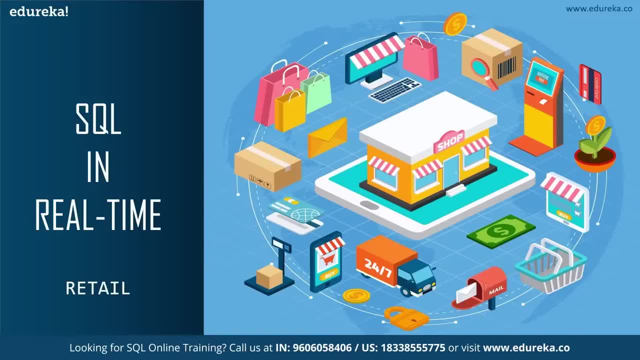 on your personalized shopping. to come up with all this, They use database and other technology. the industry utilizes the database and SQL technology extensively and retail industry customers data has to be managed effectively. There's no scope of error when it comes to handling the data with the instigation of SQL and database system. 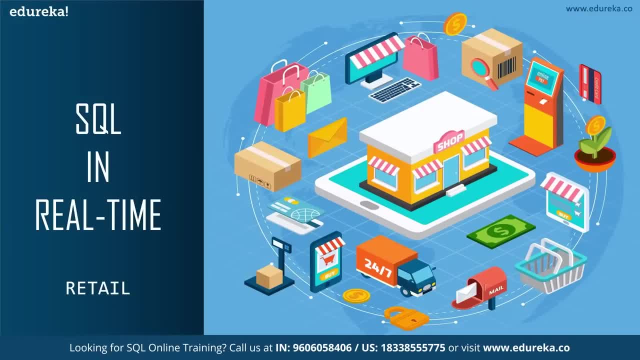 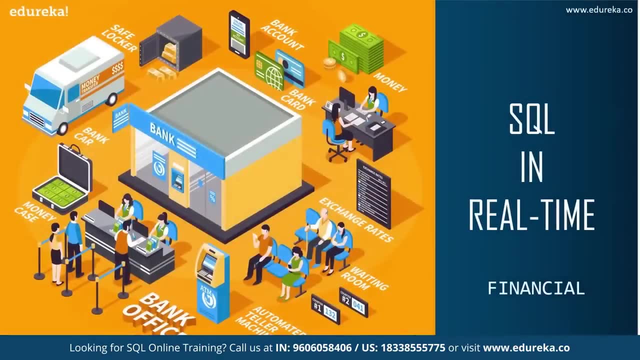 The retail industry can not only secure the data, but also can get the real-time analysis, which in turn helps him to make a lot of profit. and the final one is financial sector. when we speak about this sector, It's really hard to even imagine what goes behind the scene. 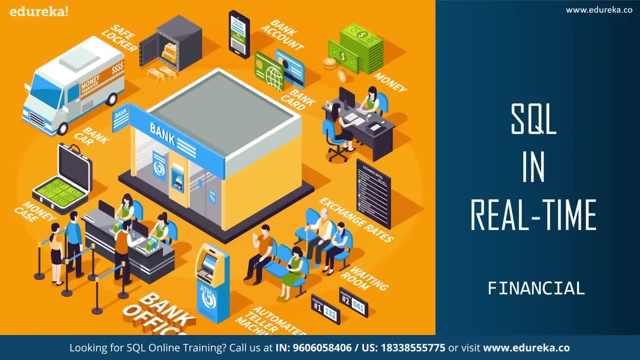 only the experts know how much data will be processed every second. managing money, assets, shares, Etc. in a real time is a tedious task. SQL and database technology is helping the financial sector to achieve its primary task. SQL queries can be also used to check the fraudulent activities looking 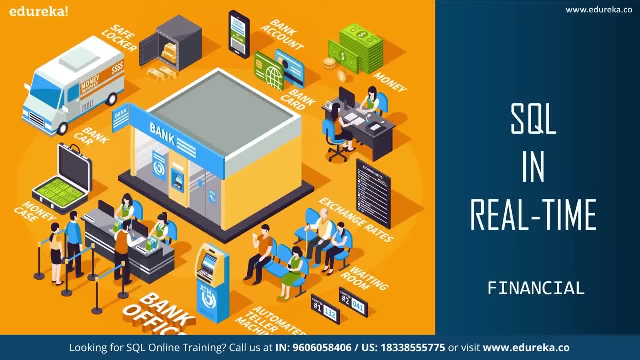 at the issues of fraudulent activity. effective fraud detection requires a financial organization to process a huge amount of customer purchasing data, So these organizations have to store and retrieve data effectively without causing any burden on another branch of the same organization. These were the few sectors and Industries where the SQL is used. 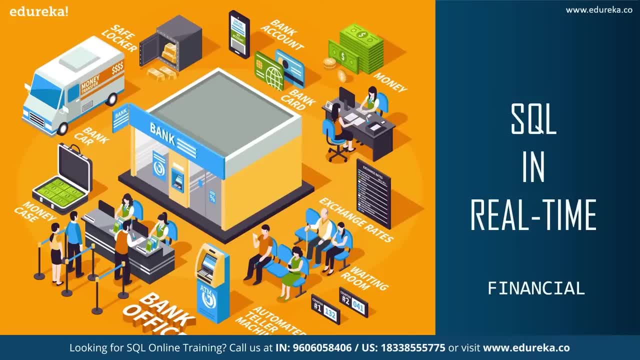 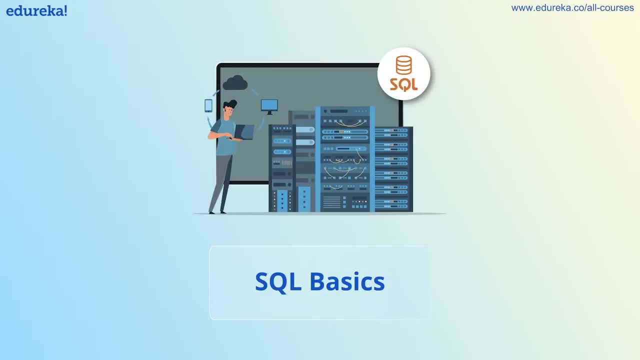 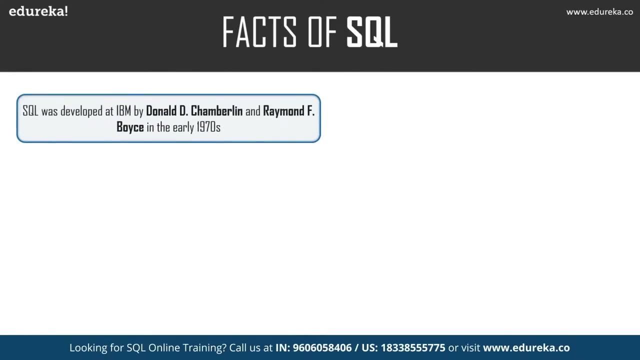 in day-to-day transaction. This brings us to the end of this session. I hope you have clearly understood What is SQL, its evolution and its application. Do you know when SQL was born? Well, let me answer that question for you: SQL was developed. 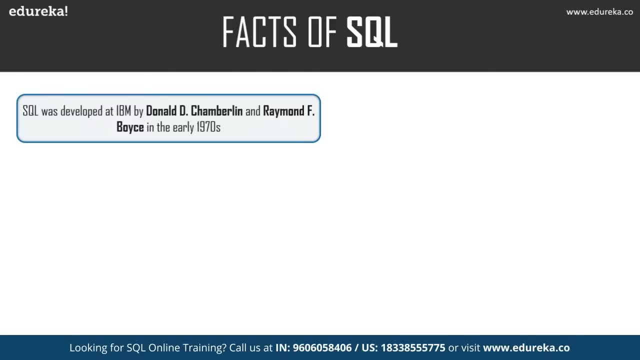 at IBM by Donald E Chamberlain and Raymond F Boys in the early 1970s. It was initially called a sequel, that is, structured English query language, but later it was changed to SQL because sequel was a trademark of UK based engineering company. SQL is said. 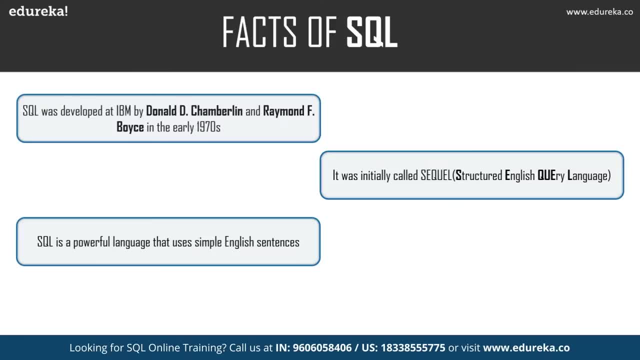 to be a powerful language. reason for that is it uses very simple English sentences and also uses very few lines. It uses common words such as select, insert, update and many more to perform its core functionalities. SQL is known to be a declarative language. When you write a query, you have to describe what needs. 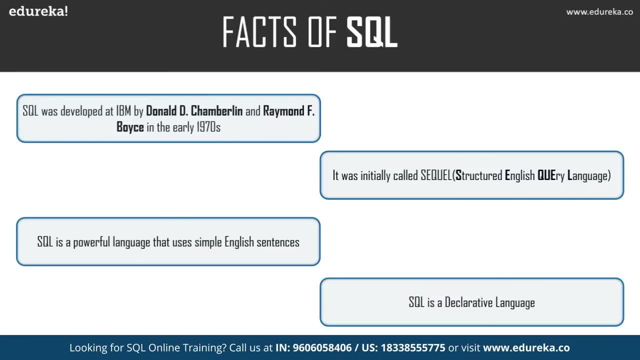 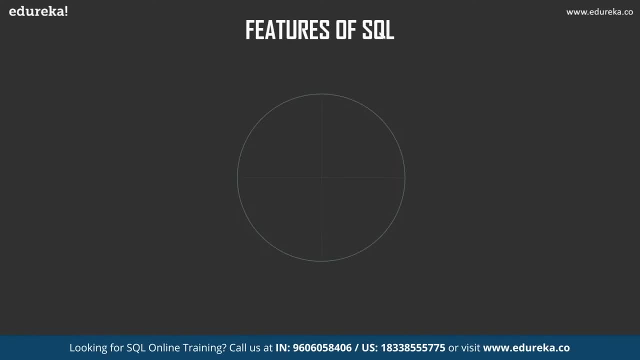 to be done and you don't have to worry regarding the flow of the query. It will be handled internally by the DBMS that you're using. Now let's look at some of the features of SQL. So the first feature is: SQL has well-defined standards. 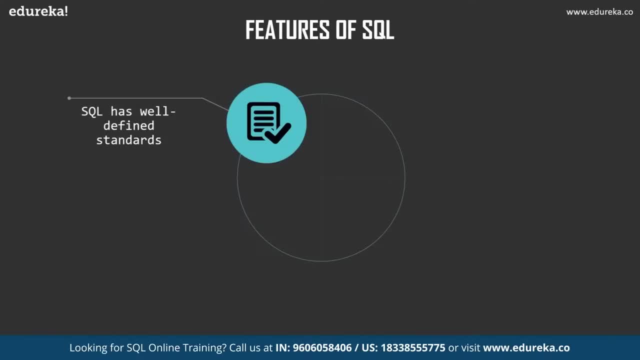 as it says. developers of SQL has clearly mentioned how exactly each and every query has to be written. There is no room for ambiguity when it comes to writing a query. the standards has to be followed. SQL is easy to learn. Yes, SQL is a language that is used to work. 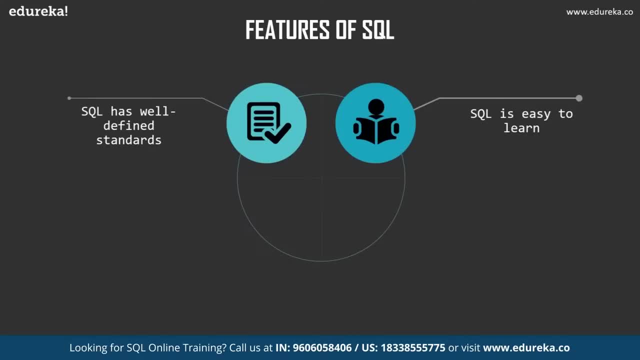 with the database. since SQL has a large user base as well as well-defined standards, for a beginner It is really easy to learn. next one is in SQL, We can create multiple views. This is one of the unique and early feature that SQL came up with. view is nothing but creating a virtual table. 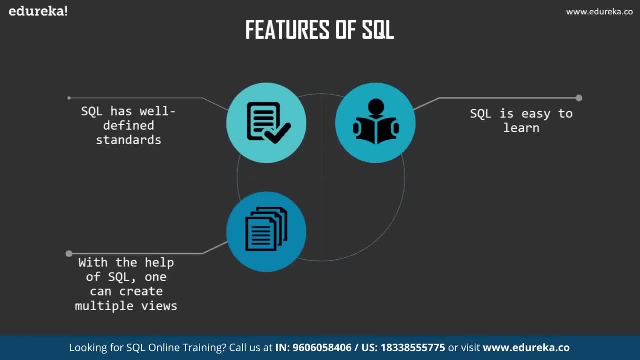 a virtual table is a temporary table for certain use. by doing this we can protect the integrity of the data. SQL has the ability to not only create a single view, but can create multiple views. Finally, SQL queries are portable in nature. It means we can execute the SQL query. 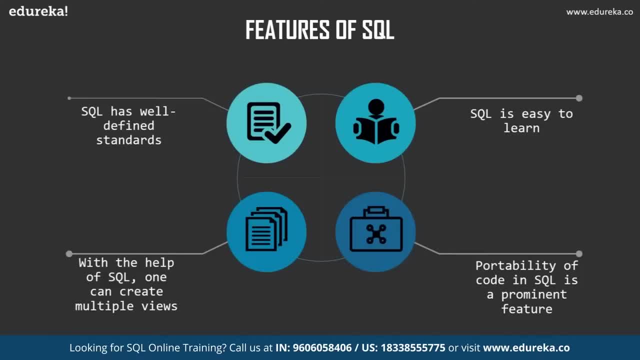 in one system and execute the same query in an another system without changing the format. but the condition is the environment setup of these two system has to be same, as the SQL query won't be executed. So these were some of the features of SQL. 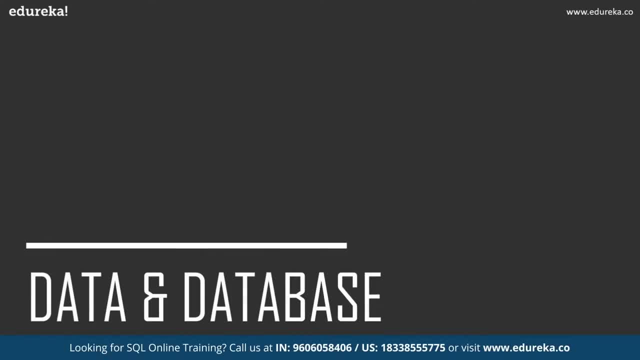 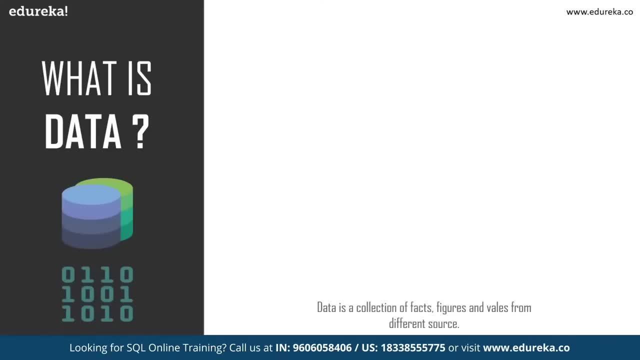 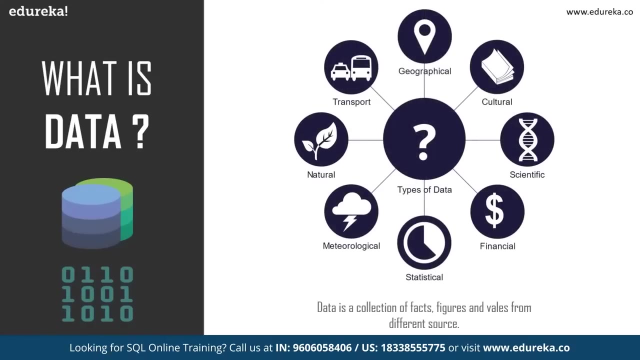 Now let's look at the next topic, that is, data and database. Firstly, let's look at what is data. So the standard definition for a data is values from different source which has been translated for some purpose, and this purpose can be anything. source for the data can be like temperature, reading. 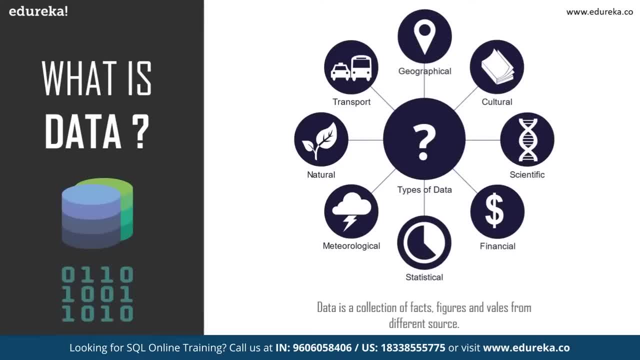 financial data, videos, blogs, text, Etc. It goes on. in the end, It should make a meaningful sense. only then we can consider it as a data. This image clearly depicts the different source of data, So we can clearly understand that the data source can be anything. 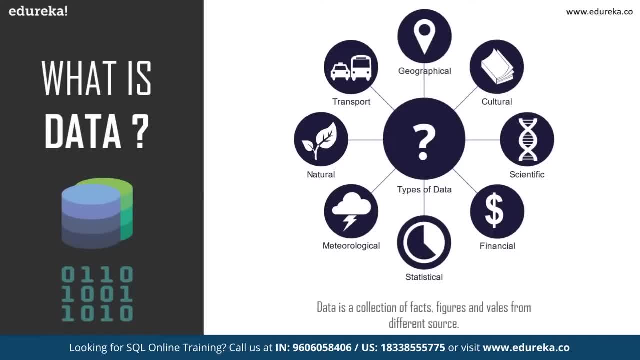 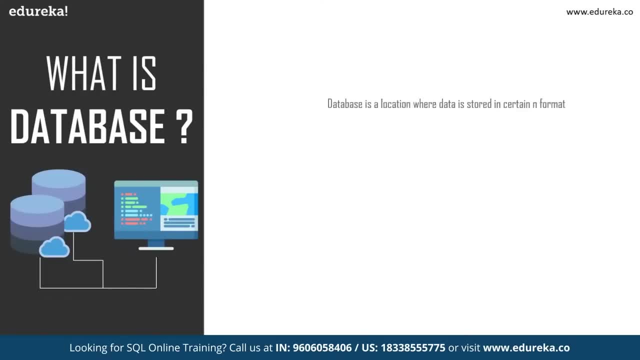 since we are clear about what data is all about, Let's head to the next topic, That is, what is database? Firstly, let's look at the formal definition for a database: a database. A database is an organized collection of data. with, the data is stored. 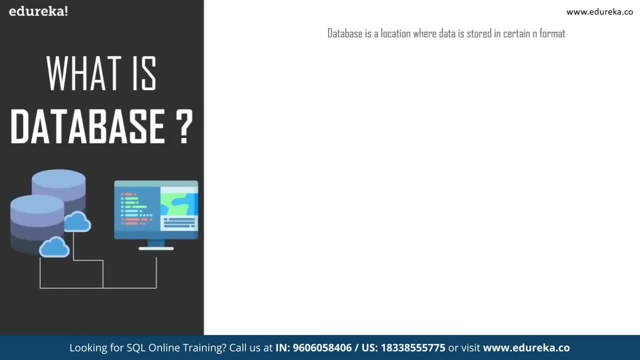 and accessed electronically from computer system. to make you understand what it means, Let me use an analogy to explain the concept of database. consider a library. Usually, the library contains a huge collection of books of different genre. here, library is a database and these books are the data in the image. 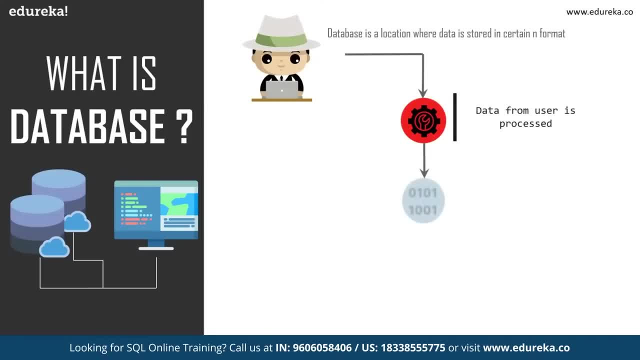 We can see a person performing an action on the data, and those action can be like create, store, update, Etc. When the user sends the instruction as well as data, it will be stored inside the database after certain process, and this entire process is bi-directional. 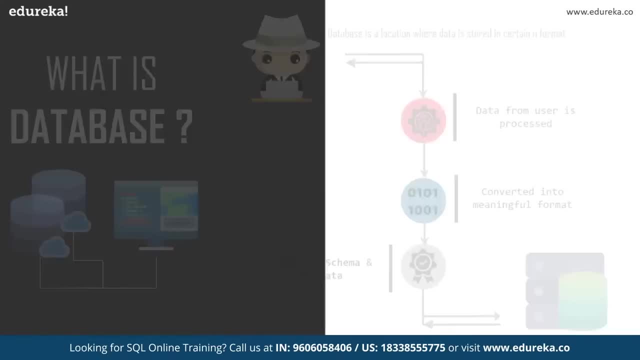 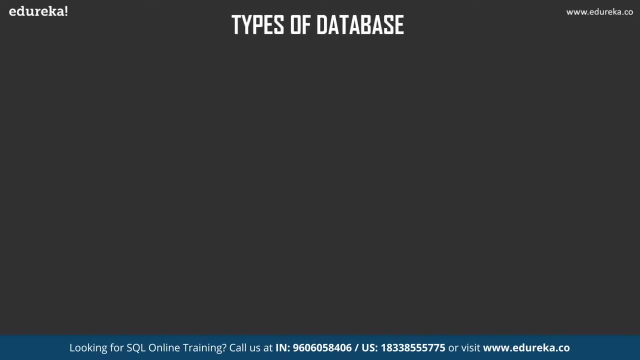 that is, control flows on both the sides. next, I'm going to talk about different types of databases. There are different kinds of databases that are in use today, and these databases are classified based on capabilities, features, functionality, size and performance. So few of them are distributed database. object-oriented database. 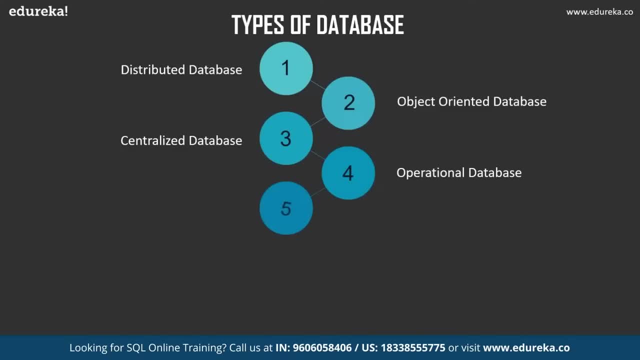 centralized database, operational database, graph database, cloud database, No sequel database and, finally, relational database. among these databases, the two popular types that are widely used are: first one, relational database and second one no sequel database. relational databases generally uses SQL language and we are going to learn more about it in the coming modules. 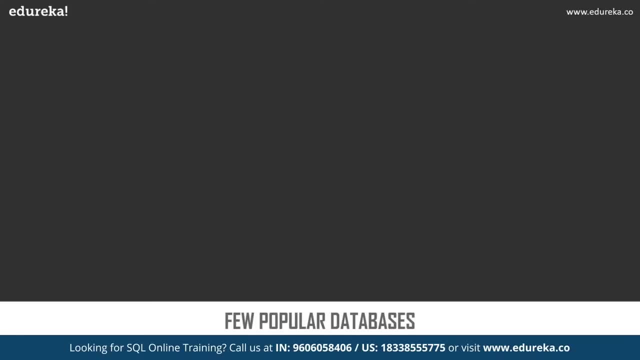 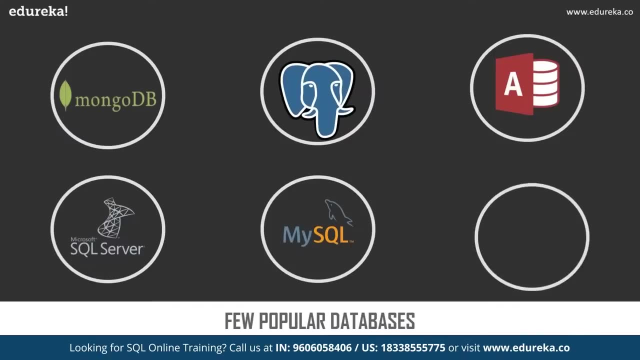 moving on, Let's look at some of the popular databases that are widely used today. So they are MongoDB, Postgres, Microsoft Access, Microsoft SQL Server, MySQL and Oracle DB. These are the few popular databases that are used today. Each one of them has its own pros and cons. 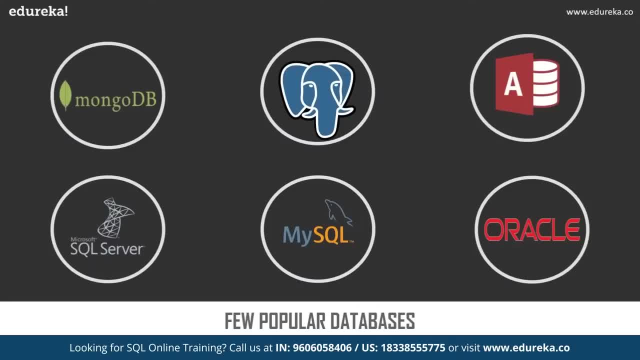 since we have already started the topic of database, It wouldn't be fair to drop this topic abruptly, So I shall discuss a few basic database related queries. The first query is how to create a database. to explain this, Let me jump into my sequel workbench. 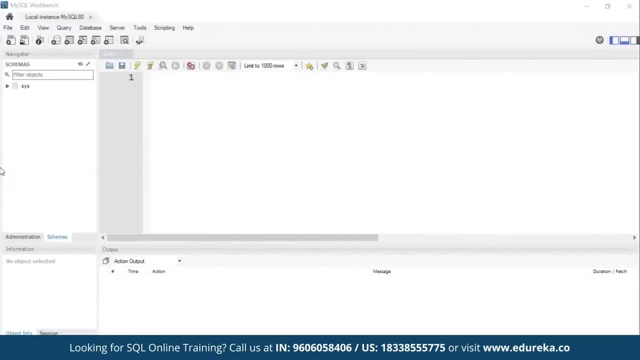 This is the interface of my sequel workbench. On the left side of the screen We can see the database. in the center area We are going to write our queries. at the bottom part We are going to get the status of the query that has been executed. 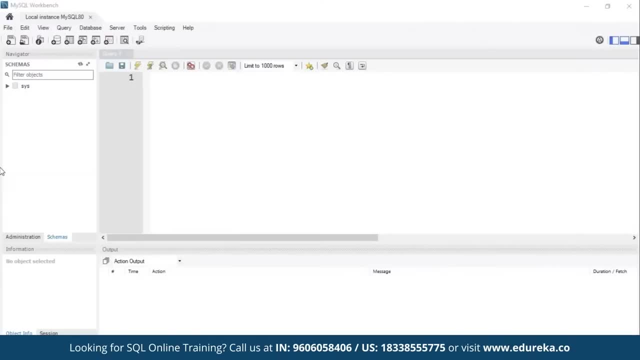 So you might wonder why I'm using my sequel workbench for executing SQL queries. Well, SQL is a language that is used to communicate with the database, But as my sequel workbench is a database management system, So my sequel workbench allows us to use SQL queries. 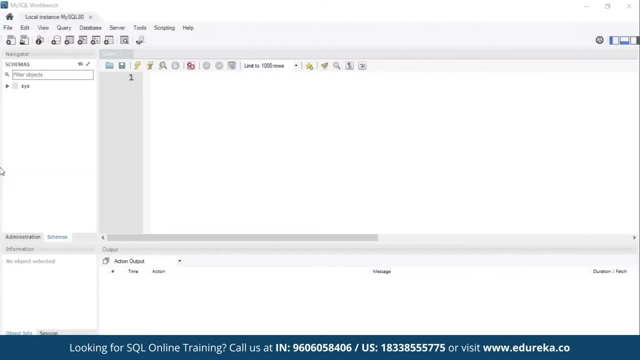 to communicate with the database country. use other DBMS? Yes, we can, but the syntax of the queries may slightly vary, So let me explain you the first topic, that is, how to create a database, and the syntax for this is Create database are the keywords used to create a database. 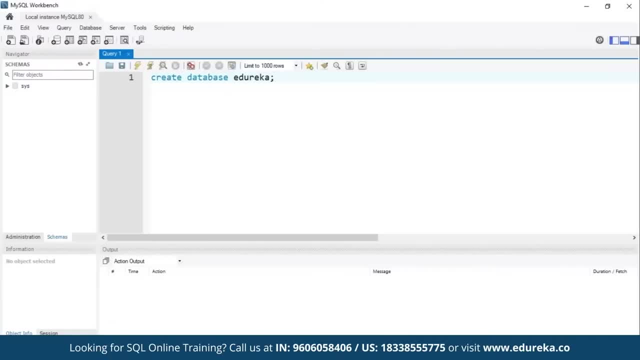 followed by that, We have to specify the name of the database. here I'm using edureka as a name for my DBMS, So let me select this entire statement and click on the lightning icon So I can see at the bottom that the database with the name edureka has been created. 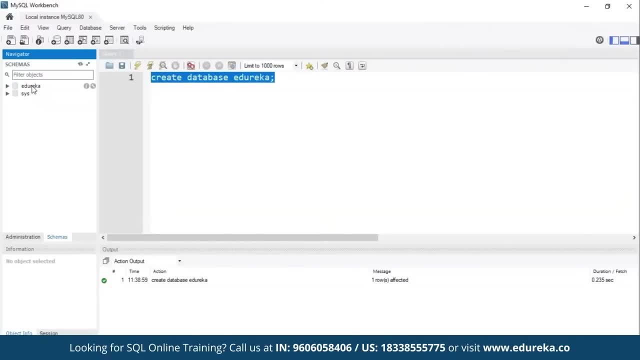 So let me refresh it so we can see that the database with the name edureka has been created. So the next topic I'll be discussing is how to delete a database, and the syntax for this is Drop database are the keyword used to delete a database. 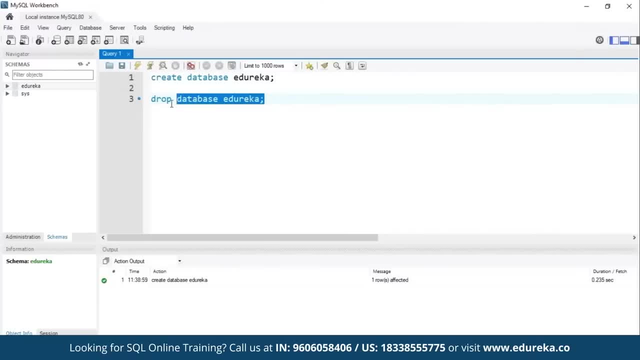 and followed by that will be the database name. So let me select this entire query and click on the lightning icon So we can see that the database with the name edureka has been deleted. So these were the few queries related to database. the next topic. 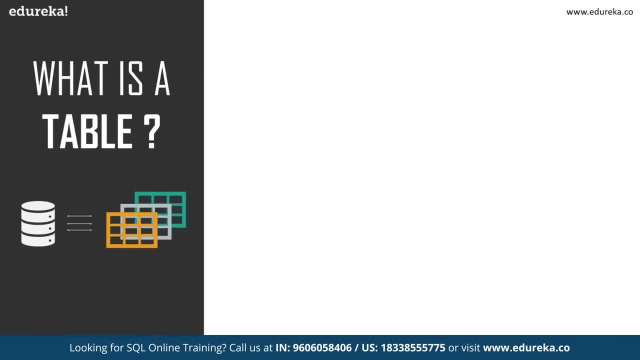 that we are going to learn is table. So what is a table? a table in a database is nothing but a collection of data. in a tabular way, It consists of rows and columns. the table contains data elements, also known as values, using a model of vertical columns. 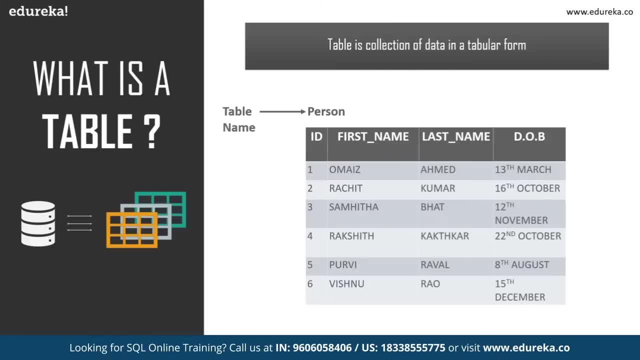 and horizontal rows. the point of intersection of a row and a column is called a cell. a table can have any number of rows, but should have a specified number of columns. to understand the concept of a table in a better way, Let's look at the image. 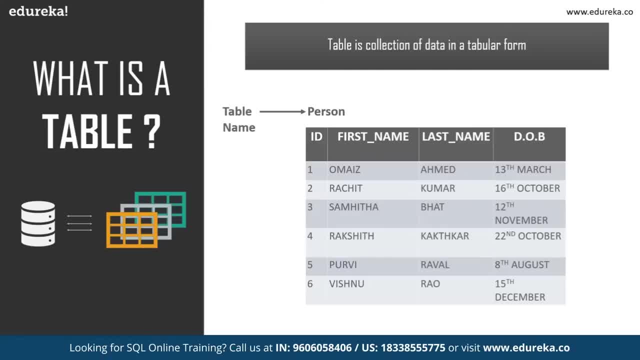 So the name of the table here is person. when we create a table It has to have a name. a table without a name doesn't exist. So what is tuples? a single row of a table which contains a single record for that relation. here There are six tuples. next is attributes: features. 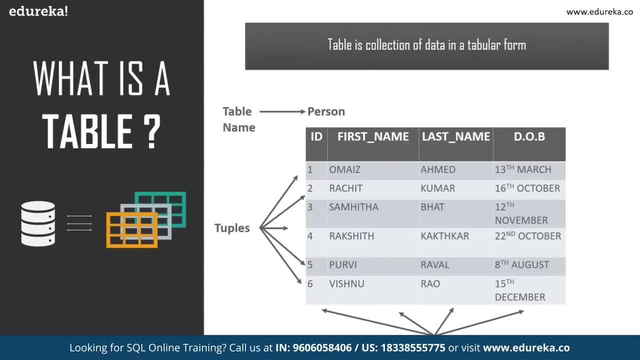 of an entity is called attribute. an attribute has a name and a data type. here There are four attributes. Those are ID, first name, last name and date of birth. So I hope you have understood the concept of table. Let's now understand the table constraints. 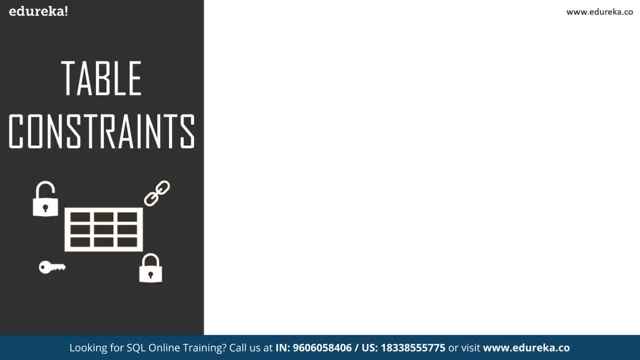 So what are table constraints? in simple words, It is a restriction that are specified by the user while creating a table. So you may wonder why these kinds of constraints are required. the answer for that is: even though a table stores the data, that data has to be of certain format. 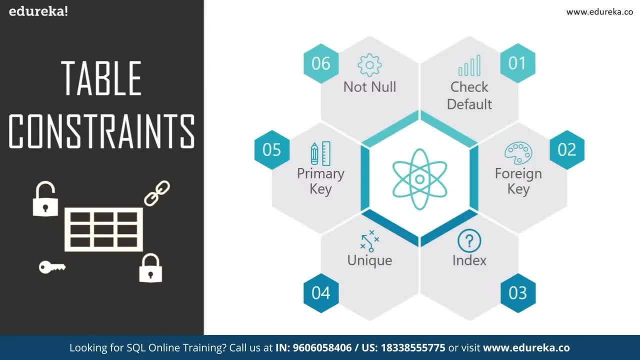 to ensure the data Integrity, We use constraints. these constraints have to be decided during the creation of a table. If you want to change the constraint, then we have to delete the table and then we have to create a new table using the new constraints. few of the constraints. 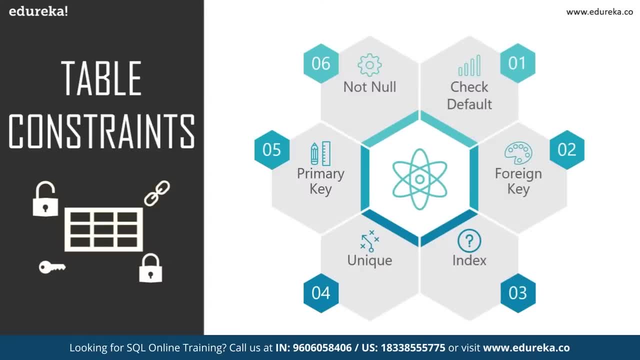 that are used most of the times while creating a table are check, default, primary key, foreign key, not null, index and unique. since we have understood what table is, let's look at some of SQL queries related to the table. The first one is how to create a table to understand this. 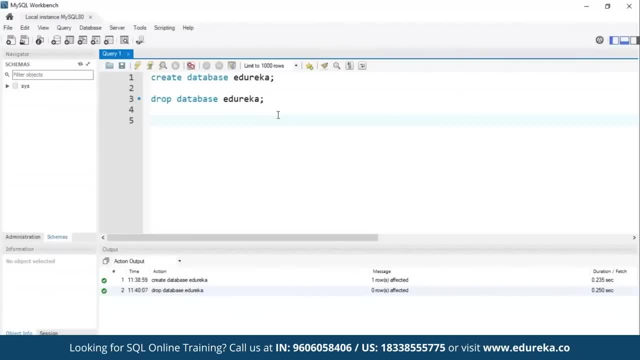 Let's head to the MySQL workbench to create a table. We need an active database. since we had deleted the previously create database, Let me create the database once again So we can see that we have a database with the name edureka. So now let me create the table. 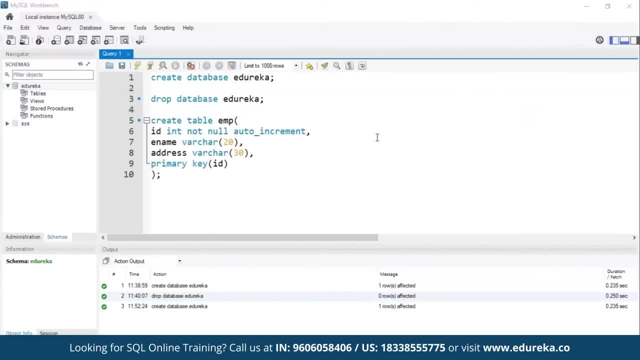 and the syntax for creating a table is create. table is a keyword used to create a table, followed by that. We have mentioned the table name. We need to make sure that the table name is unique. Keep in mind that in a database there cannot be two tables. 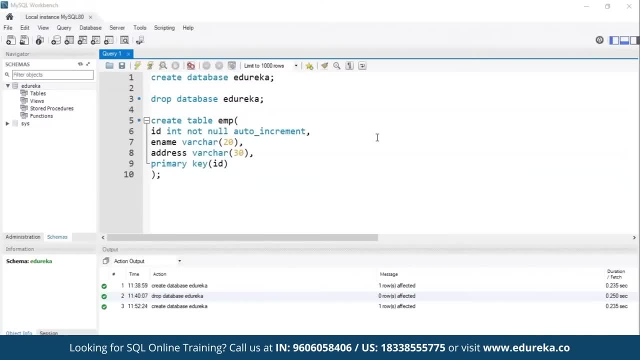 with the same name inside the table. We have declared the columns along with the data type, and we have to end the query with a semicolon. So let me execute this query So we can see that the table EMP has been created. So the next query I'm going to discuss is how to delete a table. 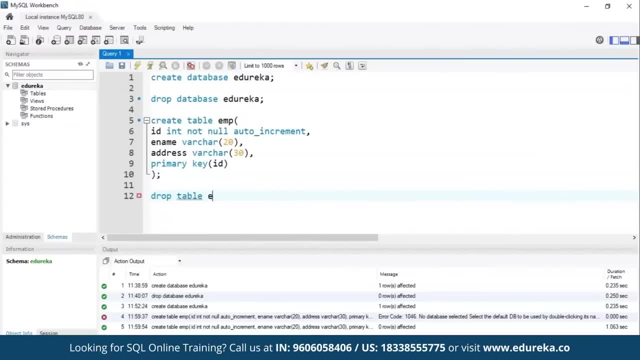 and the syntax for this is: we shall use drop table keywords to delete a table and followed by that We have to specify the table name. So let me select this entire query and we can see that the table with the name EMP has been deleted, with all the basic introduction understood so far. 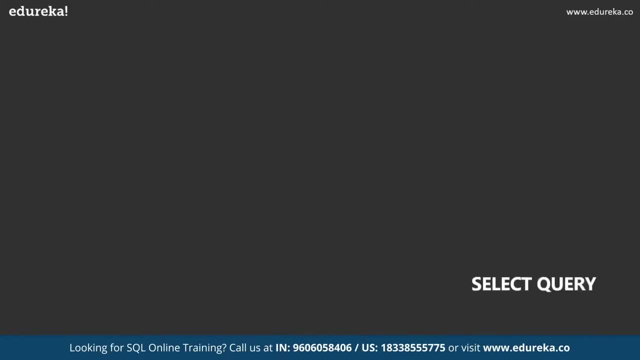 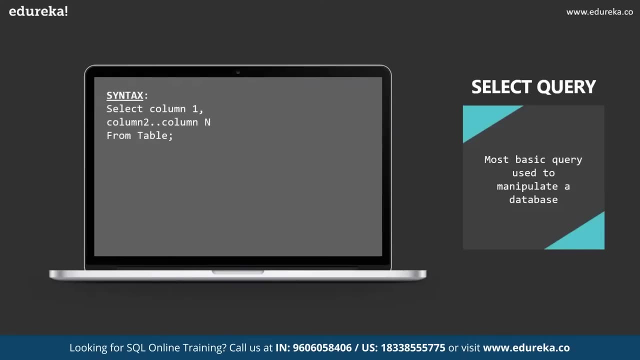 Let's now understand some SQL basic queries. Let me begin this by introducing the most basic and widely used query, that is, select statement, and the syntax is select column name. from the table name We can specify the name of the columns that are present in the table. 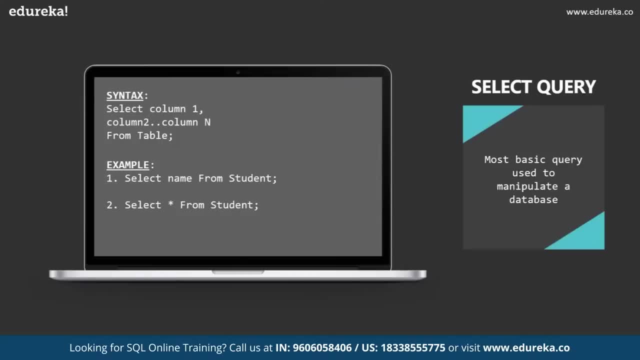 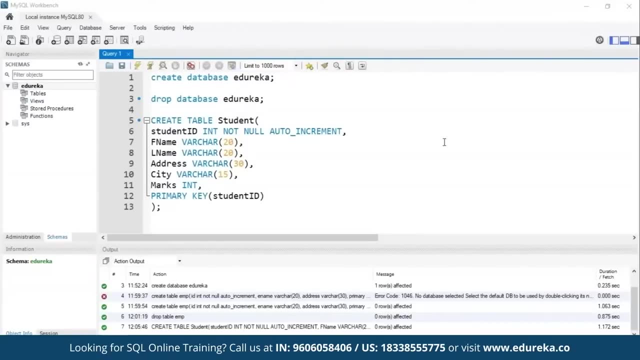 Also note that if you want to display all the columns of a table, then use star operator. now let's jump into execution part to explain the entire SQL queries. I'm using student table and the student table has student ID, first name, last name, address. 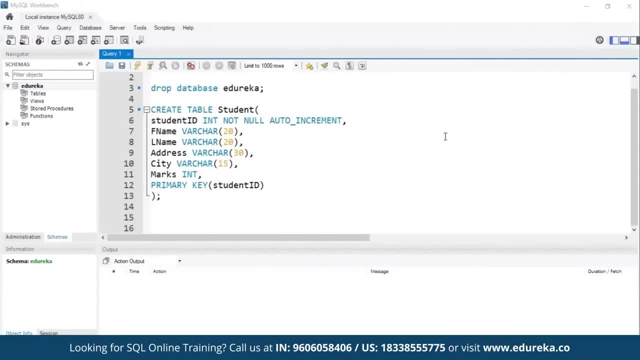 City and marks as its columns. So the syntax for select statement is Select star from student. since we have to display all the columns, I'm using star operator, So let me select this entire query So we can see that the entire table has been displayed. 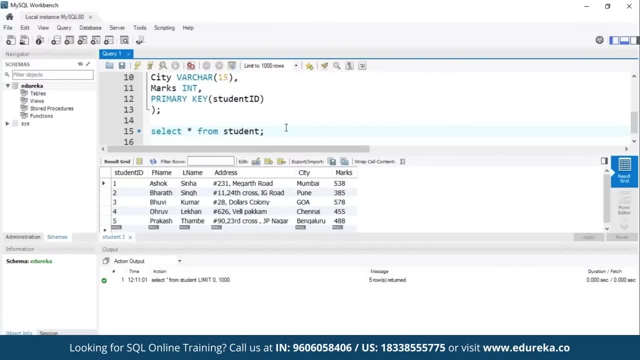 So this is one of the way in which we can use select statement. The another method is: if you want to select a particular column, then we have to specify that column name and the syntax for that is. so we can see that from the table. 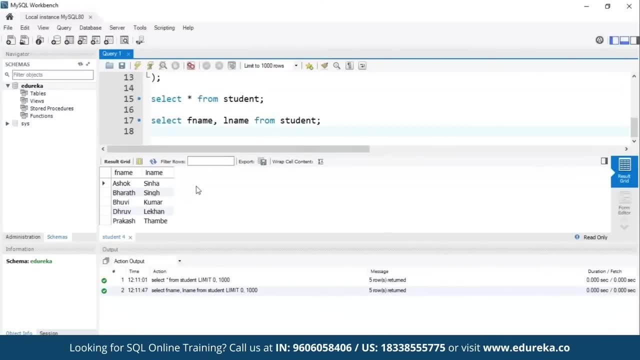 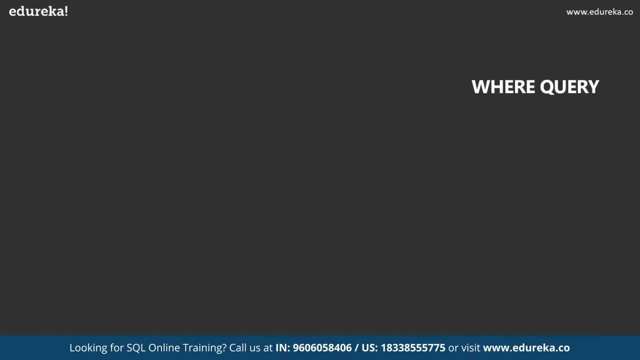 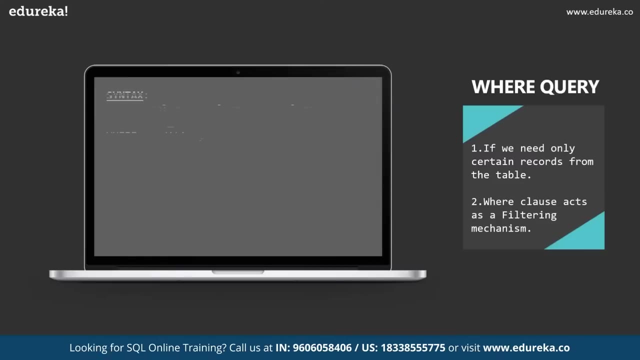 We have selected only first name and last name. Usually, select statement is used to select the data from the database. So the next SQL query that I'm going to discuss is where Claus, where Claus is used to filter records, where Claus is used to extract only those records. 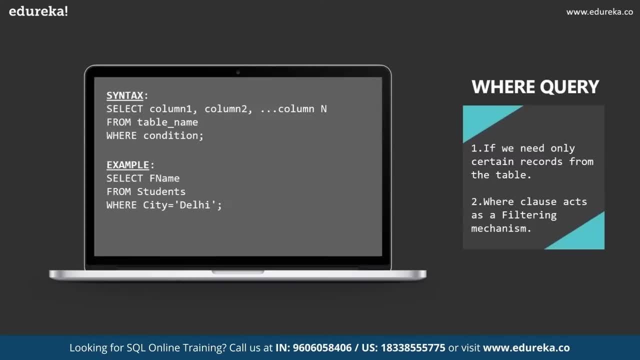 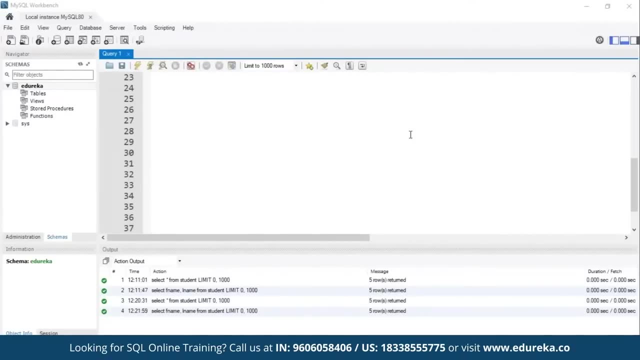 that fulfill the specified condition to demonstrate where Claus. Let me assume this scenario. If I want the name of the students who are from the city Goa, then my where Claus query will be something like this: Select first name from student where City is equal to Goa. 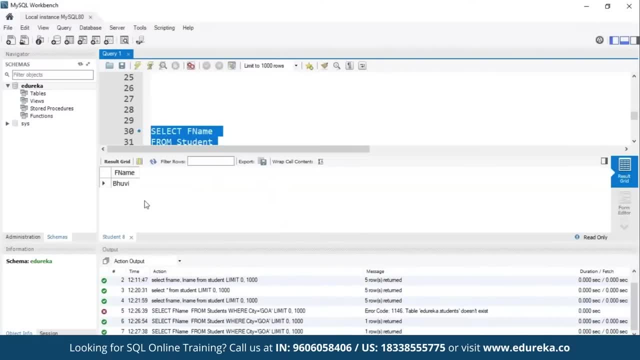 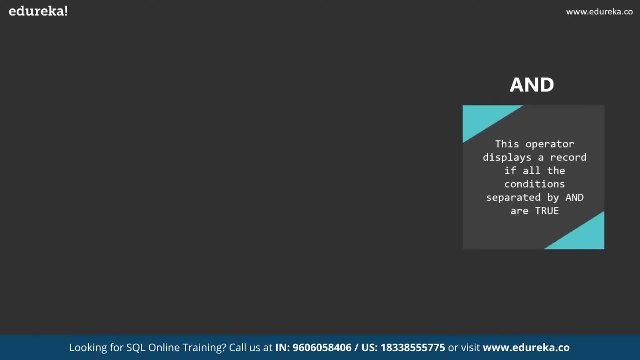 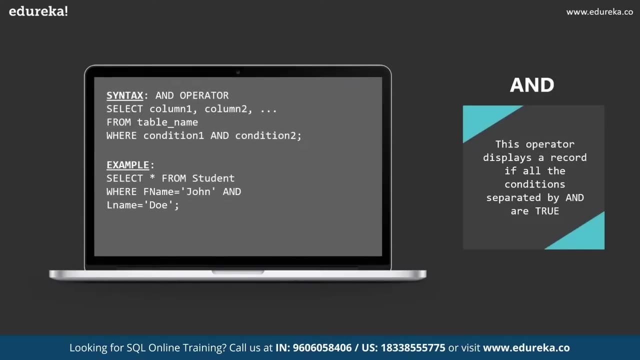 So let me select this query and execute it. So this is the output. Now let's look into and or not statements. If we need to add two or more conditions in the where Claus, then we can use the above mentioned operators. These keywords will add more complexity to the query. 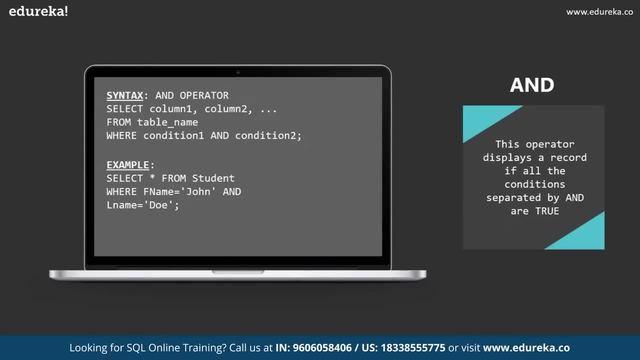 So the first operator is and operator. this operator display a record if all the conditions separated by the and operator are true. Let's look at the syntax. select columns from table where condition 1 and condition 2 has to be true to understand the example. 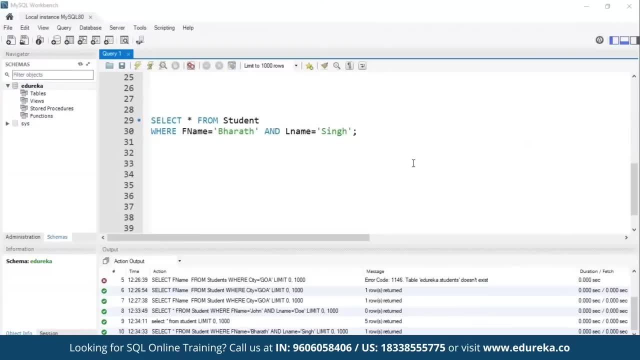 Let's dive into the demo part. I want to display the details of the student who has the first name as Bharat and last name as sing. to achieve this, I'm using and operator, So let me execute this query. Yes, I got the output for the student named Bharat Singh. 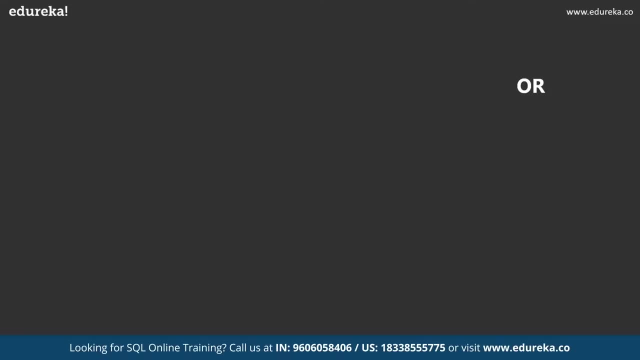 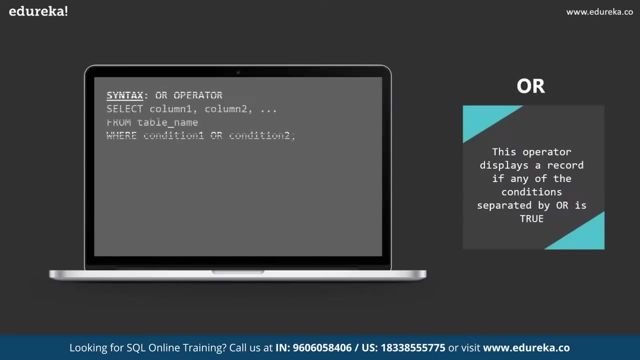 The next operator I'm going to discuss is or operator. or operator usually displays a record if any of the condition separated by or is true, and the syntax for this is: select columns from table where condition 1 or condition 2 is true. to understand the example, 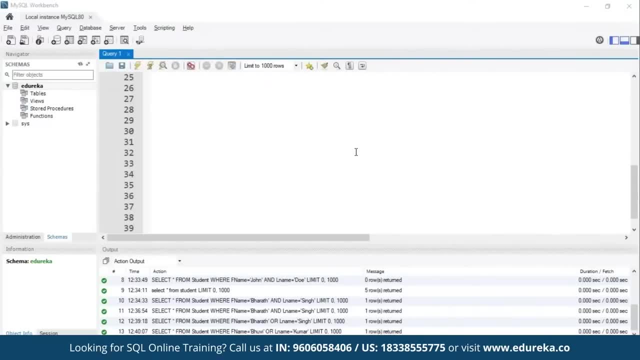 Let's dive into the demo. I want to display the details of a student who has the first name as Bovee or the last name as Kumar. to achieve this, I'm using or operator. here, Any one of the condition has to be true. 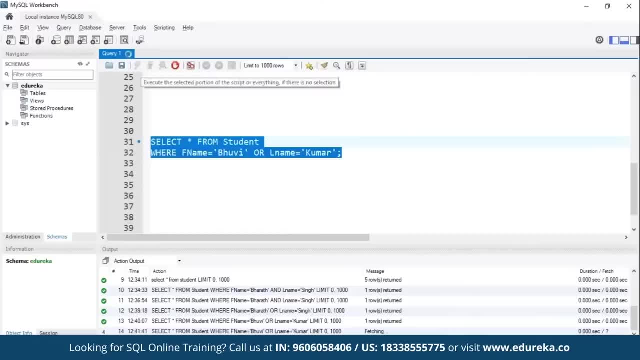 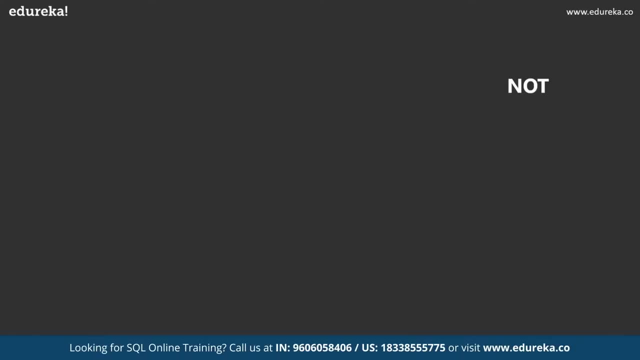 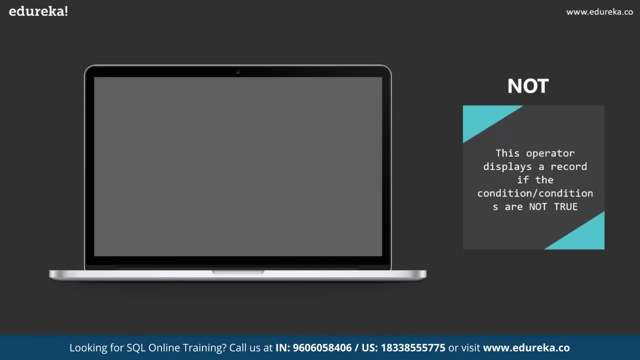 So this is the query to execute a scenario. So we have got the output for the student with the name Bovee Kumar. So let's head to the next operator that is not operator. So this operator display a record if the condition or conditions are not true. 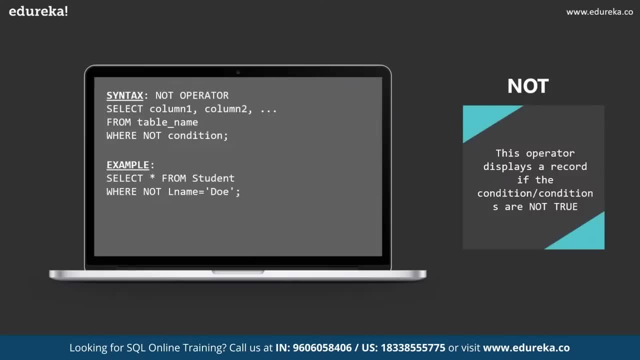 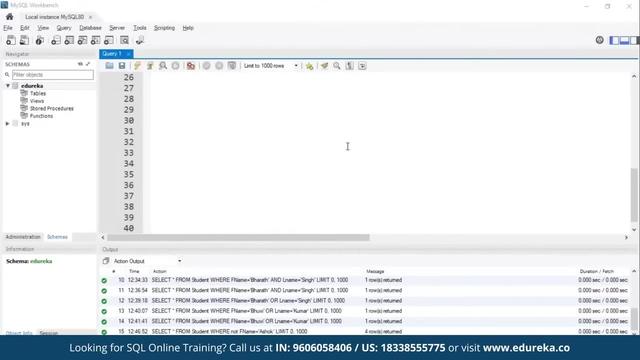 So the syntax is: select columns from table where the condition is not true. Let's see how this example works here. I want to display the details of the student who does not have the first name as Ashok. to achieve this, I'm using not operator. 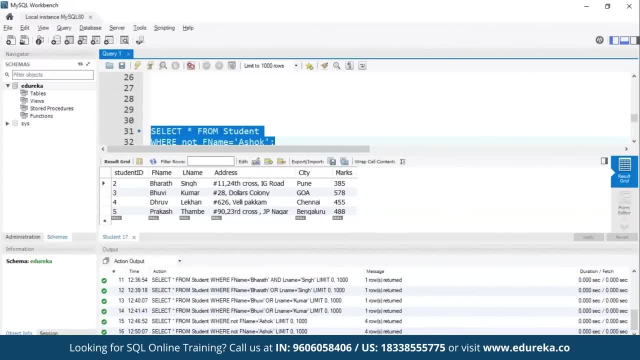 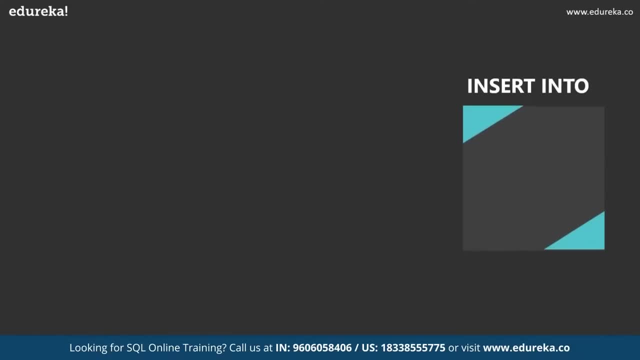 In this we can see the details of all the students except Ashok. So the next query I'm going to discuss is insert into. if you want to insert any record or data into a table, then we can use insert query and the syntax for this is: insert into is a keyword. 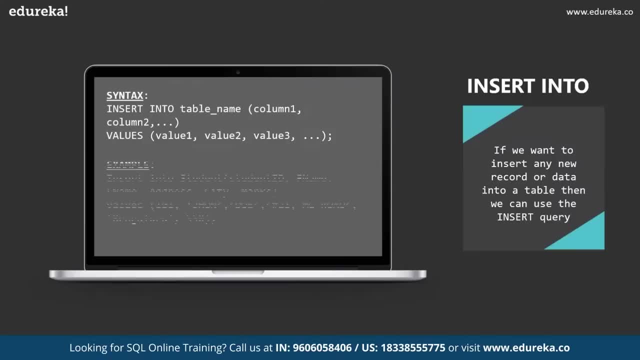 that is used in insert query, followed by that We have to specify the table name and columns. after that We have to specify the values. Let's look at the example to clearly understand the table name and columns. Let's look at the example. 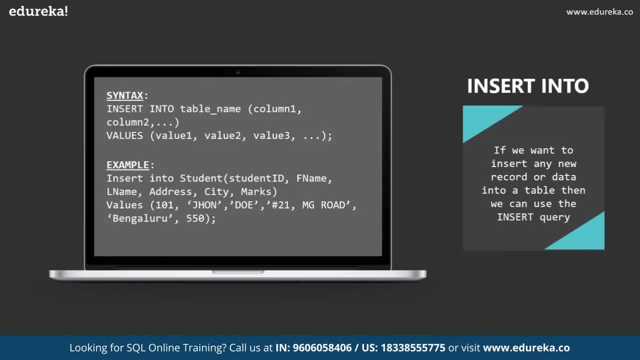 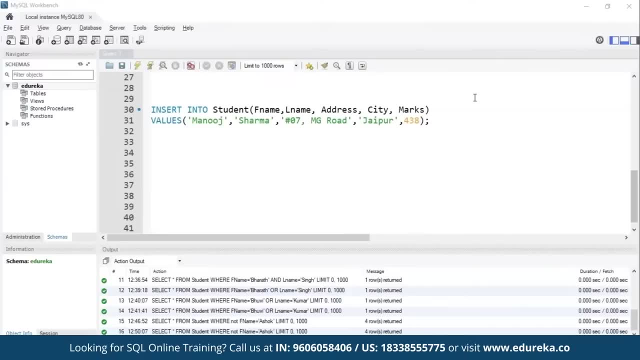 To clearly understand how exactly this query works. So this is the example for insert query. So we are going to insert first name as Manoj, last name as Sharma, address as 07 MG road and City as Jaipur. Also, the marks is 438.. 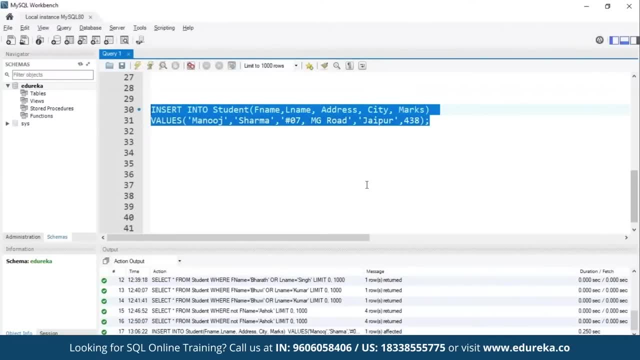 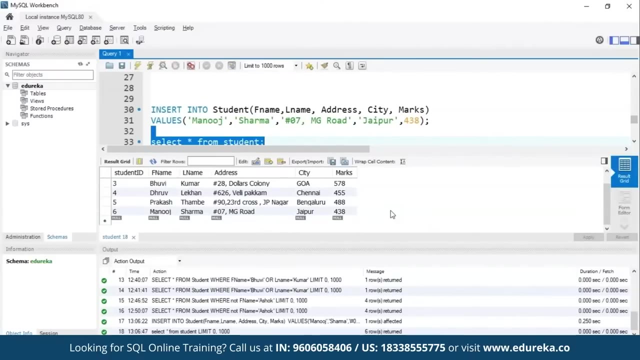 So let me execute this query So we can see that the data has been inserted. to check whether the data has been inserted or not, Let me use select query So we can clearly see that Manoj Sharma details has been added to the table. 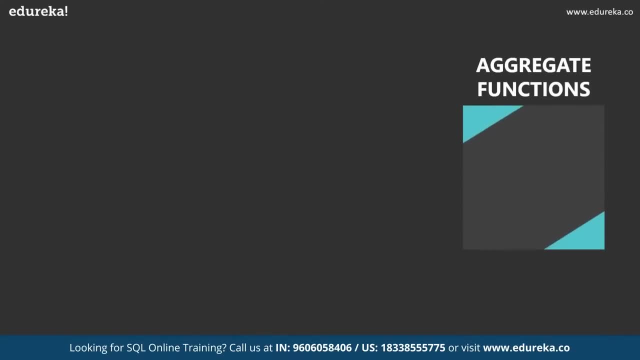 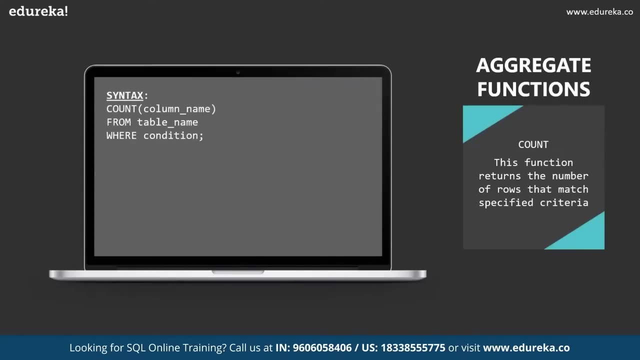 Next I'll be discussing few aggregate functions, and aggregate function is a function where the values of multiple rows are grouped together as input on certain criteria and a single value is written. We often use aggregate functions with the group by and having clauses of the select statement. 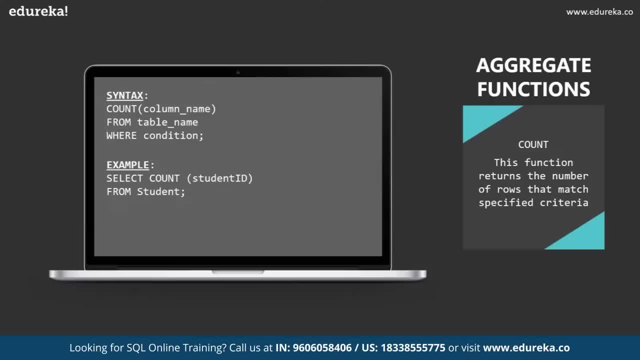 So we will be discussing group by having in the later part of the session. some of the aggregate functions are count, some average, minimum and maximum, So let's discuss each one by one. So the first one is count. this function returns the number of rows that match specified criteria. 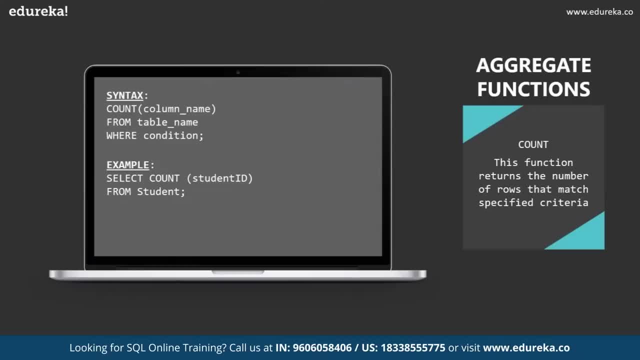 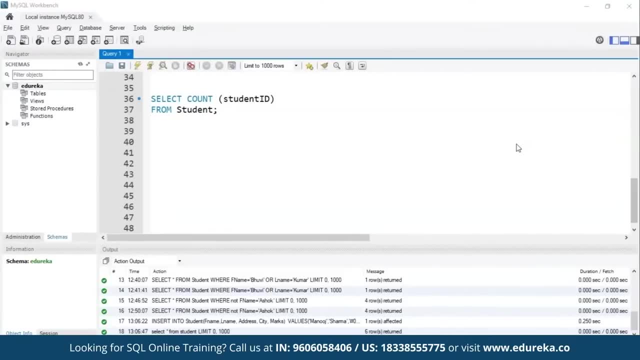 So the syntax is count of column name from table where the condition. so now let's try this example in my sequel workbench. using this query, I will calculate the number of student ID that is present in the table. So let me select this query in the output. 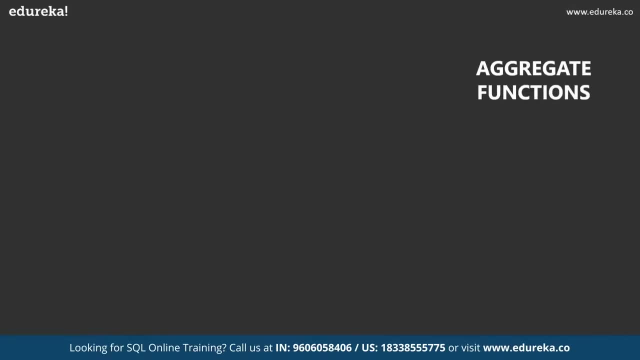 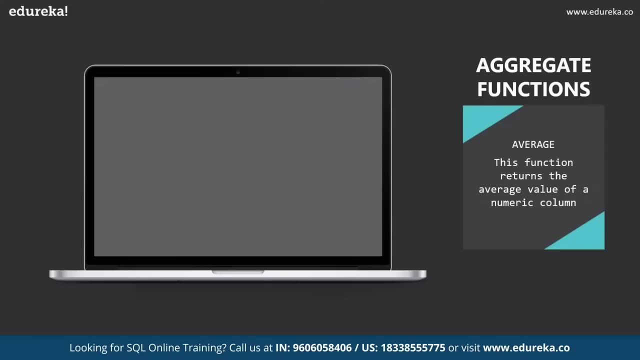 We can see that the count of the student ID is 6.. The next aggregate function is average, and average function returns the average value of a numeric column. So the syntax for this is: select average of column from table where condition. let's execute this example here: 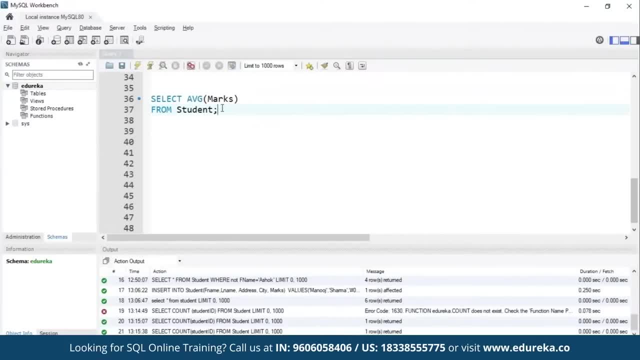 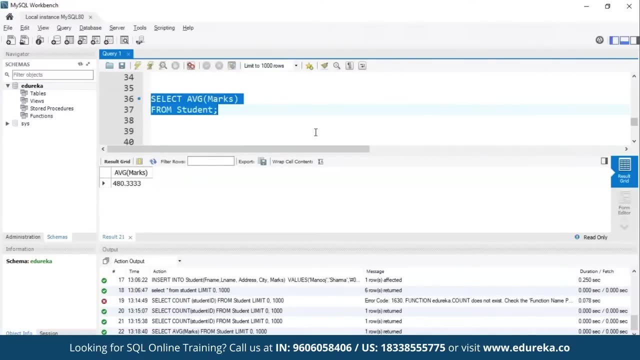 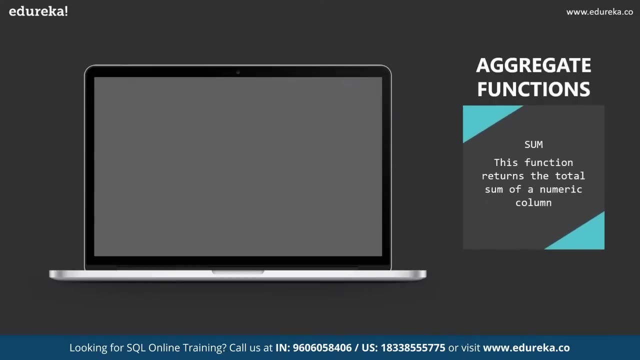 I'm trying to find the average marks code by all the students, So let me select this query. So the average marks code by all the students is 480. point three, three, three. the next aggregate function is some. usually some function returns the total sum of that particular column. the syntax is: select some. 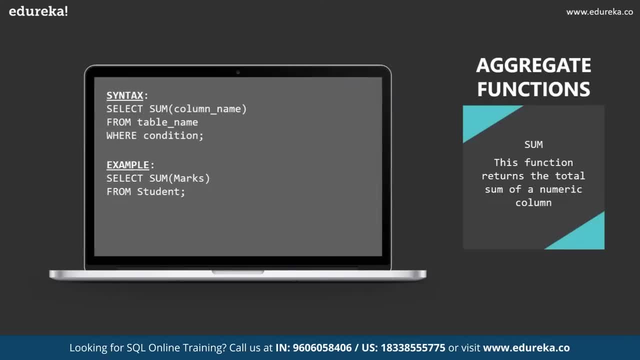 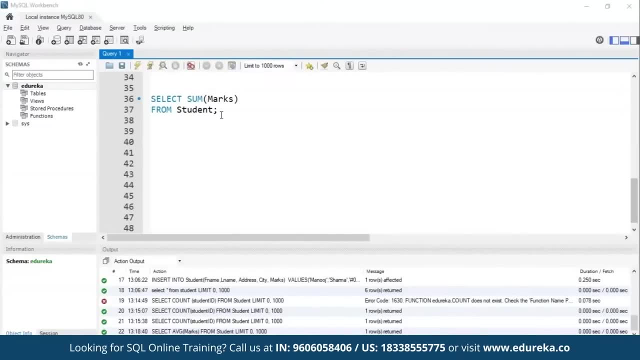 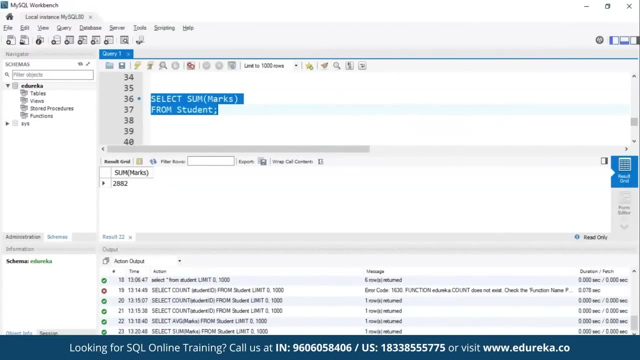 of column from table where condition. So let me execute this example. in this example I'm trying to find the total marks code by all the students, So let me select this query. The total marks code by all the students is 2882.. 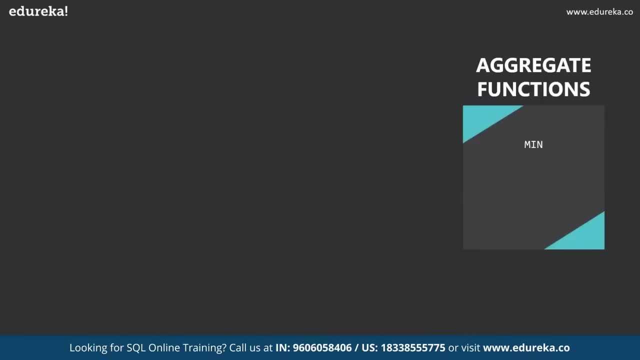 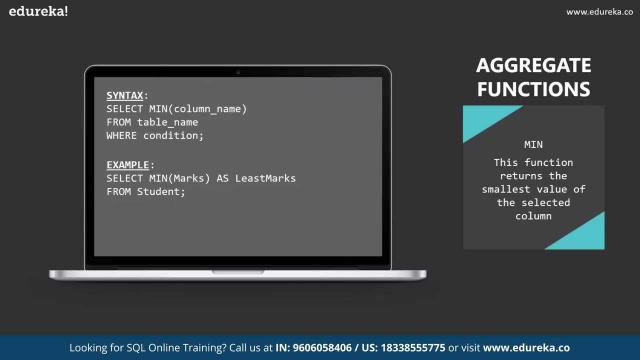 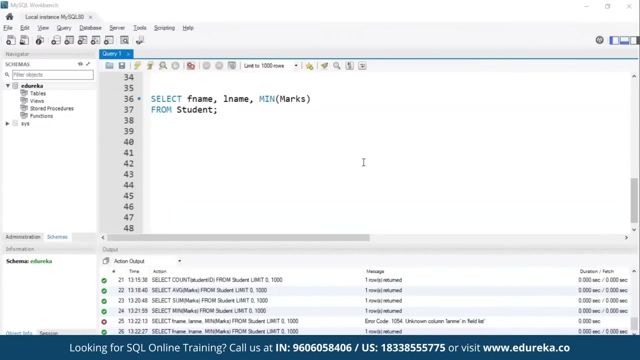 Moving on to the next aggregate function, That is, minimum. minimum function will return the smallest value of the selected column and the syntax is: select men of column from table where condition. So let me execute this example. If I want to know the student name who has scored minimum marks, 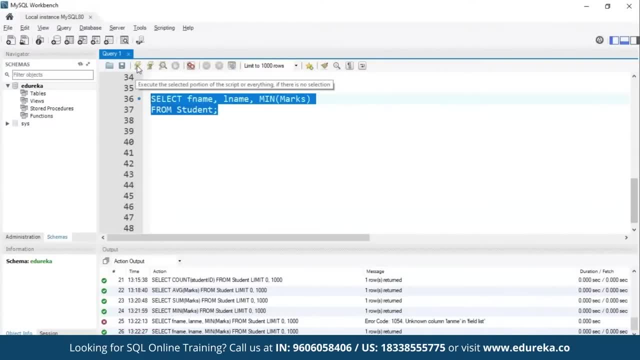 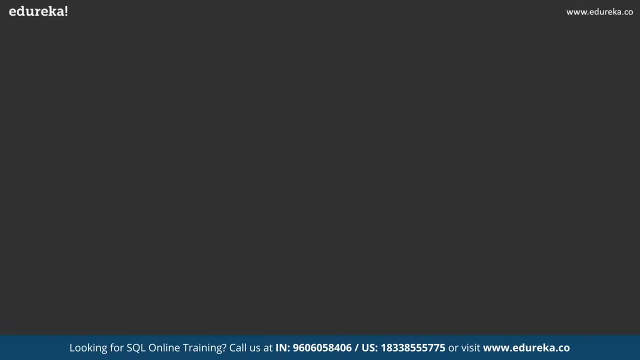 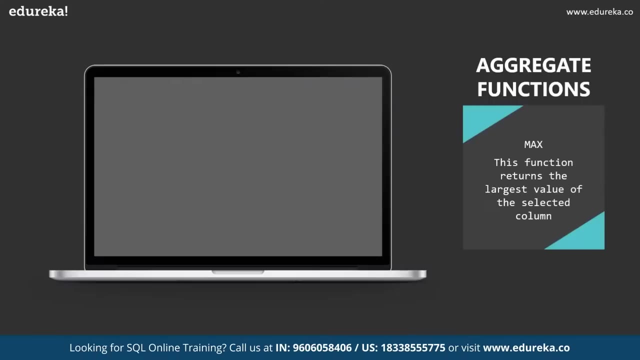 I'll use this query, So let me select this query. Ashok Sinha has scored 385 marks, and this is the minimum marks in this entire table, and the last aggregate function that we want to discuss is Max. Max function returns the largest value from the selected column. 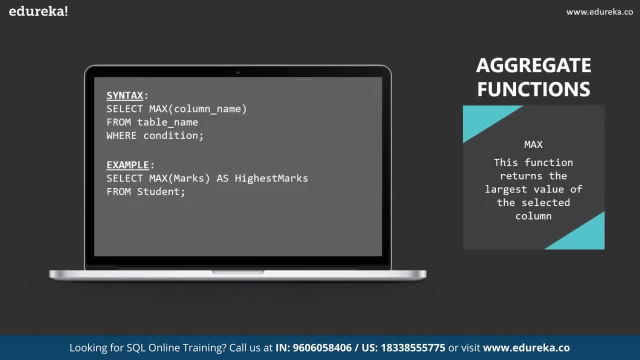 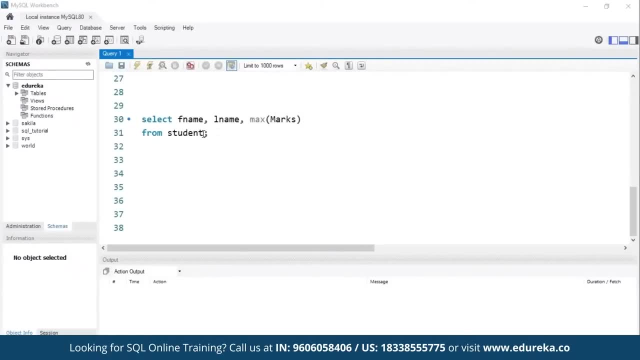 and the syntax is select Max of column from table where condition. let's execute this example. So this is the example for maximum function. So let me execute this query So we get the output. that is: Bharat Singh has scored 580 marks, So 580 marks is a maximum marks in the entire table. 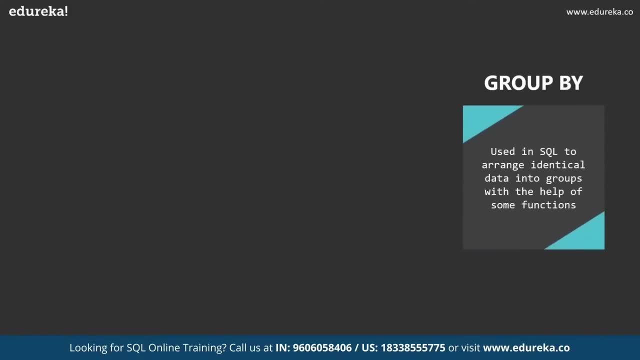 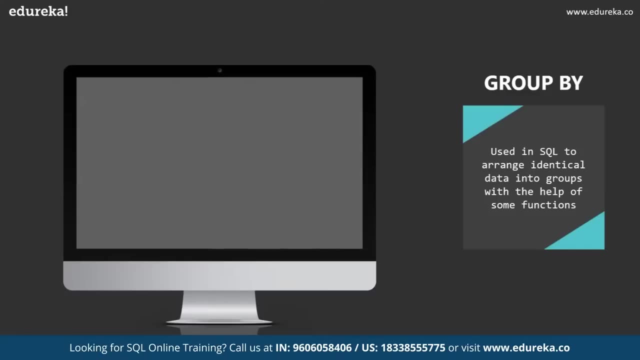 Next SQL query is grouped by group by is the functionality used to arrange a similar type of data into a group. For instance, if the column in a table consists of similar data or values in different rows, then we can use group by function to group the data. 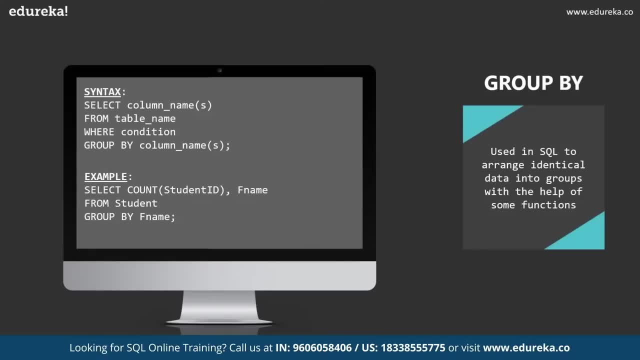 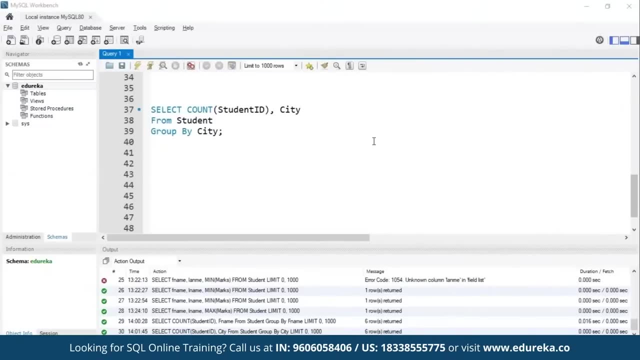 The syntax is select column from table where condition group by the same column. Let me execute this example. I want to count the number of student who are from different cities. If there is any student from same City, then the count will be incremented at the end. 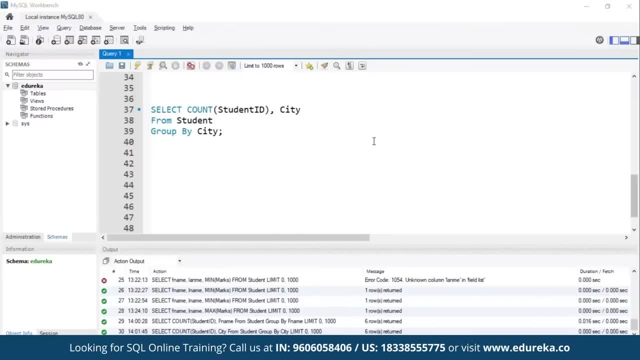 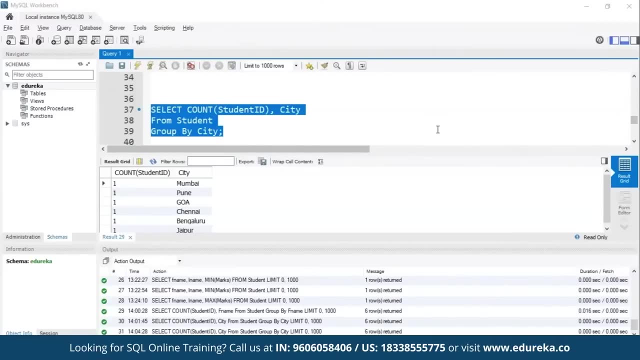 The output will have all the city name with the count of the students from that particular City. So let me execute this query. We got the count of student from different cities. since all the students are from different City, We can see that the count is one in all the cases. 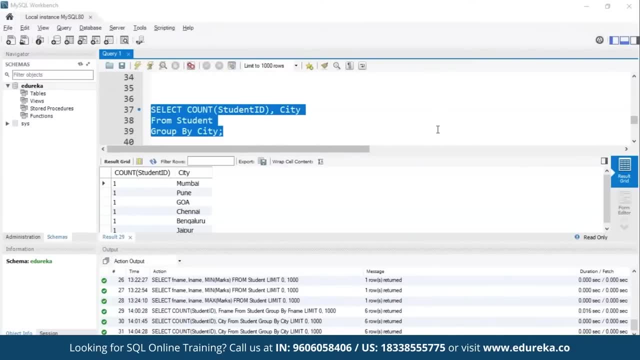 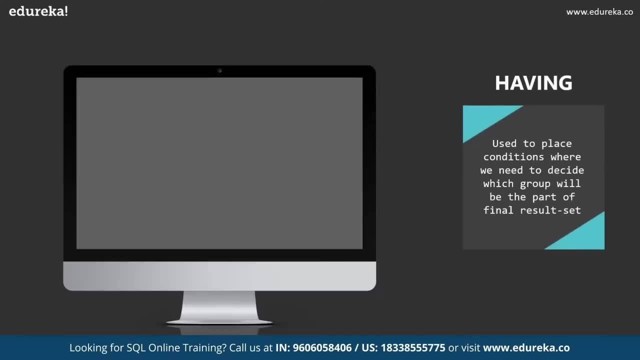 if the data is large, we can clearly get to know how effective this query is. Next query is having. this class is used to place condition where we need to decide which group will be part of the final result set. The having clause was added to SQL. 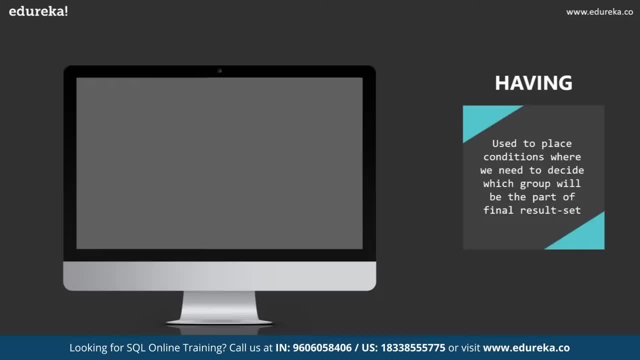 because the where keyword could not be used with aggregate function, such as some count, min, Max, Etc. So the syntax is: select column from table where, condition, group by the column and having condition. So let me execute this example in my sequel workbench so that you'll get an idea about having clause. 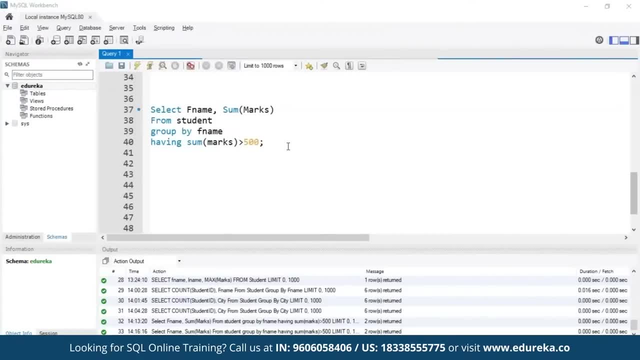 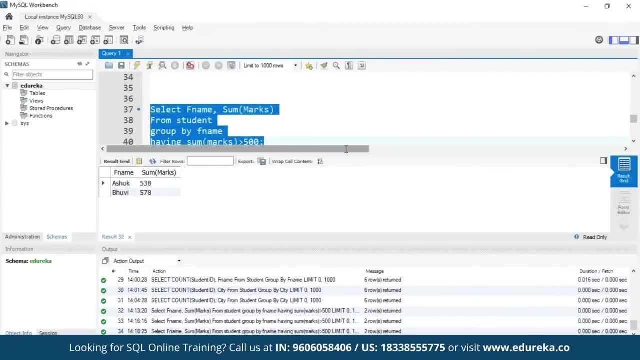 from the table. If I want to display the students who have scored more than 500,, then I'll specify that condition after having keyword. So let me execute this query So we can see that there are two students, Ashok and Bovee, who are scored more than 500 marks moving. 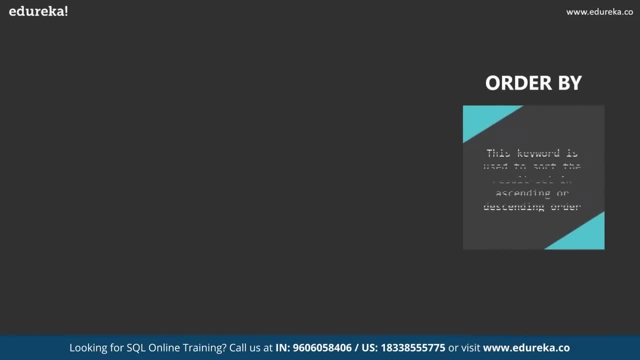 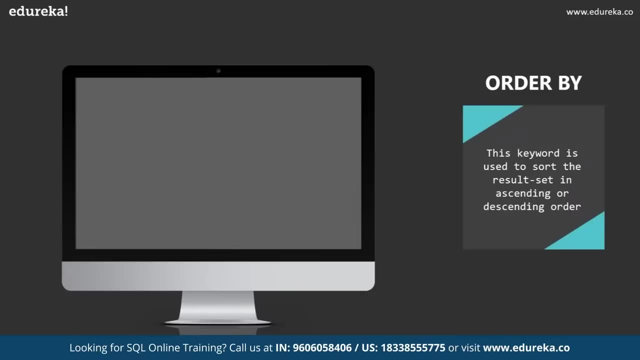 on to the next query, that is, order by order. by keyword is used to sort the result set in ascending or descending order. This keyword is used to sort the result set in ascending or descending order. the order by keyword shall sort the record in ascending order by default. 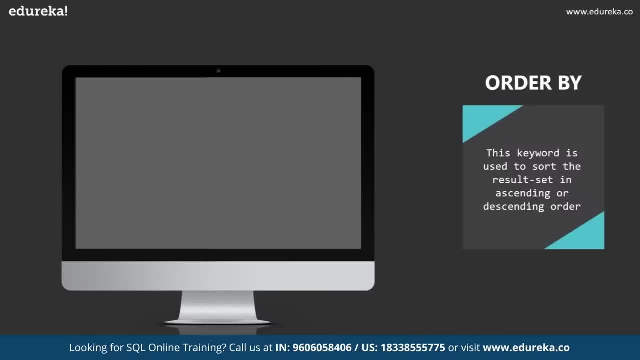 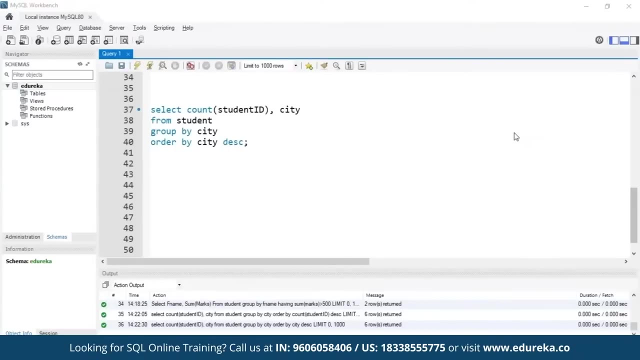 If we want to sort the record in descending order, then we need to use the descending keyword. So let me explain the syntax: select columns from table order by columns, either by ascending or descending. Let me execute this example. in this example we will get the count of students from different city. 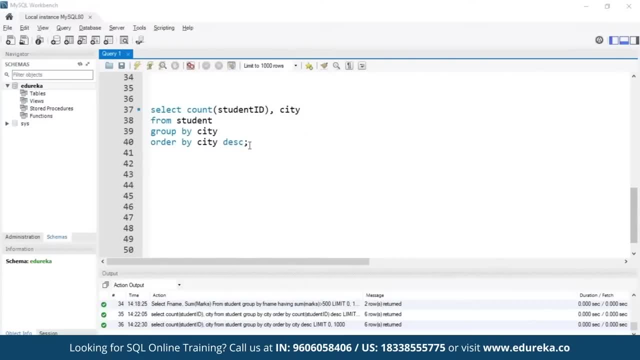 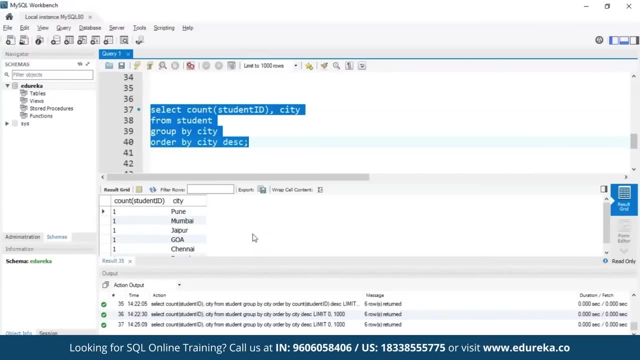 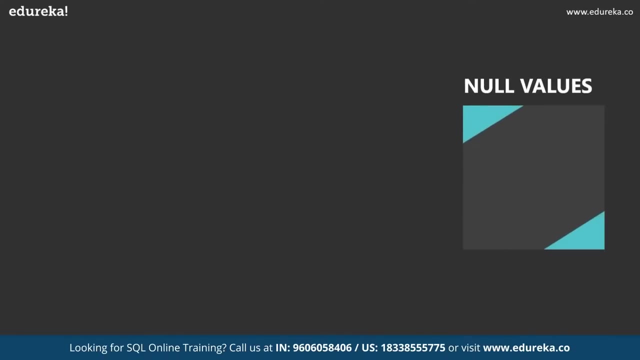 and we are arranging the city in descending order. So let me execute this query. We can see that the cities are arranged in descending order based on the starting alphabet. The next SQL query that we are going to learn is null values. in SQL, we use the null term to represent a missing value. 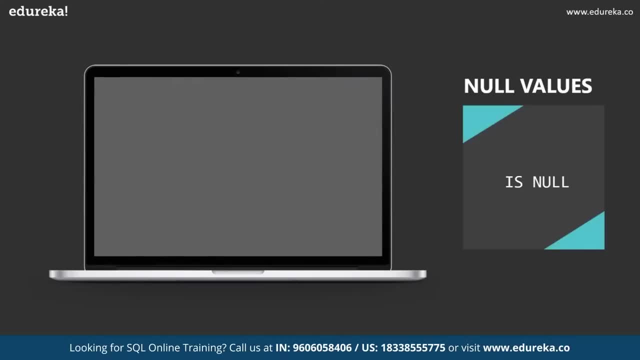 a null value in a table is a value that appears to be blank. a field with a null value is a field with no value in SQL Keep. note that a null value doesn't mean that the value is equal to 0. to check the null value: 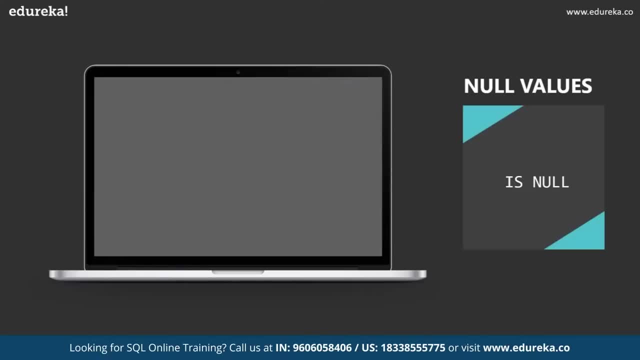 We are not supposed to use the operator such as greater than less than equal to. these operators are not supported in SQL. We have special keywords. Those are: is null and is not null. first Let's look at the is null operator. is null operator is used. 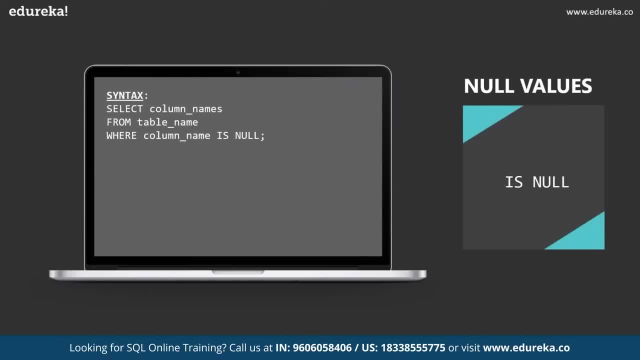 to test the empty values, and the syntax for this is: select columns from table where column is null, So let me execute this example. I want to display the student's name whose marks is null, So let me select this query and let me execute this. 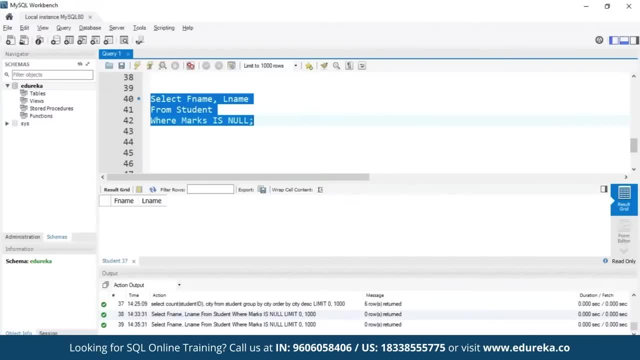 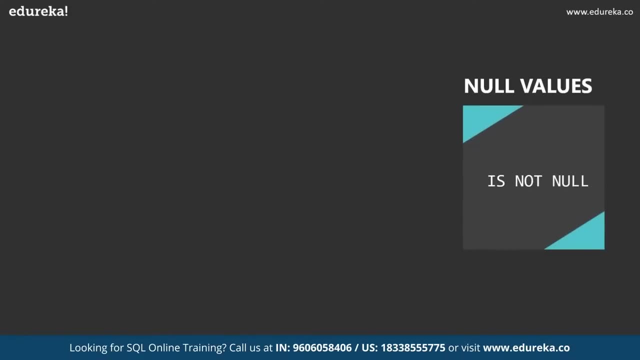 Since all the students have marks and none of them has null value in the output, We don't have any student names. The next query is: is not null? The is not null operator is used to test for non-empty values and the syntax is: select column from table. 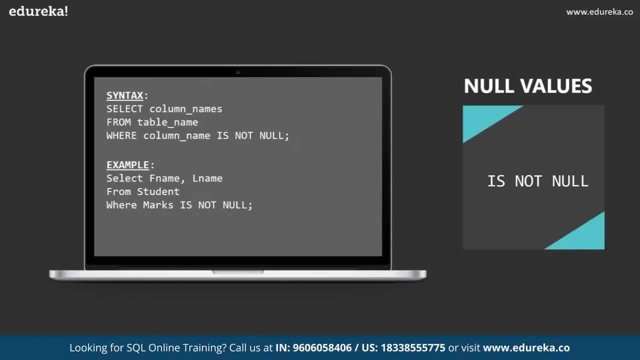 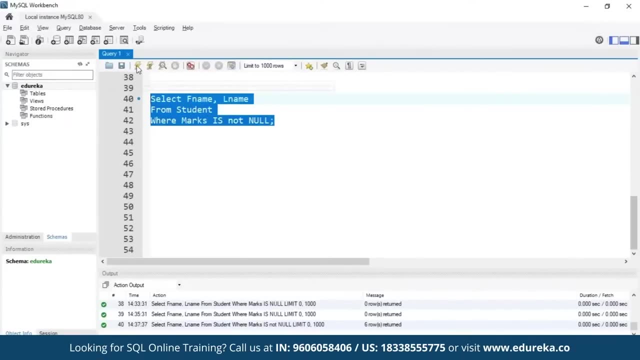 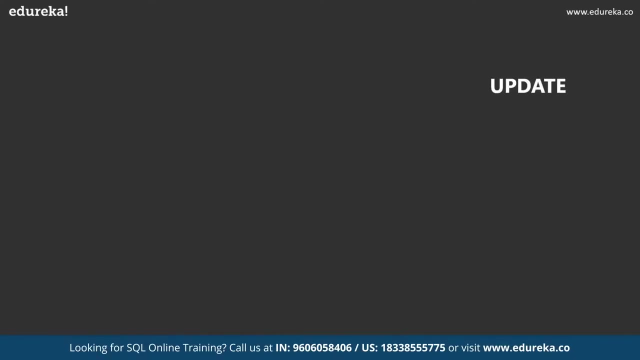 where column is not null. So again, let me execute this example. I want to display the student names whose marks is not null, So let me execute this query. Since all the students have marks, all the student names are displayed. Let's move to the next query, that is, update generally. 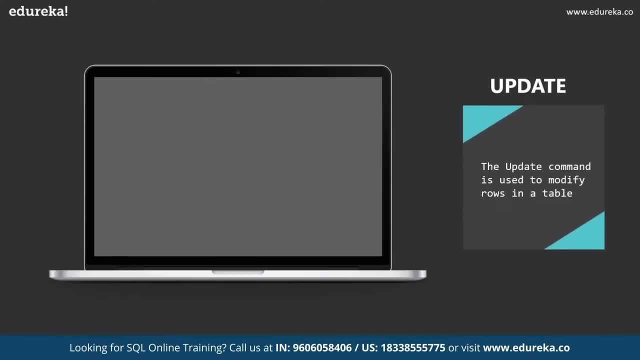 the update command is used to modify rows in a table. The update command can be used to update a single field or multiple fields at the same time. Let's look at the syntax for update statement. update table set column equal to value where- condition. let's execute this example here: 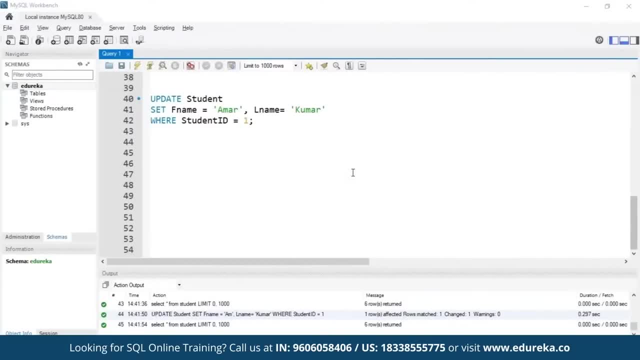 I want to change the name of the student with student ID 1. previously, the student with student ID 1 was Ashok sin now. Now I want to change his name to Amar Kumar. So let me execute this query So we can see that the student name has been updated. 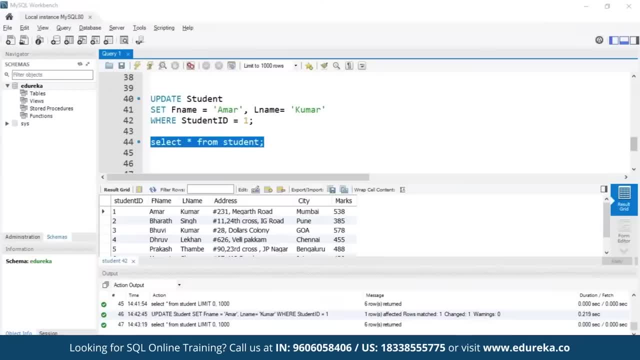 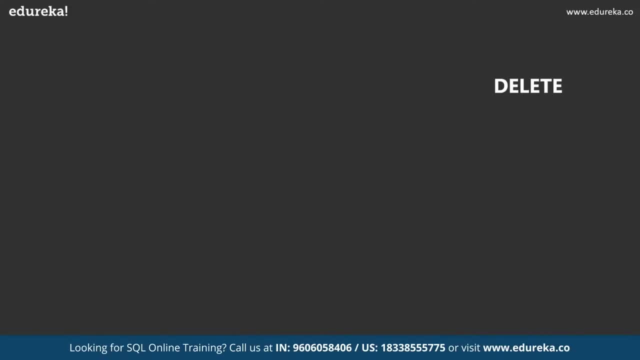 To check the student table. Let me execute this query and we can see that the name of student ID 1 has been changed from Ashok sin, not to Amar Kumar. the next query We are going to discuss This is delete. the SQL delete command is used to delete rows. 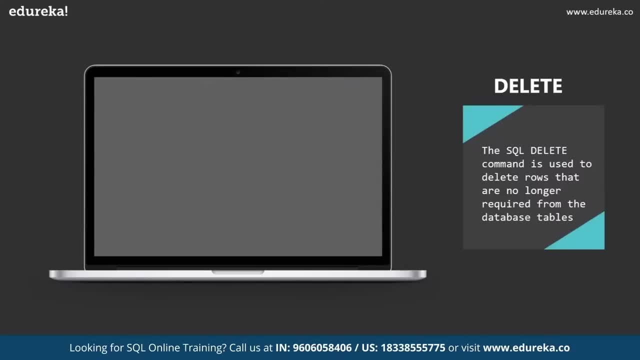 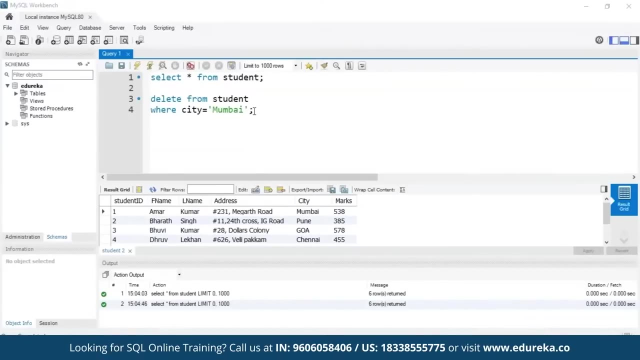 that are no longer required from the database tables. It deletes the whole row from the table. The syntax is delete from table where condition, so let me execute this example. If we want to delete a record from student table where the city is Mumbai, Let me execute this query. 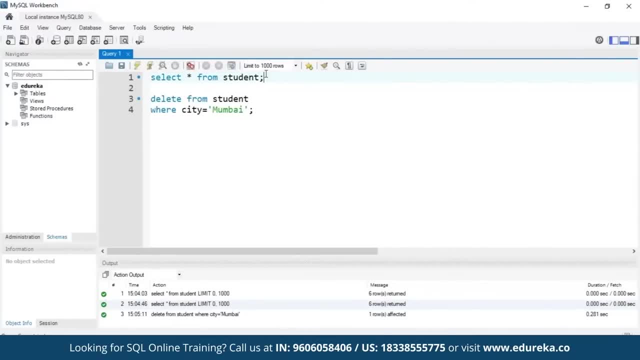 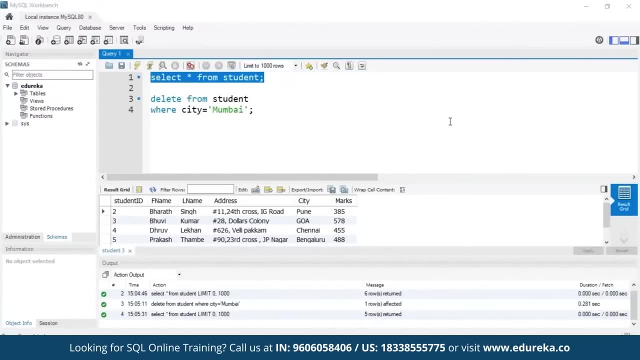 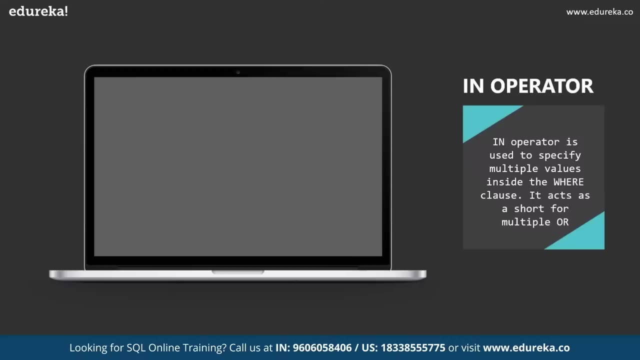 So we can see that the query has been executed. to check the table, Let me execute this statement And student with the ID 1 has been deleted. next Let's discuss in and between operators. in, operator is used to specify multiple values inside the where clause it acts. 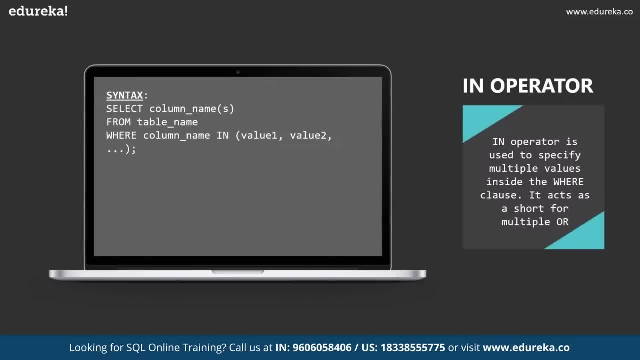 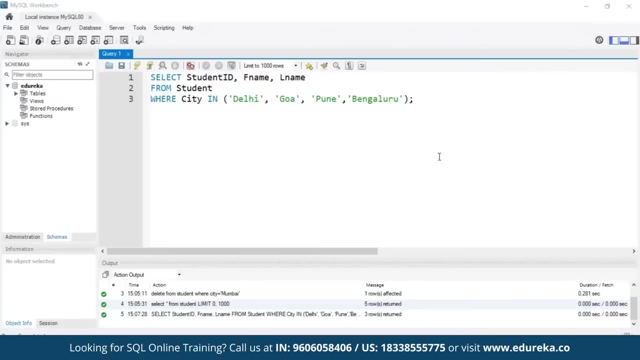 as multiple. or let's look at the syntax: select column from table where column in value. Let me execute this example. If we want to display the record of a student who are from certain City, then we can use in operator in the given example. 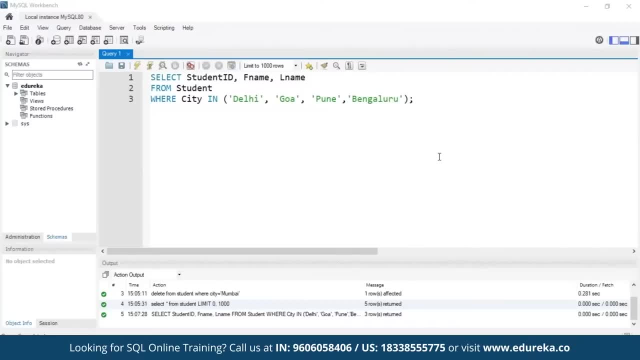 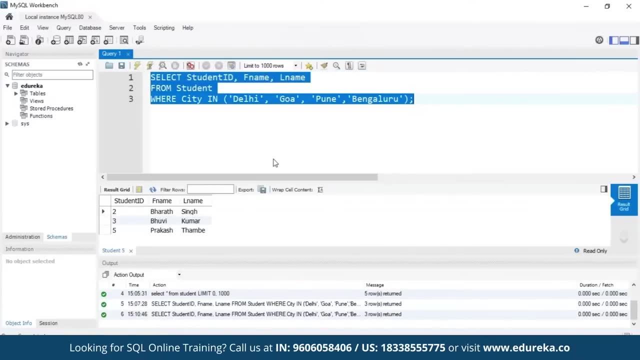 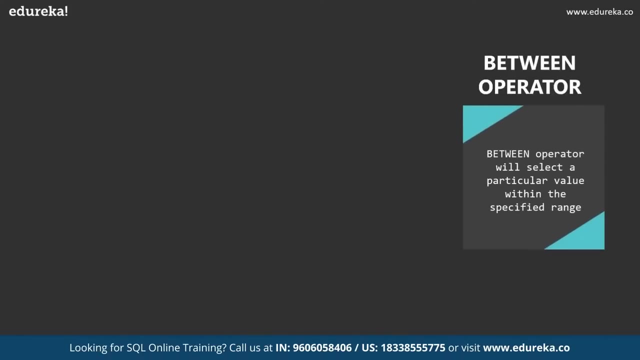 Let's display the name of the students, along with their IDs, who are from Delhi, Goa, Pune and Bengaluru. Let me execute this query. In the output, only those students from the specified City name are displayed. The next operator is between: between operator will select. 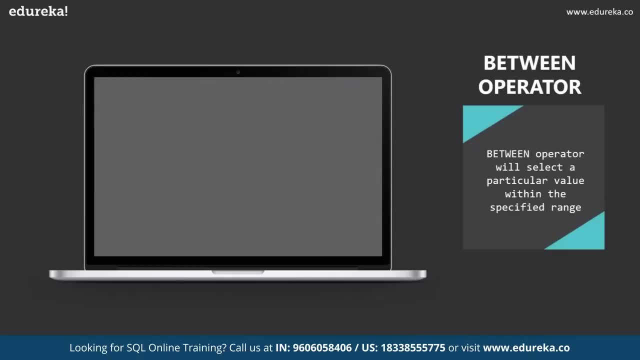 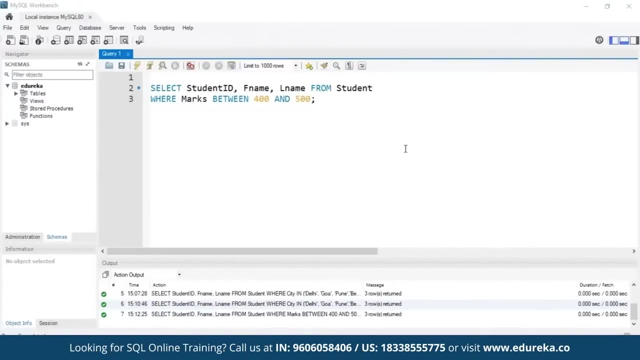 a particular value within the specified range, It is compulsory to add the beginning and the end value. Let us look at the syntax. select column from table where column name between value 1 and value to. let's execute this example: If you want to display the record of students whose marks 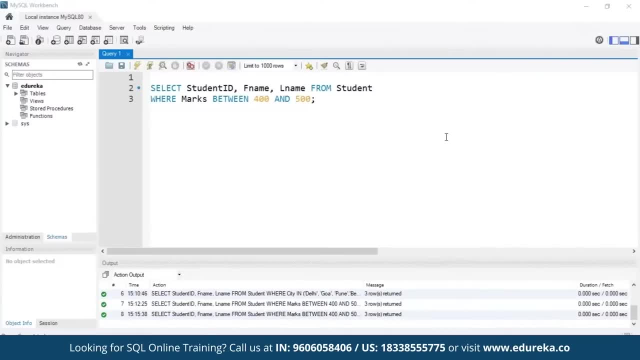 are in certain range, then we can use between operator. in the given example, Let's display the name of the student, along with their ID, who has scored in the range of 400 and 500.. So let me execute this query. In the output only those student records. 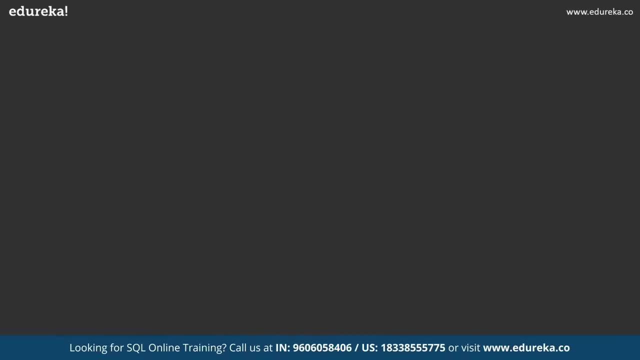 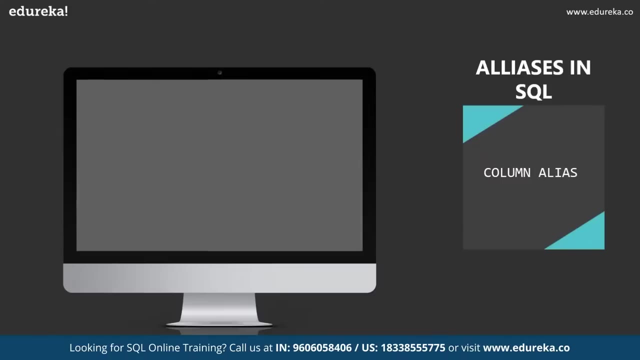 who have scored in the range of 400 and 500 has been displayed. So the next topic we're going to cover is aliases in SQL. Alias is a process of giving a table or a column a temporary name so that it helps when the query is complex. it increases the readability. 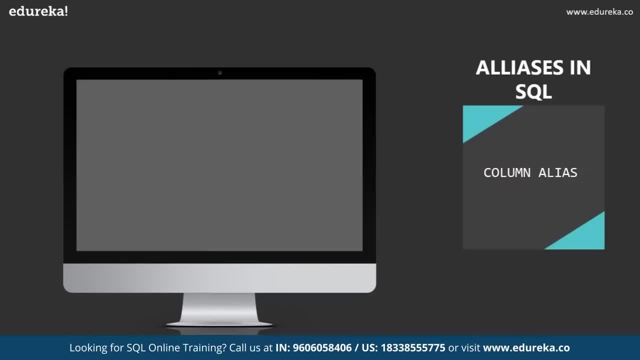 of the query. this renaming is temporary and the table name does not change in the original database. We can alias our column or a table. So the first concept is column aliasing and the syntax is select column name as alias name from table. So let me execute this example in the student table. 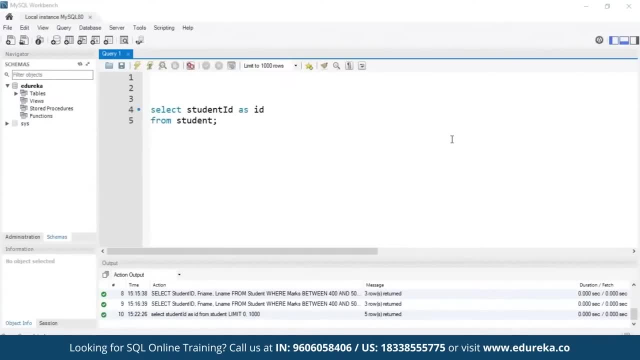 The column name student ID is bit long. when we write a nested query We might face some trouble in order to tackle such situation that alias that student ID column as ID. So let me execute this query And we can see that the column student ID has been aliased. 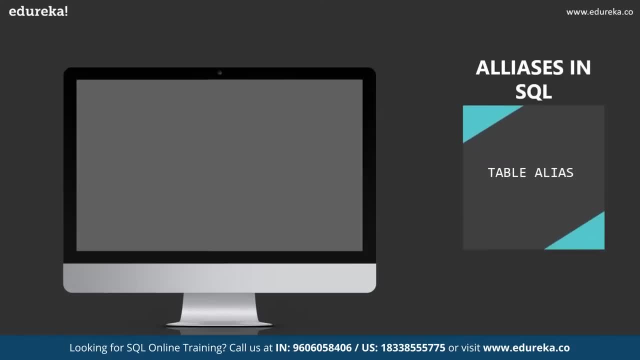 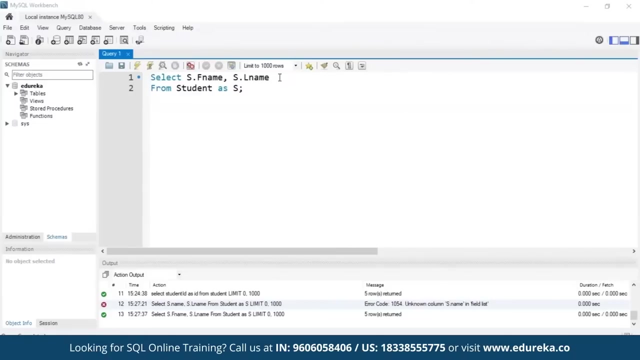 to ID. next is table aliasing. Now let's look at the syntax for table alias, and the syntax is: select column from table as alias name. So let's execute this example. We generally use as keyword in aliasing, So let me execute this query. 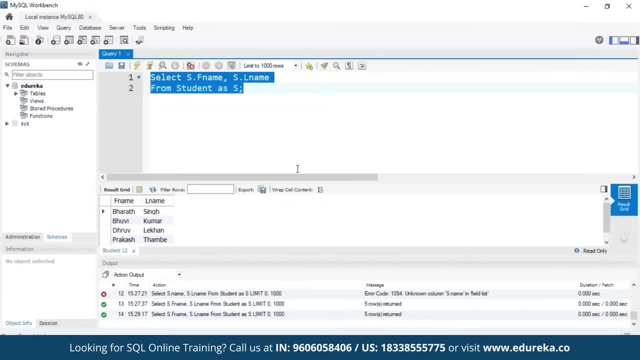 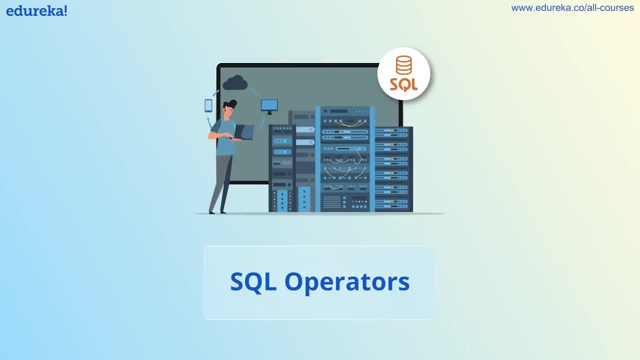 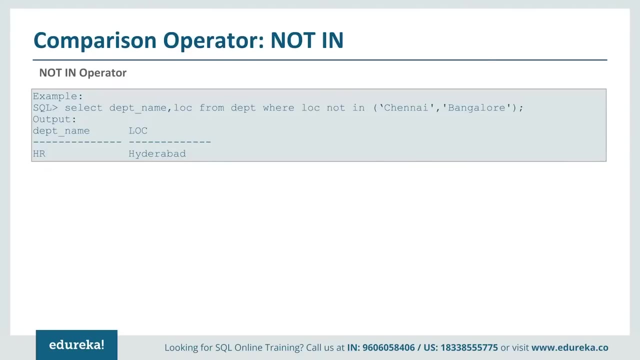 By using the technique of table aliasing, I have displayed the names of the students from the student table. So that was a basic concept of SQL. Not in, so not keywords is not, is basically logical operators and it is used along with other operators like in and other. 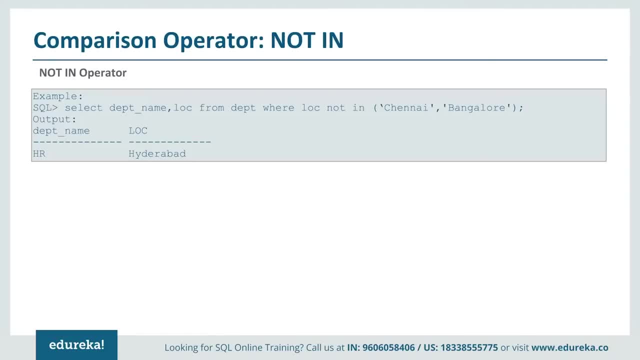 so we have just seen one example where we want to show the departments which are not in Hyderabad. So this is the repetition of the same example. The previous example which I showed. I include only one locations, but we can use multiple keywords. If you're using the in keywords will see the example. 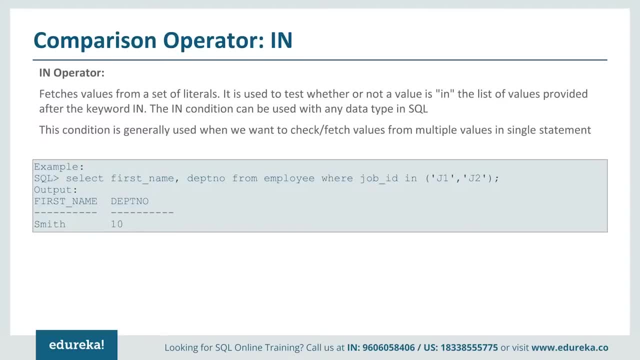 It's not in in operator fetches values from a set of literals. So this conditions is generally used when you want to fetch values from multiple values in a single Statement. So it's not that I can use, only in, I can use our operators. 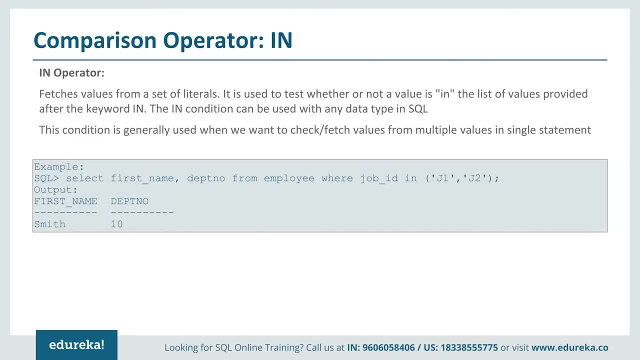 So if they only one or two conditions, I can either use our operator or in operator. But if the values are more, it is not good idea to use so many or operators or logical operators. Let's assume I want to see the results: intensities. 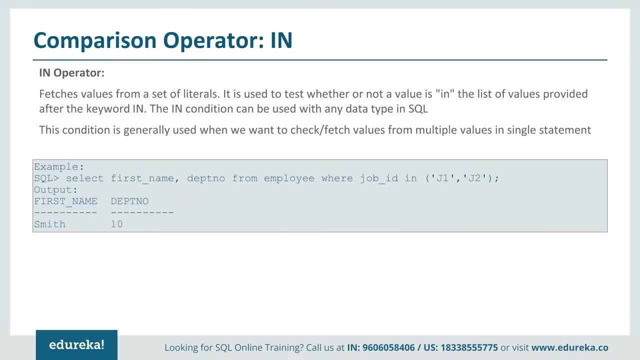 So if I write, if it like where location is equals to Mumbai or New Delhi or Hyderabad or Bangalore or Chennai, it is not readable, It's not good. So instead of writing so many or operators, we can use in operators, So the in operator, we basically include all the values. 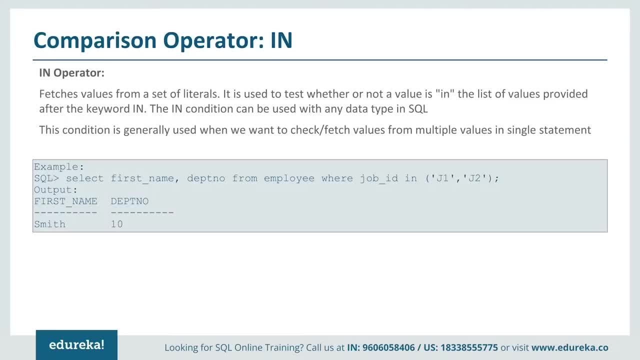 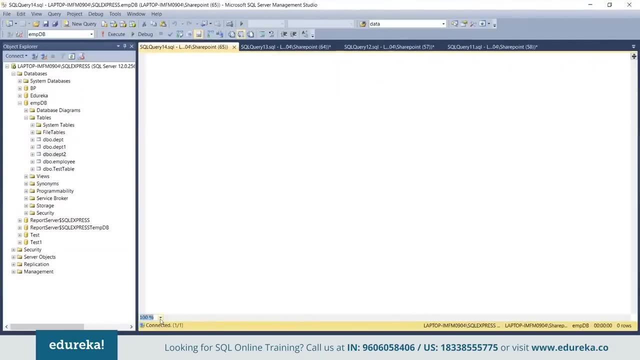 out of which we want to filter our results or we want to fetch our values. Let's see with an example. So let me open a new query window and right select Some department. So if I want to see the results or see the departments, 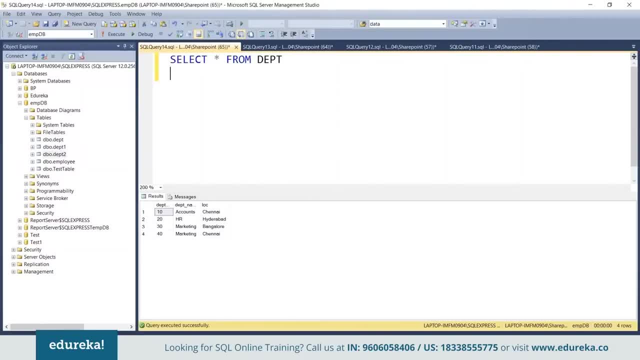 which are either in Chennai or Bangalore. So how right, right, select star from Department their location in. it can be in any one of these location. That's how we are. Bangalore. Don't forget to include strings or characters in single codes in SQL. So this is: 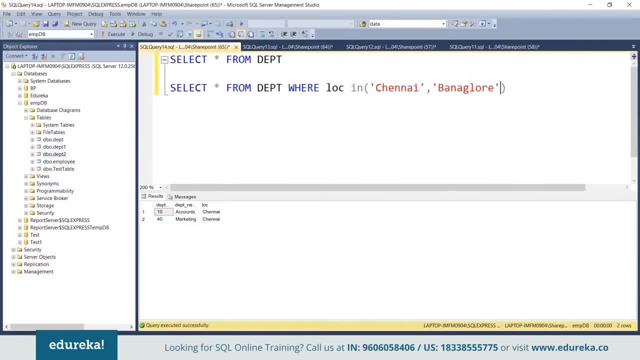 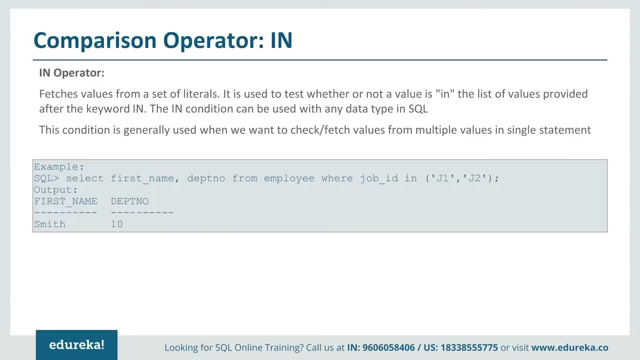 Fetch the desired results so we can use multiple values in the parenthesis if we used in comparison operator. So if I use not in, then this will go in a negation and will show the opposite of what in operator is doing. So we have discussed not in as well as in. 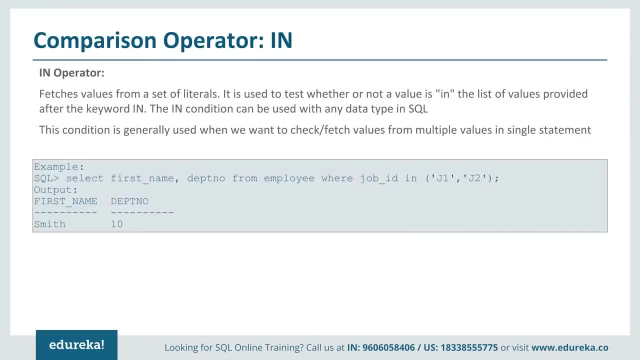 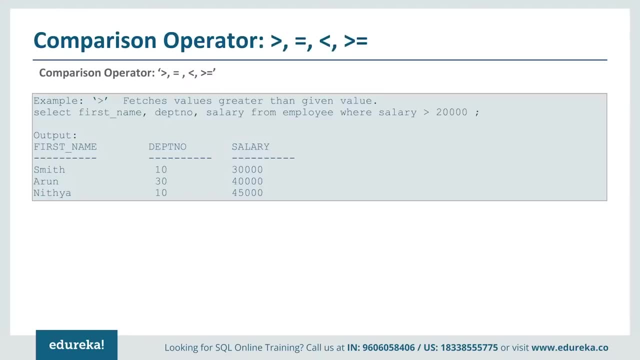 so if there are multiple values instead of or we have to use- it is good practice to use in keyword Then basic compression operators. We have greater than equals to, less than greater than equals to, So this is pretty much self-explanatory. So if I want to select the employees whose salary is greater than 20,000.. 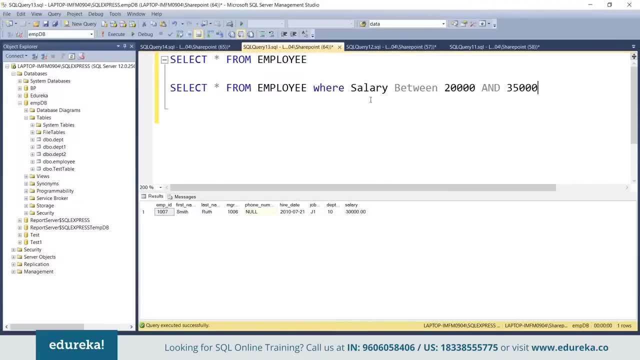 So let's see how we'll get the results. So I can use the previous window. So where's salary? instead of this, I can write salaries greater than 20,000.. So I'm getting three results. So I have three records, or three rows, or three employees. 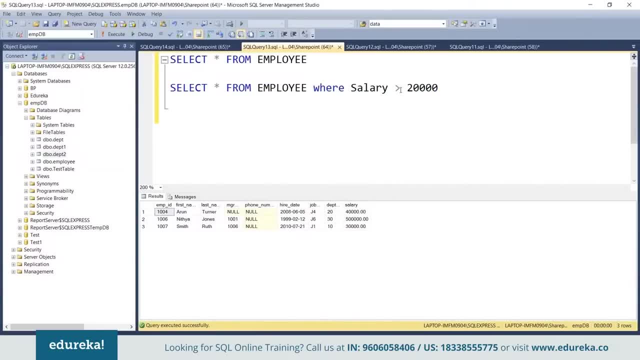 Whose salary is greater than 20,000.. So if I include greater than or equals to, then I guess I'll get four reasons. Oh, I don't think. so We have a salary of 20,000 here? No, we don't have. so let's take the example of 30,000 here. 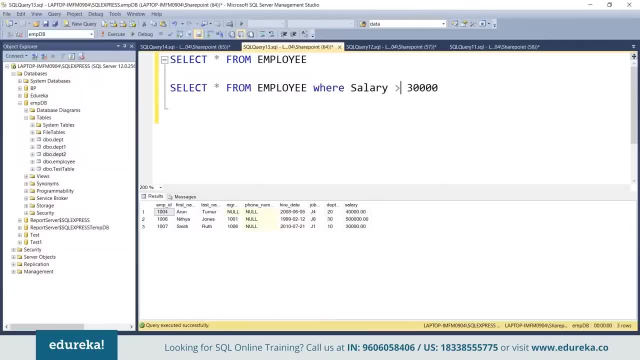 So we'll get the three results, But if I remove the equals to keywords, then of course we'll get only two rows in the result set, And if I use the equals to, then we'll get the only single row which will satisfy the desired or required condition. 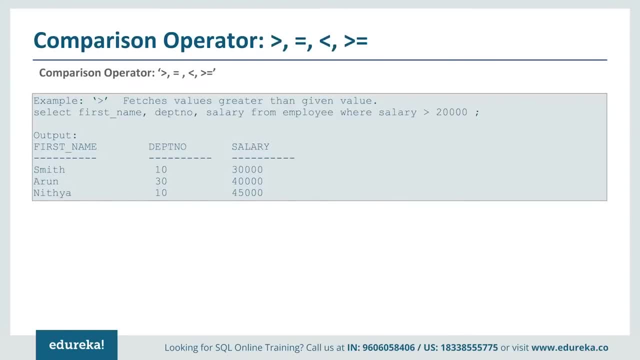 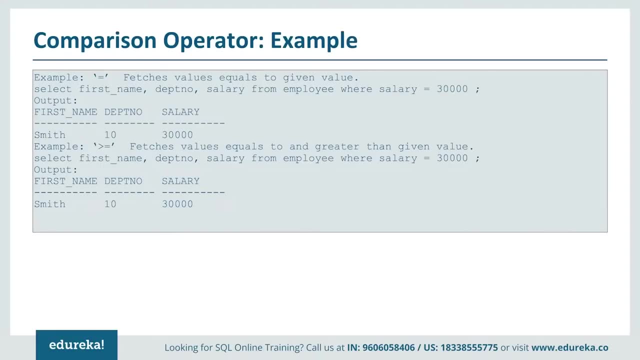 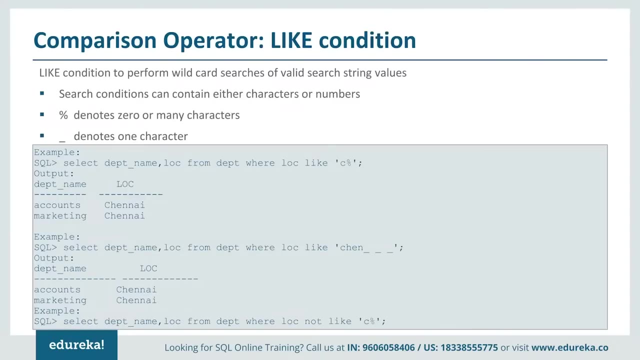 So this is how we use a various operator: greater than equals to. less than greater than equals to. again This example, you can use equal operator. It will satisfy the desired conditions. fresh. the results comparison operator is the like how we use the like keywords in comparison operator. 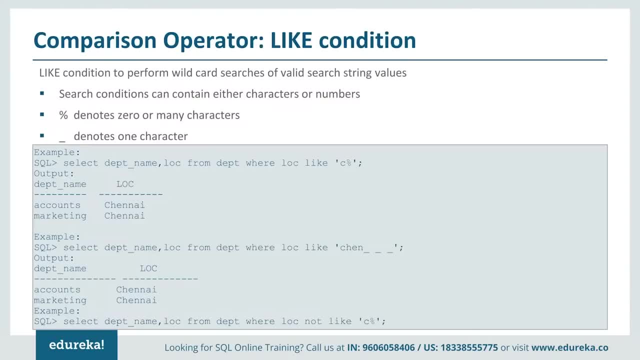 So generally we use like operators to perform wildcard searches of valid search string values. as I mentioned earlier, that like keyword is generally used when we are filtering or fetching the strings. So it used with two wildcards. One is percentage, percentage denotes zero, many characters, and underscore denotes one characters. 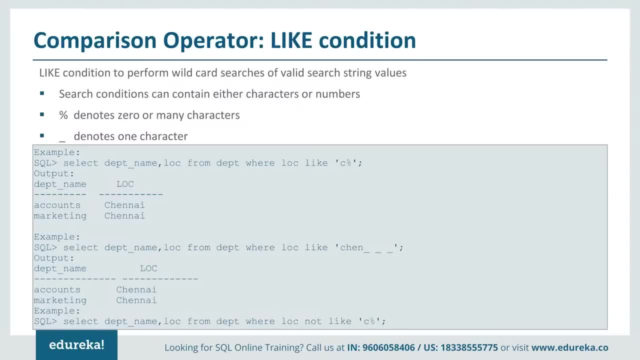 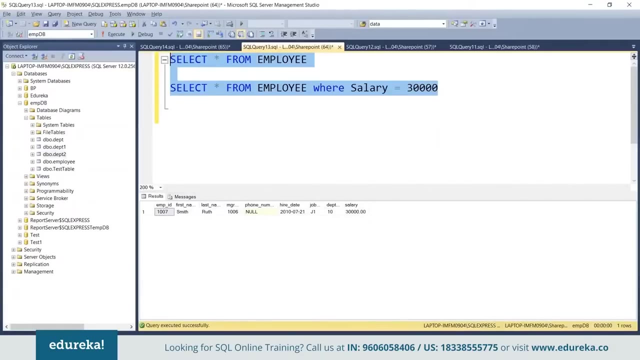 So let's see. So in the first example, as you can see, I'm getting the values from the department table. Those locations starts with C or the C alphabets. Let's see how we can use it. So we'll first see how we use the percentage wildcard. 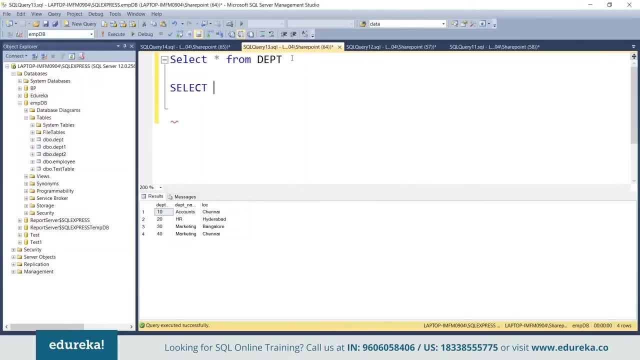 So if I want to know that, what are the different departments where the location start with the alphabet C? So we'll write selects star from Department where LLC. I have to use the like keyword, Like parenthesis and then the keyword C with a percentage sign that is wildcard. look at the results. 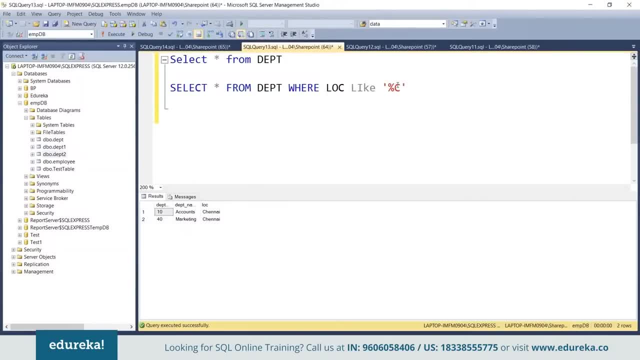 If I just change the order, if I'll write the wildcard first and then see, it means I have to show the departments whose location ends with C. So if I'll write it I here, then again I'll get the desired cell because I am fetching the rows. 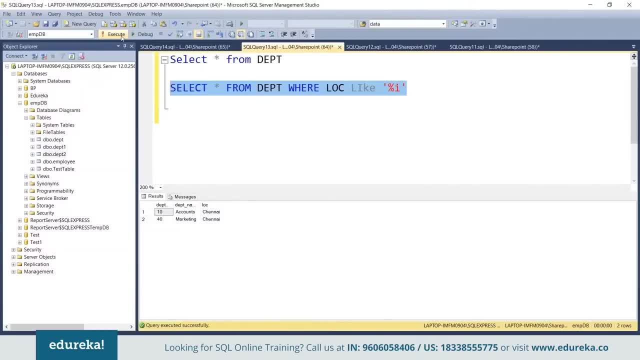 whose location ends with the I keyboard or I alphabet. So if I use first wildcard and then alphabet, it means it ends with. if I first use the alphabet and then wildcard means it's start with. if I write something like this: it see, then wildcard and I, it means it start. 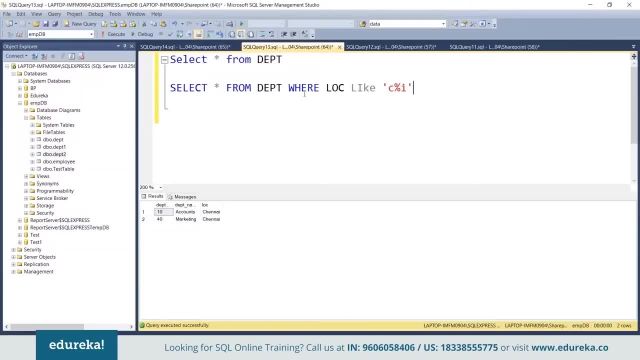 with C and it ends with I, so fetched me the locations who start with C, because I'm using the C before the wildcard and since I'm using I after the wildcard, so it ends with I. if I'll execute this query again, it will show me the same results, because if I change it, 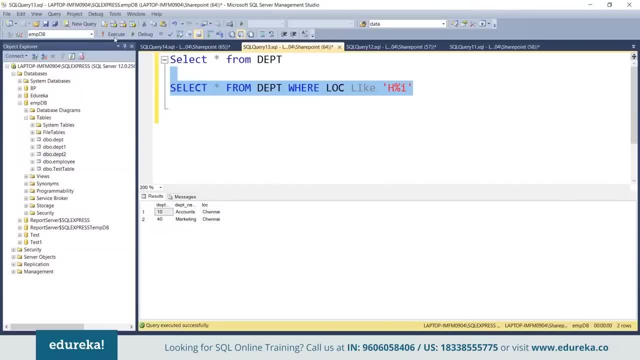 for example, I'm starting with edge and ending with I, so there's no department with such a condition. So we'll get the empty diesel set knife. I need to show that. show me the department who starts with H. in that case, All I have to do is that we have to remove the I, so we have. 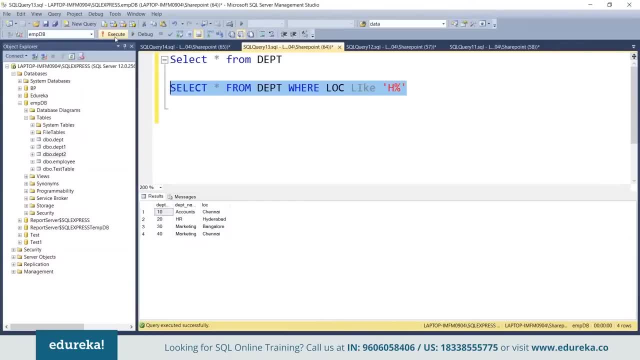 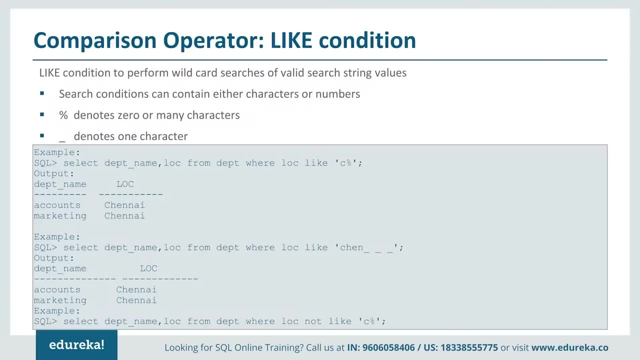 to use the keyword before the wildcard and it will show us the result. So, along with percentage signs, we use underscores also as a wildcard. So in this example, as you can see, the second example, select department or location from Department where locations like, so it means the first three words should be CHEN. 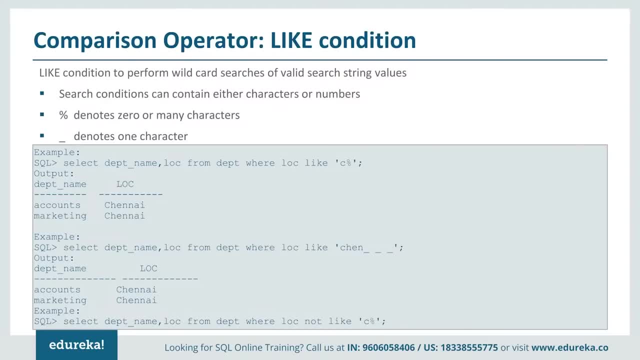 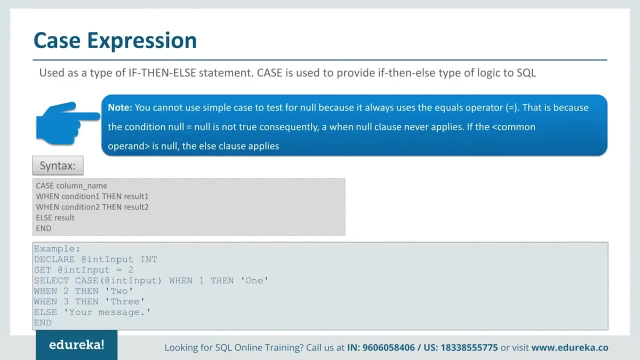 then we can use underscore. So we have to first satisfy the first keyword. So the first three should be this. So this is how we use the underscore wildcard. The last topic of this module is the case expression. So case expressions helps us to kind of. 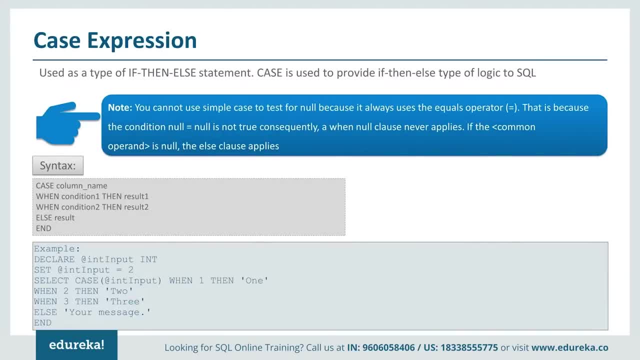 you know, simulate the if, then else statement, like in most of the programming language, we use if else. So this helps us to write the same. only point with a key statement, is that, as you can see in the note, we cannot use null values in the case statement. 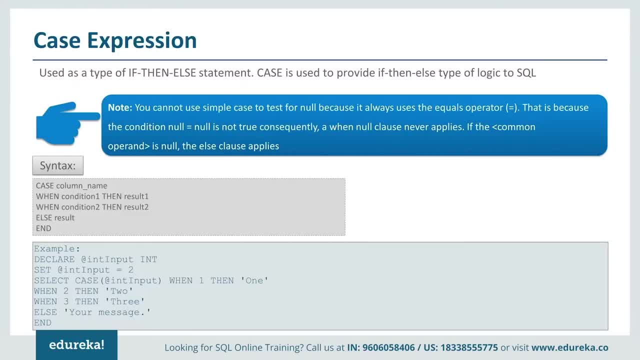 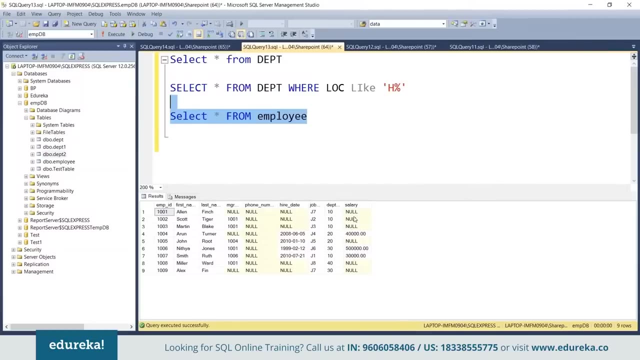 because it always use the equals to operator and we cannot use equals to operator with the null keyword We have to use is null. that I will show you after this example. So let's assume I'm fetching values from employee. So if I'm looking for the salary column, 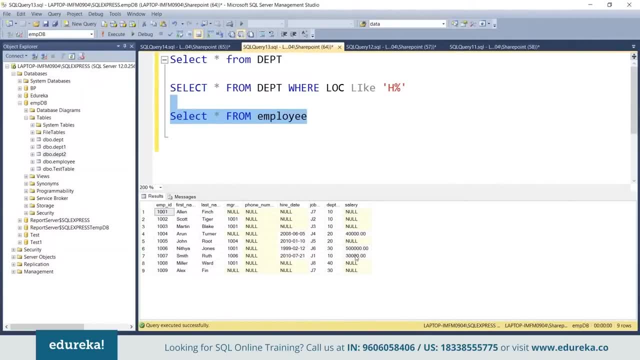 there are a few rows which are having null values and there are a few rows which having values in it. So if I want to see that, what are the different employees which have a null values for the salary column? So if I try to write where salary equals to null, 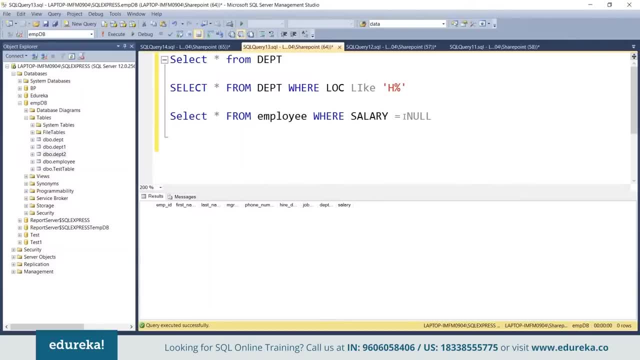 then I won't get any result here, because equals to operator does not work with null. So if I'm checking now, we have to use is null. If I'll execute this query again, I'll get the desired result. If I want to check, if I want to fetch the columns. 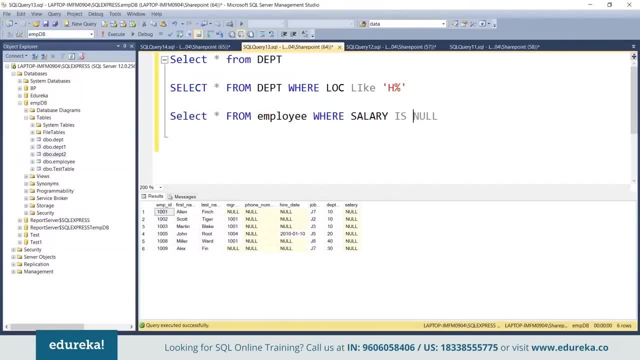 which do not have null values for the salary column, then we have to use is and then we have to use the not logical operator is not null, So not logical operators is always used in combinations with other operators, We get all. the employees Do not have null values for the salary column. 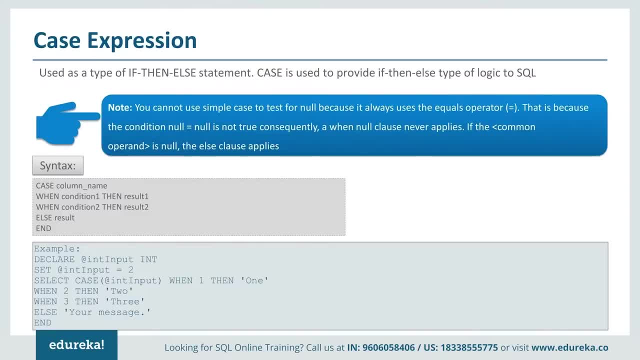 So that is the reason we are using case expression, So we cannot use the null values, Otherwise it will break, because we use the equal operators and equal operators not used along with null. So this is how the syntax of case expressions. as you can see, we have declared a variable. 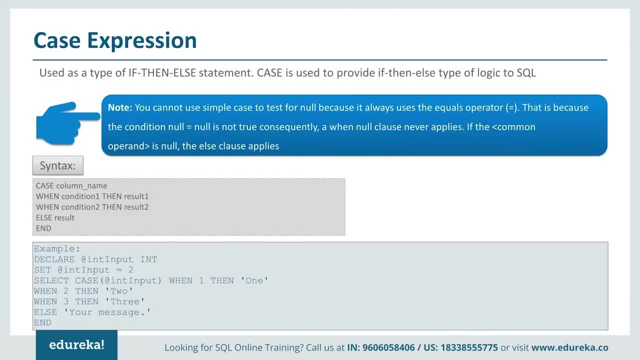 int, input and type of int- and we have set the values- is equals to two. It's just an example. So we have hard coded the value here in this example. So we are selecting case. I'm just selecting that if the value is one, 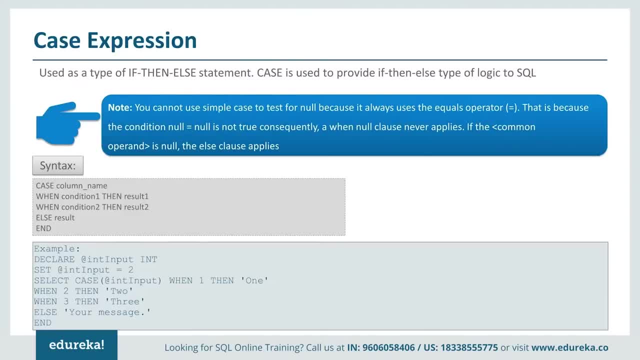 then we'll show the output as one. when it is two, then we'll showing the output as two. when it is three, then we are showing output as a three, and if it is not out of any these three values- one, two and three- then we'll show the messages. your message. 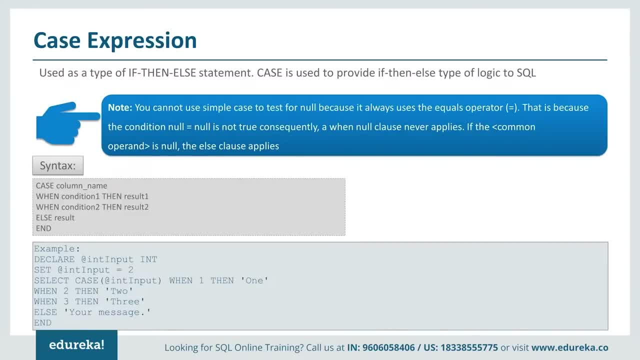 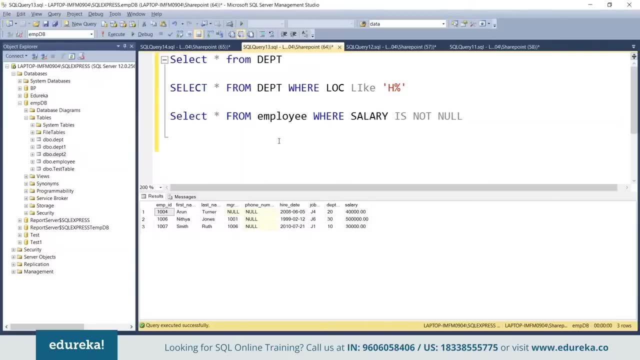 This is how we are doing in this example. So let me give you one example for that. Let me do one thing. Let me find out the states of the cities where my department is, So, as we know that Chennai is in Tamil Nadu and Bangalore is in Karnataka, 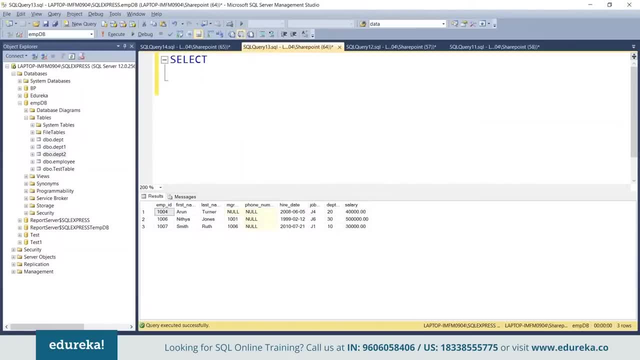 So let's see how we can do that using a key statement. So we have to write select, then case keyword. in the case keyword will define which columns you want to fetch. So I'm fetching the location and then we'll write the van condition. 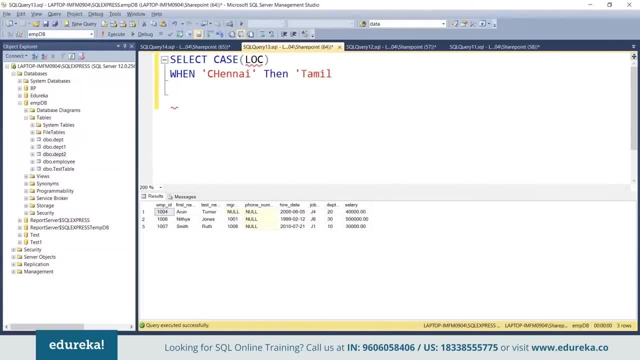 So I'm writing van Chennai, then show the result as Tamil Nadu, van Bangalore, Then let's say Karnataka and I'm writing an else condition if it is not part of anything, So let's just write no idea. So we have to end the van condition. 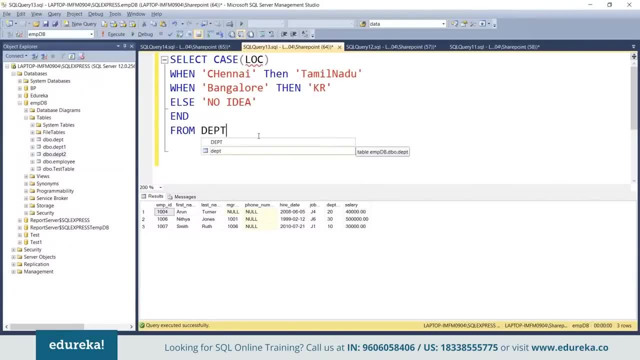 then we have to write from which tables we are basically fetching this record. So if I'll execute this query, I'll get see. if it is Chennai, I'm getting the result as Tamil Nadu, and if it is Bangalore, then I'm getting as KR. 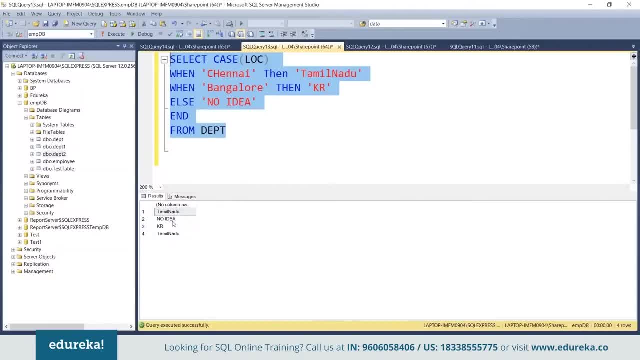 and since there's some departments which do not have any values, like Hyderabad, So we are getting. is this no idea? So this is how we can use, if else, conditions and SQL statement or select statement by using case expression. important point is that we should not deal with where we using null. 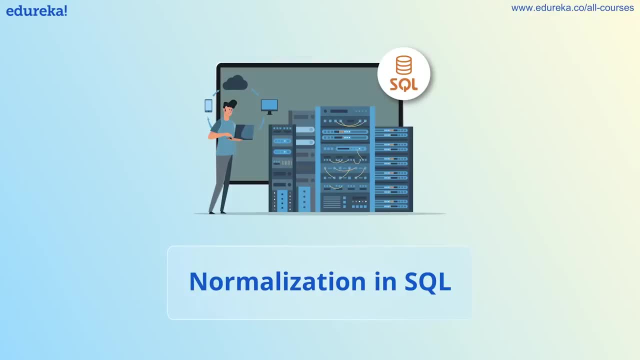 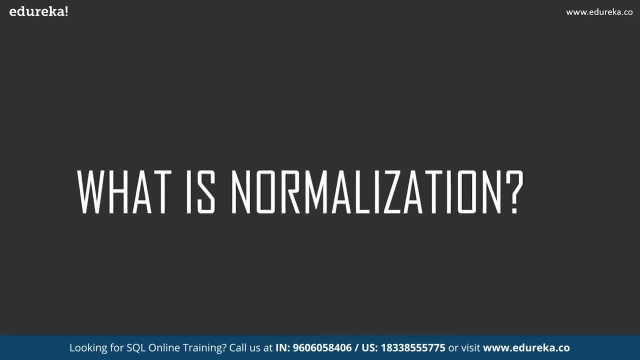 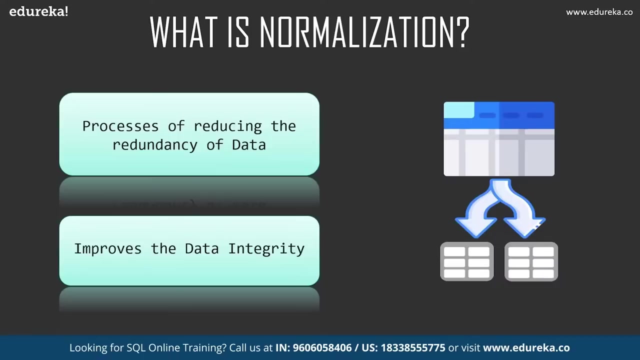 because we use equals to operator. What is normalization? database normalization is a technique of organizing the data in the database. It is a systematic approach of decomposing tables to eliminate data redundancy. It is a multi-step process that puts data into tabular form, removing the duplicated data. 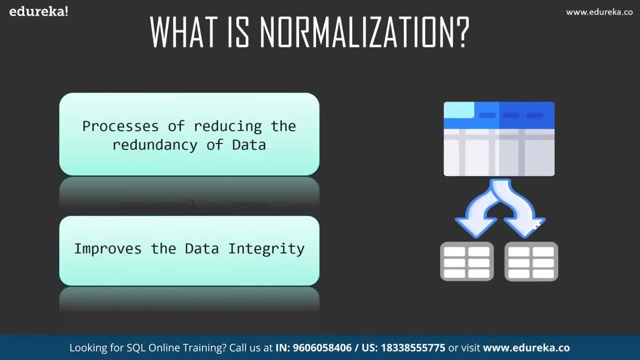 from its relational tables. on the screen We just saw that the table is getting decomposed into two smaller table. Is it really necessary to normalize the table that is present on the database? Well, every table in the database has to be in the normal form. 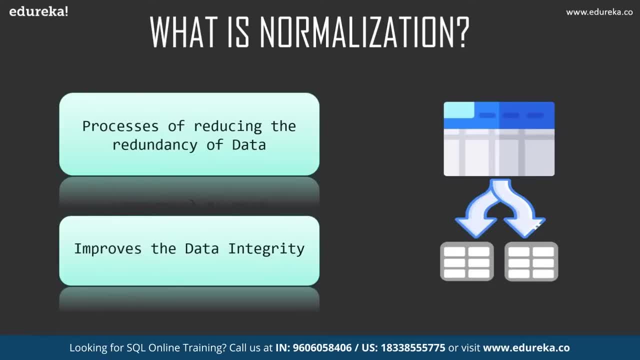 So normalization is used mainly for two purpose. So the first one is it is used to eliminate repeated data- having repeated data in the system not only makes the process slow but will cause trouble during the later part of transactions- and second one is to ensure the data dependencies make some logical sense. 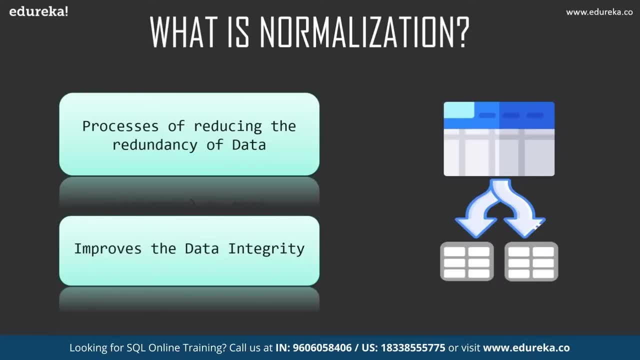 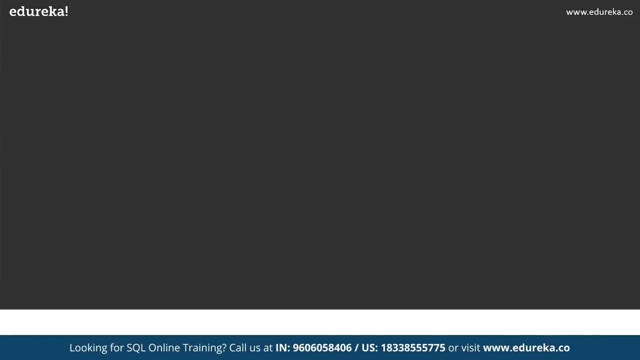 Yes, Usually the data is stored in database with certain logic. huge data sets without any purpose are completely waste. It's like having an abundant resource without any application. the data that we have should make some logical sense. Normalization came into existence because of the problems that occurred on data. 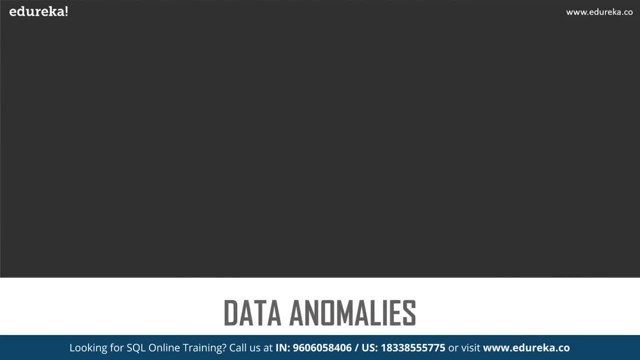 Now let's look at those problems, and these are known as data anomalies. If a table is not properly normalized and has data redundancy, then it will not only eat up the extra memory space, but will also make it difficult to handle and update the database. 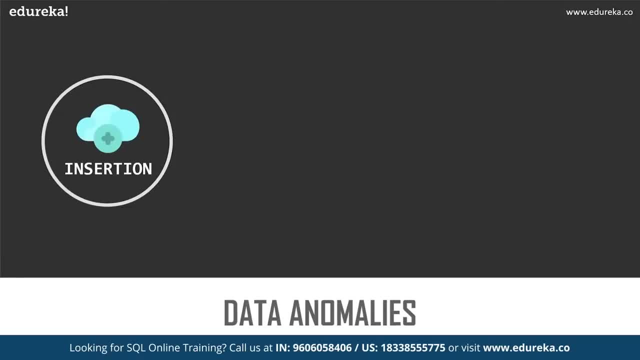 Let's look at the first anomaly, that is, insertion anomaly. Suppose: for a new position in a company. Mr Raksha is selected, but the department has not been allotted for him. in that case, If we want to update his information to the database, 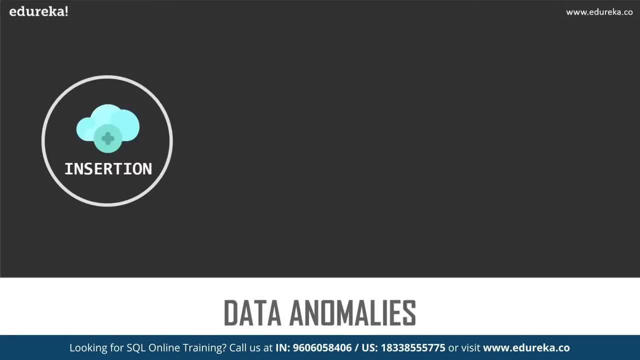 we need to set the department information as null. Similarly, if we have to insert data of thousand employees who are in similar situation, then the department information will be repeated for all those thousand employees. This scenario is a classical example of insertion anomalies. The next one is update anomaly. 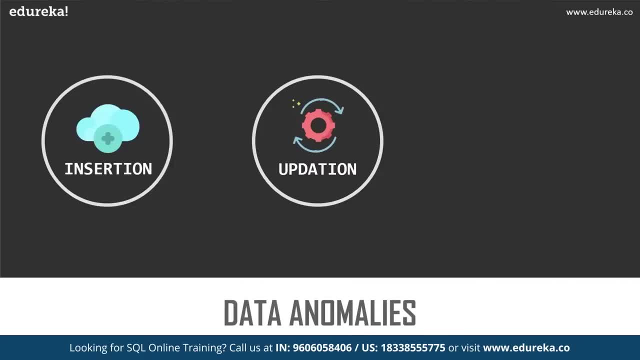 What if Mr Raksha leaves the company or is in no longer the head of the marketing department? In that case, all the employee records will have to be updated And if, by mistake, we miss any record, it will lead to data inconsistency. 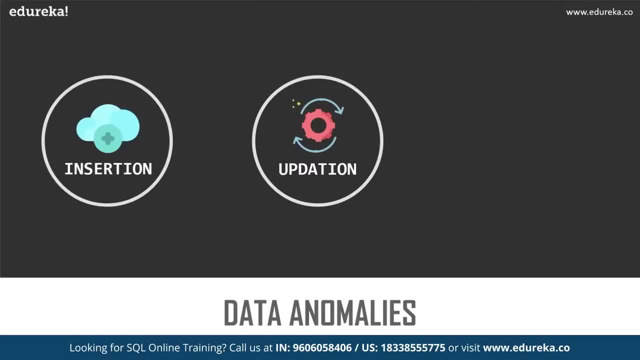 This is nothing but updation anomaly. And the final one is deletion anomaly. in our employee table two different pieces of information are kept together, that is, employee information and department information. Hence, at the end of financial year, if employee records are deleted, we will also lose the department information. 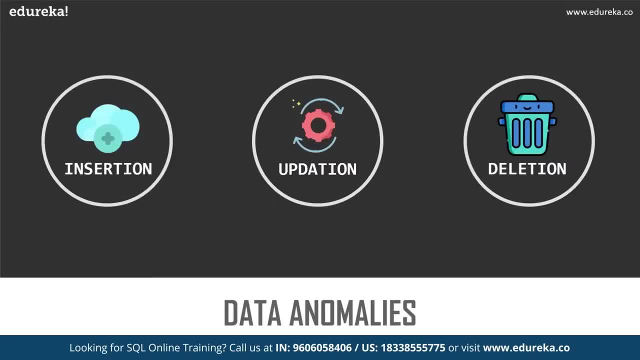 So we will have to update all the employee records and the data inconsistency. We will also lose the department information. This is nothing but deletion anomaly. So these were some of the problems that occurred while managing the data. to eliminate all these anomalies, normalization came into existence. 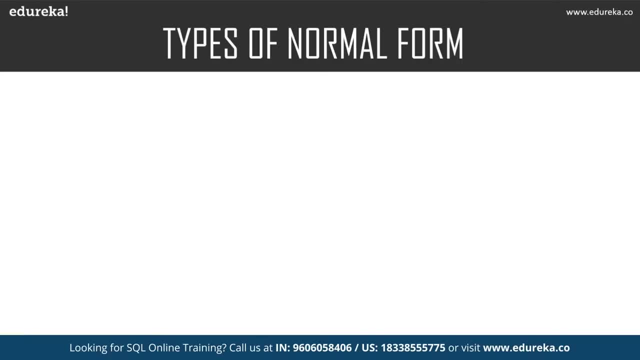 There are many normal forms which are still under development, but let's focus on the very basic and the essential ones only. So we will be talking about first normal form, second normal form, third normal form and finally end this session with Boy Scout normal form. 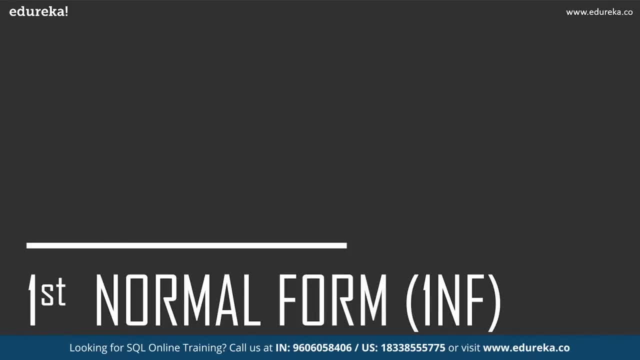 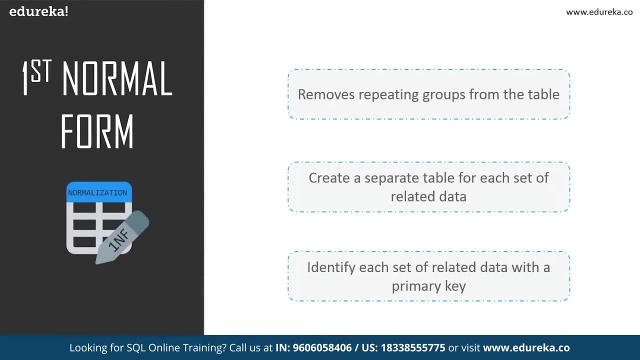 So, without wasting further time, let's proceed to first normal form. in first normal form We tackle the problem of atomicity here. atomicity means values in the table should not be further divided. in simple terms, a single cell cannot hold multiple values If a table contains a composite or multi-valued attributes. 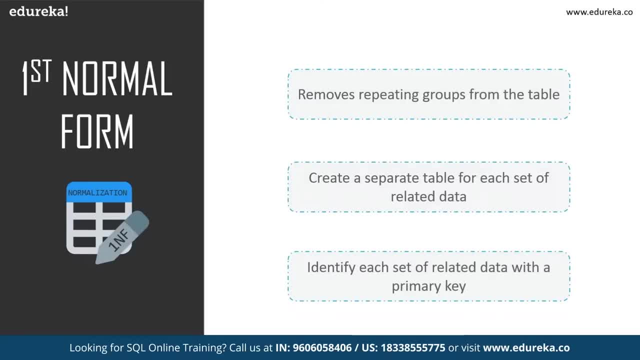 it violates the first normal form. So the following functions will be performed in first normal form. The first one is it removes repeating groups from the table and next it creates a separate table for each set of related data And finally, it identifies each set of related data. 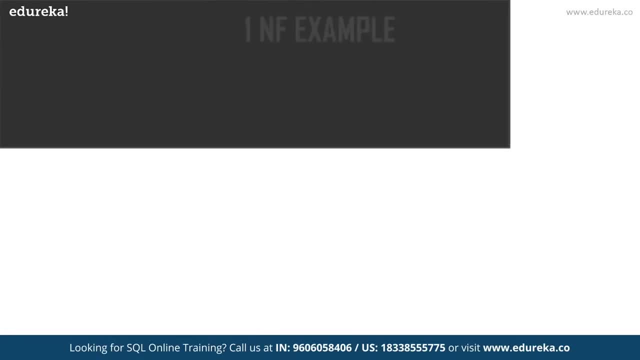 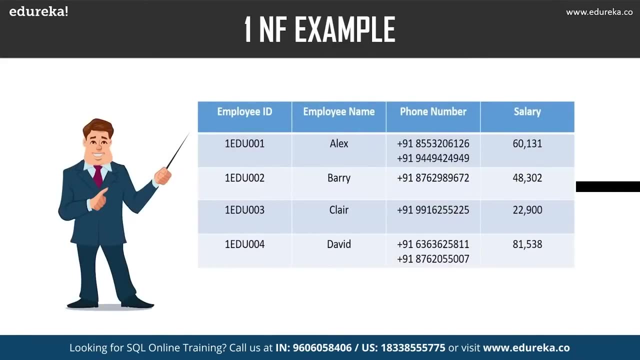 with the primary key. to understand this in a better way, Let's look at the given table. in the employee table We have employee ID, employee name, phone number and salary as columns. We can clearly see that the phone number column has two values. does it violates the first normal form now? 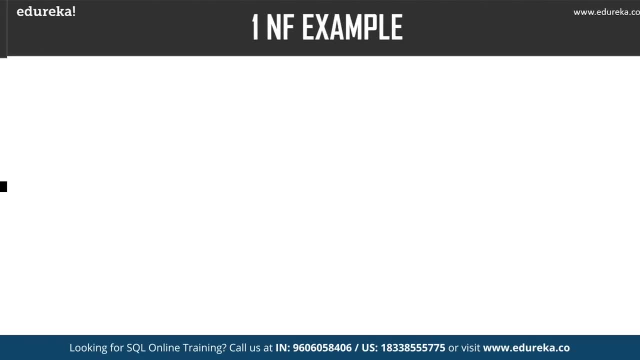 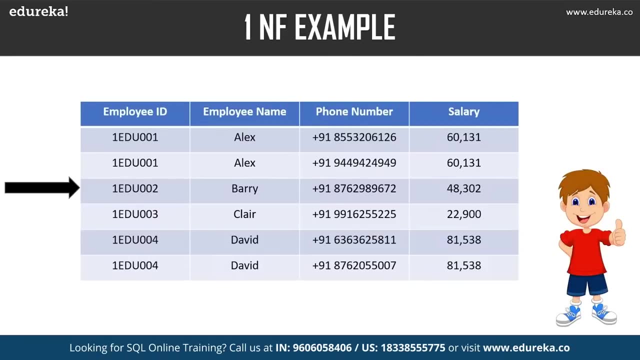 if we apply the first normal form to the above table, we get the following result: in this table, each and every row, as this thing, that is, no cell, has multiple values, The table has achieved atomicity. first normal form is simple and can be easily identified in the table. 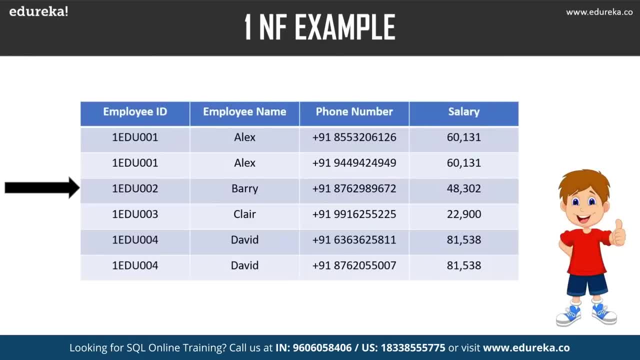 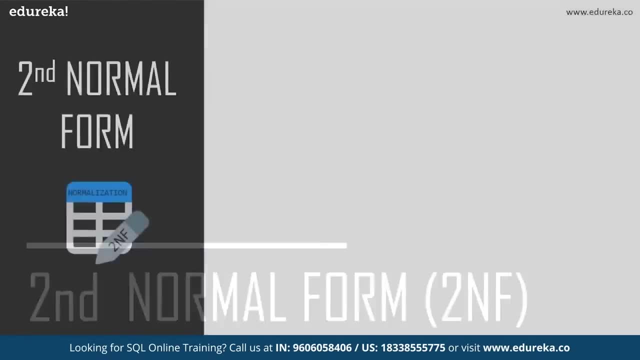 We can clearly see there is no multiple values in each and every column. Thus the first normal form is achieved. Now let's move to second normal form. second normal form was originally defined by EF chord in 1971. a table is said to be in second normal form only. 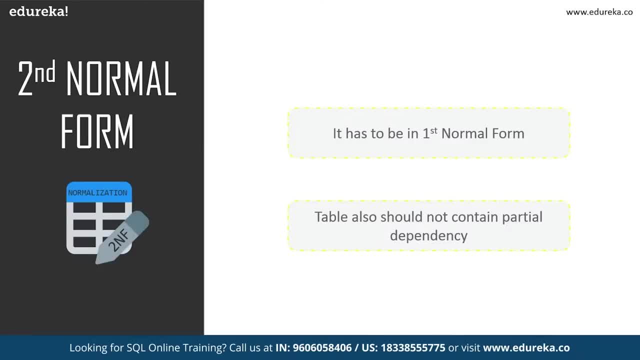 when it fulfills the following condition. The first condition is it has to be in first normal form and the second one is the table also should not contain partial dependency. here partial dependency means the proper subset of a candidate key determines a non-prime attribute. 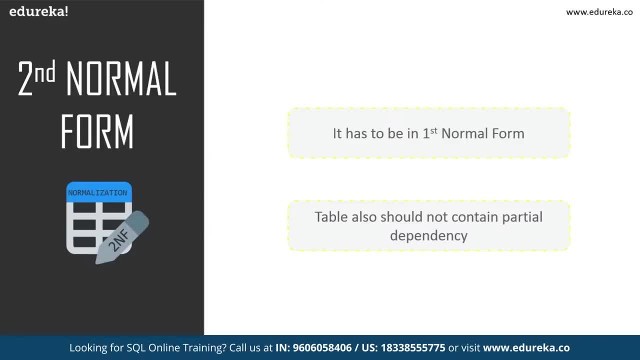 So what is a non-prime attribute? Let's understand this in a simple way: attributes that form a candidate key in a table, The table are called prime attributes and the rest of the attributes of the relation are non-prime. for a table, prime attributes can be like employee ID. 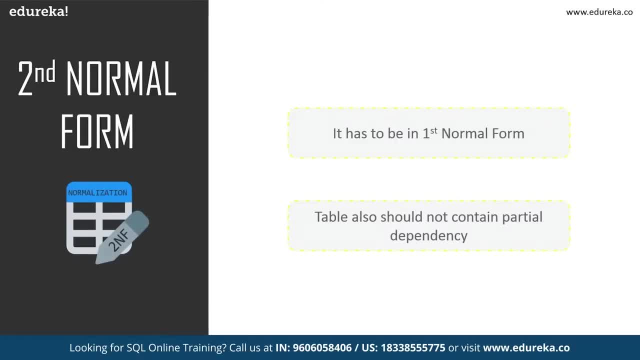 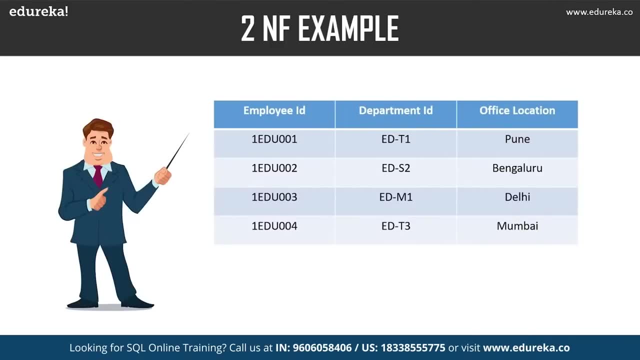 and Department ID and the non-prime attributes can be like office location. to understand second normal form, Let's consider this table. This table has a composite primary key that is employee ID and Department ID makes the primary key. the non-key attribute is office location, in this case, office location. 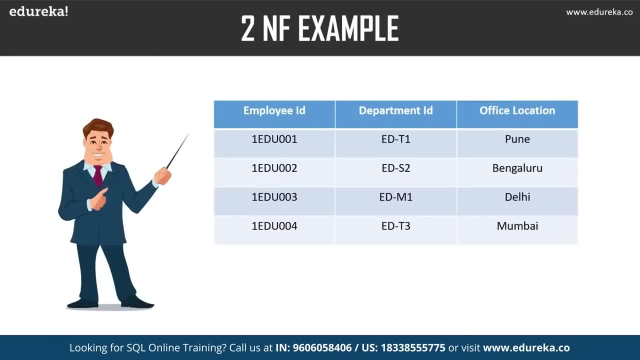 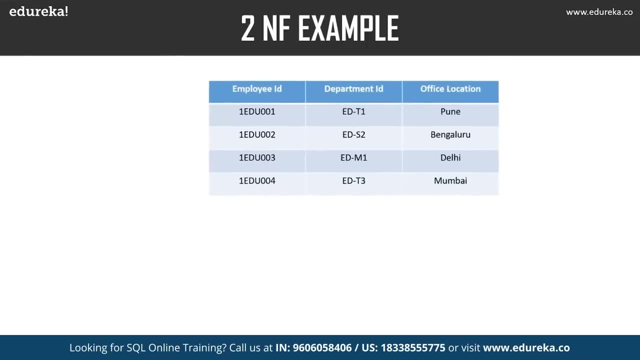 only depends on Department ID, which is only the part of primary key. Therefore, this table does not satisfy the second normal form. So what to do in such scenario? The answer is simple: split the table accordingly to bring this table to second normal form. 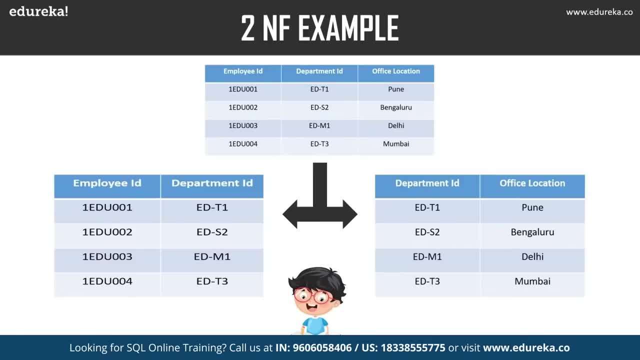 We need to break the table into two parts, which will give the following tables. The first table has employee ID and Department ID as columns. The second one has Department ID and office location as columns. As you can see, we have removed the partial functional dependency. 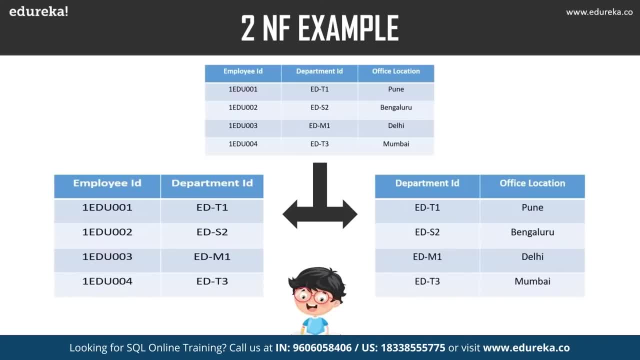 that we initially had. now in the table, The column office location is fully dependent on the primary key of that table, which is nothing but Department ID. I hope you have understood second normal form Now that we have learned first normal form and second normal form. 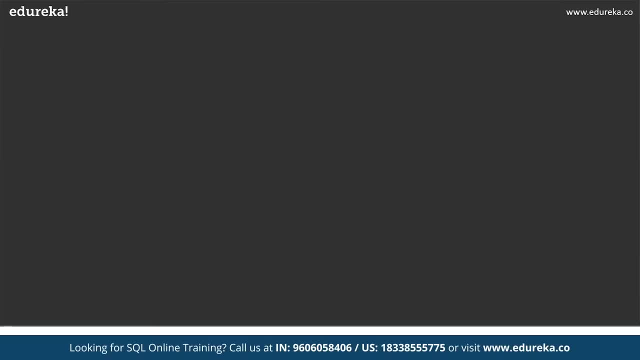 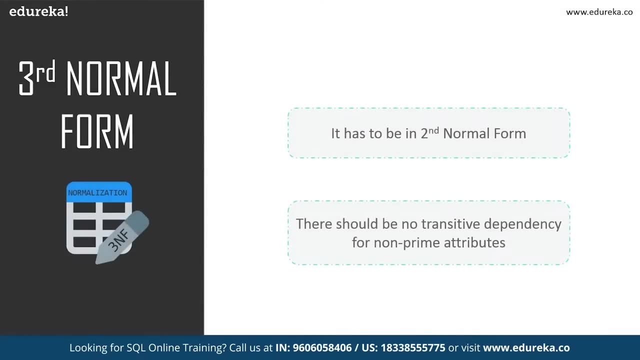 Let's head to the next part of this normalization. Next topic is third normal form. Third normal form is a normal form that is used in normalizing the table to reduce the duplication of data and ensure referential Integrity. The following condition has to be met by the table. 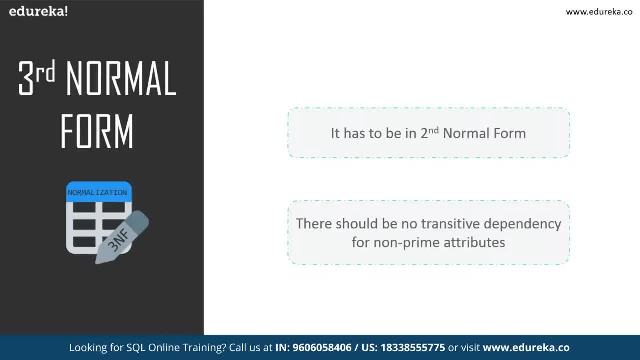 to be in third normal form, And the first condition is: the table has to be in second normal form and the second condition is: no non-prime attribute is transitively dependent on any non-prime attribute which depends on other non-prime attributes. I know it's a bit confusing. 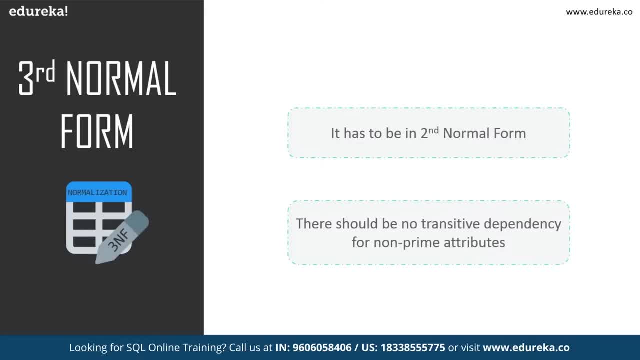 So let me make it simple for you. It's like if C is dependent on B and in turn B is dependent on a, then transitively C is dependent on a. this should not happen. in third normal form, all the non-prime attributes must depend only on the prime attributes. 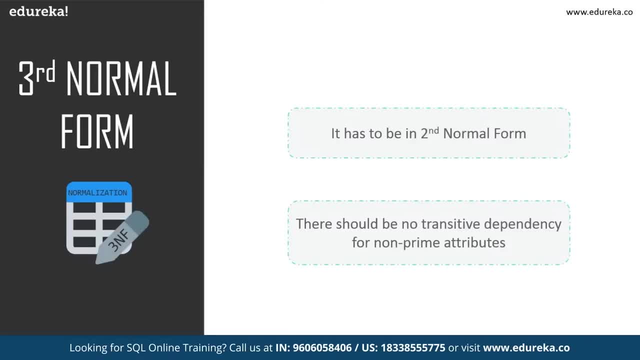 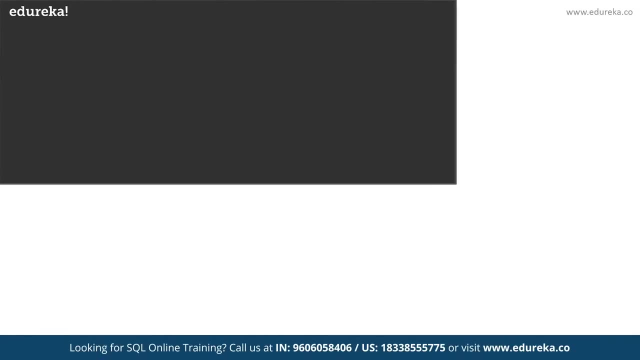 So these are the two necessary condition that needs to be attained. So why was the normal form designed? Firstly, to eliminate undesirable data anomalies. next one is to reduce the need for restructuring over time. Finally, to make the data model more informative, since we have understood the third normal form. 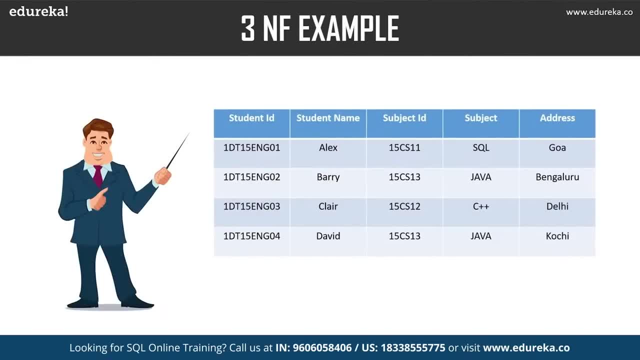 Let's look at the example table. in the above table, student ID determines subject ID and subject ID determines subject. Therefore, student ID determines subject via subject ID. This implies that we have transitive functional dependency and this table does not satisfy the third normal form. 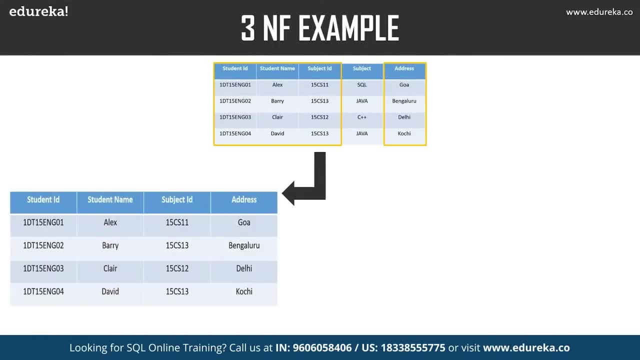 Now, in order to achieve third, normal form, We need to divide the table as shown below. Firstly, let's divide the table, And so student ID, student name, subject, ID and address. in it, All the columns are referring to the primary key, which is student ID. 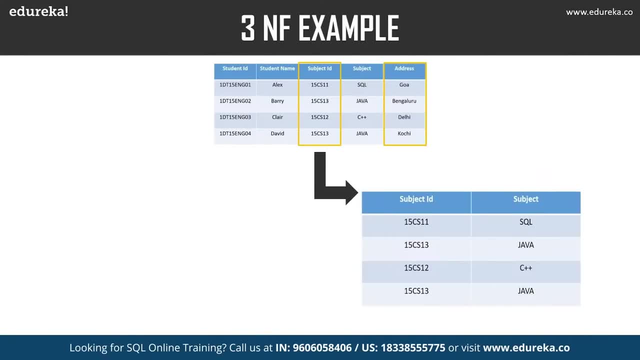 Let the second table have subject ID and subject column. So subject is dependent only on subject ID and not on student ID. as you can see from the above table, All the non-key attributes are now fully functionally dependent only on the primary key in the first table columns. 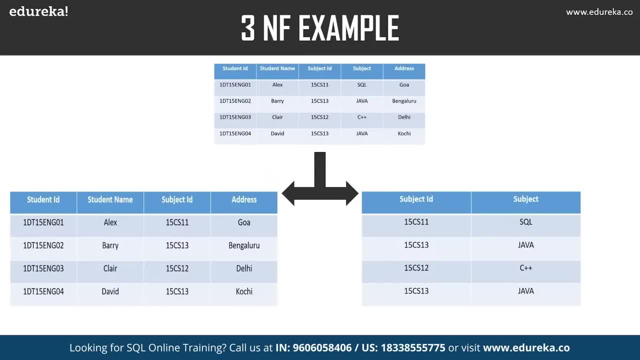 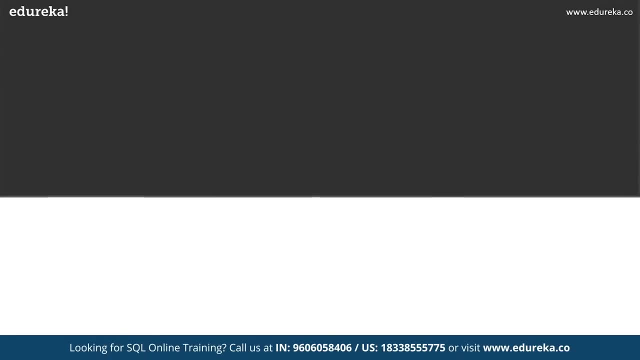 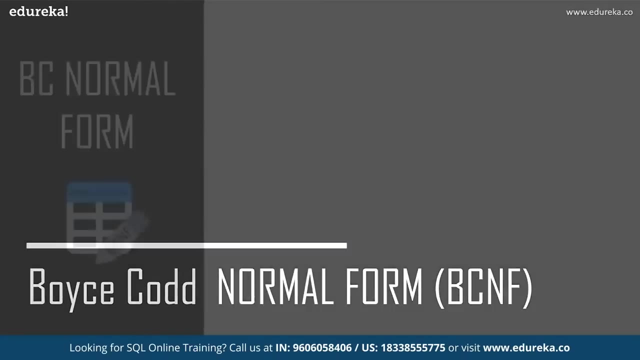 such as student name, subject ID and address are only dependent on student ID. in the second table, subject is only dependent on subject ID. with this being understood, Now we can proceed further to next normal form, That is, Boyce-Cord normal form. This is also known as 3.5 normal form. 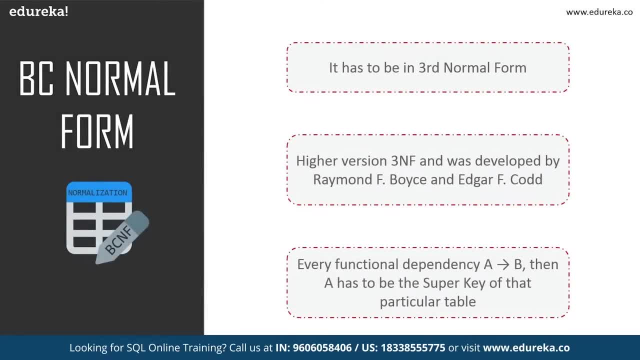 It is the higher version of third normal form and was developed by Raymond F Boyce and Edgar F chord to address certain types of anomalies which were not dealt with. third normal form. before proceeding to Boyce-Cord normal form, The table has to satisfy third normal form. 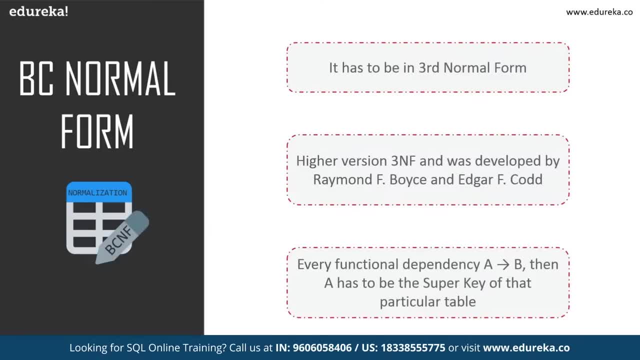 in Boyce-Cord normal form. If every functional dependency that is a implies B, then a has to be the super key of that particular table. So what is a super key? A super key is a group of single or multiple keys which identifies rows in a table. 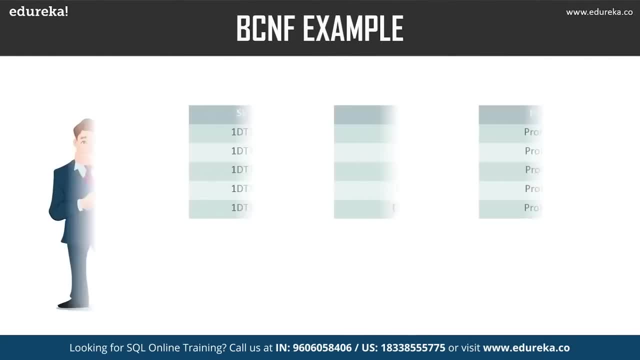 Let's look at the table to clearly understand Boyce-Cord normal form. in the given table, One student can enroll for multiple subjects. There can be multiple professor teaching one subject and for each subject a professor is assigned to the student. These are the necessary condition of the stable 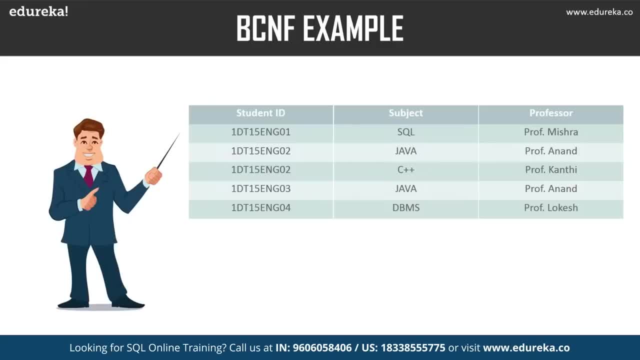 in this table All the normal forms are satisfied, except Boyce-Cord normal form. Why? as you can see that student ID and subject form the primary key, which means that the subject column is prime attribute. but there is one more dependency, that is, professor is depending. 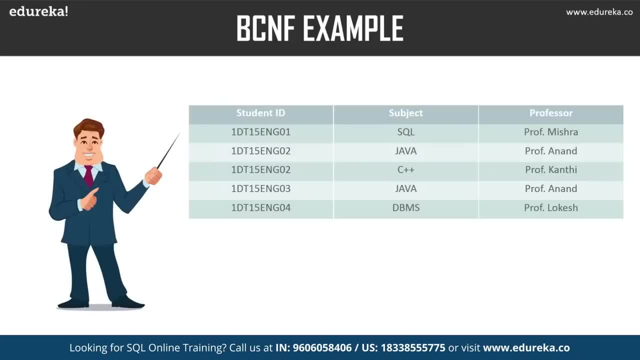 on subject. and while subject is a prime attribute, Professor is a non-prime attribute which is not allowed by Boyce-Cord normal form. Now, in order to satisfy the Boyce-Cord normal form, we will be dividing the table into two parts. 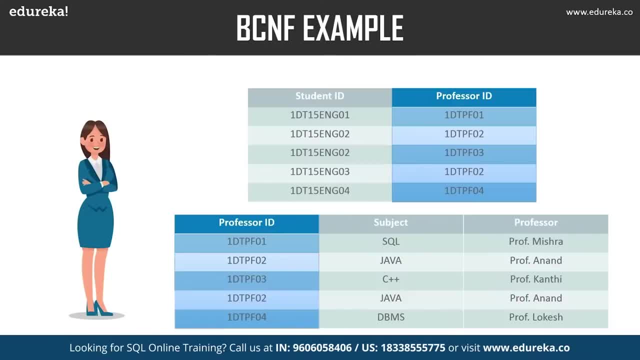 The table at the top will hold student ID, which already exists, and we will create a new column that is professor ID, and in the second table, which is below, will have the columns professor ID, professor and subject columns. Why do we need to have a new column? that is professor ID. 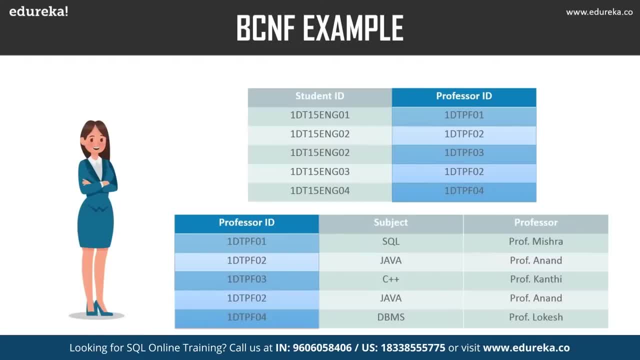 by doing this We are removing the non-prime attributes functional dependency in the second table. professor ID will be the super key of that table and remaining column will be functionally dependent on it. by doing this We are satisfying Boyce-Cord normal form. 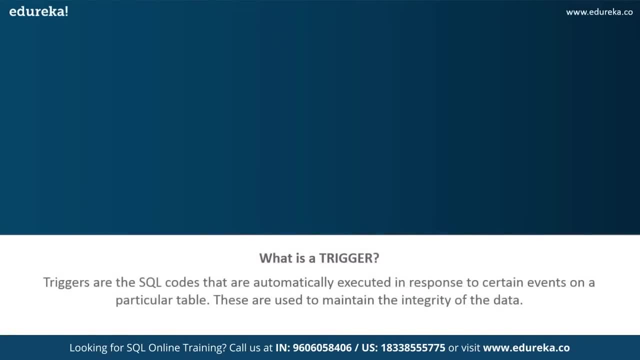 What are triggers? triggers are the SQL code that are automatically executed in response to certain events on a particular table. These are used to maintain the integrity of the data in a given table. a trigger in SQL works similar to real-world trigger. I know this is a formal definition. 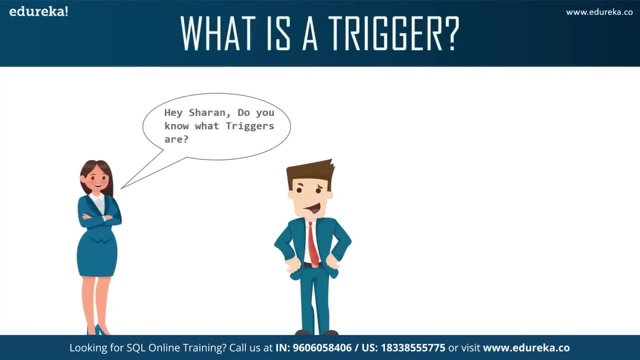 but let's try to understand it in a better way. here We can see Anna is asking Sharon about triggers. Sharon imagines trigger to a falling Domino's. How does a falling Domino's is related to a trigger? Let's move further and see the explanation given by Sharon. 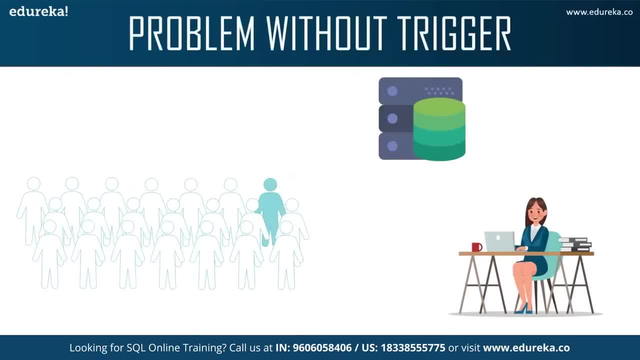 Anna is a marketing officer in a company. When a new customer data is entered into the company's database, She has to send the welcome email to each and every new customer. if it is one or two customer and I can do it manually, But what if the count is more than a thousand? 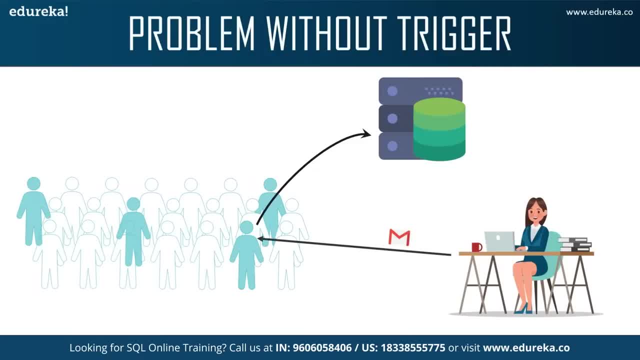 It will be a repetitive and tiring job. efficiency of Anna may drop well. in such scenario, triggers come in handy. Anna can easily create a trigger which will automatically send a welcome email to new customer Once the data is entered. enter into the database after creating a trigger. 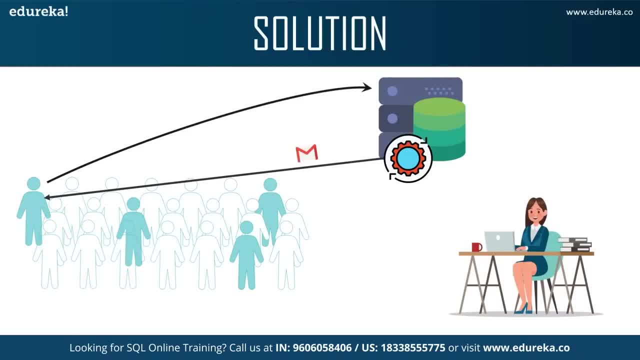 in the database of the company. She doesn't have to monitor the trigger frequently. the efficiency of the work is increased. with this analogy given by Sharon, I hope you're clear. with the introduction of trigger, Let's head to the next topic, that is, syntax. 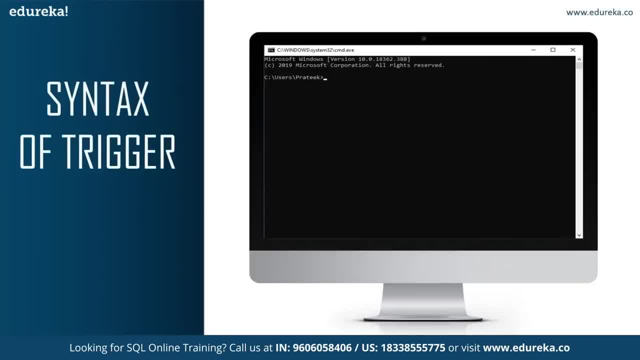 and example of a trigger. on the screen We can see the syntax of a trigger and let me explain each and every part in detail. The first part is create- trigger. these two keywords are used to specify that a trigger block is going to be declared. 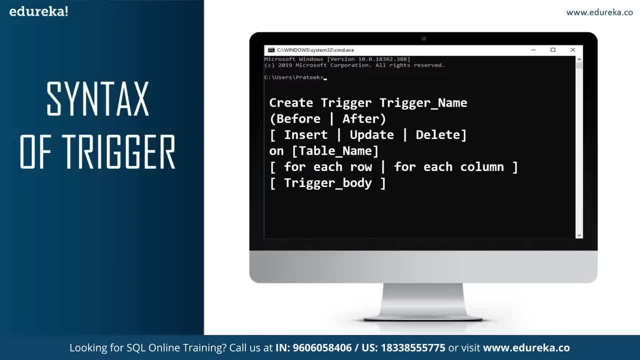 The next one is trigger name. It specifies the name of the trigger. trigger name has to be unique and shouldn't repeat. the next one is before or after. this specifies when the trigger will be executed. It tells us the time at which the trigger is initiated. 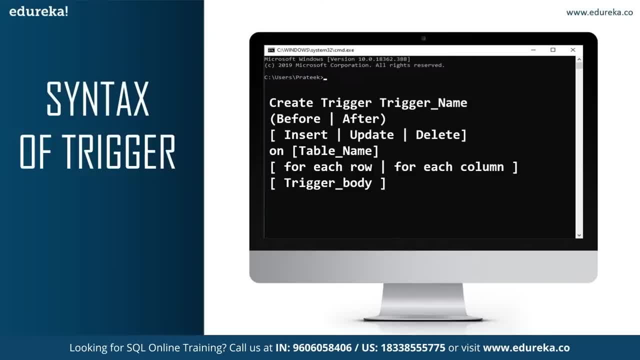 that is, either before ongoing event or after the ongoing event. before triggers are used to update or validate record values before they are saved to the database, while after triggers are used to access fields, values that are sent by the system and to affect changes in other records- the records. 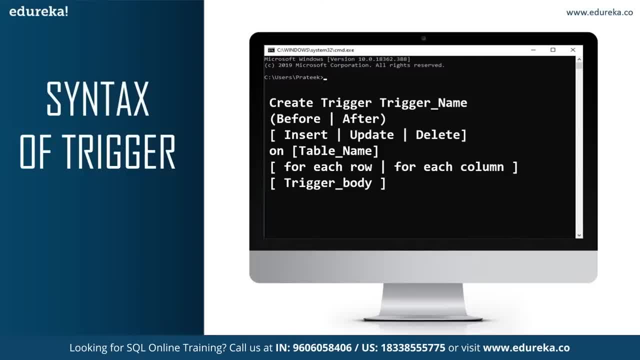 that activate the after trigger are read-only. We cannot use after trigger if we want to update a record, because it will lead to a read-only error. the next part of the syntax is insert, update or delete. These are the DML operations and we can use either of them in a given trigger. next is 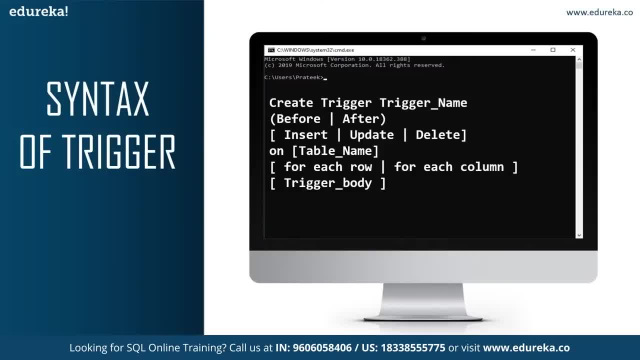 on table name. We need to mention the table name on with the trigger is being applied. Don't forget to use on keyword and also make sure the selected table is present in the database. The next part is for each row or for each column row level. 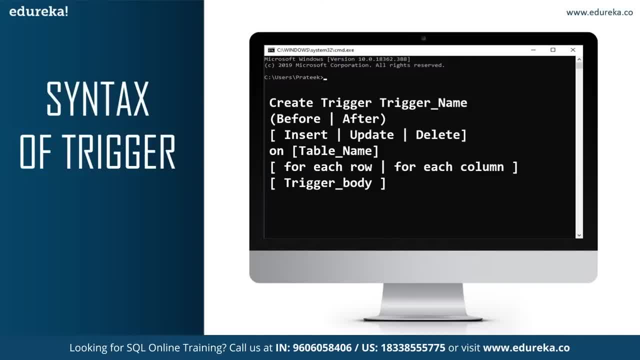 triggers get executed before or after any column value of a row changes, while column level triggers get executed before or after the specified column changes. the final part of the syntax is trigger body. It consists of queries that needs to be executed when the trigger is called. 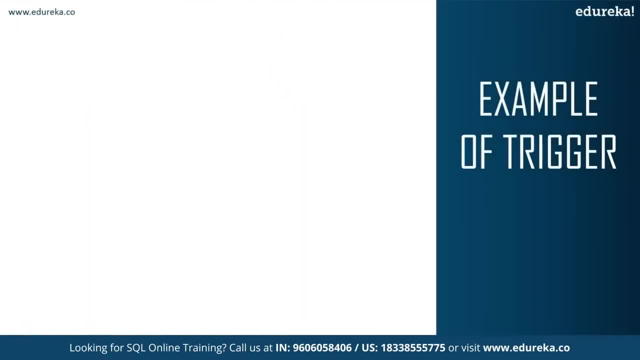 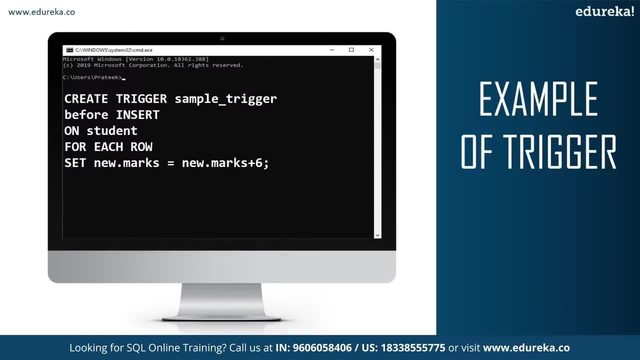 So this was a brief introduction to syntax of a trigger. on the screen We can see an example for a trigger. in the given trigger We are trying to calculate the marks of a student as soon as his details are updated to the database. here We are adding hundred marks to the marks column. 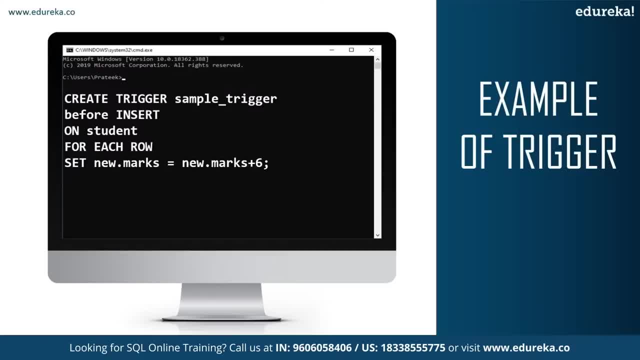 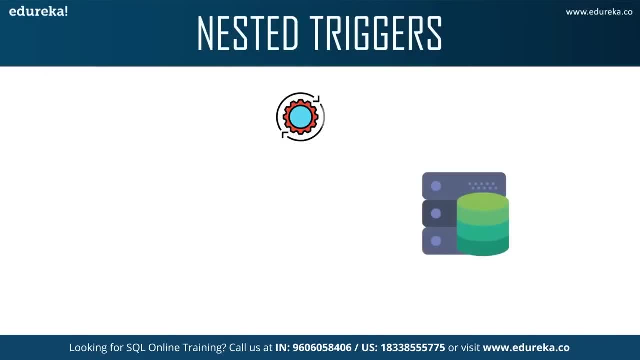 of each new record. also make a note: new keyword refers to the row that is getting affected. So this was all about a simple trigger, but we can also create a nested trigger that can do multiple process also. handling it and terminating it at the right time is very important. 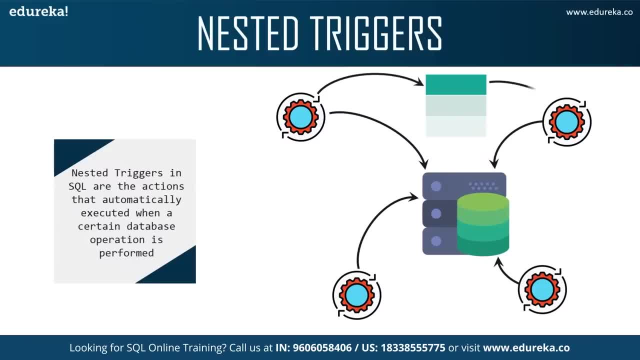 If we don't end the trigger properly, it may lead to an infinite loop. You might be wondering in which scenario we can use the nested trigger. rather than giving you a tailored answer, Let me share a scenario with you which will help you in understanding the nested trigger in a better way. continuing. 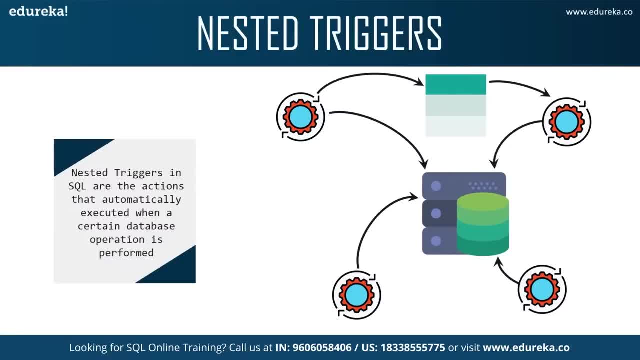 from the earlier scenario and I sent an email for every new customer that was added to the company's database. Now what if she wishes to keep a track of numbers of customers to whom the email was sent? now, Anna needs to create a nested trigger to keep the track. 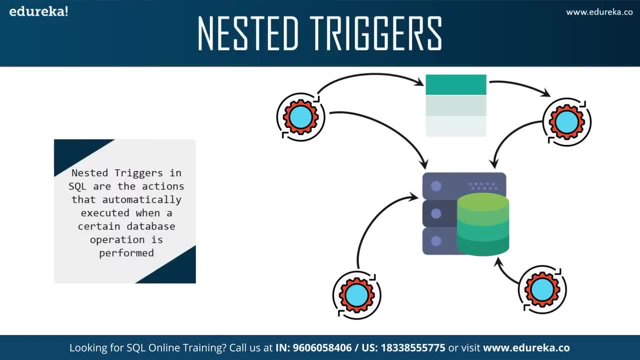 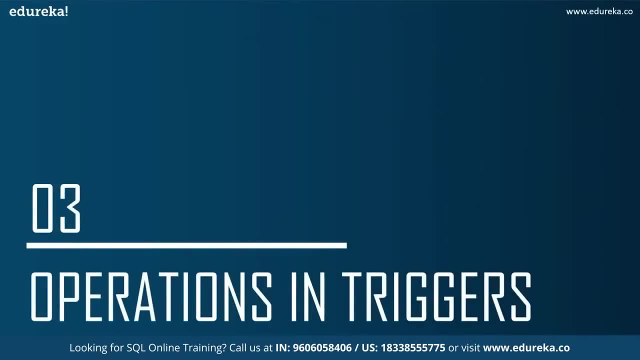 of the count along with sending an email, doesn't it sound simple? So that was all about the syntax of trigger. Let's now try to implement an example of trigger in SQL. So the next topic is operations in trigger. we can perform many operations. 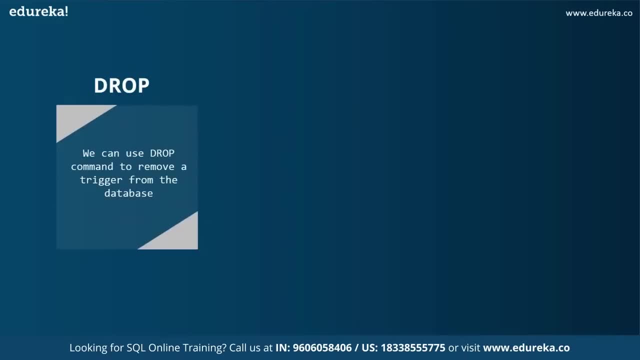 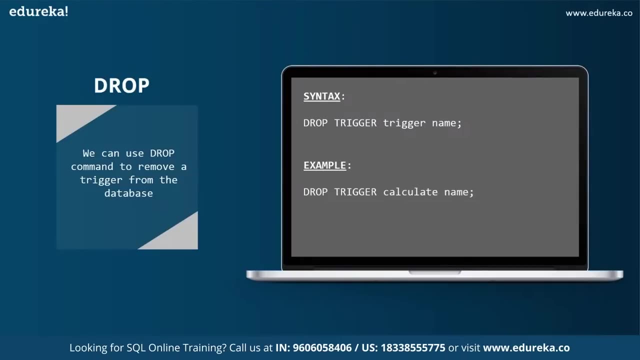 Using triggers. some may be simple and some may be little complex, but once if we go through the query, it's easy to understand. the first operation is drop. We can use drop command to remove a trigger from the database and the syntax for this is drop trigger trigger name. 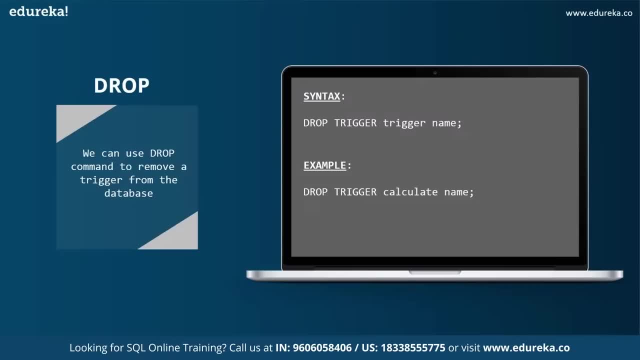 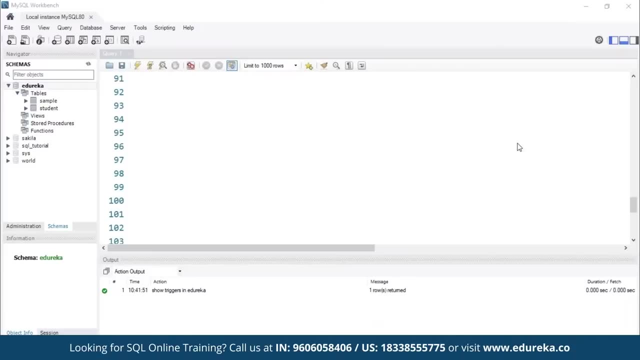 to understand this in a better way, Let's head to my sequel workbench. I hope you know how to use my sequel workbench. If not, then check SQL basics for beginner video by a Eureka for better understanding of how my sequel workbench will work. to drop a trigger: 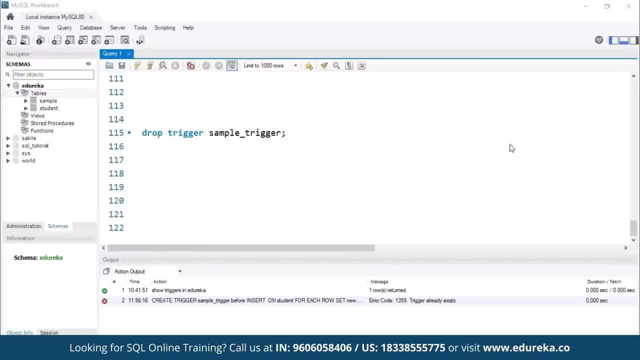 from the database. The trigger has to be present in our database, So this is the syntax used to drop a trigger. So let me execute this query So we can see in the status bar the trigger with the name sample trigger has been dropped. 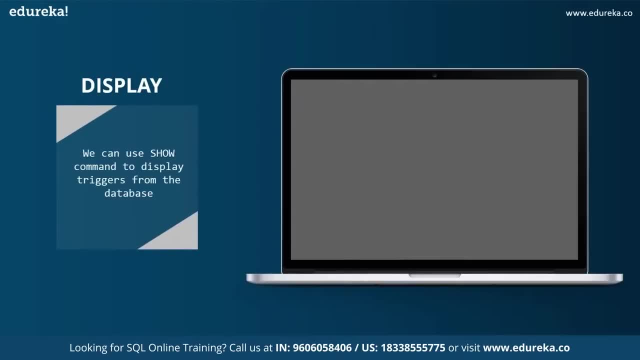 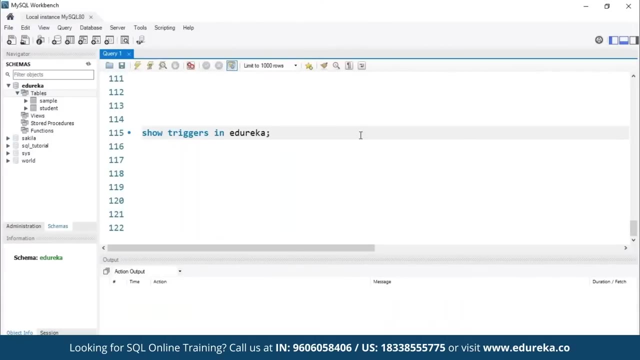 Let's head to the next operation, that is, display. We can use show command to display the triggers from the database, and the syntax for this is show triggers in database name. So let me head back to my sequel workbench to execute this command to display a trigger. 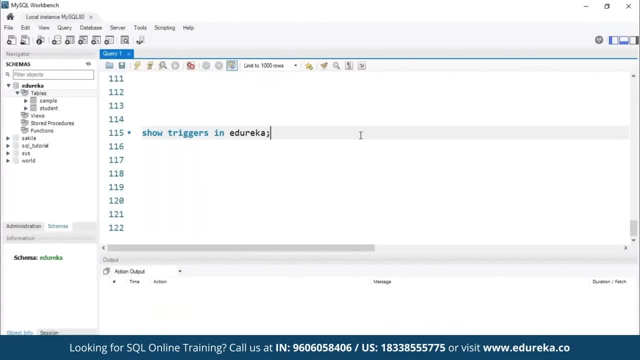 The trigger has to be present in the database, So let me execute this SQL query to display the triggers that are present in my database. I can see that the trigger with the name sample trigger is present in my database at Eureka, So let's head to the next operation. 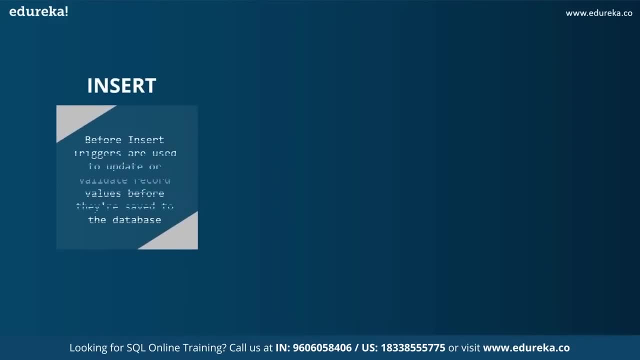 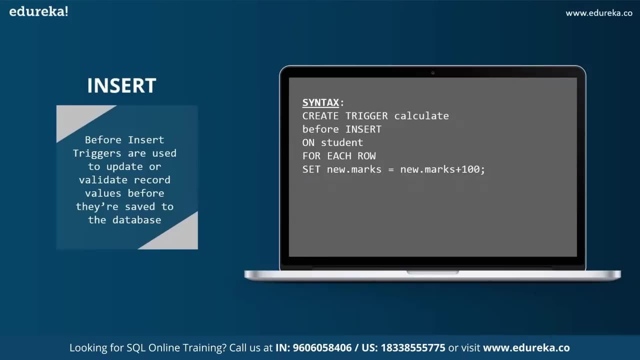 The next operation is insert and the first variant is before insert triggers. before insert: triggers are used to update or validate record values before they are saved to database, and the syntax for this is create trigger. calculate. here Calculate is the name of the trigger. before insert on the table name for each row and set operation. 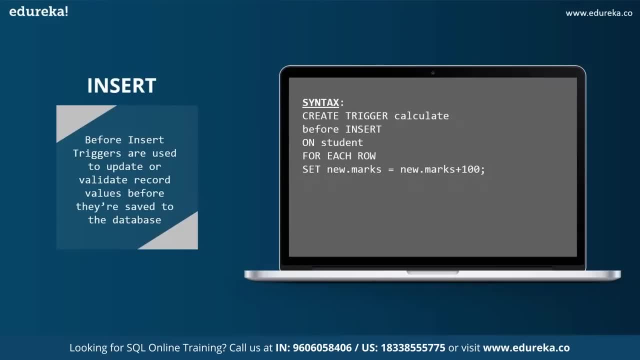 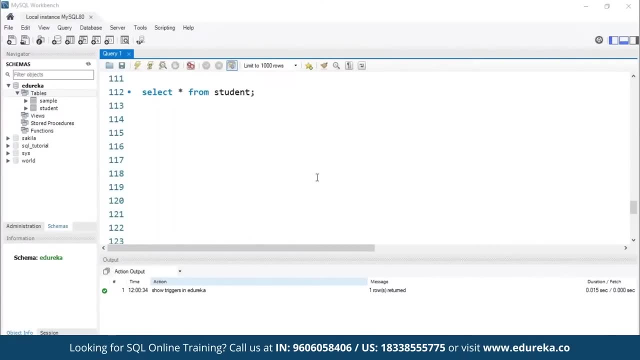 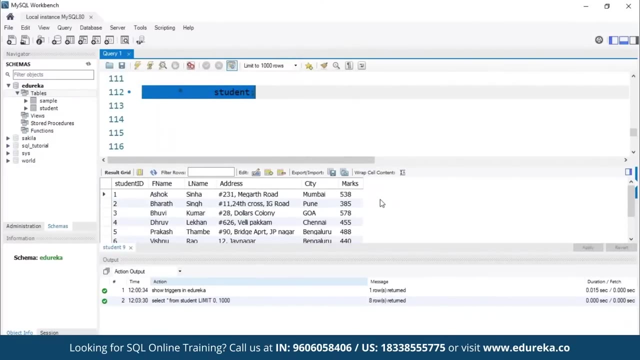 So let me head back to my sequel workbench to execute this query. before explaining, before insert Trigger, Let me explain something else. I will be using student table, and the columns of this table are: it has student ID, first name, last name, address, City and marks. 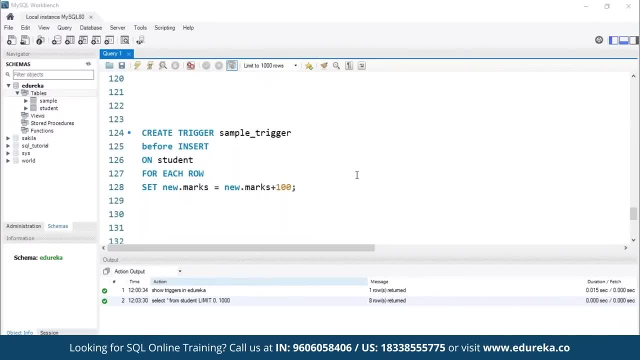 I will be creating a trigger with the name sample trigger here before insert trigger is used to set hundred marks extra for each and every student marks column when the new student value is added to the table. So let me execute this trigger And we can see that the trigger has been created. 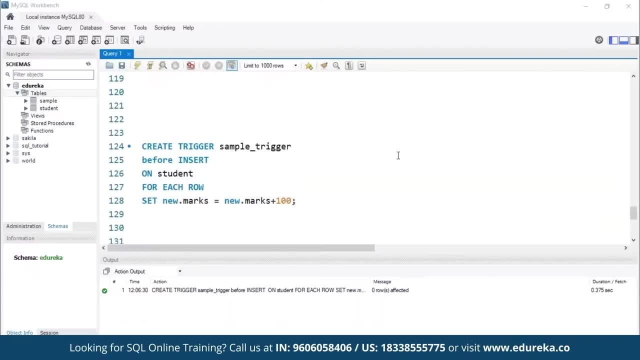 Now let me insert a record into the table. I'll be using insert into command to insert a record into the table, So let me execute this query, But before that, make sure to remember I will be adding details of Wamshe K. his marks will be 478.. 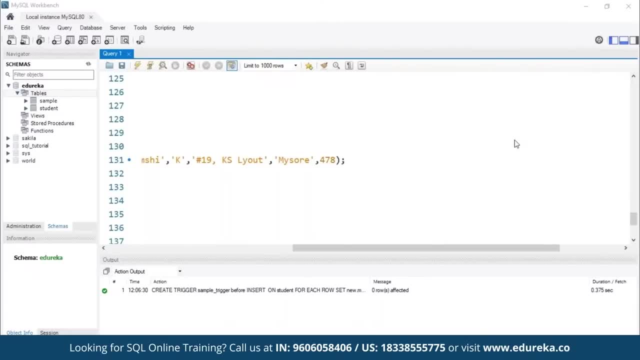 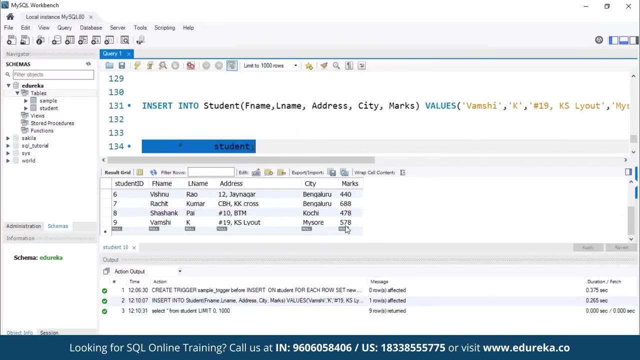 But as we have created a trigger, it has to add hundred marks extra and the resulting marks has to be 578.. So let me execute this query. Okay, the query has been inserted, So let me check the table, And we can see that the marks of Wamshe K is 578.. 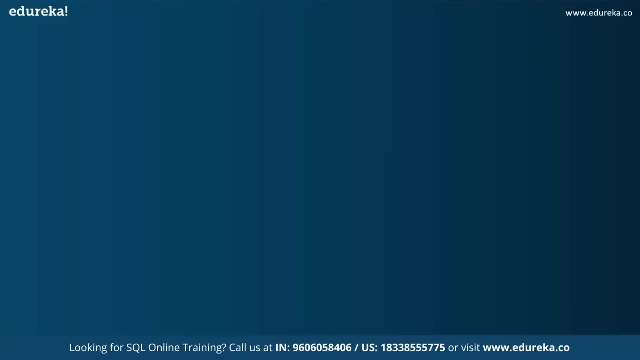 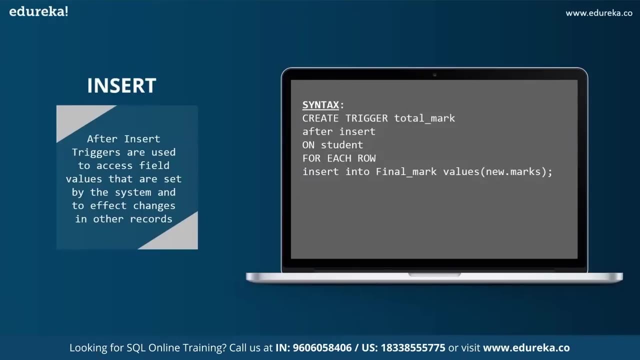 So we can clearly say that the trigger has worked. So the next variant of insert is after insert triggers. after insert, triggers are used to access fields, values that are set by the system and to affect changes in other records, and the syntax is: create trigger. name of the trigger. 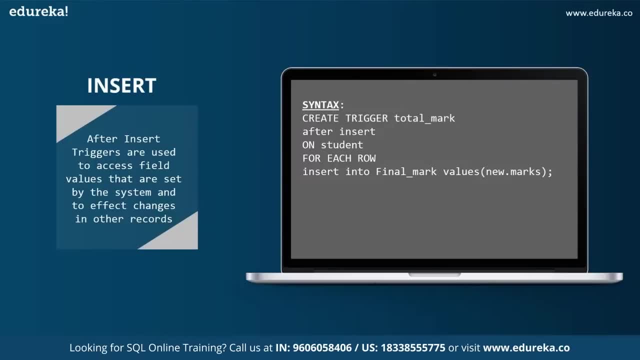 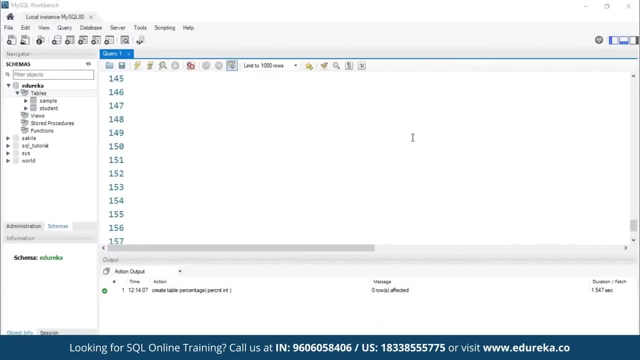 that is total mark after insert on student. student is a table name for each row. insert into final marks value of the column. So let's head back to my sequel workbench to execute this example. to use this variant, We need one more table. that is final marks table. 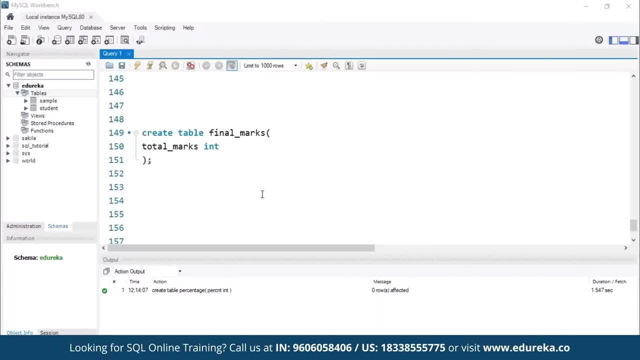 where the trigger will store. Let's see all the results. This SQL query will create a table with the name final marks. So let me execute this query So we can see in the status bar the table with the name final marks has been created. 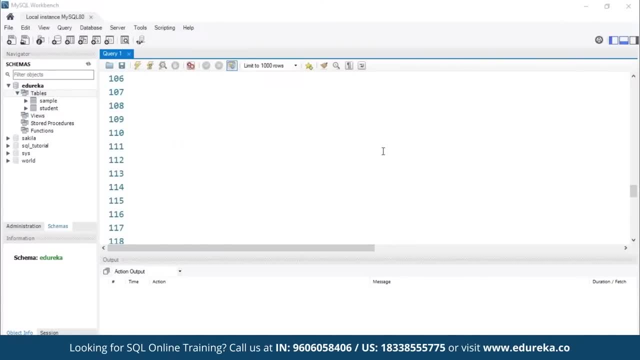 Whenever we insert data to student table, the previous trigger, that is, sample trigger, will be executed. now, with the help of after insert trigger, Let's show the marks of the student table in a final mark table. This will be the after insert trigger, and the name of this trigger is Cal. 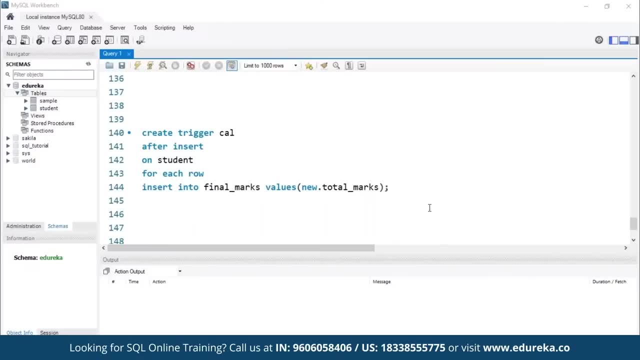 We will be updating total marks from student table to final marks table. Let me execute this trigger And we can see that the trigger with the name Cal has been created. to check the working of a trigger named Cal, Let me insert the data of Rachit Kumar into student table. 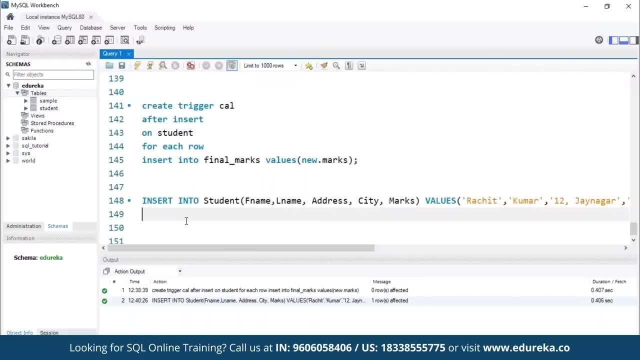 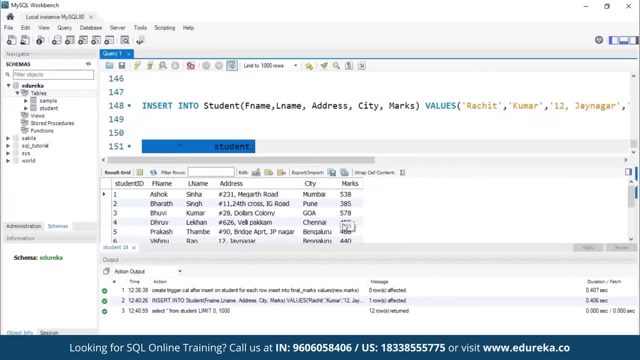 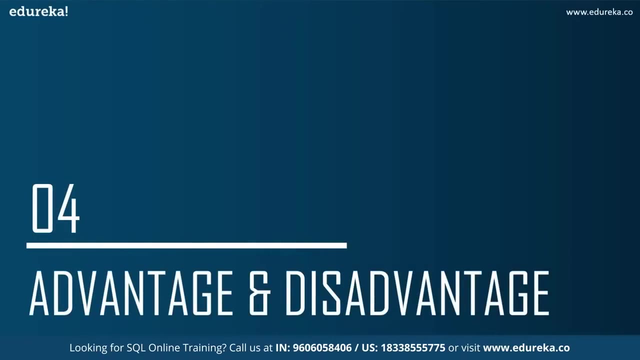 and make a note. His marks is 500, so we can see that the data has been inserted into the student table. Let me execute this query And we can see that the student named Rachit Kumar has 600 marks. Let's move to the next topic, that is, advantage and disadvantage. 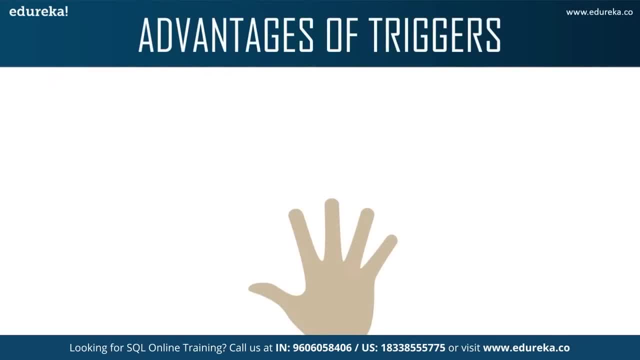 Let's look at the advantages of a trigger. First one is forcing security approvals on the table that are present in the database. The next one is triggers provide another way to check the integrity of the data. The third one is triggers counter react invalid exchanges. 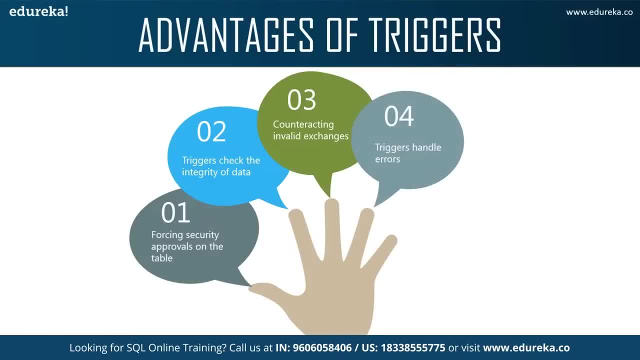 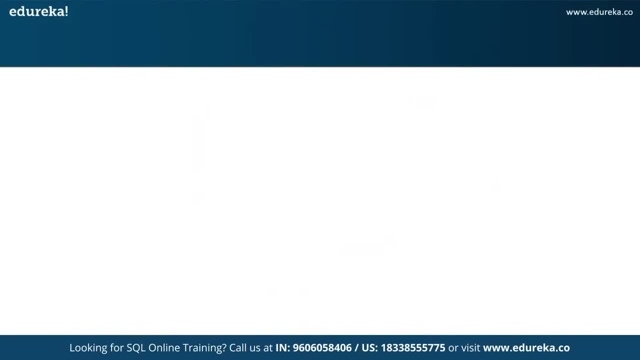 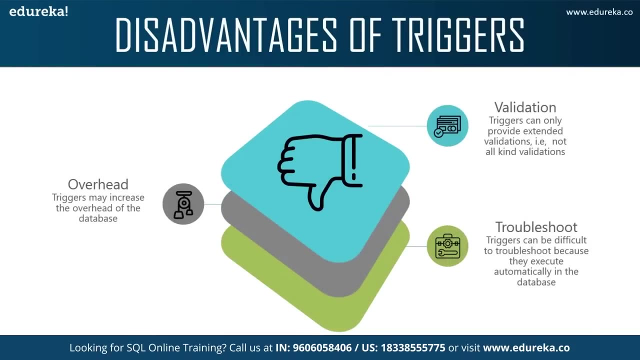 The fourth one is triggers: handle errors from the database layer. And the final one is normally. triggers can be useful for inspecting the data changes in the table. Let's look at the disadvantage of a trigger. triggers can only provide extended validation. That is not all kind of validations. 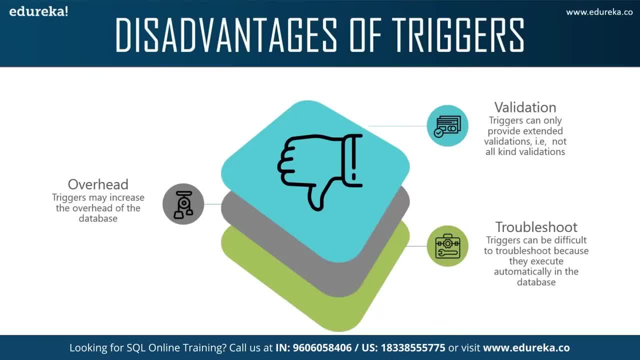 for simple validations. You cannot use not null, unique check and foreign key constraints in a given trigger. Next one is triggers may increase the overhead of a database. The final disadvantages: triggers can be difficult to troubleshoot because they execute automatically in the database. This may not be visible to client applications. 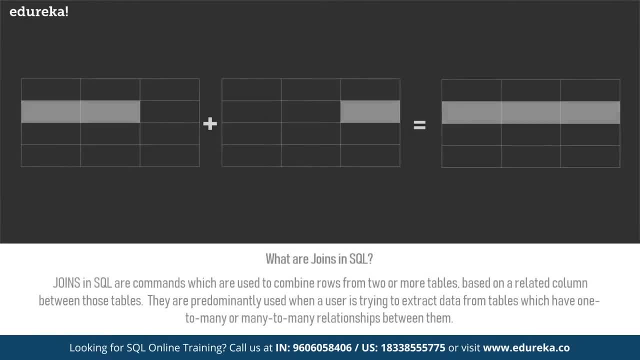 What are sequel joints? So if someone asks you what are joints in sequel? joints in sequel a commands which are used to combine rows from two or more tables based on the related column between those tables. the joints are predominantly used When a user is trying to extract data from a table. 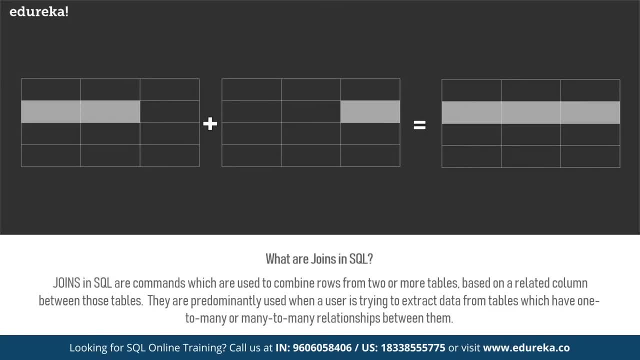 which have one too many relationships between them, or many too many relationships between them. joints in sequel are basically commands, guys, by which you can join two tables and you can get the rows of two tables based on a related column. Now, if you ask me, what are the different types? 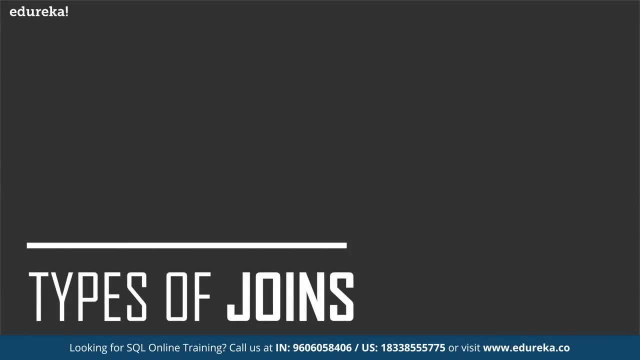 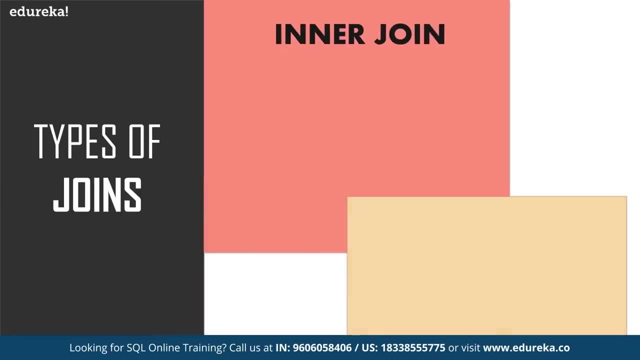 of joints in sequel. there are mainly four types of joints in sequel, that is, the inner joint, the left joint, the right joint and the full joint. So let's look into each one of them one by one, starting with the inner joint. The inner joint is a type of joint that returns those records. 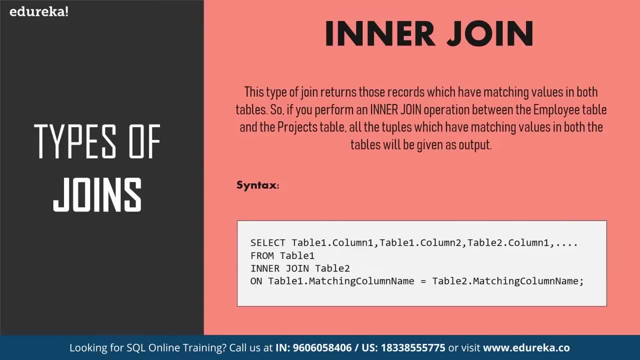 which have matching values in both the tables. So if you consider table A and table B and you apply an inner joint on both these tables, then all those records would be returned which have matching values in both these tables. So for our understanding, I'm going to consider two tables. 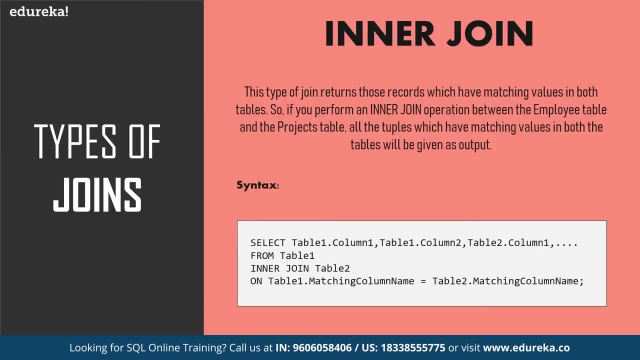 that is, the employee table and the projects table. So when I apply the inner joint on the employee table and the project table, all those tuples which have matching values in both the tables will be given us output. So the syntax for inner joint is as you can see. 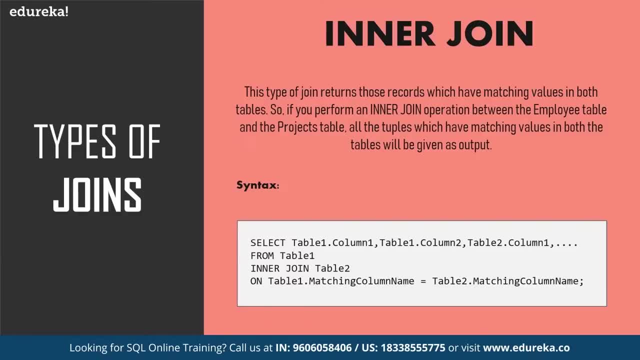 on the screen that a select table one, dot column one. table two, dot column two. table two- dot column one, and so on. So basically, these are the various columns that you want to retrieve from the respective tables, from table one, inner joint table two. that is basically. 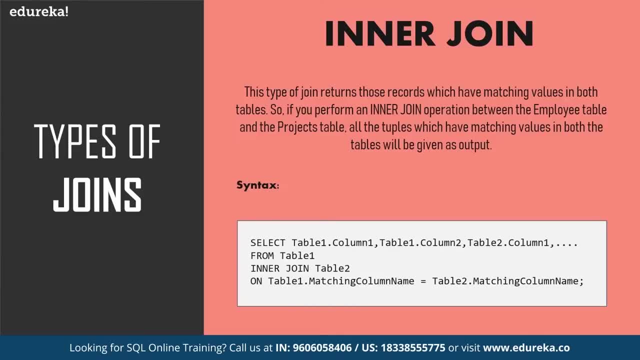 you're applying the inner joint on table one and table two and then you have to mention the related column. So that will be mentioned after the on statement. So you'll mention inner joint table two on table one. dot match in column name Is equal to table two- dot matching column name. 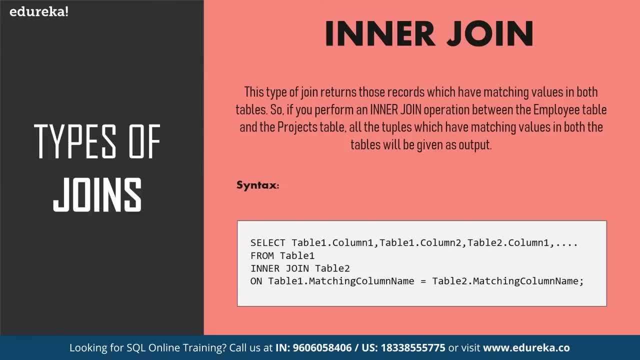 So if I have to just repeat the syntax for you, it's selling all the columns, basically whatever columns that you need, from table one, inner joint. table two on table one, dot match column name equal to table two: dot match column name. So if you want to see how inner joint can be applied practically, 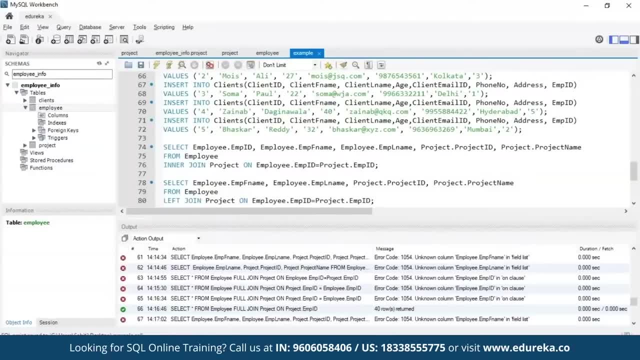 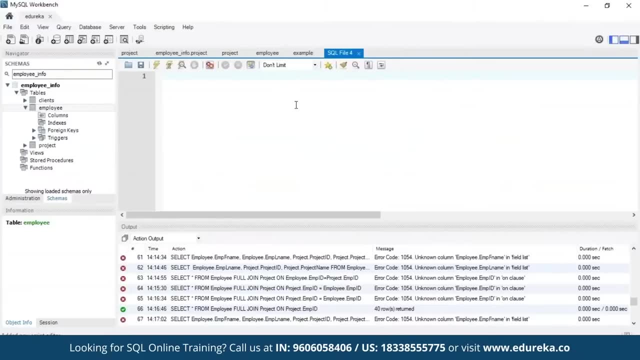 let's move on to my- my sequel workbench, where I've created these two tables, that is, the employee table and the projects table, and let's apply the joint statements on both these tables. Okay, So before I move forward with this, let me just open. 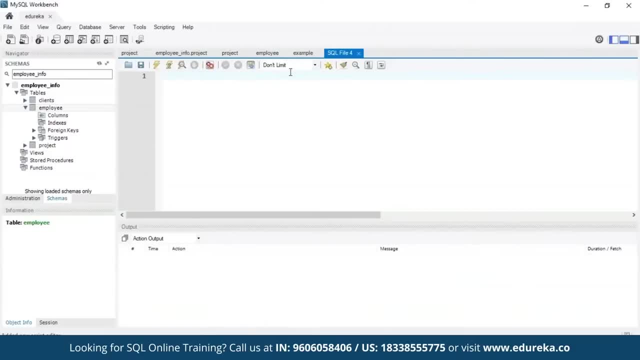 a new query tab and let me just clear all the action outputs. So now what I'll do is I'll just write a statement that is select star from employee right. So I'll just execute this particular statement and you'll see that you know. 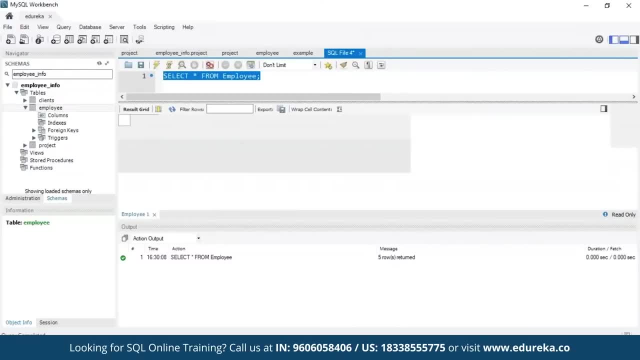 you'll get the output as all the details from the employee table that I've already created. I have around five rows with five employee IDs, and the first name, last name, age, email ID, phone number and address feed it into this table. So, similarly, I'll show you the projects table. 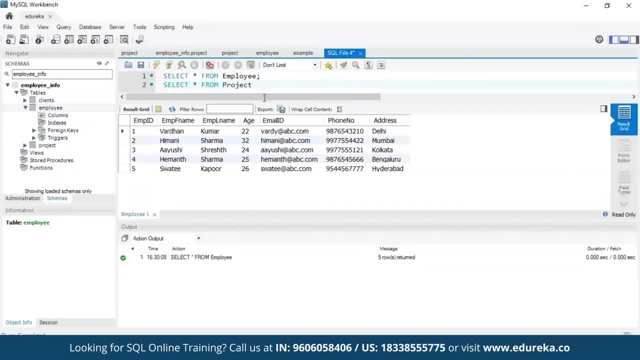 Right. So let me just remove this and let me type in project and just execute this particular statement and you'll see the different column attributes in the project table. So, as you can see, I have the project ID, the employee ID, the client ID, project name. 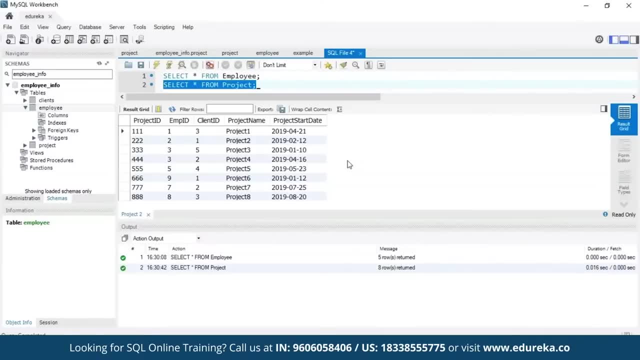 and the project start date client ID can be basically considered for all those clients, So you can have a separate table for the client IDs. So, guys, if you see in both these tables there's a matching column, that is the employee ID, right. 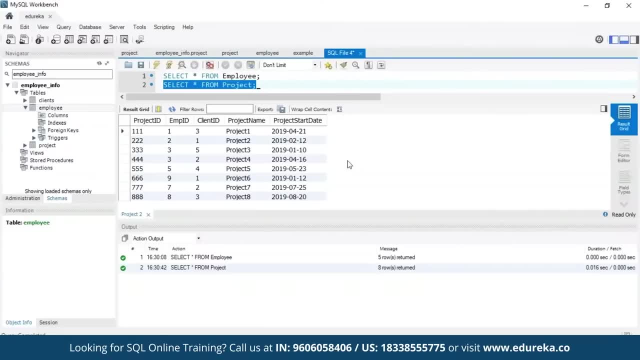 So the basic relation between both these tables is that a specific employee, having a specific employee ID, can work on n number of projects. right, He can either work on the project number 1, 2, 3, 4, 5, 6 and so on. 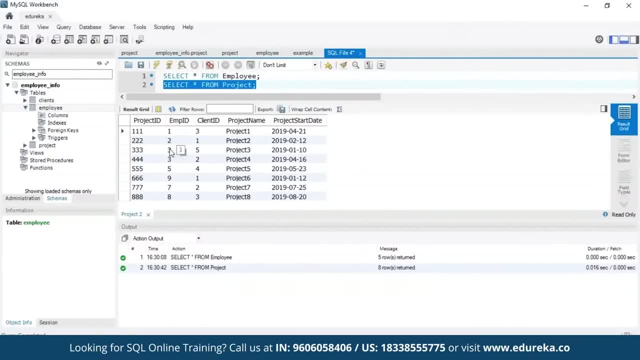 Right. So, as you can see, my employee ID 3 works on two projects, That is, the triple 3 project and the triple 4 project, and similarly, you can see that you know there are employees with the employee IDs 9, 7, 8,. 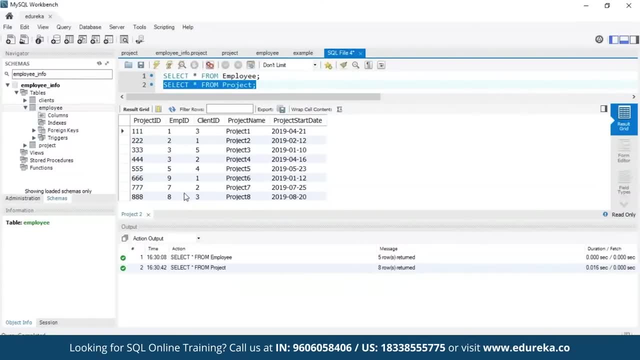 but yes, their information was not present in the employee table right. So let's apply the joint statements on these tables and understand what we get us output. So initially I had explained you what the inner joint was. So when you apply inner joint and two tables, 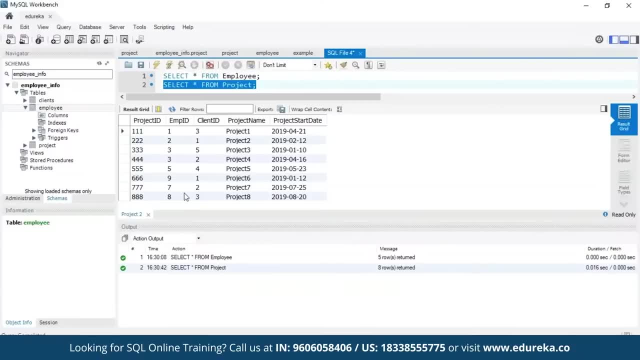 you can clearly see that. you know you get matching values from both the tables. So what I'm going to do is I'm going to apply inner joint on both these tables. So for that you simply have to write a query. So what I'll do is- I've already executed it before- 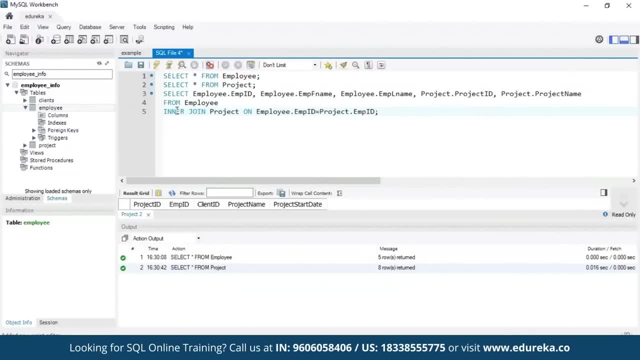 I'll just copy and paste the query over here so that I can explain it for you guys. So what I've done is I've just selected the employee ID, the employee first name, the employee last name, the project ID and the project name to be retrieved from both. 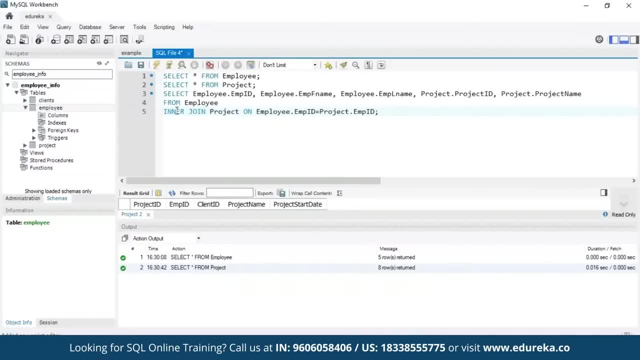 The employee in the project tables and then I've applied an inner joint on the employee in the project table. So for that I've just written a query. as you can see on the screen, It's select employee dot mpid employee dot. MF. name employee. 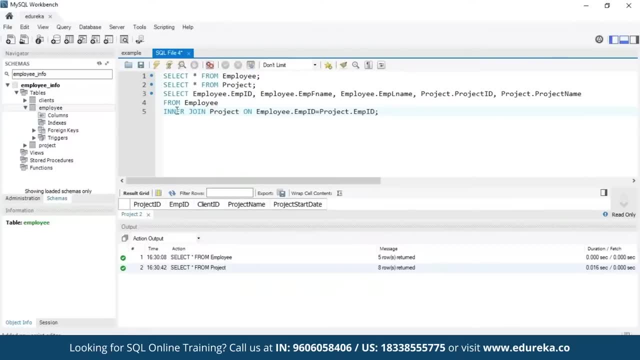 dot ML name. that is basically the first name and the last name. then project dot project ID. project dot project name from employee in a joint project on employee dot mpid is equal to project dot mpid because mpid is basically a matching column in both the tables right. 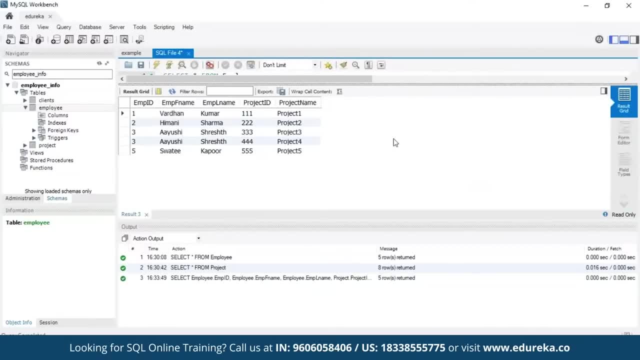 So let's just execute this particular query. So when you execute this particular query, you can clearly see that all the matching values from both the tables have been retrieved. That is basically all the employees working on a specific project and their respective employee ID. employee first name, last name, project ID. 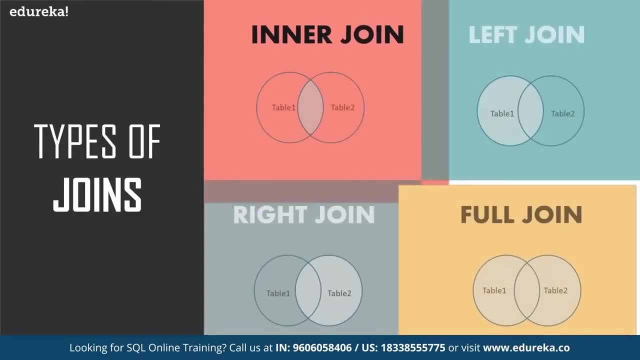 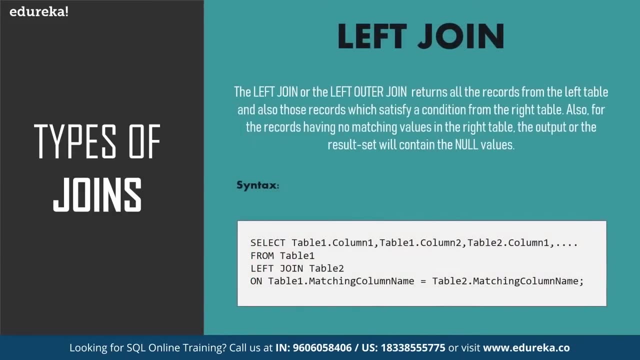 in the project name has been retrieved. So, guys, that was about in a joint. Now let's move forward to our next type of joint, That is, the left joint. Now, as you can see on the screen, now the left joint, or the left outer joint, returns all those records. 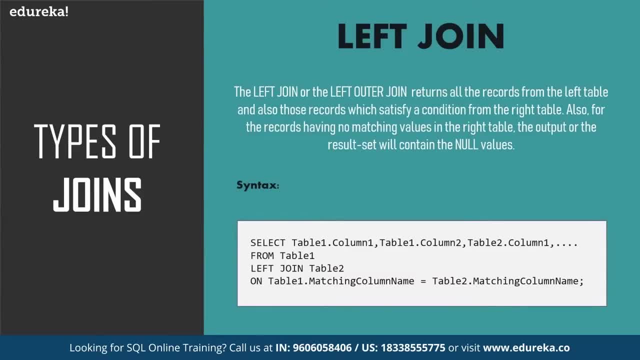 from the left table and also those records which satisfy a condition from the right table. So if you consider table A and table B as two tables on which you want to apply the left joint, then table A would be considered as the left table and table B would be considered as the right table. 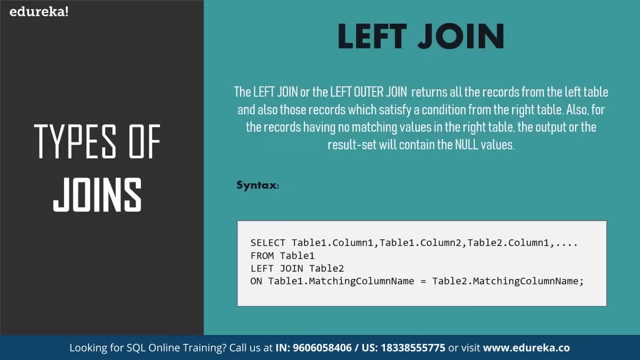 And when you apply a left join on table A and table B, you'll clearly see that you know all the records from the left table would be retrieved and also the records with satisfy a condition from the right table would also be retrieved. Also, let me tell you that you know the records. 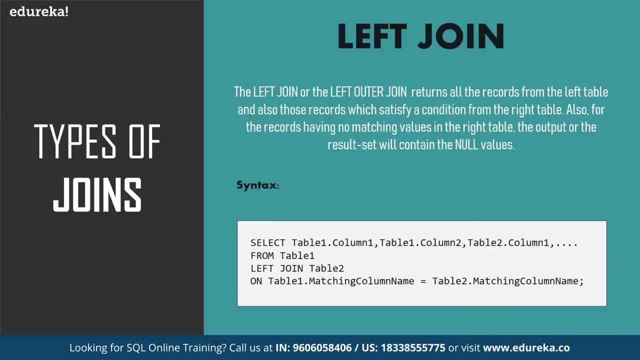 which have no matching values in the right table, the output or the results All set will contain the null values, right? So basically, if you have around three rows from the left table which have no matching records from the right table, then those records will have null values. 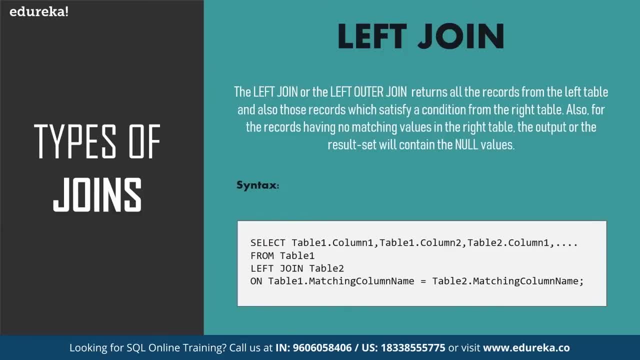 So the syntax for left join is as you can see in your screen. It's just similar to inner joint. You just have to replace the word inner joint to left joint. You can change the syntax like you know. select table 1, that column 1. table 2: dot column 2. 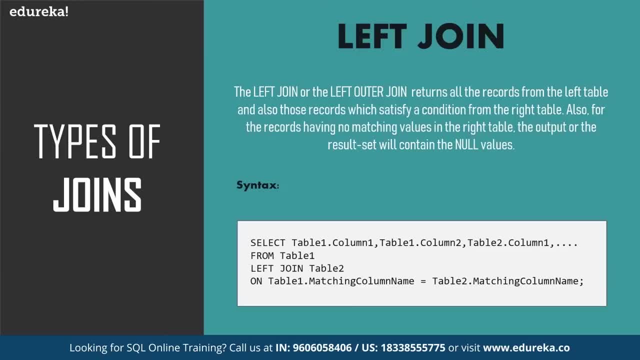 and so on. that is basically the different column attributes that you want to retrieve from table 1 and then left join table 2 on table 1: dot matching column name equal to table 2: dot matching column name. So, guys, that was about left joint. 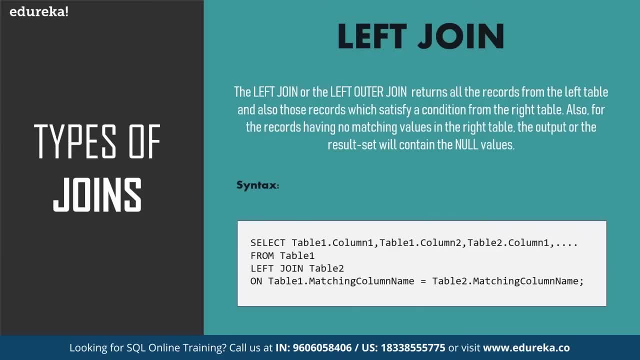 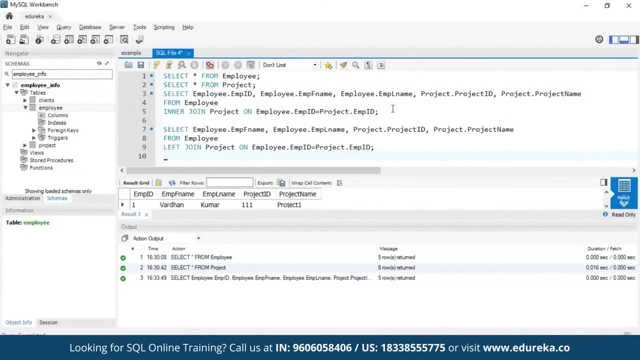 So now let's just again shift back to my mysql workbench and then I'll show you how you can apply the left joint. I'm just going to use the similar query. So what I'm going to do is I'm going to retrieve the first name. 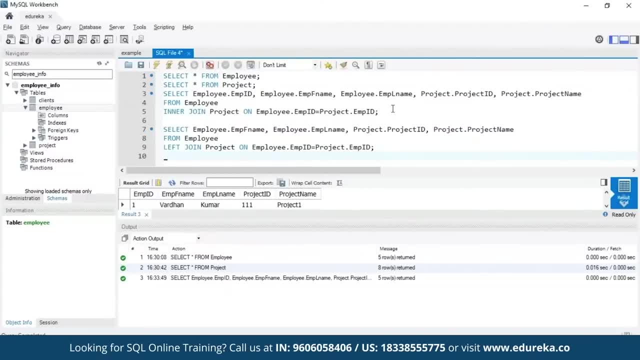 the last name, the project ID and the project name from both the employee and the project table and then apply a left join on it. So for that I've written a query. as you can see on the screen that is select: employee dot amp name. employee dot- amp. 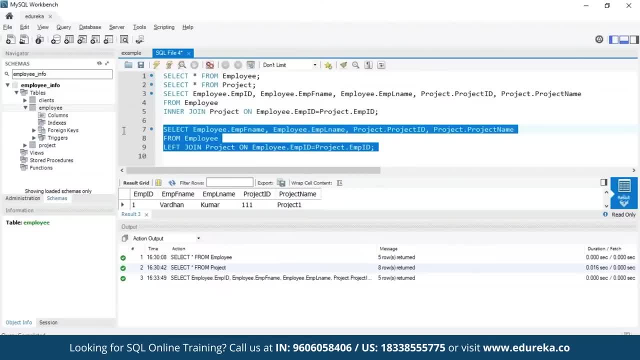 L name: Project dot project ID. project dot project name from employee left. joint project on employee dot amp ID is equal to project dot amp ID right. So basically that is because you know this is the matching column between both the tables, So I'm going to just execute this particular query. 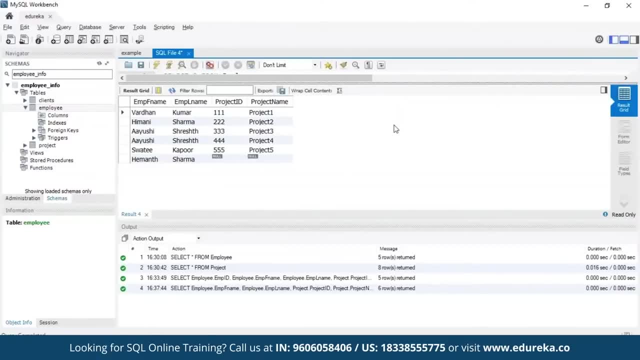 So once you execute this query, you can clearly see the output: all the records from the left table and for those records which do not have any matching record for the right table, We have a null value present. So, if you remember, we had five employees in the employee table. 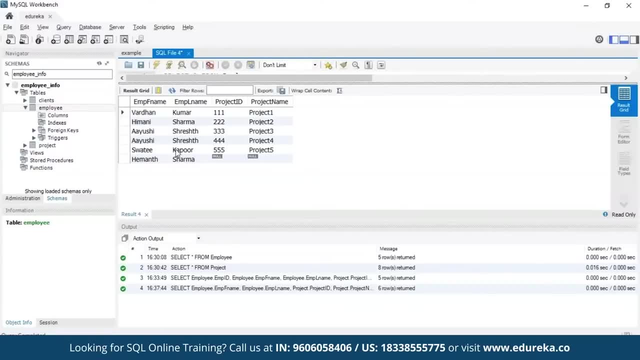 right? So basically that was warden Himani, Ayushi Swati and payment and, if you remember, I, you, she worked on two projects, So both the project details are present over here and he month worked on no project, right? So since he worked on no project, the values present. 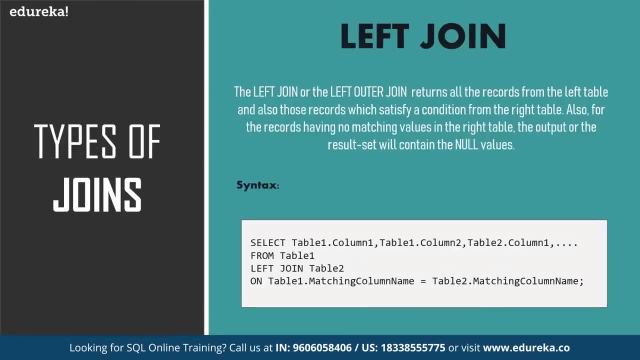 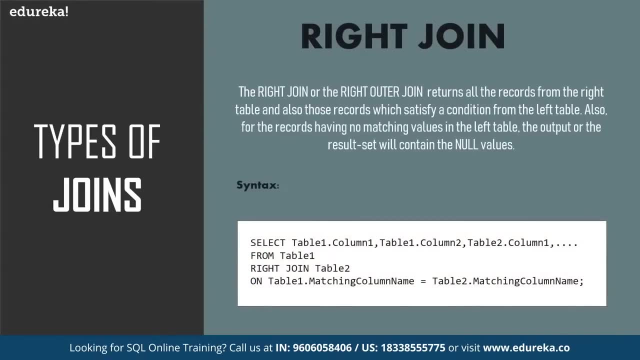 in the project ID and the project name are null values by default. So, guys, that was about the left joint. Now let's move forward to the next type of joint, That is, the right joint. So the right joint, or the right outer joint, returns all the records. 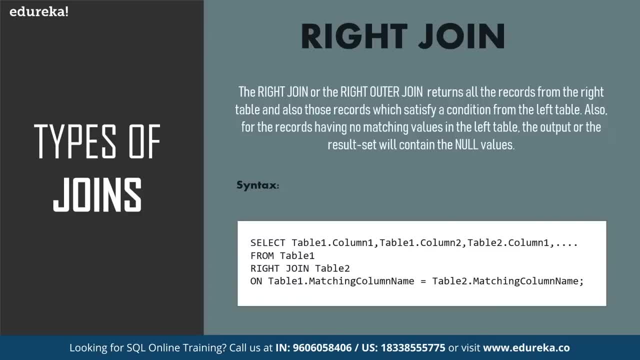 from the right table and also those records with satisfy a condition from the left table. So I know, guys, this sounds quite similar to the left outer joint. Yes, it definitely is. the only difference between both of them is that, you know, the right outer joint returns all the records from the right table. 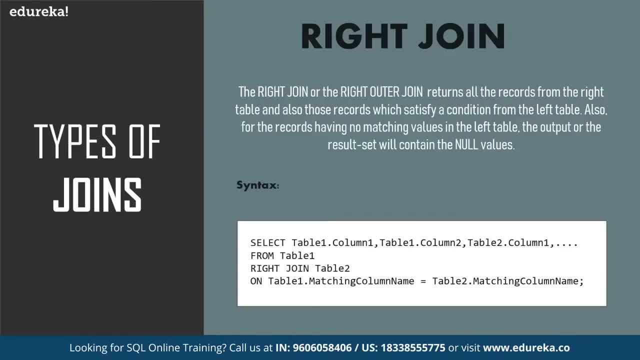 and also the records with satisfy a condition from the left table coming to the left outer joint. the left outer joint returns all the records from the left table and also those records with satisfy a condition from the right table, So it's just vice-versa of both of them. 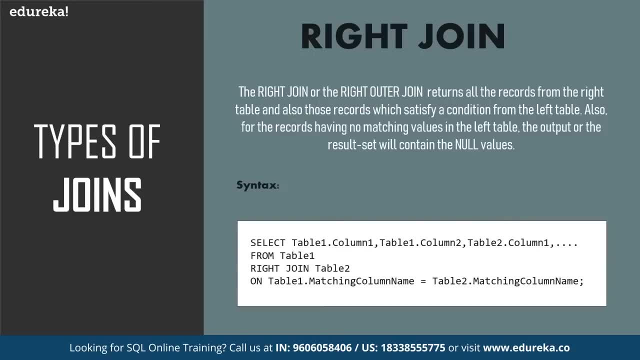 and also, you know the records which have no matching values in the left table. the output or the result set would contain the null values. So, guys, that was about the right joint. Now, the syntax of right joint is as you can see in the screen. 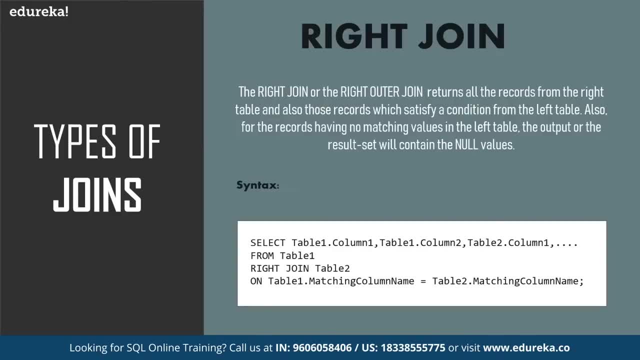 It's again really similar to the left joint. It's simple, It's select: table 1- dot column 1. table 2- dot column 2 and so on. So basically all the column values from both the tables that you want to retrieve from table 1, right joint, table 2. 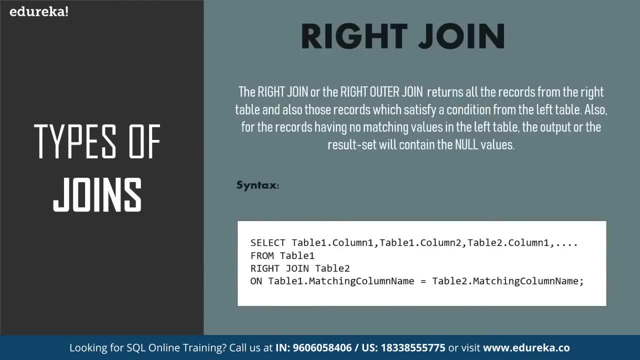 on table 1: dot matching column name equal to table 2- dot matching column name. So the only difference between syntax, if you've seen the three joints that you saw till now, was the word inner left and right. else everything else would be same, So you just have to apply the same logic. 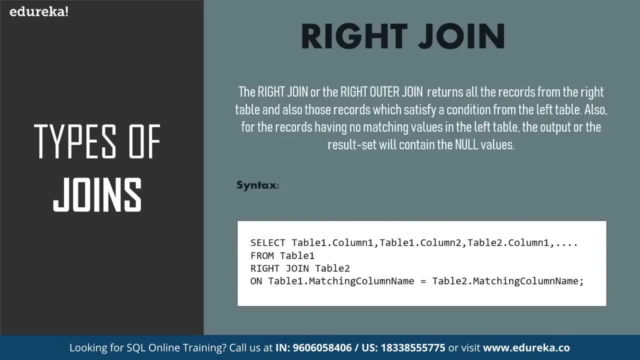 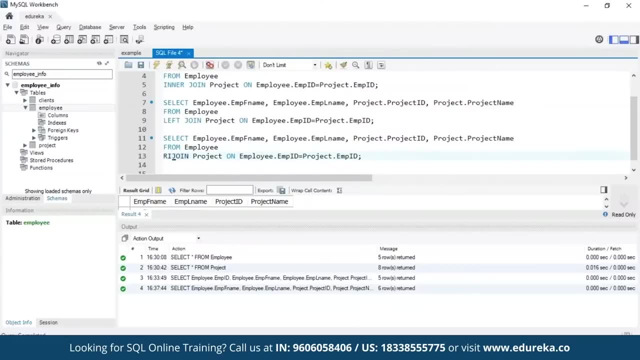 So for that, what we'll do is we'll again shift back to my mysql workbench. Now what I'll do is I'll just copy the query, I'll paste it over here again and then I'll just change this word to right. So I'll just apply: right, join. 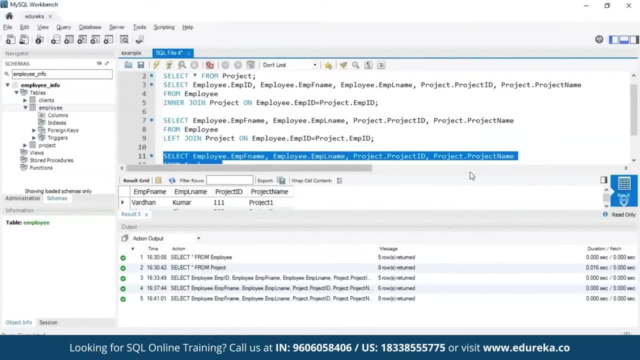 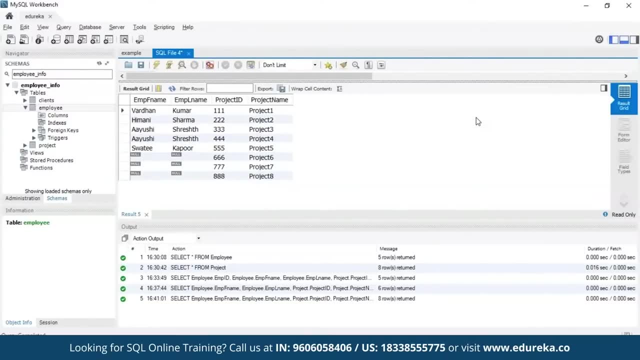 Now I'll just execute this query again. So when we execute this query you'll clearly see that you know the employee. first name, last name, project ID and project name are retrieved from both the tables. All those records from the right table are we retrieved. 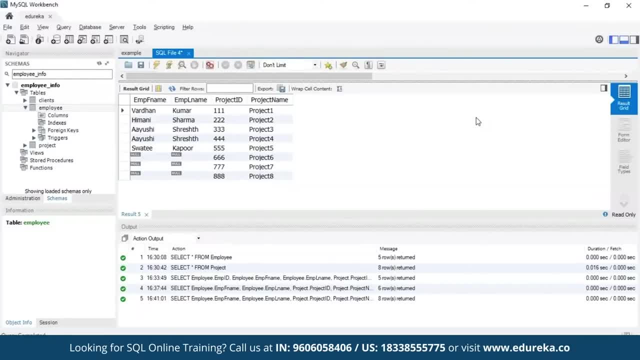 and the records which satisfy a condition from the left table are also retrieved. But yes, those records which have no matching values from the left table have null values present in the record. You can clearly see that you know word in Himani, Ayushi and Swati worked on projects. 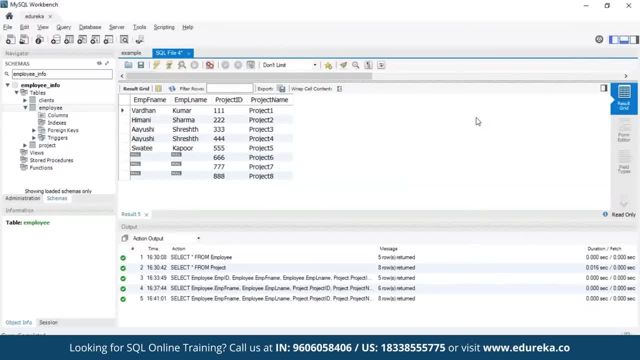 and then they had this specific project IDs and project name. But yes, they were employees who worked on project 6, 7, a, but their employee information was not present in the employee table. So that's the reason there's null value present in the records of 6, 7, 8 project. 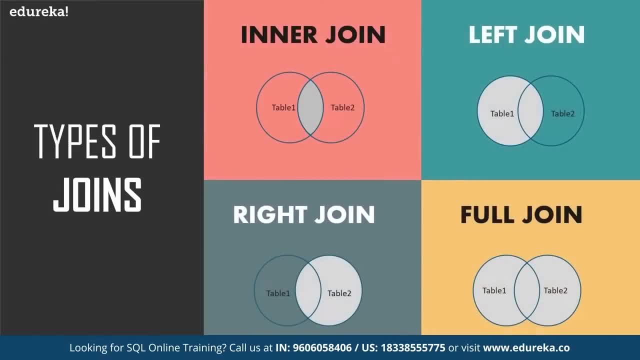 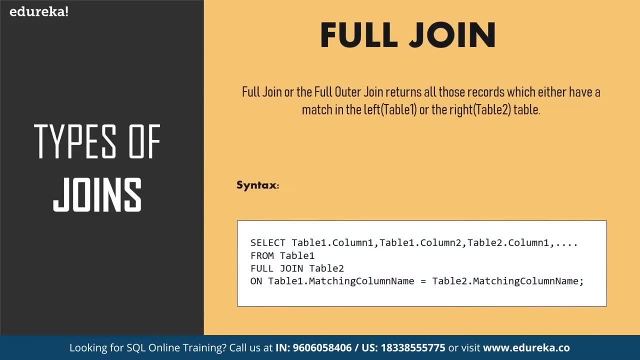 So, guys, that was about right. join. Now moving forward to a final type of join, that is, the full join. So the full join, or the full outer join, returns all those records which either have a matching value in the left table or in the right table. 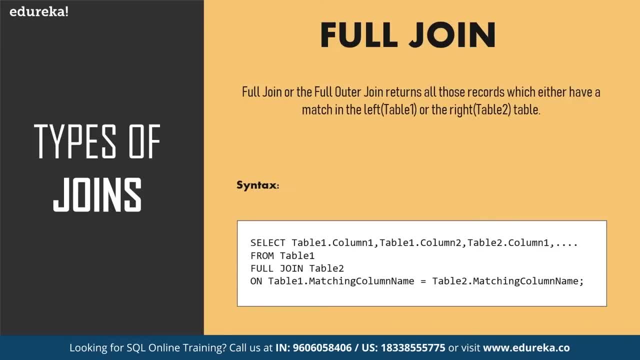 So, basically, if you consider table A and table B and you apply full join on both these tables, then it will return all those records which either have the matching value in table A or in table B. Now the syntax for full join is really simple. 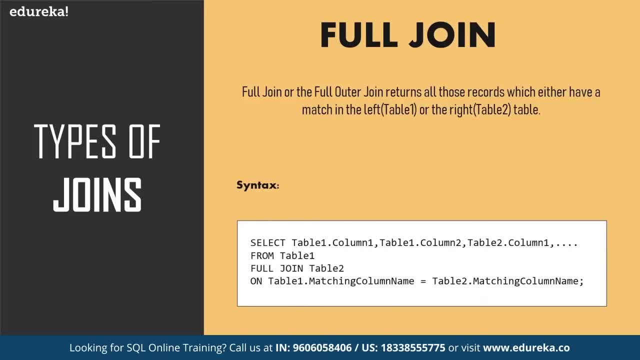 It's again the same as the other three joints, but you just have to mention the word full join. So the syntax is: select: table 1.. Column 1, table 2. Column 2, table 2. Column 1 and so on. basically different column attributes. 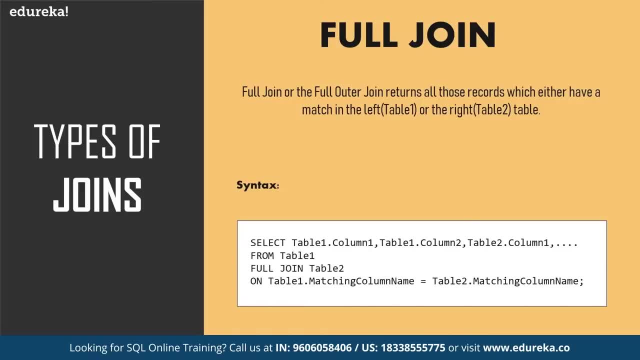 from table 1: full joint table 2 on table 1: dot matching column name equal to table 2: dot matching column name. So that's basically again the related column. that is basically a matching column. now to see how full join works, Let me just shift back to my, my sequel workbench. 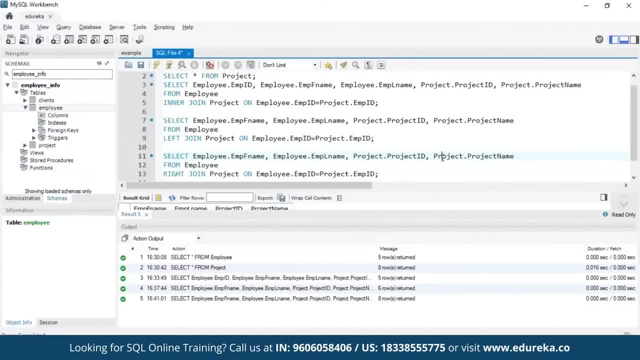 Now let me just tell you one thing over here Now, since I'm showing you how to apply joins on sequel, Let me just tell you that you know, on my sequel the full joint is not applicable. So that's the reason, since I'm showing you on my sequel workbench. 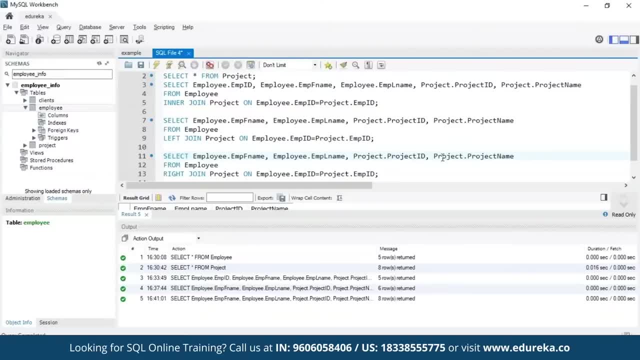 the word full join will not work. to just show you the working of full join, I'm just going to use the word Union in between both these queries. So what's going to happen is we're going to retrieve all the values from the left table. 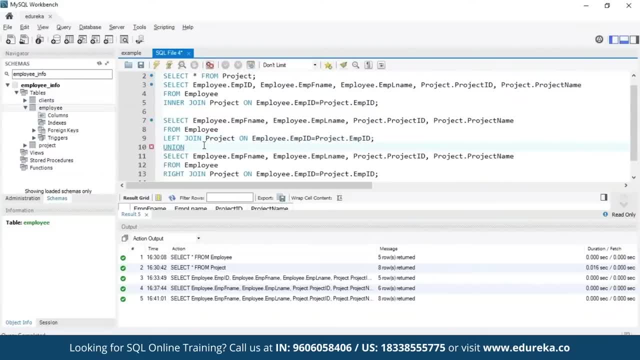 and the matching value to the right table, that is, through the left joint, and then we go to Union it with all the matching values from the right table and also the values with satisfy condition from the left table. So this is nothing but full joint. But since we're working on my sequel workbench, 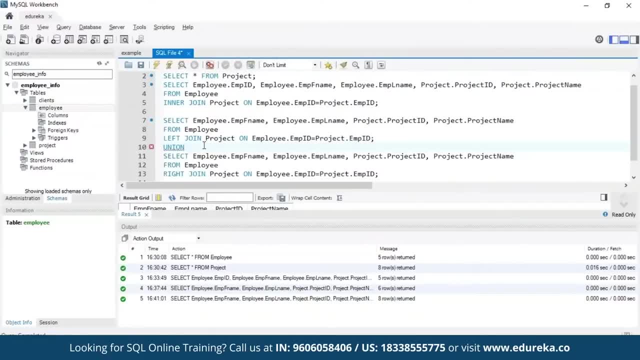 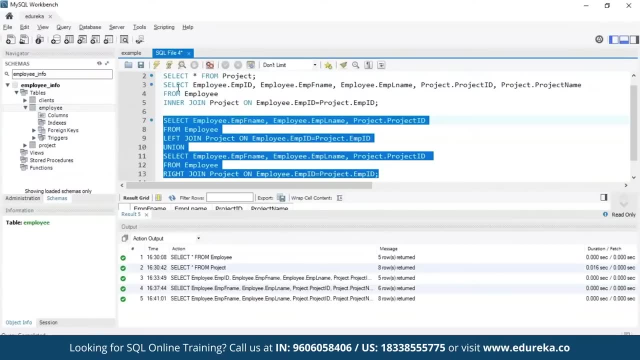 and the word full joint doesn't work, So I'm going to just use the word Union. I'm just going to retrieve the project ID, the employee first name and the employee last name. So what I'm going to do is I'm going to just execute this particular query. 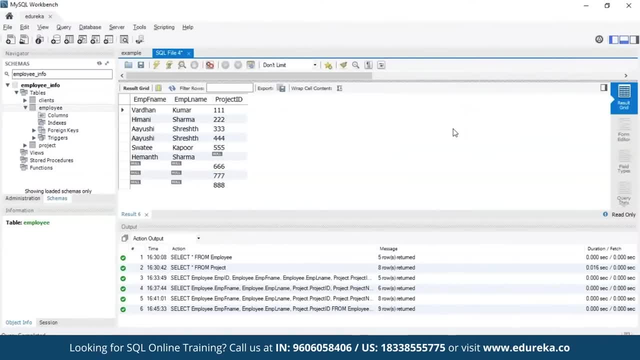 So when I execute this particular query, you'll clearly see that you know we're getting all the values from the left table which satisfy a condition from the right table and also all the values from the right table which again satisfy a condition or match the values from the left table right. 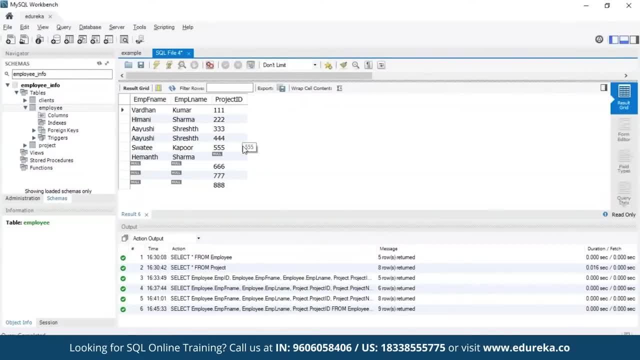 So if you consider the first left joint condition, where we got all the employee details and the project details, you'll see that you know we've got Warden Himani, Ayushi, twice Swati, Haman and the respective project details, since Haman did not work on any project. 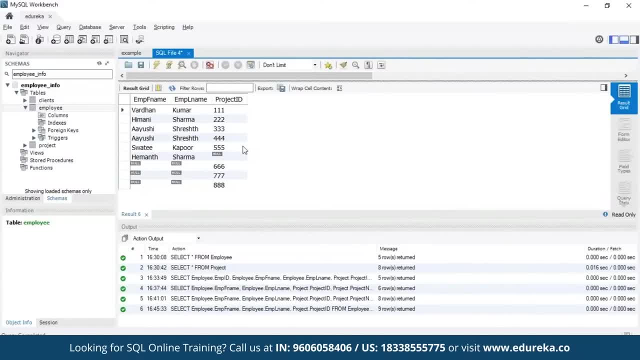 The project ID was null over here now. Similarly, if we consider the output for the right joint, where, you know, we took all the records from the right table and took matching values from the left table, We saw that, you know, for the project ID is triple 6, triple 7, triple 8.. 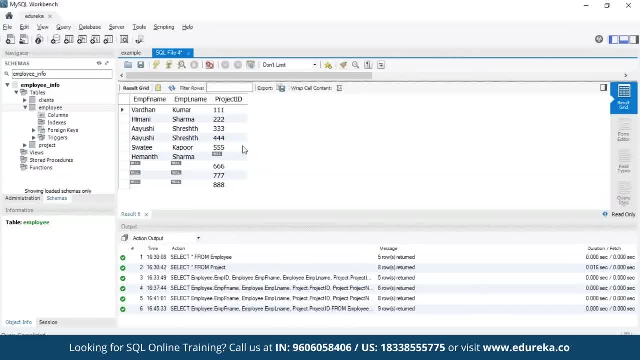 There was no employee information present, right? So that's the reason we have null values over here for employee first name and employed last name. So, guys, that was about full joint, So I hope you've understood the different types of joints. The syntax is really simple. 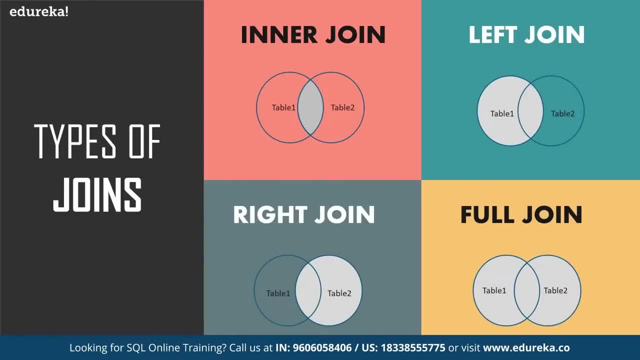 for all the different types of joints- guys, You just have to change the word- and all the different types of joints. for inner joint, You use the word inner. for the left joint, You use left joint. for the right, you use the right joint. and for the full joint, you use the word full joint. 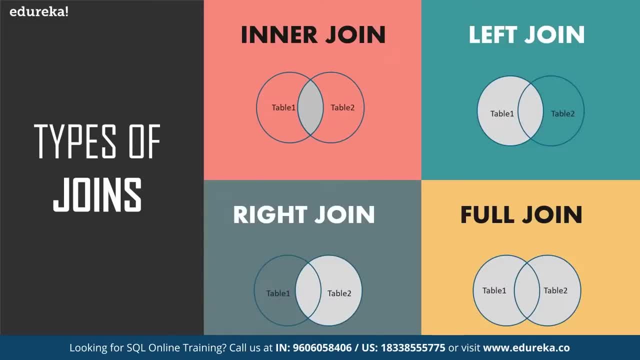 So if you just want to apply left joint, what you simply do is you mention all the columns, that is, you mentioned the keyword select and mention the table name, dot, column name, and then you mentioned from table 1, left joint, table 2 on and then you mentioned the matching column names. 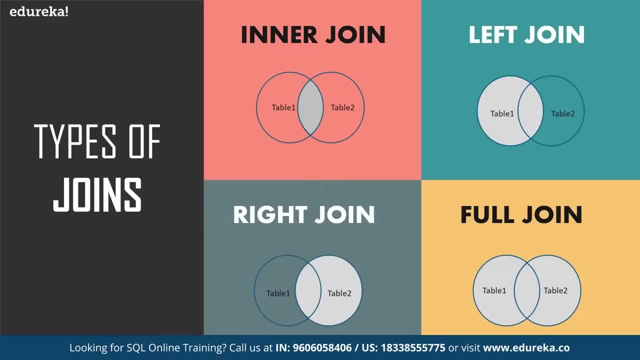 from both the tables, right? So you mentioned table 1, dot matching column name equal to table 2, dot matching column name. So, guys, that's how you can use the different types of joints. I hope it's really clear to you guys. 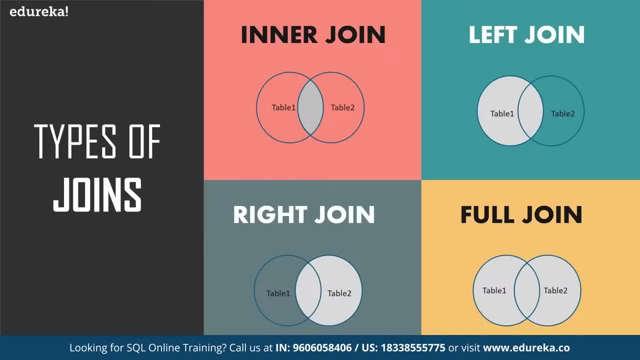 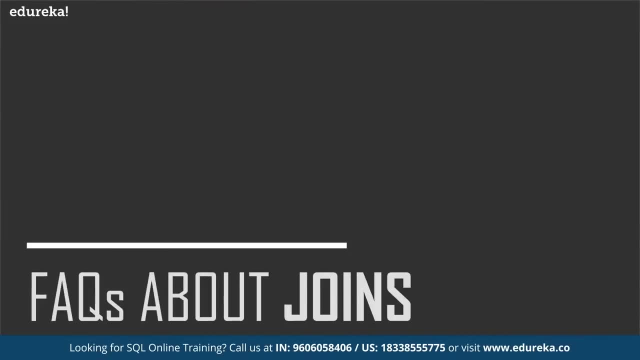 If you have any further queries then you can definitely let us know in the comment section. Now that you know the different types of joints in sequel, Let me just cover few important questions that are generally asked in interviews about joints. So the first question is: what is a natural joint? 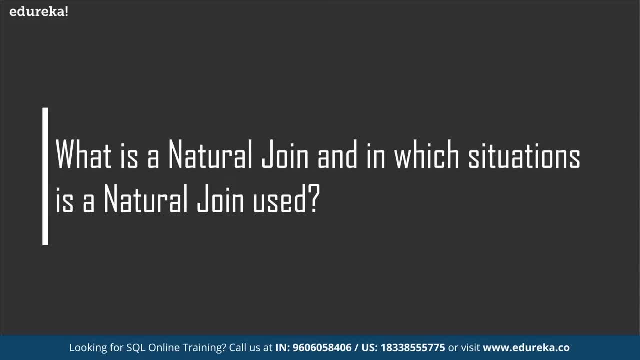 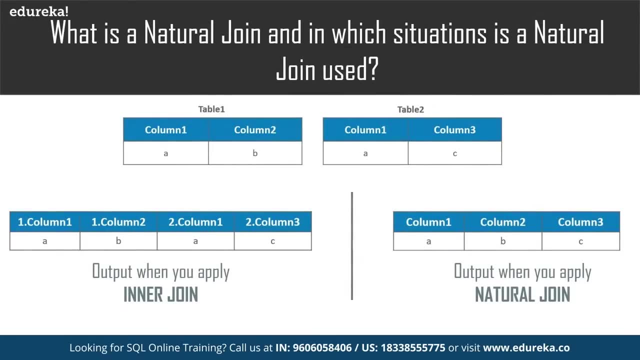 and in which situations is a natural joint used. a natural joint is also a joint operation that is used to give an output based on the columns in both the tables between which the joint operation is implemented. So that's what a natural joint is, guys. It basically aims to give you output based on the columns. 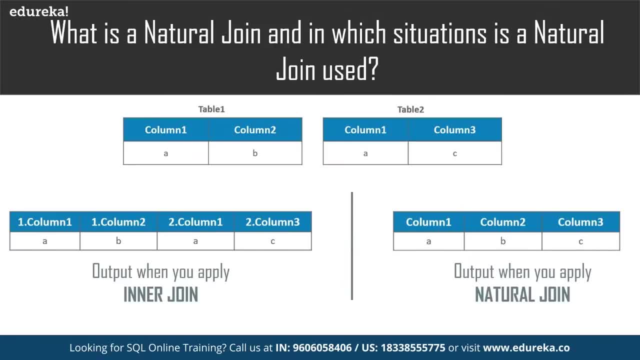 between which this joint is applied. Now, basically, natural joint is used when you want to make sure that you know the number of columns returned are less. So, for example, if you see on the screen we have two tables right, That is table 1 having two columns. 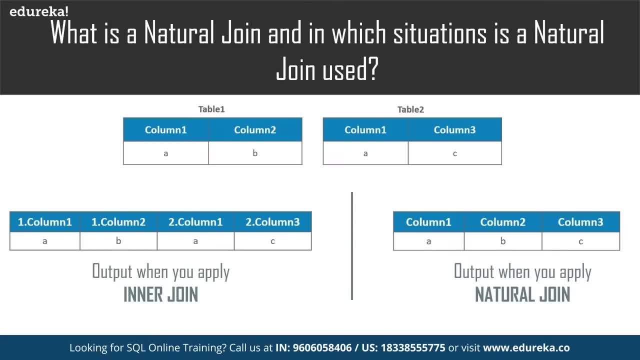 and table 2 having two columns over here. The table 1 had column names- column 1, column 2- and table 2 again has column names: column 1 and column 3.. Now, if you apply a natural join on both these tables, 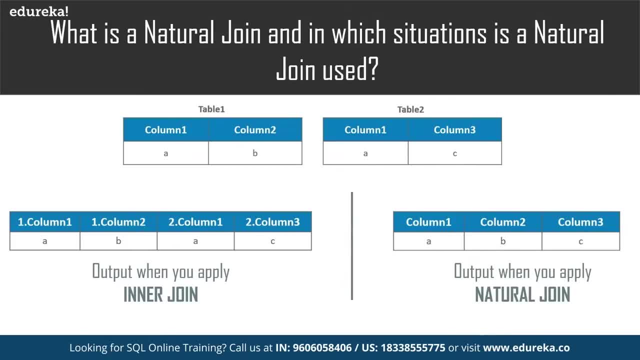 you'll clearly see that you'll get an output as column 1, column 2, column 3 and the respective records. but in the same scenario, if you apply an inner joint- what you will clearly see- that you know you'll get an output like one dot, column 1. 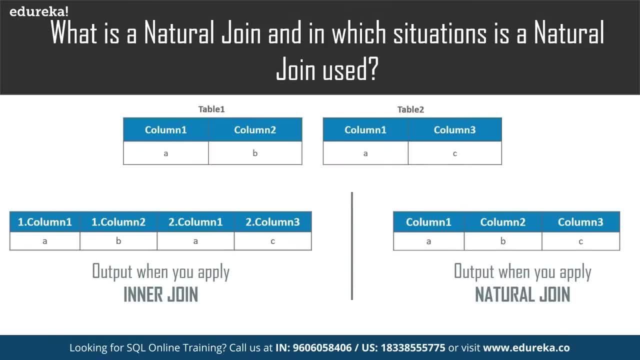 that is basically for table 1, dot column 1 and then one dot column 2. that is table 1- dot column 2, and the respective records would be stored. Now, if you see over here, you'll clearly see that you know when you apply the inner joint you'll have a redundancy of data. 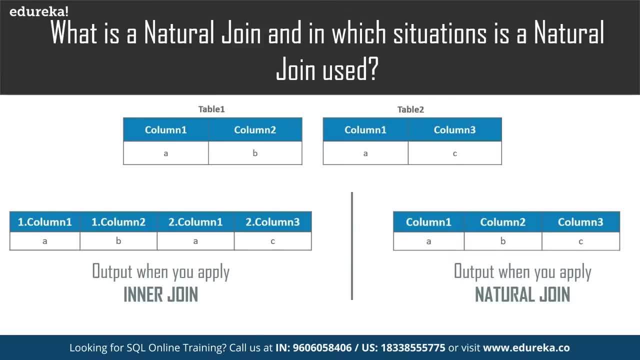 that is, you know, the column 1 data is getting repeated again. That is, basically it is repeated twice, but in this case of natural joints just mentioned once. So this was a scenario of two tables where you know the output was so simple. 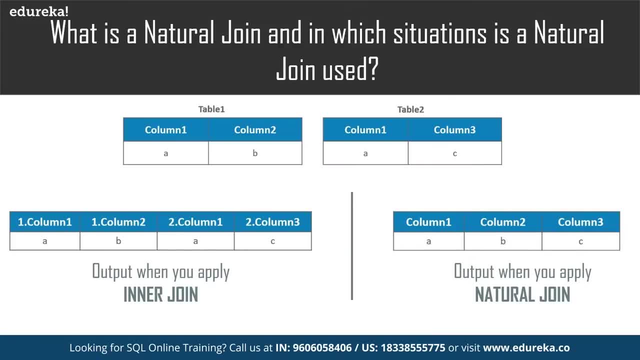 but yes, if you look into daily basis, where you know database administrators deal with n number of tables and that they want to apply the joint operation on these two tables, You'll clearly see that you know if they apply an inner joint then that would create a lot of problem of redundancy of data. 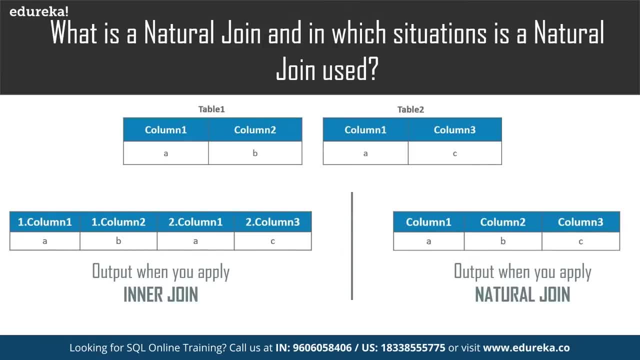 and obviously more number of columns would be generated. But yes, in the same scenario, if they apply a natural joint, the number of columns would be reduced at a maximum extent. So that's the situation, guys, where you apply a natural joint. So if you're ever, as you know, 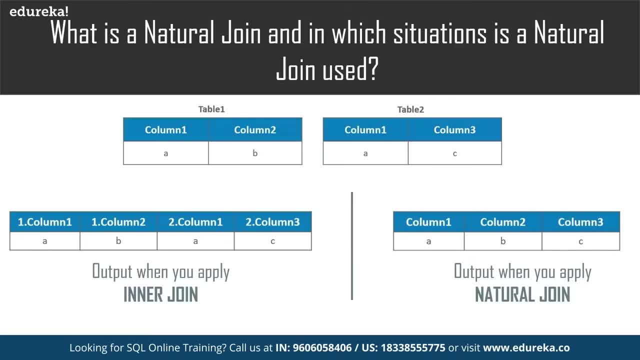 in which situations do you apply a natural joint? You can just answer this question by simply saying that you know you can apply a natural joint when you want the number of columns to be less. So I hope I'm clear with this point. Now, moving on to our second question. 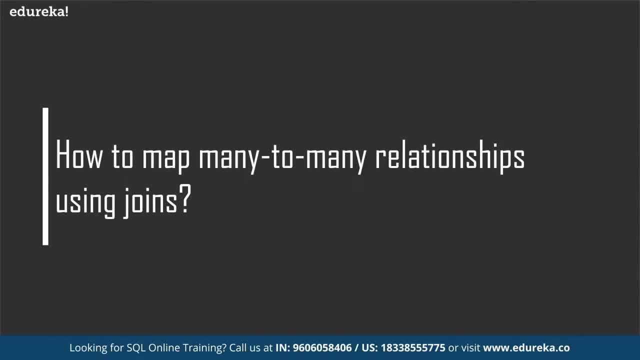 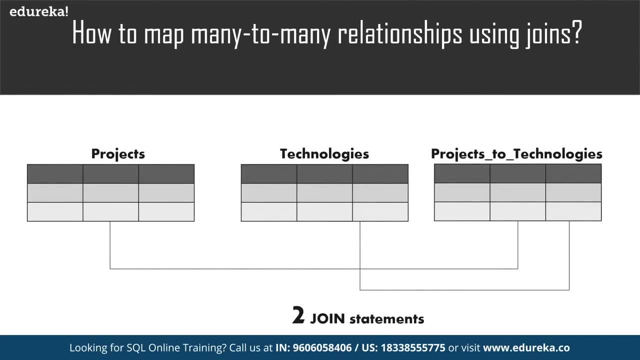 that is how to map many to many relationships using joints. Now, it's a known fact that you know the joints are basically used to map one to many relationships. But yes, if there's a confusion, you know how to map many to many relationships. 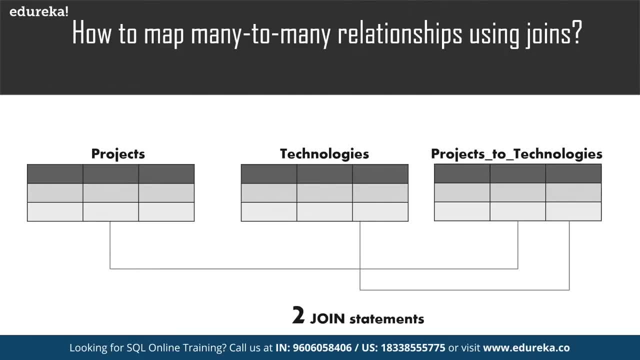 Let me just tell you that you know you need to use two joint statements. So to explain you why two joint statements are required, you can consider a scenario where you have creep tables, that is, the employee table, the projects table and a technologies table. Now, let's assume that you know. 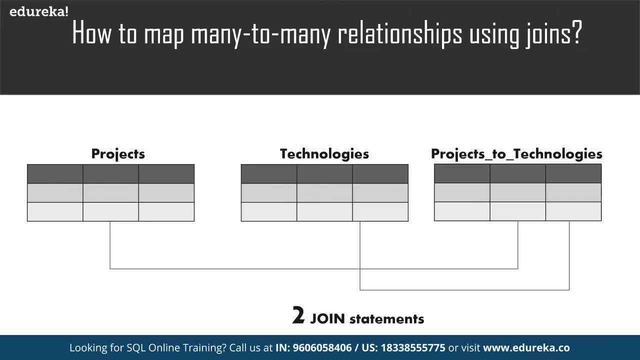 each employee is working on a single project, So this obviously means that you know, one project cannot be assigned to more than one employee. Now, similarly, if you consider, a project can be based on multiple technologies, and any technology can be used in any number of projects. 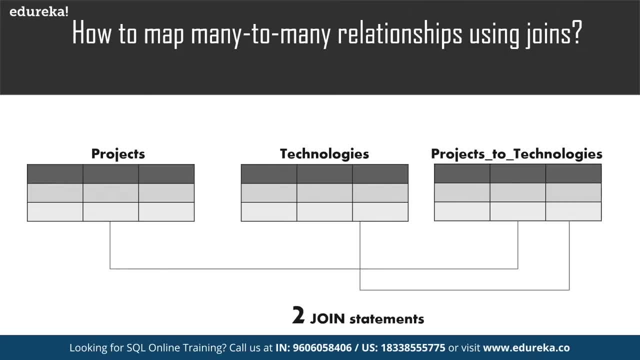 This kind of relationship is basically a many-to-many relationship. now, to apply the joint operation on the many-to-many relationships, What you can simply do is you can have three tables, that is, the projects table and the technologies table itself. So basically, these are the two tables. 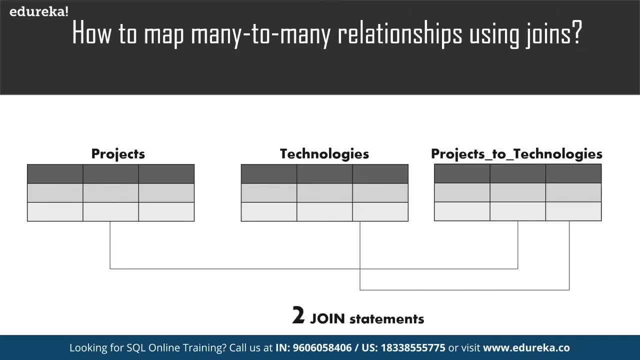 which have many-to-many relationships between each other. and also we can have an extra table, that is the project to technologies table. Now, the project to technologies table will hold the combination of project and technology in every row. Now, let's say we have a project a. let's say this project a has 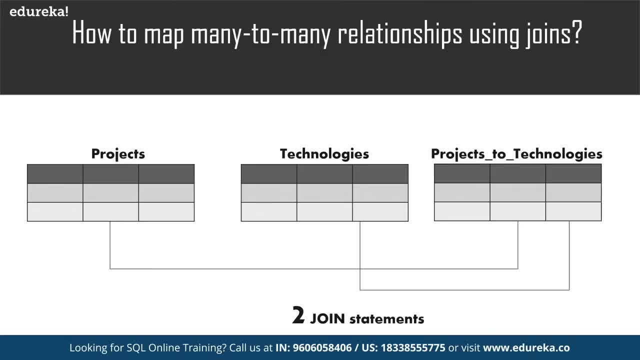 three Technologies, that is, DevOps, microservices and Hadoop. Now you have to map these Technologies to the project right now. this project to technologies table will hold the record of every project technology combination. So it will hold a record of project a to DevOps. 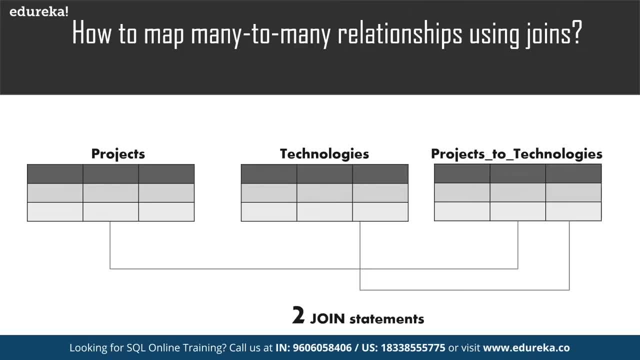 and then project a to again Hadoop and project a to microservices. Similarly, it will have n number of records for n number of projects and m number of Technologies. So this table is really, really important in this scenario and this table basically aims to map the item. 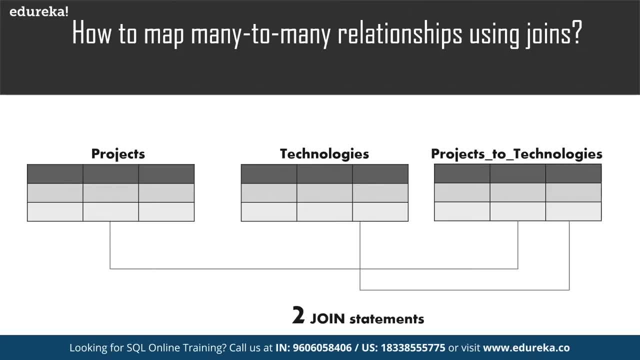 on the projects table to the items on the Technologies table, so that multiple projects can be assigned to one or more Technologies. So now that you have three tables, that is, the projects table, the Technologies and the projects to Technologies table, You need to use two joint statements. 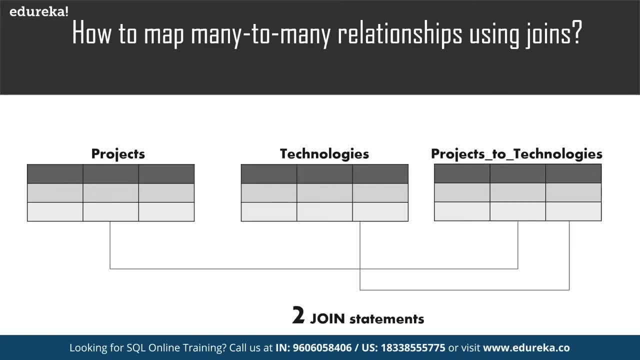 to link all these tables together. that is, use the first joint statement to join the project to Technologies to projects table, And then we have to use the second joint statement To join the project to Technologies table to Technologies table. that this is how all the projects 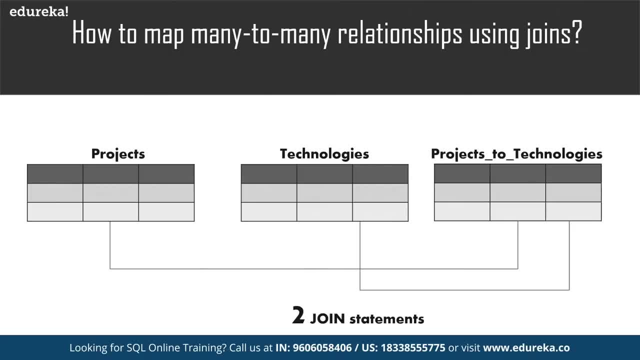 and Technologies which have a many to many relationships between them will be linked with each other. So it's really simple, guys: Whenever you have an end-to-end relationship between two tables and you want to apply a joint operation between these two tables, You just have to create another table. 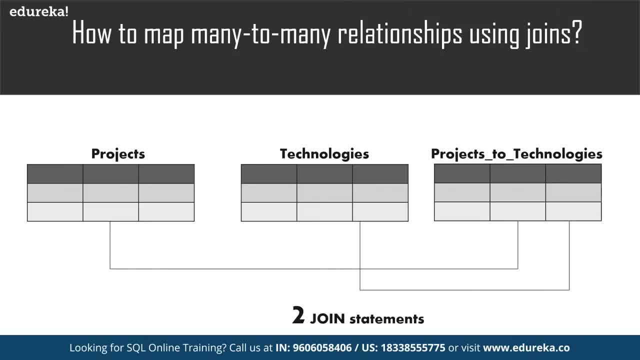 you know which can have all the combinations of the previous table, and then you apply a joint operation from table a to table C and then table B to table C. So I hope I'm clear with this point. Now let's move forward with our next question. 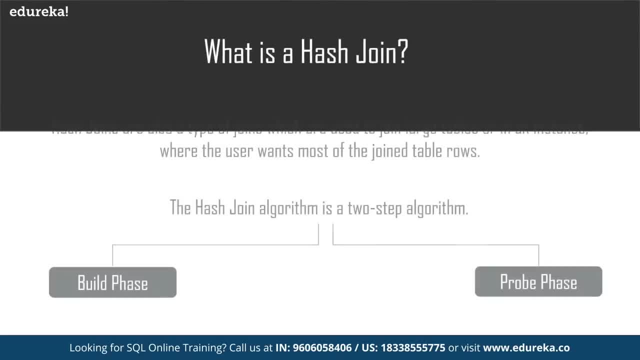 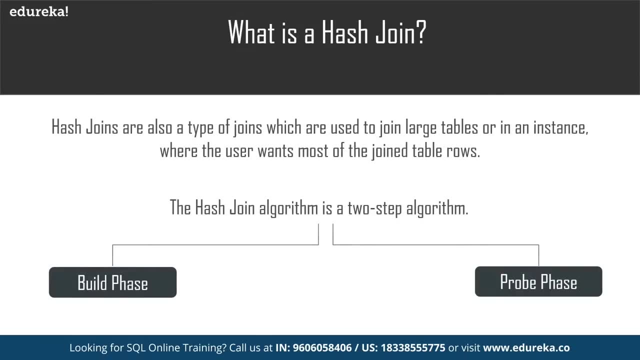 That is what is a hash join. now, hash joins are also a type of joints which are used to join large tables or an instance where the user wants most of the joint table rows. So whenever the user wants the most of the joint table rows, or when you want to join two large tables, 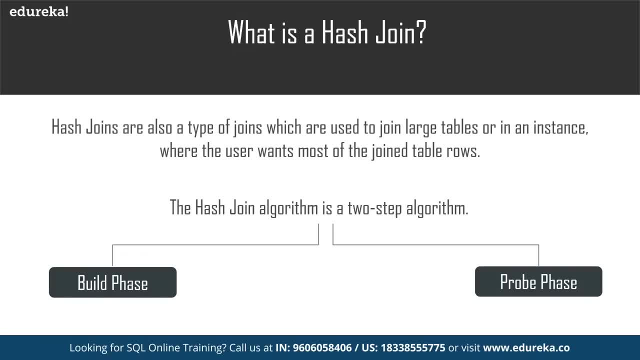 you basically use this type of joint. that is basically the hash join. and the hash join algorithm is basically a two-step algorithm, So it has mainly the build phase and the probe phase. So in the build phase you basically create an in-memory hash index. 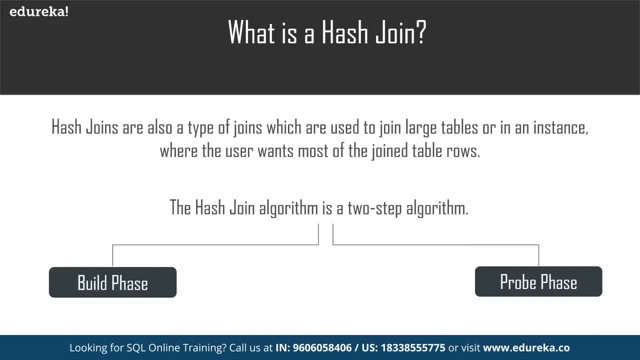 on the left side of input and in the probe phase you go through the right side of input, each row at a time, and then find the matches using the index created in the build phase. So hash join is again a type of joint which is used to join large tables. 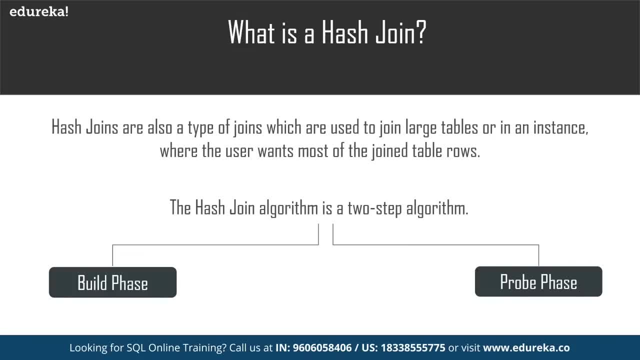 and it has mainly two steps, that is, the build phase in the probe phase. in the build phase, You basically create an in-memory hash index on the left side of input and in the probe phase you go through the right side of input, each row at a time. 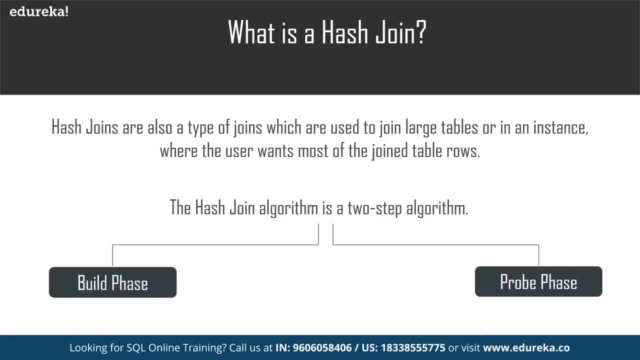 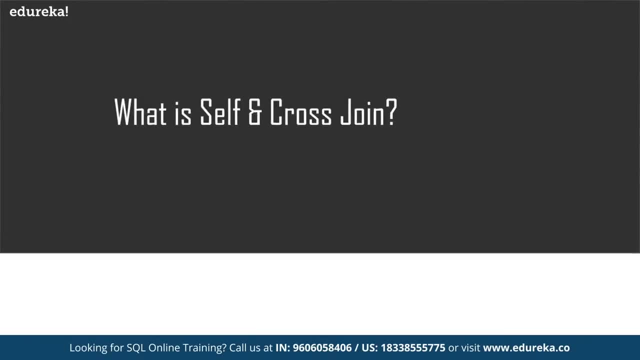 and find the match using the index created in the build phase. So, guys, that was about the hash joint. Now let's move forward with our next question, That is, what is a self-join and a cross-join? So the self-join, in other words, is a join of a table to itself. 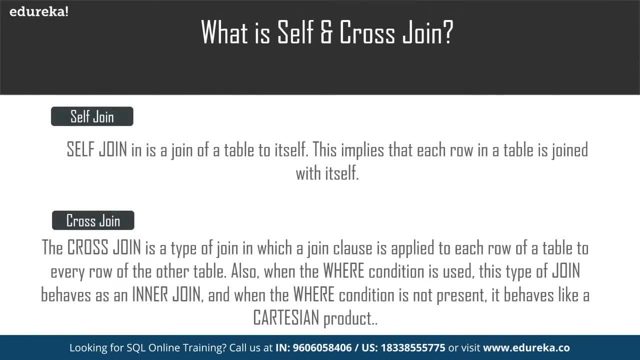 So this basically means that you know each row in a table is joined with itself. So when you apply a self-join to a table, just remember that you know each row in a table is joined with itself. Now, coming to cross-join: the cross-join is a type of joint. 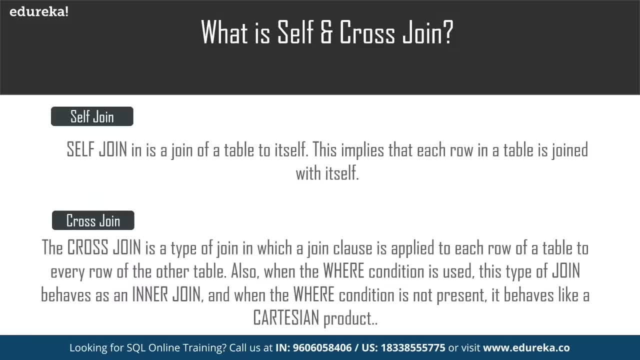 in which a joint clause is applied to each row of a table, to every row of the other table. So whenever you apply a cross-join two tables, then just remember that you know a joint clause is applied to each row of a table, to every row of the other table. 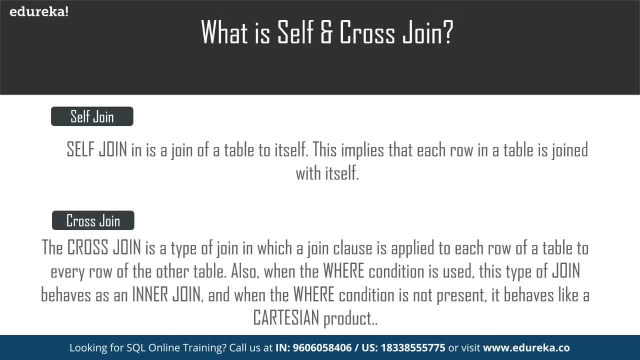 Also, when the wear condition is used, this type of joint behaves as an inner joint, and when the wear condition is not present, it behaves like a Cartesian product. So you just have to remember two points. The first point is that whenever you apply a cross-join, 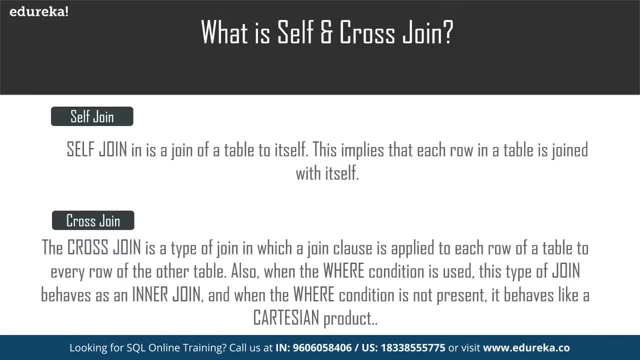 on specific tables. a joint clause is applied on each row of a single table to every row of the other table and also when the wear condition is present. this type of joint behaves as an inner joint, and when the wear condition is not present, it behaves like a Cartesian product. 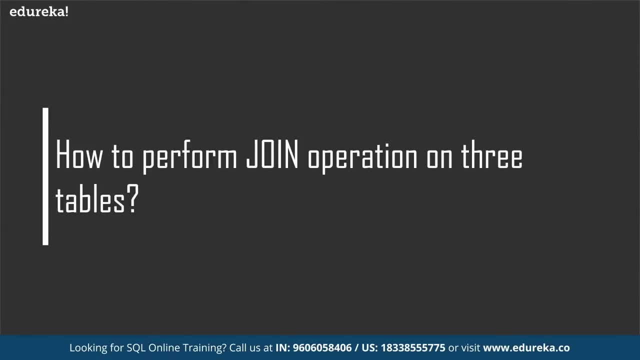 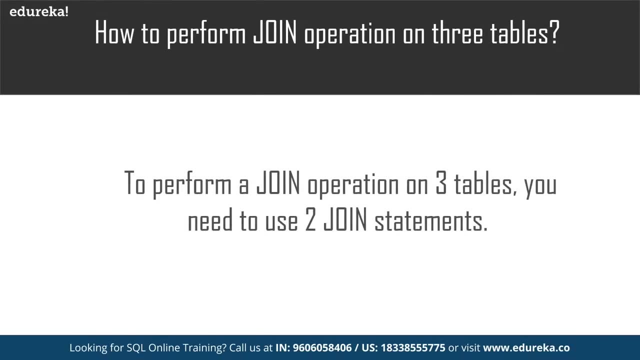 Now let's move forward with a final question, that is, how to perform join operation on three tables. Now, if you remember, in the previous questions I had discussed a question where you know we understood how to map end-to-end relationships using join operations, right? 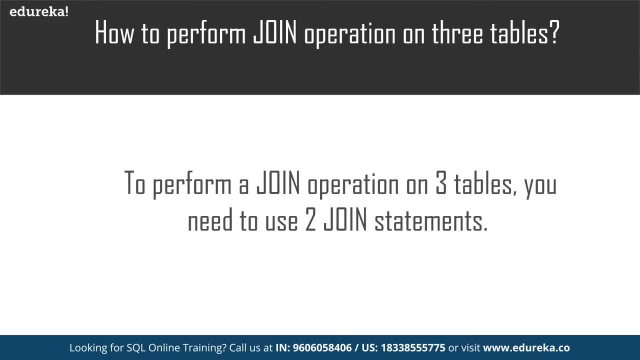 So over there, if you remember, we use three tables, that is, a project stable, the technology stable and the projector technology stable. now, to apply a join operation on three tables, We use two joint statements, right, That is to join table A to table C and then table B to table C. 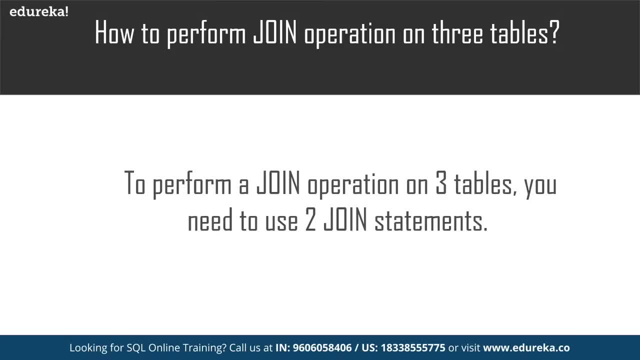 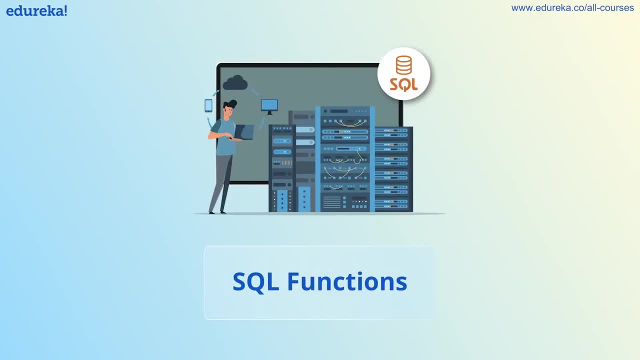 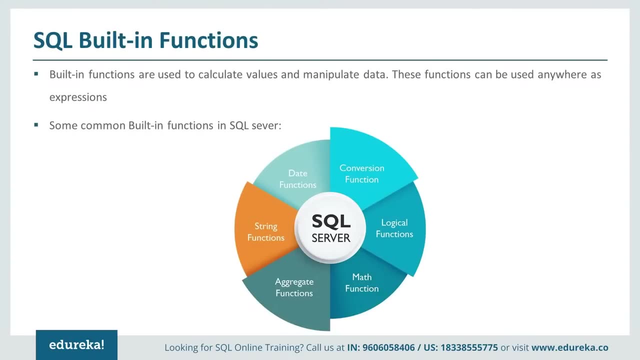 So basically, to apply a join operation on three tables, You need to use two joint statements. Built-in functions are used to calculate values and manipulate data. These functions can be used anywhere as expressions. When we say anywhere, it means we can use them in the select query, we can use them in where clause. 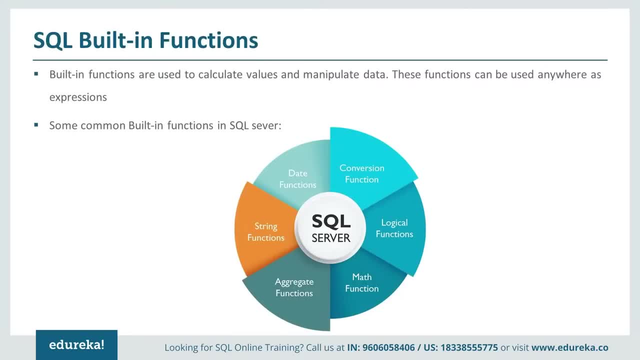 we can use them in having clause. So these built-in functions can be used anywhere, based upon the business requirement of, based upon the type of functions which we are using. So we broadly categorize the various built-in functions into the following categories, as you can see on the screen. 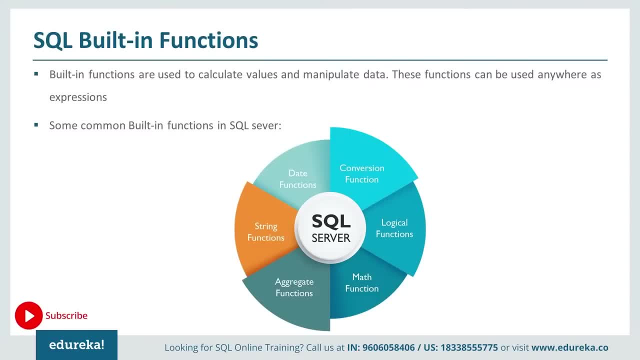 So we can divide the built-in functions into conversion functions where we convert the values from one data type to another data type. We have logical functions, math functions, to play around with the data, mathematical operations. We generally use math functions, aggregate functions, If you want to calculate, for example, average. 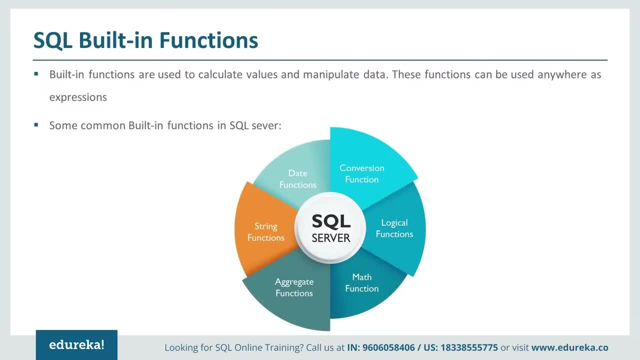 we want to calculate some or total of salary of all the employees, Then we use aggregate functions. is string functions helps us to play around with various strings Or characters in our data. Most of the string functions are somewhat similar to the string functions which we have. 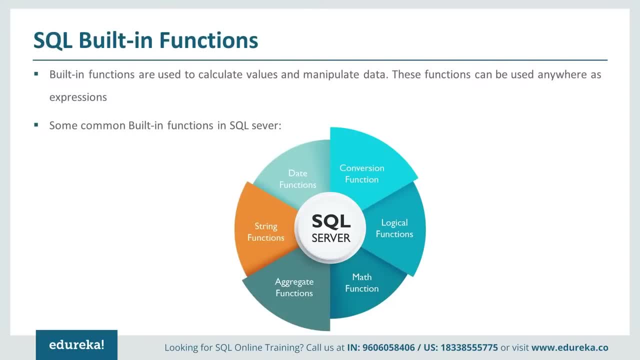 in other programming language or the basic programming languages like C, C++, C, sharp or Java date functions have all the basic functions which we can use to manipulate date or retrieve date from our database. So let's discuss all of the functions one by one in coming slides. as we discussed 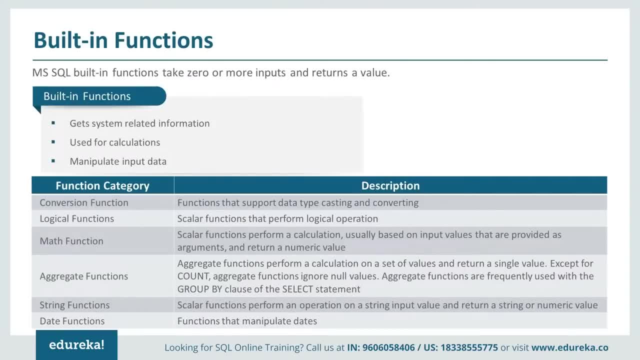 that these are the various categories. again, conversion functions That support data type casting and converting. logical functions are scalar functions that perform logical operations. These are kind of similar to the math functions are again the scalar functions which performs calculations, usually based on the input values that I provided as an argument. 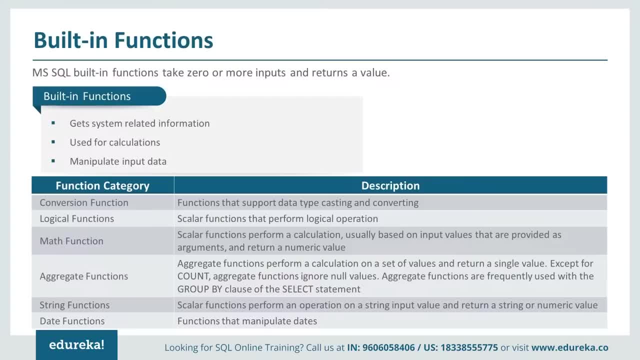 and most of the times the returns are numeric value. aggregate functions, As I mentioned, we use some, we use average, we use maximum of values. So aggregate functions basically perform a calculation on a set of values and they return a single value, except for the count. 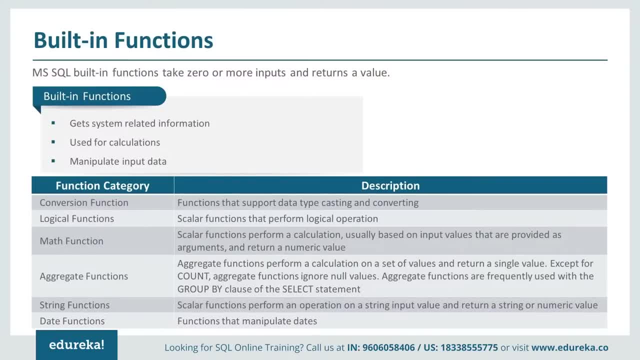 So count is also an aggregate functions other than count. all other aggregate functions ignore null values in the objective. We saw that we are going to discuss about the group by and having clause, So aggregate functions are frequently used with a group by clause of the select statement. 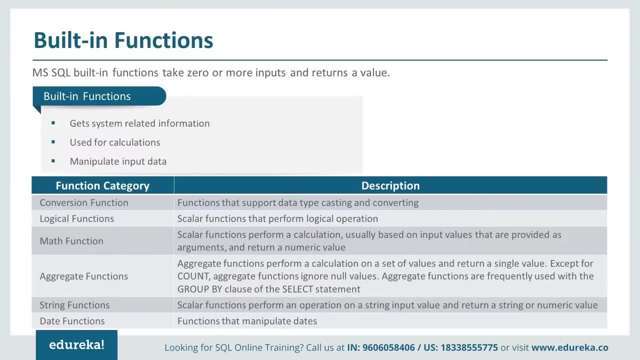 or we can say that we use group by clause only with the aggregate functions or group functions. Some people refers aggregate functions as a group functions, So don't get confused, They are one and the same thing. string functions again are scalar functions and the perform and operations 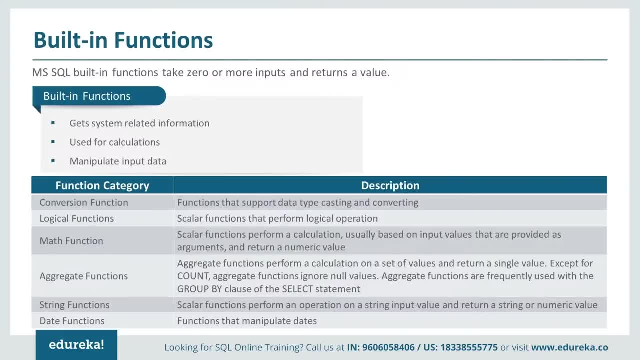 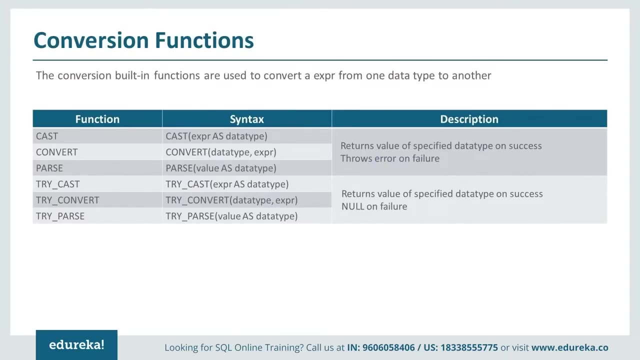 on a string input value and return strings or numerical value, based upon the kind of functions which we are using. date function: straightforward: It manipulates the dates. So let's start with the conversion functions, as the name itself suggests that it. these functions helps us to convert an expressions. 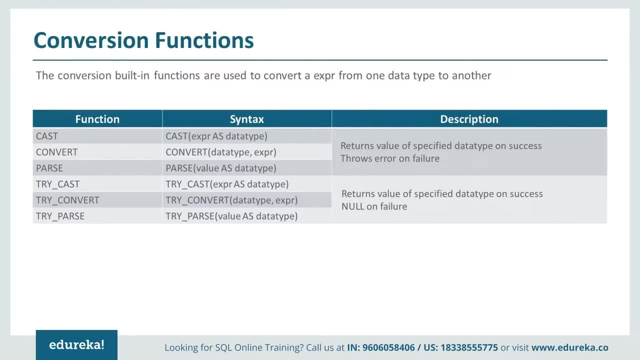 or a value from one data type to another. So we have three commonly used conversion functions- cast, convert and pass- and in the bottom three can, you can see that we have try and the score cast, We have try and the score convert and we have try and the score pass. 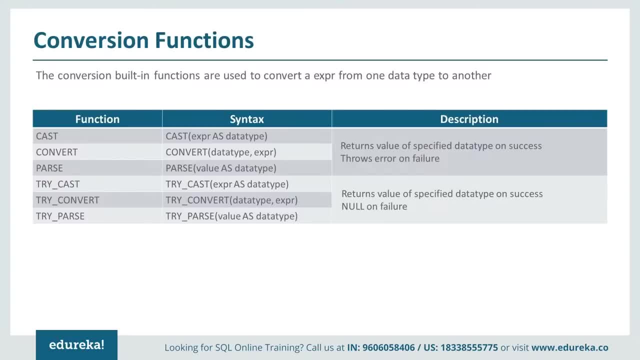 So the top three and bottom three. they give the same results. They work in the similar fashions. the only difference here is that the top three functions returns value of specified data type and, on success, throw errors on failure, Whereas the bottom three, they give the null values on failure. 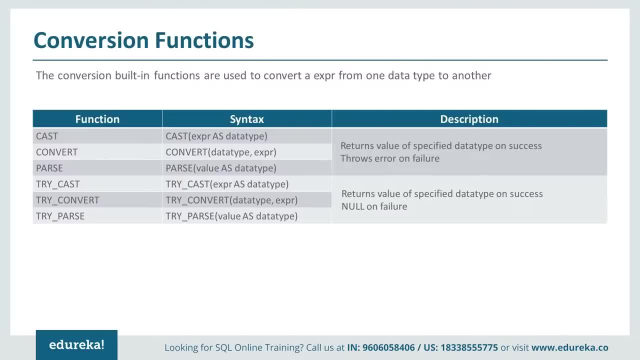 So we can relate this try as like how we have the try catch block in other programming language to handle the exception. same way We use try cast if you want to get the null values if something wrong happened while calculating the expressions or while fetching the results. same is the case with try convert. 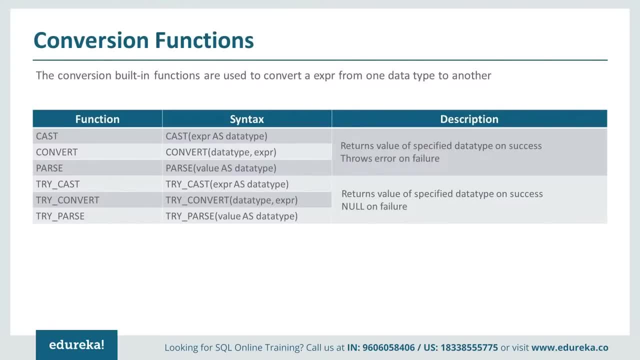 and try pass. but if any error happen while using cast, convert and pass will get an exceptions- I will get an error, whereas error can be handled by converting it to the null values If we use try cast, try convert and try pass. So, as you can see on the slide, 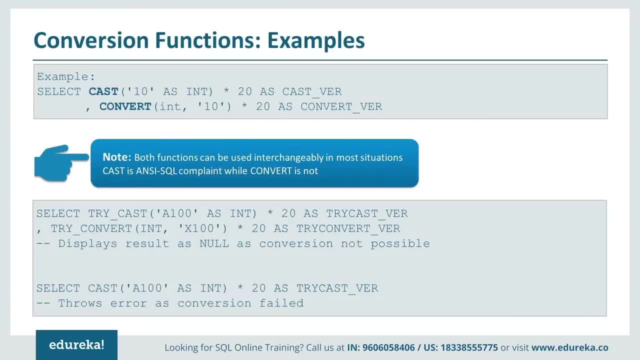 we are converting the value 10 as int and we are multiplying by 20. again we are converting int, 10 to int and again we are doing a multiplication of the value after conversion with 20.. So that what is the difference between cast and convert? 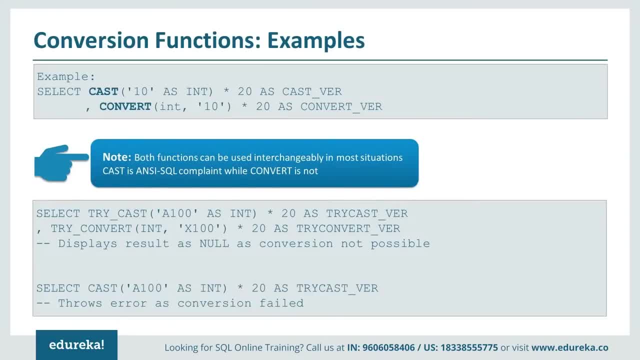 because the end result is almost similar, So both function can be used interchangeably in most of the situations. The only difference is that cast is NC SQL compliant- It follows American National Standard Institute- Whereas convert does not follow any such compliancy. 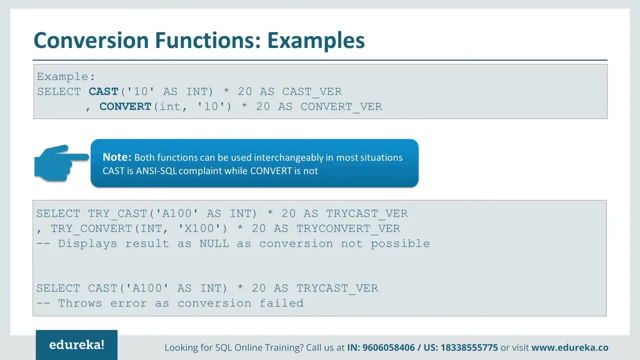 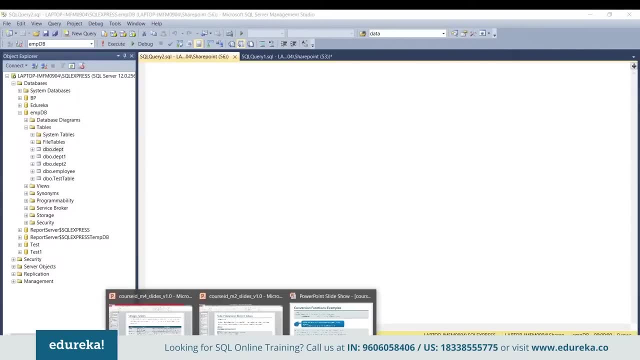 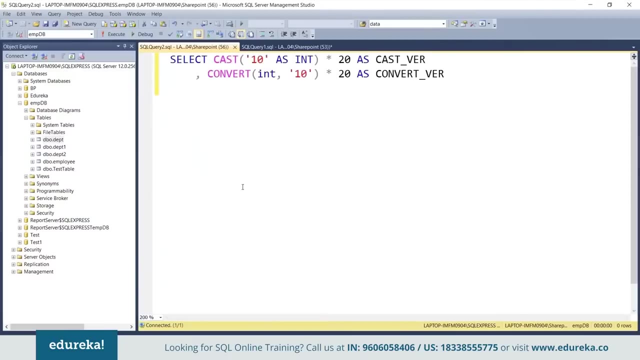 Let's see an example of these basic operation. So I'll open management studio of SQL. Let's open a new query and let me copy the example. So let me copy both examples and increase the font size. So if I'll execute, I'm getting this result. 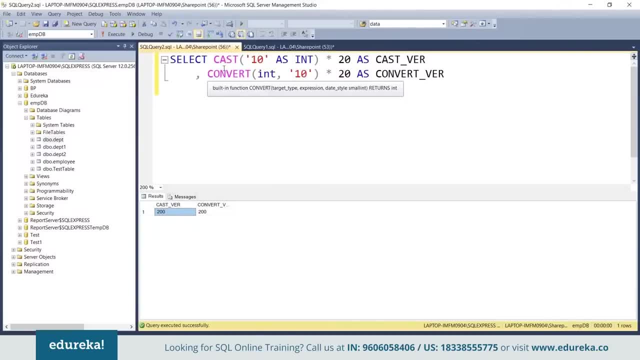 since we are converting 10 as int. and again, if you'll see, the result of cast function and convert functions is exactly similar. only difference is in the syntax. the syntax of convert function is different from cast function. So one important point I just want to mention here is: 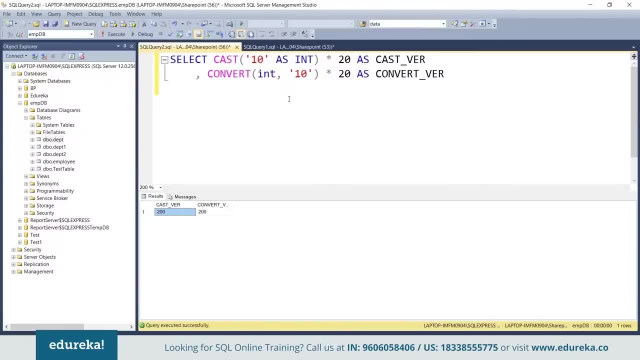 that in select operation we can use mathematical operators, like we can use plus, minus, divide and multiplications. So here, after converting 10 into int, we are multiplying it with 20 to get the end result, And this is the alias which we discuss in module 2.. 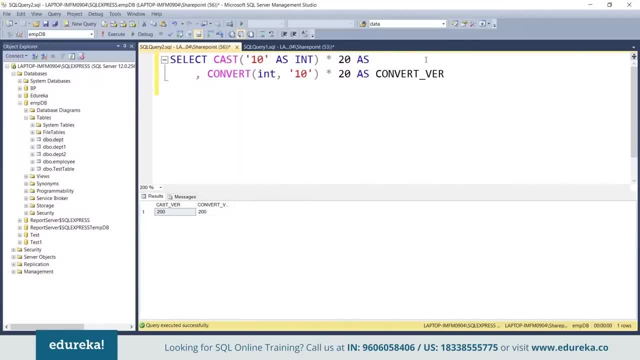 So we can change it. We can change it to any value. We can change it. Let's say I'm writing it to cast result and I can change it to convert result and file executed, I'll get the same results: cast results and convert result. here are alias: 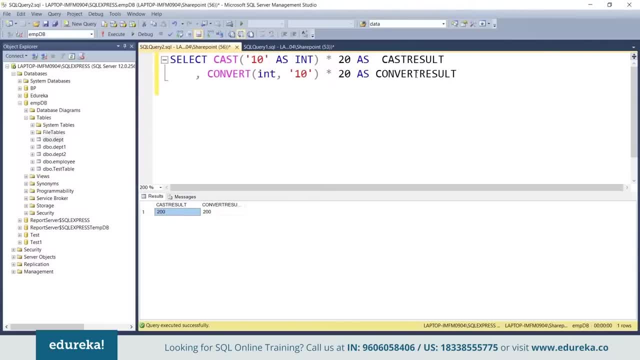 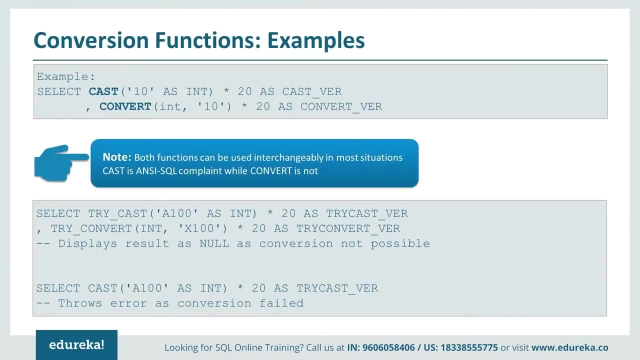 These are the alias For the columns. in the module 3 we saw that we use alias for the table. So let's see that if there's an issue while casting or converting a desired value, then we'll get an error when we'll use cast and convert, but we'll get a null value. 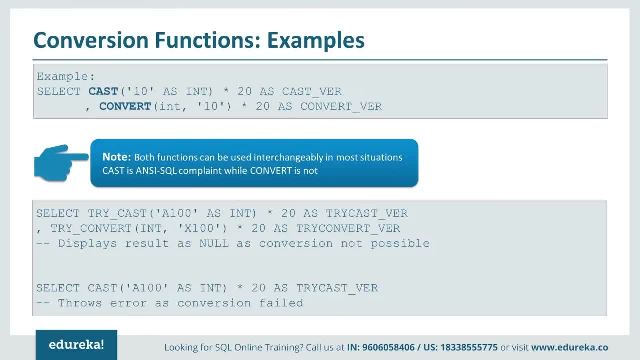 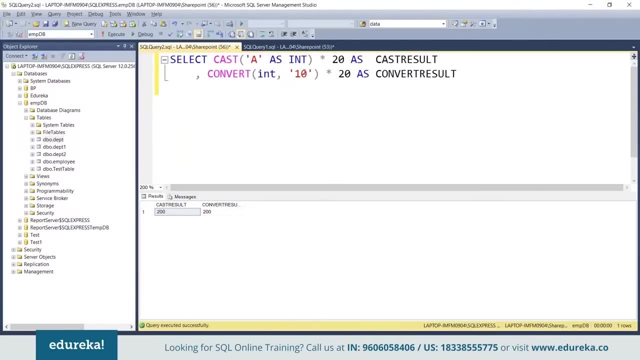 when we'll use try cast and try convert. Let's verify this using an example. So I'm trying to convert character into int, So we'll get an error. that conversion failed when converting the worker value A to data type int. Now let's use try cast. 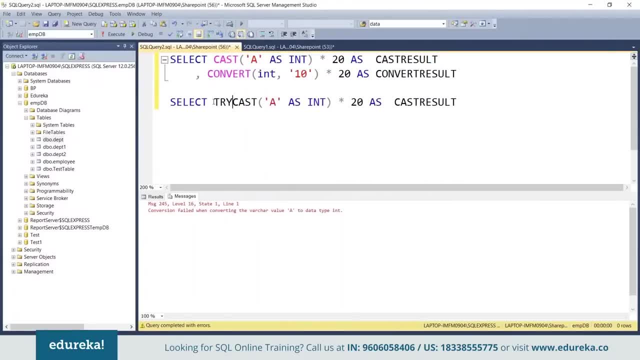 So I'll copy this statement. So let's assume I use try convert and if I'll try to convert a value which is not numeric and if I'll execute it, we'll get the incorrect syntax near the word try convert. Sorry, I forgot to write select. 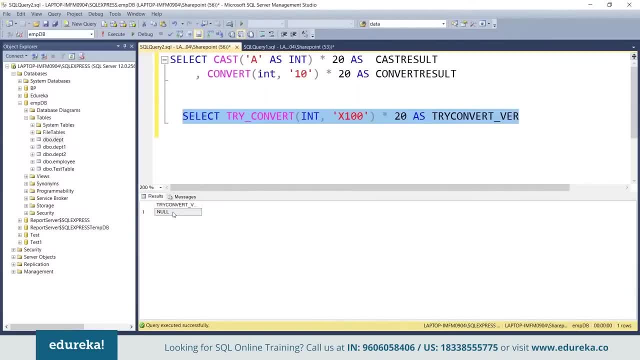 And if I'll execute it now, we'll get null value. So, instead of error, we are getting a null value if we use try convert or try cast. So, based upon the business requirement will choose either the try convert or convert. Let's move to the next function. 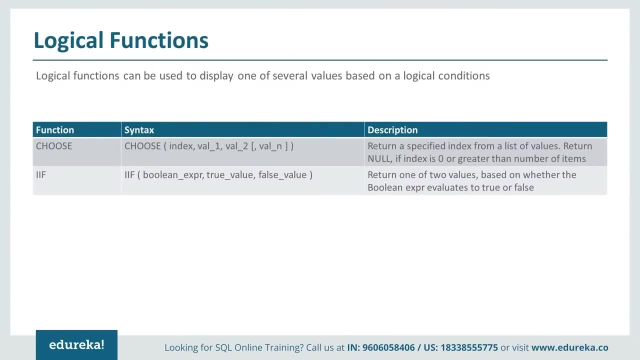 Let's discuss about the logical functions. So we have two logical function choose and if. Logical functions can be used to display one of the several values based on a logical conditions. So, as we have discussed, we have two logical function- choose and if Choose returns a specified index from a list of values. 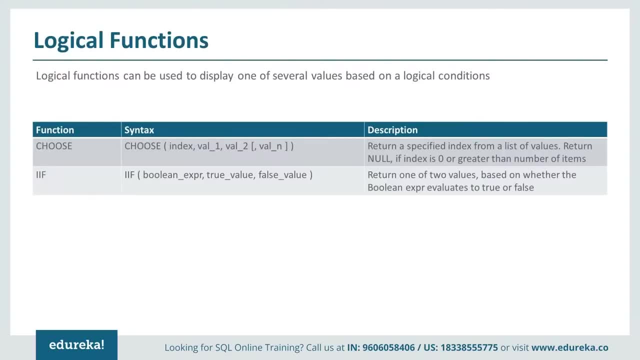 and returns null if the index is zero or greater than the number of items. Or we can say that the choose basically act as an index into an error When an array is composed of the argument that follow the index argument. So, as you can see in syntax, 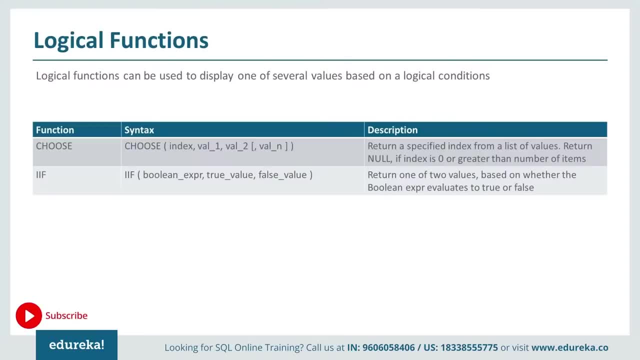 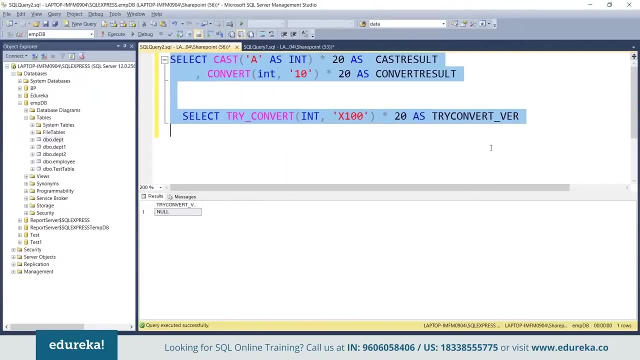 we have the choose keyword and in the parenthesis we have index. So this is the index which we have to define that what value we want to return, and this value 1, value 2 and we can have up to value n. So let's understand choose by an example. 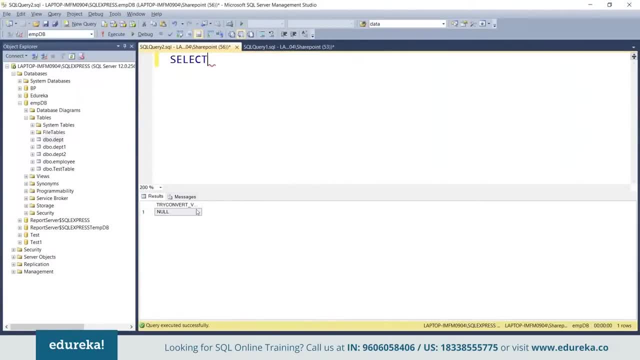 So let me write one example So that will help us to understand: Choose keywords and all these functions are basically. can you see the color code? for the keywords? We basically have blue colors, but for these functions we have pink color. So we'll define three. 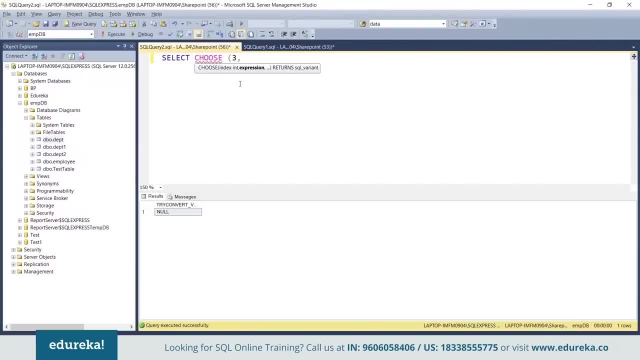 This is the index and then it's followed by the various values. Let's say, I have test as a one value. I have just as another value, third value: I'll be having rest. So if I'll execute this statement, I should get the value rest, because this index does not start with zero. 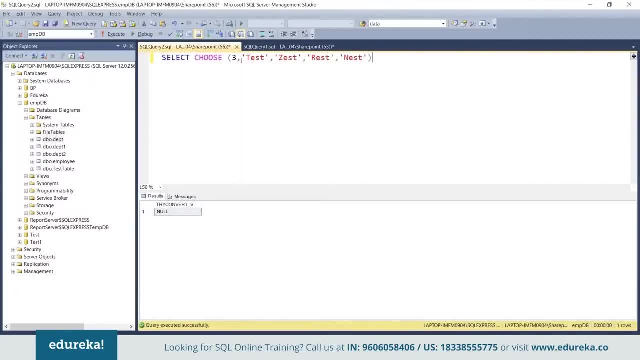 Please note it down in the choose a function. The index start from one. This is one base index, not the zero base index like we have in most programming languages. So if I'll execute this statement, I'll get rest, because we are instructing the SQL Server. 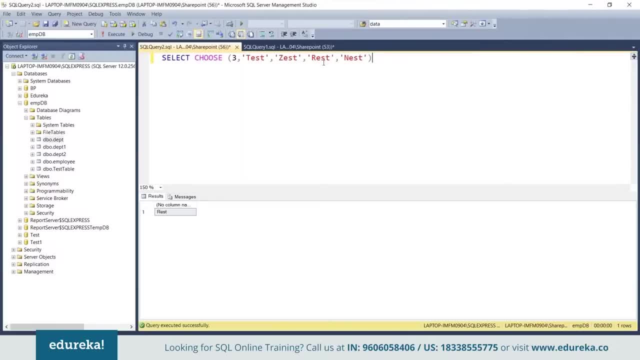 that we want the third value after the various values available. The choose function basically gives an error If you try to use the index as the value zero, or we'll try to provide the index which is outside this range. So let's understand it by an example. 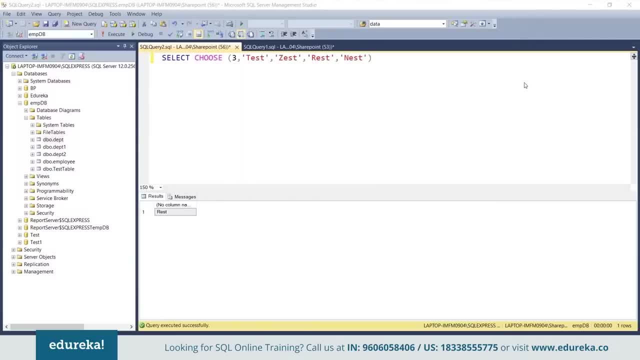 So if I provide a index zero, If I execute this, I'll get a null value. or if I provide index which is outside the bound of this array- when I say bound, if it is more than the number of values which we are trying to select from- then again, 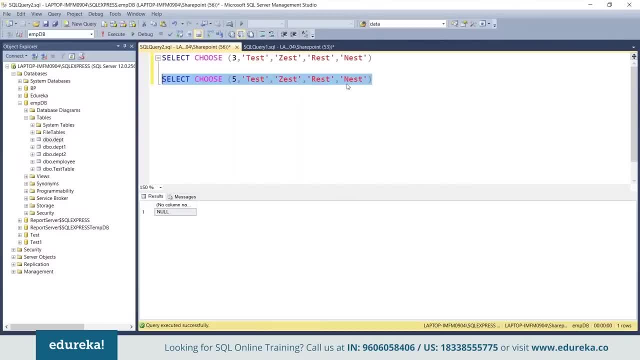 it will returns a null value. So this is. there are only four values here and I'm giving index five. So since there's no value at the If the next, it will return a null. it won't give us zero. So choose functions helps us to select from a given range. 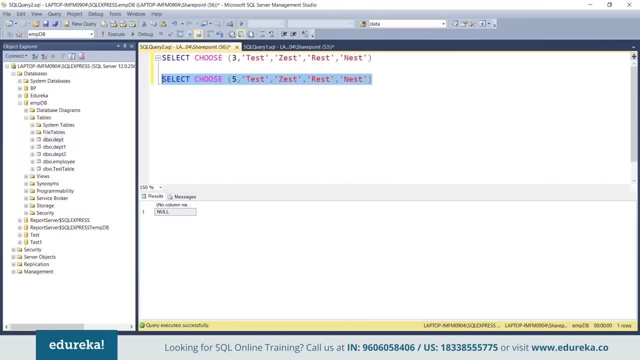 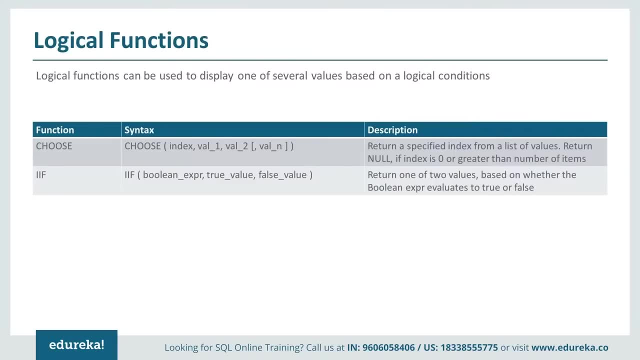 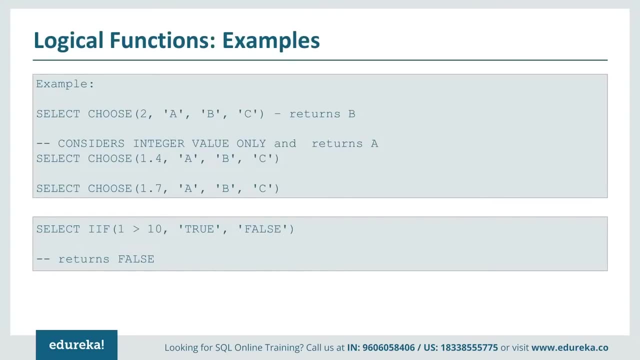 of values, like how we used to fetch the values from an array. So let's discuss the other logical function. So here, before we discuss the if, let's see these examples as well. So in the first example we are using select, choose and we are giving index to a, B and C. 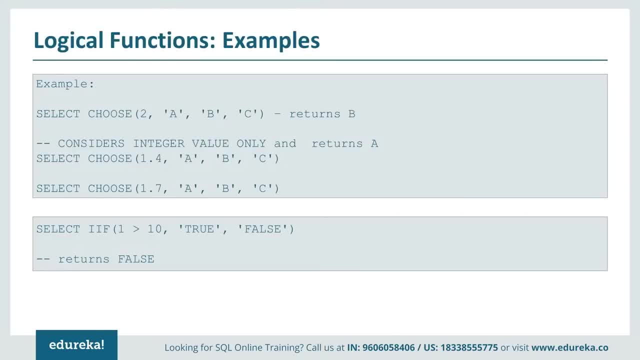 These are the three values. So this will the first First example will return the value B in the result set, because we'll count from the index one. As I mentioned, that choose is based on one index and not the zero index. So let's take the case of the second example here. 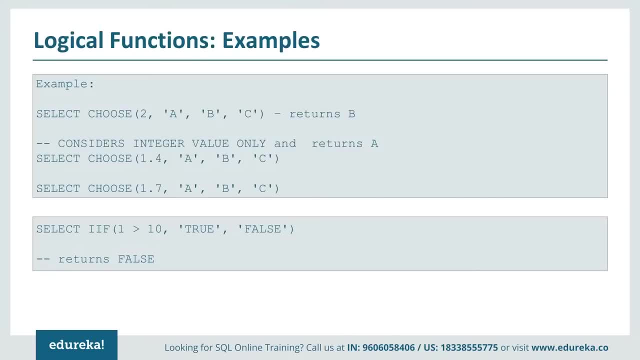 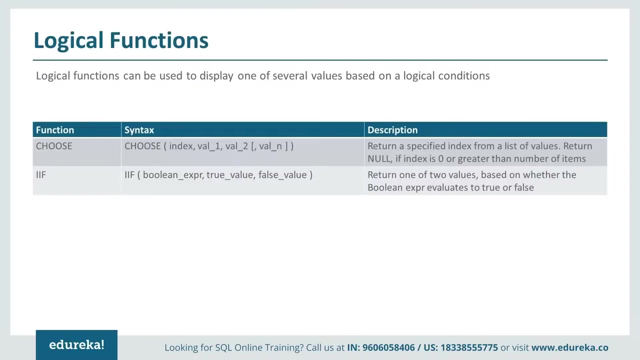 We have not provided an integer. We provide a fraction, value 1.4.. So choose only consider the integer value. in both the cases It will return a, as in the result set. So now let's discuss the other logical function. If so, let's focus on the syntax first. 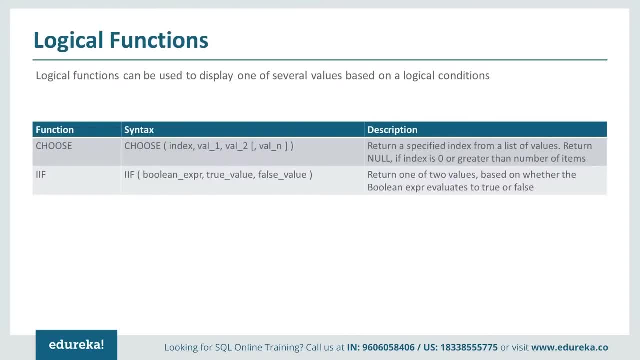 So it's followed by if keyword and then we have a Boolean expression and then true values and false values. So when we execute this function it returns one of the two values. either it will turn true value or either it will return false value. So the output- whether it is a true 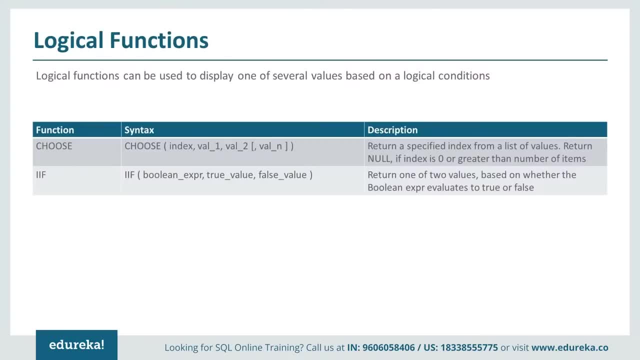 or false depend upon the evaluation of Boolean expressions, which will provide in the if function. So if is a shorthand way of writing a case expression. it evaluates the Boolean expression pass as the first argument and then returns either of the two argument based on the results of the evaluation. 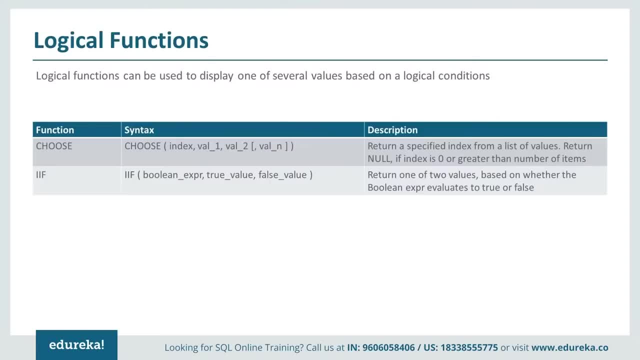 So we can even provide the nesting in the if functions. The nesting should be up to 10 level, similar to the nesting which we can have in the case expression, as it is almost similar to the case expression. So let's see or discuss the example of if logical function. 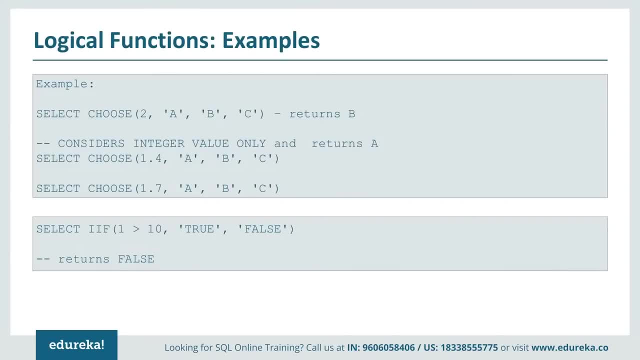 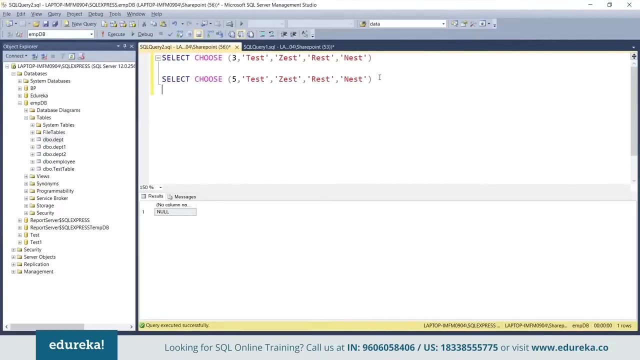 So in this case it will return false, because this Boolean expressions is not satisfying. One is not greater than 10.. So it will fetch the result false in the result set. Let's execute this example in management studio: Write if, if then you have to write the Boolean expression. 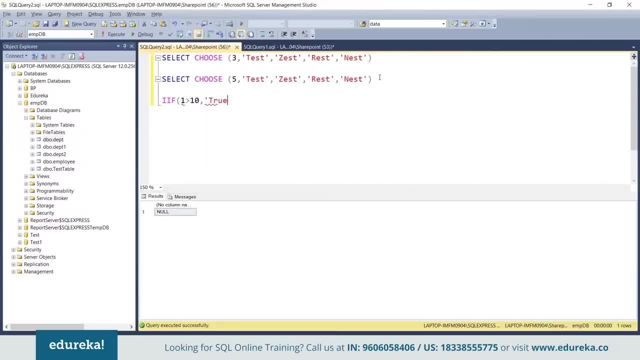 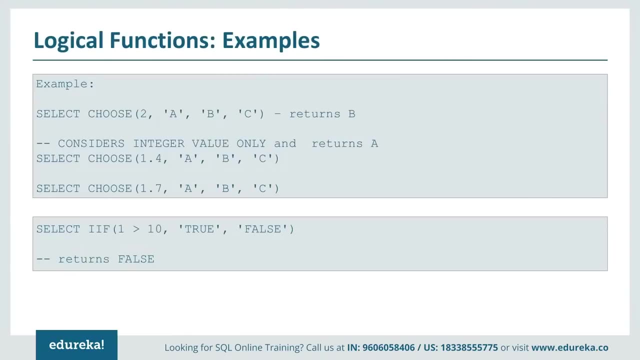 Then any value. let's say I'm just writing true- And the next value if it turns out to be false. Let's see example. The example seems to be right. Let me copy from here. Okay, so we forget to add the select keywords. 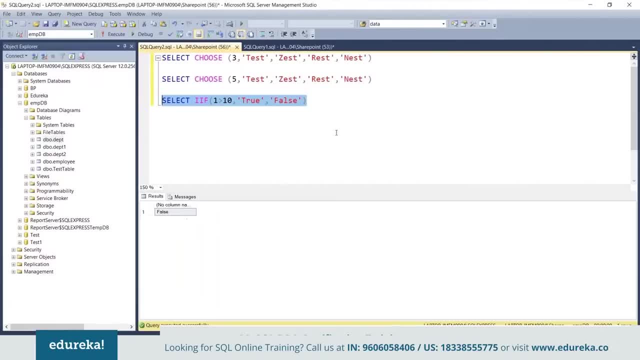 Sorry about that, And if I'll execute it will return the false. So since there is no header for the column name, we can provide an alias as well. If I'll make this statement as true. if I felt reverse the values here, Then I will get true as an output in my result set. 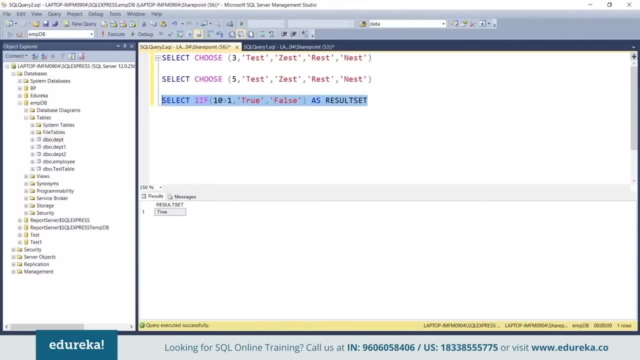 As I mentioned, if works like a case expression and we can nest it, and nesting can be allowed up to 10 level. So this is all about logical functions. So let's continue with other categories of functions. So let's discuss about the math functions. 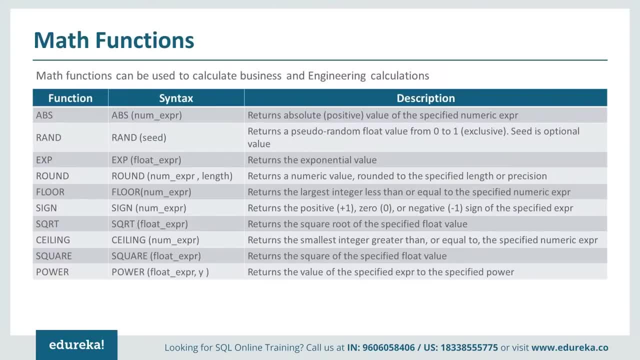 So math functions can be used to calculate business and engineering calculations. So these are various self-explanatory and we must have used these functions during our engineering classes or any other classes where you do any engineering calculation, For example when we convert it to an absolute positive value. 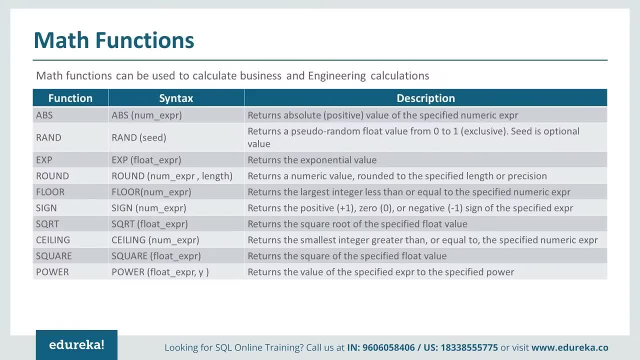 then we use ABS functions. If you want to generate a pseudo random float values from 0 to 1, then we use rank function. seed is an optional value here. If you want to return an exponential value, then we use exp function in most of the mathematical values. 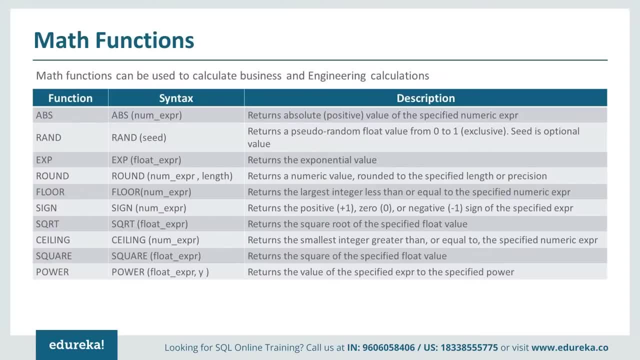 We need to round up the values. when the values are of decimal, then we use round functions, So round returns and numerical value rounded to a specific length of positions that we need to provide in the functions floor. provides or it returns the largest integer less than 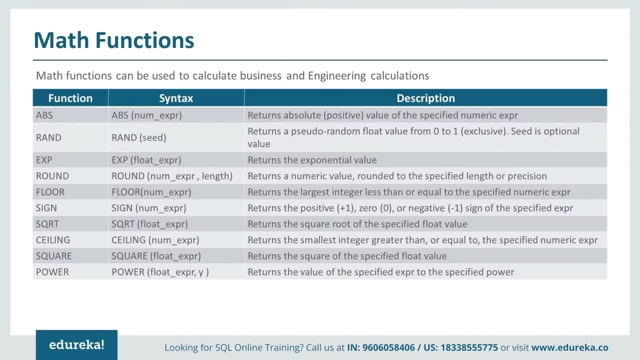 or equals to the specified numerical expressions. then we have square root. square root returns the square root of the specified float value ceiling is just opposite of the flow and it returns the smallest integer greater than or equal to the specified numeric expression. square again, and as we know, the square square of two is four. 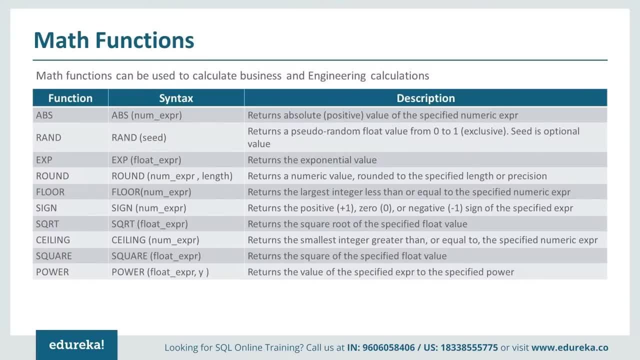 So, like we use the square functions to calculate the square of the specified float value, power power basically returns the value of the specified expression to the specified power. So these are the standard mathematical functions. We have used these functions, So here we can see a consolidated examples of all mathematical functions. 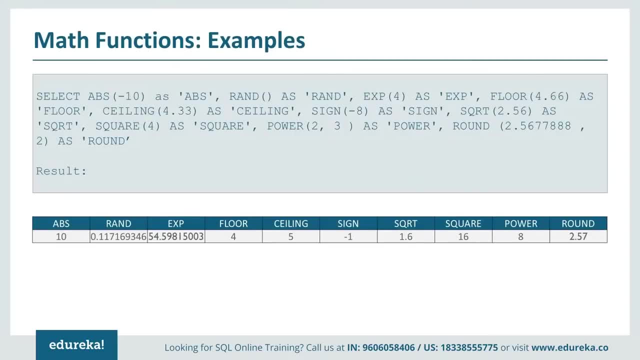 So in the first example we see select ABS minus 10. So here we are using absolute value, So it is converting the negative values to the positive value, and all these keywords are we are using as an alien, So we are using ABS as an alias. 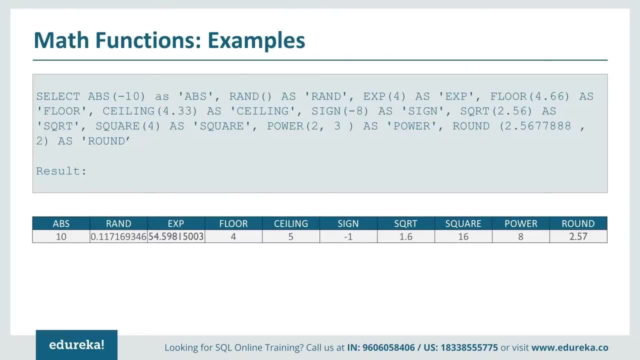 for the first column, rent, as we discuss, rent is basically helps us to get any random values We can provide the seed. seed is optional when we use this functions. So, as you can see, we are getting a random value here. exp for it basically helps us to get the exponential value flow. 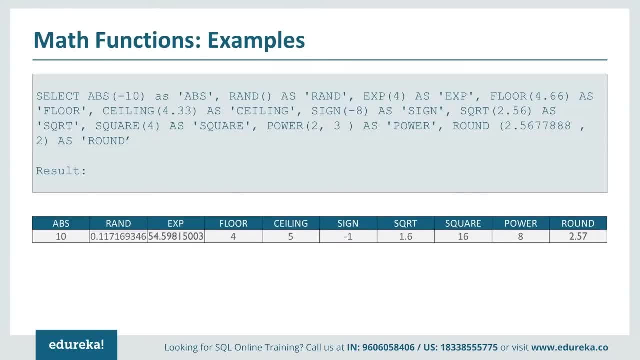 We use flow, So it will get the value. 4.66 will get the value for here, So flow we will get the value less than the nearest integer in the ceiling will get the values greater than the nearest integer. So if I'll use flow, 4.66,. 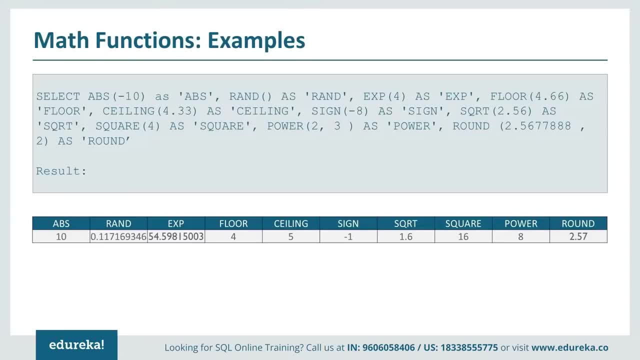 I'm getting the value for when I'm using ceiling. I'm getting value 5 here, square root. the square root of 2.56 is 1.6.. So this is the value we are getting. square is just opposed to the square root. 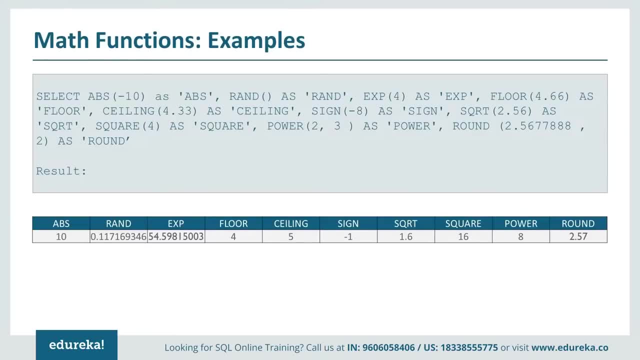 So we'll get the square of a digit which will provide in the parenthesis. So we have provided a value for. so we are getting 16 as its result. power 2, 3.. So we are basically giving power 3. the base value here is the 2, and 3 is its exponential value to the power. 3 will get 8.. 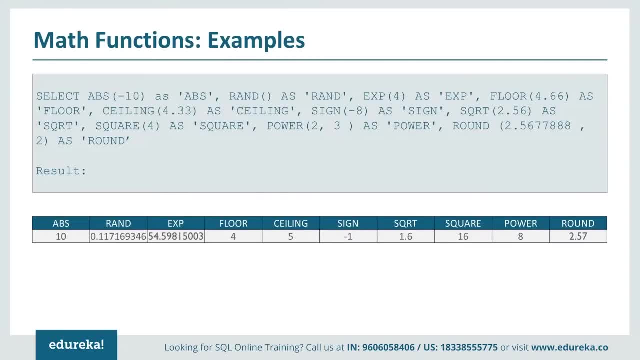 It's in Statesman. If you want to expand this, it's 2 into 2 into 2.. So we are getting 8 as its results around. function is basically is to round the values and we are using 2 as a precision value. 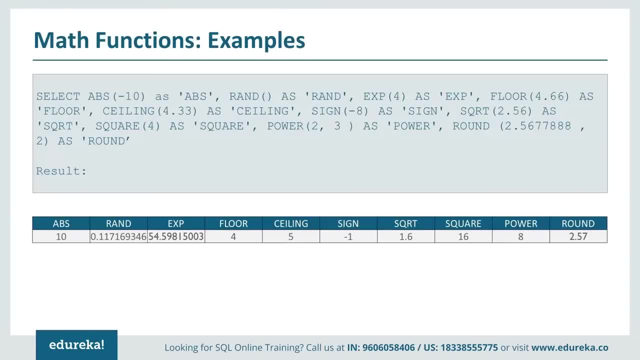 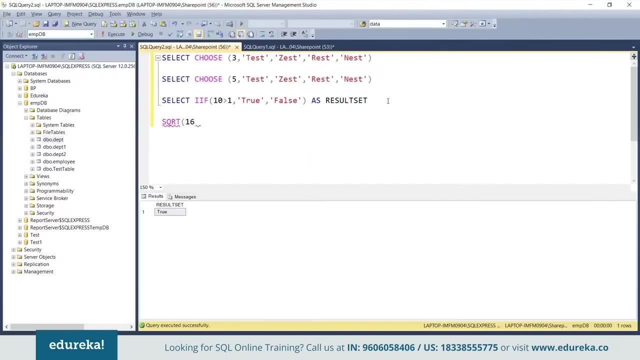 So we have provided. so it is basically rounded up to 2.57.. So let's execute few of the examples in management studio. for better clarity, Let's use the square Function and square root function first, So square root of 16, and always use the select statement, or else will get an error. 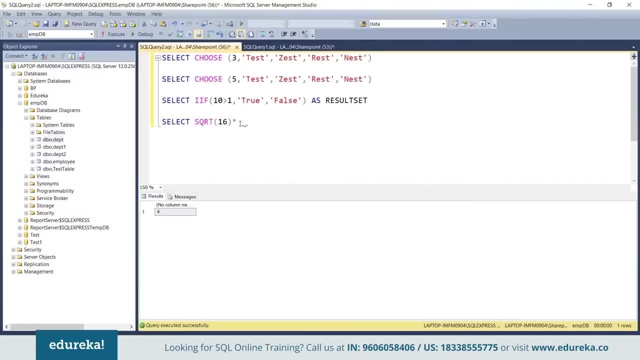 So I can even do like multiplications of various- I can use this mathematical functions and then I can multiply it, or I can use other operators like plus, minus. So if I like to do this, so what I'm doing is I'm taking the square root of 16, that will afford taking square 4, that is, 16.. 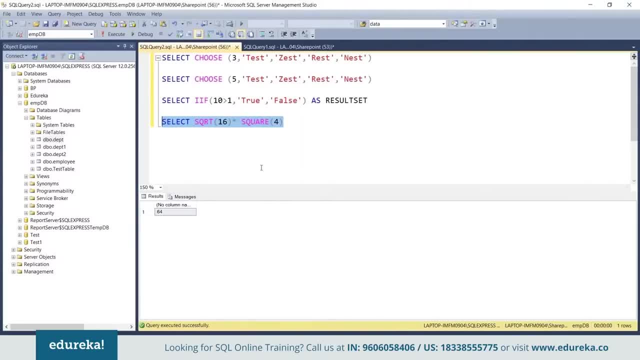 So end result should be 64. Yep, So we get the result. as you can see, guys, when we don't give the name of the column, the header is blank. So it is good practice to provide the alias. As of now, I'm giving a standard keyword, result set. if I'll execute it now, 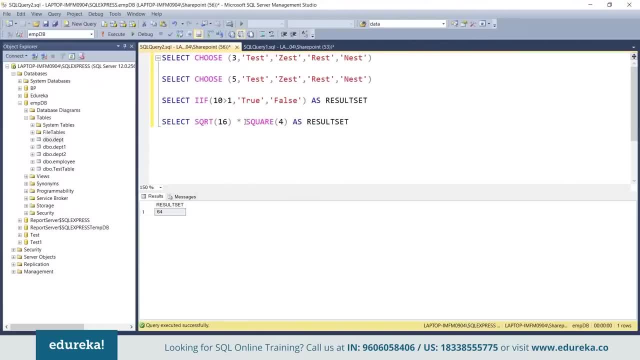 I'll get 64 is its value. I can even use other mathematical operator, I can use plus to provide the sum of these two values: 16 plus 4, 20.. So we'll get 20 in the result sets. I'm getting minus 12 its value and let's see, can be clubbed functions here. 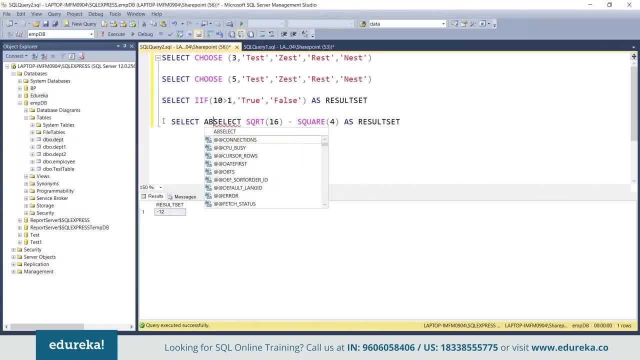 So let me write select and if I use apps function here. So now I should Be getting plus 12 because I'm using absolute function. So it will convert the negative value into positive values. So we can use, we can club, we can nest the functions. 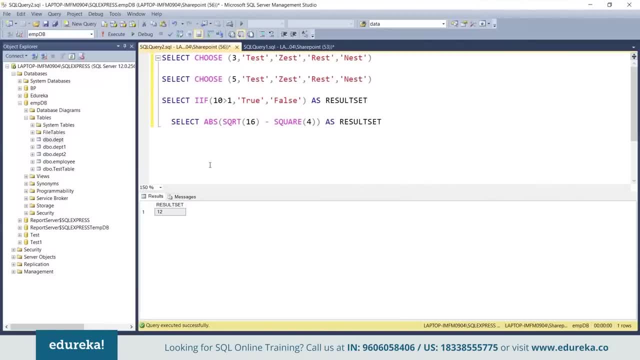 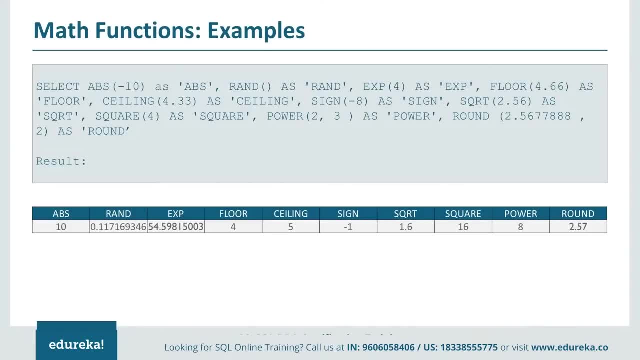 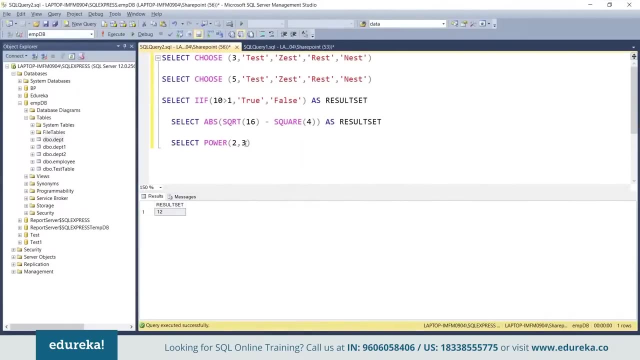 So here in the apps functions- I'm using a security functions and square functions- We can play around with these functions as per our business requirement. Let's use an example of power. Let's let's use the base value as 2 and 2 to power 4.. 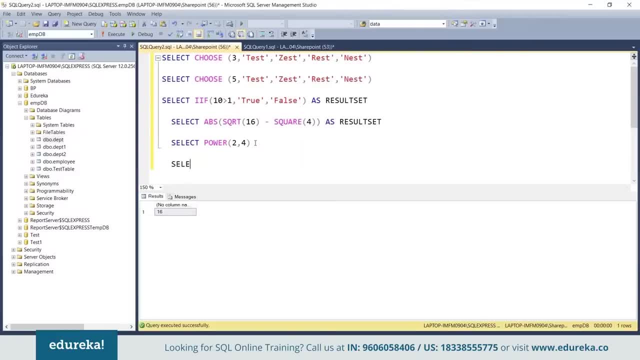 So the result will be 16.. So this is equivalent to: Sorry, If I'll expand this power, 2 is the base and 4 is the exponential, So I'll get the same results at 16.. So this is all about the maths functions. 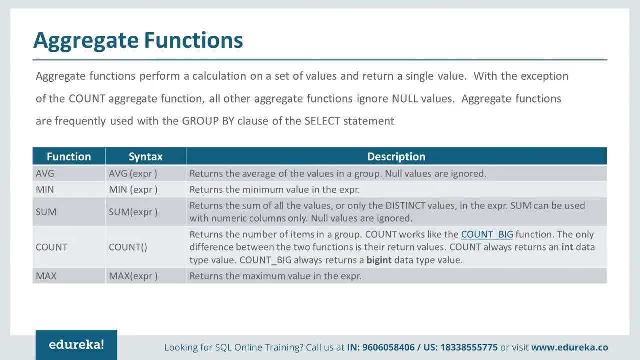 Let's move to another category: Dignose null values. aggregate functions are frequently used with the group by clause and for a filtering like. we used to filter the data using where clause. So if you're using group by clause, then we use having keyboard to filter the result set. 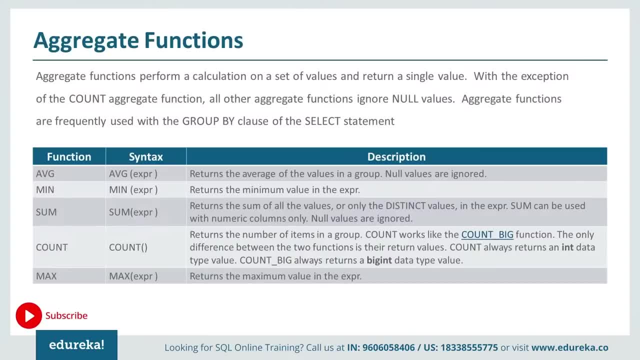 So we have a following aggregate functions: We have average, main sum, count and Max. So let's start with average function first. So average returns The average of the values in a group. as we discussed, null values are ignored. So let's take an example of average function. 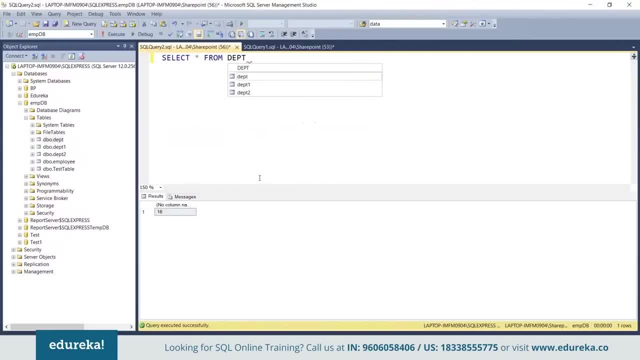 First let me fetch the values from Department table. Okay, so I can use the average functions on department number column. So I can write: select Average. Write the column number From Department. If I like to do this, I'll get the average of the values. 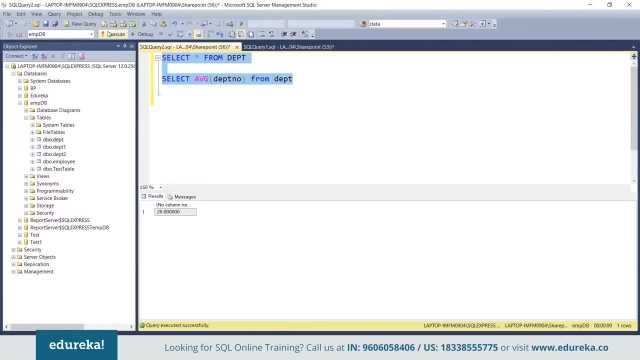 So let me execute both the queries in funko So we can compare the results. So 25 is the average of 40 plus 30 plus 2010 divided by 4.. So we can use average functions with the distinct keyword. We discuss about the distinct keyword in module 2.. 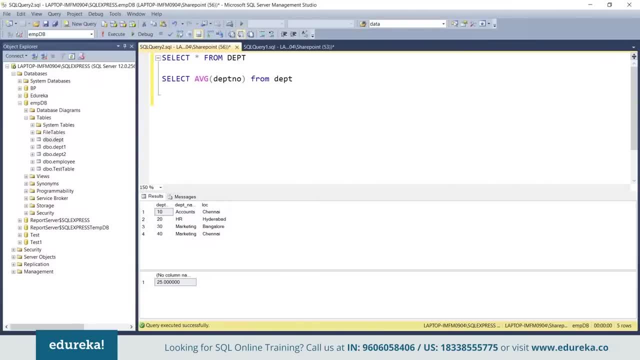 So distinct keyword helps us to fetch the unique records. So if you want to find the average of the distinct values, then we provide the distinct keyword before the column name. So let's take another example of the average function. Let me get the results from employee table. 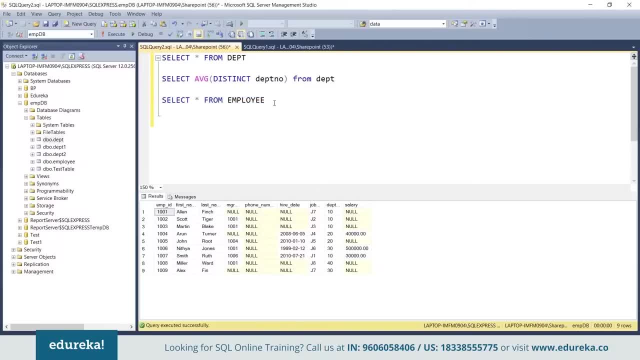 So, as we discussed that, average functions ignores null values. So if I try to get the average of salaries, so we have only three rows where the salaries present rest. All the values are null. Let's see What is the result. Select. 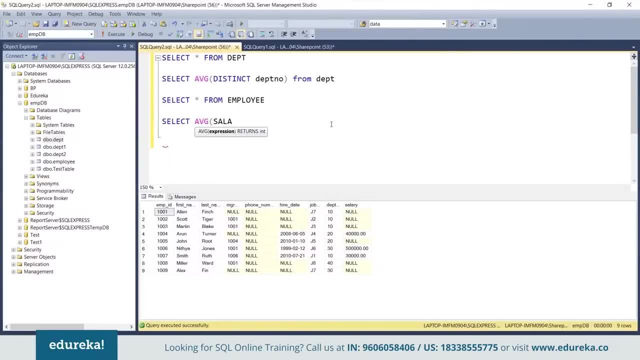 Average Provide the name of the column From employee. So this is the average. Let me execute both the statement in funko, Like I did earlier. So you're getting the average of this. So we can use average with the distinct keywords. 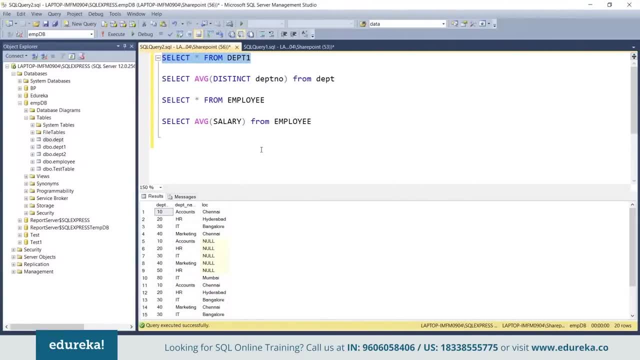 If you want to fetch the results, Okay, let's see whether we can apply the distinct here. So in the department one table we have the repeated values for the department number. So if I want to ignore the repeated or redundant data or the duplicate data, 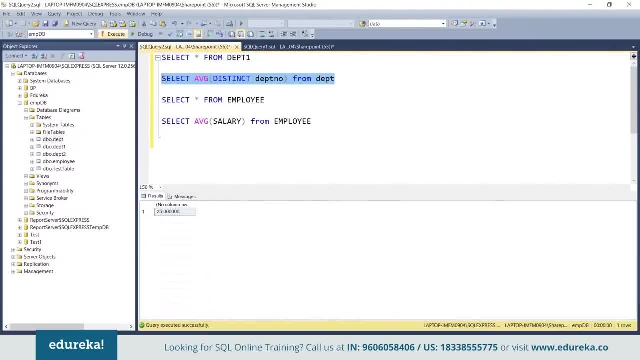 then I can use The distinct keyword. So if I execute it now, I'll get the average as 25.. But if I'll remove the distinct keyword, The results that will be different. Sorry, my bad, I'm using Department column. 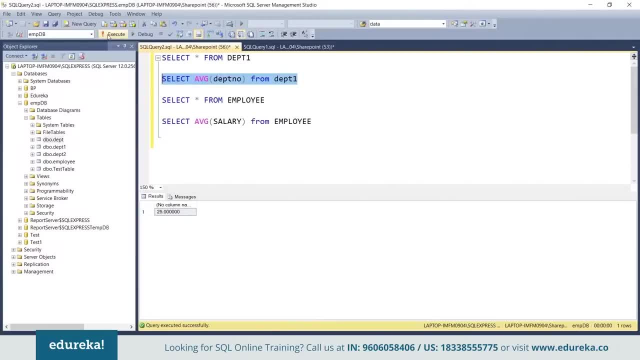 I have to change it to Department one. So let's first see the results. that, without using the distinct keyword to results, is 30. Now I'll use the keyword distinct. The value Is different because I'm just taking the unique values for my result set. 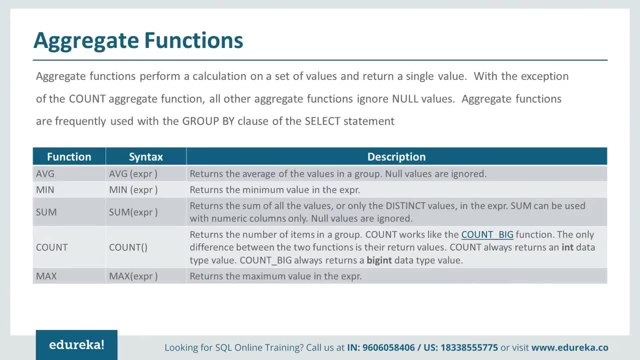 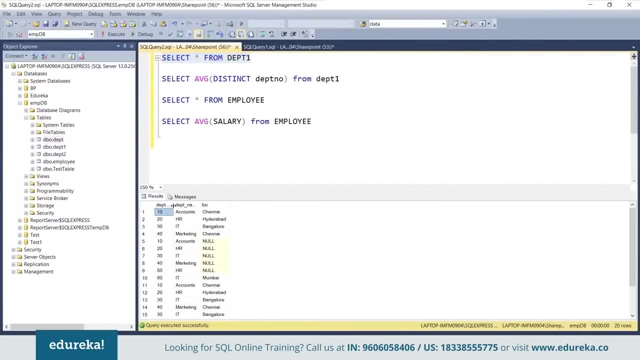 So let's move to another aggregate function. Let's discuss the main function. similar to average, min Also ignores the null value and it returns the minimum value in the expression. So if I'll see the values in the department one table and if I'll try to find the lowest value of the department number, 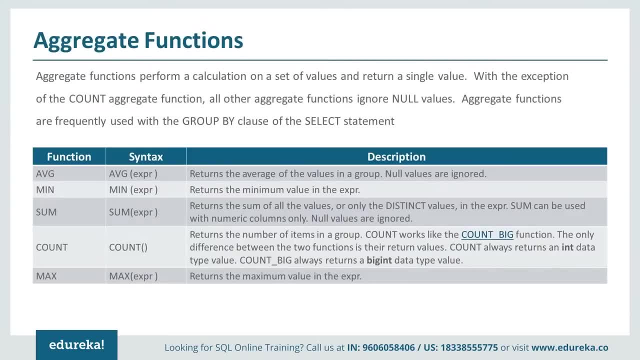 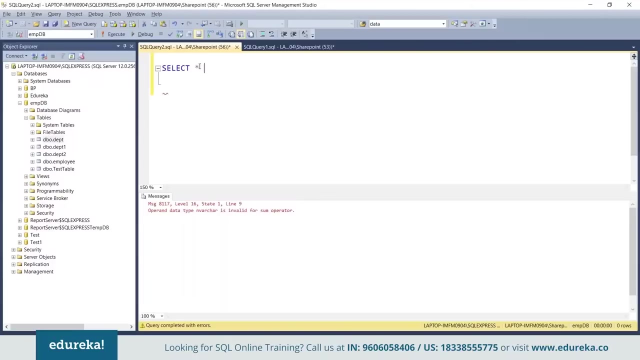 then I have to use the main function. Okay. so out of all the aggregate functions, count is only one which considers, which takes into account the null values as well. So let's see the example of count. Let's move to management studio. So I'll be using employee table, because we have a lot of null values. 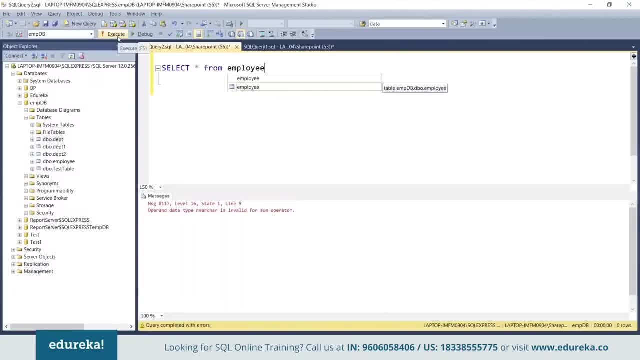 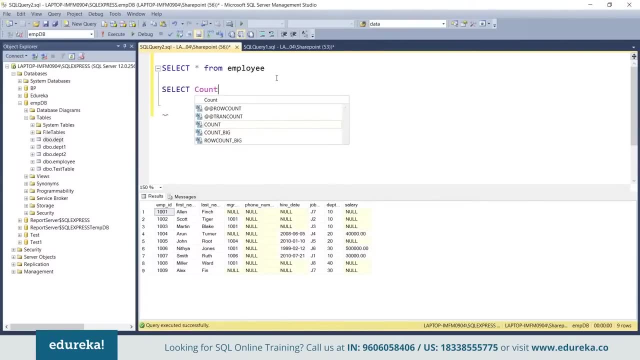 in those. I'll execute this. So let's take the count of the salary column Select Count. Oh, I have to write the column name Employee. So if I'll execute I'll get three results. But if I'll execute, 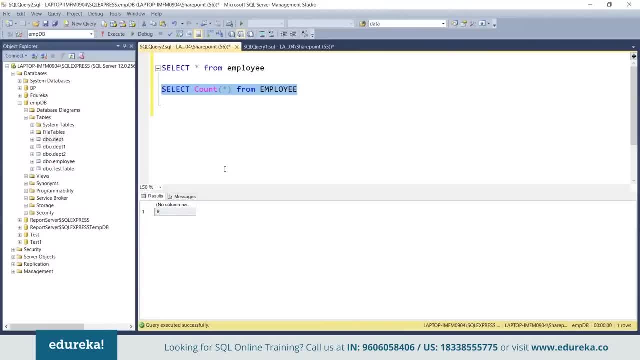 Star, I'll get nine columns. So even we can use the distinct operation here In the count function. So count, basically fetch the count of rows from a table. So let's move to another aggregate function. We have Max. So Max is exactly opposite of min. 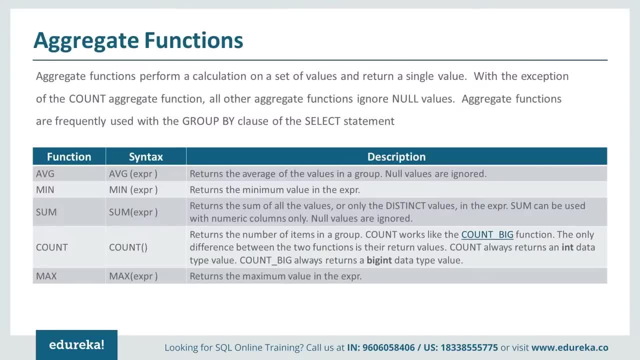 We have already shown example of minimum, So Max, we can use it for numeric as well as with the character data type. If you use for the character data type, it will show the maximum value in the sorting order. If you use with the numeric, then of course it will show the maximum. 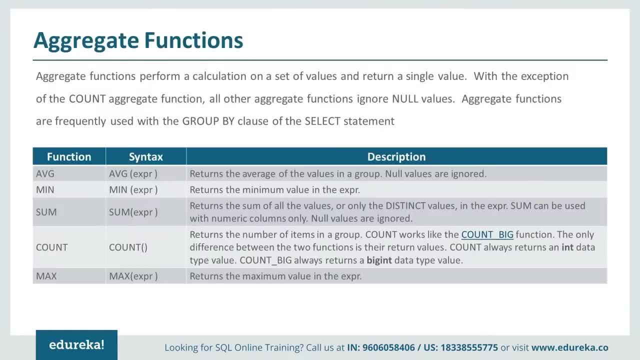 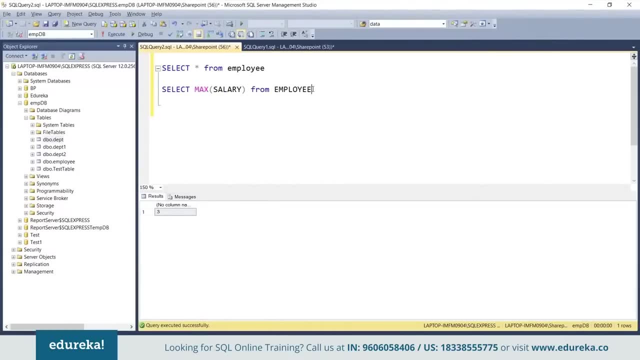 of the value, though Let's see an example of Max as well. So if I use Max, We're trying to find the maximum salary from employee table. So this is the maximum salary And if I'll try to find The location, 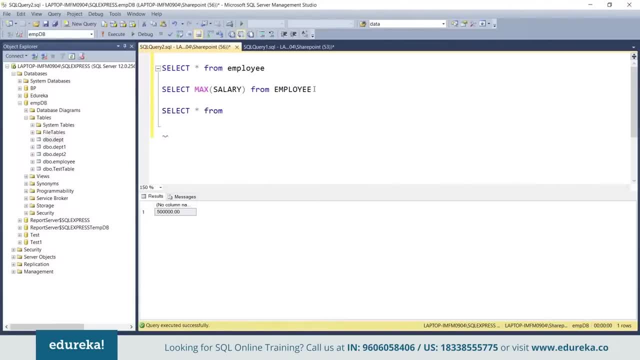 Let me first show you the various location from the department table. So, as per the sorting order, we should get Hyderabad if we'll use Max for this column. So let me write the query. Select Max LOC from department table. So let me write the query. 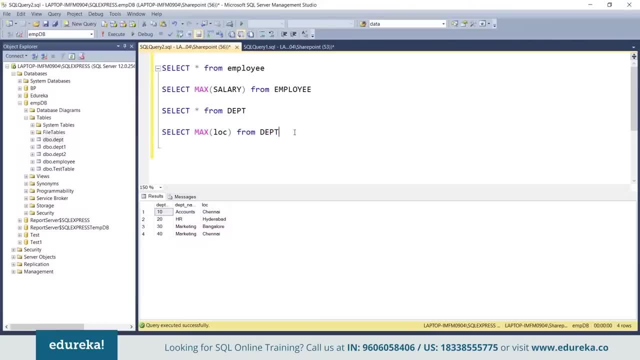 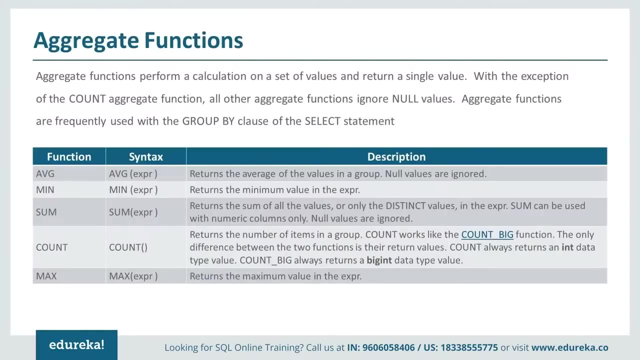 Select Department table And we can provide an alias as location. So I'll get Hyderabad in my result set. So we have discussed all aggregate functions. So the common aggregate functions are average. If you get the average of values min, as the name suggests. 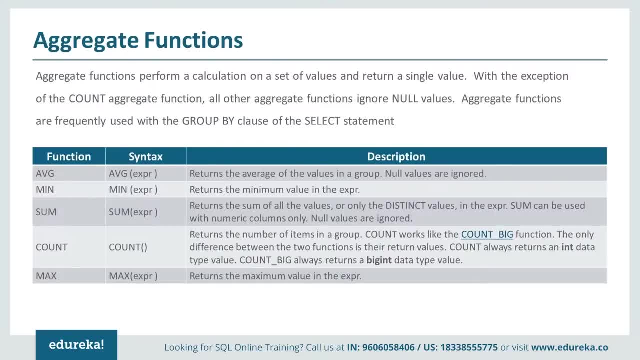 the minimum value in the expression. sum helps us in finding of the total for a column. Sum only accepts the numeric value. Count returns the number of items or rows in a group or in a table. Max returns the maximum value in the expression. So let's move to other category of functions. 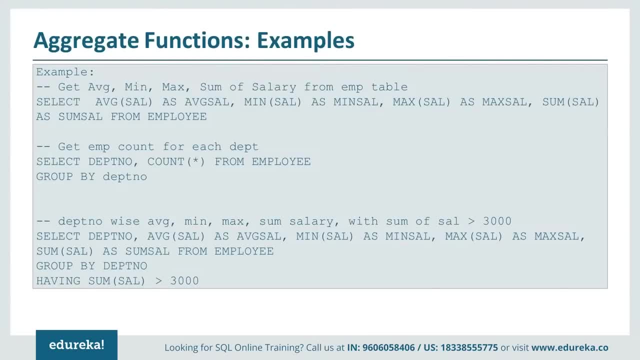 So these are the various examples. before move to other functions, Let's see the examples here. So in one example I've shown all the aggregate functions. So we can use multiple aggregate functions in the single statement, a single select statement. So in the single select statement. 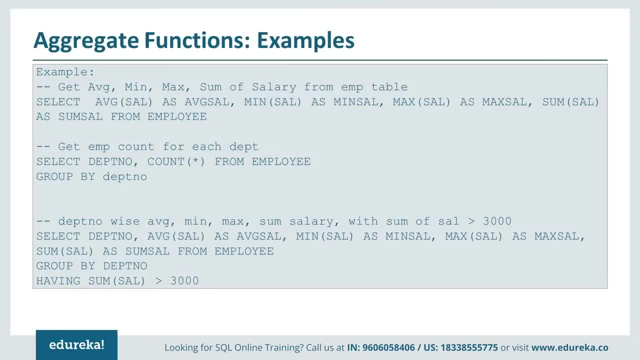 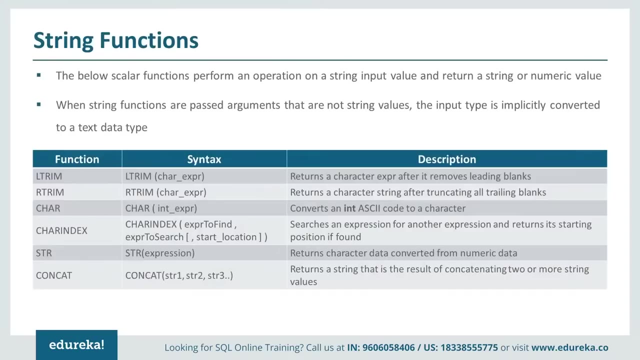 I've used average of salary, minimum of salary, maximum of salary and sum of salary from employee table. Second example is for the count functions. So we will discuss about the group functions and having functions once we are done with most of the out-of-box functions. 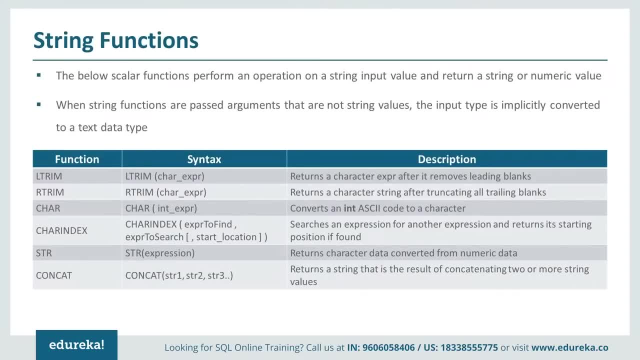 Then we have string functions. String functions are again scalar functions and they perform an operations on a string input value and the return a string or numeric value, based upon the type of functions which we are using when string functions are passed arguments that are not string values. 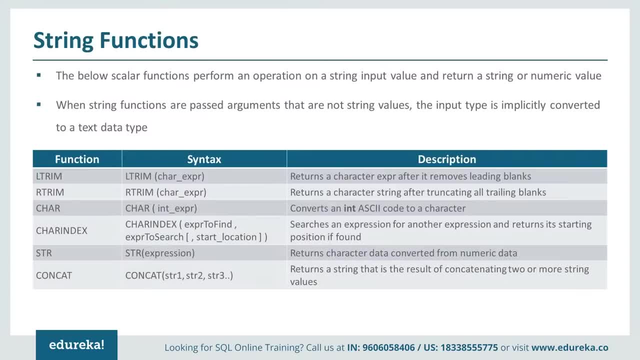 The input type is implicitly converted to a text data type. So these are the various string functions. L trim: It basically returns a character expressions after it removes leading blanks. It basically removes the blanks from the left-hand side of the string. We have our trim. 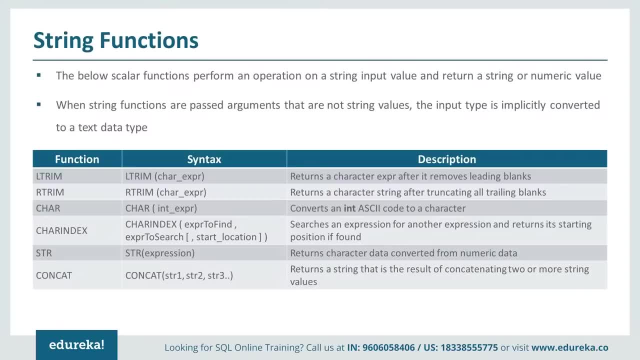 It returns the character string after truncating all the trailing blanks, basically to remove the blank from the right-hand side of a string. Care functions. converts an int ASCII code to a character Character index- find out and searches and expressions for another expressions and returns is starting positions, if found. 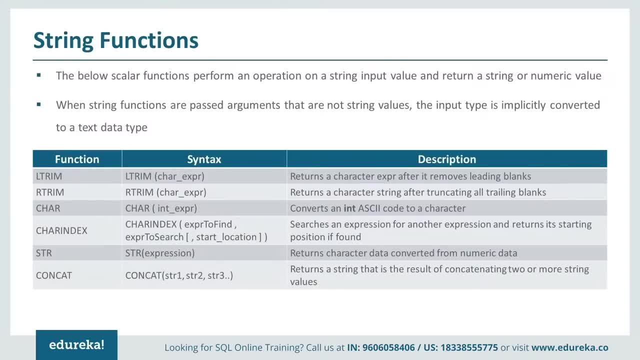 STR returns character data converted from numeric data. CONCAT return a string that is results of concatenating two or more string values. So these functions are almost similar to other string functions which we use in other programming languages. So most of the programming languages we have trim functions. 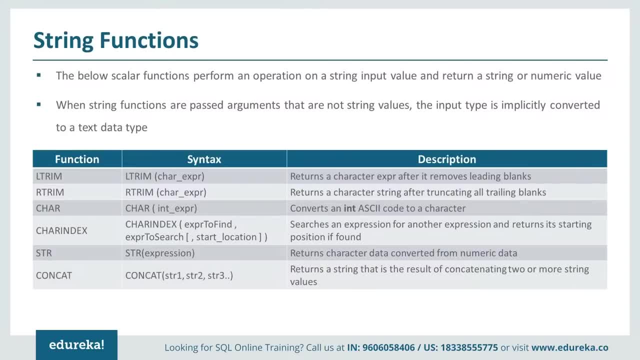 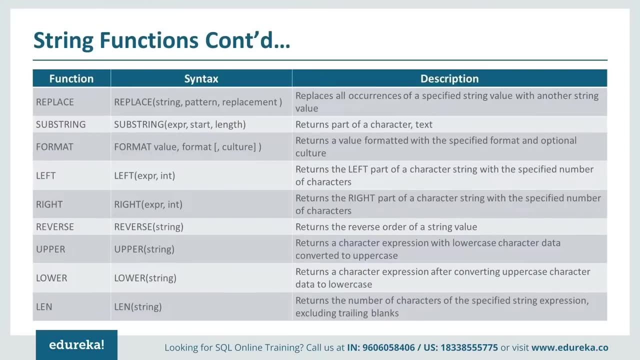 We have functions to find out the index of a character. We use concatenating operation. This is a very common string functions to concatenate two strings or more than two strings. Then we have replace functions, So replace all occurrence of a specified string value with another specific value. 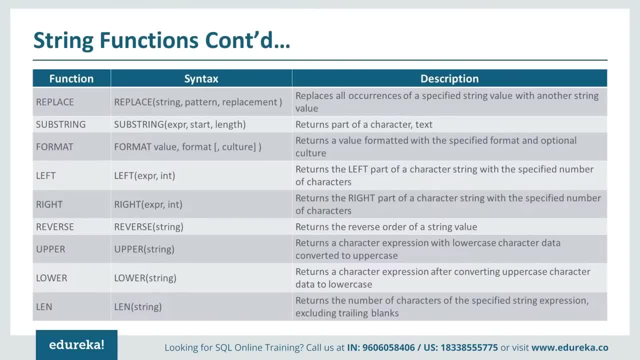 We have substring returns part of a character or text based upon the length or the start index which we give in. as we can see the syntax of the substring, We have a substring keyword followed by the expression like: the string from which we want to find out the part of a character will define the start index. 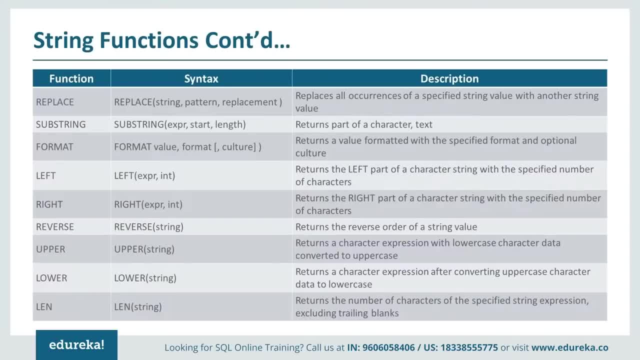 and then we'll define the length from start index till how many characters we want to fetch the substring. Then we have the format functions. We can format strings into desired format using the culture. Then we have left functions. It returns the left part of a character string. opposite of left is the right functions. 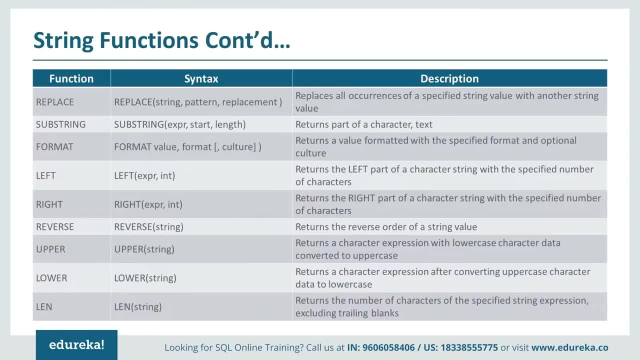 which returns the right part of a character string. reverse return the reverse order of a string value. Upper functions converts the string into uppercase, opposite of which is the lower functions, which converts the expression Expressions into lower case and in the end we have length function or alien. 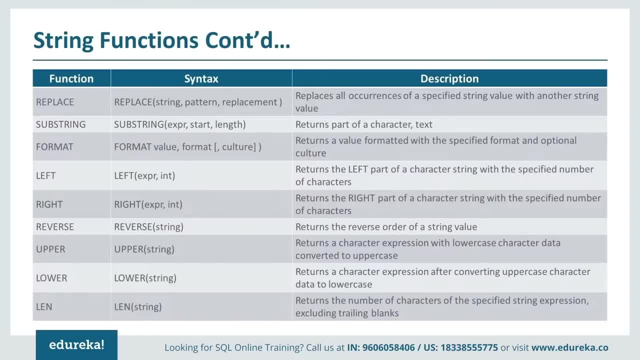 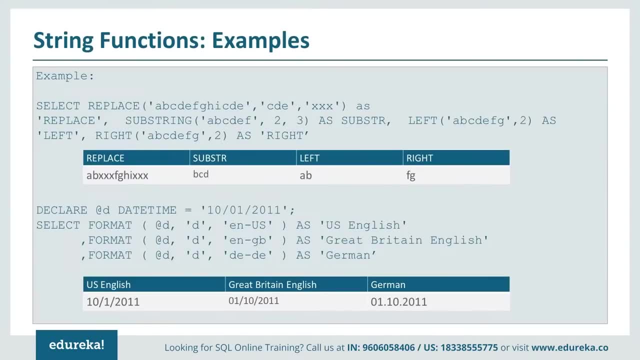 which basically returns the number of characters of the specified string and exclude the trailing blanks. So these are the various examples on our slide. So first one is for the replace function. So this is our string and this is string. We are replacing CDE with XXX as the replace. 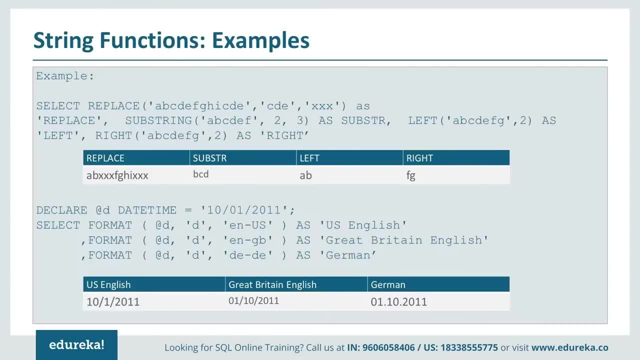 So, as you can see, in the result set here for the replace column, the value CDE is replaced with XXX. We have substring functions in the substring. We are get out of this ABCDEF, which is our main string, from index two and until length three. 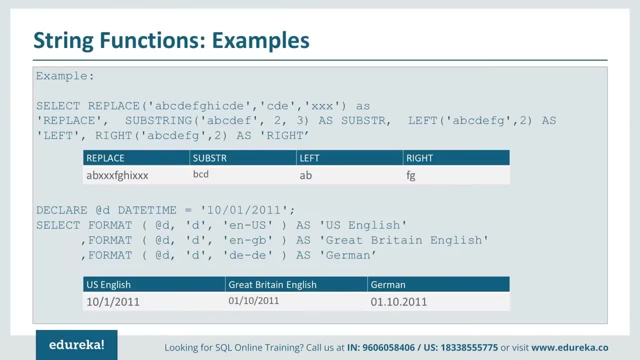 We are getting the substring. So index two is start from B and then up to three character. We'll get the substring. So we'll get B, C and D in our output. then we have left. So basically we return the left from a character index. 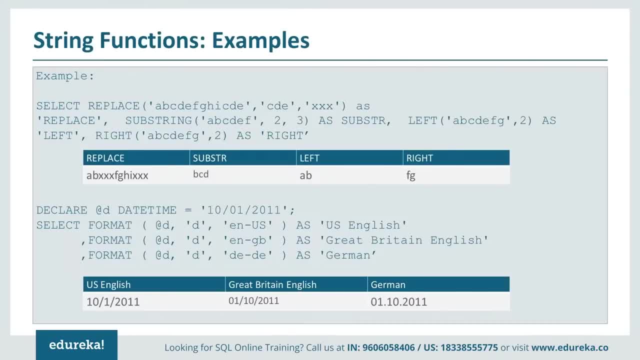 So from index two we are getting the values from the left, So it is A and B. from the right We are getting the value of B, C, D, So in the end we have the examples of date and time and format. So here we have provided the various cultural values. 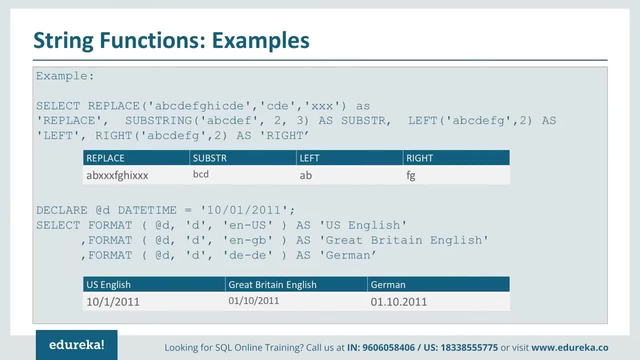 So first is for US English, second is for British English and third is for the German. So, based upon the info culture, we basically get the different results here. So most of the string functions are pretty much straightforward, So let's discuss about a few of them. 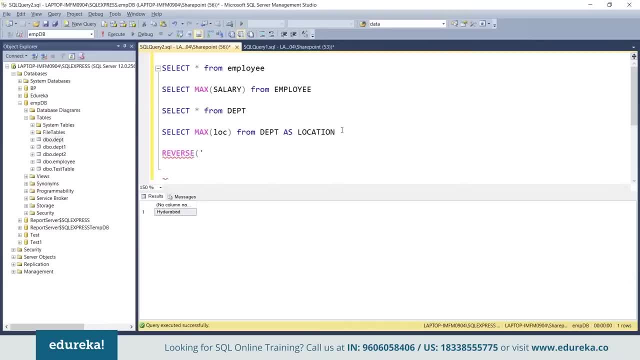 So we'll discuss about a reverse. So I'm adding a string, ABC again. I forgot to add the select statement. This will give me an error if I'll try to execute this statement without select, and if I'll execute it now, I'll get the reverse of the string. 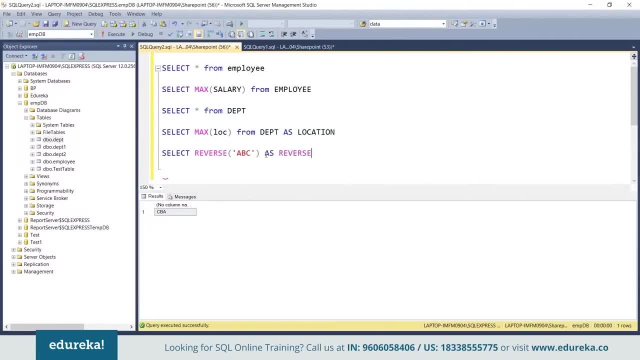 Always good to provide alias. Then we have trim and trim, Select L trim. So I have added leading blank spaces in this string and if I'll execute this, the leading spaces has been trimmed. same way I can use a trim if I'll use a trim. 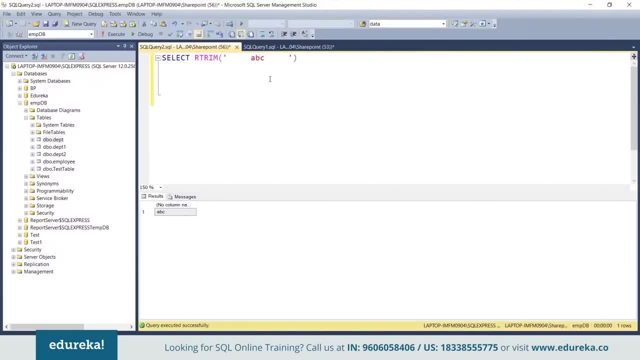 than only the trailing spaces will be removed, not the leading one. if I'll execute this, I'll get this result, and if I use trim, then we'll consider for both. We do not have trim here, So a trim removes the leading spaces and our prim removes the trailing spaces. 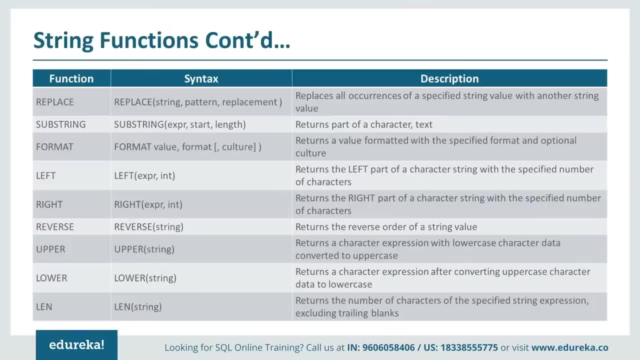 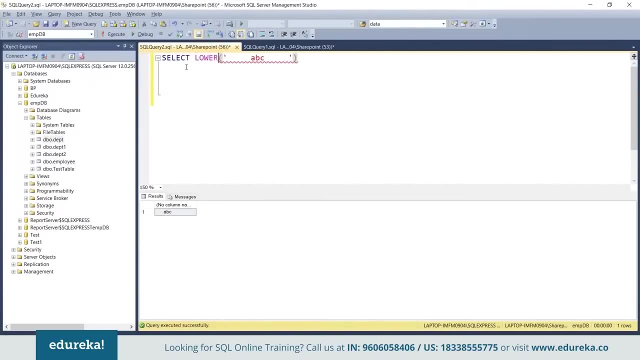 So this is all about the string functions. You can practice about the other string functions. They are pretty much straightforward. Let's see an example for the upper and lower functions as well. So if I use lower here, I'll get the same result. 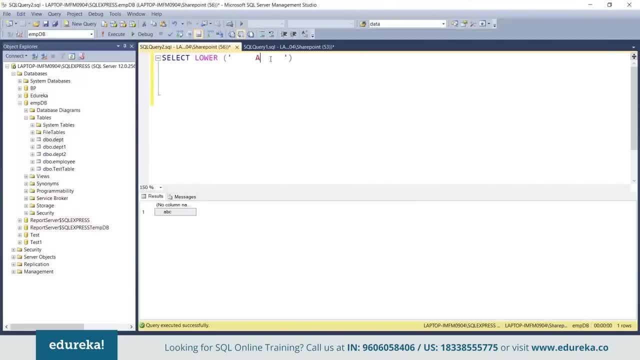 But if I use or let me convert, let me first write the uppercase character, So it's converting to lowercase. And if I'll write the lowercase, if I'll use the upper function, it convert it to uppercase. So all other string functions are also self-explanatory. 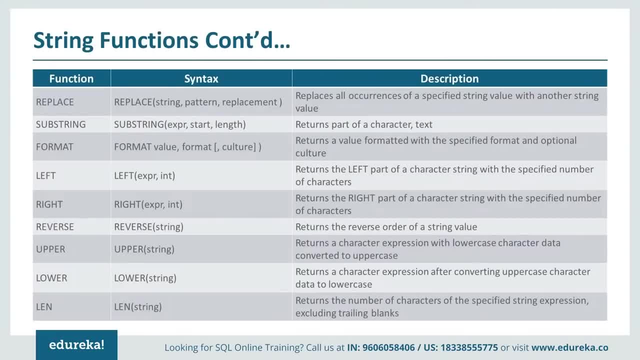 Please try all of them so that you will have an idea. And if you will try all of these, you will come to know that, if the situations arise, you can start using those. So let's move to other functions: the date and time functions. 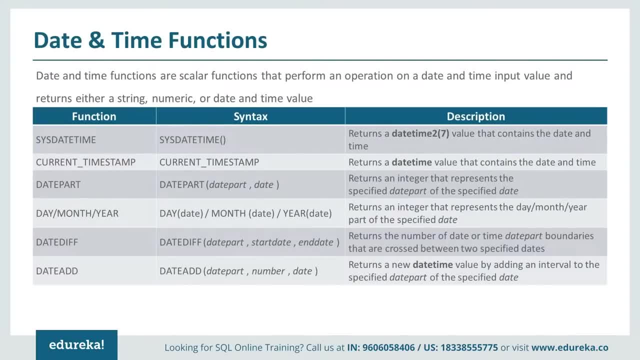 So date and time functions are again scalar functions. They are hundreds of functions that performs an operations on a date and time input value and it is either a string numeric or a date and time value. So, as you can see in the screen, 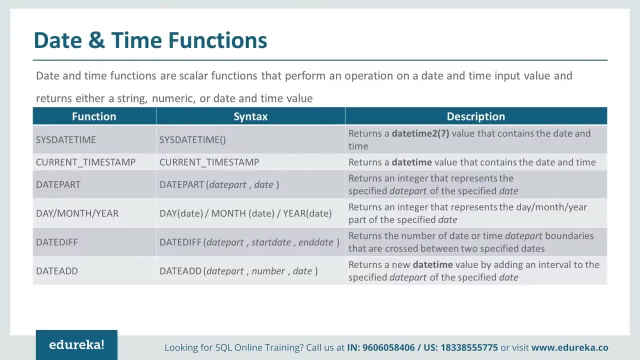 they're various, are are date and time functions. Again we have, since date time it returns at date time value that contains the date and time, it's current timestamp, against return at date time value that contains the date and time Dayt-part, basically fec as the date part of a date component. Day, monthlyonlineonlineonlineonlineonlineonlineonlineonlineonlineonlineonlineonline, and information that annual, part, date, quarter and iner MailOnlineonline Magazine will put each indeed code type號 code that contains the date and time value matches duration value. 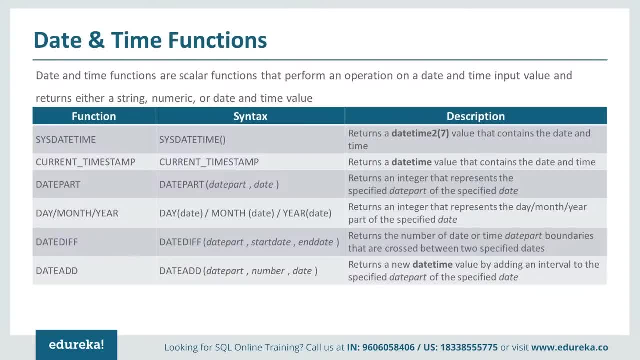 that represents the day, month and year part of the specific date Date. if returns the number of date or time date part boundaries that are crossed between two specific dates And date, it functions returns a new date time values by adding an interval to the specific date part. 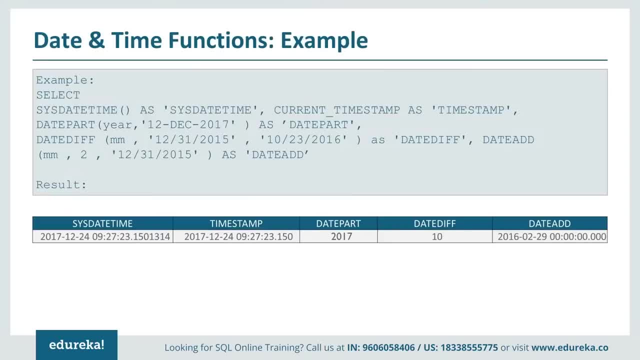 So let's see the examples of date and time functions. Sys date time: it returns the system date times. It has date component as well as the time component. Current timestamp also gives the current date and time. Date part basically provides, if it will provide year here. 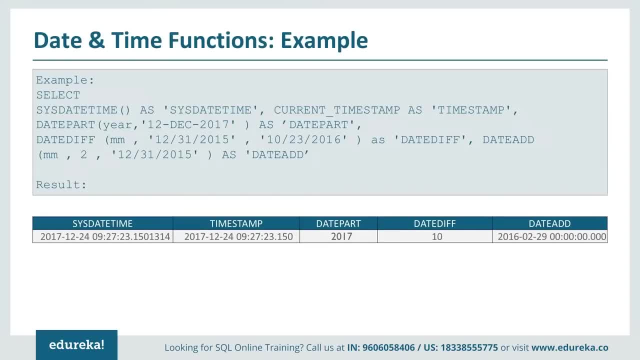 then it is providing the year of the date part. If I provide here the DD, it provides the day. If I provide MM, it will provide a fresh value of the month Date difference. so, again, if we are providing MM, so we are getting the difference of month. 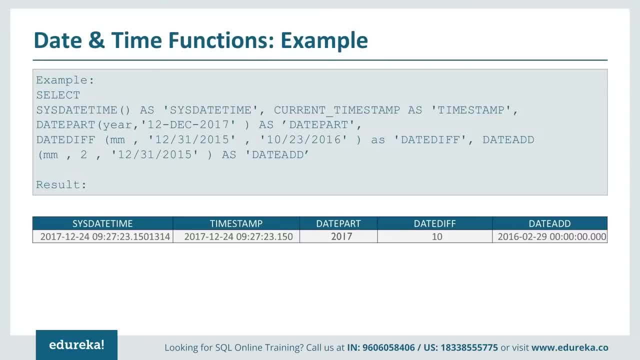 between these two dates. If I provide DD, then it will provide me the difference of date and time. So we are getting the difference of the month between the two dates. So date add is that I am adding two months. So this is how we have to do. 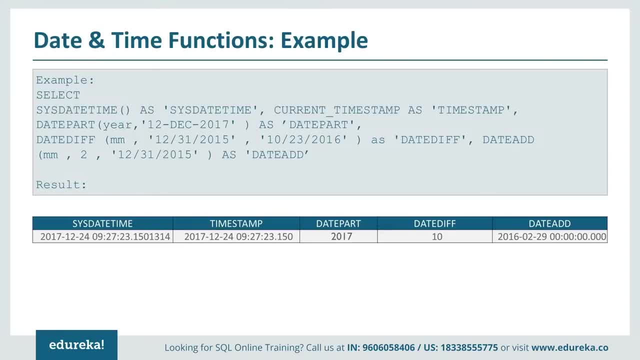 Since we have provided MM, MM specify for month here. If I provide the DD, then it will add two days Since we have provided MM here, so it will add two months to the current date. So let's see one example here. 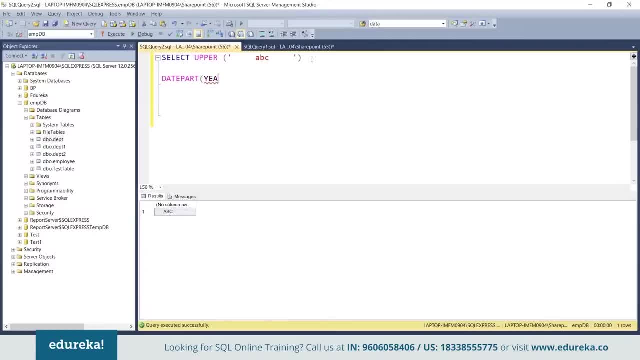 Date part year Now, let's say MM, And then we can provide the date. It's providing the month. it's the 12th month since I'm using December, If I'll change it to October and if I'll execute it again. 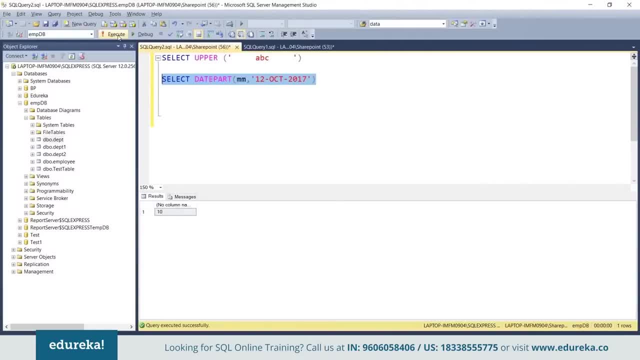 it will show me that I've already done So. this is how we use the date part, And let's see the date head function. So if I execute it now, it will add two months. I can also provide DD here, So it will add two days. 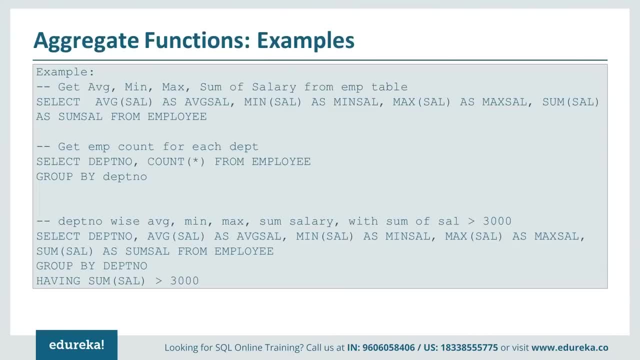 So this is all about the date functions. So now let's discuss about the group by clause and having clause. So, as you can see, we are using group by keyword here and we are using having keyword here. So let's discuss about the group by and having clause. 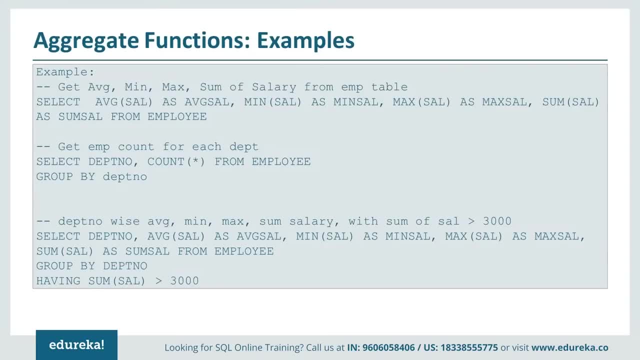 Let's discuss group by first. The SQL group by clause is used along with the group functions to retrieve data grouped according to one or more columns. The important part here is that the group by clause should contain all the columns in the select list except those used along with the group functions. 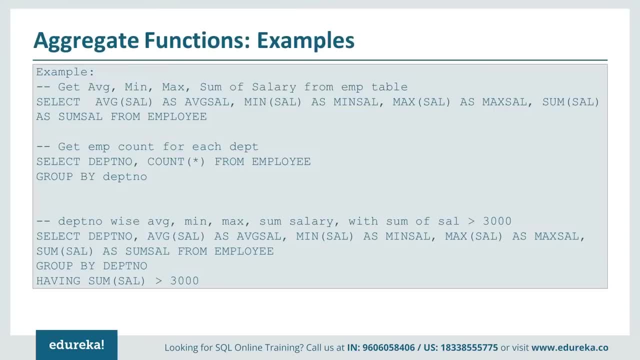 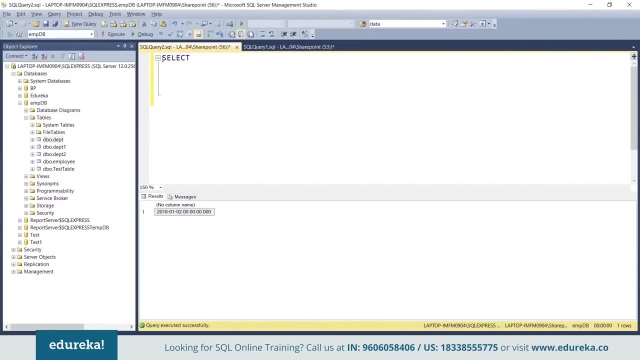 So let's see an example of group by functions for better understanding. Let's move to Management Studio And we will use department one table for group by clause. Let me first execute this query. So what I'm going to do, I'm going to group. 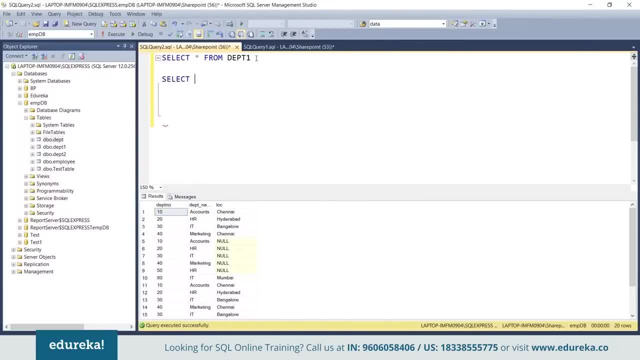 by the department number, So I'll find select count of rows from department one. Then I'll use group by clause, Then I'll use group by clause, Then I'll use group by keyword And I want to group the data by department number. 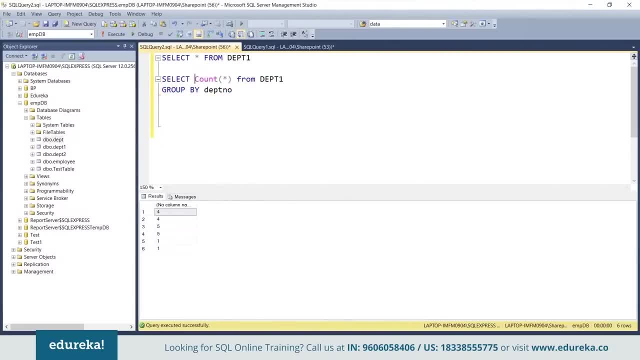 So can you see It's grouped. Or even I can write the department number And let me write the alias for this, And I'm writing the alias here as department number. If I'll execute this, I'll get. So we have count four for the department number. 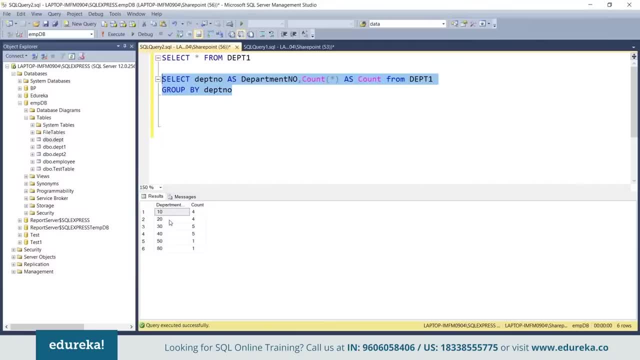 There are four values for the department number 20.. Same way five values for department number 30,, five values for 40, one values for department number 50, and one value for department number 80. So we use group by functions generally. 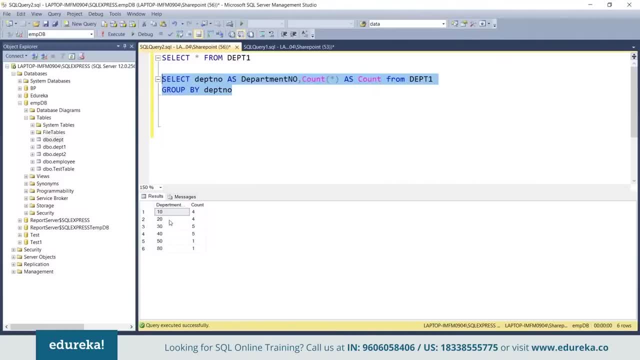 in association with aggregate functions, So it helps us in grouping the data in a table. The important part here is that we have to use all the columns in the group by which are there in the select statement. So if I'll try to include location here, 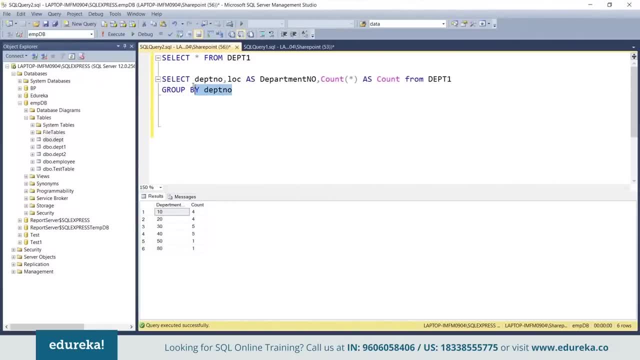 there's one more column locations in the department, one table. But if I'll try to execute it now I'll get an error Because all the columns other than the aggregate functions should be there in the group by clause. So if I'll include the other table as well, 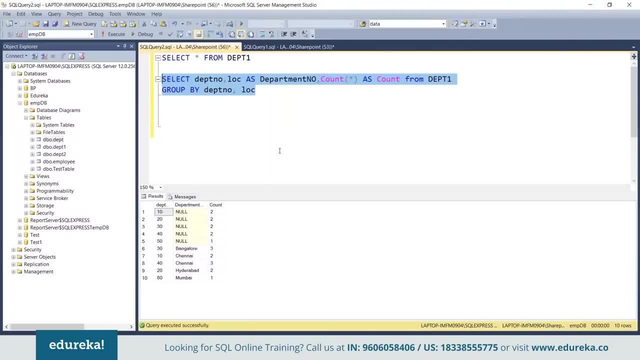 then the query will be executed successfully. So in order to execute group by successfully, we have to include all the columns which we are including in the select statement in the group by clause, And also we can include multiple columns in the group by clause. 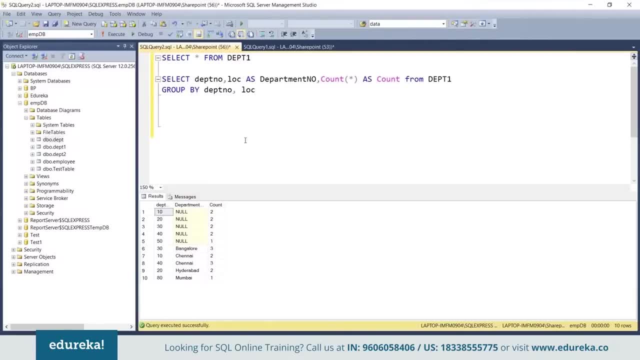 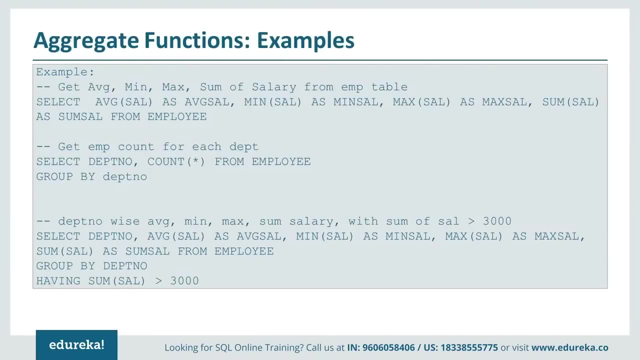 It is not that we have to use only the single column. So group by helps us to group the data in a single table And it is generally used along with other aggregate functions. So let's see the example. So here we are, basically again grouping. 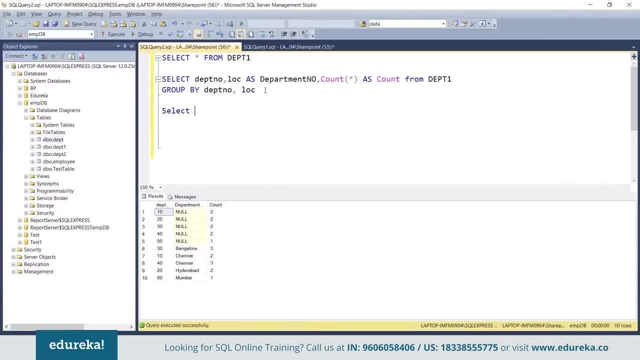 by the department number here. So let me fetch the results from the employee table So here we can group the records again using the department number or using the job ID. So if I'll to use for the employee table I'll write select job ID, job underscore ID. 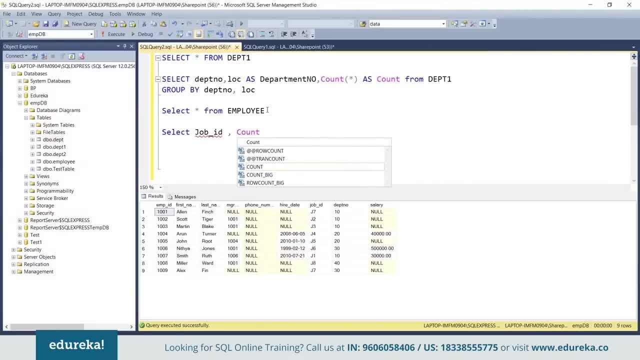 And then again I can use, for example, let's say count. It's not that we have to always use the count aggregate function, We can use other aggregate functions, also From employee. And then I'll write group by job id, so this will group the data according to the job. so only for a job id 7, we have two rows. 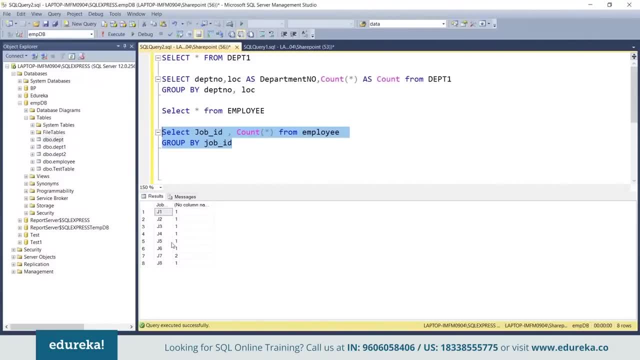 for all other job ids. we have a single row. so we are clear with the group by now. let's discuss with. let's discuss the having a keyword. so the having clause was added to sql because the where keyword could not be used with the aggregate function. we cannot use a. 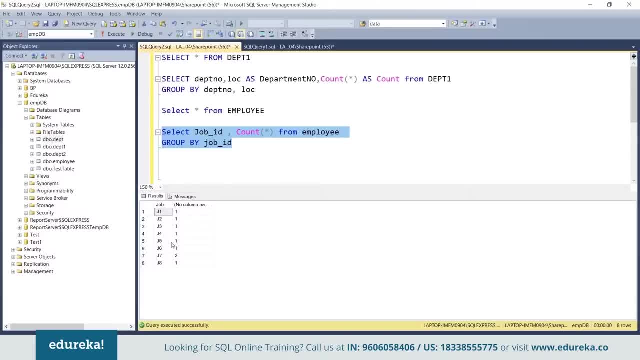 var keyword with this aggregate function. so having applies to the summarized group records, whereas vare applies to the individual records. so if it is a summarize record or the group, when we use group by, then we have to use having and if it is the individual records then we'll. 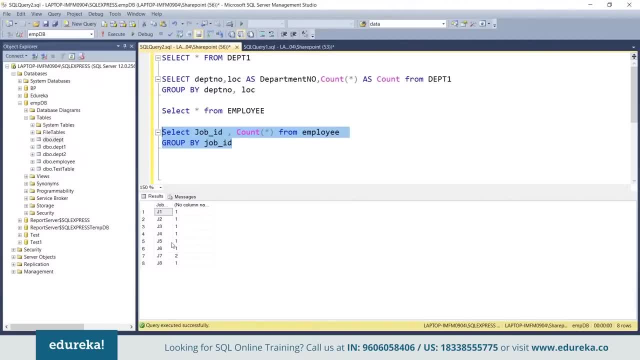 use the vare clause. so if we'll use the having close only the groups, that meets the having criteria returned in the result sets. and having keyword requires that we'll use group by in our sql query so we can say that the having clause is used in combination with the group by clause. 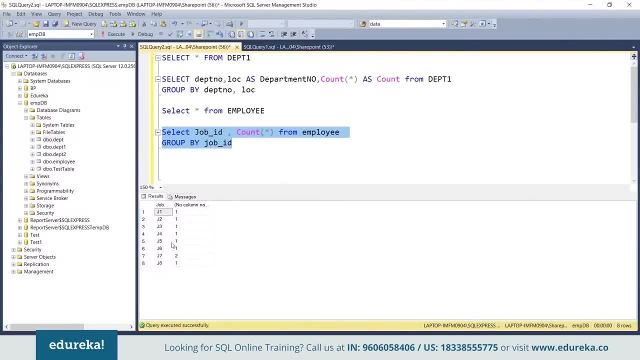 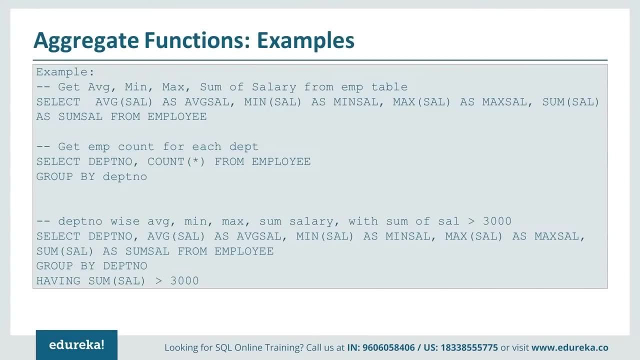 to restrict the group of return rows to only those who where the to only those which is matching the conditions or where the conditions is true. so let's see an example. so here in this example, we are selecting the department number, taking the average salary, minimum salary and the maximum salary, and and we are finding that if the having the sum of the 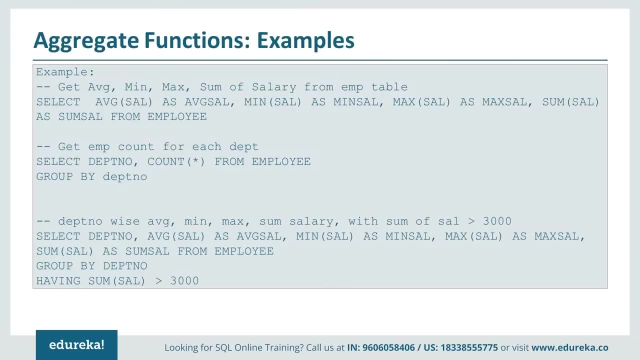 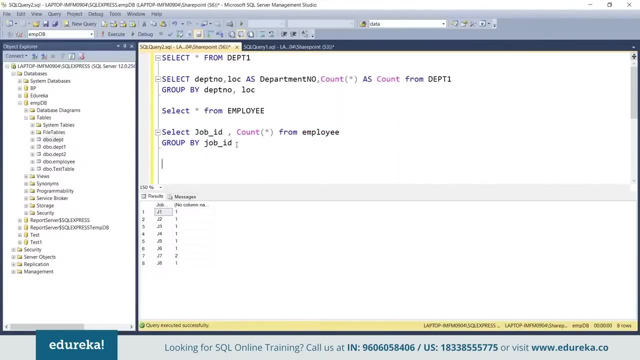 salary is greater than 3000 fetches only those results. so let's write. let's see this example in the management studio and i can write here: having salary greater than argument is greater than, let's say, thirty thousand. oh, we have to include the with the minimum salary. 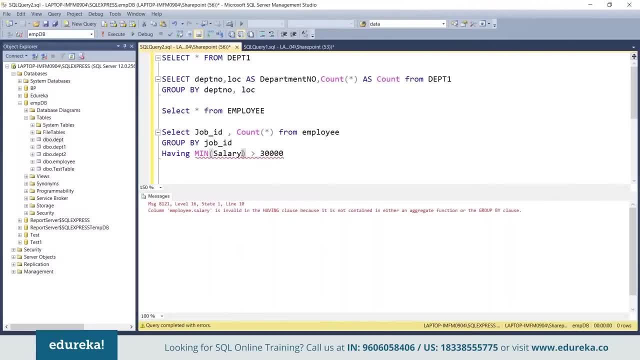 we have to use the aggregate functions in the having clause. yeah, so we get only two results. so let me first show you the result sets. so we have, uh, three rows which are having the value for the salary column: j4 having salary of forty thousand. j four having salary of forty thousand. 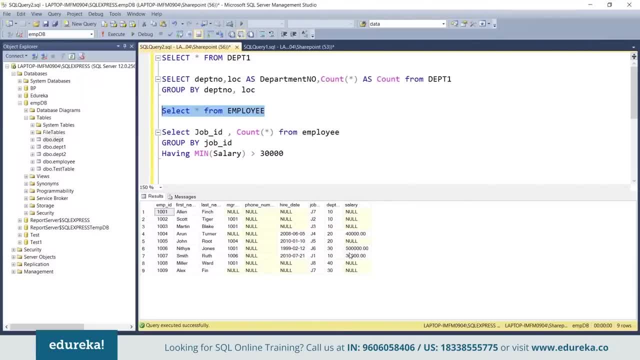 J5 is blank, so we have J6 as 500,000 and then we have J1 as 30K. So, as per our query, we should get only the two results, that is, J4 and J6, because these are the only two rows. 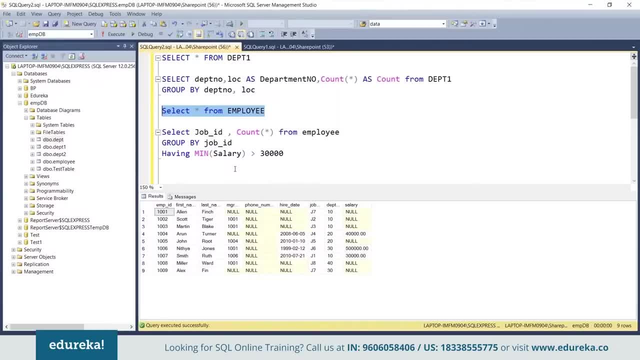 which are satisfying the having clause. So having is kind of we used to filter the result sets, but with the aggregate functions we cannot use where command, so we are supposed to use having clause. This is it about the various after box SQL functions? 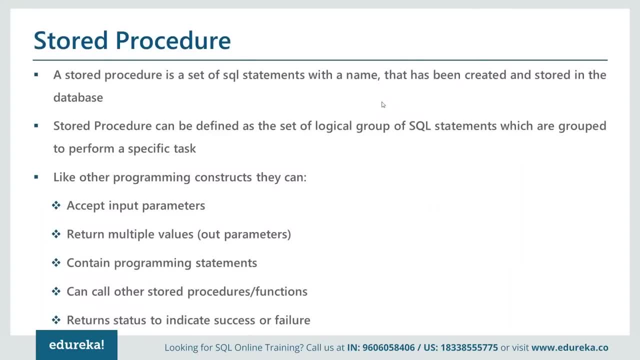 And first we'll discuss about the store procedure. A store procedure is a set of SQL statements with a name that has been created and stored in the database. So when we execute or when we write SQL statement but we are not storing those queries. 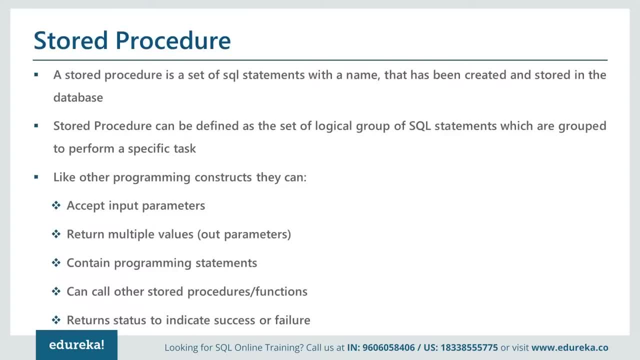 but in store procedure we can write a set of SQL statements and we can, you know, execute them and they can store in the server. So every time I don't have to write SQL queries, I can write my business logic in the store procedure. 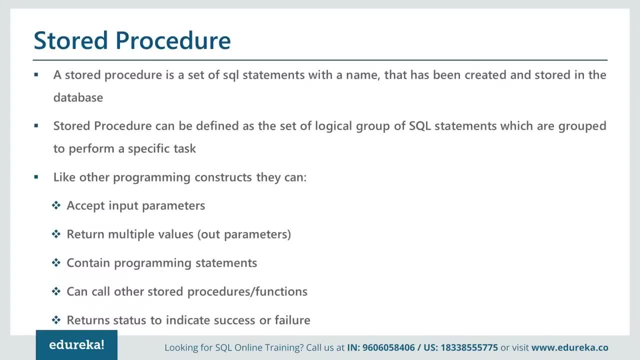 So store procedures can be defined as a set of logical group of SQL statements which are grouped to perform a specific task. So basically, in store procedure we write most of our business logic. So, like other programming languages, store procedures accepts input parameters. 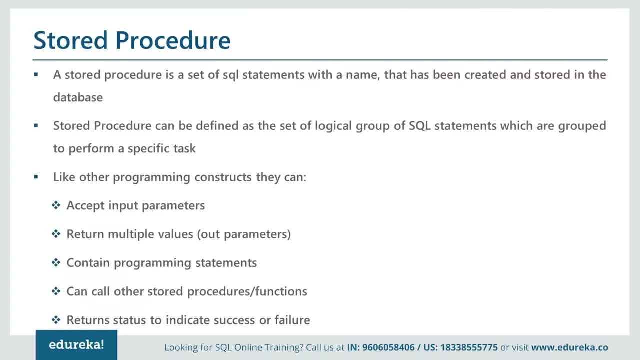 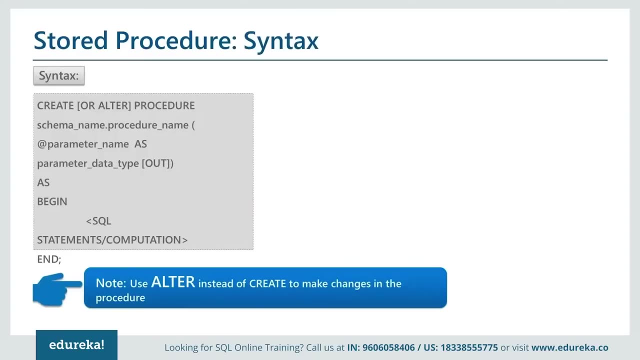 they return multiple values by means of out parameters or output parameters. They contains programming statements. A store procedure can call other store procedures or functions or return status to indicate success or failure. Let's see the syntax of store procedure first. So this is the syntax. 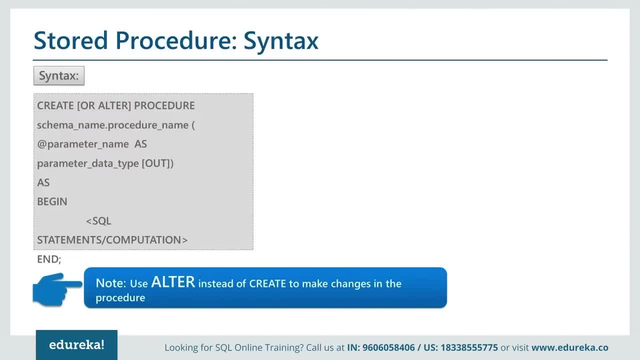 We have create keyword. to create a store procedure, We have to write create, followed by a keyword procedure- name of the store procedure which we want to create. If you want to provide any parameter in the store procedure, then we'll provide the parameter name. 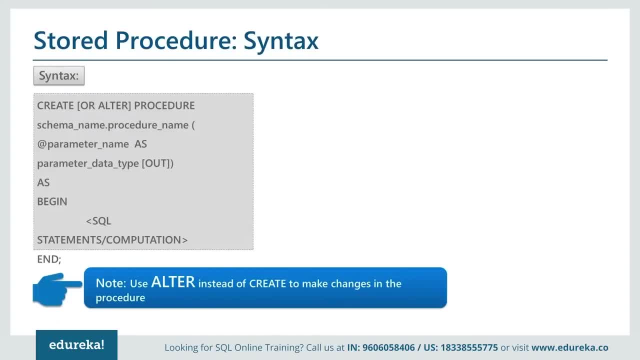 If you want to create the parameter as an output parameter, then we have to use the keyword out or output, followed by as keyword, and we'll write begin and whatever the statement or competitions we want, we'll write that and in the end we have to write end keyword. 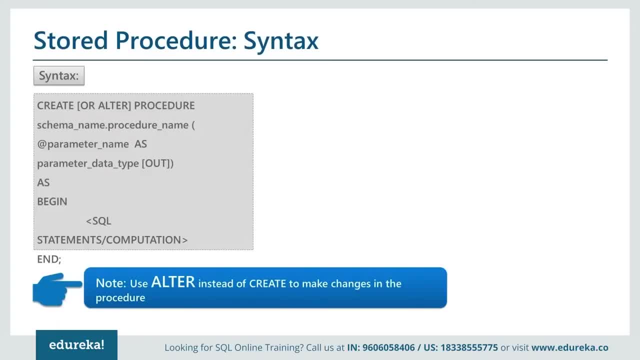 So in the syntax it is mentioned that it is create or alter. So if you want to modify the existing store procedure, then we have to use the keyword alter. If we are creating the store procedure first time, then we have to use the keyword create. 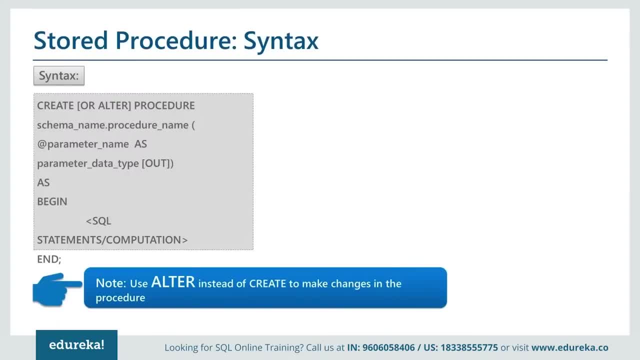 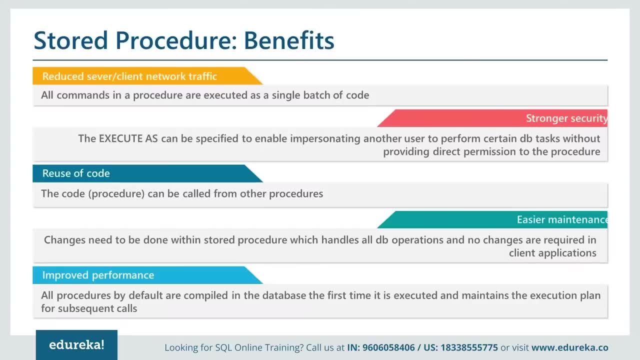 So alter keyword is used if you want to modify any existing store procedure. Now why we create store procedure when we can write SQL queries? So here are the some of the benefits of creating store procedure. All commands in a store procedure are executed as a single batch of code. 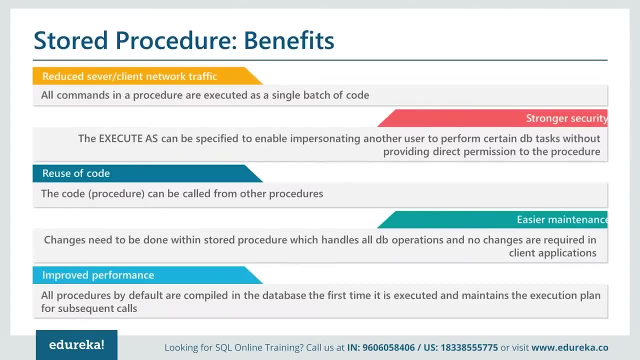 When we execute queries in SQL, generally each query goes as a single batch. but when we execute store procedure, though it may have multiple SQL statement, all SQL statement are executed as a single batch of code. So by doing this it reduce the server or client network traffic. 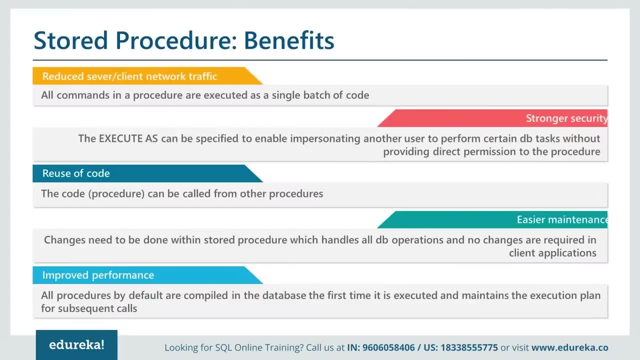 and improves the performance. Store process helps us in achieving strong security in SQL because we can impersonate another user. Execute as can be specified to enable impersonating another user to perform certain database tasks without providing direct permissions to the processor. So it makes our environment more secure. 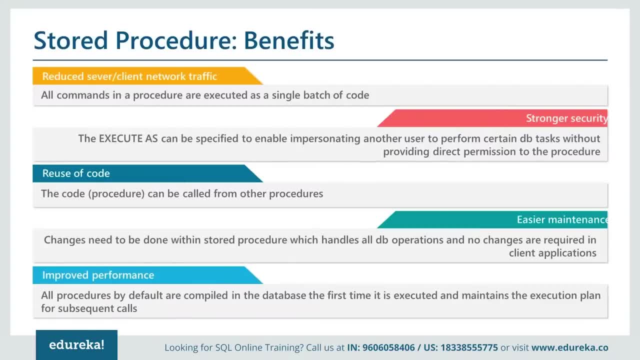 Reuse of code Store process helps us in achieving reusability because, as we discussed in the previous slides, we can call another functions or store process from one store process. Easier maintenance changes need to be done within the store process. So in order to do this, 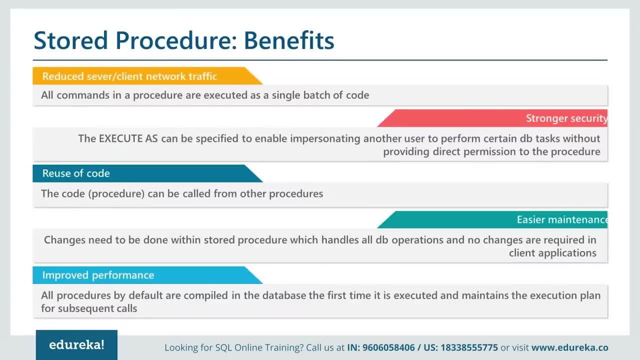 we need to use a store process which is a store process which handles all DB operations and no changes are required in client applications. So sometimes we move our business logic to the store processor. So if any changes are required, we need to modify our business logic. 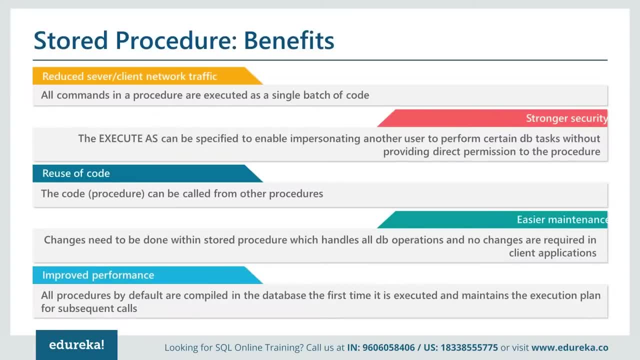 then we don't have to change our client applications or our code. We have to just modify the store process and execute it again. Also, if there is any error, only one store process instead of looking for multiple SQL statements. That is the reason store process are easier to maintain. 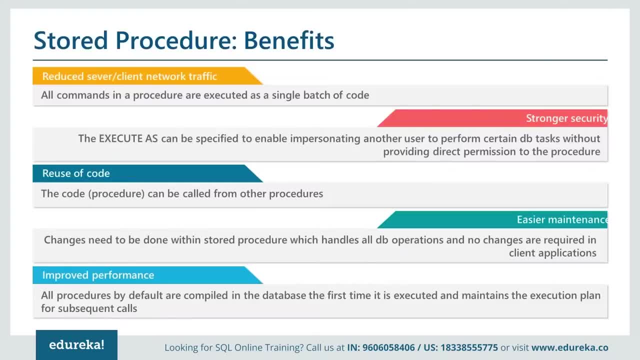 Improved performance. All procedures by default are compiled in the database the first time it is executed And it maintains the execution plan for subsequent call. So if we'll execute, or if we'll call or run the store process again, it will take less time. 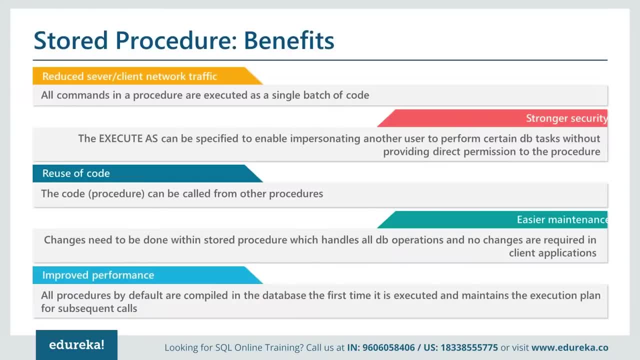 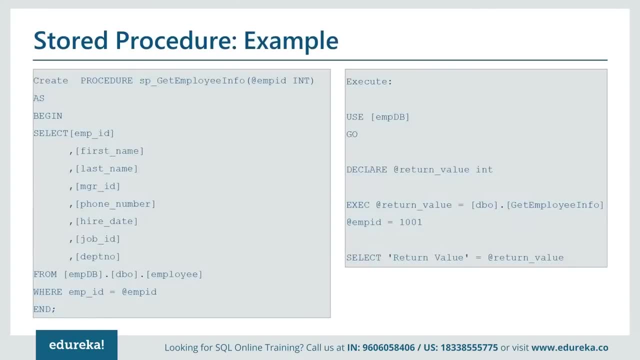 because it is already compiled in that database the very first time. So by doing this the performance of applications has increased. So on this slide we can see an example of store procedure. So we're creating a store procedure, So we are writing first the create keyword. 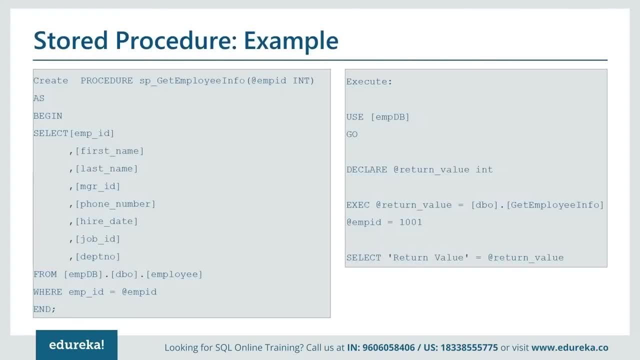 followed by the procedure. SP underscore: get employee info- is the name of the store procedure, This store procedure. we are passing a parameter- employee ID- whose data type is int, followed by the basic syntax. we are defining The keyword as in begin, And then we are writing the basic query. 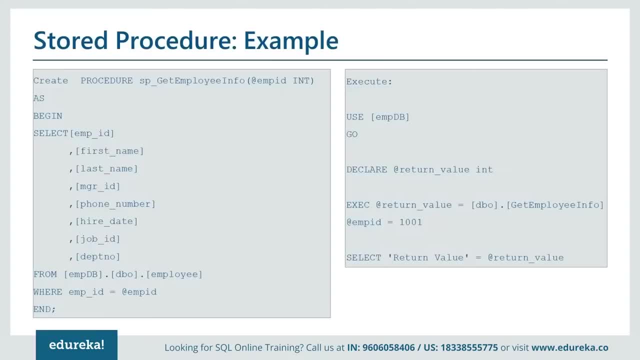 that select employee ID: first name, last name, manager ID, phone number, hire date, job ID. These are the columns of table employee. And then we are passing the condition. We are filtering the records from employee table by using a where clause. 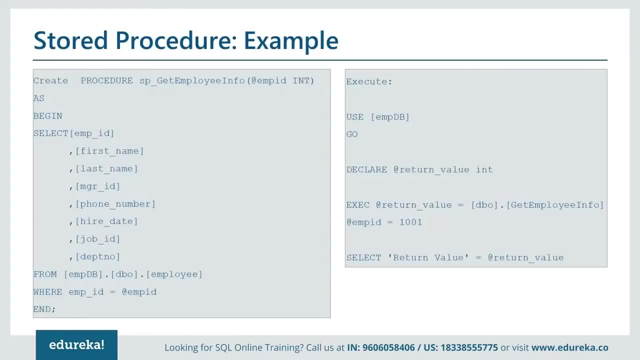 And in the where clause we are not hard coding any value. We are equating it with an employee ID, which is the parameter. So when we'll execute the store procedure, we will pass the parameter. So let's see a few example of the store procedure. 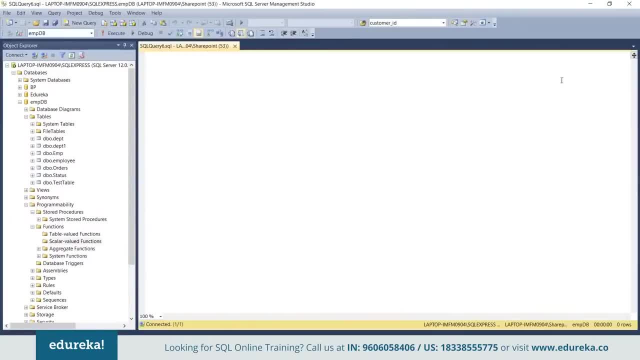 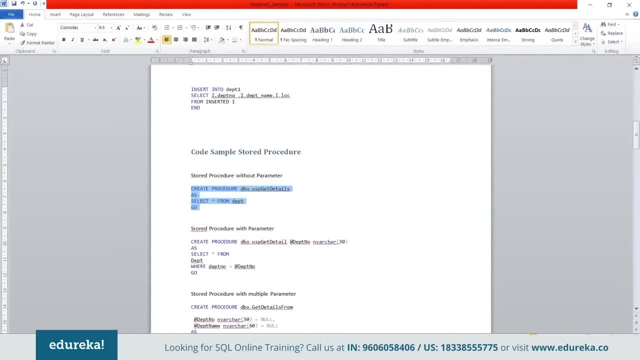 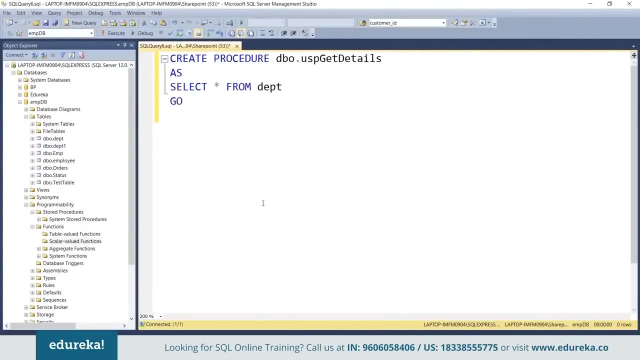 So let me open management studio. So let me open the examples I already have. So let's create a store procedure without parameter first. It is not that every time when we'll create a store procedure we have to define a parameter. So I'm writing the create keyword, followed by the procedure. 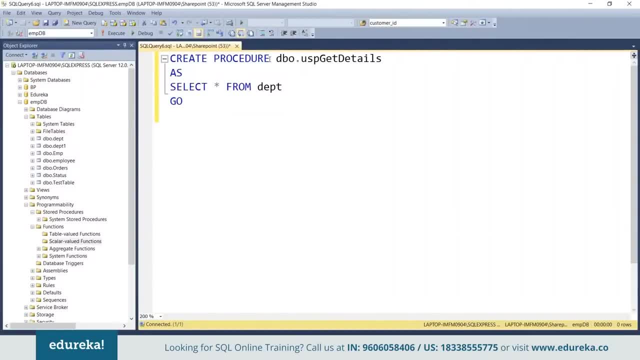 and all reserved keyword will be highlighted in the blue color. Then I'm providing a name of the store procedure. So I can provide any name here. So I'm providing a get details or I can mention it to give it more meaning: get department details. 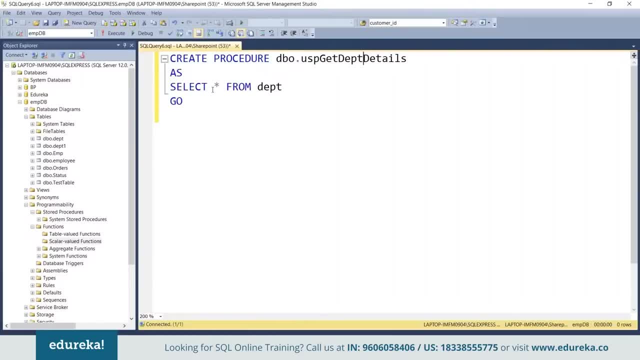 And the store procedure. I've simply written a one select query, that select star from department, And I'll execute this query. Command completed successfully means we have successfully created the store procedure And we have successfully created the store procedure And we have successfully created the store procedure. 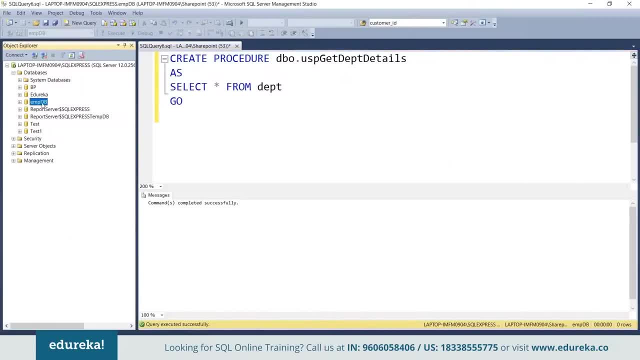 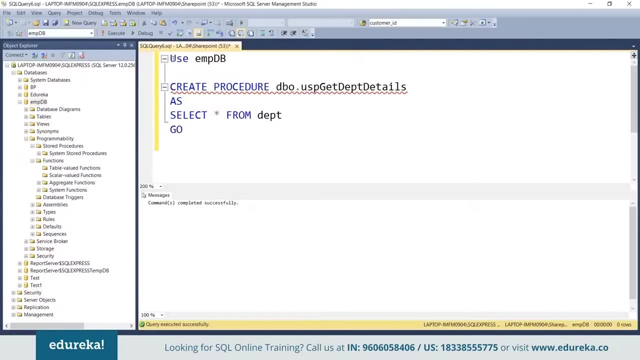 Now where to check for the store procedure. So I'll first expand the database under which I'm creating the store procedure. An important thing is that we have to use the database first, that under which database we want to create a store procedure. So always write the name of the database. 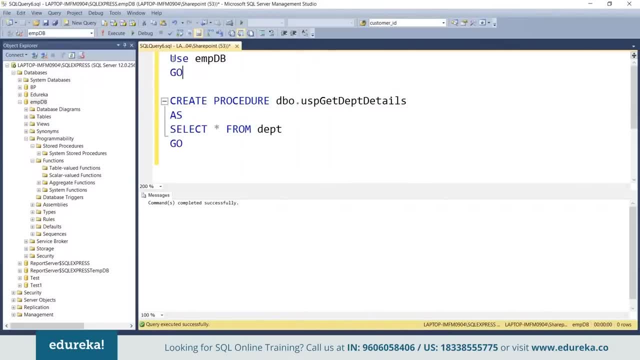 use keyword followed by a go keyword. Now, if we'll try to execute this statement again, I'll get an error that this is already an object name. USP: get department details in the database. So since I've already created this store procedure. 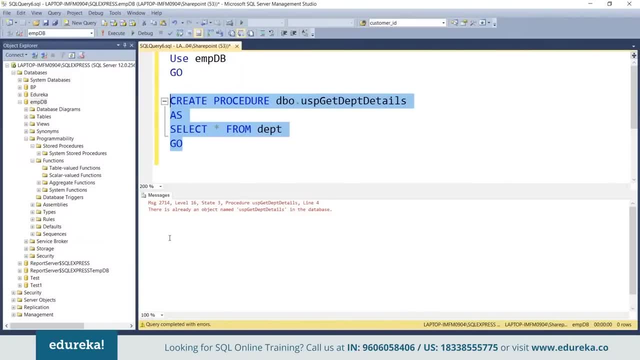 I will try to create it again. It will give an error. So, when you provide a name of the store procedure, please ensure, or please check, that this, the name which you are providing, is unique and it does not exist in a database in which you are creating that store procedure. 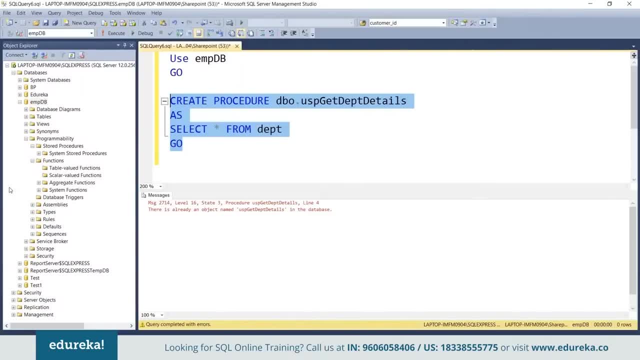 So if I want to check the name of the store procedure, I want to check where exactly the store procedure has been created, I have to expand the programmability folder. Under programmability folder we have a separate folder for the store procedures. Let me refresh it. 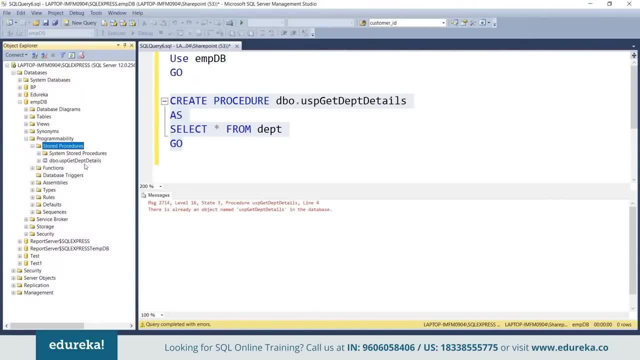 So here we can see the store procedure. DBO, USP get department details. So from this object explorer I can modify the store procedure, I can execute the store procedure or even I can delete it. So to delete it. 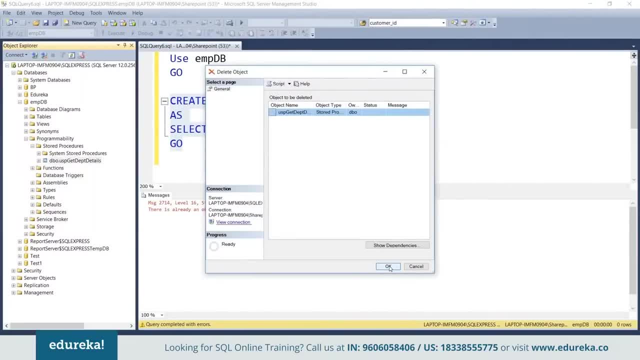 we have to simply click delete. here We'll again reconfirm whether we actually want to delete the store procedure and if there are any dependency of the store procedure, we can check it with the show dependency. So when we delete something from our database, 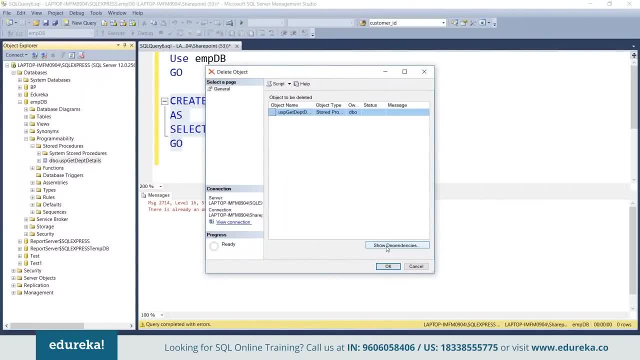 it is better to check the dependency. If there are any dependency, we'd rather not delete that particular object. So as of now, we know that there's no dependency, so I'm just clicking okay here and it will delete the store procedure. 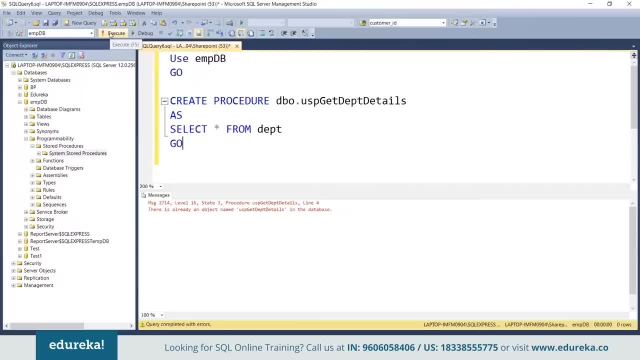 Since we have deleted the store procedure and now if I'll execute this statement again, it will be executed successfully, as there was no store procedure in our database and by execution of the statement we'll again create that store procedure. So if I'll refresh this store procedure again, 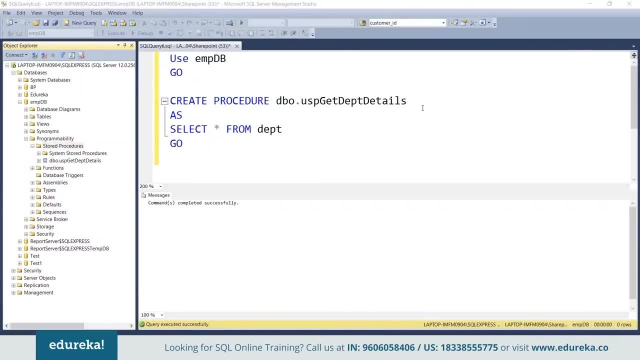 I'll see the store procedure. Now we have created the store procedure and we'll see how we can execute this store procedure. To execute the store procedure, we have to write one command, So there are various keywords which we can use to run this store procedure. 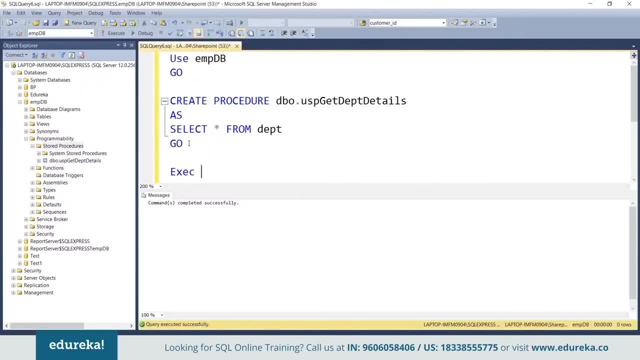 The first one is we have to write this keyword, exeC, followed by the name of the store procedure. So if I'll execute this, it will execute the store procedure and it will return this query or this result set because in the store procedure. 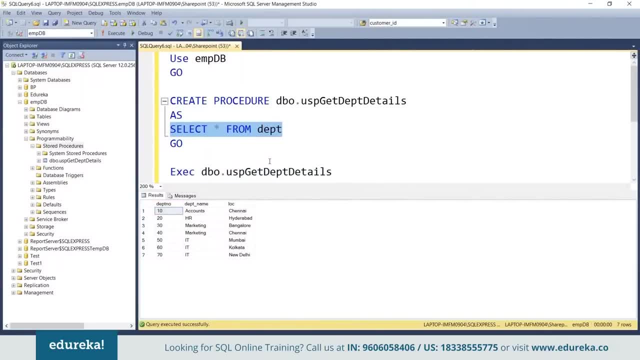 we have given only one select statement, that select star from department, and the department table has three columns, So we are getting all the rows because we have not specified any var condition. So this is an example of a store procedure without a parameter. Since the store procedure doesn't have any parameter, 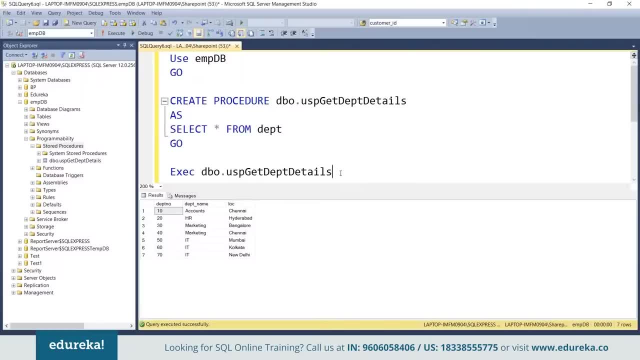 we are not passing any parameter while executing this store procedure, So it is not mandatory to provide the exeC keyword while executing the store procedure, even if it provides the variable, the name of the store procedure. and if you'll execute it, it will fetch the same results. 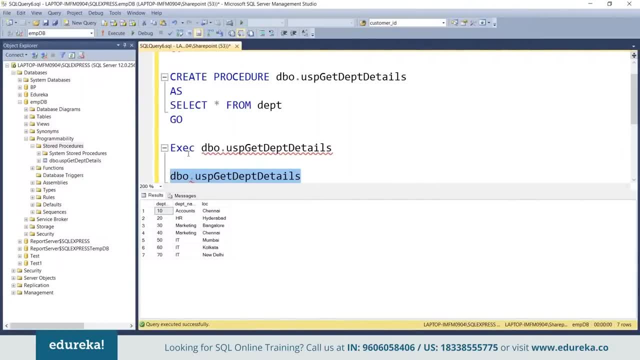 So exec keyword or execute keyword is optional while executing the store procedure. So let me again delete this store procedure. So while creating the store procedure again, we can either provide the create procedure or we can even provide the short form that create proc, Even if I'll execute the statement. 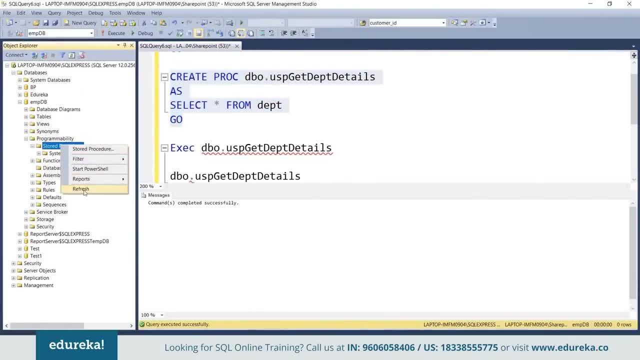 it will be executed successfully and, if I'll refresh this node, we can see the store procedure has been created successfully. While executing again, it is optional to provide the execute keyword. Similarly, while creating the store procedure, we can either provide create proc or create procedure. 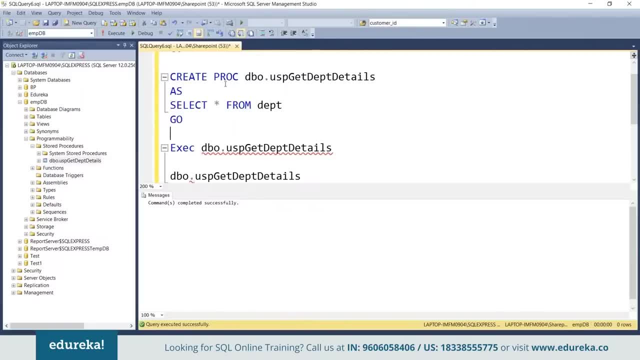 Now let's see how we can create a store procedure with a parameter. So I'm opening a new query window, I increase the font size for better visibility. So this is an example of a store procedure with a parameter. So here we are, providing the parameter department number. 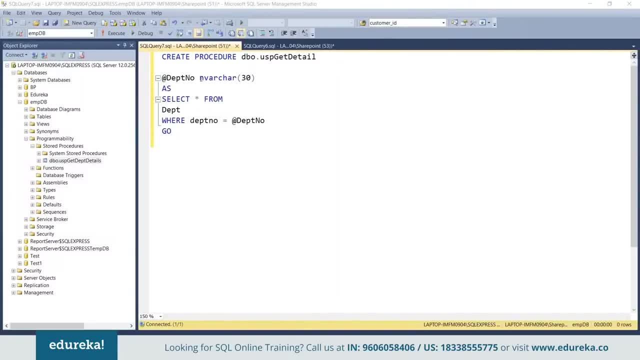 So here we have department number as a parameter and the data type of this parameter is nvacare and length is 30. So in the previous example we have written a select statement, but without the where clause. Here I'm providing or I'm filtering the record or rows. 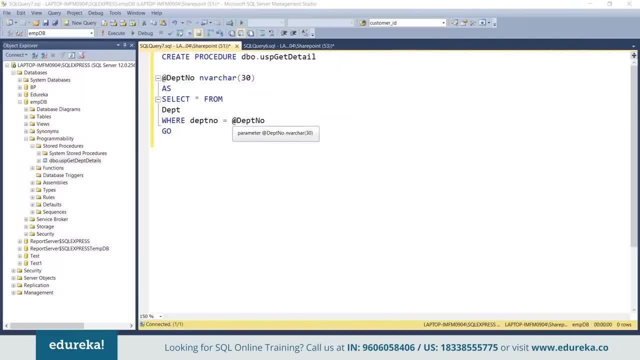 by using where clause and the where clause, I'm checking the department number with the parameter which will pass while executing the store procedure. So let me create the store procedure first and then we will execute it. The command completed successfully means the store procedure has been created successfully. 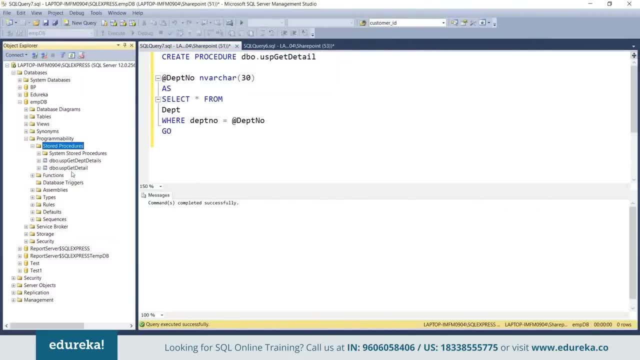 So let's again refresh this node. yeah, So now, when we are executing this store procedure- even like, as we saw- that we can provide the execute keyword or we can even directly write the name of the store procedure, or, if you're using the management studio, 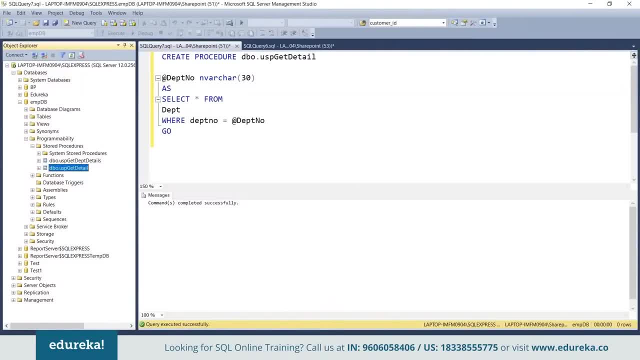 we can right click the store procedure and then we can click execute store procedure. So the execute store procedure will open this window and if there are any parameter, it will pass. it will check whether what value we want to pass to this particular parameter, As we know that we have various values. 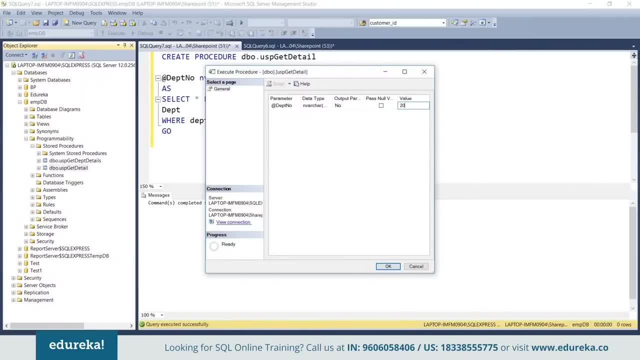 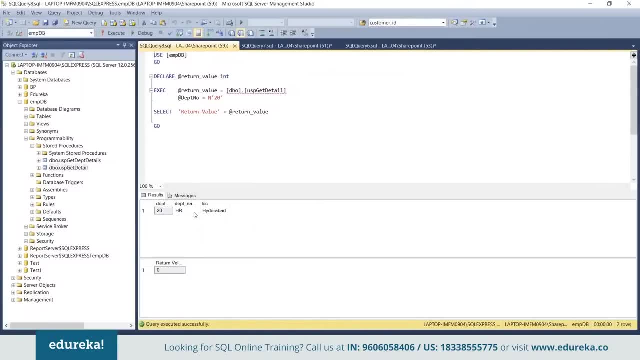 of department number start from 10 to 80. So I'm passing 20 as a value for the department number and I will click OK. The moment I'll click OK, I'll get this result. So in earlier example we got all the rows in the result set. 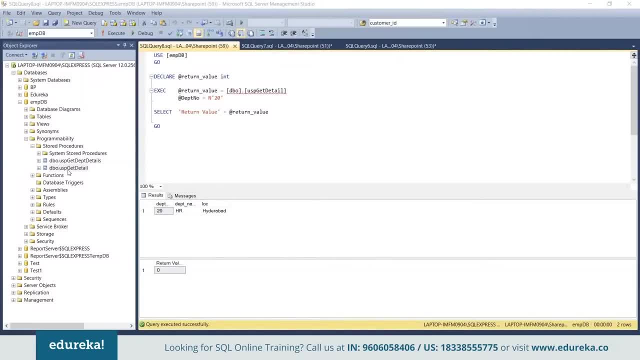 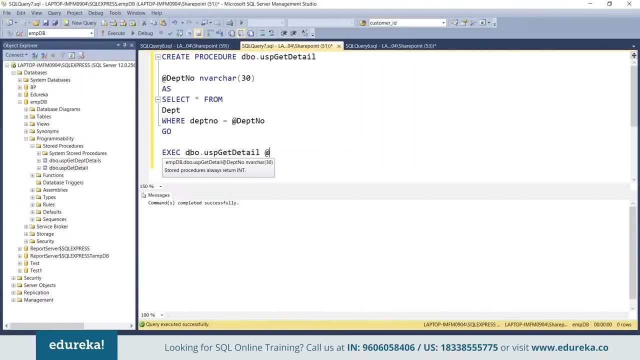 So if we do not want to execute the store procedure from the object explorer, then again we have to write the same command. We have execute keywords Followed by the name of the store procedure, and then we pass the parameter. In our case, the parameter is department number. 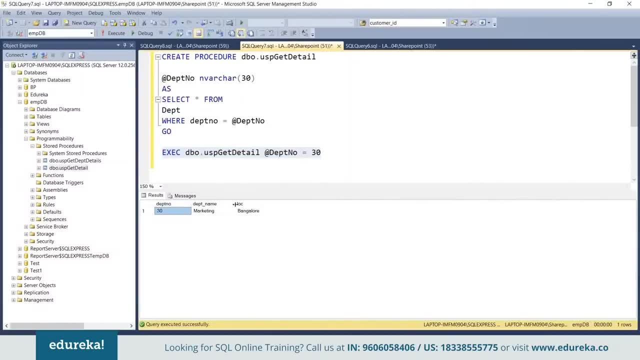 So now this will give the desired result. So this is how we create store procedure with parameter and this is how we execute the store procedure which has a parameter in it. Now, if you'll try to execute this store procedure without providing the parameter, 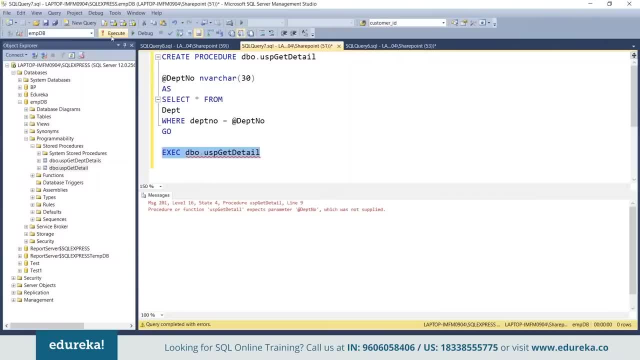 now let's see what happens. See, you'll receive an error. The processor or function usb get detail, expect parameters, which was not supplied. It means, when we created the store procedure, we have ensured that the parameter which we are providing in a store procedure is mandatory. 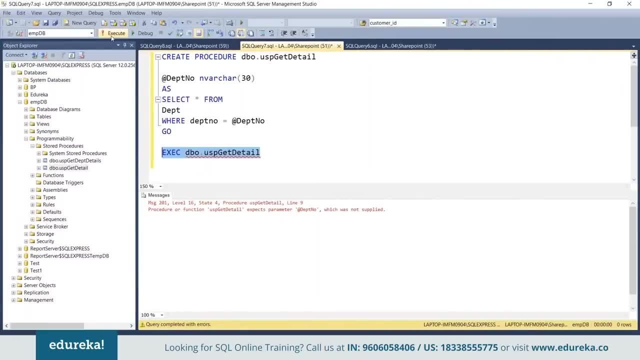 Why? Because we have not explicitly defined that this parameter can accept null value as well. So if you want to make the parameter null, then we have to explicitly provide the null keyboard. So let me modify this store procedure, or let me first delete this store procedure. 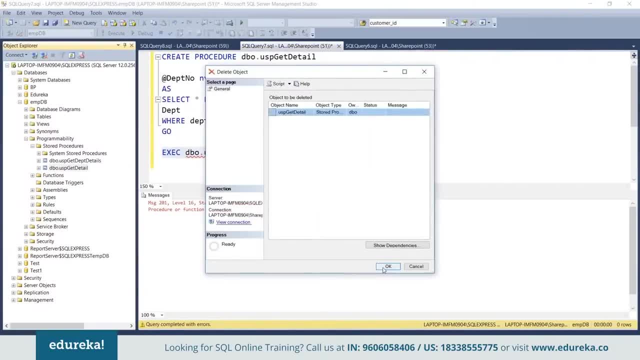 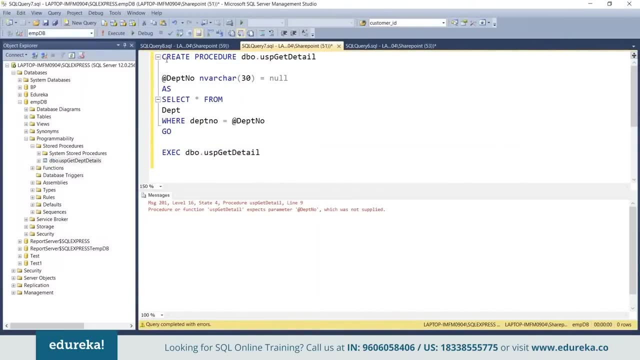 and then we'll recreate it again. So I am just deleting this store procedure And in order to make our parameter optional instead of mandatory, we have to provide the keyword null And I'll execute the statement again to create the store browser. now, if i'll execute this store processor, we won't 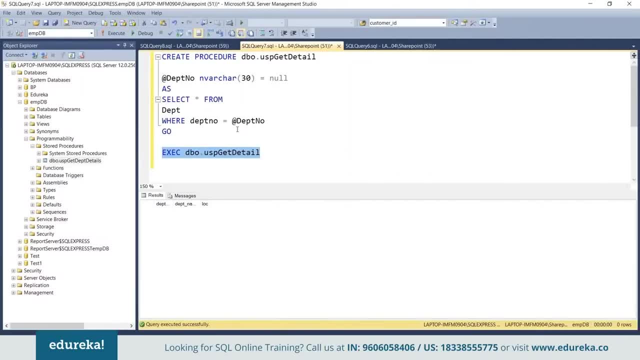 receive an error, but we won't get the value because we are checking the null value and if i not provide any null, so it will not return any result. but yes, the error is gone. so this is how we make the parameter optional, by providing the null keyboard. now let's see how we can create. 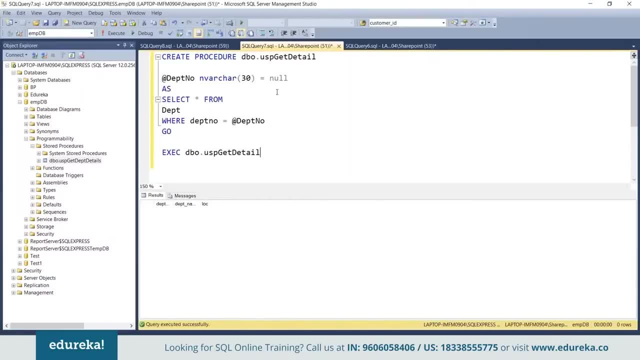 a store browser with multiple parameters or is it possible to create a store browser with multiple parameters? yes, it is very much possible to create a store browser which accepts multiple parameters. so let's see it with an example. let me open a new query again, and we already have. 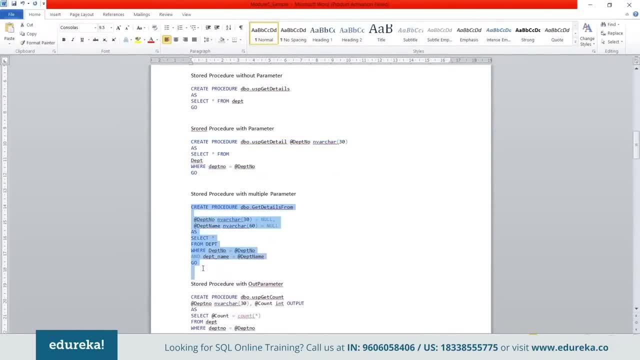 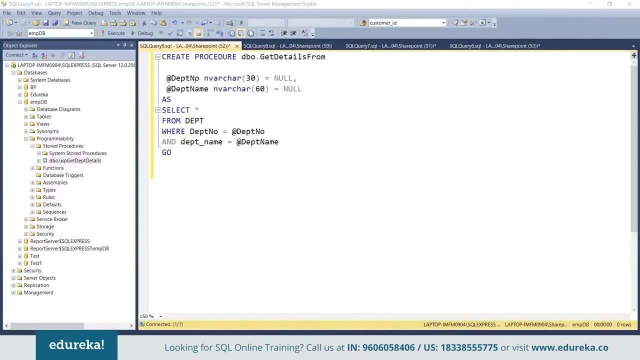 an example handy with us, let me paste it in management studio. so we have this store processor and here in this store processor we have defined two parameters. one is department number and department name. we have make both of these uh parameters as optional by providing the null keyboard. so if you want to create or we want to define multiple parameters, 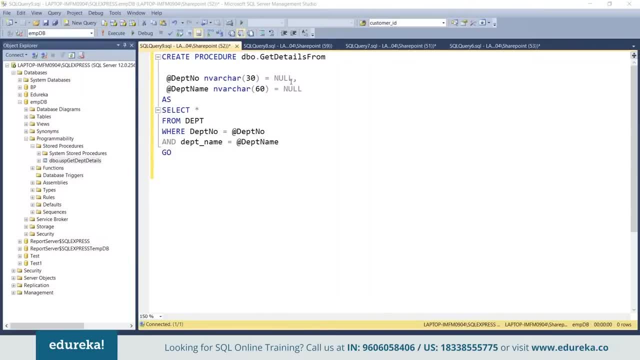 in the store processor. all we have to do is that we have to separate the two parameters with a comma. that's it rest. everything is same. we have to provide an as as keyword after the parameters, and then we'll write the store processor body in. here we are again. 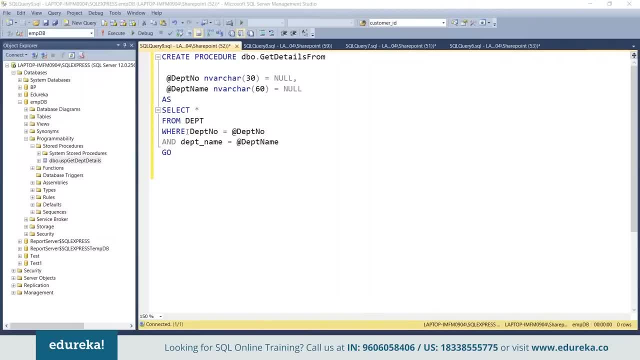 writing a select statement, but we are adding a where clause to filter the result sets by providing two conditions, and we are using logical operator, that is end, to combine two conditions. so let me execute uh, these statements to create a new store processor with multiple parameters. so store- 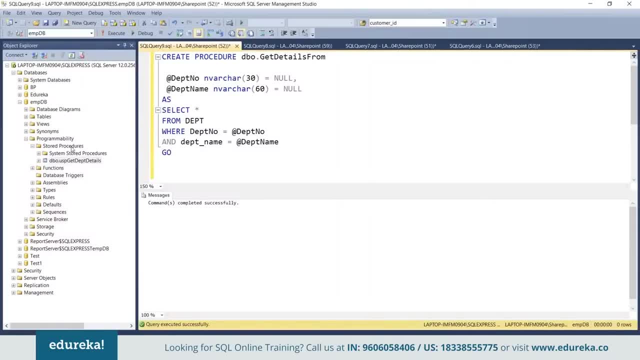 or person has been created successfully, we'll refresh this node. and this is a stored person, so let me first see the data in our table so that we can provide the right parameters values to get the values in the result set. okay, so i'll pass the parameter of department number as 50 and department name as it, so let's. 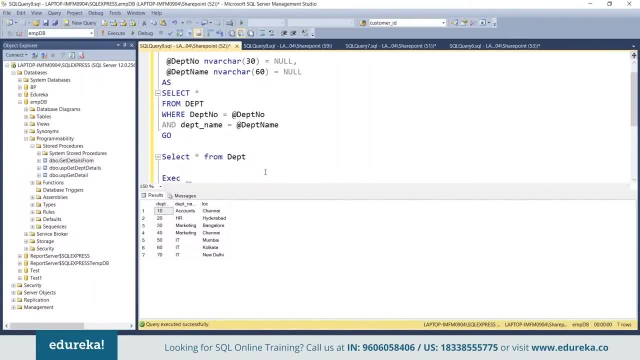 So all I have to do is I have to provide the keyword execute, name of the store process, get, get details. from then we have to provide the value for first parameter, that is, department number, its value. So we have decided to pass its value as a 50. 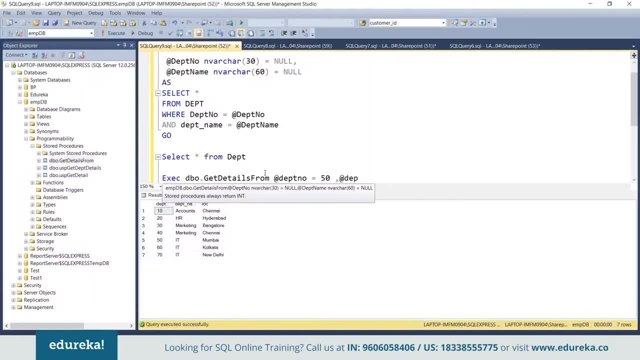 and then we'll provide the value for another parameter. Since it is string, we have to include. it is in single quotation. And now I'll execute this and we'll get the design result. that department name is ID and it's located in Mumbai. 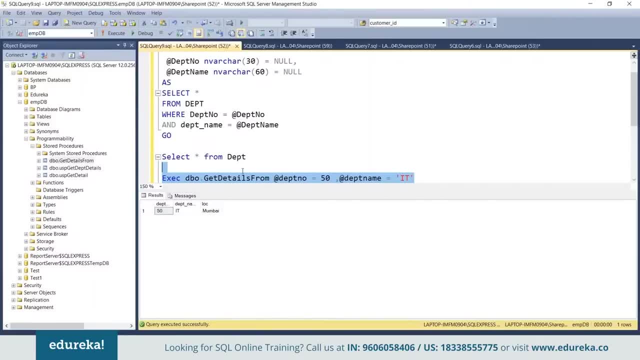 So this is how we'll execute and the store processor with multiple parameters. So we'll write the name of the store processor and the first parameter, then write a comma and then the second parameter, and so on. It is also in other store processor. 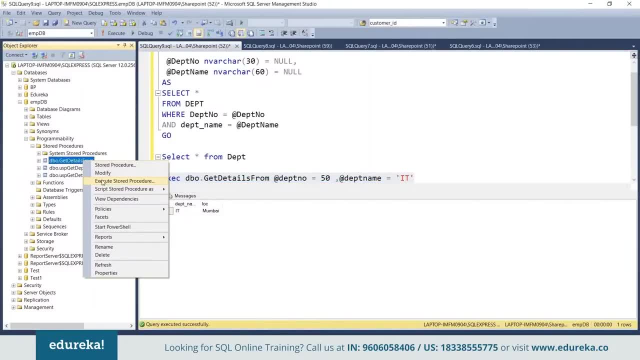 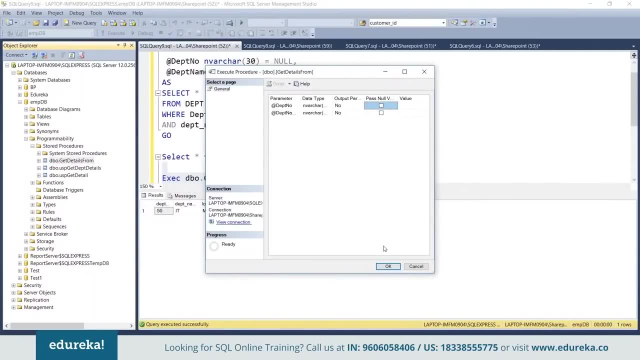 If you want to execute it from the object explorer, then you have to right click the store processor and click execute store processor And get both the names. we'll pass the value here and we'll click OK. If I'll click it, OK now. 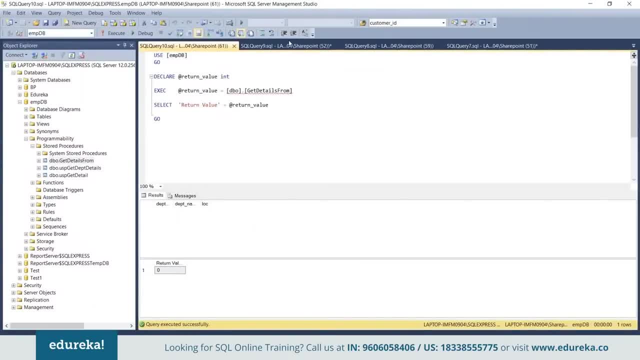 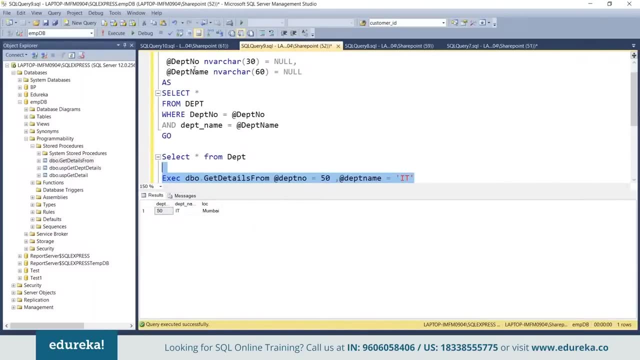 though there won't be any result in the results end. but it won't show any error because while creating the store processor, we have defined that these two parameters can accept null value, So they are not mandatory. these are optional. That is the reason, even though we won't provide any value, 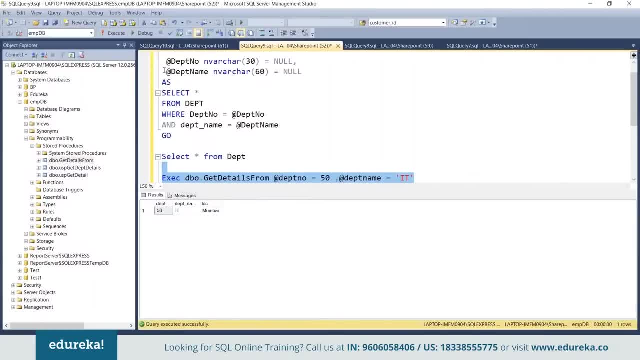 we won't receive one While executing the store processor. Now let's discuss about the output parameter in the store processor. So if we want to return the value of the parameter, then we have to define an extra keyword that is out or output. 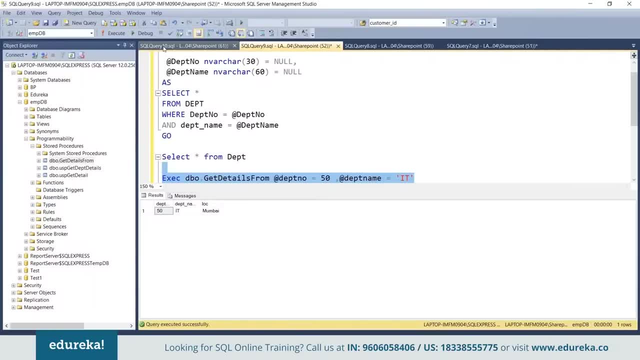 Both keywords are valid, whether we use out or output against the name of the parameter whose value we want to return. So let's see it with an example. So I'll open a new query In the store processor. I have two parameters. 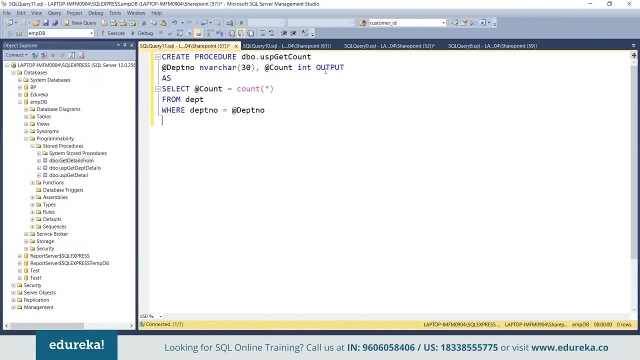 One is the department number and one is count. So we have defined a keyword output which suggests that this parameter will be the output parameter, So we can pass the value to this parameter. and this parameter will also return the value after execution. So we can provide the keyword output or out. 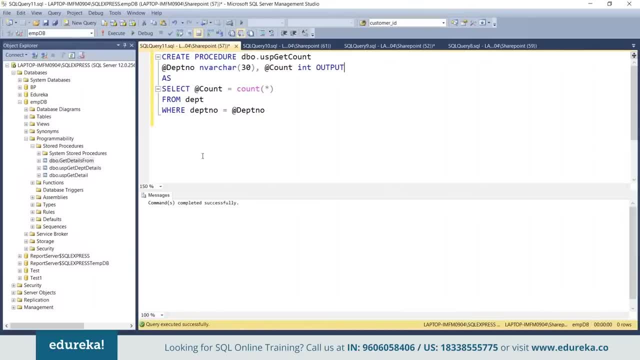 There's no difference. The end result will be the same. So that's created. We'll refresh the node of the store processor To see the results. Yep, we have the store processor Now. in order to execute this, we have to do like this. 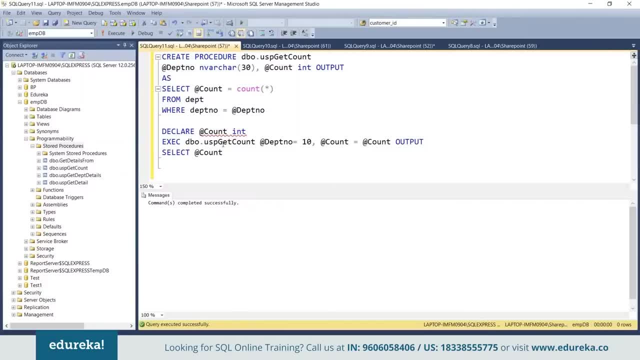 We have to first declare the count, int, followed by the executive name of the store processor. We'll provide the value. This is how we have to define if it is an output parameter, And then we are writing the select statement to see the value of the count. 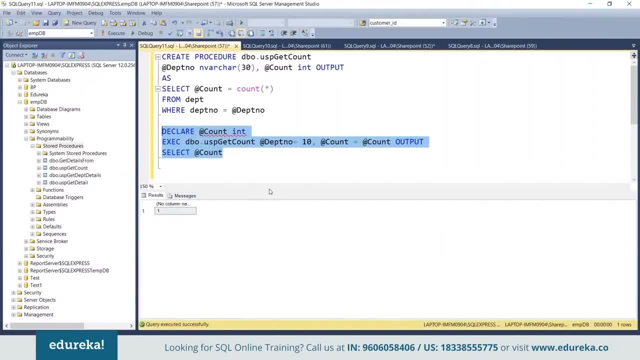 So let me execute this. So the count is one, because there's only one row with the department number 10.. So this is how we use the output or out keyword against the parameter. Now let's see how we can add comments in the store process. 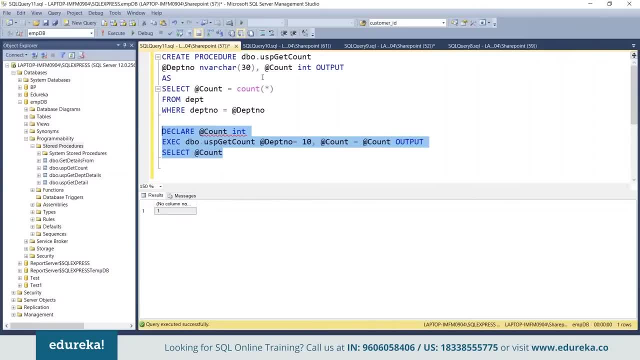 So we can add the comments in two ways: One is the line comment and one is block comments. So if you need to provide the line comments, then we have to use two dash followed by a statement, And, in order to forward, slash and then star. 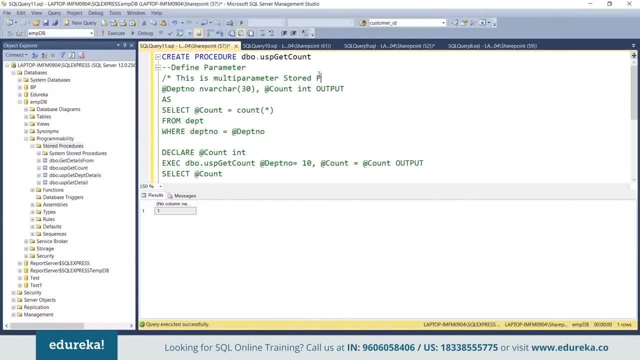 I'm just writing. this is multi-parameter store processor Having output parameter. Again, we'll write star and a forward slash. So this is how we define the comments in a store processor, Not only in a store processor. we can write or define the comments. 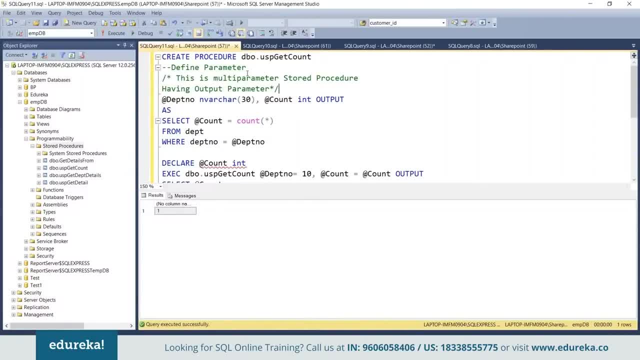 anywhere in our SQL queries, Whether it is a functions or normal SQL statements or it is a store processor. So line comments or single line, we use two dash And for block comments we use forward slash and star. So let's see how we can handle the exception. 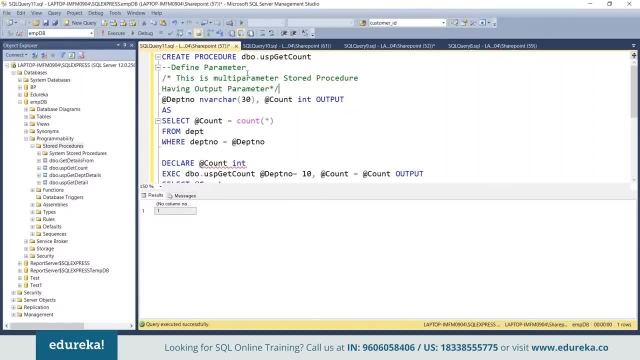 in the store processors. So if you have handled the exceptions in your programming languages like C, C++ or like Java or C sharp, Then we use try cache there And along with try cache sometimes we use finally block, because finally always execute. So if you want to close some, 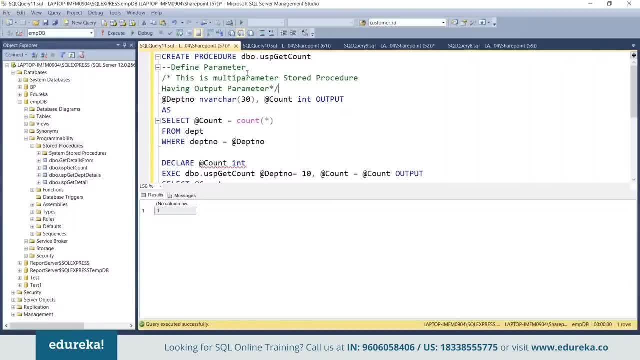 like, we want to close some connections or we want that some statement to execute, no matter whether there's exception or not, Then we write those statements in the final block, So we do not have any final block in the store processor or SQL. Let's see how we can define the try and cache blocks. 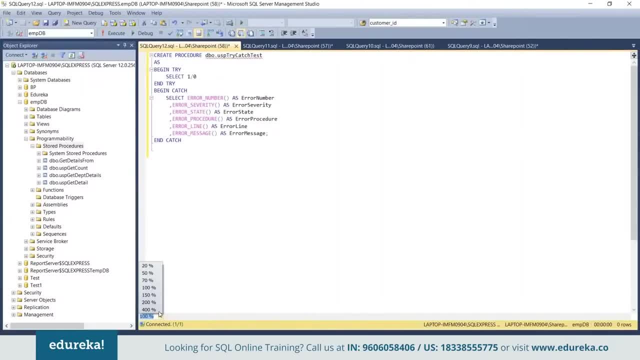 in the store processor. With an example, Let me first increase the font size. I'm creating the store processor with the name dbo-usb-try-catch-test And to write a catch block we have to provide the syntax begin try. 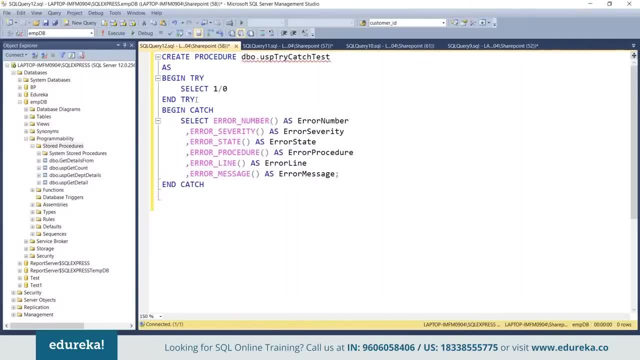 Then in the body we'll write whatever the statement we want to write And then followed by the end try, So end, try basically ends the try block. After that we'll provide begin, catch And in the catch see what we are doing here is that. 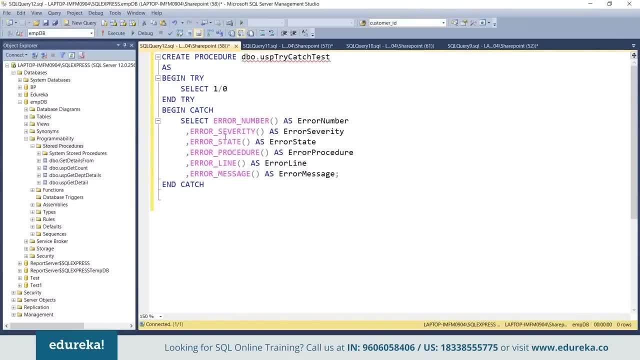 we have written a select statement that we are providing. what is the error number? What is the severity of this error? What is the state processor in which line the error is encountered and the error message? So let's create the store processor first. 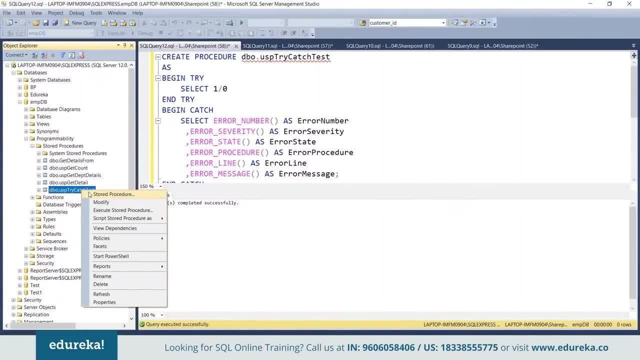 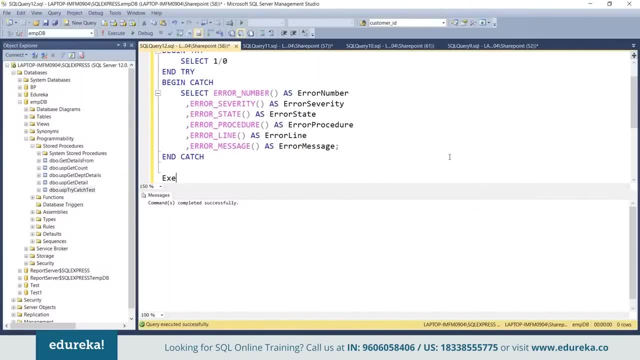 And then we'll refresh this node. So we have the store processor And now the store processor do not have any parameter, So I'll execute the store processor. Execute keyword followed by the name of the store processor: No parameters. so we are not passing any parameters. 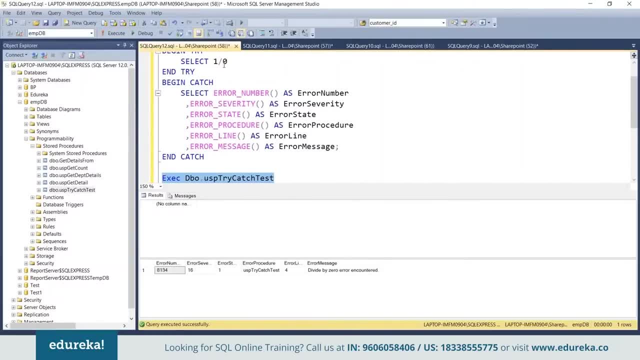 while executing it. And see, since we are dividing by zero, it will give an error, It results in infinity. And see, since it will go to the catch block, since error has encountered. So we have written the statement in the try block. 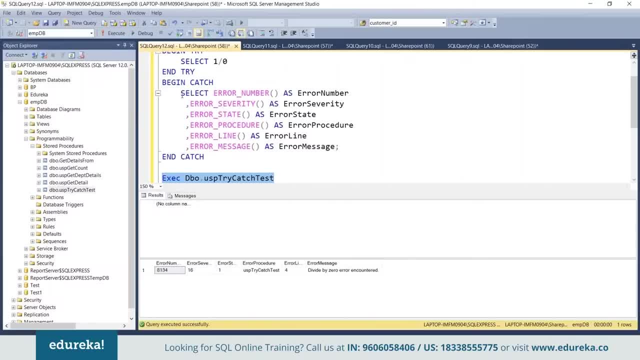 So in the catch we are handling the error number, handling the exception and while handling the exception, we have written a select statement which provide all these values. So the error number is at one, three, four error severity is 16, so these are the you know. 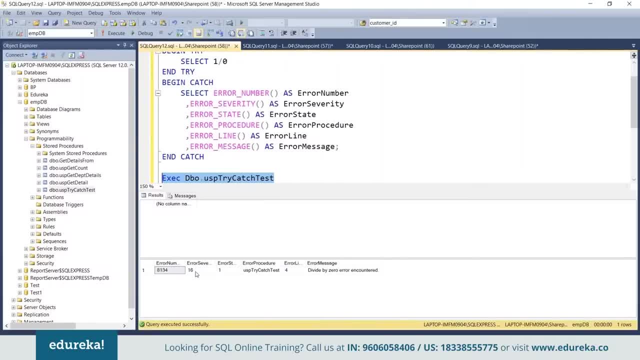 predefined severity levels So we can check on. Google said what the severity error, severity 16, means. Then we have error state in which process of the error has occurred. so it will give you the name of the processor. The name of the processor is USP. try catch test. 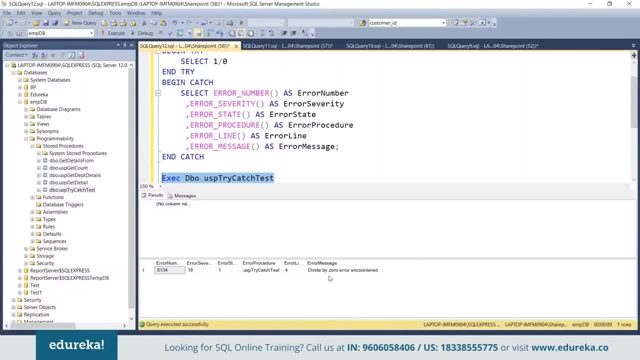 Error line is four and the error message that we are dividing by zero. So we'll get the message that divide by zero error and countered. So this is how we mentioned try catch block in the stored processor. We have seen various examples of the stored processor. 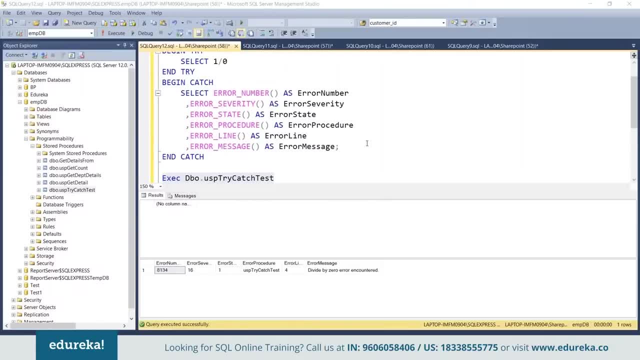 So we have created the stored processor without parameter with parameter. We have created a stored processor with multiple parameters. We have seen that, how we can, you know, include comments in the stored processor using single line comments or block comments, And we have seen that, how we can handle the exception. 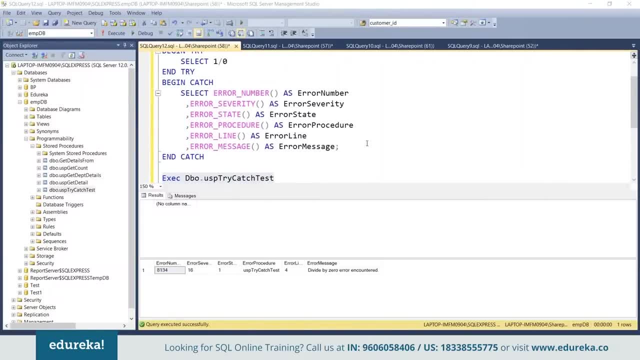 in the stored processor. So this exception handling is not only for the stored processor. we can handle these exceptions in functions as well. So we can write try block and followed by a catch block. In the catch block again we can write the select statement. 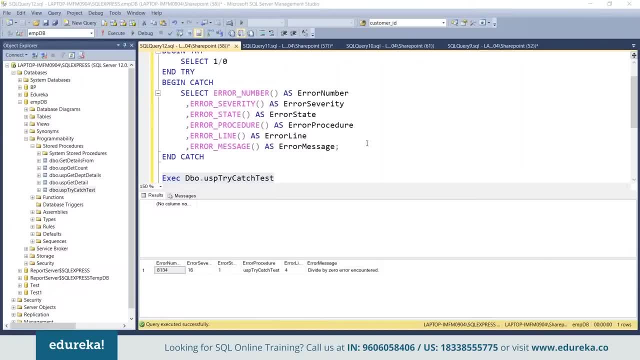 to show the message that where exactly? what is the severity level? what is the error message? We can even provide the custom error message. it's up to us. So let's move to the next topic. So I hope you are clear with the concept. 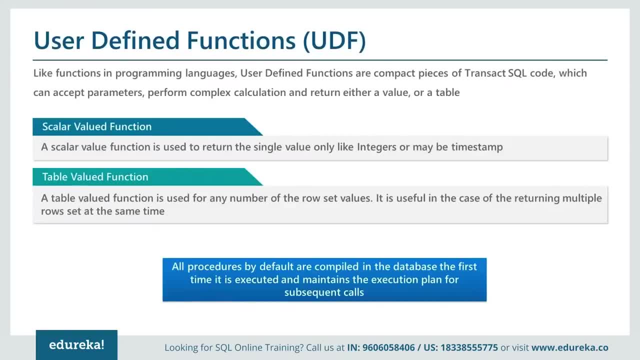 of stored processor in SQL. Let's move to the next topic. The next topic is user defined functions. So, though SQL Server provides list of many predefined functions that are built into the T-SQL language, these supplied or out of box functions helps in extending the capabilities of SQL. 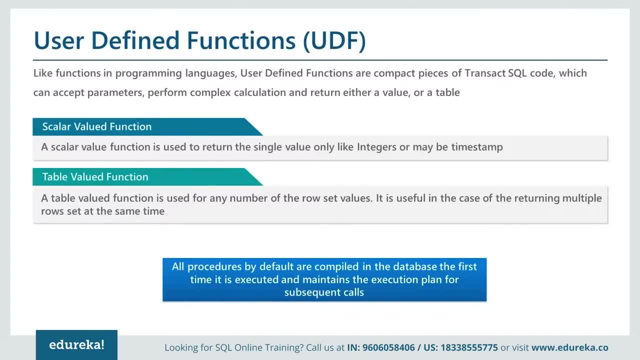 by providing the ability to perform, like string manipulations, mathematical calculations, data type conversions by using convert or cast functions, et cetera. But sometimes these out of box functions or inbuilt functions are not enough And there are certain functionalities which is not provided by these functions. 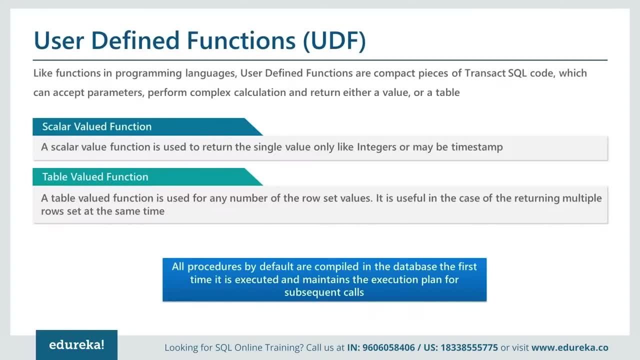 So this issue can be easily addressed if we can create some user defined function. So, like functions in programming language and all programming language, we write functions. There are some functions which do not return any values. they are functions which returns a value and we pass parameters. we do not pass parameters. 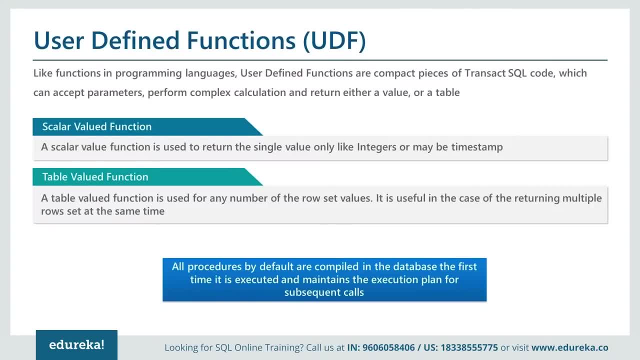 while you know calling the functions. So user defined functions in SQL are almost on the same lines of the functions in other programming languages. So user defined functions are compact piece of transect SQL code which can accept parameters, like how we pass the parameters and store process the same way. 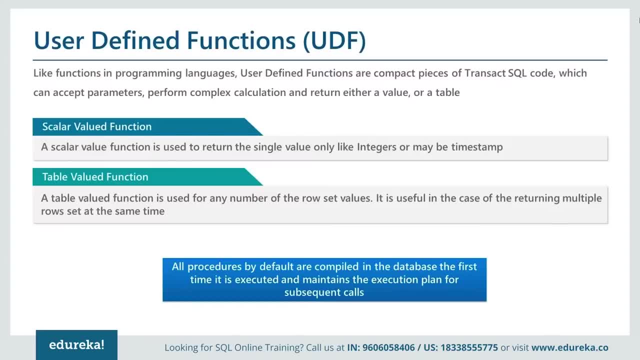 Functions can also accept parameters. Functions can perform complex calculations and return either a value or a table. So this return type is basically based upon what kind of functions we are creating or executing. So let's discuss what are the various benefits of user defined functions. 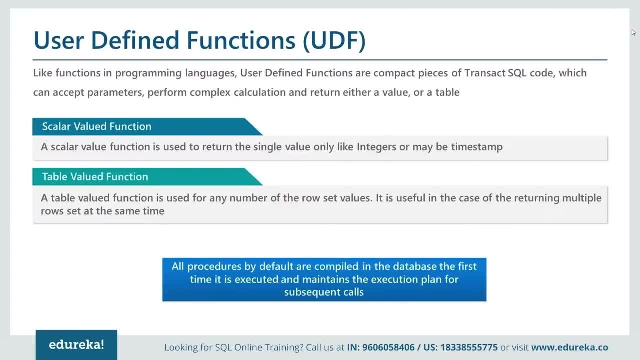 So again, like store processor functions also helps us in achieving the concept of reusability. It will prevent us from writing same logic multiple times. We can dump a set of SQL statement in a function and we can call it as many as times. 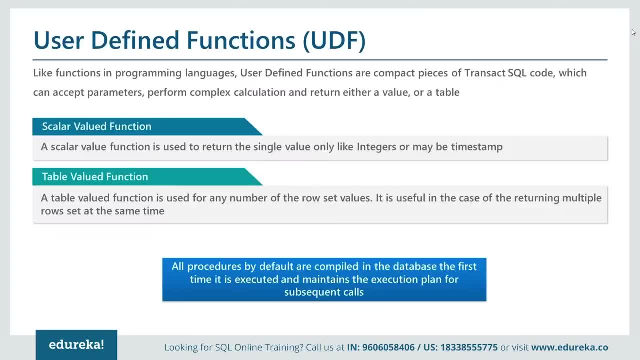 Like store processor. they also improve the performance because the user defined function reduce the compilation time of SQL query by caching the execution plan and reusing it. Functions are also easier to maintain Because functions help us to separate the complex calculations or the complex business logic. 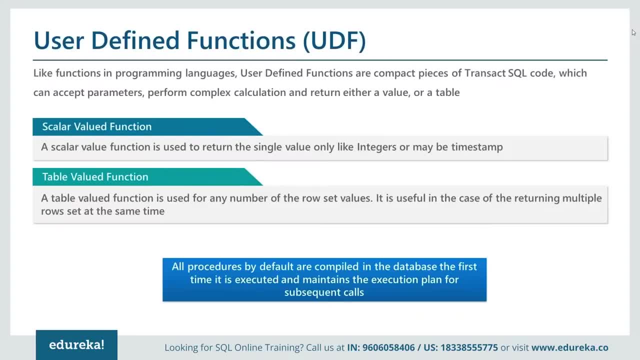 from the regular SQL query So that we can understand and debug the query quicker and better. It again reduce the network traffic because of its caching. plan Functions again can be used in where clause as well. By this we can limit the number of rows sent to the client. 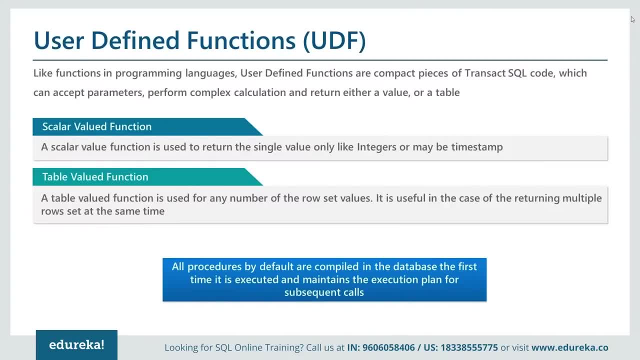 So we can use functions in select the function and we can use the functions in where clause. Now let's discuss about the structure of the functions. User defined functions are composed of two parts. One is header and one is function body. We'll see in some examples that how we create functions. 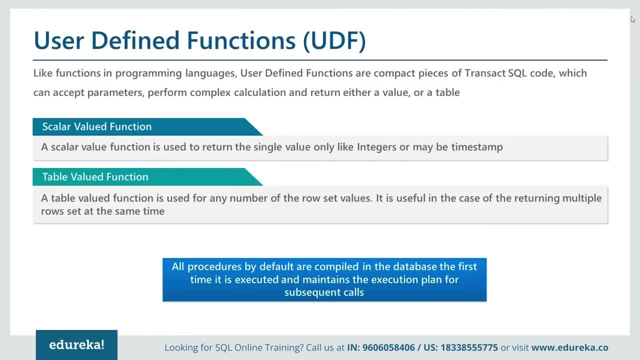 So the header contains the function name- input parameters- if there are any input parameters, because, again, the parameters are optional, whether it's the store processor or whether it is a user defined function. Along with that we have the function name. 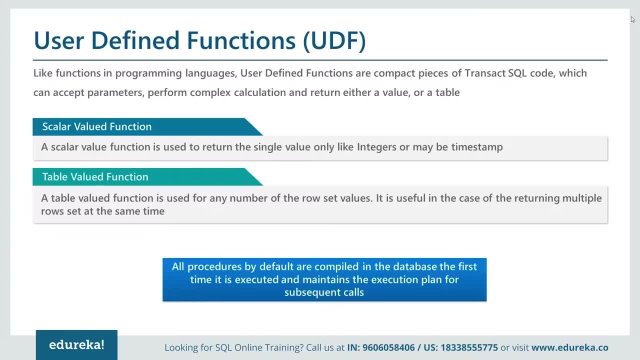 Along with parameter, we have written parameter info, its name and type, in the header section. The function body contains the logic, any business logic. So it contains one or many SQL statement, depending upon what we are writing in the function body, As you can see on the screen. 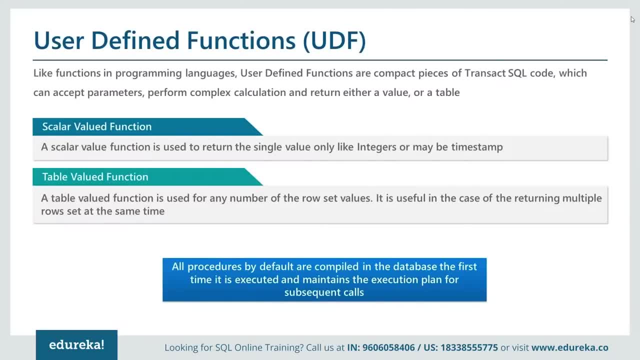 there are. if you need to divide the user defined functions in some broad category, then we can divide into two broad categories. One is the scalar value functions and the other is the table valued function. The table value function can again be divided into a line table value functions. 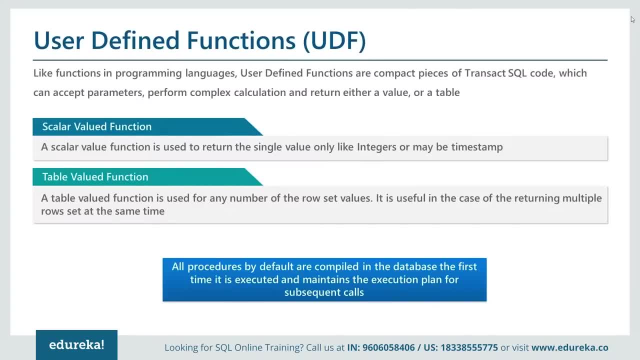 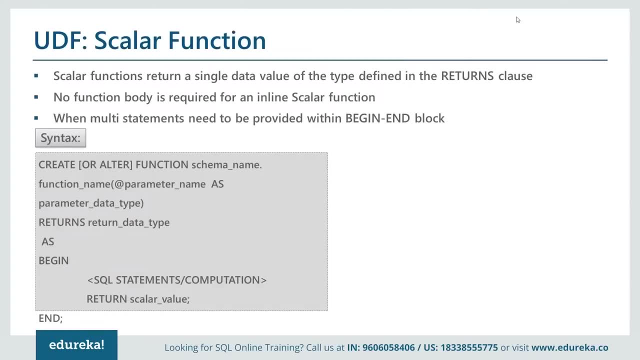 and multi statement table valued functions. Let's move to the next slide. Let's first discuss about what are the scalar functions in SQL. Scalar functions returns a single data value of the type defined in the return clause, If it is a line scalar function. 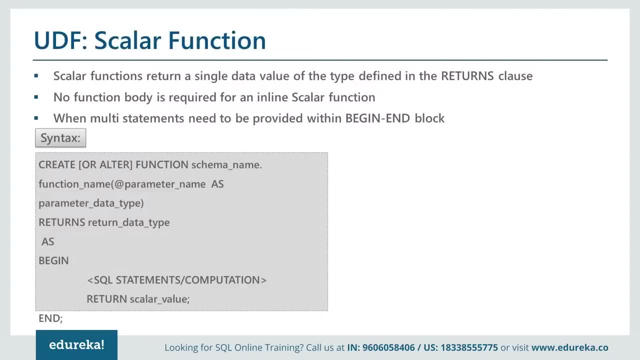 we even don't need a function body- Scalar functions- when multi statements need to be provided within beginner and block. So let's discuss about the syntax. As I mentioned that, the syntax contains header and body, So the create alter function, it is basically the header of the functions. 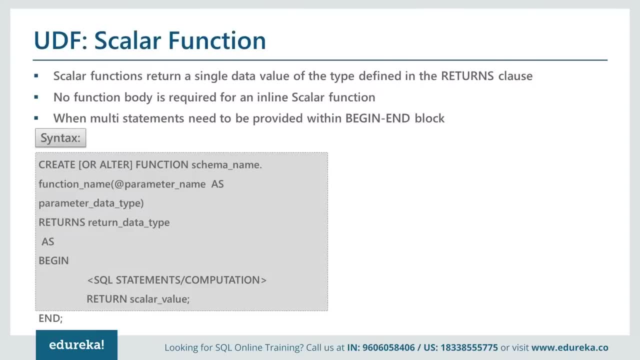 In the header we can define the parameters, the return type parameters, And then in the beginner and we define the function body. What are the SQL statement or any computations or any calculation Which we are doing? we basically do it in the body of the function. 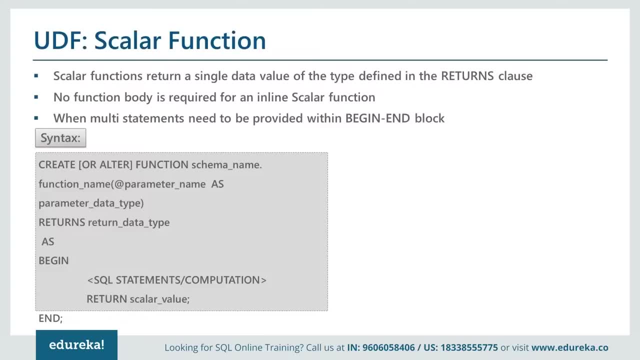 So, if we need to summarize, the scalar functions are functions which returns a single value. They return scalar values or single values that can be used anywhere. a constant expression can be used And every function, whether it's a scalar or whether it is like table, value functions. 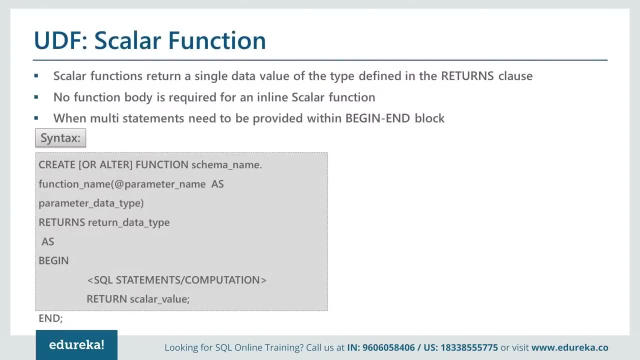 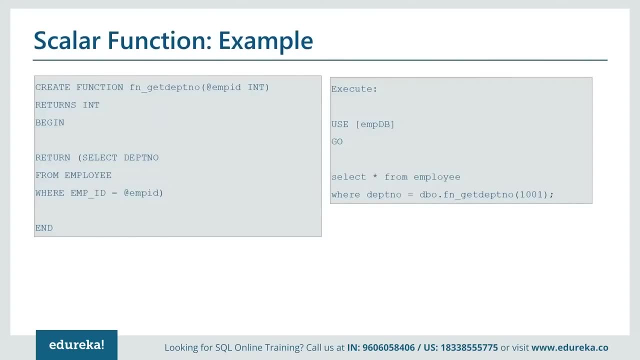 every function must return a result using the return statement. This is kind of mandatory. So let's see some examples of the scalar functions. So in this example we are creating a function with the name FN, underscore- get department number. So we are creating a parameter: employee ID. 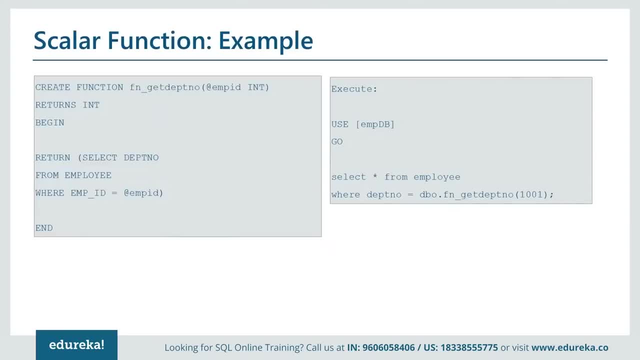 of the data type int. here This functions basically returns int data type. Then there's a begin keyword. After begin keyword we are defining the body. The body we are writing select department number from employee Where employee ID is employee ID. Where, at the rate, employee ID is the parameter. 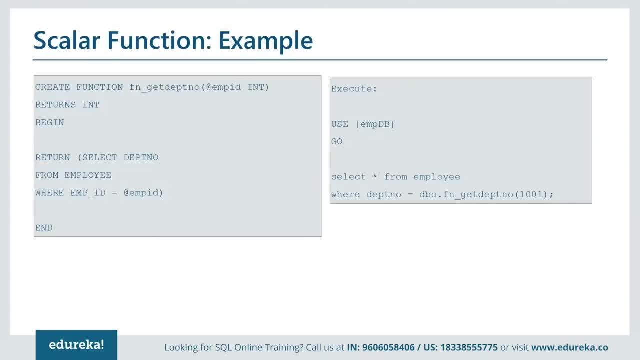 which will pass when we execute this function or will run this function. So, the right hand side, we are executing these functions and we are executing these functions in the where clause, Just pay attention. So the where clause we are mentioning where department number equals to: 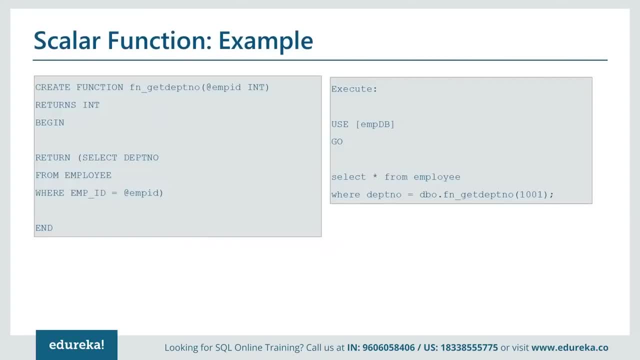 and then we are calling the function by providing the parameter. So when this function will execute, it will be replaced by the value which the function will return, And then that value will be used in the where clause to filter the data. So let's discuss some examples of functions. 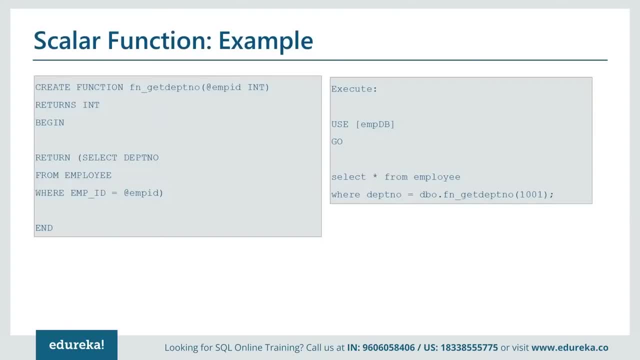 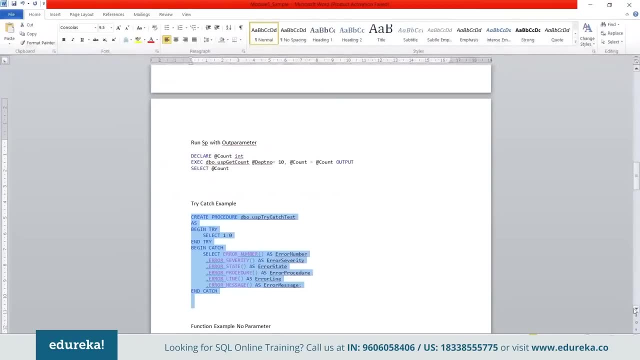 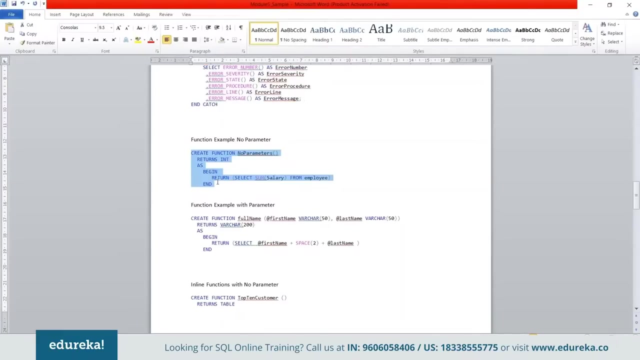 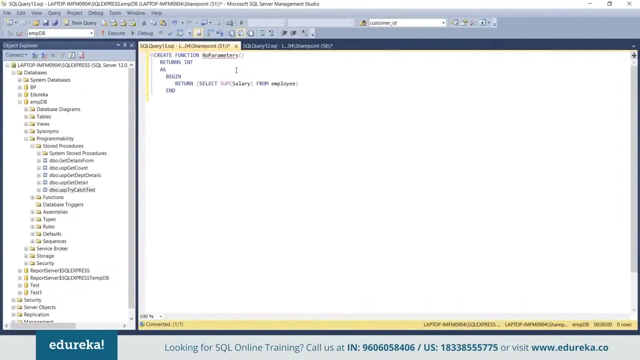 for better clarity, Let me open management studio. Let me close these queries first. So we'll first create a function, a scalar function, without any parameters. So this is the name of the function: no parameters. We are not creating any parameters here. 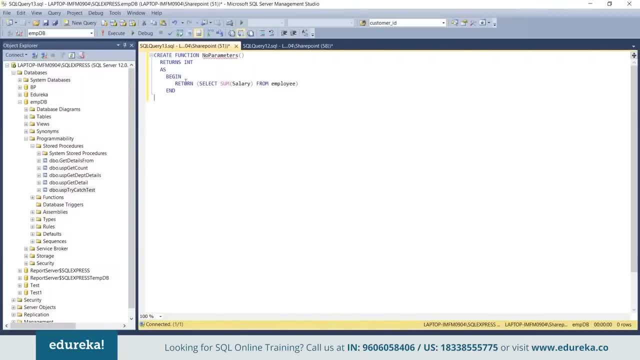 The return type is int And I'm just returning in the return statement. You have just provided a SQL statement that select some salary from employee. After executing, this function will be created. This is a scalar function, So if you want to verify whether the function 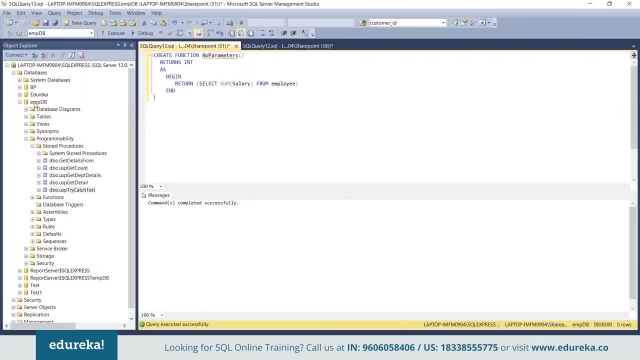 has been created successfully, then we have to refresh our database. So we have created this function in employee DB database. I'll refresh that and I'll expand the programmability. In programmability node we have sub node called functions. Again, in functions we have four nodes. 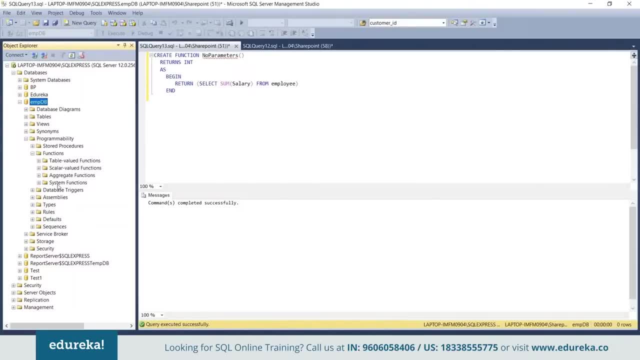 table: value functions, scalar value functions, aggregate functions and system functions. If I'll expand the scalar value functions, we can see the name of the functions here. So in order to execute this function, we have to write select statement followed by the name of the function. 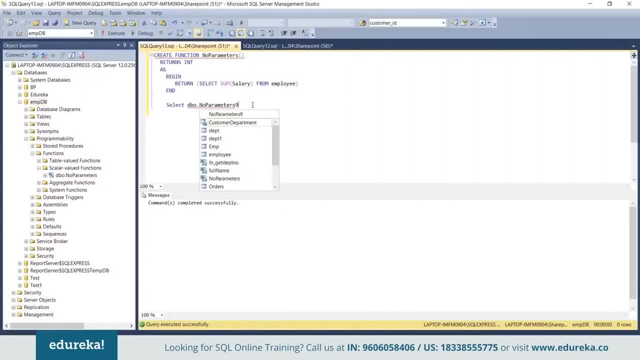 If I'll execute, we have to write the parenthesis, So this function will return the sum of the salary from employee table. So let me show you the data which is there in the employee table So that we can verify our result, whether we I got the right result or not. 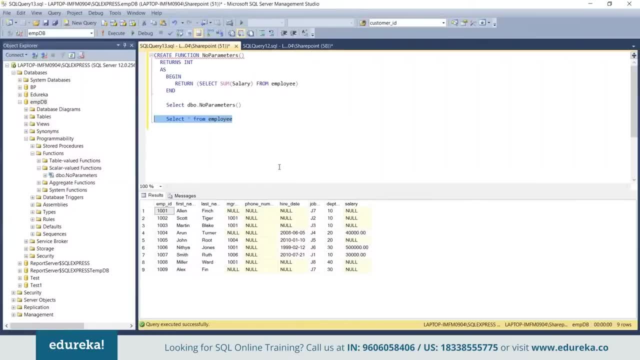 So if you'll calculate this, we'll get 570K. This is the sum of the salary for all the employees, Since we have salary for the three employees, three employees only. So this is how we'll create the functions, without any parameter. 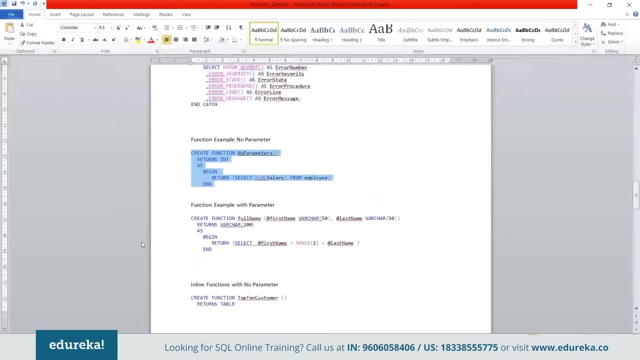 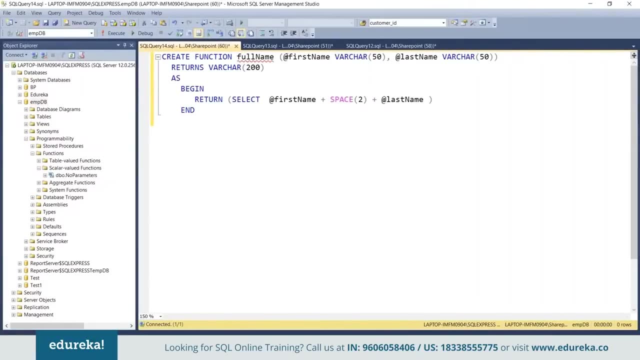 Let's see how we can create a functions with parameter. So in this function we are providing two parameters: first name and the data type of the parameter is varchar50.. The second parameter is the last name and the data type of second parameter is, again, varchar. 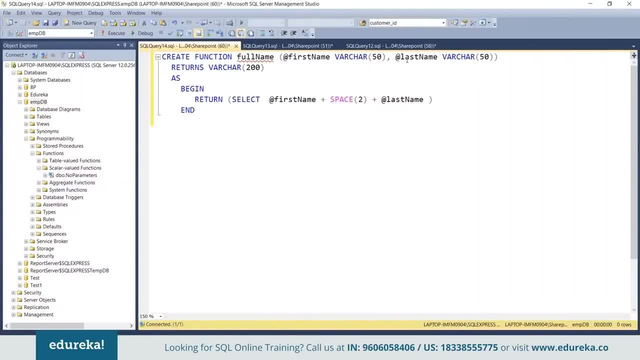 with the same length as of the first parameter. Return type is also of the same data type, And then in the body we are executing the SQL statement. So what we are doing, we are just concatenating. So if it is a mathematical operations, 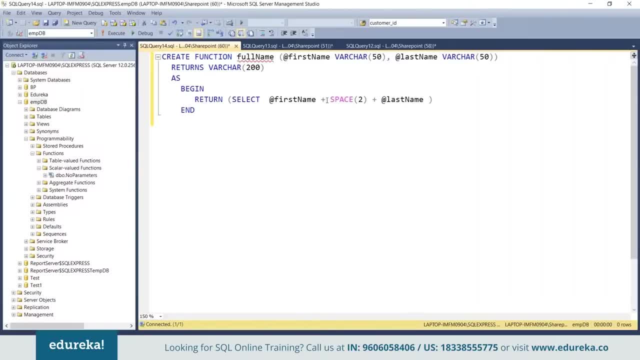 if we provide the plus operator, then we'll add the two values, But if it is string or varchar, then it will concatenate the string. Space is a function and it is an inbuilt function in SQL, which basically add a space, empty space. 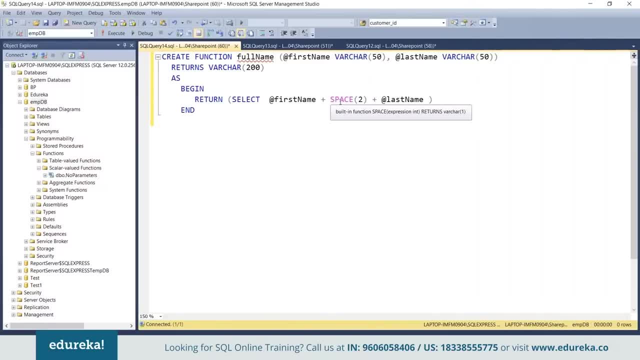 so what we are doing, we are concatenating first name and last name and we are adding a space between the two names to make it more readable. So, as you can see, when I'm hovering over the space, a keyword, it is giving me a message. 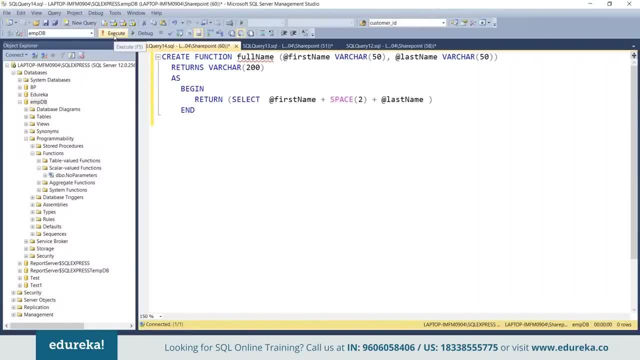 that this is a built-in function, So let me create this function first. Function has been created Again. this is a scalar function, but with parameters. Let me refresh the scalar valid function node and I can see the function Function name. 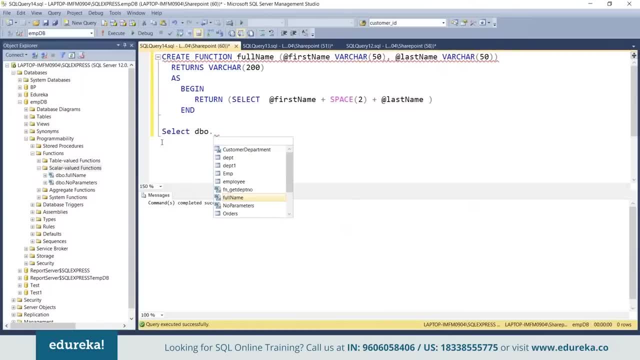 Let me execute this function- name of the function- and then we have to pass the parameters. So I pass two parameters here- comma- and then even the second parameter Why I'm enclosing it in single code: Because this is a string type. 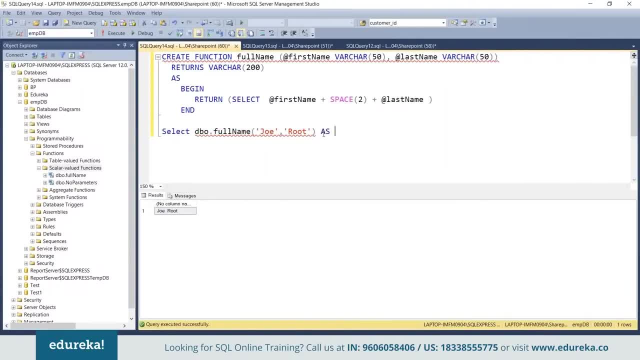 and if you want to add an alias for the column name, we can mention it as full name. So if I'll execute it again, we'll get the result your root here. So this is how we'll create a functions with multiple parameters. 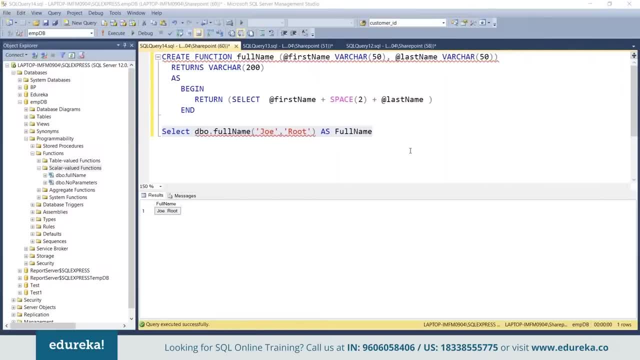 And we can call the functions in the select statement, or we can- sorry, let me call in the select statement, right, and we can even call the functions in WebClaus, as we saw in the example in the PPT- Again, the previous example. 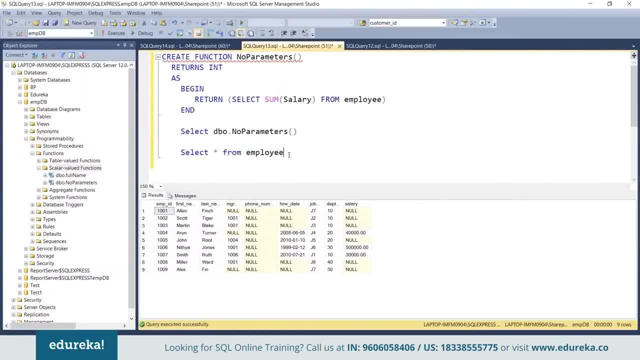 let me first increase the font size. We can even use the functions in the WebClaus right. You can even use the functions in the WebClaus right in the day clause. so how we can use it. let's assume I'm calling this query. select star from. 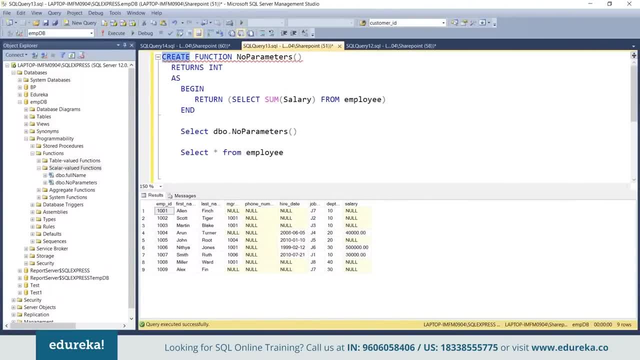 employee and let me first alter this function. so to alter this function, we have to use the alter keyword and instead of some I'm just finding the average salary of the employee. then I'm executing again. so this is how we modify the function, existing function. same way we can. 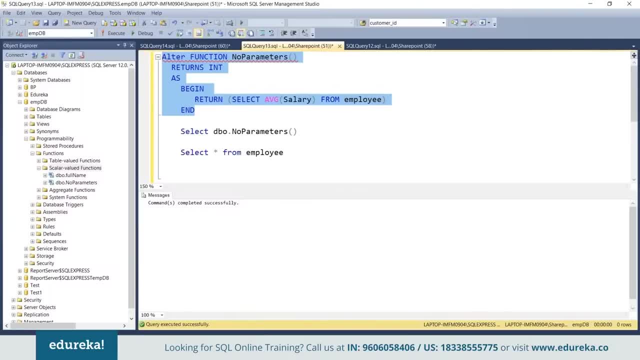 modify the store procedure also. so alter is the keyword which helps us to modify the existing functions as well as existing store procedure, if I have to use the functions in the way clause. so this is how we'll do. let me show you. so I'm writing a query, so what I want to do is that I 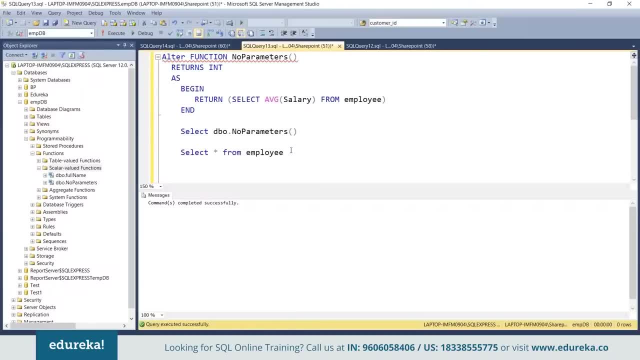 want to select the employees whose salary is greater than the average salary. so I'll write back class where salary is greater than the average salary. so I'm writing where loss where salary is greater than the average salary. so I'll right where clause where salary is greater than the感覺. 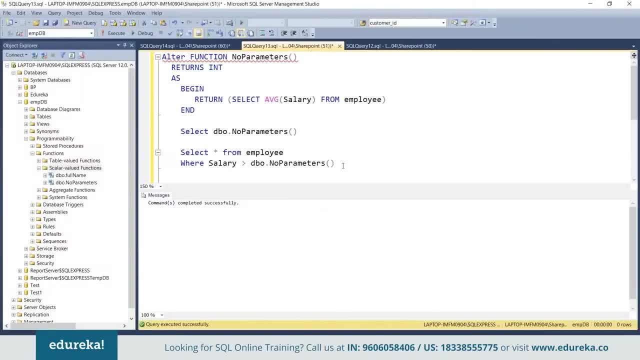 or greater than then I'll call the function. So if I execute it now, I'll get only one result, because there's only one record of one employee whose salary is greater than the average salary of all the employee. So this is how we can include. 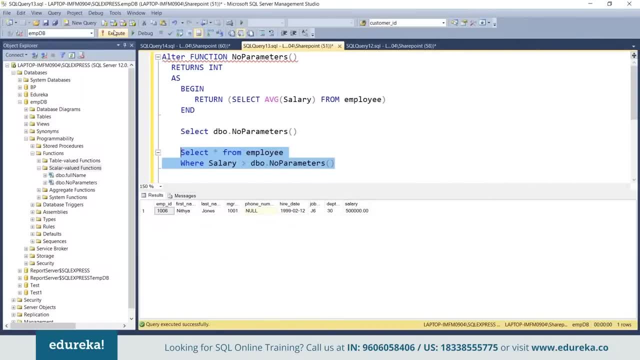 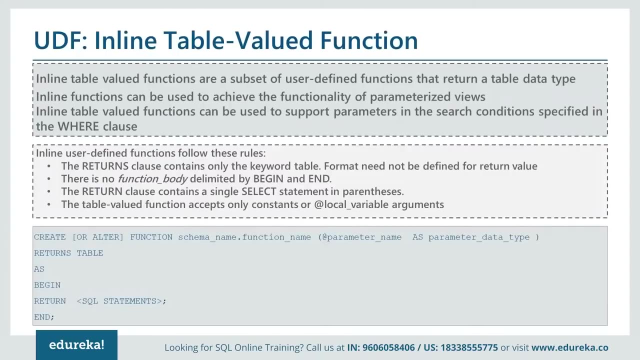 or we can call the function in where clause as well as in the select statement, as per our business requirement. So let's move to the next topic. So we are clear with the scalar functions, I believe. So let's move to the next type of function. 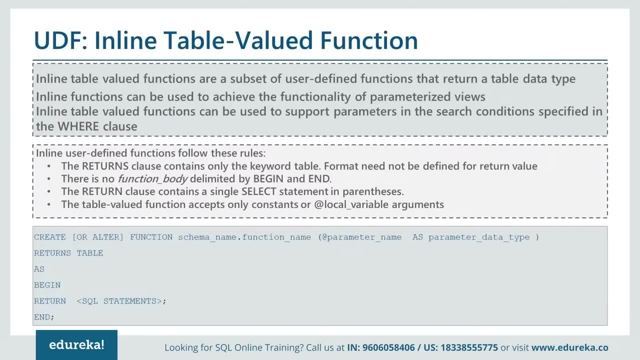 that is, the table valued functions. And, as I mentioned earlier, we have two types of table valued function. One is inline, one is multivalued. So inline table value functions are a subset of user defined function that returns a table. So scalar functions returns only single value. 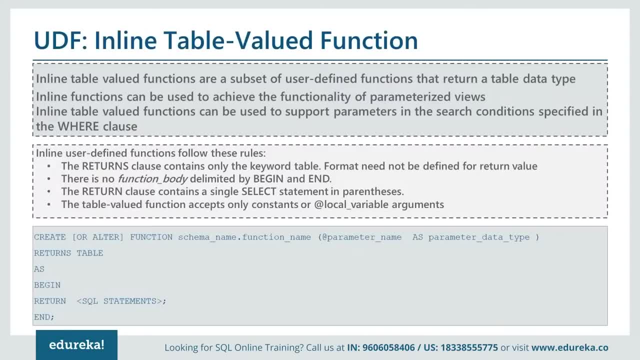 whereas the inline table value functions returns the entire table. So inline functions- if you remember, we have created view in a first module, So we can use inline functions. if you want to achieve the functionality of parameterized view, Inline table value function can also be used. 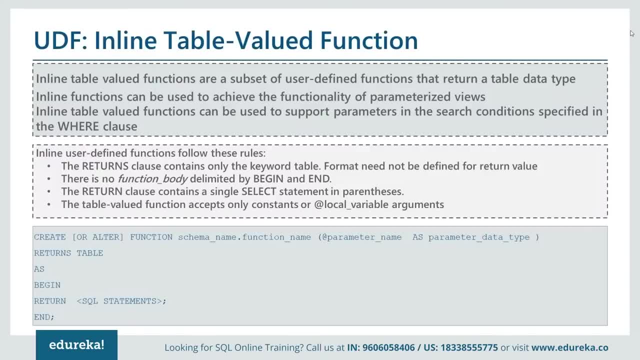 to support parameters in search condition specified in the where clause. So these are some of the rules which are common for the inline table valued functions. The return clause contains only the number of table valued functions, is only the keyword. table Format need not to be defined for the return value. 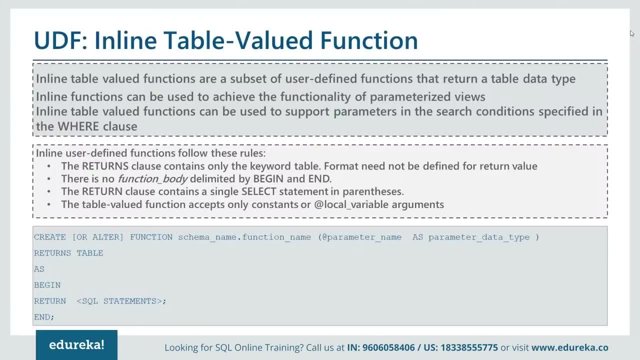 There's no function body delimited by begin and end. The return clause contains a single select statement in parenthesis and the table value function accepts only constants or the local variable arguments. This is the syntax for the inline table value functions, as you can see in the slide. 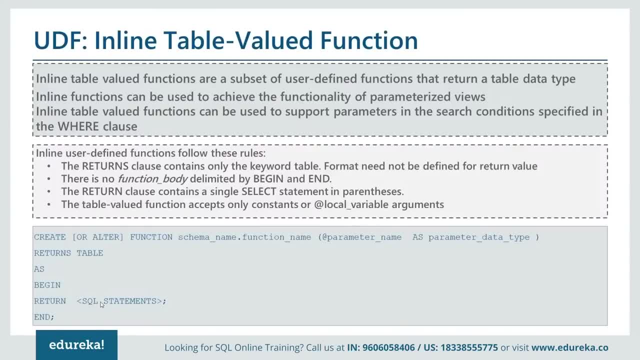 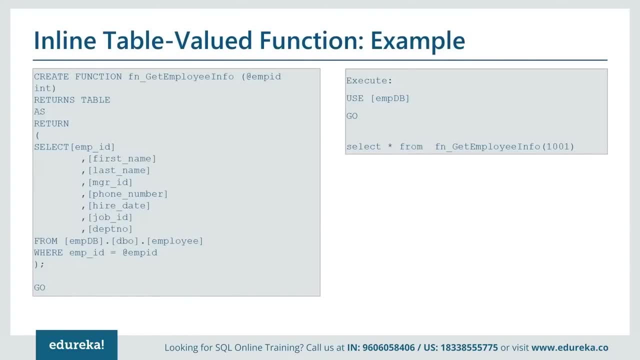 So the return type is table here and we generally have the SQL statement. So this is an example. The last slide, we saw the syntax. this is the example. So here in this example we are creating a function: get employee info. You're passing the parameter employee ID. 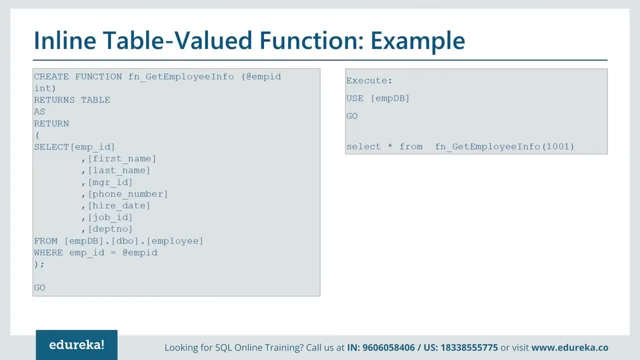 and it is returning the values as a table, not as a single value, And the return statement. we are providing the select statement where we are returning the values of employee table and we are filtering the results ends by using the parameter employee ID, And this is how we'll execute. 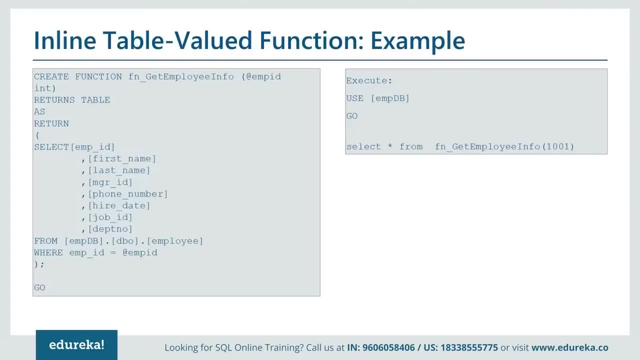 So, if you remember, when we executed the scalar value function, we did not use select star from. We simply mentioned select and the name of the function. But if you are using table value function, then we are using the select star from because we are kind of, as you mentioned, 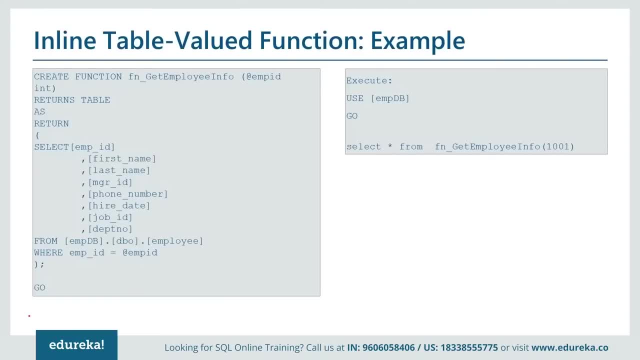 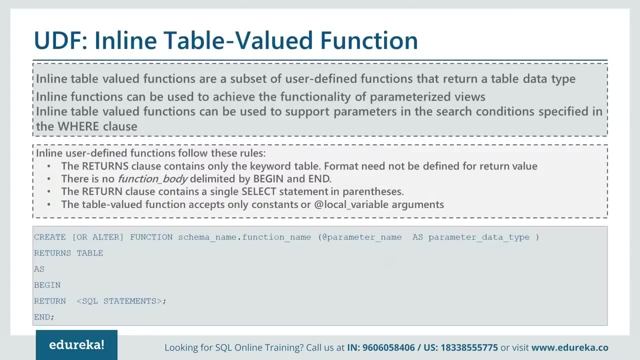 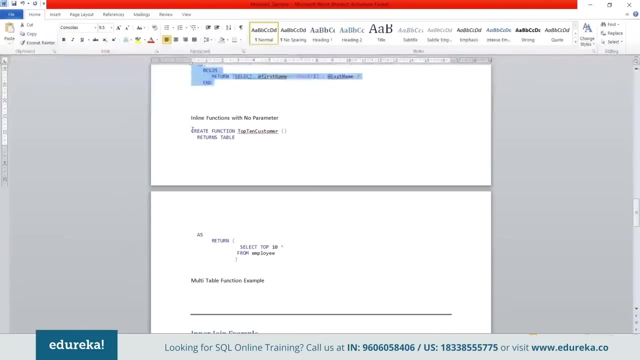 we kind of use it for parameterized view. So if you need to fetch the values from view, then again we use select star from the name of the view. So let's see an example of inline table value function. Let me open management studio. 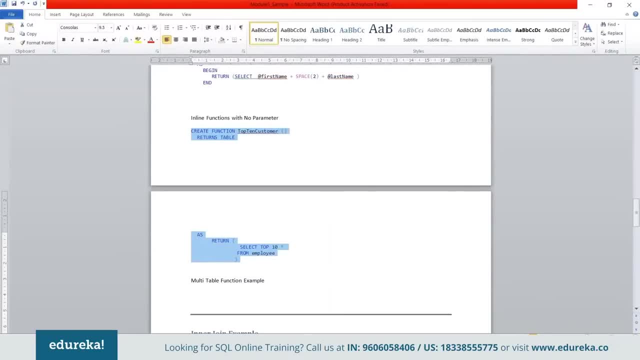 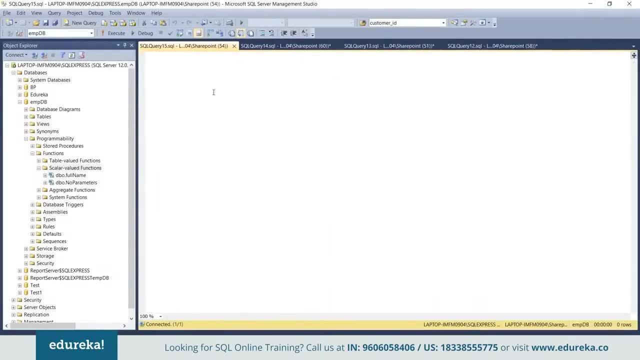 So this is example of inline functions with no parameter. We can create parameter in the same way we created the parameter or we define the parameters for the scalar value functions. So I'm creating a function, top 10 customers. We are returning a table. 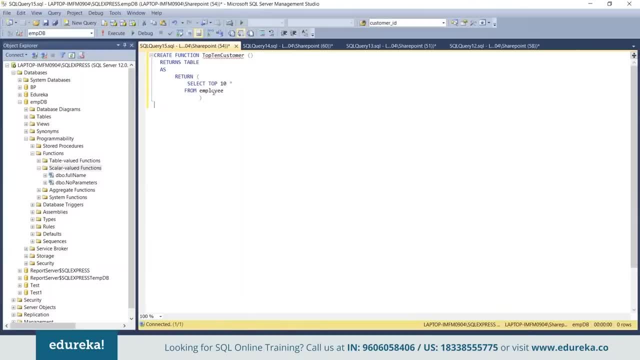 And in the return statement I'm just writing: select statement. select top 10 from employee. Let me execute this to create this function. Now I'll execute this function. So to execute this, I have to mention the select class, select star from, and then the name of the function. 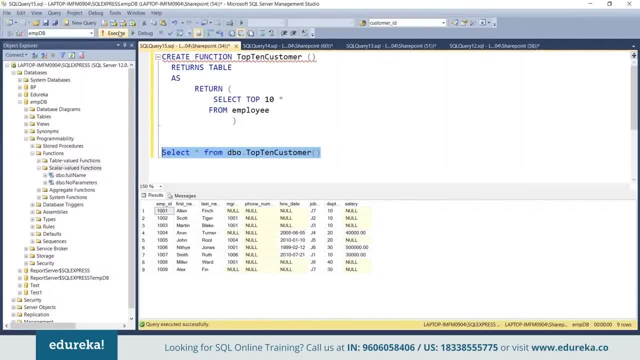 So I'm getting. so there are only nine rows, so it's just fetching the nine only. So, if I can go ahead and modify it, instead of top 10, let me modify it. Let me modify it to top five. So to modify the function, we have to use the alter keyword. 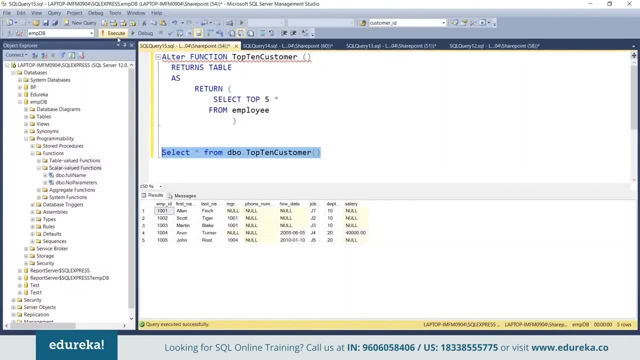 So we got the top five results. This is how we create the inline table value function. So this is example of the functions without any parameters. If required, we can go ahead and create a parameter as well. So to create the parameter, we have to define the parameter name here. 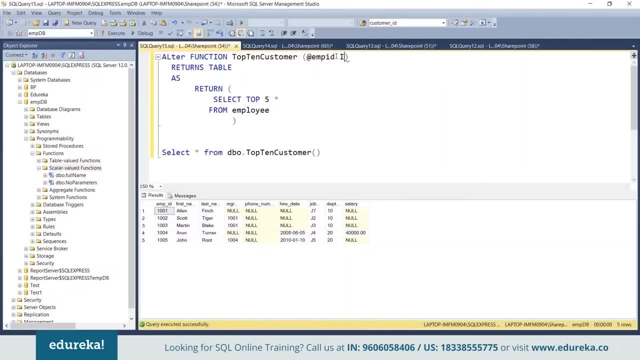 And then we can. we have to provide the name of- sorry, the data type of a parameter And then we can write a where clause. Now, let's say, where employee ID is greater than employee ID. Come on, execute it successfully. 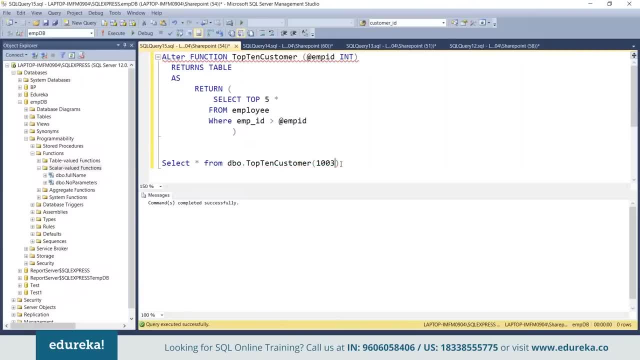 And now, if I to run this, I'll pass a value to the function. If I'll execute, it will get the values And the result set whose employee ID is greater than 1003.. I hope this is clear And let's move to the next topic. 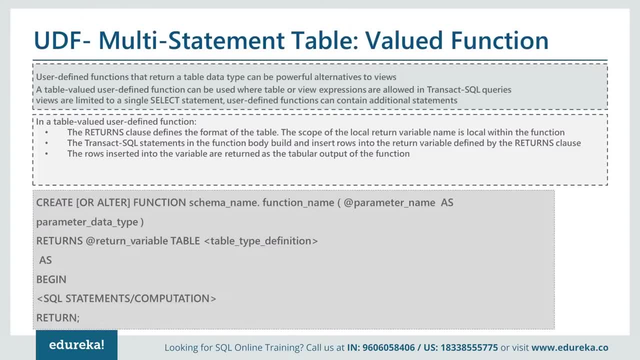 So we'll discuss the next category of table valued function, that is the multi statement. So in the inline function we can use a single statement, But in multi statement table valued function- we can use multiple statements. So again, they also return a table data type. 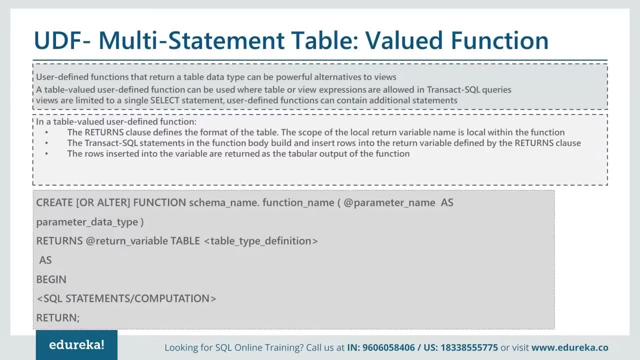 So the return clause defines the format of the table. We cannot provide the format in the inline table value function but yes, we can provide the format. We can provide the format of the table in multi statement table valued function, The transact SQL statement in the function body. 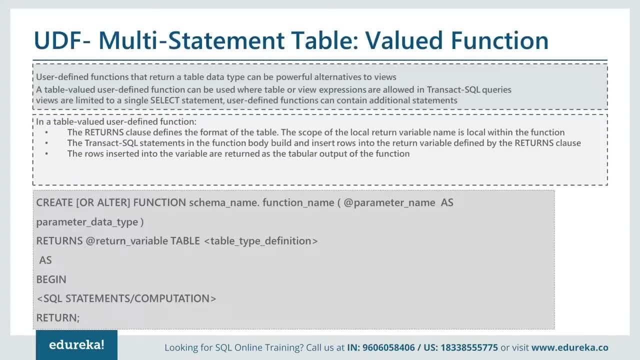 build and insert rows into the return variable defined by the return clause, And the rows inserted into the variable are written as the tabular output of the function. So here we have the syntax for this. To modify, we use altered keywords. To create, we use create keywords. name of the function. 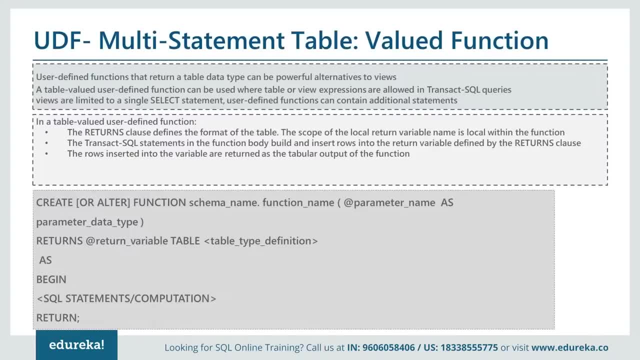 If you wish, we can define the parameters which you can consume In the function body. return type will always be the table, But here we can define the format which is not available in the inline table: valued function. Let's see an example. 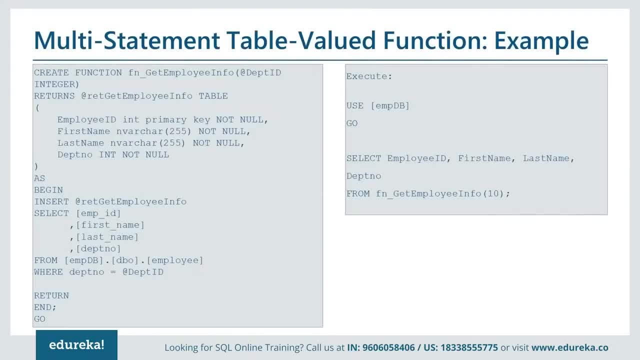 So this is an example here. So we are defining the format of the table and we are defining, like that, this: the table will be the retired get employee info and we are providing four columns here and we are defining the data type, We are defining the constant on the table. 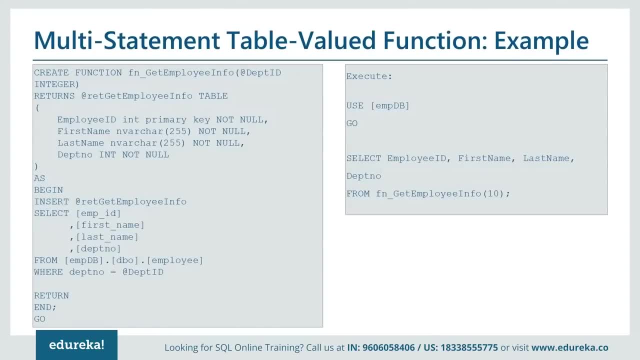 We are defining whether there's a null constraint or not on those columns And in the function body, we are inserting records in the table and we'll fetching from the employee and we are filtering the results set by using the parameter which will pass when we'll execute the function. 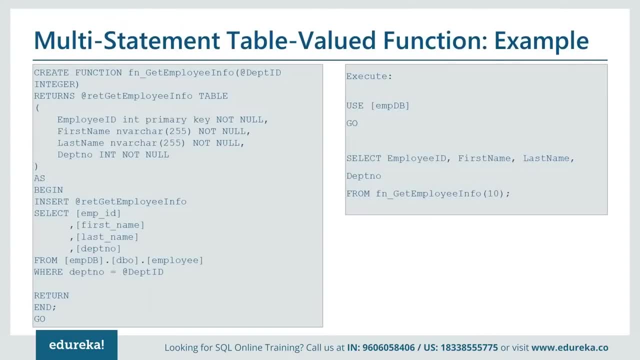 So let's see one more example other than this, So you can use the same example and execute it. We'll try to write the entire thing. then it will take time, So I'm skipping the example in management studio, But the basic difference between management studio. 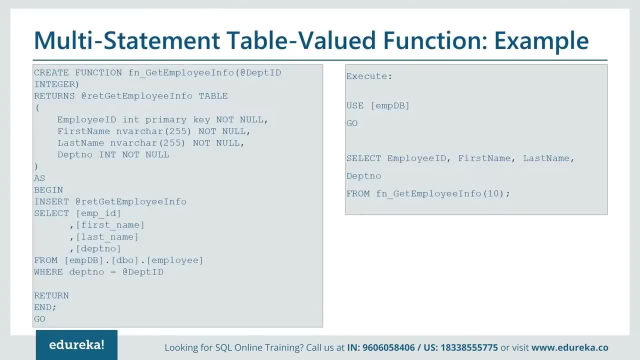 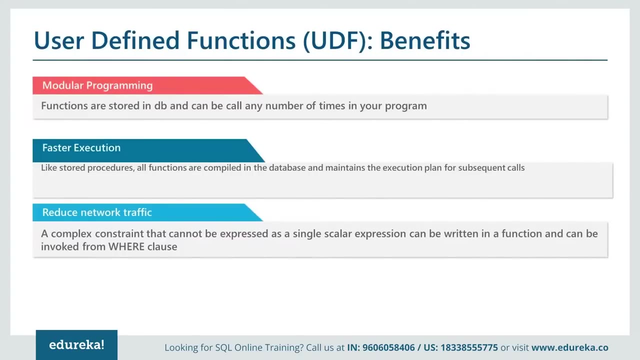 and the table valued function is that here we can format the table and we can use multiple statement in the function body, which is not the options in the inline functions. So we already discussed the benefits of user defined functions model of programming. It saves time because we can write. 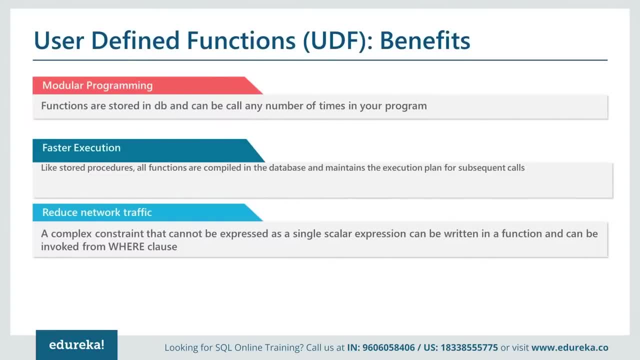 or dump the statements in a function and use it or call it as many as number of times. It's faster executions. because of this, It caches the execution plan and use it for the subsequent calls, and it reduce the network traffic. So these are few of the main benefits. 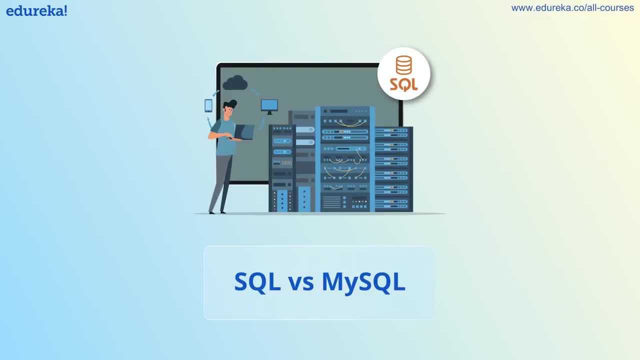 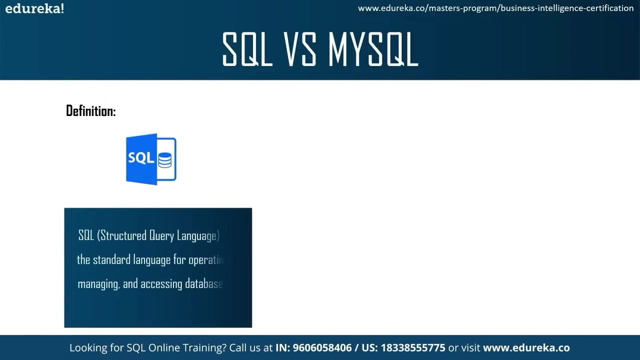 of user defined functions. Now let's come to our topic, that is, SQL versus MySQL. So as the first topic of comparison, we have the definition. So what is the definition of SQL? SQL is the standard language for operating, managing and accessing databases. 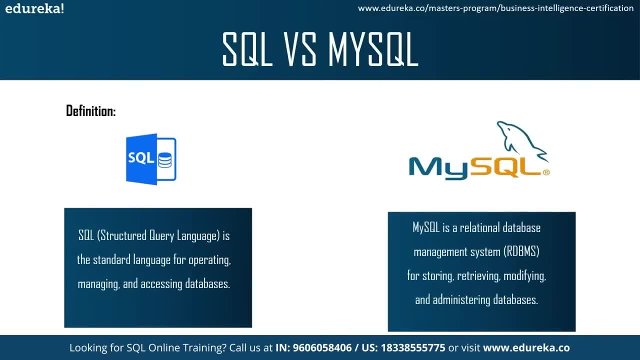 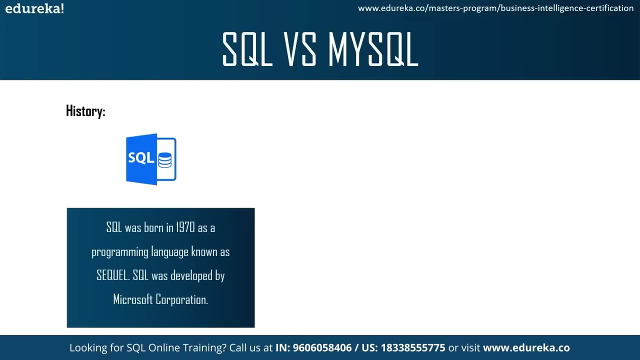 Now let's see what is the definition of MySQL. So MySQL is a relational database management system for storing, retrieving, modifying and administering databases. So next point is history. So for SQL. SQL was born in 1970 as a programming language known as SQL. 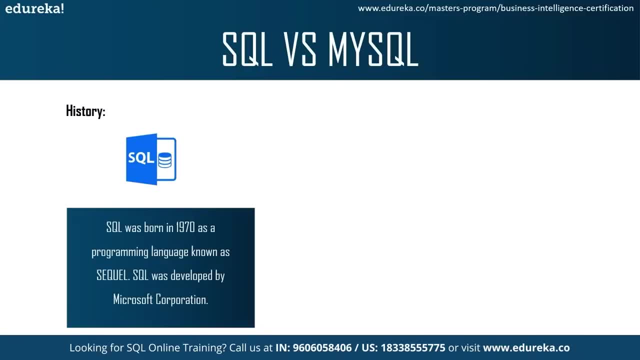 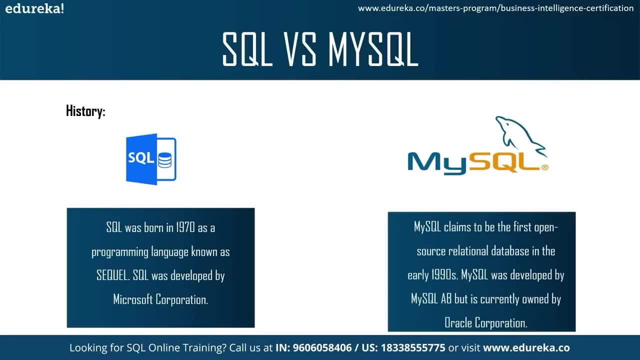 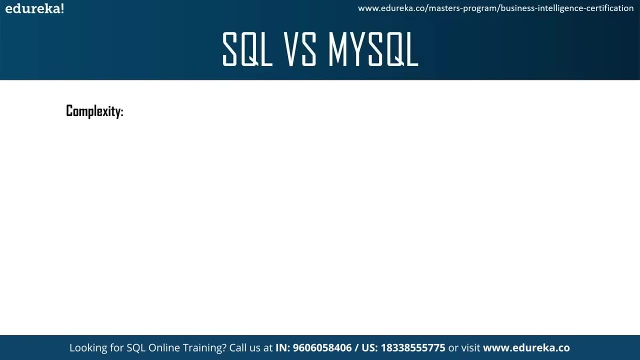 It was developed by Microsoft Corporation, but now it is also known as SQL. While MySQL claims to be the first open source relational database in the early 1990s, It was developed by MySQL AB and is currently owned by Oracle Corporation. Now looking into the complexities to use SQL efficiently. 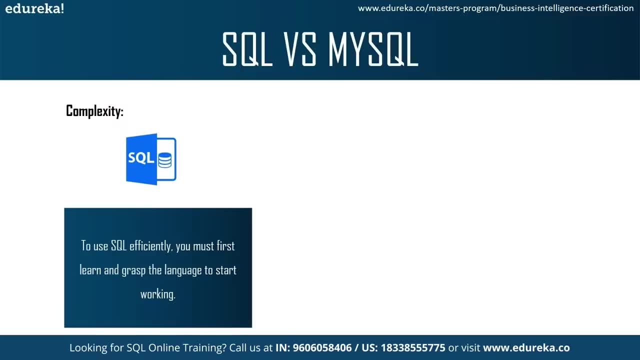 you must first learn and then grasp the language to start working with SQL, While for MySQL, you can easily access it by downloading and installing the same. Now coming to the usage: SQL is a programming language, So it can be used by querying and operating. 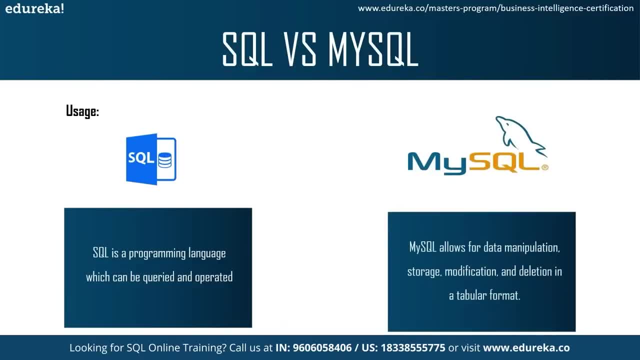 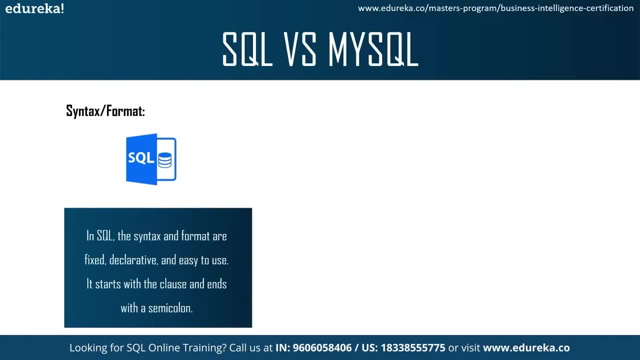 While MySQL allows for data manipulation, storage, modification and deletion in a tabular format, Now the syntax or format. So SQL is a programming language, as we all know. now The syntax and format are fixed. It's declarative and easy to use. 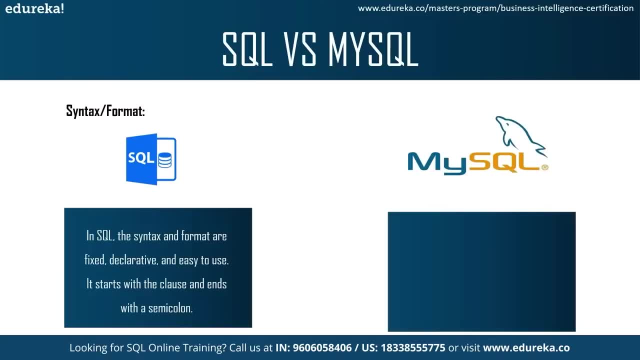 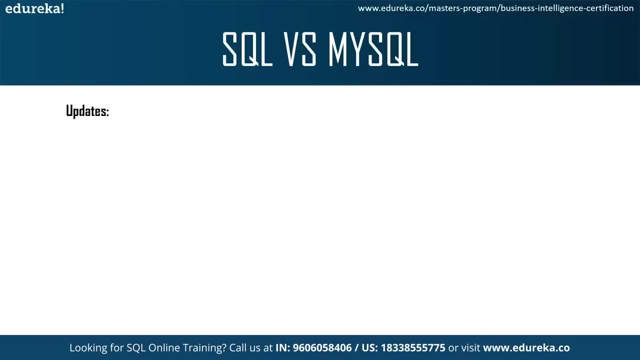 It starts with a clause and ends with a semicolon, While MySQL is a software and it is not a programming language. Hence it does not have any commands or any format. Now the updates. Since SQL is a programming language, it is fixed and command remains unchanged. 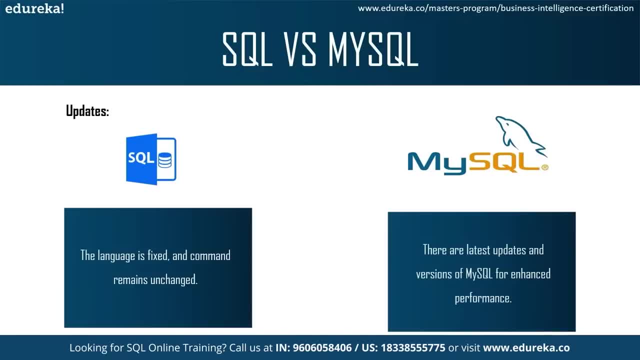 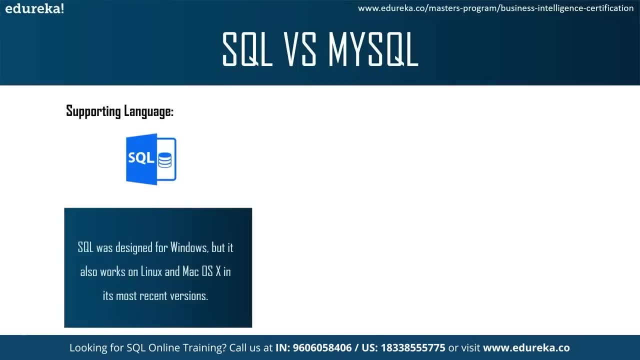 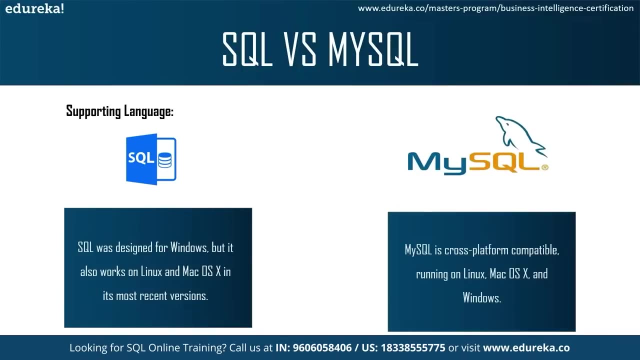 and we can't update it, While MySQL has its latest updates and versions for enhanced performance. Now for supporting language. SQL was designed for Windows, but it also works on Linux, Mac OS in its most recent versions, While MySQL is a cross-platform compatible. 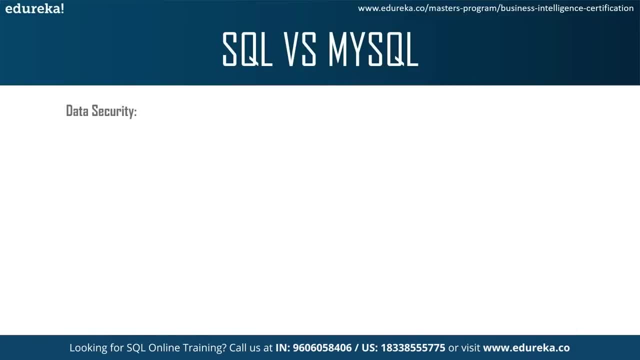 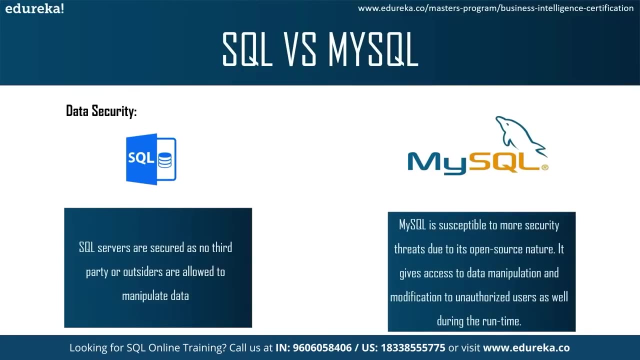 running on Linux, Mac OS and Windows as well. Now coming to the data security: SQL servers are secured, as no third party or outsiders are allowed to manipulate data, While in MySQL, it is susceptible to more security threats due to its open source nature. 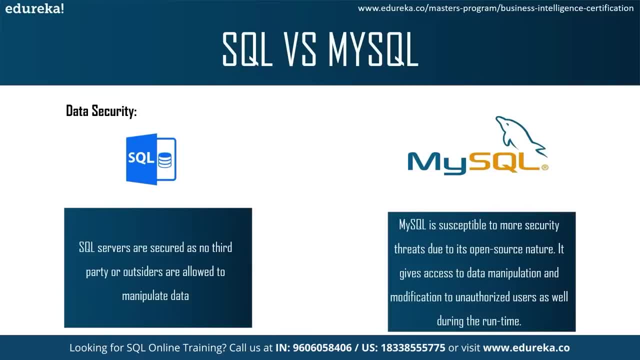 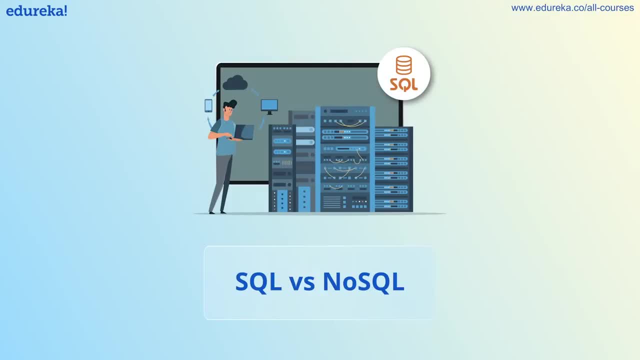 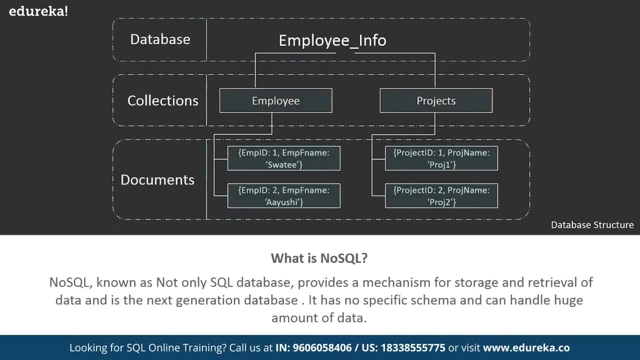 It gives access to data manipulation and modification to unauthorized users as well during the runtime. Now let's just understand what is NoSQL. NoSQL, or most commonly known as not only SQL database, provides a mechanism for storage and retrieval of data and is the next generation database. 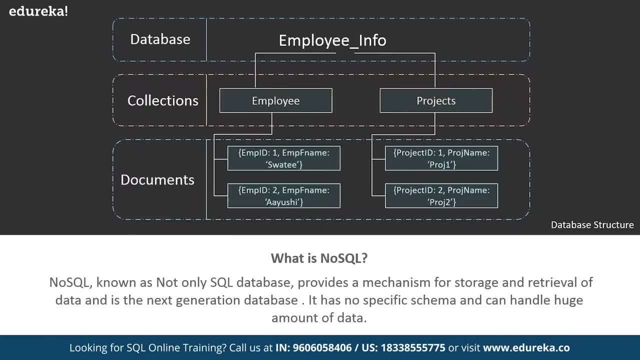 This kind of database has no specific schema and does not have tables with rows and columns storing data values, but can definitely handle large amount of data. So, if you consider the example on the screen, we have an employee database which has two collections, that is, the employee and the projects collection. 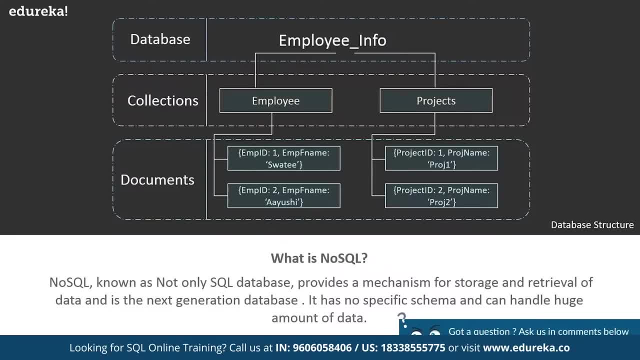 Now, each of these collections have documents, which are basically the data values. So if you just want to understand these terms, then you can just consider the collections to be your tables and the documents to be your fields in the tables. So if you compare a SQL database and a NoSQL database, 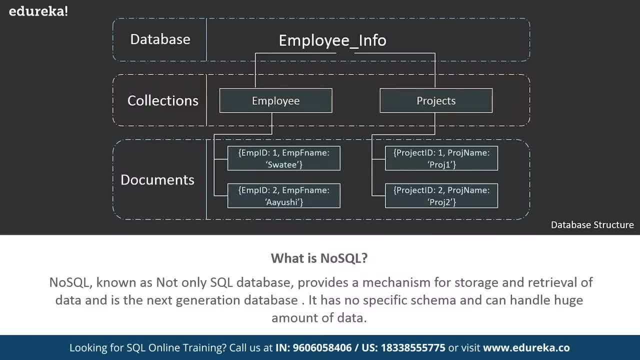 for example, let's just say we have an employee database where you know there's an employee table with around 10 columns, right, That is basically the 10 fields Now in the NoSQL database. what will happen is the employee table itself. 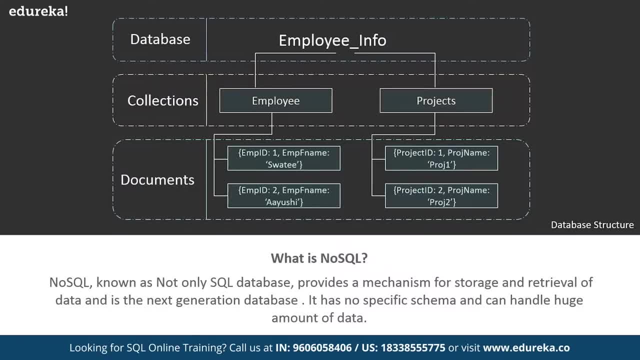 will be taken as a collection and each of these fields will be considered as documents. Now, the most interesting part of NoSQL is that these kind of databases do not have to use the same schema for the presence of multiple documents in one collection. So, since NoSQL has dynamic schema, 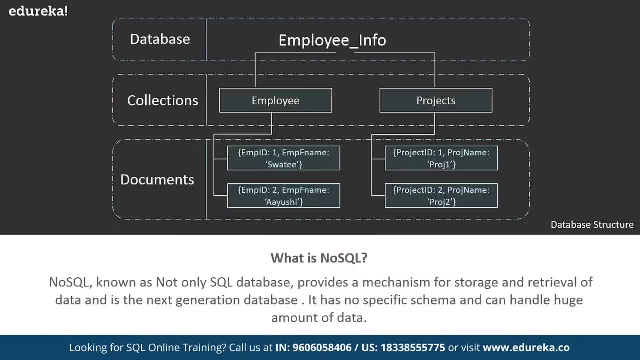 that means that you know multiple documents can be present in a single collection and also each collection can have different documents. So you can have a document in the collection which has both employee ID and employee name and also you can have a document in the same collection. 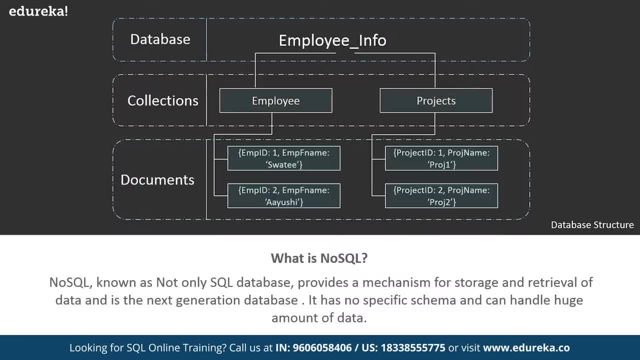 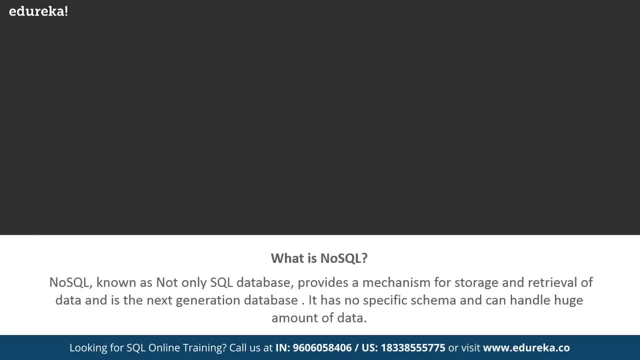 which do not have the ID, and just toast the name. So that's how, guys, you can play around with collections and documents in NoSQL database. Apart from this, Let me just also tell you that you know there is no specific query language present in NoSQL. 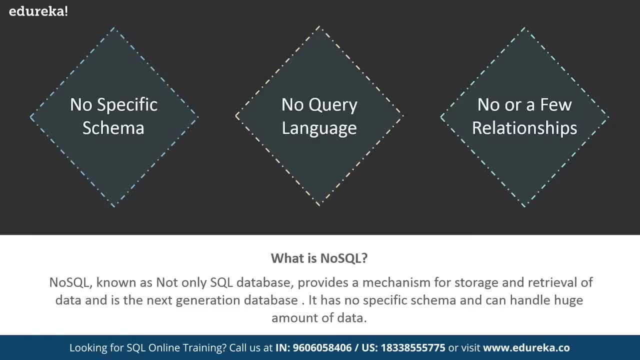 So, basically, the language that you use to retrieve data is completely infrastructure based. that is basically how you store your data and where you store your data. Lastly, there are no or very few relationships present in a NoSQL database, as you do not have a predefined schema. 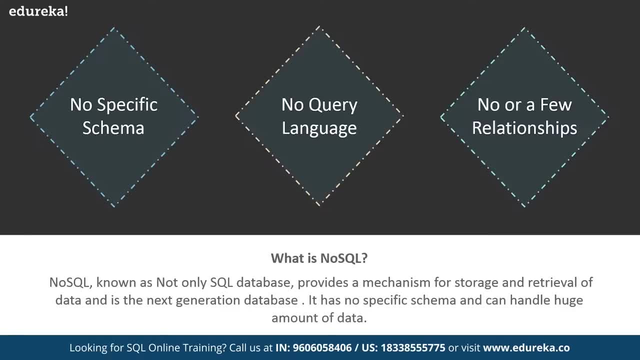 but you do have a dynamic schema in which we can put all the required information in a collection. right, When you have a dynamic schema and you have the option of putting all the required information in a single collection and the collection can differ in the same schema itself. 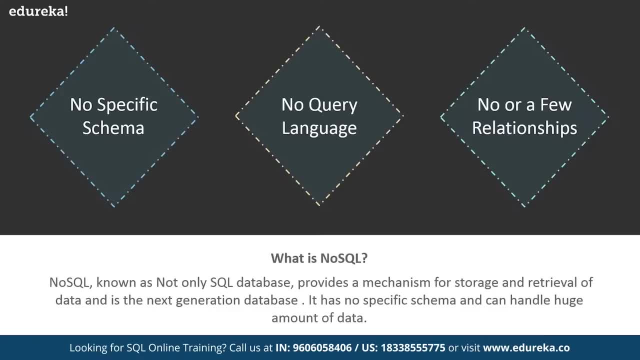 You actually do not need any relationships to be present, right? So that's how, guys. NoSQL does not have, or has very few relationships. So, guys, if I just have to summarize NoSQL for you, then NoSQL is a type of database which do not have a predefined schema, a query language. 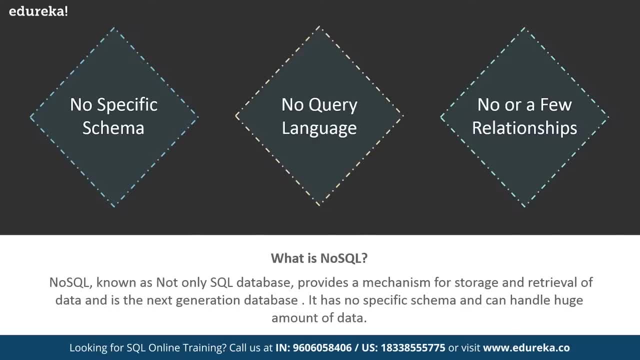 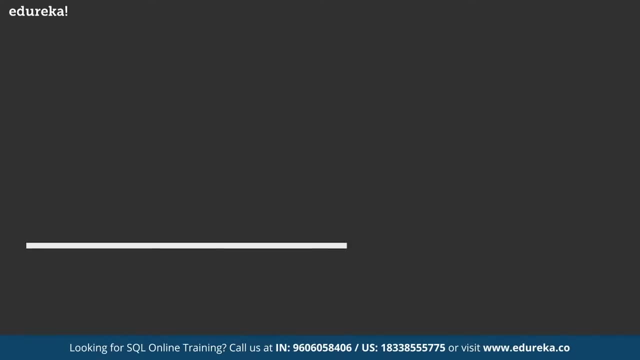 and has no tables. It follows a method of storing data in a dynamic schema with less or no relationships, and can handle humongous amount of data. Let's now see how these databases stand against each other. So in the space of will be comparing both these databases. 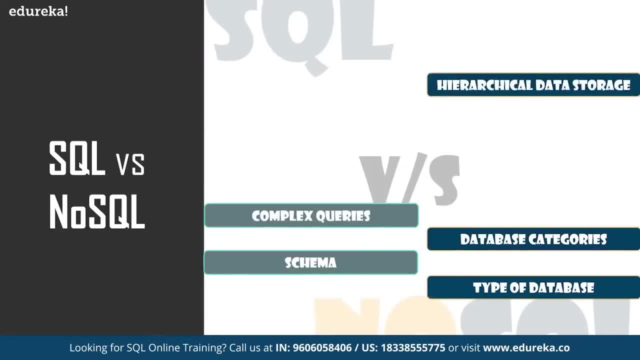 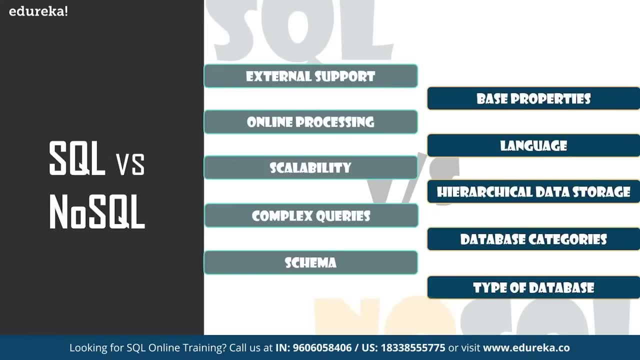 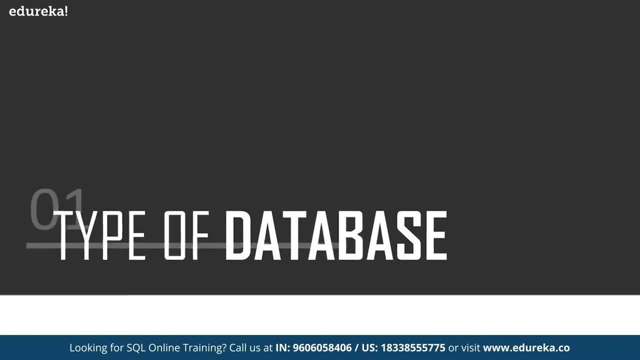 based on the ground, such as the type of database, schema, database categories, complex queries, hierarchical data storage, scalability, language, online processing based properties and external support. Let's get into the detail with the first comparison factor, that is, type of database. Now, when we compare these databases based on this factor, 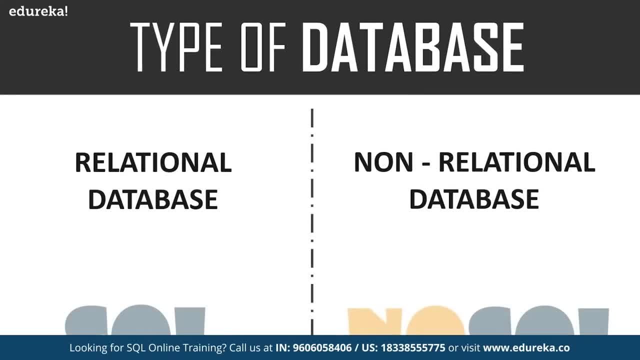 let me just tell you that. you know, SQL is essentially called a relational database and it organizes structured data fields into defined columns. So database can have n number of tables and each table can have m number of columns with the data stored in it. 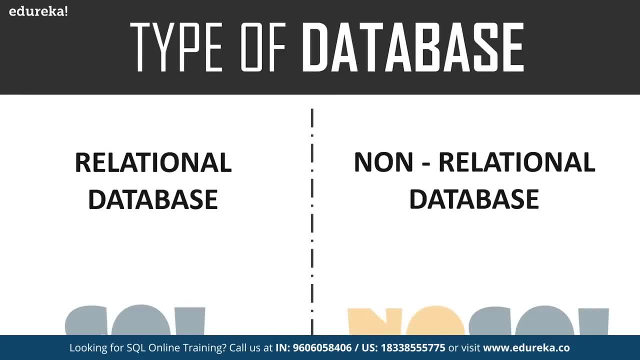 Each table can be related to the other tables also, right? So if you have around 10 tables, then those 10 tables can have around 2 to 3 columns, or you can say more than that- columns in each table- and all these 10 tables can be related to each other coming. 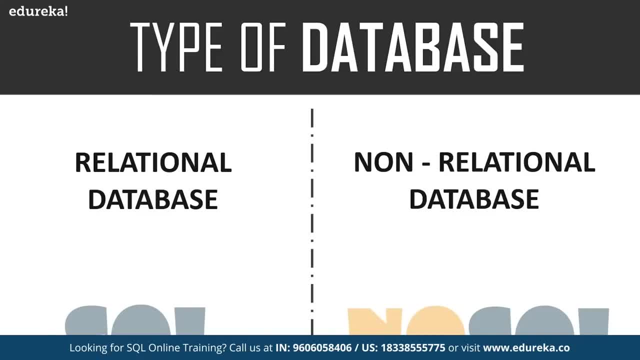 to NoSQL. NoSQL is a non-relational database which provides a mechanism for storage and retrieval of data. in the NoSQL database, data is modeled in the form of collections and hence it tries to avoid relations, as I just explained you before. so, guys, if you have to compare these databases based on this factor, 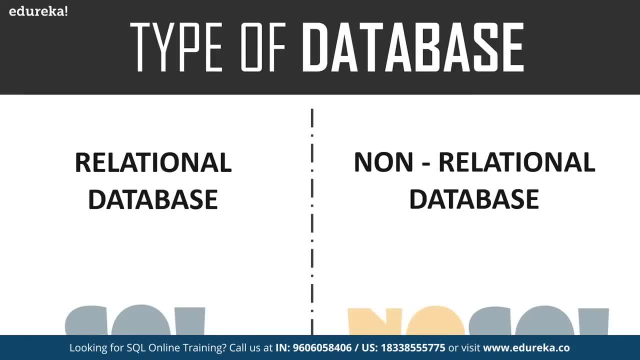 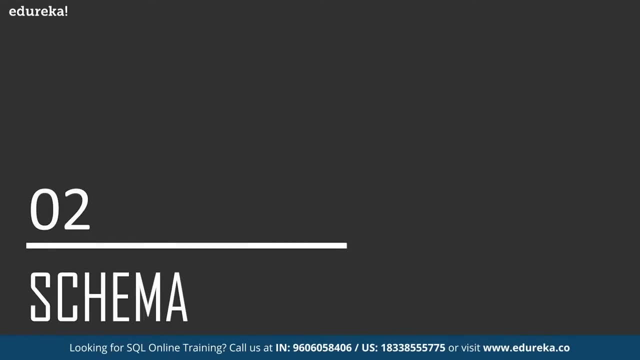 then SQL is essentially a relational database and NoSQL is a non-relational database or a distributed database. next, We'll be comparing these databases based on the schema. while comparing these databases based on this factor, Let me tell you that sequel needs a predefined schema. 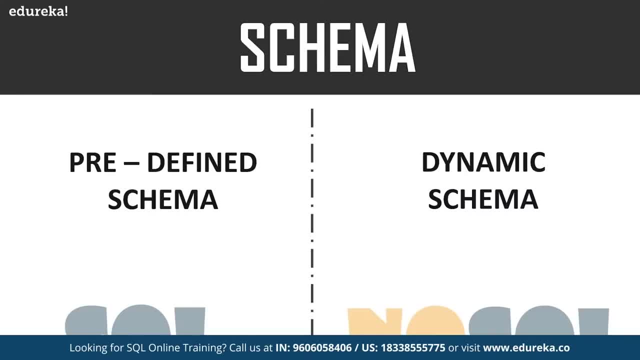 for structured data. So before you start using sequel to extract and manipulate data, you need to make sure that you know your data is predefined in the form of tables coming to NoSQL. Well, NoSQL databases have a dynamic schema for unstructured data. 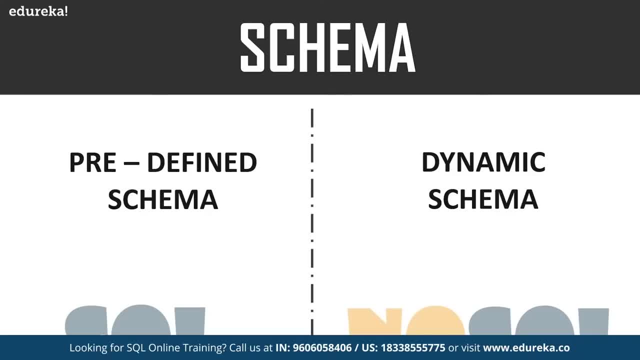 So if you're using the NoSQL database, then there is no predefined schema present and the complete schema of your data completely depends on how you wish to store the data, that is, which feels that is basically which documents that you wish to store in which collections. 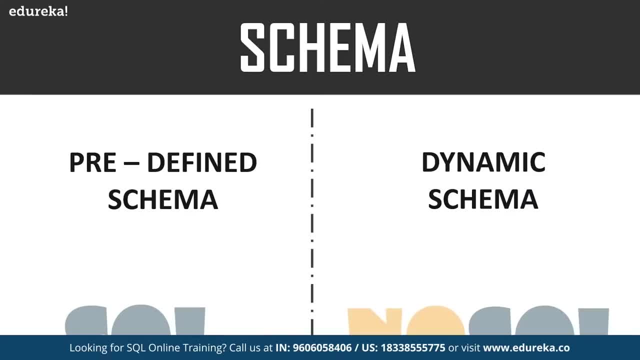 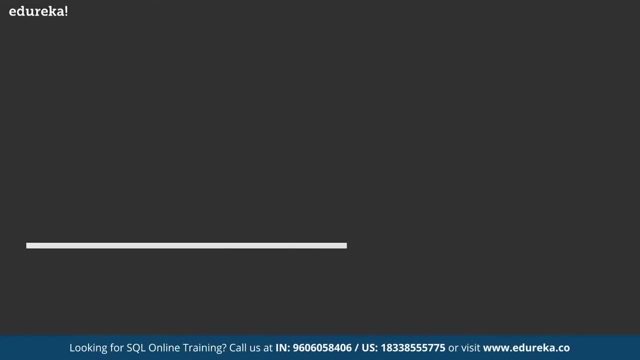 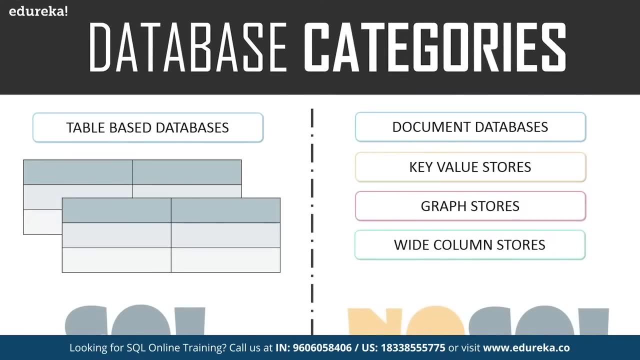 and how you wish to store them. So, guys, that was about schema. the sequel has a predefined schema and the NoSQL has a dynamic schema. now moving on to the next parameter, which is database categories. now, sequel databases are basically the table based databases. So, as I explained in the previous factors, the sequel databases, 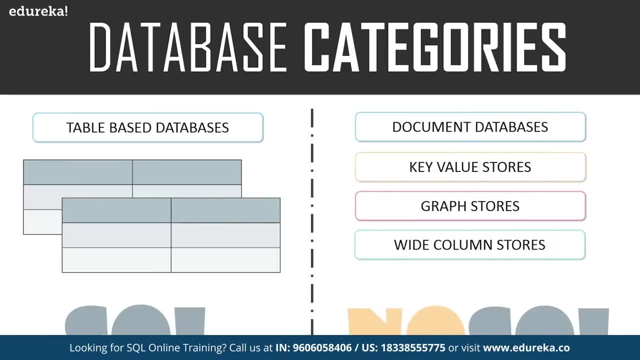 can have n number of tables related to each of them and each table can have m number of rows and columns storing data in each cell of the data. now, Similarly, if we talk about the NoSQL databases, the NoSQL databases have mainly four categories of databases, that is, document database. 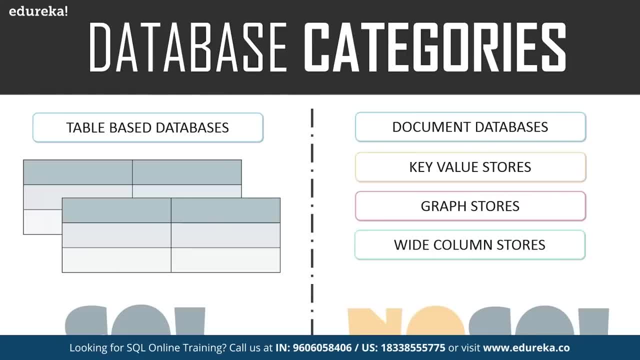 the key value stores to graph stores and the white column stores. coming to the document database. Now, this kind of database pairs each key with a complex data structure known as a document. It can contain many different key value pairs, or the key error pairs, or even the nested documents. coming to the key value stores: 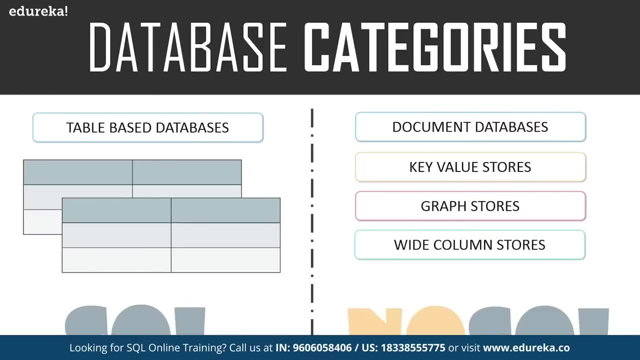 These are the simplest form of NoSQL database, So every single item in the database is stored as an attribute, name or a key, together with its value. now coming to the craft stores. The craft stores are basically used to store the information about Network, such as the social connections. 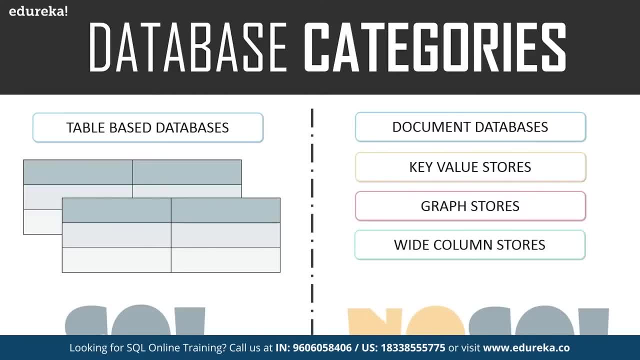 Now the craft stores mainly include the Neo4j and the hypergraph TV. coming to the last kind of database category of NoSQL, that is, the white column stores, the white column stores, such as Cassandra and H ways, are optimized for queries over large data sets and stores columns of data together instead of rows. 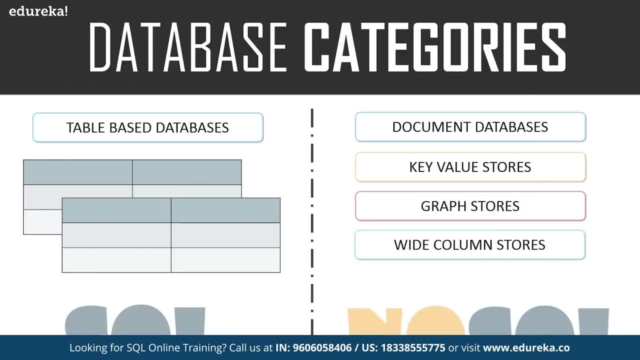 So, guys, these were mainly the four categories of NoSQL database, that is, the document database, the key value stores to craft stores and the white column stores. now, this might have given idea of you know, the sequel databases basically represent data in the form of tables which consist of n rows of data. 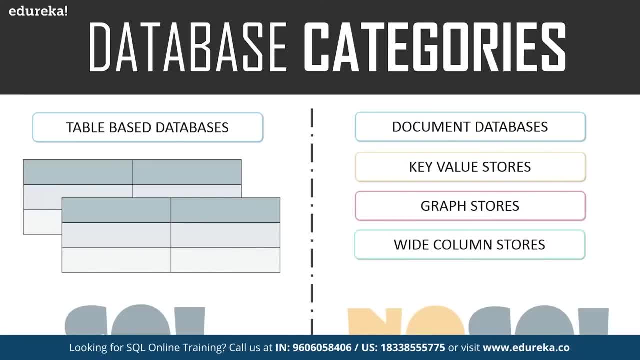 Whereas the NoSQL databases are the collection of key value pairs, documents, graph databases or white column stores which do not have a standard schema definitions which it needs to stick to. so, guys, this was the main difference between sequel and NoSQL: that sequel is basically the table-based databases with a predefined schema. 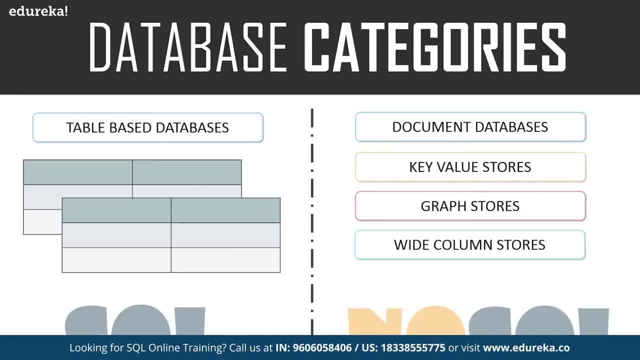 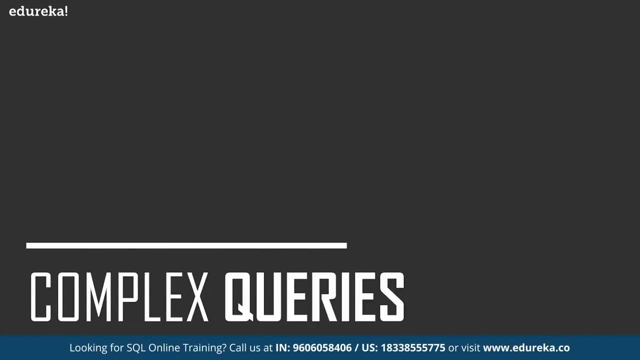 and the NoSQL databases mainly have different categories of databases with a dynamic schema. So I hope I'm clear with this point. next Let's discuss how these databases fit for complex queries. Now, when we talk about complex queries, let me just tell you that you know sequel is a good fit. 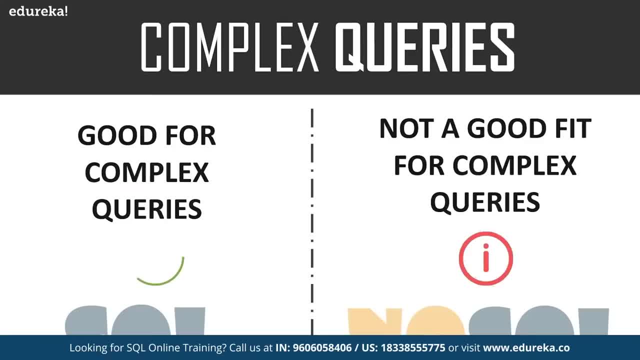 for complex query environment, as the schema and sequel databases is structured and has proper tables. So even if you wish to apply nested queries with many sub queries inside the outer query, you can easily do by using the proper table and column names and you can retrieve the required data coming. 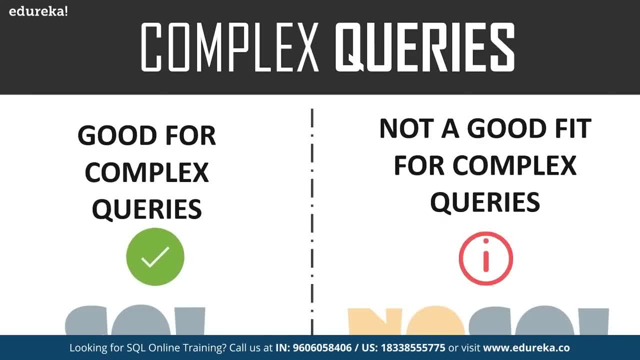 to the NoSQL databases. The NoSQL databases are not a good fit for complex queries as they don't have standard interfaces to perform complex queries and the queries themselves in NoSQL are not as powerful as the sequel query language. So this is basically because you know. 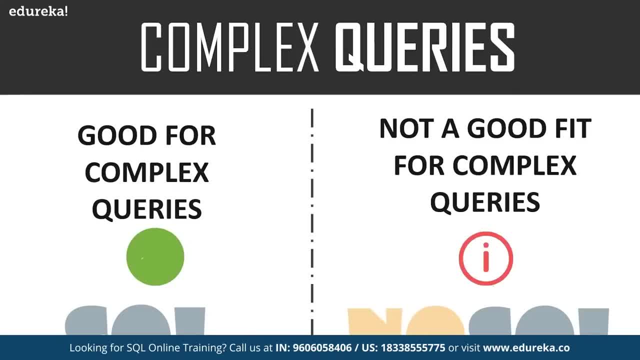 they're not written in a specific language, and the language in which they are written is completely based on the database infrastructure, or you can see the schema. So if you have to compare how these databases fit for complex queries, then let me tell you that sequel is a better fit. 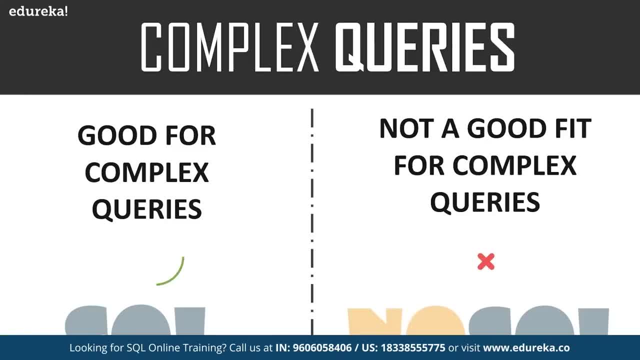 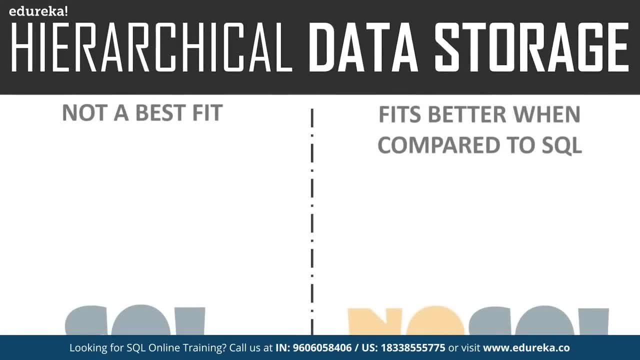 for complex queries when compared to NoSQL. Now, moving on to the next factor of comparison, that is, hierarchical data storage. Now, when we compare the databases based on this factor, let me tell you that the sequel databases are not best fit for hierarchical data storage. 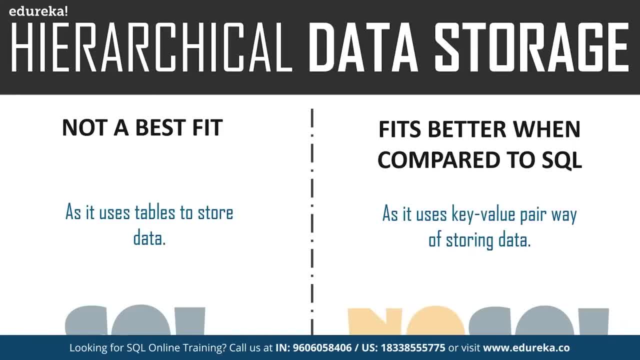 Now, this is because as the number of tables increase, the complexity of relating them to each other also keeps increasing. now, in such a scenario, you cannot relate humongous amount of tables with n number of columns to each other, right? but coming to NoSQL database, the NoSQL database fits better. 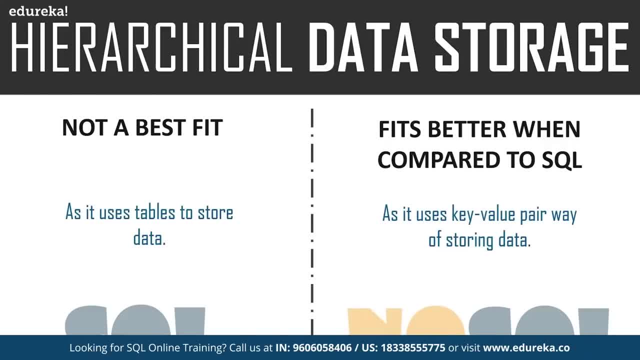 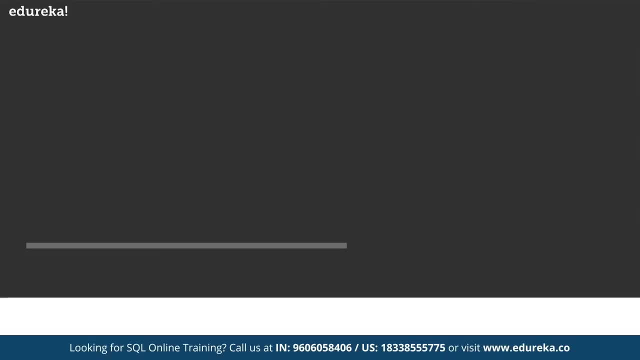 for hierarchical data storage, as it follows the key value pair way of storing data, similar to the JSON data. Now, NoSQL databases are also highly preferred for large data sets when compared to the sequel database, and one such example is HBase. So basically, HBase is used for this purpose. next point: 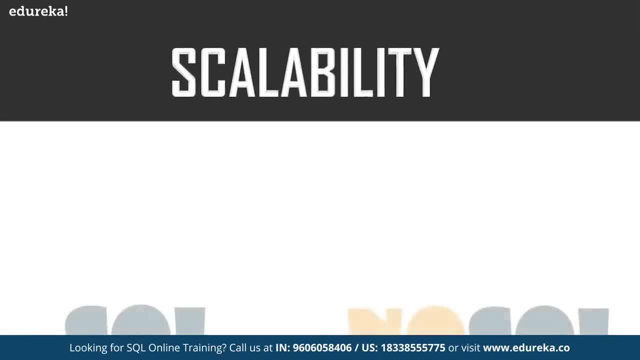 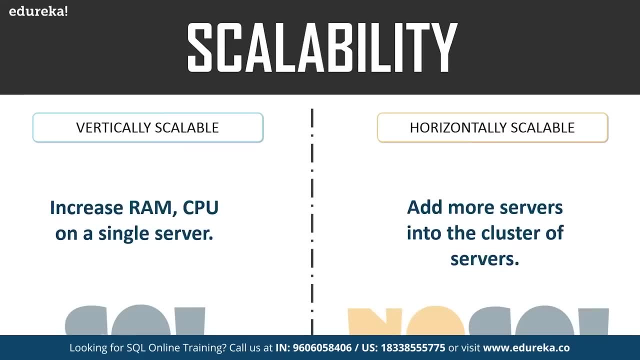 of comparison will be scalability. now sequel database is our vertically scalable. You can load balance this database by optimizing your hardware requirements, such as increasing the CPU, RAM, SSD, etc. on a single server. on the other hand, the NoSQL databases are horizontally scalable. You can do load balancing by adding more servers. 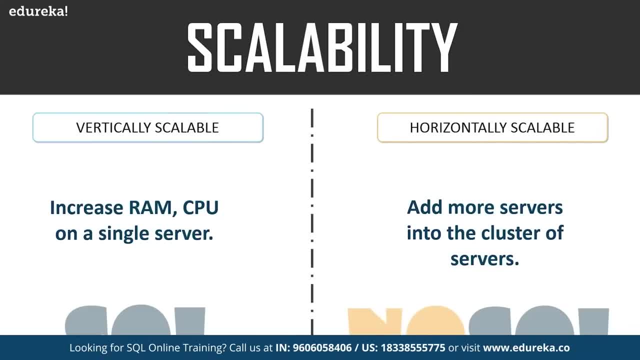 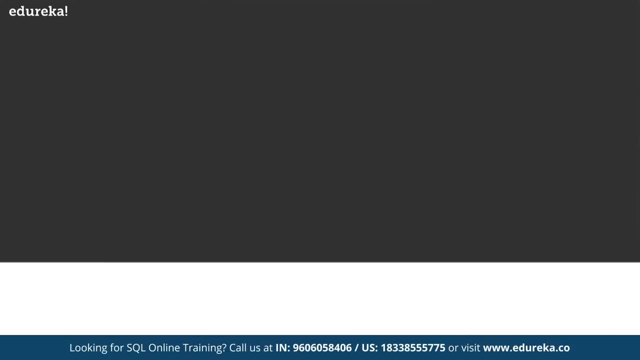 to your cluster so that, with the help of these servers, you can handle large traffic. So, on the note of scalability, sequel is vertically scalable and NoSQL is horizontally scalable. next, We'll be comparing these databases based on language. the sequel databases have a specific language. 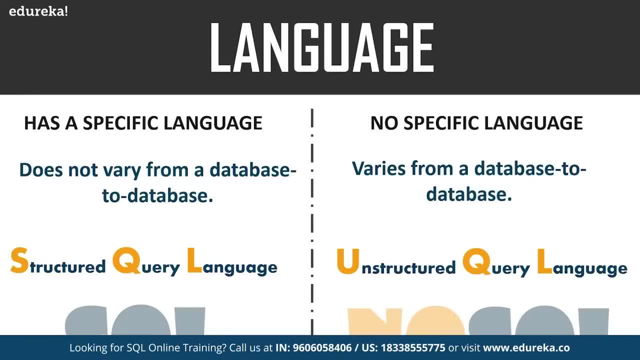 and it does not vary from database to database. So basically, the sequel databases use the structured query language for defining and manipulating the data, which is very powerful. coming to NoSQL, The NoSQL has no specific language and it varies from database to database. in the NoSQL databases, 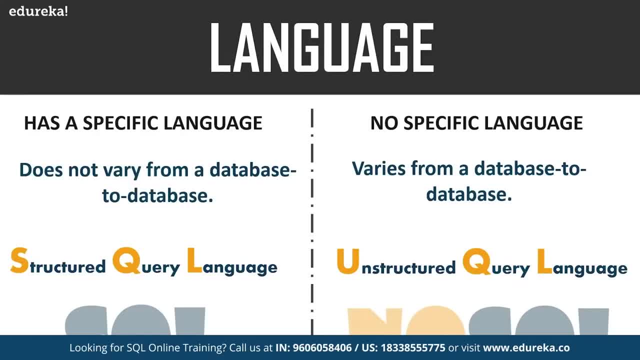 The queries are focused on the collection of documents and sometimes the language used in NoSQL is also called unstructured query language. So on the note of language guys, the sequel uses a proper, defined language, that is the structured query language, and NoSQL has no specific language. 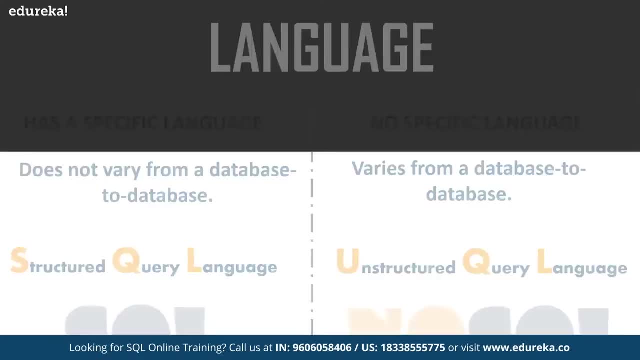 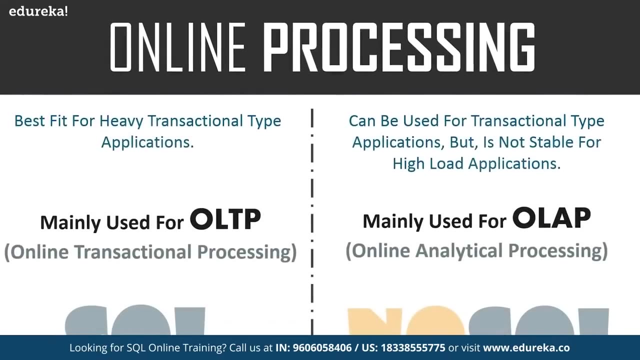 and the language differs from database to database. Now, moving on to the next parameter, which is online processing. now, when we compare both these databases based on online processing, sequel databases are the best fit for heavy-duty transactional type applications, as it's more stable and promises the atomicity. 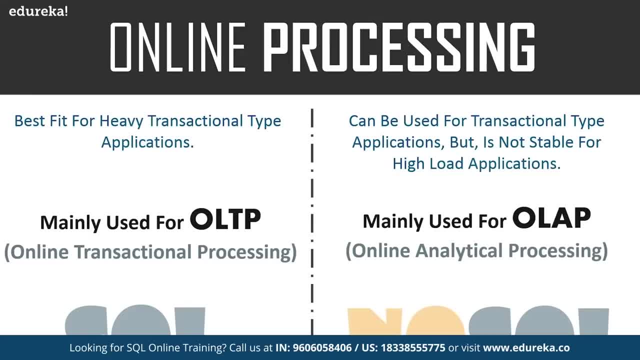 as well as the integrity of data. While you can definitely use NoSQL for transaction purpose, yet it is still not comparable and stable enough and high load for complex transactional applications. So you can understand by this that you know sequel is mainly used for OLTP, that is, basically online transactional processing. 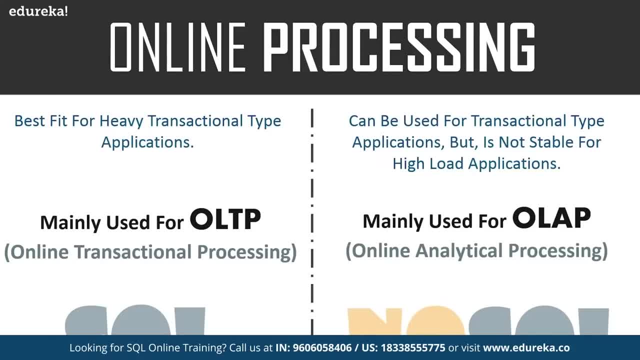 and NoSQL is mainly used for OLAP, which is online analytical processing. So if I have to just explain these terms- OLTP and OLAP- for you, then OLTP is basically characterized by large number of short online transactions, such as insert, update and delete. the main emphasis. 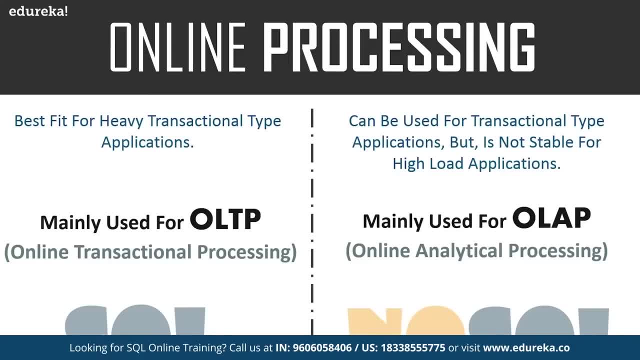 for OLTP systems is to put on a very fast query processing, maintain data integrity in multi-axis environments and an effectiveness measured by number of transactions per second. in OLTP databases There's proper, detailed and current data and the schema used to store transactional database. 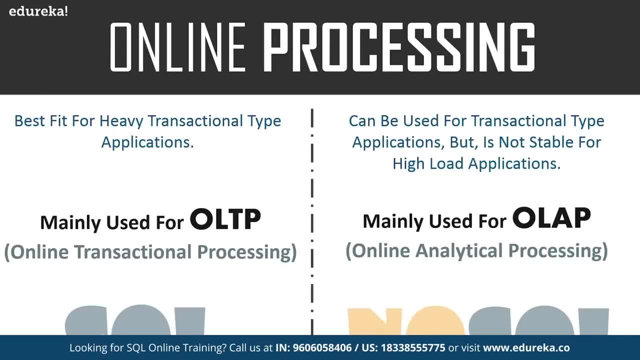 is, in the entity model, usually 3nf. now coming to OLAP, that is basically online analytical processing. This is basically characterized by relatively low volume of transactions and queries are often very complex and involve aggregation. for OLAP systems, response Time is an effectiveness measure. 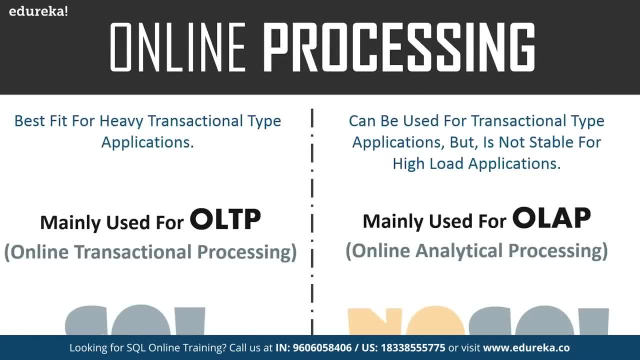 and OLAP applications are widely used by data mining techniques. So in the OLAP database there is aggregated historical data stored in multi-dimensional schemas, usually the star schema. So, guys, that was about OLTP and OLAP, So you can just understand this point that you know, sequel. 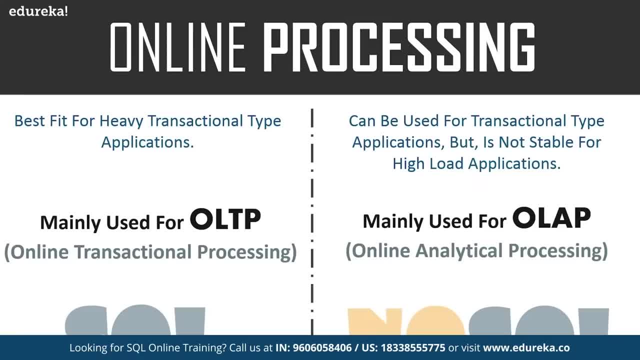 is mainly used for heavy transactional type applications and no sequel is basically used for analytical processing and can definitely be used for transactional type applications, but yet it is still not stable for high load applications. So now the next point of comparison we have is base properties. 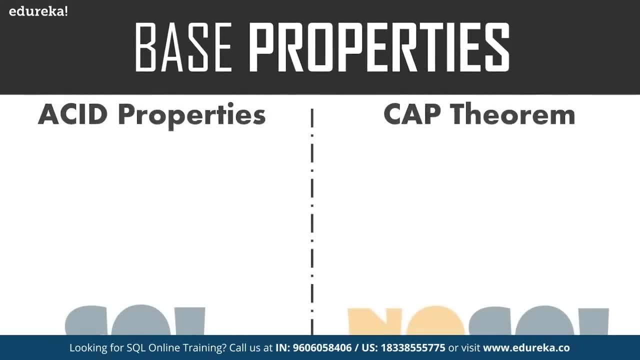 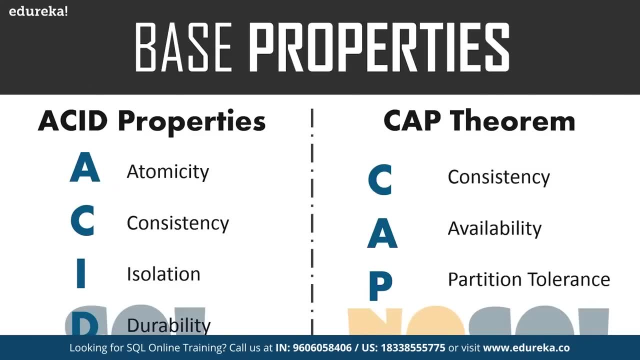 a sequel databases emphasize on the asset properties, that is, the atomicity, consistency, isolation and durability, Whereas the no sequel database follows the cap theorem, that is, the consistency, availability and partition tolerance. So let's talk about both of them one by one, starting with the asset properties. asset properties mainly stand. 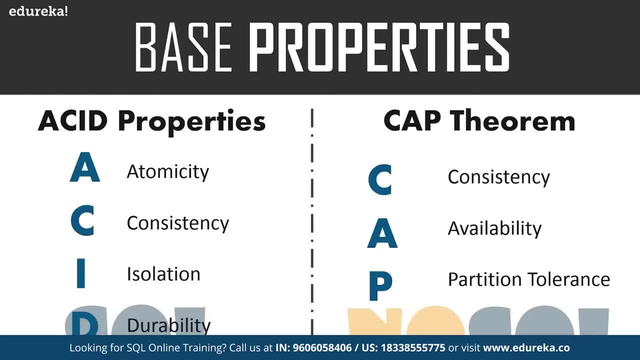 for atomicity, consistency, isolation and durability. now, atomicity basically refers to the transactions that are completely done or failed, where the transaction refers to a single logical operation of data. Now, this basically means that you know, even if one part of the transaction phase, the entire transaction phase. 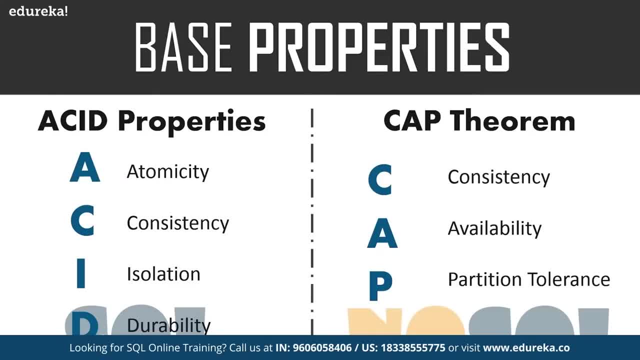 and the database state is left unchanged. coming to consistency: the consistency ensures that data must meet all the validation rules. in simple words, you can just say that you know your transaction never leaves the database without completing its state. coming to isolation: The main goal for isolation is basically the concurrency control. 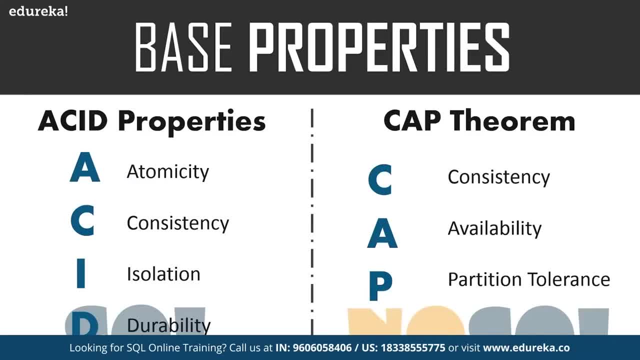 and finally, the durability. the durability means that you know if a transaction has been committed, it will occur whatever may come in between, such as the power loss, crash or any sort of error. So, guys, that was about the asset properties. that is basically the atomicity, consistency, isolation. 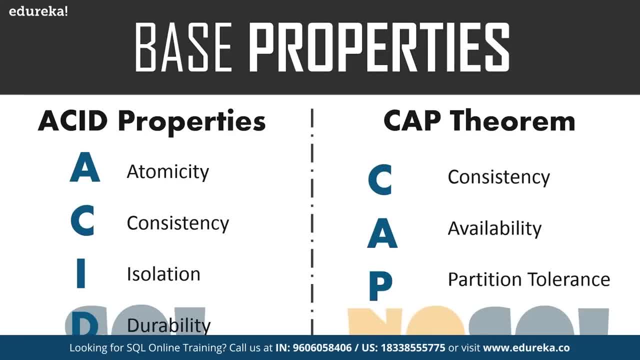 and durability. coming to the cap theorem, the cap theorem, or the Eric Brewer's theorem, states that you know we can only achieve at most two out of three guarantees for a database. that is basically the consistency, availability and partition tolerance. So here the consistency means that you know. 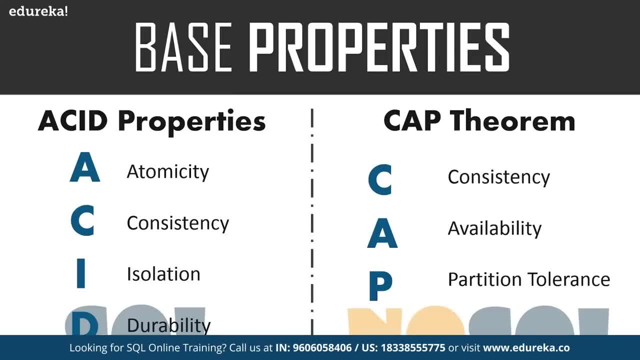 all the nodes in the network see the same data at the same time, or the reader gets most recently written data coming to availability. availability is the guarantee that every request receives a response about whether it is successful or failed, And the more number of users a system can cater. 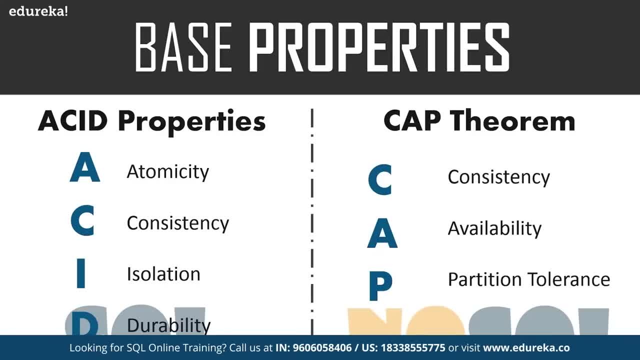 to a better is the availability coming to the partition tolerance. The partition tolerance is a guarantee that the system continues to operate despite arbitrary message loss or failure of any part of the system, In other words, even if there is a network outage in the data center. 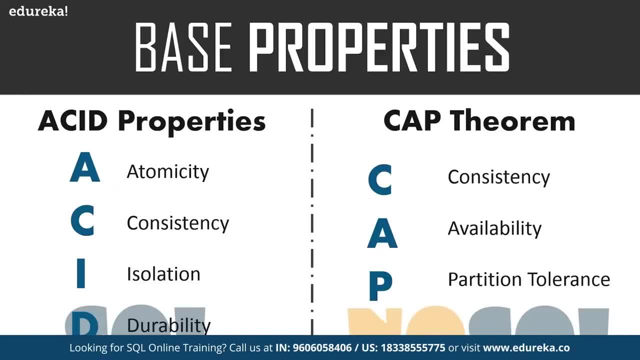 and some of the computers are unreachable till the system continues to perform. now, out of these three guarantees, that is, the consistency, availability and partition tolerance, no system can provide more than two guarantees. Now, since in the case of distributed systems, the partition of Network is must, the trade-off is always. 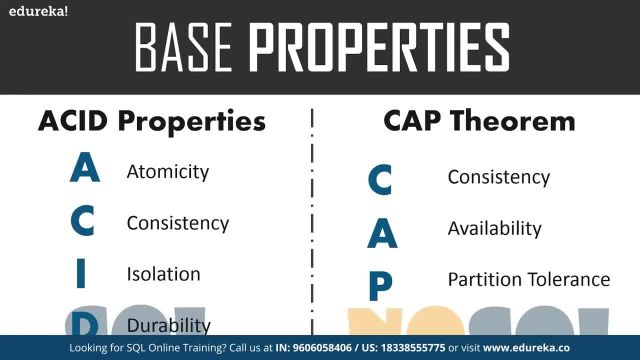 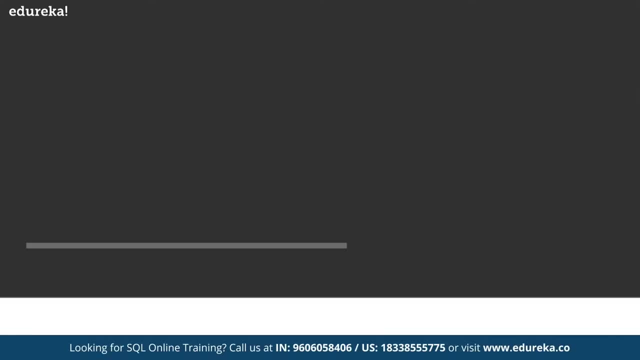 between consistency and availability. So you can just understand that. you know, no sequel cannot provide consistency and high availability together. So, guys, that was about the base properties. sequel is completely based on the asset properties and no sequel is based on the cap theorem. Finally, the last but not the least factor: 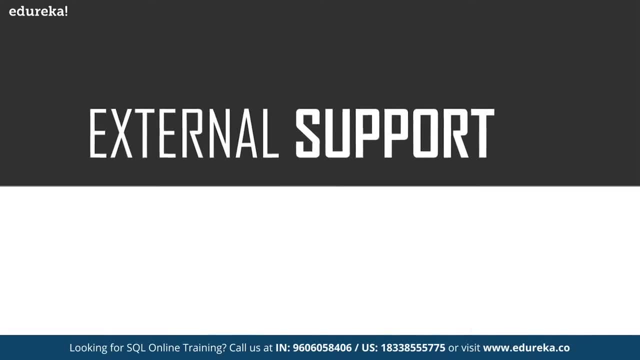 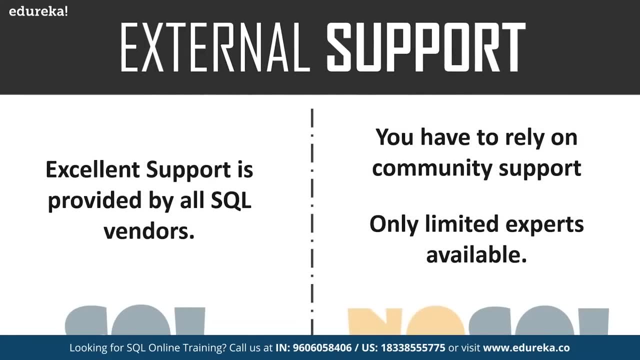 of comparison is external support. now, external support is available for all sequel SQL database from the vendors. There are also a lot of independent consultations who can help you with SQL database for a very large-scale deployment. This is mainly due to since sequel has been 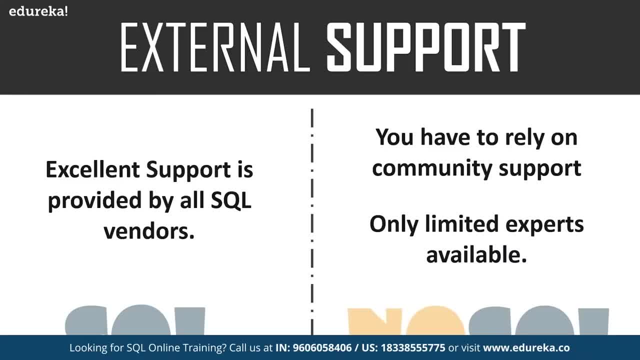 into existence since more than 40 years and people have been using sequel regularly, now coming to no sequel for some no sequel databases. You still have to rely on the community support and only limited outside experts are available for you to set up and deploy your large-scale no sequel deployments. 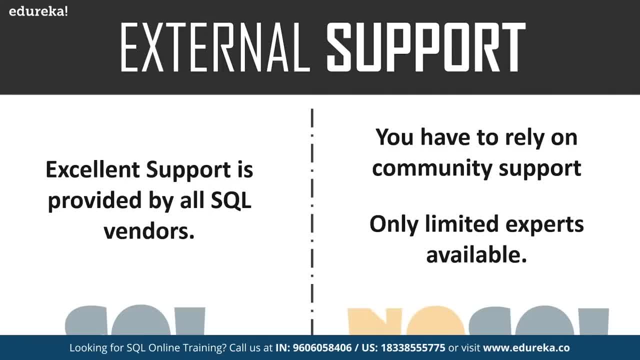 This is mainly because no sequel has come into existence and many of them haven't explored it yet. much So, folks, with this we come to an end of this phase of between sequel and no sequel. I hope all the comparison factors were clear to you guys. 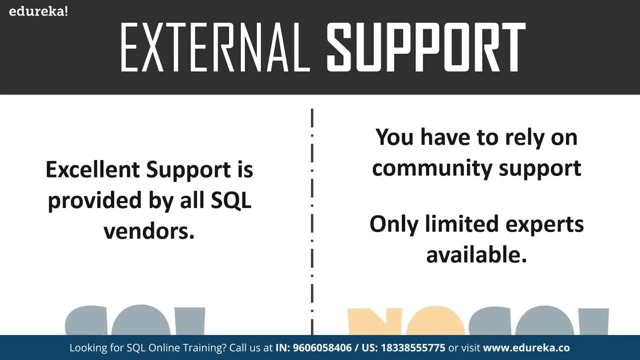 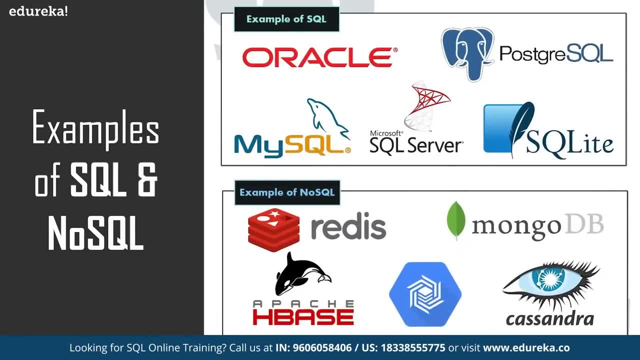 Now in this session, since we have discussed so much about sequel and no sequel, Let me just show you some examples of the same. So, as you can see on my screen, these are the examples for sequel and no sequel. So the popular examples for sequel are the Oracle. 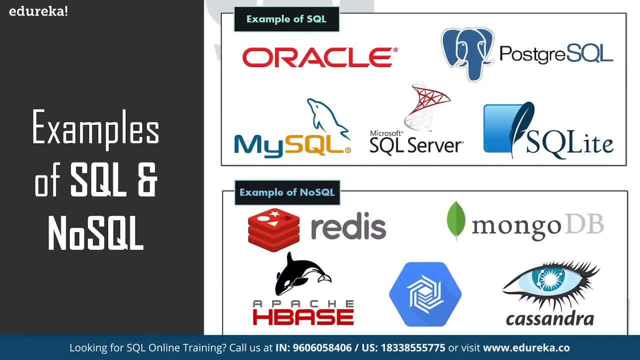 the Postgres sequel, the my sequel, the Microsoft sequel server and sequelite. Now coming to the examples of no sequel. the examples of no sequel are Redis, MongoDB, Apache, HBase, Big Data table and Cassandra- now out of the lot. the most popular databases in today's market are basically the my sequel and MongoDB. 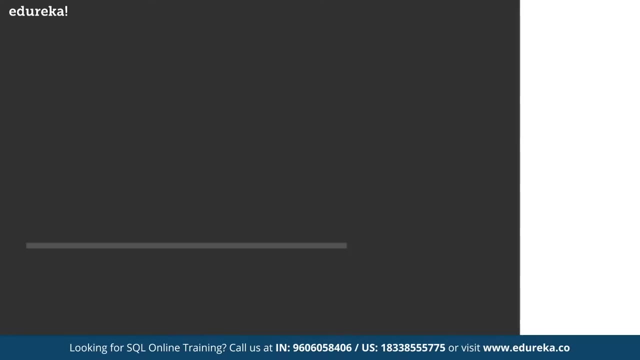 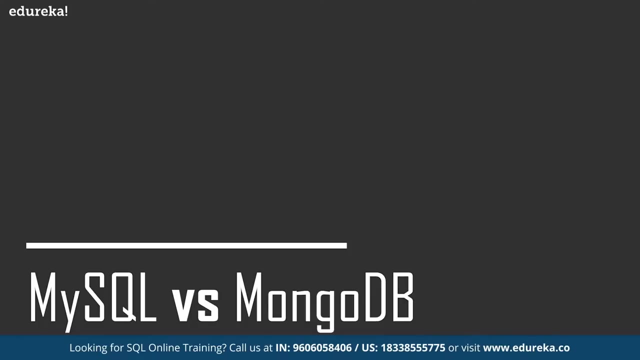 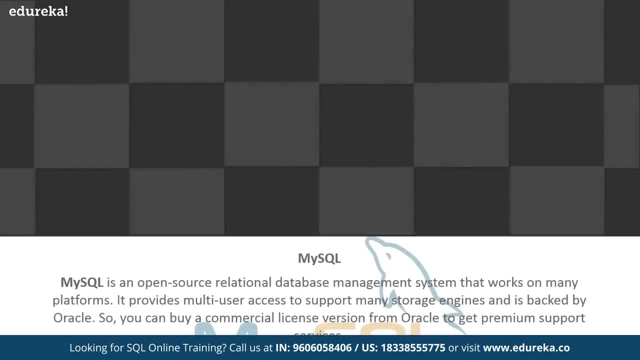 from the sequel and the no sequel sections. So next in this session will be comparing my sequel and MongoDB based on various parameters. Now, before I move on with the comparison of my sequel and MongoDB, let's first understand what is my sequel and what is MongoDB. starting with my sequel, 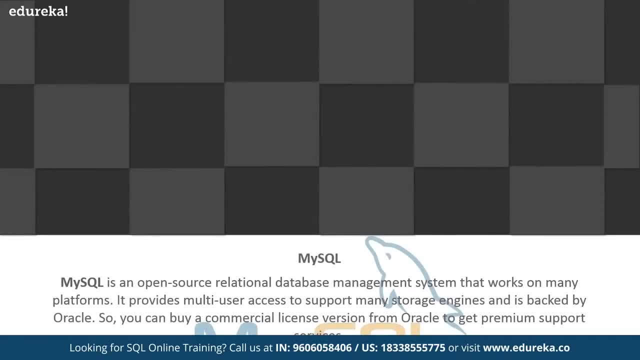 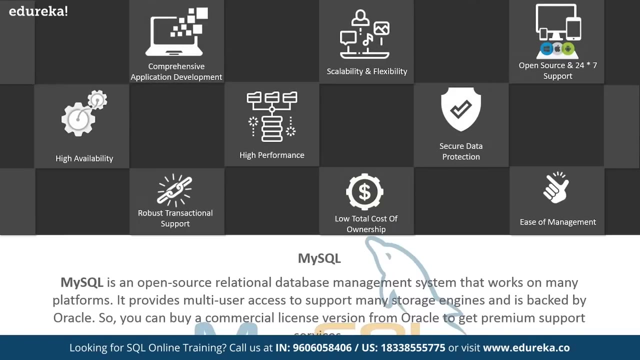 My sequel is an open-source relational database management system that works on many platforms. It provides multi-user access to support many storage engines and is backed by Oracle, so you can buy a commercial license version from Oracle to get premium support services. Now the features of my sequel are, as you can see on my screen. 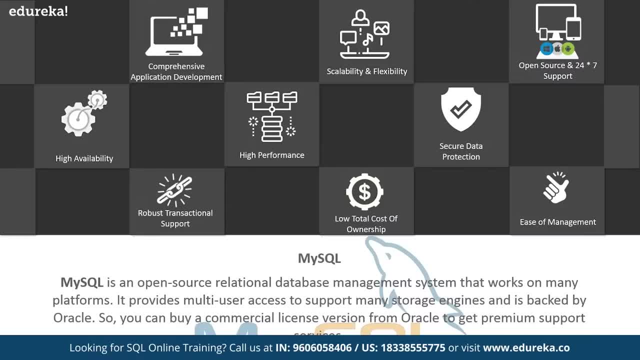 So, basically, my sequel provides comprehensive application development, scalability and flexibility, and it's open source and provides 24 into 7 support. provides high availability, high performance, support, secure So data, provides robust transactional support, requires low total cost of ownership and provides ease of management. now coming to comprehensive application development. 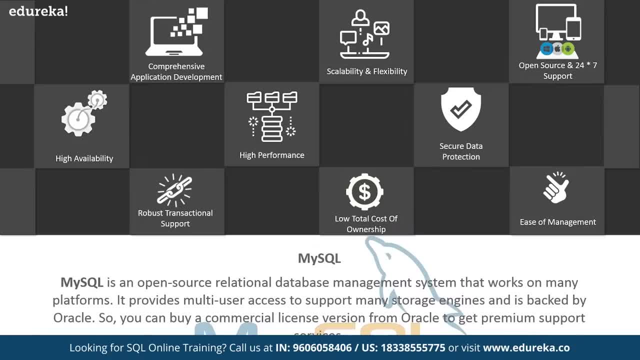 My sequel has plug-in libraries to embed the database into any application, So it basically supports stored procedures, triggers, functions, views and many more application development, coming to scalability and flexibility. with my sequel, You can run deeply embedded Applications and create data warehouses holding a humongous. 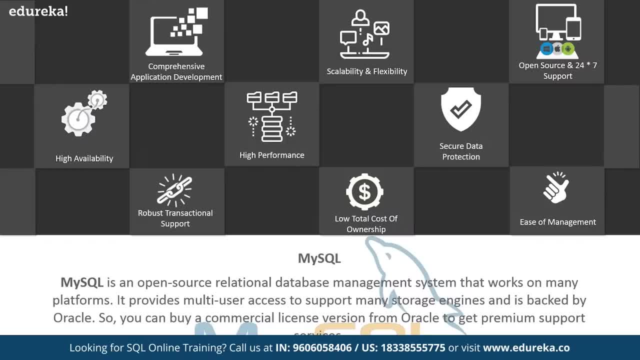 amount of data. next, talking about open-source and 24 into 7 support: this relational database management system can be used on any platform and offers 24 into 7 support for open-source and Enterprise Edition. talking about high availability, my sequel can run high-speed master slave. 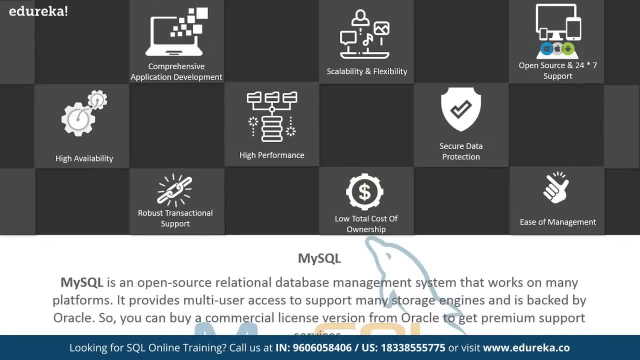 replication configurations and it offers various cluster servers. talking about high performance, my sequel provides fast load utilities with distinct memory Caches and tables index partitioning. next, about data protection, my sequel supports powerful mechanisms to ensure that only authorized users have access to the databases. next, talking 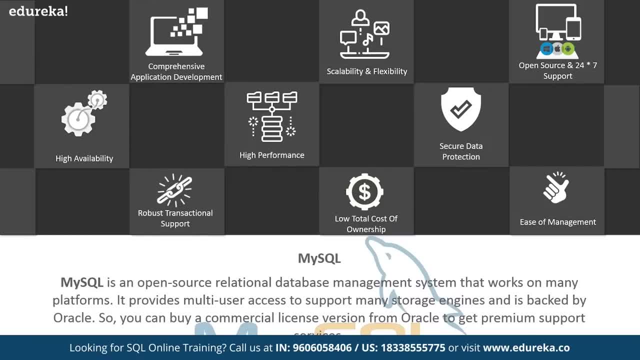 about robust transactional support. my sequel holds the asset properties, that is, basically the atomicity, consistency, isolation and durability properties and allows distributed multi-version support. and talking about low total cost of ownership, my sequel- make sure that you need- reduces the licensing costs and hardware expenditures. 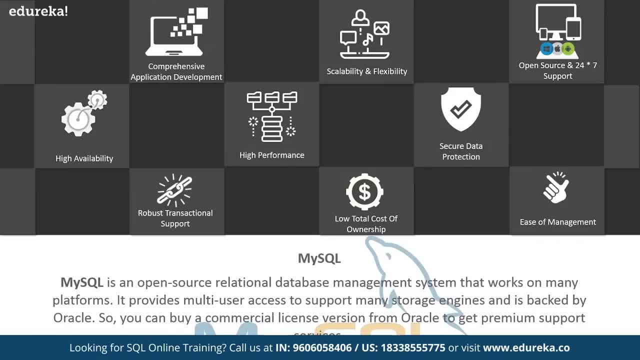 And talking about, finally, the ease of management. this software can be easily downloaded and also uses an event scheduler to schedule a task automatically. So, guys, the features of my sequel are basically the comprehensive application, development, scalability and flexibility, open-source and 24: 7 support, high availability, high performance, secure data. 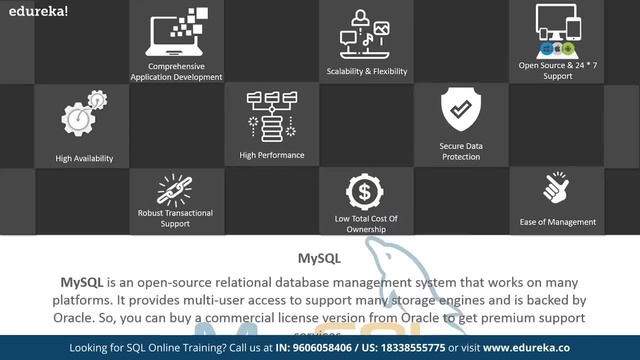 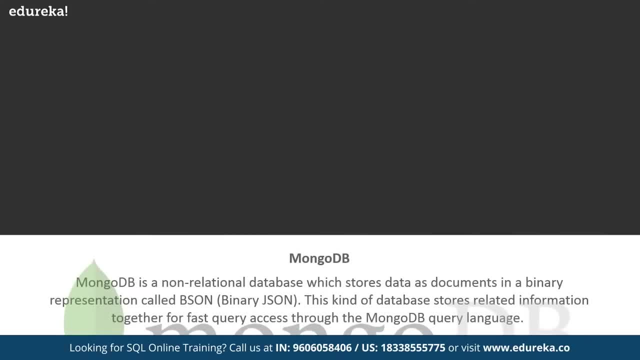 protection, robust transactional support, low total cost of ownership and ease of management. now coming to MongoDB. MongoDB is a non-deletion database with stores data as documents in a binary representation called Bson, that is basically binary Json. this kind of database stores related information together. 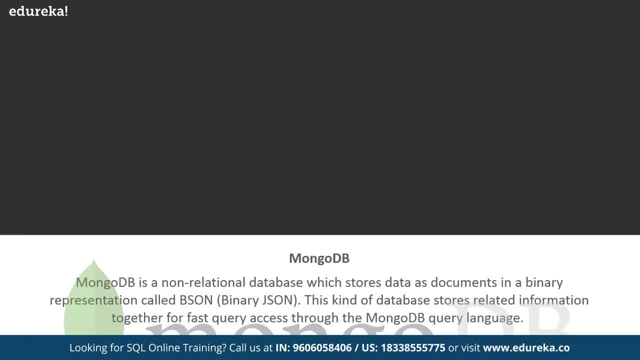 for fast query access to the MongoDB query language. the features of MongoDB are as you can see on my screen, that is, indexing, replication, ad hoc query schema list and sharding. talking about indexing MongoDB: indexes are created in order to improve the search performance. next, talking about replication: MongoDB. 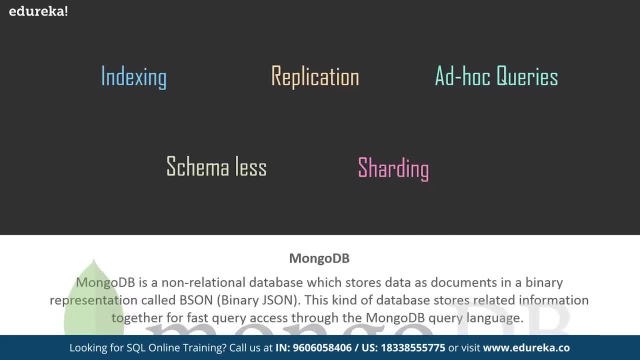 distributes Data across different machines. coming to ad hoc queries: MongoDB supports ad hoc queries by indexing the Bson documents and uses a unique query language. coming to schema list: It's very flexible because it's schema list database and is written in C++. and talking about sharding, MongoDB uses sharding. 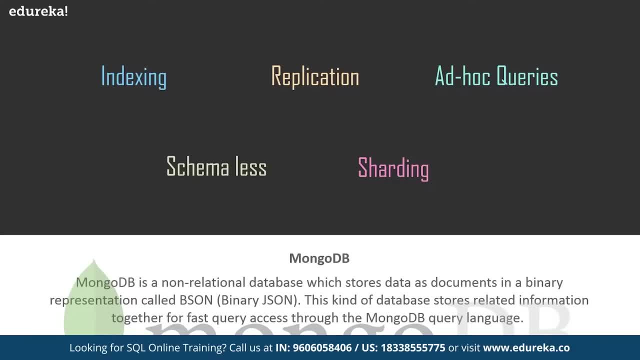 to enable deployments with large data sets and high throughput operations. So, guys, these are the mainly five features of MongoDB, that is, indexing, replication, ad hoc query, schema list and sharding. So there's, Now that you know what my sequel is and what MongoDB is, let's 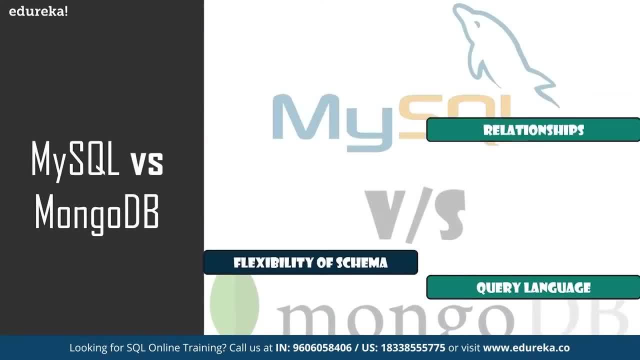 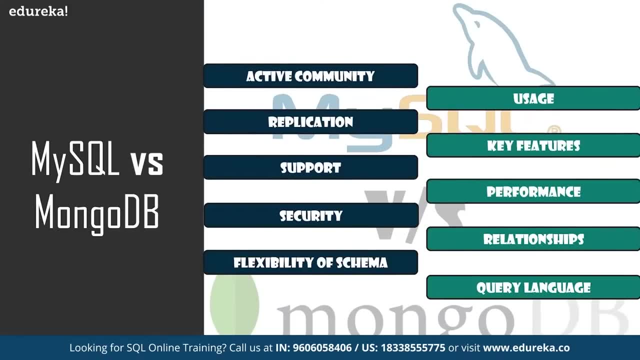 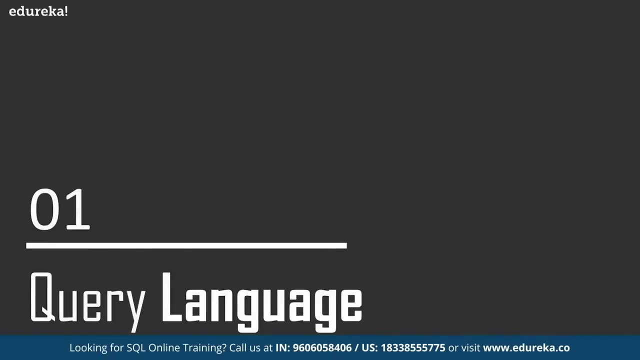 compare these two databases based on the grounds that you can see on the screen, that is the query language, to flexibility of schema, the relationships, security, performance, support, key features, replication, usage and active community. So now let's get into detail with the first comparison factor, that is, the query language. 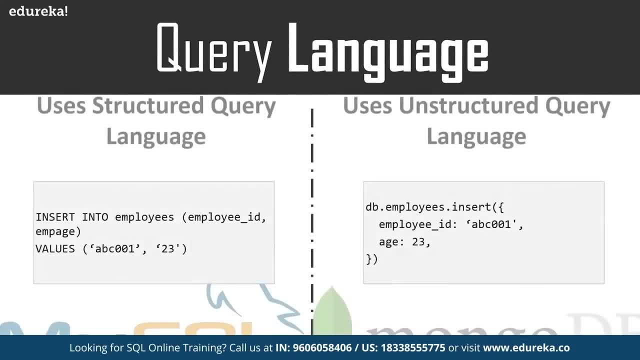 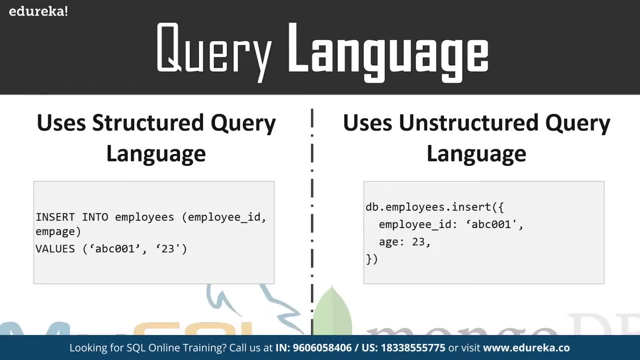 Now my sequel uses the structured query language to communicate with the database. Not only is it simple, It is also very powerful Language, which consists of mainly two parts, that is, the data definition language and the data manipulation language. MongoDB, on the other hand, uses an unstructured query language to build. 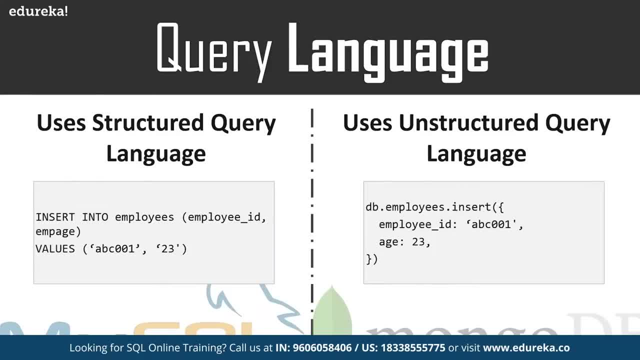 a query in Jason documents, You need to specify a document with various properties You wish the results to match. it is typically executed using a very rich set of operators that are linked with each other. using Jason now, MongoDB treats each property as having an implicit Boolean and it basically also supports Boolean or queries. 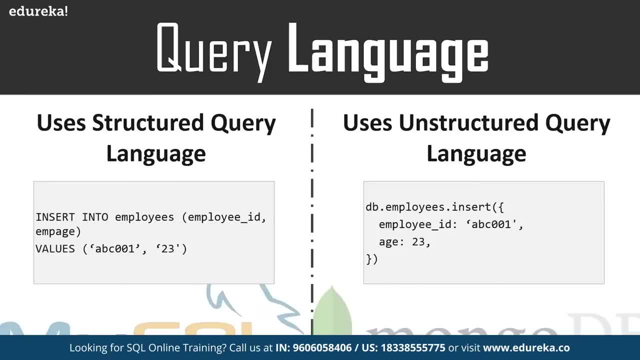 but you must definitely use the special operator dollar or to achieve it. So to make you understand better, I've considered the example on the screen. So to insert the data into the employees table in the sequel query you just have to type in: insert into employees. 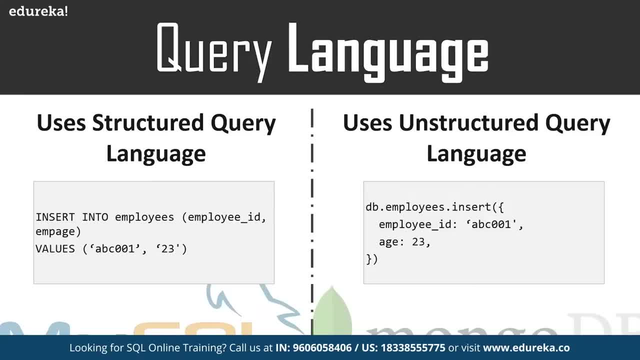 That is basically your table name and insert into is your SQL syntax. and then you mentioned the column names, that is, the employee ID and employee age, and then you use the SQL syntax, that is the values, and mention the values for the fields. So to just insert data into the table. 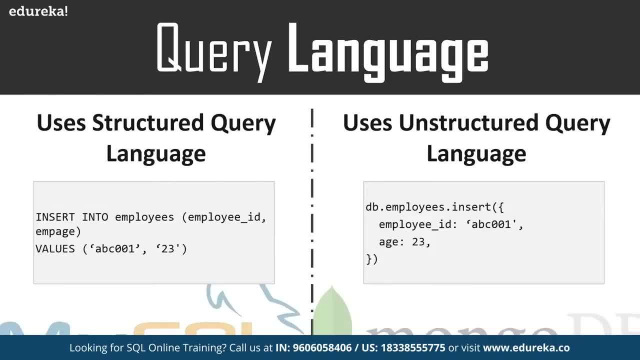 Well, you mentioned: insert into employees employee ID, employee age values, and then you mentioned the values. now, similarly, in the same scenario, If you wish to insert the data into a collection which is stored in the MongoDB database, What you simply have to do is you have to mention DB dot. 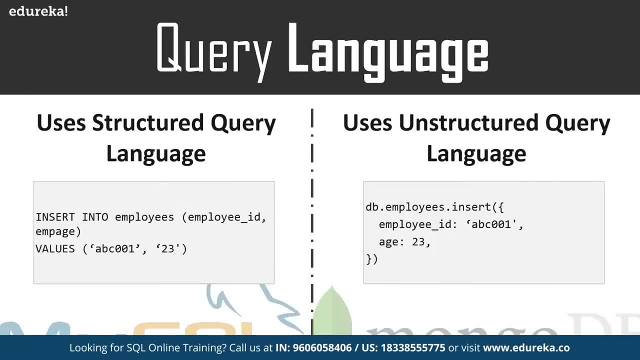 employees dot. insert where employees is the collection name, and then you have to mention employee ID and then mention the value and then mention again age and the value. So basically over here, employee ID, and age are basically the fields. So, guys, this is how you know the query language. 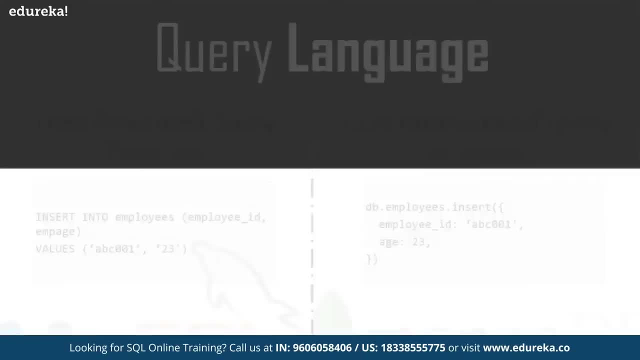 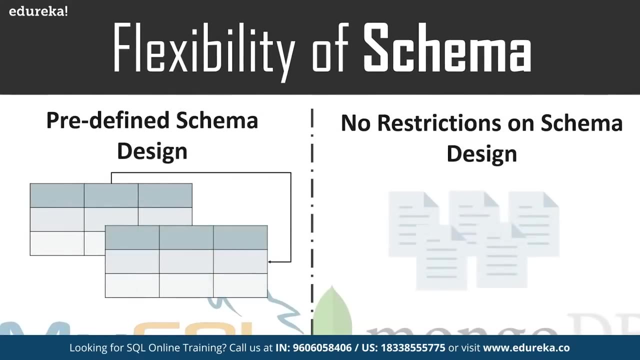 Between my sequel and MongoDB differs. next, We'll be comparing these databases based on the flexibility of schema. now, in the perspective of flexibility of schema, Let me tell you that you know, before you can store anything in my sequel, you need to clearly define tables and columns. 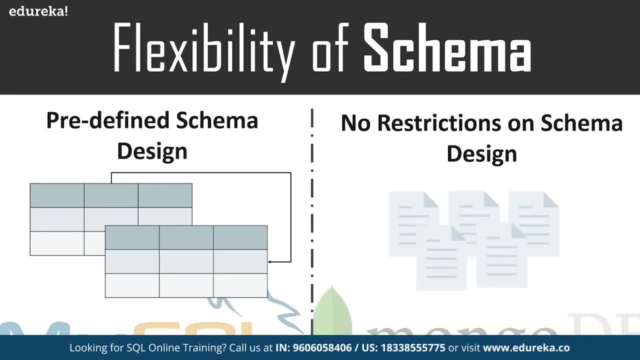 and every row in the table should have the same column. Now, This is basically because there isn't much space for flexibility in the manner of storing data If you follow normalization. for example, if you have an employee database, you need to create a table which can hold the data. 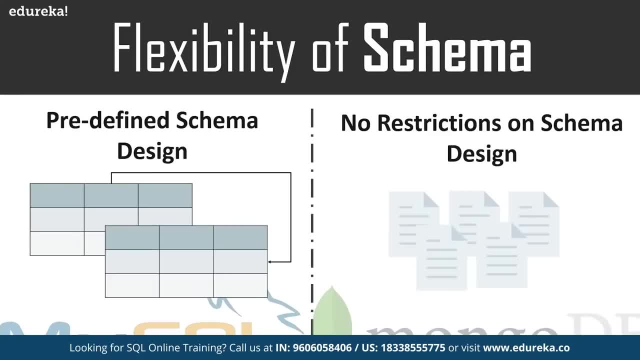 of employees. Now This table. You can have many attribute values, such as the employee ID, employee name and so on. now, similarly talking about MongoDB, One of the best things about MongoDB is that you know there are no restrictions on the schema design, so you can directly drop a couple of documents. 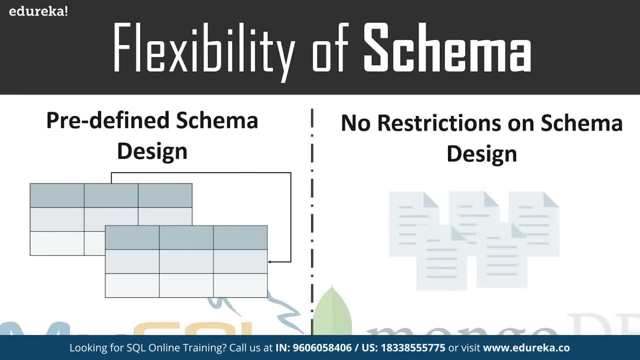 within a collection and it isn't necessary to have any relations between those documents. Now, the only restriction with MongoDB is that you need to frequently optimize your schema based on how the application will be accessing the data. now MongoDB stores the data in the JSON type manner. 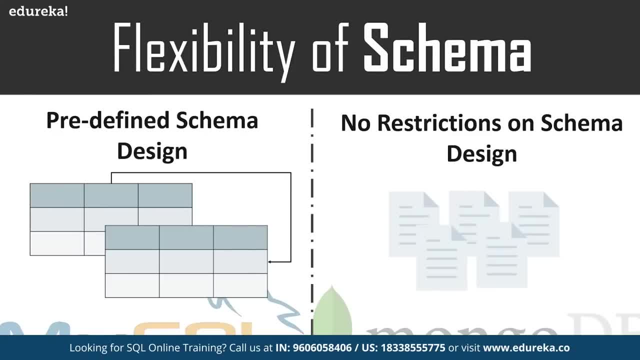 So, if you consider the previous example, there is the employee table. the data in MongoDB would be stored, as you know: employee ID- and then we have to mention the employee ID. that is basically the value for employee ID, then employee name and then you have to mention the employee name: employee. 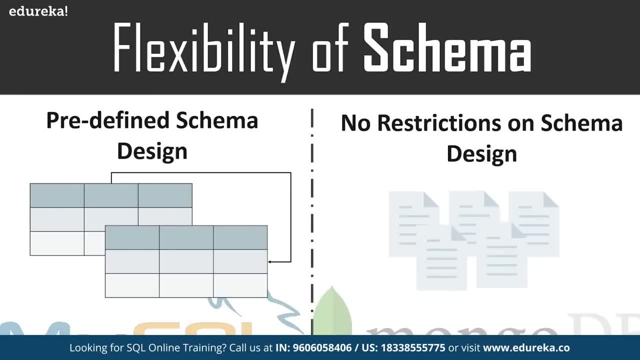 age and so on. So basically, this will be considered as a document, and now these documents can be stored in a collection as well. So basically, MongoDB creates schema list documents which can store any information you want, though It may cause problems with the data consistency. 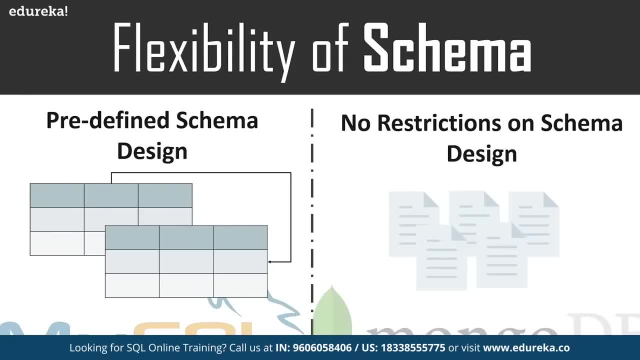 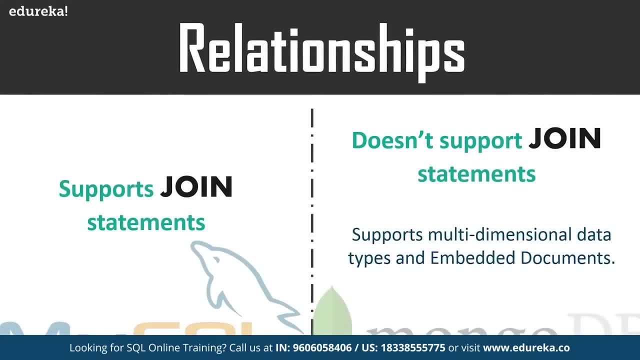 Whereas the MySQL follows a strict schema template. now, moving on to the next parameter, which is relationships. now, when we talk about relationships, MySQL supports the join operations. So, to explain you in simple terms, join makes the relational database relational. So, basically, the join allows the user to link the data. 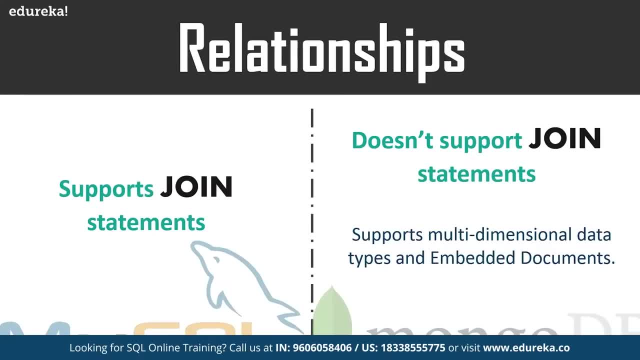 from two or more tables in a single query with the help of the select command. So, for example, if you want to retrieve the data from the employee in the projects table based on the matching column, you can easily obtain the desired data by applying any type of joints. just the inner left right. 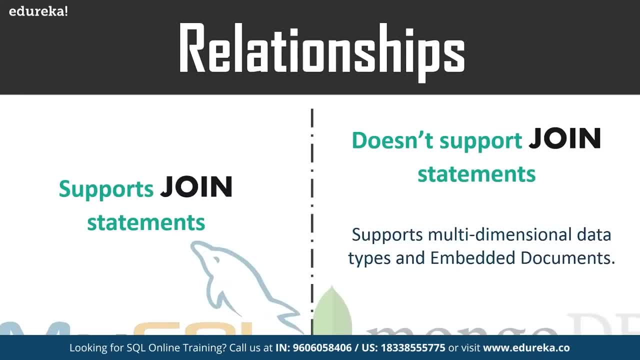 or full, based on your need. now coming to MongoDB, Well, MongoDB does not support the joint statements, but it supports the multi-dimensional data types, such as arrays and even other documents. So the placement of one document inside another document is basically known as the embedding of document. 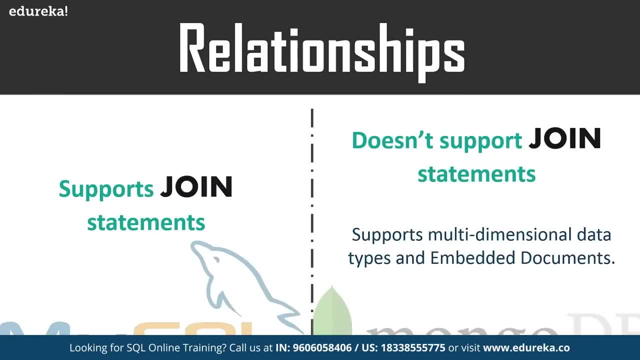 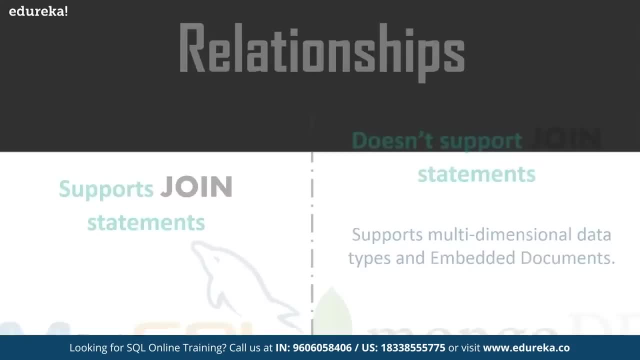 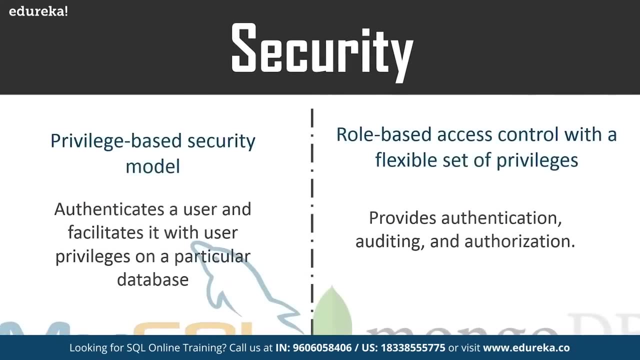 and MongoDB supports the embedding of documents. So, talking about relationships, guys, MySQL supports the joint statements and the MongoDB does not support any joint statements. Next, Let's discuss the security factor for both of them, the talking about MySQL first. MySQL uses a privilege based security model. 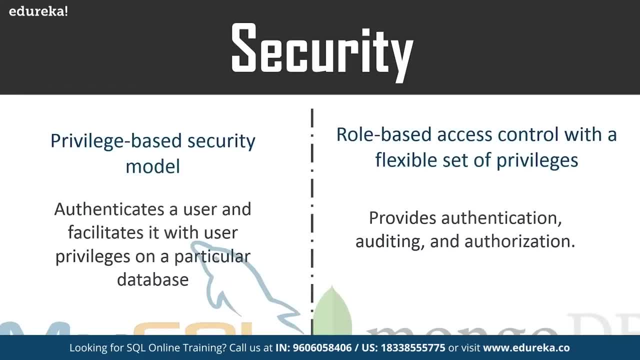 This means that you know it basically authenticates a user and facilitates it with the user privileges on a particular database, such as create, select, insert, update and so on. now coming to MongoDB. MongoDB uses a role-based access control with the flexible set of privileges, its security features. 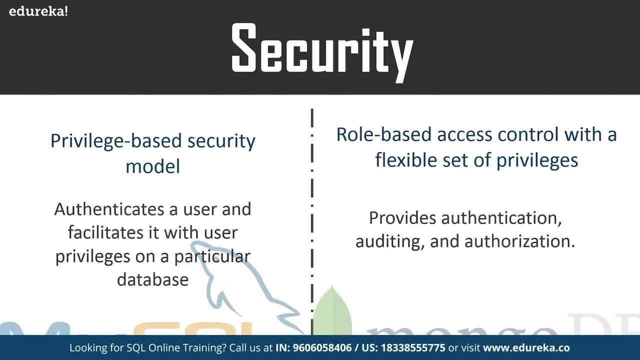 basically include the authentication, auditing and authorization. not only this, but it is also possible to use the transport layer, security and the secure socket layer for encryption purposes in MongoDB. So basically, this ensures that you know it is only accessible and read it by an intended client. 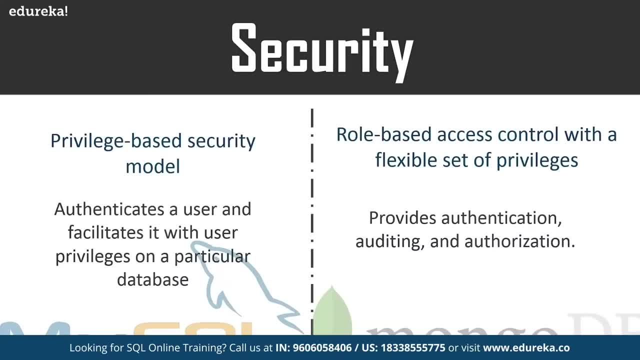 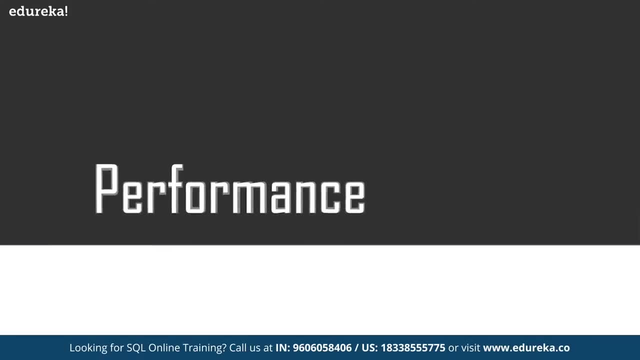 No other client can go through the documents. So, guys, that's how the security is provided in MySQL and MongoDB. now let's move forward to the next factor of comparison, that is performance. So I'm comparing MySQL and MongoDB on this parameter. MySQL is quite slower in comparison to MongoDB. 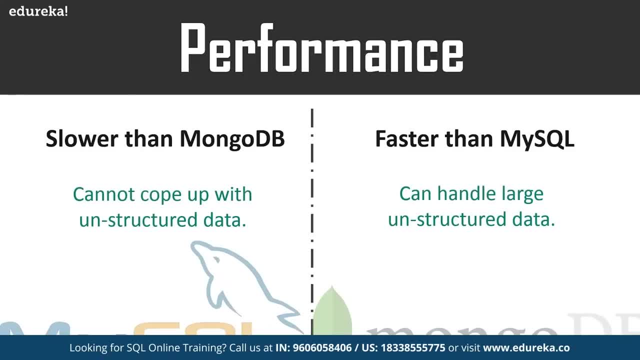 when it comes to dealing with the large databases. This is mainly because, you know, my sequel can't cope up with large and unstructured amounts of data, Whereas MongoDB can. so that's the reason, guys, MongoDB is much faster than MySQL. now talking about MongoDB, MongoDB. 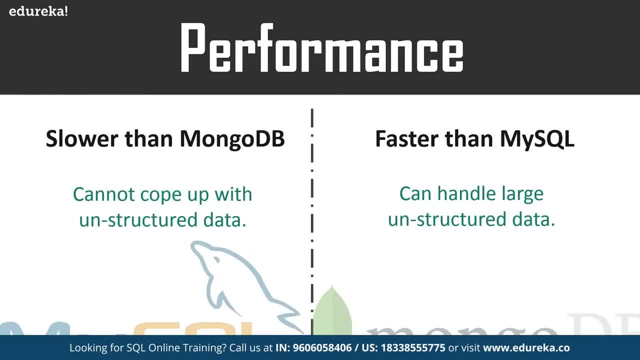 has the ability to handle large unstructured data. It's much faster than MySQL because it allows the users to query in a different manner that is more sensitive to workload. But yes, there is, as such, no benchmark on. you know which database is faster, because you know. 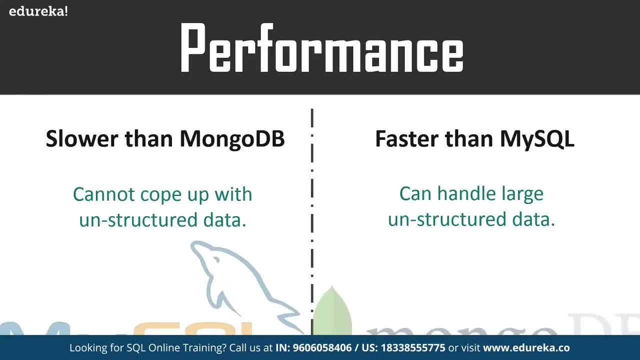 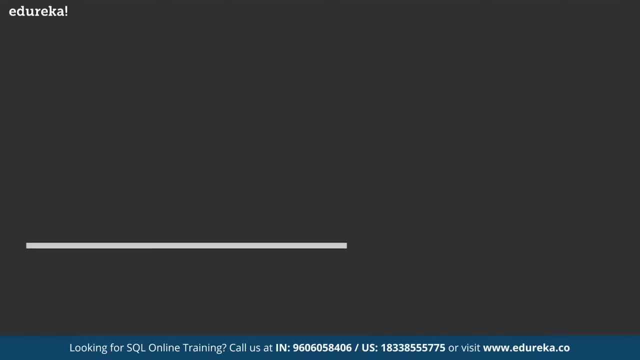 only your demands, your data and your infrastructure can tell what you need and which database can provide you the output faster. So, guys, that was about performance. next, We'll be comparing these databases based on support. Well, both of them offer excellent support 24-7. 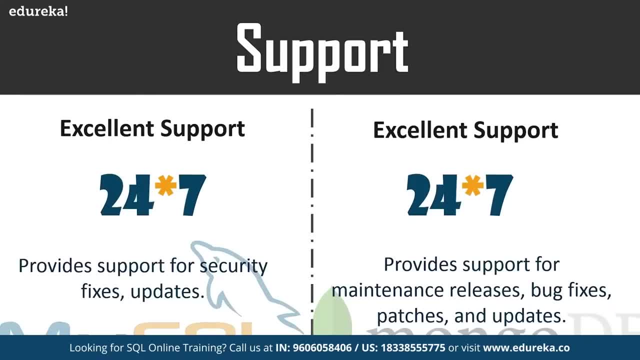 for security fixes, maintenance releases, bug fixes, patches and updates. So there is, as such, no difference between both of them based on this parameter, as both of them offer good support. So, guys, that was about support. now, moving on to the next parameter, which is key features. the key features: 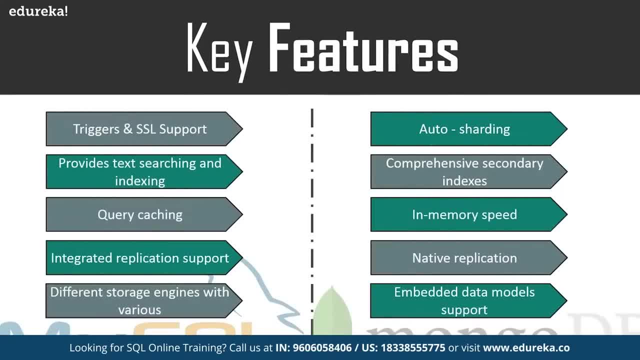 Of my sequel in MongoDB are as you can see on my screen. Let's start with my sequel first. the key features of my sequel are mainly triggers and SSL support. provides text searching and indexing, also allows query caching, provides integrated replication support and also provides different storage engines. 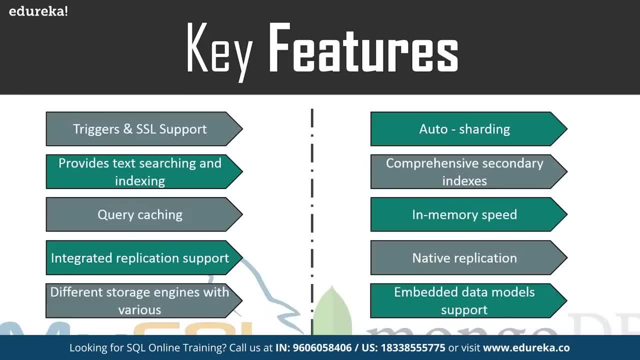 So, guys, these were the key features of my sequel, not talking about MongoDB. MongoDB supports auto sharding, comprehensive secondary indexes in memory speed, native replication and embedded data model support. So these were few features of my sequel and MongoDB. So, yes, there are various differences between both these. 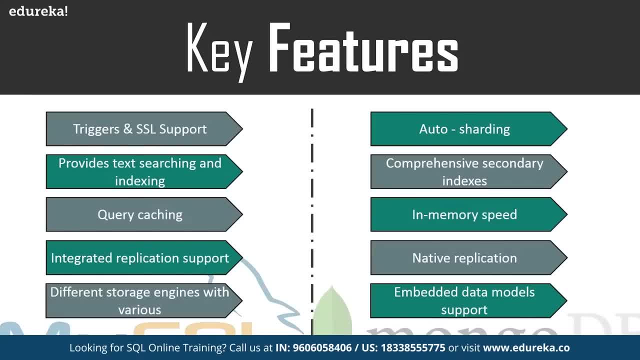 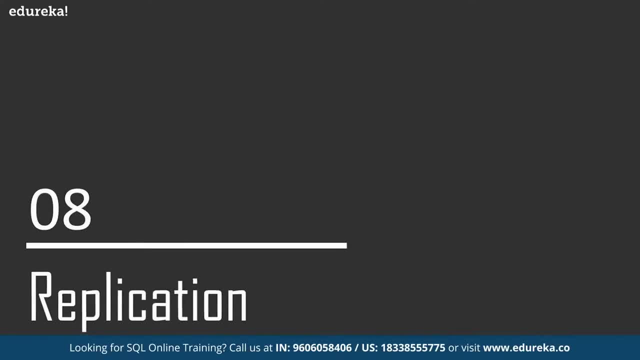 databases. but there are few key features, you know, which help both my sequel and MongoDB to win in their own market. Now, next point of comparison we have is replication. Now my sequel supports the master slave replication and the master master application. as of my sequel, 5.7.6. 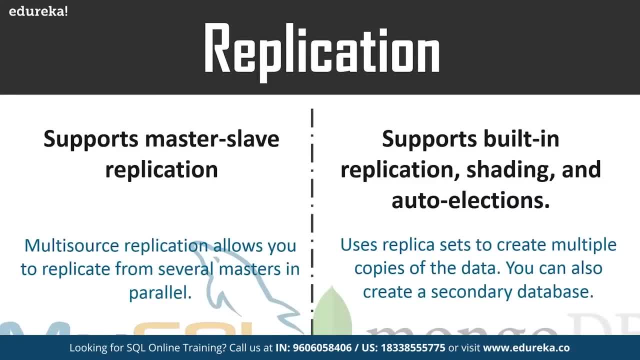 and later, and this kind of multi-source replication allows you to replicate from several Masters and parallel. talking about MongoDB, MongoDB supports the built-in replication sharding and Auto elections. So by using Auto elections you can set up a secondary database to automatically take over if the primary database phase, so sharding allows. 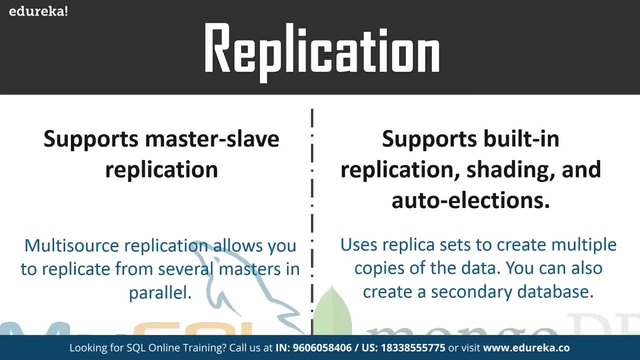 for horizontal scaling, which is difficult to implement in my sequel, as my sequel is vertically scalable. not only this, but MongoDB also uses replica sets to create multiple copies of data, So each member of the replica set can have the role of primary or secondary at any point in the process and the read. 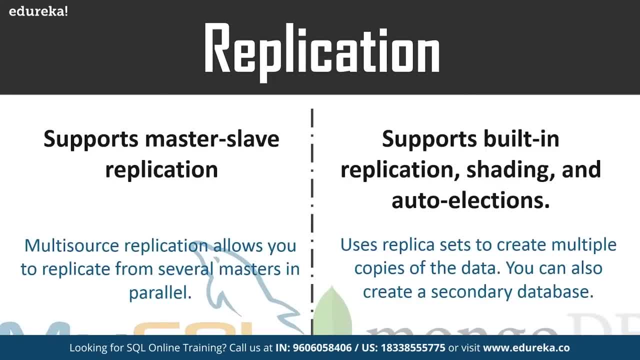 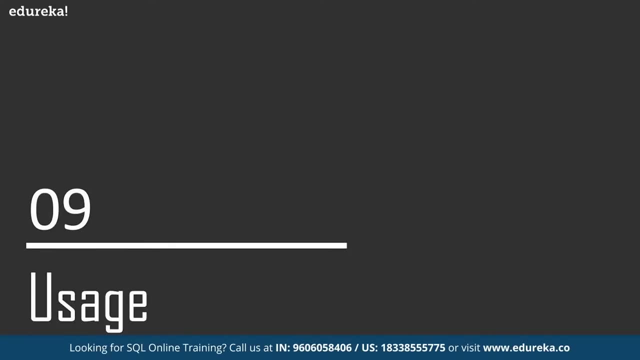 and write. These are done on the primary replica by default and then replicated to the secondary replicas. So, guys, this was about the replication. my sequel supports the master slave replication and the MongoDB supports built-in replication, sharding and Auto elections. next We'll be comparing these tools based on usage. now, 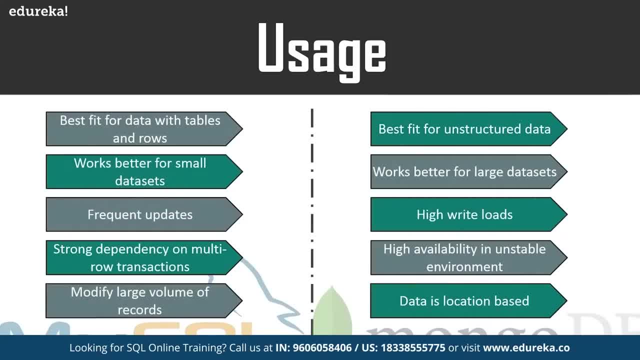 for this factor. I'm going to tell you where you can use my sequel and MongoDB, So let's start with my sequel first. my sequel is the best fit for data with tables and rows. this works better for small data sets and allows frequent updates. 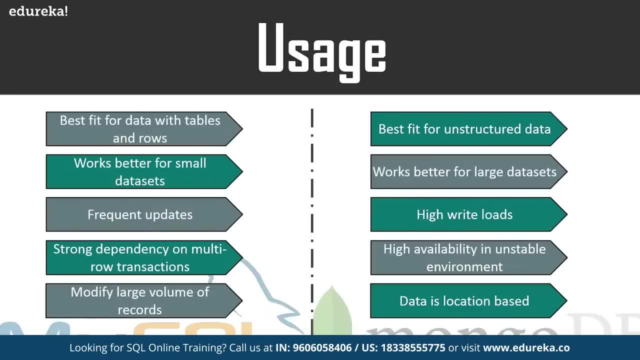 My sequel is also used for strong dependency on multi-year transactions and is also used when you want to modify large volumes of records. talk about MongoDB. MongoDB best fits for unstructured data and works better for large data sets. This is also used when you have high right loads. 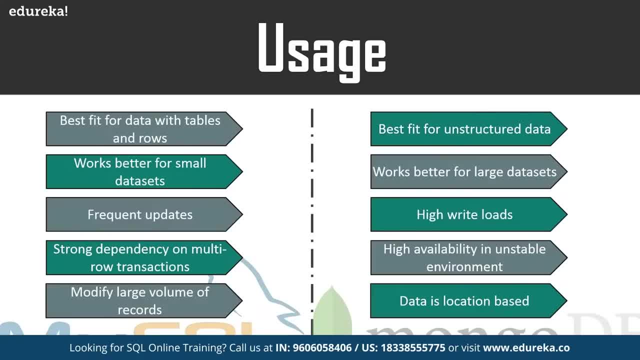 and high availability in unstable environment and the data is completely location-based. So this was about my sequel and MongoDB guys. my sequel mainly best fits for data with tables and rows and MongoDB Best fits for unstructured data. Finally, the last but not the least, factor of comparison: 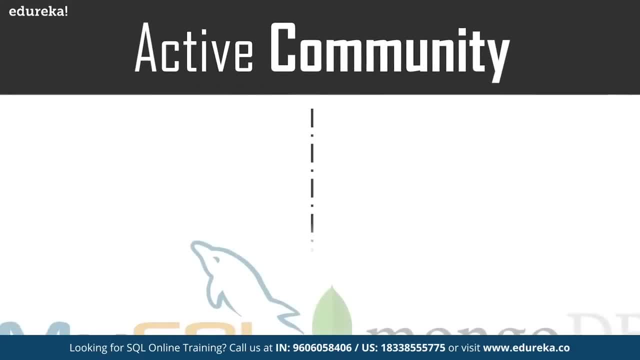 is the active community. the my sequel database is mainly owned and maintained by the Oracle Corporation, So they offer a developer zone on the my sequel website and the community for my sequel is, I would say, much better than that of MongoDB. So if you want to support both of them, offer good support. 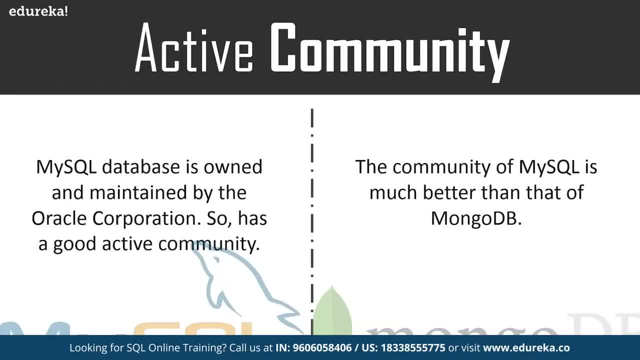 but yes, if you talk about active community, then my sequel has a better active community than compared to MongoDB. So, guys, now that I've told you so much about my sequel and MongoDB, Let me just shift to my my sequel workbench and MongoDB compass, so that I show you how you can create tables. 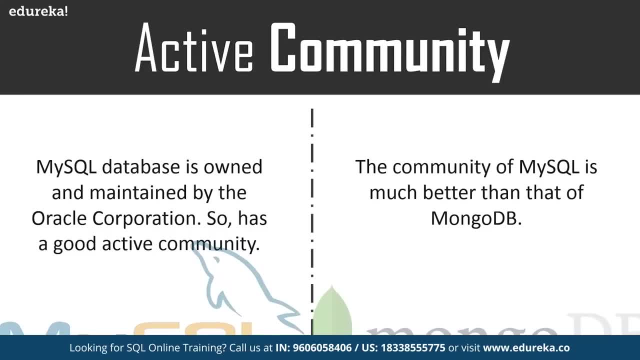 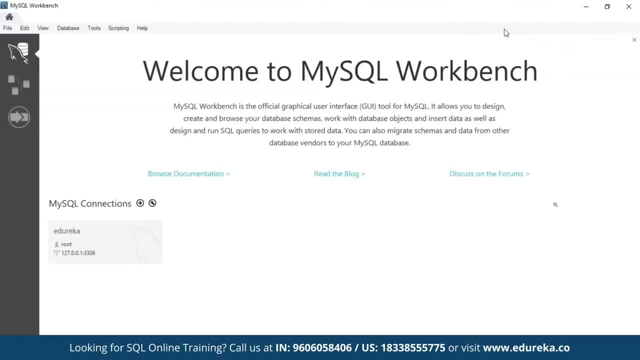 and databases in my sequel and how you can create databases and collections in MongoDB. So first we'll be looking into my sequel. So for that I'll open my my sequel workbench. So, as you can see on my screen, this is my my sequel workbench. 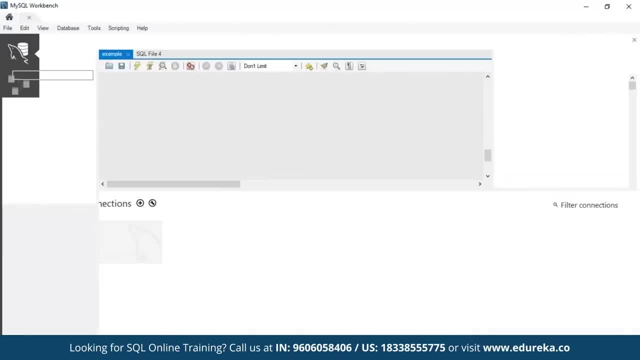 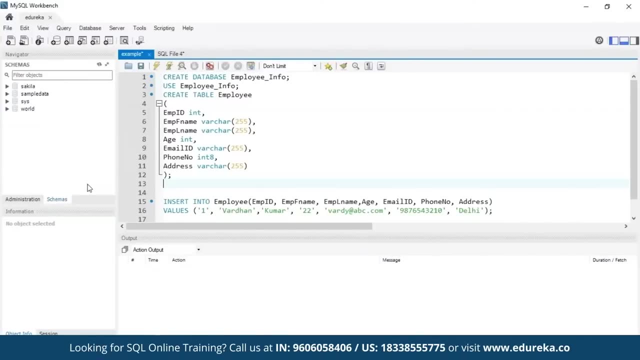 So I'm just going to open my connection. So, guys, this is how your my sequel workbench looks now, to show you how you can use my sequel. I've already written the commands, So I'm just going to tell you how you can use them. 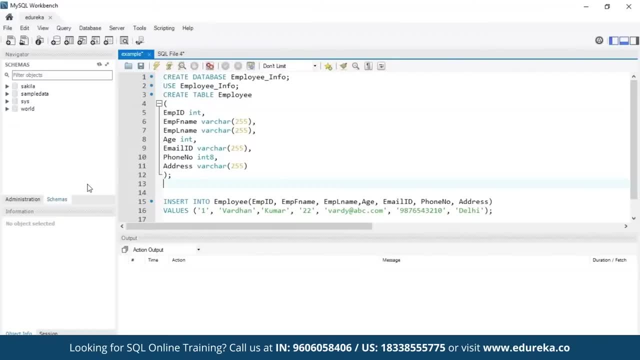 So to create a database, I've used to query create database and I've mentioned the database name, that is, employee info. So this is a sequel language, guys, where you know create and database are the sequel syntax and employee info is the data parameter. So I'm going to just execute this particular query. 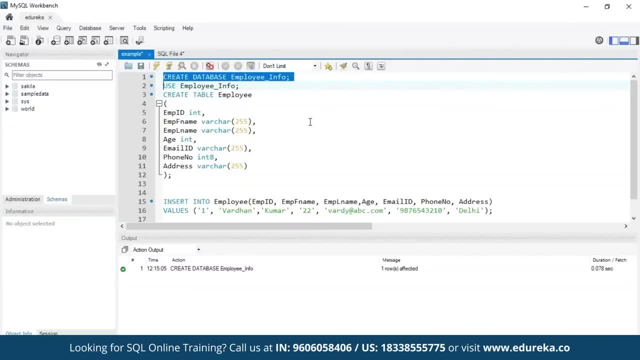 Now, once the query is executed, you can clearly see that you know the database has been created. now to use this database, You can just directly use database name, that is employee info. So if I just execute this query again, you'll clearly see that you know. 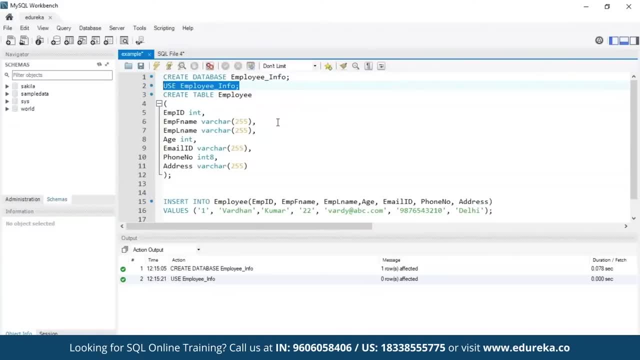 we'll be using this particular database now to create a table inside this particular database. You can use the query, like you know, create table, table name and then you mentioned all the field names and the data types. right, So we are. I have different field names, like the employee ID. 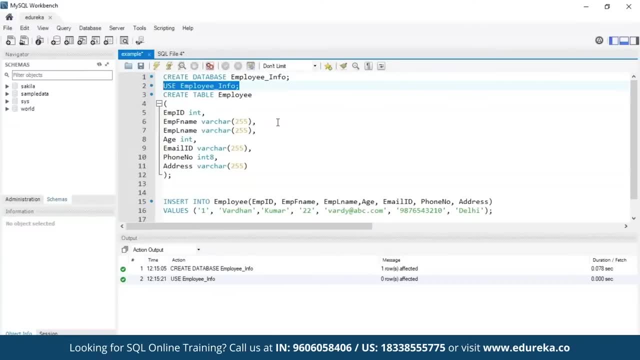 employee: first name, last name, age, email ID, phone number and address and their specific data types. right, So I'm going to just execute this particular query. So once I execute this particular query, you can see that you know a table has been created. 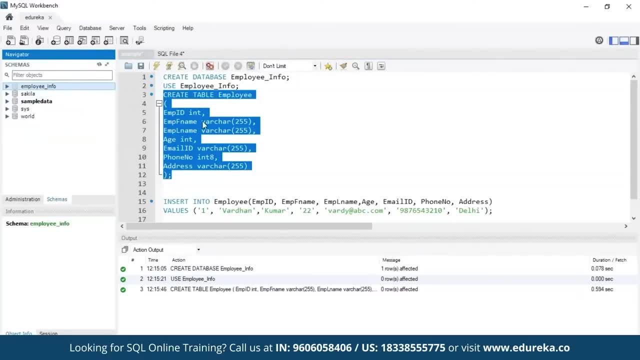 So now, if we just look into our databases, we have a database that is employee info and then we have a table inside it. now to insert data into the table, What you can use is you can just use the query insert into table name that is employee. over here, mention all the field names. 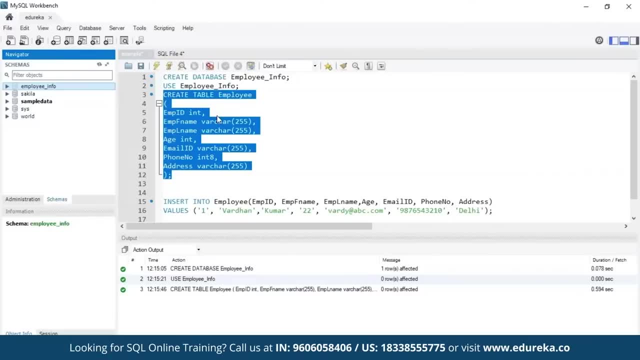 then use the SQL syntax keyword values and then mention all the values. right? So we are. I've written a query as insert into employee employee ID: first name, last name, age, email ID, phone number, address values and then I've mentioned the values, right. 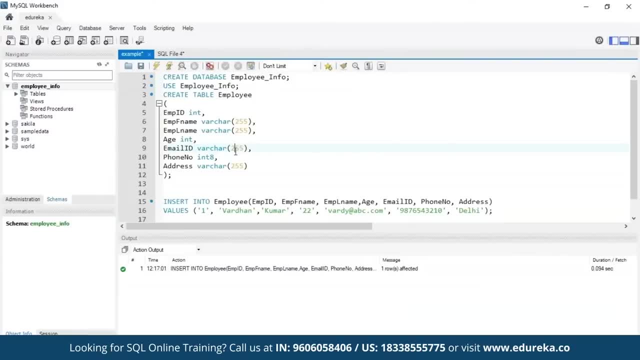 So I'm going to just execute this particular query. So once the query has been executed you can clearly see that you know the data has been inserted into the table. So I'll just go to the employee info table. go to the tables option. 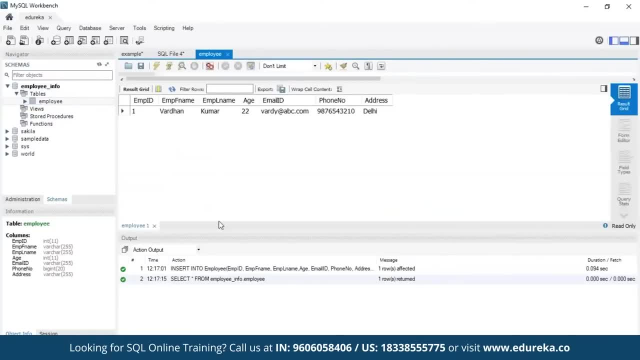 go to employee and then I'm going to just look into the table. So when I just check into the option of view, you can clearly see that you know our first record has been inserted. So, guys, that's how it's really simple to use my SQL. 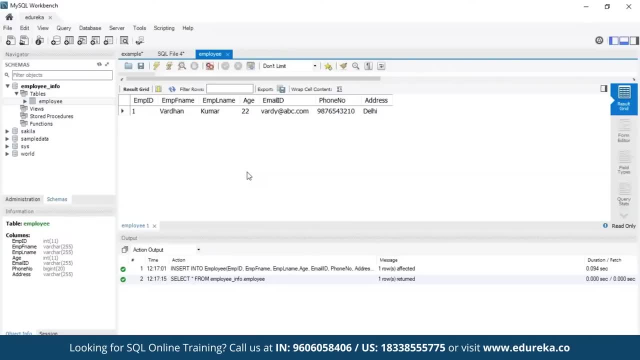 and with the help of my SQL workbench, you get the GUI experience. you know where you can easily mention your required queries and then get the outputs right. So that was about my SQL workbench, guys. now shifting to MongoDB compass. So, guys, 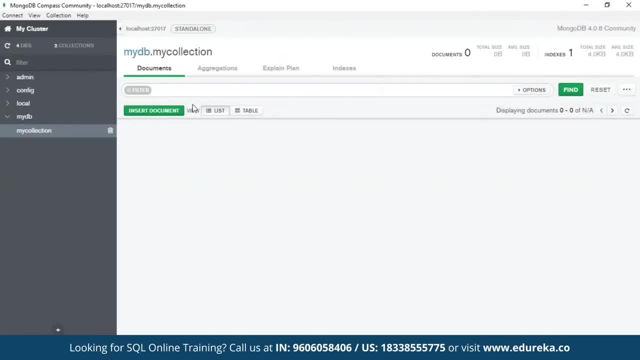 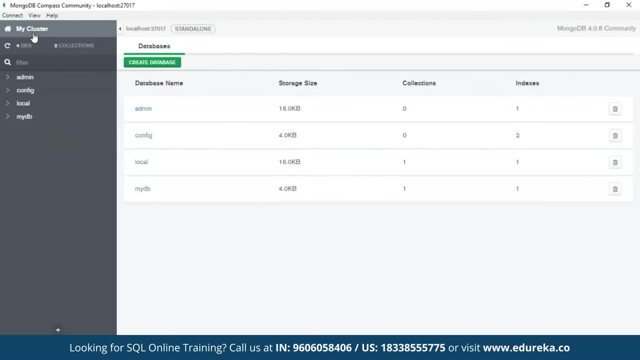 this is how the MongoDB compass looks. so basically, I've already created a database. Now, if you just wish to go and check how a database has been created, What you can simply do is you can go over here to my cluster And once you go to my cluster, you get an option of create database. 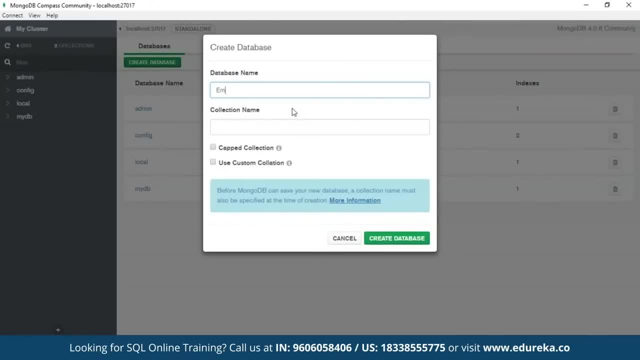 right. So I'm just going to create a database. So let's say I mentioned it to be employee info and then over here, since I've told you, database has collections and then collections have documents. So basically a group of documents is collections and a group of collections is a database. 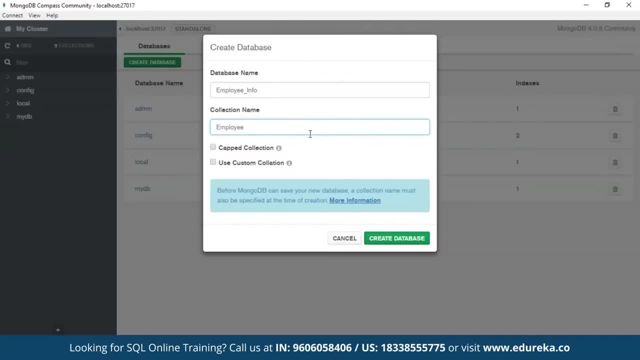 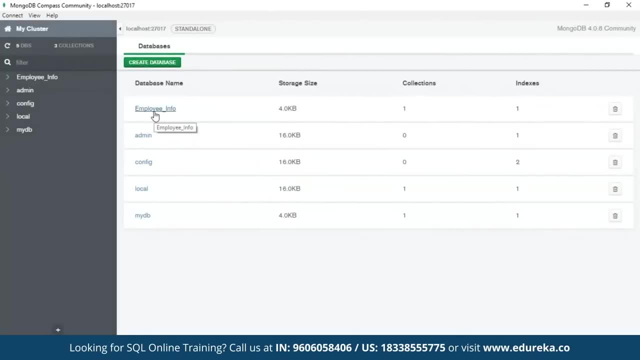 I'm going to mention my first collection name- Let's say you know employee- and then I'm going to just click on create database. So once I click on create database you can clearly see that you know my database has been created. that is employee info. 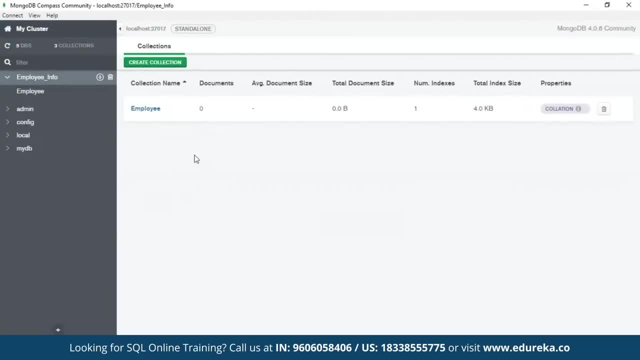 So I'll click on this and you'll see that. you know we already have a predefined collection created. Now, apart from this, you can also have a number of collections to be created, But since I'm just showing you how you can use MongoDB, 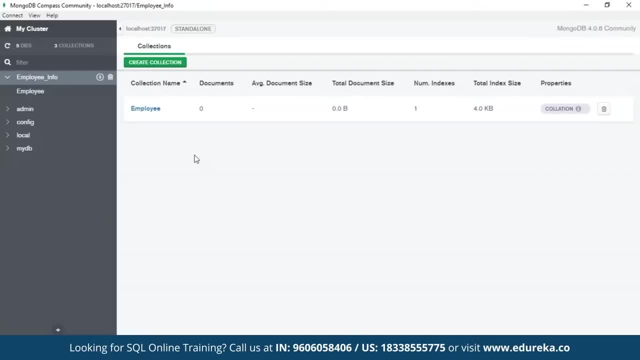 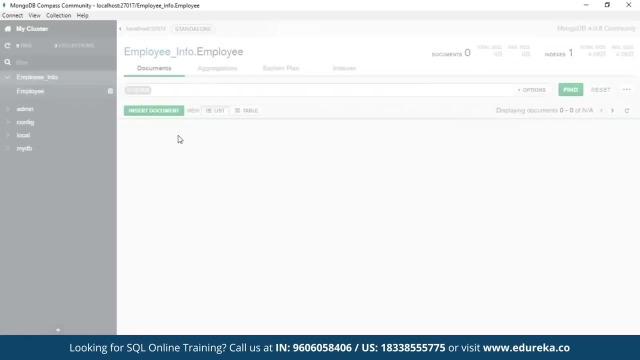 I'm not going to create many more collections. This is just a single collection that I've already created. Now, what you can do is you can again create documents. It's inside this particular collection. to do that, You have to click on this collection. 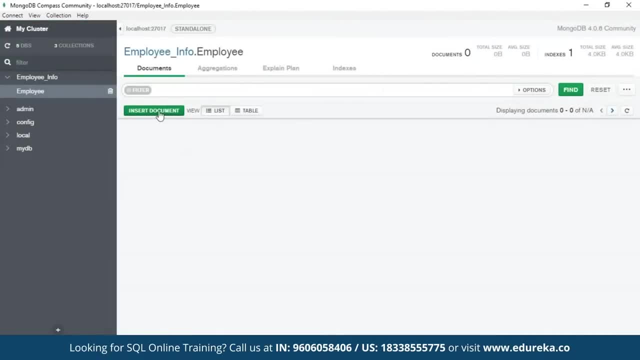 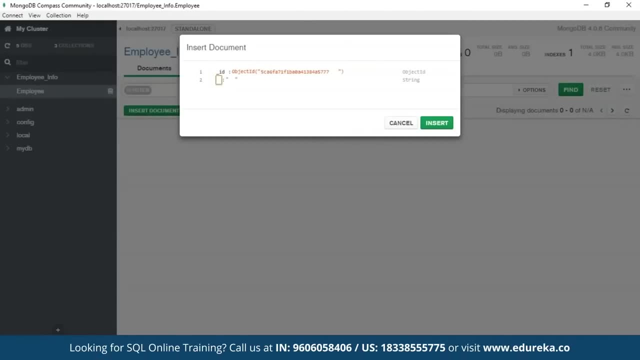 That is the employee collection, and over here you get an option for insert document, right? So you can just click on this option of insert document, mention the required values. That is basically the ID, dot, object ID. So basically over here you can just mention employee ID. 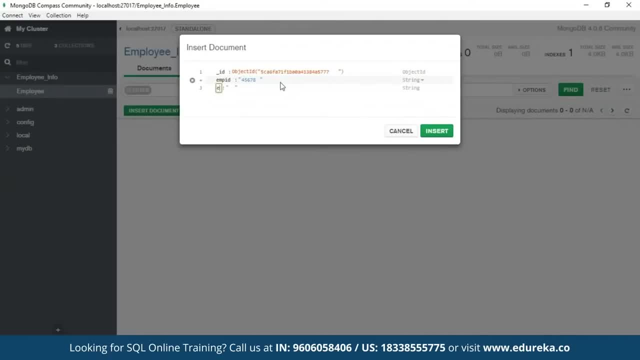 and in this section you can just mention the employee ID. Now, similarly, you can mention the employee name also, and over here I'll mention the employee name to be, let's say, sahiti, right now. over here, If you see, we can also use the data type. 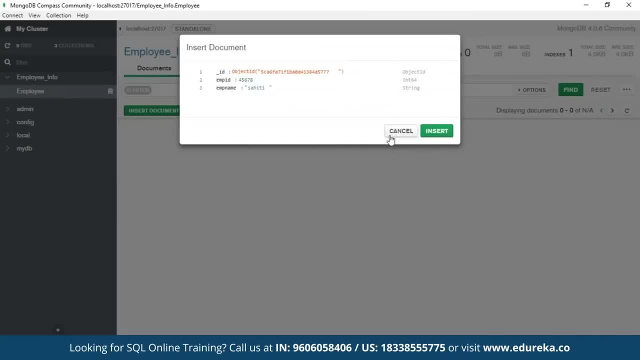 So let's just say, you know our employee ID should be int, So I just mention it to be end and employee name to be string, right? So that's how you can mention the data types for your documents And then, once you've inserted all the required values, 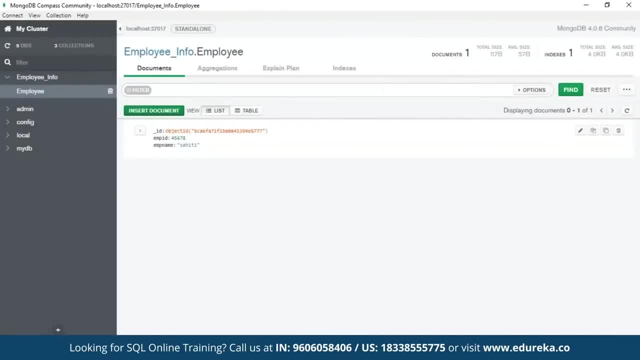 you can just click on insert. So once you click on insert you can clearly see that you know your document has been created. now this you can either view in the form of a table that is basically you know which document ID basically has which employee ID. 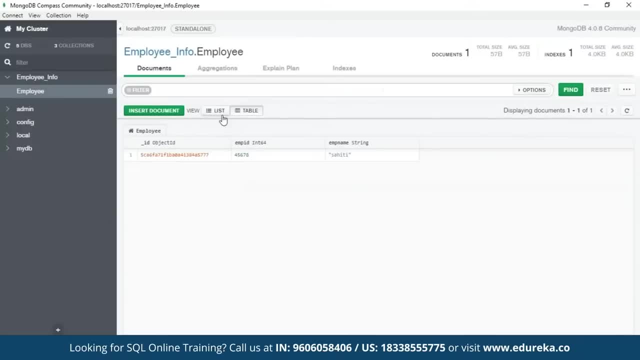 that is, which data type and also the employee name, or you can also view it as a list, So I was previously viewing it as a list. This is how you can create a database and then create a collection and documents. Well, I'm not going to go in depth of how you can use this. 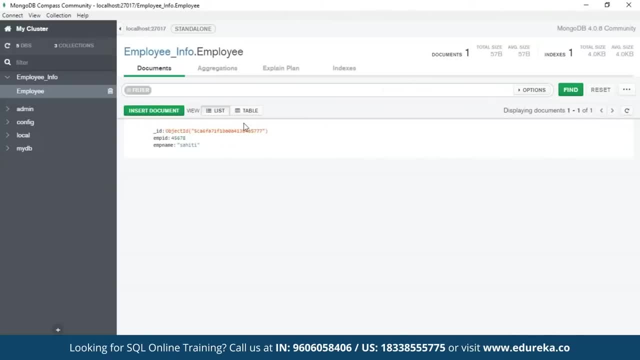 MongoDB compass and how you can explore much more features of this. So, guys, it was just a short demo on. you know how you can use my sequel workbench and MongoDB compass to handle structured data and unstructured data. So, folks, with this we come to an end of this space. 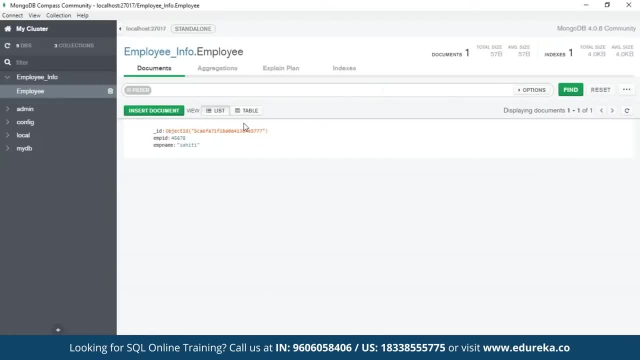 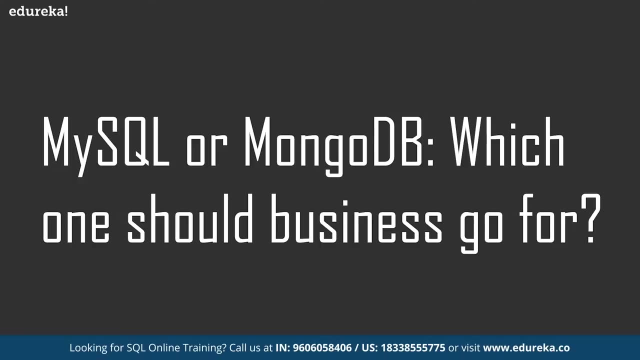 of between my sequel and a MongoDB, and I hope you understood all the points now. but knowing so much about my sequel and MongoDB would have definitely raised a question on your mind whether to use MongoDB or my sequel for your businesses. So, guys, well, there is no clear winner between both of them. 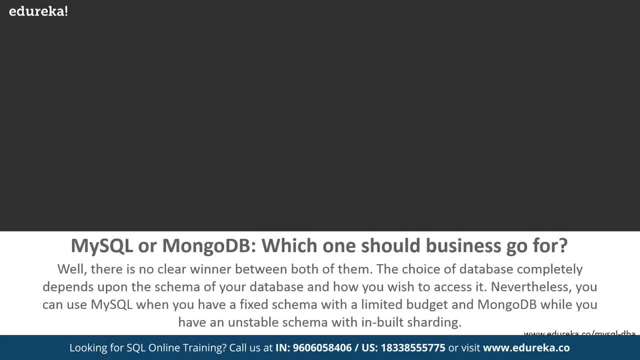 the choice of database completely depends upon the scheme of your database and how you wish to access it. Nevertheless, you can use my sequel when you have a fixed schema- high transaction, low maintenance, data security, with a limited budget and MongoDB- while you have an unstable schema. 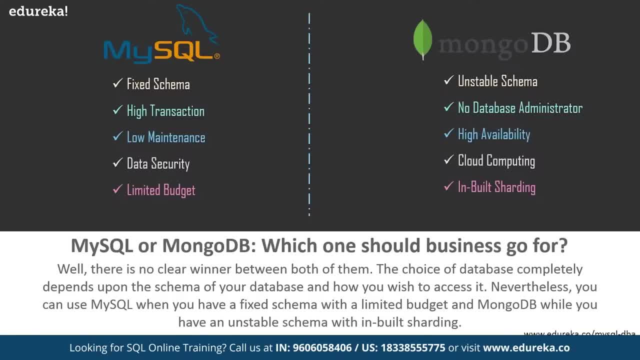 no specific database administrator, high availability cloud computing involved with inbuilt sharding. So, guys, this is when you use my sequel and MongoDB. There's no clear between both of them. It completely depends on you which type of database you would want to go for for your businesses. 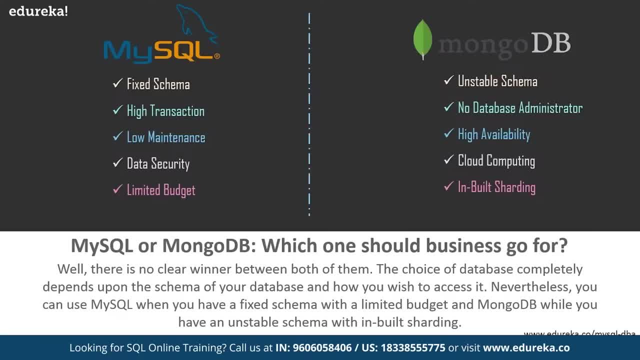 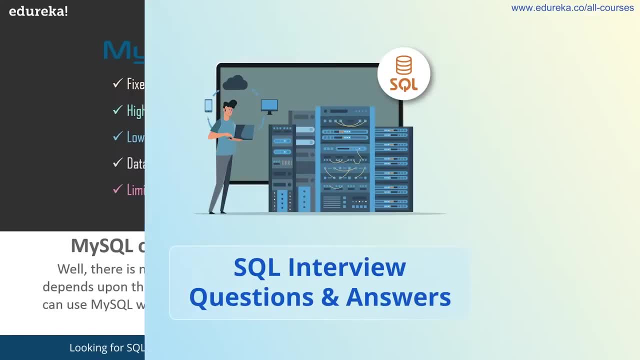 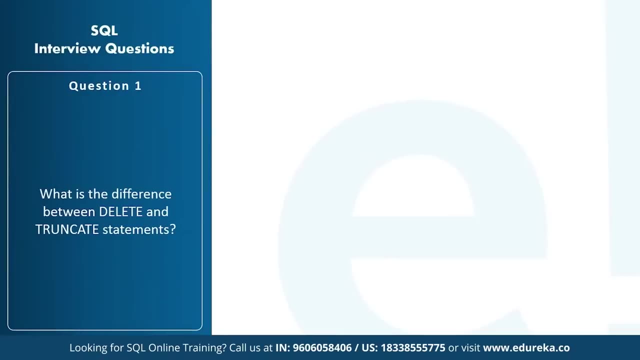 and how you think your business will be benefited by choosing which database. so there won't be any final verdict as to which among them is best, as each one of these Excel based on your requirements. So the first question that we have is: what is the difference? 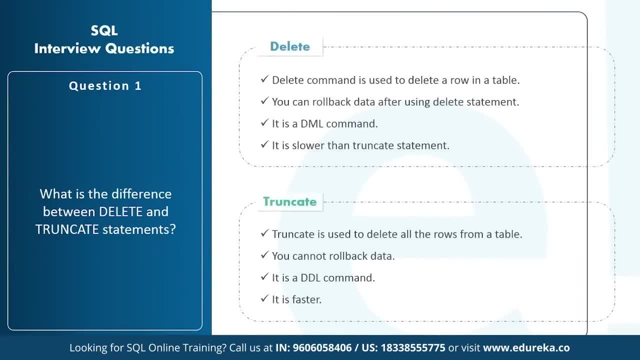 between delete and truncate statement. So I'll start by explaining you What is the delete command? Well, the delete command is basically used to delete a row in the table, So you can also roll back data after using the delete statement and it is a data manipulation command. coming. 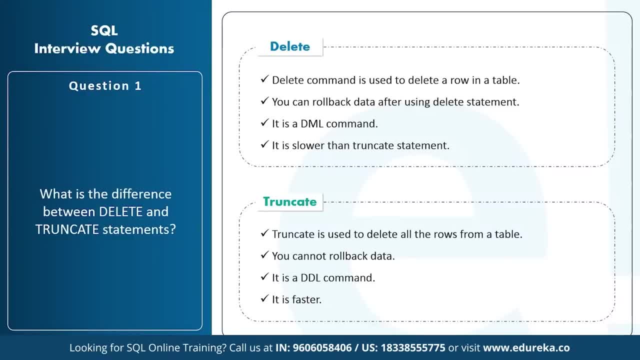 to the truncate statement. The truncate statement is basically used to delete all the rows from a table and you cannot roll back the data. This is a data definition language command and it is faster than the delete command. So if anyone ask you the difference between the delete, 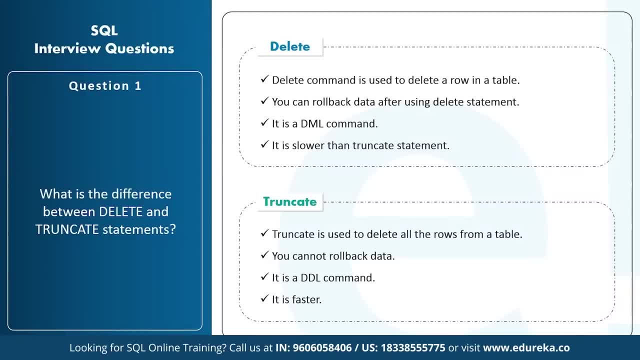 and the truncate statements. don't forget to mention that. you know, the truncate statement is definitely faster than the delete statement and the truncate statement is from the data definition family and the delete statement is from the data manipulation family. right now, moving on to our next question. 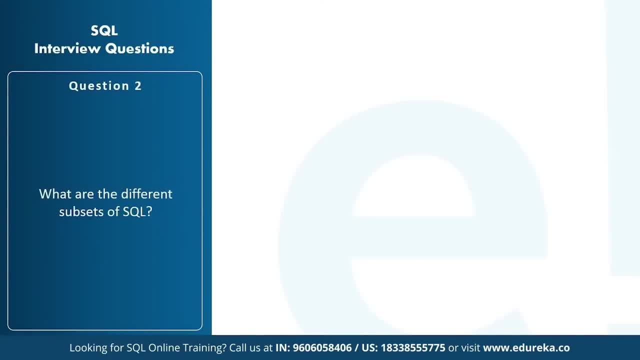 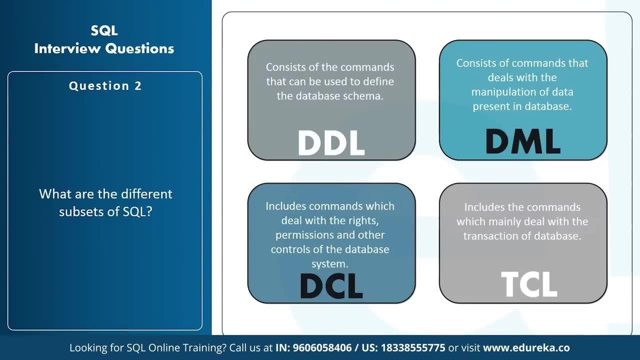 That is, what are the different subsets of sequel? Well, the different subsets of sequel are mainly the data definition language to data manipulation language, the data control language and the transaction control language. now, coming to the data definition language, this set of language Consists of the commands that can be used. 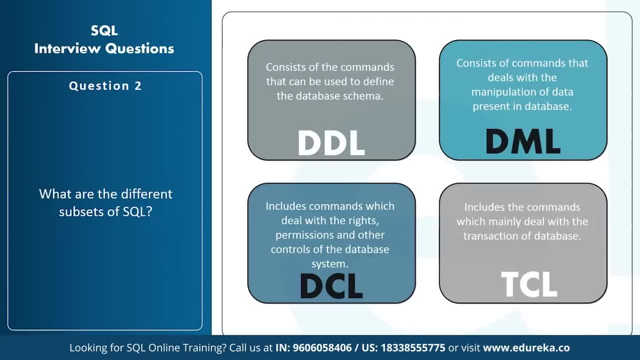 to Define the database schema. So whenever you want to Define the database schema, you can use the commands from this particular language. coming to the data manipulation language, the manipulation language consists of all the commands that deal with the manipulation of data present at the database. 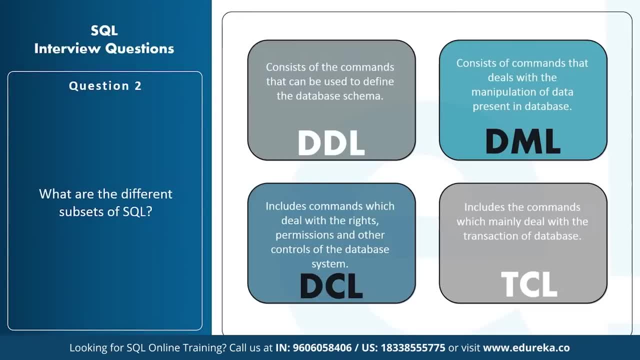 So, for example, if you have n number of tables and you want to manipulate the data and present in those tables, then you use data manipulation commands. coming to the data control language, The data control language includes the commands which deal with the right permissions and other controls of the database systems. 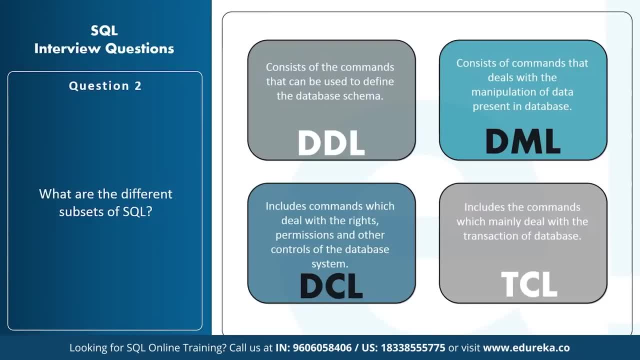 So, for example, you work for an Enterprise and the Enterprise has a database. now, obviously, all the employees will not have the access to the database, right? So data control language mainly deals with how you give the user permissions to access to the database. now, coming to the last type of language, 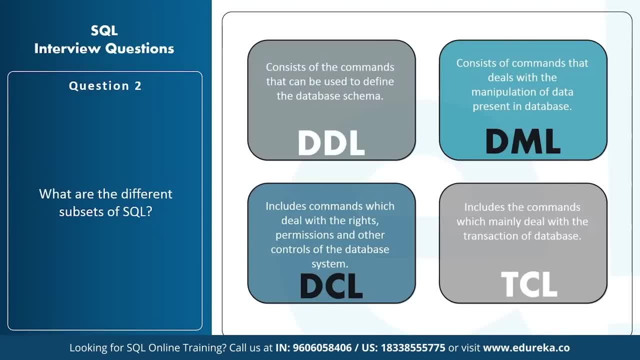 that is the transaction control language. This basically includes the commands which mainly deal with the transaction of the database. whenever you want to roll back or you want to perform any various kind of transactions, Then you use the set of commands from this language, right? 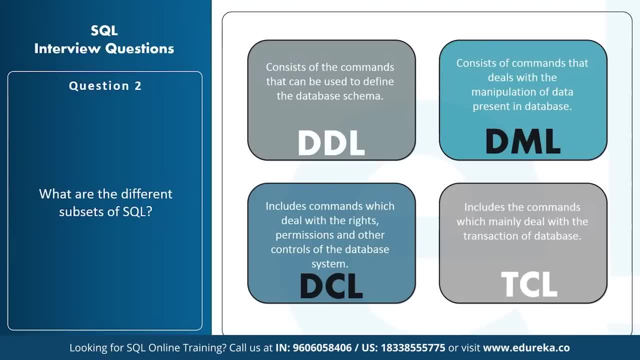 So I hope I'm clear. So, as I said, there are mainly four different subsets of SQL that you should mention. that is, the data definition language to data manipulation language, the data control language and the transaction control language. now moving on to our next question. 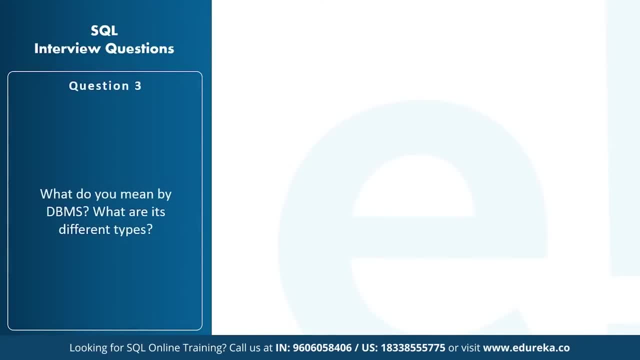 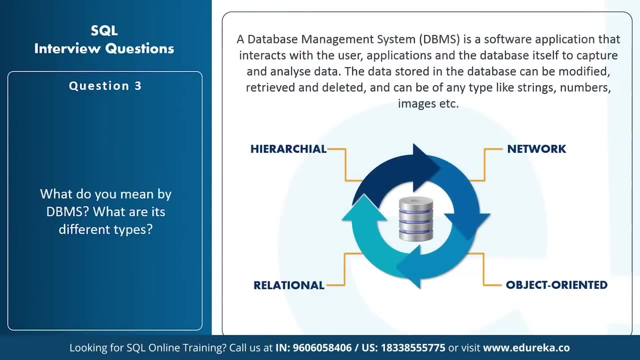 That is, what do you mean by database management systems and what are the different types of it. So now, if I have to define the database management system for you, then a database management system is a software application that interacts with the users, applications and the database itself to capture. 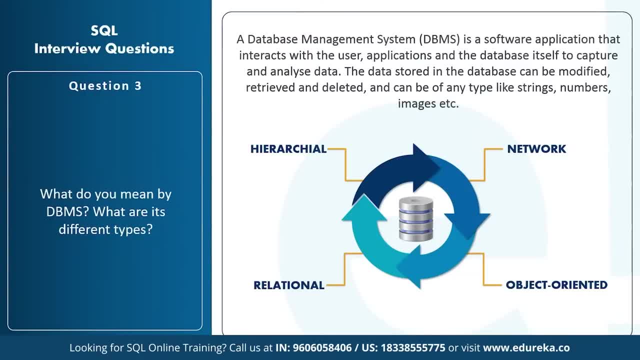 and analyze the data. so the data stored in the database can be modified, retrieved and deleted and can be of any type, like the springs numbers, images, Etc. So you can basically store any kind of data. Now the different kinds of database management systems are the hierarchical, the relational, the network. 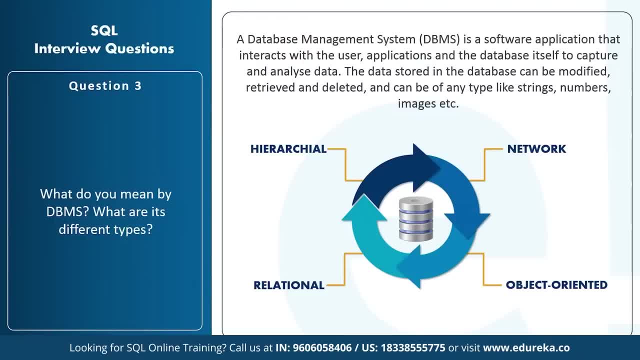 and the object-oriented database management systems. the talking about the hierarchical database management systems. this type of database management system has a style of predecessor and the successor type of relationship, So it has a structure similar to data for tree, when in the notes report represent the records and the branches of the tree represent 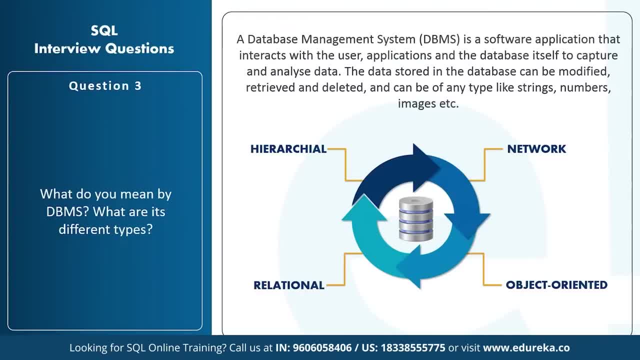 the fields. coming to the relational database management system, This type of database management system uses a structure that allows the user to identify and access data in relation to another piece of data in the database. The network database management system supports many to many relations where in multiple member records can be linked. 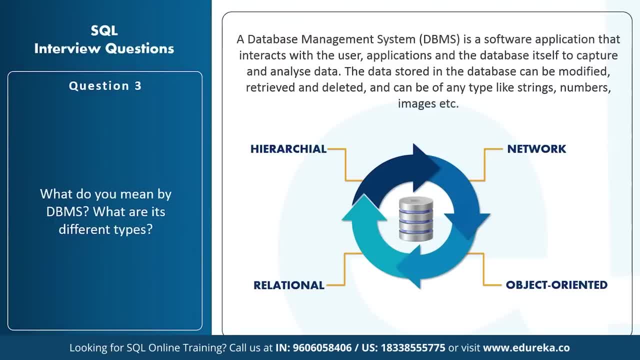 and the object-oriented database management systems uses small, individual softwares called objects, and each object contains a piece of data and the instructions for the actions to be done with the data. So I hope I'm clear with this point. So now, moving on to our next question, that is, what do you mean? 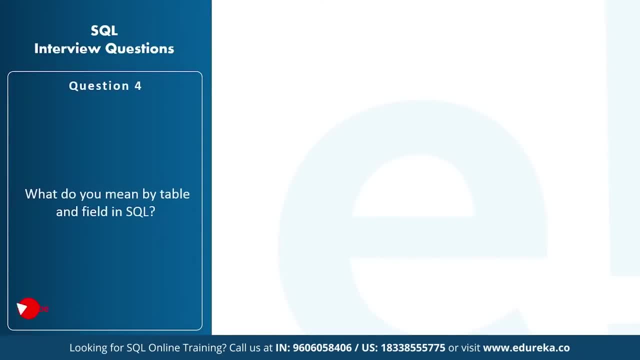 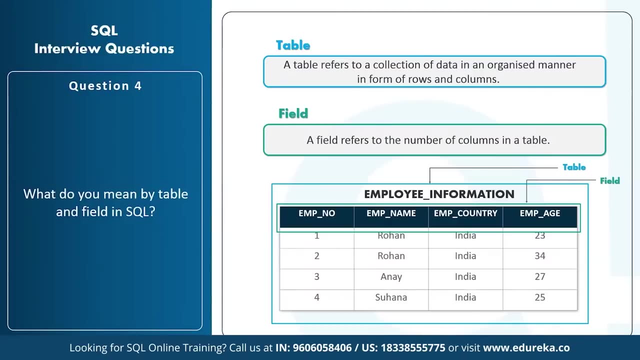 by a table and a field in sequel. So now, the answer to this question is quite simple. a table basically refers to a collection of data in an organized manner, in forms of rows and columns, and the field refers to the number of columns in the table. 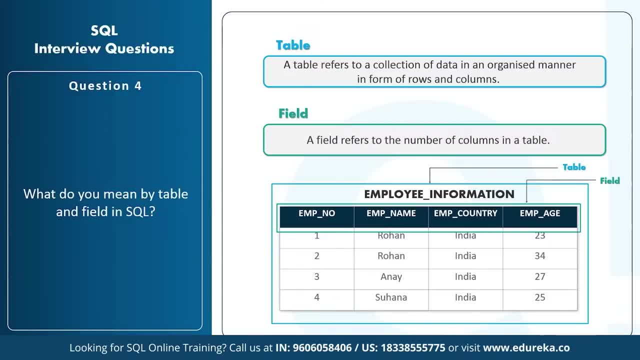 If you have to explain anybody what table and field mean. So basically, in sequel you have a database and a database consists of n number of tables, right? So that is basically a table and the tables have fields with a few column names, right? 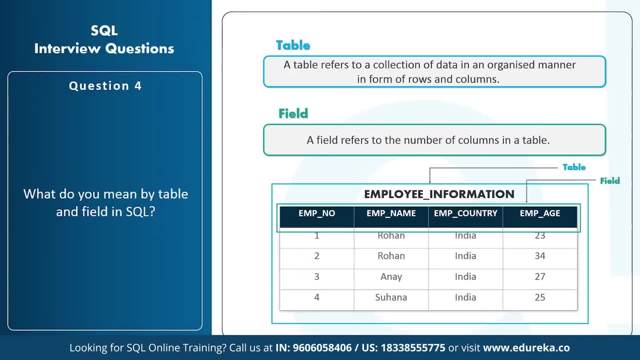 So the column names are basically the fields. so you can explain with an example, as you can see on the screen. So over here I have an employee information table into which the employee information table is a table, and the column names in this particular table are the fields. 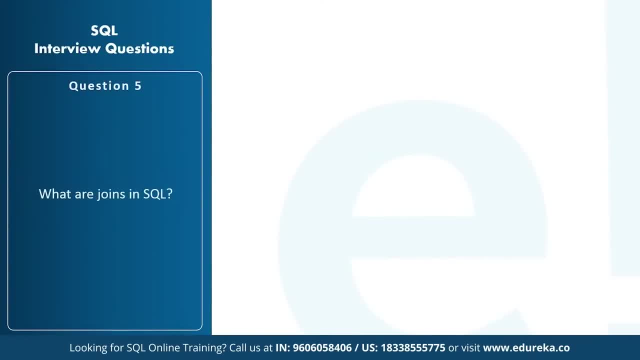 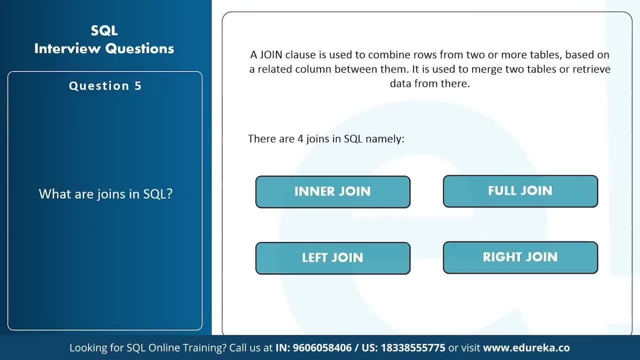 now moving on to our next question, That is, what are joints in sequel? Now, this is one of the most popular questions that is generally asked in your interviews. So, basically, a joint clause is used to define, to combine rows from two or more tables based on related columns between them. 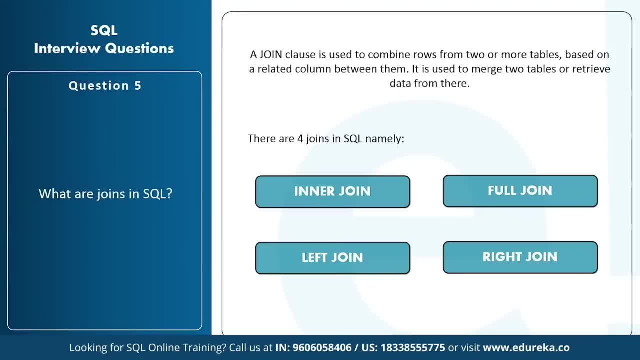 It is used to merge two tables or retrieve data from there, and there are mainly four types of joints in sequel, that is, the inner joint, the full joint, the left joint and the right joint. right now, moving on to our next question, That is, what is the difference between car? 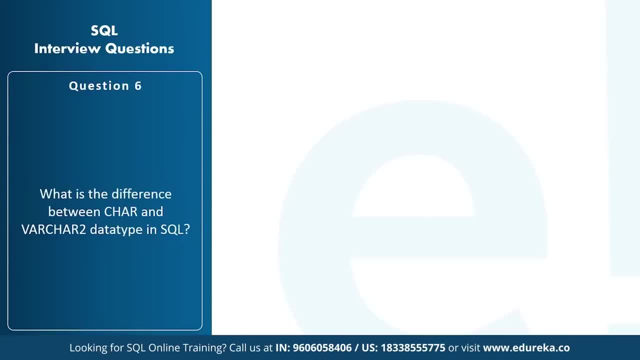 and varchar to data type in sequel. So this is one of the most confusing questions that is generally asked in your interviews you, since you know generally people get confused between what is care and what is varchar data type. now, both care and varchar to are used for character data type. 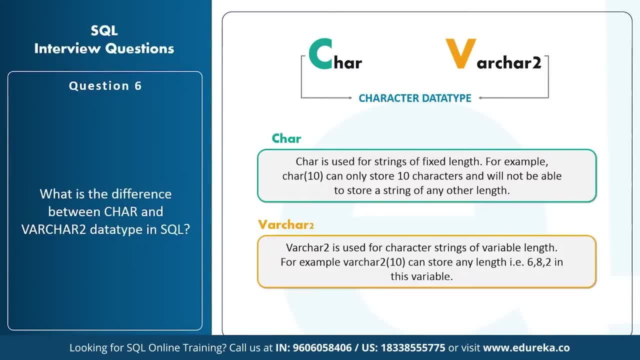 but varchar to is used for character string strings of variable length, Whereas the CAD is used for strings of fixed length. So whenever you have strings of fixed length, then you use the CAD data types, and whenever you have strings of variable length, then you can use the varchar to data type. 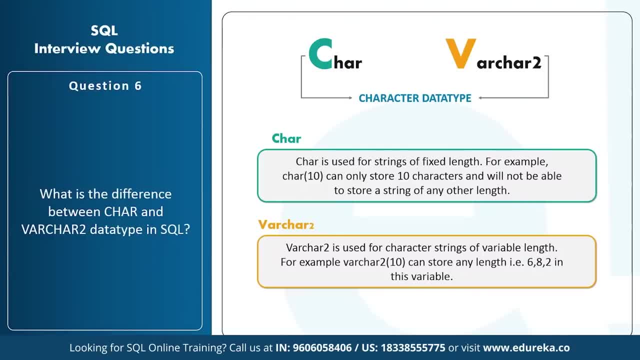 Now, for example, CAD 10 can only store 10 characters and will not be able to store a string of any other length, Whereas the varchar to 10 can store any length, that is, either 6 to 8. It completely depends on the variable right now moving. 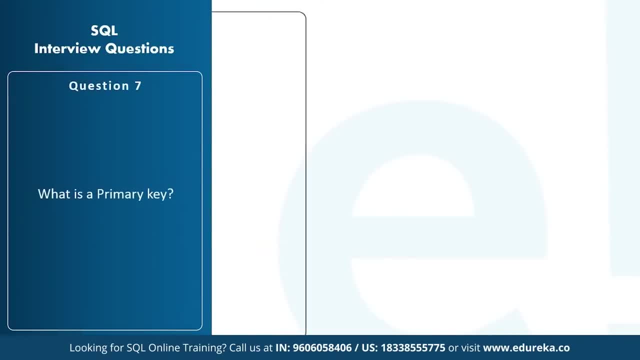 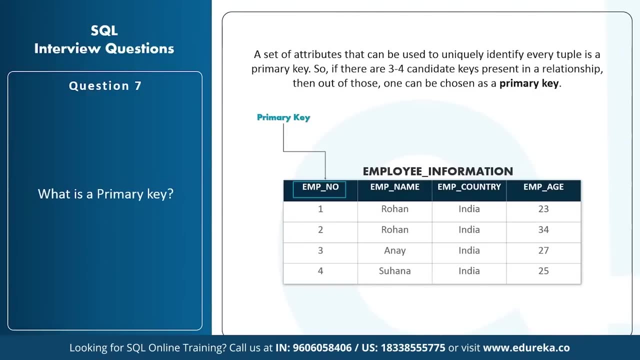 on to our next question. That is, what is the primary key now when you're working in the database field? obviously a company who can have n number of databases having n number of tables inside this. now each and every table in the database has to be connected. 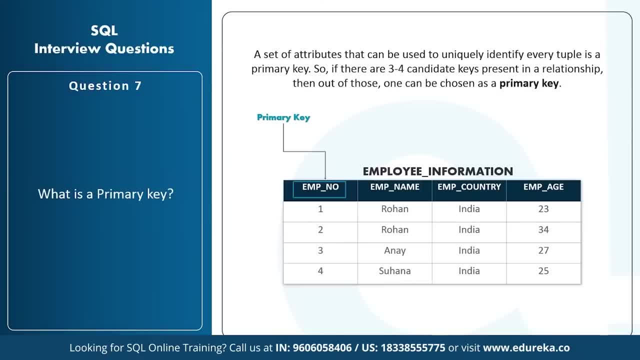 with the other table right now. for that We need to uniquely identify a table, or you know you can say you need to uniquely identify a column. So basically, primary key is a set of attributes that can be used to uniquely identify every tuple. So if there are around 3 to 4 candidate keys present, 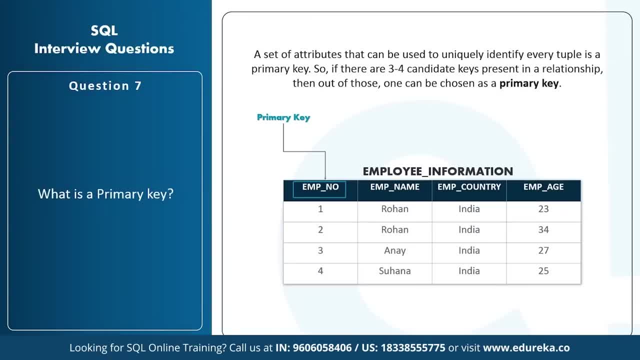 in a relationship, then out of those one can be chosen as the primary key. now, as you can see on the screen, We have an employee information table which has columns, like you know: employee number, employee name, employee country and the employee age. now obviously, you can uniquely identify. 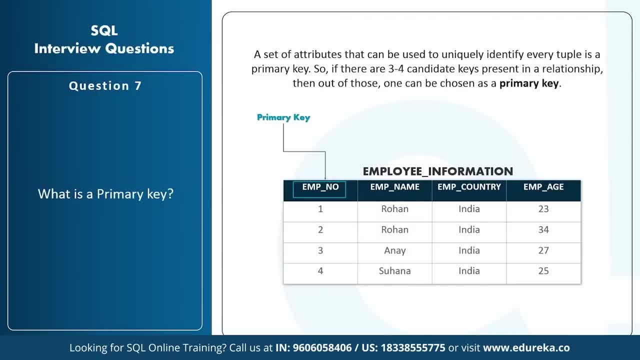 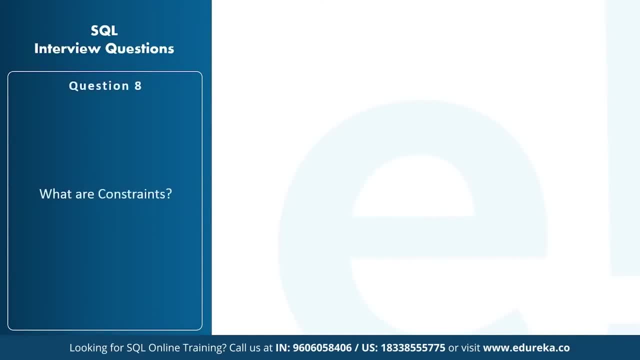 each and every employee with the employee ID right. So basically that will be a primary key. So we hear: employee number will be a primary key. Now let's move on to our next question, That is, what are constraints? so constraints are basically used. 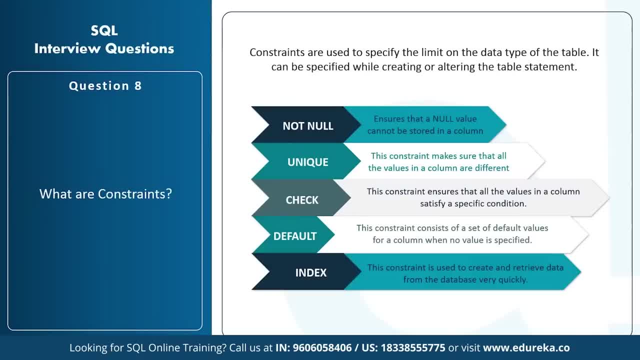 to specify the limit of the data type of the table, right. So whenever you're creating a table, then you can use the constraints to set a limit of the data type of the table. It can be either specified while either creating the table or, you know, while you're altering the table statements. 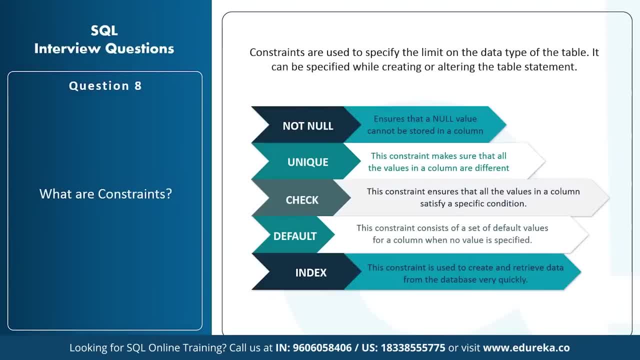 so it can be basically specified in both the ways. now There are mainly five constraints that you need to understand about. that is the not null constraint, the unique constant, the check constraint, the default constraint and the index constraint. that the not null constant, basically ensures that a null value cannot be stored in a column. 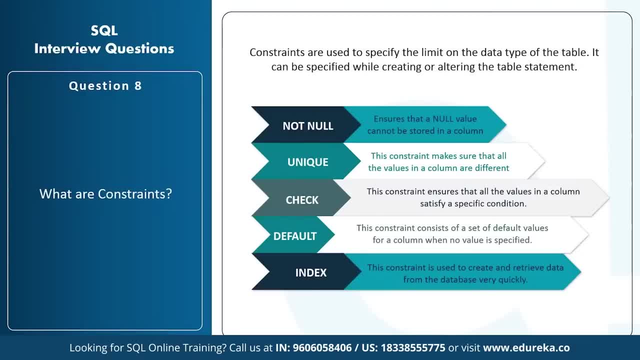 So, whenever you mention this particular constant into a column of your table, then this particular constraint will make sure that you know. no null value can be stored for that particular column in the table. Moving on to the next constant, that is, the unique constant, this constant, make sure that you know. 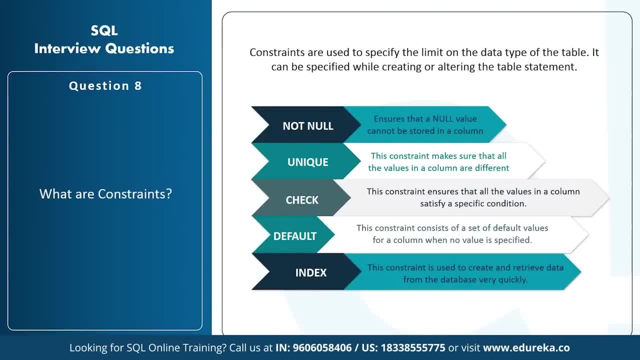 all the values in the column are basically different. So if you need to make sure that you know in a column you have unique values for each and every row, then you can use this particular constraint. now moving on to the next constant, that is, the check constraint. 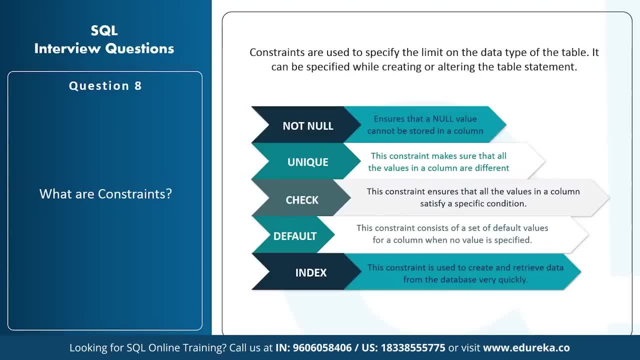 the check constant basically ensures that all the values in the column satisfy specific condition. So if you have a condition, you need to make sure that you know only the values that satisfy the condition are stored in the column. Then you can use this particular constraint. now talking, 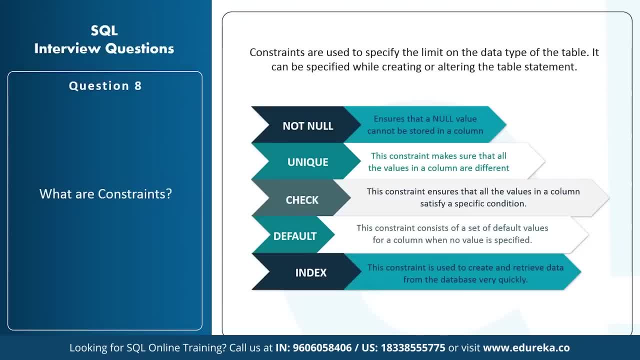 about the default constraint. default constant consists of a set of default values for a column but no value specified. So, for example, in the table of 10 rows, you know you have a column in which you do not specify all the values for all the 10 rows. 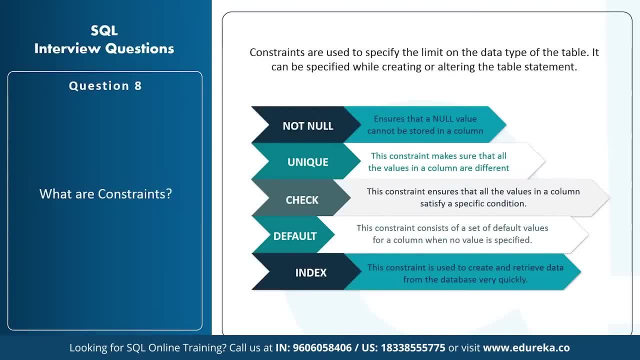 Then you can make sure that you know you have set the default value, and the default value will be automatically stored whenever you don't mention a value in that call. Now, moving on to the last type of constraint, that is, the index constraint- the index- 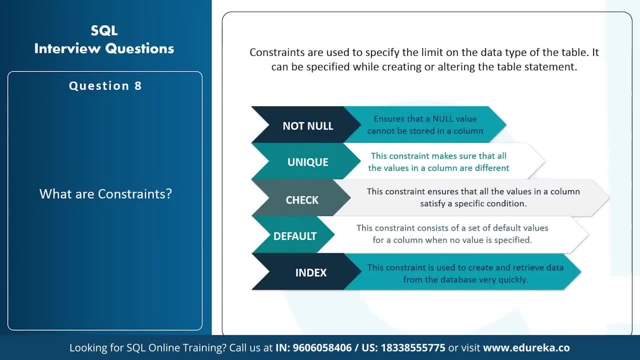 Constraint is used to create and retrieve data from the databases very quickly. So I hope I'm clear with the different types of constraints that you need to answer about when you're asked this question about what are the constraints that you know? now let's move on to the next question. 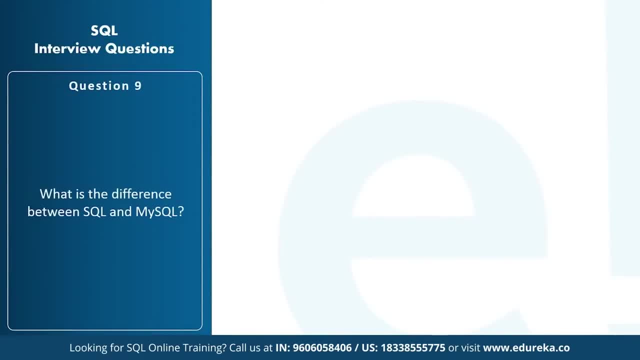 That is, what is the difference between sequel and my sequel? now, this is one of the most popular questions that is generally asked, you know, because since people generally get confused between what is sequel and what is my sequel. So let me just explain you the simple difference. 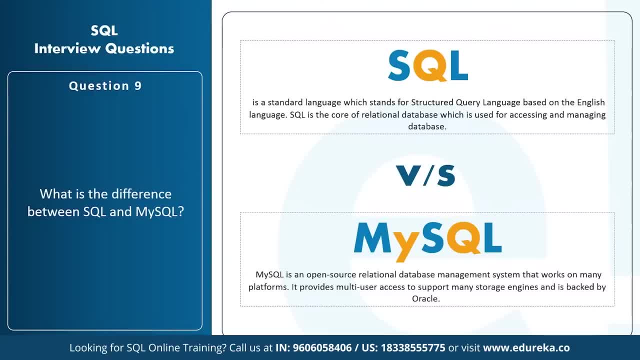 between both of them. So sequel is basically a standard language which stands for structured query language based on the English language, Whereas the my sequel is a database management system. So sequel is basically the core of relational database which is used for accessing and managing the database. 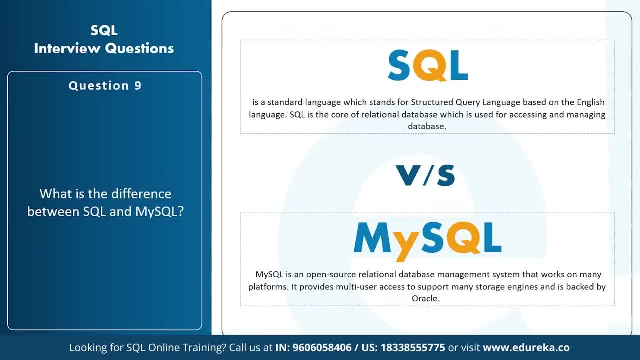 Whereas my sequel is a relational database management system which works on many platforms. So basically, this provides multi-user access to support many storage engines and is backed by Oracle. So that's the basic difference between sequel and my sequel, guys. Sequel is basically the core of relational database. 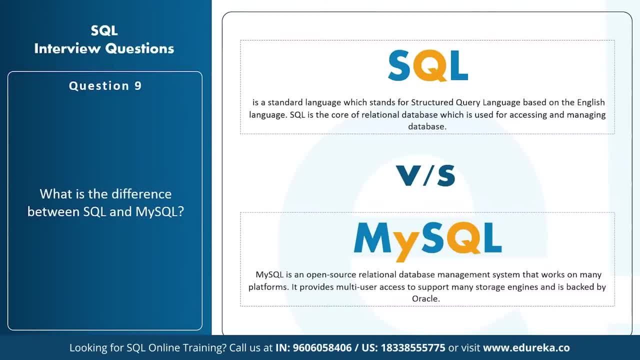 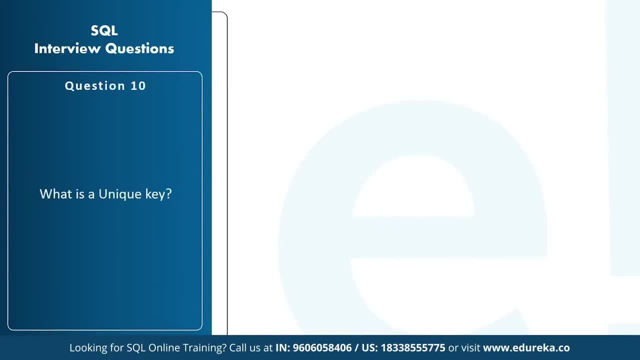 which is used for accessing and managing the database, and my sequel is an open-source relational database management system. Now let's move forward to our next question, That is, what is a unique key now? unique key basically identifies a single row in a table. 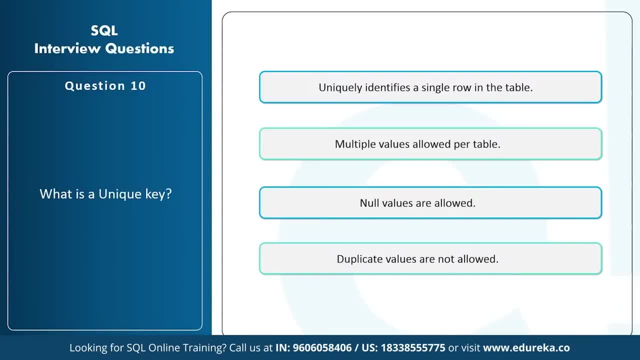 This basically allows multiple values per table and also the null values are allowed. So you'll have to make sure that you know whenever you're using the unique key. you need to have an idea that you know it identifies a single row in the table. multiple values are allowed. 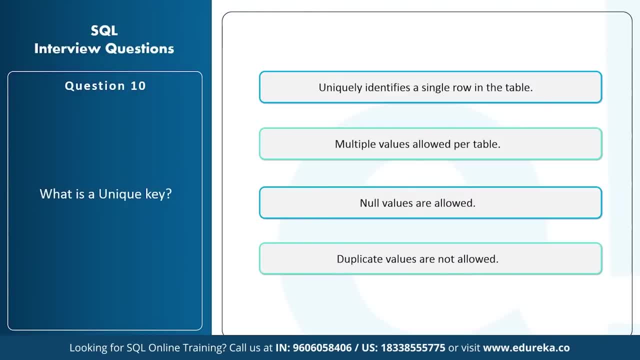 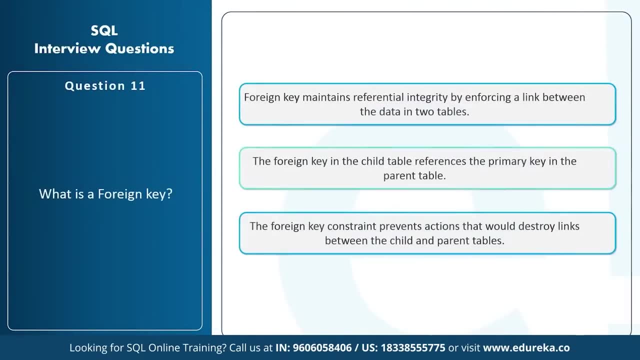 for the table, and also, null values are allowed, but, yes, duplicate values are not allowed. All right now moving forward to a next question, That is, what is a foreign key? a foreign key basically maintains referential Integrity by enforcing a link between the data in two tables. the foreign key- 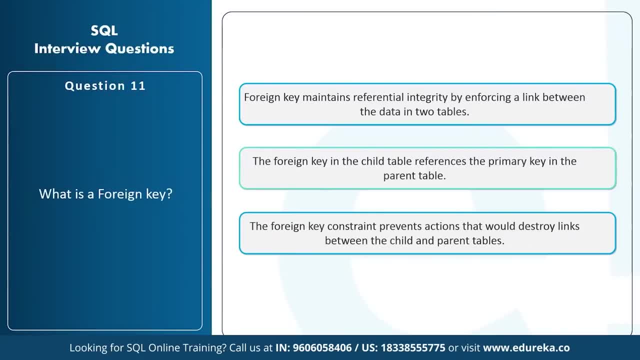 in the child table references the primary key in the parent table and the foreign key constraint prevents actions that would destroy the links between the child and the parent table. So if you have a database and you know if you have around 10 tables in that particular database, 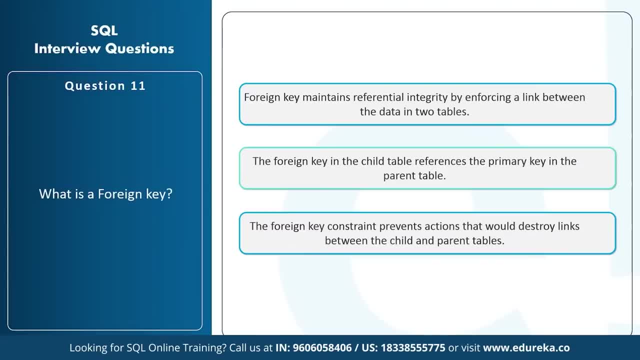 and then, if you want to maintain relations between all these tables in the database, then you need to use the primary key- foreign key concept, so that you identify the relation between both these tables with the help of foreign key. now moving forward to a next question, 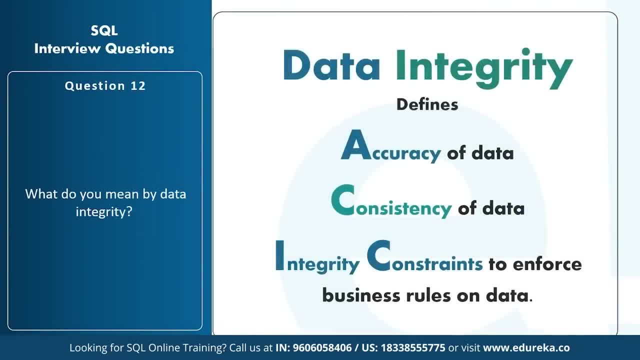 That is what do you mean by data Integrity. now, data Integrity basically defines the accuracy of the data, as well as the consistency of data stored in the database. It also defines the Integrity constraints to enforce business rules on the data when it is entered into an application or a database. 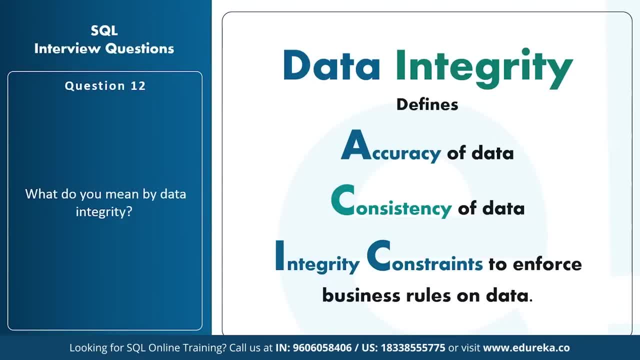 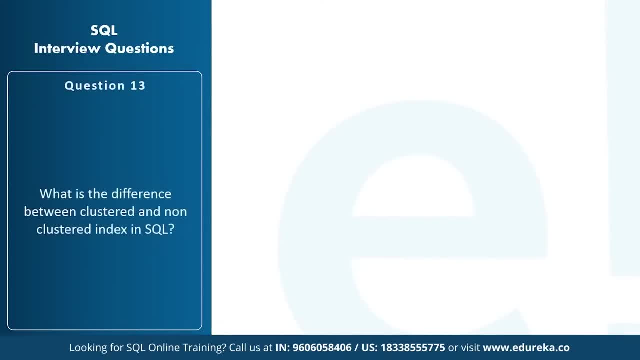 So if you have to answer this question, then you can answer by saying that you know. data Integrity basically defines the accuracy and the consistency of data. Now let's move forward to a next question, That is, what is the difference between the clustered and the non-clustered index in sequel? 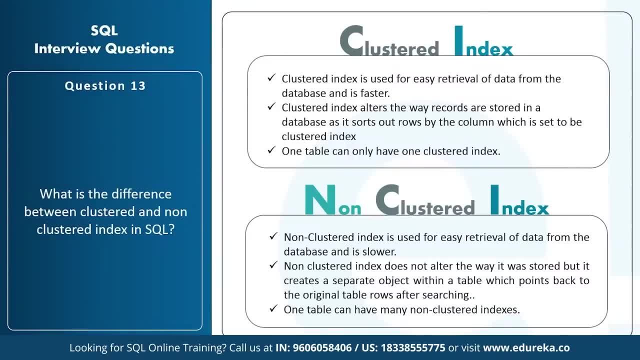 The clustered index is basically used for the easy retrieval of the data from the database and is faster than the non-clustered index. The clustered index alters the way records are stored in the database as it sorts out the rows by column, which is set to be the clustered index. 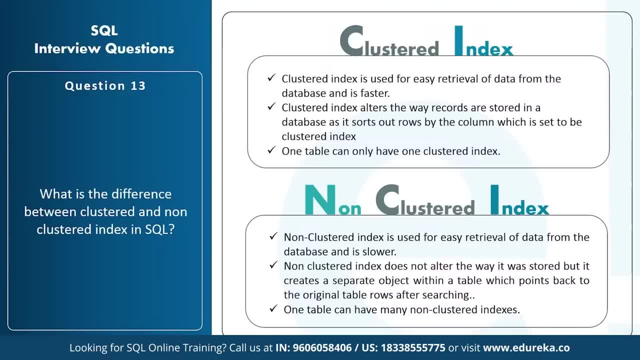 and only one table can have a clustered index coming to the non-clustered index. The non-clustered index is also used for the retrieval of data from the database, But, yes, it is slower than the clustered index. The non-clustered index does not alter the way it is stored. 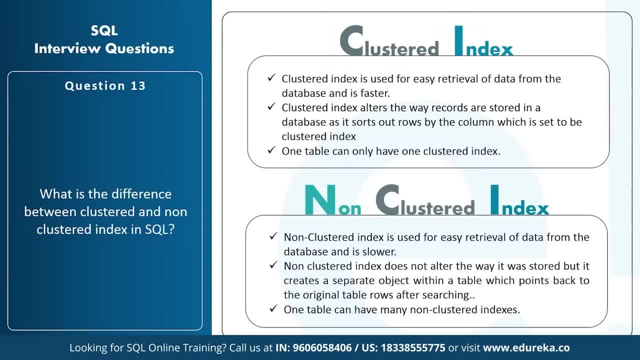 But yet it creates a separate object within a table which points back to the original table rows after searching, and also one table can have many non-clustered indexes. The main difference between both of them are: both are used for easy retrieval of data, But, yes, the clustered index is faster. 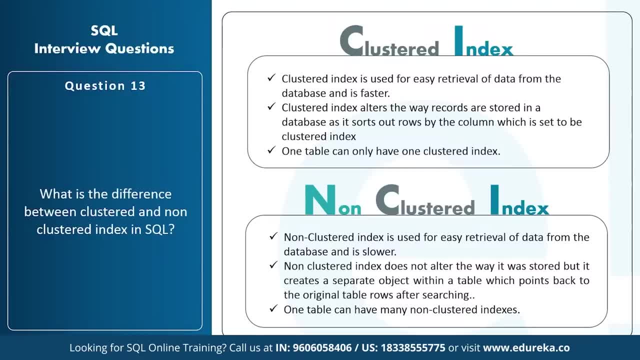 than the non-clustered index, and only one table can have only one clustered index. But yes, a single table can have many non-clustered indexes. Apart from that, the third difference between both of them is also that, you know, the clustered index alters the way records are stored. 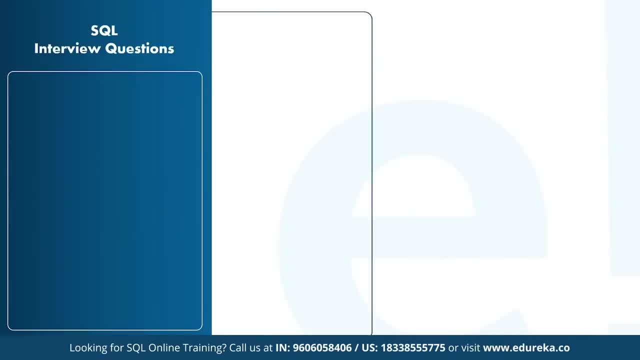 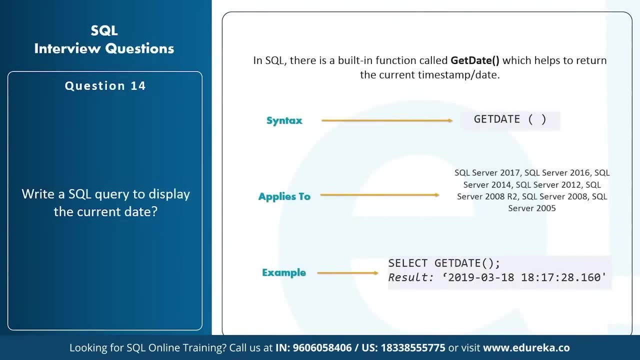 in the table, and the non-clustered index does not do that. Now let's move forward to our next question, that is, write a sequel query to display the current day. Now, when you attend the interviews for a database administrator, let me just tell you that not only the theoretical questions, 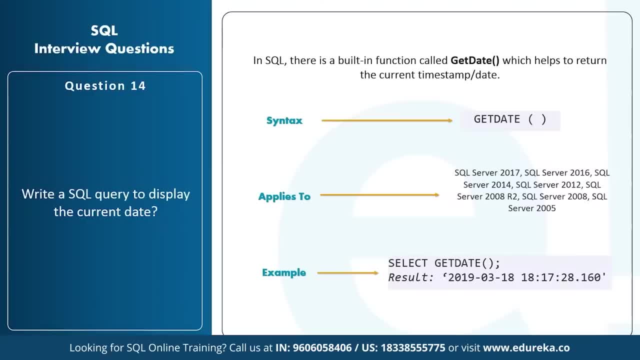 are asked. but, yes, you're sometimes asked to write the queries also so they can give you some scenario based questions or they can just ask you few simple queries that you need to make sure that you know. you know that, so that's the reason that this question could be asked: that you know. 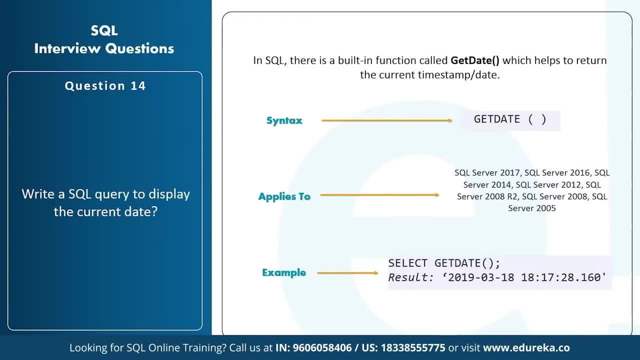 write a sequel query to display the current date. Now in sequel, to display the current date, We have a function known as the get date. So basically, with the help of this function you can return the current date and time stamp. So the syntax of the function is really simple, is just get date. 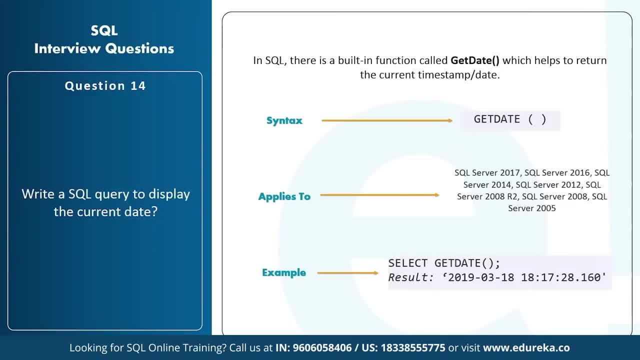 and it applies to sequel server 2017, 16, 14, 12, 2008, R2 2008 and 2005.. If you just have to give an example to the interviewer about how to write a query to display the current date: 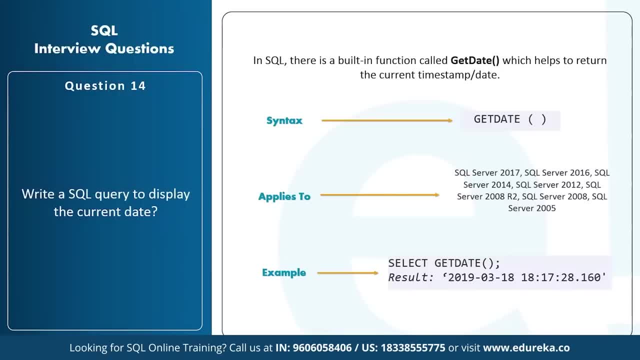 you can just mention the query. like you know, select get date. So when you execute this particular query, you would see an output that you know the current date and time would be displayed as out. right? So that's how you can write a query to display the current date. 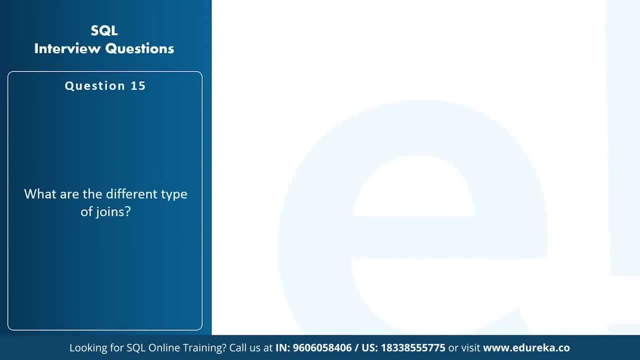 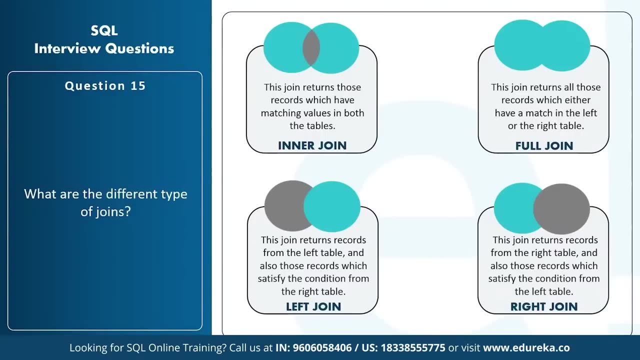 Now moving forward to the next question, that is, what are the different types of joints? So, as I mentioned before, there are mainly four types of joints that you need to talk about. that is, the inner joint, the full join, the left join and the right joint. 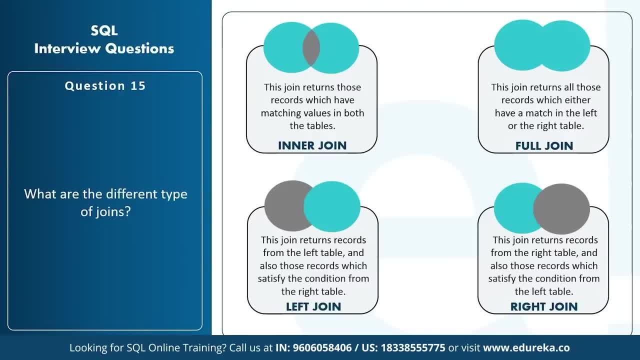 So, talking about the inner joint, this joint basically returns those records which have matching values in both tables. now consider two tables, table a and table B. Now, when you apply the inner join on board of these tables, you will observe that you know, the output would be all those. 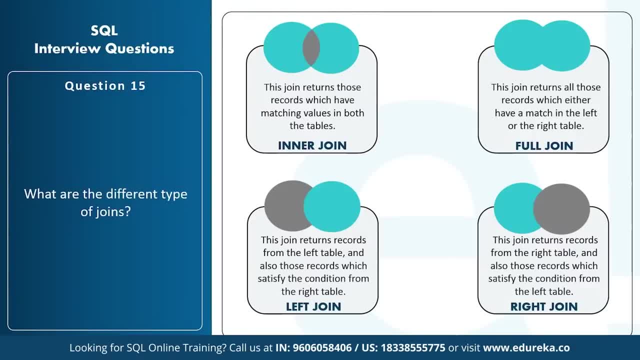 records which have matching values in both the tables, that is, table a and table B. We're talking about the full joint. The full joint basically returns all those records which either have a matching value in the left or the right table. So whenever you apply full join on both of these tables, 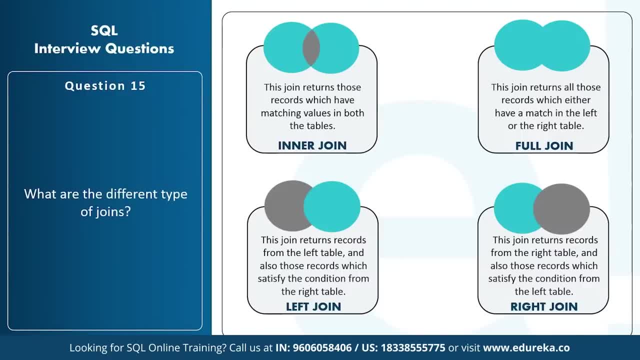 you'll see that. you know you'll get an output of all those records which either have a match in the left or the right table. now, talking about the left join, the left join returns the records from the left table and also those records which satisfy the condition from the right table. 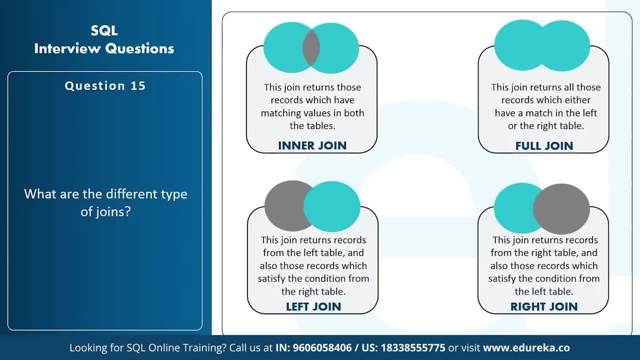 So if you have table a and table B and you apply a left joint to both of these tables, then the output would be all those records from the left table and the records from the right table which satisfy the specified condition. Similarly, the right joint is just the vice versa. 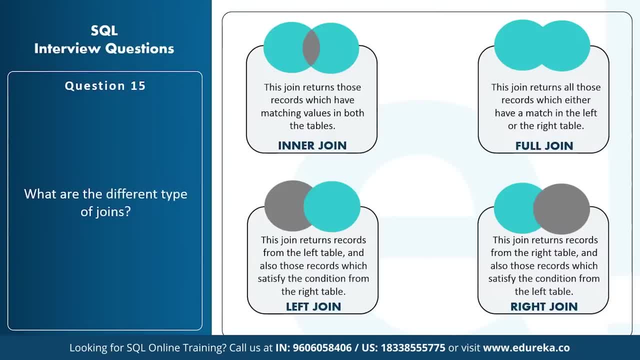 The right joint basically returns the records from the right table and also those records which satisfy the condition from the left table. So whenever you apply the right joint to table a and table B and consider that you know the table B is right table, You'll get all those records from the table P. 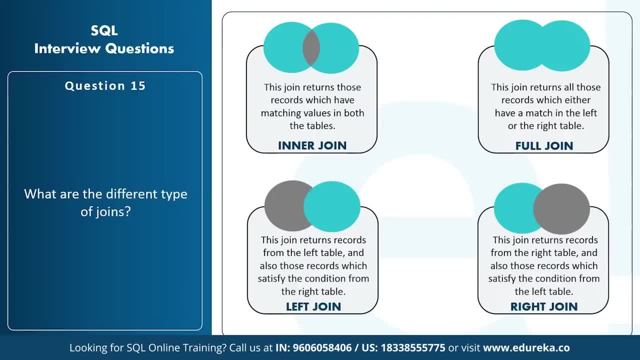 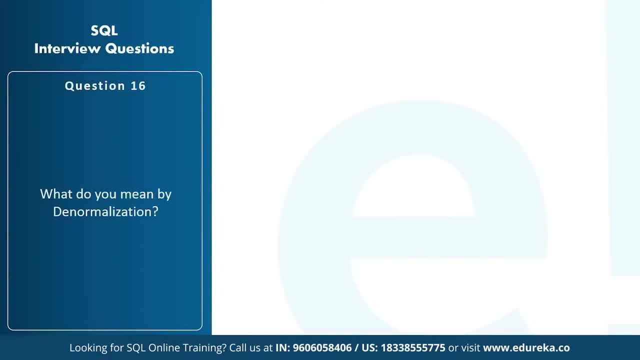 and also matching records from table a which satisfy the condition. So these are the various types of joints that you need to talk about, guys. now moving forward to the next question, That is, what do you mean by denormalization? now, denormalization basically refers to a technique. 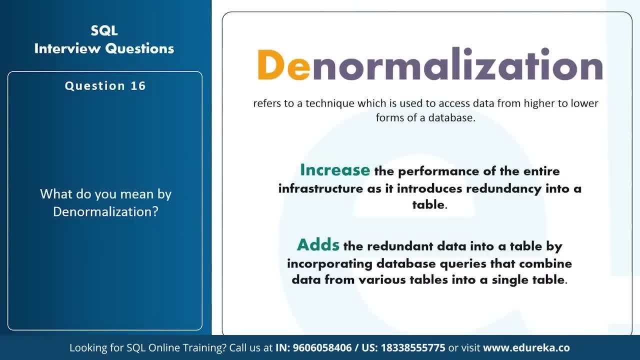 which is used to access the data from higher to lower forms of database. It increases the performance of the entire infrastructure as it introduces redundancy into the table, and it also adds the redundant data into a table by incorporating database queries that combine data from various tables in a single table. 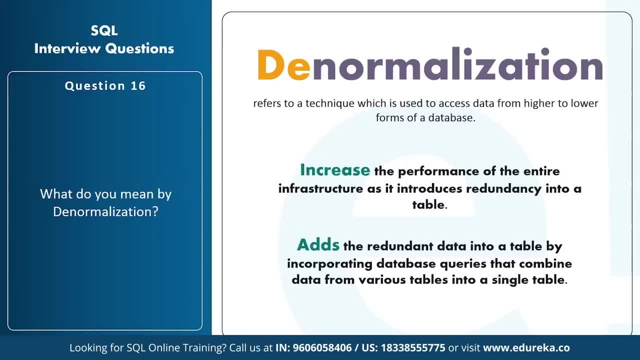 So if you have to just explain denormalization, you can just say that you know it is a technique which is used to access data from higher to lower forms of database, and it basically adds redundant data into the table by incorporating database queries that combine data from various tables. 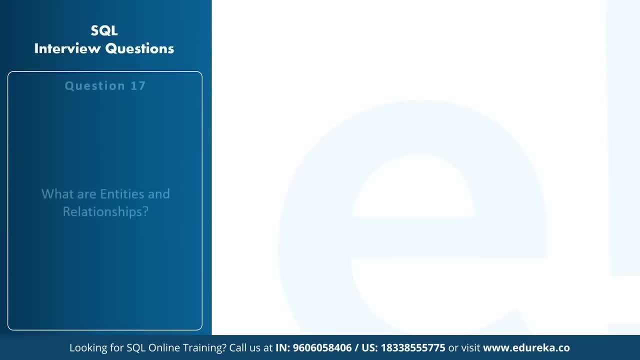 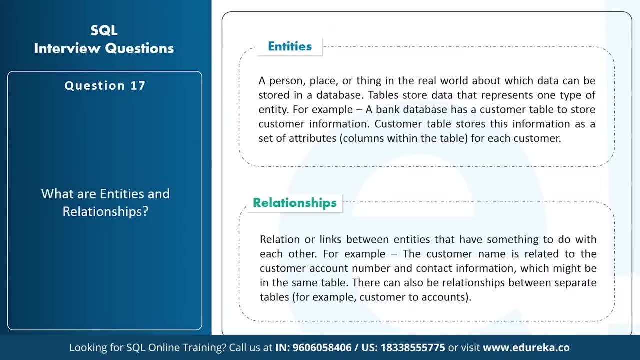 So I hope I'm clear with this point. now moving forward To the next question, That is, what are the entities and relationships? So let me just explain you what entities are first. So entities can be anything like in a person, place or a thing in real world about which data can be stored. 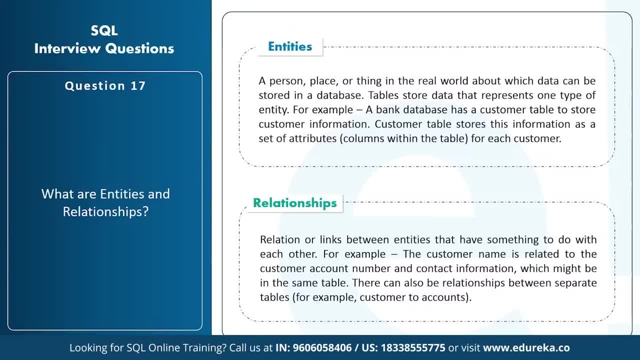 in a database, So table stored data that represent one type of entity. So, for example, a blank database has a customer tables to store the customer information. Now the customer table stores this information as a set of attributes, that is basically the columns within the table for each and every customer. 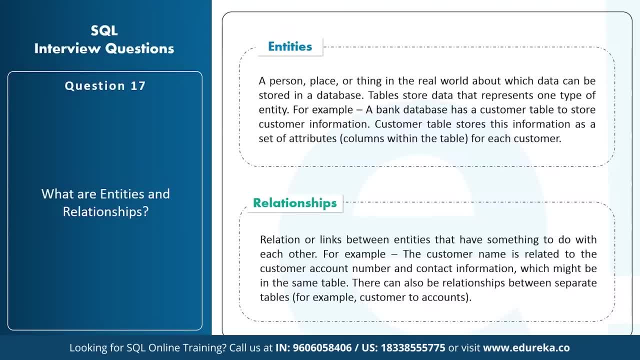 So if you consider, you know a customer table has around five parameters like customer ID, customer name, customer phone number, customer email ID and so on, then all these customer ID, customer name, customer phone number are basically the column names, that is, the attributes for the entities. 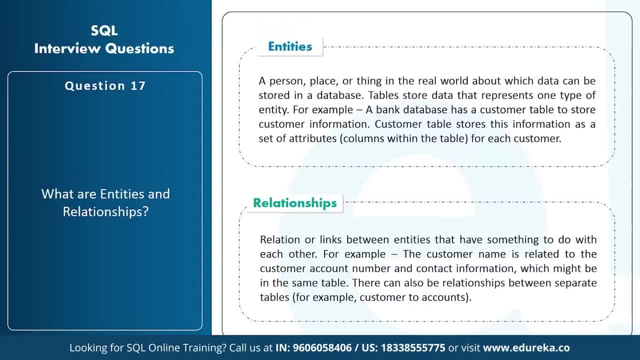 and customer information will be the entity. the talking about relationships, relational links between the entities that have something to do with each other, is basically relationships. So, for example, the customer name is related to the customer account number and the contact information. right now this might be in the same table. 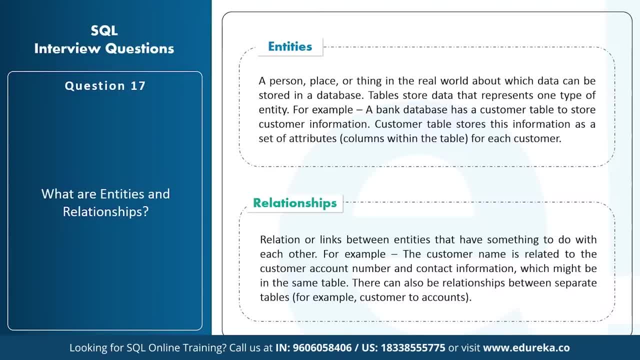 or it could be in any other table Also, right? So if you have two tables, out of which one table has the customer name and the other table has all the other information, like the customer ID, customer name and so on, now these two tables will be related to each other. 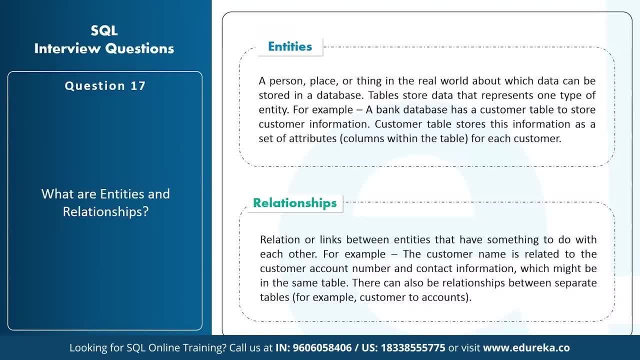 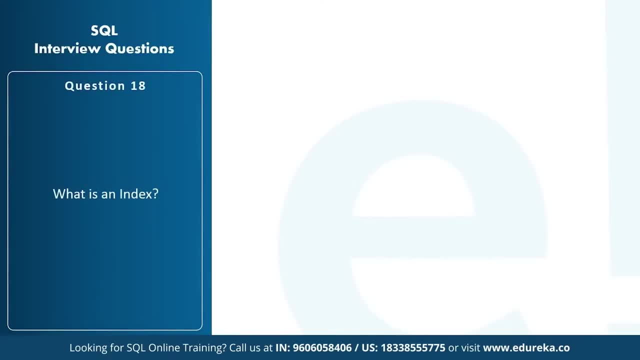 with the relationship so that the customer details could be retrieved. Now that particular information is basically relationships. now moving forward to our next question, That is, what is an index? in the previous questions I talked about the non-clustered index and the cluster indexes, right? 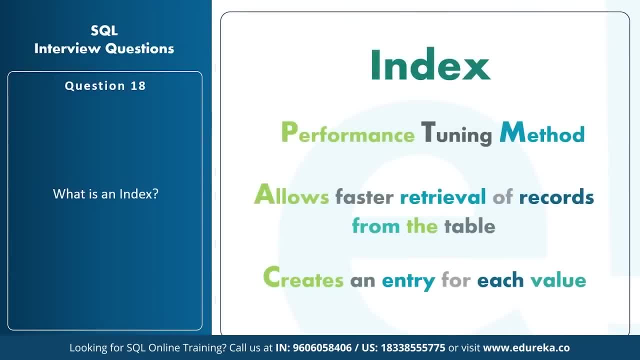 But what exactly is index now? index basically refers to a performance tuning method of allowing faster retrieval of records from the table. So, as I mentioned before in the clustered and the non-clustered indexes question, both of the indexes are basically used for easy retrieval of data, right? 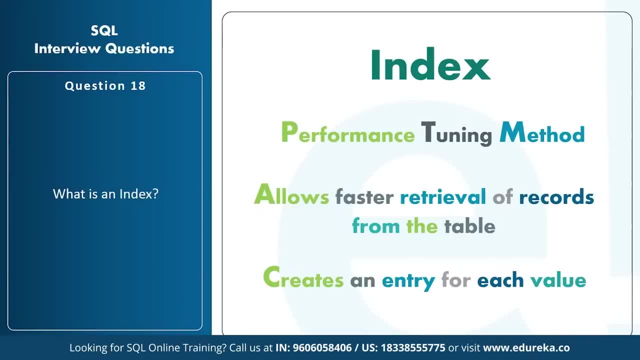 So that's what an index does. This is basically a performance tuning method to allow faster retrieval of data from the table, and also an index creates an entry for each value. So to allow the faster retrieval of records from the table, It basically creates an entry for each and every value. 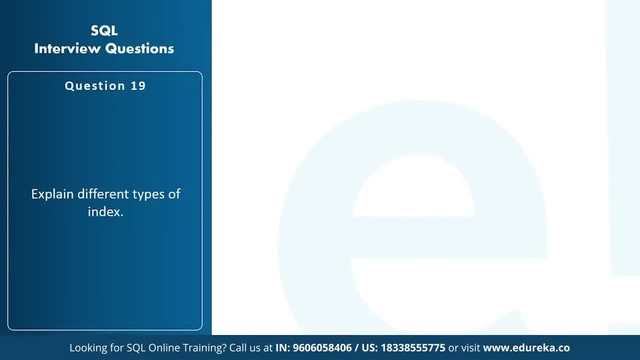 Now let's move forward to the different types of indexes. So well, I've already explained you about two types of indexes, that is, the clustered and the non-clustered index. But yes, let's understand again about both of them. and also an additional index, that is the unique index. 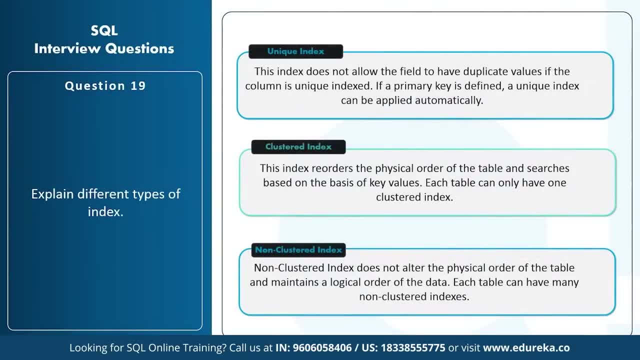 So mainly there are three types of indexes that is used, that is, the unique index, the clustered index and the non-clustered index. the unique index basically does not allow the field to have duplicate values if the column is unique indexed. So if a primary key is defined, a unique index. 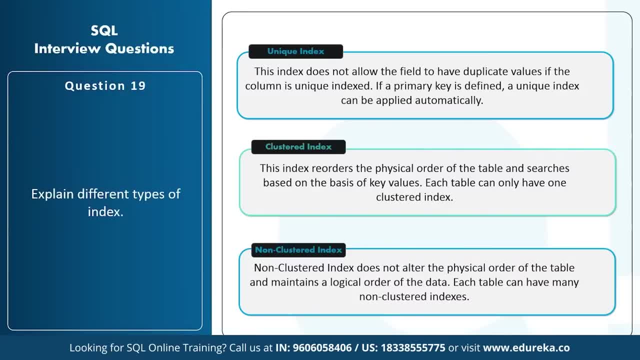 can be applied automatically. So unique index is mainly used because when you do not want any duplicate values to be present in the column. now, moving to the clustered index. the clustered index basically reorders the physical order of the table and searches based on the basis of key values. 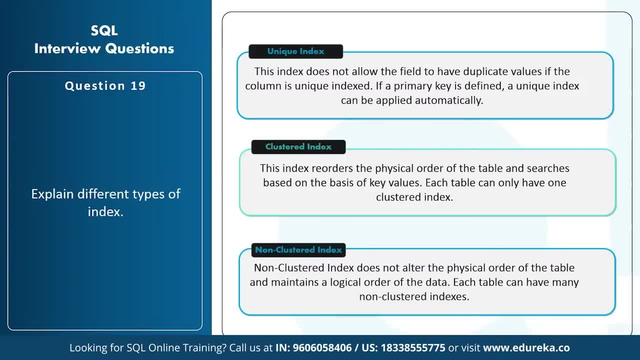 So each table can have only one clustered index. coming to the third type of index, that is, the non-clustered index to non-clustered index does not alter the physical order of the table and maintains a logical order of the data. So each table can have many non-clustered indexes, right? 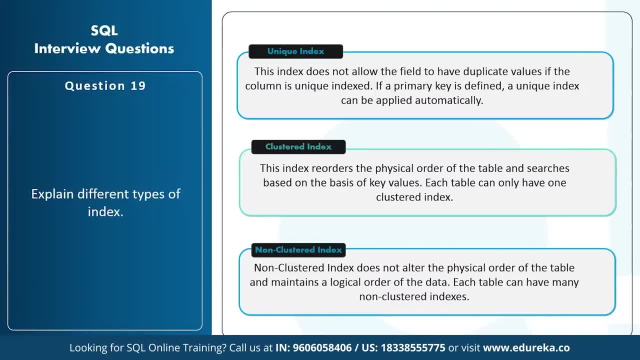 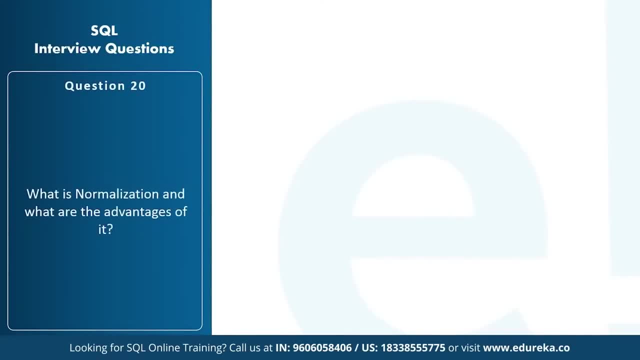 So basically, guys, there are three types of indexes that you need to explain about. that is, the unique, the cluster and the non-clustered index. now moving forward to our next question, that is, what is normalization and what are its advantages? So normalization is basically the process of organizing data. 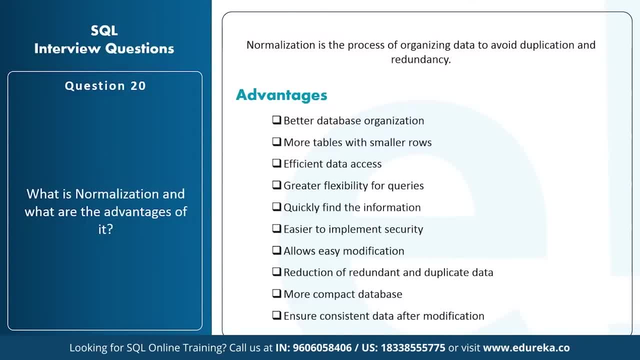 to avoid duplication and redundancy. So it's basically the opposite of denormalization that we just talked about in one of the previous questions. So if you just have to define normalization then you can see that unit is a process of organizing data to avoid duplication and redundancy. 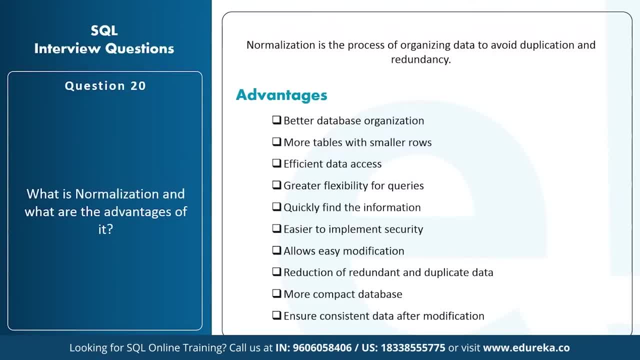 Now. the advantages of normalization are as you can see on the screen. It offers better database organization, more tables with smaller rows. efficient data access. greater flexibility for queries quickly finds the information easier to implement. security allows easy modification. reduction of redundant data and duplicate data. more compact database. 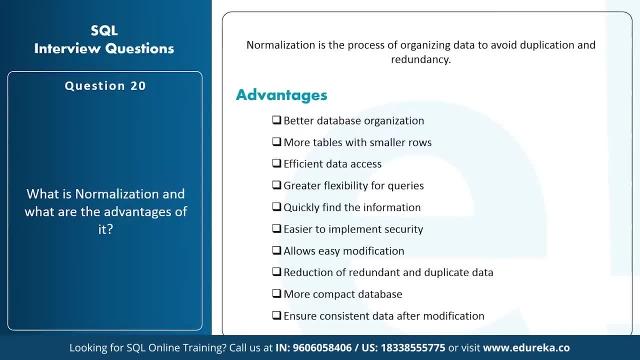 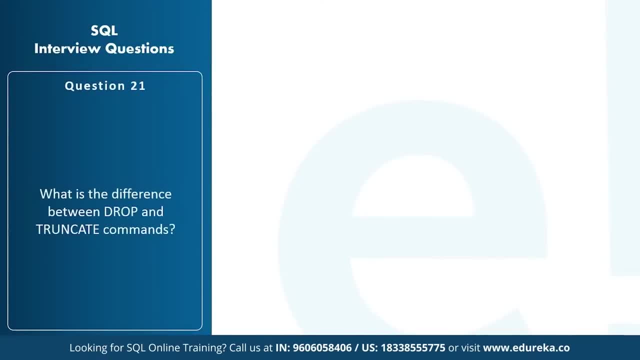 and ensures consistent data after modification. So, guys, these are few advantages of normalization. now let's move forward to our next question, That is, what is the difference between the drop and the truncate commands? The drop command basically removes the table and it cannot be rolled back from the database. 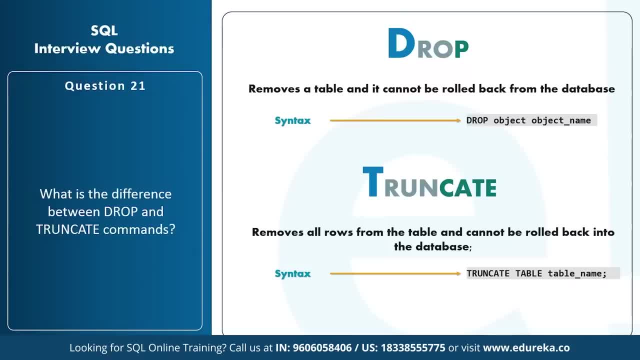 Whenever you use the drop command, just remember that you know you completely drop the complete table and it cannot be rolled back from the database. and the truncate command removes all the rows from the table and also cannot be rolled back into the database. So the drop command. 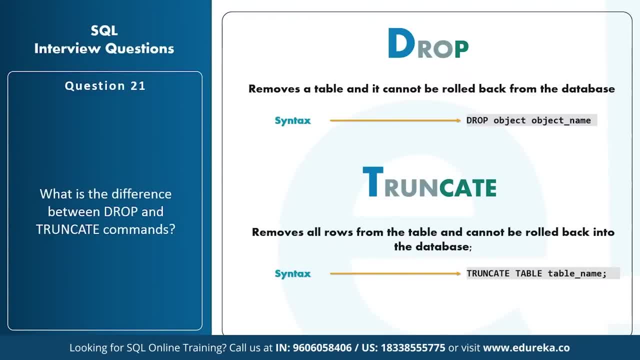 and the truncate command differ by this. So whenever you use the drop command, you drop the complete table, and whenever you will use the truncate command, you will remove all the rows from the table. The syntax of both the commands are almost same. The syntax of drop command is basically drop object. 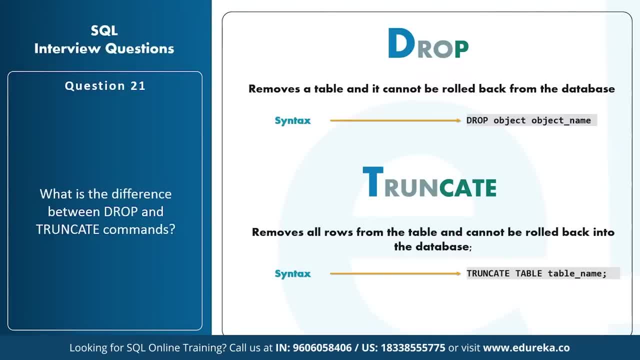 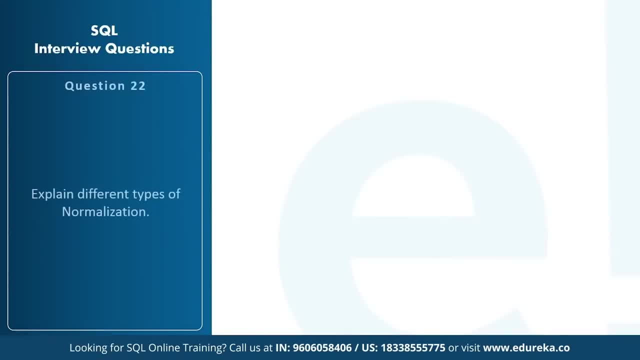 and object name. that is basically the table and table name, and the syntax for truncate command is truncate table and table name. So, guys, that was about the drop and the truncate command. Now let's move forward to the next question, That is, what are the different types of normalization? 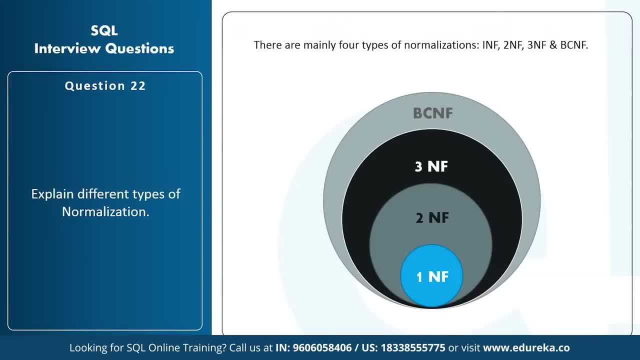 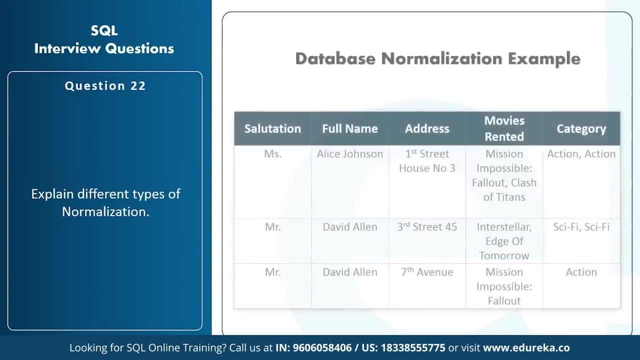 So there are mainly four types of normalizations, that is, 1NF, 2NF, 3NF and BCNF. Now let me explain you the different types of normalization with an example. So, guys, this is the table that we're going to consider for the example. 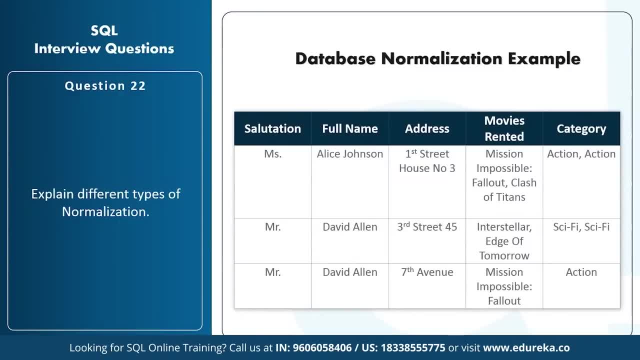 Now you basically have to apply normalization to this particular table. now, to apply normalization to this particular table, You'll clearly observe that you know there is Alice Johnson who has a particular address and has rented few movies from a specific category, and the category action is mentioned twice over here. 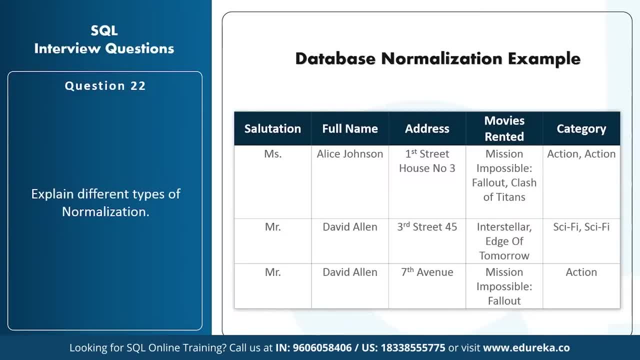 Similarly, David Allen's address has been divided into two different record and the movies rented and the categories have also been divided into two different records. right now, to apply normalization to this particular table, You first have to apply the 1NF. that is the first one. 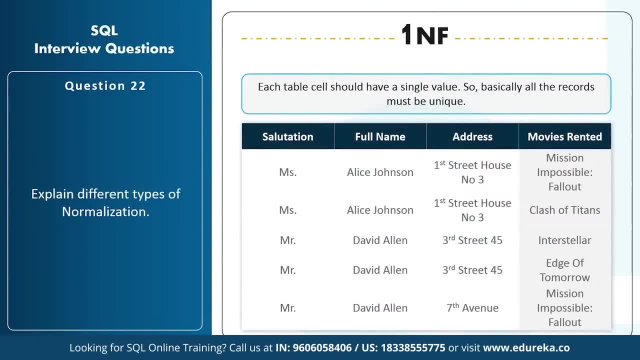 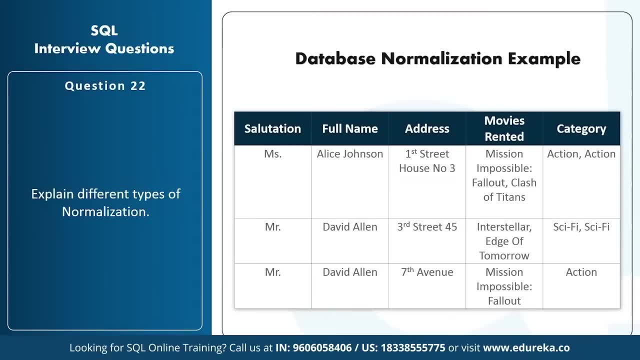 First normalized form. So for a table to be in 1NF you need to make sure that each table cell should have a single value. So basically all the records must be unique. So as you saw, in this particular table we had redundant values in the same record right. 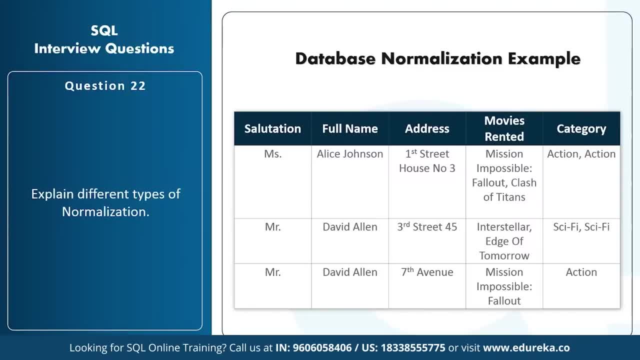 So we're going to have each cell with a unique record. So we'll have record such as you know, Miss Alice Johnson, first Street House, number three, Mission Impossible, and the second record as Miss Alice Johnson, first Street House, number three, Clash of Titans. Similarly will have Mr. 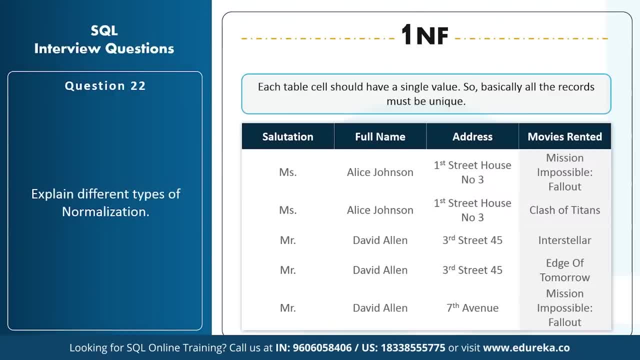 David Allen, Third Street 45 with Interstellar, the Mr David Allen third Street 45 with Edge of Tomorrow, and similarly Mr David Allen seventh, and your Mission Impossible fallout. So that's how, basically, you get your table into 1NF. 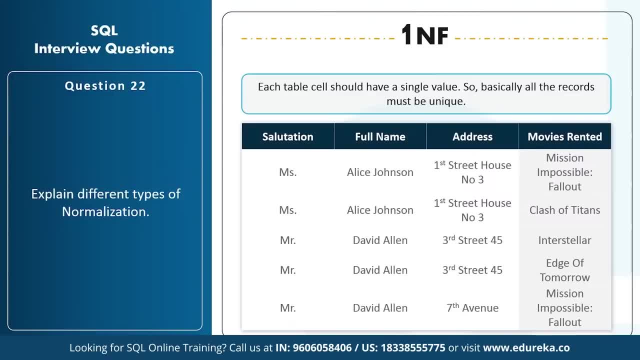 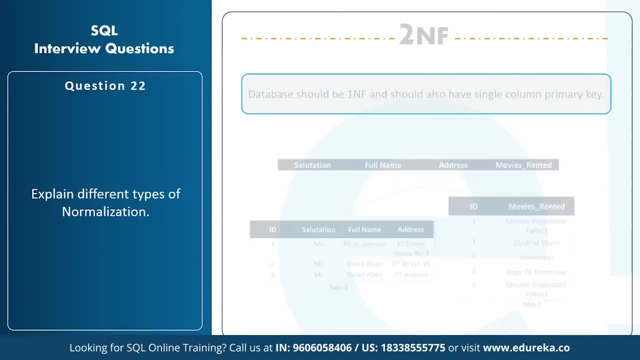 You have records with unique value in the complete table. Now, as you can see on the screen, this is a table for 1NF. Now you have to divide this table to 2NF. So when I say 2NF, that is the second normalized form. 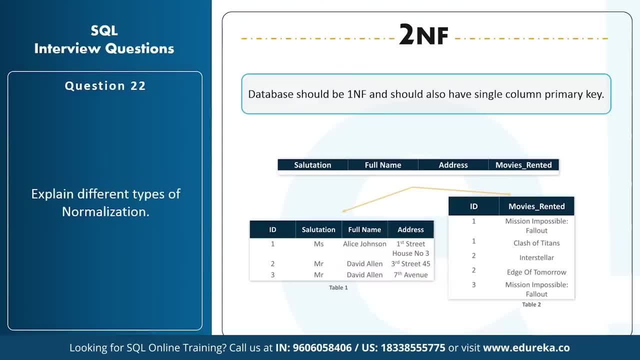 you can divide this table into two different tables. So to have a table in 2NF you need to make sure that you know the database should be in 1NF and should also have a single column primary key, since the table is in 1NF that we considered. 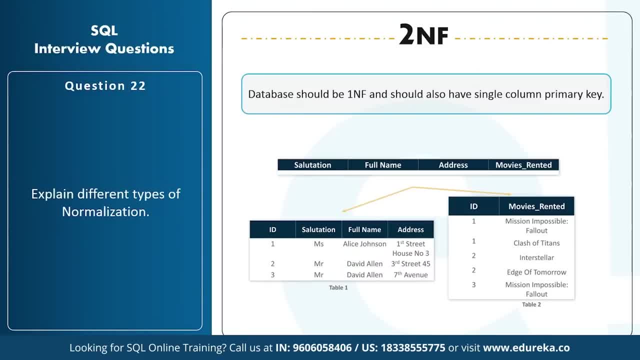 that's applicable to our situation. Now let's move forward to the 2NF. now in the 2NF You'll clearly see that you know we have salutations, full name address and movies rented. right now to divide this table into two different tables. 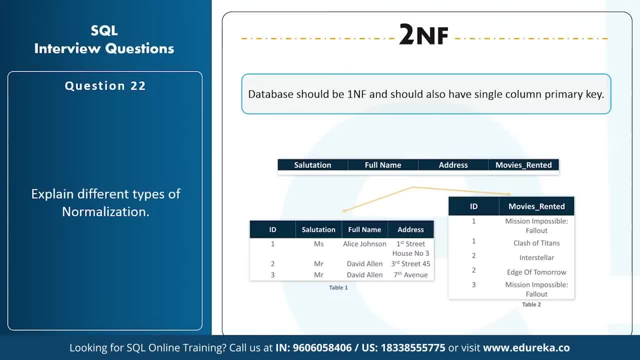 You can clearly see that. you know I've added an ID to both the tables. So I've added ID salutation, full name and address and ID movies rented. So Miss Alice Johnson, staying in First Street House number three, must have rented Mission Impossible. 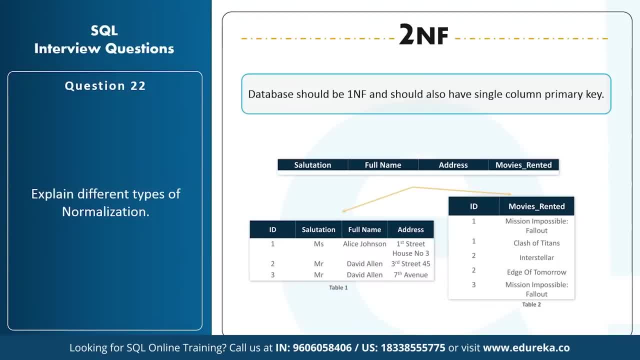 Similarly She must have rented Clash of Titans. Mr David Allen saying in third Street 45 has rented Interstellar and Edge of Tomorrow, and Mr David Allen staying in Seventh Avenue has rented Mission Impossible Fallout. So that's how I've divided the table into 2NF. 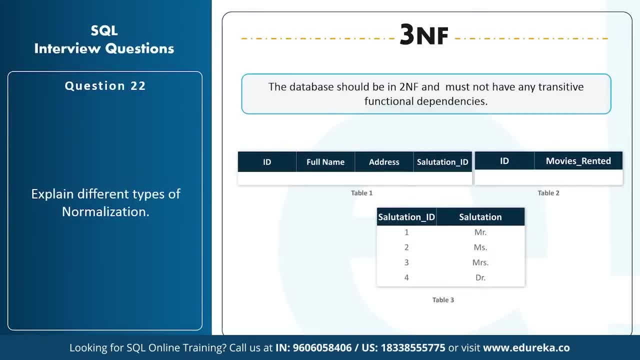 Now moving forward to 3NF. now a database to be in 3NF, You need to make sure that you know your database is first in 2NF and must not have any transitive functional dependency. So for that, what you're going to do is you're going. 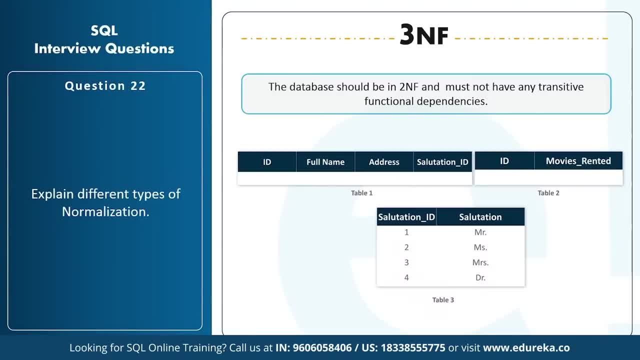 to further divide the two tables into three tables, as you can see in the screen. So we're going to have an ID, full name address and salutation ID, and also another table with ID, movies, rented column attributes and the third table with salutation ID and salutation. 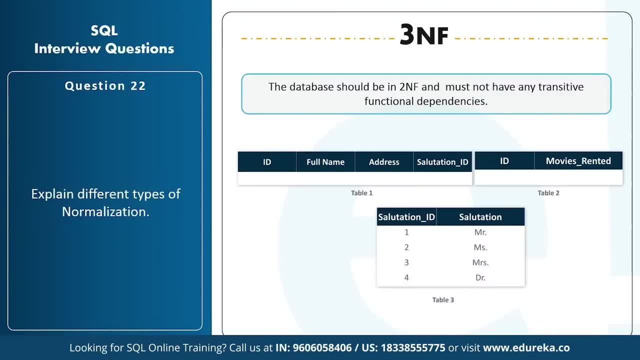 So, basically, we're going to identify Mr with one, Miss with two, Mrs with three and doctor with four. So that's how we're going to get our tables to 3NF. Well, guys, with this we come to an end of this particular example that you know. 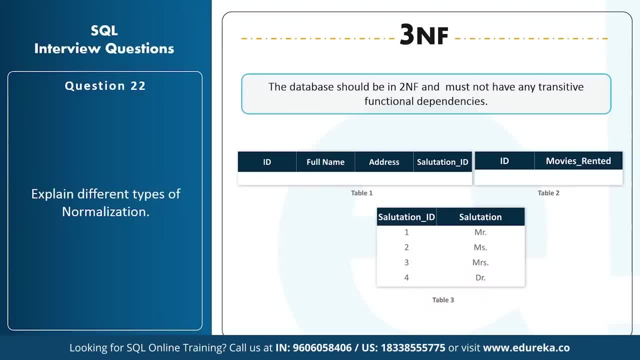 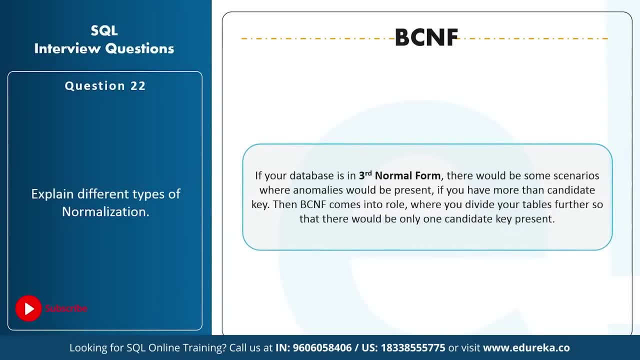 our table has been completely normalized and the highest normal form available for this particular table is 3NF. now moving forward to the final type of normalization, that is, BCNF. Now, if your database is in third normal form and there would be some scenarios where anomalies would be present, 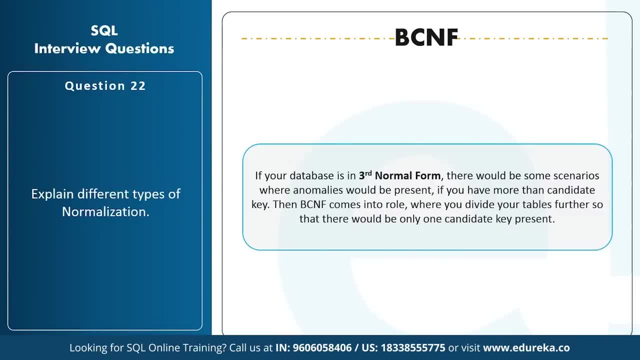 and if you have more than one candidate key, then BCNF comes into role when you further divide your table so that you know there would be only one candidate key present. So, guys, these are the various types of normalization, that is, 1NF, 2NF, 3NF and BCNF. 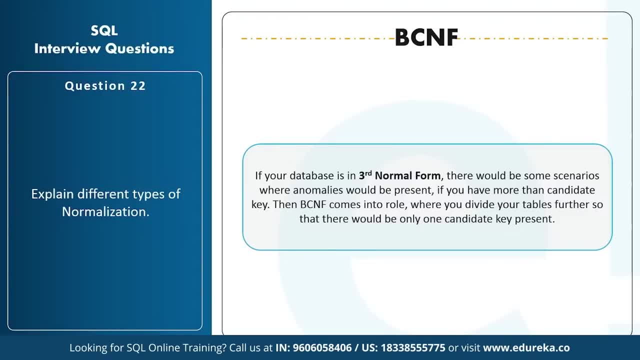 So in 1NF there is no repeating groups within the rows. in 2NF, every non key column is dependent on a whole primary key. in 3NF It is completely dependent on the primary key and no other non key column values. and in BCNF, 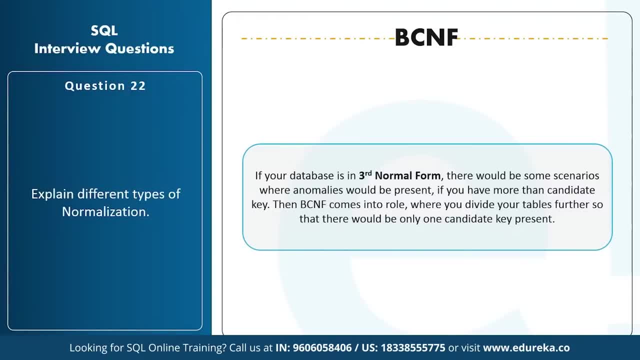 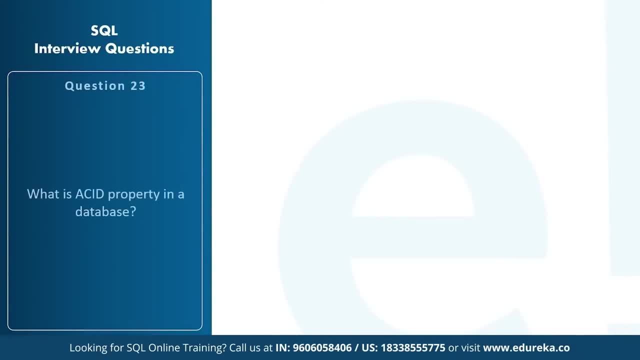 you have to make sure that you know there's only one candidate key present in the table. So, guys, these were the different types of normalization that you need to understand about. now. let's move forward to our next question, That is, what is acid property in database? the asset property. 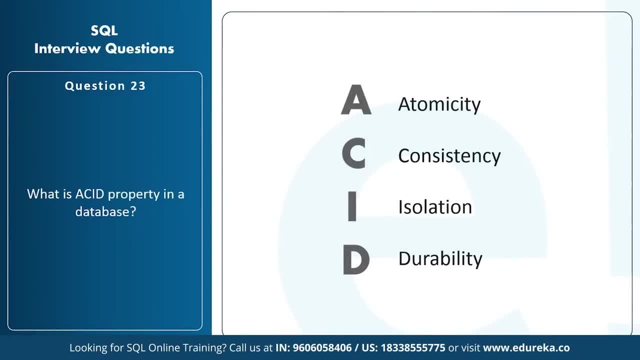 mainly stands for atomicity, consistency, isolation and durability. It is basically used to ensure that the data transactions are processed reliably in a database system. So if you have to define asset property in a database, then you have to define all these terms individually. a stands: 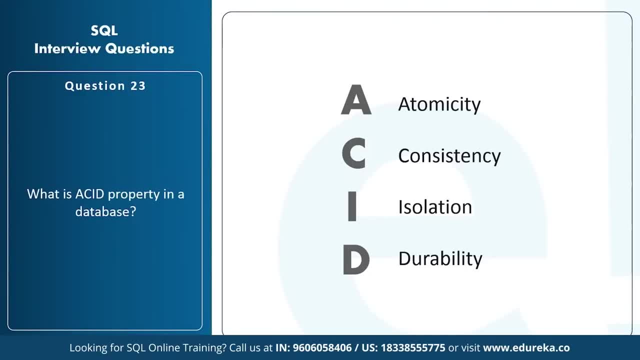 for atomicity. So atomicity refers to the transactions that are completely done or failed. where transaction refers to a single logic operation of a data, It means if one part of any transaction fails, than the entire transaction fails and the database state is left unchanged. coming. 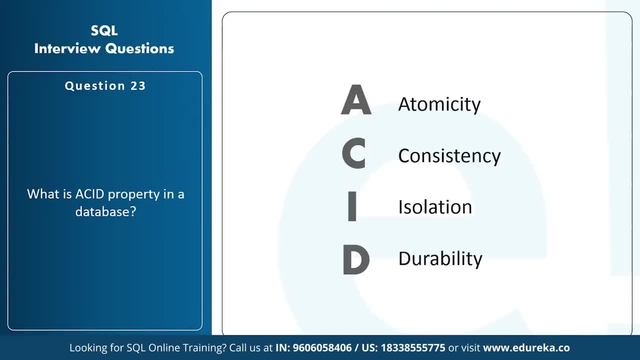 to consistency. consistency ensures that the data must meet all the validation rules. in simple words, you can say that you know your transaction never leaves the database without completing its state. third part, that is isolation. The main goal of isolation is the concurrency control. and the last part, that is durability. durability means 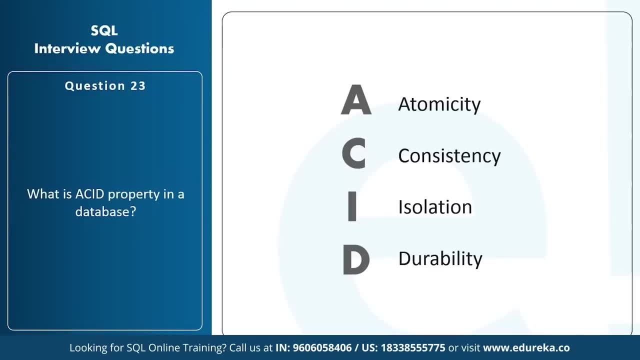 that if a transaction has been committed, it will occur whatever may come in between, such as power loss, crash or any sort of error. now let's move forward to our next question. That is what you mean by a trigger in sequel. So triggers and sequel are. 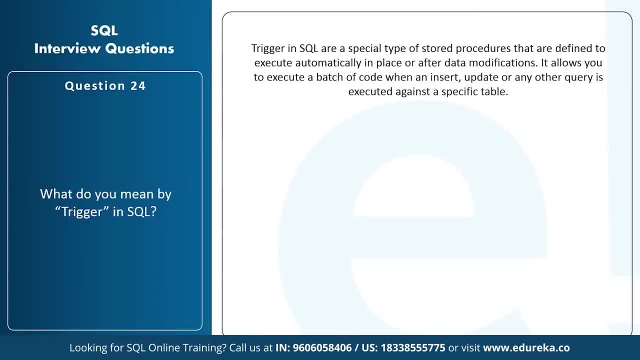 a special type of stored procedures that are defined to execute automatically, in place or after data modifications. It allows you to execute a batch of code when an insert, update or any other queries executed against the specific table. So, guys, there are mainly six type of triggers. 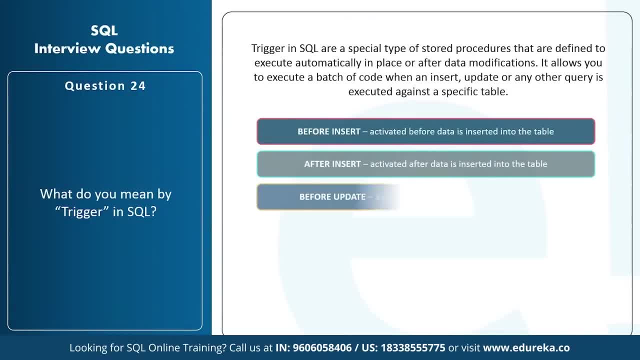 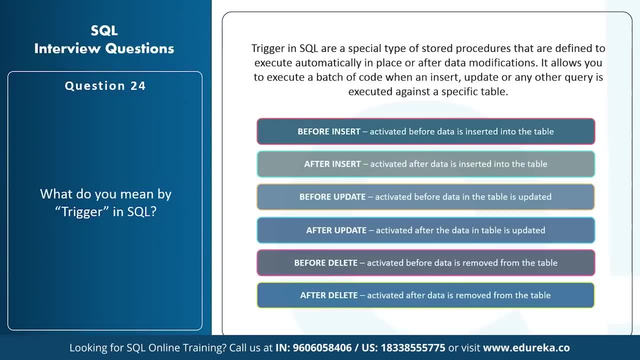 that you need to understand about that's the before insert, after insert, before update, after update, before delete and after delete. So basically the two main key terms that you need to understand at the before and the after. so these are completely applied on the insert, update and the delete commands. the before insert is basically activated. 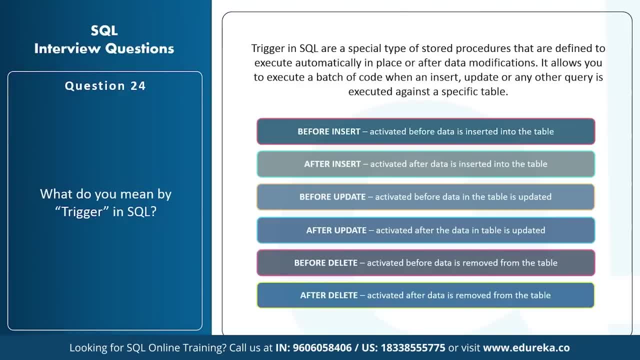 before the data is inserted into the table, The after insert is activated. after the data is inserted into the table, the before update is activated. before the data in the table is updated and the after update is activated. after the data and table is updated, the before delete is activated. 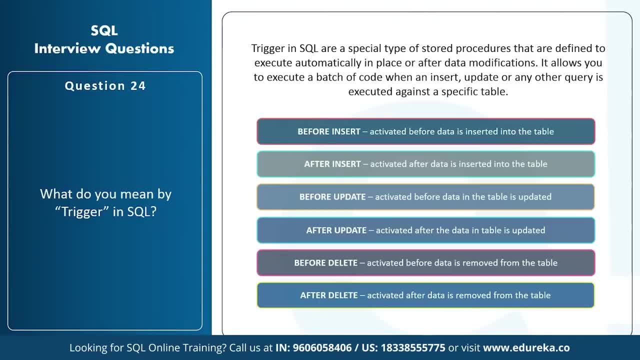 before data is removed from the table and after: delete is activated after the data is removed from the table. So, as this is what a trigger in sequel is, it is basically a type of stored procedures that is defined to execute automatically in place or after data modifications. 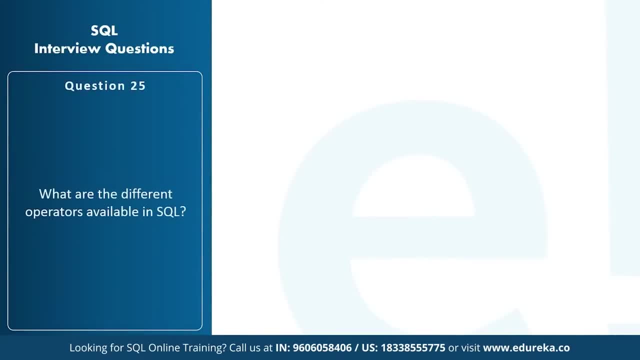 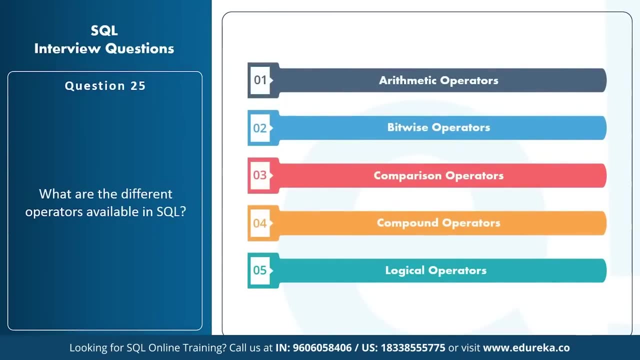 Now let's move forward to our next question, that is, what are the different types of operators available in sequel? So there are mainly five types of operators available in sequel, That is, the arithmetic, bitwise, comparison, compound and the logical operators. So, guys, these are the main five types. 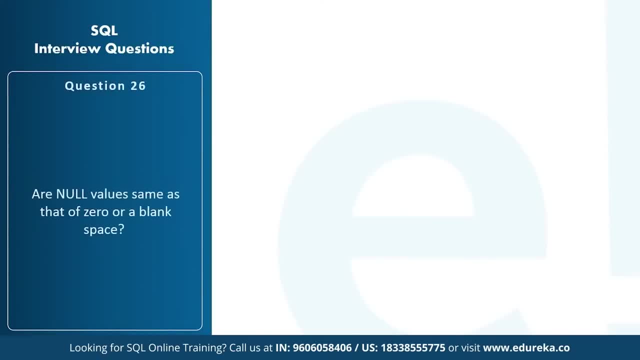 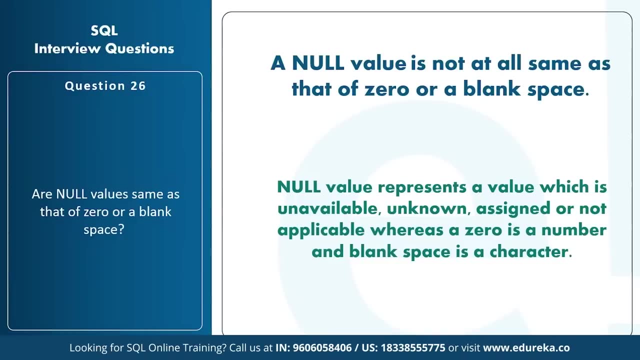 of operators available in sequel. So now let's move forward to our next question, That is, our null value same as that of zero or a blank space? a null value is not at all same as that of a zero, Zero or a blank space. a null value mainly represents a value. 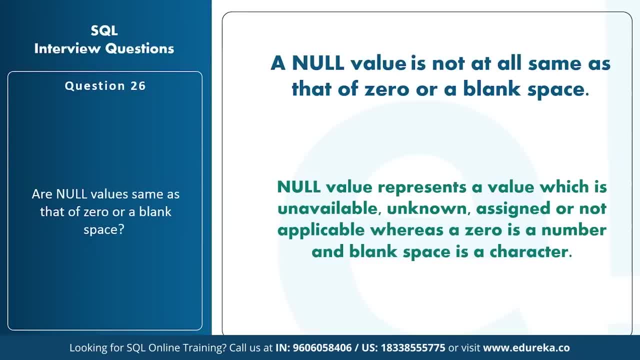 which is unavailable, unknown, assigned or not applicable, Whereas a zero is a number and a blank space is a character. So if anybody asks you if null values are same as that of zero or blank space, please say it's no, because you know the null values is basically anything which is unavailable. 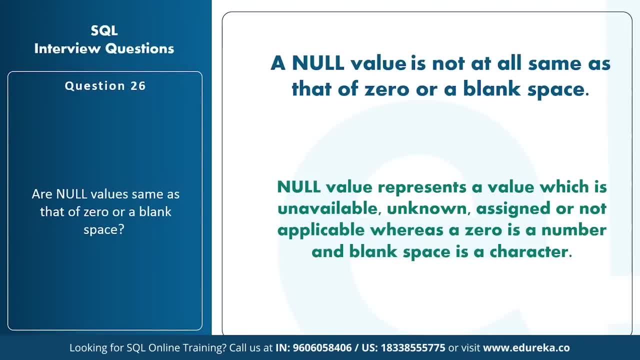 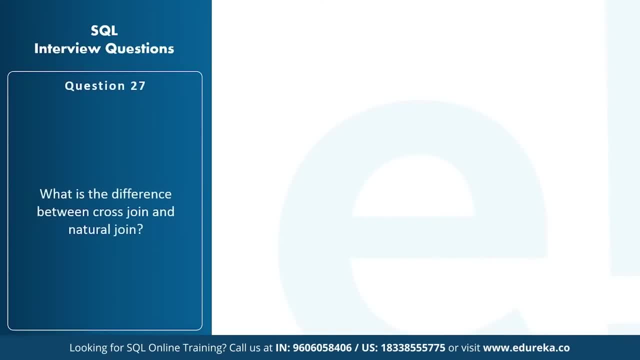 unknown and is assigned or not applicable, But as a zero is a number and a blank space is a character, Now let's move forward to our next question, That is, what is the difference between a cross joint and a natural joint? The cross joint produces the cross product. 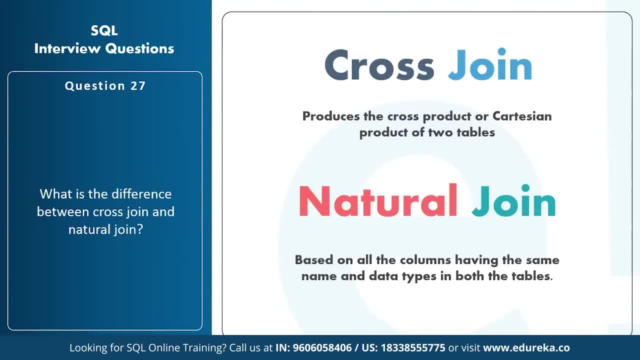 or Cartesian product of two tables, Whereas the natural joint is based on all the columns having the same name and data types in both the tables. The main difference between both of them is that in the cross joint basically produces the cross product of both the tables. 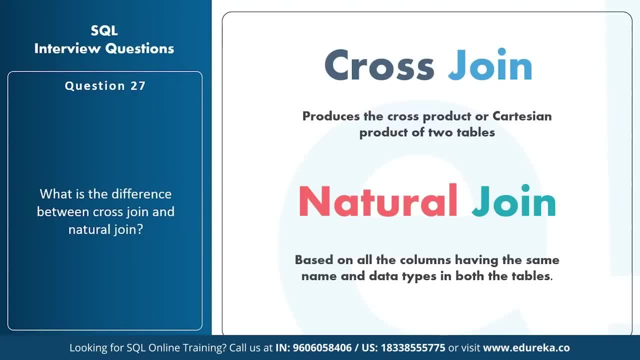 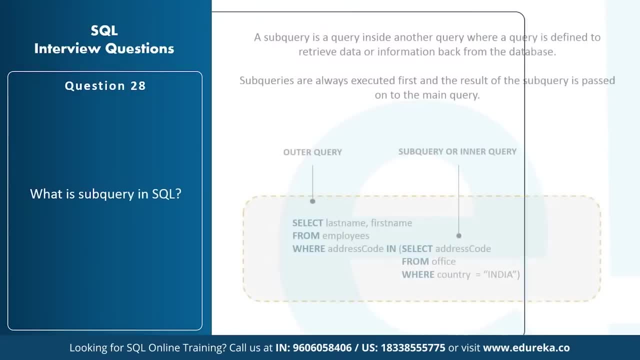 and the national joint is completely based on all the columns having the same name data types in both the team. Now let's move forward to our next question, That is, what is a sub query? in sequel, A sub query is basically a query inside under the query, where a query is defined. 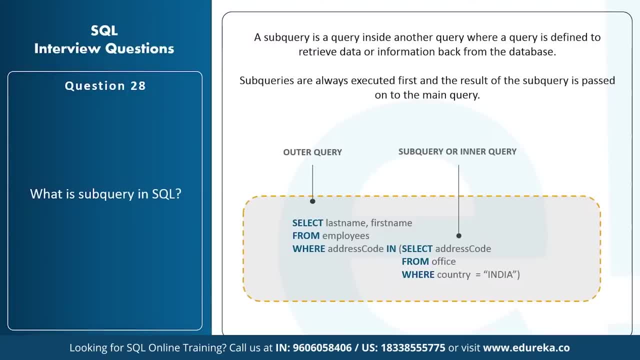 to retrieve data or information back from the database. So sub queries are always executed first and the result of the sub query is passed on to the main query. So, as you can see on my screen, I have an outer query inside which I have a sub query or an inner query. 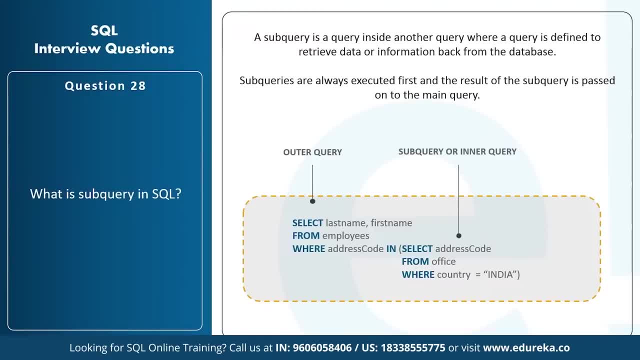 So basically, this query is assigned to retrieve data from the database and then this query will be executed first. So if there are any errors in this query, then the complete query would not be executed. only when the sub query is completely executed, Then the outer query will be executed. 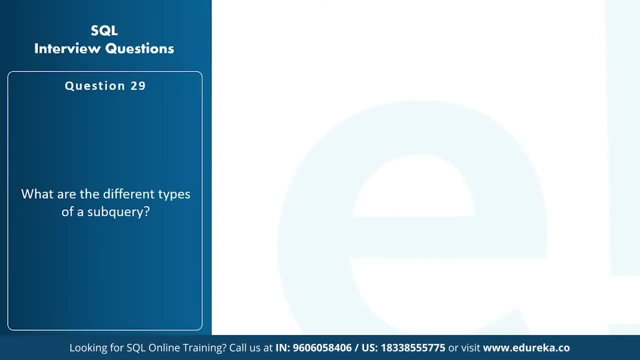 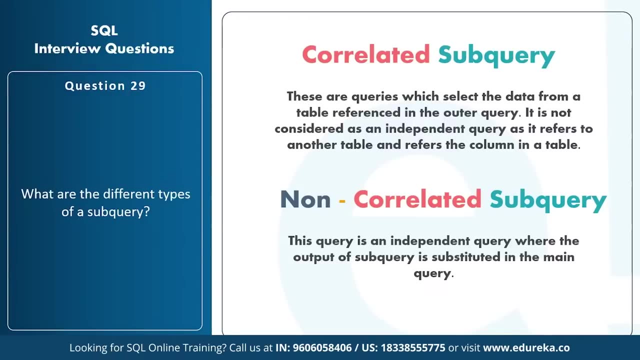 Now let's move forward to our next question, That is, what are the different types of sub query? Now, there are mainly two types of sub queries, that is, the correlated and the non correlated sub query. The correlated sub queries are basically those queries 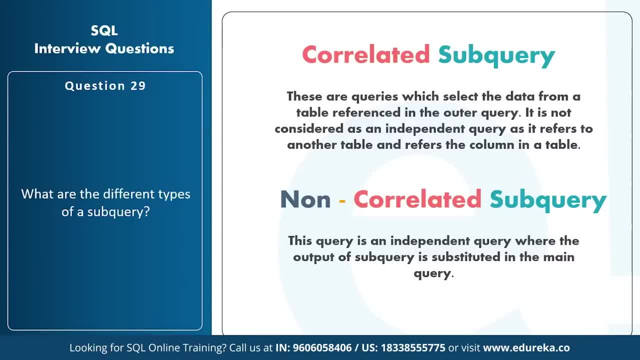 with selected data from a table reference in the outer query. It is not considered as an independent query as it refers to another table and refers to column in a table. The non correlated sub query is an independent query where the output of the sub query is substituted. 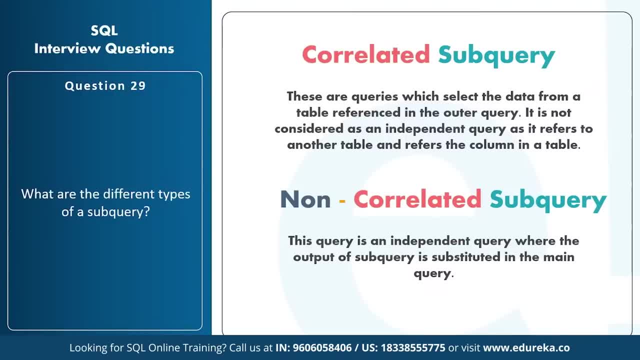 in the main query, So you'll have to understand the difference between both of them. If you do not understand by definition, you can definitely go and execute the commands, write the two different types of queries in your sequel and you'll get to know what I'm talking about. 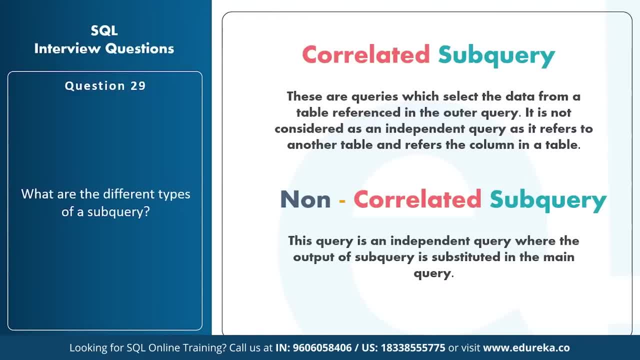 Basically non correlated type of sub query. the output of the sub query will be substituted into the main query. and correlated type of sub query. The query is select the data from a reference table in the outer query. Now let's move forward to our next question. 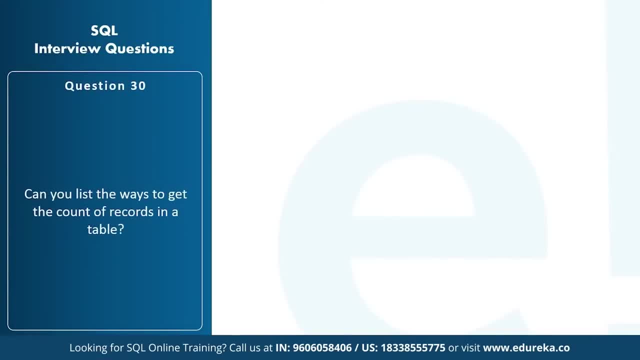 That is, can you list the ways to get the count of records in a table? now, to count the number of records in the table, you can use various kind of queries. So there are mainly three queries that I've mentioned over here. that is, select star from table. one star means basically select. 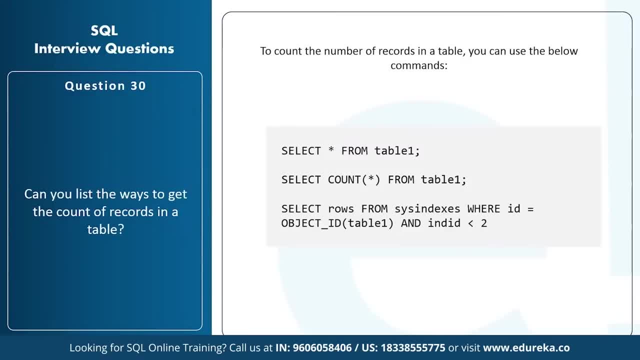 all right. when you want to select all the rows, all the records from a table, you can use star. next, when I say select, count, star from table one, that is basically you select all the records from the table one and then you count them. and coming to the third query, 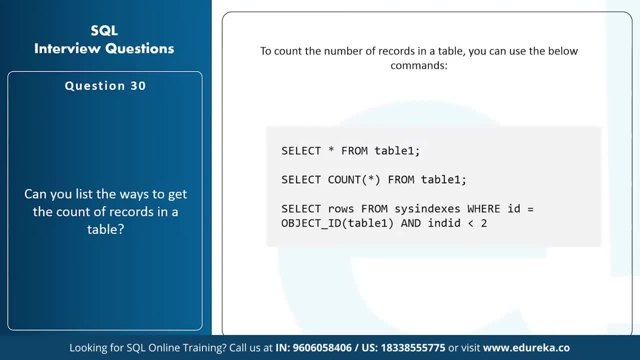 that is, select rows from system indexes where ID object, ID of table one and indeed is less than two, That means it's basically Council number of records in the table with system indexes. These are the various ways to count the number of records in a table. 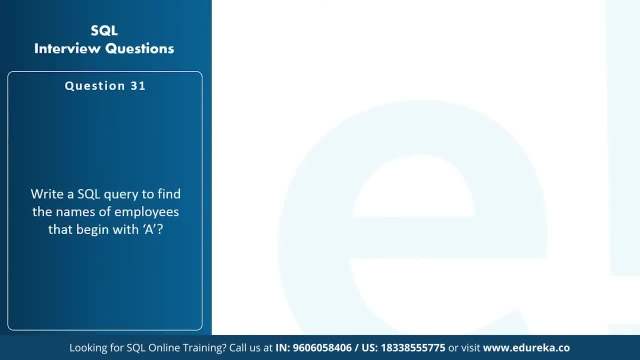 Now let's move forward to our next question, that is, write a sequel query to find the names of employees that begin with the alphabet a. now, to display the name of employees that begin with a, you can type in the command, like you know, select star from table name. 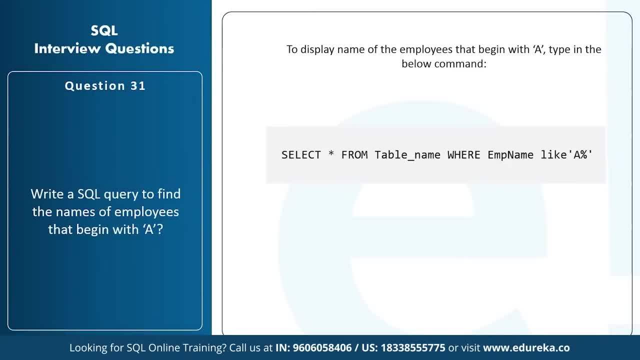 where you mention your table name, where employee name, because I'm considering an employee table in the scenario like a person in codes. So when I say a person, all those names starting with a and having any letters or any characters after that would be selected. So, guys, that's how you can write a query to find the name. 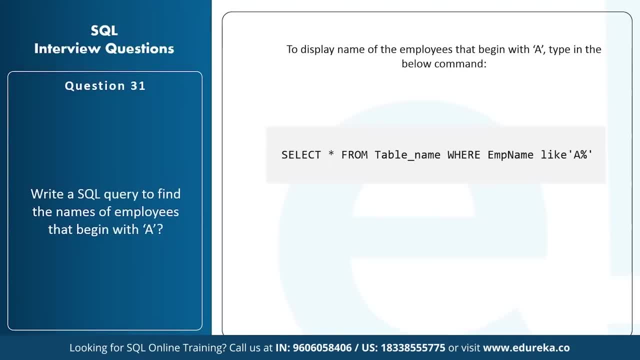 of employees that begin with a. now suppose if you want to write a query to find the names of employees that end with a, what you can simply do is you can again write the similar query. like you know, select star from table name where employee name like percentage a right. 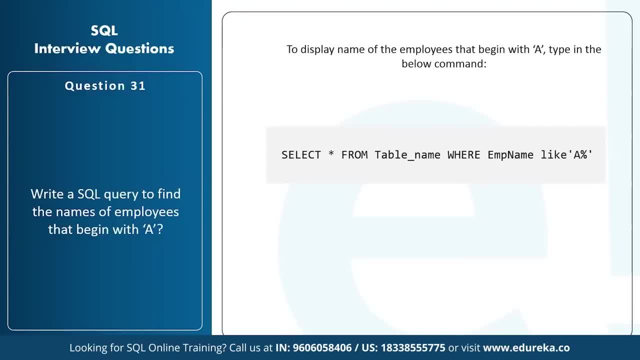 So where the percentage comes forward- that means you know all the names that start with any alphabet but end with the a will be considered. now let's move forward to our next question, That is, write a sequel query to get the third highest salary. 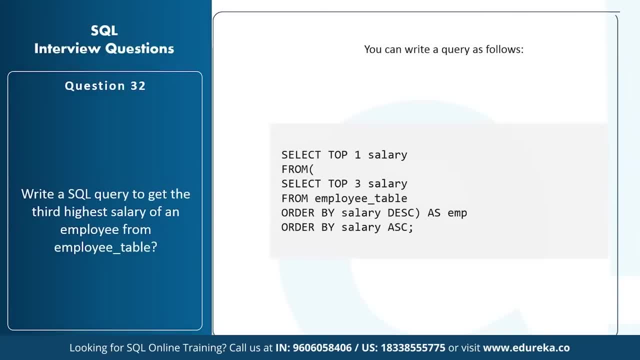 of an employee from an employee table. now, to get the third highest salary of an employee from an employee table, You can write a query. as you can see on the screen, You can just mention select top one salary from and then write a sub query which says select top three salary from employee table order. 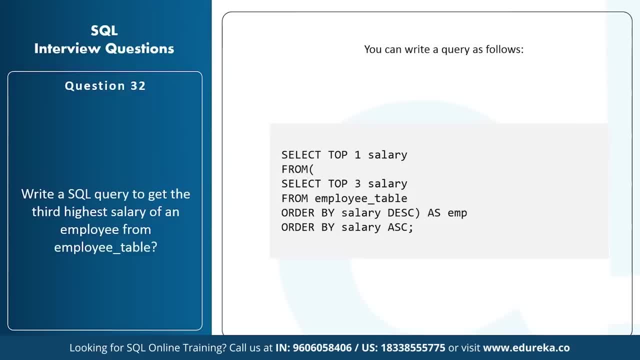 by salary in a descending order as M, and then again order by salary in ascending For the outer query. so you can write a query like this: guys, Now let's move forward to a next question, That is, what is the need of group functions in sequel now? 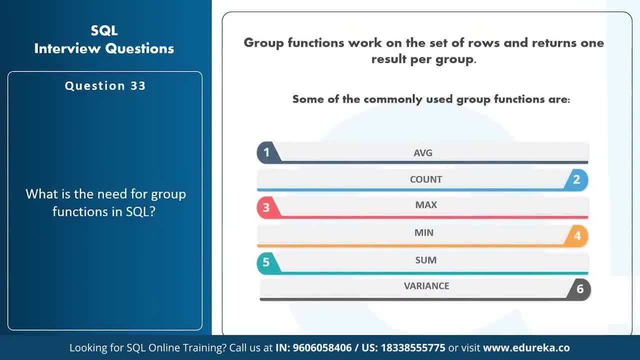 group functions work on a set of rows and return one result per group. So basically, some of the most commonly used group functions are the average, count, Max, min, sum and variance. So when you say what is the need of group functions in sequel, The need is basically because the group functions work. 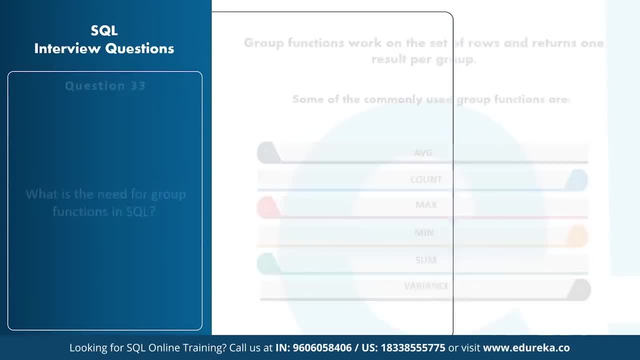 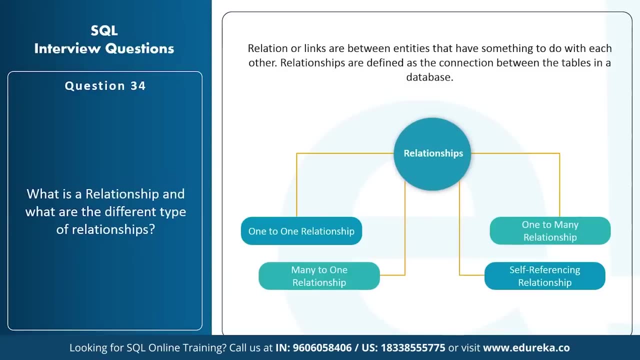 on a set of row and return one result per group. Now let's move forward to the next question, that is, what is a relationship and what are the different types of relationship? so relation or links between entities that have something to do with each other can be basically termed as relationships. 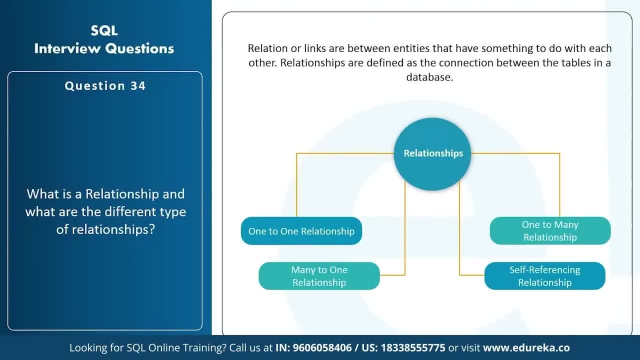 So relationships can be also defined as the connection between the tables in a database, right? So the different types of relationships are the one-to-one relationship, the one-to-many relationship, many to one relationship and the self-referencing relationship when you have a relationship. 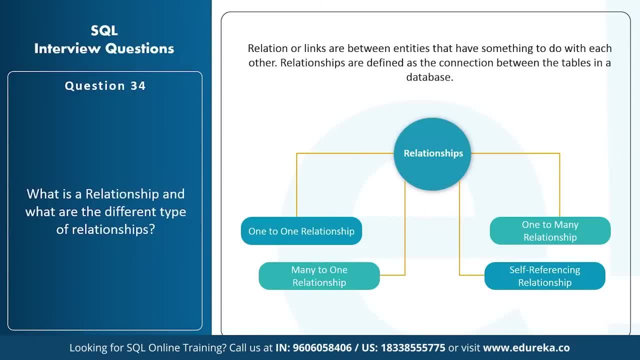 for between two tables at his table a and table B. So when I say one-to-one relationship between both the tables, table a and table B, a single record in table a will be related to a single record in table B. coming to one-to-many relationship, a single record in table. 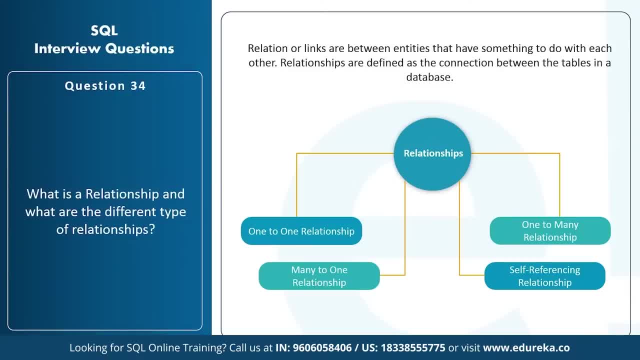 A can be related to many records in table B. next, coming to the many-to-one relationship, many records in table a can be related to one record in table B. coming to self-referencing relationship, the self-referencing relationship basically means that you can have a single table. 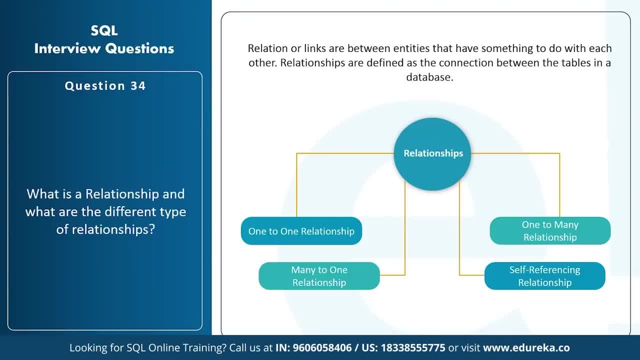 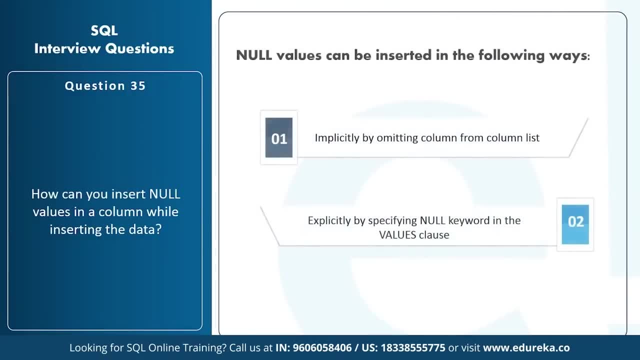 out of which two columns are related to each other with the relationship. now let's move forward to our next question, That is, how can you insert null values in a column while inserting data? now, to insert null values in a column while inserting the data. 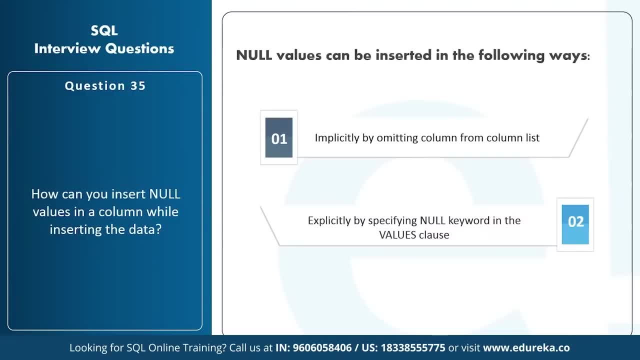 You mainly have two ways, that is, either by implicitly, by omitting columns from a column list, or explicitly, by specific null keyword in the values clause. So, as these are the two ways through which you know you can insert null values in a column while inserting the data, 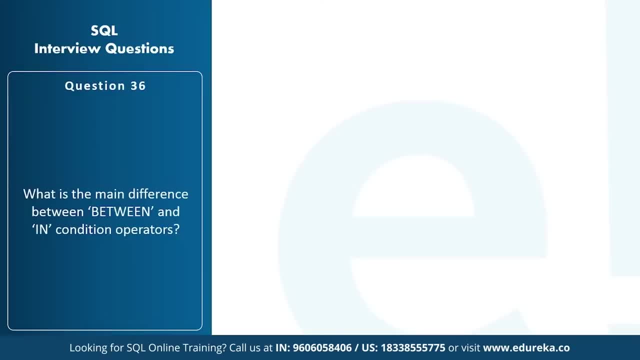 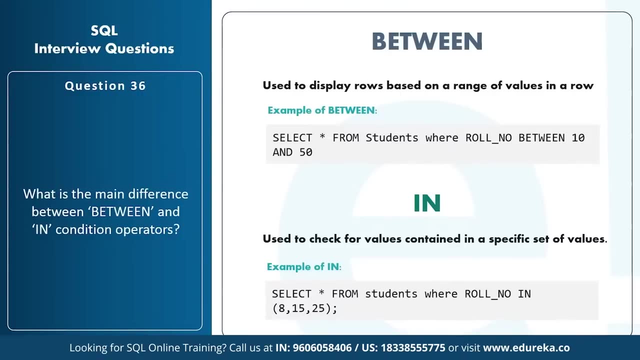 Now let's move forward to the next question, That is, what is the difference between the between and the in-condition operators? the between operators basically used to display rows based on a range of values in row, Whereas the in-condition operators used to check for values contained in a specific set of values. 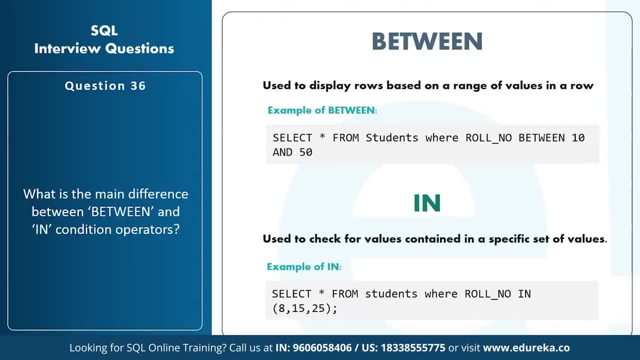 So if you have to explain with an example for between and the in-condition operators, then you can use the example on the screen. You can just write a query like in a select star from students by row number between 10 to 50. So all those records from the students table would be selected. 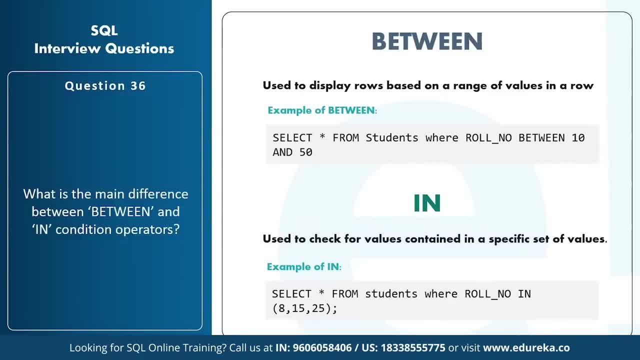 whose roll numbers It stands between 10 to 50. coming to the in-condition operators, You can use a query like this: like you know, select star from students where roll number in 8, 15, 25.. So all those records from a student table would be selected. 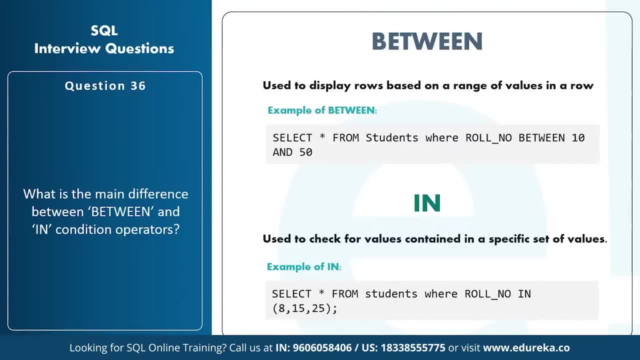 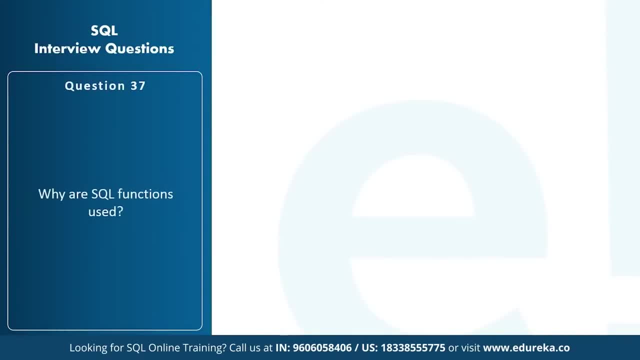 where the roll number would be either 8, 15 or 25.. So, guys, that is the main difference between the between and the in-condition operators. Now let's move forward to our next question. That is, why are the sequel functions used? the sequel functions? 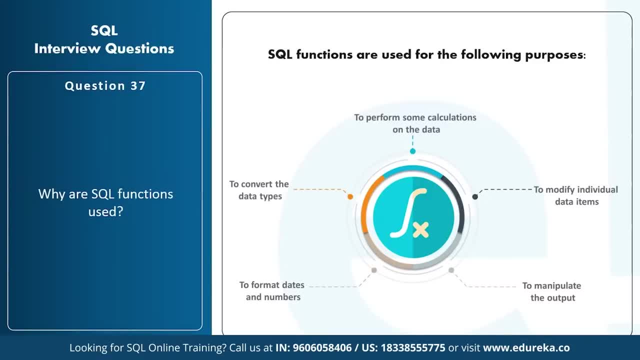 are used to perform some calculations on the data, to modify individual data items, to manipulate the output, to format dates and numbers and also to convert the date types. So if you want to perform these activities, or you know if you want to perform these actions, 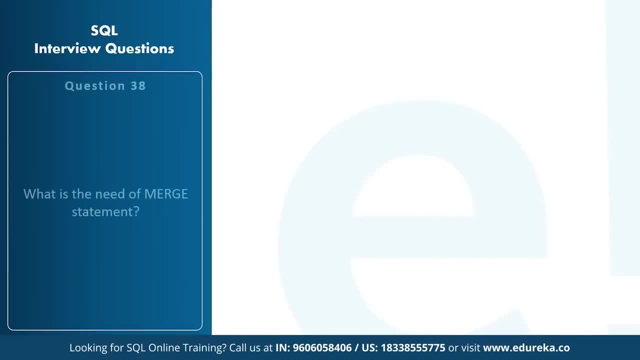 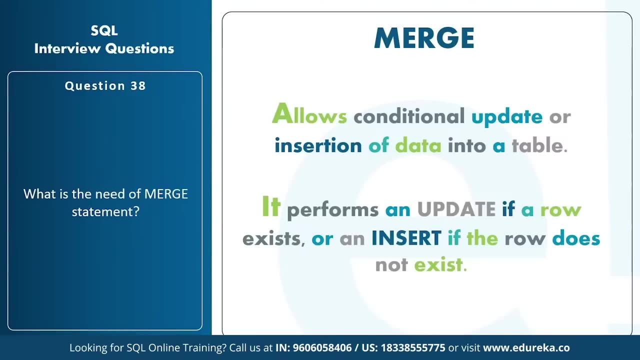 then you need to use the sequel functions. Now let's move forward to our next question, That is, what is the need of merge statement? This statement is basically used to allow conditional update or insertion of data into a table, So it performs an update if a row exists. 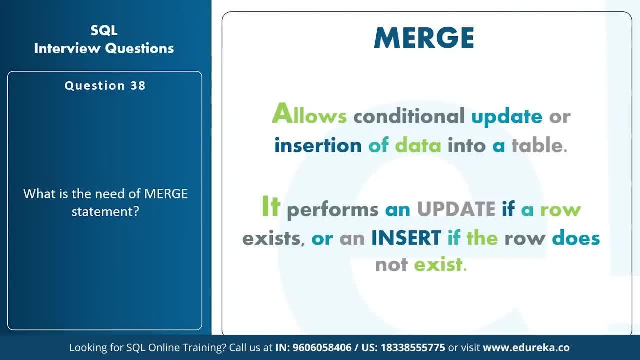 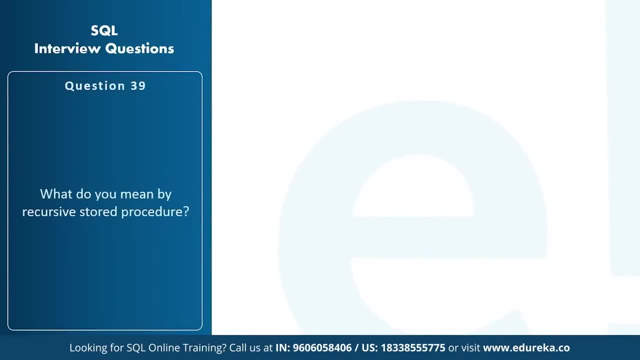 or an insert if the road doesn't exist. So basically, the need of merge statement is that you know it allows conditional update or insertion of data into a table. Now let's move forward to our next question, That is: what do you mean by recursive stored procedure? 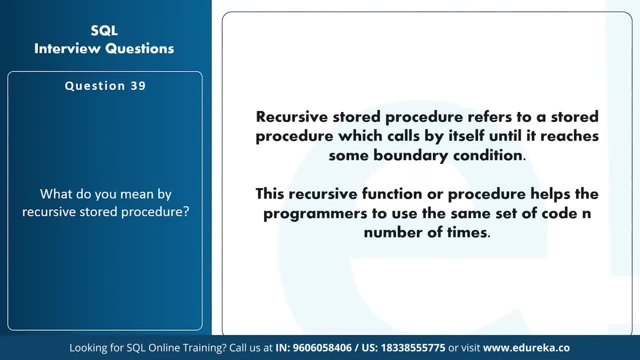 recursive stored procedures refers to a stored procedure which calls by itself until it reaches some boundary condition. this recursive function or a procedure helps the programmers to use the same set of code n number of times. So basically, you'll first mention the boundary condition and then you'll use the recursive stored procedure. 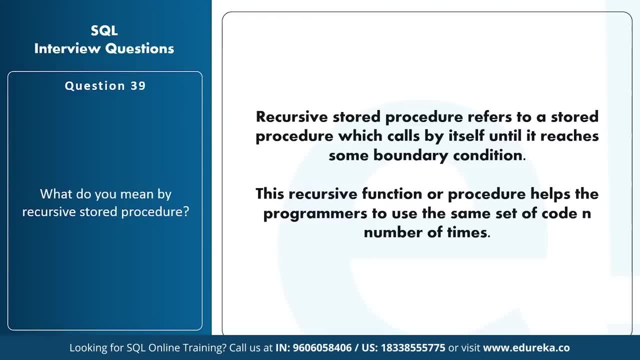 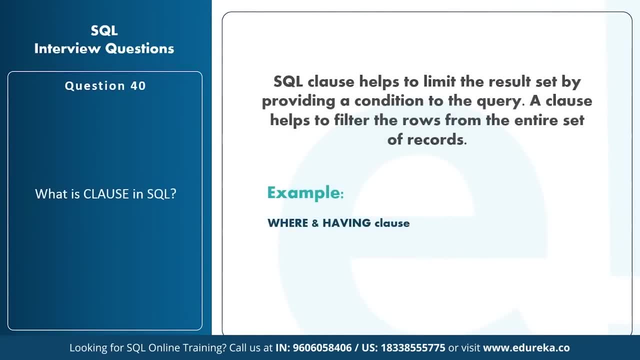 to check, you know, if it calls by itself till it reaches, which is the specified boundary condition. Now let's move forward to our next question, That is, what is a clause in sequel? now, sequel clauses basically helps you to limit the result set by providing a condition to the query. a clause helps. 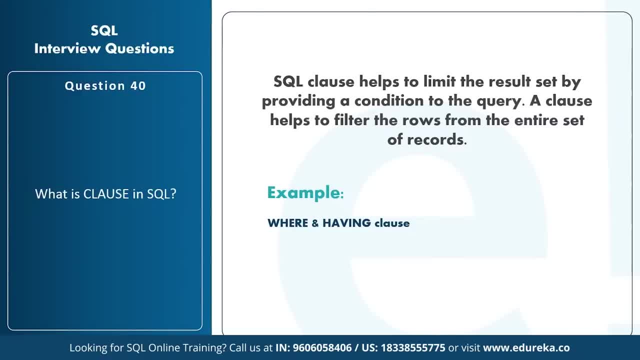 to filter the rows from the entire set of record. So for you better understanding, the example is basically where and having clauses. So when you write a query, you having these two particular clauses, you basically mention a condition into these particular clauses, right, Like where student number is equal to 2. 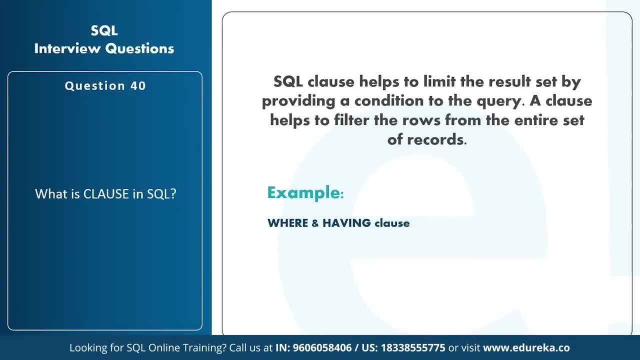 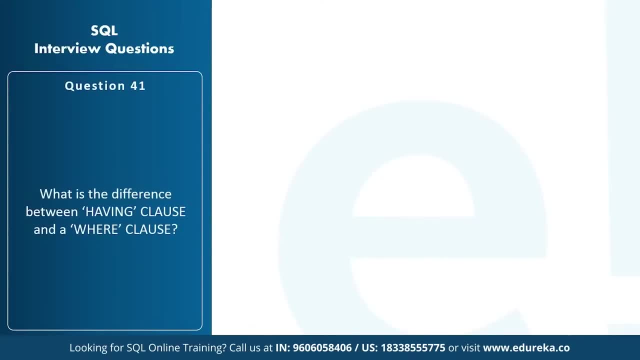 or having you know rule number greater than 5, and so on. right, So that's how you can use a clause in sequel. Now let's move forward to our next question, That is, what is the difference between the having clause and the where clause? that the main difference. 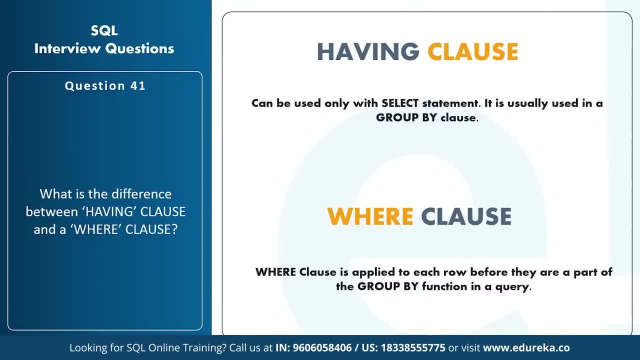 between having clause and where clause is basically that you know the having clause can be only used with the select statement. It is usually used by the group by clause and whenever group by is not used, having basically behaves like a where clause. coming to the where clause, the 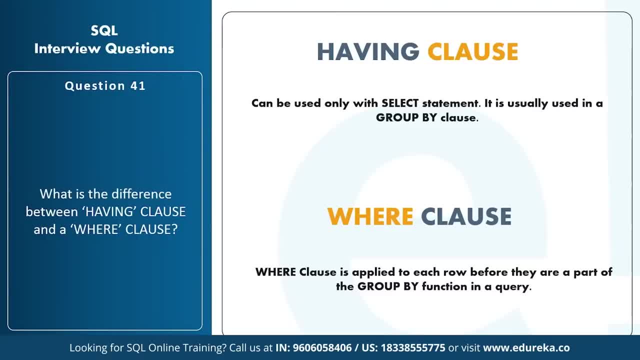 where clause is applied to each row before they're a part of the group by function in a query. So having clause is basically used with the select statement and it is usually used in the group by clause when the having clause is not used with the group by clause. 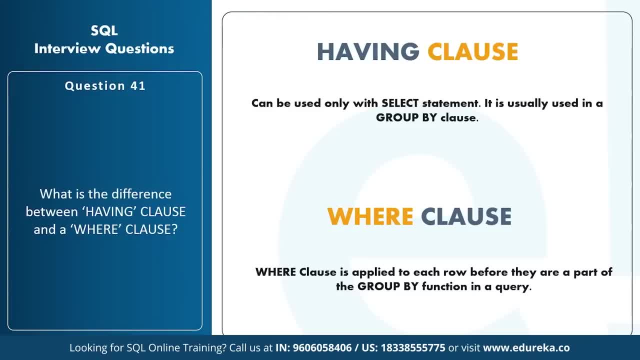 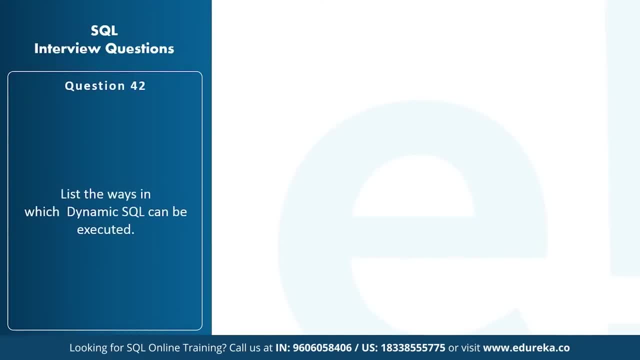 the having clause behaves like a where clause. so, guys, that was about the difference between the having clause in the where clause. now let's move forward to our next question, that is, list of ways in which dynamic sequel can be executed. the ways in which dynamic sequel can be executed are: 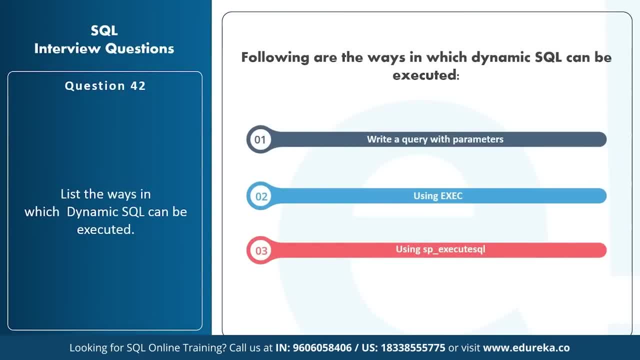 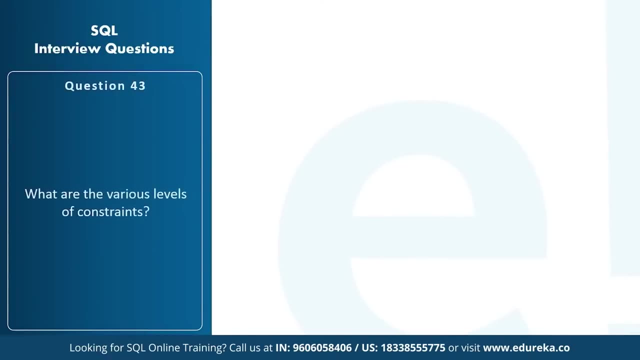 by writing a query with parameters, using exec and by using SP hyphen: execute sequel. So there are basically three ways in which dynamic sequel can be executed. that is, by writing query with parameters, using exit and using SP underscore: execute sequel. now moving forward to the next question, that is, what are the various levels? 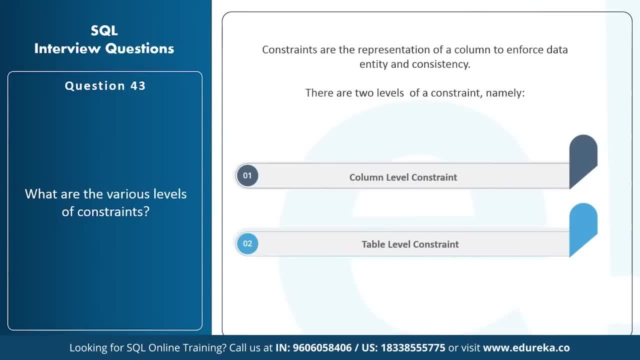 of constraints. the constraints, as I mentioned before, are basically the representation of a column to enforce data entity and consistency. So, Bailey, there are two levels of constants, that is, the column level constant and the table level constraint. now let's move forward to our next question. 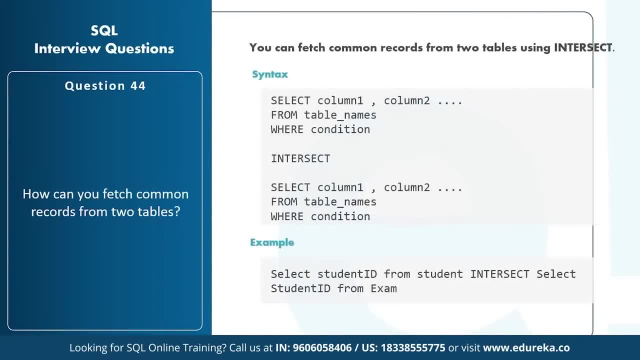 That is, how can you fetch common records from two tables, while you can fetch common records from two tables by using the intersect statement. So the syntax of intersect statement is as you can see on the screen. It's basically select column 1, column 2. 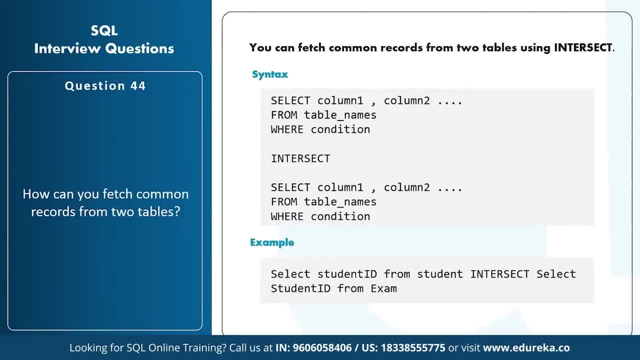 and so many columns from the table name where condition, basically where you mentioned the condition over here. Then you mentioned the keyword intersect and then again mentioned another table name, right? So that is again you mentioned. select the columns from a specific table where the condition matches. 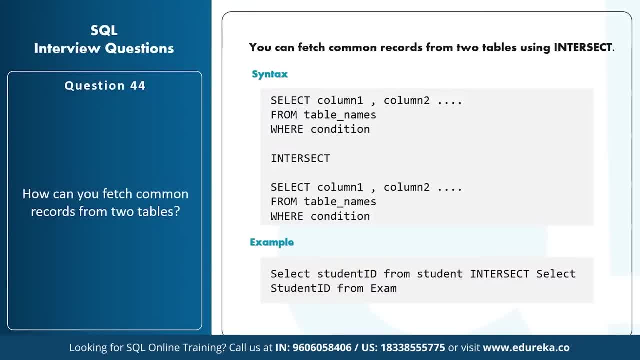 So that's how you use the intersect format. So for your better understanding, you can see the example on the screen. you can see. you know that I have used select student ID. that is basically a single column from student. then use the intersect command and then again I have mentioned select student ID. 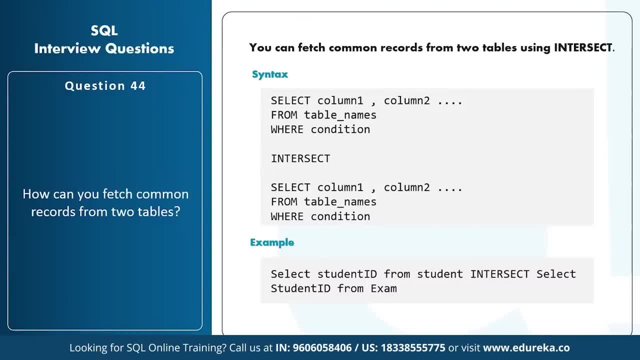 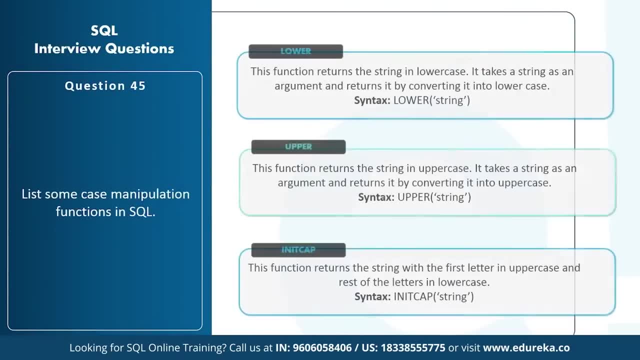 from a different table. that is exam. So that's how you can fetch common records from two tables. Now let's move forward to a next question, that is list some case manipulation functions in SQL. So there are mainly three case manipulation functions in SQL, that is, the lower upper and the init cap. 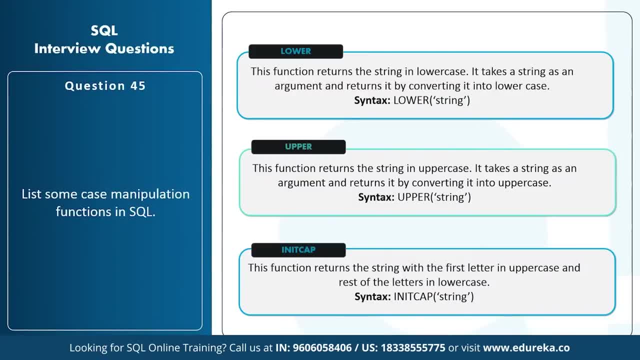 the talking about the lower function. This function basically returns the string in lower case. It takes a string as an argument and returns it by converting into a lower case. The syntax of this particular function is basically lower and in brackets. you mentioned strings and quotes. now moving. 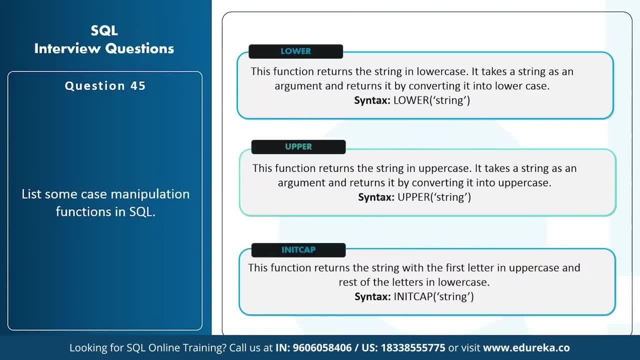 forward to the next function, that is, the upper function. This function returns the string in uppercase. It takes a string as an argument and returns it by converting it into an uppercase right. So the syntax for this particular function is upper and in brackets. you mentioned the spring within the codes moving. 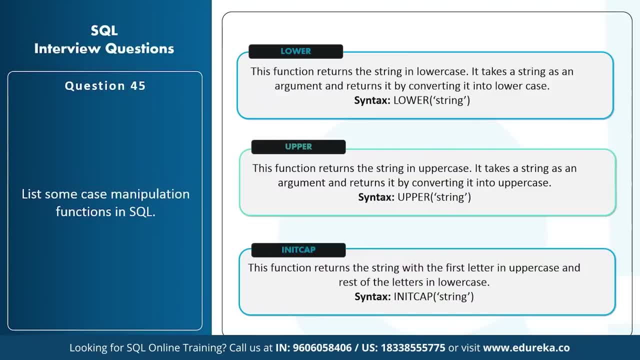 forward to the third function, That is, the init cap. this function returns the string with the first letter in uppercase and the rest of the letters in lower case. So the syntax with this function is basically init, cap and in brackets You mentioned the string with quotes. 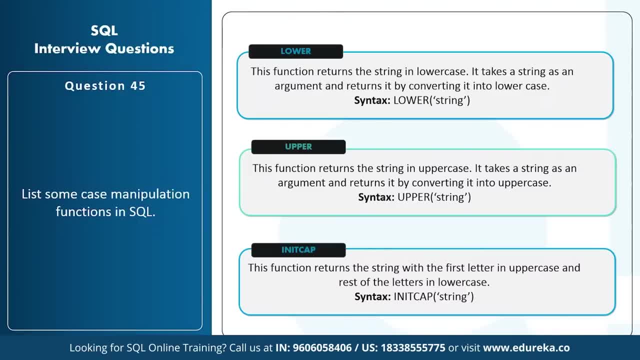 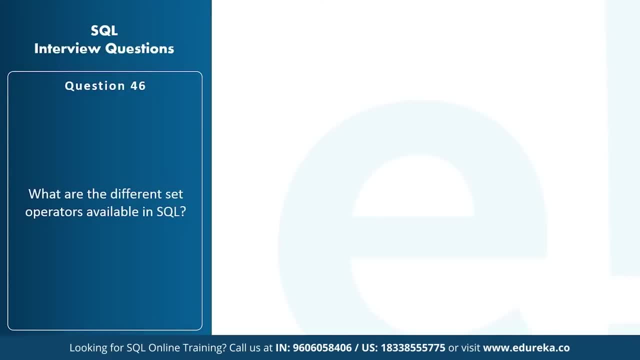 So, guys, these were the three case manipulation functions in SQL. now let's move forward to our next question, That is, what are the different set operators available in SQL? So the different set operators available in SQL are Union, intersect and the minus operators. So let's talk about Union first. 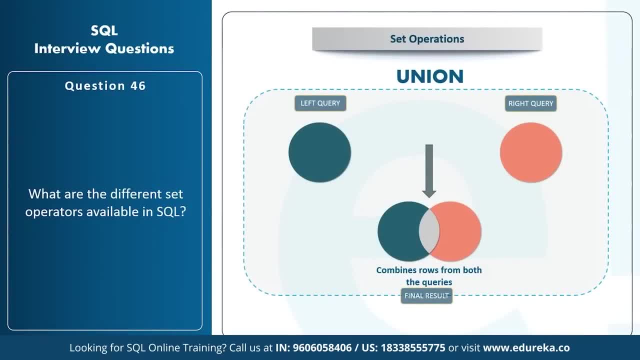 So when you consider two queries, that is, the left query and the right query, And you apply the Union operation, you will see that you know it will combine rows from both those queries. You'll get an output of, you know, all those records from the left table. 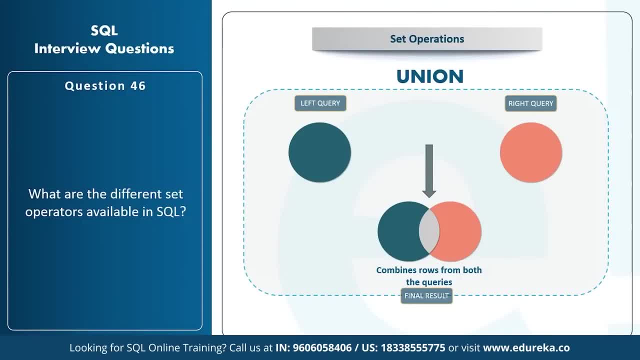 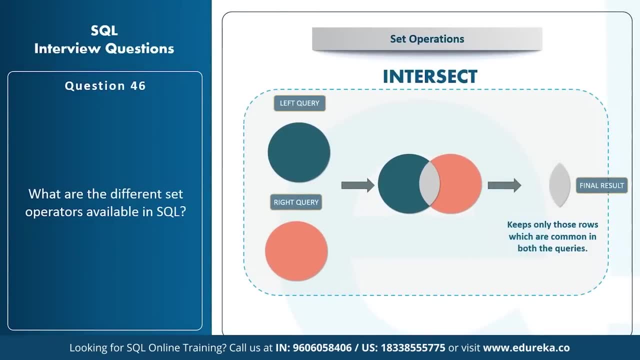 That is basically the left query and also from the right query That is the right table. moving forward to the next operation, It is the intersect operation. So when you apply the intersect operation to the left query and the right query, you'll see that you know. 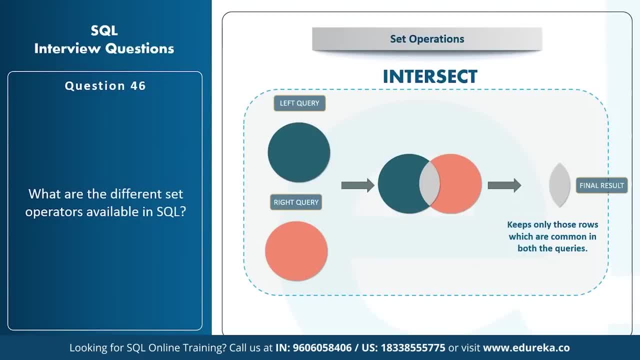 you'll get only those rows which are common in both the queries, right? So, for example, you have 10 rows in the first table and 10 rows in the second table, but the common rows and both these table are just two rows. 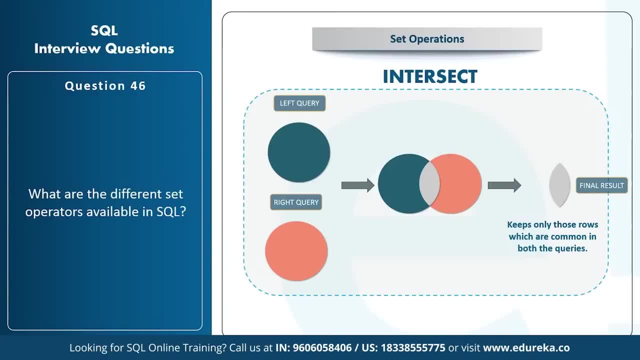 So you'll get only those two rows as an output to this particular operation. moving forward to the third type of operation, that is, the minus operation. So when you apply left query minus right query, you'll see that you know you'll get the only those rows from the left query. 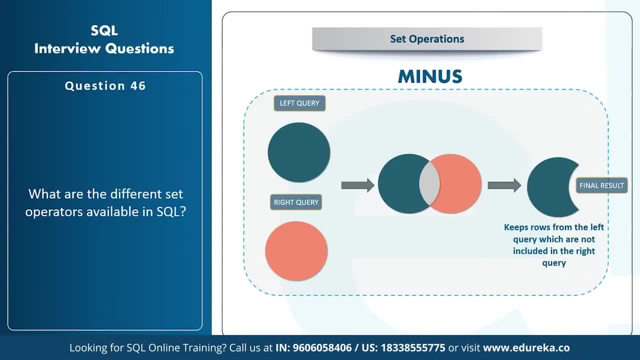 which are not included in the right query as an output, and when you apply the operation of right query minus left query, you'll see that you will get only those rows as an output from the right query which are not included in the left query. 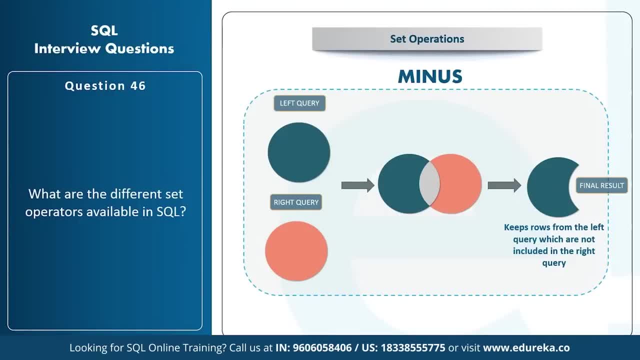 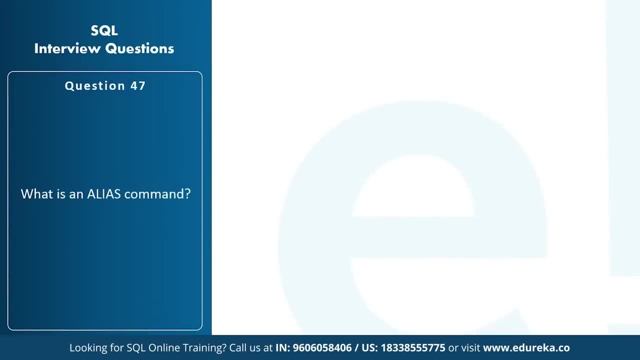 So, guys, These were the different set operators available in SQL. that is, the union operator, the intersect operator and the minus operator. Now let's move forward to our next question, That is, what is an alias command? now, alias name can be given to any table or any column. 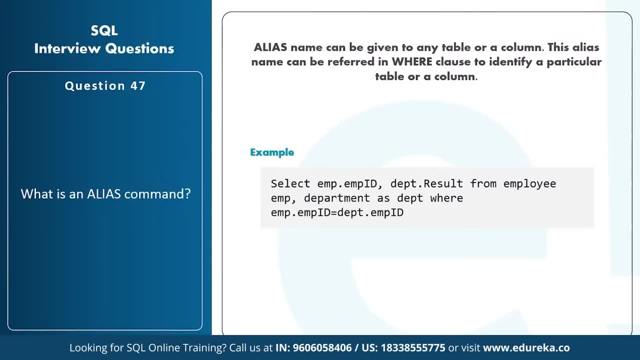 So this alias name can be referred in where clause to identify a particular table or a column. So that's basically an alias command. So, for example, if you see on the screen you see a query right like select M dot, employee ID department dot. result from employee M department as depth. 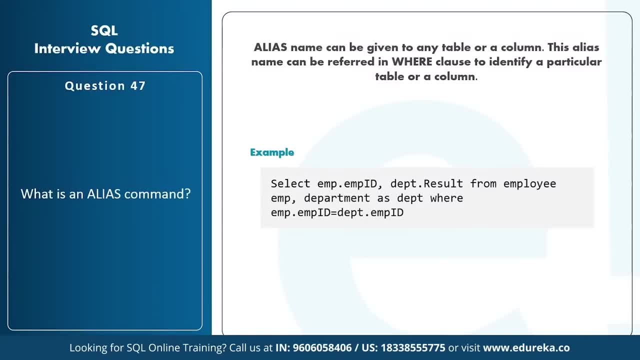 where M dot employee ID is equal to department dot employee ID. So what I've given over here is that I've given an alias name to the employee table as M and for the department table I've given an alias name as debt. So that's how you can use the alias command, guys. 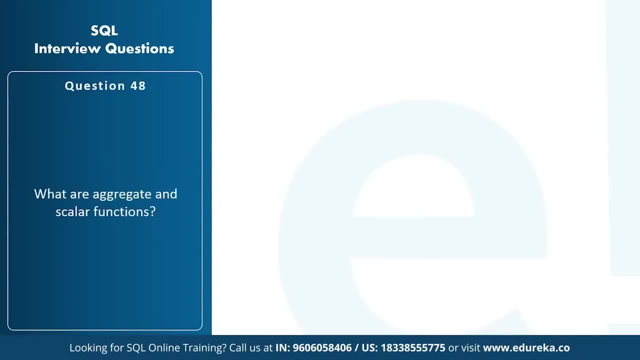 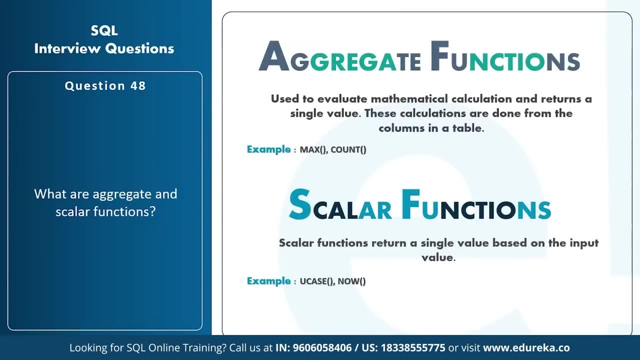 Let's move forward to the next question Now, that is, what are aggregate and scalar functions? The aggregate functions are used to evaluate mathematical calculation and return a single value. These calculations are done from columns in the table. So, for example, if you need to consider the aggregate functions, 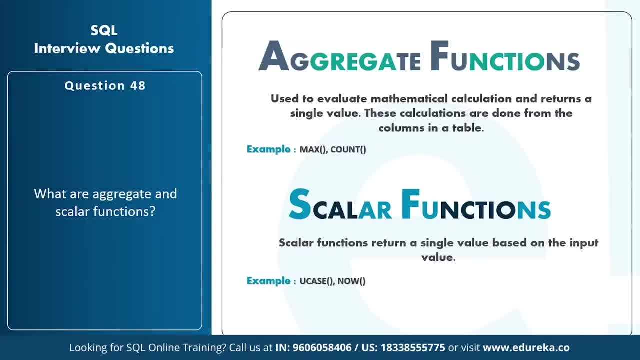 then you can consider the Max function and the count function as an aggregate function. now, coming to the scalar functions. The scalar functions basically return a single value based on the input value. So if you need an example for scalar functions, then you can consider the UK's. and now a scalar functions. 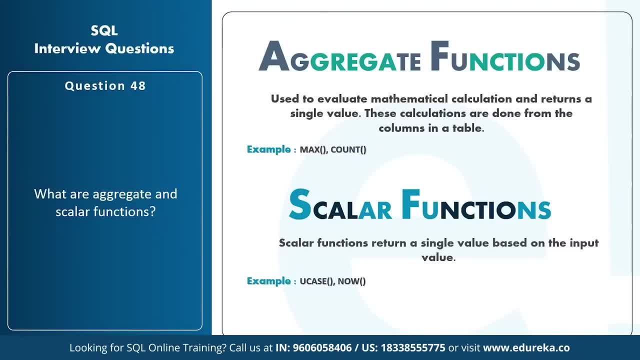 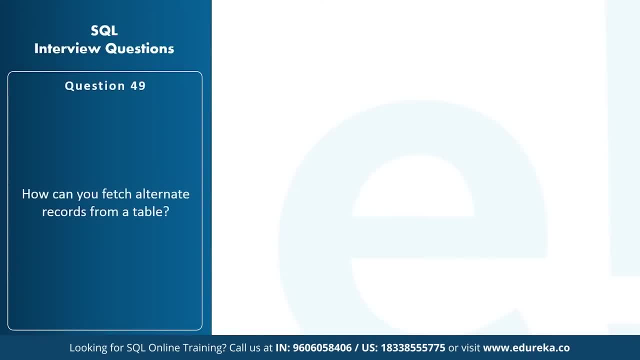 as their calculated with respect to the spring. So, guys, this is what aggregate functions and scalar functions mean. Let's move forward to the next question, That is, how can you fetch alternate records from a table? when you answer this question of how you can fetch alternate records from a table, 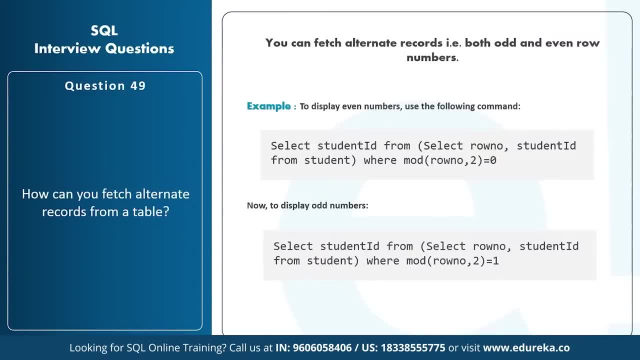 please make sure that you mention a point: that you can fetch alternate records, That is, both the odd and the even row numbers. now, to display the even row numbers, You can use the command, like you know, select student ID from: select row number: student ID. 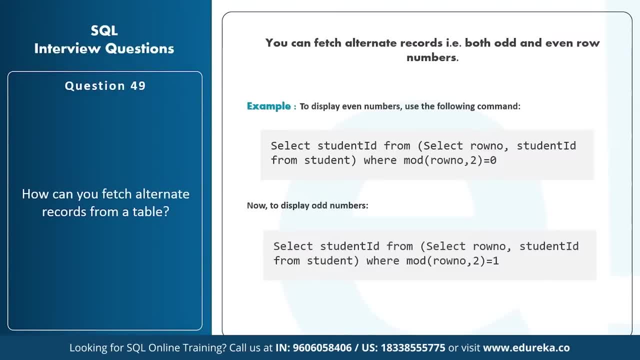 from student again- where mod row number, comma 2 equal to 0.. So we're using this function of where mod row number, comma 2 equal to 0, right? So when you divide the row number with 2 and if you get the reminder as 0, 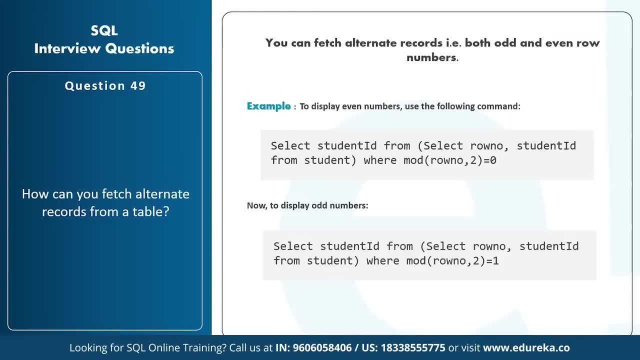 then that particular row Number would be an even number And similarly, if you get a reminder as 1, then that particular row number would be an odd number. That's how you can segregate the alternate records, That is, the even number records and the odd number records. 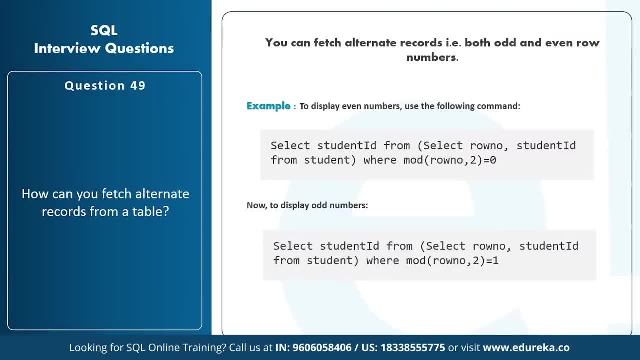 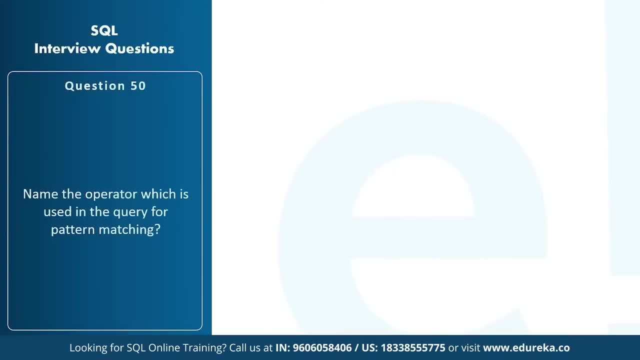 You just have to mention the condition: mod row number- comma 2, equal to 0, if or even, and mod row number, comma 2, equal to 1, for odd. Now let's move forward to the next question, that is, named the operator which is used in query for pattern matching: the operator. 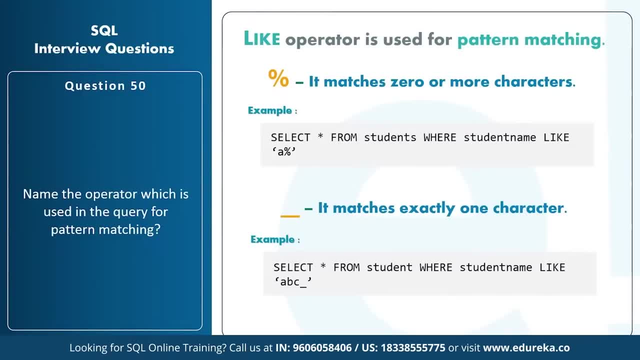 which is used in the query for pattern matching is basically It's the like operator. So in like operator you can use either the percentage sign or the underscore sign. the percentage sign basically matches to 0 or more characters. if you use the percentage sign in the query, like you know, select star from students. 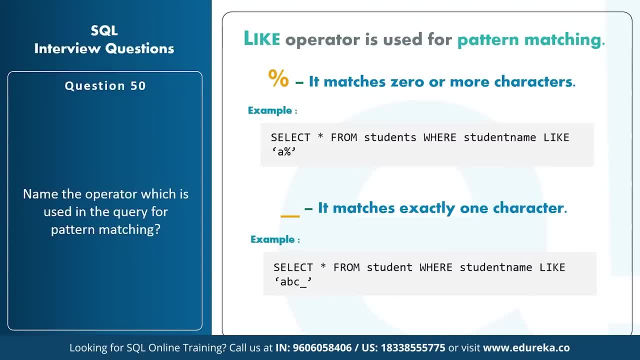 where student named like a percentage. So all those student names whose name starts with a and ends with any character will be taken into account and all the information related to all those records will be retrieved and coming to when you use the underscore sign. the underscore sign. 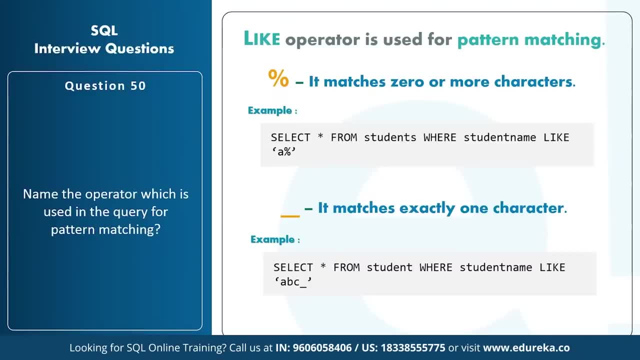 basically matches exactly one character. So when you use the underscore sign in the query, like you know, select star from student where student name like ABC underscore. So all those records you know whose student name has a characters which match the pattern ABC and any character present after that will be taken into account. 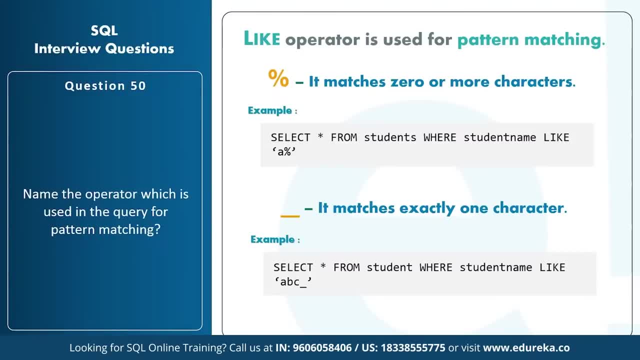 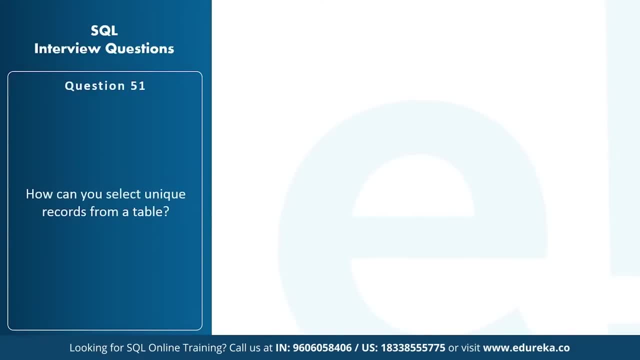 So is. that's how you can use the like operator for pattern matching. you can either use the percentage sign with it or an underscore sign with it. Now let's move forward to the next question, That is, how can you select unique records from a table where you can select unique records? 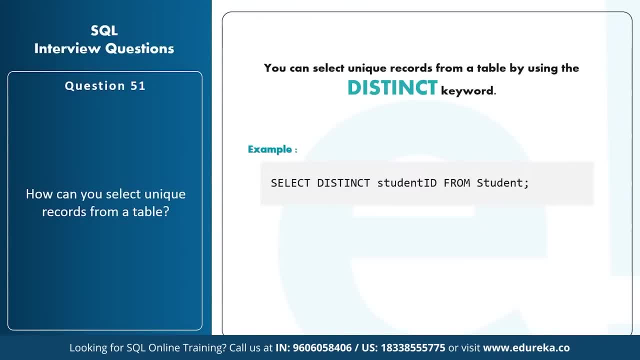 from a table by using the distinct keyword. So, for your better understanding, you can write a query, like you know, select distinct student ID from student right. So with the help of this query, all the unique records from the student table will be selected. 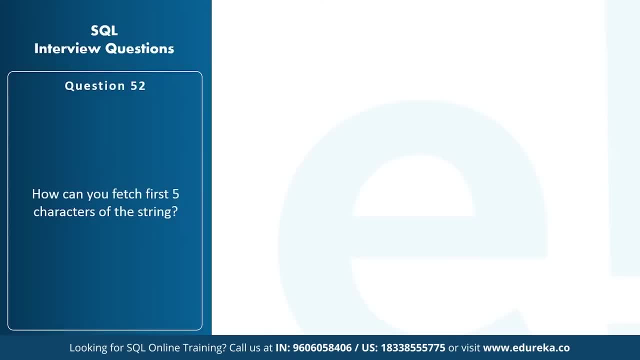 Let's move forward with the next question, That is, how can you fetch first five characters of a string? now, there are obviously a lot of ways to fetch the characters from a string, So for your understanding, I've mentioned two examples over here. that is, either you can use the substring command. 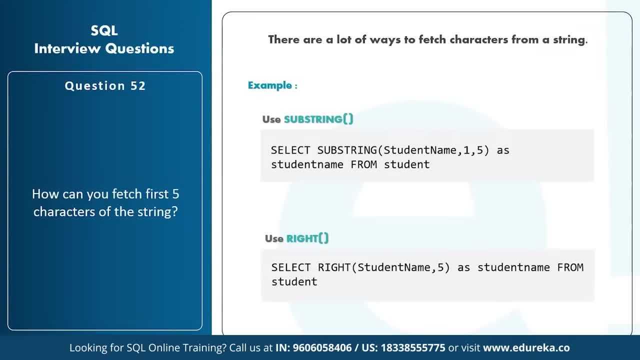 or the right. So when you use the substring statement, you can use the statements like you know. select substring. student name 1 to 5 as student name from student. the first five characters of student name will be retrieved from the student table Now. 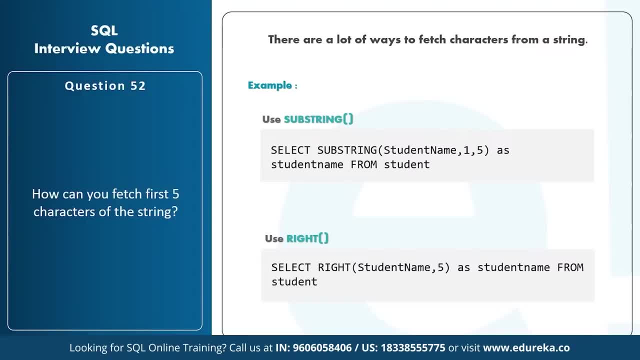 Similarly, when you use the right statement, you can use the statements like you know: select right student name, comma 5 s to the name from student Right. So with this query again, all the first five characters of each and every student name from the student table would be retrieved. 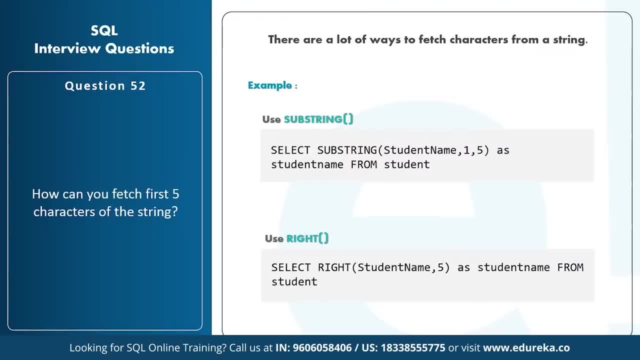 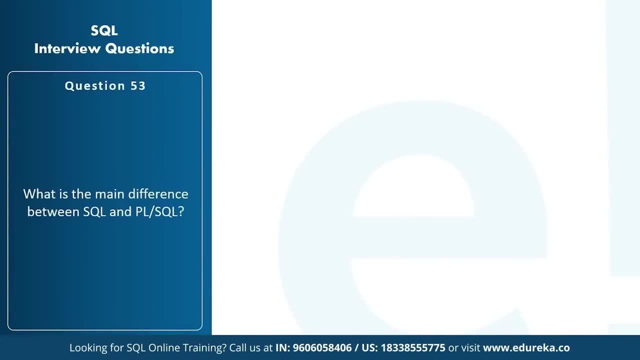 So that's how, guys, you can fetch the first five characters of a string. that is, either by using the substring statement or the right state. now let's move forward with the next question, That is, what is the main difference between sequel and PL slash, sequel, now sequel. 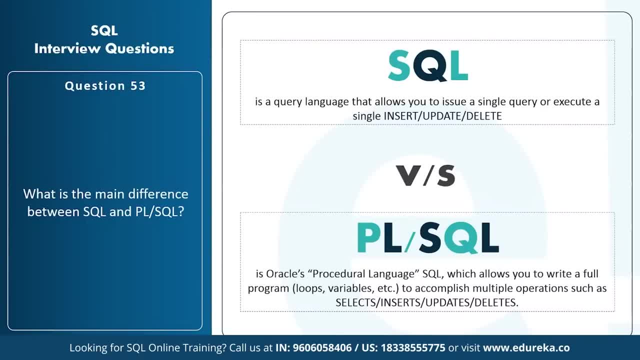 as I mentioned before, is a query language that allows you to issue a single query or execute a single insert, update, delete- Whereas PL slash sequel- that is basically oracles procedural language sequel- allows you to write a full program of loops, variables, etc. to accomplish multiple operations such as select inserts. 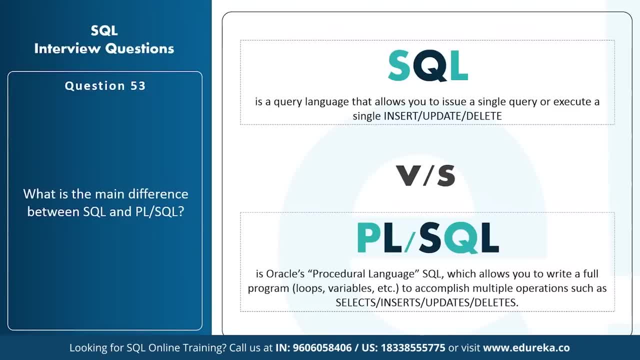 updates and deletes. So, guys, that is the main difference between sequel and procedural language sequel. in sequel You just have to write a single query to execute insert, update and delete. and in procedure of angle sequel You have to write full program with loops and variables to perform multiple operations like insert, update. 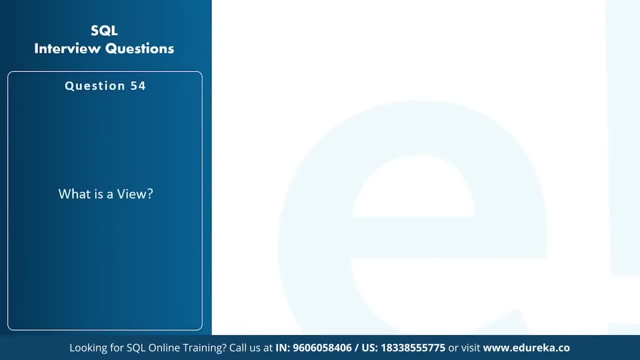 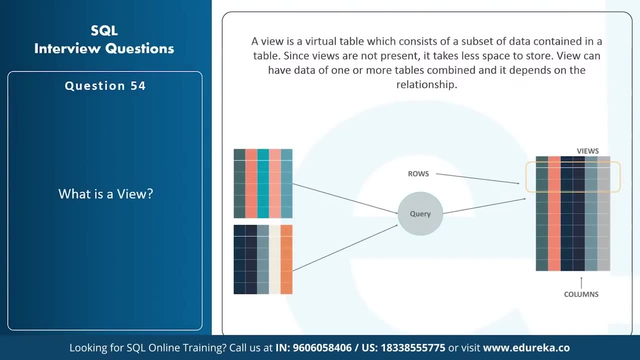 delete and selects. now let's move forward to our next question, That is, what is a view of? you is basically a virtual table which consists of a subset of data contained in a table. since views are not present, It takes less space to store. 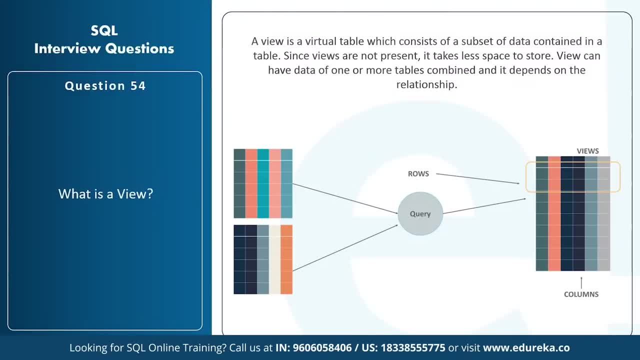 View and views can have data of one or more tables combined based on the relationship. So, as you can see on the screen, I have two tables of you know n number of rows and columns. now, once I execute a query to form a view, you can clearly see that you know. 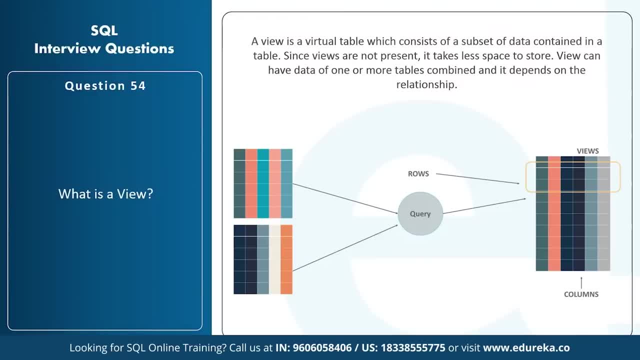 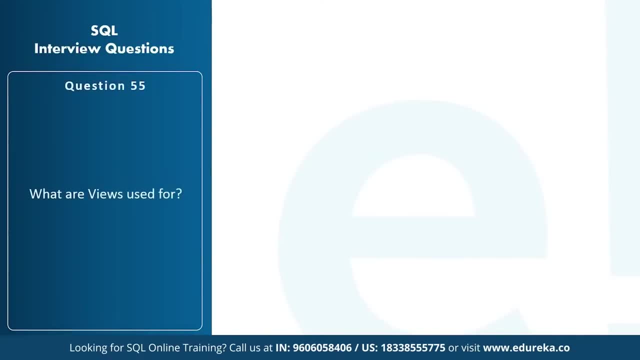 it has combined the columns and the rows from both the tables and has created a view of both of these tables into a single table. That's what a view is. now Let's move forward to the next question. That is what our views used for. so views. 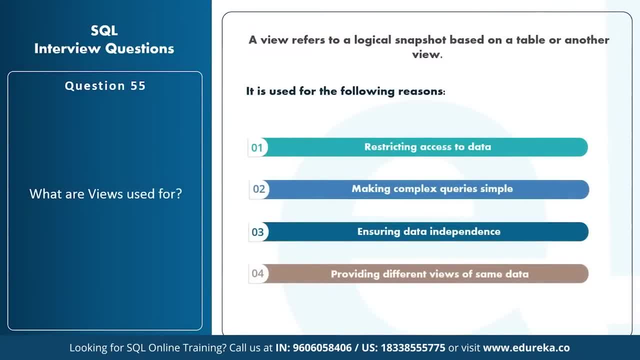 as I just explained, basically refer to a logical snapshot Based on a table or on any other view. it is used for restricting the access to data, making complex queries simple, ensuring data independence and also providing the different views of the same data. So that's what views are used for now. 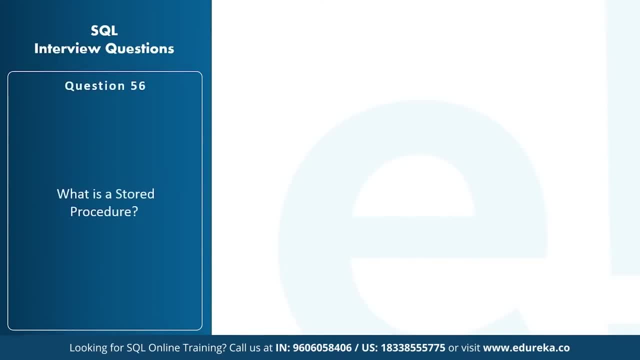 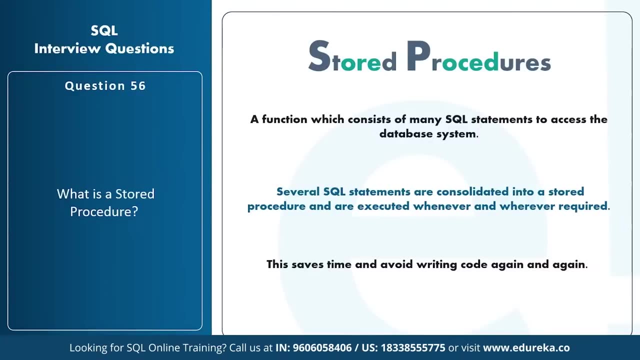 Let's move forward with the next question, That is, what is a stored procedure? a stored procedure is basically a function which consists of many SQL statements to access the database system. several SQL statements are consolidated into a stored procedure and are executed whenever and wherever required, which obviously saves time. 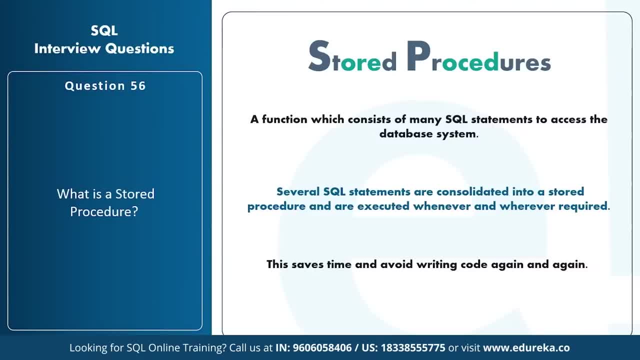 and we can avoid writing code again and again. So with the help of stored procedure, you can make sure that you know several SQL statements are executed again and again and you don't have to write the query for it again because you know you, if you just have a stored procedure, 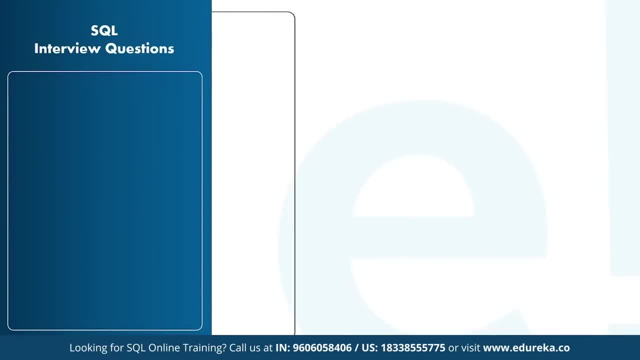 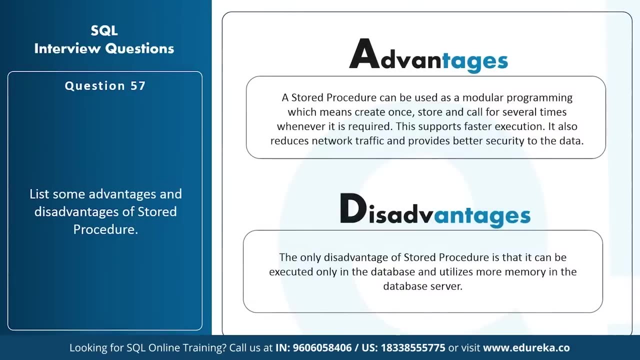 for it. it will automatically execute the queries for you. Now let's move forward with the next question, that is, list some advantages and disadvantages of stored procedure. Let's talk about the advantages first. So a stored procedure can be used as a modular programming, which means create one store. 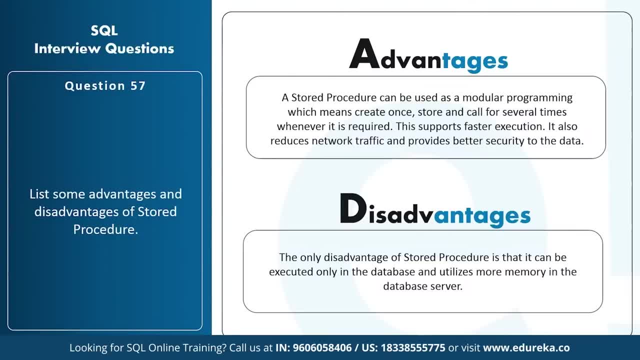 and call for several times whenever it is required. The supports faster execution and it also reduces Network traffic, which provides better security to the data. coming to the disadvantages of stored procedure, The only disadvantage of stored procedure is that it can be executed only in the database. 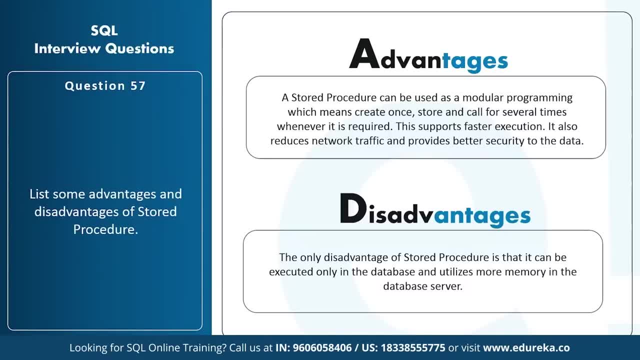 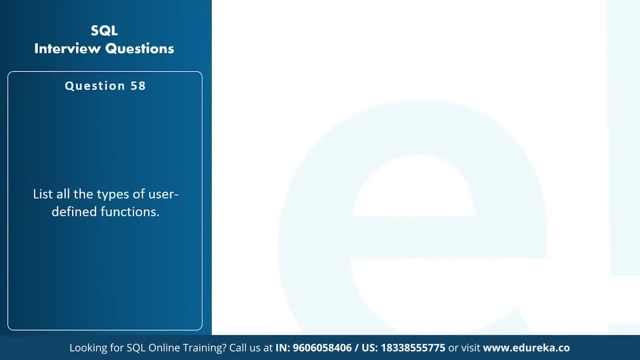 and utilizes more memory in the database server. So as that was about the advantages and disadvantages of stored procedures, Now let's move forward with the next question, That is, list all types of the user-defined functions. So there are mainly three types of user-defined functions. 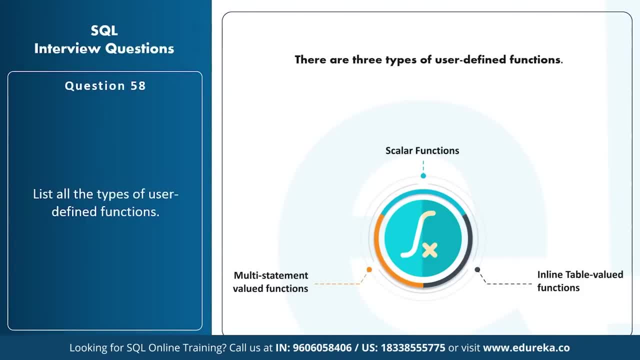 That is, the scalar function, the inline table valued functions and the multi statement valued functions. So you mainly have to mention these three functions when you're asked about the different types of user-defined functions. next, Let's move forward and understand what do you mean by collation. 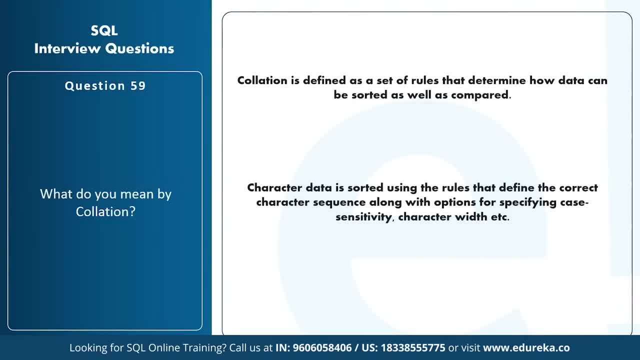 So collation is defined as a set of rules that determine how data can be sorted, as well as compared. So character data is sorted using the rules that define the correct character sequence, along with the options for specifying case sensitivity, character width and Etc. So that's what a collation is, guys. 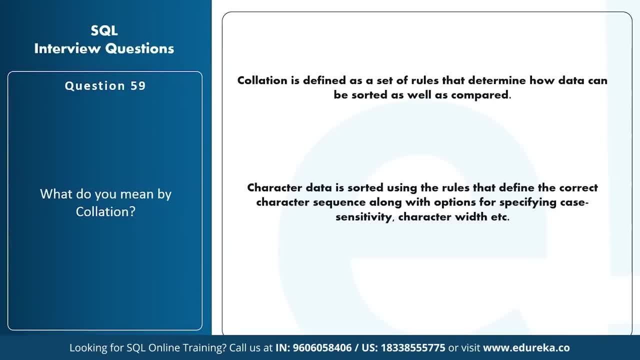 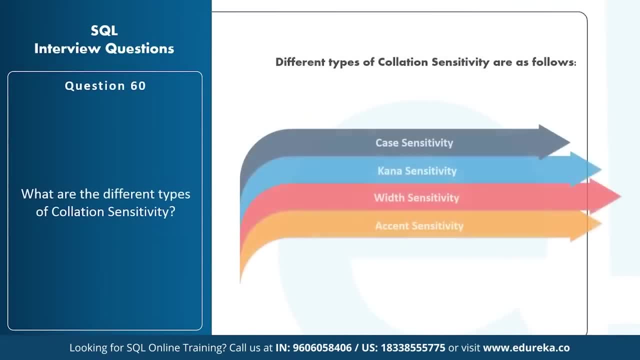 It is basically a set of rules that determine how data can be sorted as well as compared. Now let's move forward with the next question, That is, what are the different types of collation sensitivity? So the different types of collation sensitivity are: the case sensitivity, the corner sensitivity. 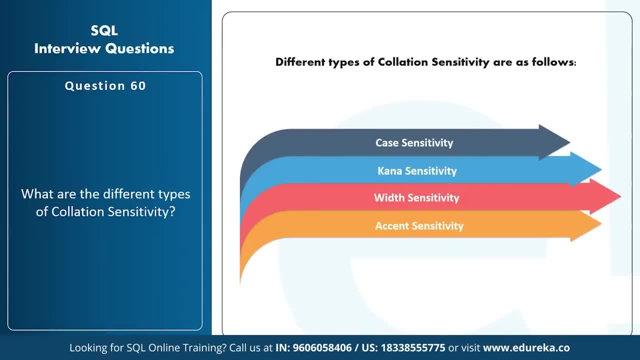 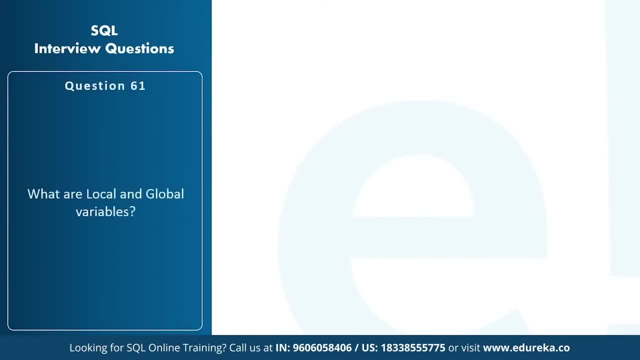 the width sensitivity and the accent sensitivity, So that these are the mainly four types of sensitivities of collation. So I hope that you've understood till now. next session, Let's understand What are the local and the global variables. now talking about local variables first. these variables can be only used. 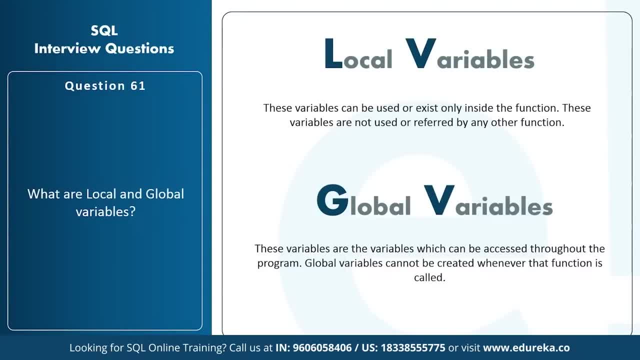 or exists only inside the function. These variables are not used or can't be referred by any other function, right? So whenever you want to use local variables, then you need to understand the fact that you know they can be only used or exists inside a single function. 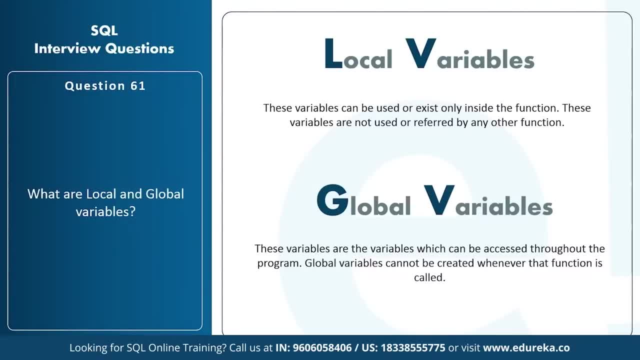 and they can't be referred by any other function. coming to global variables, These variables are the variables which can be accessed throughout the program. So global variables cannot be created whenever the function is called but, yes, they can be accessed throughout the program. 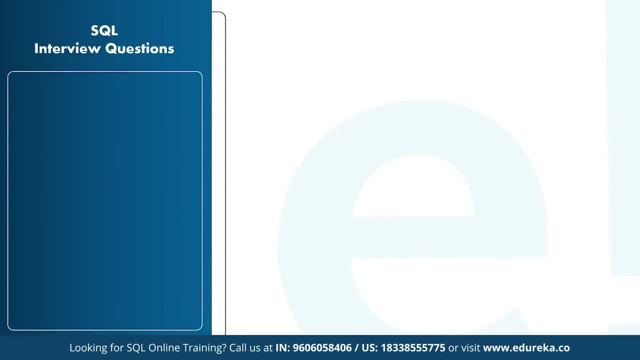 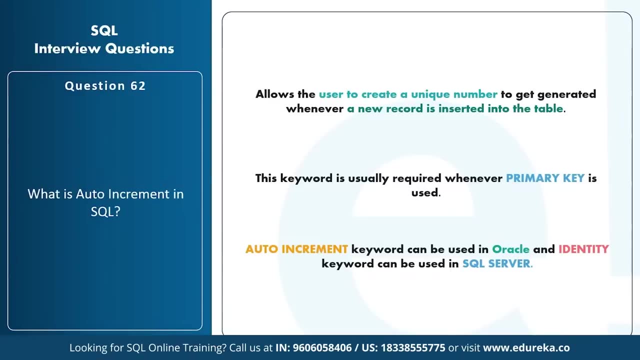 So, guys, that was about the local and the global variables. Next, Let's move forward and understand what is auto increment. in sequel, auto increment keyword allows the users to create a unique number to get generated whenever a new record is inserted into the table. So this keyword is usually required whenever primary key. 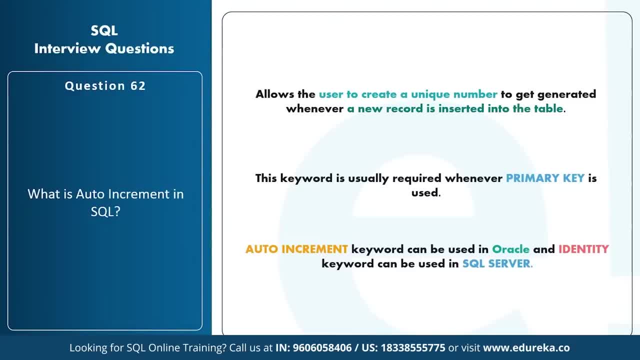 is used, and auto increment keyword can be only used in Oracle, whereas the identity keyword can be used in the sequel server. So that was about auto increment in sequel guys. next Let's understand What is a data warehouse. data warehouse refers to a central repository of data. 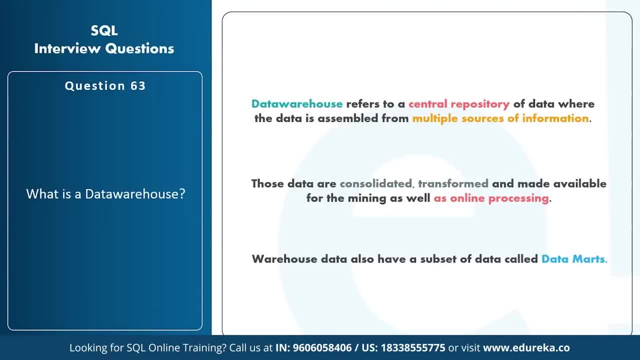 where the data is assembled from multiple sources of information, those data consolidated, transformed and made available for the mining as well as to online processing. warehouse data also has a subset of data called the data match, So data warehouse can be understood as a central repository of data. 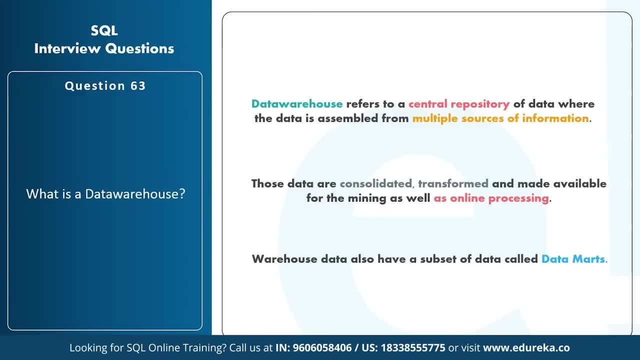 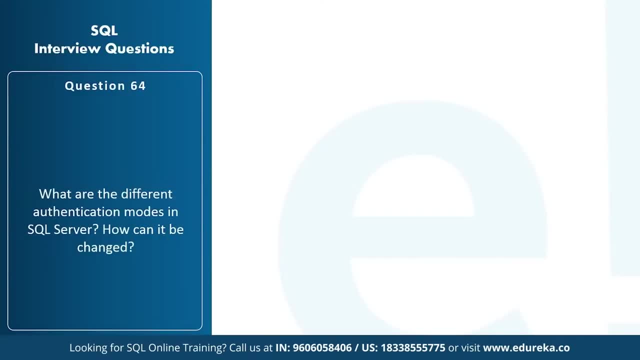 where the data is assembled from multiple sources of information. So, guys, that was about data warehouse. Now let's move forward and understand what are the different authentication modes in sequel server and how it can be changed. the different authentication modes in sequel server are basically the Windows mode. 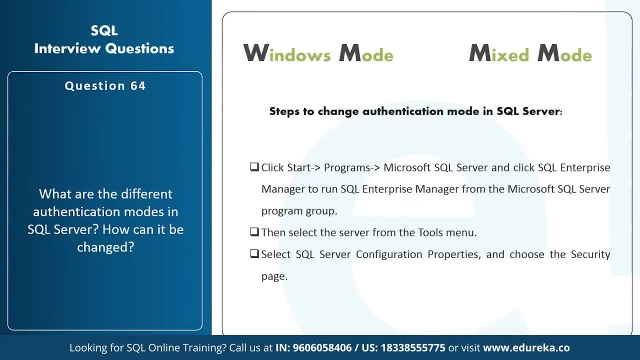 and the mixed mode. So these two modes are basically used in sequel Windows, and to change the authentication modes in sequel server, What you can simply do is you have to follow the steps that I've mentioned on the screen, that is, you have to first click on start, then go to programs. 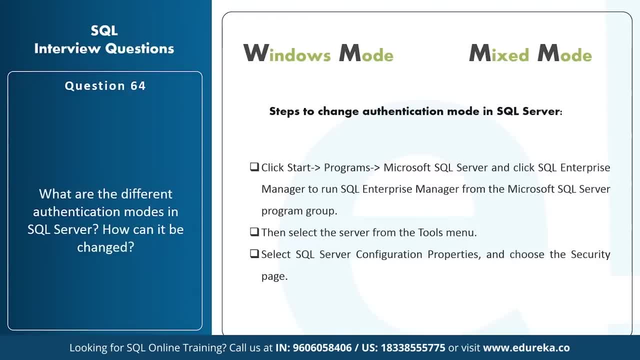 and go to the Microsoft sequel server and click sequel Enterprise Manager to run sequel Enterprise Manager from the Microsoft sequel server program group. now to change the authentication modes in the sequel server, You can follow the steps that I've mentioned on the screen, that is, you have to click on start, go to programs, go. 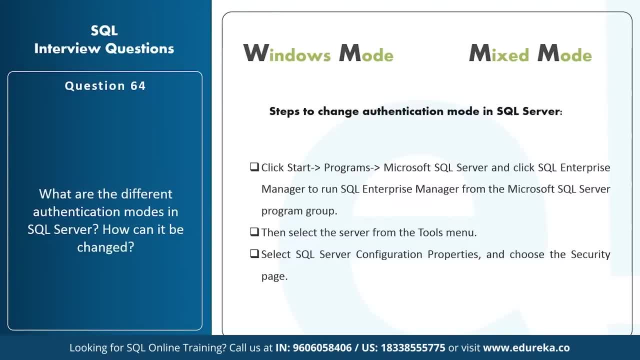 to Microsoft sequel server and click sequel Enterprise Manager to run sequel Enterprise Manager from the Microsoft sequel server program group. then select the server from the tools menu and select sequel server configuration properties and choose the security page right. So that's how you can change the authentication mode. 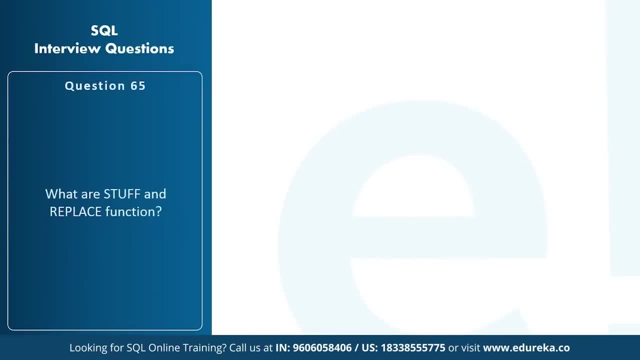 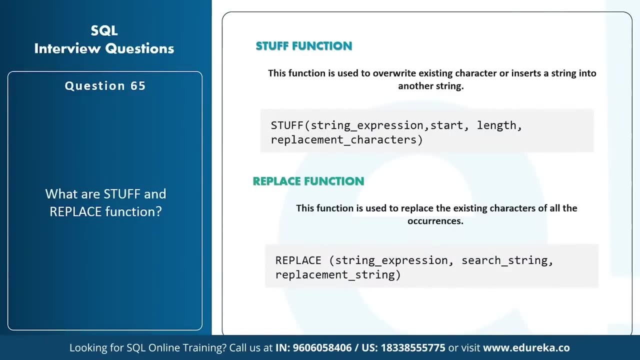 in the sequel server. guys. Now let's move forward with the final question in the session, that is, what are stuff and replace function? So talking about the stuff function first. this function is basically used to overwrite existing characters or insert a string into another string. 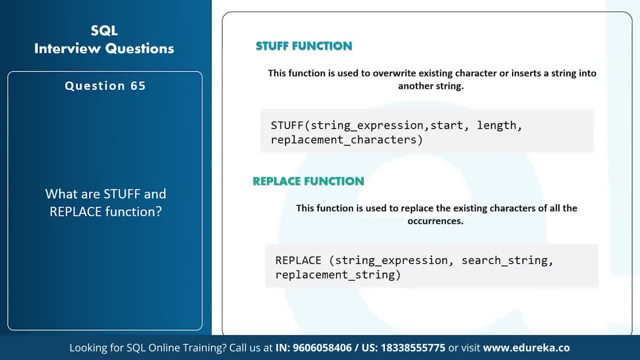 So the syntax with this function is basically stuff: string expression, start, length and replacement characters- where the string expression is basically the string that will have characters substituted. start represents the starting position, the length refers to the number of characters in the string which are substituted and the replacement string are the new characters. 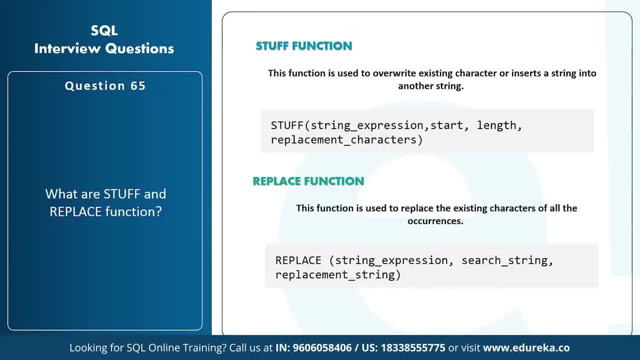 which are injected in the spring. coming to the replace function, This function is basically used to replace the existing characters of all the occurrences. So the syntax for this particular function is that: replace string expression, search string replacement string, where every search string in the string expression will be replaced. 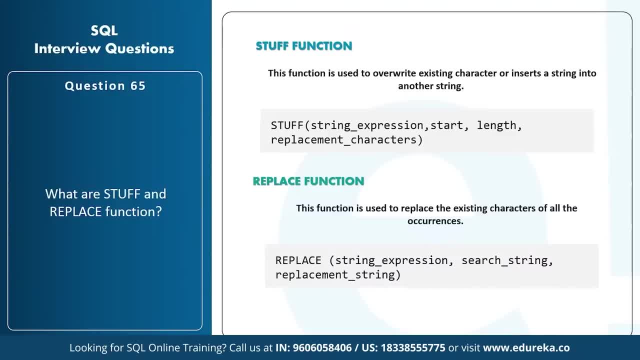 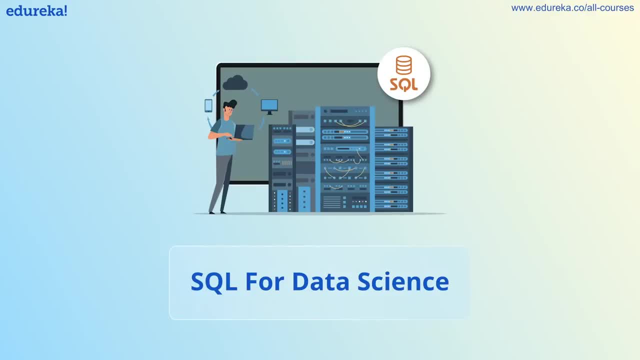 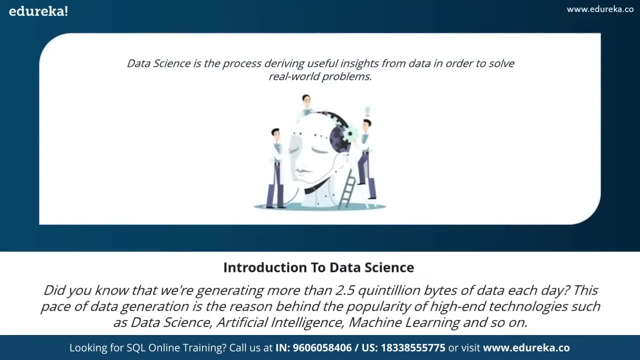 with the replacement string- I hope I'm clear- with the stop function and the replace function. So, guys, these were the questions that could be asked in your interviews. Now, what exactly is data science? now, data science, in simple terms, is the process of deriving useful insights from data in order. 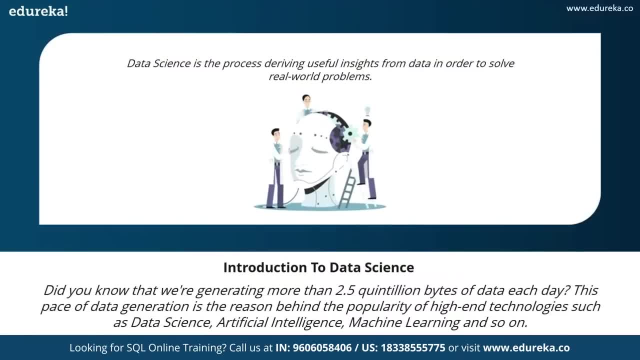 to solve real-world problems or in order to grow a business. now, data science was introduced because we are generating an immeasurable amount of data. For example, there's a fact that we're generating more than 2.5 quintillion bytes of data every day, and at this pace. 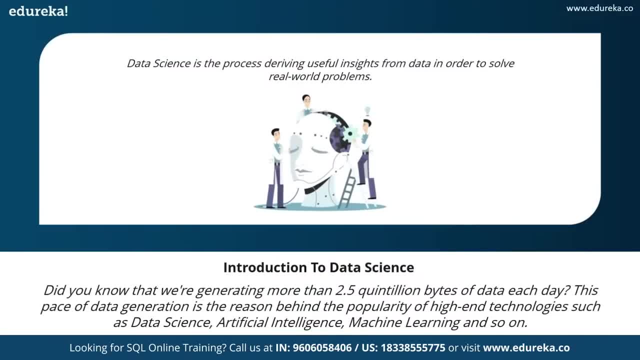 it's only going to grow because right now, everything runs on data. So the idea behind data science is to take up all this data and, you know, derive useful insights or derive knowledgeable insights from this data so that you can grow your business or you can solve a problem. 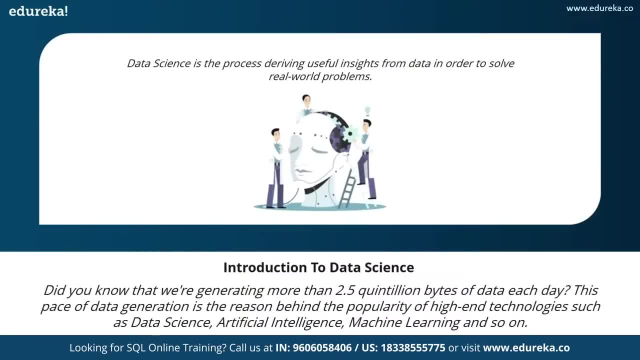 That's what data science is all about. the data is the key in data science And since we are producing so much data, is the perfect time for you to learn data science. and data science basically covers artificial intelligence, machine learning, natural language processing- all All of these processes are covered under data science. 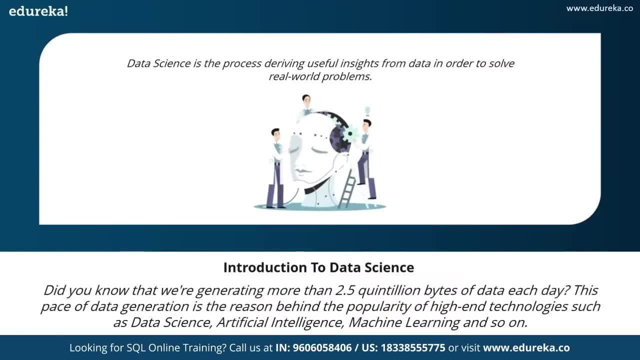 So that is one of the reasons why data science has become so popular: because of the amount of data We're generating, we need methods and Technologies that can handle so much data, and they can, you know, derive something useful from the data. So that's a small introduction to data science. 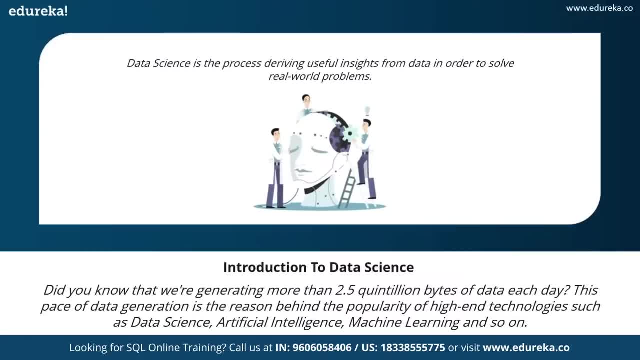 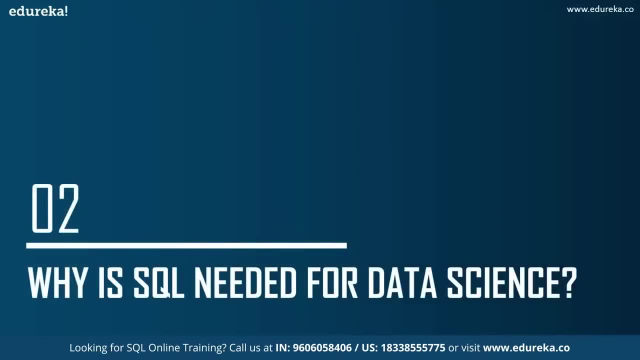 And if you guys want to learn more about data science, I'll leave a couple of links in the description box. Now let's move ahead to our topic of discussion. first, We'll understand why we need SQL for data science. So, like I said, data science is basically all about deriving. 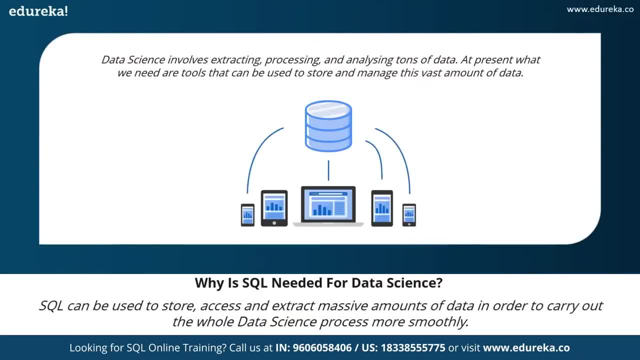 useful insights from data. data science involves extracting, processing and analyzing tons and tons of data. at present, What we need are tools that can be used to store and manage this vast amount of data. Now this is where SQL comes in. SQL can be used to store. it can. 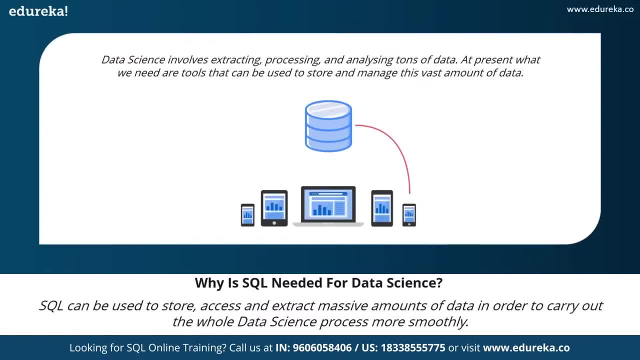 be used to access and extract massive amounts of data in order to carry out the whole data science process more smoothly. So SQL, as acquiring language, it can be used to perform a lot of querying operations, a lot of search operations, extractions and editing and modifying your 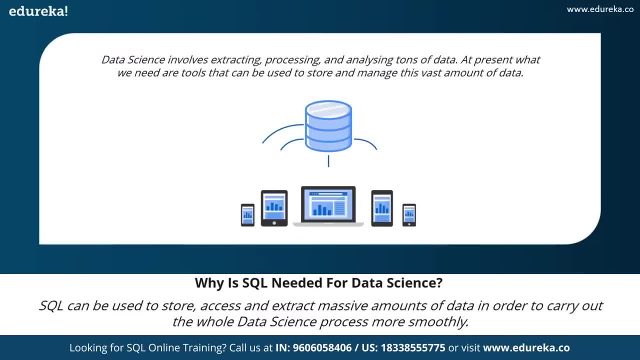 data. So we need a huge management system and, along with that, we need a language that can perform all the operations that we want to do on our data. That's where SQL comes in. So, like I said, we'll be using my SQL today, and let's understand why I've. 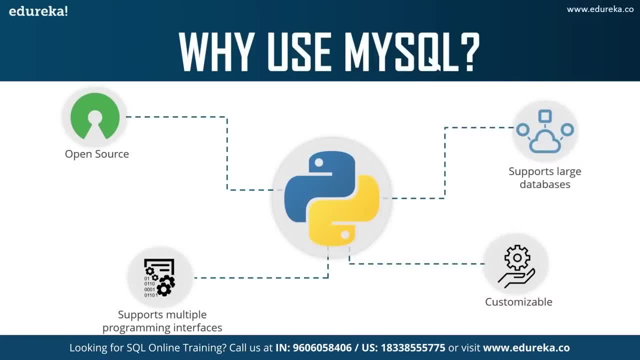 chosen my SQL now. First of all, my SQL is very easy to use. You have to get only the basic knowledge of SQL right. You can build and interact with my SQL with just a few simple SQL statements. right, and SQL statements are quite easy. 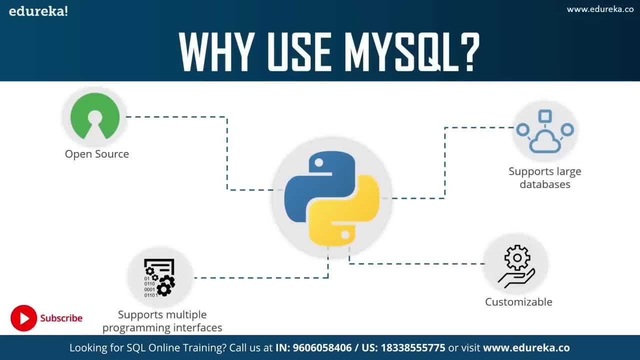 Like they're a lot like your English language. I feel like it's the most basic and the most understandable language There is querying language. apart from this, It is also very secure. actually, my skill consists of, you can see, a solid data security layer. 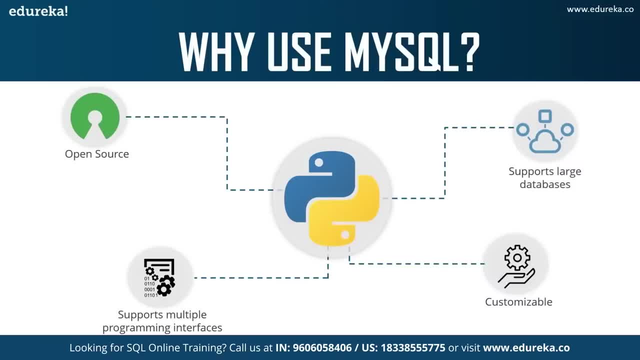 which will protect all of your sensitive data, or your confidential data from any intruders. passwords are encrypted in my SQL, So that's a good advantage of using my SQL. apart from that, of course, it's open source, So it's free to download and to use. you can just go to the. 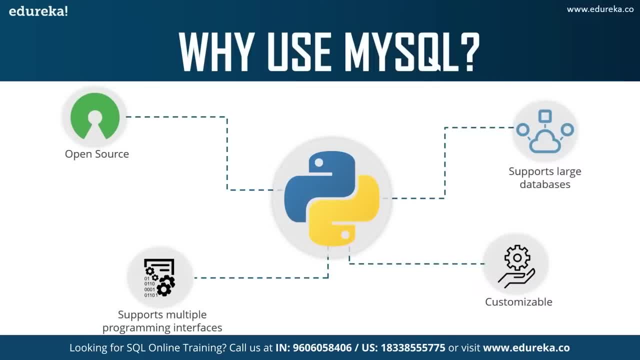 official website and download it in a matter of minutes. Then, of course, it is scalable as well. right, It can handle almost any amount of data. right, It supports large databases, up to as much as 50 million rows. Those are more right. 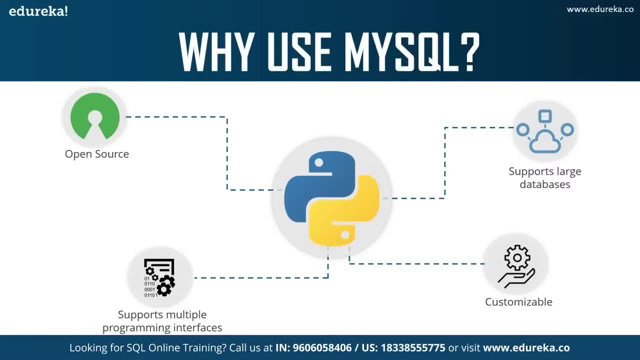 That's the amount of data that you can store in my SQL, and the default size limit is about 4 GB, if I'm not wrong, and you can also increase this number to a theoretical limit of around 8 TB of data. I think you'll have to pay a little bit of money for that. 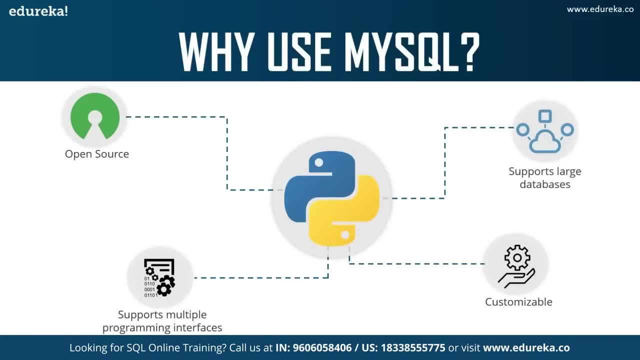 But I feel like 4 GB is a lot, first of all, to have a data set of that sites. Then another important point is that my SQL follows a client server architecture. So this is where you basically have your data Based server, which is your MySQL, and you have many applications and programs. 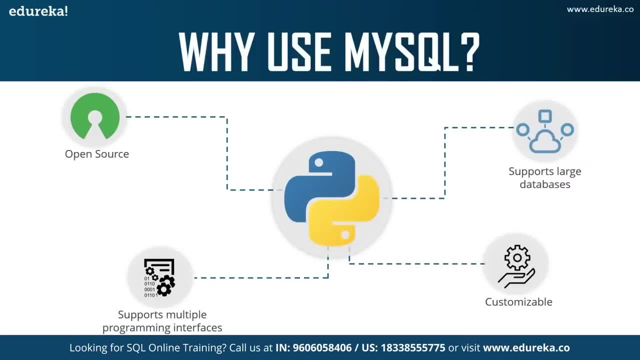 as your clients, right, and these communicate with the server. This is where they query data, They save changes, the update the data, and all of that, Not only this. MySQL is compatible on many operating systems. It is easy to run on a lot of operating systems, such as. 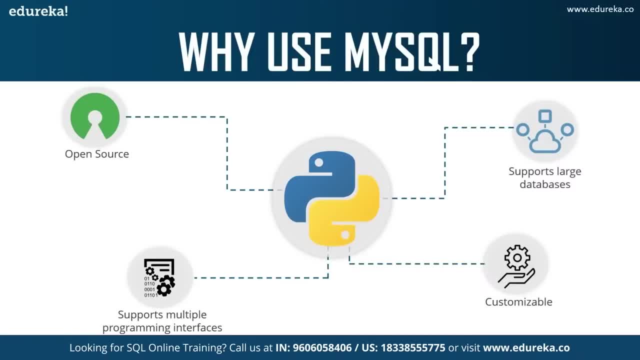 Windows, Linux, Unix and so on. Now MySQL actually provides a functionality that the clients can run on the same computer As a server, or they can even run on another computer. So basically, communication via a local network or the internet. Another important point is that they are quite a number of. 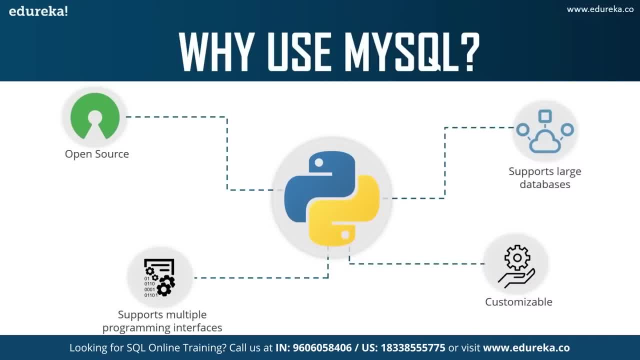 api's and libraries for the development of MySQL applications. So basically, it has support for multiple programming interfaces, right, So client programming. you can use languages like C, C++, Java, Pearl, PHP, Python and so on, and all these languages are easily compatible. They provide api's so that you can integrate and you can 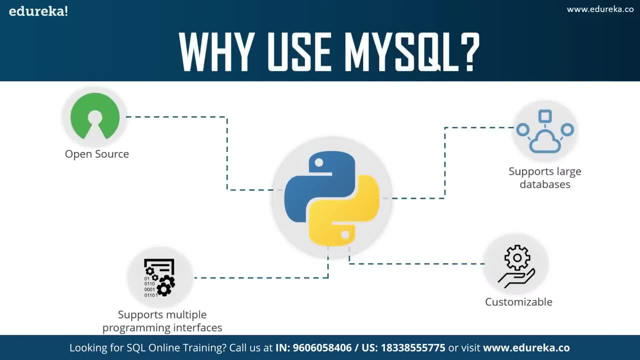 perform or you can build applications using these languages. and since python is one of the best languages for data science, MySQL is perfect for data analysis, storing data and querying data. You can easily work with MySQL and python to build applications and query data, and all of that right apart from that. 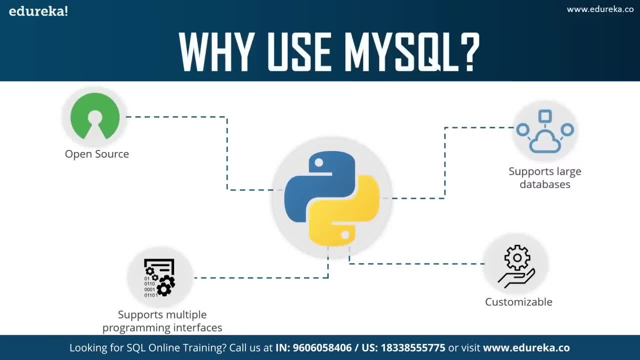 It is also customizable, like I said, and it's also platform independent. right, It's not only your client applications that can run under a variety of operating system, but MySQL itself can be executed under a number of operating systems. The most important ones are your Mac operating systems, Linux. 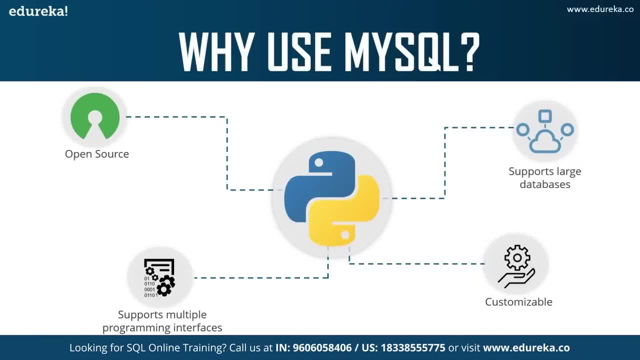 Microsoft Windows and so on. apart from that, We also have speed right. MySQL is considered a very fast database program and this speed is actually being backed up by a large number of benchmark tests. and apart from that, it's highly productive because it uses triggers, It uses stored. 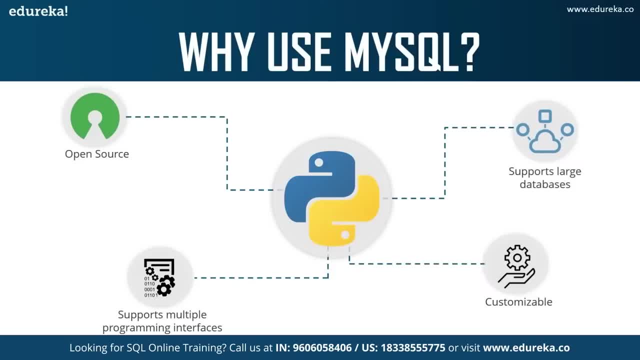 Seizures and views, and this basically allows the developer to give a higher productivity. So these are a few reasons why you should go with MySQL right. I feel it's one of the most easiest to use and it's one of the most compatible databases that are there now. 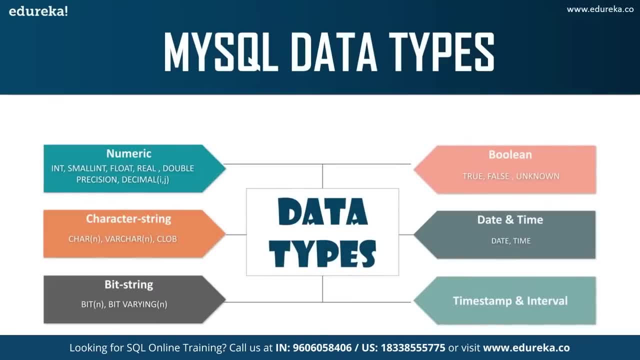 Let's move on and discuss a couple of basics about MySQL. So we'll discuss the data types which come under MySQL. We have numeric, we have character string, We have bit string, boolean, date and time and timestamp and interval It under numeric. it includes integers of various sizes. 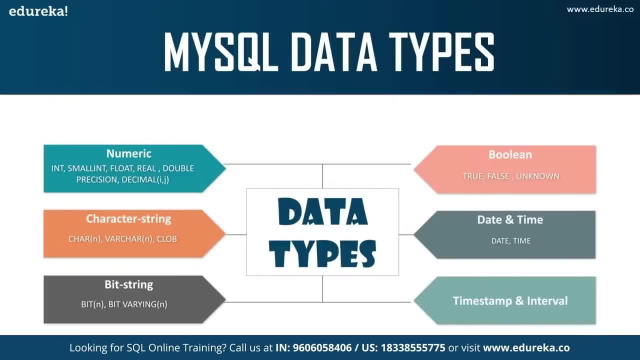 There is a floating point of various Precision's and formatted numbers under character strings. These data types either have a fixed or they have a varying number of characters. Now this data type also has a variable length string, which is called character large object, which is used to specify columns. 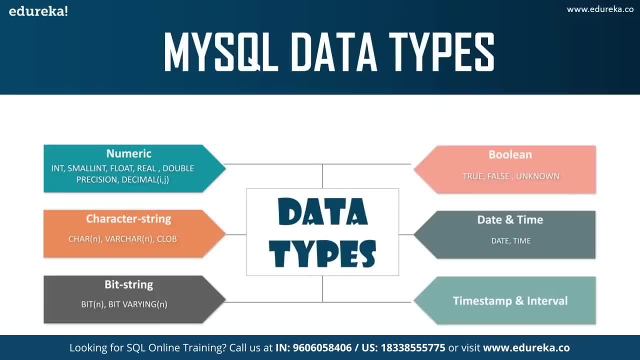 that have large text values, So it supports large text values as well. Apart from that, there is bit string. Now these data types are either of a fixed length or varying length of bits. Now there is also a variable length bit string data type. 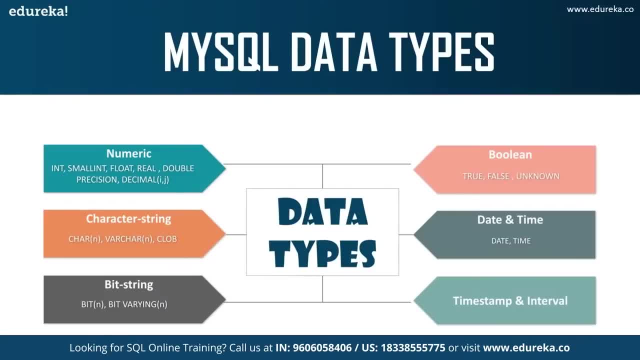 which is called binary large object. Now, this is available to specify columns that have very large binary values, such, as you know, maybe images and so on. then we have the boolean data type. now, this data type, as the name suggests itself, It has true or false values and since SQL has null values, 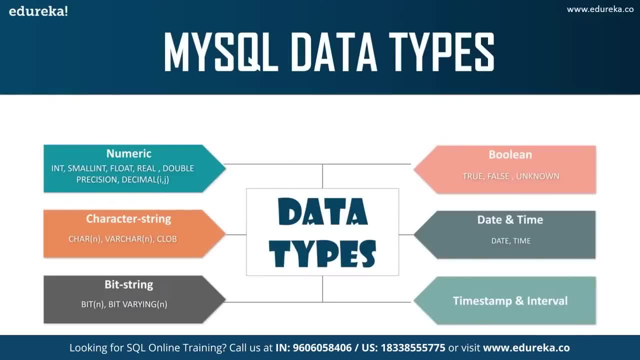 A three-valued logic is used, which is unknown. That's the third value. then we have date and time. So the date and time is like any other date variable. the date data type has your month and day in the normal date form and similarly, the time data type has components like our minute. 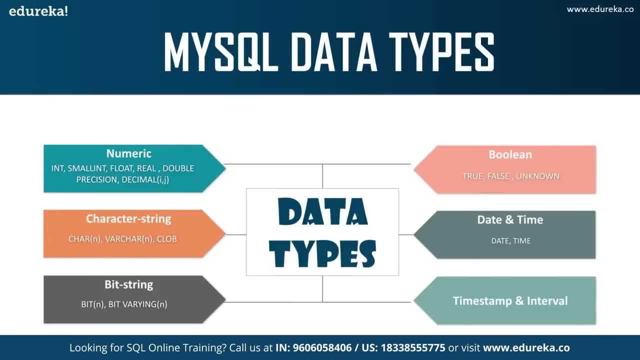 and second. now, obviously, these formats can be changed based on your requirement. next, We have the timestamp and interval data type. So the timestamp data type includes a minimum of three of six positions for decimal fractions of seconds and an optional with time zone qualifier in addition to your date. 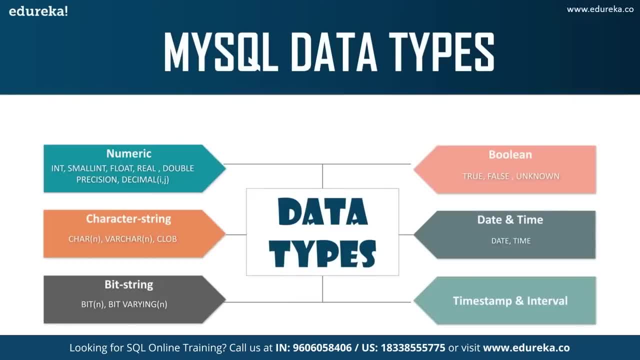 and time fields. So the interval data type will basically mention a relative value that can later be used to increment or, you know, decrement an absolute value of time or date or any of that sort, or basically a timestamp right, so you can increment or decrement any absolute value using the interval data type. 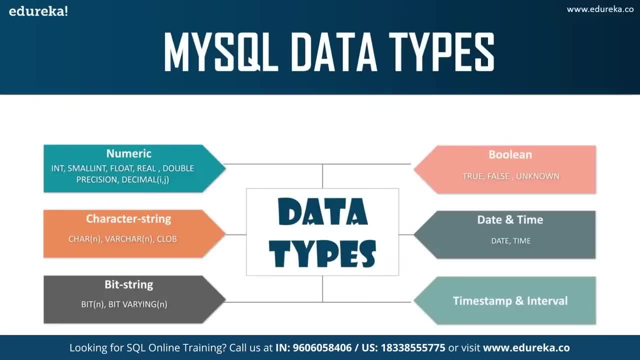 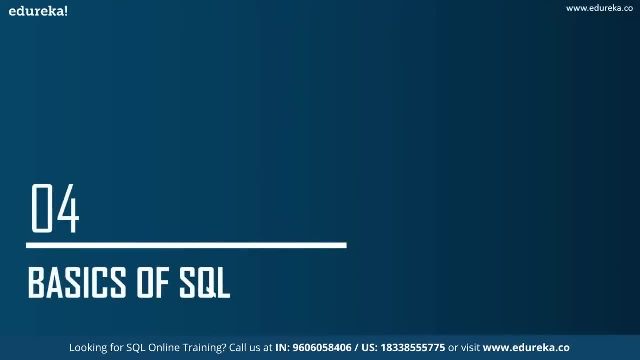 So, guys, this was a little bit information about the different data types that are there. now Let's discuss a little bit of basics of SQL. Like I said, I'm just going to brush up a couple of topics because I'm hoping that you all have a good understanding of. 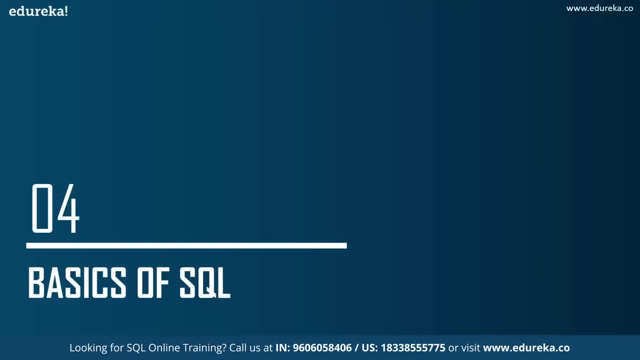 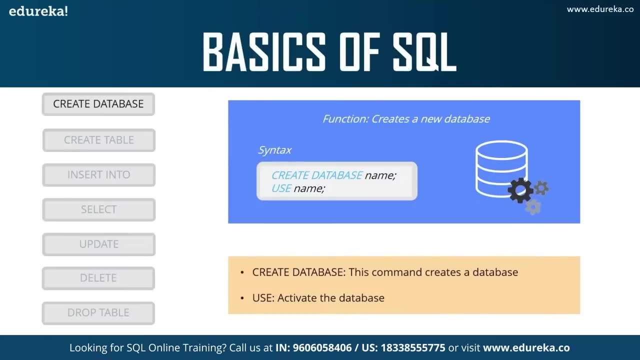 the querying language. So let's just brush up a little bit. So first of all, we have the first command, which is create database, and this is a very general-purpose command right. It basically creates a new database for you. So the syntax is just create database and the name of your. 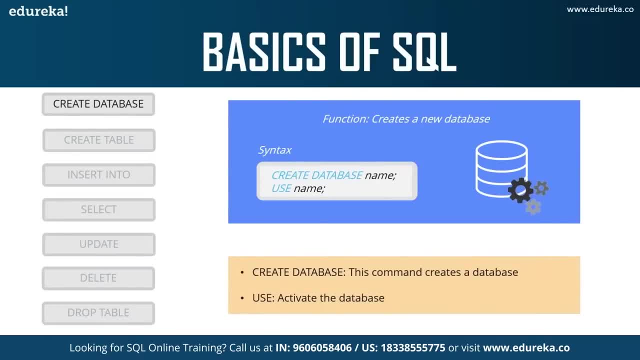 database. Then, once you create it, in order to initialize and use it, you just use the command use and the name of the database that you created. and remember that at the end of each command you have a terminator, which is a semicolon, and also your commands are usually written in capital letters so that you 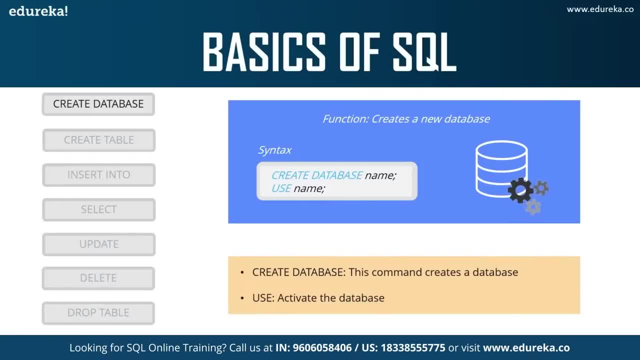 can differentiate your commands from your table columns or table names and all of that, So it's a good practice If you write all your commands in capital letters. next we have create table. now tables are the most important part of a database, right? So create table is a simple command that will create a new 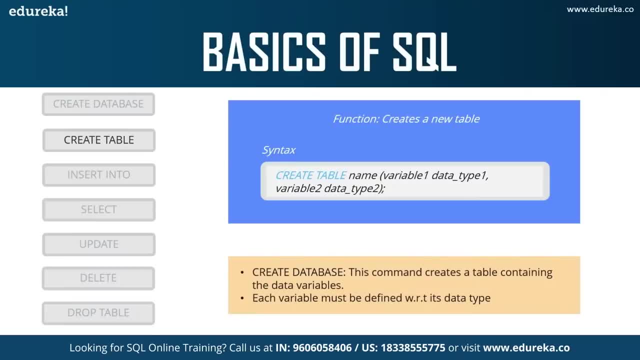 table for you, and it can contain a lot of data variables of different data types, and so the syntax is simple. The command is create table, the name of the table you want to create, and then, within the table, whatever variables you want, you can mention the name of the variables with their. 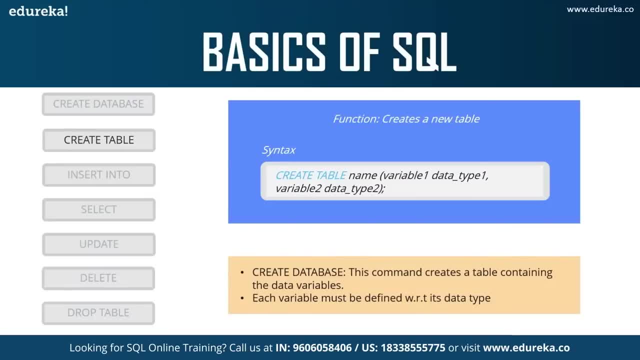 respective data types, like, for example, if your variable is age, then your data type will be an integer or something like that. Similarly, you can add another variable like name, and you can have the data type as a character. So it's as simple as that. 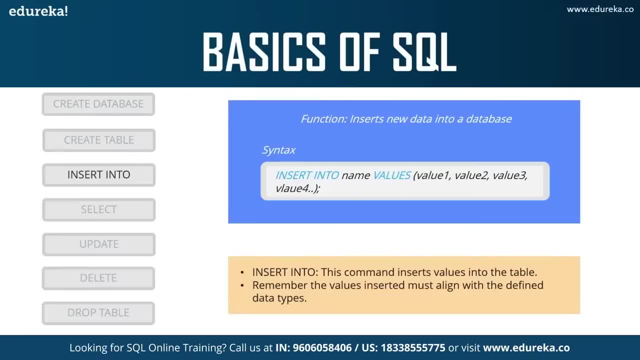 It's very understandable, the language. and then let's talk about insert into. now this command is used to insert new data into your table. Now, usually what happens is when people insert values into the table, they forget the data type that they've defined under that particular variable. 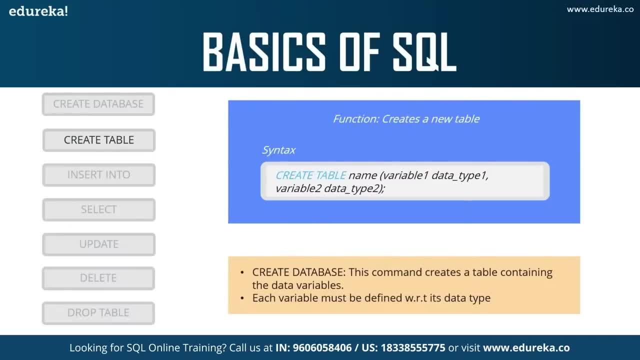 So remember that the values that are inserted must align with the defined data types. So, for example, if your variable is age and instead of putting your numerical three you've put your character three, basically you've typed out thre, and that's not going to work because you already 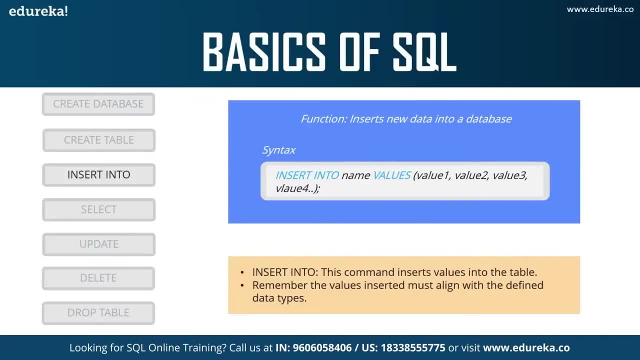 defined your age variable as integer, So you'll get an error there. So make sure that the values that you're inserting into your variable are the same data type as you've defined your variable as okay. So make sure that happens, and these are very simple things. 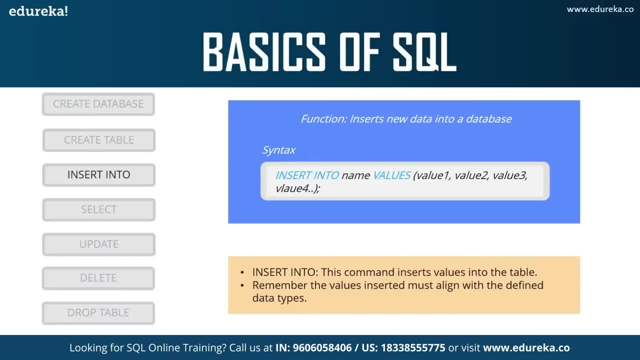 guys, I'm sure you guys are aware of this. now Let's look at our next command, Which is select. so this is one of the most important commands when it comes to SQL, for data science and because mainly it's all about extracting useful insights and extracting particular 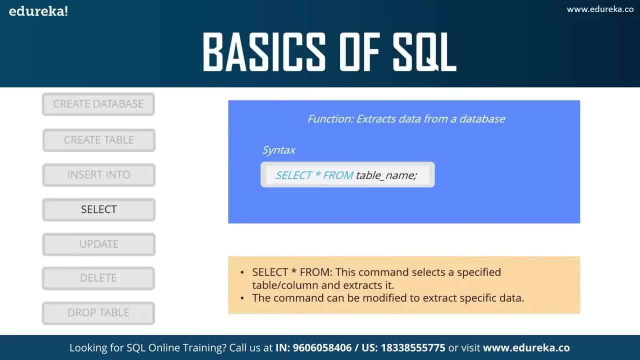 type of data from your database and we'll see how often we'll use this command when we perform our demo today. This is one of the most simplest and, in fact, it's one of the most important commands in SQL. Okay, so, basically, select will select a specified table. 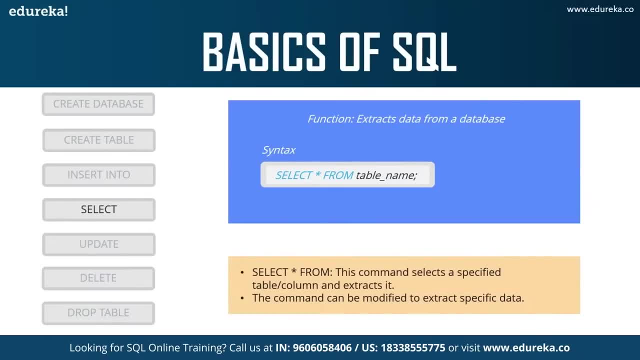 or a column and it will extract the values from it. Okay, so select star from and table name is your syntax. Now we'll be using this in the demo, So don't worry if you do not know exactly what this does. Just remember that your select command is for extracting data. 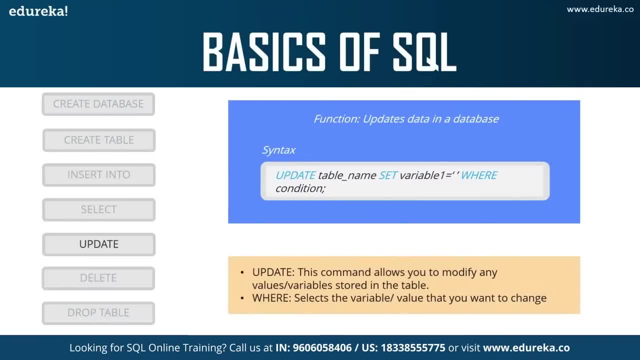 from your table. Next we have the update command. So update will basically allow you to modify any values that are stored in your table, and the where clause here will select the variable or value that you want to change. So it's basically: it will highlight the variable or the. 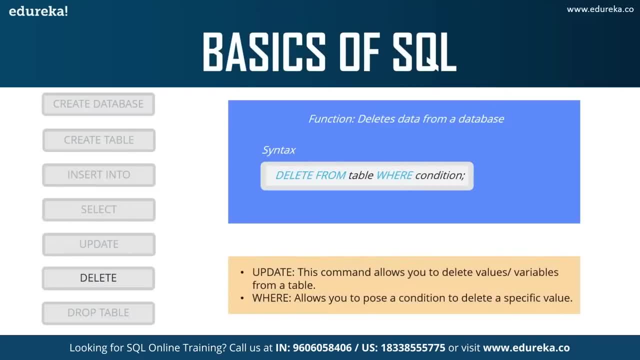 value, or I'll try to identify the value that you want to change. next, We have the delete command. now delete will basically delete data from your data set or from your table, as the name itself suggests. So delete from the name of your table and where, with the? 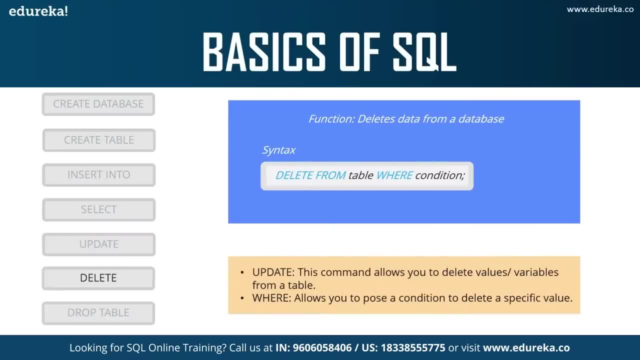 condition. it's as simple as that. next, we have a drop table. So this command is basically used to delete a table and all the rows in the table. So your table will get deleted from your table, From your database. That's what happens with drop table. 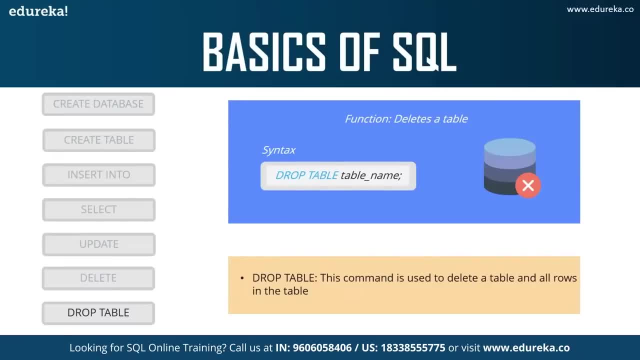 These were a couple of commands that I thought you should brush up on. I'm sure you guys are already aware of these commands, but in case there are a few few who don't know much about SQL, I'll leave a couple of links in the description box. 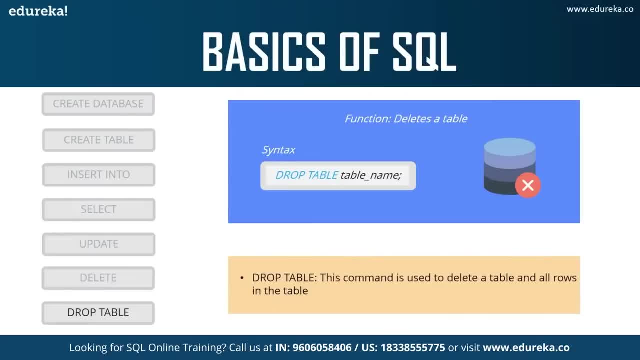 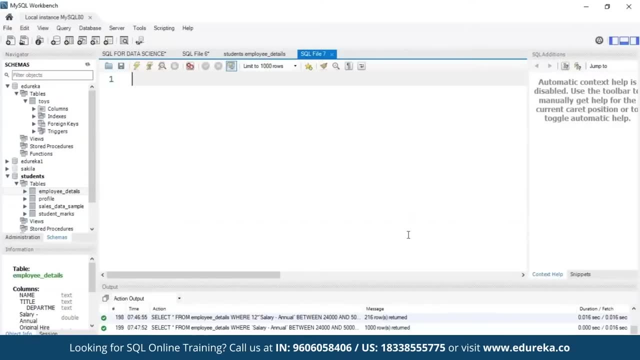 You can go through those videos and then maybe come back to this if you're specifically looking for SQL for data science. Now let's get started with our demo, which is quite interesting. So, guys, with this demo, I'll be using the MySQL workbench. 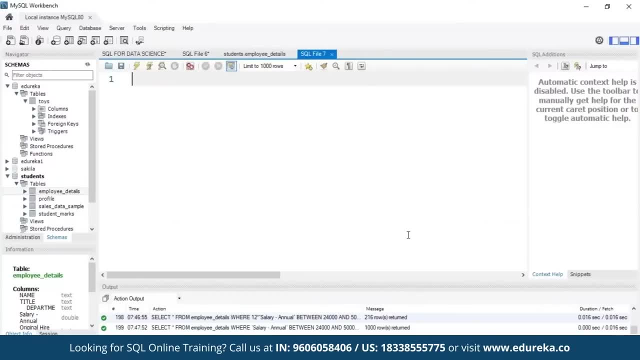 So it's quite easy to install. It'll just take like 15 to 20 minutes. I'll leave a link in the description box. We have a short video where in we're showing you how to install the whole workbench. So once you've installed MySQL, we'll start by creating a database. 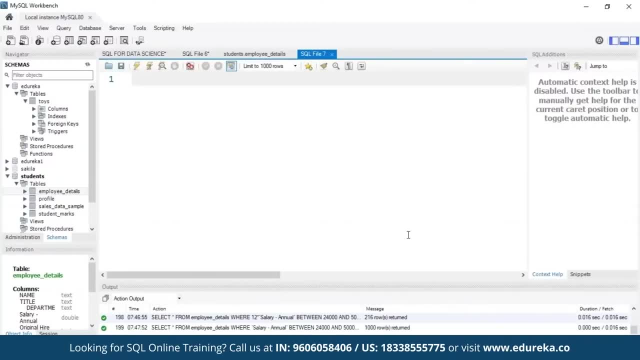 and we'll import a data set into our workbench. So I'm going to import a existing data set. right, I'm doing this because we are doing a more advanced tutorial. This is not about creating tables and, you know, extracting values from tables. 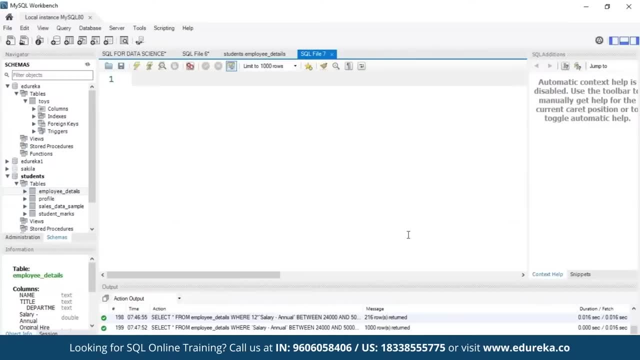 Instead, This is about deriving useful insight from your data. So usually for data science you don't have to sit down and create tables and you know, do those basic commands and said you have to explore the data variables. So usually there's a humongous data set that needs to be explored. 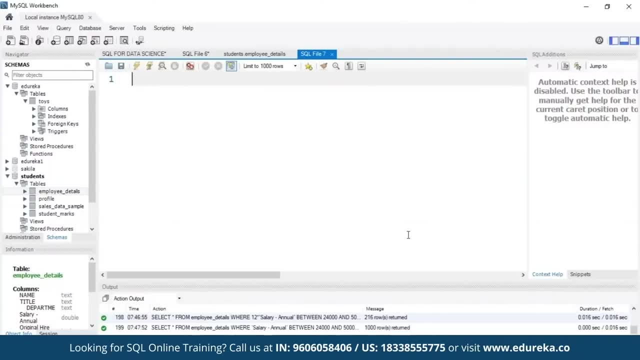 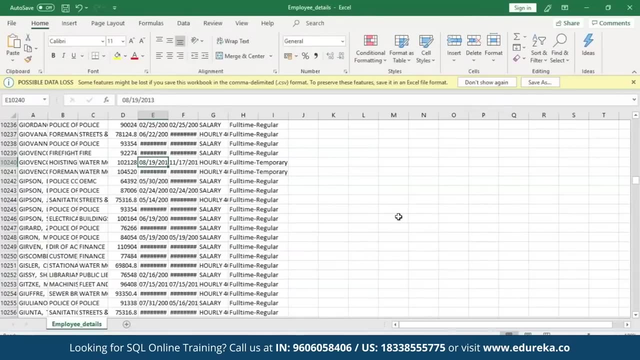 and analyzed in order to derive something useful from it, And so that's what we're going to do today. So I've already imported a CSV file. Let me show you what the file looks like. That's what this is, our CSV file, and this basically contains: 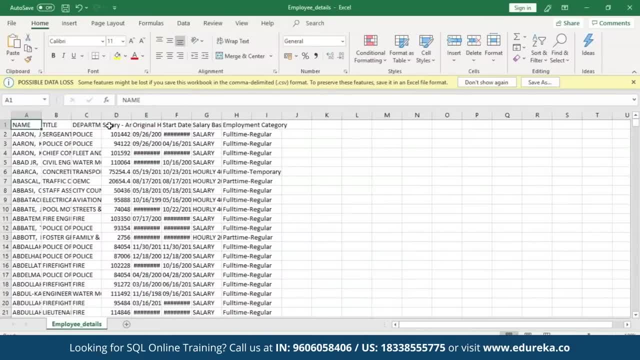 details about employees. So basically, the name of the employee title is the job title of the employee Department, is the department that the employees working in. then we have the animal salary, We have the hiring date, We have the start date in the present position. 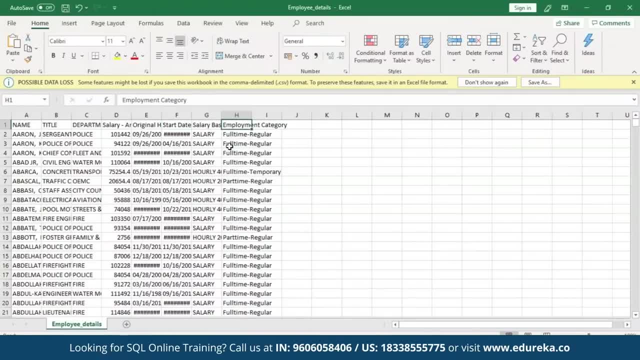 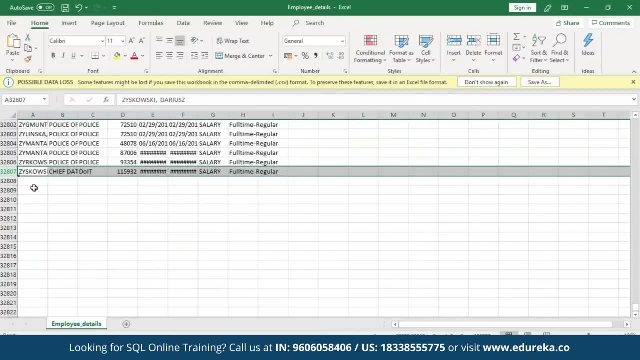 We have the salary and we have the employment category- whether your full-time employee or whether your part-time employee. So our data set has around 32,000 observations, right? So this is a very huge Data set and I basically downloaded from the internet. 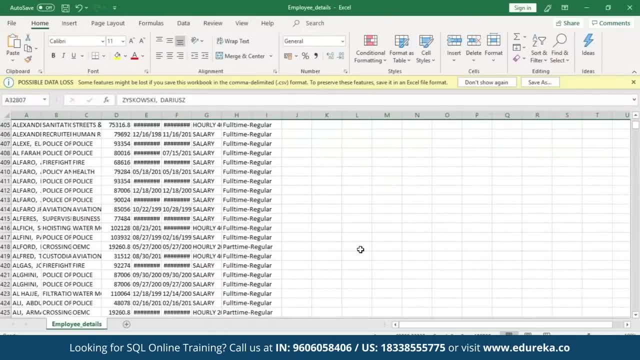 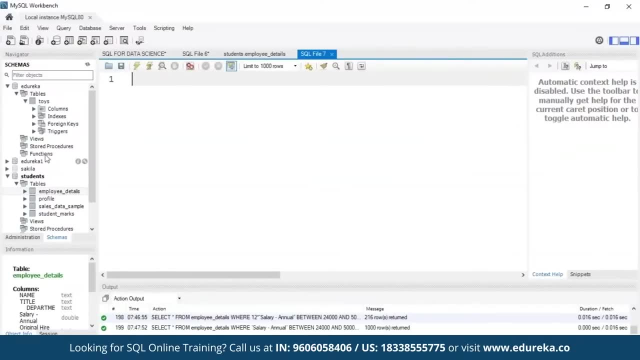 You can find a lot of data sets on the internet and you can perform all of the data analysis in no time. So if you don't know how to import a data set in your, my SQL workbench quickly show you how it's done. So I've already created a database here, now creating a 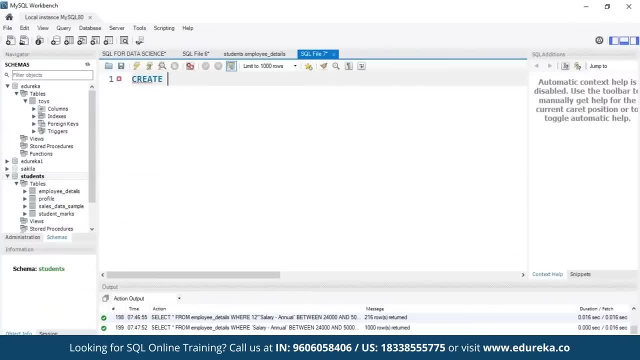 database is as simple as this. right, You just have to do create Database and name of the database- Let's say tutorial, And then if you want to use it, you just use the command use tutorial. It's a basically tutorial database gets activated. 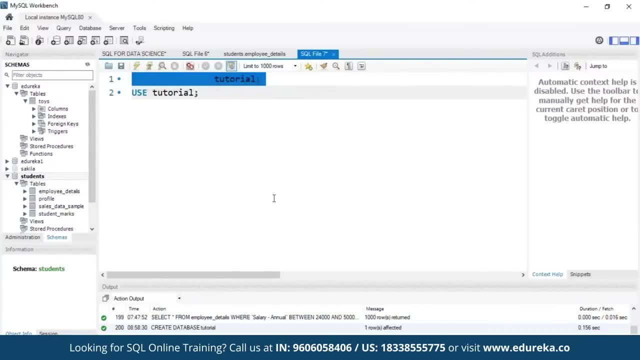 Now all you have to do to run is you have to use this right use tutorial. So we've basically activated our database. now for this tutorial. I've already created a database, So I'm going to use that database itself. Name of my database is students. 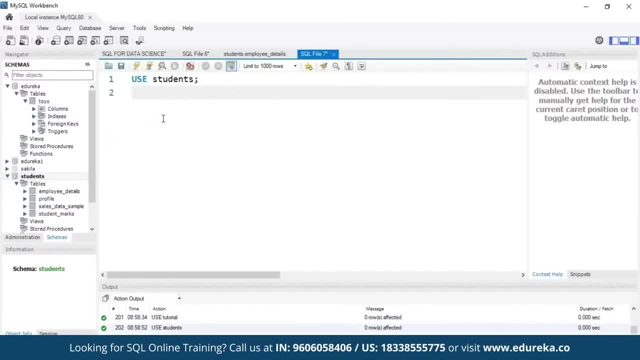 And so let's activate this database right now. in this I have a couple of tables and we are going to be focusing on this table: employee details. So this is the table that I imported. so, guys, for those of you who don't know how to import a CSV file into your my 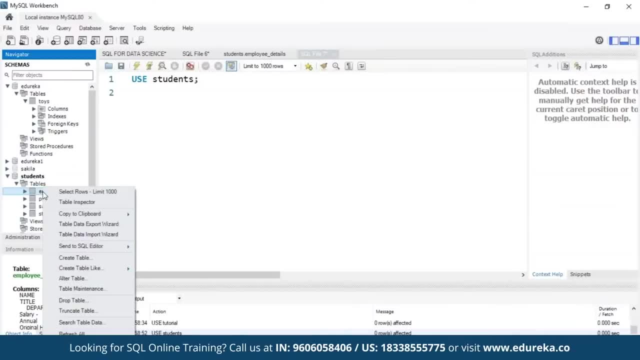 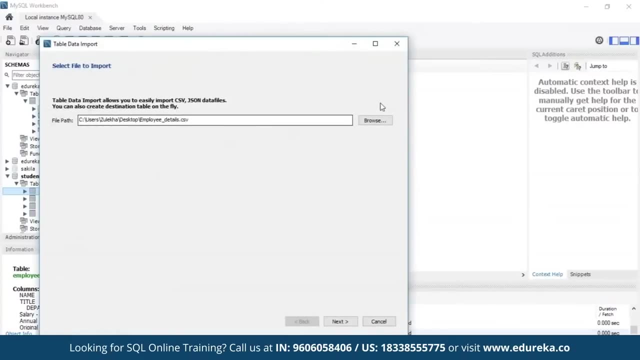 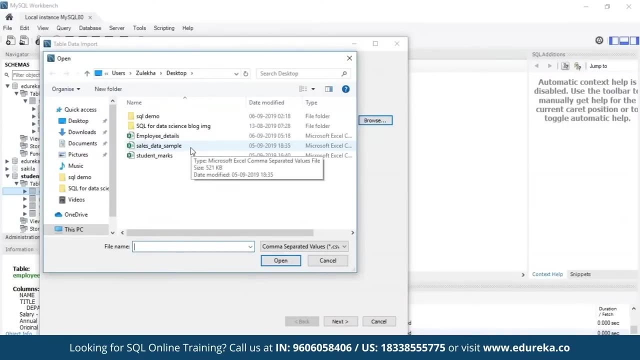 SQL workbench. All you have to do is go to tables. right click on any table and go to table data import wizard. Right click on this and browse for your SQL workbench, Your CSV file. Okay, just to take an example, I'll consider this CSV file. 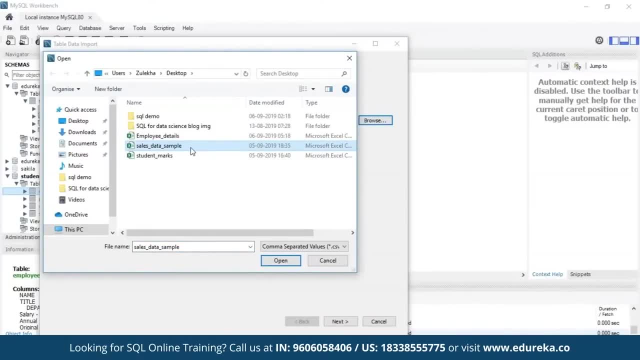 I'm not going to import the CSV file that we're going to be using right now, because that is a very, very huge CSV file and it'll take a lot of time for me to import that CSV file into the workbench to save up on some time. 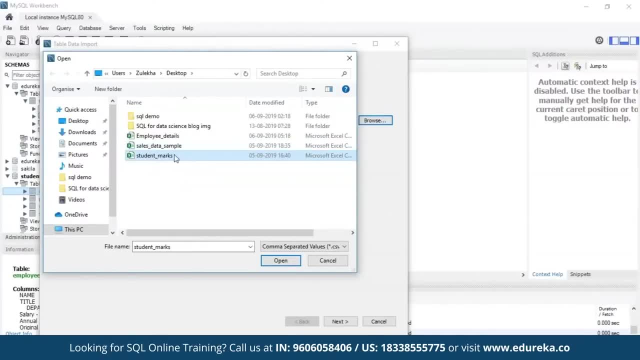 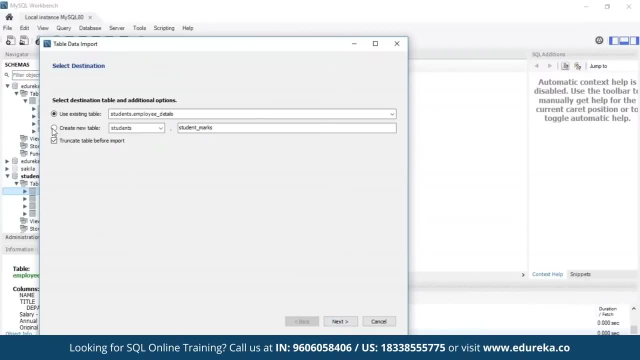 I'll import a small CSV file and I'll show you all right. So I'm selecting this file. students marks. Let's open it Right and go to next. After that, create a new table, a. basically, what you're doing here is you're going to create a new table that corresponds. 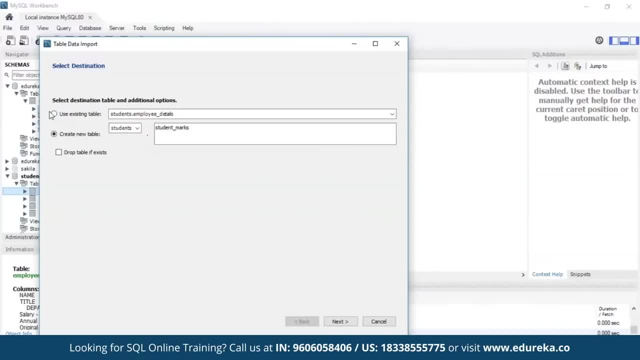 to all the columns that are there in your CSV file. either you can create a table on your own and click on use existing table, or you can allow my SQL workbench itself to create a new table for you. That's what I'm going to do, because obviously it's simpler. 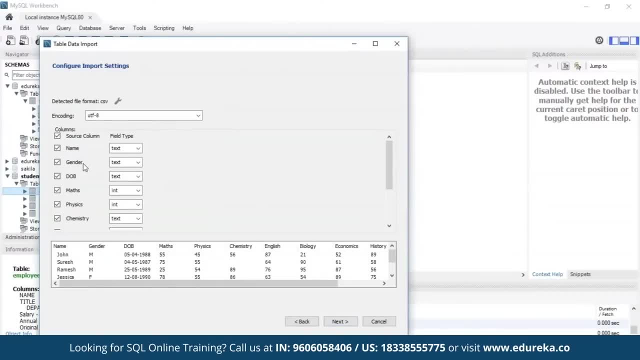 then click on next. So this is basically all the fields that are there in my CSV file. It will collect all the fields In my CSV file and it will create a table out of it. right? This is my CSV file, Basically. 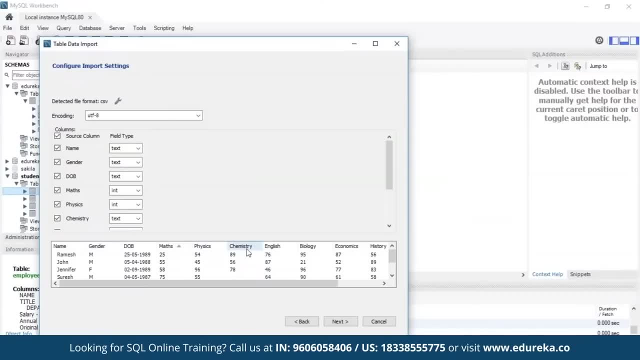 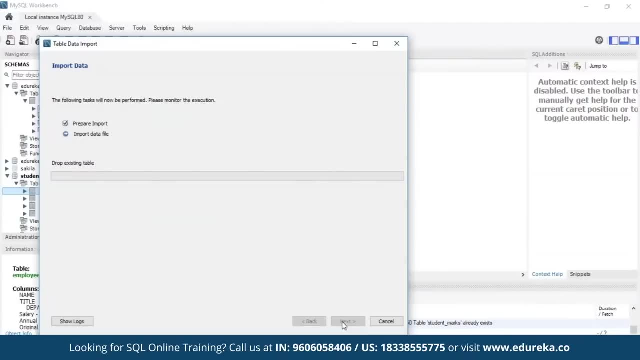 It has name, gender, date of birth, math, physics, chemistry and all of that. These are just records of students and their marks. then if I click on next and next again, Yeah, data gets imported. next five records are imported. click on finish and refresh. Here you'll see student marks. 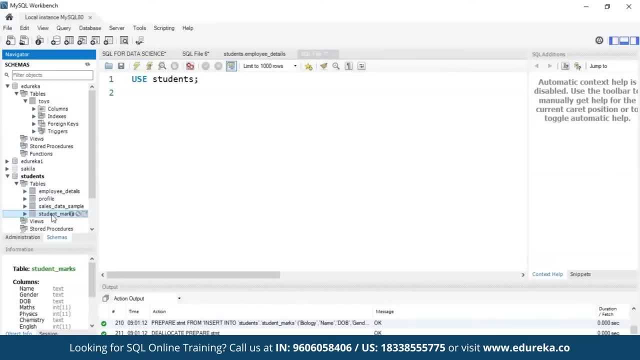 So this was the CSV file that I just imported into my SQL workbench. So, guys, that's how you import a CSV file as a table into your my SQL workbench. So if you want to see this table, right, the CSV file that we imported as a table. 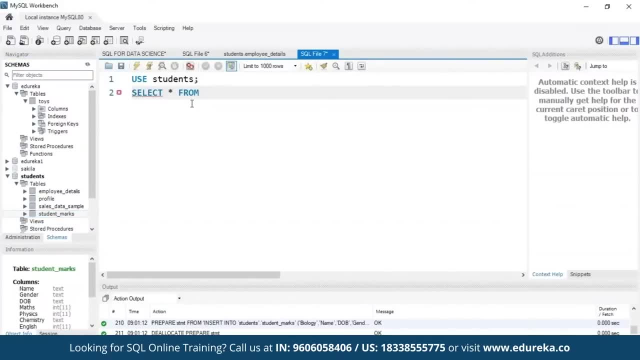 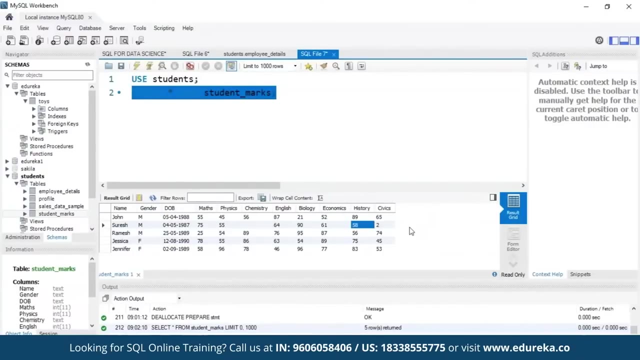 All you have to do is select start from and the name of the table. It is student, underscore marks, So let's just run this. So here you can basically see the entire CSV file that we imported into a table. So, guys, that's how simple it is to import a CSV file into. 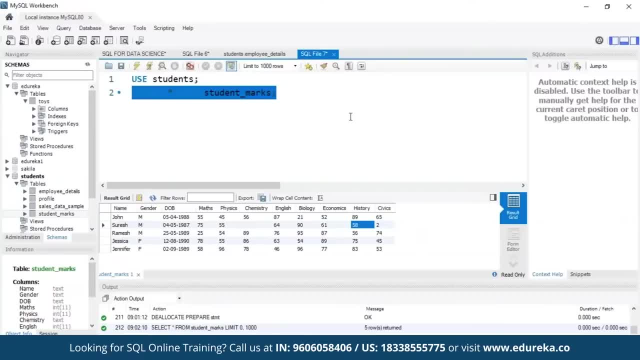 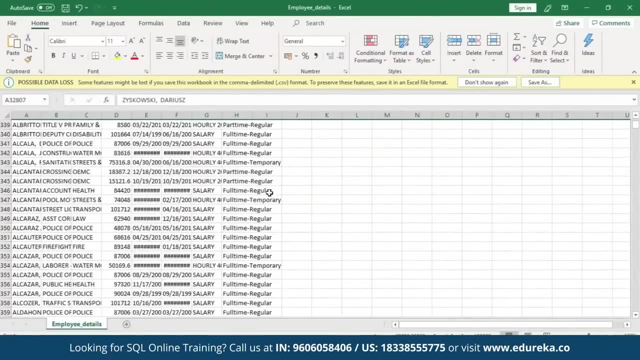 your my SQL workbench in order to perform data analysis. So now let's clear this up. So for this demo, like I said, we'll be using employee details data set. This is a very huge data set and let's just get started. 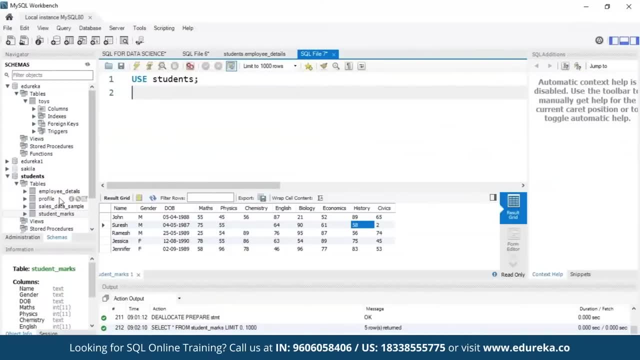 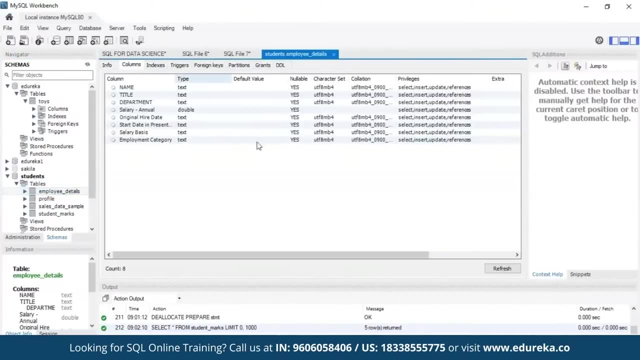 I've already imported the data set here as a table right, If you take a look at this: employee details. so these are the columns in my table. We have: name of the employee title. is the job title of the employee Department. is the department. 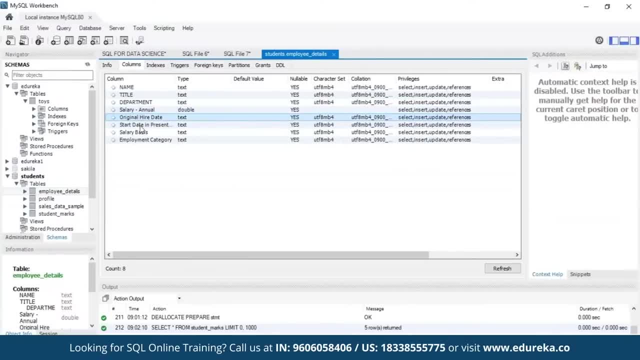 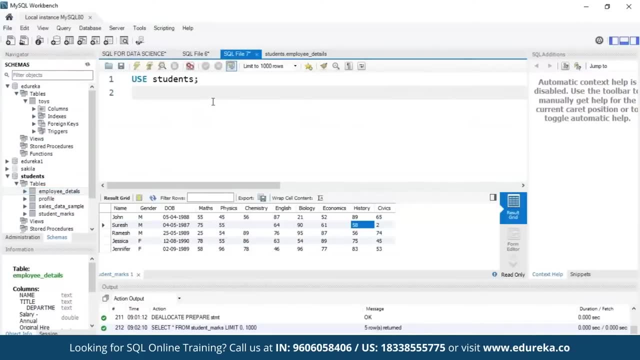 He works in salary- annual salary- Then we have hiring date, start date, salary, basics and we have employment category. All right, so let's start by performing some sort of data analysis. So first, what we'll do is let's just view the entire table. 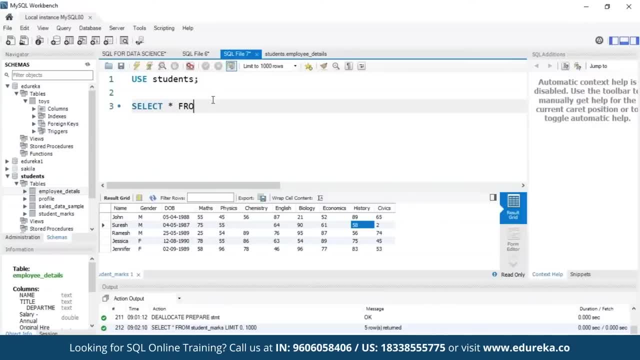 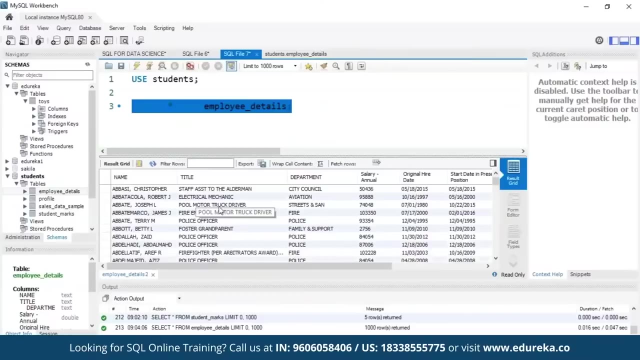 that we have. For that, All you have to do is select star from the name of the table. employee details is the name of the table in my case, So I'll just run this command Right. So this is the entire table that just got loaded. 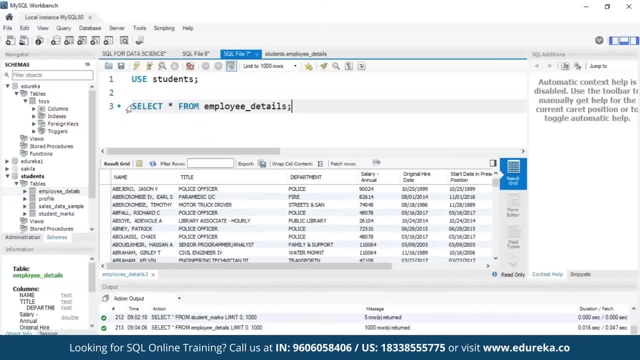 right, So this will just extract your entire table for you, Since I did select star from and name of the table, So my entire table is extracted here. right, If you take a look at this, the whole table is being extracted here. 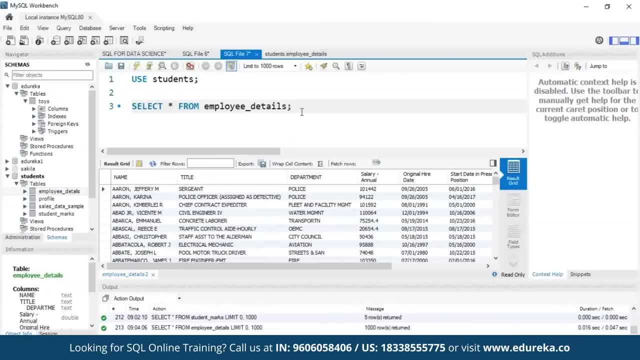 right Now. let's do something a little more complex. Now let's write a query to find the salaries of all the employees. for that, What you have to do is select again now name of the column that has the salary. Okay, 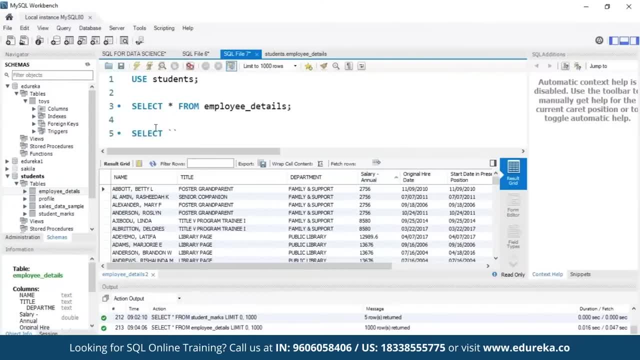 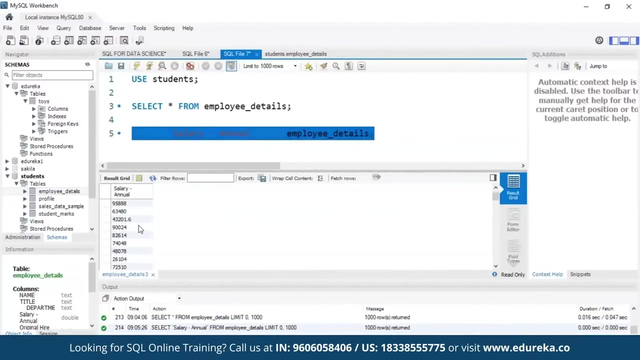 in our case it is salary annual right, So let's write that down salary Annual right from the name of your table employee details. So let's run this. So this query basically just gave me the salary column in my table right: salary annual. 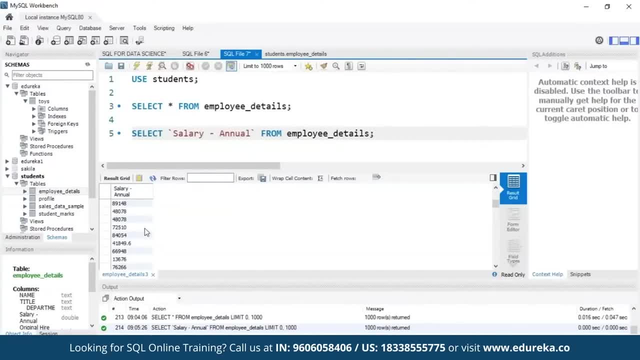 This is the salary of all the employees that are there, Right? It's as simple as that. Now let's write a query to display the unique designations for the employees. Basically, unique job roles will display. So for that again, we have select because we're extracting. then we have a keyboard. 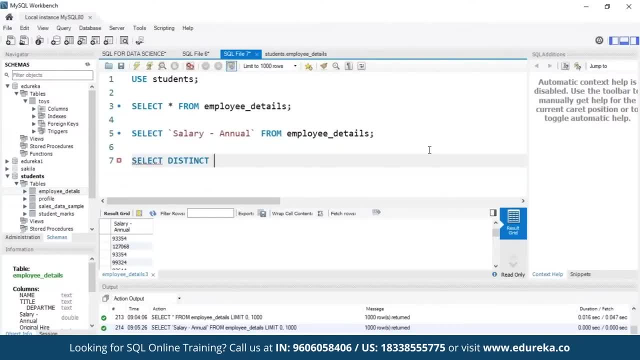 called distinct. since we are trying to display the unique designations, It'll just take the designations that are unique. It won't take your repetitive designations. For example, they might be 10 employees who are working as data analysts, So we'll just consider that as one. 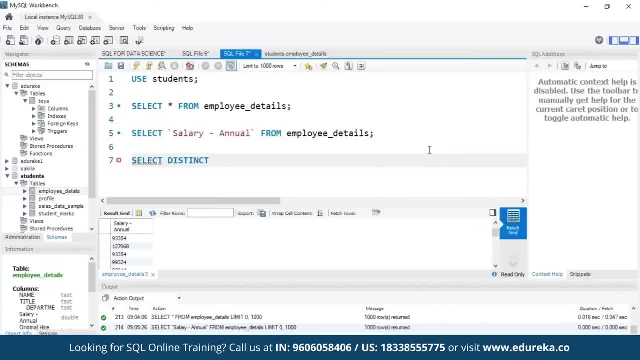 So we're just extracting the unique designations for the employees. That's why we have the word distinct here. Next, our job title is in the variable title, So that's why I've written title here And then we have from and the name of your table. 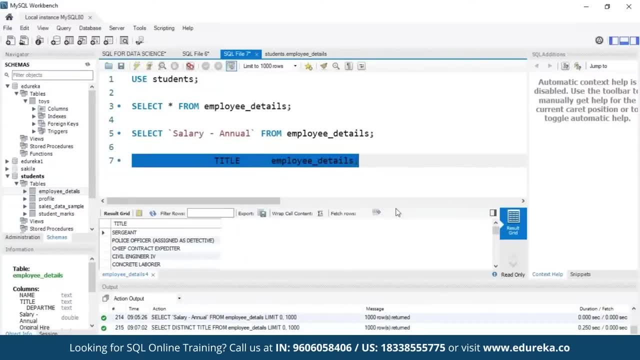 Right, Let's run this command. So here you can see that there are different job titles in our data set. We have Surgeon, we have police officer, we have chief contractor, Expeditor, we have civil engineer, concrete laborer. 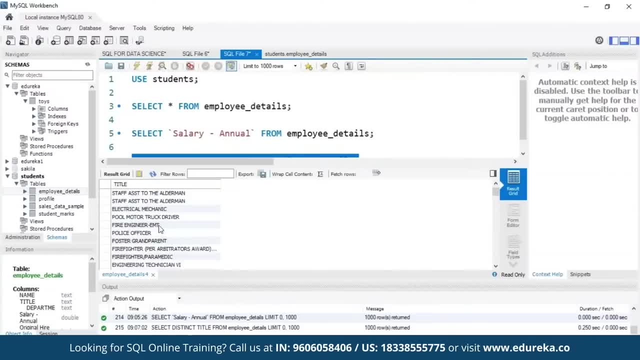 we have traffic controller pool motor. This is police officer and this is police officer assigned as detective. Wow, that's interesting, And so, basically, this query gave us the unique job roles that are there in our data set. Now let's try something else. 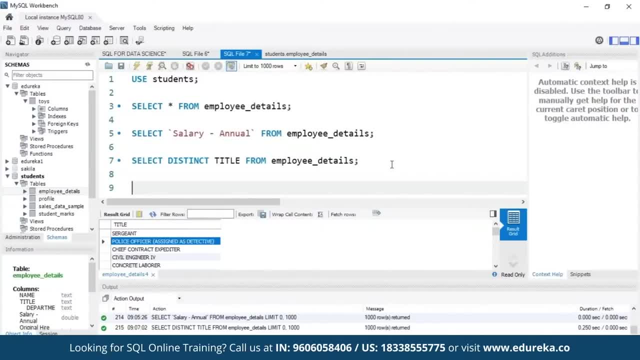 Let's write a query to display the unique departments with their jobs. So let's extract that. So select again. since we are trying the unique, we are going to use a distinct keyword and we are going to extract the unique departments and the job titles. 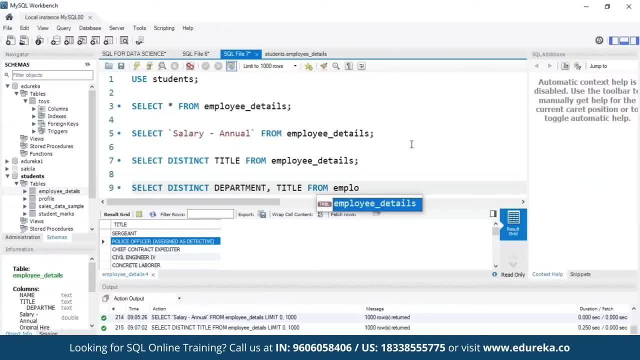 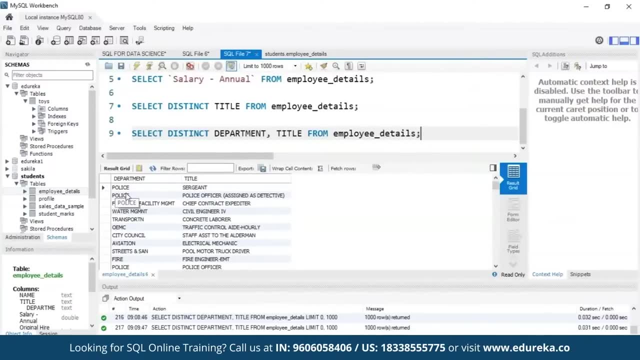 And from the name of the table. So let's run this code Now. under police department, we have different job titles. That's why this is repeated here at we have police officer. Then there is fleet and facility management, under which we have a chief contractor as Expeditor. 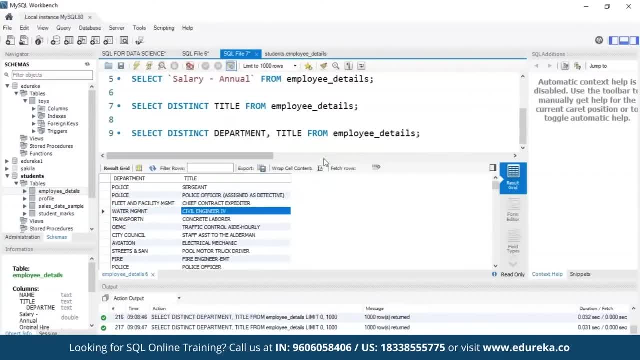 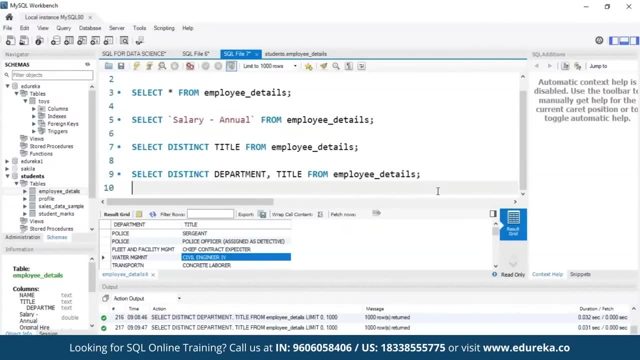 under water management Department, We have a civil engineer, and so on. And so, guys, this query was pretty simple. It just gave us the distinct departments according to their job titles. Now let's perform another query. We'll write a query to list the employees who are working in a particular department. 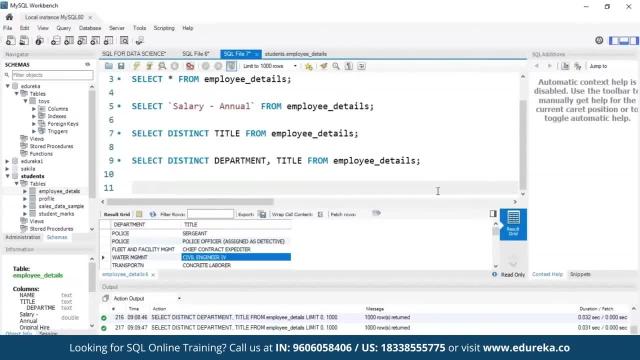 Let's say the fire Department. again, since we're extracting, will use the keyword select. after that select star from and the name of your table, Where. so this is where the where clause comes, and we're trying to identify a particular Department. So we'll put where. 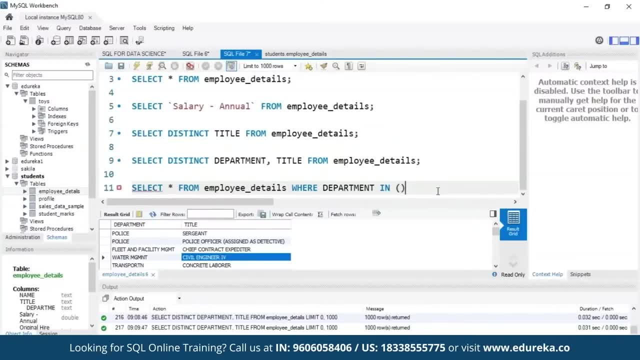 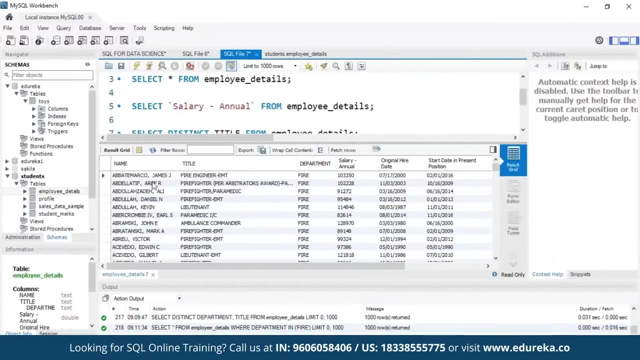 depart meant in the name of the department that we're looking for, Let's say fire Department. that sounds interesting, So let's run this All right. So here you can see that we've just got employee details of all the employees that are there in the fire Department. 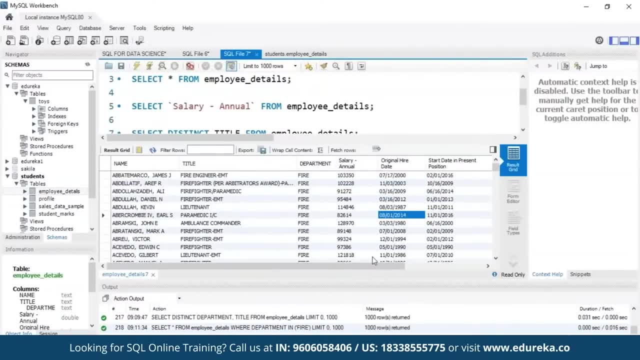 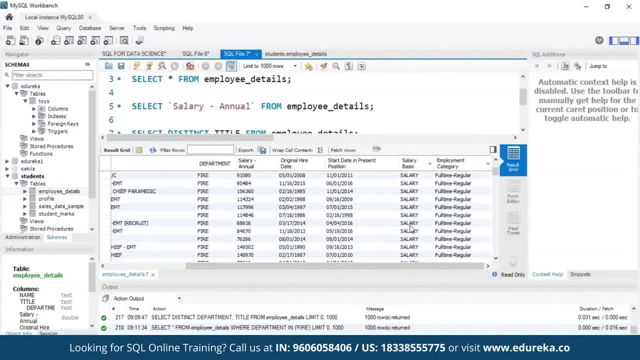 These are their salaries, These are the dates that they were hired on and, apart from that, this is the employment category: full-time, part-time. salary basis is whether you're getting paid hourly or whether you're getting paid on a daily basis. So these are the details of all the employees. 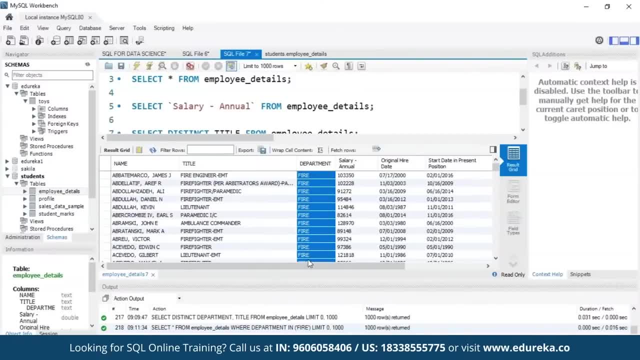 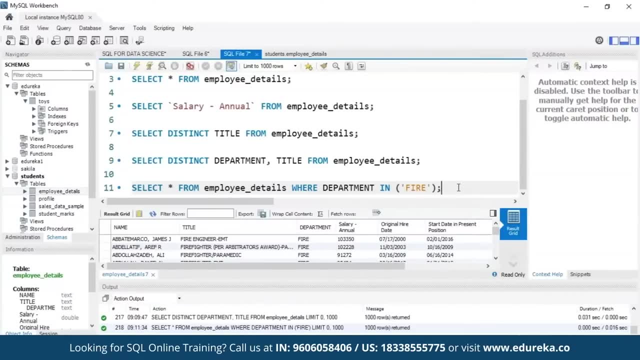 that are working in the fire Department. If you see that here it's entirely fire Department, So that was also quite simple. So this is how SQL is. the language is very, very simple because it's pretty understandable. like you can read the statement and you can understand what exactly I'm trying to extract. 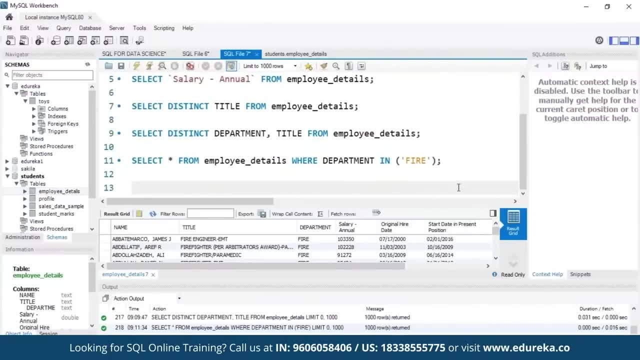 or what exactly I'm trying to do next. Let's try to do something interesting. Let's say that we want to write a query to list the employees who do not belong to a particular Department. Let's say that we're trying to list out the employee details. 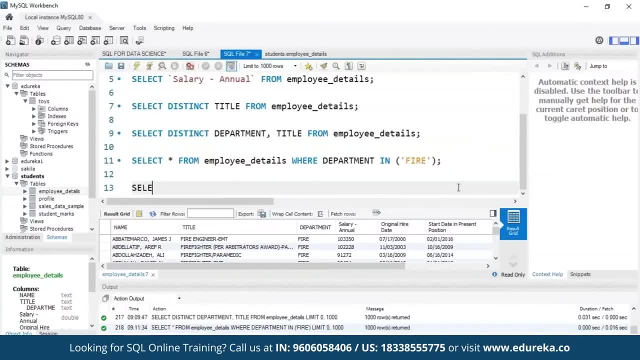 of employees which are not in the police Department. So for that it's quite similar to our previous query. So you write select star from name of your table again Where Department not in. that's the only difference. Okay, not in. and the name of the department that you want to exclude. 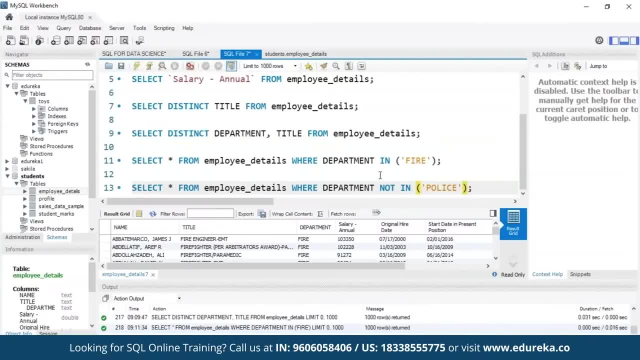 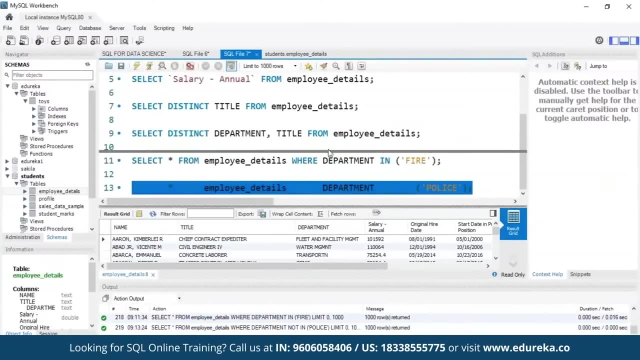 So this time let's say police Department. So we want only details of employees That are not there in the police Department. So let's run this, So all the departments here will have everything apart from your police Department. Okay, so we have fire. 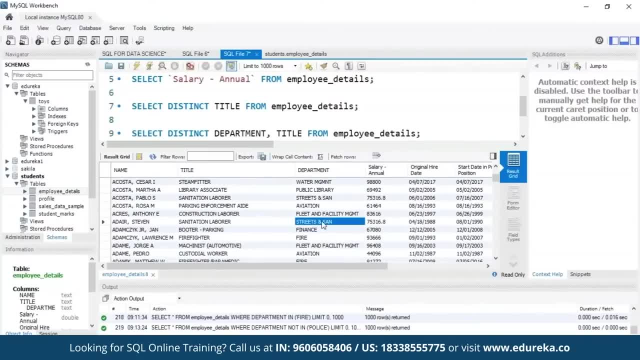 We have water management, We have law, We have streets and San, we have Finance Department, We have fleet and facility management and all of that. So basically, we excluded our police Department and printed out the details of all the employees which are in every other Department. 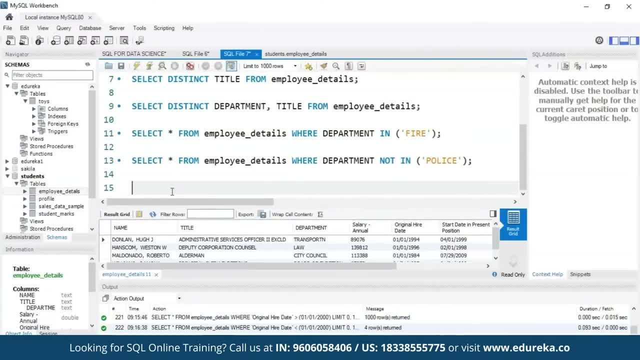 apart from the police Department, from the police, All right. So now let's write a query to list the employees who joined before a particular date. So for that again, we'll start from select star, from name of your table right, and we'll add the where clause. and here we'll mention: 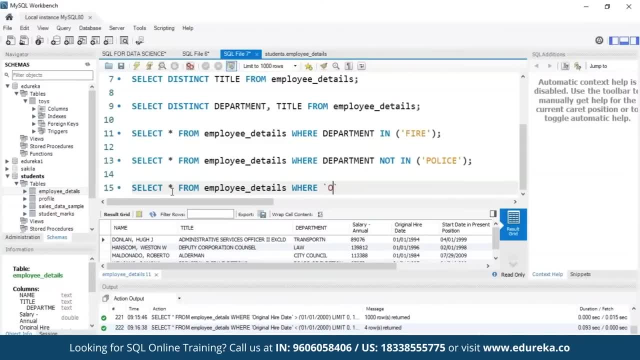 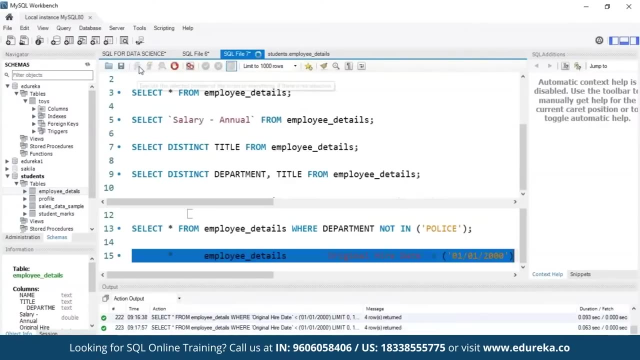 our original hiring date. since that's the name of the variable that has the higher dates in it, Let's keep it less than A particular date. Okay, let's choose first of January 2000.. Let's run this code, And so when you run this code, you'll find all the employees that 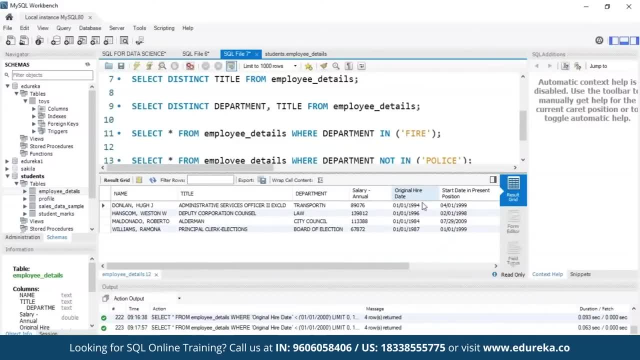 were hired before 2000.. So if you see original hire date, all of this is before 2000.. Some of them were in 1994, 1996, 1984 and 1987. So the only four employees who are hired before the year 2000. 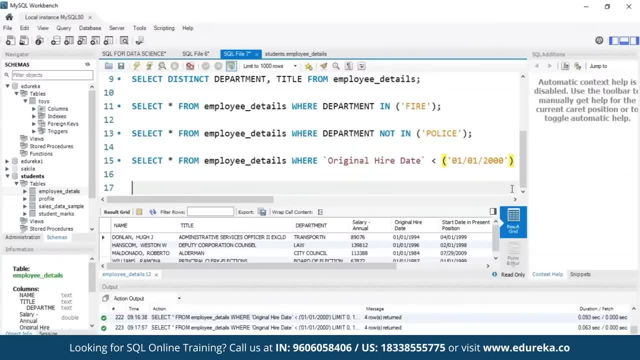 basically before the first of January 2000.. Now let's try another query. Let's write a query that will display the average salaries of all the employees who work at a particular Department. Okay, let's choose the surgeon Department. So basically, we're going to display the average salaries of 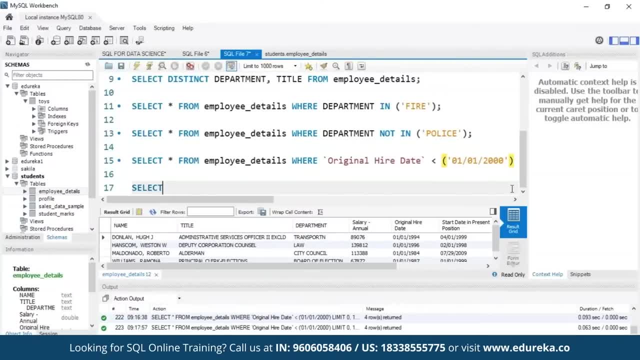 all the employees who are working as surgeons. So for that again it starts from select. since we have to calculate the average salaries, We'll use a function called average, which is a predefined function in sequel, and average Of which column it is a salary, column, salary. 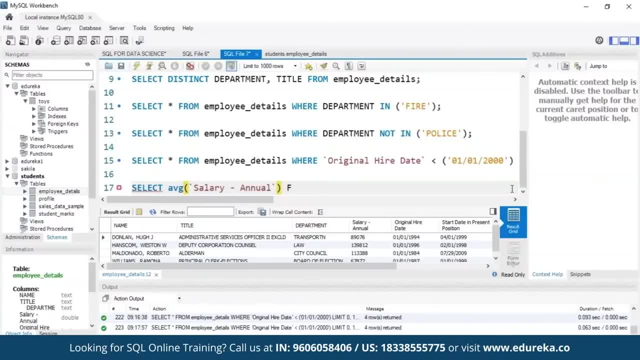 Annual And let's mention the name of the table from employee detail. Some error. Let's write down the whole statement and then we'll see what the error is. this and you're going to select The job title as a surgeon- Basically the average salary of a sergeant. Let's run this first and we'll find out what the error is. Okay, there is no error. I have no idea why I'm getting this. So the average salary is around 1 lakh 6000 and change right for a surgeon. 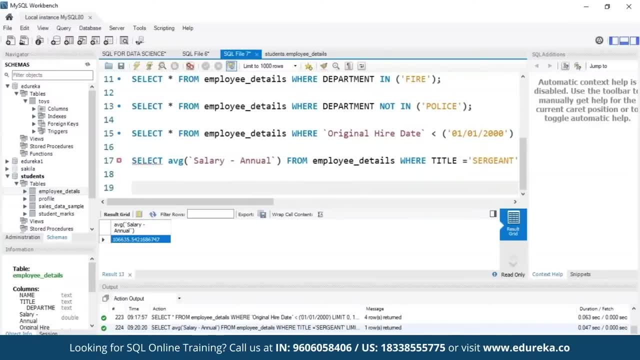 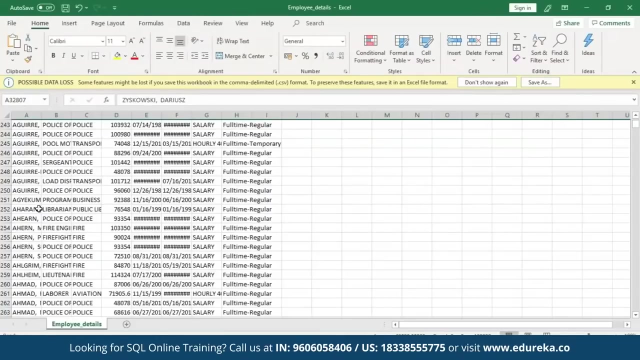 So now let's try another query. What we can do is we'll write a query to display the details of a particular employee. Some name will select at random. Okay, so select star from name of your table: employee details where name is equal to, let's look for a particular name. 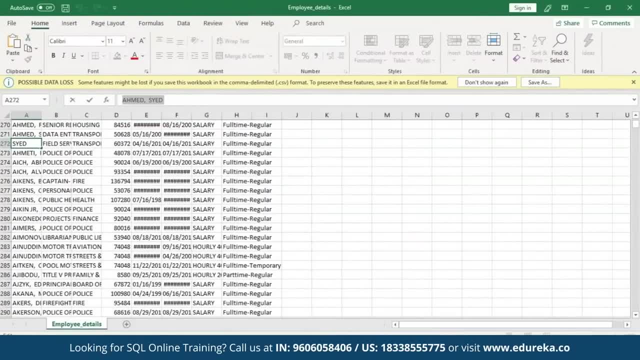 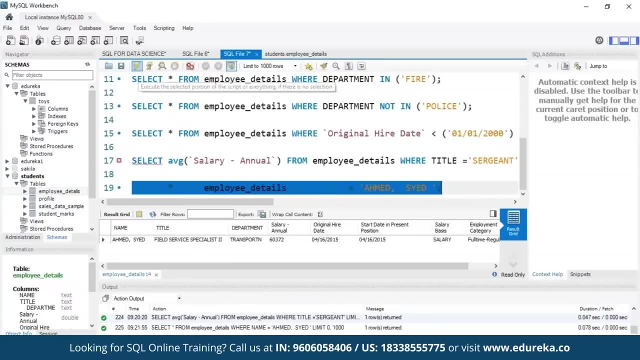 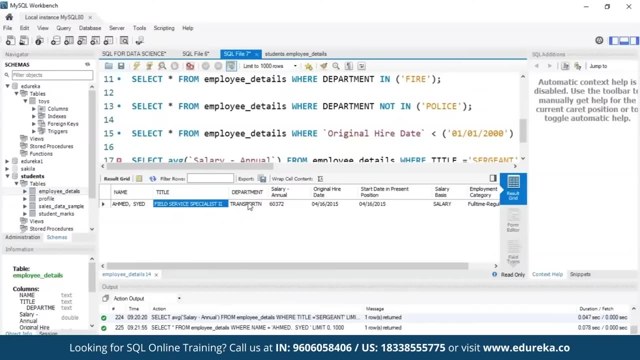 Ahmad Syed. Okay, So this is the name of the employee. Let's paste that name over here, Right? Hopefully they should give us an output. Let's run this. So now we have the details of this particular employee, who is Ahmad Syed, his title, job title, his department, his salary. 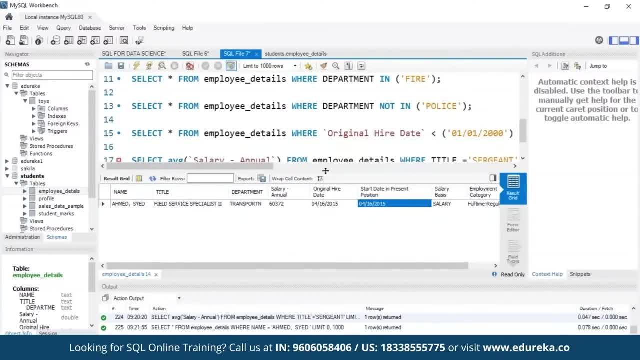 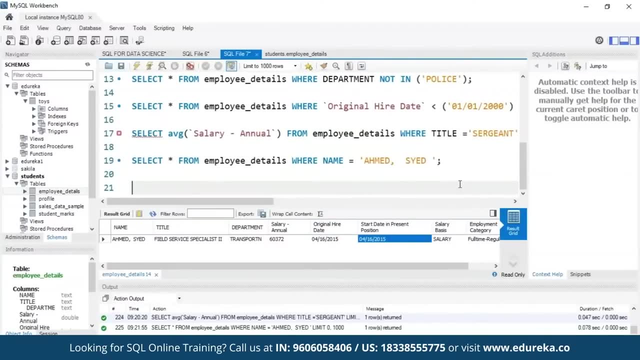 all the details about him. So we just printed all the details about a particular employee. Now let's try something else. Let's write a query to list the employees whose salary is, let's say, more than 3000 after giving a 25% increment to their salary. 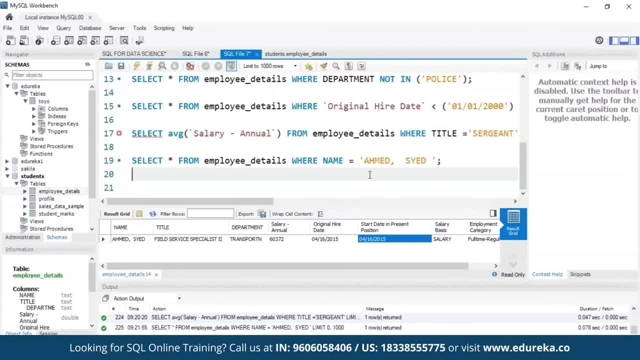 Now let's do a little bit of math. So we list down employees whose salary is more than 3000.. So we list down employees whose salary is more than 3000.. So we list down employees whose salary is more than 3000. 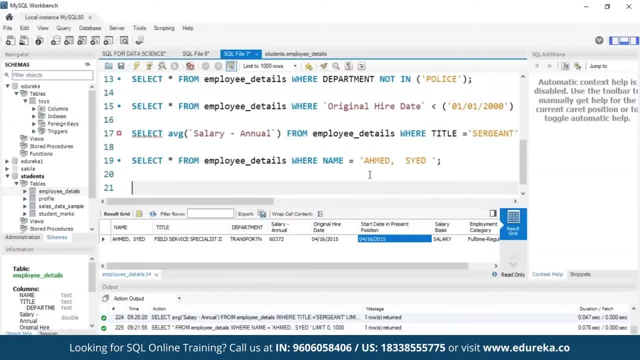 after giving them a 25% increment. So let's write down a query for that. So again, start off with select star from the name of your table, where here will specify the condition: basically, after giving them a 25% increment, 1.25 into the salary. 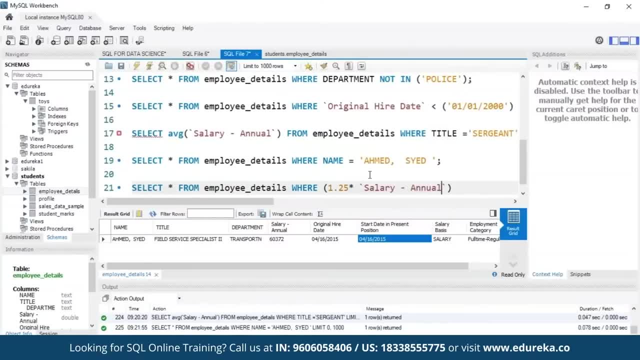 So salary annual, And after giving them a 25% increment, their salary should be at least 3000.. All right, so this is exactly what we're doing here. Let's run this code and let's see if we're getting anything. 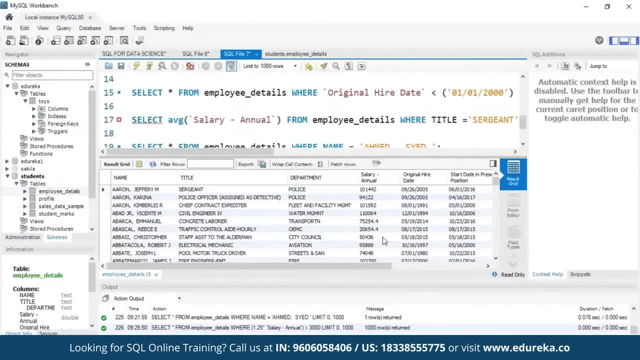 So here are the employees whose salary is more than $3,000, after giving them a 25% raise. So, basically, these guys are promoted. This is a list of all the employees. So that's quite simple, guys. It's basic math implemented in one line of code. 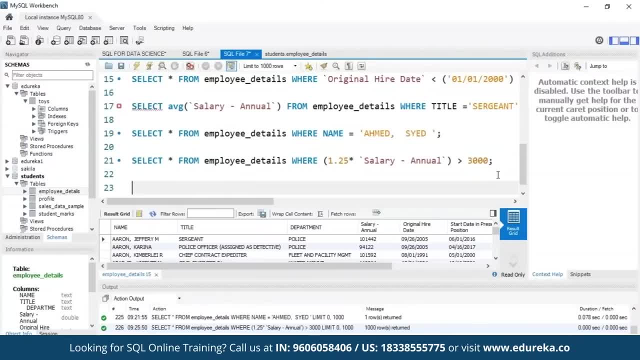 That's how simple SQL is. a lot of data scientists require this kind of tool because querying even your complicated math and even complicated things from your database becomes very easy when you make use of SQL languages. It becomes extremely easy to even do the complex things. 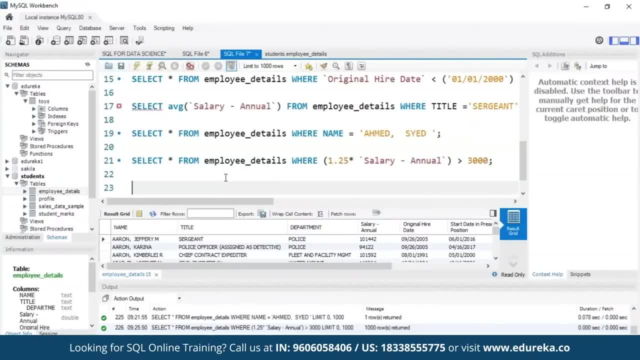 Now, I just did this in one line. So now let's try something else. Let's write a query to list the employees whose salary is less than a particular number. Okay, let's say less than $3,500.. So let's. 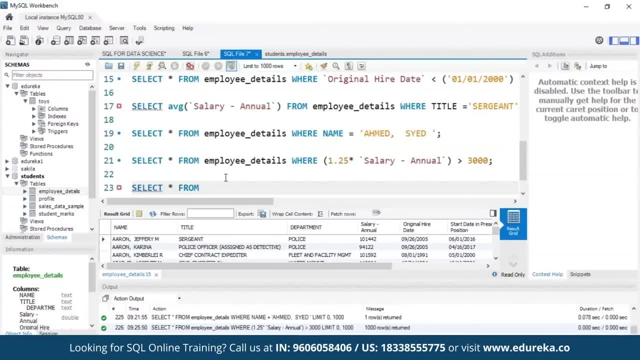 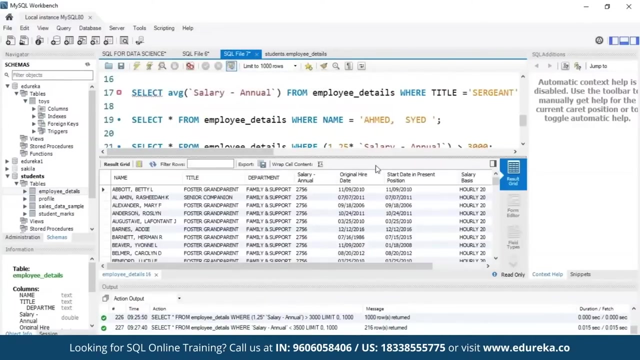 write a query basically for employees whose salary is less than $3,000 or $3,500.. Where salary annual is less than, let's say, $3,500.. So let's run this line of code. All right, so we have a couple of people whose salary is less. 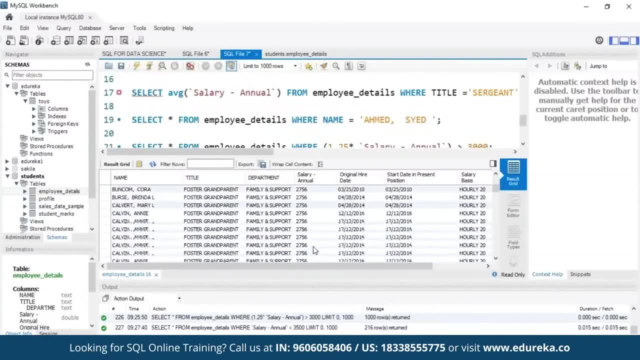 than $3,000.. So we have $2,017.. 56 like maximum of these people have 2007 56. Okay, So basically this is a list of employees whose annual salary is less than $3,000.. That's also quite simple to do. 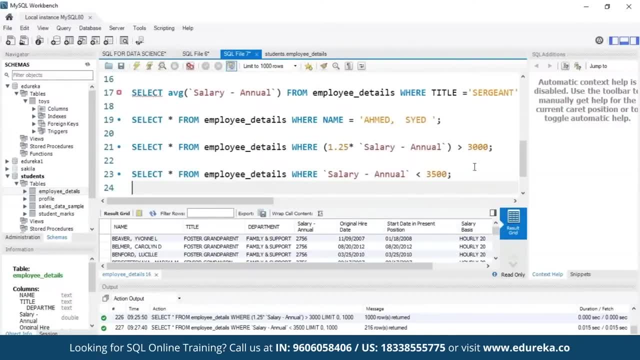 It's just one line of code. Now let's try something else. We'll write a query to list the names and a particular set of details about an employee who joined before a particular date. Let me write it down for you, and then we'll understand what. 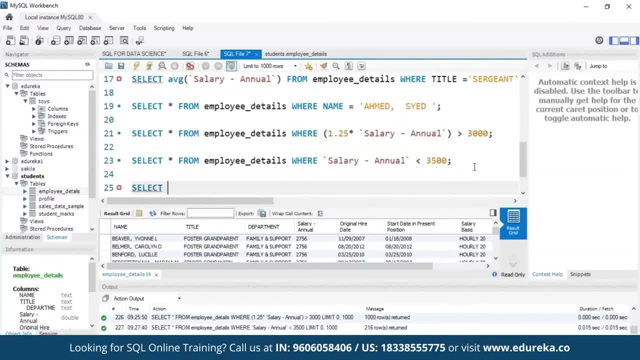 exactly I'm doing. So let's now we'll define a variable so that we can basically extract a number of columns. Okay, so let me write this down and then I'll tell you what exactly I did here. name, and let's also get their salary. 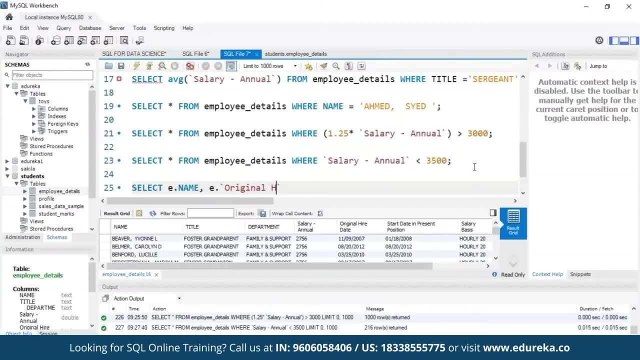 right original Hiring date. Then we'll also get the salary From the name of the table Where The hiring date- Let's say it was lesser than and give a random number- 0, 1, 0, 2, 2008.. 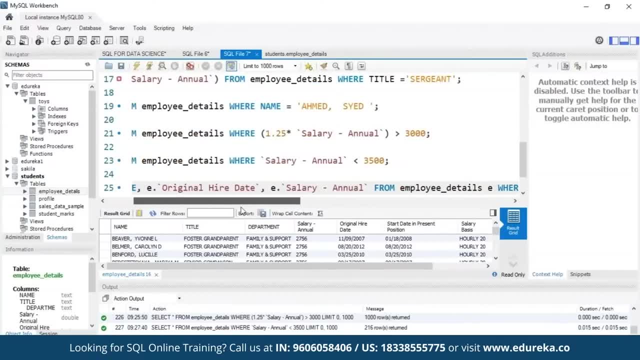 Now, what exactly I'm doing here is I'm basically listing out the name of the employee, the hiring date and the salary of all the employees that have joined before a particular date, Okay, basically before this date. That's what I've done here. 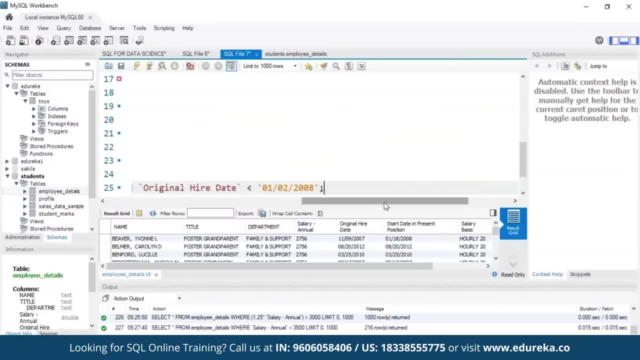 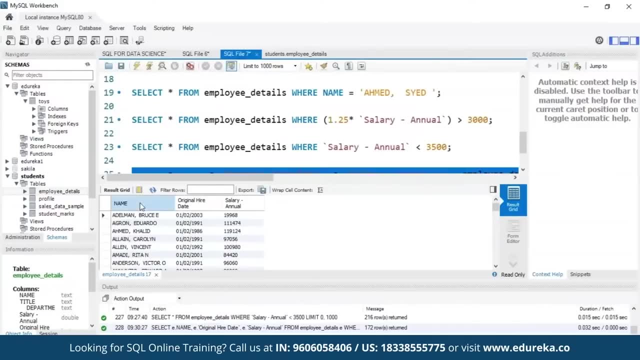 Let's run this line of code and let's see if it works Right. So here we have the name, the hiring date and the salary of individuals that have joined before a particular date in 2008.. So it's as simple as that. 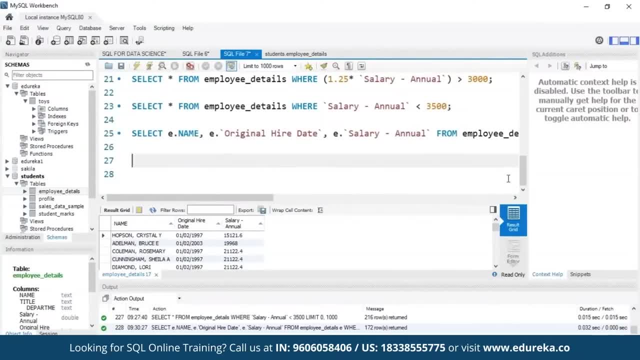 Now let's write a query in SQL to list all the employees who joined on a particular date. Okay, let's say we want the details of all the employees Who joined on October of 2013, or something like that. For that again it starts off with select start from. 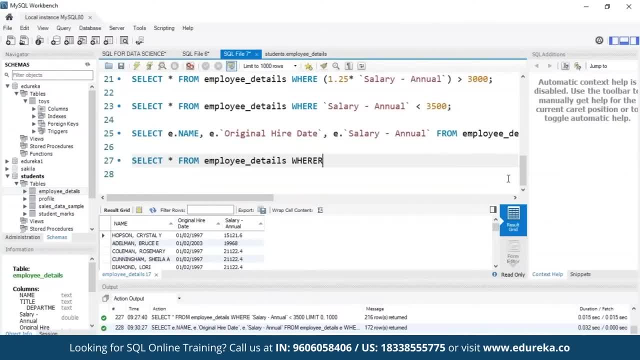 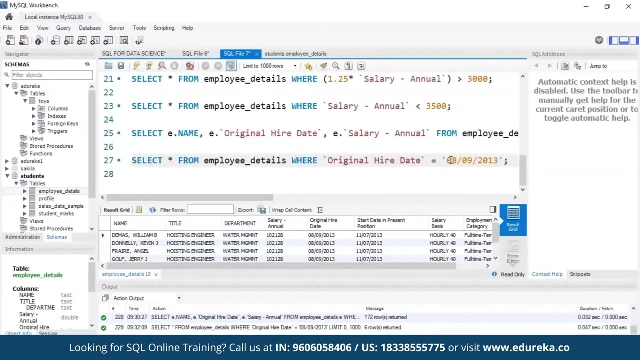 the name of the table, We'll add the where clause along with the hiring date, original hire date, a particular date, Let's say 0 8 2013.. Let's run this line of code. So, basically, we list down employees that were hired on. 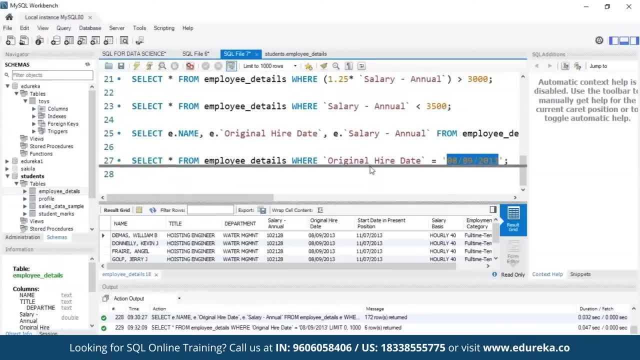 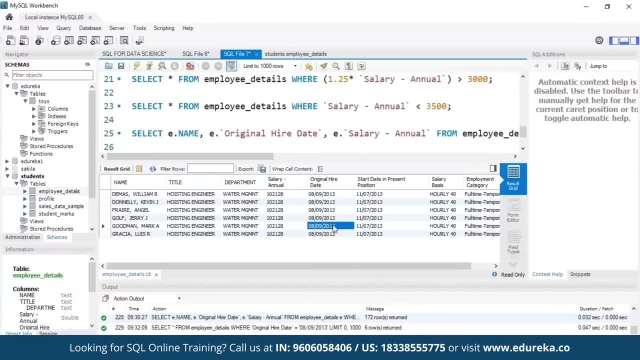 this particular date. Okay, These are details of all the employees that were hired on the same day. So we have around six employees that were hired on the eighth of 2013- some date, right? So, guys, that's what you see. SQL is a very easy language. 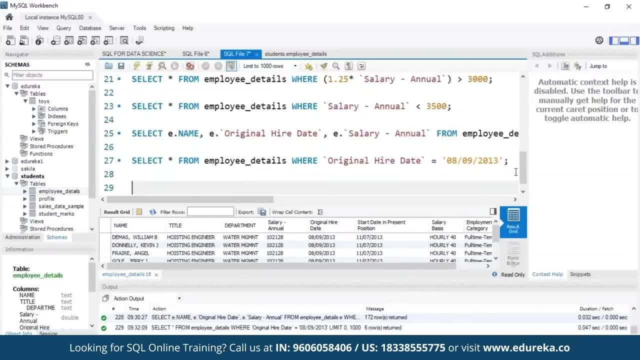 You just have to understand what you're trying to extract. That's all you just have to know like five to ten basic commands, and these basic commands can do wonders. They can extract and manipulate data in such a way that you know you can perform proper data analysis, data processing. 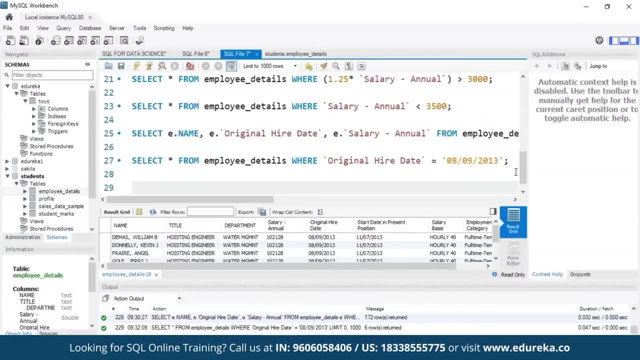 and so on. Now let's try one last query. Let's write a query to list the employees whose annual salary is within a particular range. for this, again, We have select start from name of the table, Employee details, and let's add the where clause and here we will say salary. 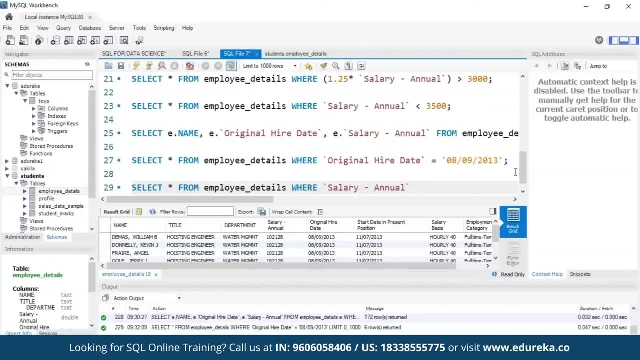 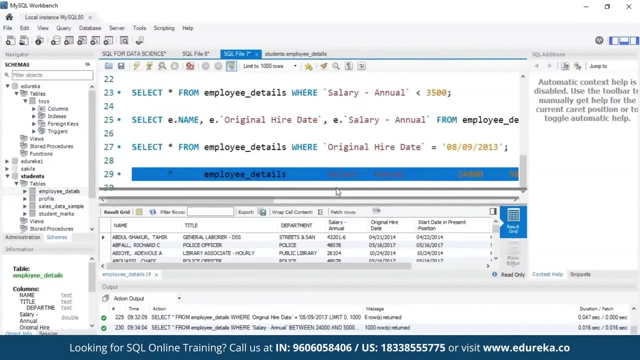 and annual is between between, as another keyboard, So between two numbers. okay, let's say between on $24,000 and let's say 50,000.. Right, Let's run this line of code, All right. So here you can see that all of these employees have a salary. 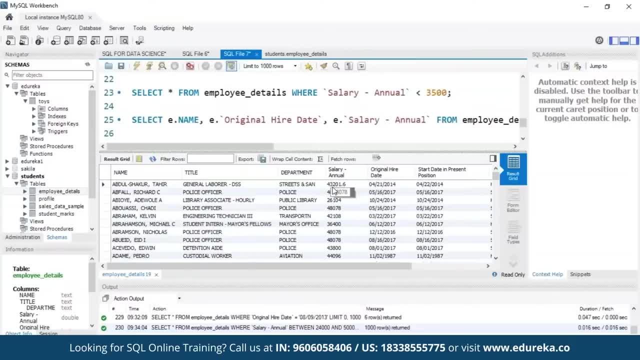 range between 25,000 and 50,000.. So 43,000, 201.. We have 42,000.. You have 44,000.. We have 45,000, 48,000 as a maximum salary, All right. 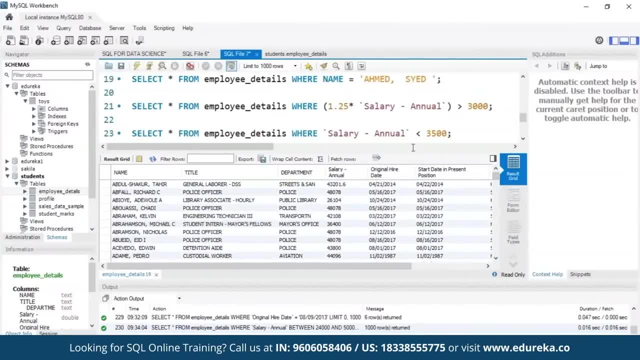 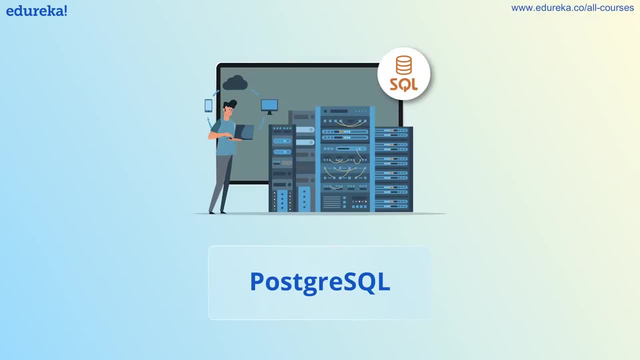 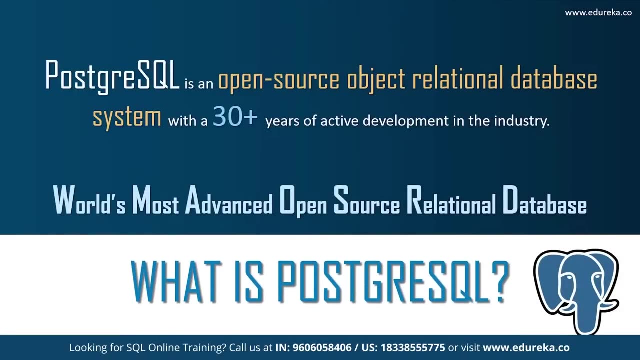 So this is basically how you perform querying using SQL. What is Postgres SQL Now? Postgres SQL is an open-source object relational database system with the 30 plus years of active development in the industry. So basically, if you have to understand Postgres SQL guys, 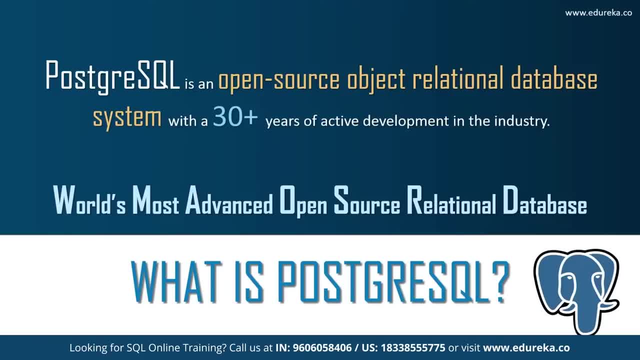 a. Postgres SQL is basically a programming language, or maybe you can understand that you know a language to which you can handle open-source relational database systems and then handle databases. Postgres SQL is world's most advanced open-source relational database. So, guys, this is a really great topic to start learning about databases. 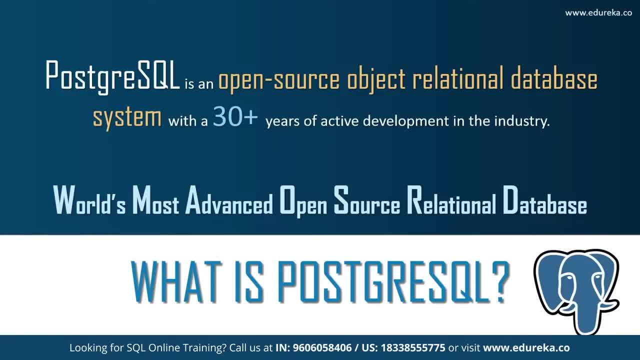 So if I have to just define Postgres SQL for you, then you have to understand Just two points over here- that it is open-source and it is used for handling databases in the form of object relational database system, So the data present in the form of relational database. 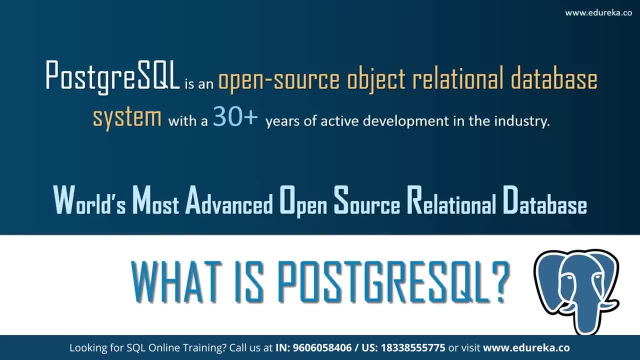 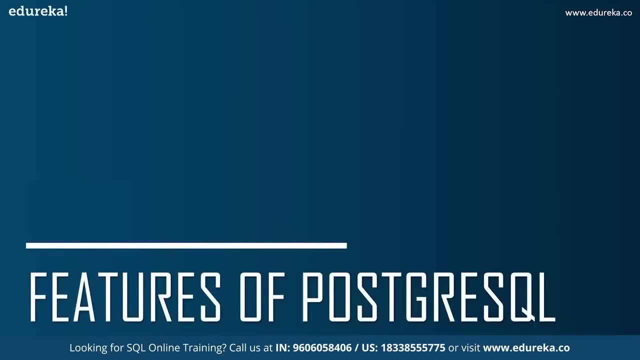 but, yes, it is object oriented. That's where Postgres SQL comes into picture Now, since Postgres SQL is so popular in the industry. next let's look into the features of Postgres SQL. So the features of Postgres SQL are, as you can see on my screen. 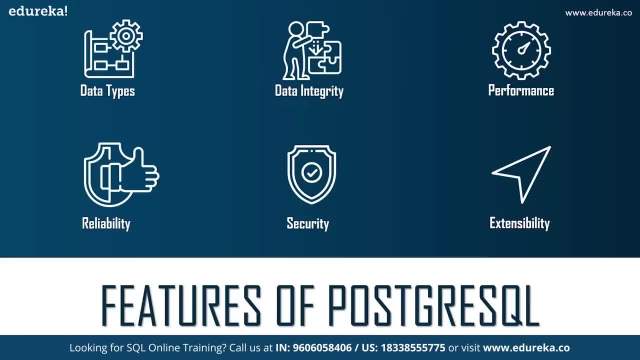 that is basically the data types to data Integrity, performance, reliability, security and extensibility. So, talking about data types, when I say data types, what I mean by that is Postgres. SQL provides various kinds of data types to store data in any format, such as you know. 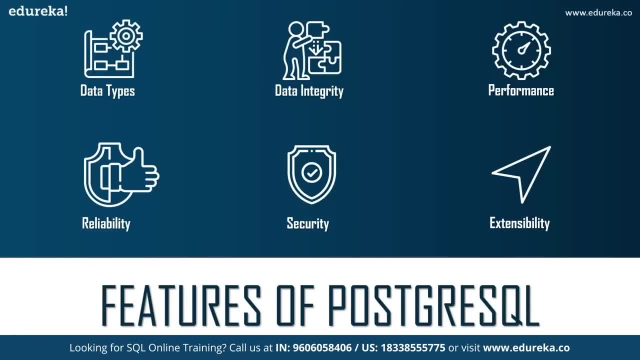 integer, numeric data type, Jason XML file, maybe in the form also of point line, circle, polygon, and also you can have custom data types. So there are various kind of data types, like you know: the primitive one, the structure, the document, geometry and customizations. 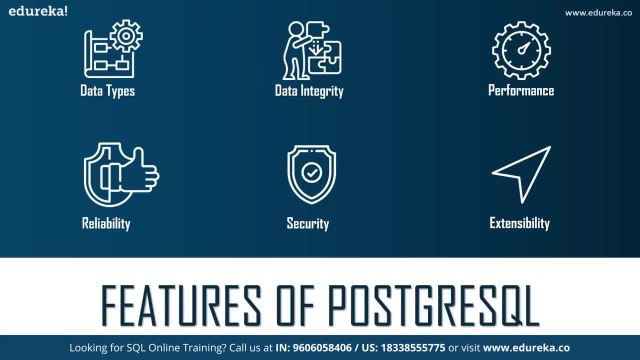 So we'll not get into the depth of. you know the different data types Related to Postgres SQL. You can go to their official document and check what are the different data types that you know Postgres SQL provides. well, I would leave that to you. moving on to the next feature: data Integrity. 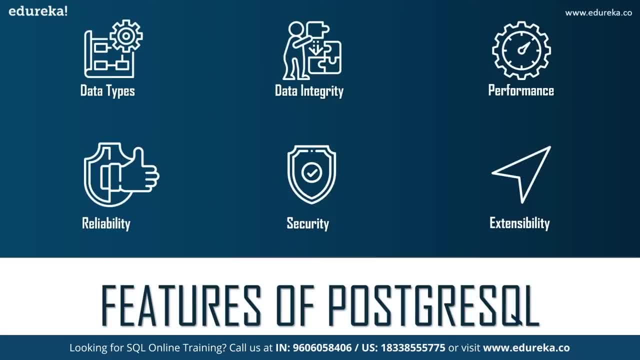 So when I say data Integrity, what I mean by that is you know your data is secured. So, basically, whatever data that you have, it's made sure that you know it's there's no redundancy, and then it's stored in the proper format with the help of you know. 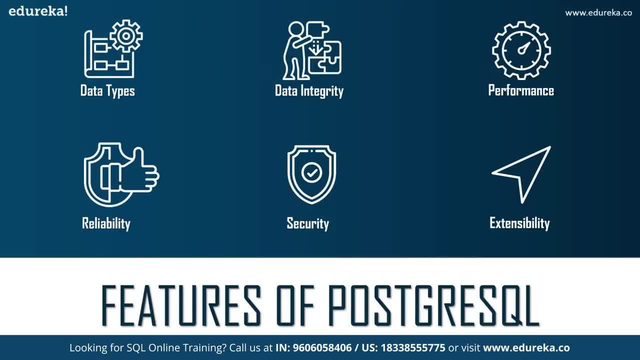 various constraints and keys used in databases, like primary key, foreign keys, exclusion constraints, unique constraints and explicit locks, and so on. right, So that's how, basically, your data Integrity is met. coming to the next feature, that is performance. now, performance is something that's very important to all of us. 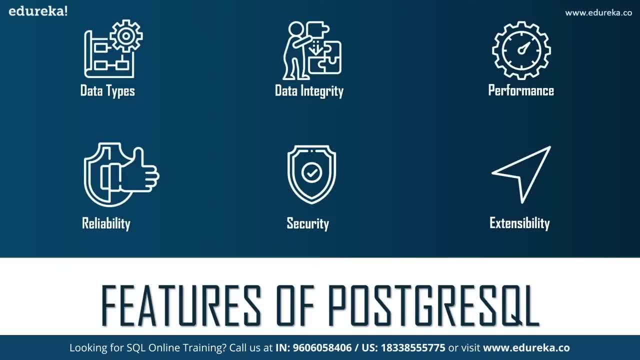 right, because all of us want a good performance for any action that we do in industry basis right now. since Postgres SQL means with good performance standard, that clearly implies that you know it has been used for more than 30 plus years of active development now to enable performance in Postgres SQL. 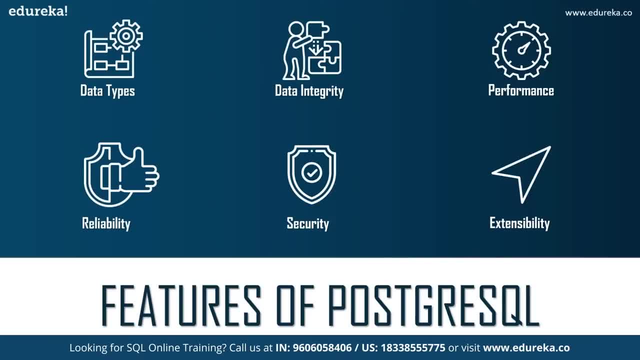 We have various features, like we have indexing, or maybe sophisticated query planner, multiversion, concurrency control, table partitioning, just-in-time compilation of expressions, and so on. now moving on to the next feature, that is, reliability. now Postgres SQL also proves itself in the factor of reliability. 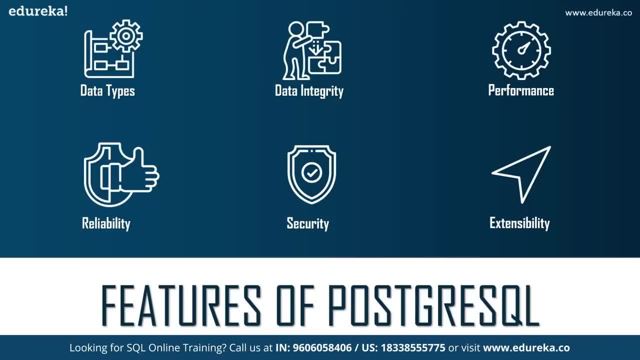 that is because you know it has various functionalities like right-ahead logging, replication, point-in-time recovery, active standbys and tablespaces. finally, coming to extensibility now, obviously any database that you wish to use, you would obviously want to extend it to maybe any application. 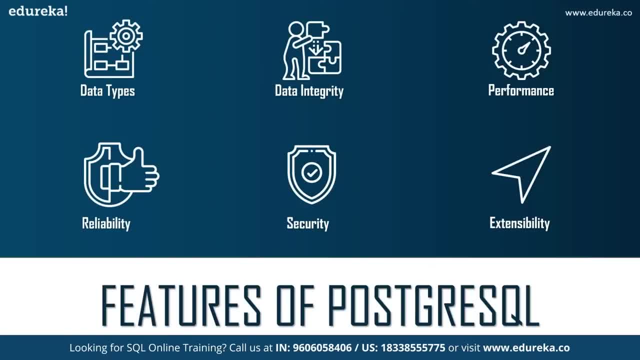 that you might be using in the industry or maybe in your company or also on an individual basis. Well, Postgres SQL provides all those functionalities with the help of stored functions and procedural language, foreign data wrappers and many extensions that you'll see further in the session. 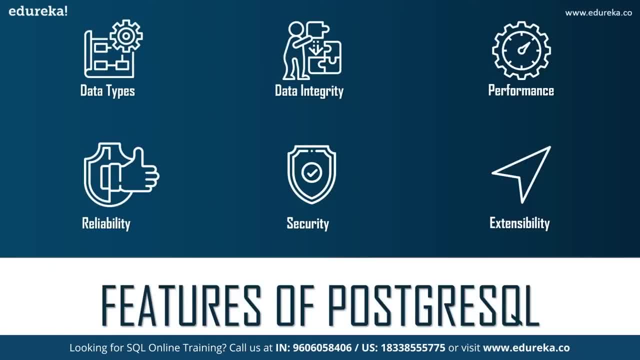 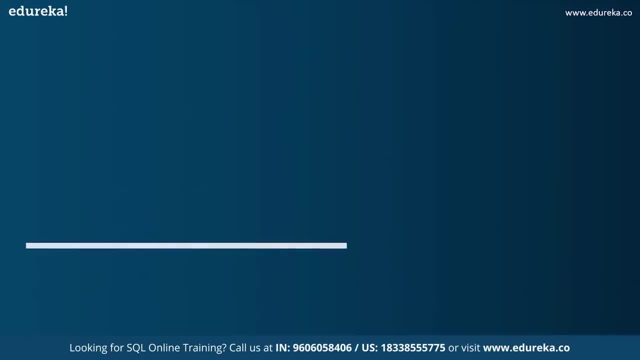 So, guys, these were the main six features of Postgres SQL, that is, data types, data Integrity, performance, reliability, security and extensibility. So now that you know what is Postgres SQL, let's next look into how you can install Postgres SQL. So what I'm going to do is I'm going to install Postgres SQL. 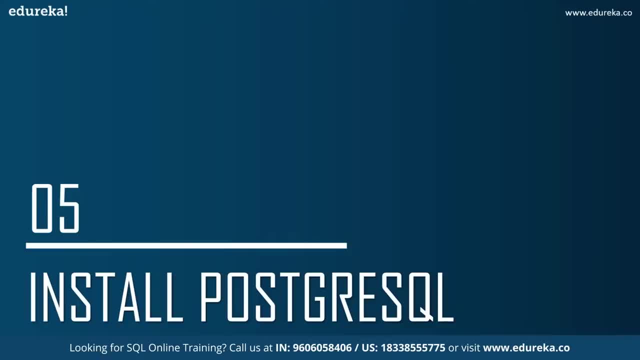 on Windows. So, apart from that, if you want to install Postgres SQL on any other operating system, well, the steps are really simple and the steps are almost same. So let's get started by installing Postgres SQL. So what I'm going to do is let me open my Google Chrome. 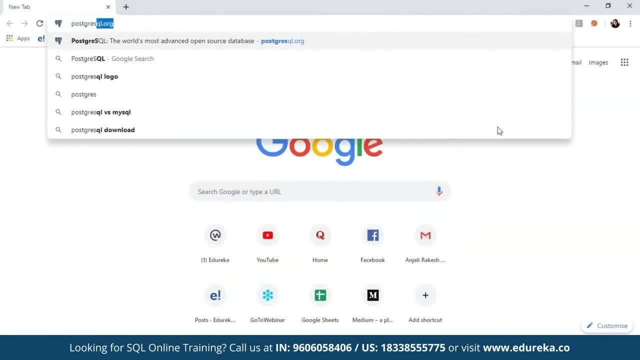 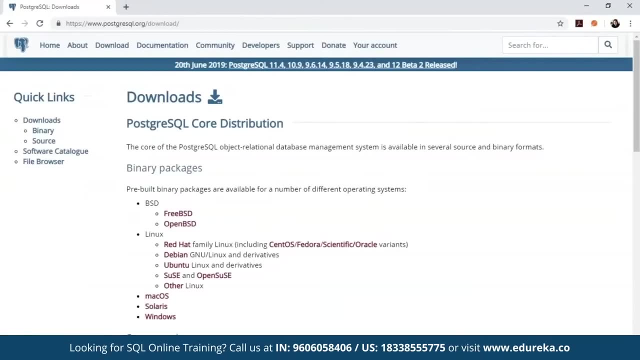 and then let's say, I just type in Postgres SQL download, right, So once I type in, you have to first to go to the official website, that is, Postgres SQL dot org slash download. So this is where, basically, you'll have to go. 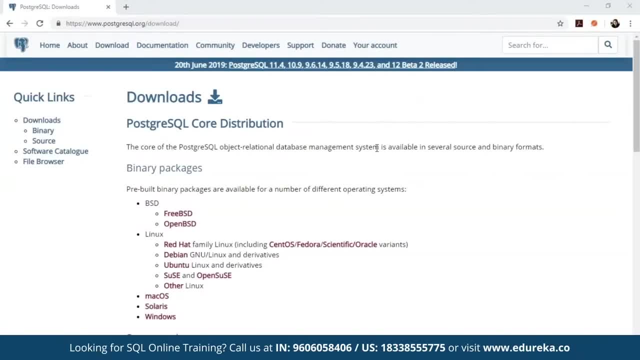 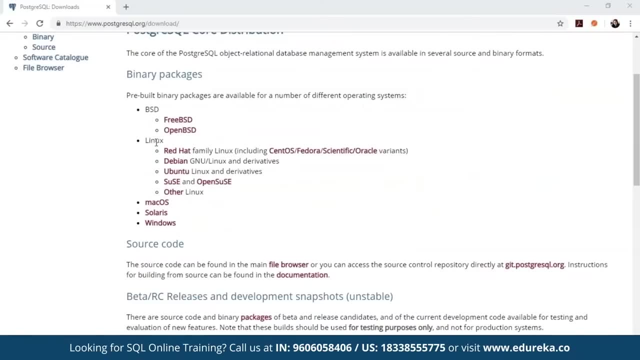 to first start installing Postgres SQL. So what I'm going to do is basically, I have to install on Windows, right? So we here, you have to start choosing your operating system. So if you wish you install a Linux, let's say you know one, two. 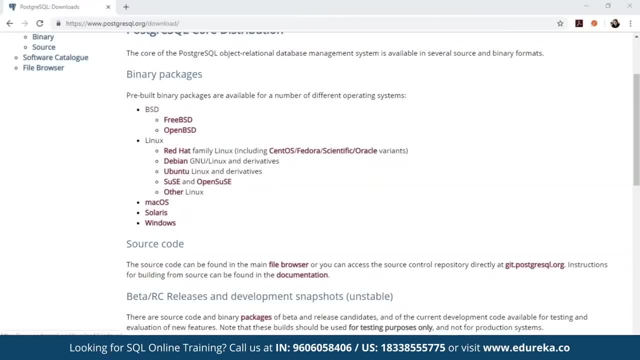 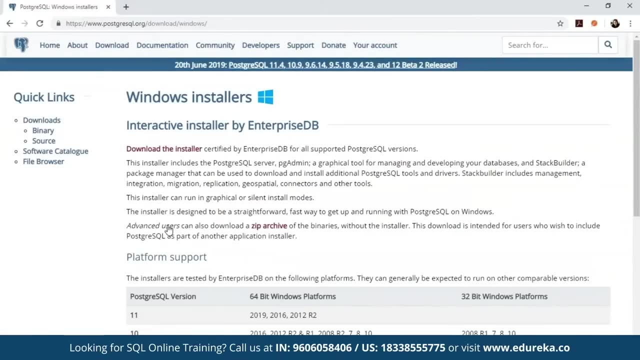 then you would choose this option. But since I'm going to install on Windows, I'm going to simply choose this particular option. So if I click on Windows over here, you'll be next redirected to this particular page. Now, this is the page. 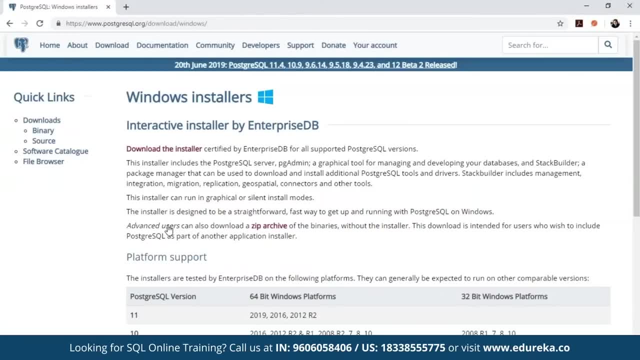 So basically, you have to install the installer right. So basically, every operating system that you choose, the official website of Postgres SQL will redirect you to a particular page which will have this particular installer. So over here you can see that I have the Windows installer. 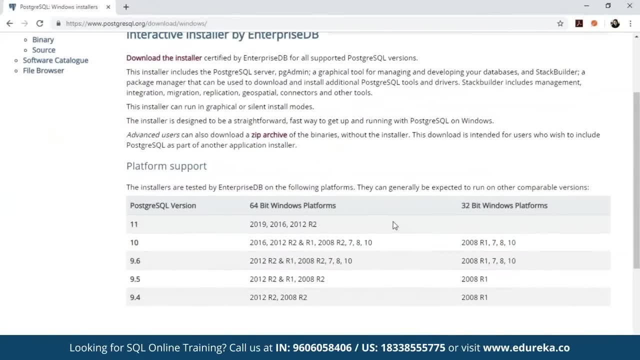 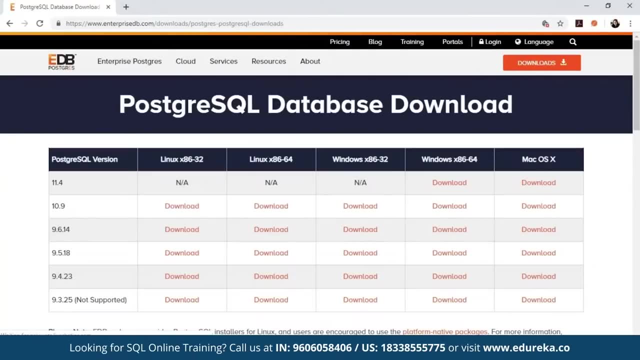 and then I have to install, and then you can see the platform support right. So what I'm going to do is I'm going to just click on this option: download the installer. Now, once I click on download the installer, this is where, basically, you have to choose your configuration. 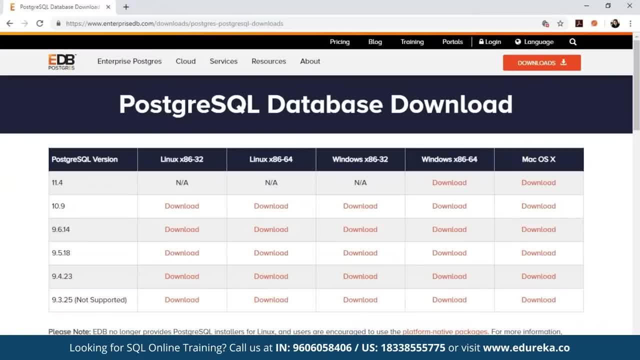 right. Either it is Linux or Windows or Mac OS. That's completely your choice on what operating system that you wish to choose. since I've been installing on Windows, I'll choose Windows 64-bit, right, So I'm going to choose this particular option of download. 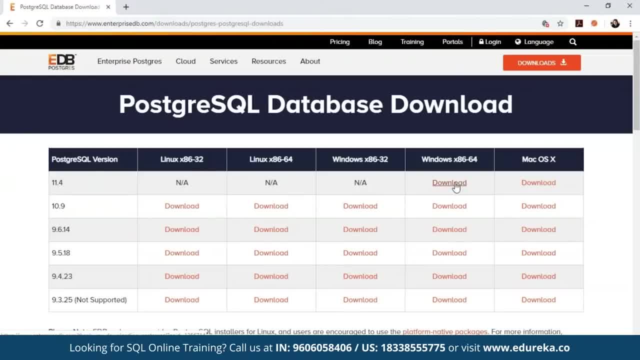 and please remember the fact that you know try to install the most latest version so that you can get the maximum features that you want. So I'm going to install the 11.4 version for Windows 64-bit, right? So I'm going to just click on download over here. 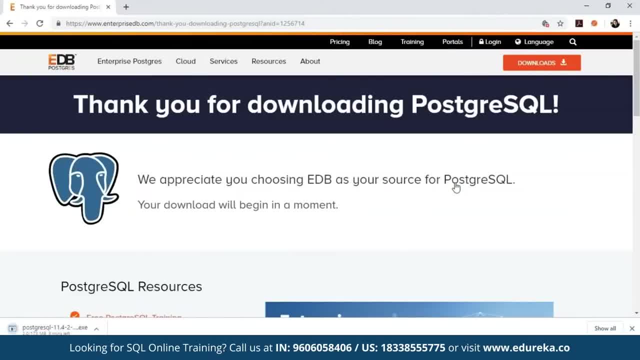 and then you see that you know you'll be redirected to this particular page that you know. thank you for downloading Postgres sequel. and also on the left hand side you'll see that you know Postgres sequel is getting downloaded, right. 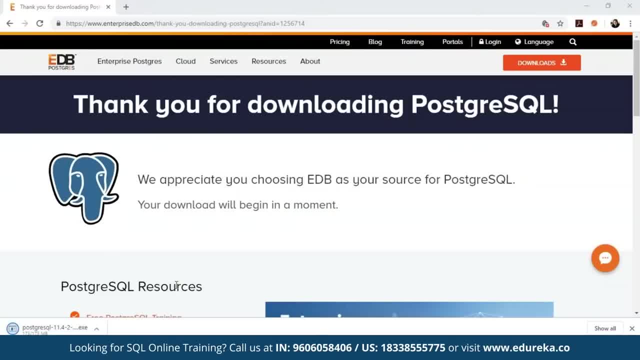 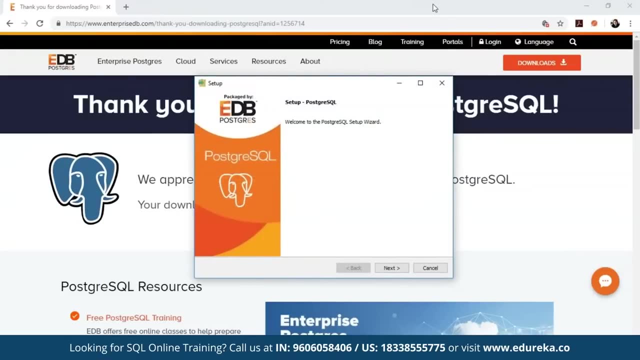 So let's wait for it to download. All right, so as you can see on my screen, it has got downloaded, So I'll just double click it so that we can open Now, once you double click on the setup, you'll see that you know, this particular dialog box opens. 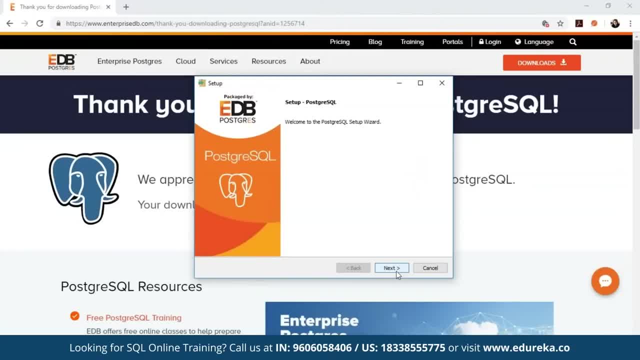 which says welcome to Postgres SQL setup. This is right, So now you just have to click on next and then you have to choose the installation directory. I'm going to let it be as it is, So by default, minus C, program files, Postgres SQL and level. 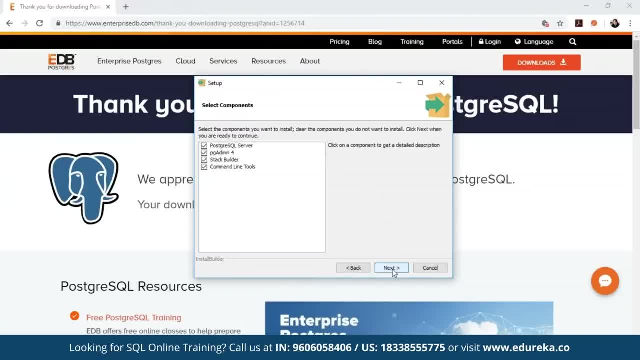 so that will be basically my installation directly, and then I'll click on next. once I click on next, you'll get an option basically on the various components that you wish to install. Well, I wish to install all of them. So basically, I'm installing the server, the PG admin. 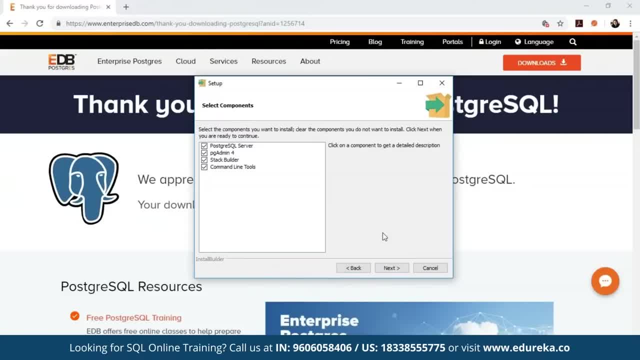 the stack builder and the command line tools. So now over here, let me tell you that you know, the PG admin is the official GUI for Postgres SQL, So we'll be working on the GUI for this particular session. So I'm going to just let it be as it is. 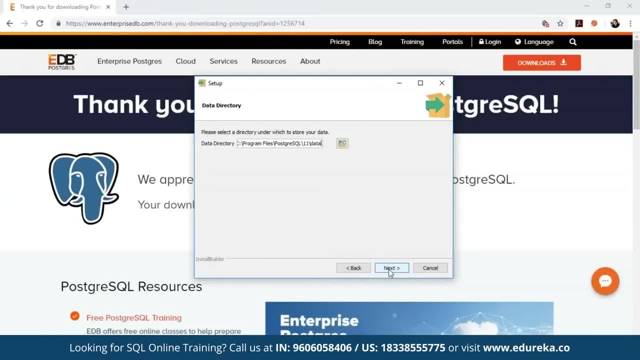 since all of them are checked in, and then I'll click on next. once I click on next, I have to next choose the directory under which I'll basically store my data. right, So this is basically my data directly, that is C program files, Postgres, SQL, 11 data. 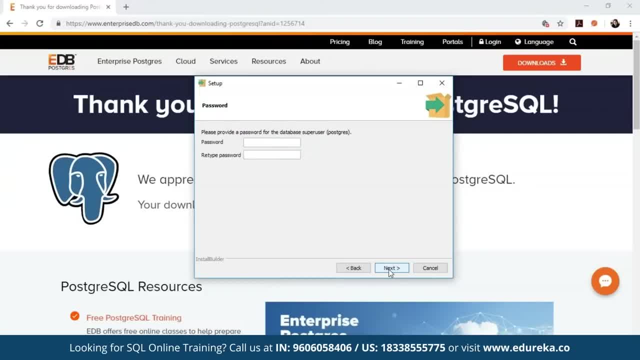 So I'm going to let it be as it is and then I'll click on next. once I click on next, I have to mention my password for the database super users. So just mention the password, any password that you wish to, and please remember the fact that you know. 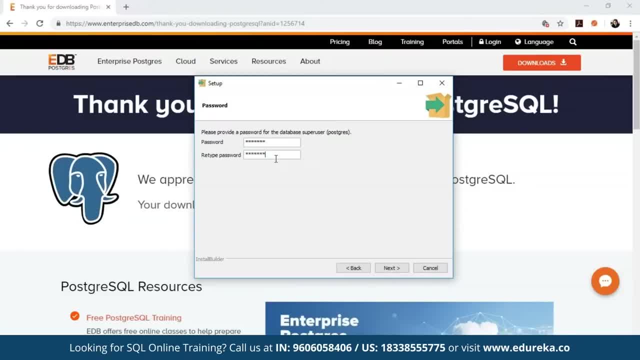 you have to remember this password to configure your server right. So do not forget this password and please make sure that you remember this password. after that, just click on next again, and then you have to select the port number. So I'm going to let it be as it is. 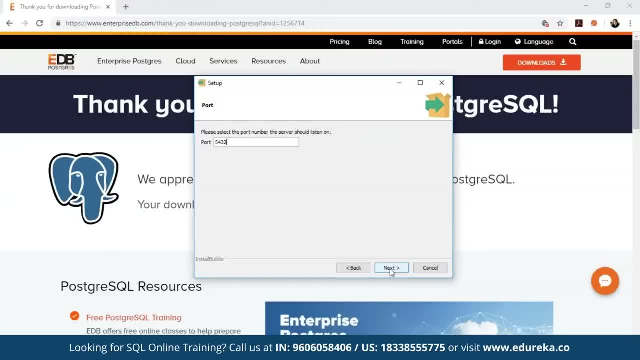 So basically, my server will run on the port 5032 and then I'll click on next. once I click on next, you'll see that you know I can choose the default local to be used by the new database cluster. So I'm going to let it be. 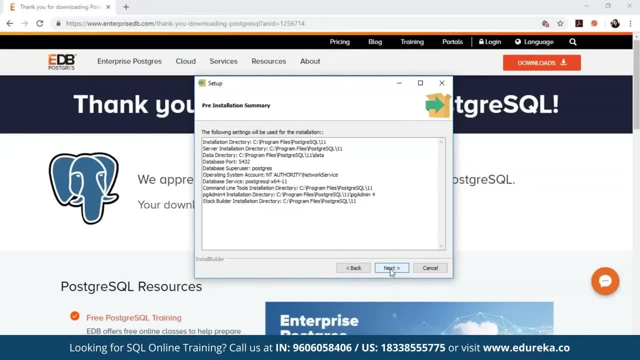 as it is and then I'm going to click on next. once I click on next, you'll see that you know, basically the following setting will be used for installation. that is basically. whatever you have selected till now will be shown over there. That is the installation directory. 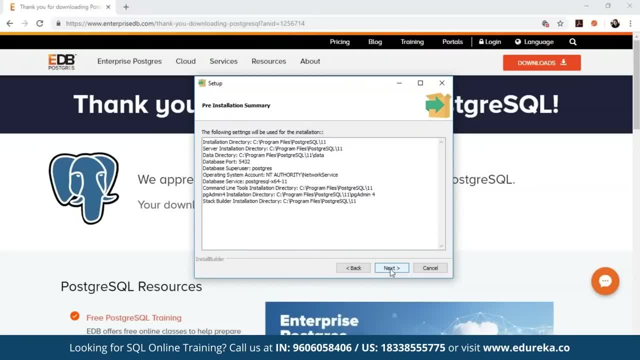 the server installation directory, the data directory, the database port, the database super user and so on right, and then I'll click on next over here again, And now you'll see a confirmation that you know. the setup is now ready. to begin installing Postgres SQL. 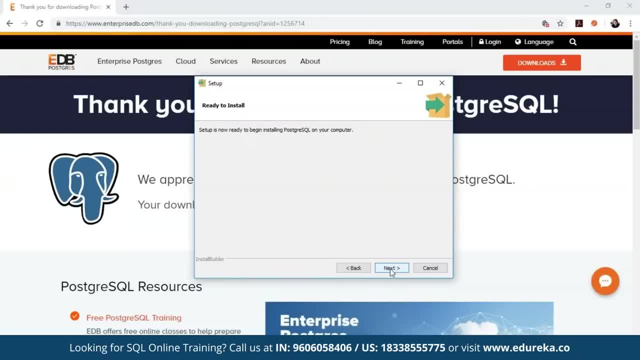 on your computer. If you're fine with it, you can just click on next. else You can just go back, make the changes and then again come back to this particular dialog box, right? So I'm fine with it. So I'll just click on next over here. 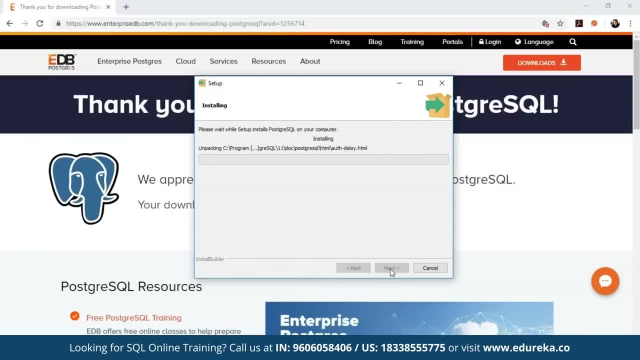 and then you'll see that you know Postgres SQL is getting installed on my sister, So let's wait for it to install. All right Now. once the installation is done, you get a confirmation wizard that you know the setup is finished installing Postgres SQL. 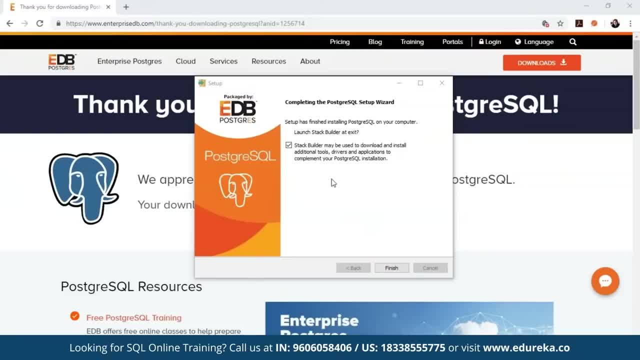 on your computer right, so you can just click on finish and then if you want to launch the stack builder at your exit, you can just check in this box. but I'll just uncheck this particular box and then I'll click on finish once I click on finish, basically. 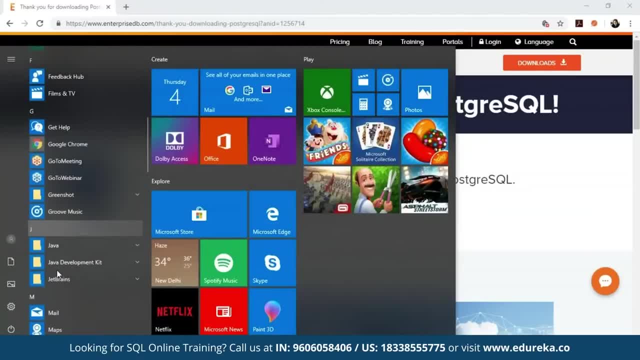 guys, your installation is done. now, if you search for Postgres SQL on your system, you'll clearly see options of the various stuff that we have installed right. So, as you can see on my screen, we have PG admin, We have the sequel shell. 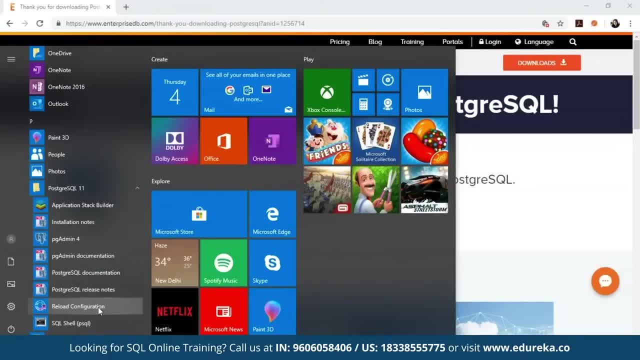 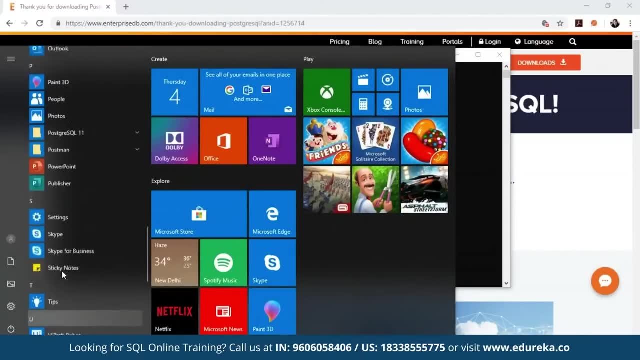 We have the documentation, the PG admin documentation to release notes and so on. right, So what I'm going to do is I'm going to open the sequel shell and also the PG admin, So let me just open. All right, Now, once you open the PG admin, 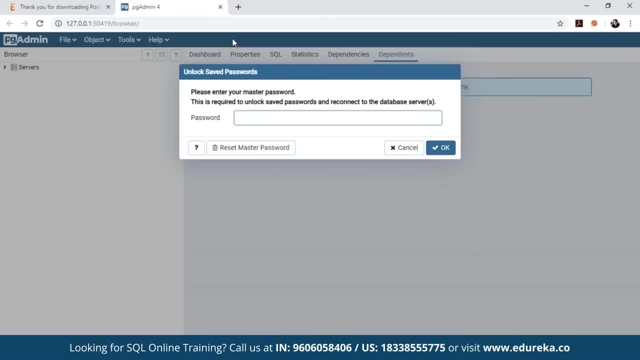 you basically are asked for the master password. So, if you remember, while installing I asked you to enter a password, right? So that's basically the password that you have to mention over here. So I'll just mention my password Right now. once the password is enter, you'll clearly see. 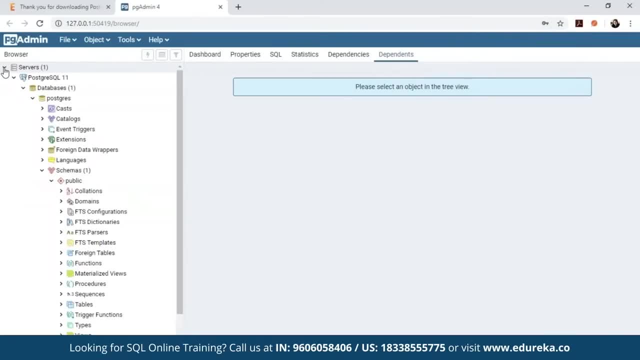 that you know we have a server and then automatically the server gets connected to databases and the super user database that is Postgres, right under this particular database. What we're going to do is we're going to basically use the different commands, that is, the different sequel command categories. 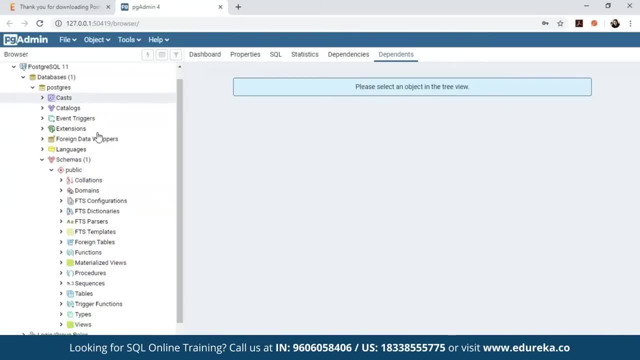 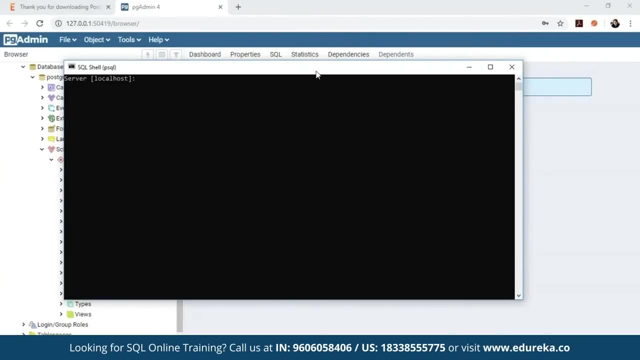 and then we're going to create a schema table and then we go to choose how we can play around with databases, right? So on the sequel shell, what you can do is you can again similarly connect to the server. So you just pass, basically have to click on enter. 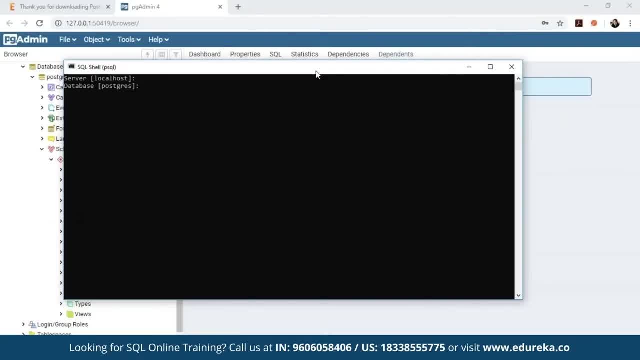 because you're connecting your server on the local host, So I'll just click on enter that the database, basically the super user database, is Postgres, So I'll click on enter again. The port has to be the same, that is 5, 4, 3, 2.. 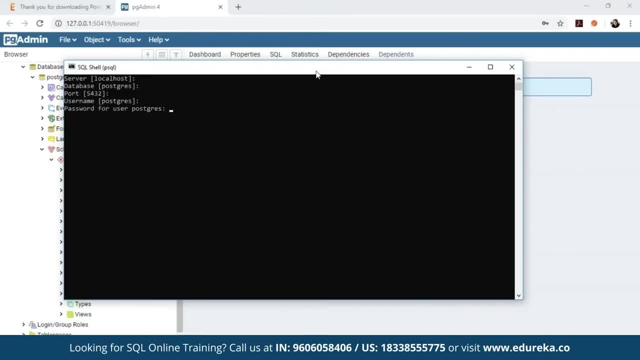 I'll click on enter again. The username will be Postgres. So I'll just click on enter again and password is basically what password you mentioned while installing right. So you'll mention the same password and then you'll see that you know. once you hit on enter, you'll clearly see. 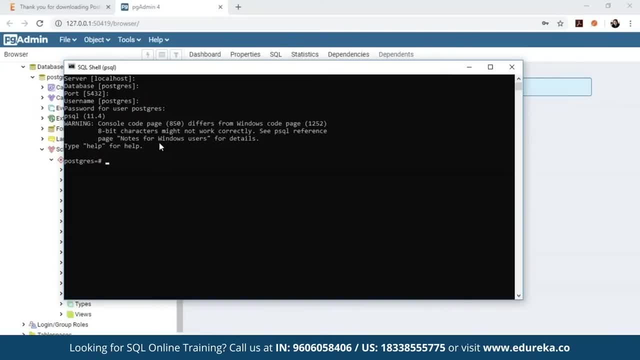 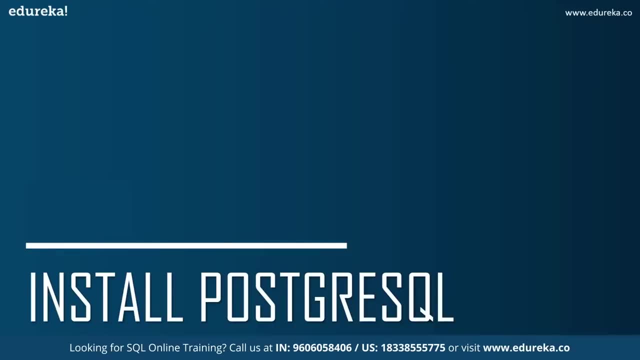 that you have been redirected to Postgres. So, basically, that's how, guys, you can configure server either on the PG admin and also on the sequel shell. So, guys, that was about installation of Postgres sequel on Windows. I hope you've understood all the steps. 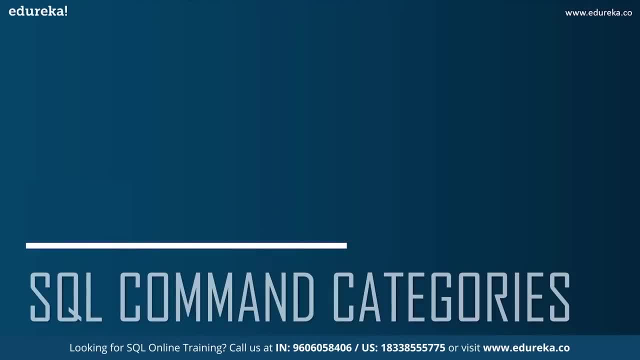 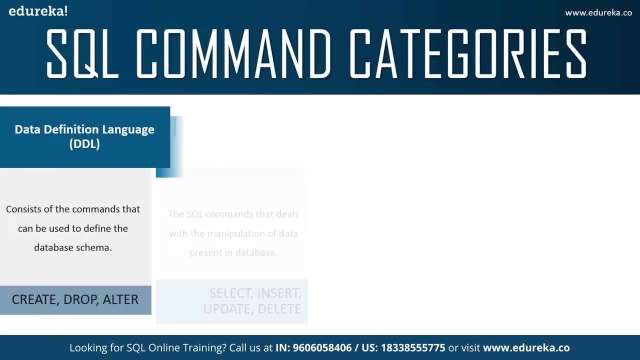 So, now that you've installed Postgres sequel on your system, next Let's look into the sequel command categories. So, as I said, there are mainly four command categories, that is, the data definition language commands, the data manipulation language commands, the data control language commands. 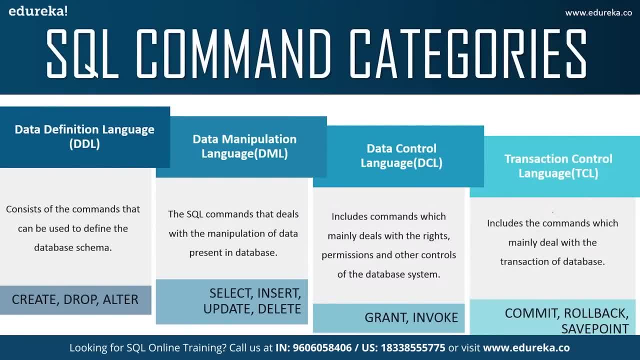 and the transaction control language commands, right? So basically, guys, these are the main four command categories of sequel, That is, the DDL commands, the DML commands, the DCL commands and the TCL commands. the DDL commands basically consists of the commands which can be used to define your schema, right? 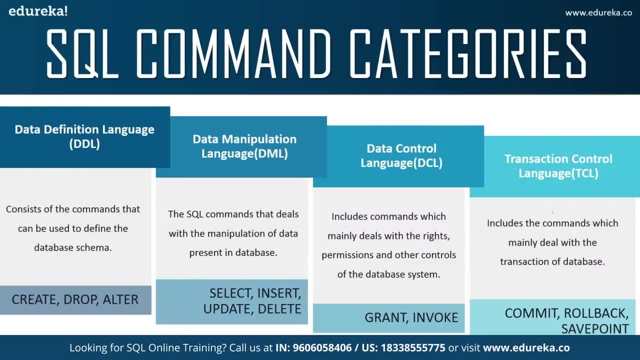 So you can create a table, you can create a schema, you can create a view and so on. So basically all those commands which define the database of the schema, basically how your data has to be represented and what would be the way this table- So maybe let's say which table- will be related to other table- 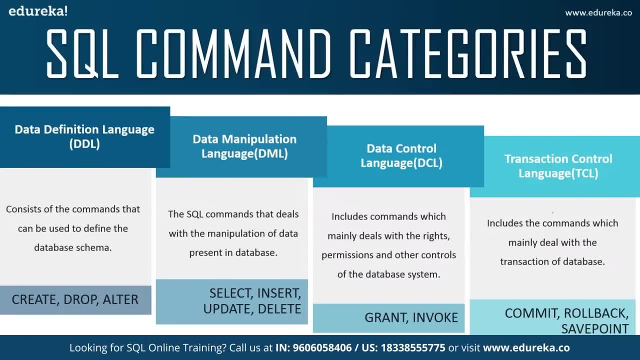 and so on will be all under this particular section, that is, the data definition language commands. coming to data manipulation language commands, the DML commands basically consists of those commands which deal with the manipulation of data present in the database, So all the manipulation that you'll do in your databases. 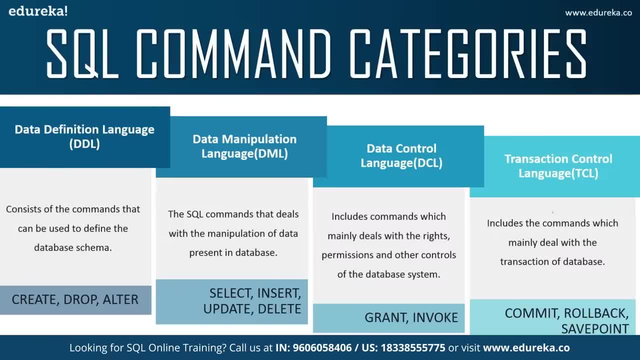 will be with the help of the data manipulation language commands. coming to the data control language, The data control language commands basically includes those commands which deal with the rights, permissions and other controls of the database system. like you know which database has to be granted. 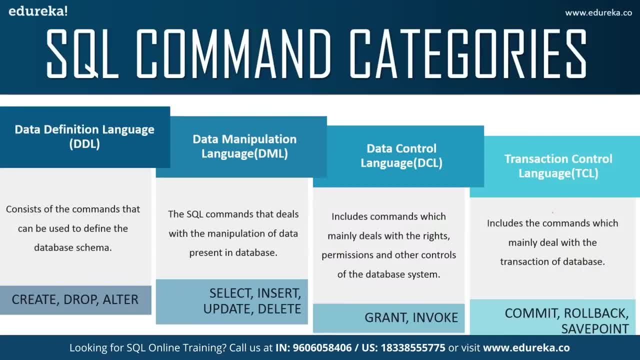 to any specific user, or maybe that particular database will be open to public, and so on. and finally, coming to transaction control language commands, So the transaction control language commands basically include those commands which mainly deal with the transaction of the database. So, guys, these are mainly the four different command categories. 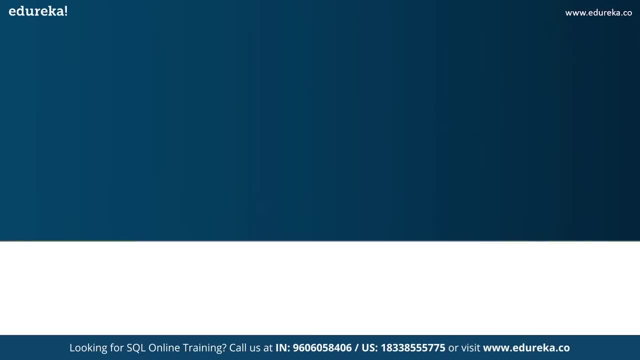 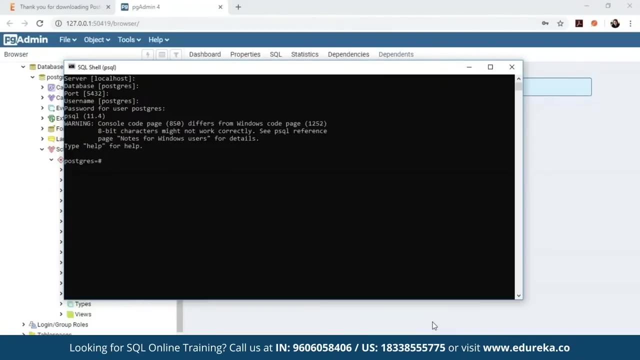 that is, the DDL, DML, DCL and TCL. So, without wasting any further time, let's look into the DDL commands. Now. what I'm going to do is I'm going to show you how you can write commands on the sequel shell. 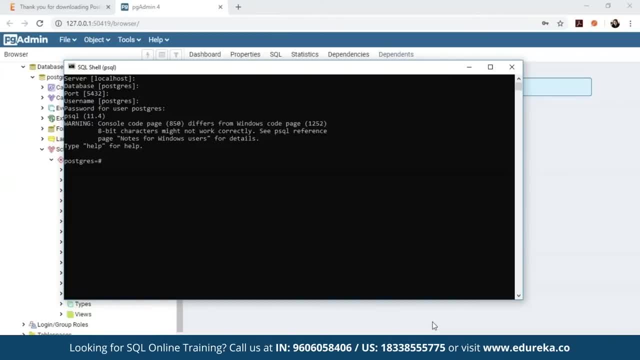 and then I'm going to use the PG admin right, So it's really simple. PG admin is the GUI for posters sequel in today's market. in Industries, People are mostly using PG admin because you know they can connect this particular database to various other external tools also, so that you know. 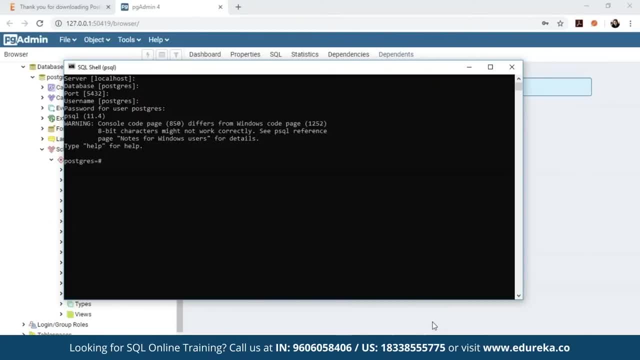 they can manipulate the data and maybe they can generate reports and so on. right, So I'm going to initially show you how I can SQL shell for few commands, and then I'll completely shift over to the GUI. So now let's say: you know? 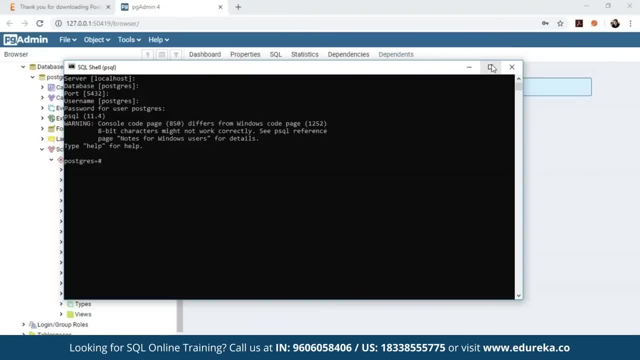 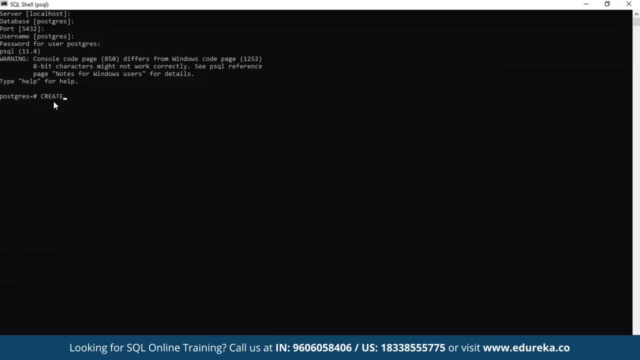 you want to create a screamer. How do you think you can create a schema? Well, the command is really simple. for that You'll have to use create, right? So what you'll do is basically you'll type in create schema and let's say, we mentioned the schema name. 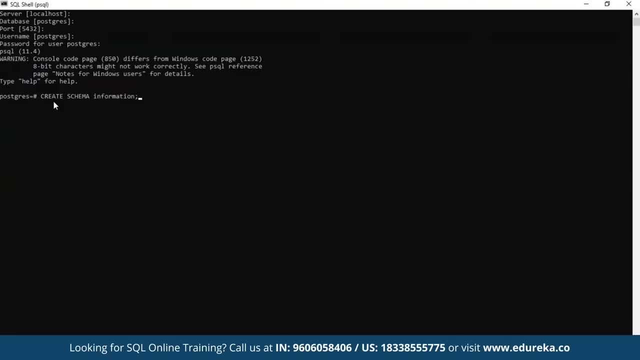 to be information, right, Right. so I'm going to use caps so that you understand that. you know that's the particular syntax and the small case letters to understand. that's the name That I'm giving and that's completely your choice on how you wish to do. 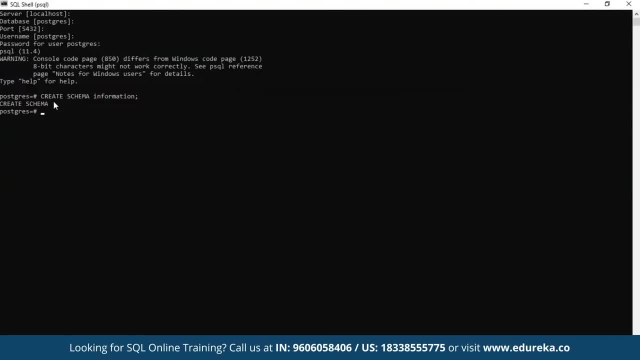 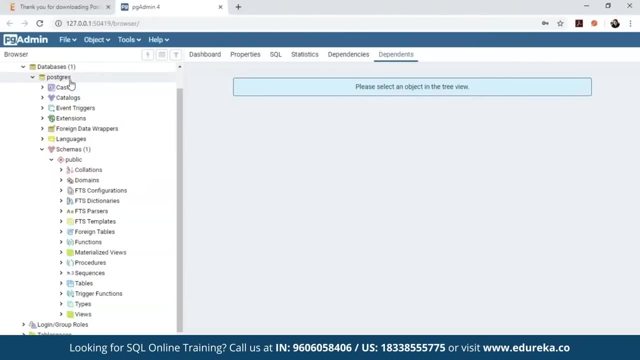 and then I'll end with a semicolon and click on enter. Once I click on enter, you'll see an output that you know: create schema. That means you know a schema has been created. Now, if I go back to my PG admin. 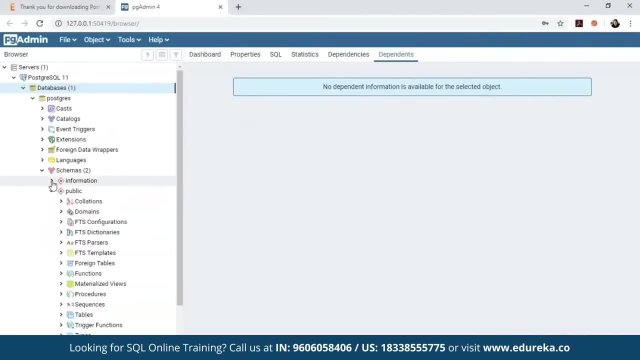 and then let's say, you know, I just refresh over here, So automatically you'll see a schema. that is information, right? So basically, whatever I've created in SQL shell is automatically seen in PG admin, right? So that's the reason I told you, it's easy to visualize. 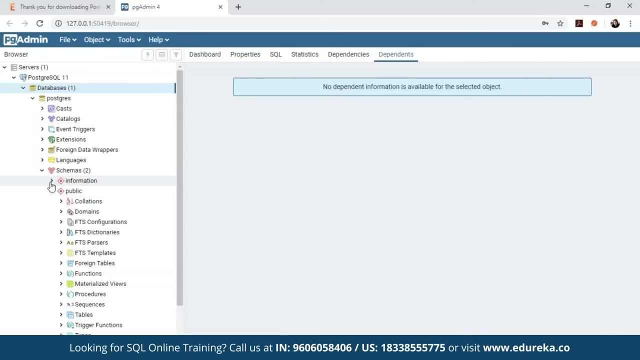 and use It's GUI over here Now. similarly, if you wish to create a new schema over here, what you can do is you have the schema option right. you right click over here, choose, create and choose create schema automatically. You just have to mention the name. 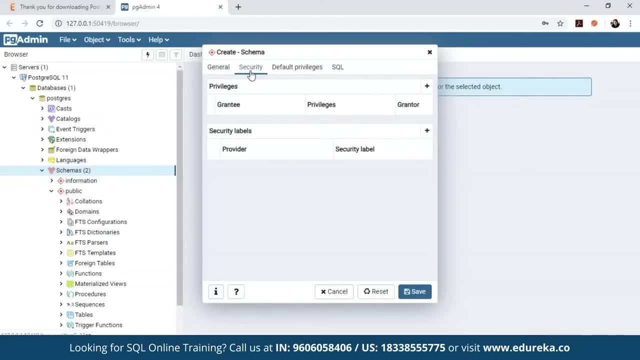 Let's say I mentioned sample and then I'll leave the other details to be the same, that the security default privileges and sequel right. So in sequel you'll basically see that you know the syntax that I just mentioned in the sequel shell, that is, create schema and then schema name. 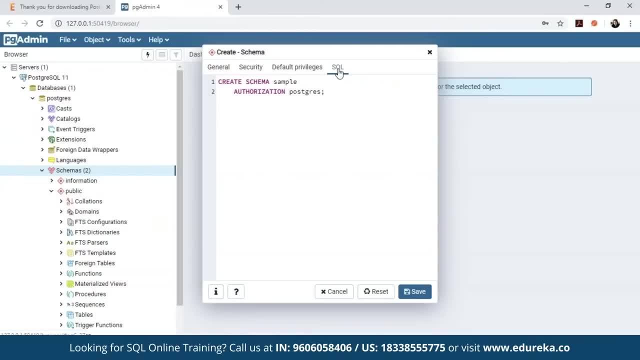 and authorization. Postgres, That's basically a database super user. Well, that's by default in sequel shell because you know we are already under Postgres. So that's the reason we didn't have to give it over there. So I'll just click on save. 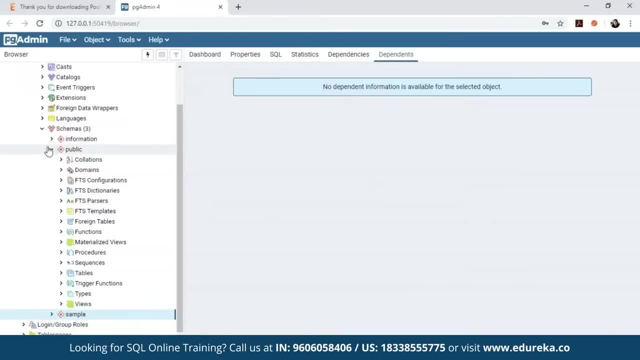 and then, once I click on save, you'll automatically see that a schema has been created that is basically sample. So now I have the information schema, the public schema and the sample schema. Now the public schema is created by default and the information was the one that I created in sequel share. 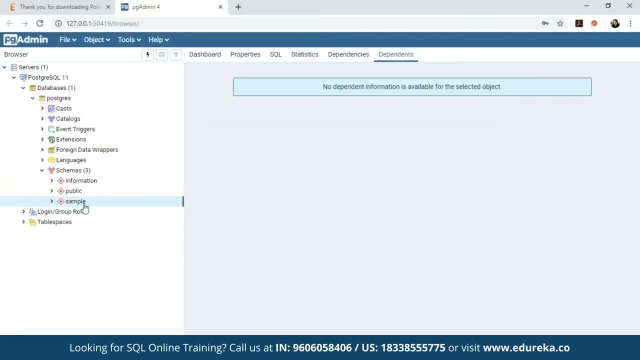 and the sample is the one I created in GUI, So you see right how simple it is. now, If you're getting confused how you can write queries in GUI, Well, don't worry, We have a query tool also. So if I right-click over here, 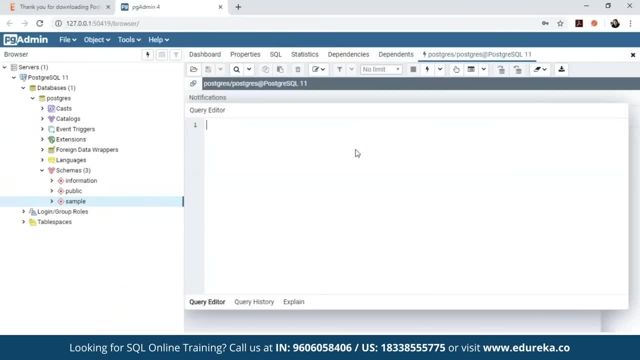 and then if I choose query tool, you'll see that you know, automatically you'll get a workspace where you can basically put all your queries. I'm not going to do that now. next, what I'll do is, let's say, you know, we want to use this particular schema. 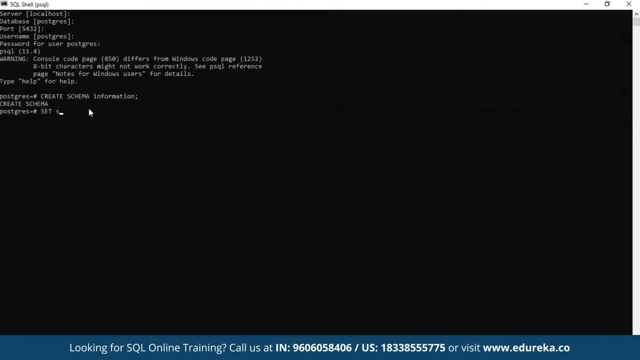 So what I'll do is I'll just type in the query set search path to, and then I'll mention the schema name, right? So I'll mention information Over here. So automatically you'll see an output that you know it is set to information, right. 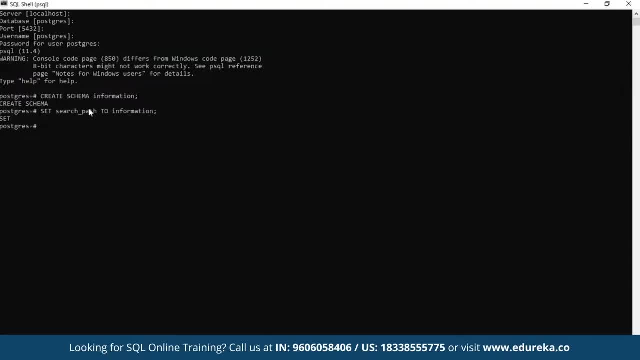 So, whatever actions that I wish to perform- like you know, creating tables or maybe views, and all, all of them will be basically under this particular schema. Now, once the path is set, let's say you know we want to create a table right. 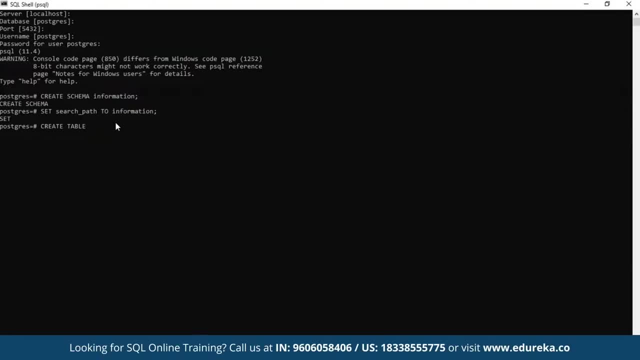 So for that you'll type in create table and then you'll mention this table name. So let's say I mentioned students and now each student will basically have various attributes, right? For example, let's say I am a student, now I'll have a name. 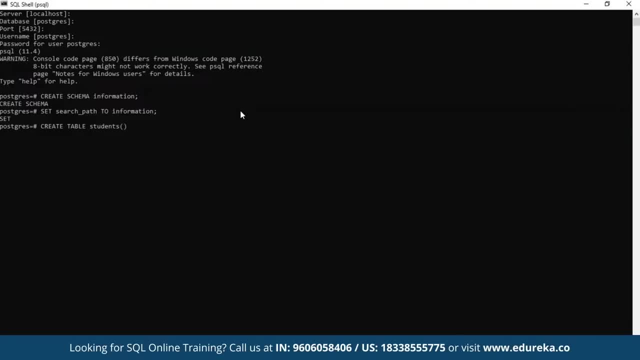 I have an age, I have a date of birth and so on. So basically all those values will be a column. So I'll just put it in brackets. and let's say I mentioned student ID and end to be data type and let's say further: 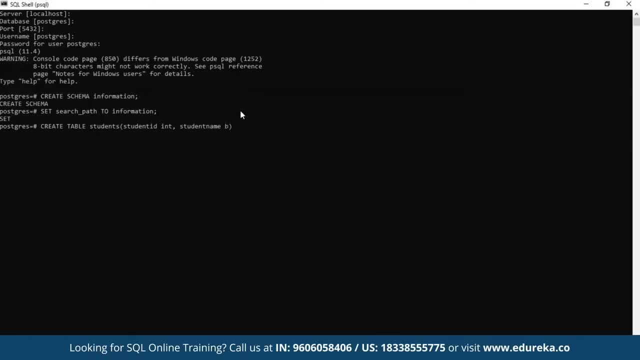 I again mention student name and then let the data type be where care: 255 characters, right. And then what I'll do is I'll put a semicolon at the end. Once I click over here, Once I click on enter, you'll clearly see an output. 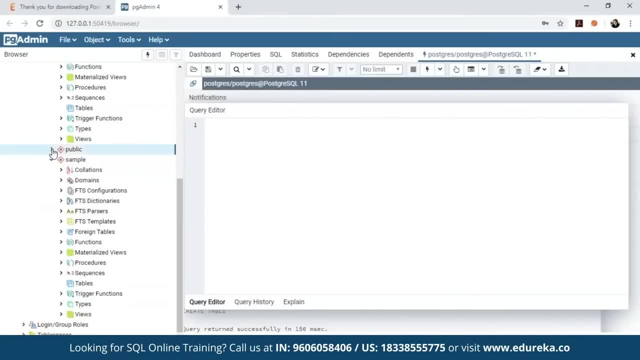 that you know. create table. Now let's go back over here and then let's just basically refresh the schemas, right? So I'll just refresh the schemas and under the information table You'll clearly see an output that you know we have a table students. 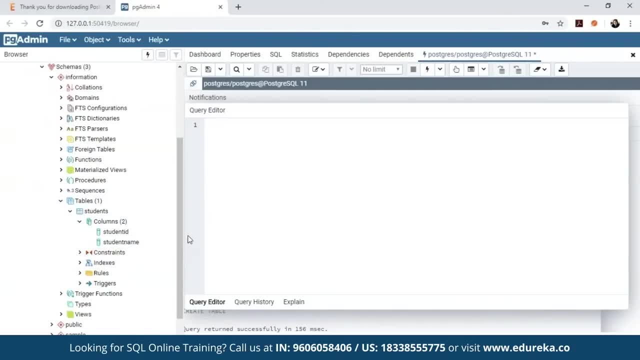 and then it has columns: student ID and student name. So basically, that's how you can create a table, basically on the sequel shell guys. Now if, similarly, if you wish to create a table in the PG admin, what you do is you right click on the table over here go. 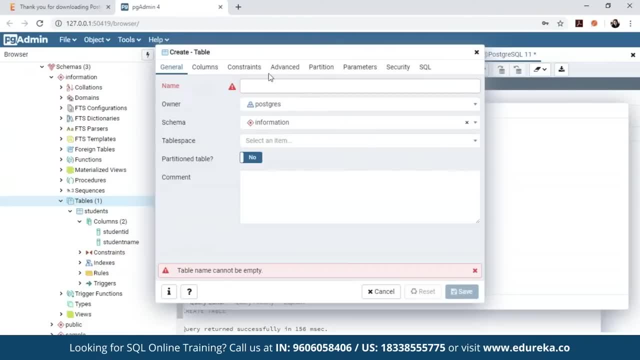 to create, choose table and then basically you have to mention the name, right? So, for example, let's say we mentioned the table name to be teachers and then the owner to be postgres, the schema to be information. So you'll have to basically choose the schema. 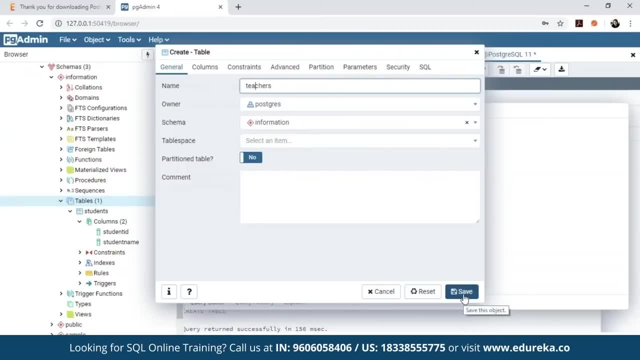 under which you wish to create the table and then you click on save. So if you click on save without choosing the columns, then remember that you know this particular table will have no columns. So if you wish to add columns, you can just add column over here. 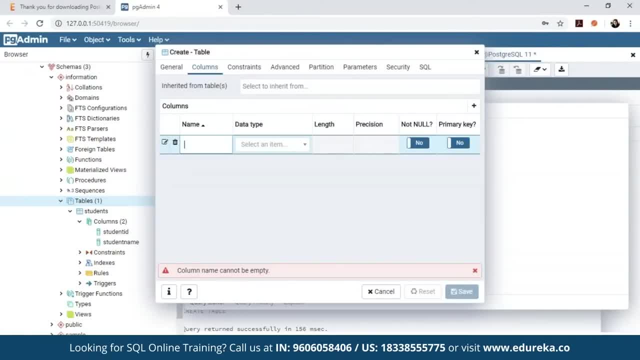 For example it's I wish to add column right, So I'll go to plus button over here, choose the name, Let's say you know teacher ID. Let's say data type to be int right, and then you know not null primary key and all. I'll come later on the session. 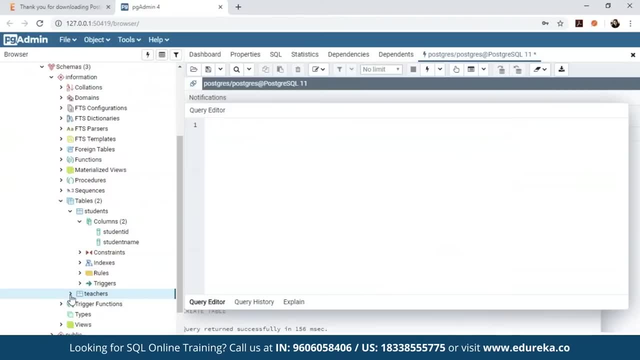 right, So I'll click on save over here. So once I click on save, you'll see that you know, automatically a teacher's table will be created with a single column that is teacher ID. So, guys, that's how basically you can create tables in the sequel shell and PG. admin. 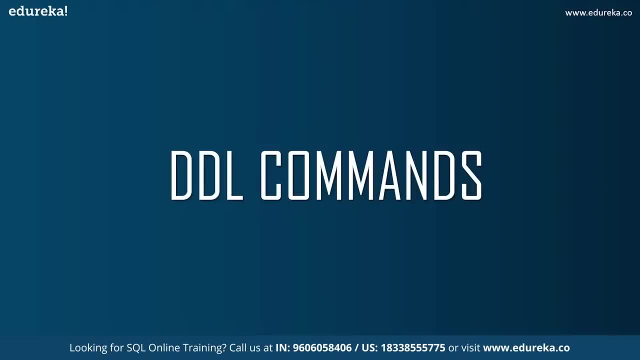 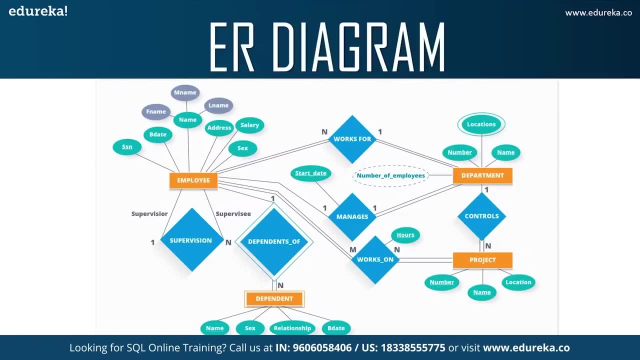 Now, before I move forward and show you the various other commands related to DDR, Let me cover a concept known as entity relationship diagram. Now, this particular concept is important over here because you know you have to understand how to create tables and how you have to relate those tables to the other tables. 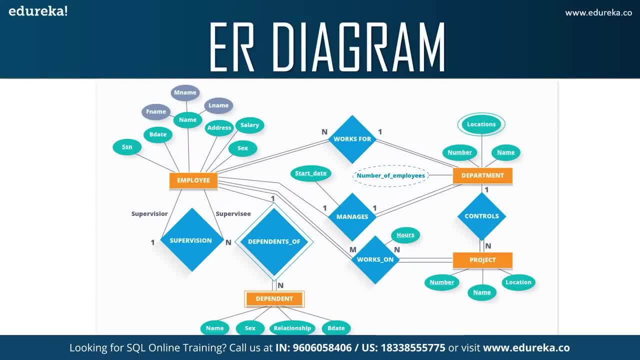 and basically what will be the column values for this particular table. So, as you can see on my screen, guys, this is the example for entity relationship diagram that I'm going to consider for this particular session. now, based on this particular diagram only, I'm going to basically take forward my session. 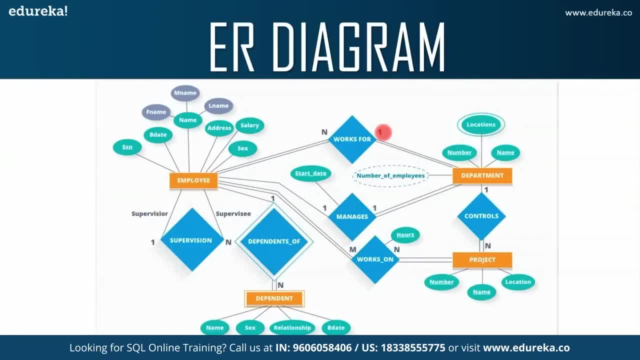 to show you the different commands also now. entity relationship diagram basically is a simple diagram through which you can understand the various relationships between two different tables or two or more tables, right, For example? let's say, you know we have this particular entity relationship diagram right now. 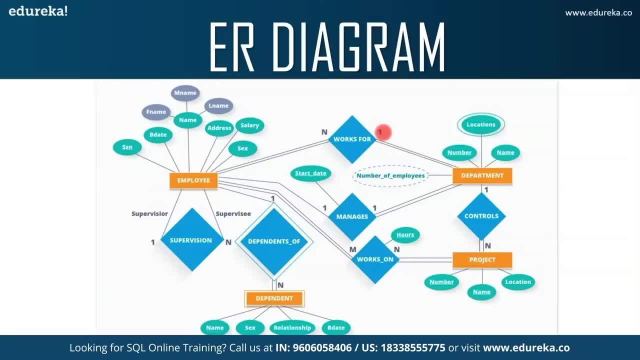 over here We have employee, department, project and dependent over here. Now all the rectangular boxes on this particular screen will represent entities. Now, what I mean by entities is basically that you know, for example, let's say, I'm a person right now. 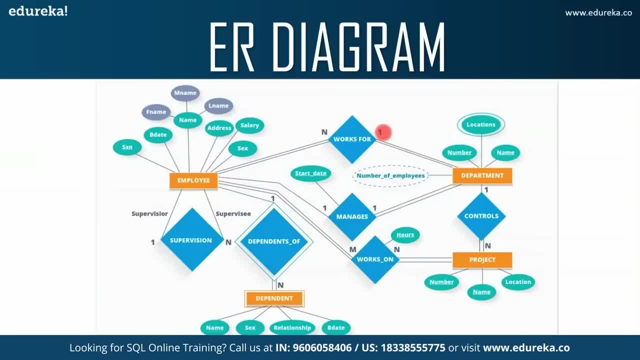 I have a name now. my name, my age, my phone number, my date of birth, my address- all these are basically my attributes, right, and I'm, as a person, can be unique, Identified with the help of these particular attributes, right? So whatever can be uniquely identified with the help. 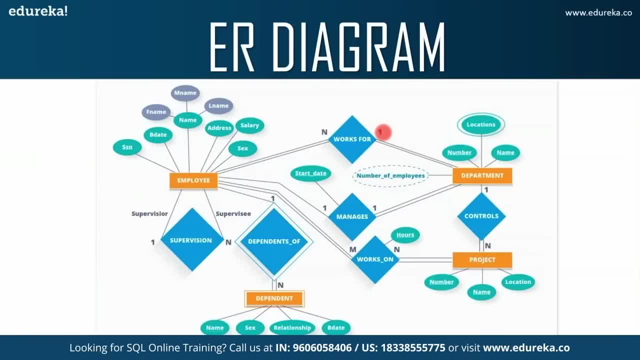 of attributes is basically entity, right, So I am an entity. So, for example, I'm sahiti, right? So my name, my age, my date of birth, all of this will be attributes through which anybody can identify me as sahiti. 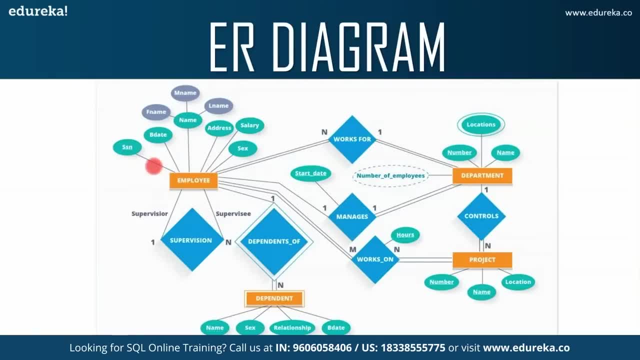 right. So over here any employee can be uniquely identified with the help of an SSN. That is basically a social security number, or you can simply understand as ID name, now name. further can have the first name, the last name and the middle name. now address salary and sex. 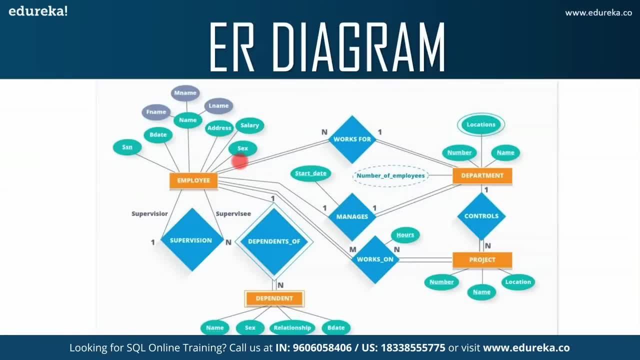 right. So basically, all these attributes can uniquely identify an employee, right? So employee over here is an entity and all these particular attributes are basically the factors to which you can identify. So when you build a relational database management system, what happens is that employee will become the table name. 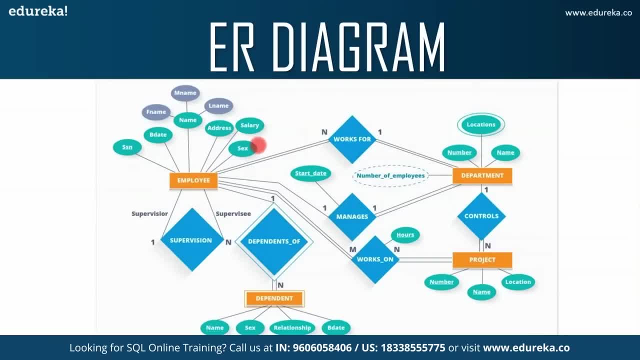 and all these particular values- that is basically the attribute values- will be the column names, right? So you'll have a column name with SSN, bird date, First name, middle name, last name, address, salary and sex, right? So all this basically will be your column name. 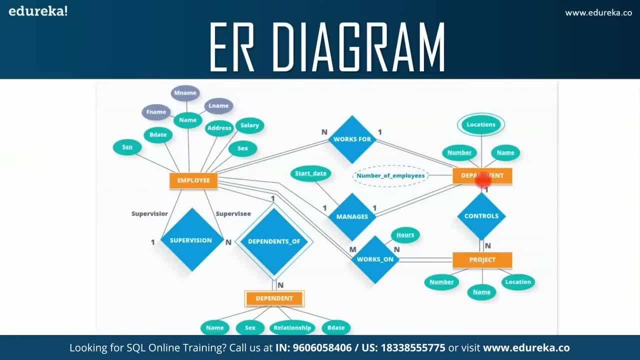 and then employee will be a table name. now, similar is the case with the other factors also. for example, if you take Department now a department can be uniquely identified with number and name right. So these two will be attributes and the locations is basically a multi-valued attribute. 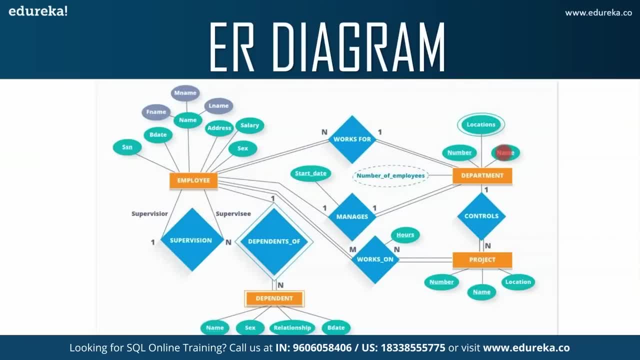 Now, when I say multi-valued attribute, what I mean by that is, an attribute can have various factors, right? For example, let's say location, What will be your address? You can have so much of Street. Let's say, you know 5th Street, 4th Cross Road, and let's say Queens Road. 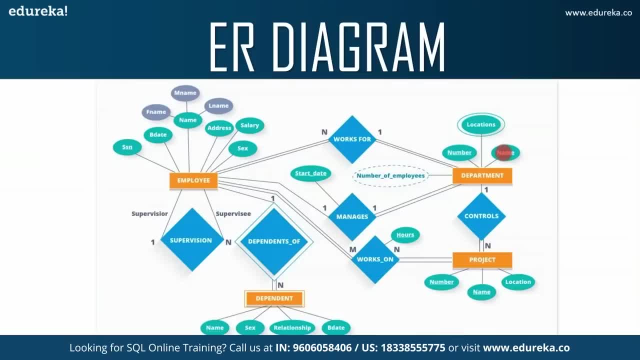 right. So this could be basically your location right now. This has various attributes, like you know. maybe you can have 5th Street, like the streets can be put into one value, and maybe the Queens Road, basically the main locality, can be another value. 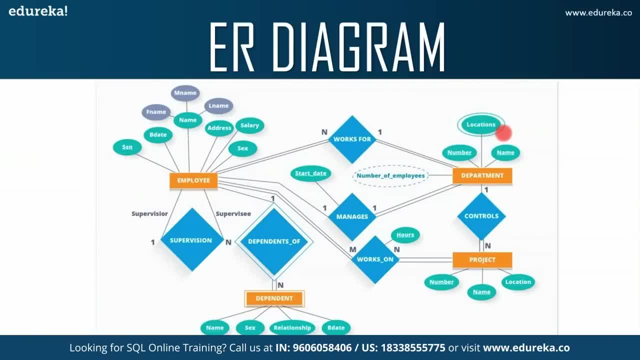 right. So basically it's a multi-valued attribute. That's what basically double ellipses me. apart from that, Also, please remember that even this particular attribute will be included into the columns part, So you'll have a department table with the department number. 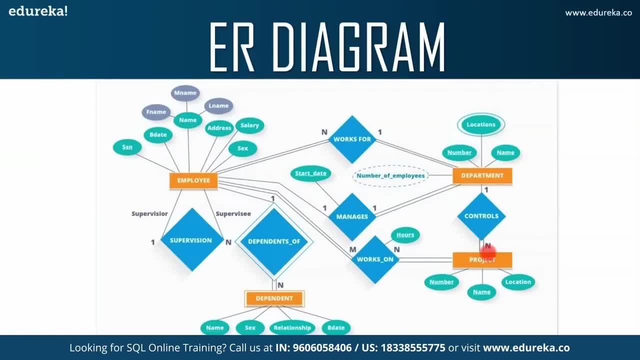 and department name as columns now. apart from that, next Let's look into project. The project is again another entity, right? So every project can be again uniquely be identified with the project number and the project name and the location. right now We are the project number. 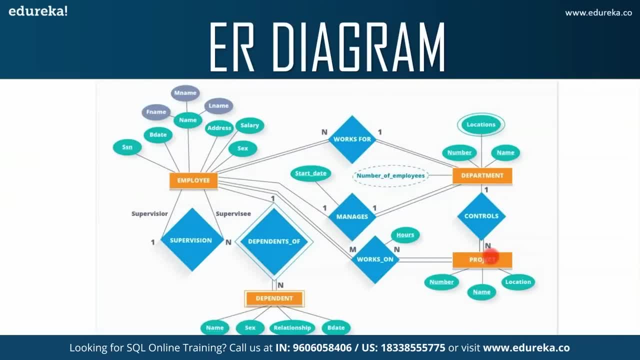 and the project name will be unique for each and every project. So that is the reason for every entity, for this particular entity. These two attributes are very important over here, because every project can be uniquely identified with the project number and the project name. and finally, coming to dependent, 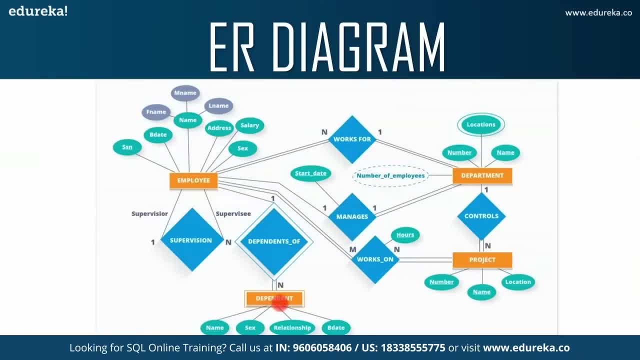 Now you must be wondering over here: Why does the dependent entity have two rectangles right? That is because you know it is a weak entity. What I mean by weak entity is basically that you know the dependent entity is basically dependent on the employee entity. 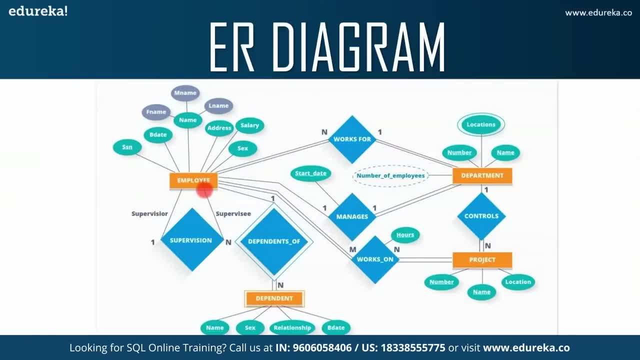 right. For example, let's say: you know I as an employee- right, So I am an employee. and then maybe I'm going for an insurance- right, And then I have an health insurance. who, in my next nominee, let's say, is my sister? 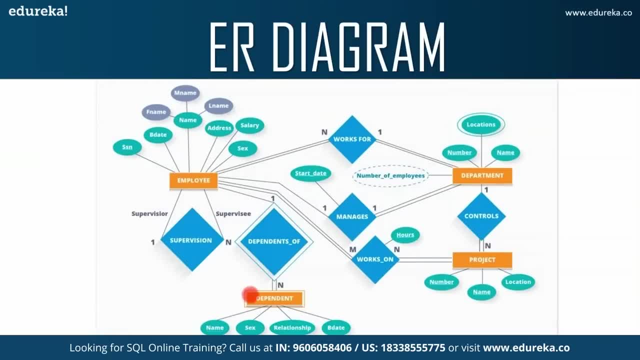 So what happens over here is basically that you know this particular entity is dependent on the employee entity. My details will be basically taken from the employee entity, right? So, for example, let's say I am an employee, then all my details will be taken. 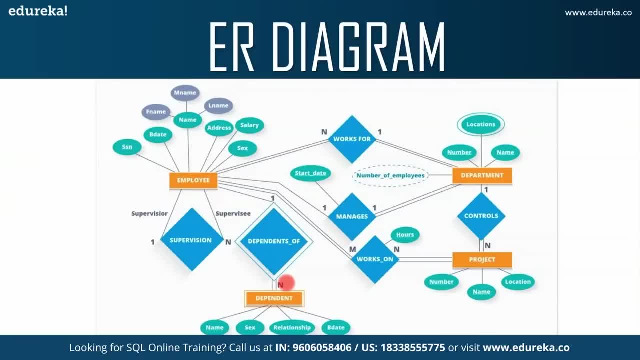 from the employee entity, right? So that is the reason. basically, the dependent entity is completely dependent on the employed entity. So that's what you have to understand over here. When I say weak entity, you have to understand that unit is dependent on any other particular entity. right now, over here. 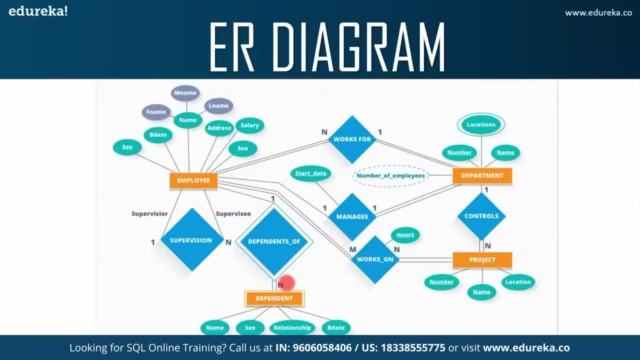 I hope you understood what is entities and what is attributes. next, If you look into the diagram, we have ways of the factors, like you know, these diamonds, and then we have double lines, We have single lines and so on. right, So let's look into what they are. 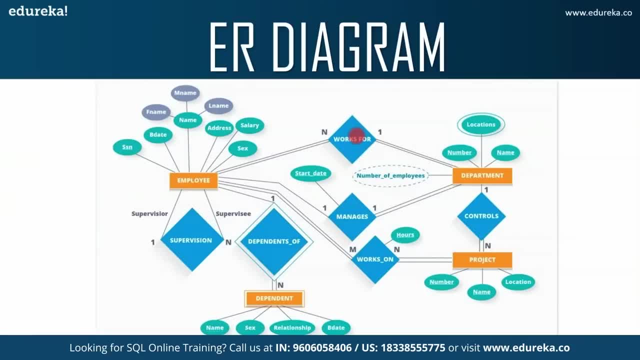 So, coming to diamonds over here, when I say diamond what I mean by that is that is basically the relationship set. So what is relationship set? So if you have to understand this, then you can understand that. you know employees are related to every department, right? 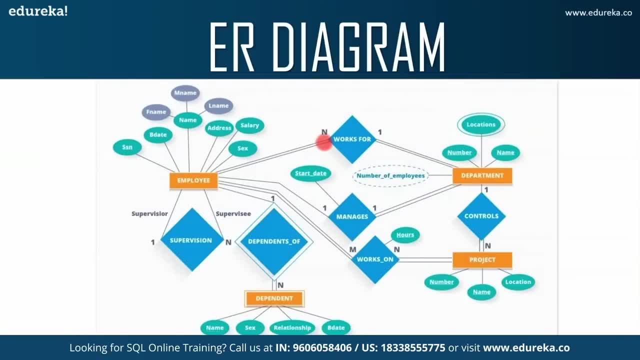 So if you take your company, any number of employees, like you know, more than one instance of the entity is basically associated with one Instance of the department, right? So in simple terms, if you just have to understand it like, let's say: 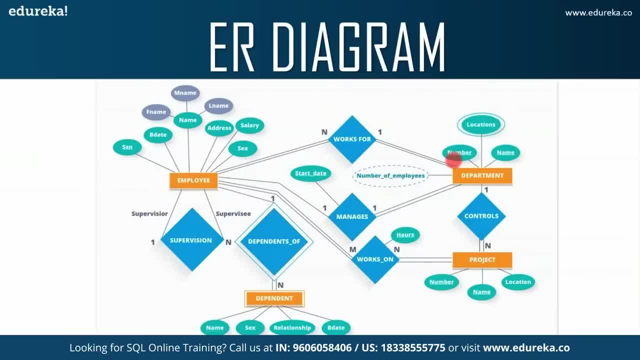 you know, 10 employees are working in one particular department, Let's say IT department. So that's how, basically, you can understand this. now, coming to the next relationship, that is, manages. now There's a relationship between employees and department, also right. 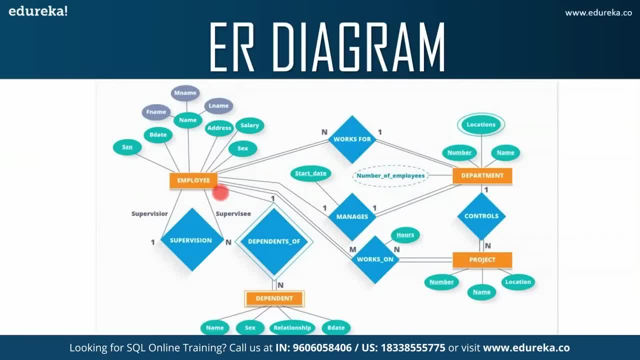 So there is a department and then there is a manager for each and every department, right? So now not all employees are managers for the departments, right? So it could happen that, you know, only one instance of the employee entity is basically associated with one instance of the department entity. 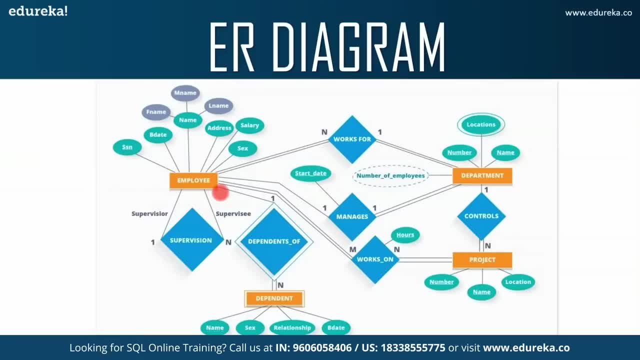 right? So let's say, now we have the IT department. now, Now the IT department can basically have only one manager, the HR department can have only one manager, and so on, right? So basically all of them are also employees, right? So that is the reason there is a relationship between employees. 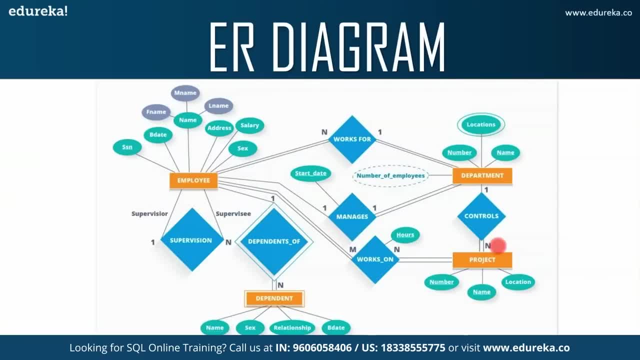 and department over here. now coming to the next relationship that is works on now. It is obvious to the fact that you know all the employees must be working on some of the other projects, right? For example, let's say you know 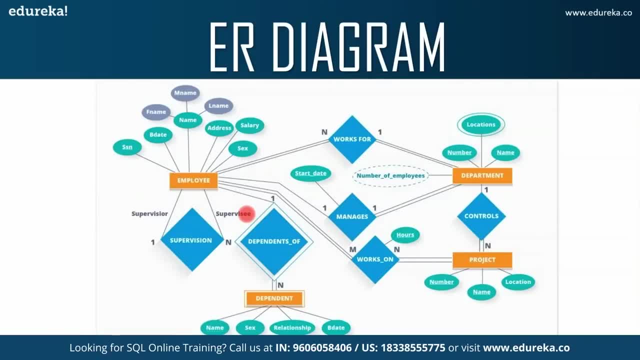 we can have 10 employees working on Two projects, or maybe you know the same number of employees working on some other projects also. right, It's never that in industry, that a single employees working only on single project and not more than one project. 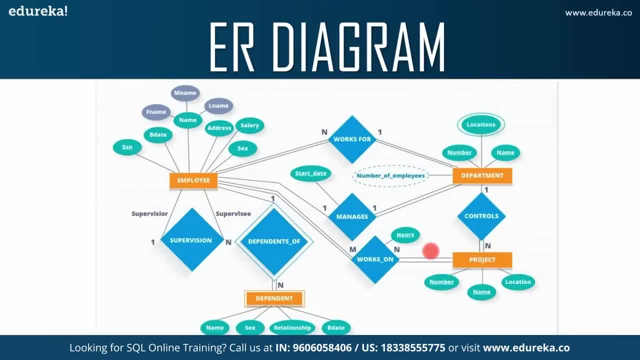 right. So in this particular relationship- that is the reason we have M- is to end basically by that. what I mean: that you know, more than one instance of the entity employee is basically associated with more than one instance of the other entity, that is, the projects entity. 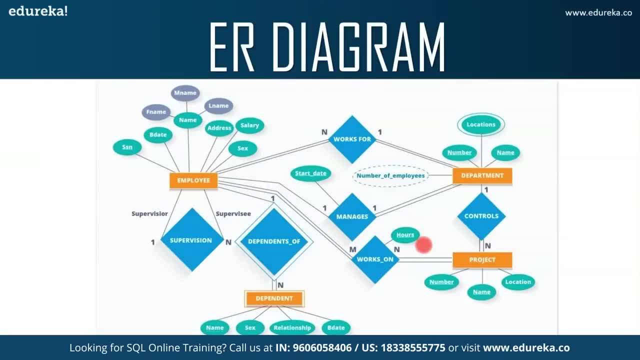 right. So that is because any number of employees can work on any number of projects. Similarly, let's look into the next relationship, that is, dependence of. what I see in the relationship of dependence of is basically one is to end. that is because you know. 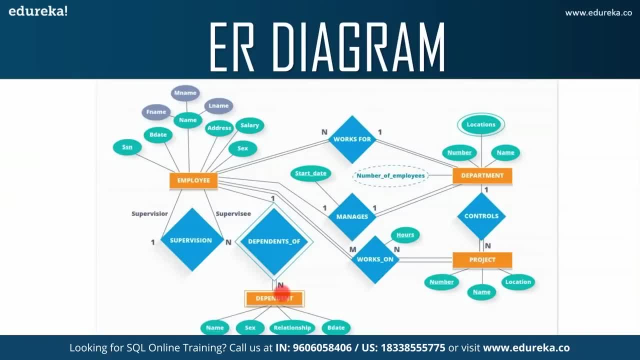 one employee can have any number of insurance. right, You can have a life insurance and so on. So that is the reason: basically you have one is to end relationship. and then you have the relationship of dependence of, because your dependence entity is completely dependent on the employee entity. and finally, coming to self referencing, 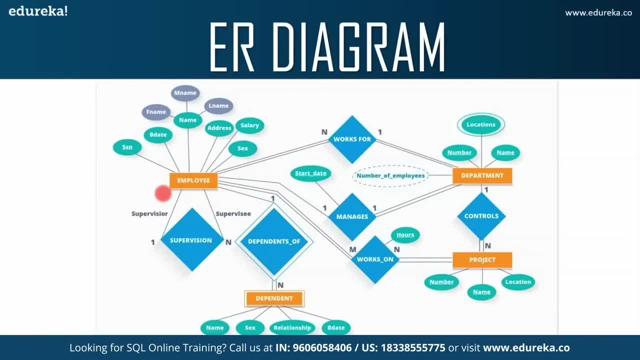 relationship over here. What I mean by self referencing relationship is basically that you know, for example, let's say you have a boss right now. your boss can handle 10 people right, So basically he's your supervisor and then he supervises 10. 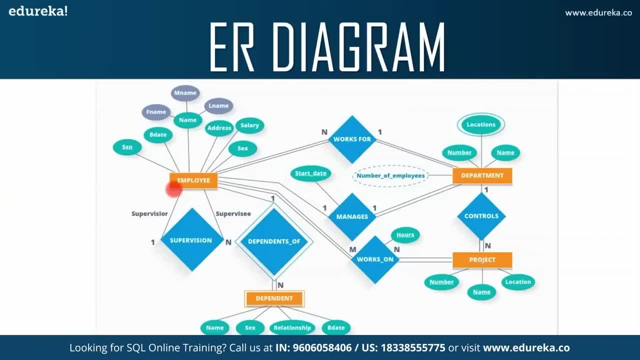 people, right, and he himself is also an employee and all the 10 people are also employees, right. So that is where this particular relationship comes into picture. that is, one is to end, right. So one instance of the employee, where employee is basically a supervisor, can supervise more than one instance of the other. 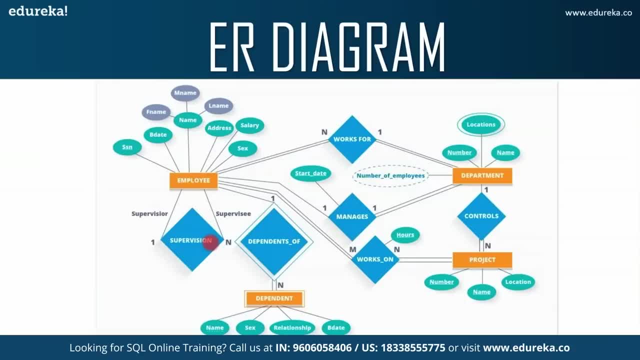 employees right. So basically that's how it happens is. you basically have different relationships like this, guys. If I have to just summarize the different relationships, then you have: one is to one, one is to end, n is to one, m is to end, right, and then you also have self referencing relationships. 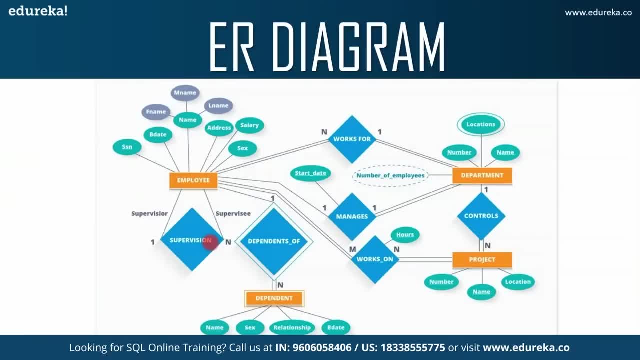 So if you have to talk in technical terms, then you have one to one relationship, one to many relationship, many to one relationship and many to many relationship. apart from that, We also have the self-referencing relationship that I just spoke about. now, if you observe, the complete entity relationship. 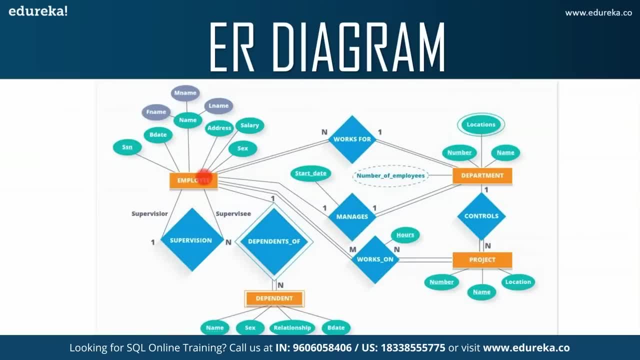 diagram over here. So I hope you've understood How entities, attributes and relationship works in the databases. right now let's look into the double lines over here. What do you think the double lines mean? What I mean by total participation is basically that you know. 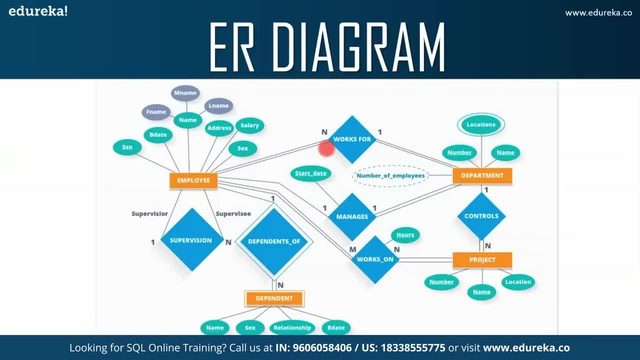 each entity in the entity set must at least have one relationship in the relationship set. So basically, each entity in the employee must work in some of the other Department, right? So that is the reason we basically have total participation over here. moving on to the next relationship, 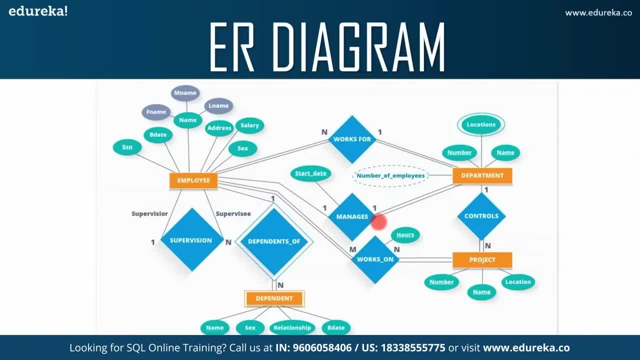 You can see that. you know it's not necessary That every employee manages some of the other person, right? So that is the reason we don't have total participation on this particular side. But, yes, every department has a boss, right. 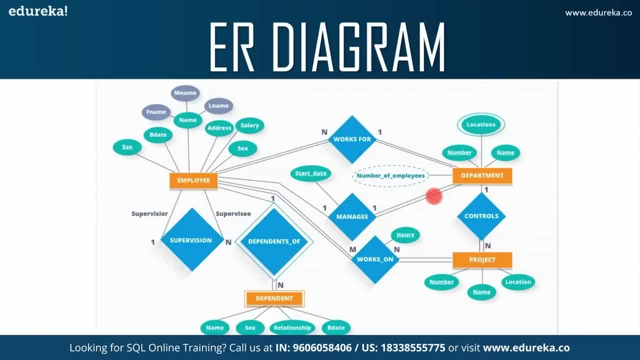 So every department has a manager. So that's the reason we have total participation on this particular side, that is, from managers to Department. moving on to the next relationship, That is basically employees to project. If you see, every employee has to work on some of the other project. 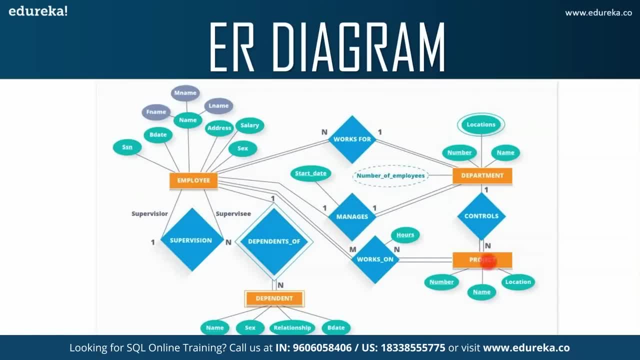 right? So that is the reason we have total participation on both the sides that you know, every employee basically will be working on something or the other thing, and every project will have a set of employees working on it, right? So that is the reason we have total participation over here. 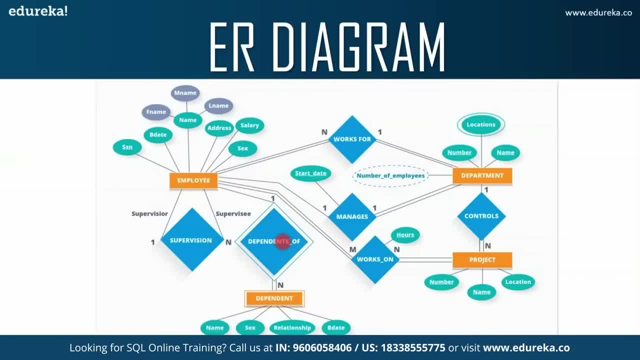 coming to the next relationship, You can clearly see that you know that the dependents are basically completely dependent on employees. So it's the total participation towards from the dependent side and not from the employee side, because then it can happen that, you know, maybe an employee doesn't have some insurance. 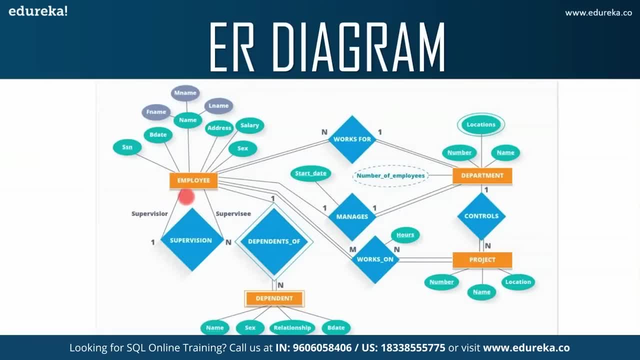 or maybe an employee doesn't have any insurance, right? So in that scenario, what basically happens is that you don't have total participation over here, but you have total participation On this particular side. and now, finally, coming to this particular relationship, If you observe over here, 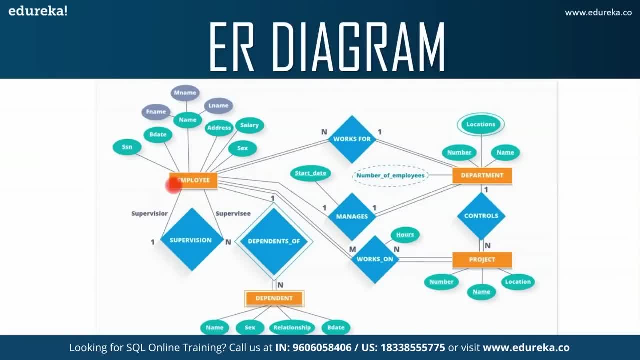 we do not have any total participation. That's because you know it's not necessary that every person in the employee table, Basically every person in the company, should be a supervisor of somebody. right, It's not necessary like that. Maybe a fresher is just not a supervisor. 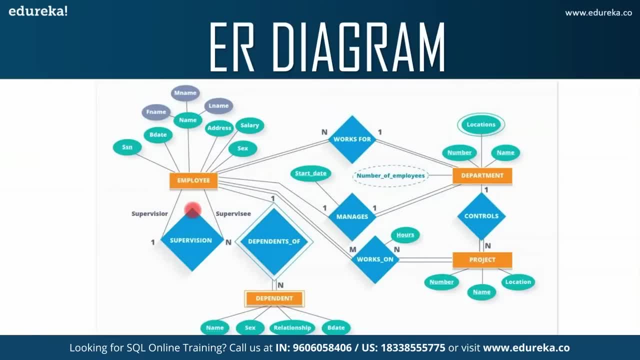 So in that scenario, basically total participation will not hold true. So that is basically, guys, how you can build up an entity relationship diagram for the scenario that you have. I took a company database where you know you have various entities like employees, Department dependent. 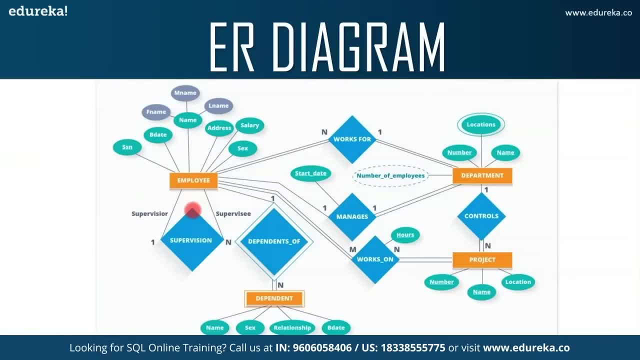 project, and then they are related to each other in some way or the other and each of these entities have various attributes. So remember the fact that you know, when you build a relational database, you have entities which will basically become your tables. then you have attributes. 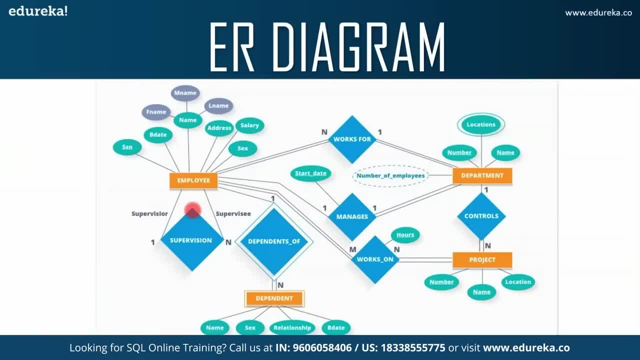 So your attributes will basically become your column names and then you have relationships. So, guys, this was all about entity relationship diagrams. You basically have entities, attributes and the relationships, Right? So I hope you've understood how my ear diagram looks like now, as I was talking about different kinds of attributes. 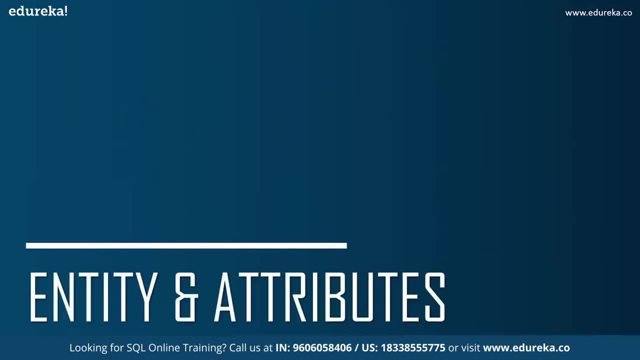 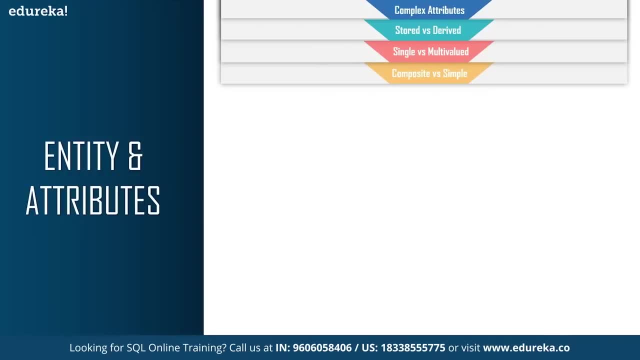 Let me next take you through. What are the different kinds of attributes that you see? So you must have observed, right? We had multivalued attributes, We had derived attributes, and then we have complex attributes and composite attributes. So basically, there are various attributes, like 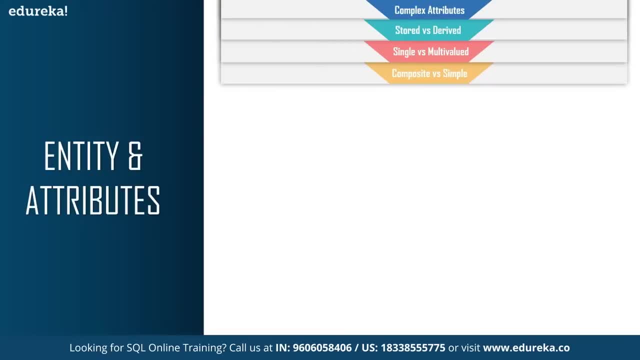 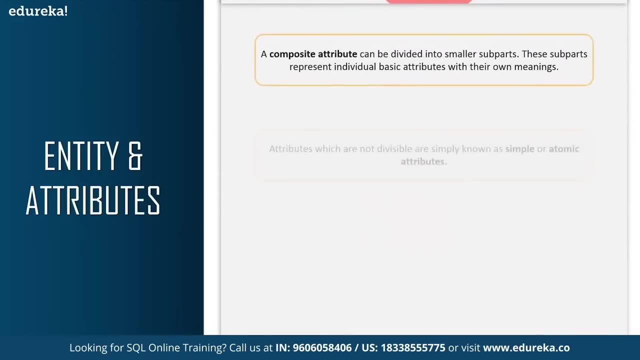 you know composites, simple, single, multivalued, stored, derived and complex attributes. So let's look into each one of them one by one. So, talking about composite and simple attributes, guys, if you remember the entity relationship diagram I showed you, I told you that the name can have first name. 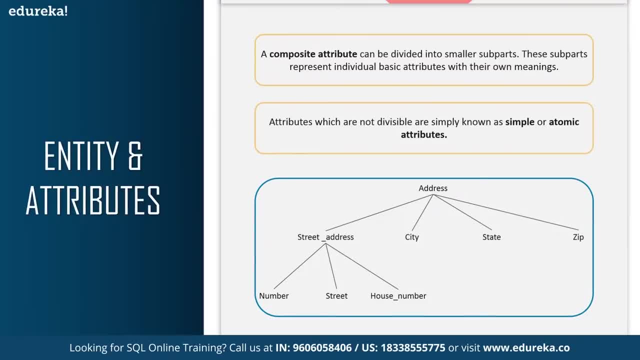 last name and middle name. the first name, last name, middle name will basically be my simple attributes and the name altogether will be my complex attribute. So basically, if I have to define in single terms, then a composite attributes can be divided into smaller subparts and these subparts can represent individual basic attributes. 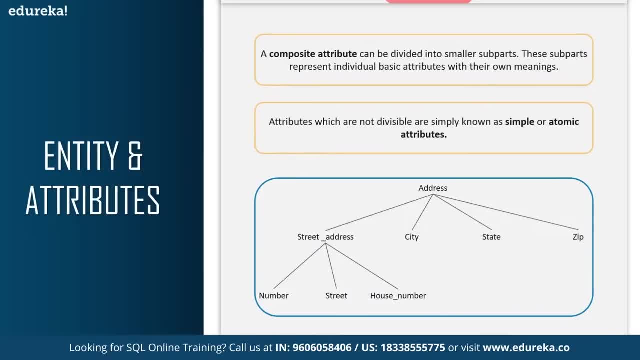 with their own meaning. For example, let's say we have address right now. address can have Street address, City State, zip and Street address can be further divided into number, Street and house number. now City State, zip, number, Street and house number will basically be your simple attributes. 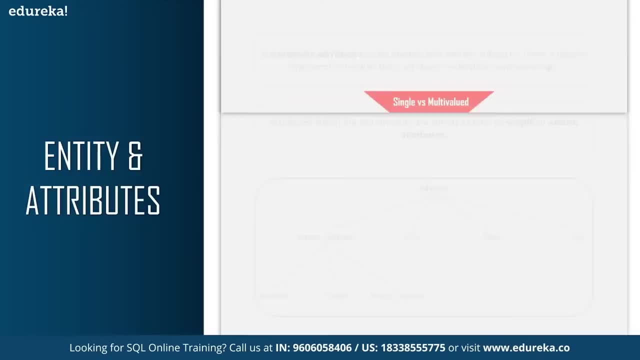 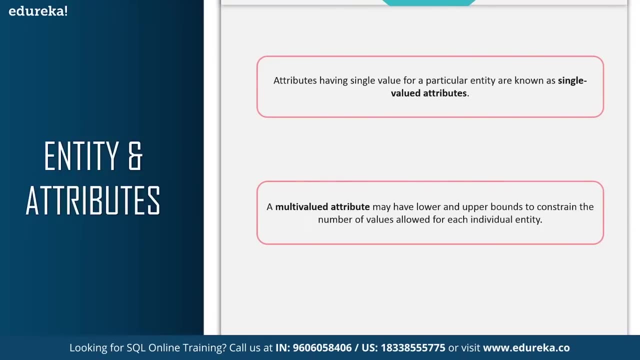 So this was about composite and simple guys. Now let's move forward with the next type of attributes at a single and multivalued now attributes having a single value for a particular entity unknown. a single value attributes and a multivalued attribute may have lower and upper bounds. 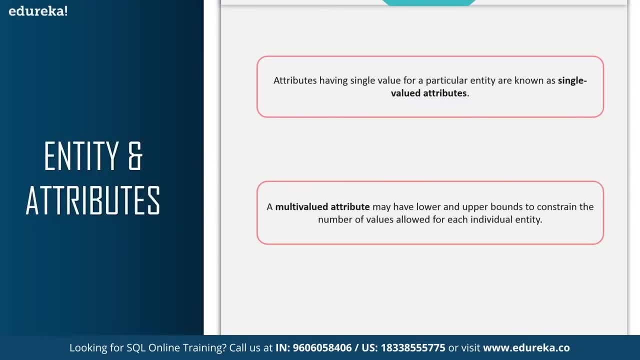 to constrain the number of values allowed for each individual entity, So you can have a single attribute and a multi attribute in an entity. and I forgot to tell you one thing over here: Every entity is uniquely identified, right? So, as I told you, employee had SSN. 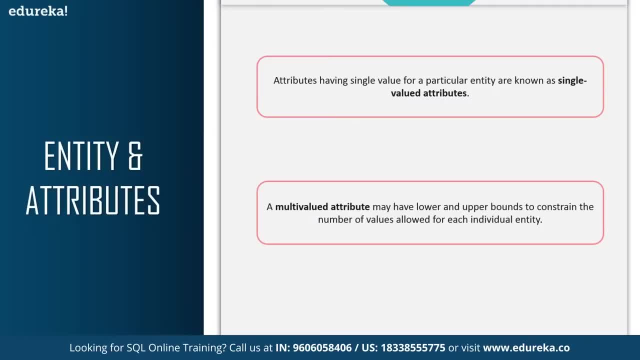 that is the social security number. Now, that is basically uniquely identified, right? So there is the SSN. So over here, that will be basically a unique attribute to which the complete table will be identified. next, Let's move forward with the next type of attribute. 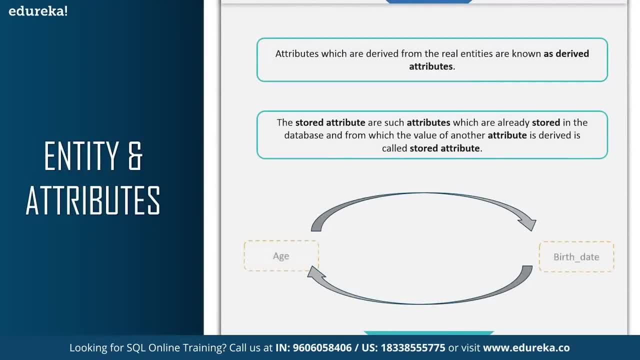 that is stored versus derived. So the attributes which are derived from the real entities are known as derived attributes and the stored attributes are the attributes which are already stored in the database and from which the value of another attribute is derived. So, basically, if you consider age from age, 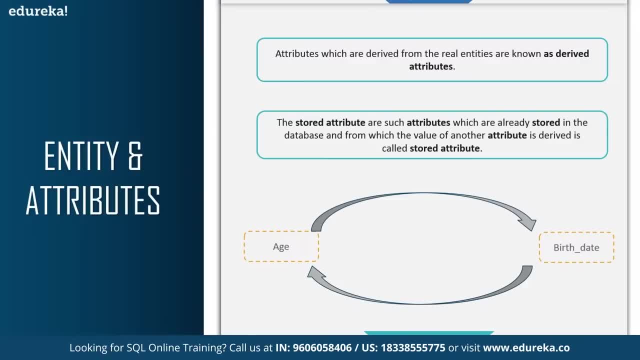 you can derive birth date right And from birthday you can derive age right. So I'm not saying, in the matter of exact birthday, you can like. let's say you're 23 years, So you can derive the fact you know. 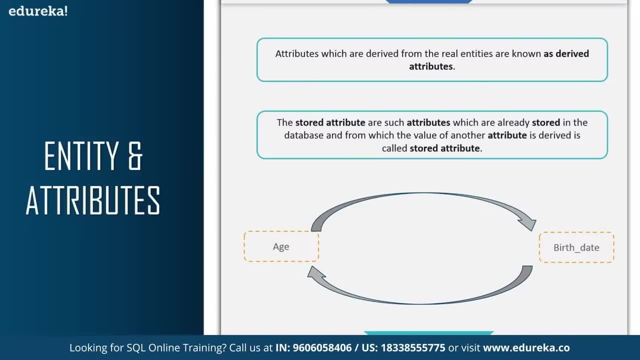 at the birthday could be either in 95- 96, and if you know the year born is 95- 96, then automatically you can derive an age that you know the age could be 23 years, right? So that's how basically you can understand stored. 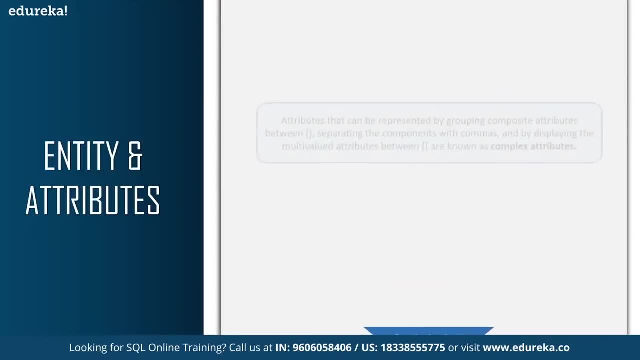 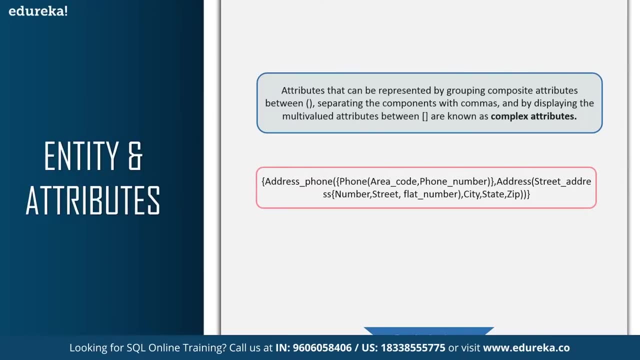 and derived attribute. and finally, coming to complex attributes, the attributes that can be represented by grouping composite attributes- between you know, brackets, by separating the components with commas and by displaying multivalued attributes with square brackets, are known as complex attributes. right, So basically, an address can have phone number. 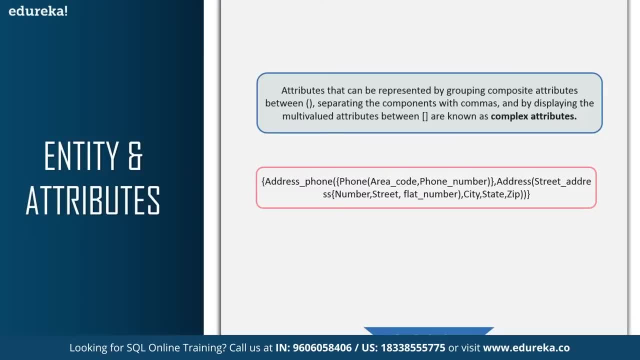 and then the phone can have again like area code and phone numbers and then moving forward, where you can have again address, and maybe address can again have street address, number, street, flat number, state, zip code and so on. So basically this is how you can Define complex attributes, guys. 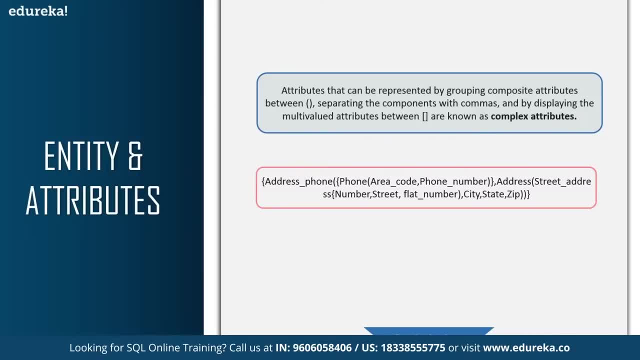 So, guys, that was about entity relationship diagram, So I hope you have understood how entities work, how attributes work, how a table name can be found and how columns are formed and how each table can be related to the other table, because this concept is really important to understand. 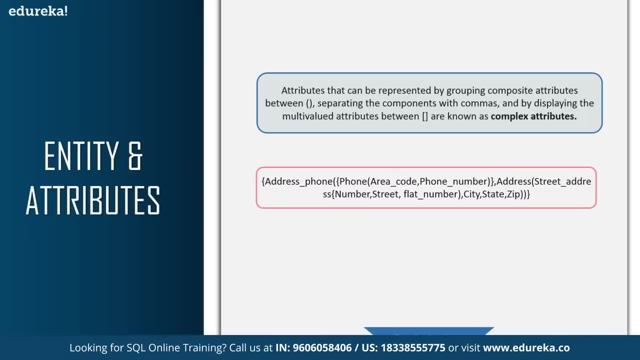 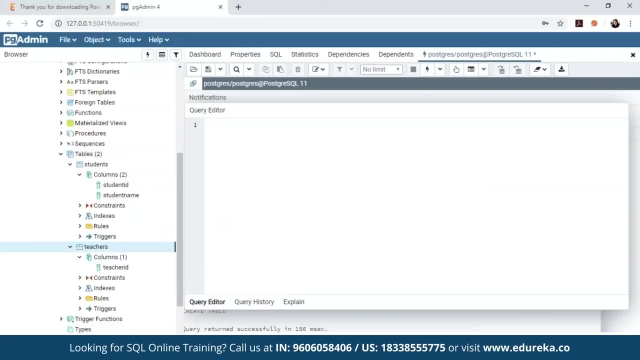 so that you understand the further concepts, like you know, the keys in databases and the constraints used. now, before I wrap up this entity relationship diagram, let me just shift back to my PG admin and show you the simple commands, like DDL, like you know, the create, truncate, alter and so on. 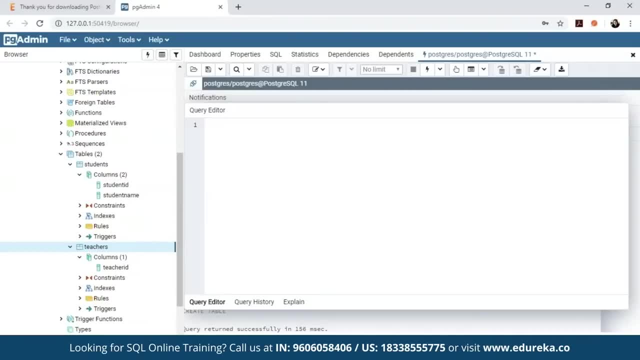 So, for example, let's say you know you want to truncate the table, right. So when I say truncate, what I mean by that is you basically delete all the data present in the table, but you do not delete the table itself. 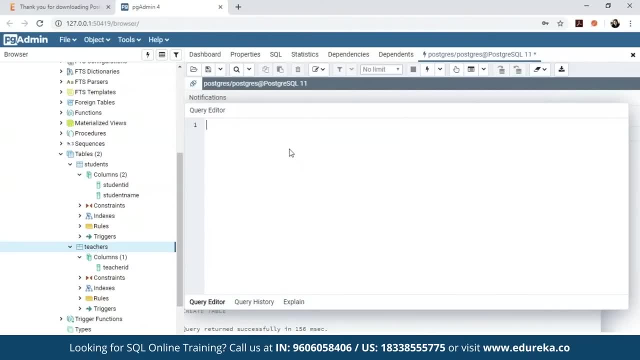 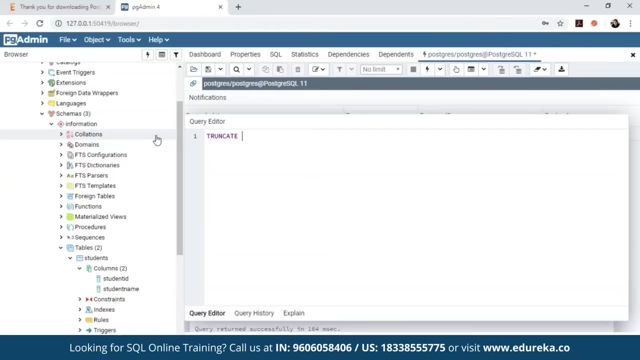 Now, since we haven't added any data into the table, I'll just show you the syntax so that you can understand. So let's say, you know you want to truncate table students, right? So for that, what you'll do is you'll type in truncate table. 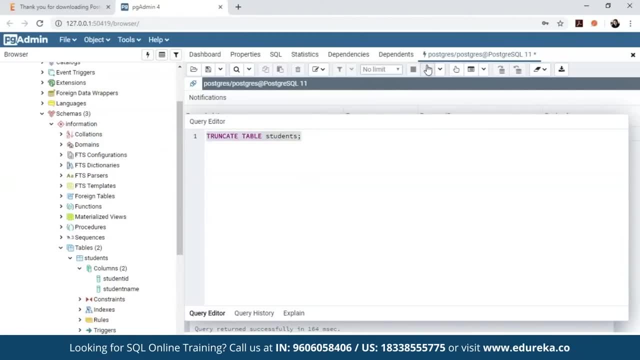 and then you'll mention students, right, and then you'll execute Right. once you execute, you'll see the output that you know: truncate table. The query has been returned successfully. now, since we have no data is present, You cannot see any particular output, but if you had any data present in the table, 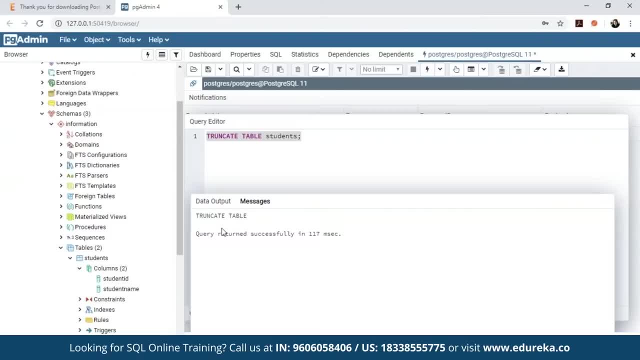 you would see that you know all the data would be removed from the table. Let's say you know you want to rename the table. Let's say you want to rename the table students to, let's say, info students, right, So to rename the students, you basically have to use: 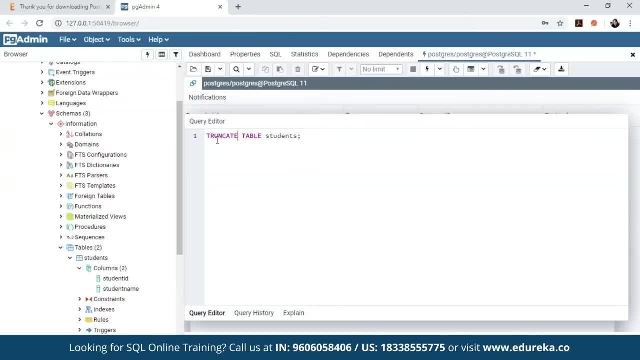 to DDL statements, that is, alter table and rename right. So for that, what you'll do is you'll type in alter table and then you'll mention the original name that students and then you wish to rename right. you type in rename to and then you'll mention the new name. that is, info students. 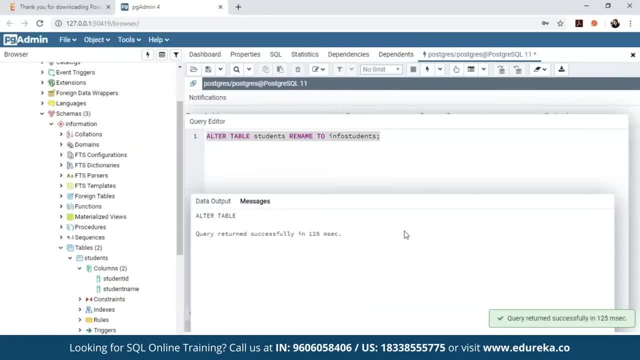 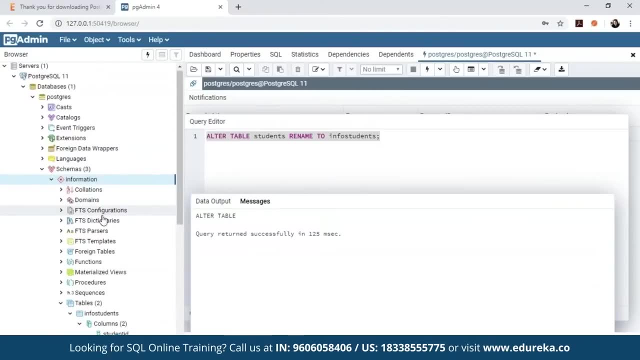 Right, and then you'll execute. Once you execute, you'll see that you know all the table. the query has been returned successfully. So what I'll do is I'll just refresh this particular schema and then you'll automatically see that you know. we see an output of info. students, right? 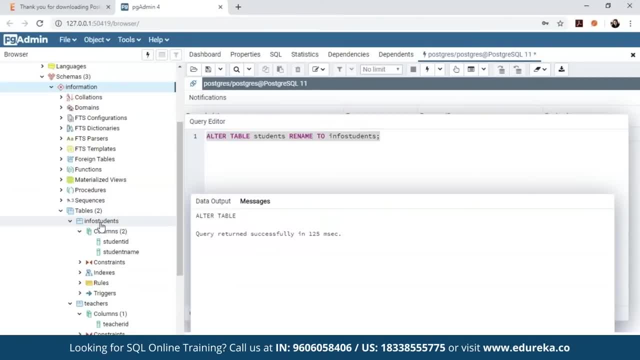 So that means our table has been renamed. now, for example, let's say, you know we want to add a new column, So for that again you'll use the alter statement. So I'll just type in alter table and then I'll mention the table name. that is, info students. 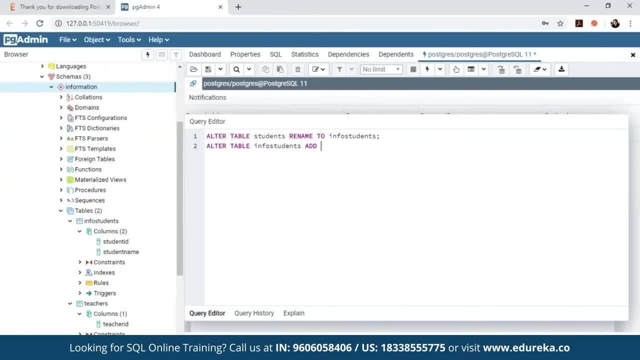 and then what you'll do is you'll mention add and then you'll mention the column name. that is, let's say you know, date of birth, and then the data type of it. Let's say date right, and then you'll end with semicolon. 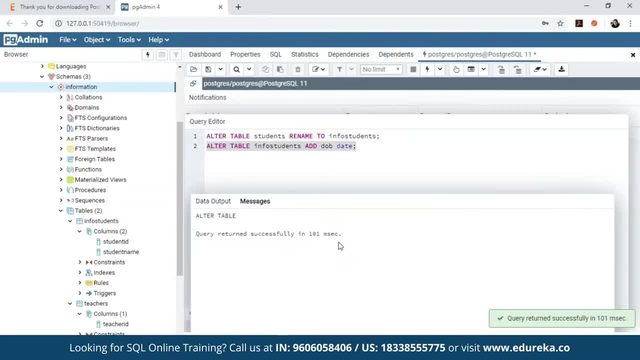 and then you'll execute. once you execute you'll see that you know the query has been returned successfully. So if I just refresh this part again and you'll see automatically that you know a new column has been added onto the table, that is date of birth. 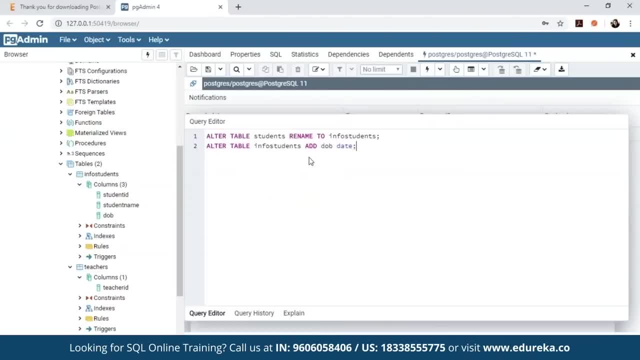 So this was just for a single column, guys. Now you can add multiple columns also. So, for example, let's say I want to add two more columns, right, So what I'll do is I'll just remove this. Let's say, you know, 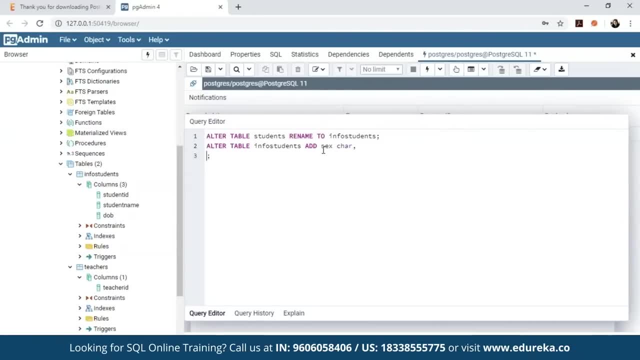 I want to add gender, So I'll just mention sex character and again comma and add, let's say, class. Okay, class is a keyword, So I'll mention standing under and then integer right, and then I'll again execute. once I execute, I'll again refresh. 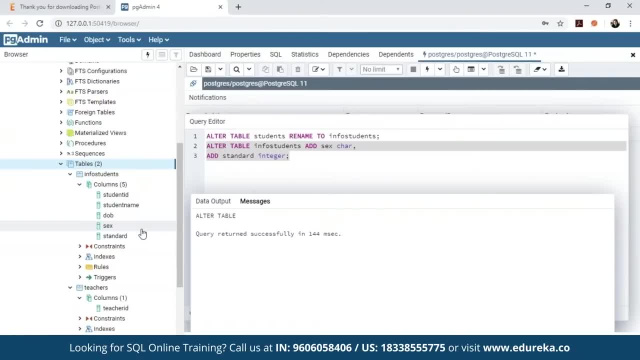 and when I refresh you'll see that you know automatically my sex and standards. So basically, the gender, date of birth and standard have been added as new columns, right? So that's how, basically, you can add a single column or you can add multiple columns now. 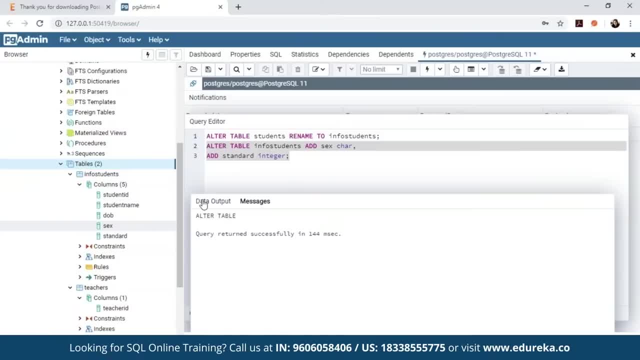 you can also alter the data type of the particular column. For example, I want the data type of the standard column to be changed to, let's say, character. So for that, what you will do is you'll basically mention all the table info, students. that is basically the table name. 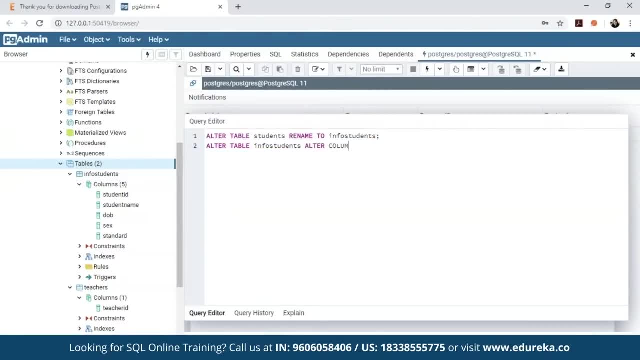 and then what you'll do is you'll mention alter column and then you'll mention the column name. that is basically standard, and then you can mention the keyword type, and let's say we mentioned character, and then I'll execute. and now, once I execute, and then, if I show you the properties, 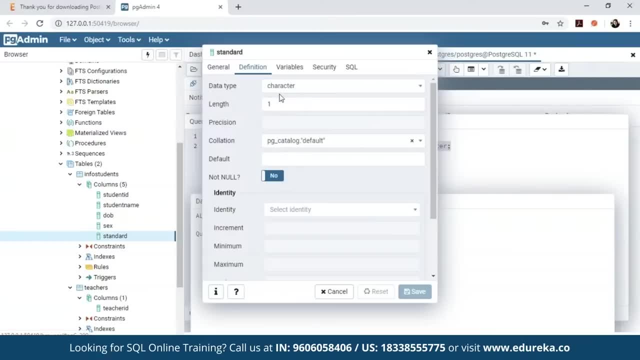 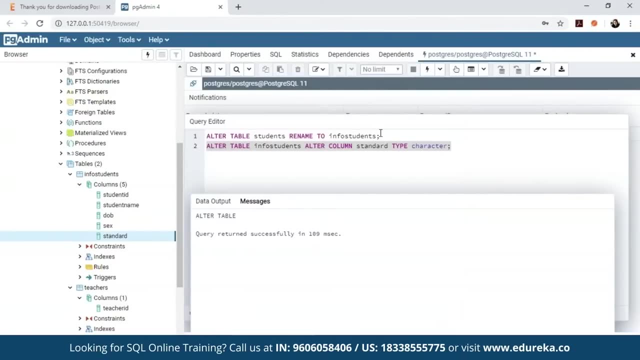 of this particular column, you'll automatically see that you know the data type is character, right. So basically, guys, that's how you can also alter a particular table or maybe column, Maybe if you want to rename and all. now let's say you know. 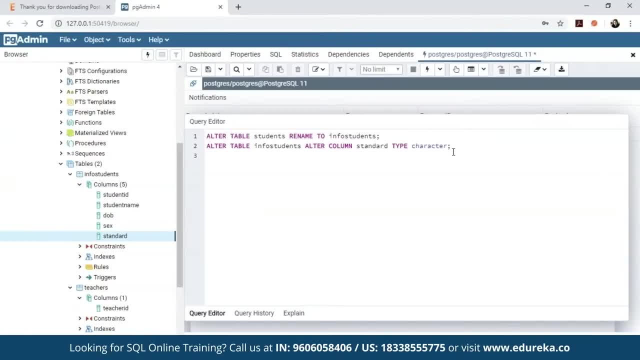 you want to drop this particular column. So for that what you do is you type in alter table, mention the table name again. And then what you do is you mention the keyword drop column and then you mention the column name, right, And then you just execute. now, once you execute, 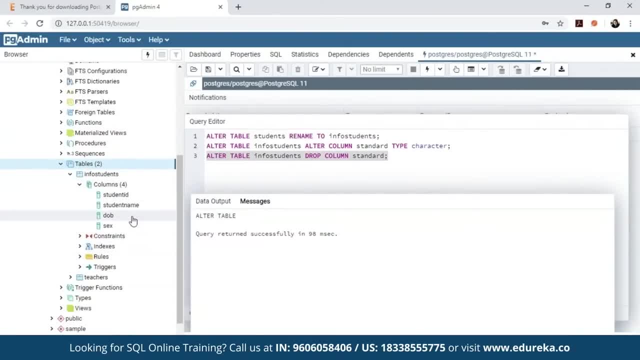 and let's say, if I refresh this, you'll clearly see an output that you know your standard column is gone, Right? So that's how, basically, you can drop a column now. Similarly, if you want to rename a column, it's really simple. 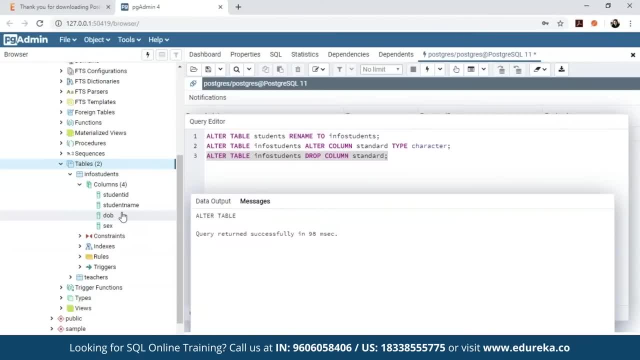 You have to write a query, like you know, alter table, the table name, and then you have to mention rename column and then you mentioned the column name to the new column name, right? For example, let's say I want to change the column name of sex. 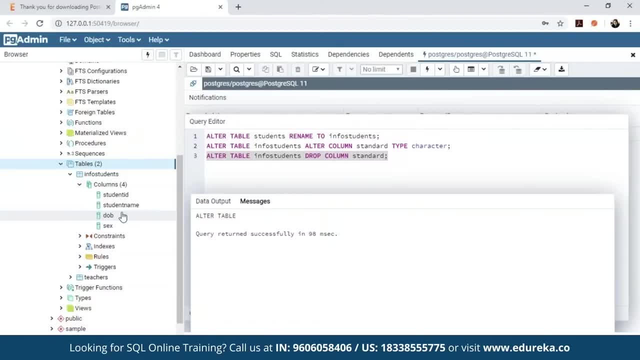 So what I'll mention is: alter table info. students rename column sex to gender. So that's how you can basically rename a column also now. simply, let's say: you know if you want to drop a table? now, if you want to drop a table. 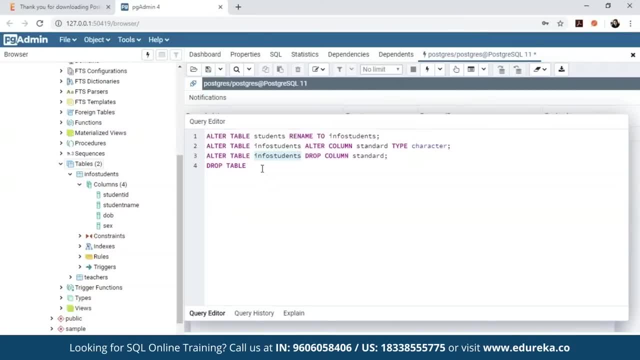 I'll mention drop table and then I'll mention the table name, right. So I'll just click on execute and then you'll see that you know, automatically your table will be dropped. So if I just refresh this, you'll see that you know. 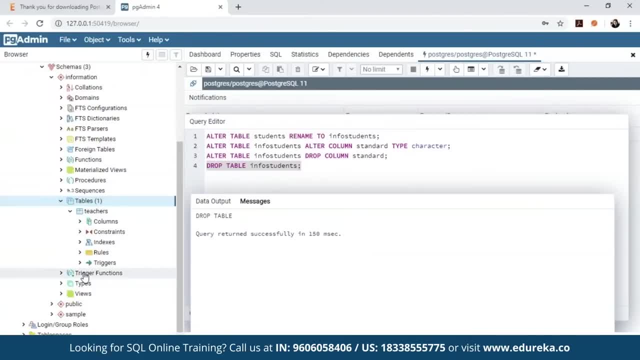 we just have one particular table, that is, teachers, and the students table is gone. So, guys, this is how basically you can work on PG admin for basically the DDL commands. right, What I'm going to do is, for this particular session, I'm going to consider the ER diagram. 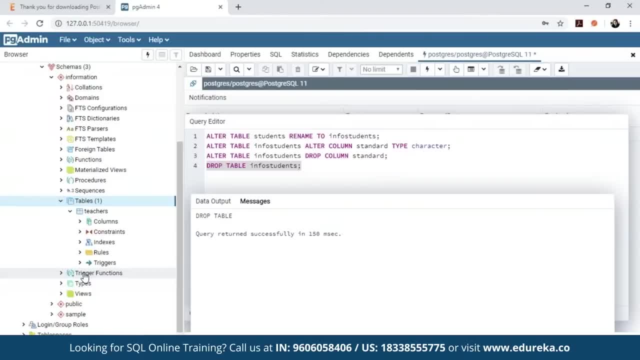 as I mentioned before, right, So I'm going to create tables and manipulate data with those particular tables only. So, before I move forward with this session, what I'll do is I'll explain you the different keys and constraints used in the database. 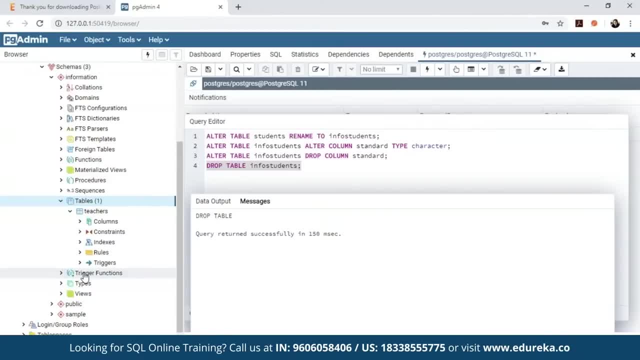 so that it's more clear to you how you can create the database in a more structured manner, and then we'll move forward with the various manipulation commands. until then, What I'll do is I'll just delete this particular table, So I'll right-click here, go to delete and click on. 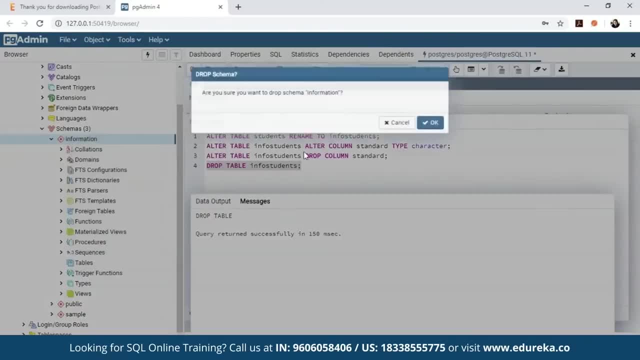 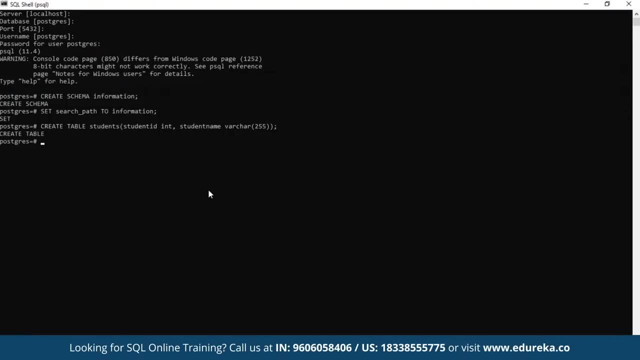 Okay, and then let's say: you know, we will delete this particular schema also, so that there's no confusion at all, And then what I'll do is I'll close this shell. So so, guys, remember that you know I am using PG. admin. 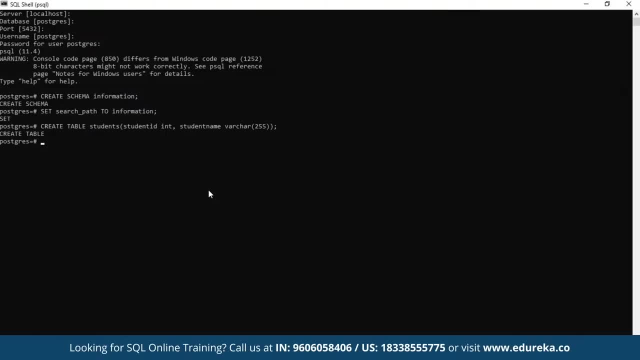 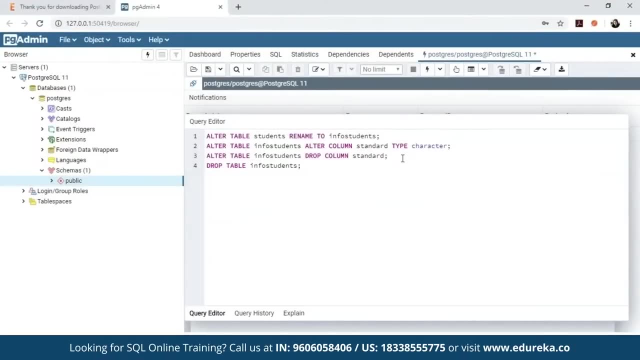 Well, you can use the same queries that I mentioned there on SQL shell also, and you'll see the same output. So I hope that's clear. So I'm going to close the sequel shell and then I'll continue with this session. So now moving forward with this session. 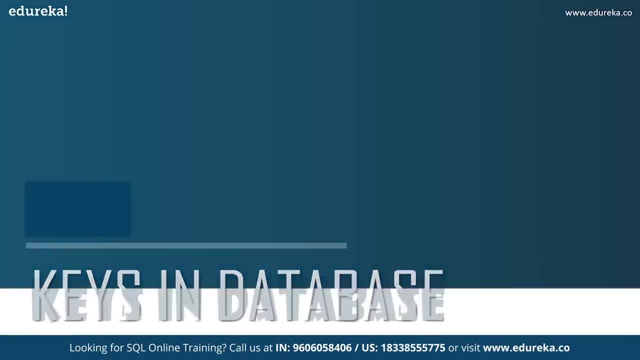 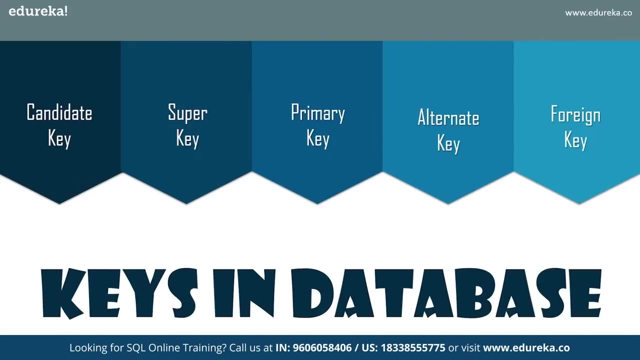 let's start with the next topic, that is, keys in database. So there are mainly five types of keys in database, that is, the candidate key, the super key, the primary key, the alternate key and the foreign key. So, talking about the candidate key, the candidate key is basically the minimal set of attributes. 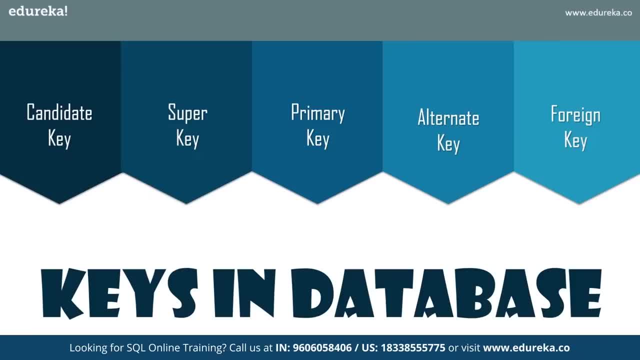 which can uniquely identify a tuple. So any minimal set of attributes which can uniquely identify a tuple is known as a candidate key. So the value of the candidate key will be unique and non-null for every tuple. So if you have to identify a specific tuple, 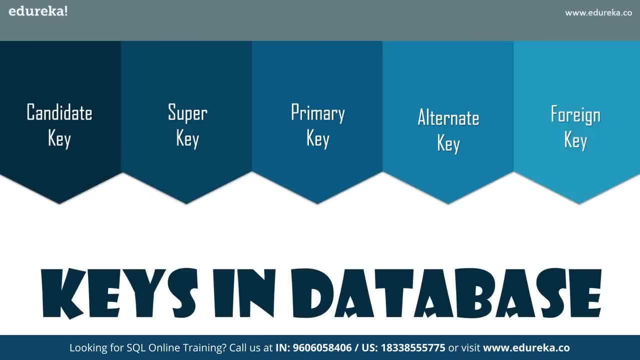 let's say sahiti, age 24,. let's say date of birth: 30 October, and so on, so on, so on. then you need a particular candidate key to uniquely identify my tuple right, So that particular can be my employee ID, and so on. 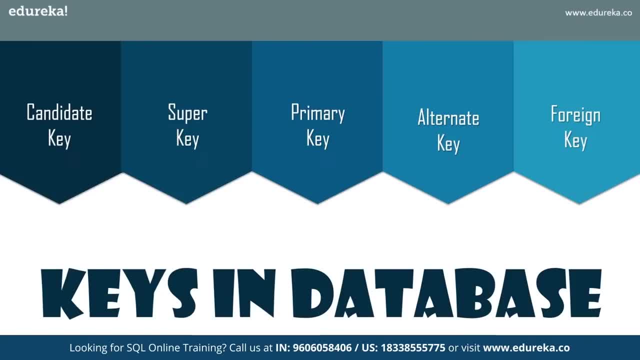 Now let me tell you one thing over here. They can be more than one candidate key in a relation also. So a candidate key can also be either simple key or a composite key. now coming to super key. Now, super key is basically again the set of attributes. 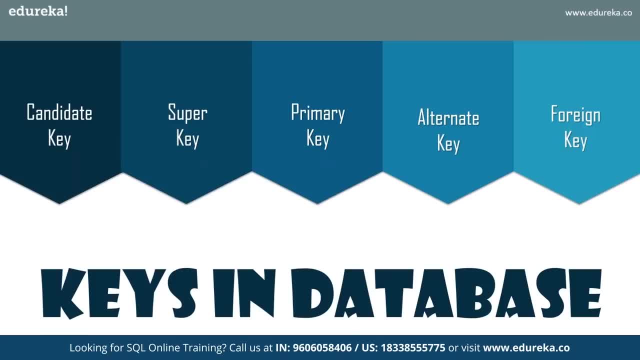 which can uniquely identify a tuple. So any set of attributes which can uniquely identify tuple is known as a super key, but it's not the minimal set of attributes. The minimal set of attributes is the candidate key, but as any set of attributes which can uniquely identify is known as a super key, 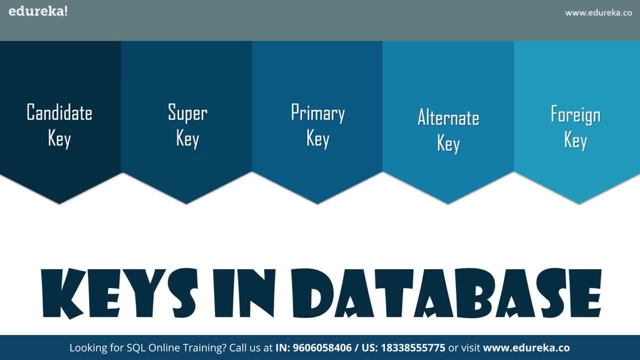 So when you add zero or more attributes to a candidate key, it becomes a super key, but the vice versa is not true. So a candidate key is definitely a super key, guys, but the super key is not a candidate key. So that's what you have to understand now moving. 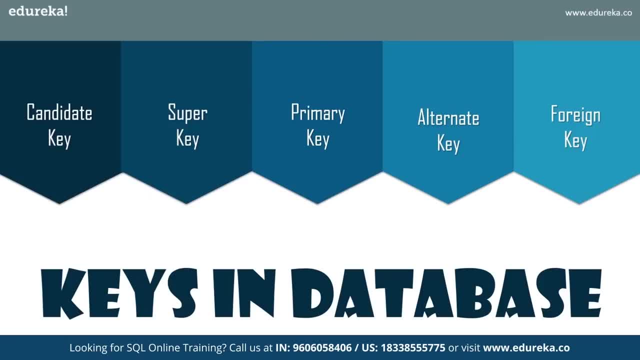 on to primary key. The primary key is also a set of attributes which can be used to uniquely identify every tuple. Now, if you remember the entity relationship diagram that I was explaining you, I said the employee table has a special social security number to which every tuple will be identified, right? 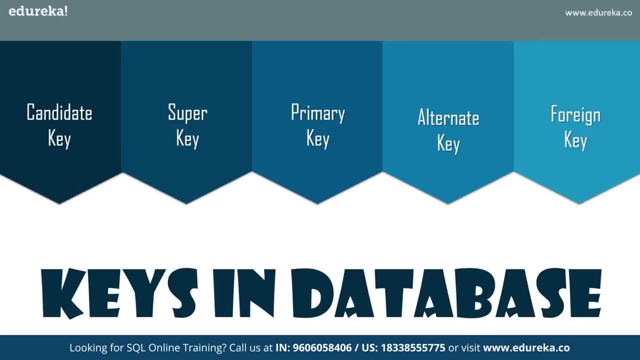 So that particular social security number will be the primary key to which every tuple will be identified. and now, apart from that, they can be more than one candidate key in a relation, right? So out of all the candidate keys present in the relation, you can choose any one key as the primary key. 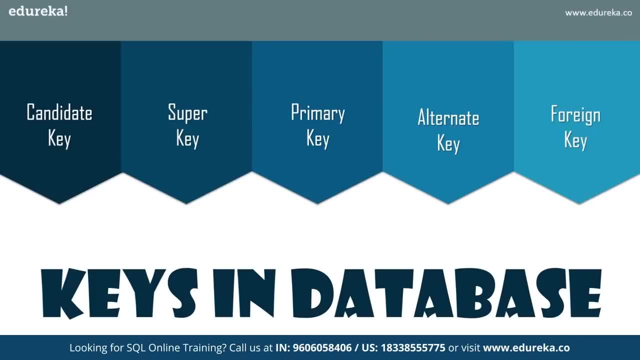 So if you have around five candidate keys, out of them, one can be definitely your primary key for that particular relation. moving on to the next type of key, that is, the alternate key, So the candidate keys other than primary keys are basically the alternate keys. 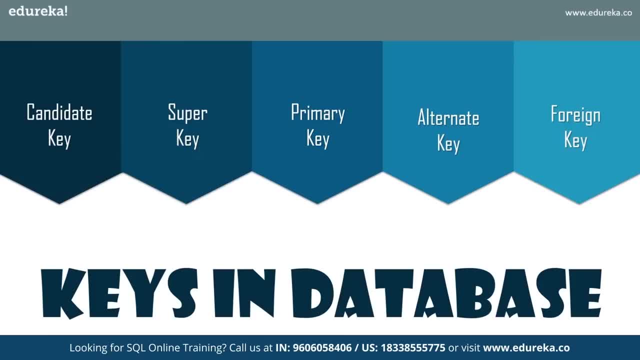 So, as I was giving you an example of five candidate keys, So if there are five candidate keys in a relation, then out of which, if let's say you know, the first key is chosen as the primary key, then the other four keys will be the alternate keys. 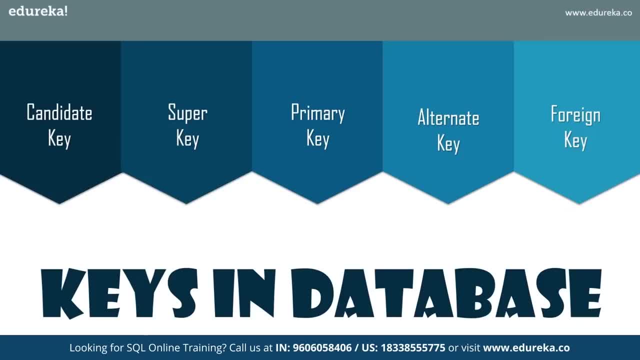 and finally, moving on to the foreign key, So the foreign key is basically the key if an attribute can only take the values which are present as values of some other attribute. So, basically, whenever an attribute can only take the values which are present as values of some other attribute. 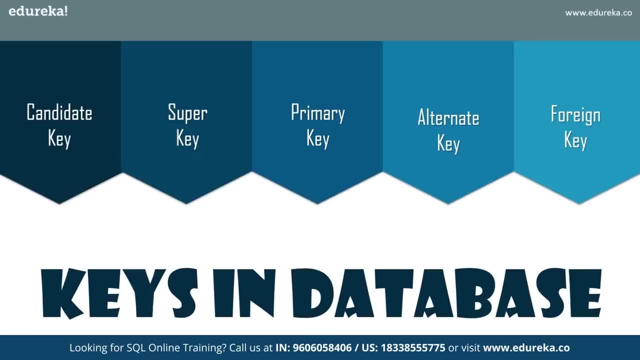 then it will be basically be the foreign key to the attribute to which it refers. So basically, the relation which is referenced is called reference relation and the relation which refers to the reference relation is called the referencing relation. So the reference attribute of the referencing attribute. 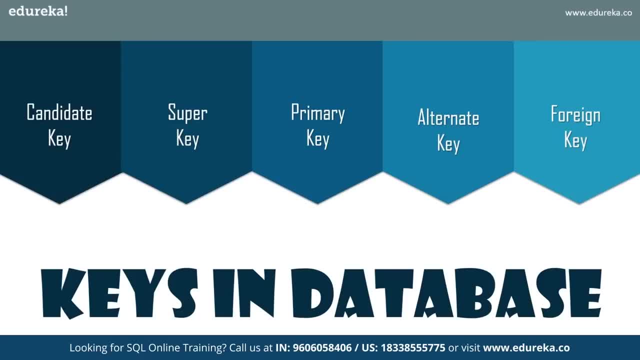 should be a primary key right. For example, let's say you know you have employee and Department. right now You want to reference Department to employee. So what will happen is you'll basically use a foreign key to validate this relationship and then you'll add a foreign key from Department to employee. 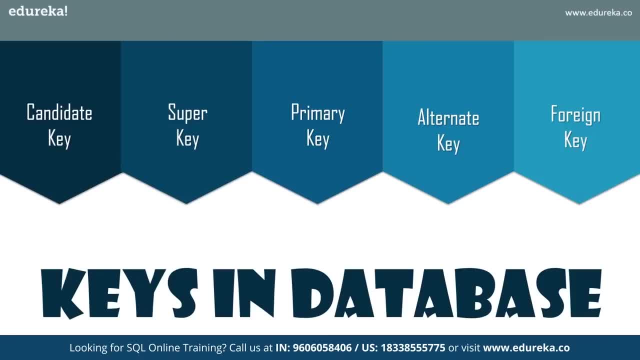 I hope that's clear. So, guys, these were the various keys that you need to understand about, that is, the candidate keys, super key, primary key, alternate key and the foreign key. So now that you know the different keys in database and you know the DDL commands also. 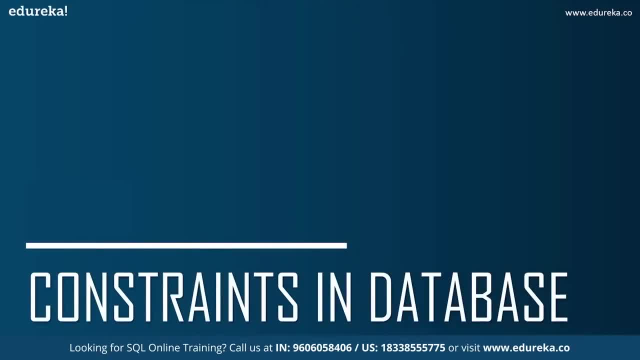 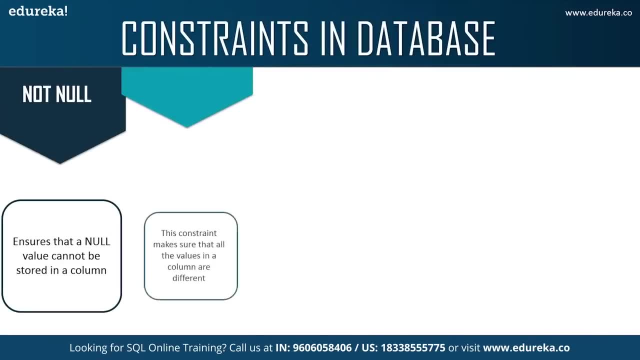 let me take you to the constraints in database so that we can quickly create the tables that we discussed in entity relationship diagram. right? So the constraints in the database are, as you can see on my screen, that is, not null, unique, check, default and index. 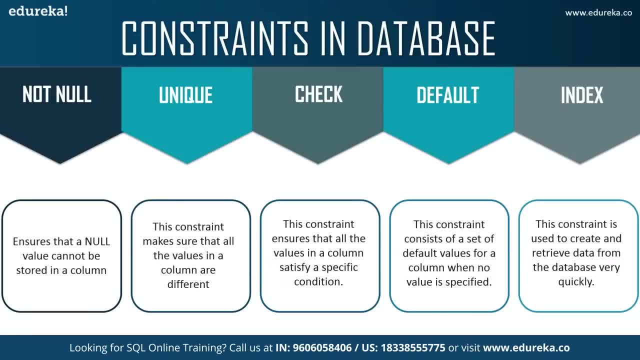 So the not null constraint basically ensures that you know a null value cannot be stored in a column. For example, let's say you know you have a student's table. now in the students table You have a column on a student ID. 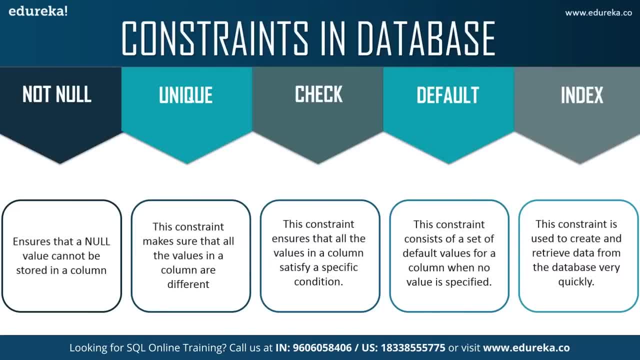 and then when you're creating the table- you mentioned the not will Constraint for this particular column- Then whenever you're inserting the data, you have to remember that you know they cannot be a null value in this particular column. That is the student ID coming to unique, unique Constraint. 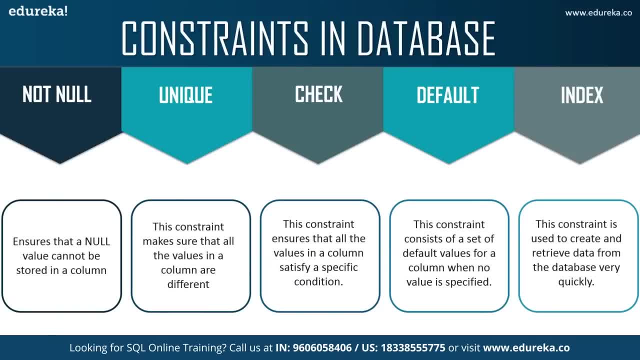 Make sure that you know all the values in the column are different. So in whichever columns that you want to store unique values, you have to use this Constraint. you need coming to check. this Constraint ensures that all the values in a column satisfy a specific condition. 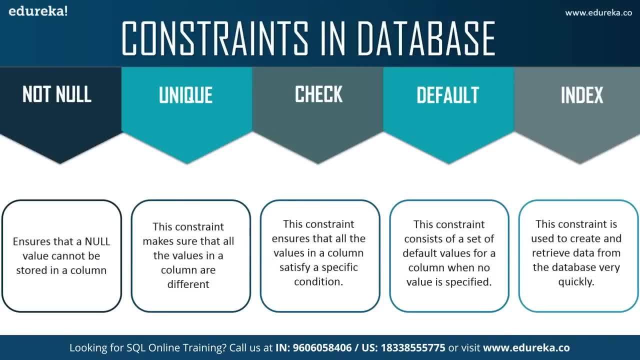 So you have to check. let's say you know we want to store the age of employees. Now let's say age has to be greater than 25.. So only the age values whose value will be greater than 25 will be stored in the each column. 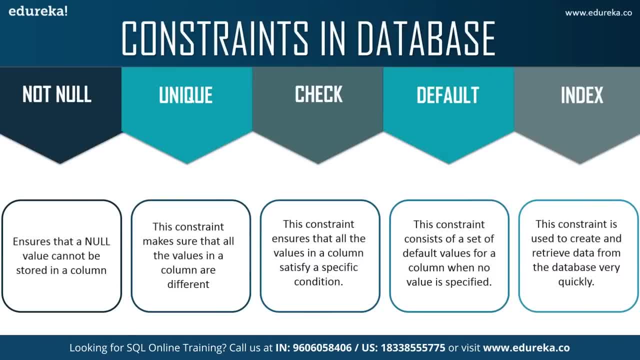 If you mentioned this particular Constraint. now, moving on to the next Constraint, that is, a default Constraint. This particular Constraint consists of a set of default values for a column when no values specified, So whenever let's say, you know you have not inserted any value specifically, 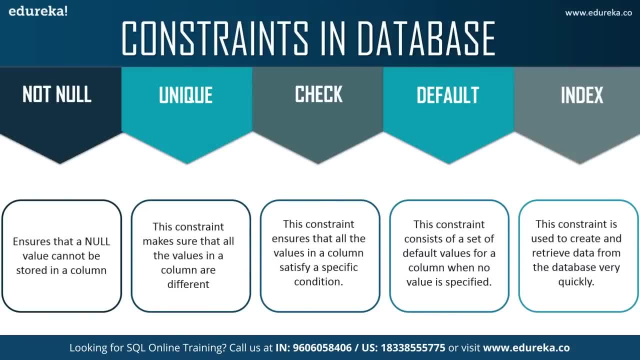 then automatically a default value will be stored in that particular cell If you use this particular Constraint. and finally, coming to the index of the Constraint, this Constraint is used to create and retrieve data for database very quickly. So if you want to create and retrieve data, 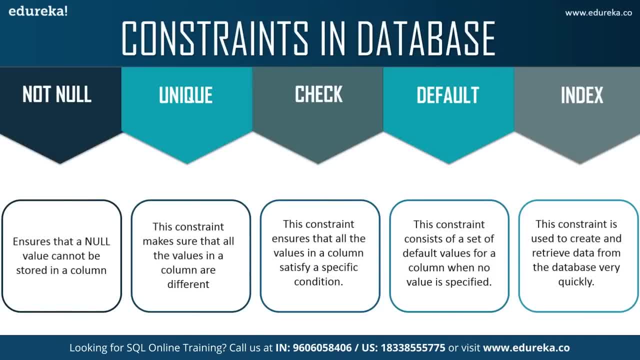 from database very quickly, then you have to use this particular Constraint that is index. So, guys, I hope the keys and Constraints concept is clear to you guys. So, now that you know we have understood the entity relationship diagram, the Constraint and the keys, 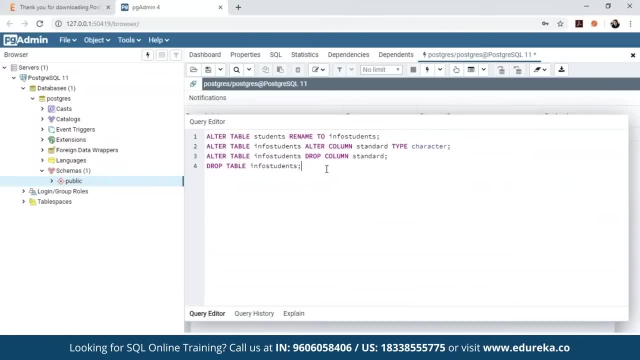 Let me shift back to my PG admin. And now let's say: you know, I'll start creating table, So I'll just show you for one table, and then I've already a set of commands that I've already executed, you know. 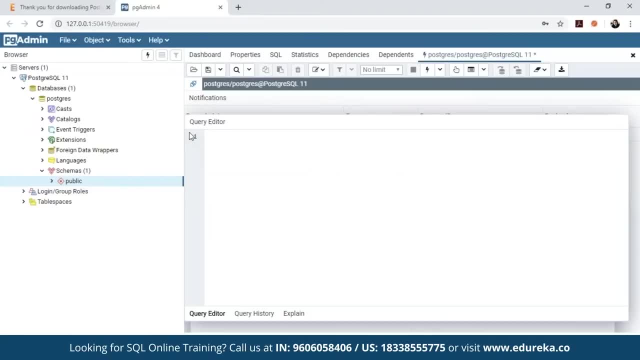 I'm just going to copy paste the command over here. So what I'm going to do is we had the employee table right. So for that, what I'm going to do is I'm going to mention create schema first, so that you create a schema. 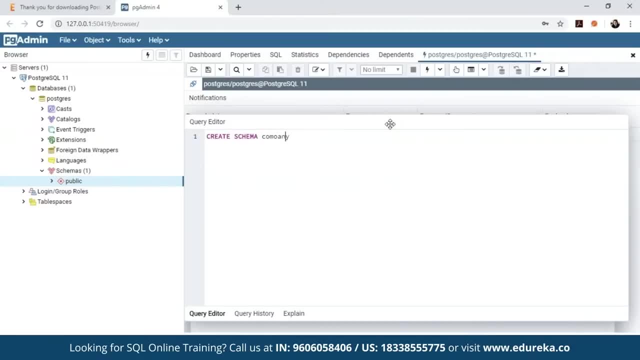 So I'm just going to mention create schema. Let's say we mentioned schema name to be company. After that, what I'm going to do is I'm going to use this particular schema, right? So I'll just mention: set search path to company. 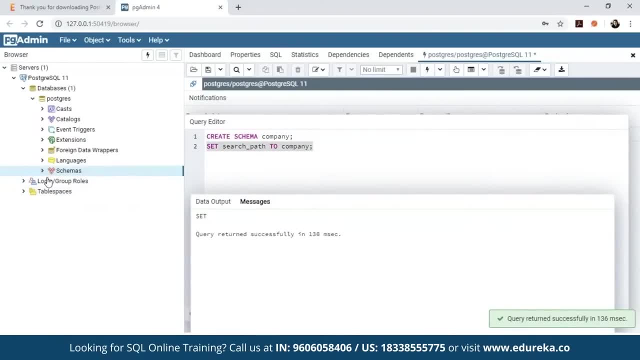 Now automatically, if I just refresh over here, you'll see that you know there are two schemas, that is, company and public. now what I'm going to do is I'm going to create tables inside this particular schema. So for that, what I'll do is- and mention, create table. 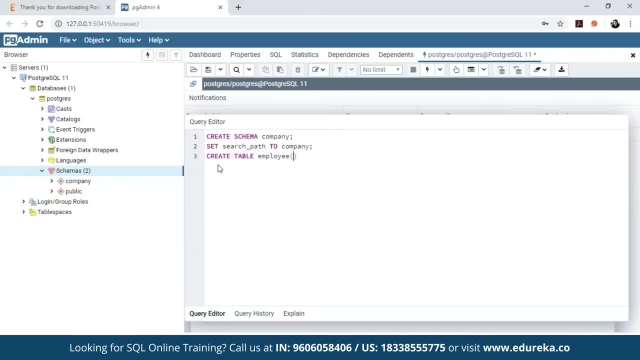 Let's say we mentioned employee and in brackets What I'll do is I'll mention all the column names. So we had first name that say we mentioned text not null. So I'm using a constraint known as not null Right. So this particular constraint is used. 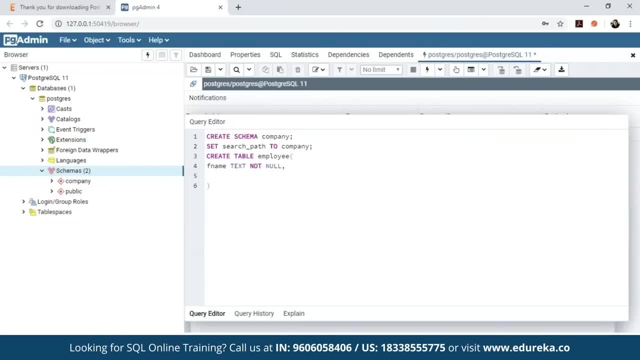 That means that you know they cannot be a null value in this particular column. Similarly, let's do for middle name Let's say care, null right. So there can be null values over here. now, last name, Let's say text, not null right now. 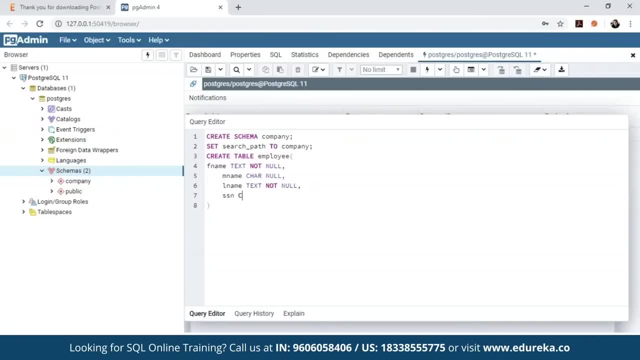 I have basically a social security number, right, So I'll put SSN. Let's say character of, say, nine characters, Let's be specific over here- and I'll put not null. So this cannot be null and I also want it to be the primary key. 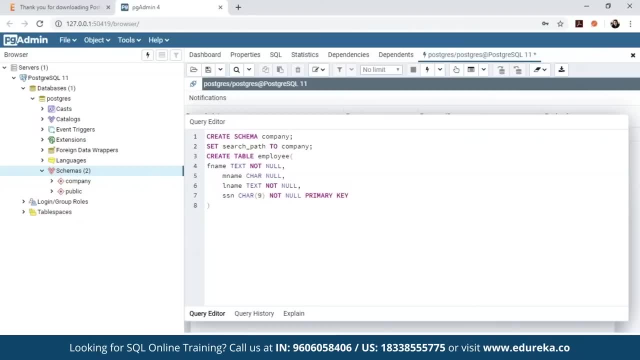 So basically, through this particular number, the complete table will be uniquely identified. after that I'll mention bird date and then I'll mention the data type to be date. right. Let's mention address and let's say I mentioned data type to be text, not none. 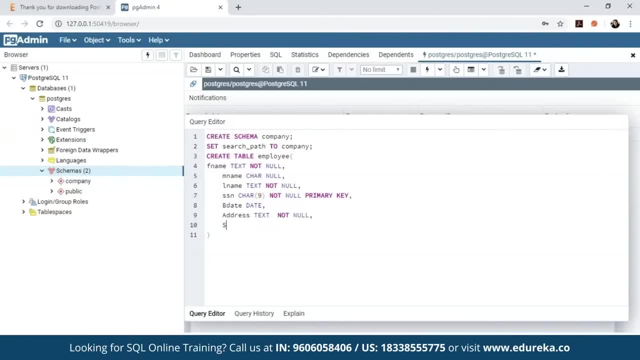 This also cannot be none right. Similarly, I'll mention sex. Let's say character Now. similarly, I'll mention salary, Let's say decimal, and then 10 to 2, and this can be null. So we don't know. it can happen that you know. 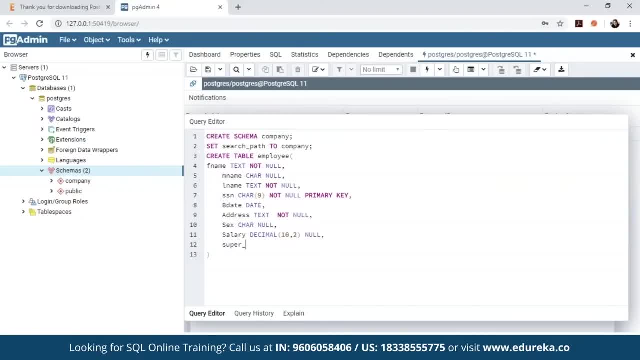 we don't know the salaries right, then I'll mention super SSN. So this is basically to identify the self-referencing relationship, if you remember right. and then I'll mention character of nine characters, and this can be null. and then let's say we mentioned department number. 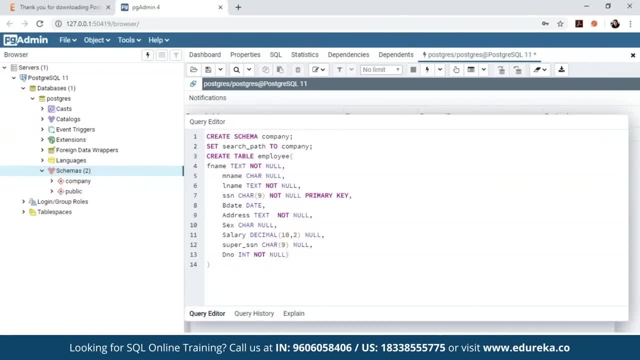 let it be in and let's say not null, because we don't want it to be not right now. What I'll do is I'll just execute this particular query Now. once I execute this particular query, you'll see that, you know, automatically we get an output. 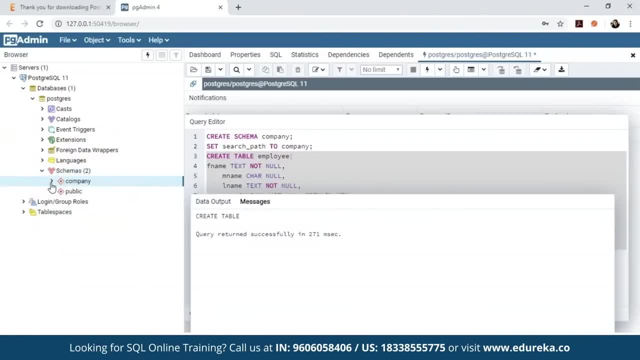 that create table, So our table is successfully created. So if I refresh this particular schema and then if I open tables, you'll clearly see that you know we have the employee tables now. Similarly, what I'm going to do is for all these particular entities. 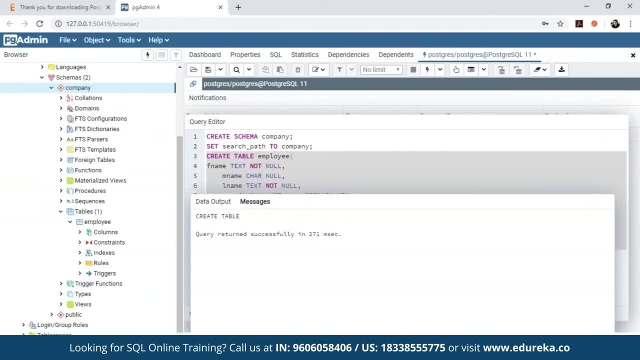 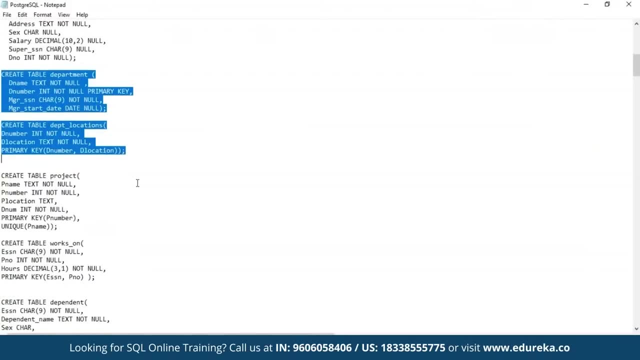 I'm going to create table right, So I already have a dog present, So I'm just going to copy paste from that. So let me just open that doc right. So let me just copy paste from here. So I'm going to copy for Department: Department locations. 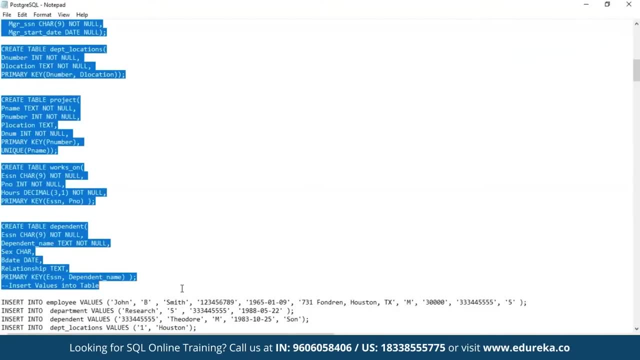 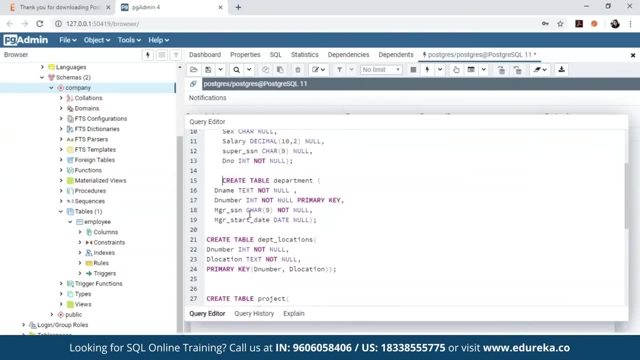 projects works on and dependent. now I'll go back to my PG admin And then what I'll do is I'll just paste over here. So what I'm doing is let me just explain you. so I'm creating a table Department with the column names as Department name, Department number. 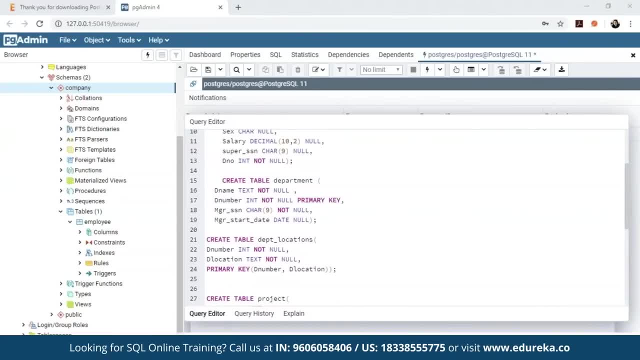 MGR assistant. that's because for the relationship of manager, right. So if you remember, if I just open a diagram, you'll clearly see that you know employee managers Department, right. So you see, for this particular relation and then MGR start date, that is because you know. 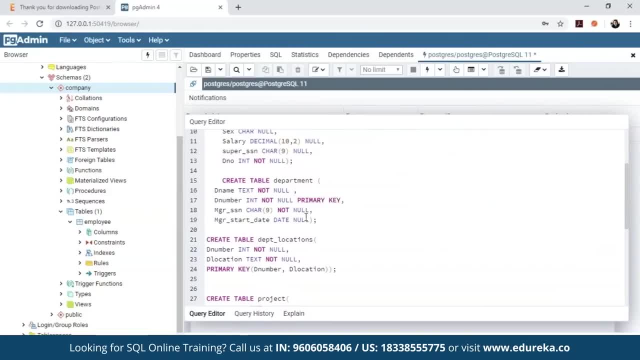 we have to consider the column present on the relationship Also, that is, managers. Similarly, I'm creating Department locations, that is, with Department number, Department location and primary key as Department number and location together. Then I'm creating a table- owners project. So the project table will have project name, project number. 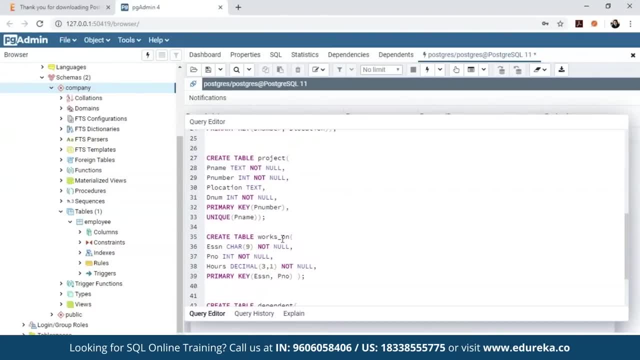 location, and then I've used the primary key to be project number, and then the project name has to be unique, right, So I've used a constraint over there. Similarly, I'm creating a table known as works on. So for the works on table, 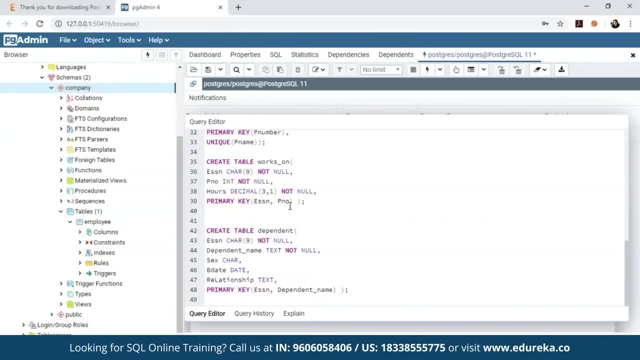 I have employee assistant, the project number, the hours work and the primary key to be the employee number and the project number. together the dependent table will again have the employee number, the dependent name, sex, birthday, relationship and the primary key to be employee assistant and dependent name right. 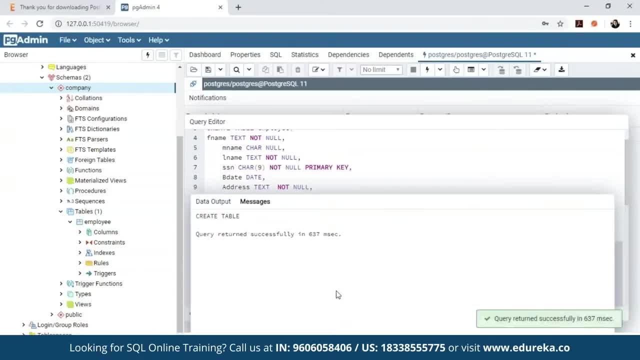 So I'll just execute all these particular queries So you can see that you know, automatically my query is got successfully executed. So I'll just refresh this particular table again. So once I refresh this particular schema, you'll see that you know. 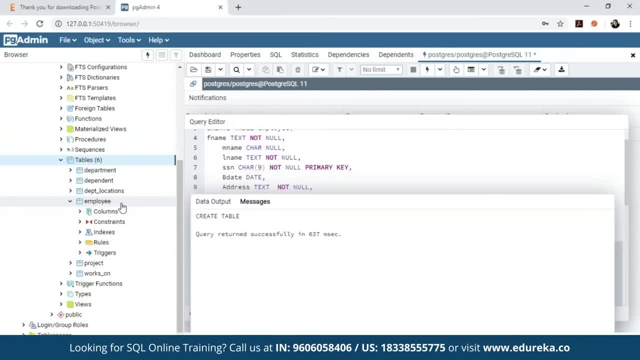 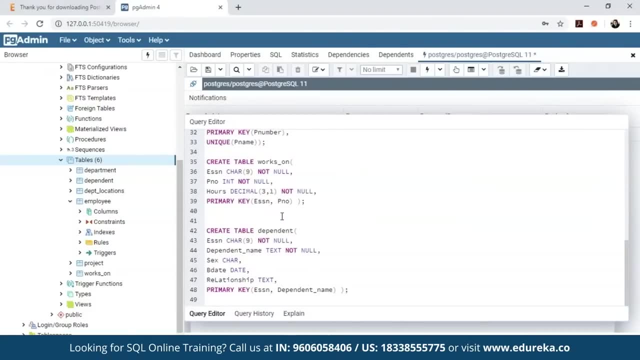 I have six tables. that is the department dependent, dependent locations- employee project works on right. So, guys, that's how, basically, you can create tables and that's how you can use keys and constraints while creating tables. So, guys, that was all about the data definition language commands. 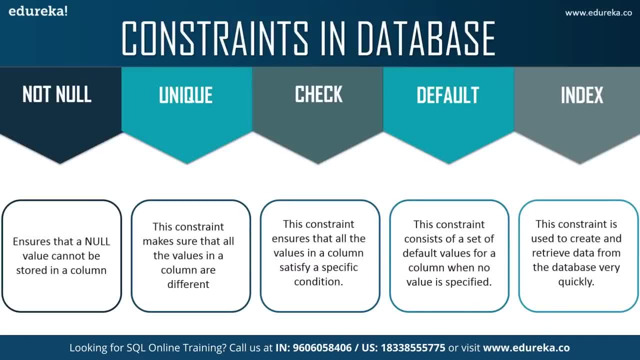 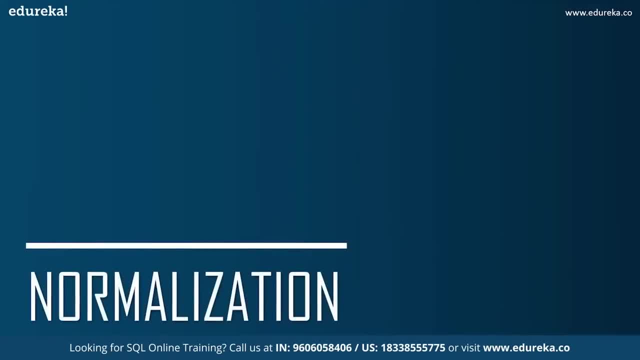 I hope you understood how you can use them and create databases. now, before I move on to the next topic, That is, the data manipulation commands, Let me take you through an interesting topic, that is normalization. So what is normalization? So, normalization is a technique that organizes tables. 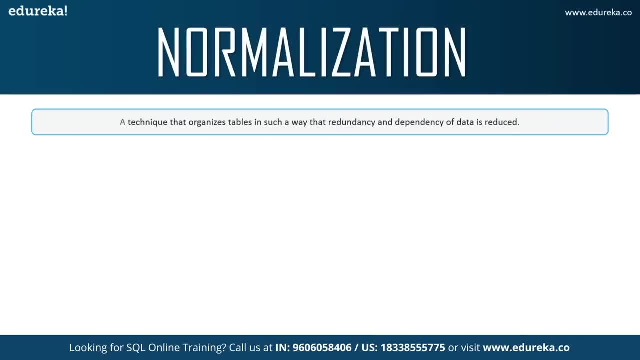 in such a way that you know the redundancy and the dependency of data is reduced. So obviously, when you're storing humongous amount of data on an industry level, there could be scenarios where you have written and sealed. So normalization is basically that technique. 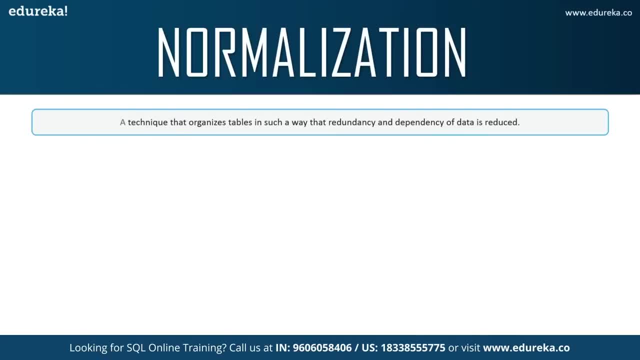 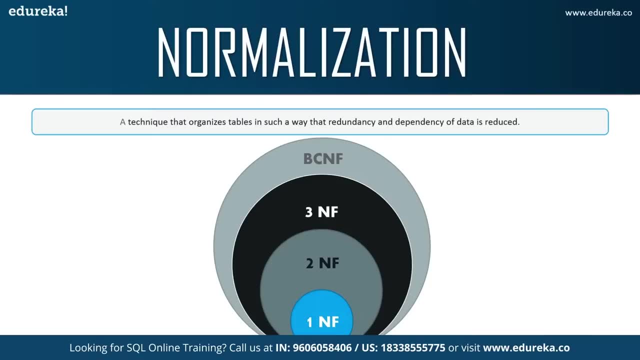 through which you know you can remove the redundancy and dependency of the data. So, as you can see on my screen, the normalization is basically at four levels, that is, one in F to nf3, nf and BCNF. So let's discuss the same now. now, before I move forward. 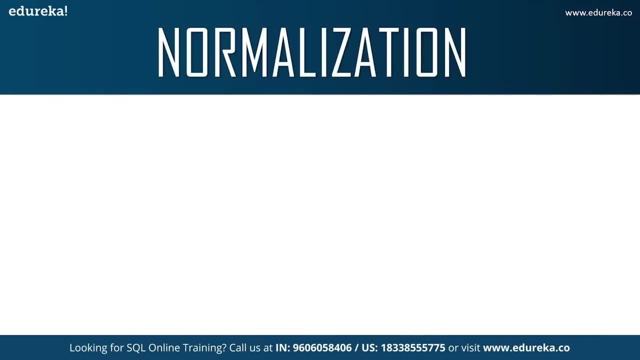 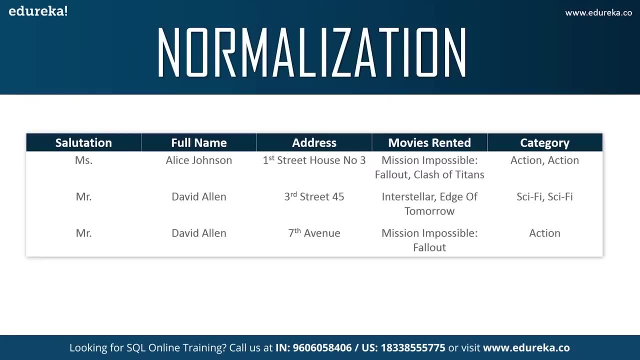 with one enough. Let me tell you that you know I'm going to consider this particular example. So the example that you can see on my screen is basically of three people you know of living in specific address and they have rented few movies of a specific category. now, 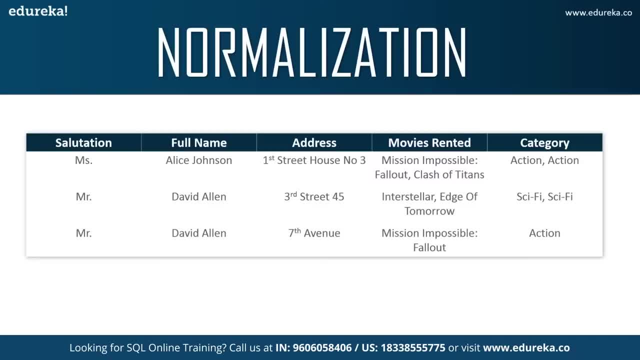 you definitely see redundancy in this particular table right. That's because you know. you see, Alice Johnson has rented two movies, that is, Mission Impossible and Clash of Titans. Similarly to David Allen's, address has been divided and also the movies rented out also been divided. 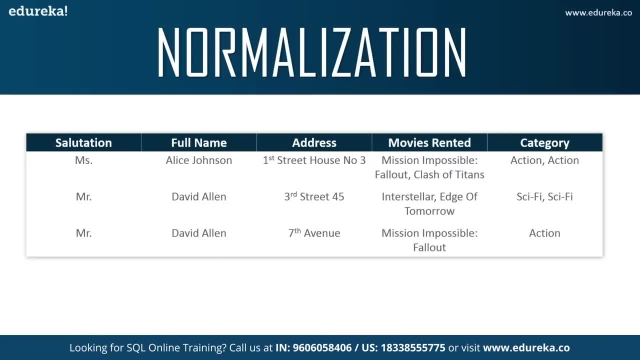 into different categories, like the sci-fi movies are put into one category and the action movies and put into the next category, and both of them are in two different tuples. This is definitely a redundant data. right Now, how do you think you can normalize the data? 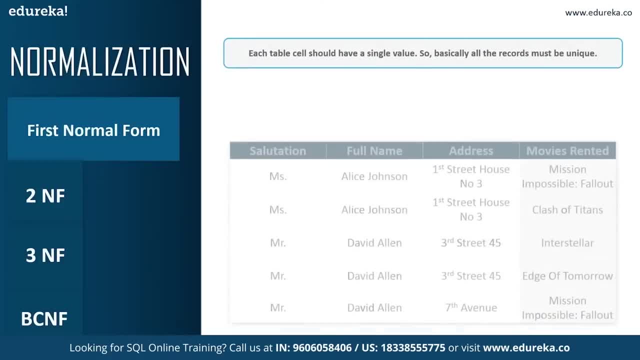 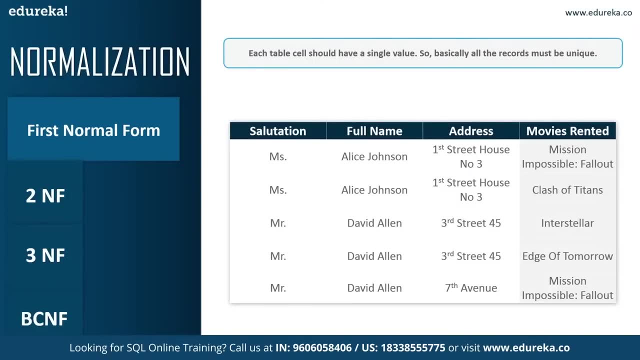 Well, we'll start with one and F now. the rule of one and F is really simple, guys. What the rule says is that you know, each table cell should have a single value, So basically any table that you have, and then you wish to normalize the data from that particular table. 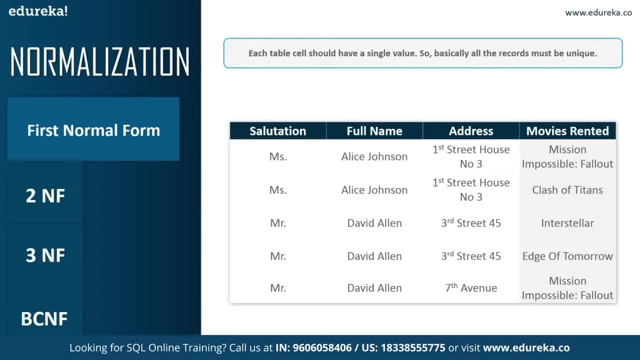 You have to make sure that you know each table cell has a single value. So, for example, we had Alice Johnson and David Allen, right? So, if you remember from the previous slide, we had movies rented together, right So for Alice Johnson. 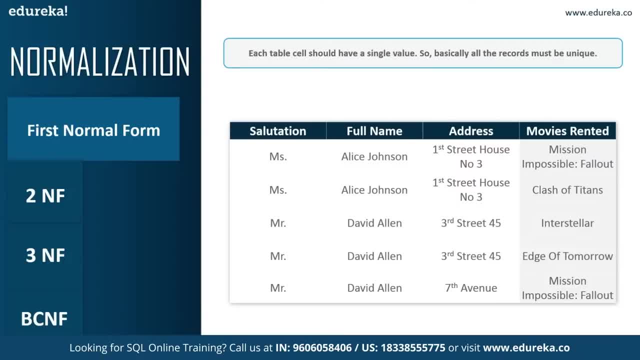 we had Mission Impossible and Clash of Titans in the same tuples and for David Allen we had the address divided but also the movies also divided. So what I've done over here is to get the data into one enough. What I've done is I've divided all the movies. 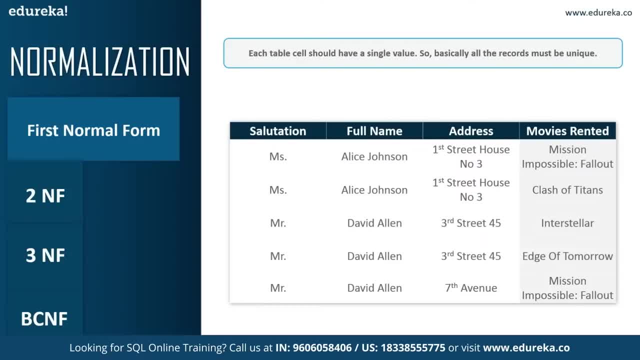 rented into different tuples. So Alice Johnson, staying in First Street, house number three, has basically, you know, specific movies rented, that is, Mission Impossible and Clash of Titans. So what I've done is I've divided both these movies into two different tuples. the same goes for David Allen. 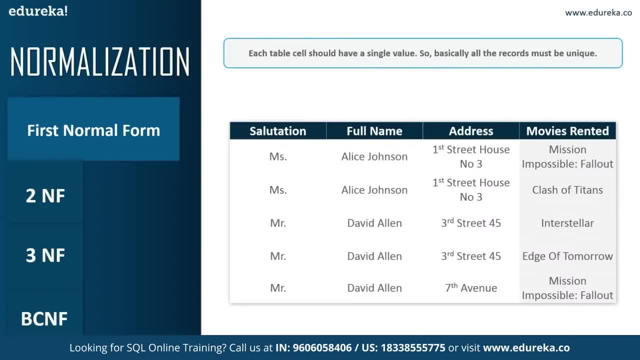 If you remember from the previous slide, what happened is that, you know, in the third Street 45 address one, David Allen had interstellar and edge of tomorrow together, right? So what I've done is I've divided those two into two different tuples again. 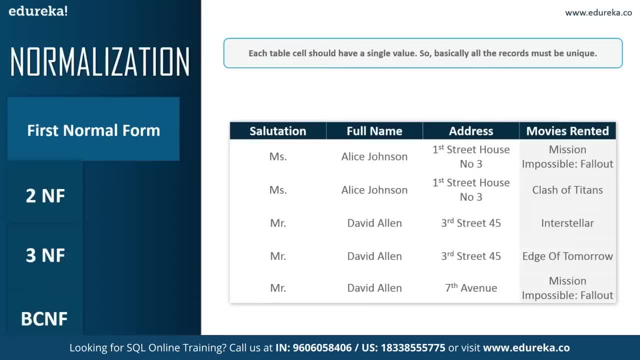 and they were Allen seventh and you into the next couple. So this is basically how I've got my table into one enough. Each table cell basically has only one single value. If you observe over here there's still a problem, right, That's because you know our address is written. 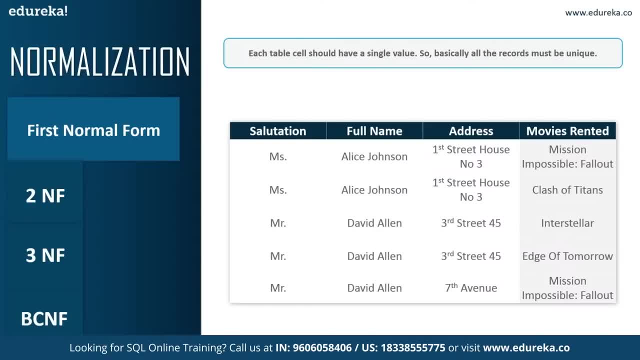 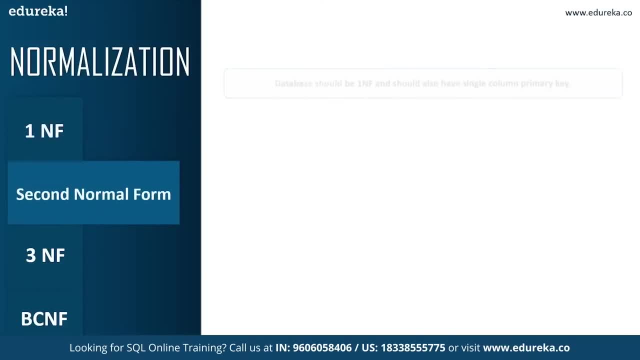 in for Alice Johnson and for David Allen. our address is redundant And, yes, it is divided. also, It's not all together. So for that, what we'll do is we'll convert this table into 2nf. So basically to normalize the database into 2nf. 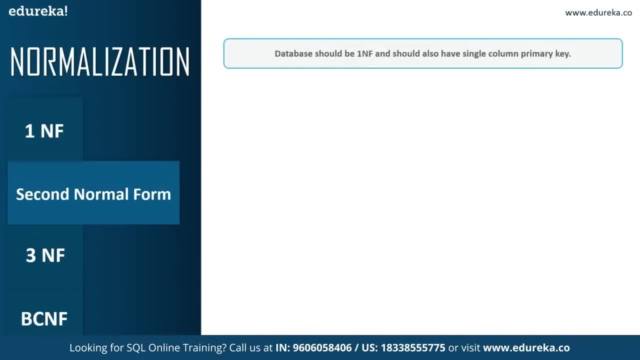 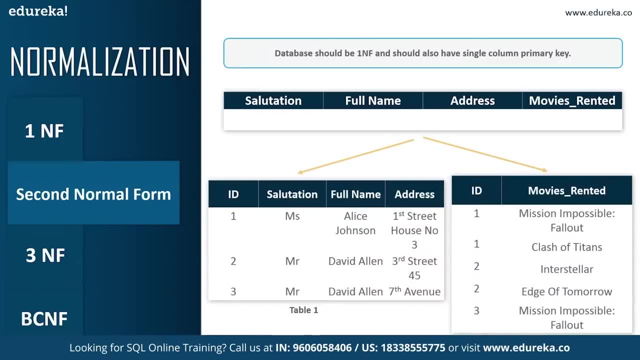 Remember the fact that you know the database should be in one enough and should also have a single column primary key. What I mean by that is you know what I'm going to do is I'm going to divide the table into two different tables, such that you know. 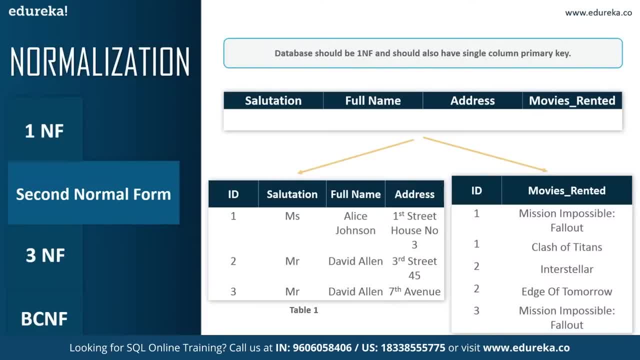 for each specific user, I'm going to identify the specific movie rented. for example, let's say, you know I give Alice Johnson, staying in first Street house Number three, ID number one. now I know she rented Mission Impossible and Clash of Titans. 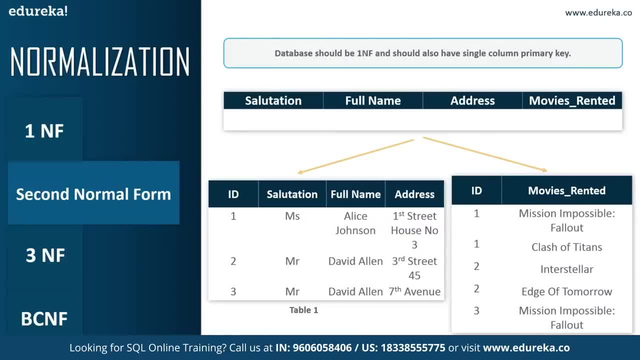 right. So what I did was I gave the movies Mission Impossible and Clash of Titans, which are rented by Alice Johnson, the ID one. similarly, what I did is for David Allen staying in third Street 45, basically, for that particular top will have given the ID to be to me know. 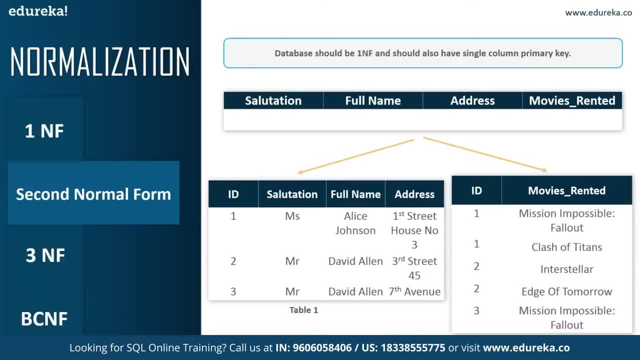 that you know he must have rented interstellar and edge of tomorrow, right. So for those particular movies I've given the ID to be to. and finally, for Mission Impossible, fallout, that is basically rented by David Allen staying in 7th Avenue, What I've given is I've given ID number three. 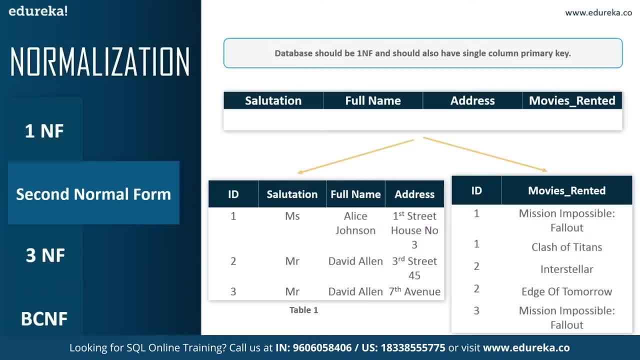 So that's how, basically, I have divided one enough table into two. and if now, if you see over here, there's still a problem right now, that's because you know we still have written in data with respect to Alice Johnson and David Allen, right? 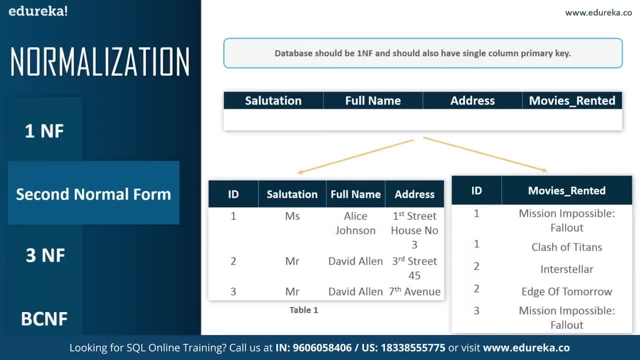 Because David Allen's name comes twice, as Johnson, who rents to movies, comes once. but yes, the address is also divided for David Allen. So to normalize this factor, what we'll do is we'll normalize again. So now we'll normalize the database, which is in the form. 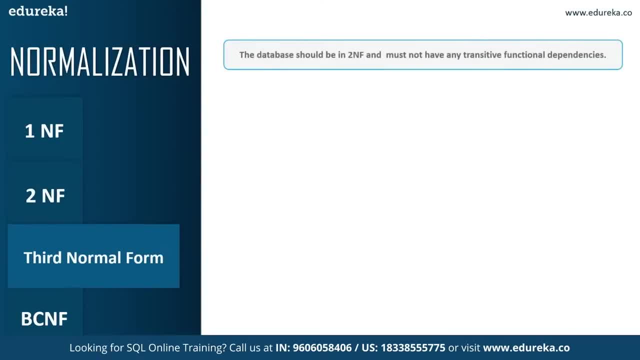 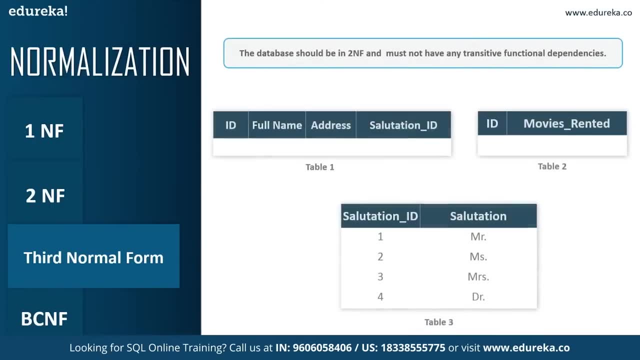 of 2nf to 3nf. Now if you want to normalize the database from 2nf to 3nf, the database should be in 2nf and must not have any transitive functional dependencies. So for that, what I'll do is I'll basically add a salutation ID. 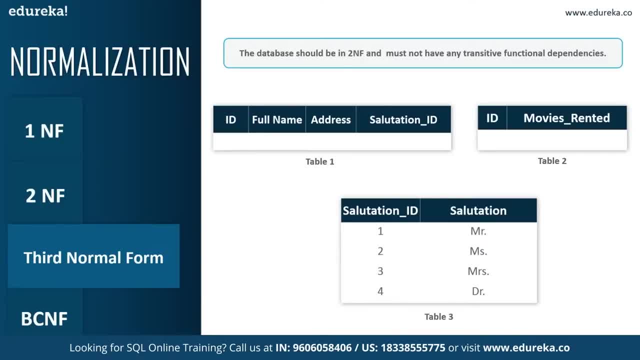 So, basically, I'm going to identify Mr from 1, miss from 2, missus from 3 and doctor from 4.. So, in that way, what will happen is that you know, David Allen's name won't come twice, because he'll be uniquely identified with mister. 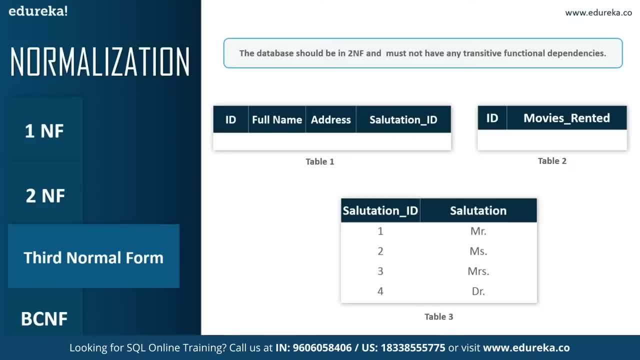 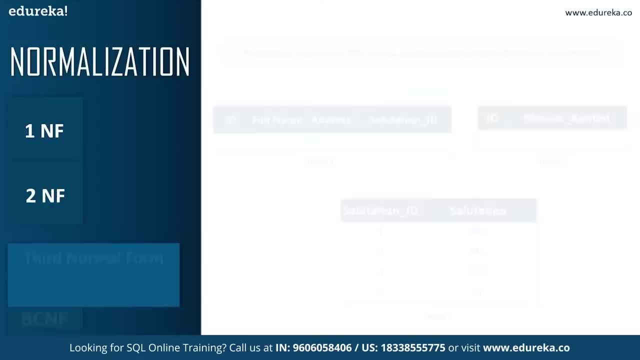 So we'll type in mr David Allen's. that will only comes once, and then all the movies will come together. So that's how, guys, basically you can normalize your database. So we've normalized from 1nf to 2nf, 2nf to 3nf. 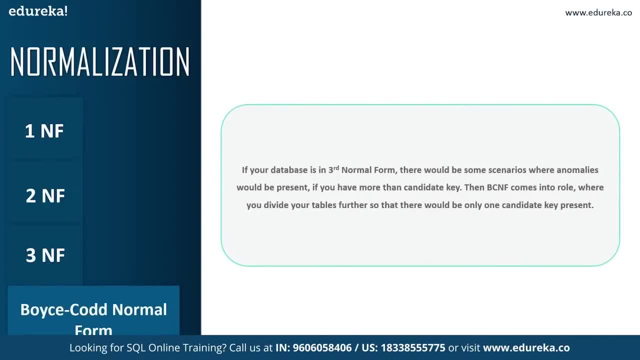 and finally comes BCNF. now, since my example ends there, So I'm not going to normalize it further, But yes, if your database is not yet normalized, you can then go forward and normalize again. that is BCNF, So to perform the normalization for the fourth time. 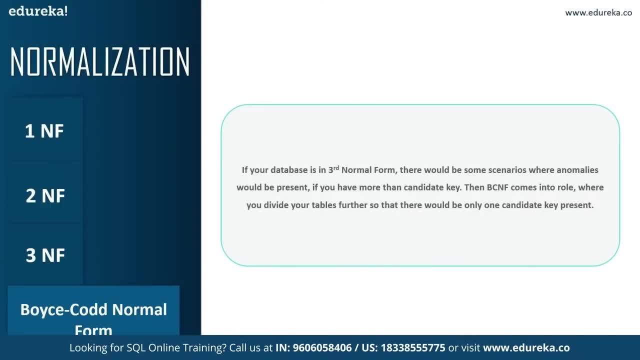 what you can do is you have to normalize, right. So the condition to normalize it again is basically that you know your database must be in 3nf and maybe you know, even after being in 3nf there would be some anomalies and it may have more than one candidate. now, 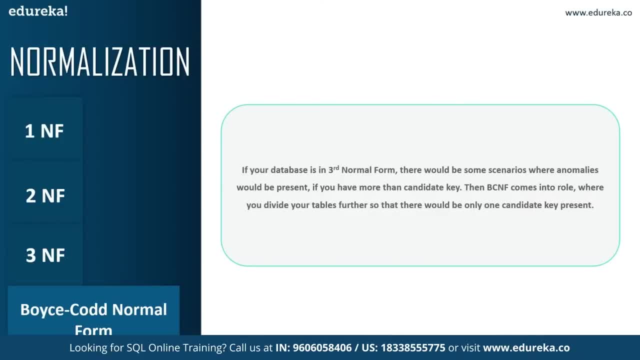 in such scenarios, what will happen is BCNF will come into the picture and then it will divide the tables further so that they would be only one candidate key present. So whenever, after 3nf, you observe that you know there's more than one candidate key, 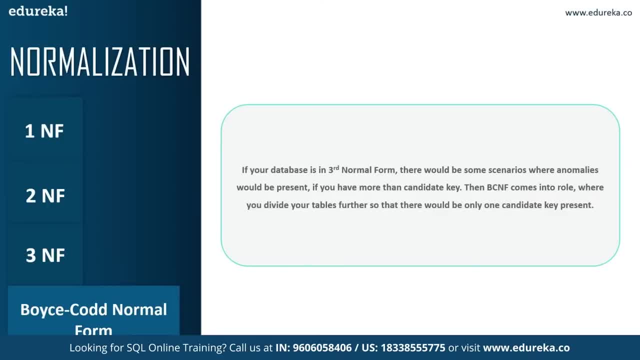 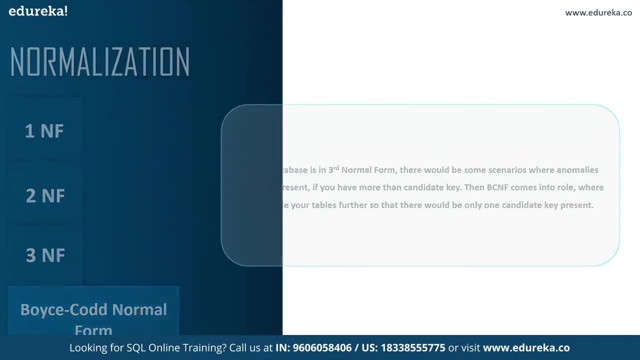 and then you'll have to normalize it again. That's where BCNF comes into picture to divide the table further. So, guys, this was about normalization. I hope you've understood how you can normalize your databases. Now let's move forward with the next topic. 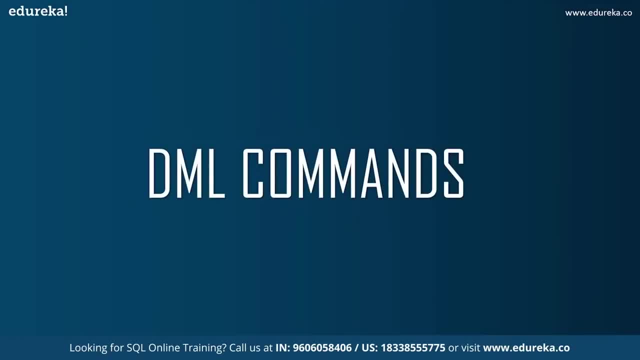 for today's session, that is, data manipulation commands. Now, the data manipulation commands, as I said before, are basically the commands which are basically used to manipulate your databases. So what I'm going to do is I'm going to manipulate data present in the database that I've created over here. 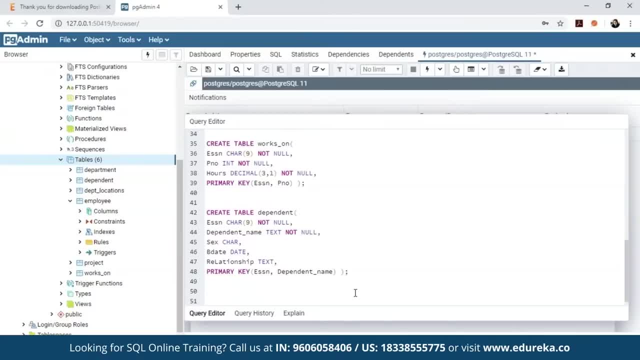 is in the six tables that I've entered. So to initially manipulate data, you need data present in your table. So now, to do that, what you have to do is you have to insert data. So to insert data, what you'll type in is insert into. 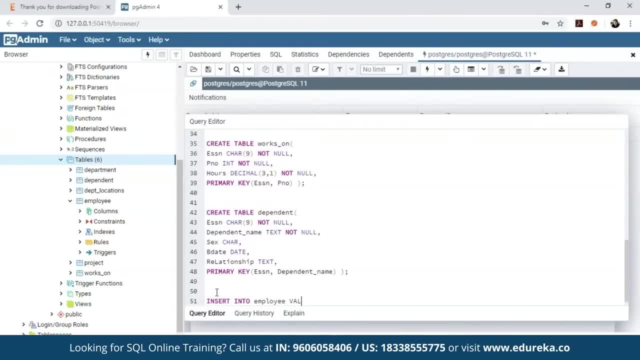 and then let me show you for employee table employee, and then you'll mention values and then you'll have to mention the values that you wish to enter, right? So let's say I'll wish to enter John as first name and let's say I'll enter middle name. 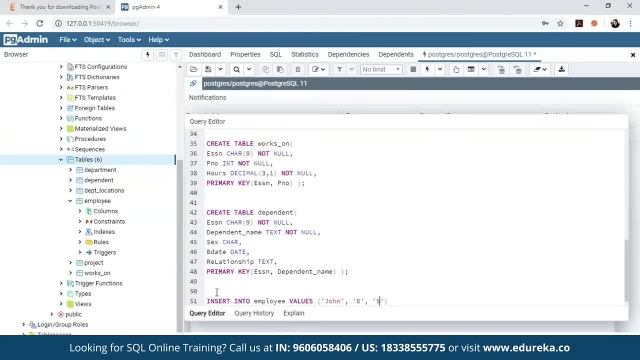 Let it be a character now. Similarly, I'll enter the next name, Let's say Smith. that is basically my last name. Sorry, the comma has to go at the end. now I'll enter SSN right after that. What I'll do is I'll enter bird date. 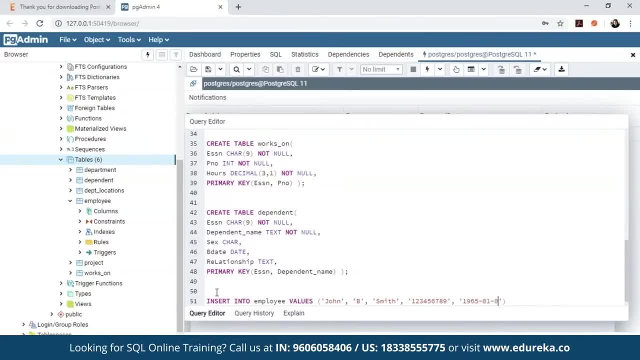 So let's say, you know I mentioned 1965, 0109.. Then let's say, you know I mentioned address. So let's say I mentioned 731, Houston, TX. and let's say further: I mentioned the gender to be mailed. 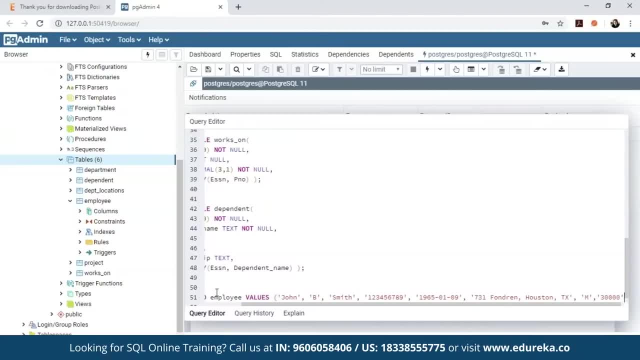 and then let's say we mentioned Sally to be 30,000, and then we mentioned super SSN. Let's say triple three, double four, four times five. and let's say we mentioned the department number to be five. Now, once this is done, 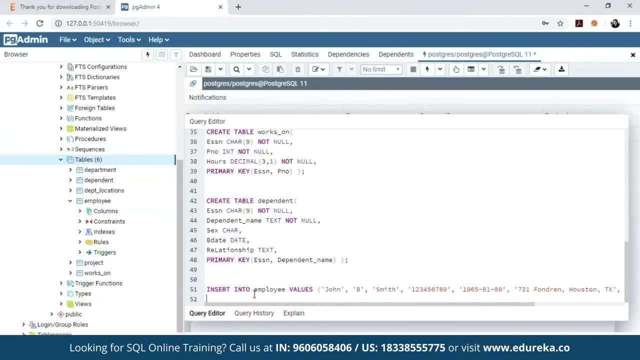 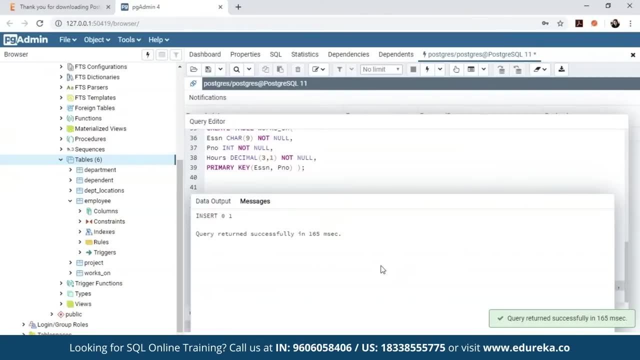 you can just execute this particular query. So what you can do is you can just hit on execute and you'll see that you know automatically the query has been returned successfully. That means the data is filled. So if you want to see the data output, what you can do is 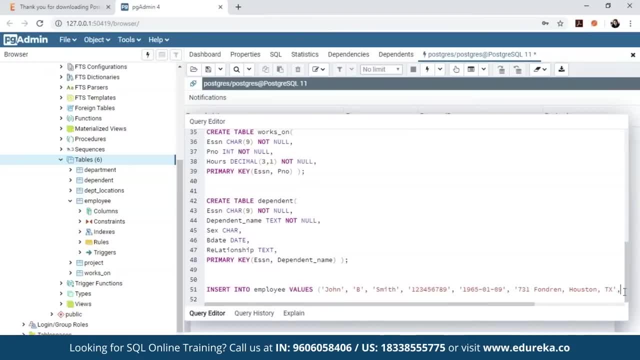 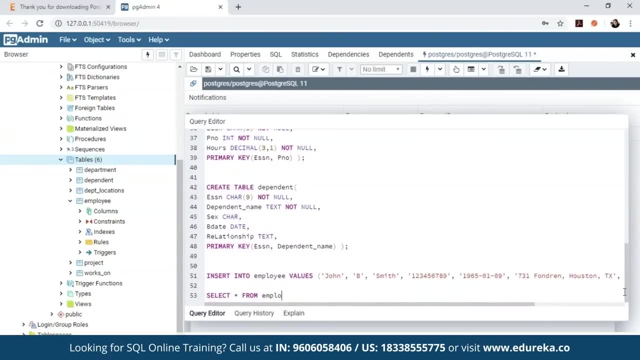 you can use the other manipulation command that is basically select star from employee, So that will basically show you all the values present in the employee table. So let me just mention that and then I'll hit on execute and you'll see that you know automatically. you see the data. 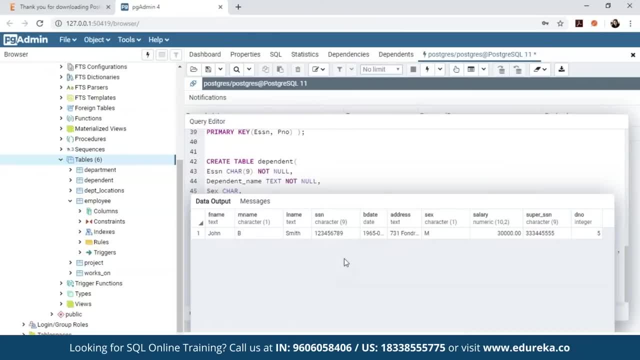 present in the table. That is whatever we have mentioned over here now. since guys filling data would be a waste of time for me to explain for each and every value. I've already put it in my talk, So I'll just copy paste from there. 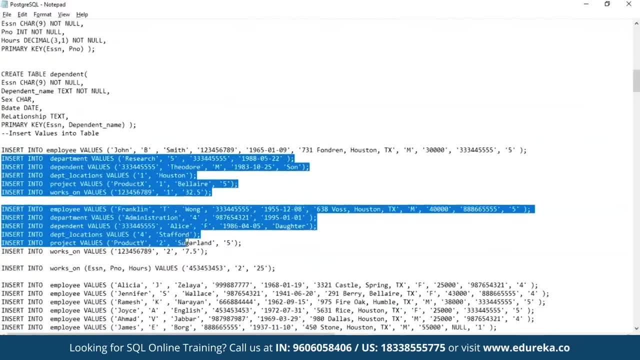 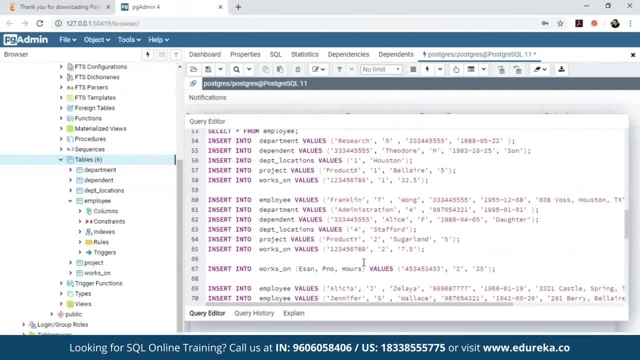 so that we can move faster in the session, right? So let me just copy paste these commands. So, if you observe over here, what I'm doing is I'm entering data into the department table, the dependent table, the department locations table, projects table, works on table, and so on. 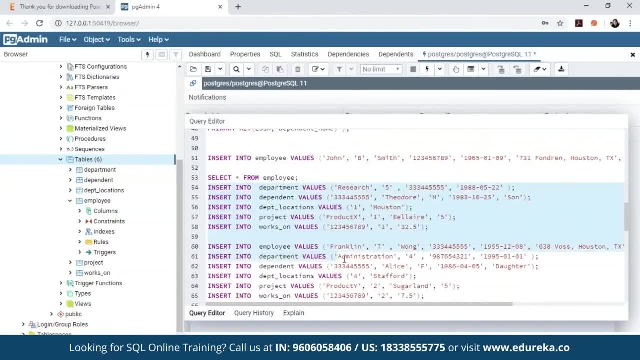 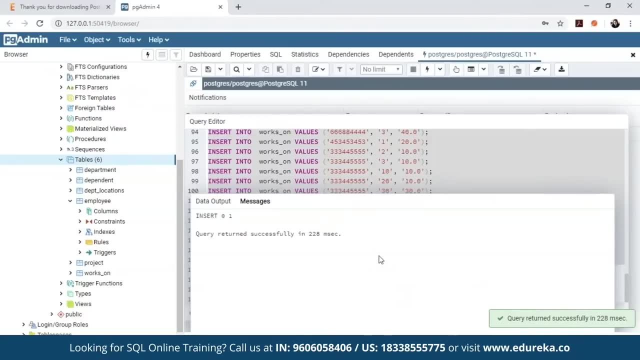 So I'm not entering just one, I'm entering quite a amount of details. So what I'll do is I'll just select all of them together and then I'll hit on execute. Once I hit on execute, you'll see that you know. 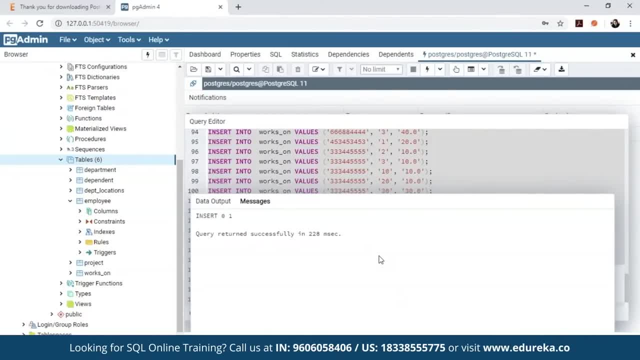 the query has been returned successfully, That means that you know automatically our data has been entered into our tables, right? So if you just want to check how if the data has been entered or not, you can similarly use the same command that I just showed you, that is, select star from. 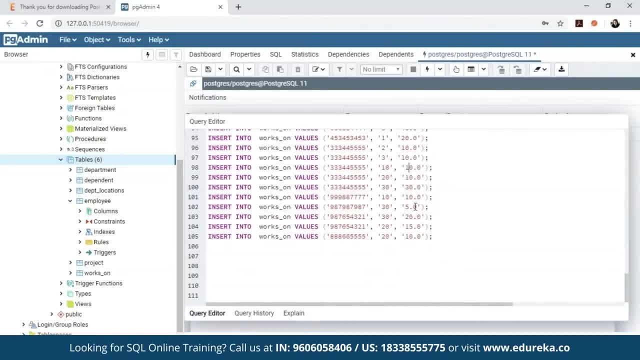 and then you mentioned the table name, So now let's move forward with the session. Now, as you remember, from the entity relationship diagram, I said there were relations between two entities, right? So those relations are basically made into picture with the help of foreign keys that I mentioned before, right? 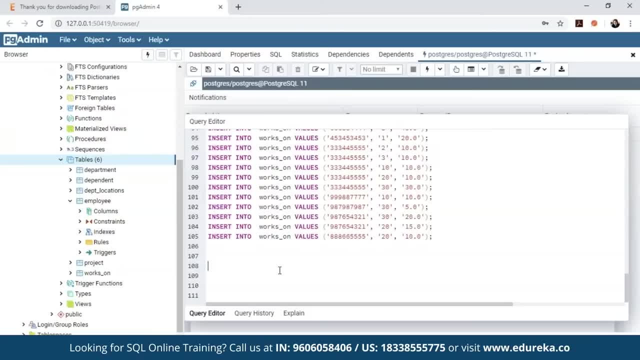 So to add foreign keys, what you'll do is you have to alter the table, since the tables are already created. So what you can do is either you alter the table or or the other way. completely round is basically whenever you're creating the table. 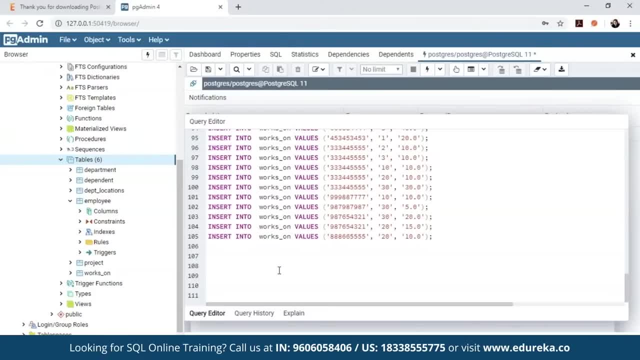 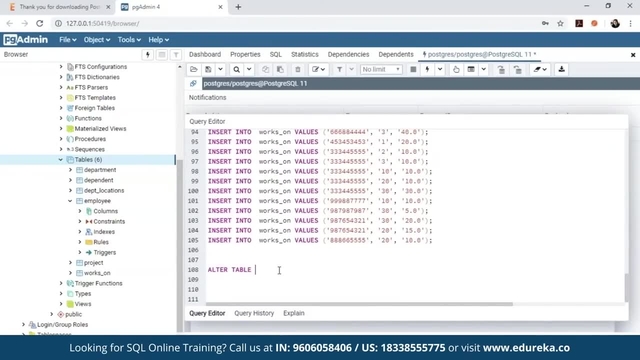 you can add foreign keys. So I'm just going to alter the table, since you know my tables are already created. So for that, what I'll do is I'll put an altar table and let's say: you know, I add a foreign key for the managers relationship. 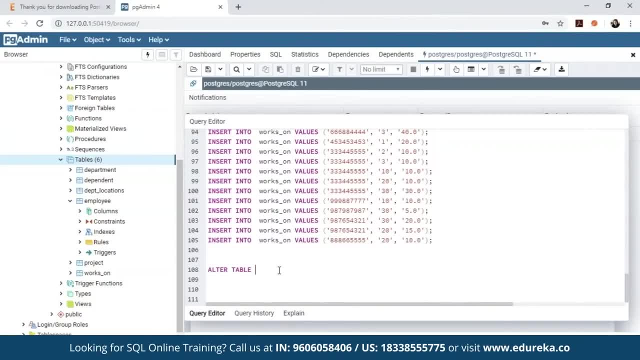 So what will happen is I want to add a foreign key for the managers relationship. Well, you know, I'll say the department is managed by an employee, right? So what will happen is Department will be our first table where we'll add a foreign key, basically MGR SSN. 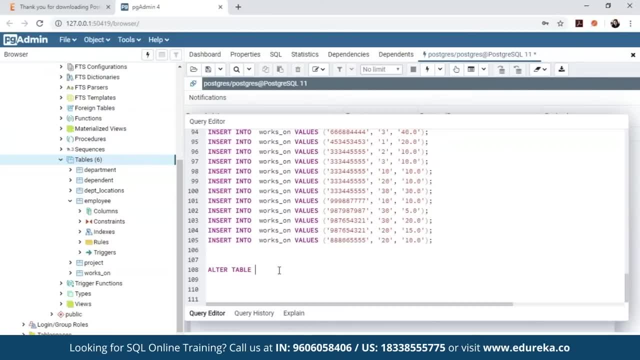 which references to employee table, because every employee manages a department. So that's what I'm going to do. So I'll mention alter table and then let's say we mentioned Department, then I'll mention add foreign key and then I'll mention the column attribute. 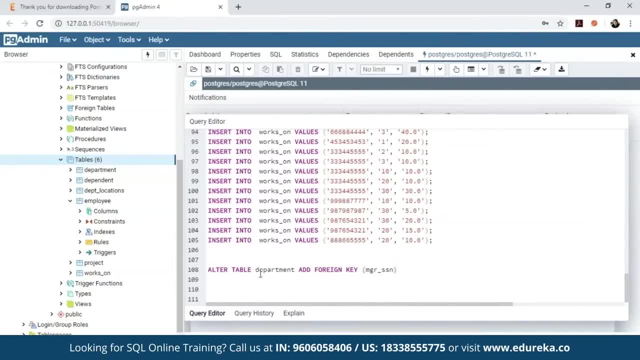 which has to match, right. So that is MGR SSN That I had created in the department table, and then I'll mention references. Oh, I'm sorry, There's a spelling mistake over here, right, And then I'll mention the table number two. 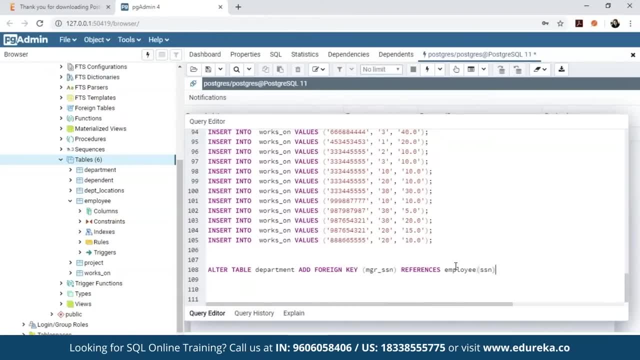 that is, employee to SSN. So basically you have to add a foreign key to each of the columns, right? So you are basically trying to connect the MGR SSN column of a department table to SSN column of the employee table. You'll just execute this. 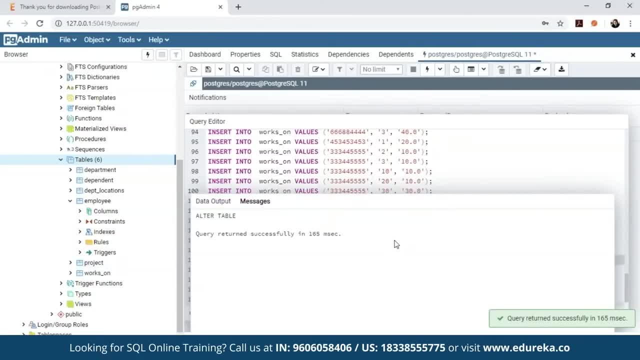 and then, once you execute this, you'll see that you know query return successfully, Which means there is a foreign key right. So, for example, let's say, if I just refresh this, and then we go to the employee table and then if we see the properties, 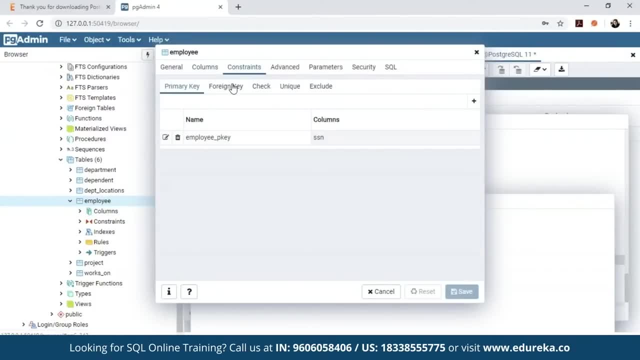 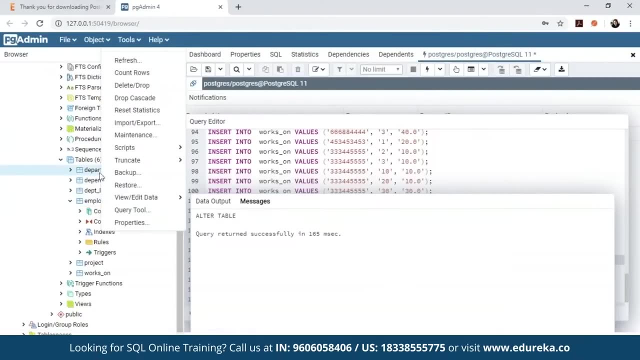 and let's say you know we go to constraints over here and in the primary key we see that you know it's SSN and in the foreign key So there's nothing over here. So I had to go to the department table. 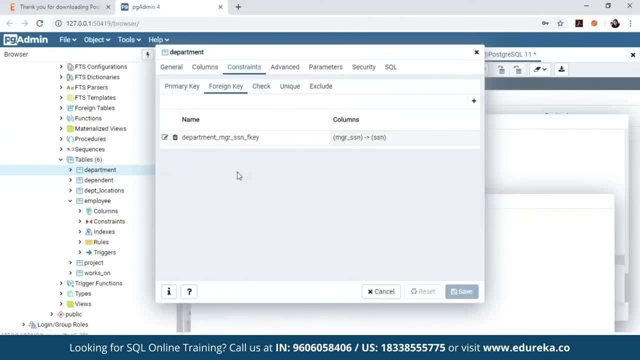 So let's go to properties, because you know we are adding the foreign key from there, right? So I go to foreign key. You see that you know MGR SSN foreign key. basically MGR SSN is connected to SSN. 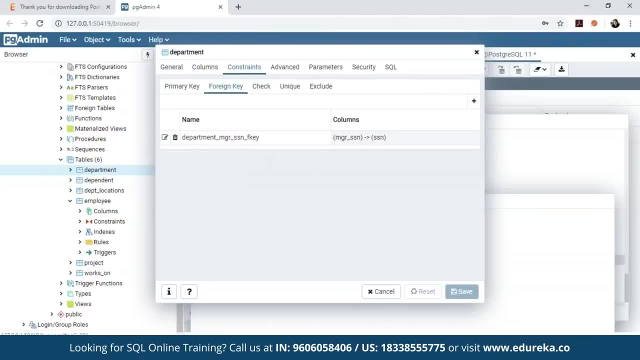 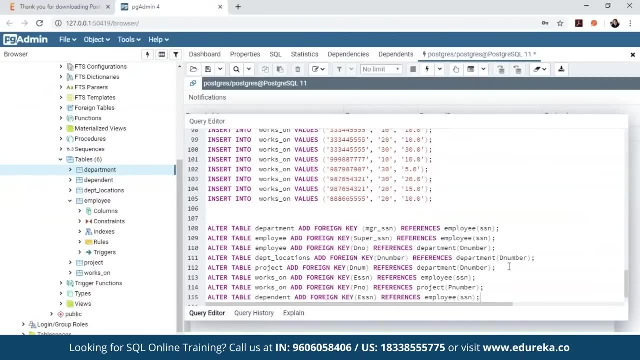 So you clearly see that you know that's how you can add foreign key. Now what I'm going to do is I'm going to add foreign keys for other tables also, so that you know we can move forward again. Let me just directly add it from here, right? 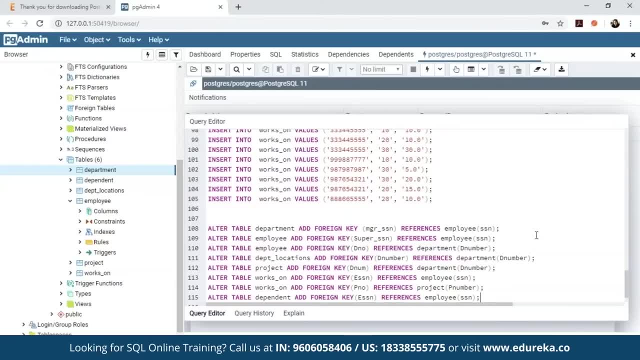 So, as you can see on my screen, I've mentioned a foreign key between employee SSN and an employee super SSN. So that was basically for our self-referencing relationship. Then I mentioned a foreign key between department number and the department. basically who works on which department? 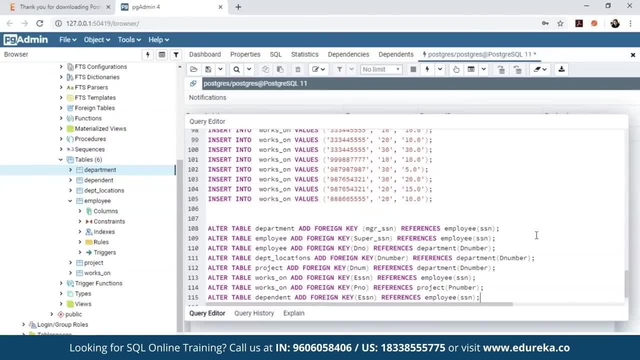 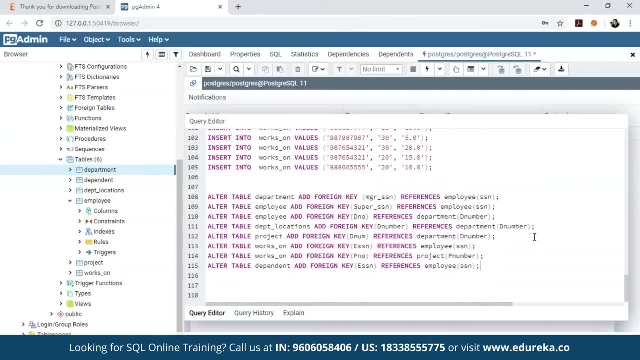 right. So for that particular relationship. after that I've mentioned a foreign key for Department locations and the department. So basically, which department is present in which location? after that I've mentioned the foreign key between project and Department. basically, which department is looking into which project? 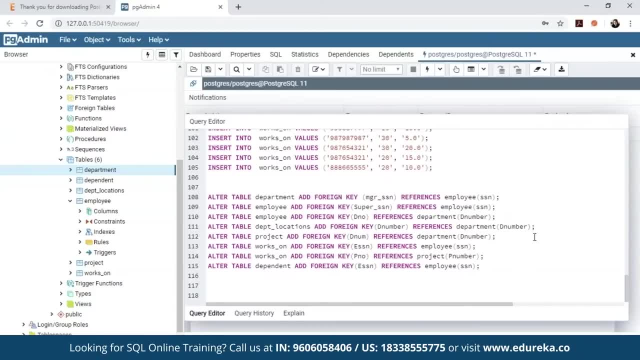 and then I've mentioned a foreign key between works on table and employee table to understand which employees working on which project or which department, and finally, on the dependent and the employee table to make sure the dependency relationship is taken into account right. So what I'll do is I'll just execute all. 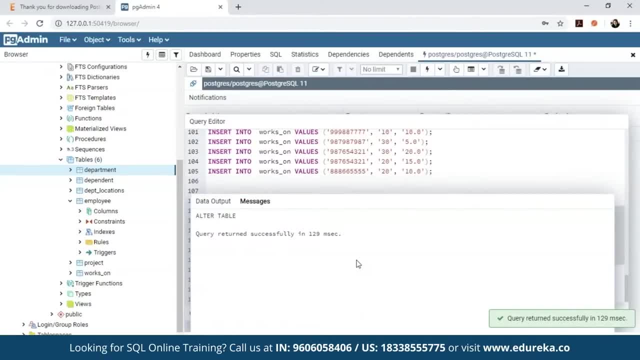 this particular foreign keys. So I'll hit on execute. you'll see that you know, automatically the query has been executed, right? So, guys, that's how, basically, you can add foreign keys to all your tables. you know, if you just refresh over here. 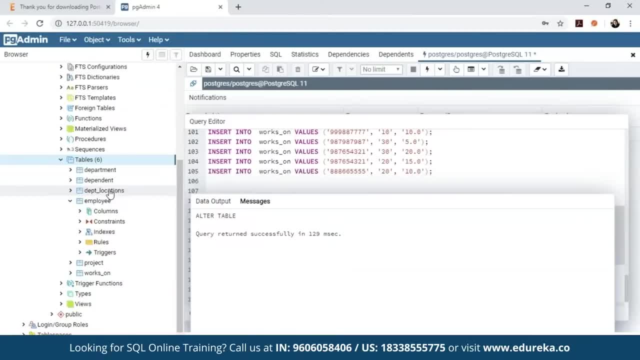 and then, if you check all the tables, you'll see that you know there's some of the other foreign key present for each and every table, that is, for each and every relation. Now let's move forward. Now, for example, let's say: you know, 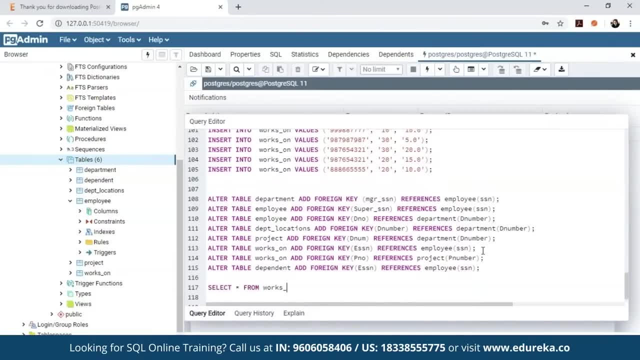 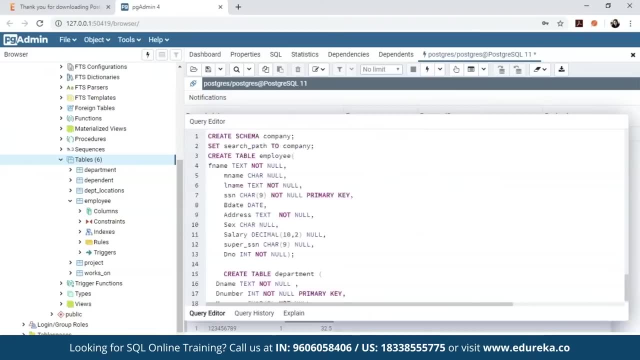 I want to see all the details from the works on table right Now. let's say: you know I want to delete records with the project number, Let's say 30. Let's try deleting, right, So if I try deleting, 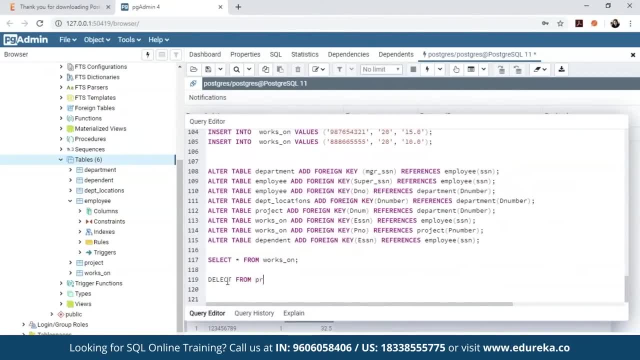 let me just write it over here: delete from. you have to delete from the project table. and then I'm saying the project number. I've considered 30, right? So I'll just type in 30 and let's see what happens when we execute this. 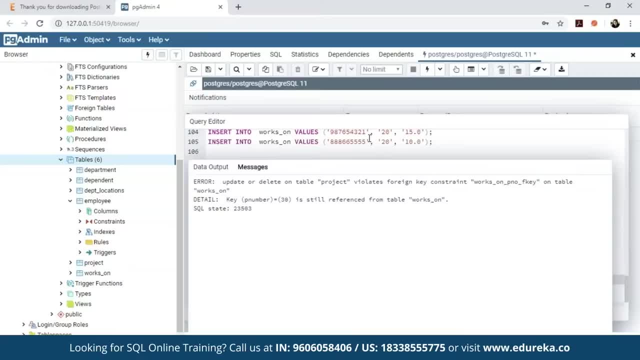 Okay, I'm sorry. Yes. Now, when you execute this particular statement, what do you say? you see an error that you know update or delete on the table project, while it's foreign key constraint because we have a foreign key with respective works on right. 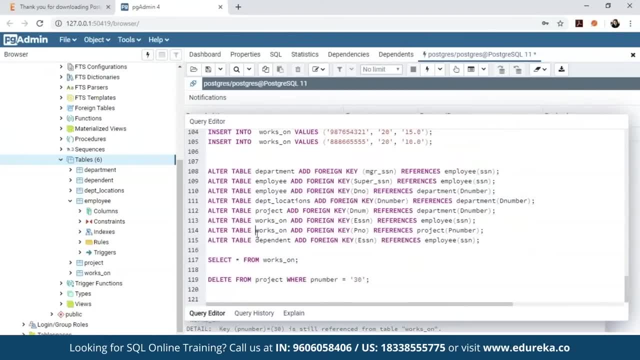 So because we just mentioned over here that you know we'll have a foreign key with works on and project number. So now that's the reason we get this error. now to resolve this error. Basically, I'm talking about the concept where you want to delete the records. 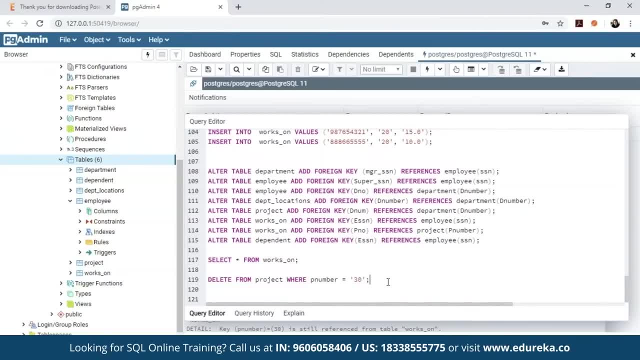 where foreign keys are present, right. So what you'll do is you'll initially delete the record from the works on table and then you'll go forward and delete the records from the project table, So you directly won't come over here. What you'll do is you'll initially delete 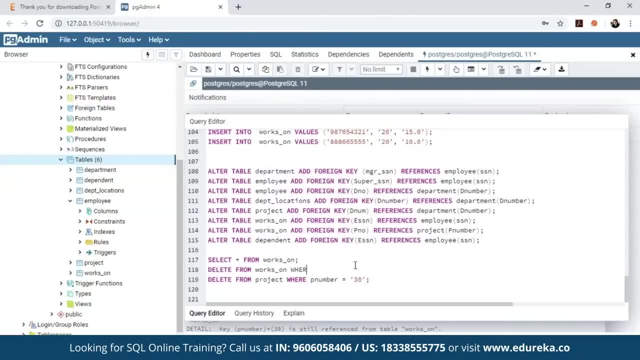 from works on table. So let's say P number is 30, right, So I'll delete the record from the works on table over here. You'll automatically see that you know query returned successfully. and now if we try deleting data from project table. 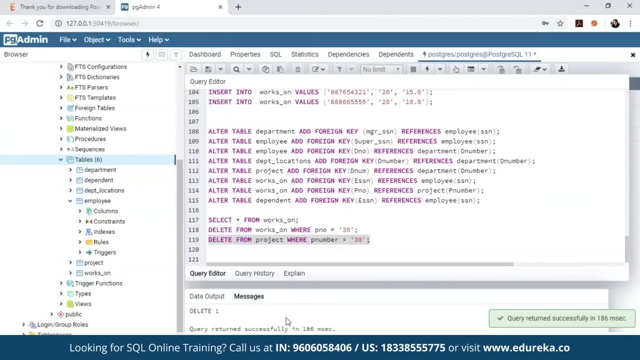 what you'll clearly see, that you know queries return successfully. That means there was no violating error, right? So what happens is whenever you have a foreign key from a table to be table, Remember that you know if you want to delete anything from the B table. 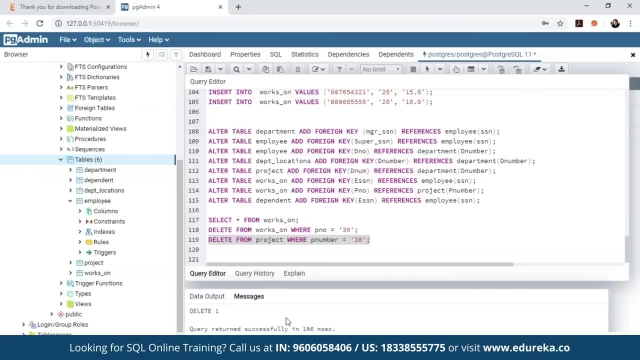 you have to first delete it from the A table and then you can go forward and delete it from the B table, right? So, guys, that was about the insert statement to alter statement and about foreign keys. Now, in this session, what I'm going to do is I'm not going to talk. 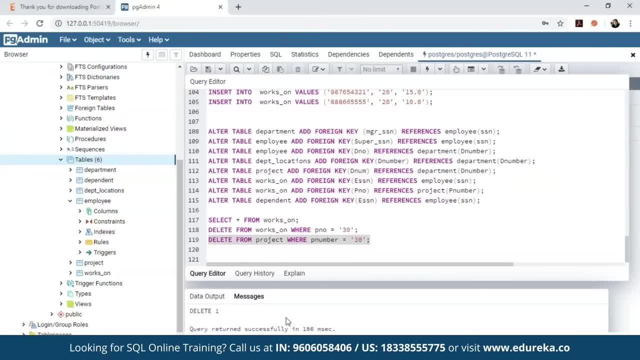 about any theory part, like what's going to happen and then how you can use. what I'm going to do is I'm going to directly jump on the query so that you can understand how you can write queries and how you can manipulate data. So let's get started. 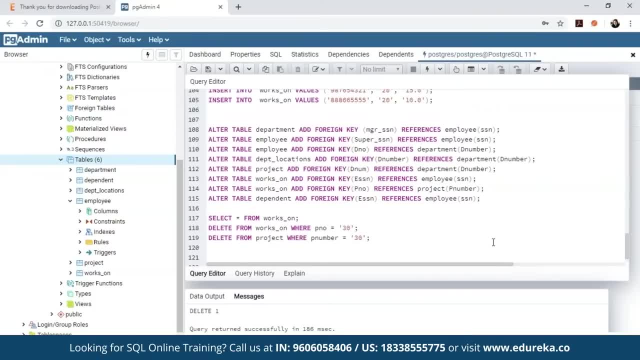 So now let's say, you know we want to update the salary of employees. So, for example, let's say I'll just see which employee salary has to be updated, So I'll just type on select, I'll start from employee so that I can see the details. 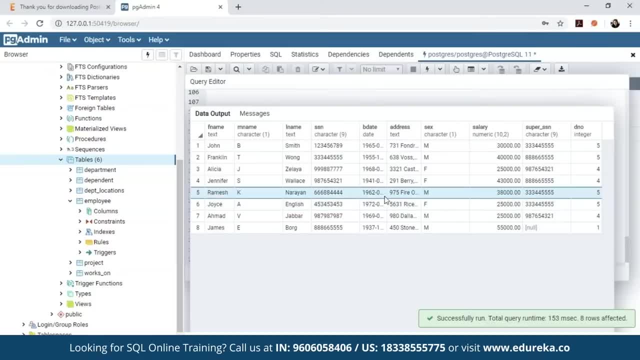 I'll just execute this. So when I execute this, you'll see that you know. I have all the details right now. Let's say: you know I want to update the salary of a person, Let's say employee, whose SSN is, let's say, triple, nine, double. 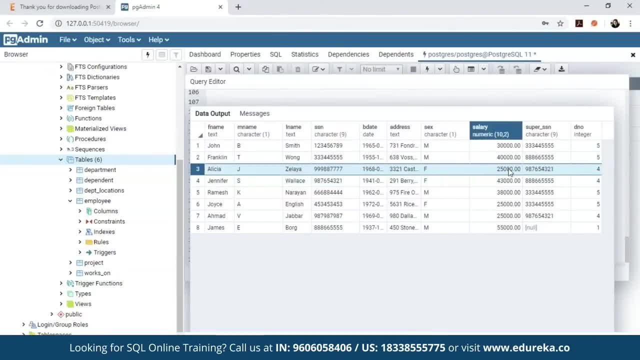 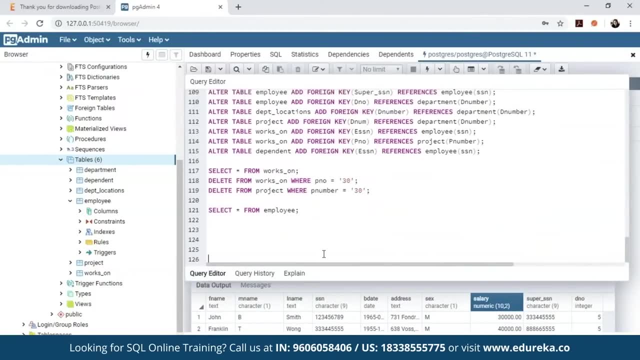 eight, four times seven. Now, let's say, the salary is around 25,000 right now. I want to update it to 27,000.. What can I do is basically, I have to use the update statement. So, to use the update statement. what I can simply do is: 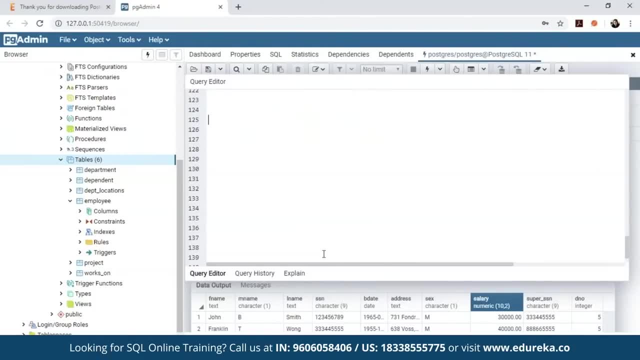 let me just bless and enter so that the screen is clear for you guys. I could just type in update and then you have to mention the table name, So that will be employee, and then you'll mention set column name, And then what you'll do is you'll mention the new value. 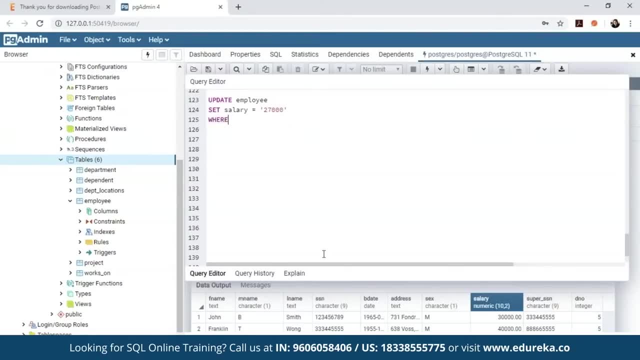 that you want, that is, let's say, 27,000, and then let's say where SSN, that is, basically, to which you can uniquely identify every tuple right. So where SSN is equal to what was the SSN. It was triple nine, double eight, four times seven. 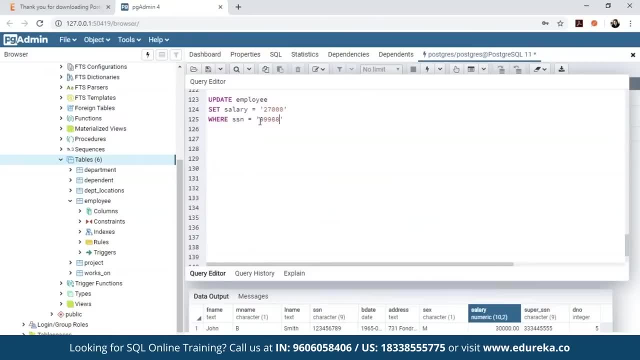 Right. So I'll just type in: triple nine, double eight, four times seven, and then what I'll do is I'll just end with a semicolon. Once I execute this, you see an output that you know. query returned successfully, right? So now let me just go back over here. 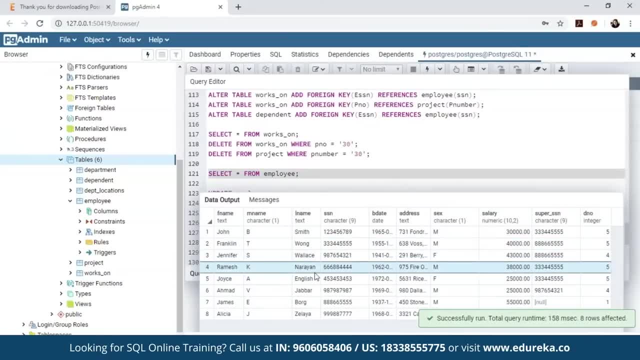 and choose select staff from employee. And now, if you go back to this particular table, you can clearly see that you know the employee who had an SSN about triple nine, double eight, four times seven has now a salary of 27,000. so, guys, that's how you can update the values. 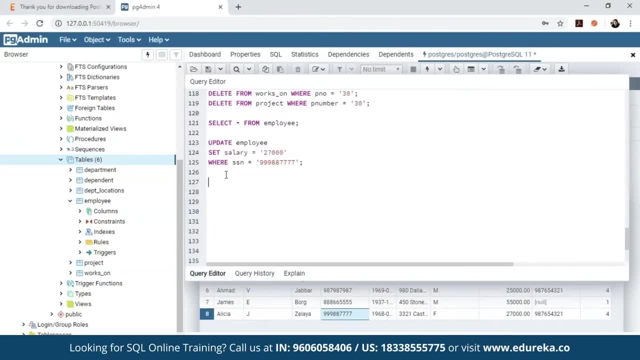 So, guys, that was about the update statement. Now let's say you want to delete or tuples data, you know, let's say more than one condition, So what you can do is you can just use the delete statement- Okay, delete from. and then let's say we want to delete it. 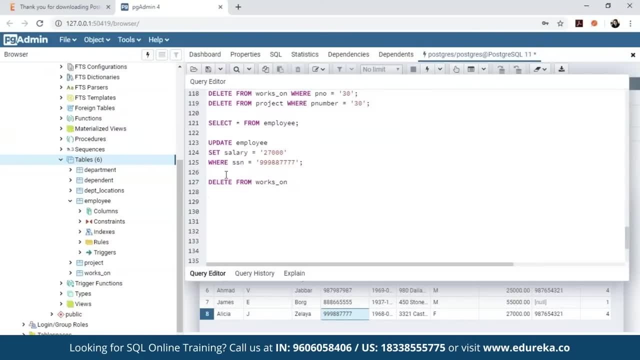 from works on table right. So I'll just type in works on and then let's say where employee SSN? because our works on table has employee SSN as column right. So we are, if you can see, we have a SSN. and let's say: 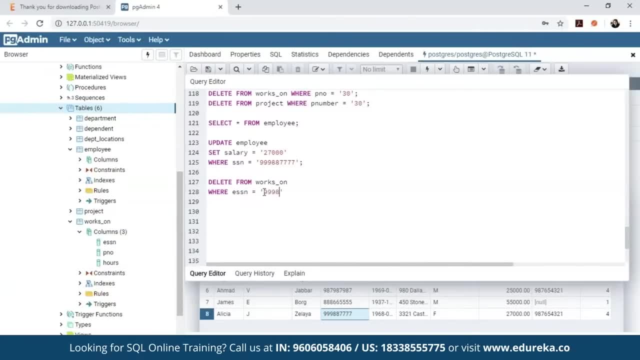 you know, we use the same employee SSN- Let's say triple nine, double eight and four times seven, and we also have project number details. right, So we are. I'll choose project number. Let's say: right, So that is basically the data had mentioned. 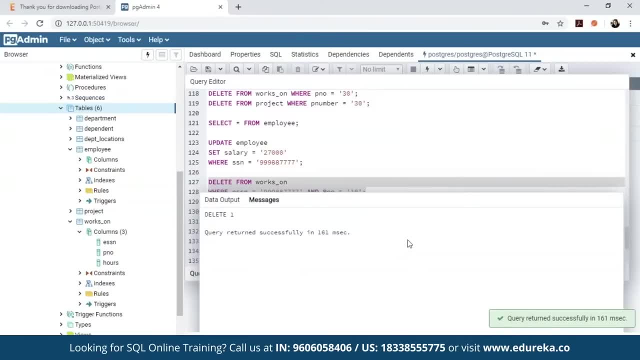 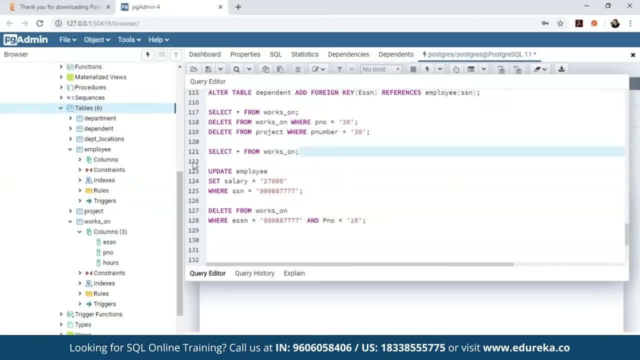 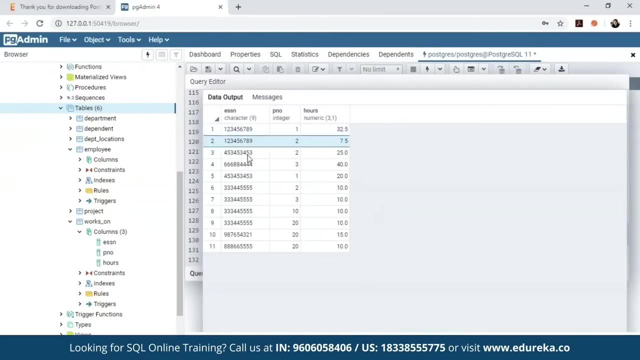 So I'll just execute this particular query and you see that in automatically is executed, right. So now if I just change this from employee to works on and then if I execute this particular query, you can clearly see that you know we have no employee with employee ID. 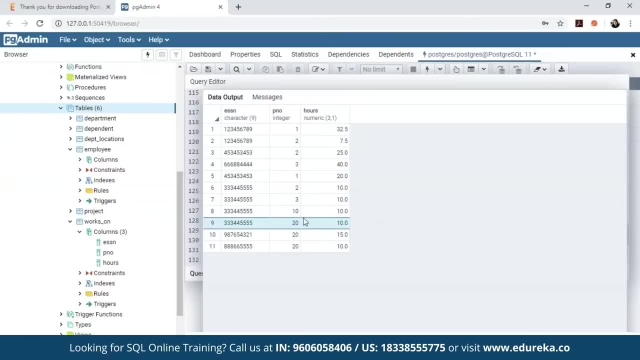 of triple, nine, double eight, four times seven and working on project number tens data present in the works on table. So, guys, that was about how you can delete, update, insert and alter. now let's move forward with one of the most important queries, that is, the select query. 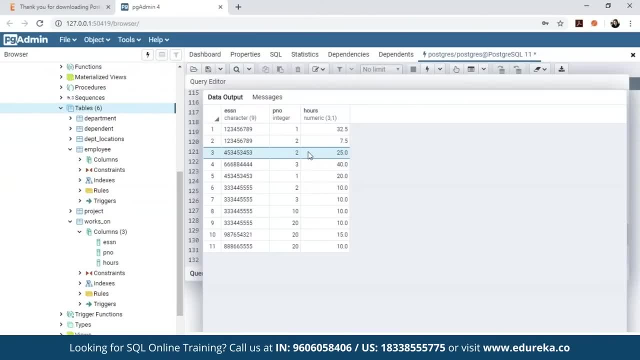 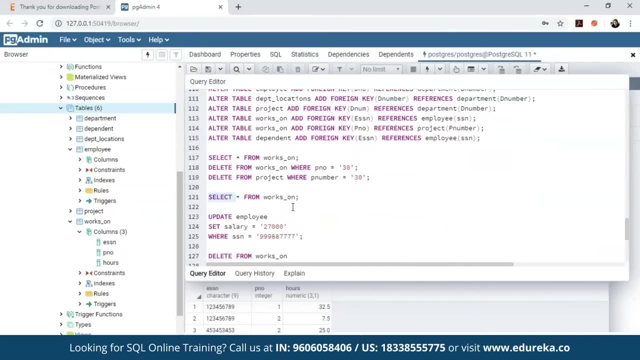 Now the select query is basically considered as one of the most important queries because you know this is the query through which you can retrieve the data. So, as you can see over here, I was using select query again and again because, you know, I wanted to retrieve the data that I have in my database. 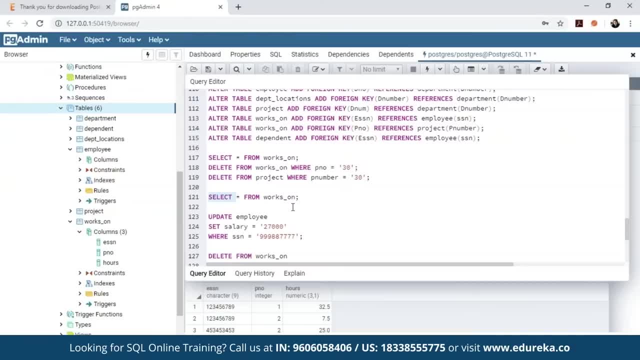 So that's where basically, the select query comes into picture. Now, when I had select star from works on, that means all the data was shown. for example, let's say I just want the first name, last name and the address from the employee table. and let's say: 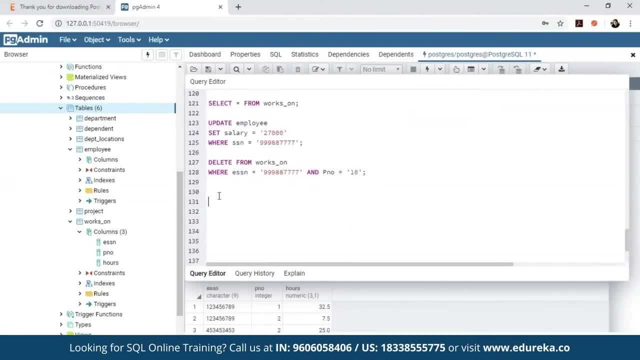 you know we are specific to Department number five. So what I can do is I can just type in select first name, last name, address and I'll mention from employee. and let's say we mentioned Department number is equal to five. So I'll execute this particular query. 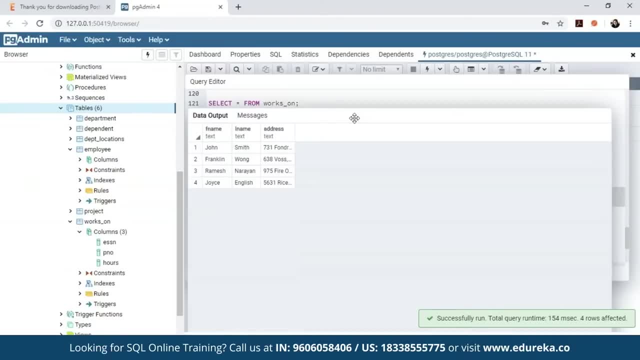 So when I execute this particular query, you can see that you know John Franklin Ramesh, enjoy. So basically, the first name, last name and address have come into picture, right. So that's how, guys, you can use a select query. 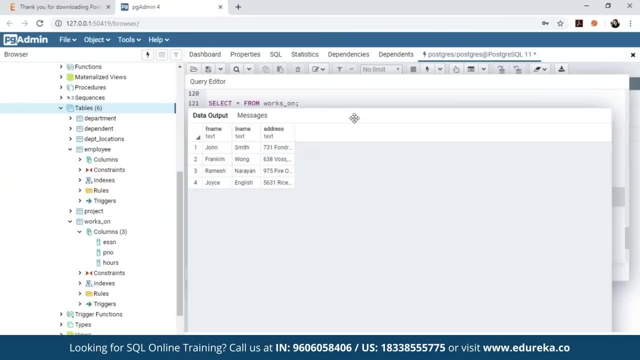 Now, This was quite a simple one. right now, Let's look into something more complicated. For example, let's say you know you want to retrieve data for every project located in Bellari, and then you want the project number, the controlling department number. 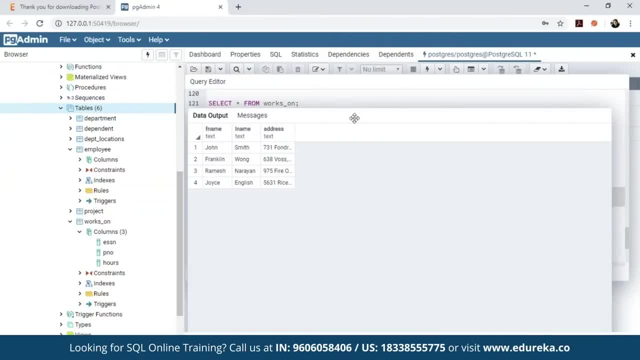 and the department managers: last name, address and birthday. So over here, if you observe what all I've ever taken into account: the project number, the department number, the department managers, the last name, address and birthday. So if you observe over here basically what's happening, is there three tables coming? 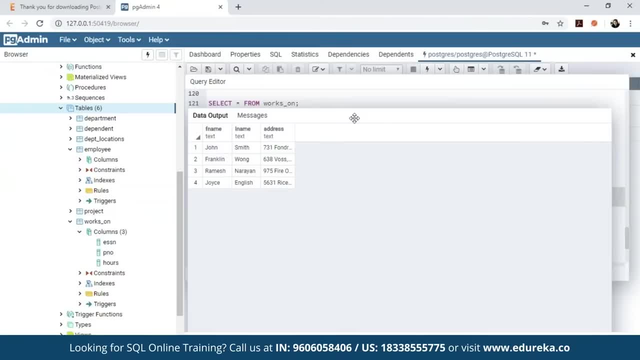 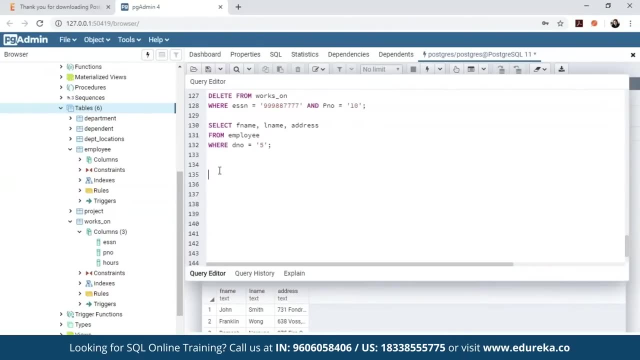 into picture, right? That's basically the project table, the department table and the employee table, So let's look into how we can write the query for this. So what all did I mention? I mentioned the project number, the department number, last name, address and birthday. 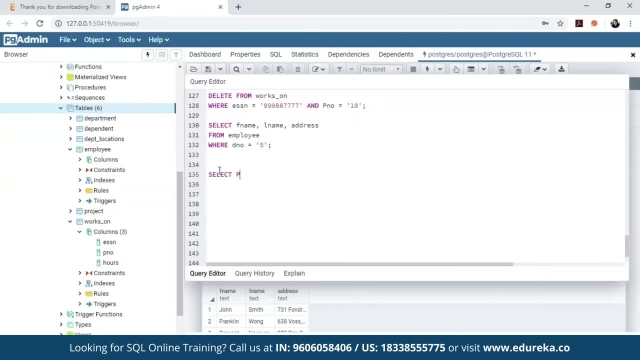 So what I'll do is I'll mention select and then I'll mention all these factors. that is project number D, now right, and then I'll mention L name, That is basically my last name, and then I'll mention address. say, we mentioned birth date. 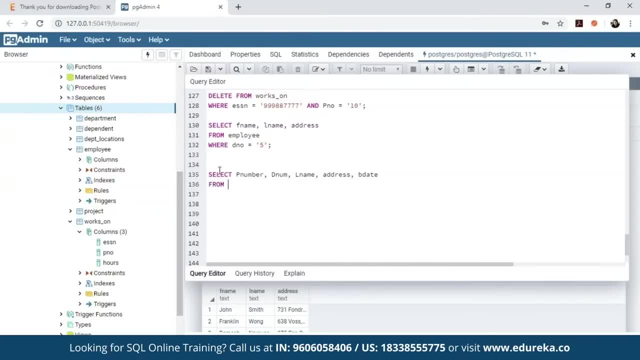 right. and then I mentioned from what are the tables that I had considered, that is, the project department and the employee right. So I mentioned project department employee Where the num is equal to the number. So basically the department number from the project table has to match the department number from the department table. 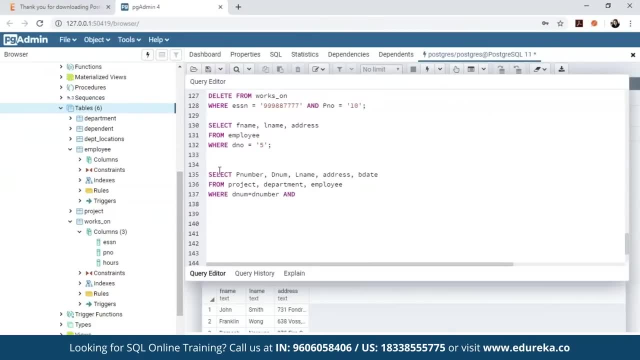 also. So that's basically: you use an operator known as and, and then you mention MGR, SSN. that is basically who manages the project- has to match with the employee code. that is right: SSN. apart from that, We also have to mention that. 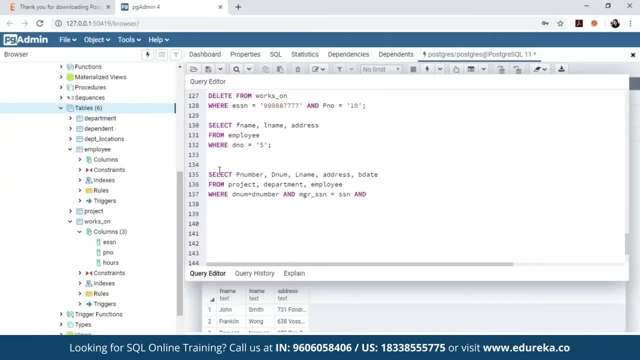 you know our project location is Bella, So we'll mention and be location is equal to in quotes, will mention Bella, right? So if I just execute this particular query, you'll see an output that you know there are no tuples with satisfied this particular condition. 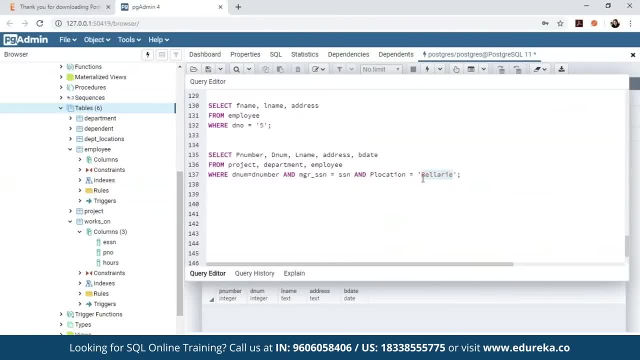 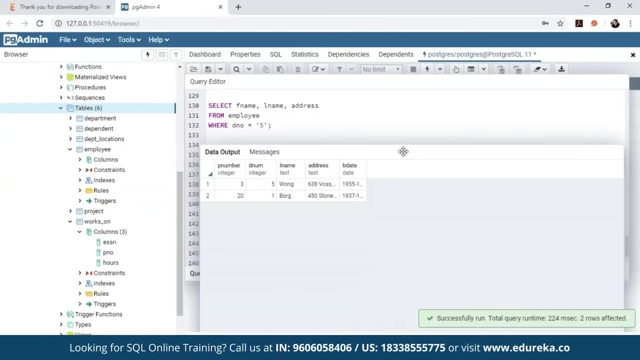 right. So what I'm going to do is let's say we change Bellari to let's say how? still right now. Let's execute again. Now, if I execute on Houston, you can see that you know we've got the project number, the denom, the last name. 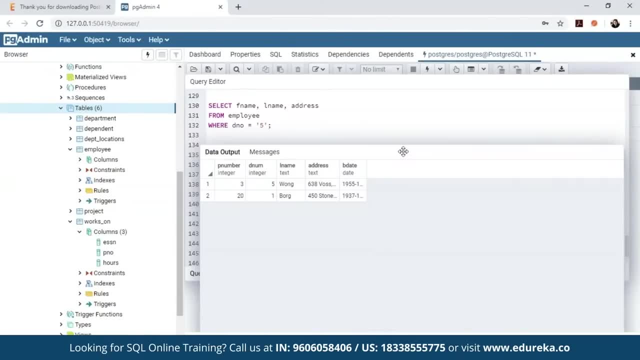 the address and the birth date of basically all those employees who work on the project, basically located in Houston. So that's how, guys, you can basically integrate two to three tables together and use the select statement to further play around with it. Now, if you remember, I was talking. 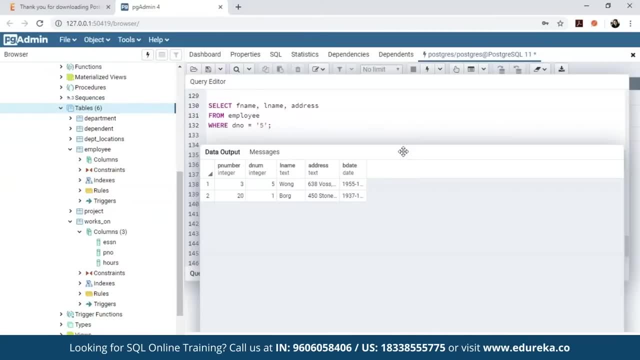 about the self-referencing relationship where you know we have employed related to himself, right? That was basically how a supervisor can have a supervisor. So, for example, let's say, you know, for each employee we want to retrieve the first name and the last name. 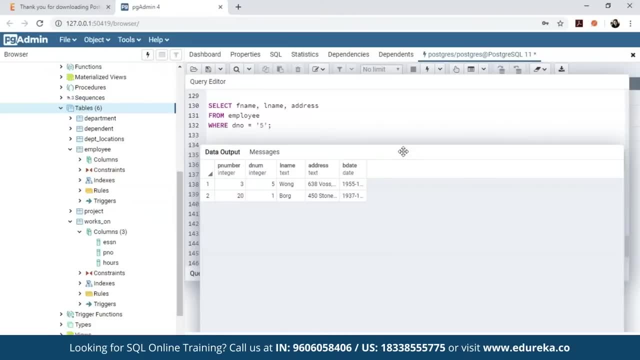 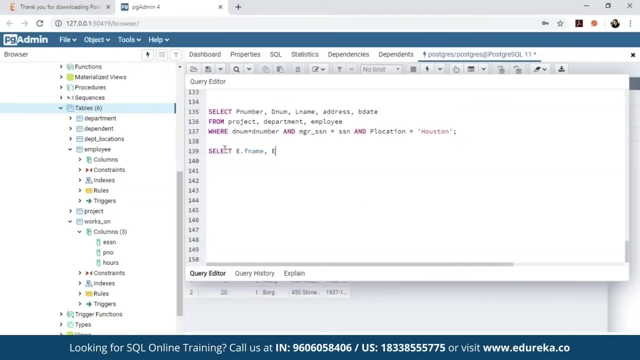 and also the first name and the last name of the supervisor, then what we can do is we can use the select statement again, right, And then I'll mention e dot F name and e dot L name. So this is basically to identify every employee, right? 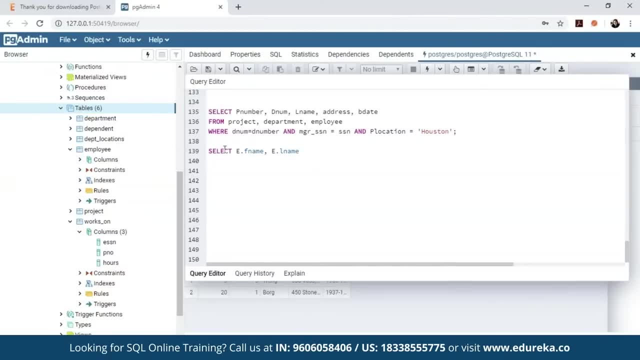 So that is basically the supervisor. Now, if you want to identify the supervisor, what I'm going to do is I'll mention s dot F name and s dot L name, and then I'll mention from, and then I'll mention employee. Sorry, let me put it in small so that it's clear to you. 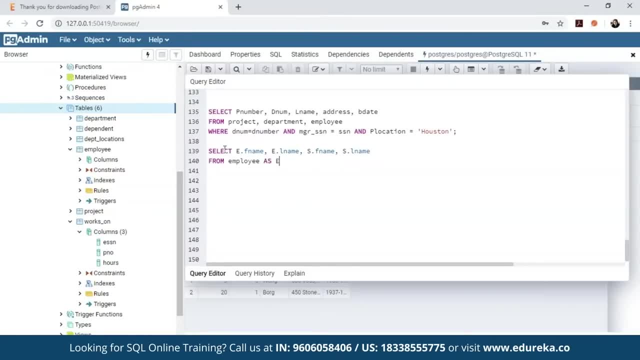 from employee As e right. so for every employee, that is basically for every supervisee, I'm identifying employee as e and similarly for supervisor I'm going to identify as s right. So I'll mention employee as s, where e dot, super SSN is equal. 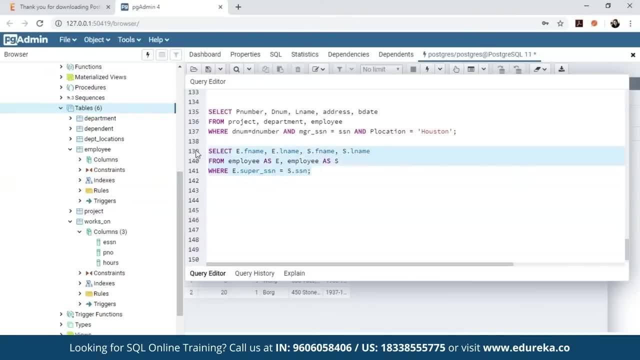 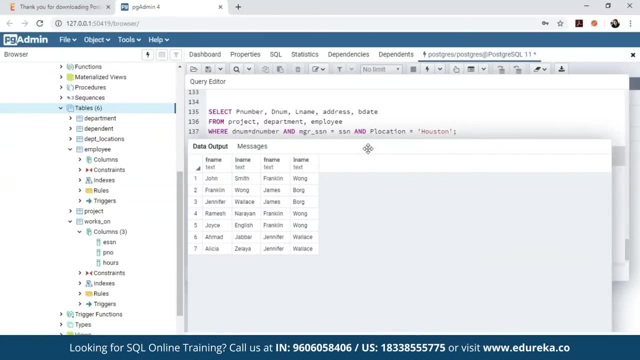 to s dot SSN. Now, if I just execute this particular query, you see an output that you know. we have the first name and the last names, We have the supervisors and the supervisors. So that's how, basically, you can play around with the names. 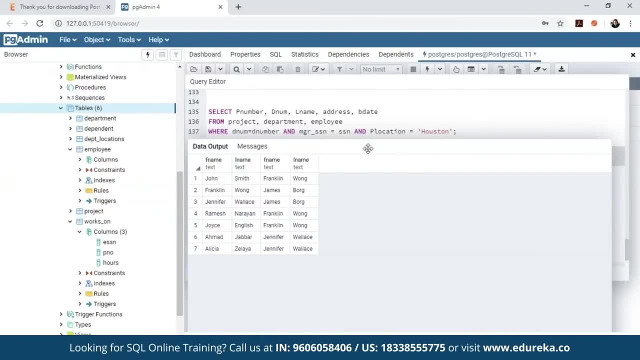 of the columns and the tables also, guys. So I hope you've understood this particular query. now moving forward, You might have heard about the term distinct, So when I say distinct, what I mean is I want to find out all the unique values, right? 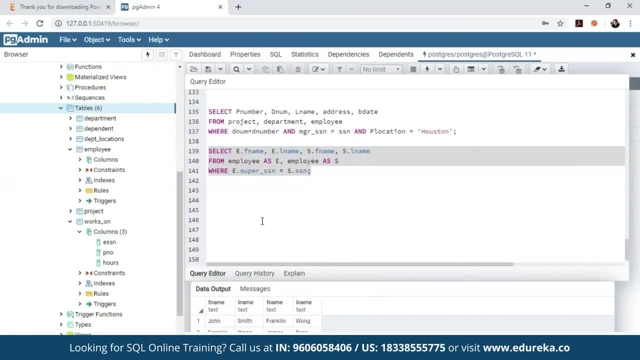 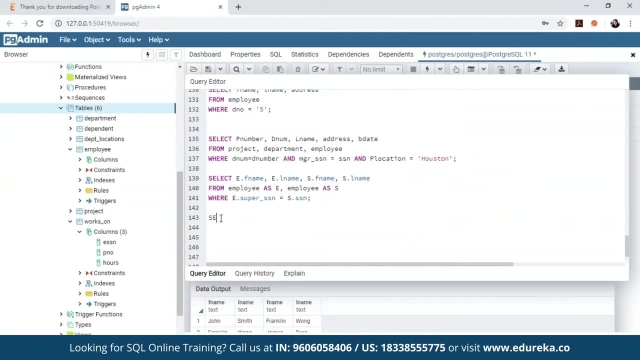 So to find out unique values you have to use the term distinct. Let's say, we want to find out the distinct salary values for all the employees, right? So now what I can do is I can just mention select distinct And then I choose the column salary from the employee table. 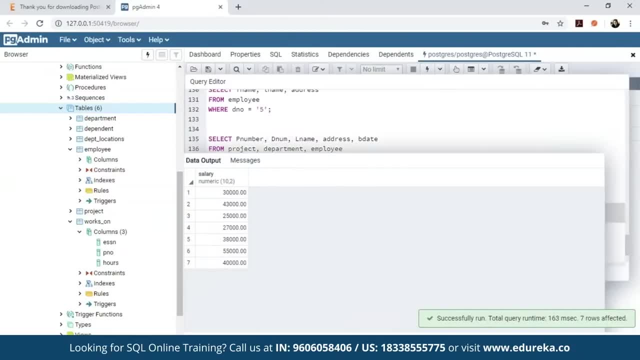 and then I click on execute So you'll automatically see that. you know we see all the distinct salary values present. So whenever you want to find out any unique values or, let's say, distinct values, This is basically the keyword that you have to use. 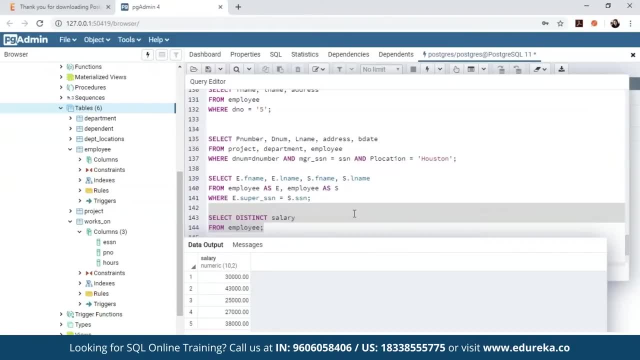 that is distinct. So, guys, that was about the distinct query. Now let's move forward and understand the cross product. now, cross product is something like, you know, when you have a into B, right? So basically, you have a and then you want to find. 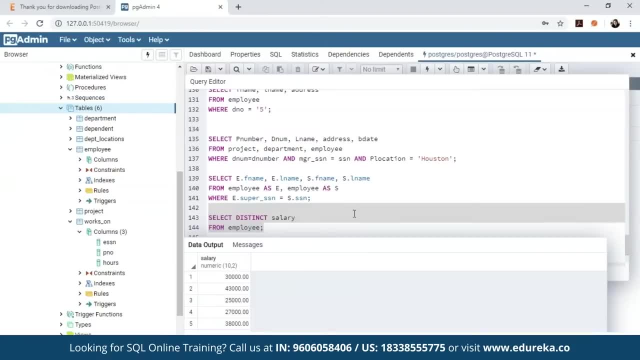 out all the combinations of a with B. That's when you use cross product, For example. let's say you know you want to find out all the SSNs, basically of all the assistance of the employee, and then you want to find out all the combinations. 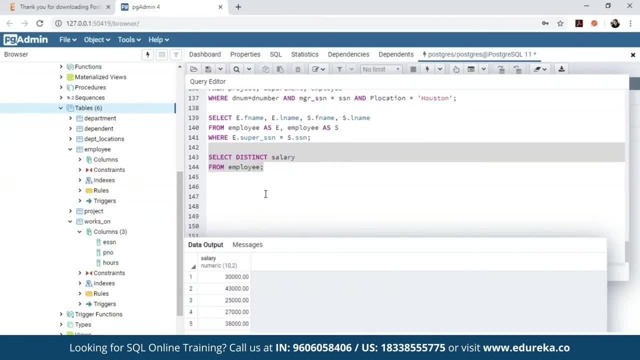 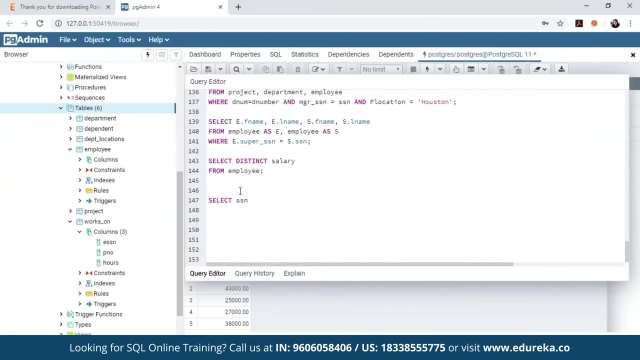 of employee assistance with the department name. So let's do that. So what we can simply do is to perform cross product. You can mention select SSN and the name from will mention employee and Department. So if I just execute this particular query, 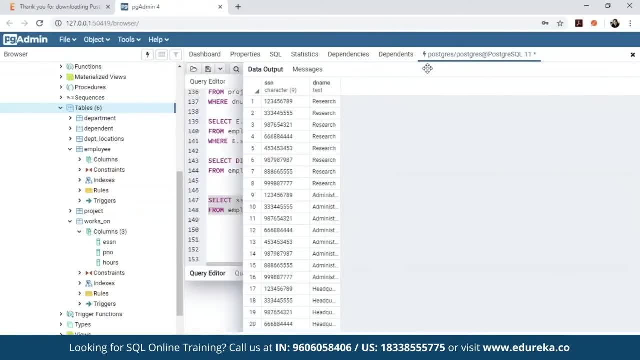 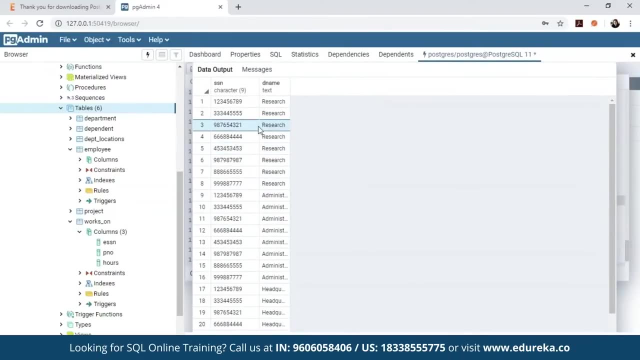 you'll see that. you know we get all the combinations of SSNs with department name, So let me just drag a little bit right. So, as you can see, we have for each SSN We have various departments, like you can see, we have the research department, the admin Department. 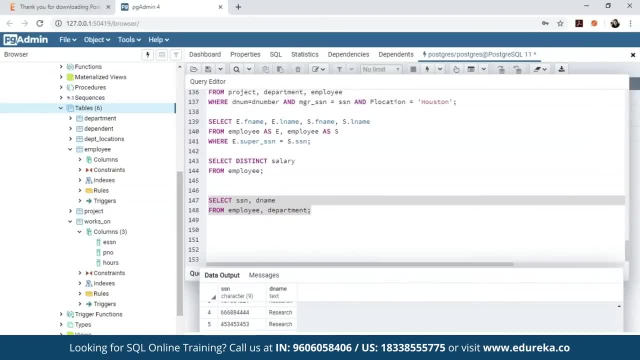 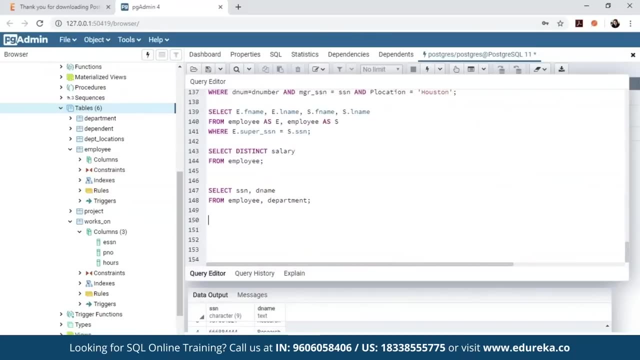 the headquarters Department and so on. So that's how, basically, you can perform cross product. Now let's say you know if you want to take this query further. so let's say you know we want to find out all the employees. 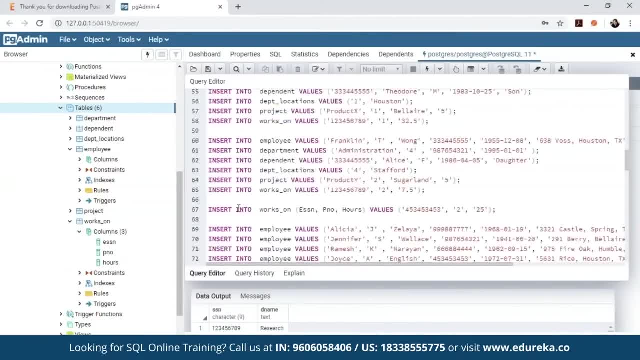 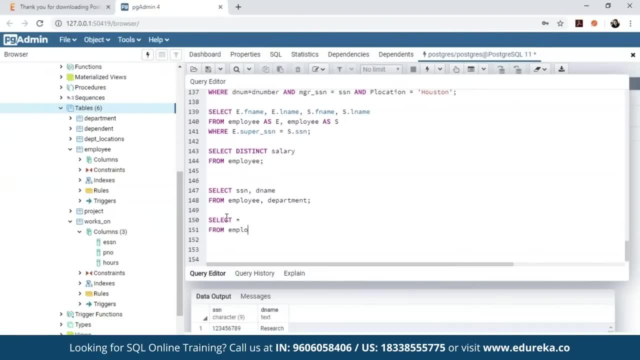 who work in the department, Let's say, administration. So what we can simply do is we'll type in select star and then I'll mention from employee Department, And then I'll mention a where condition which says the name is equal to administration And the number. 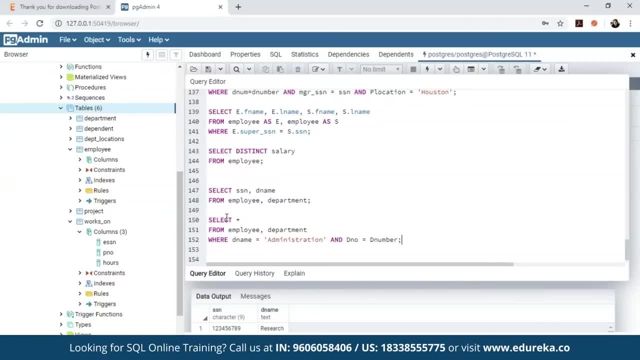 Is equal to the number from the department table. So if you have any queries with how am I mentioning the column names, you can always refer to the tables that you have, and then you can go back to the tables and check for the column names. 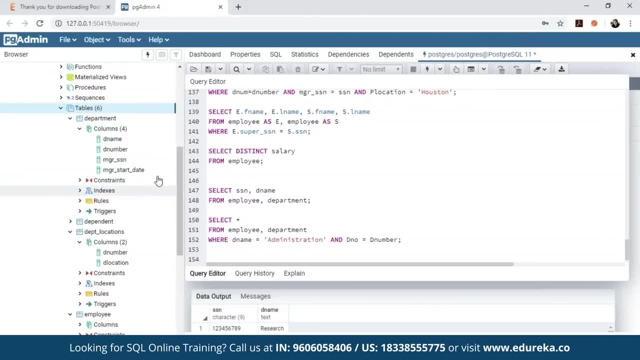 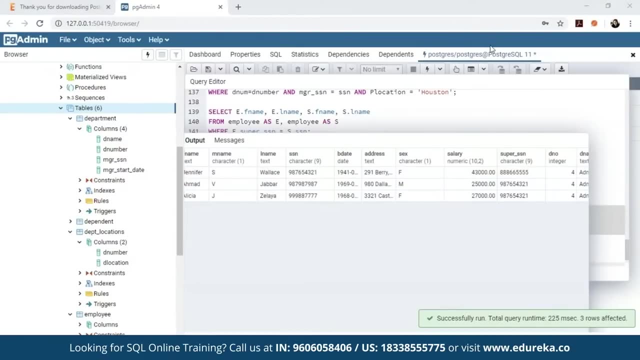 For example, let's say I go to the department, then you can see that you know I have the department number over here, So I just execute this particular query now. and once I execute this particular query, you see that you know we get all the details of all the employees. 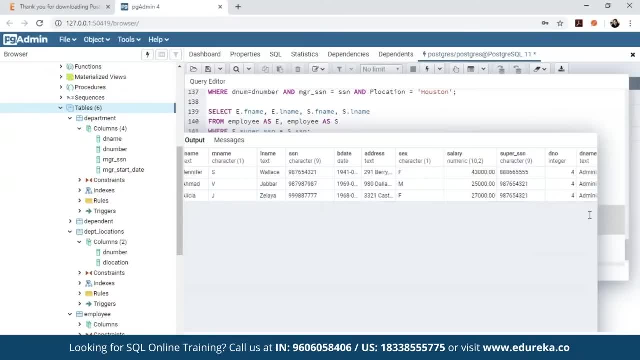 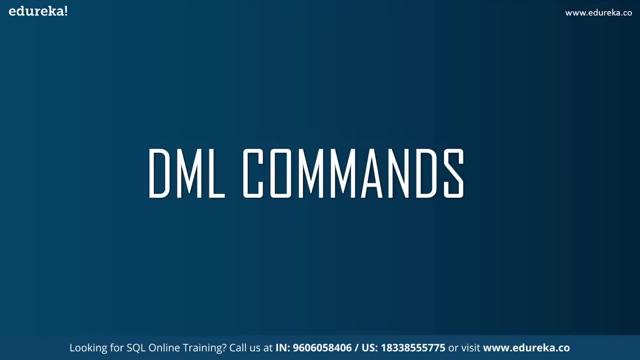 who work in the department administration, right? So if I just extend this, you'll clearly see the output, right? so, guys, that's how, basically, you can play around with the select statements. Now, before I move forward with the further data manipulation: language commands. 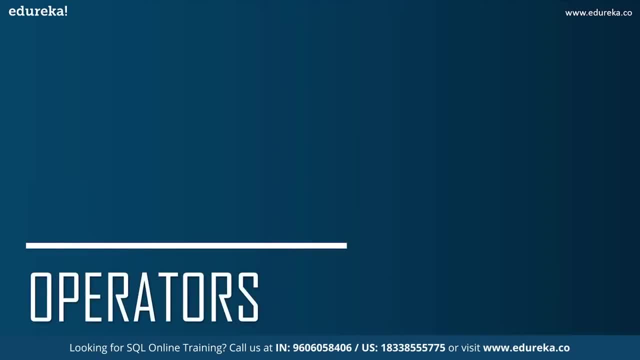 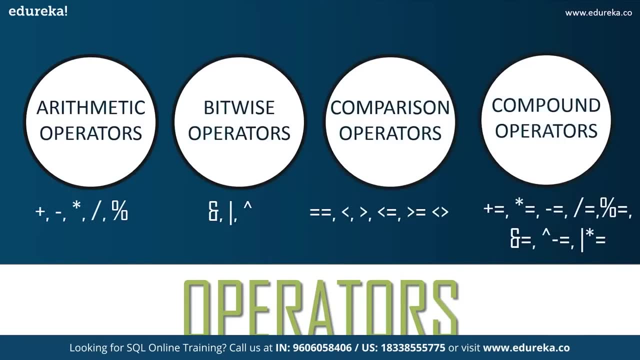 let's look into the next topic, that is, operators. Now there are various kinds of operators present in the sequel commands, that is, arithmetic operators, the bitwise operators, the comparison operators and the compound operators. So the arithmetic operators are basically used to perform the arithmetic operations. 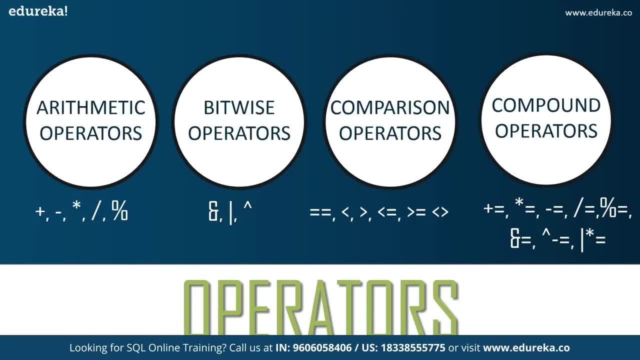 as you can see on my screen, It's plus, minus into divide and mod. bitwise has bitwise and orange or comparison has greater than less than greater than equal to, less than equal to and they're not equal to, and so on, and the compound operators have: 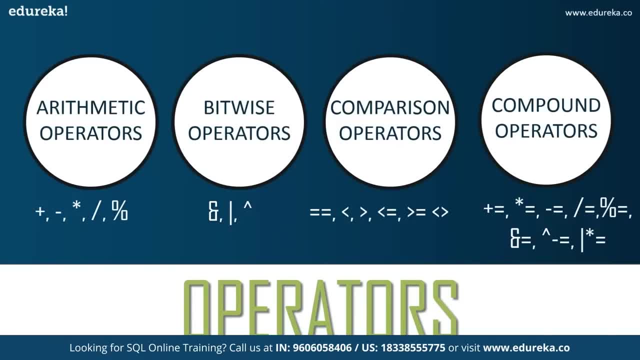 you know, increment, like you know, a is equal to a plus. one can be written as a plus equal to. so that's how, basically, you can use operators, guys. Well, I'm not going to explore more about operators, because that's a really simple topic. 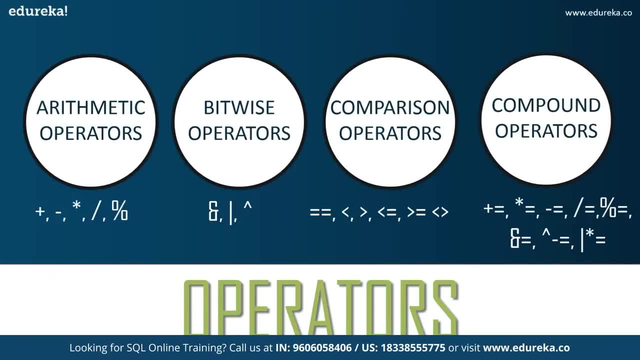 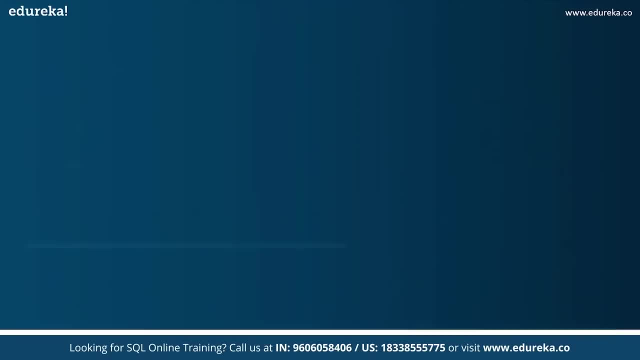 that you can explore about right. So I've just given you a basic understanding of the top operators. Well, don't worry, will be look forward into these particular operators later on in the session. So let's get started with our next topic for today's session. 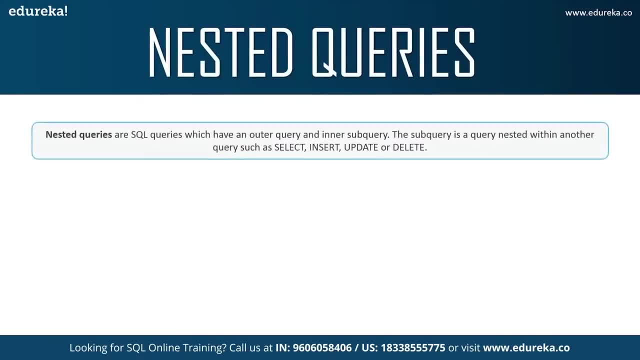 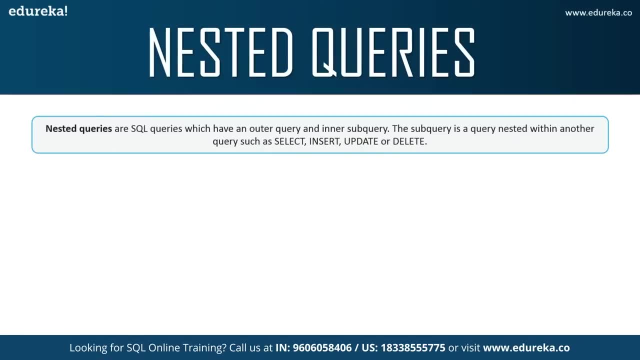 That is, nested queries. So nested queries are sequel queries, which have an outer query and an inner query. So the sub query is a query nested within another query, such as select, insert, update or delete. So, for example, if you see the screen, that is basically the outer query. 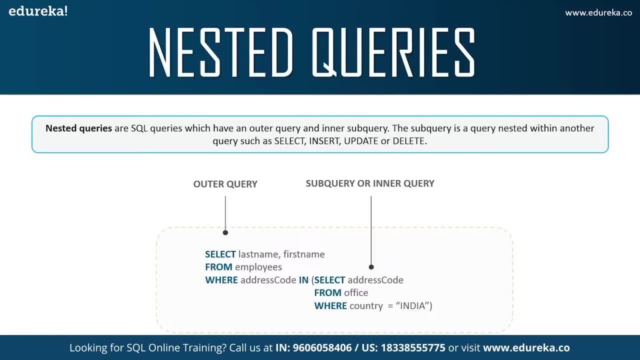 and the inner query. So I have an outer query which says select last name, first name from employees, Let's say nowhere address in, and then we choose. you know, we mention an inner query which says select address code from office where countries, India, right. 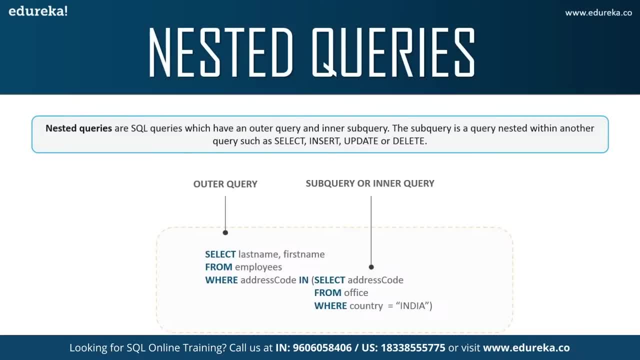 So base is so if the condition matches, then automatically this query will be executed and then we'll get the output. So this was about nested queries, guys. So now what I'll do is I'll now explain you a little bit more concepts and then I shift back to my PG admin. 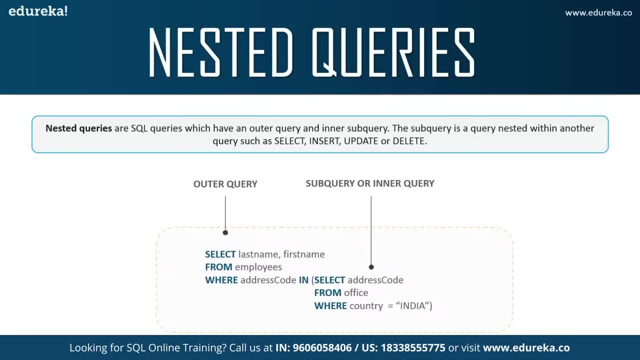 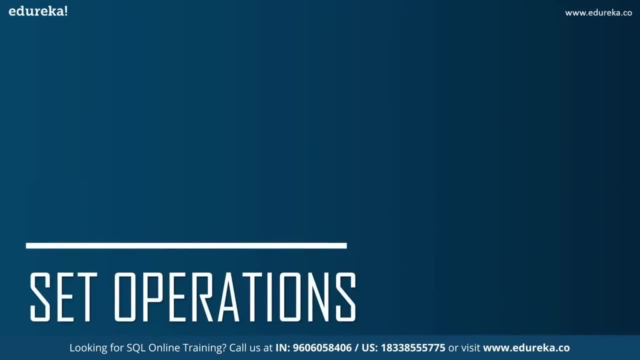 to show you how you can write nested queries and implement various other queries. So on that note. next let's look into what are set operations. Now, all of you might be knowing what are set operations, right? It's basically Union intersect and minus, for example. 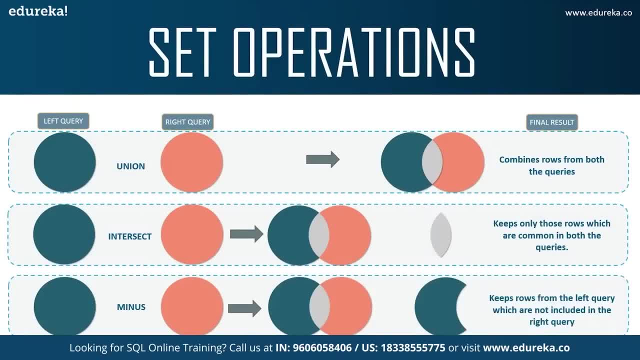 let's say you know you have set a and set B. Now, if you perform the Union operation between set A and set B, what you'll get is you'll basically get all the data present in both set A and set B coming to the intersect option. 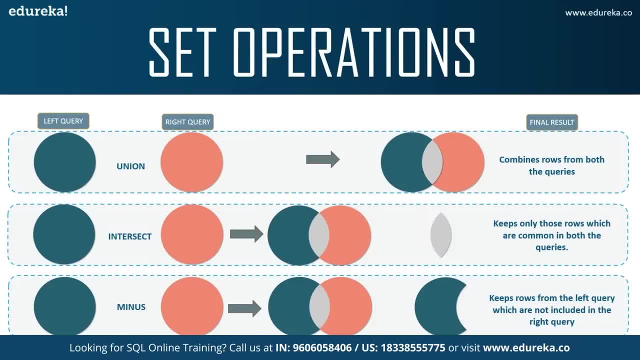 Basically, if you have set A and set B and then you feel perform the intersect operation between both these sets, what you'll get is only those rows which are common in both the queries. and finally, coming to minus status, You can basically mention minus or except right. 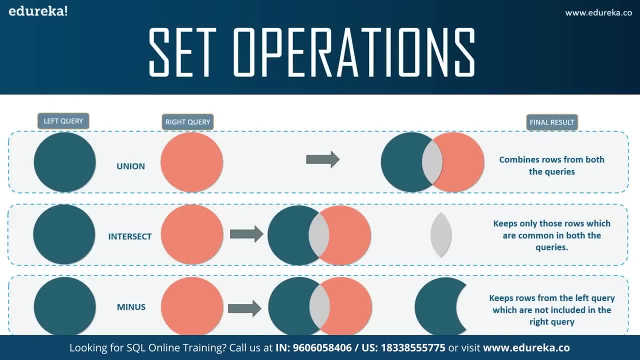 So, for example, let's say you have set A and set B, and then you mentioned set a minus set B. You basically keep all the rows from the left query which are not included in the right queries. Now the vice versa is also true. 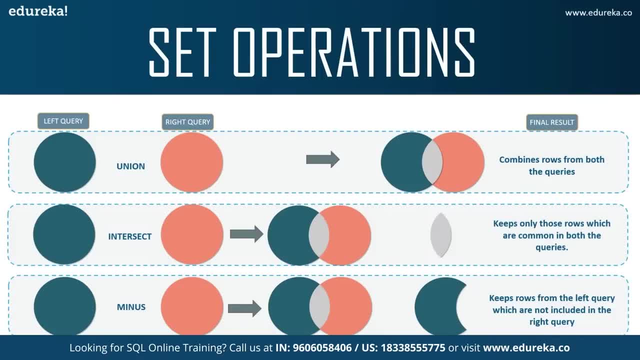 For example, if you do set B minus set A, then you keep all the queries from the right query which are not included in the left query. So that's how, basically, you can perform set operations, guys. So in the matter of database management systems, 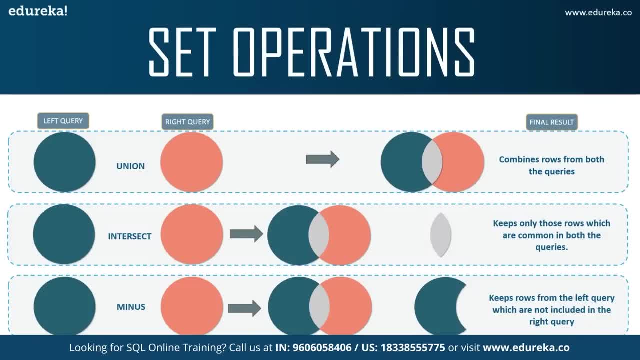 if you have to understand, then you can understand set A and set B as left query and right query. So, as you can see from the pictorial representation over here, if you do Union then you get all the rows from both the queries if you do intersect. 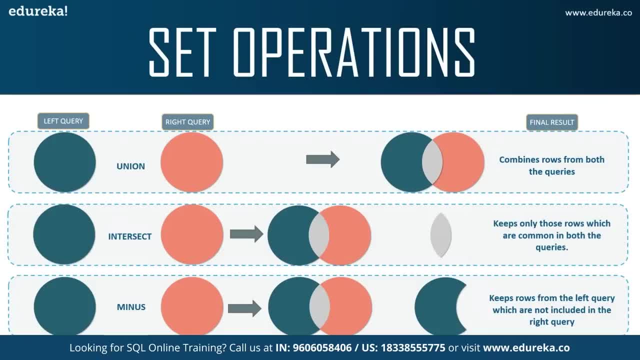 then you get only those rows which are common in both the queries and then, if you perform the minus operation or the except operation, you get only the rows from the left query which are not included in the right query, or maybe only those rows which are included in the right query. 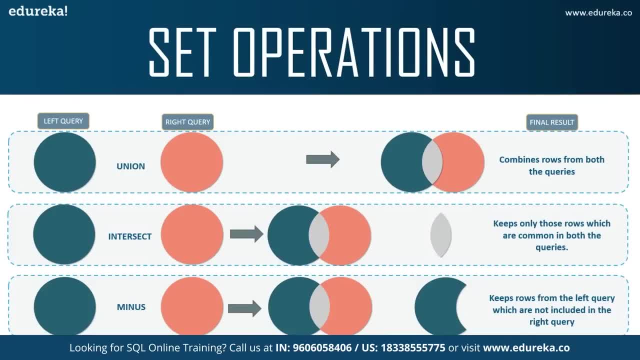 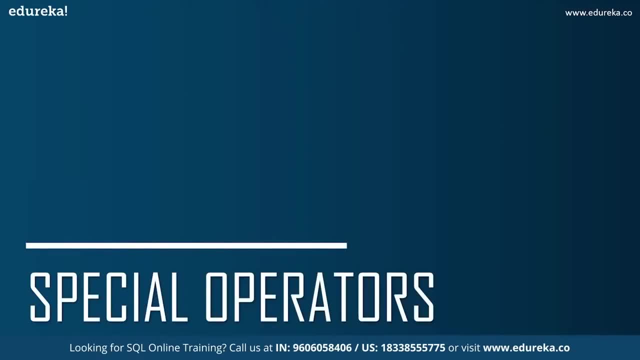 but maybe not included in the left query right. So, guys, that was about set operations. So now let's move forward and let's look into special operators. So when I say special operators, there's nothing much big deal about it, They're just few operators. 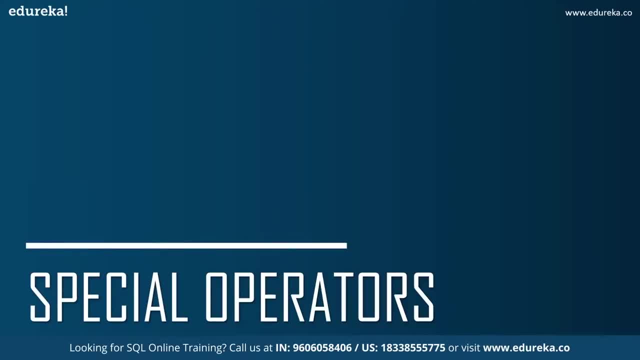 which are special, like you know. between is null, in exists all in any, so these are various operators. This is not something that you need to learn in depth. As you write queries, you should have an idea about all these operators. So when you say between operator, what I mean? 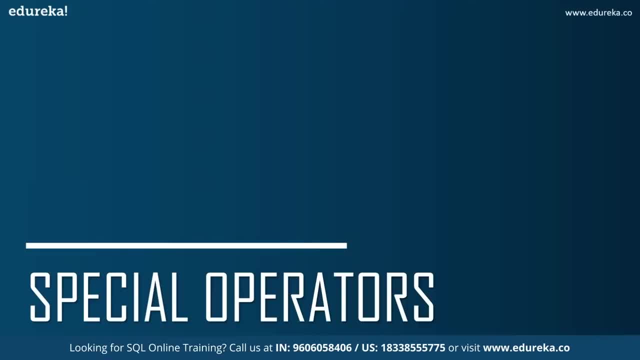 by between operator is basically that we want to mention a condition between A and B. So whatever values would satisfy the condition between A and B, all those values rows will be printed. similarly is null. So the is not operators basically used to test for the null values. now, since you know, 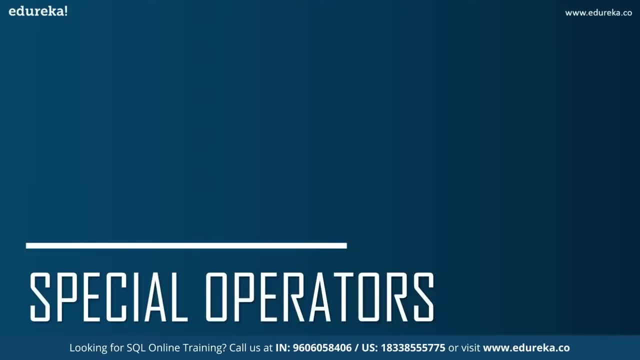 it is not possible to test the null values with comparison operators like greater than or less than we can simply use is null and is not null operators instead. So what you can simply do is you can just find out where if address is null, or maybe if the date of birth is null, and so on coming. 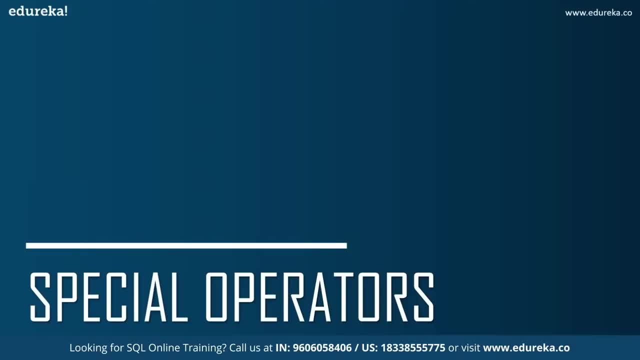 to like operator. the like operators basically used to get the date of all those values which either start with the character- specific character that you mentioned, or maybe end with a specific character that you mentioned. or it could also happen that you know you have few spaces and then you mention a specific character. 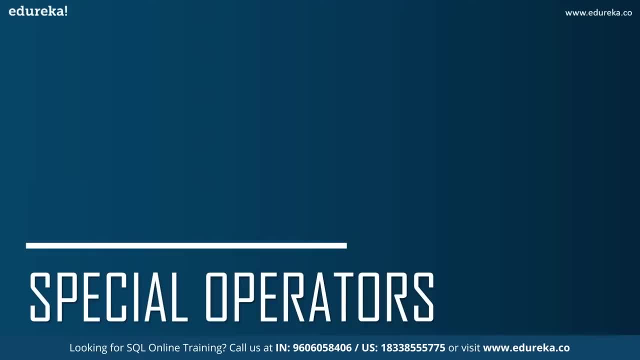 You also want all those rows coming to in operator. This is basically a shorthand operator for multiple or conditions which allows you to specify multiple values in where clause. so this is basically used when you want to use nested queries right coming to exist operator. exist operators basically used to test. 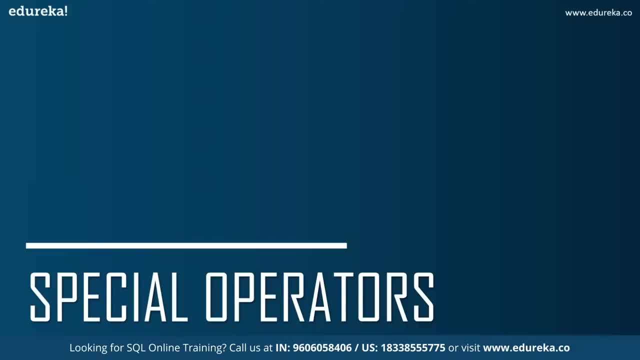 if a record exists or not. if it exists, it's fine. if it doesn't exist, then it returns an output that you know the query not found. and finally, coming to the all operator, the all operators used with the where or a having clause, and returns true. 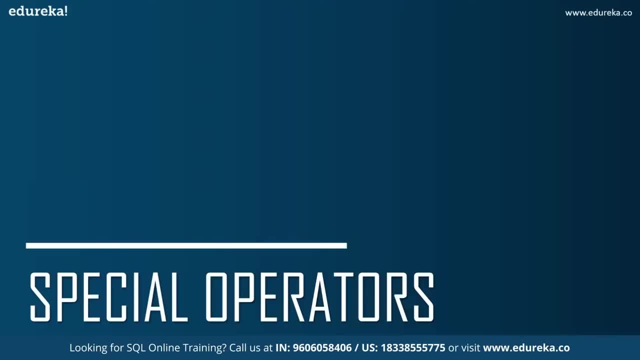 if all the sub query values meet the condition. So this was about all operator coming to any operator, The any operators you also use with the where and the having clauses and returns. true, if any of the sub query values meet the condition. apart from that over here, 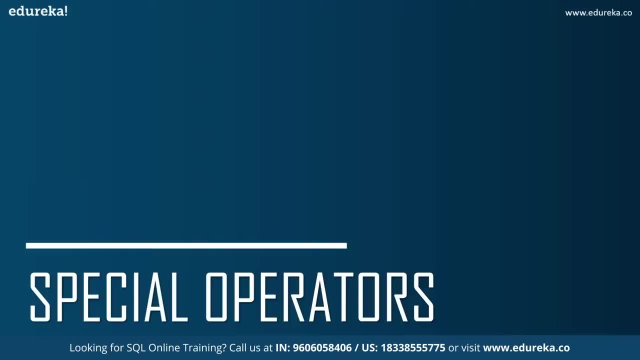 I also want to tell you about the order by, group by and the having process. So the order by is basically to order the data that you want in a specific format. Let's say, you know ascending order, descending order and so on. the group by is basically: you want to group. 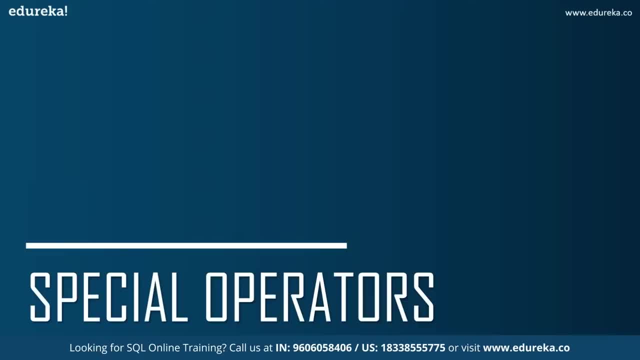 the data according to some specific column and so on. right and having is basically where you're checking. Let's say you know having salary greater than 25,000.. So only those tuples will be returned whose salary is greater than 25,000. 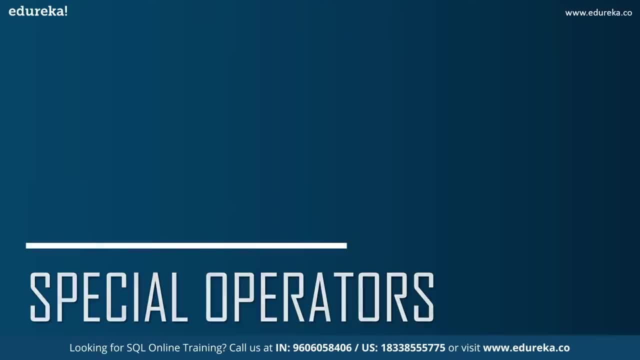 So, guys, that was about group by, order by, and having clauses also. Now let's move forward with the next one, that is aggregate functions. So aggregate functions is also one of the most simple topics. So aggregate functions is mainly used with the nested queries. 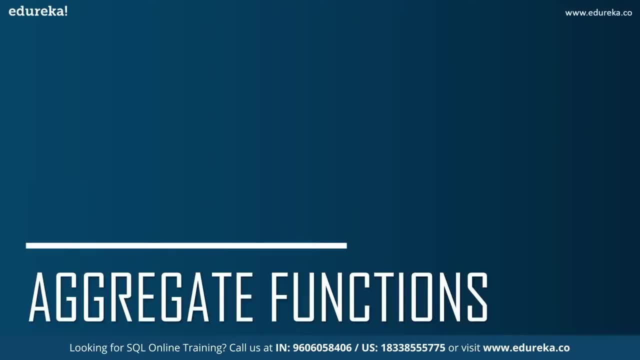 that is basically the main: Max, the count average and some so. the min function is basically used to return the smallest value of the selected column in the table. The Max function is basically used to return the largest value of the selected column in a table. The count function is basically used to count the number. 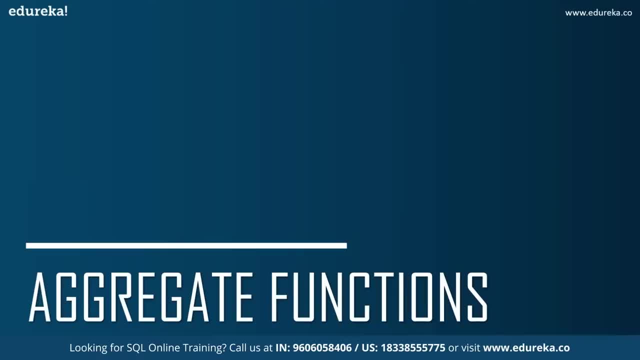 of rows that match a specified criteria. The average function returns the average value of a numeric column that you choose and the sum function returns the total sum of a numeric column that you choose. now, that was about aggregate functions, guys, So don't worry, I'm just brushing you with the topics, basically the concepts. 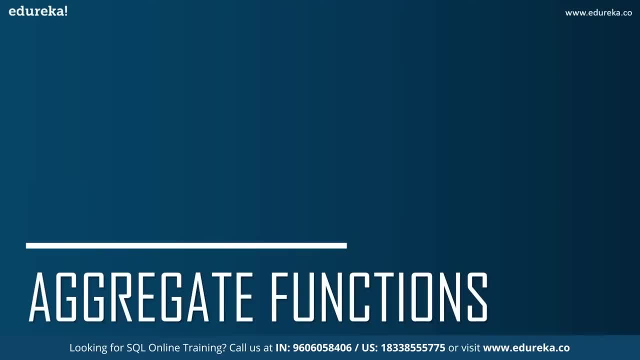 I'm going to show you how you can use all these concepts based on the queries that I'll execute on the PG admin in a while now, but before that let me just take you through the limit, offset and fetch values. So the limit is basically used to limit the number of data. 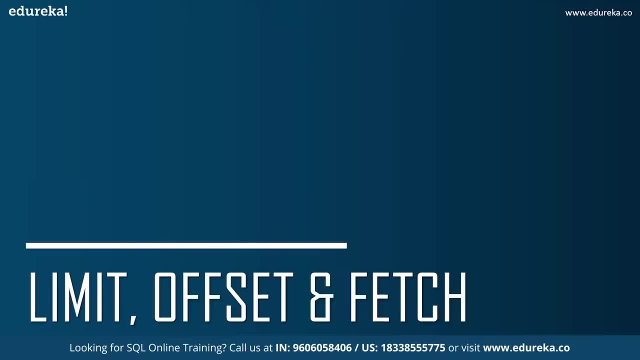 that you want to get now. We want only the data of the first fire hose. So what we'll do is we'll basically mention select star from employee limit 5.. What will happen is automatically will see the first fight up coming to offset. offset is used. 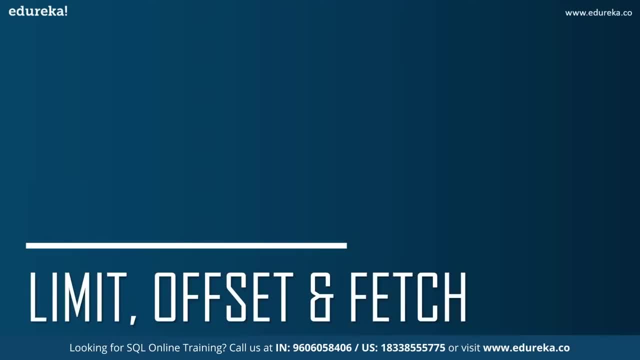 to basically select a specific number of rows after the limit, right. For example, let's say, after the fifth row, we want three rows, right? So what we'll do is we'll use the offset statement to basically mention that, you know, after the fifth row. 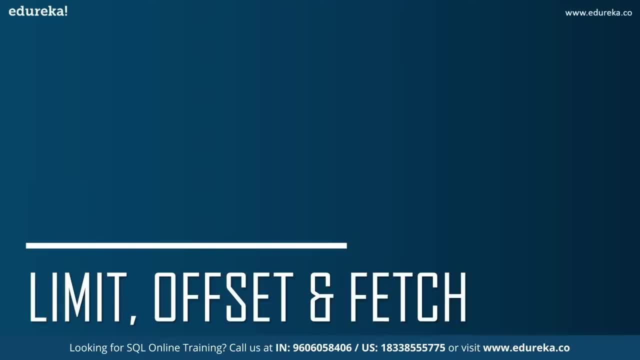 we want three rows, right? So basically, only after the fifth couple is read, automatically 678 will be printed out as an output. coming to fetch: fetch is also one of the ways to limiting the query results, right? So whenever you want to fetch. 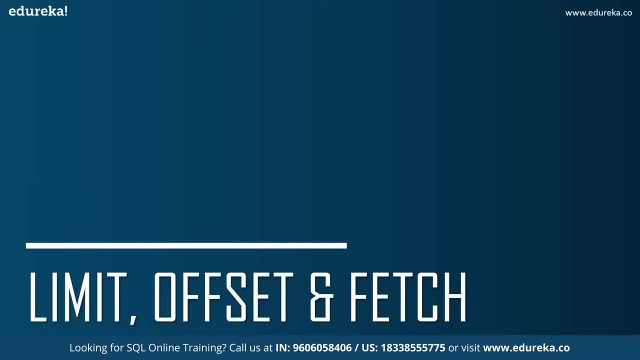 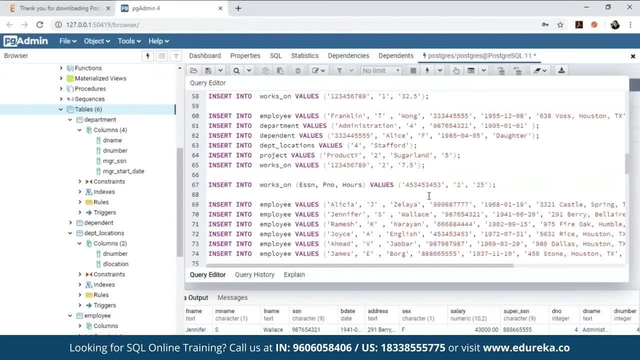 let's say first five rows only, or maybe let's say 10 rows only. then you can use the fetch statement. So I'm going to show you how that's done. Let me just shift back to my PG admin, And now what I'll do is I'll start with the first topic. 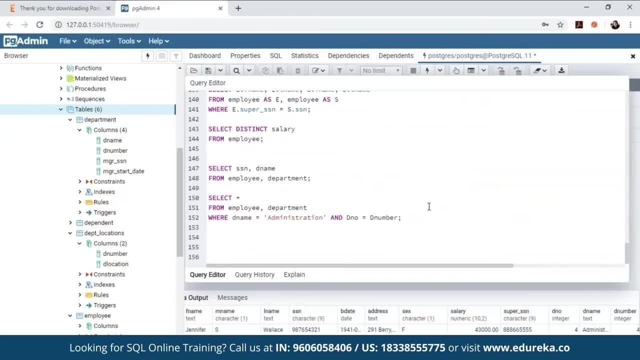 that I had discussed over here, that is, nested queries. So let's write some interesting nested queries so that you get a hands-on experience on how you can integrate into a complex queries right. So, for example, let's say: you know, we want to make a list of all the project numbers. 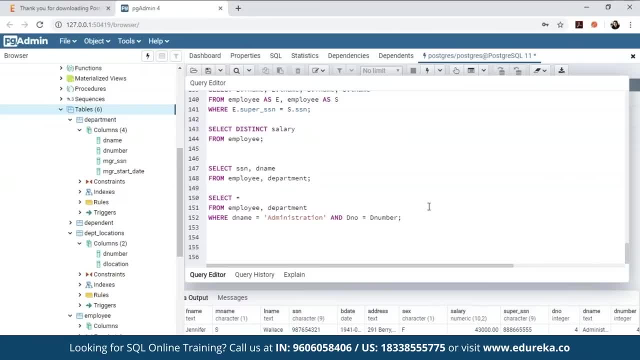 for projects that involve an employee whose last name is Smith, either as a worker or as a manager of the department that controls the project. So our main question is basically to list the project numbers for projects that involves the employee Smith. now that particular employee can either be the manager- 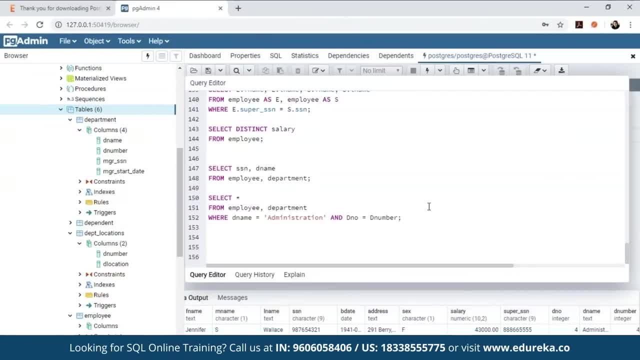 or can also be the worker of that particular department and controls a project. So to do that, what I'll do is I'll have to write a nested query. So the reason for nested query is simple. That is because you know we have to first find out all the projects where you know. 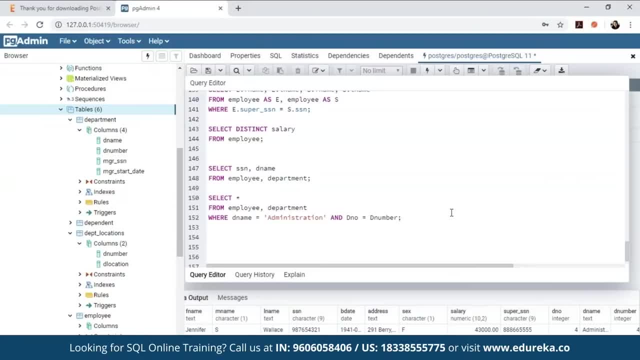 Smith is working as an employee. later on We'll find out the projects where Smith is working as a manager, right? So let's start with Smith working as a manager. So for that, what we'll do is we'll type in select this thing. 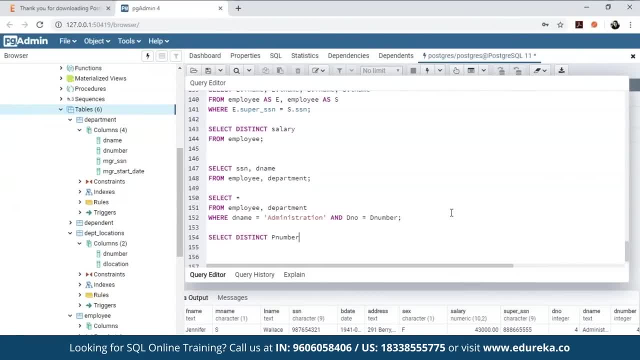 because we want unique records and let's say P number, that is basically the project number from project. and then we also want the department, because we're going to use a department table. and then we mentioned employee, because we're going to use the last name where we'll mention the num is equal to the number. 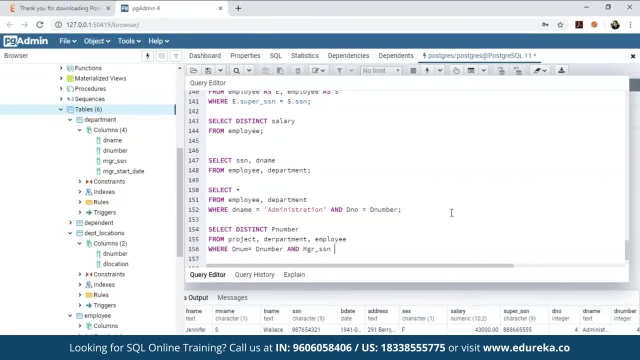 and MGR SSN is equal to SSN. Also, my last name should be Smith, right? So I'll mention: last name is equal to right. So let me just remove this, put in over here and let me put a bracket. now Let me tell you one thing over here. 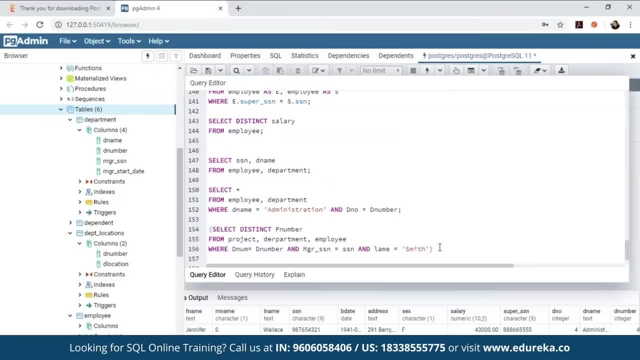 This is not the end to the query, because we also want to find out all the project numbers where employee Smith is working as a worker, right. So for that what we'll do is we'll use the set operation Union, right, Because this makes sense. 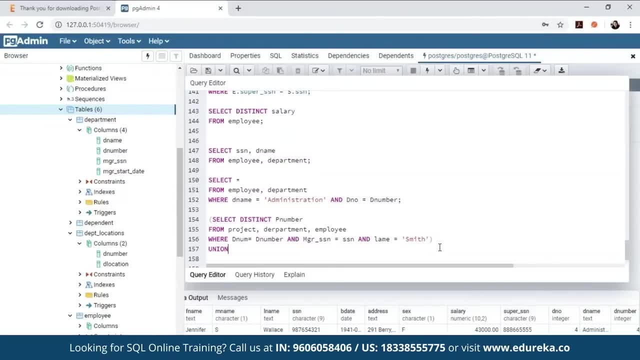 right, We want all the values from set a and then we also want all the values from set B. So that is the reason we'll use the Union operation and then we'll mention select distinct P number from project works on employee where P number is equal to P. 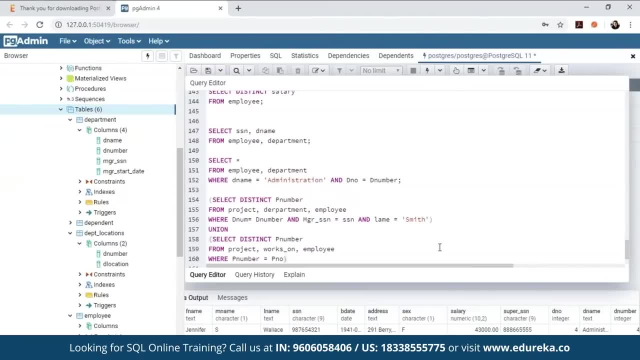 Number. that is basically the project number from the project table and the works on table and employee SSN from the works on table to SSN from the employee table. apart from that, We also have to mention that last name should be Smith, right? So we'll mention and L name is equal to Smith. 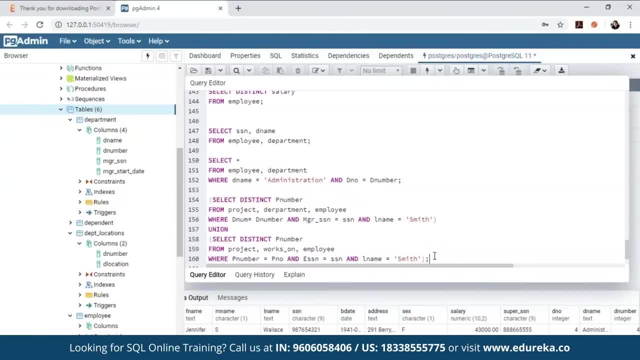 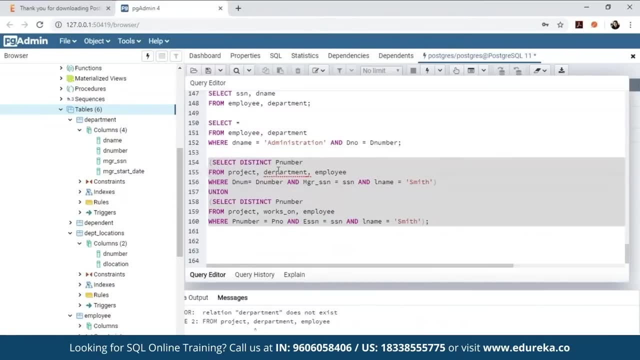 Right, So I'll end it with a semicolon and let me just remove this type over here, And then let's execute this particular query. All right, it says Department. Oh yes, There's a spelling mistake over here, right. 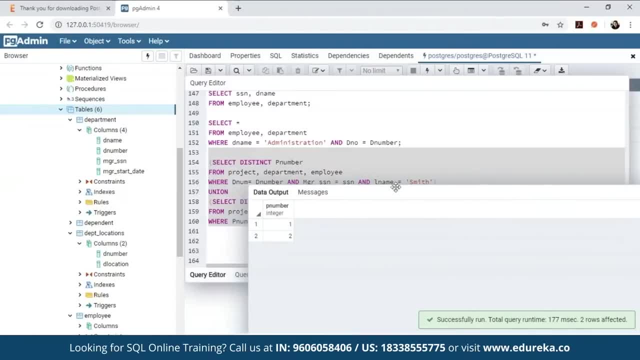 And now let's execute again. So once I execute, you see that you know I get the project number one to. that means that you know the person with the last name, Smith, works as a manager or maybe works as a worker in these two projects. 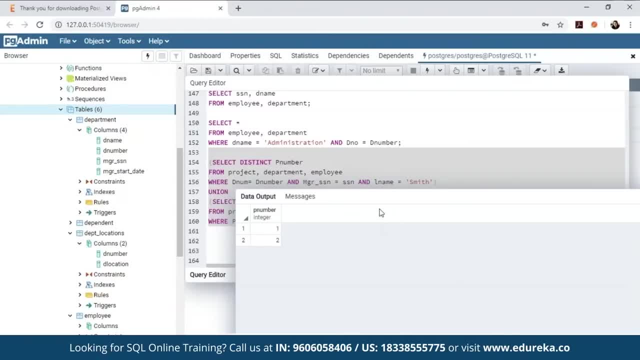 that is project number one and two. So, guys, this was a nested query with the Union operation. Now let's say you know you don't want to use any set operations and let's say you just want to write a simple query. 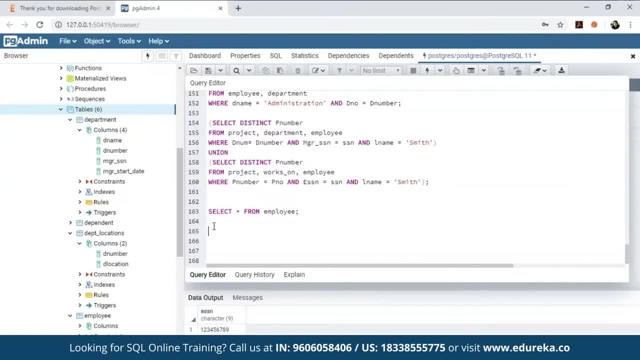 Let's take an example for them. Now let's say: you know you want to retrieve the name of employees who have no dependents, right? So we had a relationship with this. employees have dependents, right? So let's say: 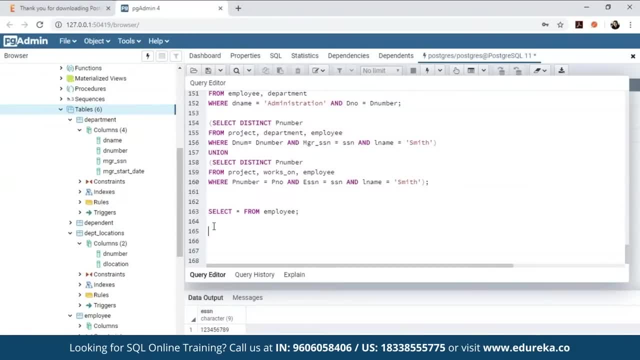 you know we want the name of employees who have no dependents. So for that what you can do is you can just type in the query: select first name. Let's say we take first name and let's say we take last name from employee. 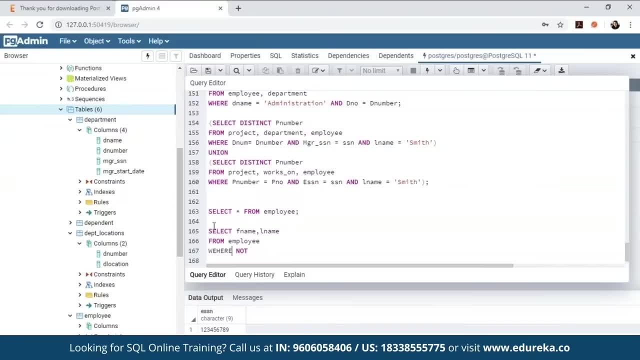 Well, will mention not. I'm sorry I have to correct the spelling of where. over here We'll mention not exist. and then I'll again mention a subway which say it select star from dependent, where we have to match the SSN right. So SSN is equal to ESS, it right? 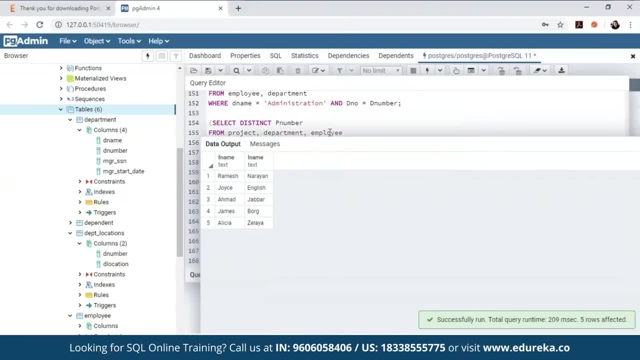 So I'll just execute this particular query and then, once we execute this particular query, you'll see an output of all those employees who have no dependents. So that's how, guys, basically you can use this operator of not exist. What I've done is: 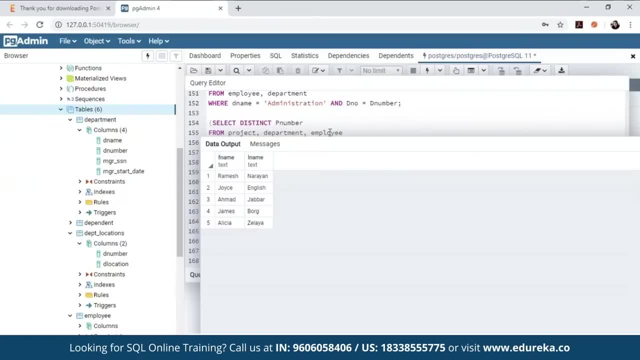 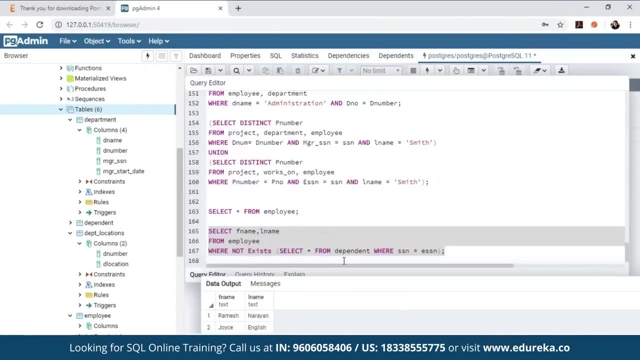 I have basically taken the operator of exists. So, if it exists, what will happen is that, initially, the sub query will be executed with, say, select star from dependent where SSN is equal to ESS, and so this query will generate all those results which have the dependents. 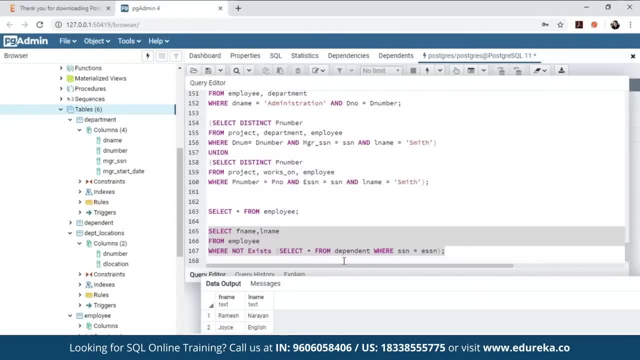 right. So basically all those employees who have dependents, that particular result will be generated over here. Then I put a not condition before that. So when I put a not condition the output gets reverse and automatically I got it output printed. So if you just mention, exists over here. 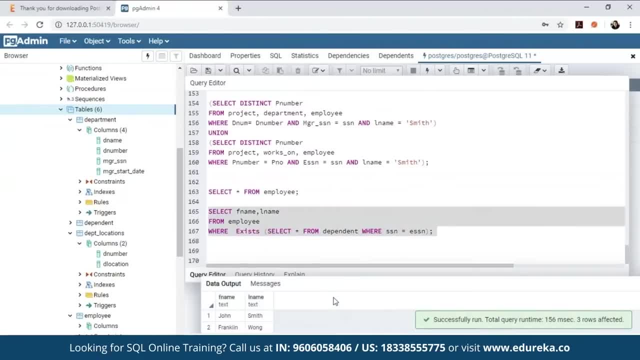 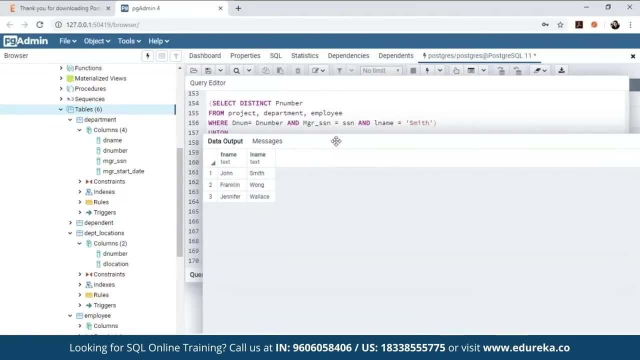 and then, if you remove not, and then again, if you just execute this particular statement, you'll see a different output. So this is basically the output of all the employees who have dependents. So now let's take this query further and let's say we want to find out the names of those managers. 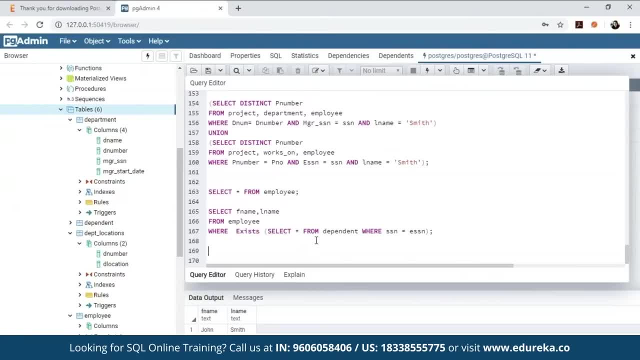 who have at least one dependent. So what I'll mention over here is I'll mention: select first name, last name from employee, where exists, and then I'll change this condition: select star from dependent where SSN is equal to ESS in, and also I have 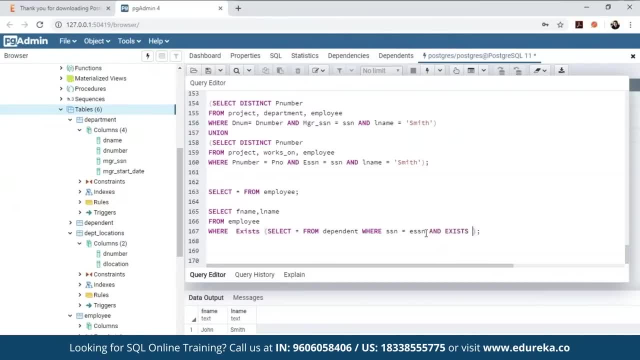 to take this condition further, which says: and exists. and then I again have a nested sub query which says: select star from Department, because we are considering manager right where SSN is equal to MGR SSN. So I'll just close this bracket over here and then I'll remove one bracket at the end. 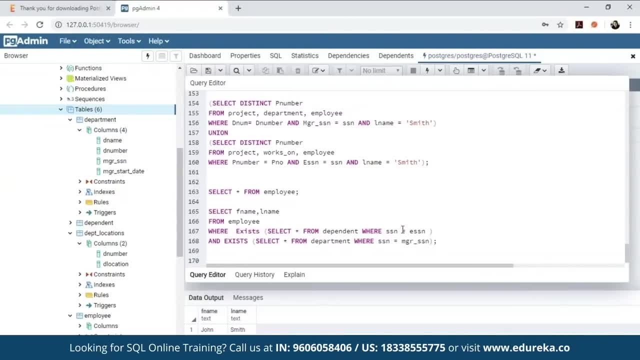 and let me put an enter So that's clear to you. So what I'm basically doing it: I'm basically listing the name of managers who have at least one dependent. So for that, what I've done is I've used an auto query. 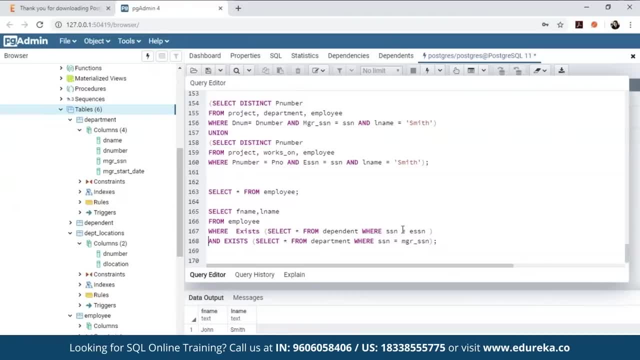 which has a sub query and underneath that I again have another sub query. So for that what I'm using is select first name, last name from employee, where exists, and then again I have a sub query which says: select star from dependent where you know SSN. 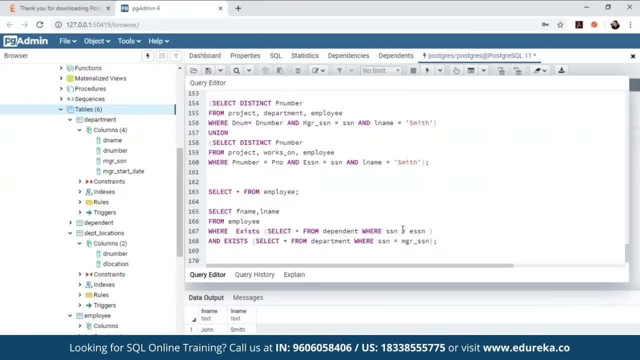 is equal to ESS. this will basically give the output of all the employees who have dependents. now. after that, we also have to match from select star, from Department Where SSN is equal to MGR SSN, which is basically the name of managers that we want after. 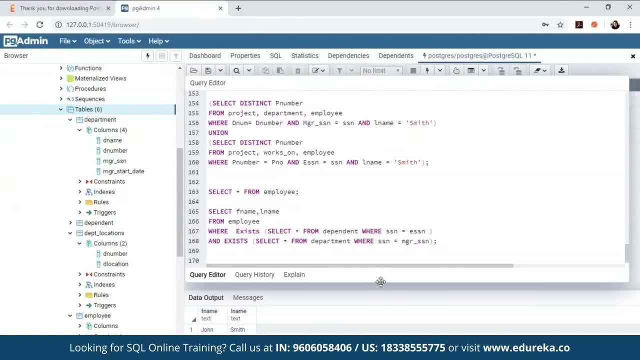 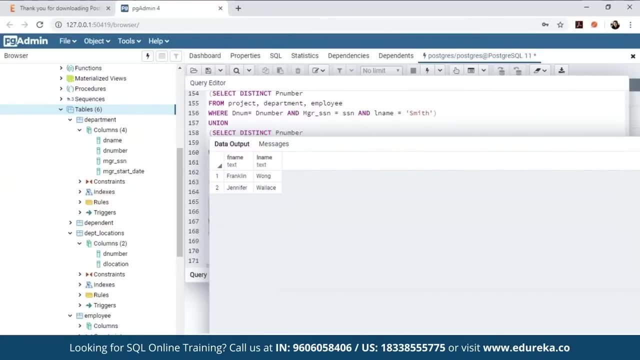 that we're taking dependents into account and then we are returning the first name of the last name. So, if you see the output, we get Franklin and Jennifer right. So Franklin and Jennifer are those managers who at least have one dependent. so, guys, that was about exists. 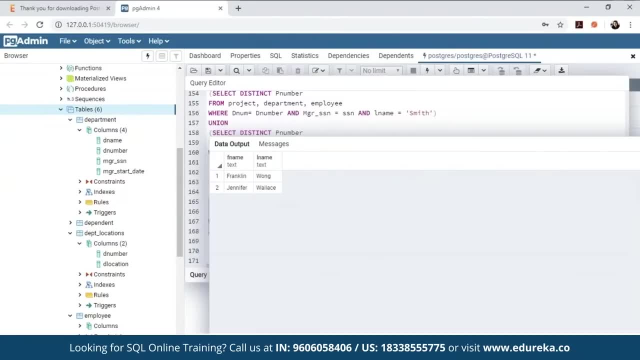 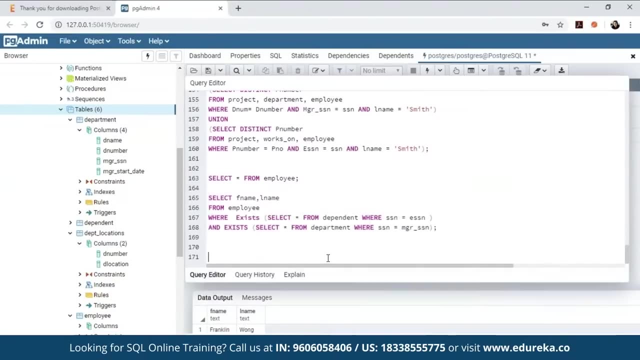 and not exists how you can use and all. now let's move a little bit further and, as I was talking about operators, like the special operators, let's look into few queries related to that. So let me just press on, enter over here So that I can make the screen clear for you. 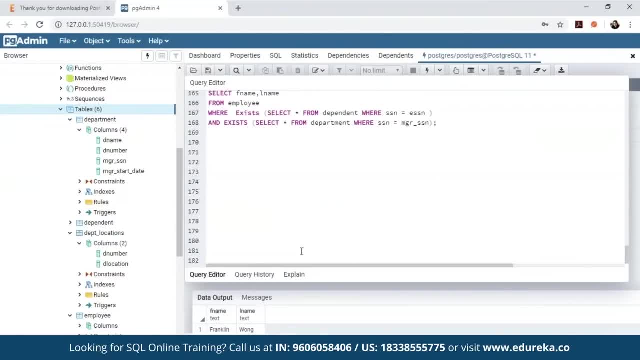 Now let's say over here, We want to retrieve all the employees whose addresses in Houston, Texas. So it's really simple. What I can do is I can just generate select SSN and first name from employee Where address like, and then in quotes: 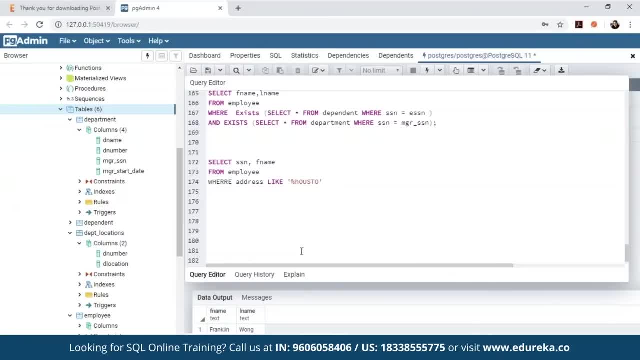 and mention percentage Houston And percentage sorry, and then what I'll do is I'll end with a semicolon over here. So I'm basically I'm generating the SSN and the first name of all the employees whose address is in Houston, Texas, right? 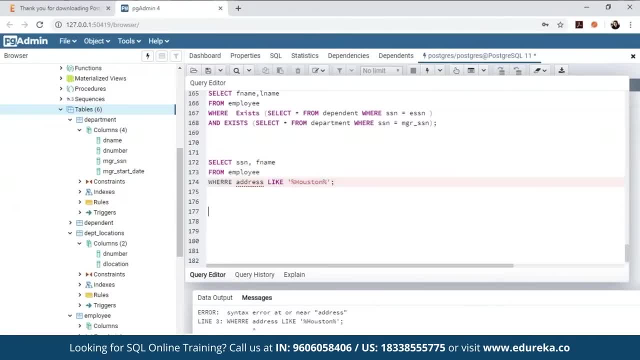 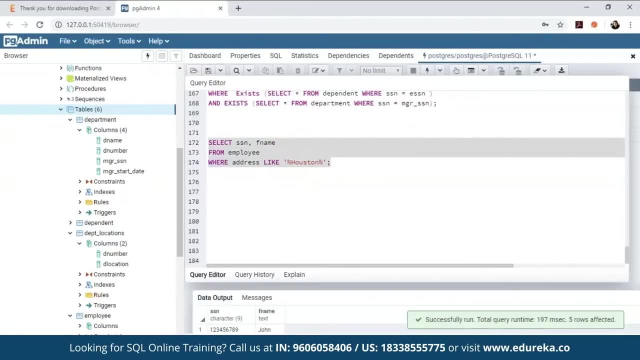 So let me just execute it. So once I execute, you see an error that you know where address. Okay, so that is basically because our spelling is incorrect over here, So let me just execute again. So once I execute, you see SSN and first name. 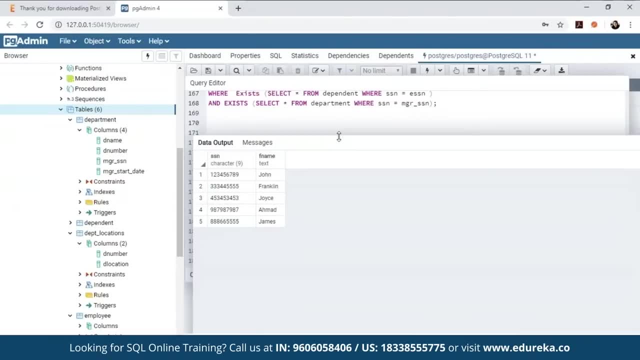 of all those employees whose address is in Houston, Texas, right? So if I want to check this information, you can go back to our employee table and then you can check the information for sure. So that's basically how you can use the like operator. 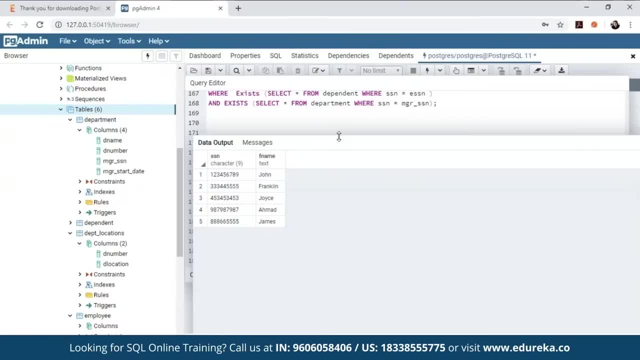 Now, let's say, you know, we want to find out all those employees whose first name, as, let's say, five characters. So if you want to mention five characters, how will you do that? Any five characters? not necessarily that you know. 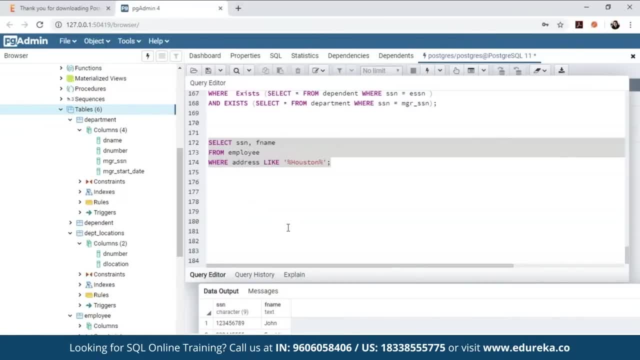 it has to start with F or S or a or any other character. It can be any character that you wish to write. So in that scenario let's just generate, select first name. and let's say: I again generate SSN from employee where first name like: okay. 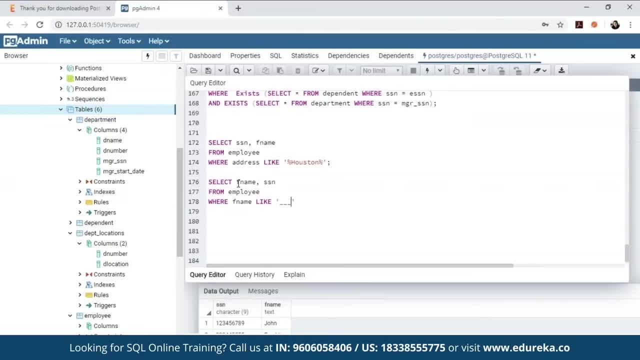 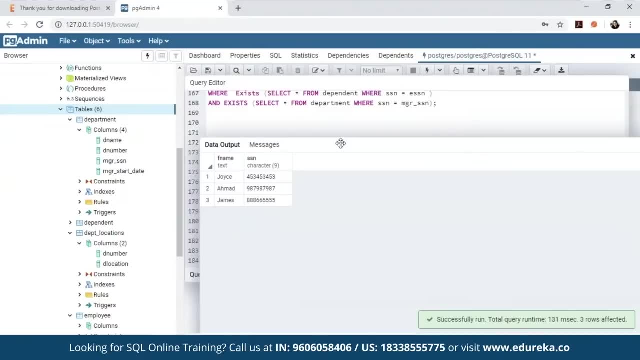 there's a typo over here, and then I'll mention five characters, right, and then I'll end with a semicolon. So let's just execute this particular query and you'll see that you know, it's just Joyce, Emmett and James who have first name, with five characters. 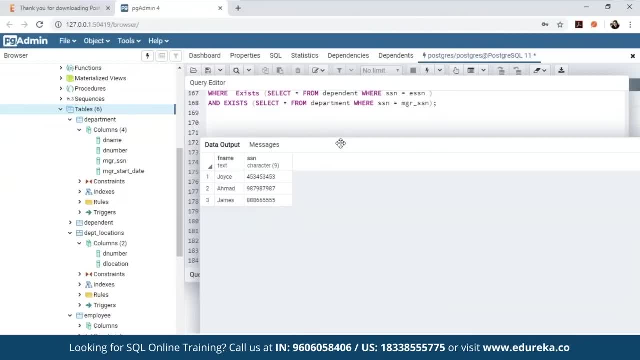 So all the other employees who have first name with any other number of characters are not taken into account. So that's how, basically, you can use the like operator guys. now let's say you know you want to use the between operator, for example. 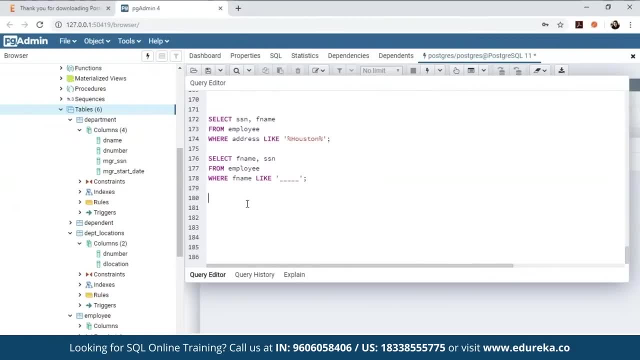 let's say that we want to find out all those employees who salary lights between, let's say, 30,000 to 45,000.. So for that I'll type in the statement: select star from employee where. and then you mentioned the nested query salary between. 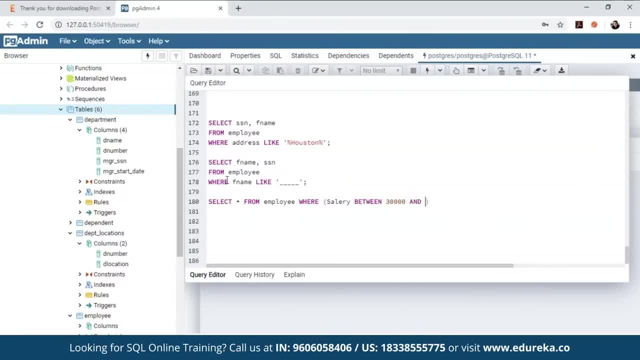 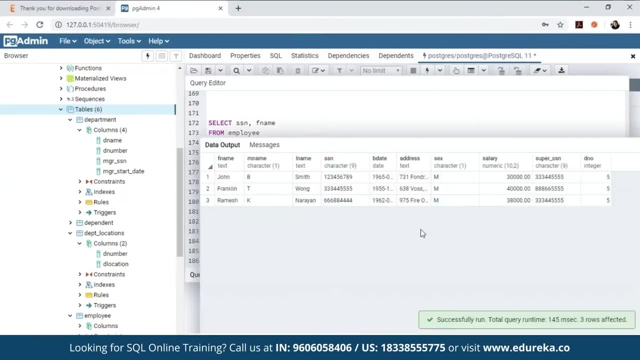 and then you mentioned 30,000 right And 40,000 right, and so let me just execute this particular query. All right, Once I execute this particular query, you get the information of all those employees who salary lies between 30,000 to 40,000.. 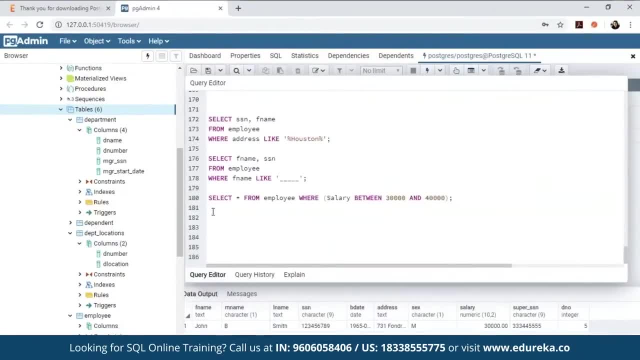 So, guys, that's how you can use the between operator. now, as I'm talking about operators, Let me just show you a simple functionality of the arithmetic operator. Also, let's say, you know, we want to show the resulting salaries of each. 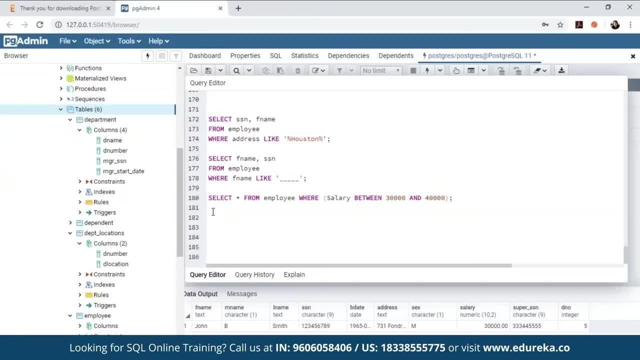 and every employee working on the product Y project. and let's say you know it's given a 20% raise. So to do that, what you can do is you can write a query. Let's say select E dot F name. So if you remember, I use the similar query previously also. 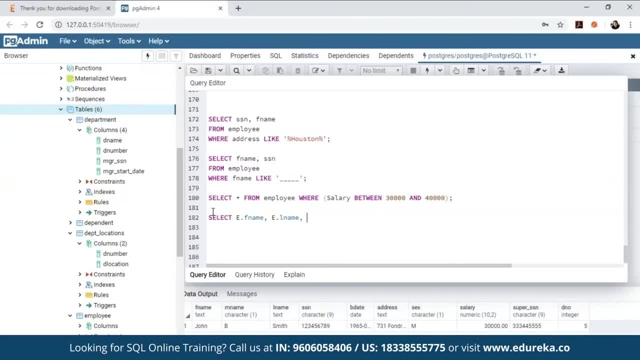 and then I choose E dot L name and then I mentioned 1.2. right into that is basically my arithmetic operator that I'm using and I'm choosing E dot salary as as, let's say, increased salary From I'm choosing employee table Because salary is an employee table. 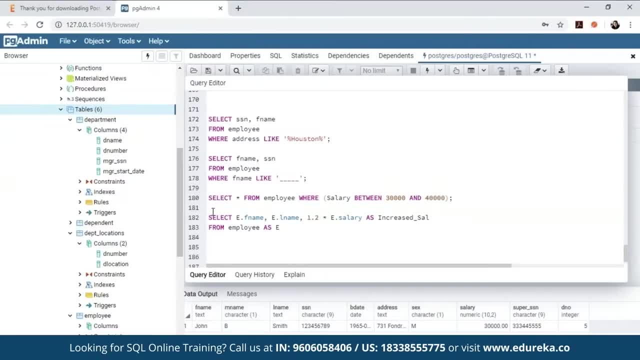 and then, since I'm using E dot F name, I'll mention employee as E and then works on W and project as P and further. what I'll do is I'll mention where employee dot SSN is equal to is equal to the works dot SSN. 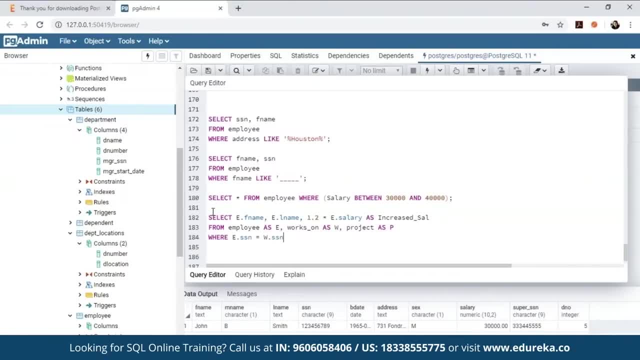 right. So whatever employees working on product Y right. So that's what we want to find out over here. So he has to first satisfy the condition of the SSN's have to match. apart from that, We'll consider and all right. 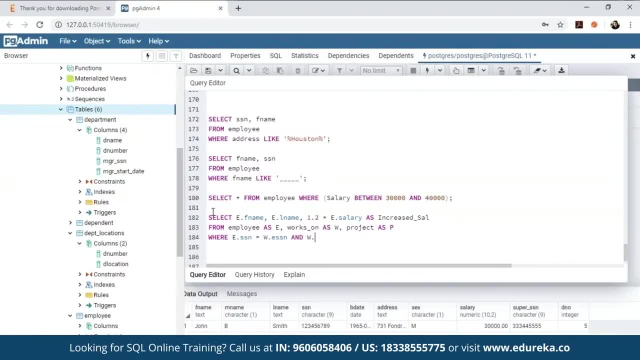 This has to be ESSN, right. and then I'll mention work dot P number is equal to P dot P number and P dot P name is equal to product Y. So let me just end this particular query over here and now executed. once I execute, you'll see that 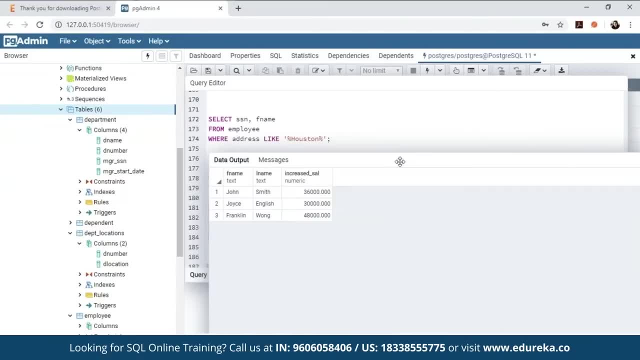 you know, we get the first name and the last name and the increased salaries of all those employees who have worked on product Y and the salaries increased by 20%. so that's how, guys, basically you can use the as operator and also arithmetic operators together. now. 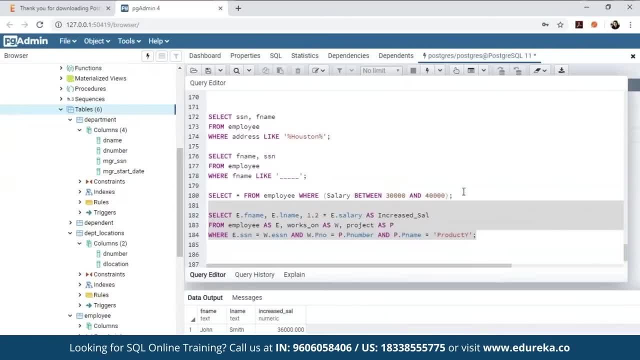 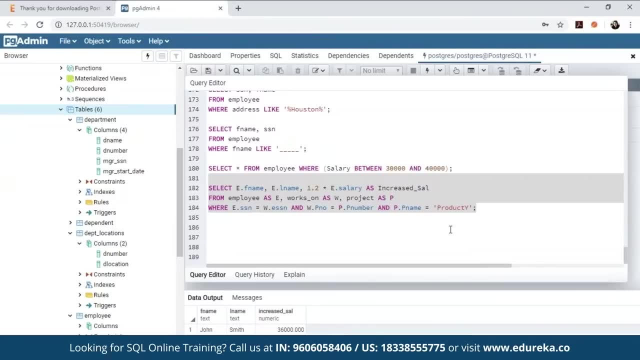 as I was talking about one more operator, that is is done. So if I have to talk about is now. let's say, you know we want to find out all those employees who do not have any supervisor, So then directly you will use is null operator. 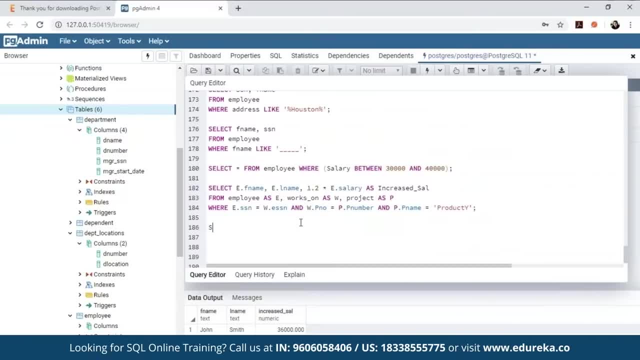 So in that scenarios, what you'll basically do is you'll write a query, like you know, select, let's say, star, from employee where super SSN is null. I'm basically using this is null operator to find out all those employees who do not have any supervisors. 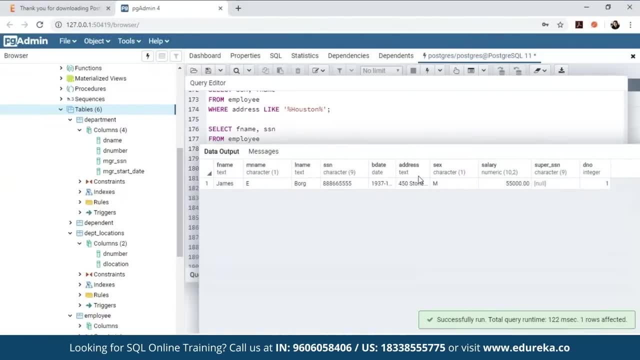 So I'll just execute this and then, once I execute this, you get the details of that particular employee who doesn't have a supervisor. So, guys, that was about operators and all. I won't go into each and every operator Now. I'm leaving the rest to you so that you practice. 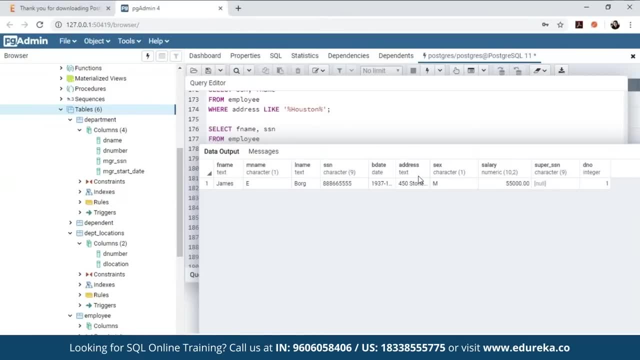 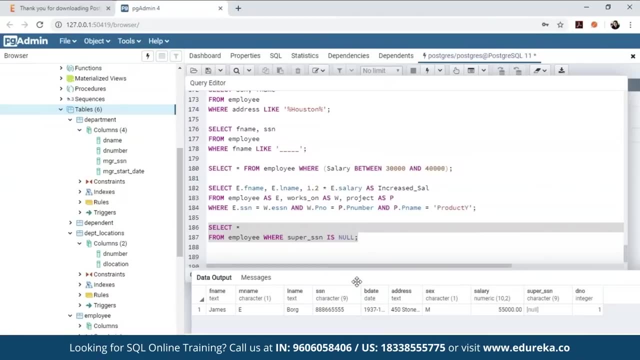 So next let's look into how you can use aggregate functions in sequel. So to use aggregate functions, what you can simply do is you basically have to use the functions as some max, min, average and count right. For example, let's say you know 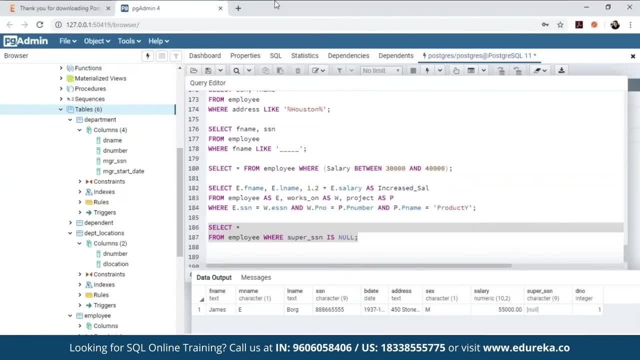 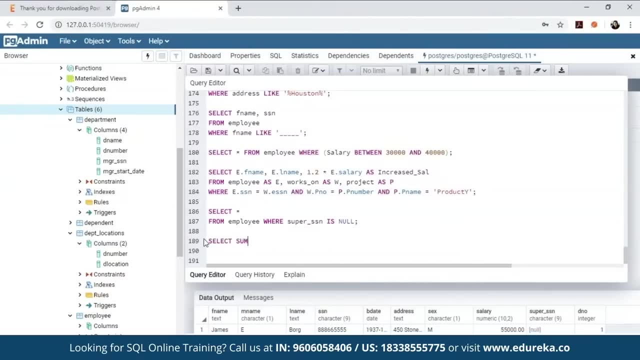 we want to find out the sum, the max, the min and the average salary from employee. Let's say so, Let's say you know, I want to find out the sum- min, max of salary from employee, right. So I'll just mention select some salary. 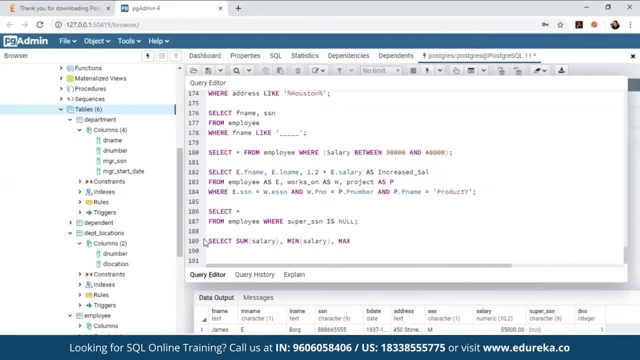 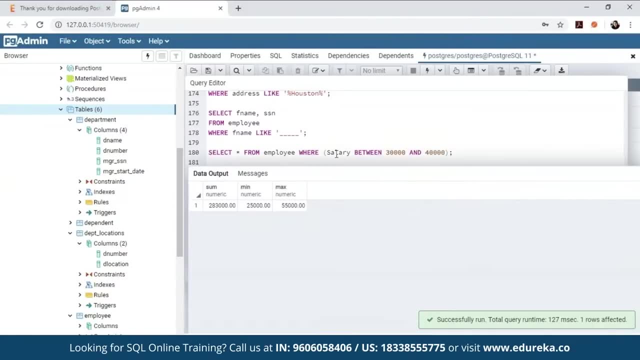 Main salary, Max salary from employee right. So when I mentioned that, you'll see that you know, the sum is so much the minimum and the maximum is so much. right, that was about some min Max. Now, let's say, you know, 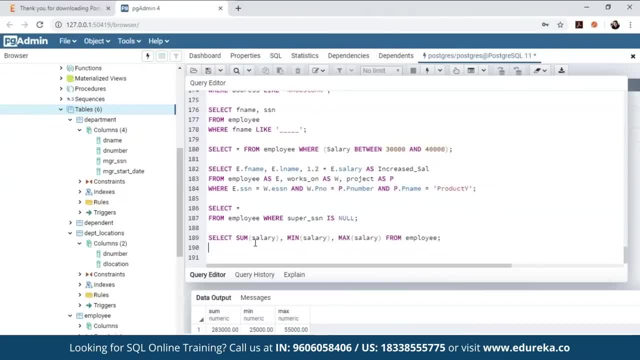 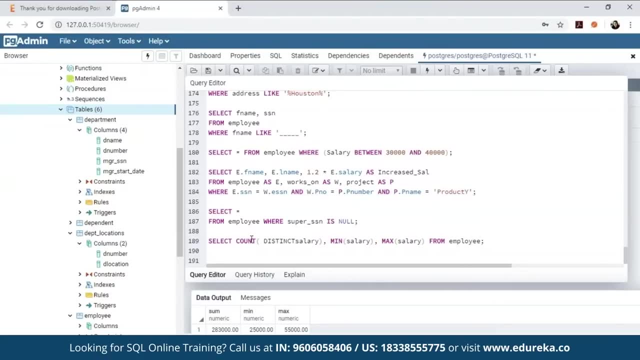 I want to count the salary. So what I'll do is I'll basically change this particular function to count right, and then I'll say: count distinct salary, because I want to count the unique ones right, and then I'll mention: from employee right. So I'll just remove this particular section, right? 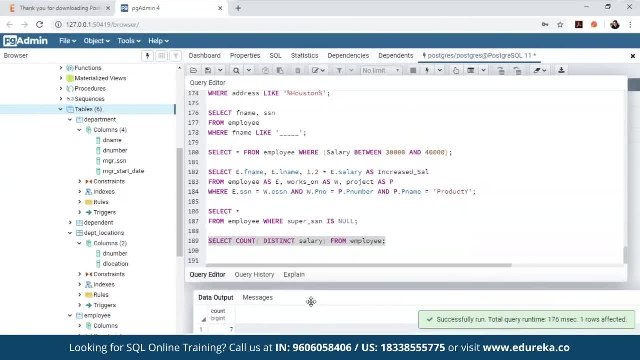 And then, if I just execute this, you'll see an output of seven, right? So basically we have seven distinct salaries. So that was about aggregate functions, guys. Now next let's look into order by group by and having clauses. So, as I mentioned before, the order by is basically used. 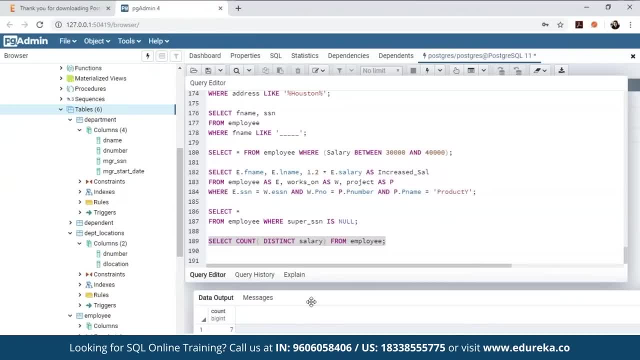 to get the output either in the ascending format or the descending format. the group by is basically used to group the data that you want by a specific column, and having is basically used to check a condition. Let's say, we want to write a query to retrieve a list. 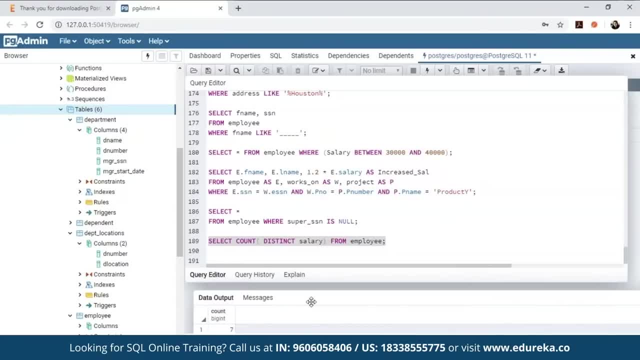 of employees and the projects they are working on ordered by the department, and within each department They have to be ordered alphabetically by the last name and then the first name. So initially they have to be ordered by department and then under each department also they have. 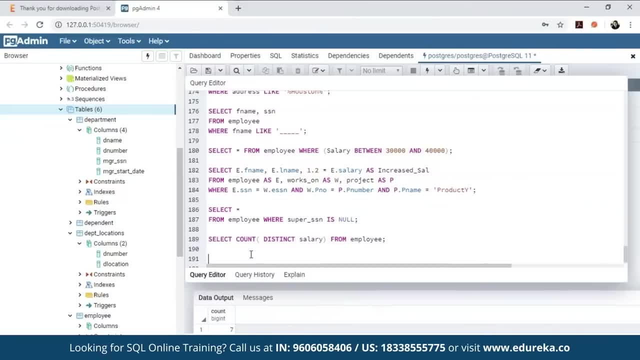 to be furthered ordered by the last name and the first name. So to do that, what you can do is you can just mention select, and then you mention D dot D name, right, And then you mentioned E dot L name. We also want the first name, right? 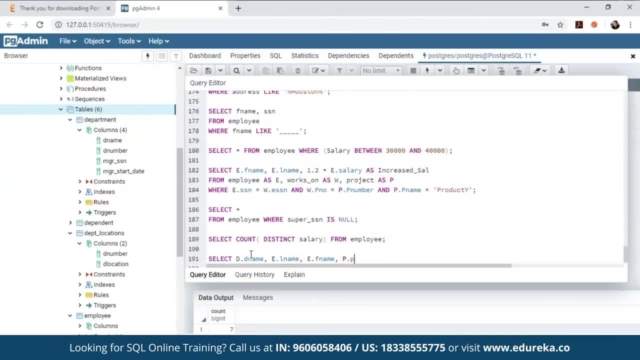 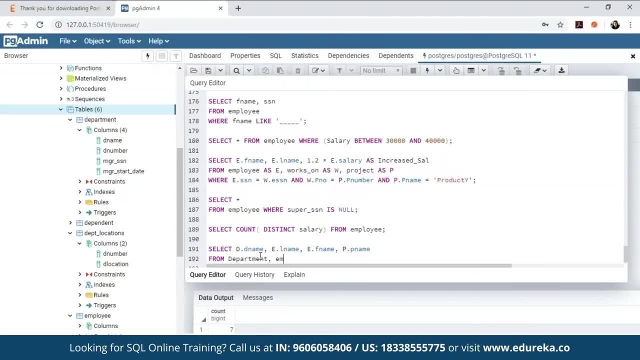 So we'll mention E dot F name, and then P dot. P name from Department is a typo. and then we also want employee, We also want works on right now, over here. We have to mention as W over here, as E over here, as D over here. 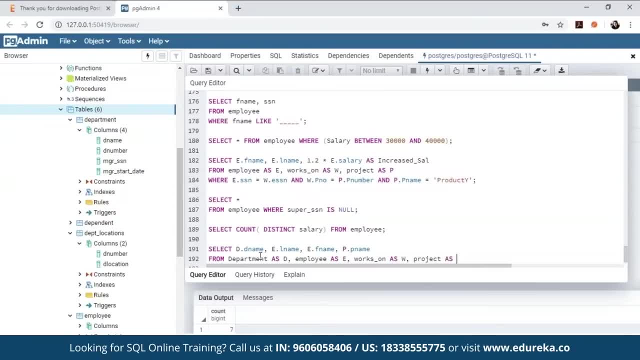 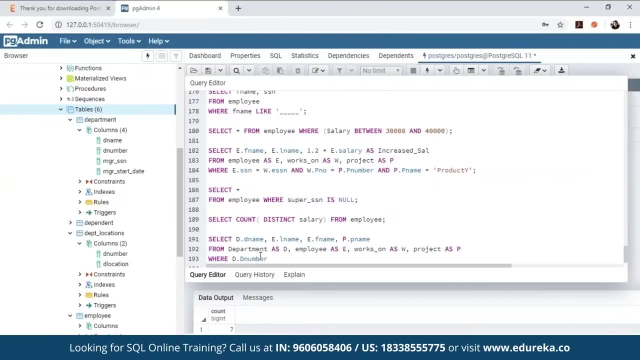 And then I forgot to mention the project. So project as P. and then you have to mention the condition which says where D E dot D number is equal to E dot D number and employee dot SSN is equal to works on that SSN and works on that P number is equal to P dot P number. 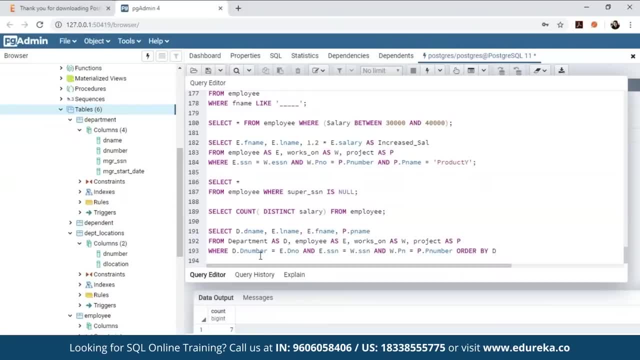 and then it is order by D dot D name, and then I mentioned E dot L name and E dot F name, right, and then I, if I just end this particular query, let's execute this particular query. you see an error that you know: W dot SSN- not found. 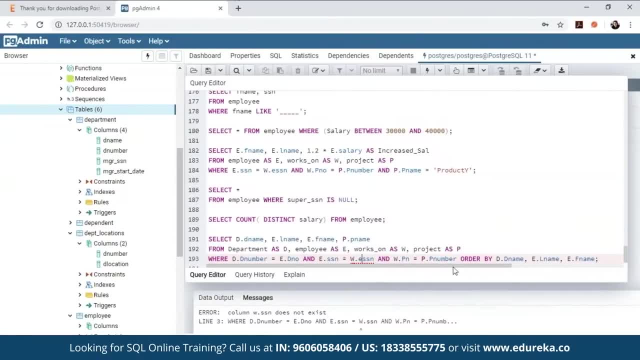 because this has to be ESSN, right? So I'll have to mention ESSN over here and then let's execute this query again. It's a type of error again, which is P dot P number. Right now let's execute again. 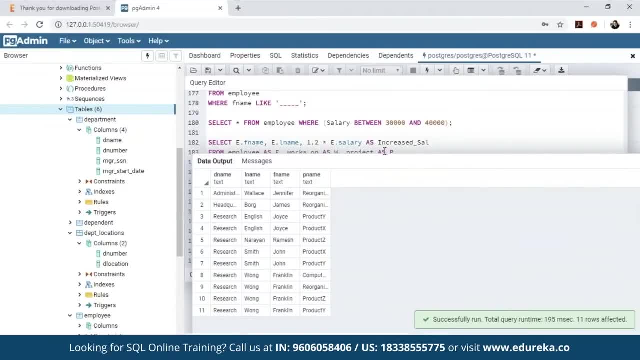 and you see an output of D name, L name, F name and project name. So initially, if you see the D name, the name is ordered by alphabetically, that is, in the ascending order from A to R, and then, under administration, Wallace and Jennifer have come. 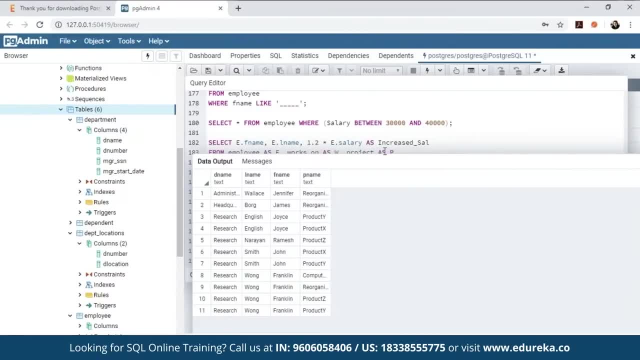 Similarly, headquarters have Borg and James. research has a lot of values, but underneath that also, we have ordered them according to ascending order, by which I mean that you know it is ordered alphabetically by last name and then the first name. So that's how, basically, guys, you can use the order by now. 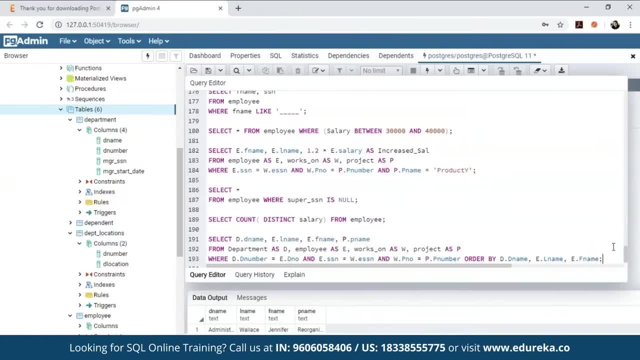 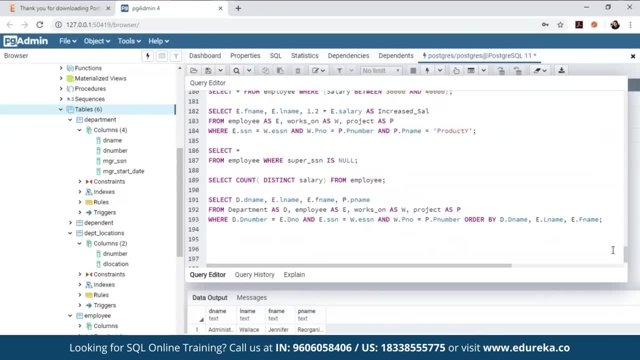 This was a little bit complicated one. If I just have to explain you with simple one, what you can do is you can consider the query of: let's say, you know, we want to find out the salary of all the employees in a descending order. 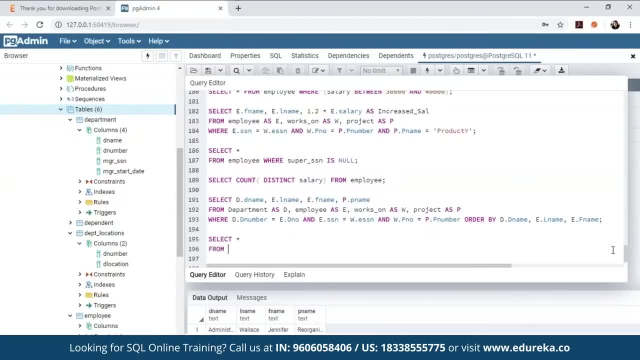 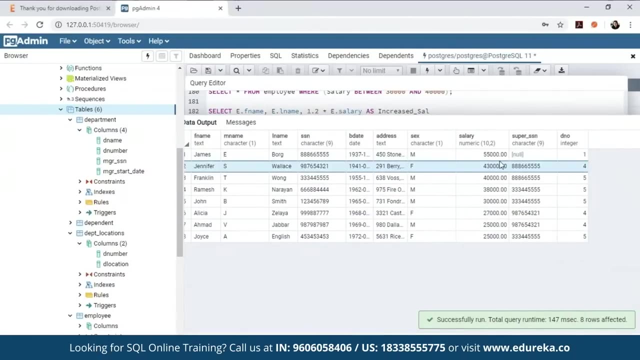 So what we do is we just type in select star from employee order by, and then we mentioned salary descending order. Right now, if I just execute this particular query, you'll see that you know, we get all the details of all the employees in the salaries of the descending orders. 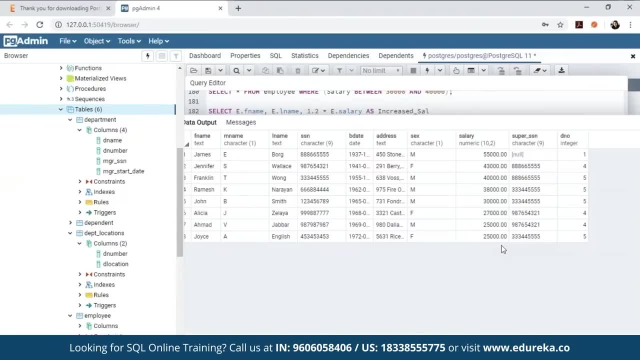 So, in the case of descending, if you mentioned ascending, then you'll get an output of all the details of all the employees in an ascending order of based on the salaries. So, guys, that was about the order by Claus. Now let's move forward with the group by Claus. 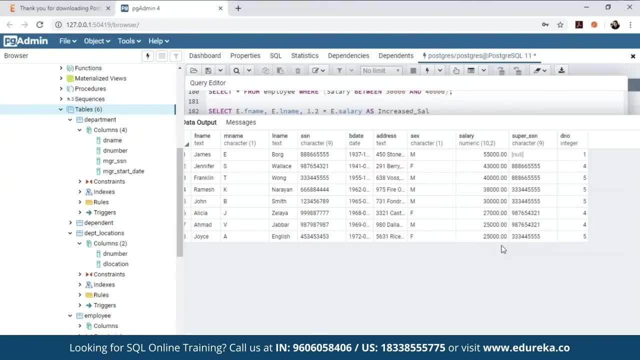 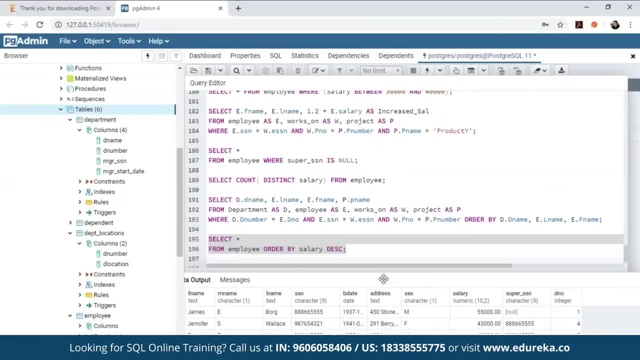 Now let's say, you know, we want to find out for each department, We want to retrieve the department number and the number of employees in the department, right, So now to retrieve the number of employees, you know the aggregate function. 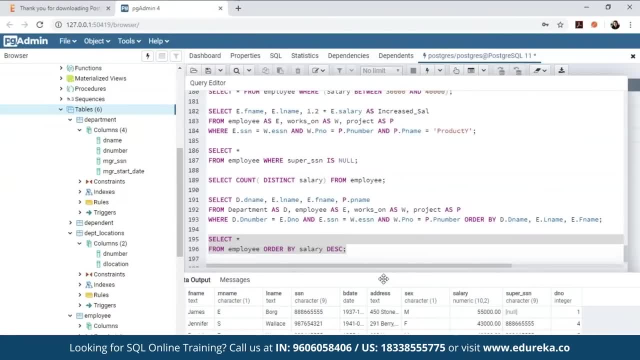 We have to use the count function and then we want to group it by the department number, right, because we have to do it for each department, right? The question says: for each department, We want to retrieve the department Number and the number of employees. 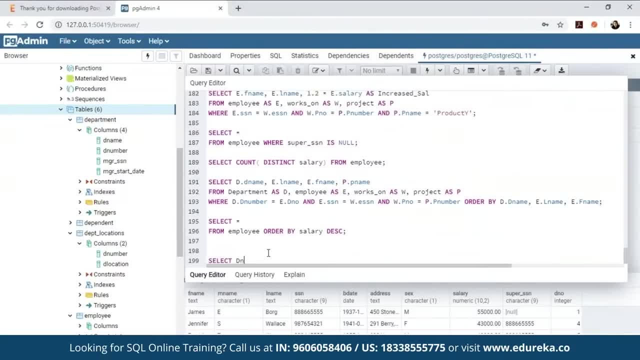 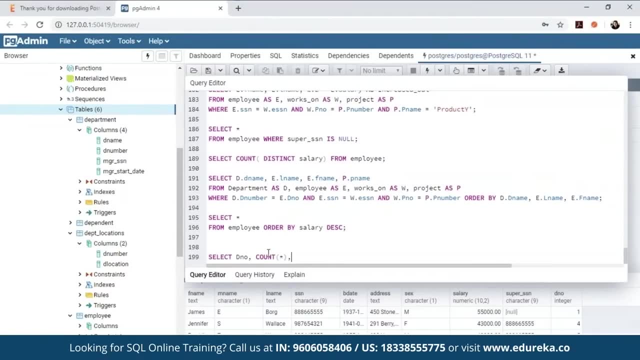 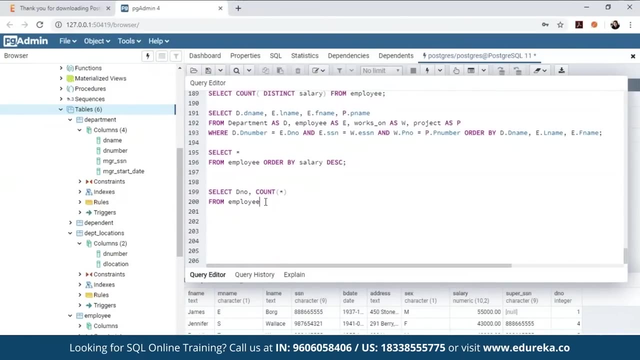 So to do that, what I'll simply do is and mention a select query department number and then account function of all the employees, and then I'll mention from employee right. So let me just press on enter so that the keyboard doesn't move. and then I mentioned group by the number right. 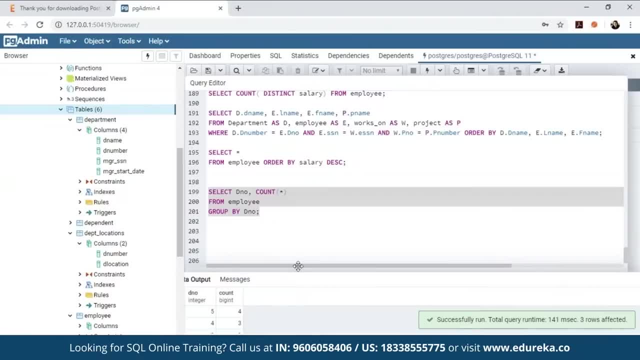 because we want to find it for each department. We're using this. So for each department, if we have a count, like you know, in the department number five, the number of employees working up for in the department number four, the number of employees working at four are three. 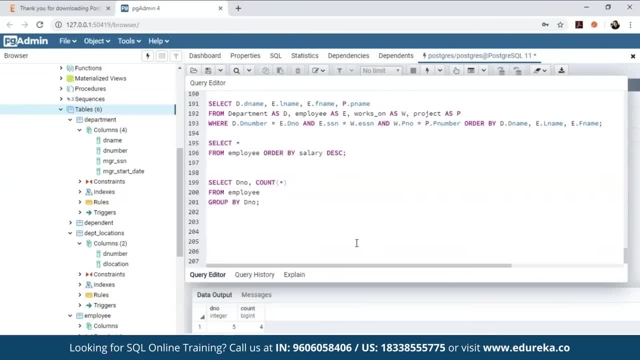 and in the department one, the number of employees working on one. All right, so that was about the group by clause guys. I hope that was simple to understand. now Let's look into the having clause. So having, as I mentioned before, is basically used. 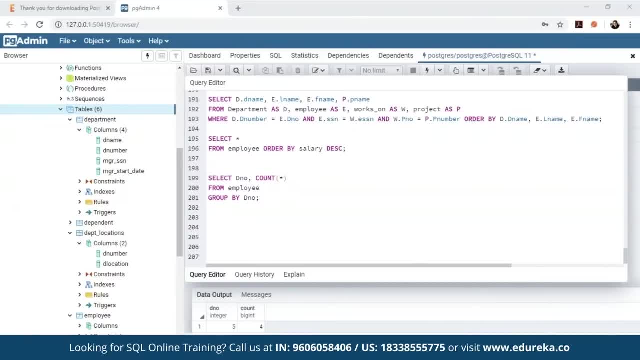 to specify a specific condition. So let's say you know, having countless than two, greater than two, having salary greater than 25,000, or maybe less than 30,000, and so on. now let's say you know we have a scenario where we want to retrieve the data. 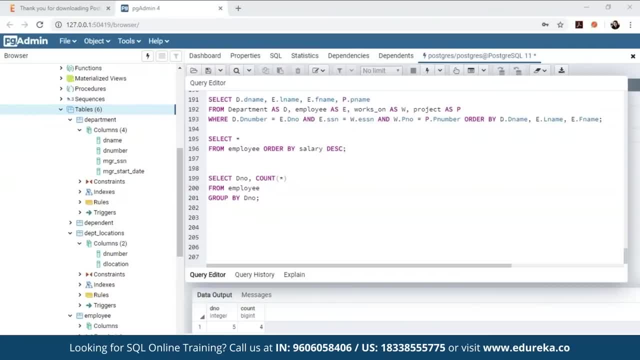 for each project on which, let's say, more than three employees work, We want to retrieve the project number and the number of employees who work on the project. I mean condition is that you know for each project that the employee count is more than three right. 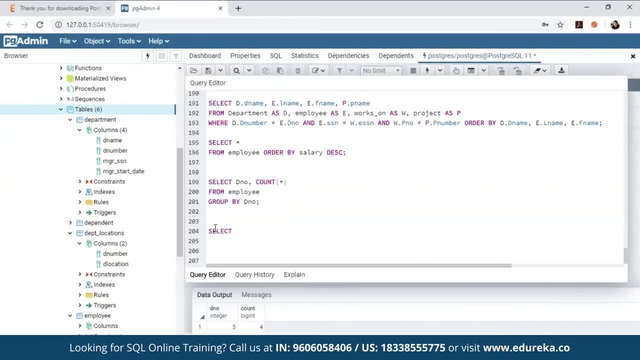 So for that, what I'm going to do is I'm going to mention the condition, select P number. that is because of the project number. and then let's say I want to count the employees right, So I'll mention count star from project works on. 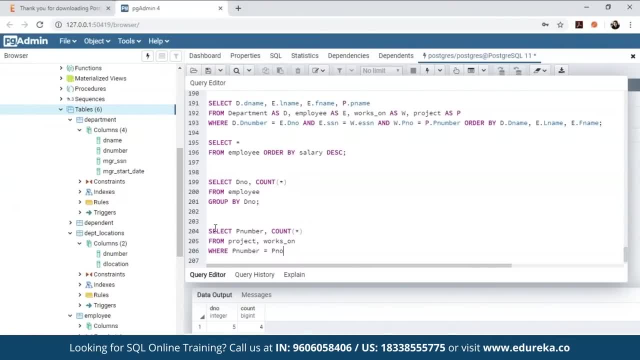 where P number is equal to P number, and then I group by for each project, right? So when you group by, you basically have to group by project number. and then I mentioned the condition having count greater than I forgot to mention the asterisk condition. over here three: 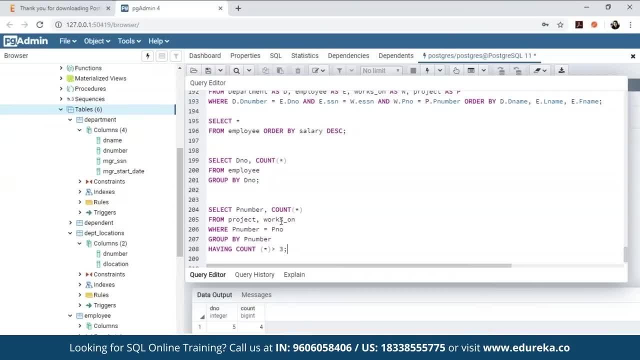 So basically I'm mentioning the condition that you know- we want to retrieve the project number and the count of employees who are working on the project, where the project number from the project table matches the project number from the works on table, and then it is group by project number. 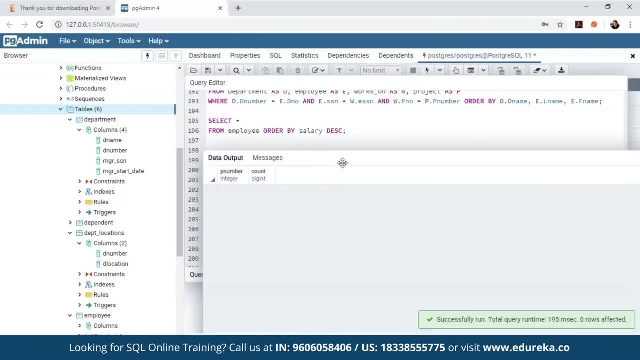 where the count is more than three. Now, if I execute this particular query, you see that you know there's no data return, right? So that may be because you know the condition is not satisfied by any of the data that we have. 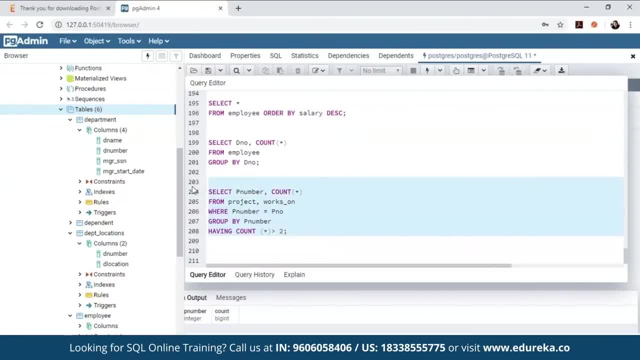 So let's say, you know we want to do it too. So I'm just mentioning the condition to be two and I click on enter and then you see that you know we get the project number. So two, where you see the count is free. 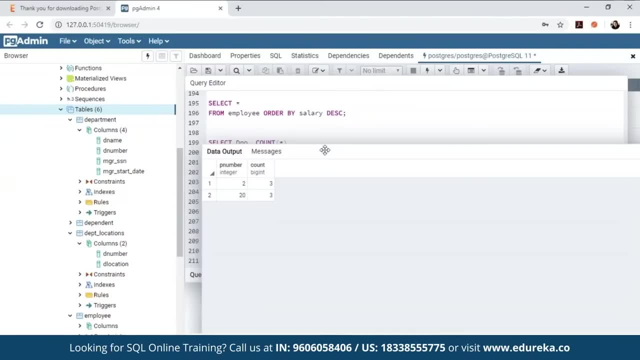 and then the project number 20 where you see the count is free. So initially when I mentioned the condition having count greater than three, the output did not come because there was no such data present. So that's the reason there was nothing return. But when we change the condition you see that. 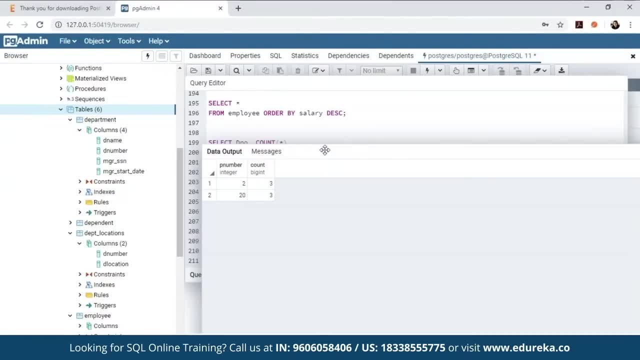 you know, we get an output of two project numbers. So, guys, that's how, basically, you can use the group by clause, the order by clause and the having clause. next, as I was talking about the limit, offset and fetch, Let me just quickly cover that particular part. 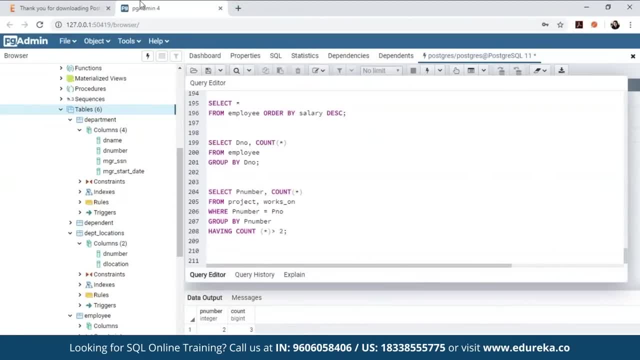 so that we can go back and learn about sequel joints. now talking about a limit, as I told you, if you want to limit the data that you want to fetch right. So basically, let's say, you know, we want to just fetch five rows, right. 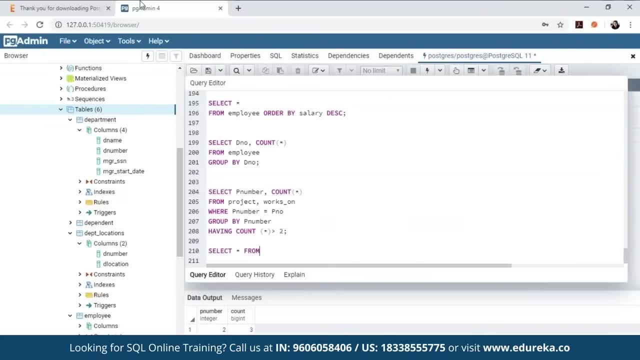 What you can simply do is you can just type in select star from, let's say, works on, and then we limit five. right, And now, if I execute this particular query, you'll see an output that you know: only five rows of data will be printed out. 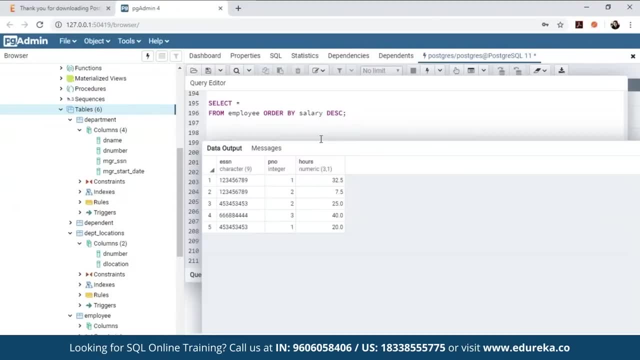 So that's because you know we're limiting the data that has to be written. now Let's say you know we want to select three rows from, let's say, works on table after the fifth row. So we want the next three rows to be printed. 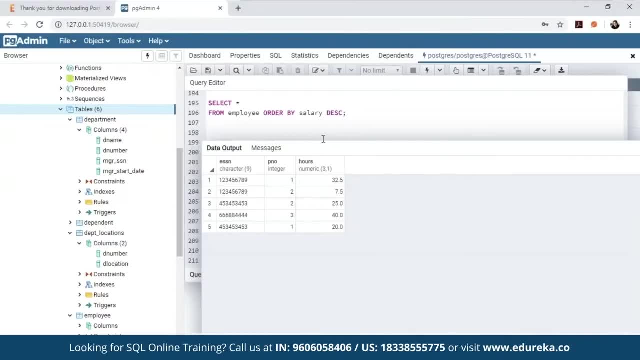 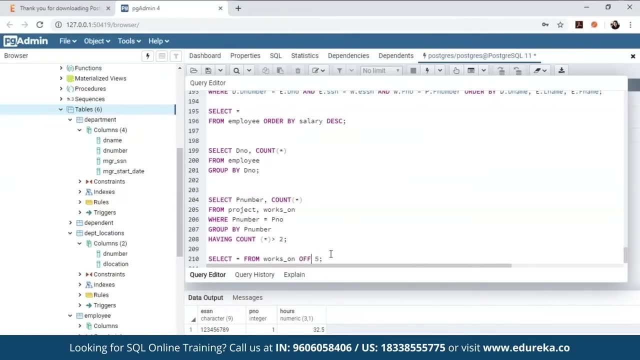 after the fifth row. So for that you have to use the offset statement. So what you'll do is you'll mention select star from works on, and then what you'll do is, instead of limit, over here, you'll mention offset five, and then, over here, you'll mention limit three. 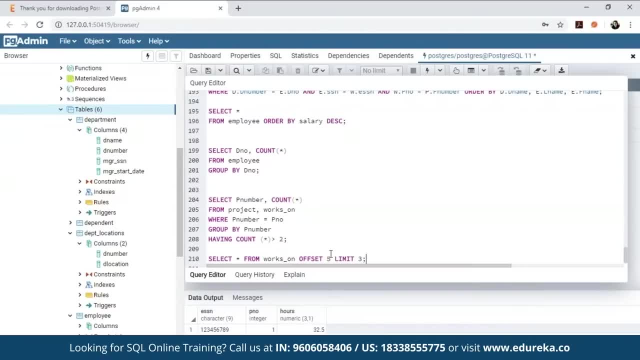 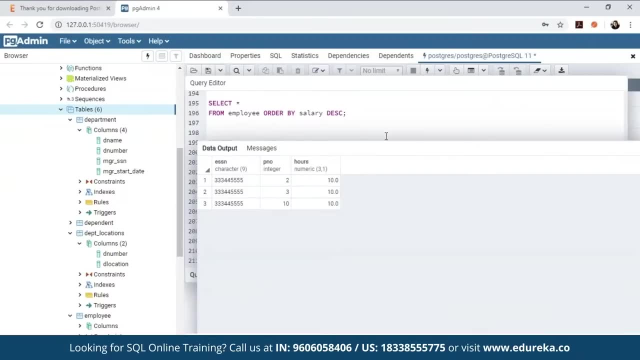 So after the fifth row, you want three rows to be printed. So that is the reason you'll mention offset pipe and limit tree. So let me just execute this particular query. So if I execute this particular query, you'll see that you know. 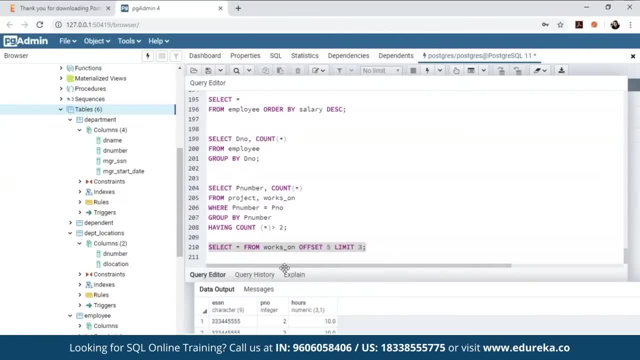 I've got the output of 6, 7th and 8th row. So basically, guys, that's how you can use the offset statement. Now let's say you know if you want to use the FET statement. So, as I mentioned before, the FET statement is also used. 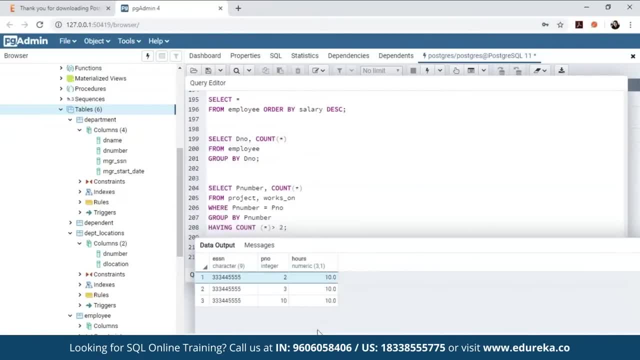 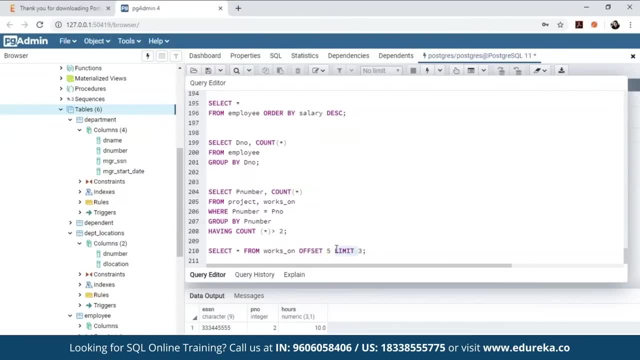 to fetch the records. So let's say, you know I want to fetch the first eight rows, So what I'll do is I mentioned select star from works on and then mention offset five, and then I'll mention first eight rows Only. so after the fifth row, what I'll mention? 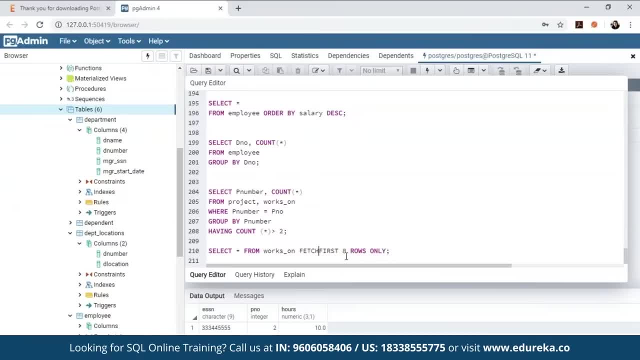 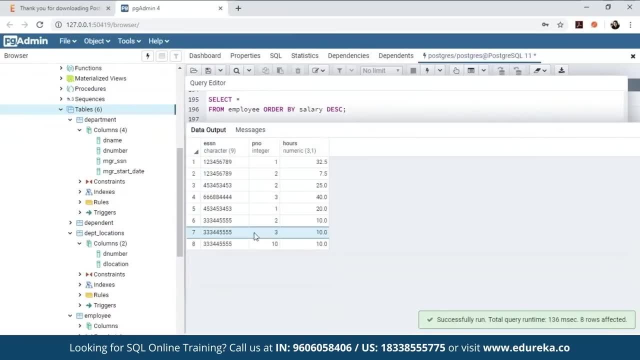 is, I'll mention select star from works on and then I'll mention fetch, first eight rows only, right. So if I just execute this particular statement, You'll see the first eight rows. So over here you can clearly see the output that you know. 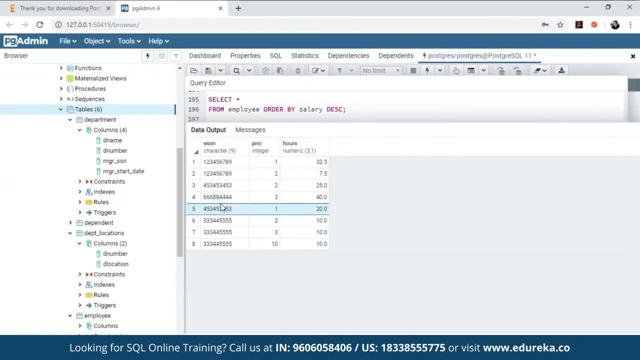 when we used limit five, you saw the first five rows. and then, when we used offset five and then limit free, we saw the next three rows. and now if you're using the fetch command where we say fetch first eight rows only, you'll see that. you know. 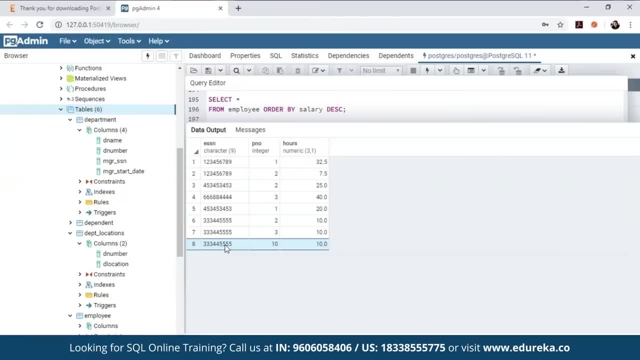 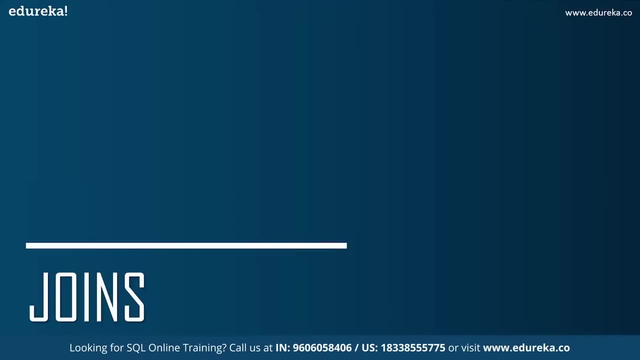 you can fetch all the eight rows, right? So that's how, guys, basically you can use the limit offset and the fetch commands. So that was about till now. Now let's go back to our PPT and next let's look into joints in SQL. 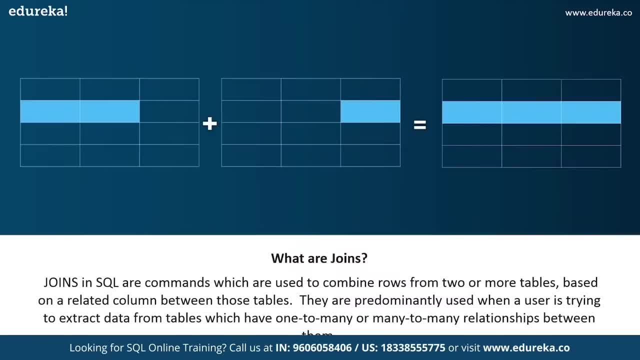 So all of you might be knowing what are joints right now. joints in SQL are commands which are basically used to combine rows from two or more tables based on a related column between those two tables. So they are predominantly used when a user is trying to extract data from the tables. 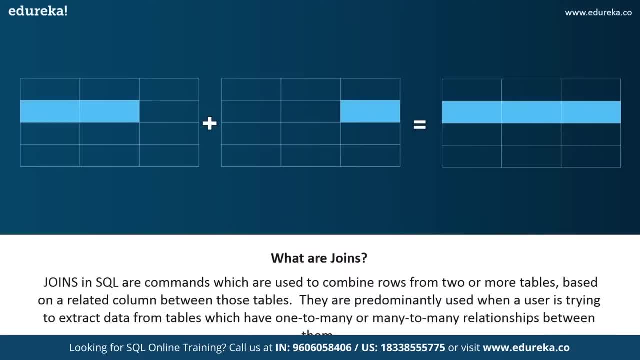 which have one too many relationships or many too many relationships between them. So if you just have to understand joints in a simple language, then joints in SQL are basic commands which are used to combine rows from two or more tables based on a related column between those two tables. 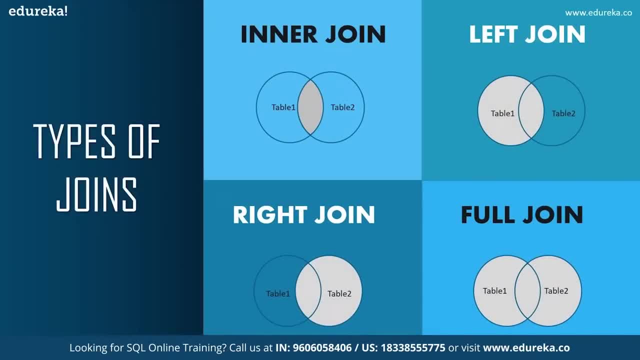 So, basically, there are four types of joints present, that is, the inner joint, the left joint, the right joint and the full joint. So, as you can see on my screen, the inner joint is the joint which is used to return the records which have matching values in both the tables. 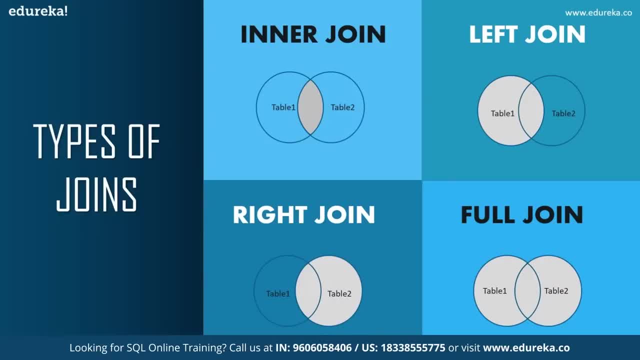 So whenever you have matching values in both the tables you use in a joint. coming to the left joint, the left joint returns records from the left table and also those records would satisfy the condition. from the right table. the right joint returns records from the right table and also those records would satisfy the condition. 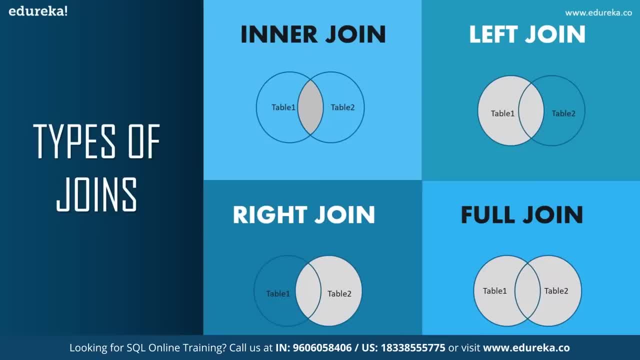 from the left table and finally, coming to full joint, the full joint returns all those records which either have a matching value in the left table or on the right table. So, guys, these were the mainly four types of joints, that is, the inner joint, the full, the left. 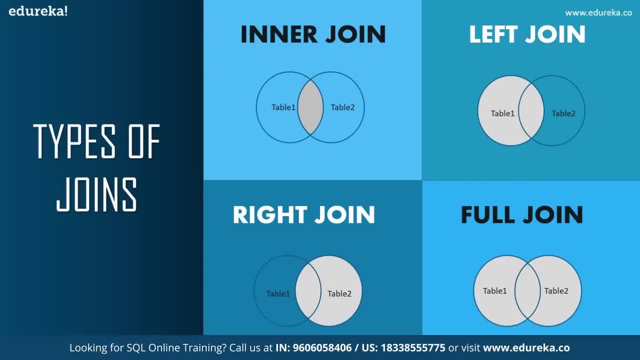 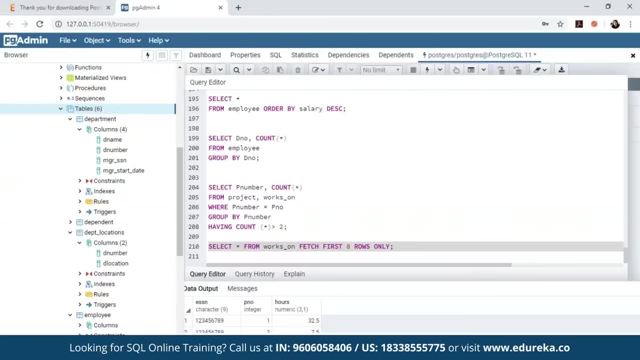 and the right joint. now let me just quickly take you back to PG admin and then let's apply a few joints on the tables that we have. For example, let's say: you know, we want to apply left joint right, as I've told you before. 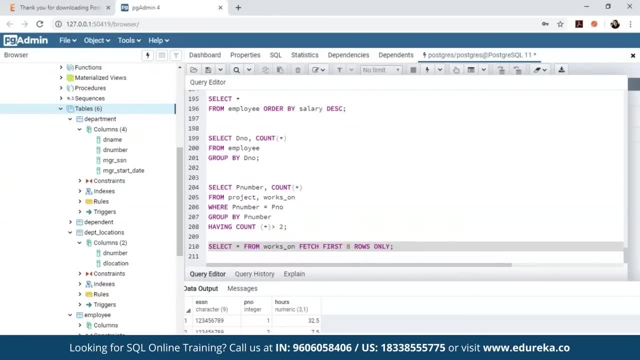 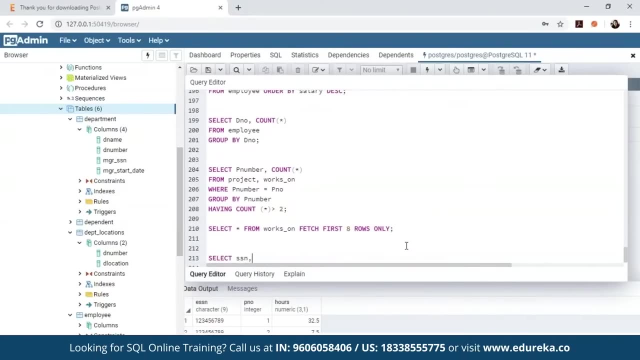 the left joint is basically going to return all those records from the left table and also all those records matching the condition from the right table. What I'll do is I'll mention select, let's say SSN. I'm going to mention first name and then I mentioned dependent dot, dependent name. 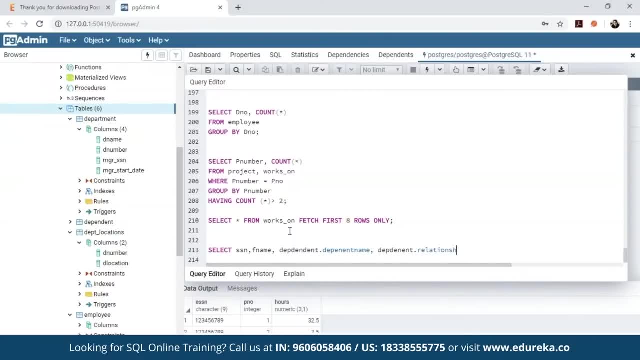 and then I'll mention dependent dot relationship, which is a column of the dependent table, and then I'll mention from employee left join, and then I'll mention the table one that is basically dependent on employee dot. SSN is equal to dependent dot ESSN. 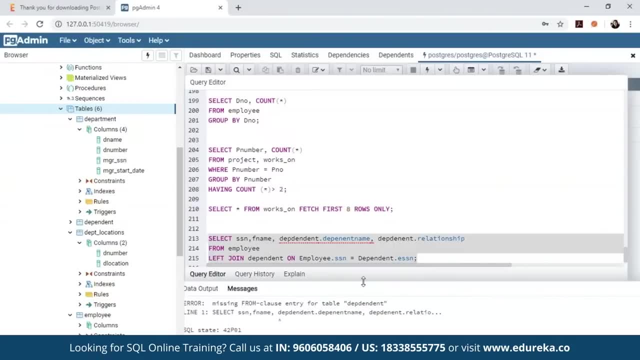 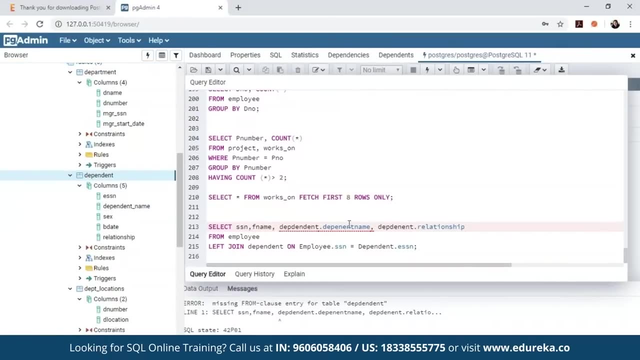 So when I execute this particular query, you see an error that you know. the table is not found because we have an error with the column name. So let's just check the column name. Okay, it's underscore, So I'll mention underscore over here. 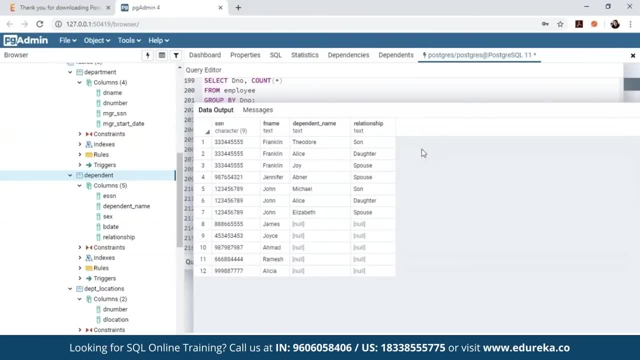 So when you see the output, you can clearly see that you know we've got all the records from the left table, that is, a dependent table, and then all the records which also matches the condition, from the right table. So that's how, guys, you can apply left, join the similarly. 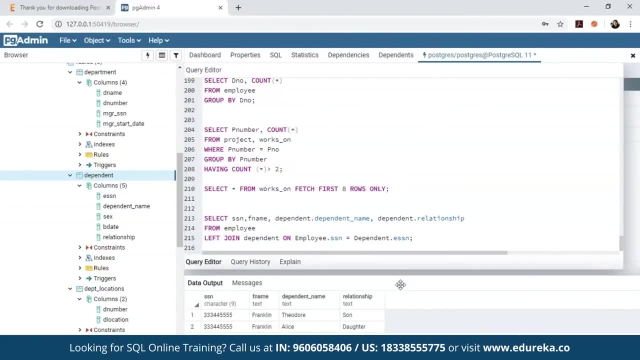 you can apply right join also. So for the same condition, let's apply the right, John, and let's see the difference in the outputs, right? So what I'll do is I'll just scroll again and then I'll just change it to right join. 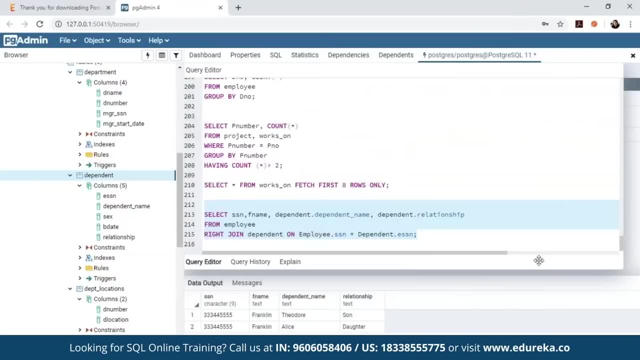 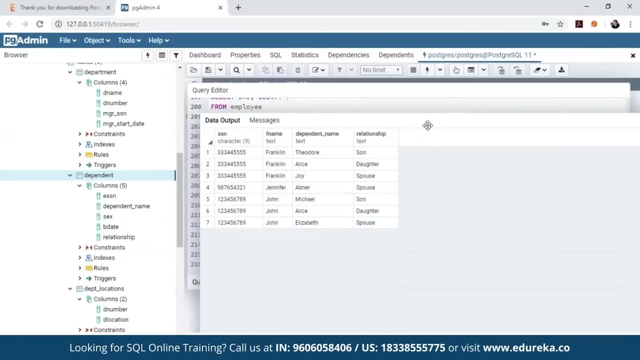 and now I'll execute again. So let me just execute this particular query, And once I execute this particular query, you'll see a difference, right? So that's basically how you can play around with joints, guys. This was about left and right. now, before I conclude, the joints. 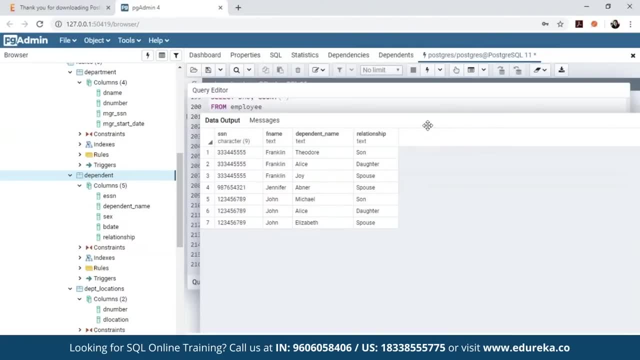 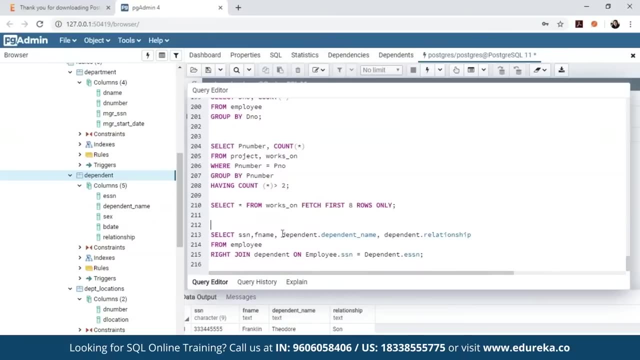 part. let me also talk about the inner joint and the full joint. So the inner joint is basically where you have matching values in both tables, right? So let's say you know we select SSN and first name and let's say you know. 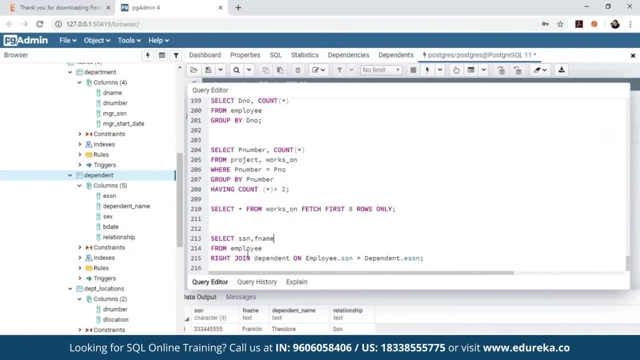 we remove this particular section and then we mentioned from employee. I'll mention inner joint: dependent On employed at SSN is equal to dependent. So we'll get all those records which have matching values in both the tables right. I'll execute this particular query. 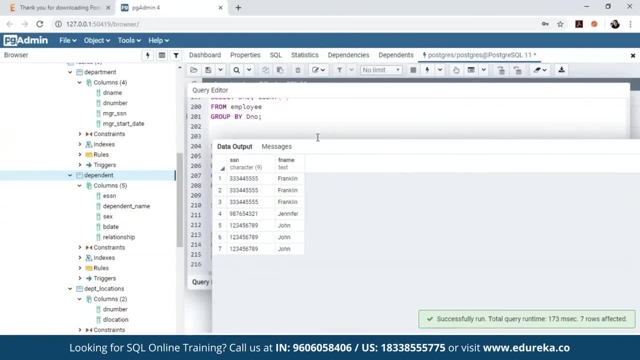 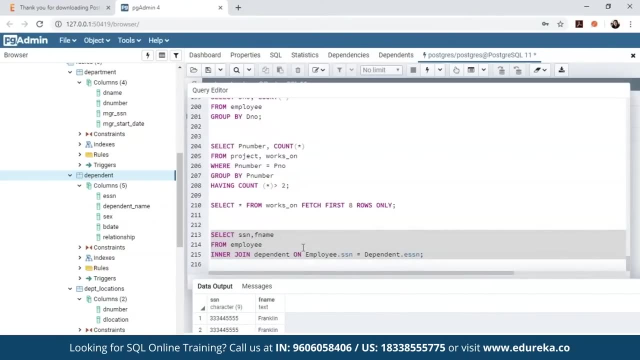 and you'll see the output right. So these are basically all those values which have a matching values in both the table a and table B And finally, let's say, you know, if I want to specify the full joint which basically will give me the output of all those records. 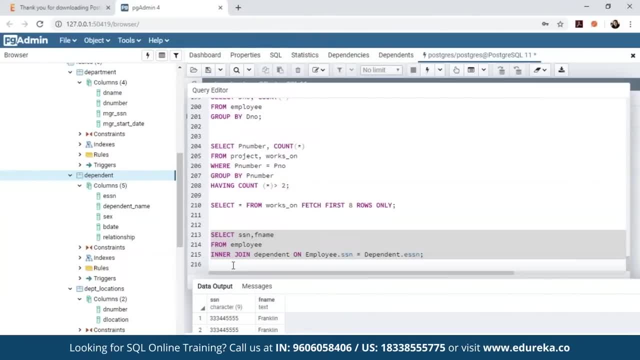 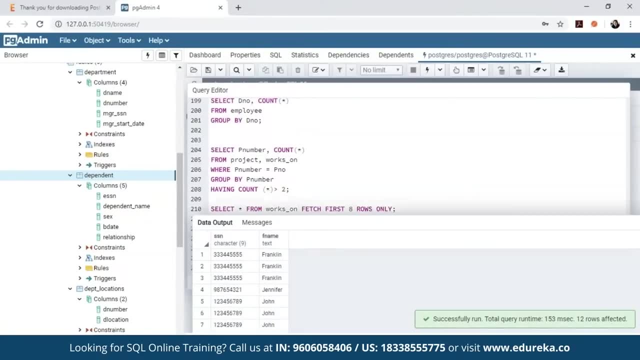 which either have a matching value in the left table or on the right table. What I can do is I can simply mention full join over here, And then I execute this and then you'll see an output like this: right? So basically, you'll see that you know. 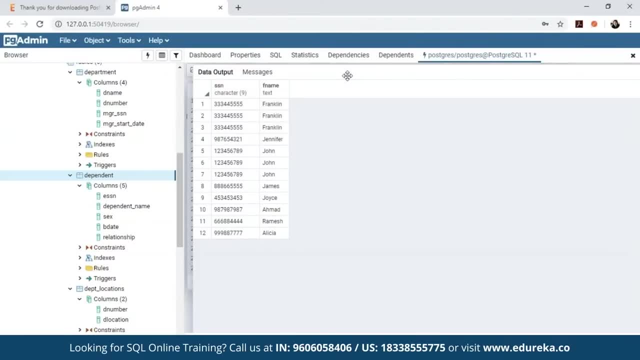 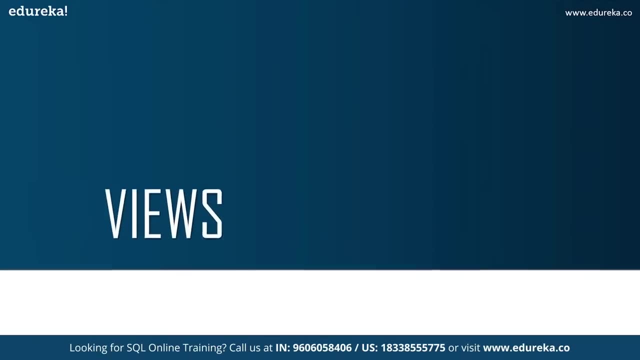 these are all the tuples which have either a matching value in the left table or on the right table. So, guys, that was about joints. next in this session, Let's move forward and take a look at the views. So views are really simple, guys, as the name suggests, views. 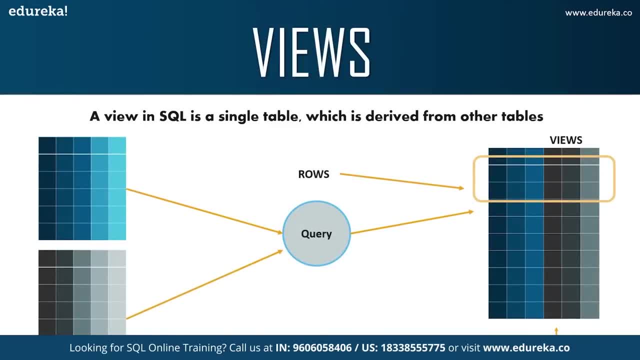 in sequel is a single table which is derived basically from the other tables. So, for instance, if you consider the example on my screen, I have two tables right now. For example, let's say I want to create a new view which will basically have a few columns or rows. 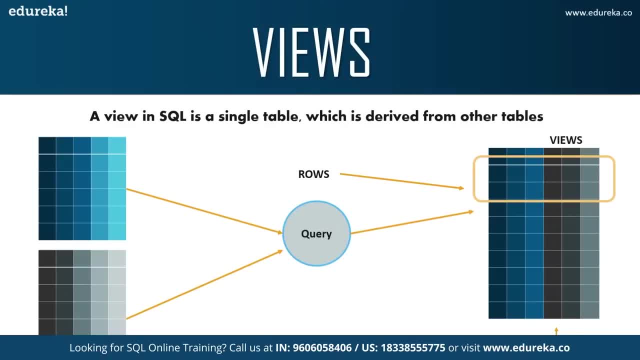 from a specific table and few columns or rows from the other table right. So that is basically my view. So now views are used in industries to basically collaborate with the data of many tables so that the company can understand how to go about the next action step. 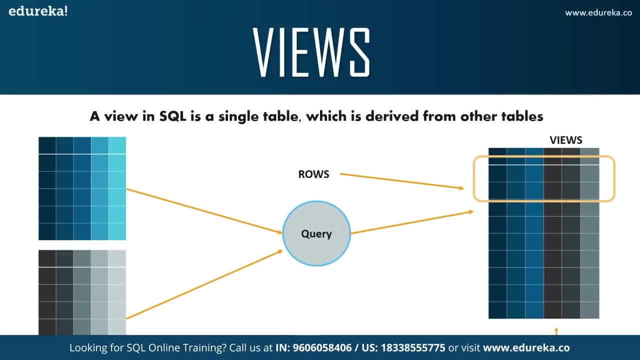 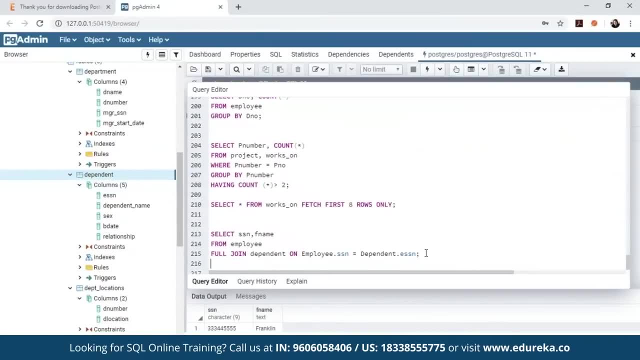 They should take while taking any specific decision. So, without wasting very any further time, let's take a look at how we can create a view. So to create a view, it's really simple: either you can use the query tool, or what you can do is you can just go to the view option. 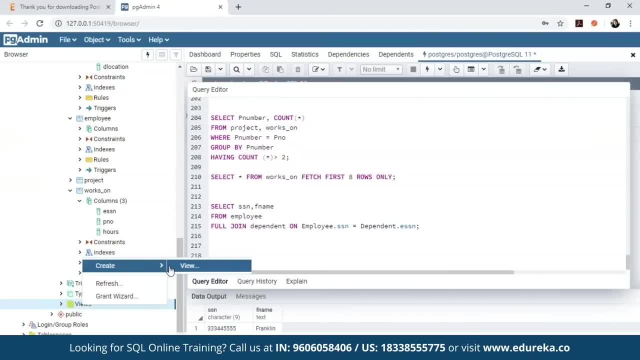 right click over here: Choose, create and choose view. since I'm writing queries for all of them, I'll show you by writing queries itself, else You can use this option also. so talking about views, So to create a view, it's really simple as you create a table. 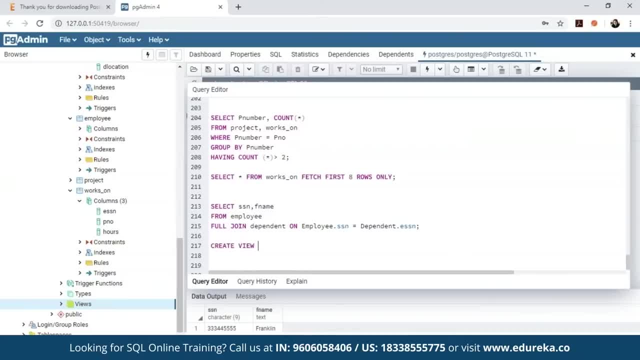 You can similarly create a view, like you know, create view and then you mentioned a view name. Let's say, we're going to create a view for the works on table, So I mentioned works on one, and then what I'll do is I'll mention the condition. 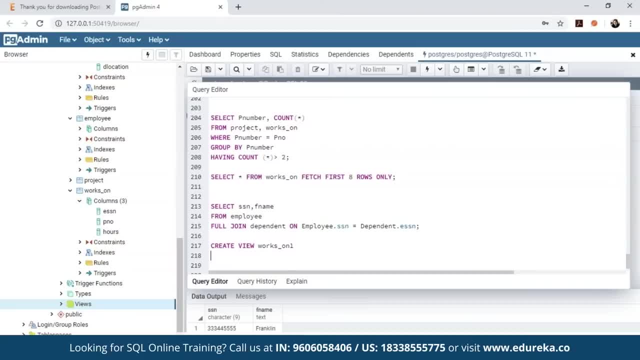 So if you stop over here, this will simply create a view and this will not store any particular data that you want. But if you start mentioning the condition, then it will have all the data according to the condition that you have mentioned, right? So, over here, what I'm doing is I'm going to mention the details. 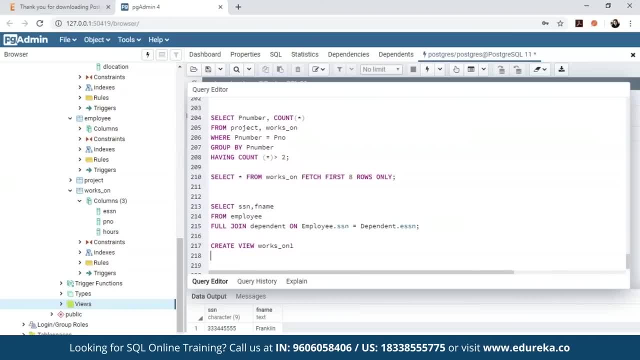 of an employee who work on a specific project. So for that I'm going to do is I'm going to just create a view over here. So, as I'm creating, so I'll type in: create view, works on, and then I'll mention the condition as select: first name, last name. 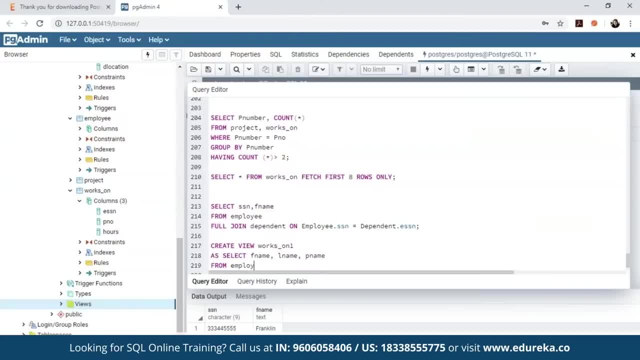 and project name. So from employee project and works on where SSN is equal to ESSN and project number is equal to project number, right? So that is basically the project number matching from the project table to the works on table and the SSN matching from the employee table. 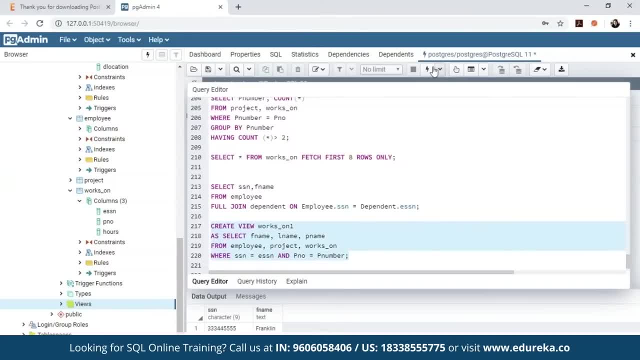 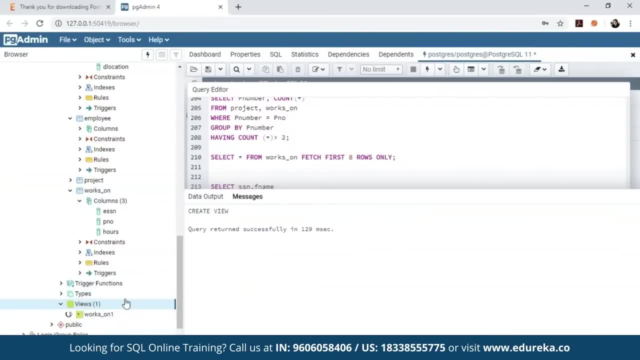 to the works on table right And then I'll just execute this particular query right. Once you execute this particular query, you see an output that you know: query returns Successfully. now, if I just refresh this particular views, you'll see a view named as works on with the columns. 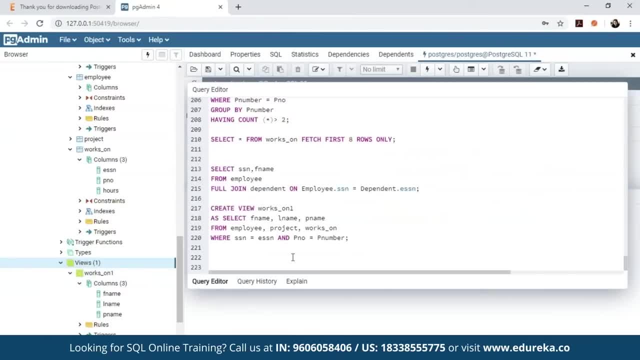 that you have mentioned. that is first name, last name and the project name. Now, if you want to see the data present in this particular view you, what you can do is you can just mention select star from, and then you mentioned the view name. that is works on one. 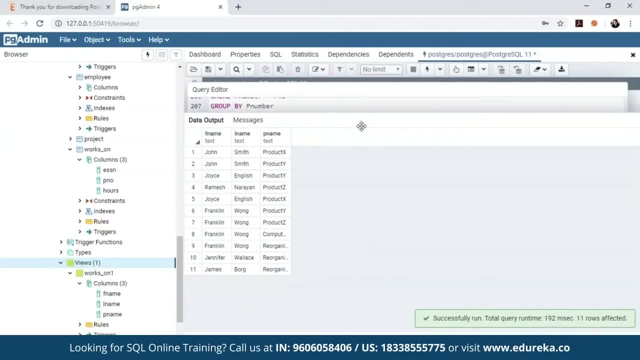 right, And then, if I execute this, you'll see the output right. So that is basically the data that is automatically present in a view, and the view is created by deriving data from other tables, like the employee table, the project table and the works on table. 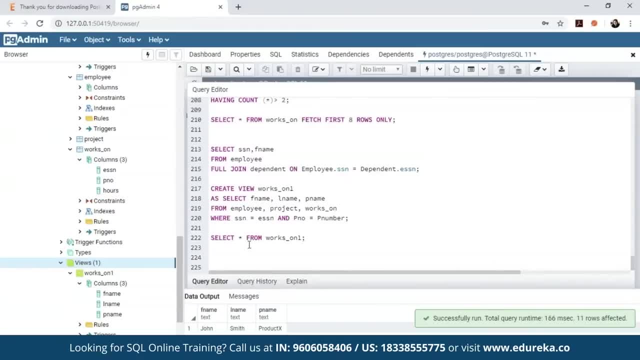 So that's how I is. basically, you can create a view. now, let's say you know you want to drop a view. dropping a view is also really simple, guys. You have to type in drop view and then the view name, right? 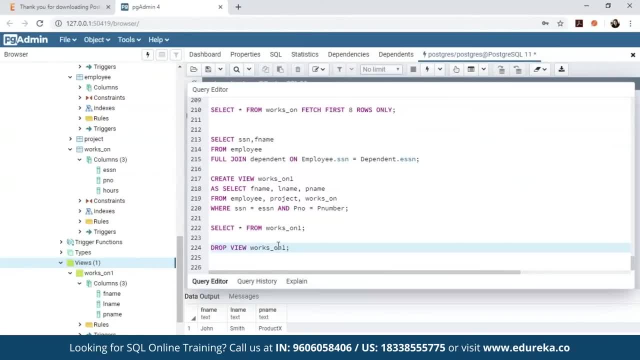 So if I mentioned works on one and then if I end with a semicolon, you'll see that you know the drop view is successful. So if I just refresh this particular section, you'll see that you know there's no view available. 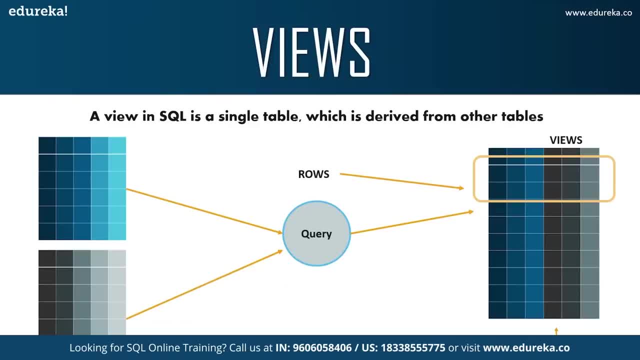 So, guys, that's how, basically, you can drop view also. so, guys, that was all about views. I'm not going to go into depth of how you can create more complicated views, and all because I've given you a basic understanding of how views are created. 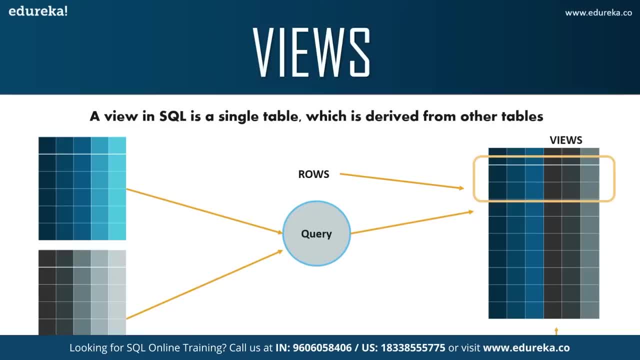 and how you can drop the views also rest. I leave it you to practice. Please remember the fact that you know I'm just giving you all the basic concepts so that you get started with Postgres SQL. But if you have to get a good understanding, 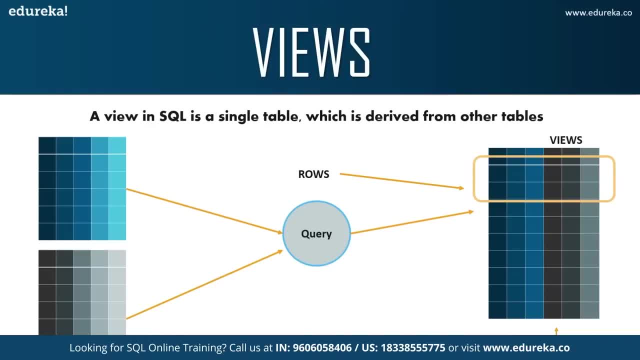 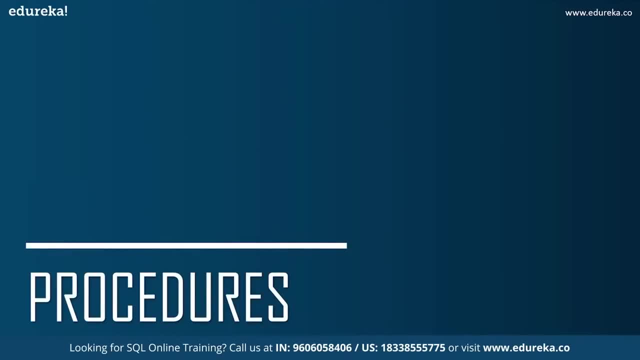 of all the databases, then make sure you have good practice on that note. Let's get started with the next topic for today's session, That is procedures. So procedures are basically a section of code. So basically you can understand procedures as a section of code or functions. 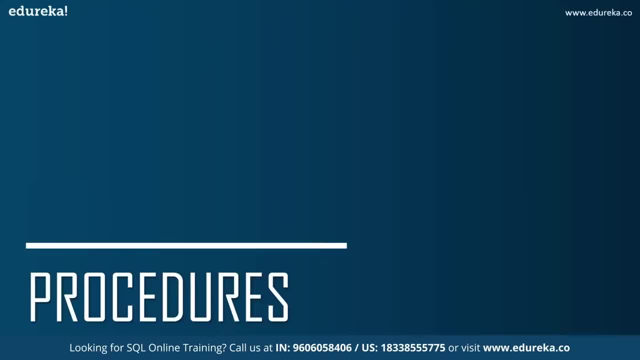 which you can save, you know, and then you can reuse it right. So whenever you want to save a section of code, or maybe a function, and then you want to keep reusing it, That's where the store procedures come into the picture. 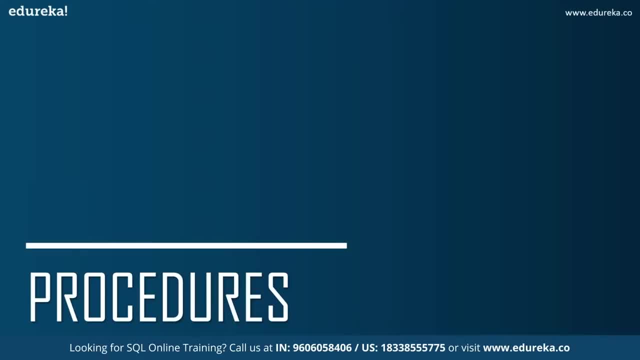 So, for example, let's say: you know you want to create procedures, right, So what I'm going to do is I'm going to create a new table. Let's stop with the example of employees and works on and so on. 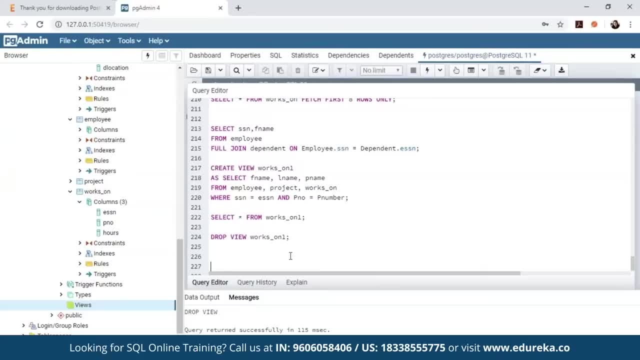 Let's move on with a new example. Let's say: you know I create two tables, So I'll mention create table and then I'll mention, let's say, the table name, table first able to be tbl1 and then I'll mention the column to be tbl1 ID. 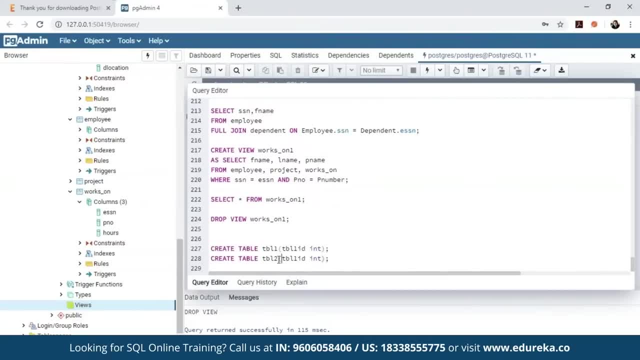 and then let it be int now. Similarly, I'll create another table also, So let me just change it to tbl2 also, and then now what I'll do is I'll just execute this particular two statements, right? So if I just refresh the section over here, right? 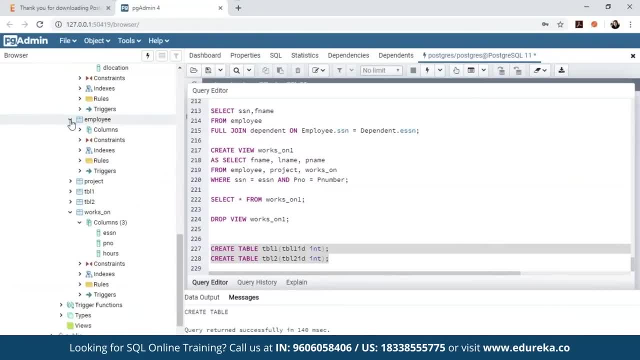 So now you will see that, you know, instead of six tables now there are eight tables, So let me just minimize the others so that you have no confusion, right? So we have two tables, that is, tbl1 and tbl2.. Now let's say, you know. 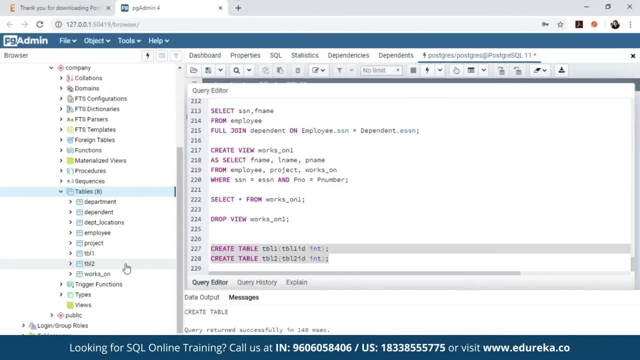 you want to create a procedure such that you know you want to insert values. So, basically, I don't want to write insert into statements 110 times. What I'm going to do is I'm going to just create a simple function through which you can insert values. 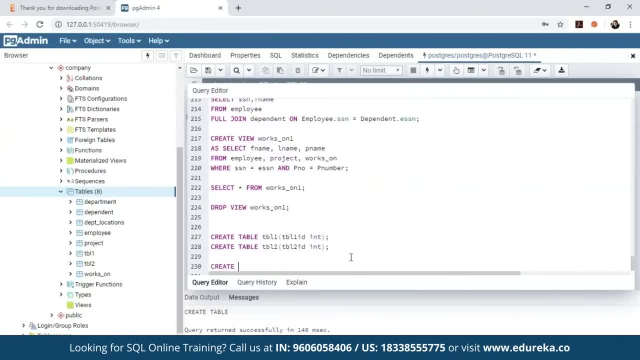 So to insert values, what you can simply do is I'll mention create procedure and then, let's say, mentioned the procedure name to be insert values. And now let's say you know we mentioned what values have to be inserted. Let's say, you know value X has to be inserted in table 1. 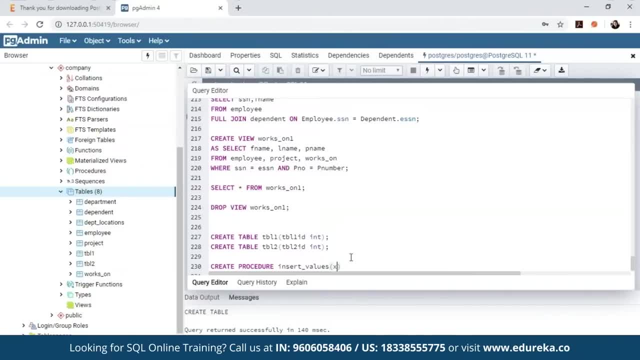 and value Y has to be inserted in table 2.. So I'll mention X integer and Y integer, and then what I'll do is I'll mention language Sequel, because it is a form of sequel- as dollar dollar, and then I'll mention insert. 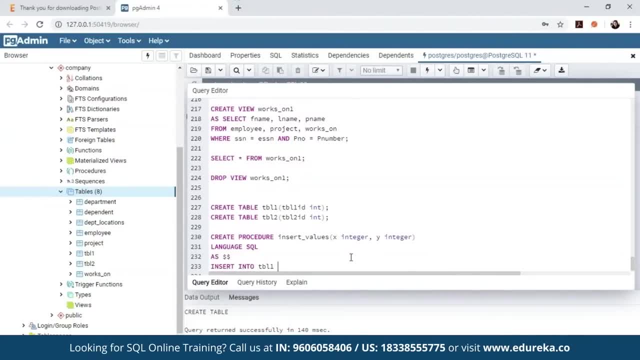 into tbl1- that is basically my first table- values X, right, and then I'll mention: insert into tbl2 values Y. after that I'll just end this section with double dollar and semicolon, and then what I'll do is I'll basically call this particular. 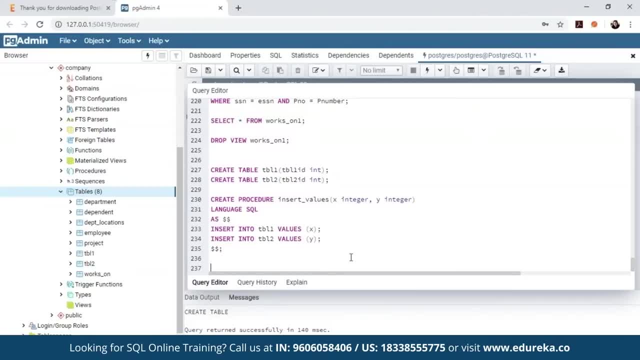 function. So this is basically how you create a procedure. But yes, if you want to reuse a procedure, then you have to call that particular procedure, Right? So for that I'll use the function call, insert values and then I'll mention, let's say, want to write. 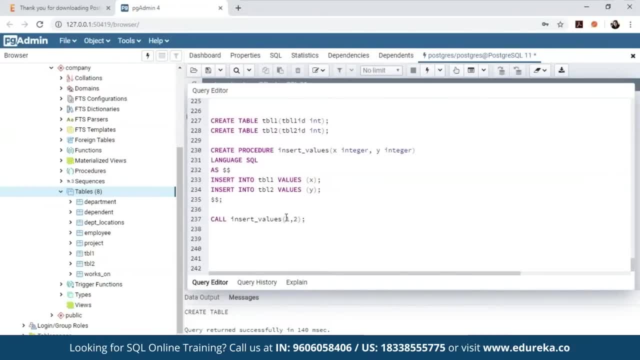 So these are basically the two values that I want to mention in table 1 and table 2.. So the table 1 should be inserted with value 1 and then table 2 should have the value 2, and now what I'll do is I'll execute this particular section. 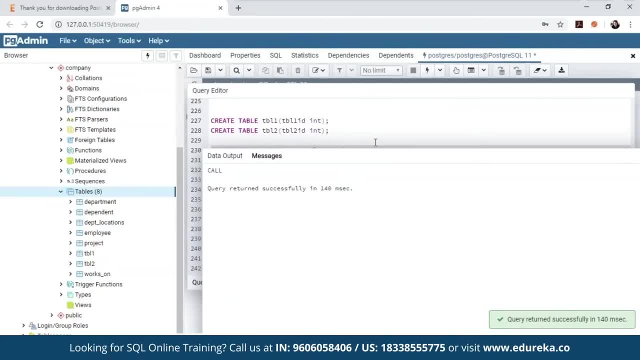 completely. once I execute this particular section completely, you'll see an output at. you know call query has been returned successfully. right now Let's just use the select statement to see whether you know the value has been inserted or not. So let's say I'll mention select star from table 1. 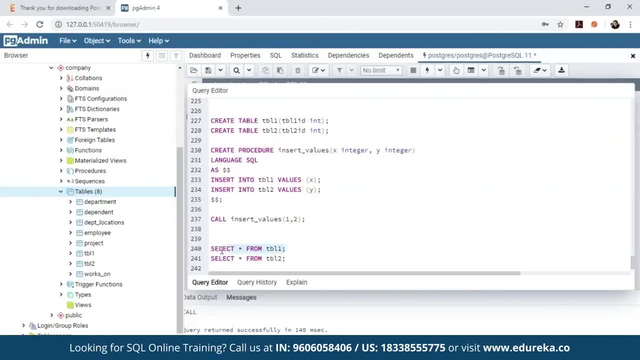 and then, similarly, I'll mention select star from table 2.. So if I just print select star from table 1, you see the value to be 1, right? I hope that you can see now, similarly, if I mentioned select star from table 2,. 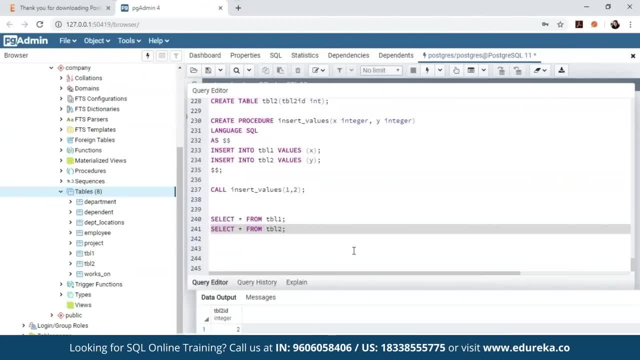 you'll see the value to be 2.. So that means our values have got inserted. So, guys, this is a really simple example. I've just taken two tables with a single column. now you can have any number of columns, and then you can mention any number of columns. 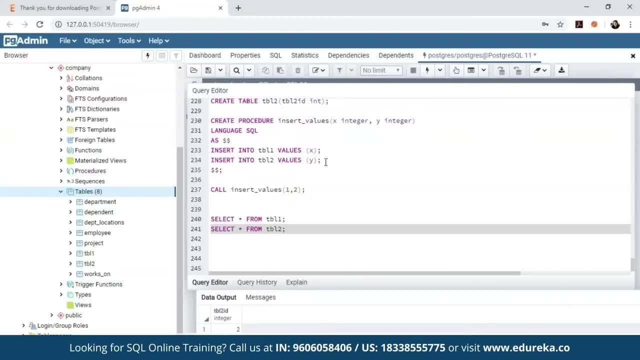 to be present over here. And then you mentioned the specific values into the insert statements And then what you just have to do is you just have to keep changing the values over here. So, for example, let's say, if I do 3, 4 over here again, 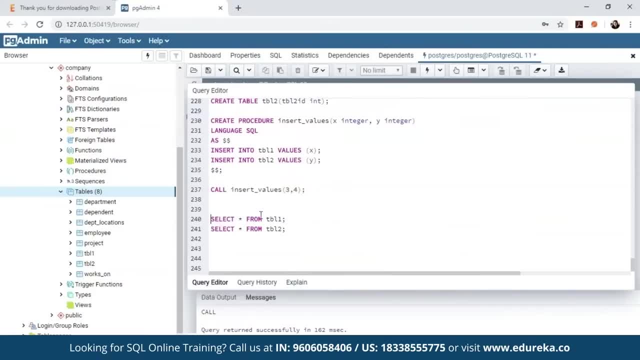 and then I execute the statement call, insert values. and then, let's say, you know, I execute the statement select star from TVL 1.. So you'll see that in a part from one We also have the value 3 now. Similarly, if I do select star from TVL 2,, 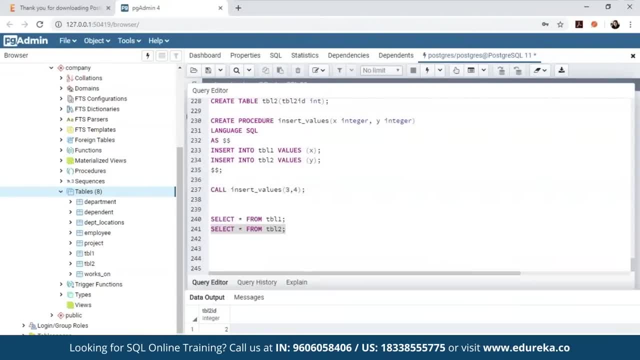 you'll see the output that you know part from 2.. We also have 4.. So that's how, basically, guys, you can create stored procedures. Well, I think it was really simple to understand how you can create procedures and so on right now. 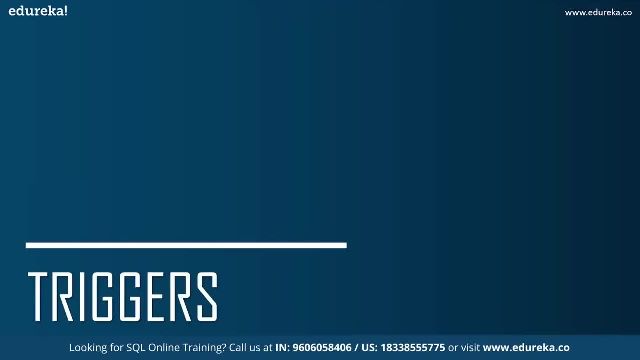 in this session. let's move forward with the next topic, that is, triggers. The triggers are a set of SQL statements which are stored in the database catalog. Now these statements are executed whenever an event associated with the table occurs, So a trigger is basically invoked either before. 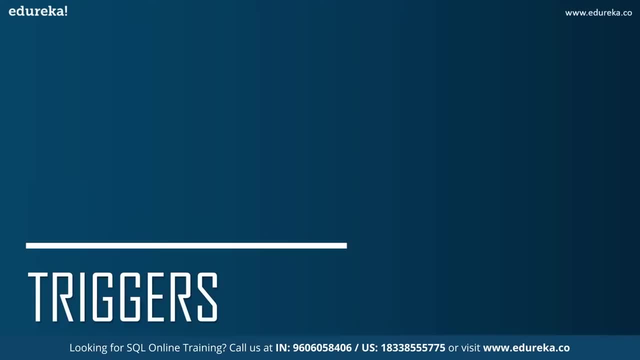 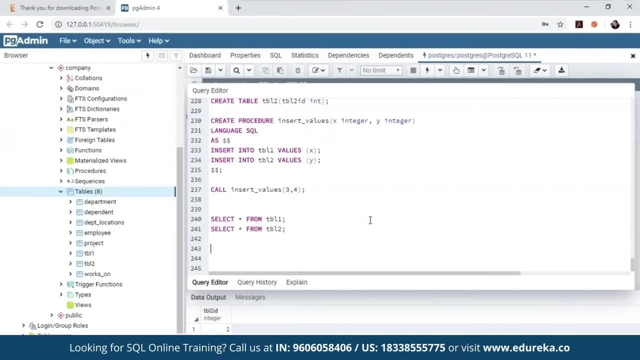 or after the data is changed by either the insert statement, the update statement or the delete statement, and it only invokes whenever there's an event associated with the table. So now let's look into how you can implement triggers in postgresql. So to implement triggers I, what I'm going to do is 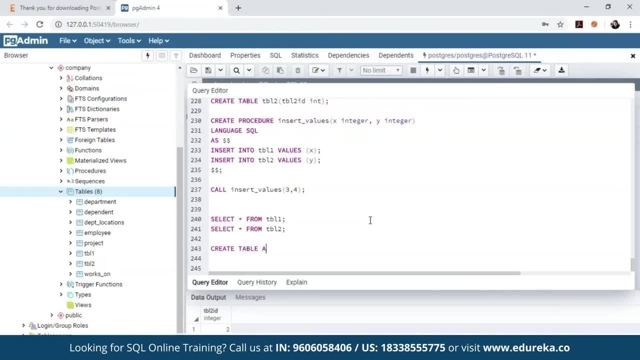 I'm going to create a table for. so let's say I create a table audit. and then let's say: you know, I'm going to consider employee ID right to be of cat type and nine characters, since our SSN is of nine characters, and then it should not be null. 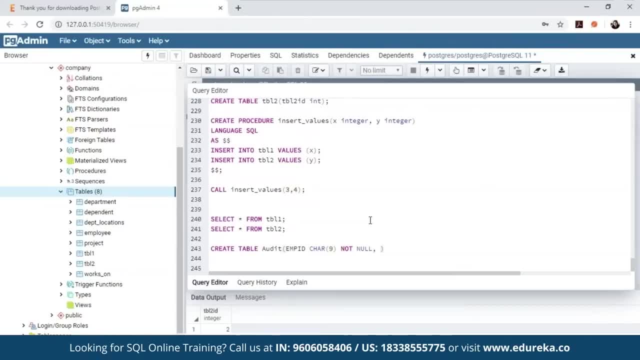 and then, apart from that, I am also going to consider: let's say, you know we have entry date right, Let's say joining date or maybe entry date, and then we have text, it's of text, data type- right, and they should not be any space. 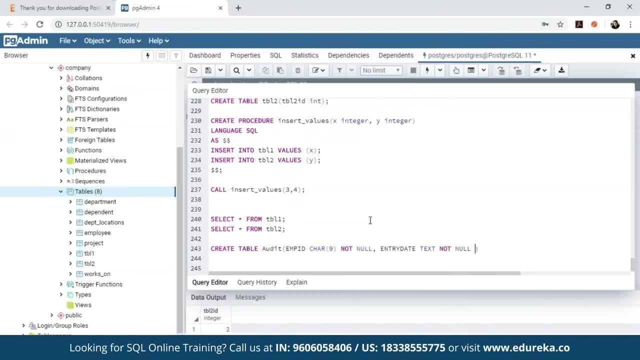 because date is also a data type, and then I'll mention not null. Now what I'm going to do is I'm going to create a function and then I'm going to create a function which returns a trigger as a specific trigger, and then I'll use that particular trigger on the employee table. 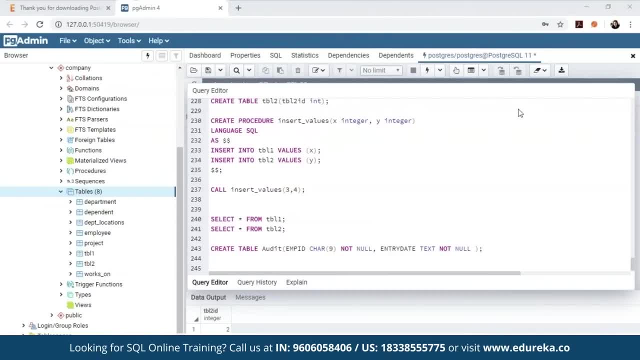 So let's do the same. Now, once I create this table audit, what I'm going to do is I'm going to create a function, audit log function, which will basically return a trigger as example table which will begin whenever you wish to insert something. 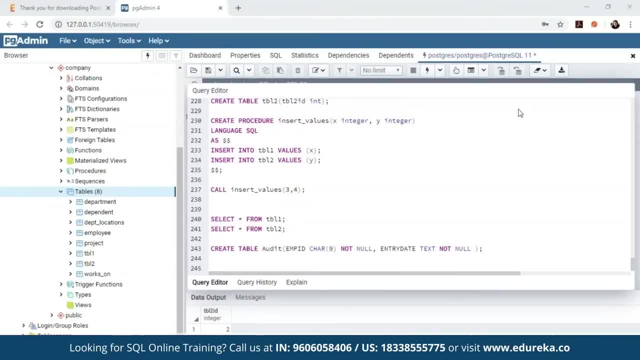 into the audit table Now. the trigger example table will be created then, so let's just do the same. So now, since I've created the table audit, let me create the function right. So to create a function, you have to type in: create or replace function. audit, log function. 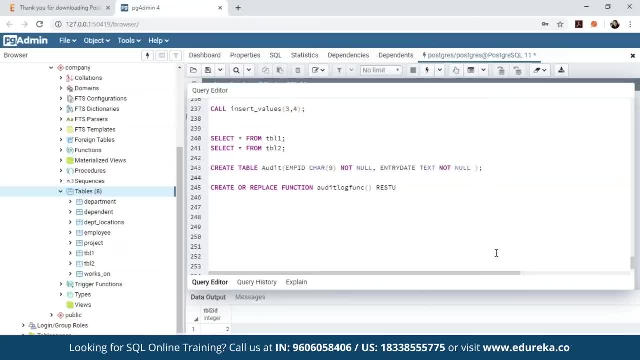 That is basically you know the function name that I'm giving, and then I mentioned returns, Trigger as, and then I'll mention the trigger name- Let it be example: table right- and then I'll mention begin that it will begin then, and then I'll mention insert into audit. 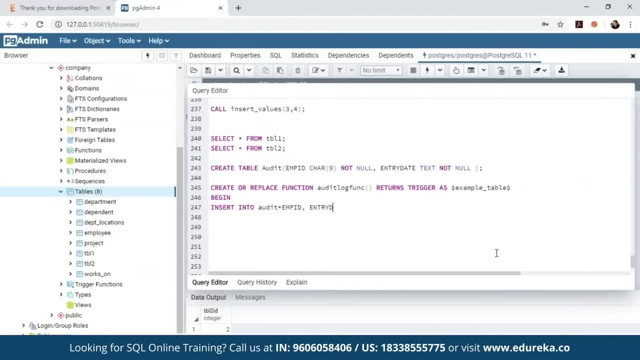 where M ID and entry date will be mentioned and values. It will be new dot SSN. a new SSN will be generated and then automatically the current timestamp will be taken as the entry date. right, So that's how, basically, you can also use timestamps also, guys. 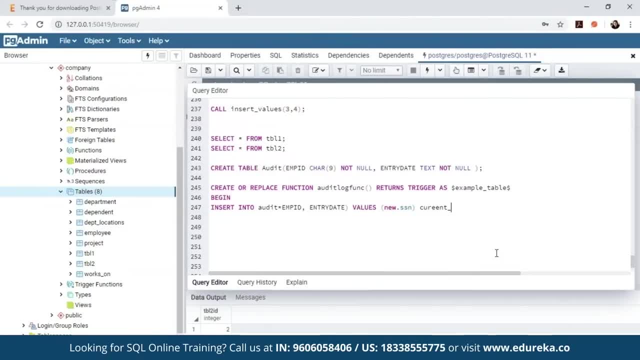 So basically what I'm doing is, whatever is the current time, I'm using that particular current timestamp. So I mentioned timestamp and then what I'll do is I'll mention return, New and then end. So this is basically the function that I'm creating. 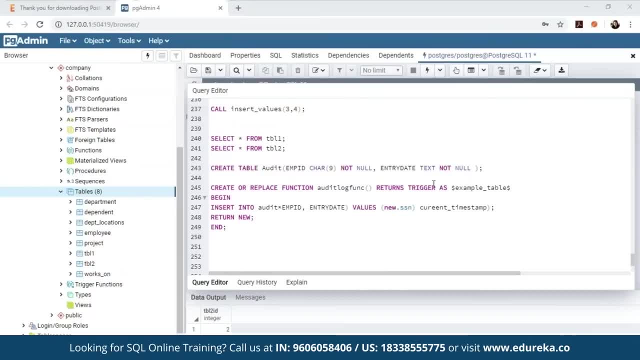 So the function basically says that you know you'll return a trigger as example table whenever you want to insert something into the audit table. Now, as I was talking about the trigger example table, we have to create that also right now. before that, I forgot to mention something over here that is: 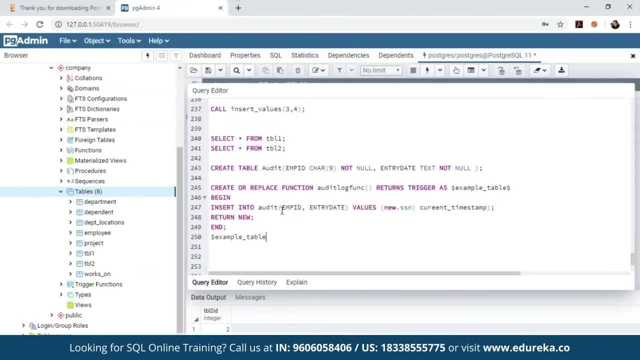 you know you have to mention example table. that is basically in language PSQL, right? So you have to mention that particular fact over here Now. after that, if you wish to create a trigger, you'll mention create trigger, will mention example trigger after insert on, basically whenever you're inserting. 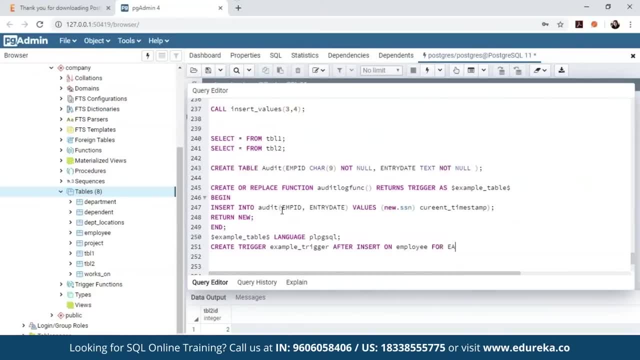 employee. for each row, I'm going to execute the procedure or the function that I just created. So that is basically my audit log function. So I'll just copy from here, paste it over here And then, finally, I'll mention the insert statement. 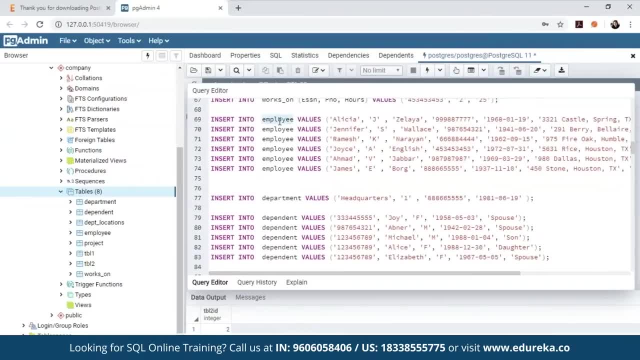 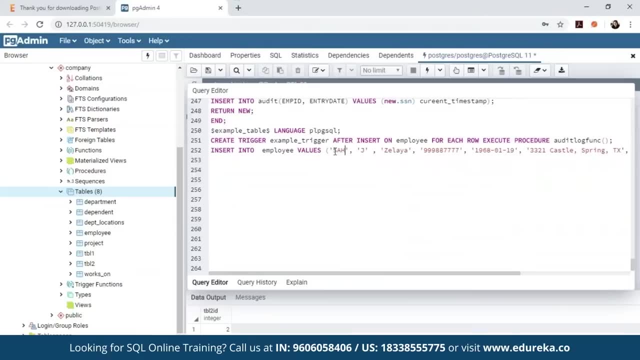 So what I'm going to do is the insert since we are doing on the employee table itself, I'll just copy this particular fact over here. And then what I'll do is I'll paste it over here and let's say, I mentioned sitey the L. 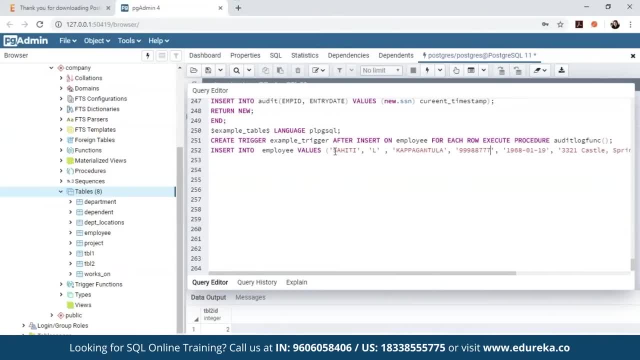 and then I mentioned Kappa Gantula and, let's say, I randomly put in details, Right. and then, let's say, I changed the salary also so that there is no redundancy anywhere, right? So what I've done over here, I've basically created a table audit. 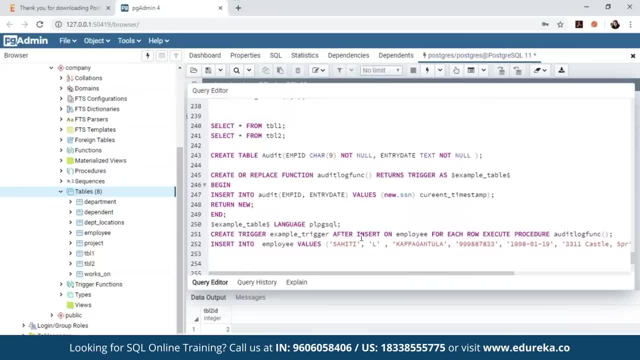 So this audit table is basically, like you know, whenever I want to insert into the employee table, a trigger will be created. So basically, a trigger will be invoked which is: after execute on, you have to mention the procedure, right? So basically, the procedure is basically the function. 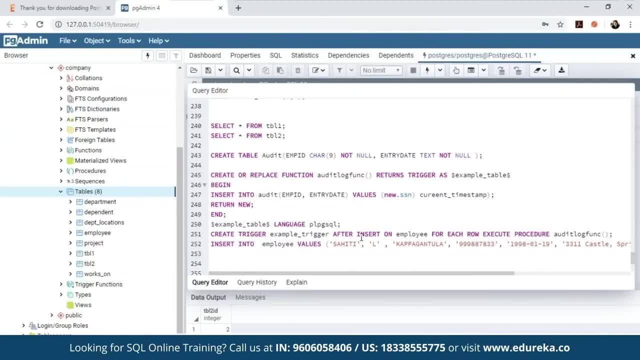 that we created. that's basically. it returns to the trigger example table where you know, it inserts into the order table automatically- that is basically the employee ID that I've mentioned over here- and automatically the current timestamp as the entry date. So let's see what happens. 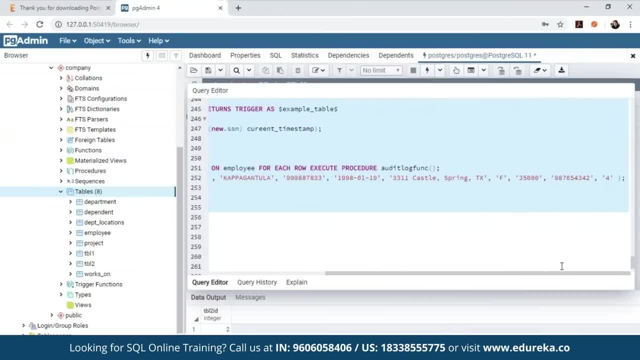 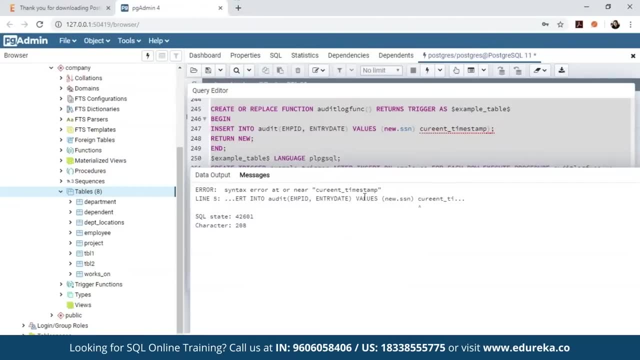 So what I'll do is I'll execute from here to here and let's just check if everything is selected Yes, and then I execute. all right, it says syntax error at employee ID value current. Oh, it's because the current timestamp spelling. 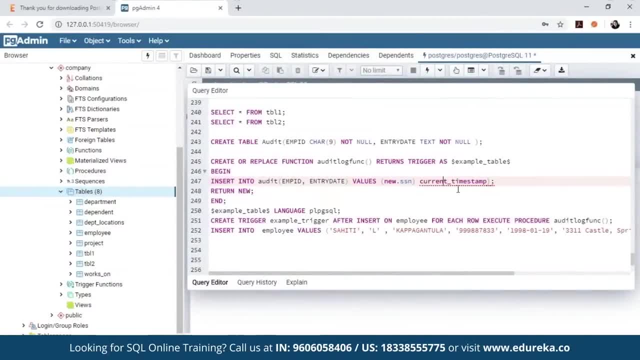 is wrong over there, So let's just correct that. Now I'll again execute this particular section again. It still says that you know there's an error over here. Yes, that's because you know I've missed comma over here, and then I'd put the point. 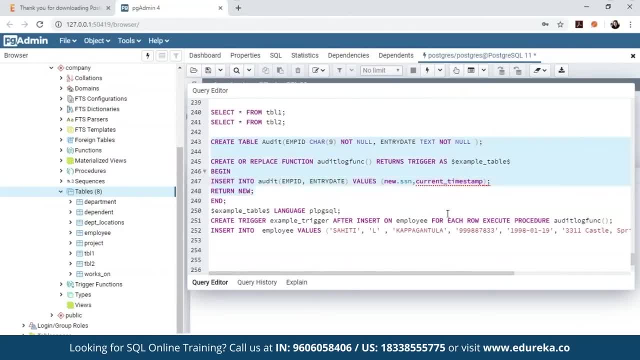 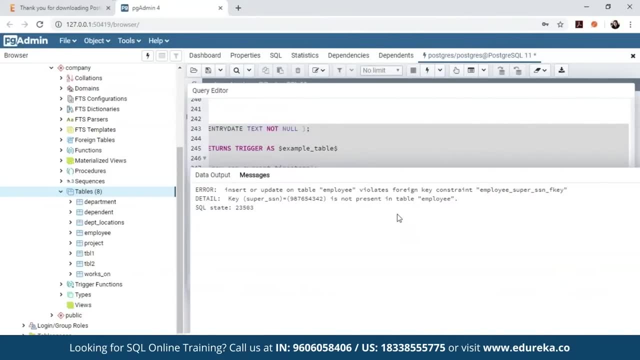 in the bracket. So I've removed the brackets and then I have to put the comma, and then again let's try executing this particular section. It says that you know the key super SSN is not present in the table. employee right. 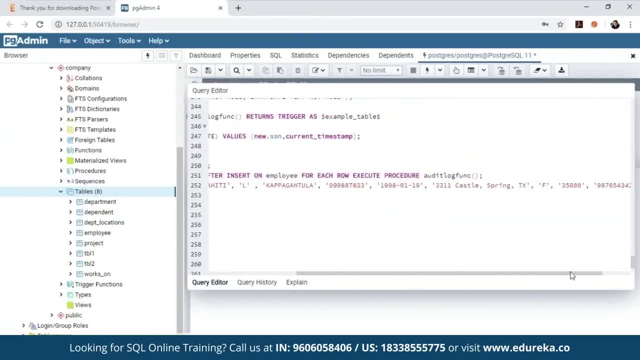 So that's because we cannot randomly do and we have foreign keys present. So let's just randomly choose any super SSN. Let's say: triple three, double four, four times five, right, And now I'll go back. and now let's execute again. 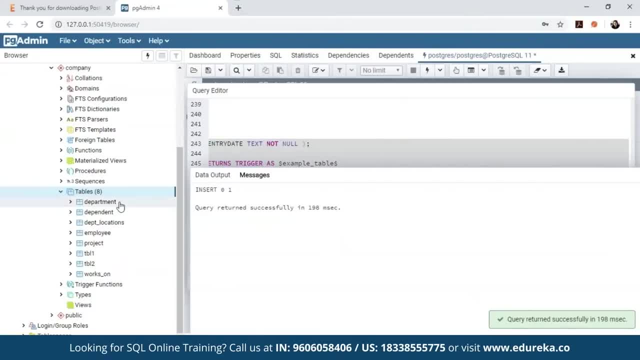 Once I execute again, you can clearly see an output that you know query returned successfully, right? So let me just refresh tables and let me just refresh triggers. So once I refresh tables, you'll see that you know there's an employee table. 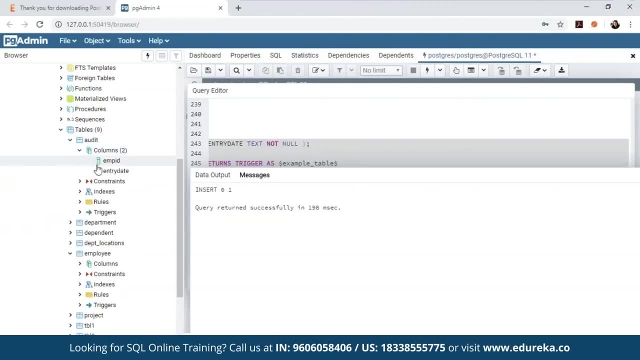 and then we also see there's an audit table and the order table has the columns employee ID and entry date right, And then we have a trigger function which says audit log function is basically the trigger function that we just created. Now, if I wanted to see the data from the audit table, 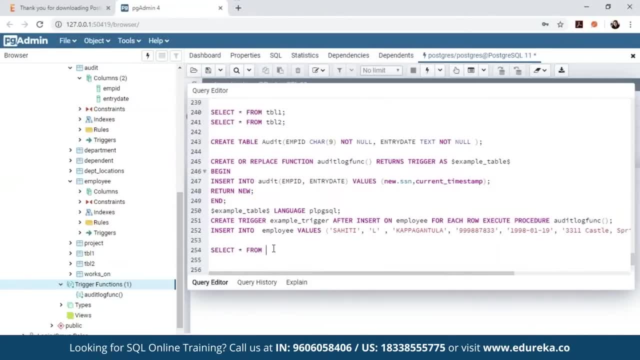 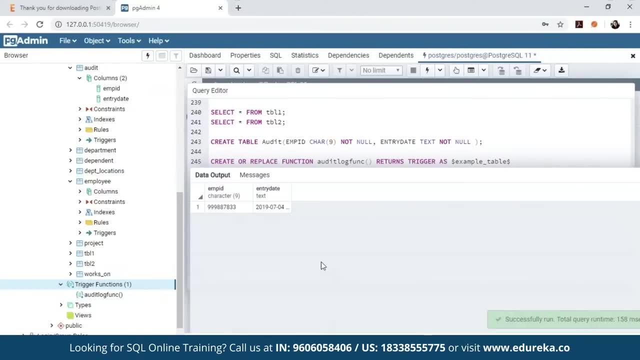 I'll just choose select star from audit And then you'll see automatically the employee ID and the date, which is basically the current time, is generated. So that's how, guys, basically you can use triggers. So with this we come to an end of the data manipulation commands. 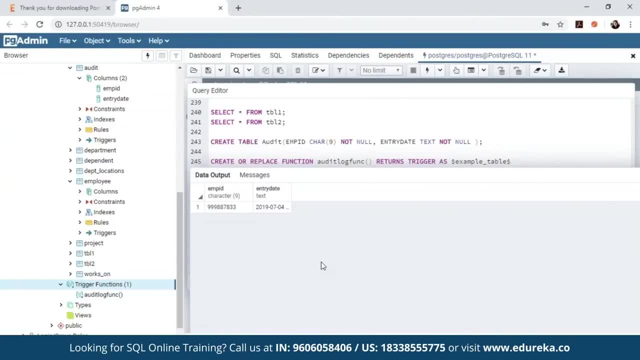 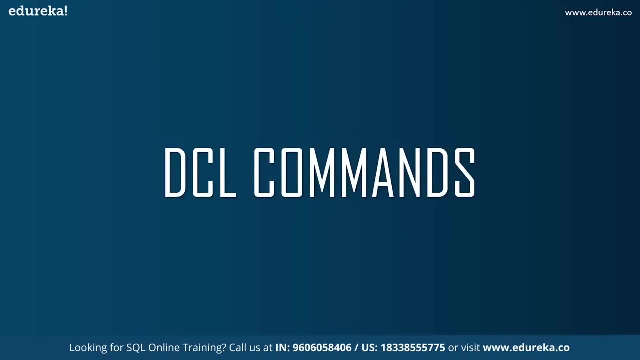 I hope you've understood all the commands in the syntax is and the statements that I just showed you. Now let's move forward with the next set of statements, That is, the data control language commands. The data control language commands, as I previously mentioned in the starting of the session. 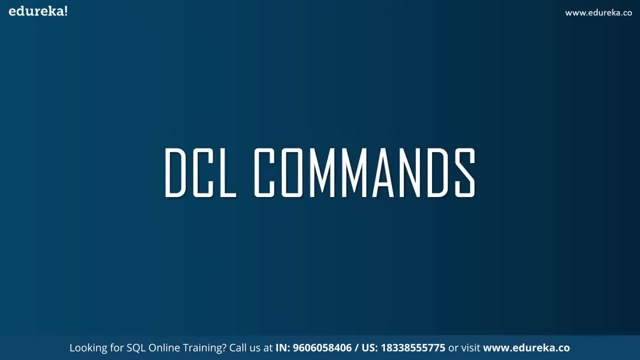 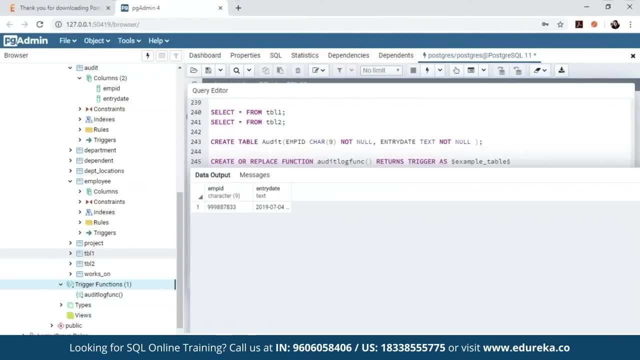 is basically used to provide rights and privileges to the users to access database views, tables and so on. So, basically, there are only two statements that you need to understand in this particular section, that is, the grant statement and the revoke statement. So let's consider the grand statement. 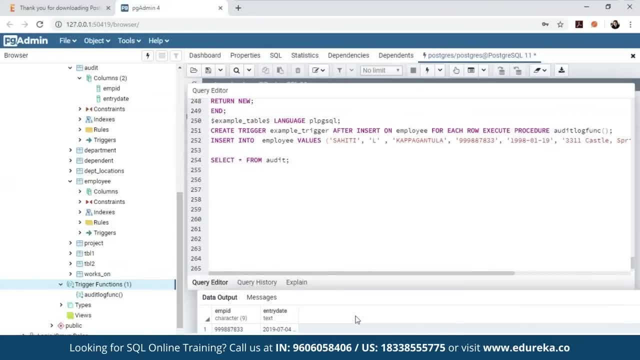 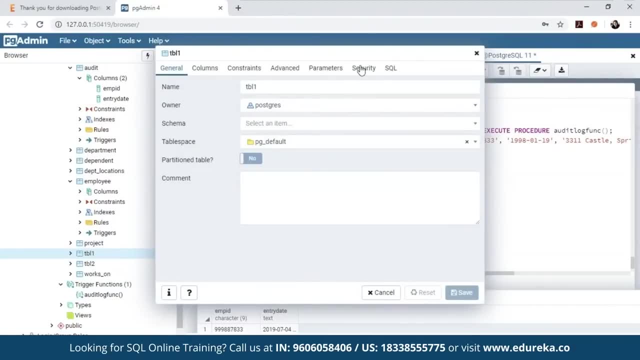 So the grand command is basically used to grant privileges to the databases or tables. For example, let's say, you know we consider the table one we created over here. So if I right-click over here and go to properties and let's say I go to securities, you see that. 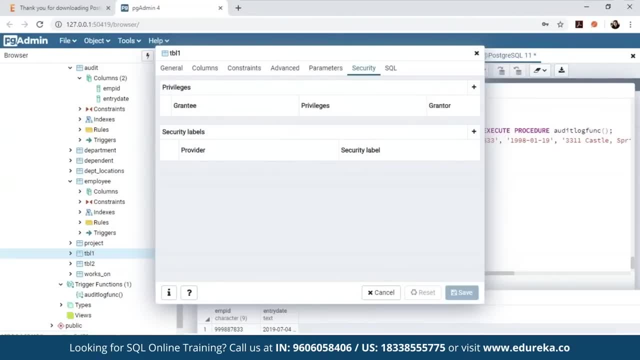 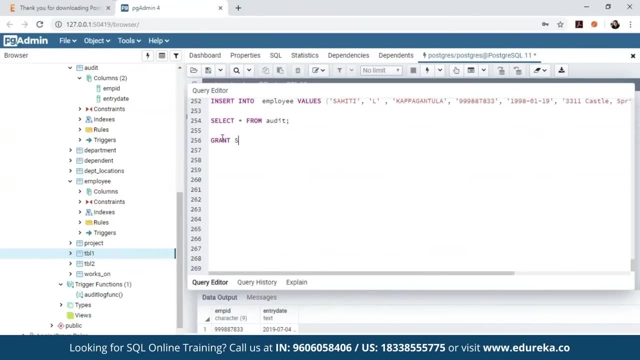 you know, there's no grantee privileges- There's nothing present over here- because there are no privileges granted to this particular table. So let's grant permissions to this particular table. So what I'm going to do is I'm going to type in Grant select. 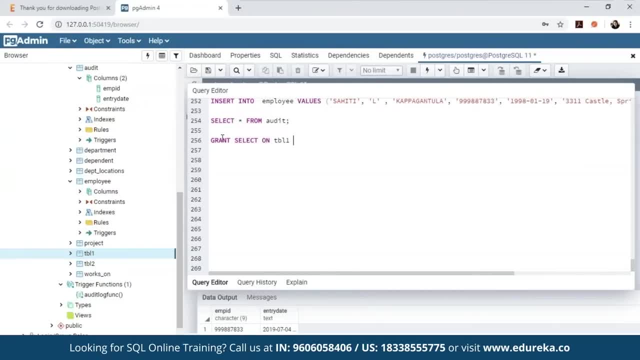 on and mention the table name, that is, table one, two, and I'll mention public, and then I'll just execute this particular query. You'll see that you know the query has been returned successfully. And now what I'll do is I'll right-click over here go. 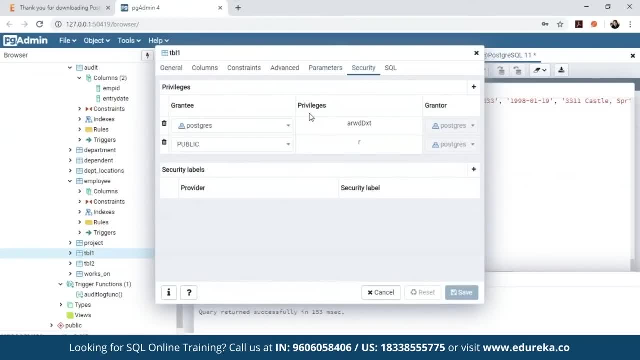 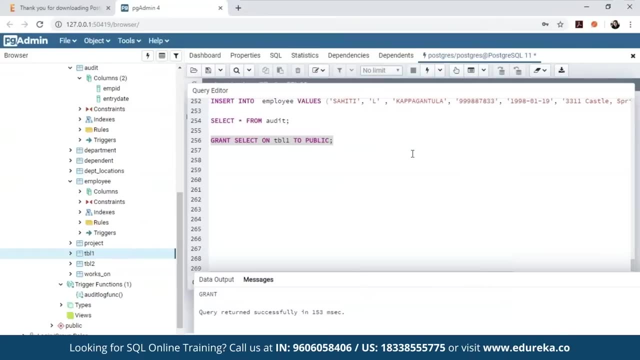 to properties and then go to parameters and then go to security over here, And then you'll see that you know automatically we have granted a public privilege to this particular table. Now let's say, you know we want to grant privileges on, basically, the command insert. 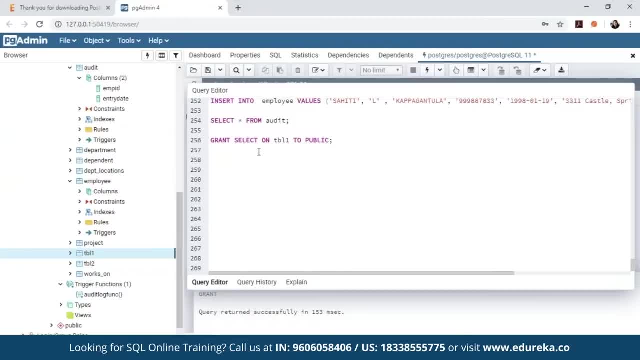 on right. So whenever there's some insert on, we want to grant privileges to the public So anybody can insert into this particular table. Now let's say: you know we want to grant insert on privileges to the employee table right. 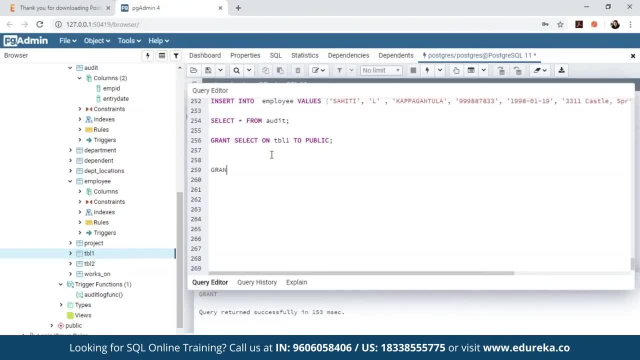 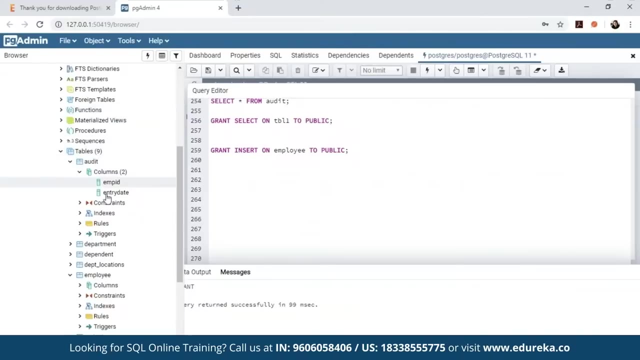 So basically anybody can insert into this particular table. So that is basically Grant insert on employee to public. If I just execute, you'll see the output of query return successfully, right. So now what I'll do is I'll just go to my employee table over here. 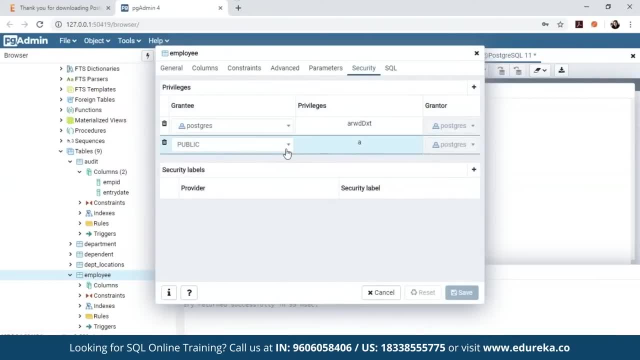 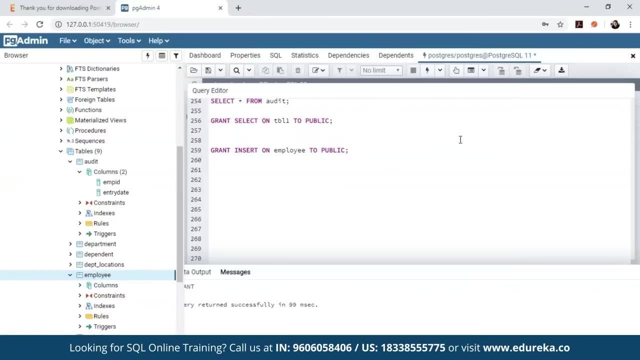 Go to properties, go to security, and you'll see public, and then you'll see a privileges of a right, basically all. so that's how, basically, you can grant privileges, guys. Now you can also revoke back your privileges, Let's say, you know? 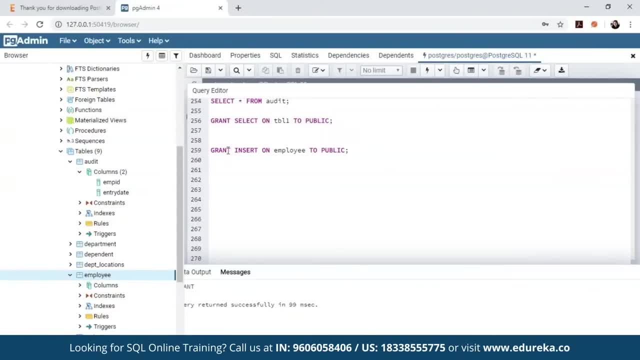 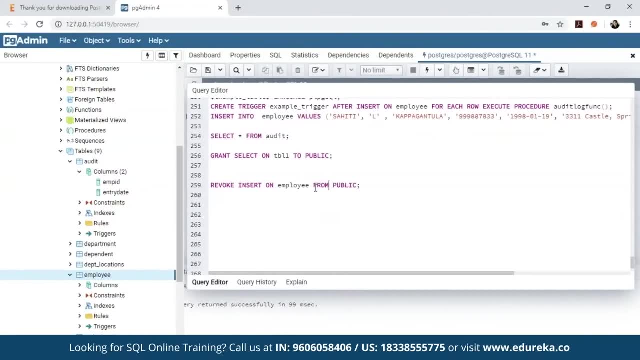 you want to revoke back the privilege that you just gave. So for that you just have to use the statement revoke right, So you'll type in revoke insert on employee, And then instead of two you'll mention from. so you'll mention revoke insert on employee from public right. 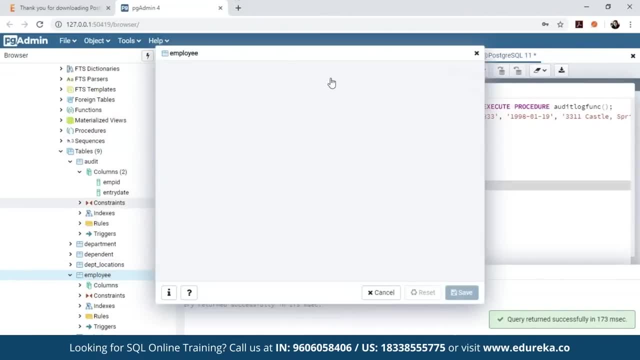 So you'll just execute this particular query and then we'll go to properties again over here, go to security, and then you'll see that you know there's no more public privilege present over here. So, guys, that's all. basically, you can control privileges. 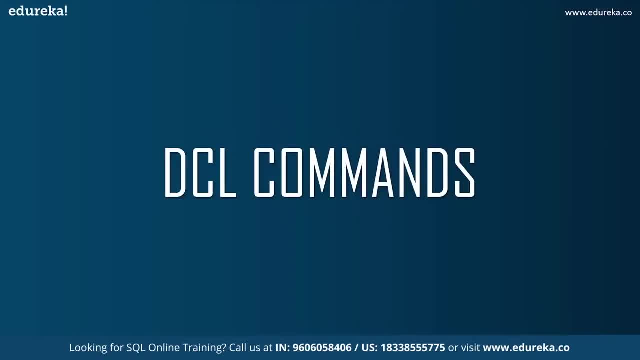 and rights for your databases and tables. So, guys, that was about data control language commands. Now, moving forward, the next type of commands that we have is the transaction control language commands. So the transaction control language commands come into the picture when you want to make sure that you know. 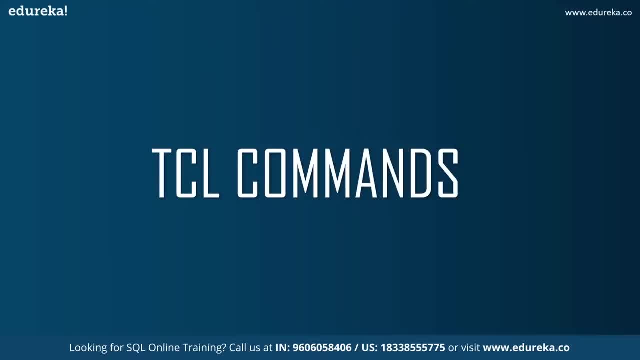 the transaction in the database is meeting all the standards. that is basically the asset properties. So asset properties are basically atomicity, consistency, isolation and durability. So basically, if you want to make sure that you know the database is making sure that the transaction properties are met, then you have. 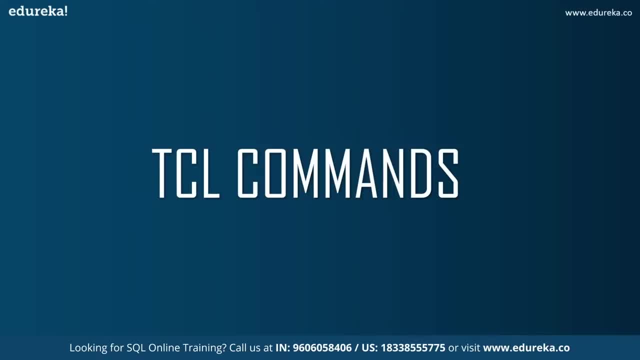 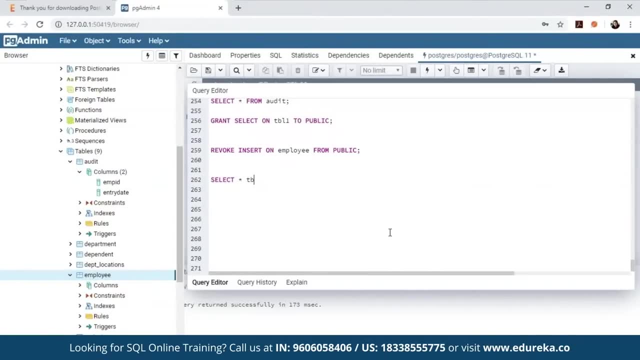 to use this transaction control language commands. So to use transaction language control commands. what I'm going to do is I'm going to perform transaction on table one, right? So let me just see what values are present in table one. So let me just see. 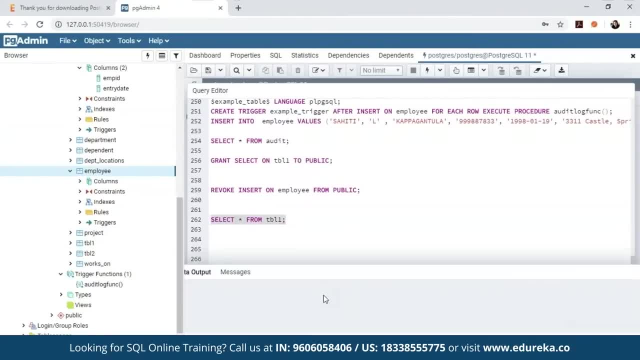 I forgot to mention from over here. So it's select star from table one and then you see one three. right Now, what I'm going to do is I'm going to insert around values till 10.. So let's insert all the other values. 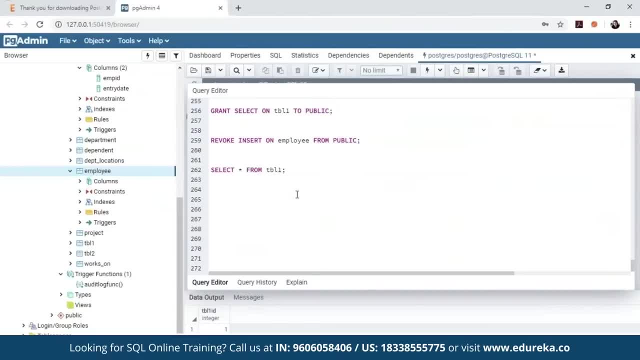 I'm just going to copy it from my dog over here. So, since I have already one and three values present over here, what I'm going to do is I'm not going to insert these values, So I just remove these and then I'll just execute them, right? 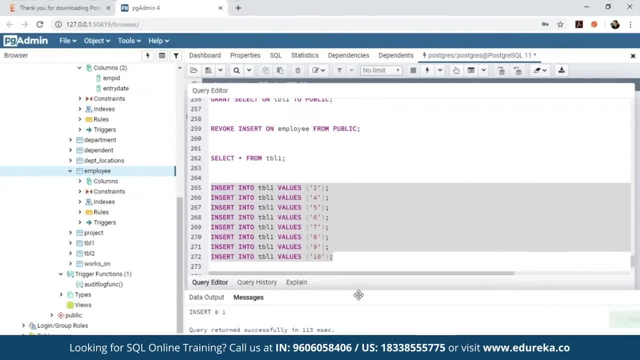 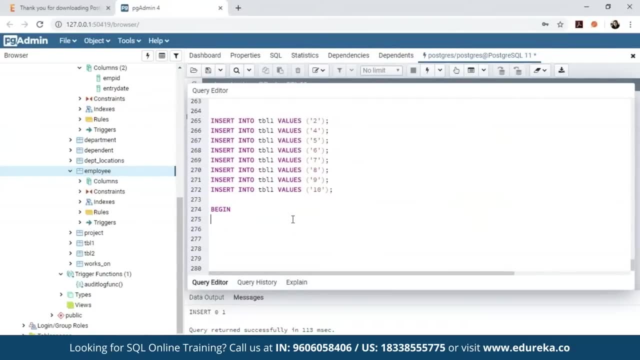 So you'll see that you know. data has been inserted into my table. Now let's begin a transaction. when I say begin a transaction, you have to use the syntax known as begin, So you'll type in begin and then let's say: you know. 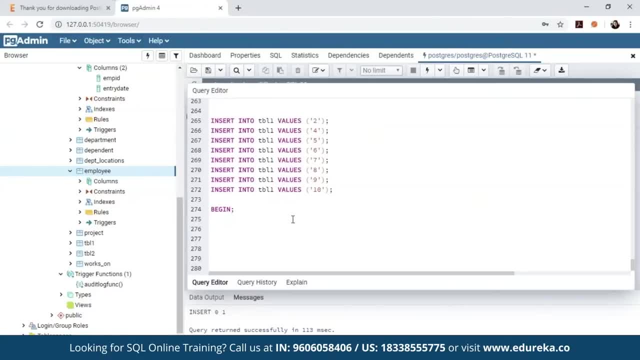 we want to delete all the values which have the ID greater than five, right? So basically, all the couple values which have the ID greater than five have to be deleted. So for that we are initializing a transaction and then I'll mention delete from and table one. 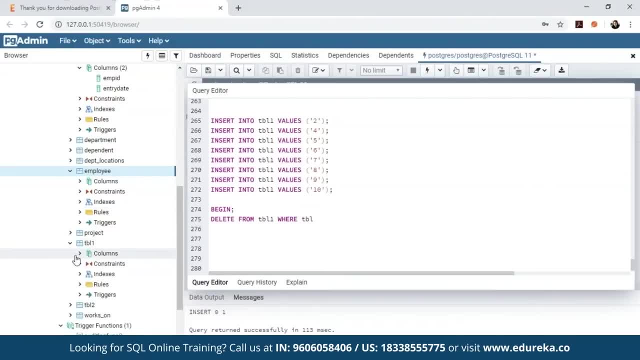 where table one ID. So let me just check the column name, That's tbl1 ID is greater than five. So I'll mention begin. So basically my transaction will begin and then what I'll do is I'll delete. So let's just do that, right. 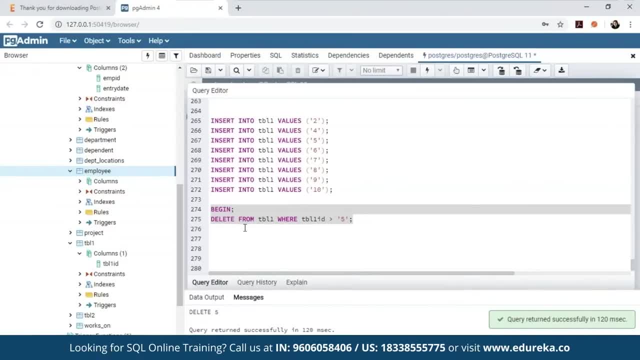 So you can see that you know the transaction is running on, and then we have deleted till five. Now let's say, you know, if I want to roll back, roll back is basically I don't want it to occur, right? So when I hit on roll back, 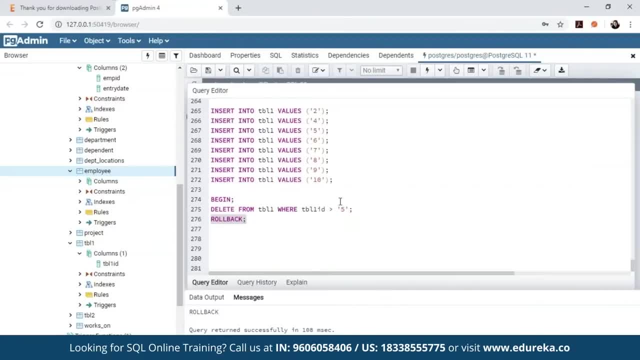 you'll see that you know, automatically all the 10 values will come back right. So if I just use the syntax of select star from table one, you'll see the output of 1 to 10 again. So what you should understand from over here is basically: 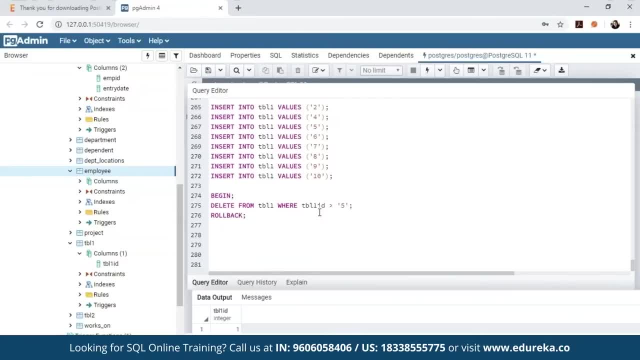 that you know, the begin is basically used to begin the transaction and the rollback is basically used to roll back from the previous transaction. So we are. what I've done is that I started a transaction and then I deleted the values greater than five, So all the values got deleted. 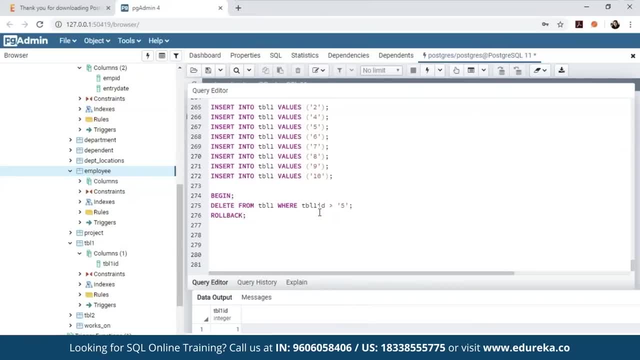 Now, when I hit on roll back, what happened is that you know the transaction got rolled back and automatically all the values got retrieved. So that's how, basically, you can do roll back now. Similarly, you can do commit right. So what I can do now 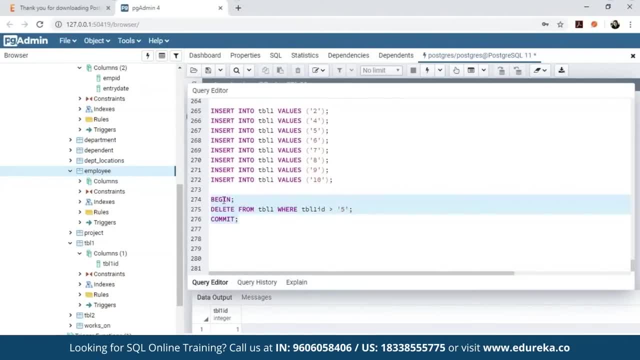 is, I can type on commit over here and then I can begin a transaction again, right? So once I begin a transaction again and once I delete all the values greater than five, and then when I hit on commit, you cannot roll back, right? So all the values will be deleted, whose ideas will be greater. 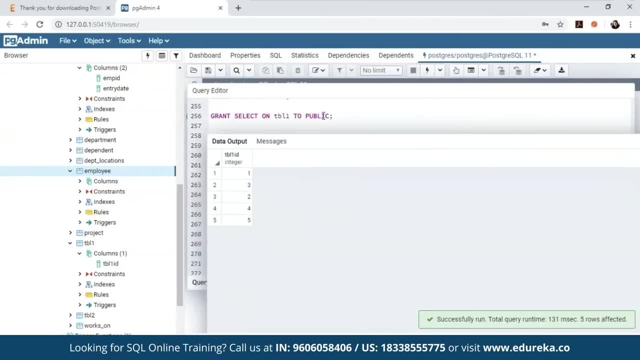 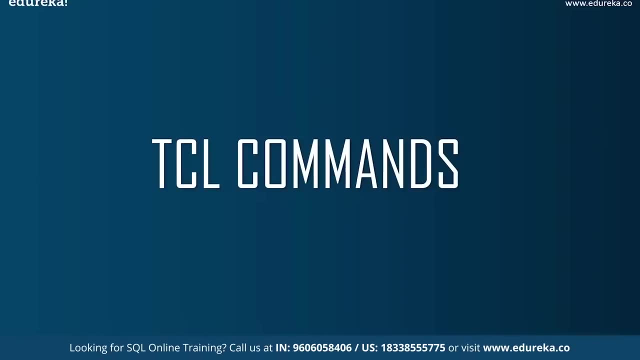 than five. So if I just execute this particular statement, you'll see that you know you only have one to five values, the. similarly you can also about the transaction using the statement aboard. So, guys, that was all about transaction language control commands. Now let's move forward with the next topic. 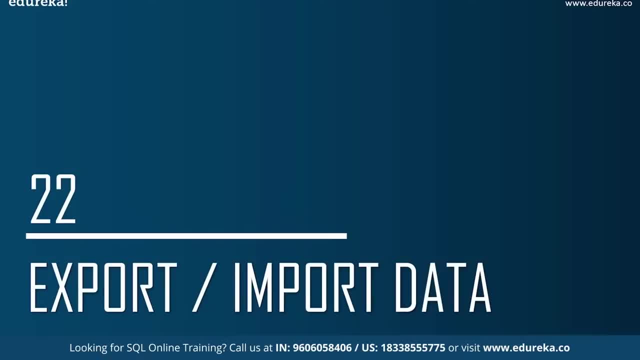 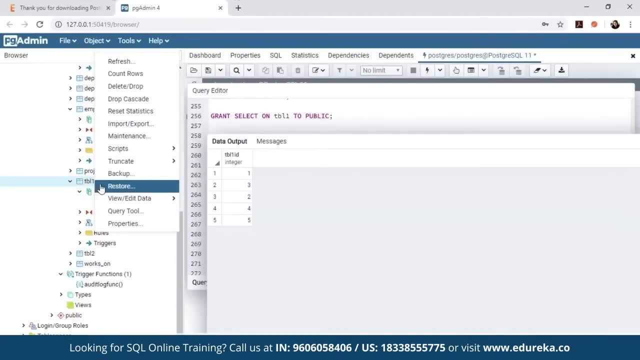 That is how you can export and import data. Well guys, exporting and importing data is really simple. For example, let's say you know I want to export and import data of the table one values, right? So what I'll do is I'll right click over here. 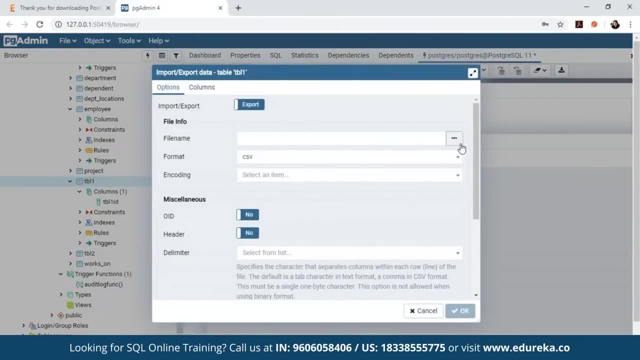 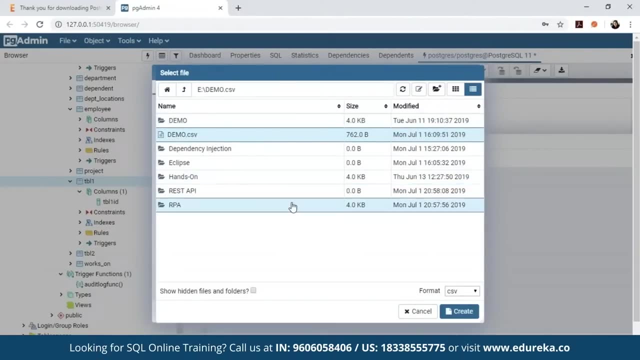 and then go to import, export option, And then what I'll do is I'll mention the file name, right? So basically I'm exporting and I'll search for, let's say, democsv, right? So now democsv is present in my e folder, right? 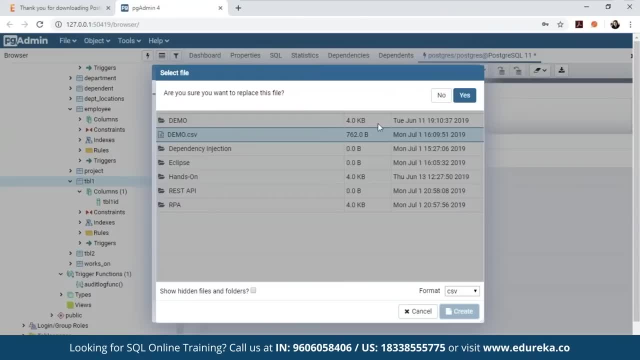 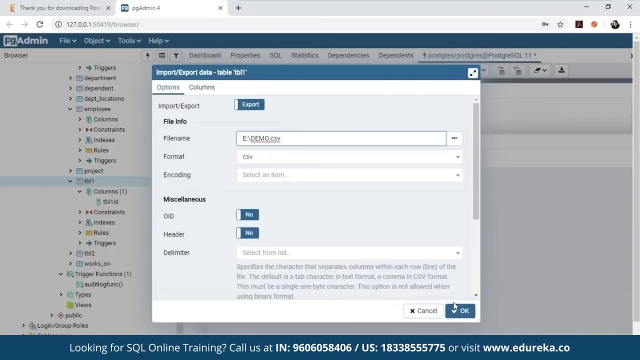 I'll choose that, and then I'll click on create. once I click on create, You'll see that. you know, if I want to replace, well, I have a pre-existing file, So I'm just allowing it to replace. well, you can do that, right, and then you'll click on. 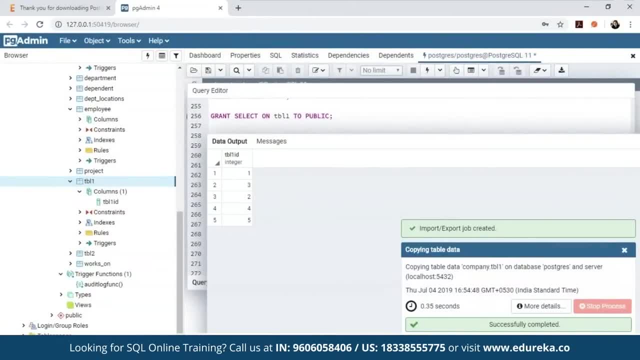 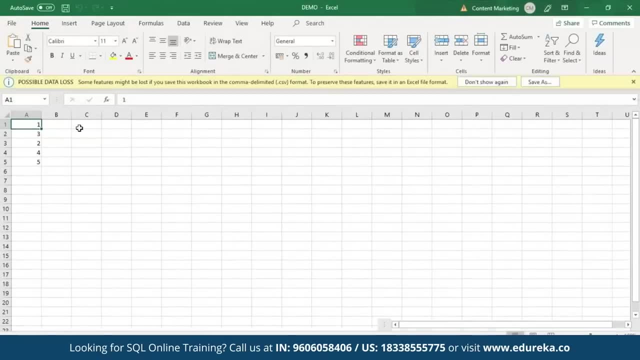 Okay. once you click on okay, you'll automatically see that you know the details have been copied right. So what I'll do is I'll go over here, go to e folder- mine- and go to democsv. So in the democsv you can see that you know. 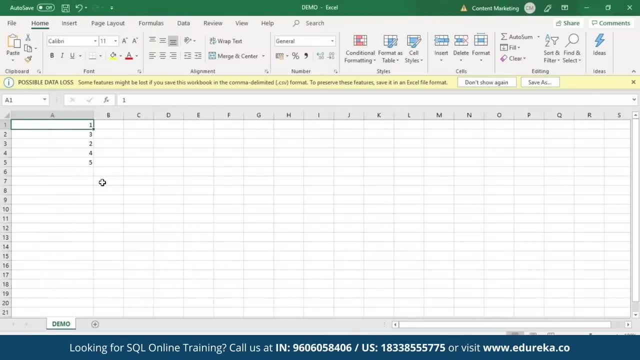 we've got the data one to five, because we just had one row column that is one to five and we just deleted the other values. So that's how, guys, basically you can also export and import data. It's really simple in pg-admin. now, finally, coming to the final topic, 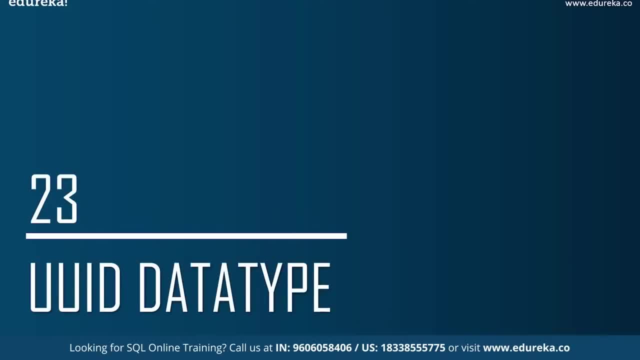 for today's session. That is, the UU ID data type. Now, the UU ID data type is basically the data type which is based to uniquely identify a particular value right. For example, as I was talking in employee, I said SSN right. 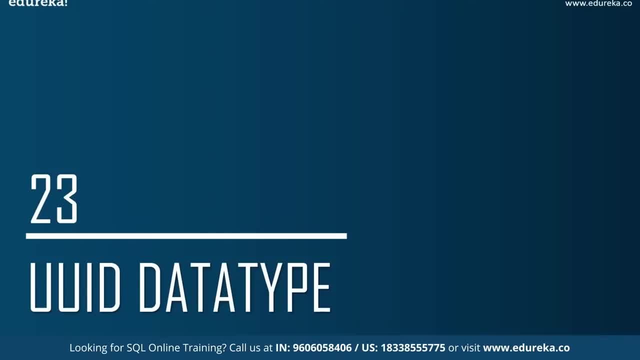 So for every value I had to insert an SSN. basically I had to insert an value. Maybe, if you don't want to do it, what you can do is you can just directly use this particular extension and then you can directly use that particular value. 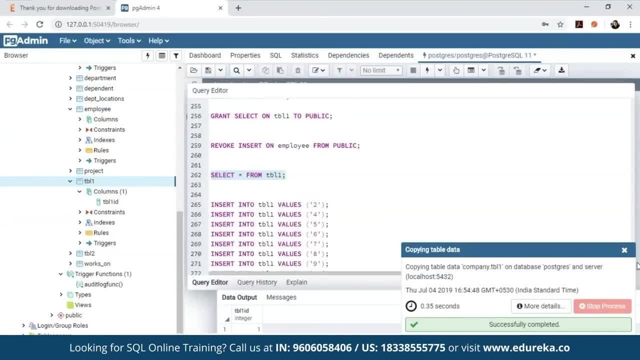 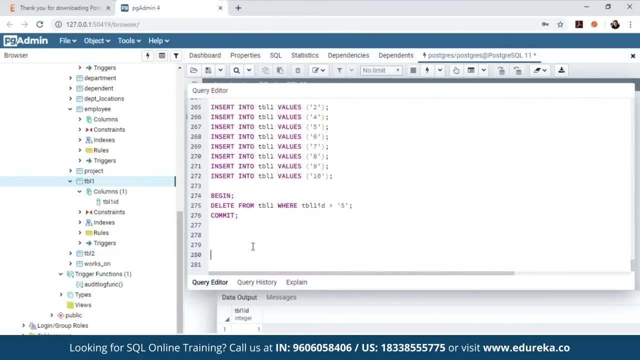 So now let me just shift back to my pg-admin. Now let me close this particular part, Let me scroll back and now let's say: you know, we want to see first What are the available extensions, right? So I'll just type in select star. 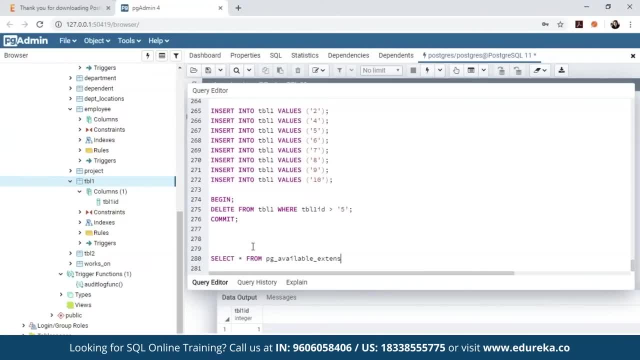 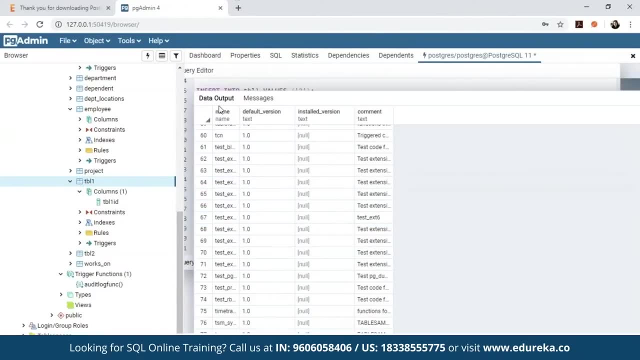 from PG hyphen available extensions. So I'll mention this and I'll click on execute. Once I click on execute, you'll see that you know we have name, we have default value, We have installed version and we have comment right. 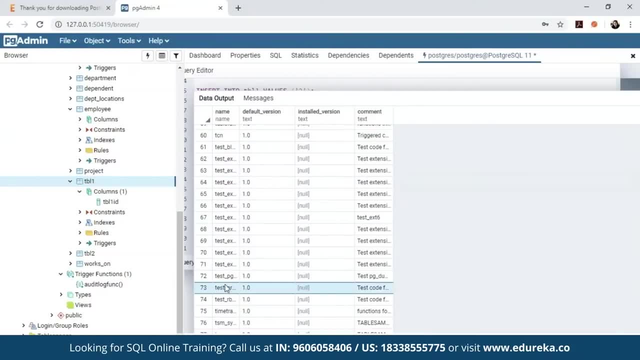 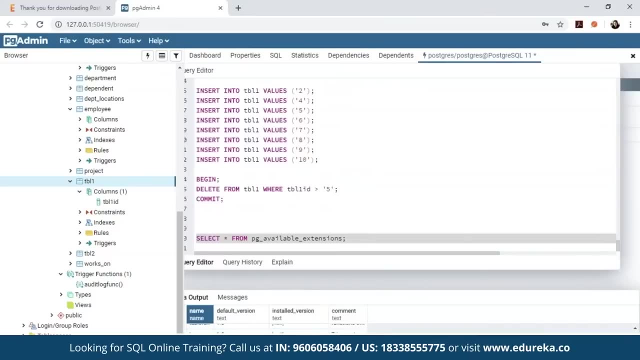 So we have a lot of available extensions, But what I want to use is the UU ID OSP right. So if I scroll down more, you'll see this particular one right. that is UU ID OSP. That's what we want to use over here. 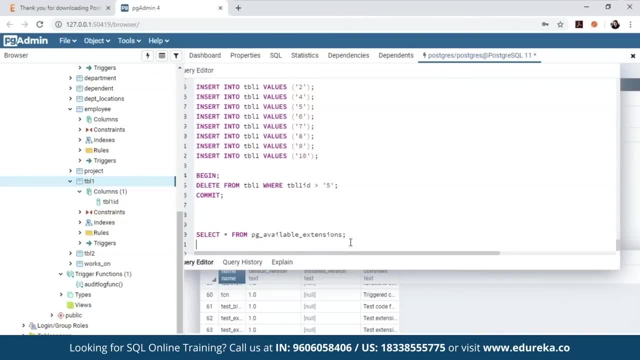 So initially, if you know, if you do not have this extension, what you can do is you can just create this extension. So you'll type in create extension and mention if not exists, and then you'll mention UU ID, hyphen, OSP. So this has to be in single quotes. 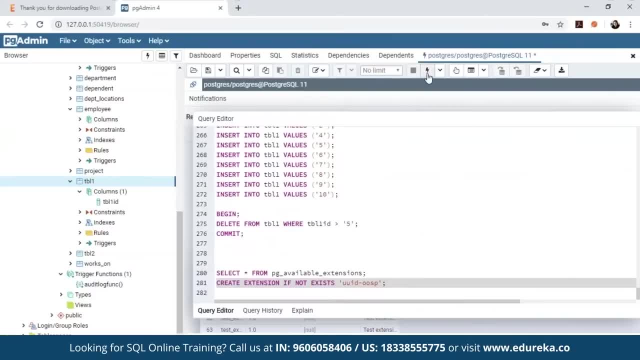 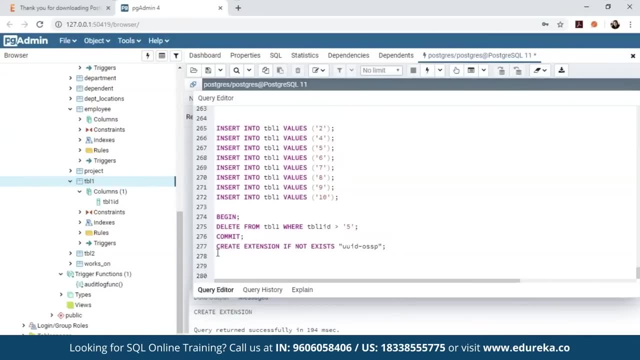 and then you'll just execute this. So let me just execute this by dragging this down. So it says it's not fine. Oh yes, It has to be in double quotes itself. That was my bad. So when you create extension, if not exists UU ID, OSP. 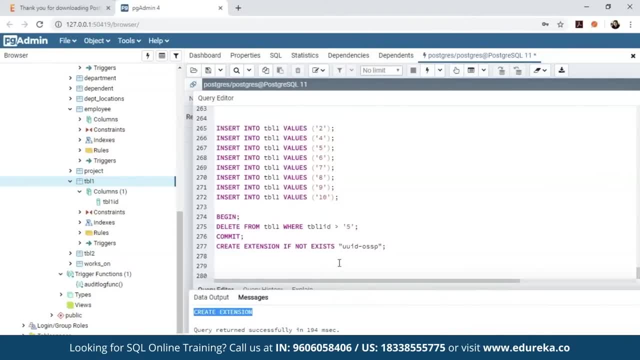 you see an output of: you know, create extension. Now what you can do is you can just directly select from the available extensions. Now, once I create the extension and then, if I select UU ID generate before, you'll see that you know, automatically a new ID is getting generated. 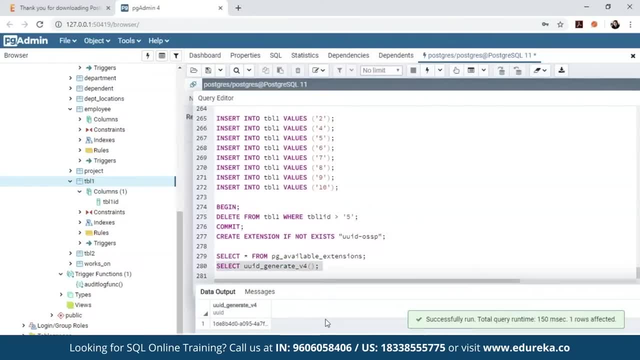 right Now. the next time I execute this particular statement again, you'll see that you know a different ID will be generated. So that's how, basically, you can use UU ID as a primary key for the table. So, for example, in the social security number. 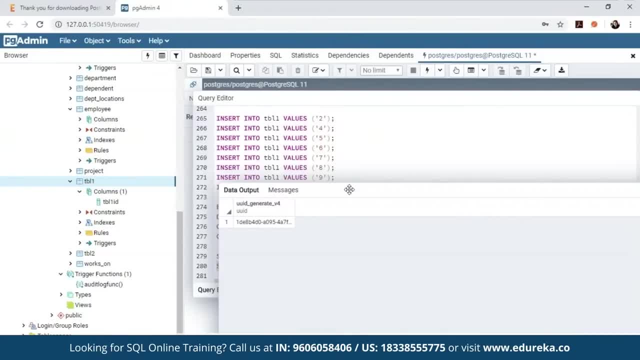 of employee table. you could have using this now. in that scenario you don't have to sit and mention the SSN over there. You can just put the specific function, that is, UU ID underscore, generate underscore v4, and automatically you'll see that you know. 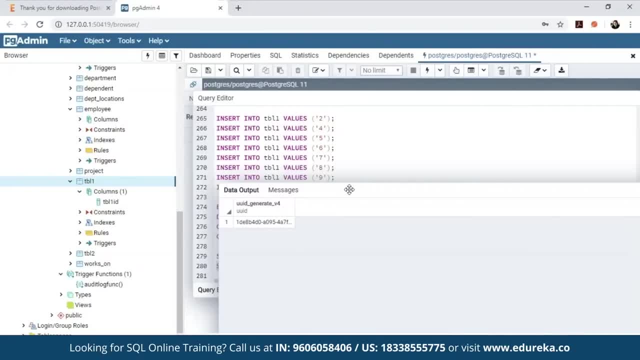 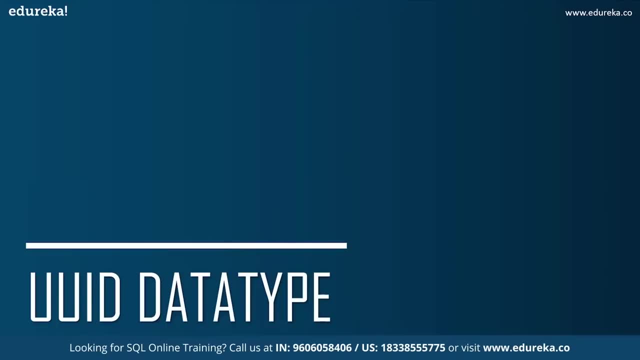 every time you hit the query, you'll see a new ID will be generated, right? So, guys, that was all about UU ID data type. Now you can use UU ID data type as a primary key to uniquely identify your data type. What is database management system? 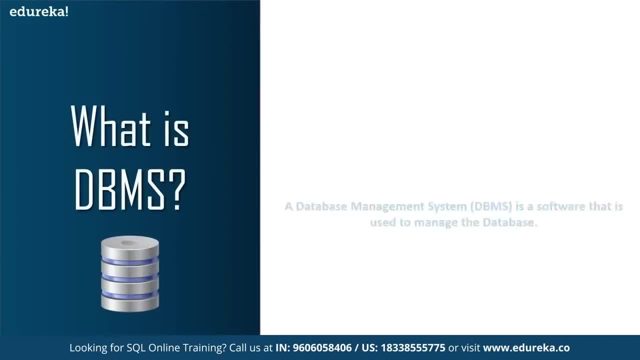 and what are its different types. database management system, or most commonly known as DBMS, is a software application used to access, create and manage databases. with the help of DBMS, You can easily create, retrieve and update data in the databases. a DBMS consists of a group of commands. 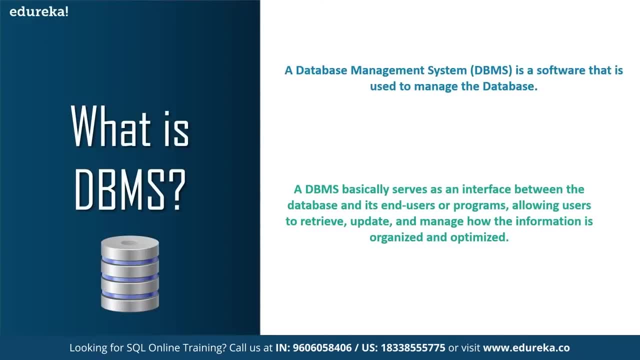 to manipulate the database and also access an interface between the end users of the database. So if I have to just summarize DBMS for you, then DBMS allows the users to define the data, to update the data, to retrieve the data and also for the administration of the users. 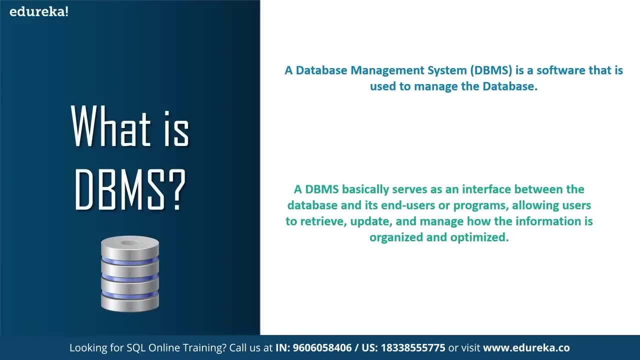 when I say define the data, it allows the users to create, modify and delete the definitions which define the organization of the database. when I say update the data, what I mean by that is that it provides access to the users to insert, modify and delete the data from the database. coming to retrieve data: 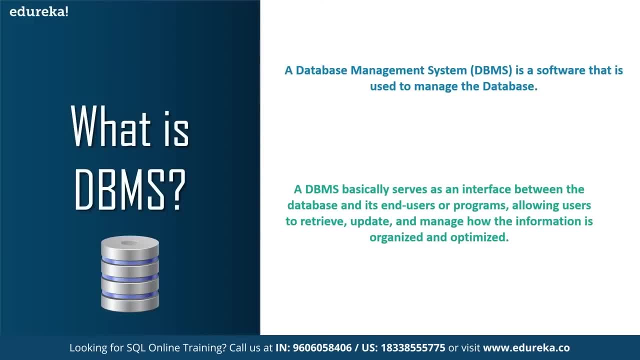 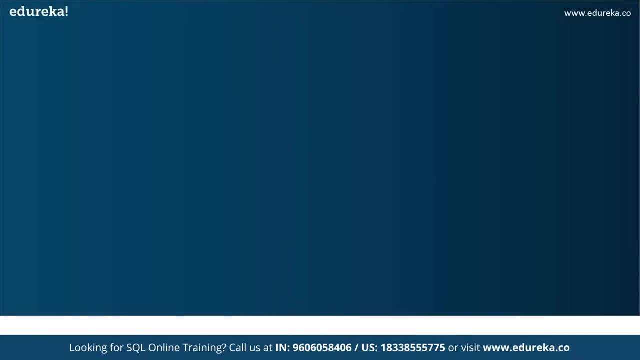 It allows the users to retrieve the data from the database based on the requirement. and, finally, coming to administration of users, It registers the users and monitors their action and enforces data security, maintains data Integrity, monitors performance and deals with the concurrency control. So, guys, that was about DBMS. 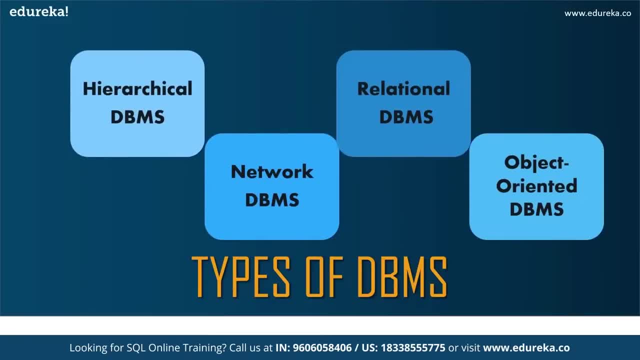 Now, there are mainly four types of DBMS, that is, the hierarchical DBMS, the network DBMS, the relational DBMS and the object-oriented DBMS. talking about the hierarchical one, as the name suggests, this type of database management system showcases a style of predecessor and successor type of relationship. 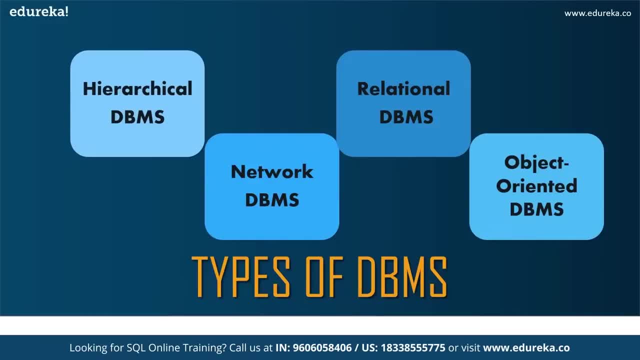 So you can consider it to be similar to a tree, where in the nodes of the tree represent the records and the branches of the tree represent the fields. coming to relational database management system, This type of database management system has a structure which allows the users to identify and access the data. 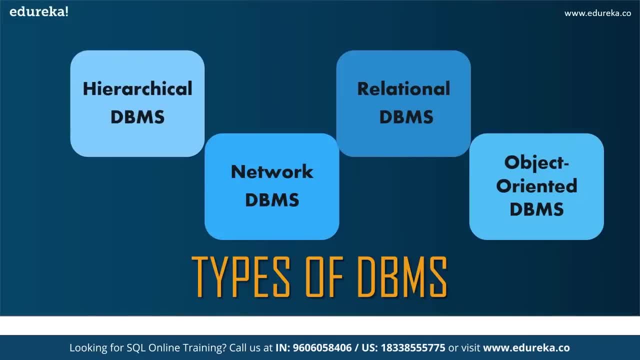 and relation to another piece of data in the database. in this type of database management system The data is stored in the form of the tables. coming to the network database management system. The network database management system supports the many to many relationships where in multiple user records can be linked. 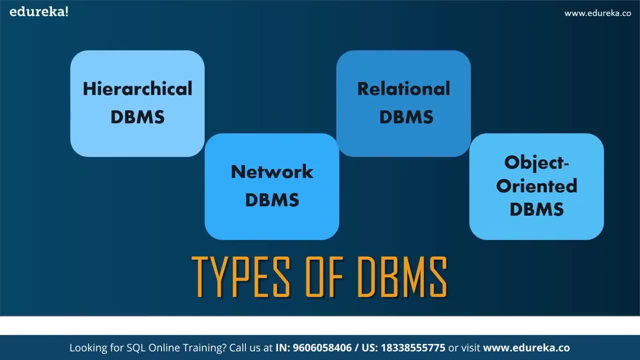 And finally, coming to object-oriented database management system, this type of database management system uses small, individual softwares called objects, and here each object contains a piece of data and the instructions for the actions to be done with the data. So, if you ask me, if you popular database management software's? 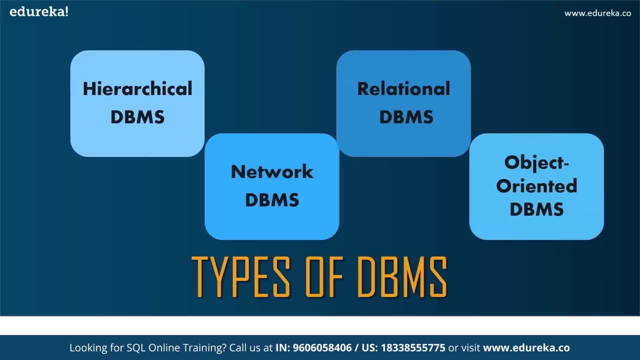 then they are my sequel: PostgreSQL, Oracle, SQLite, MariaDB and Microsoft SQL Server. Now, all these softwares are based on different types of database management systems available in the market, So it's completely based on the user's choice- or I would say your choice- on which type of database. 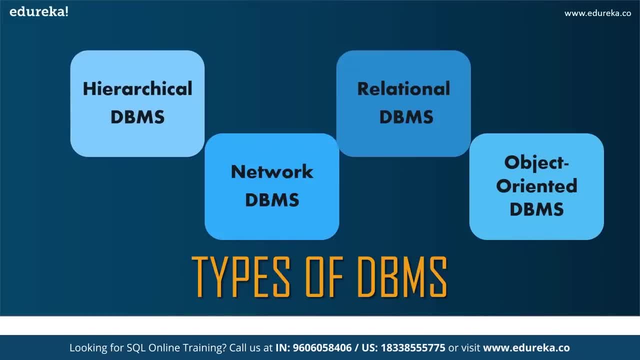 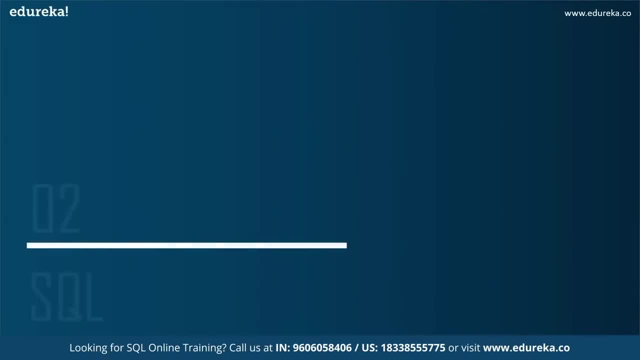 you want to work on and what type of DBMS would benefit you more. So I hope that you've understood what is DBMS and what are the different types of DBMS. Now let's move forward with the next topic for today's session, that is, sequel: structured query language. 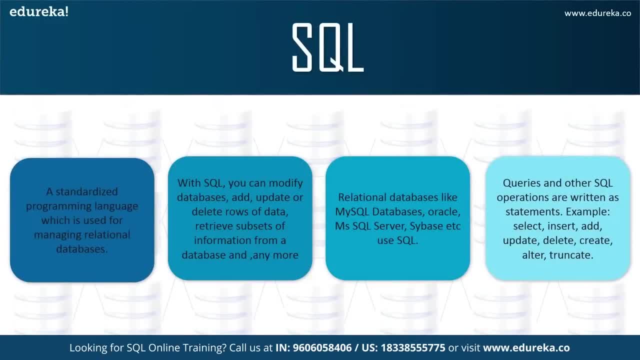 or pronounced as SQL, or sometimes also known as sequel, is a standard language for dealing with the relational databases. not to explain you further, Let me take an example for you Now. if two people want to communicate with each other, then they have to use certain language. 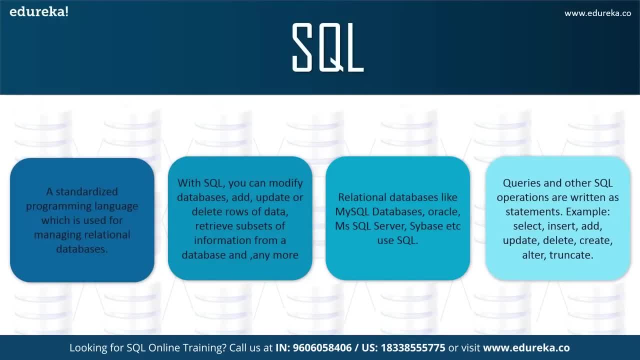 which is understood by both of them, right? So if we consider these two people as one as the user and other as the database, then the language which is used to communicate between these two is nothing but the structured query language. So, similarly, how a language has a grammar, 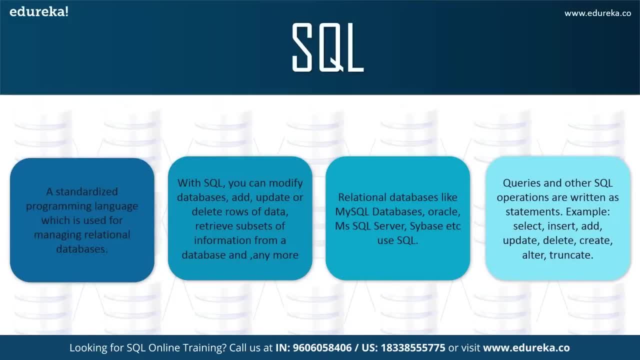 and various rules on how it could be used. even sequel has its own directives. sequel is effectively used to insert, search, update, delete and modify the database records and it doesn't mean that you know sequel cannot do things beyond that. it can do things beyond that also. it can provide you integrity checking. 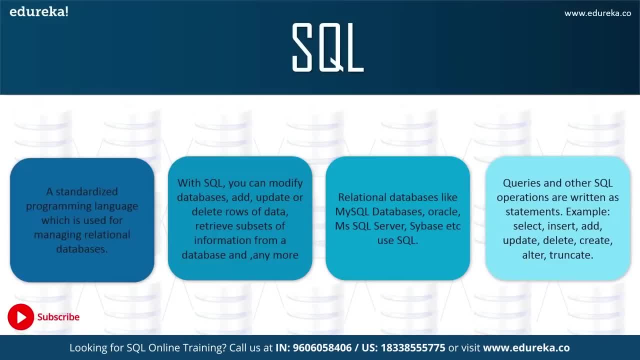 It can also provide you with embedded DML, which is used for general-purpose programming languages. It has various sets of commands to create different kinds of use, tables and other networks to understand the database effectively, and many such more. So, guys, this was about the basics of sequel and DBMS. 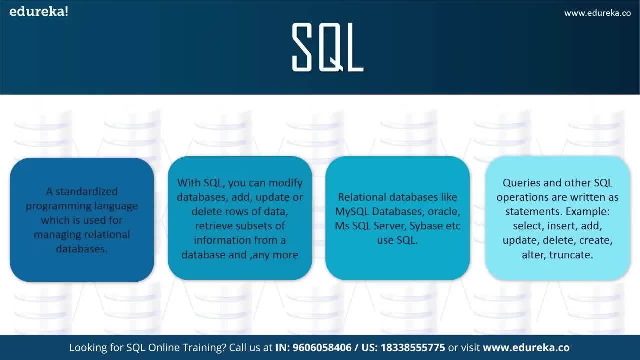 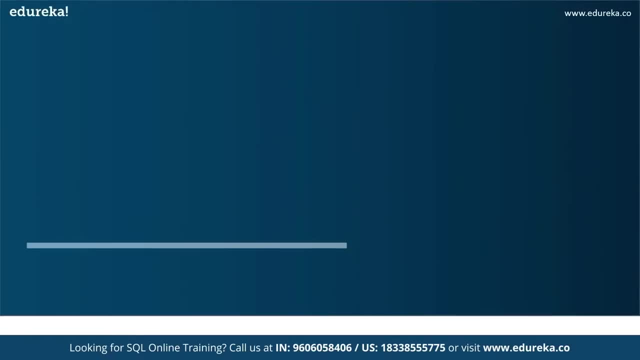 If you want to learn more about sequel, then you can refer to our session on what is sequel and I'm sure you'll get a better idea of what is sequel. But since this session is based on sequel server, let's get into the main topic for today's session. 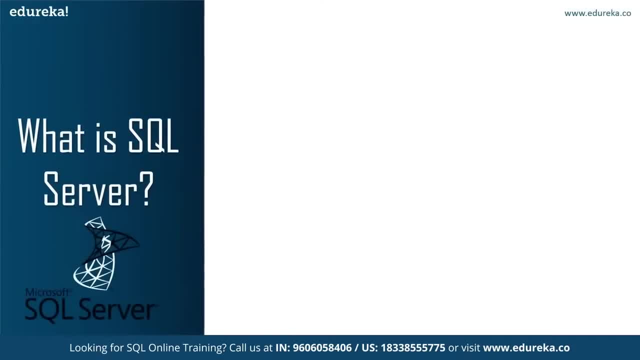 That is what is sequel server now. Microsoft sequel server is basically a relational database management system which supports the structured query language and comes with its own implementation of the sequel language, which is known as the transact sequel or the dsql. So it basically has an integrated environment. 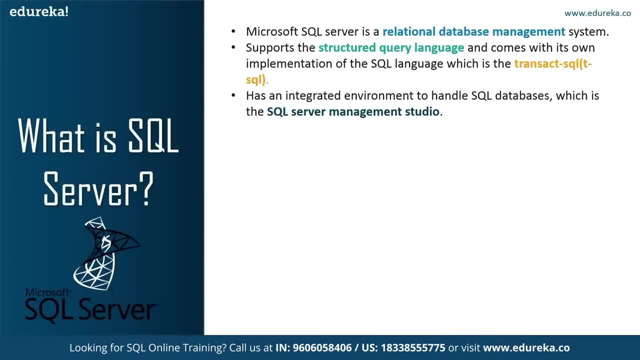 to handle sequel databases, which is nothing but the sequel server management studio. Now the key components of sequel server are: as you can see on my screen, We have a database engine and this component is basically used to handle storage, rapid transactions, processing and securing the data coming. 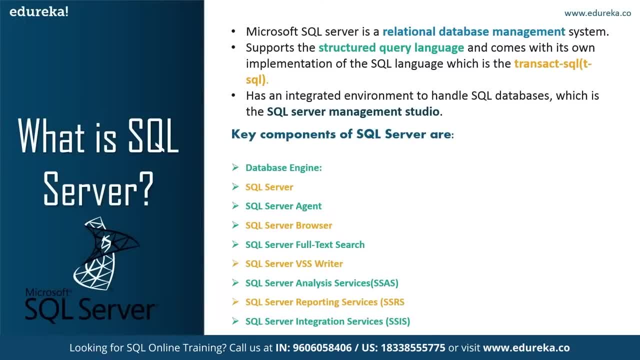 to sequel server service. This service is used to start, stop, pause and continue the instance of the Microsoft sequel server. moving on to the next component, which is the sequel server agent, the sequel server agent service plays the role of the task scheduler and is triggered by any event or as per the requirement coming. 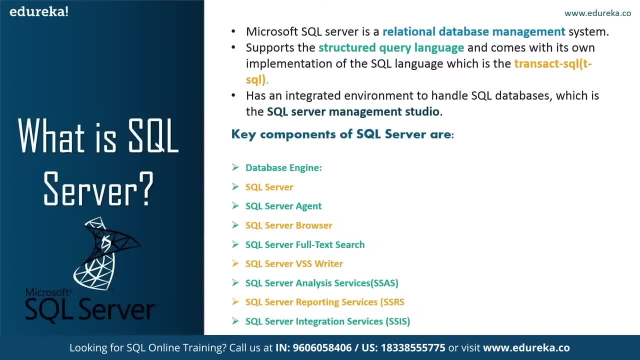 to sequel server browser. This service is used to connect the incoming request to the desired sequel server instance. coming to sequel server full text search. This is used to let the user run full-text queries against the character data in sequel tables. coming to sequel server: VSS writer. 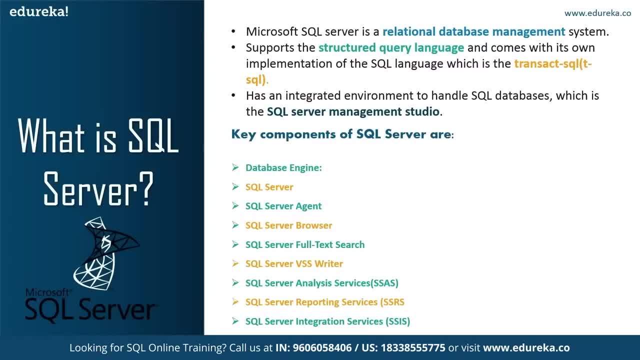 This particular service allows backups and restoration of data files when the sequel server does not run. moving on to the next component, at a sequel server analysis services, that is, SSAS, This service is used to provide data analysis, data mining and machine learning capabilities. The sequel server is also integrated with Python. 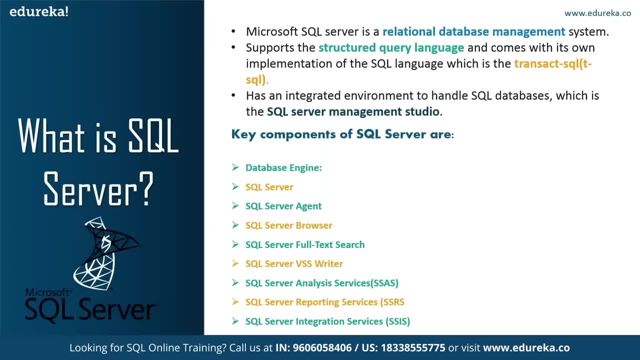 and R for Advanced Data analytics. coming to sequel server reporting services, which is SSRS as the name I suggest, this service is used to provide features and decision-making capabilities, including integration with Hadoop. finally, coming to the last component at a sequel server integration services, that is, SSIS. 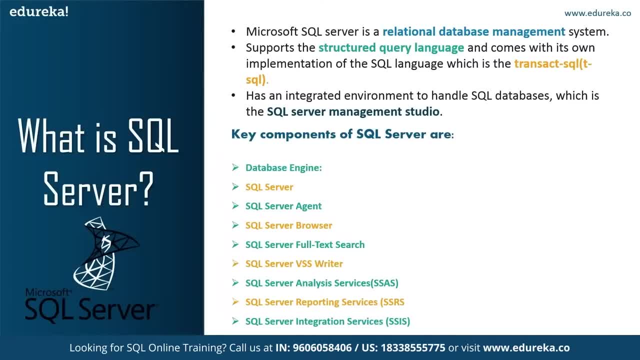 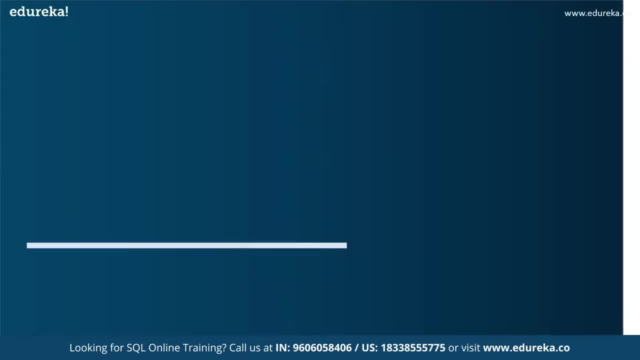 This service is used to perform the ETL operations for different types of data from multiple sources of the data. So I hope that you have understood what a sequel server. now let's move forward with the next topic for today's session, that is, features of the sequel server. 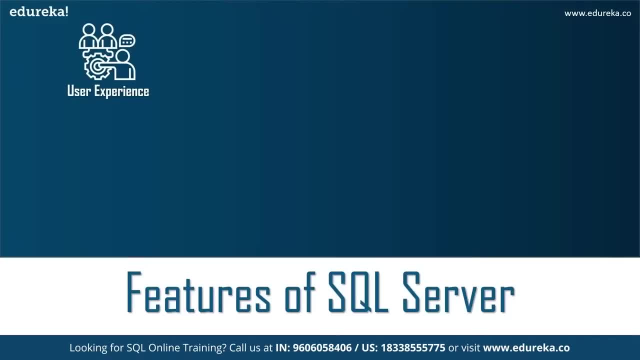 So the first one is user experience. So when I say user experience, what I mean by that is that you know sequel server can be used on various operating systems like Windows, Linux and talker, So you just have to develop once and deploy anywhere with their consistent experience, from on-premise to cloud right. 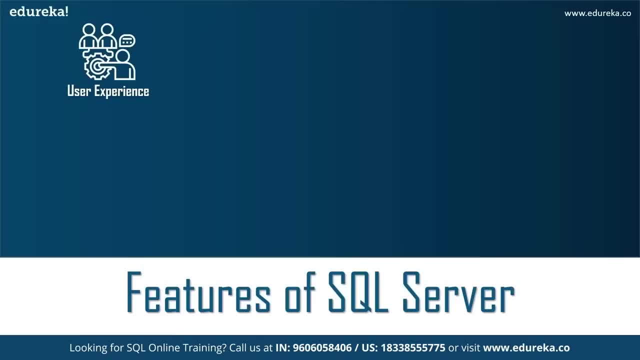 Not only this, but they make sure that you know you as a user, get a consistent experience from on-premise to the cloud, and also provide easy-to-use tools and the connectors so you can use the Azure Active Directory and the sequel server management studio to manage your database infrastructure across on-premise. 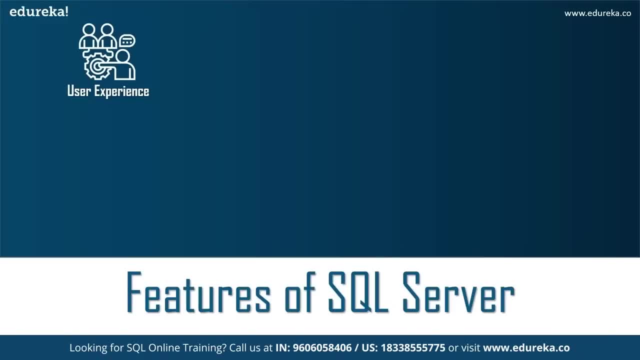 sequel server and also Microsoft Azure. So isn't that great guys. now moving on to the next feature. The next feature is availability. So when I say availability again, what I mean by that is that you know sequel server. make sure that you know. 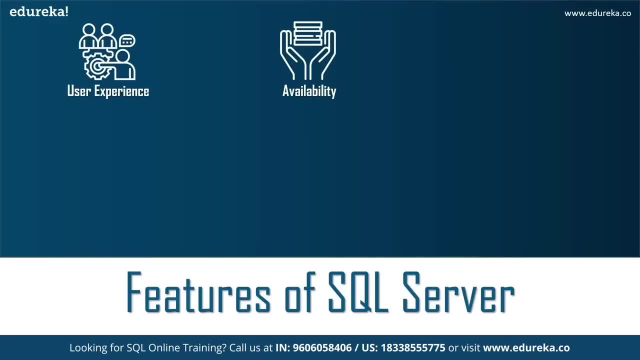 it provides high availability and disaster recovery. So with this you can gain mission-critical uptime, fast failover, easy to set up and load balancing of the readable secondaries. with the enhanced sequel server versions So you can get unified solutions for high availability and disaster recovery on Linux and Windows. not only this. 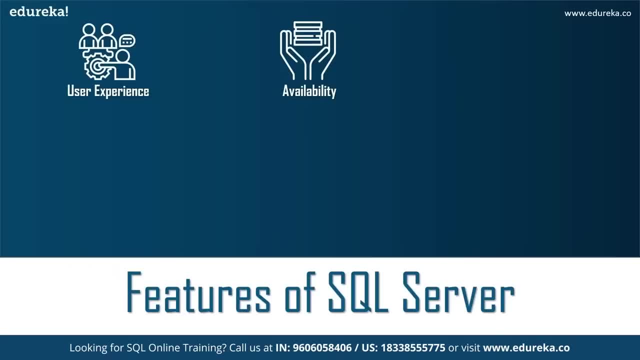 but you can also put up an asynchronous replica in the Azure virtual machines for the hybrid High Availabilities. So that was about availability, guys. moving on to the next feature, that is performance. So when I say performance, what I mean by that is to know. 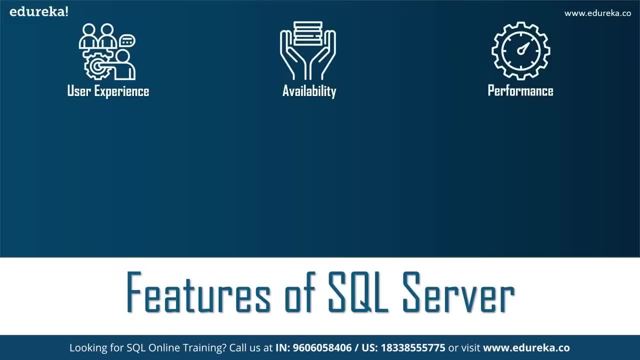 you can scale your price and performance in a parallel manner. So sequel server make sure that you know your real-world application performance benchmarks are set and then your application using the sequel server database is not failed on or is not turned down right, so you can get great performance for your application. 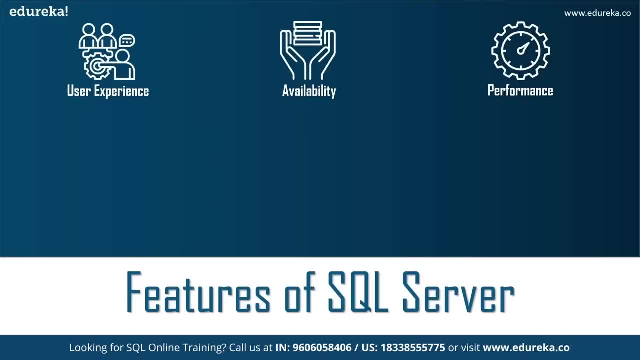 and it is also one of the highest performing data warehouses. moving on to the next feature, That is, analytics. So when I say analytics, what I mean by that is that you know sequel server provides the built-in analytics, or you can say the built-in database advanced analytics. 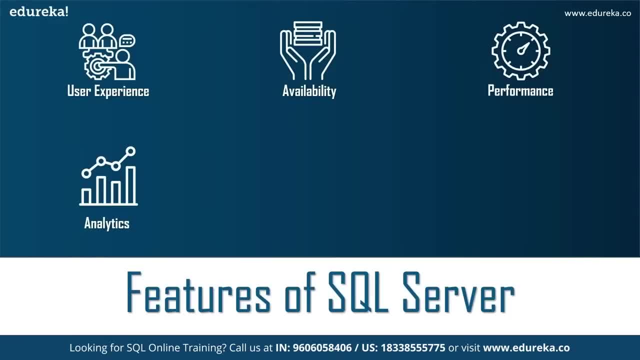 So with the help of the built-in analytics and the sequel server machine learning services using R and Python, you can move beyond the reactive and into predictive and prescriptive analytics by performing advanced analytics directly within the database. So by using multi-threading and massively parallel processing, you'll gain insights faster. 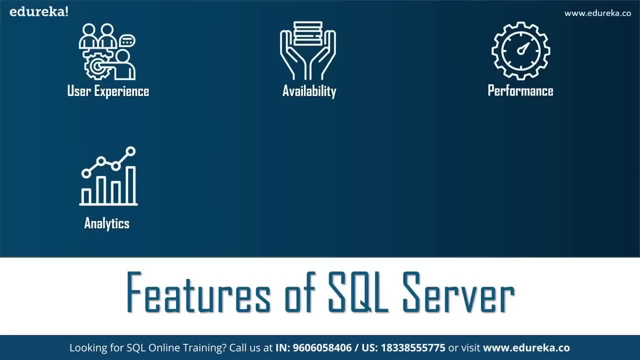 than using open-source are in Python. So, guys, that is one major plus point of sequel server. now, moving on to the next feature, that the security. so security, as the name suggests, I would say that you know it provides less vulnerable databases, So you can make sure that you know. 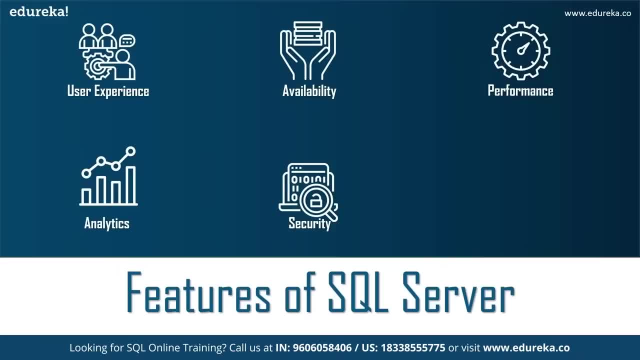 your data is protected in a proper manner and it is less vulnerable to any other major attacks. not only this, but you can also make sure that you know you have levels of security and compliance for the databases. now coming to the final feature, guys, that is, business intelligence. 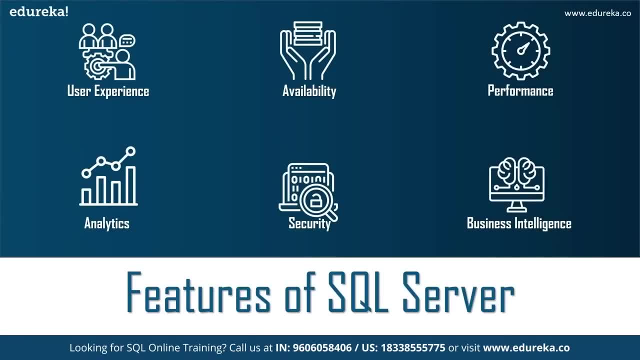 So obviously, as the name suggests, business intelligence is almost used in today's market in every company, and every company needs a manner to understand and visualize the reports and also gain insights right. So sequel server provides you with this feature and allows you to build comprehensive Enterprise scale. 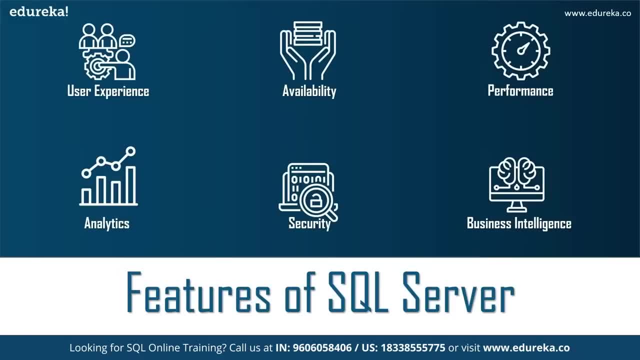 analytic solutions by benefiting from the fast performance of in-memory built into the tabular model. So, basically, what happens is that unit reduces the time to insights using direct querying against tabular and multi-dimensional models. So, guys, that were the features of sequel server. 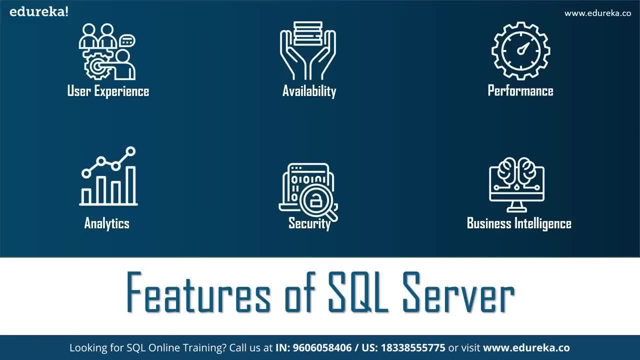 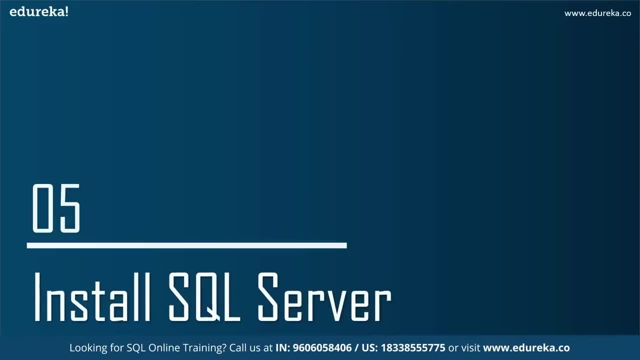 So I hope that you have understood what is sequel server and its features. So now that you know the basics of database management system sequel- sequel server, let's move forward and install sequel server. So to install sequel server, what you have to do is you have 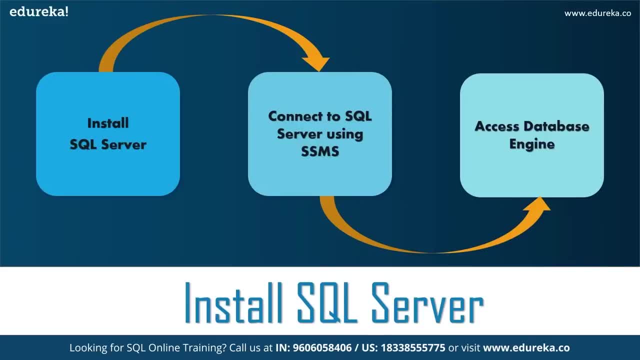 to follow the steps that you can see on my screen. initially, you have to install the sequel server, and then you have to connect to the sequel server using SSMS, That is, the sequel server management studio. after that You have to access your database engine. 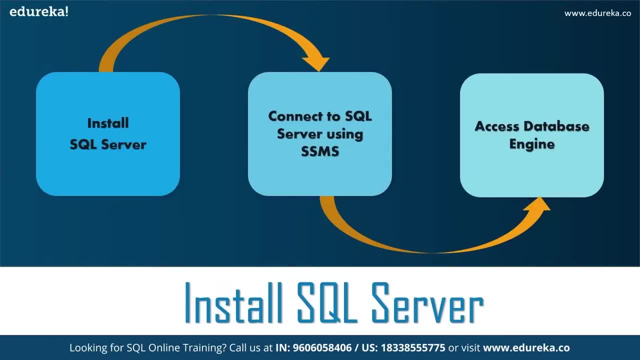 I hope I'm clear with this points. All right, so let's start with the installation of sequel server. So initially what I'll do is I'll install the sequel server, then I'll connect to the sequel server using sequel server management studio and then I'll access the database engine. now 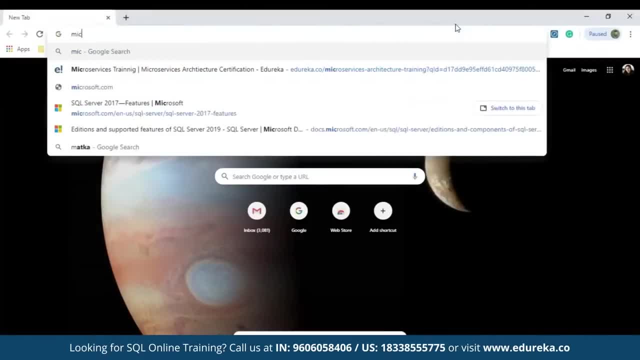 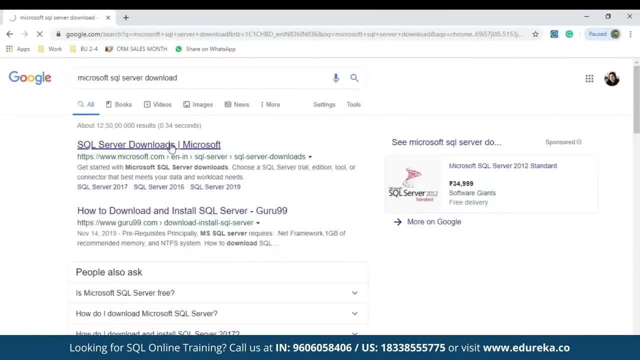 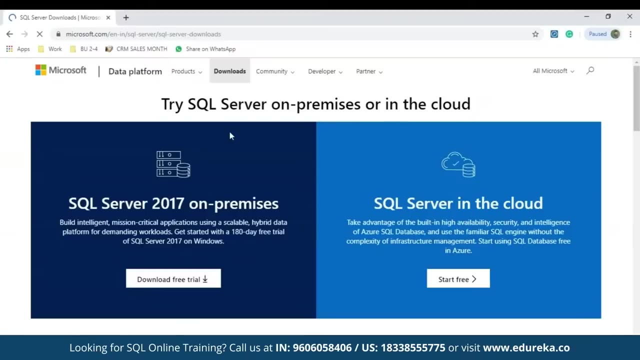 to install the sequel server. What do you have to do is you have to go to this official website of Microsoft sequel server download. Right, so I'll just go to this particular page And once you go to this page, you see this: two options at a sequel server 2017 on-premises. 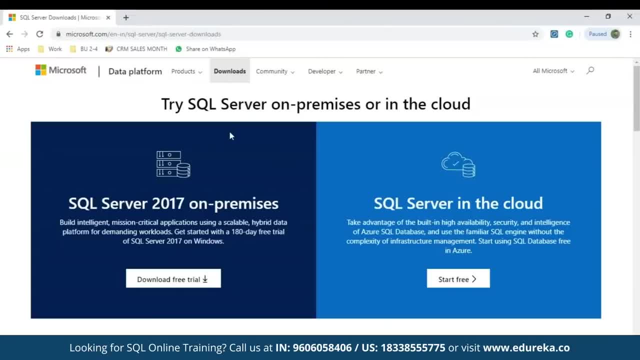 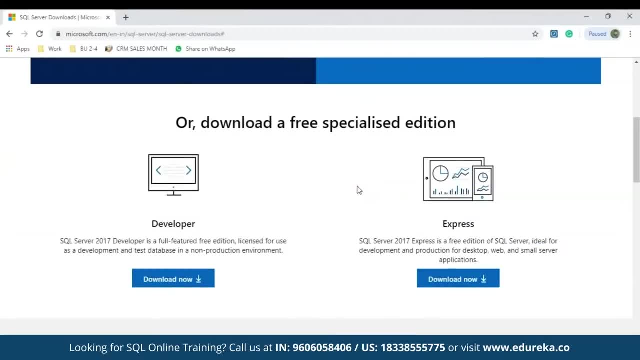 and on the cloud. Now, what this means is that you know you can either use sequel server locally on your system or maybe on the cloud. So now what you have to do is you have to scroll down this particular page and you will see this option of developer. 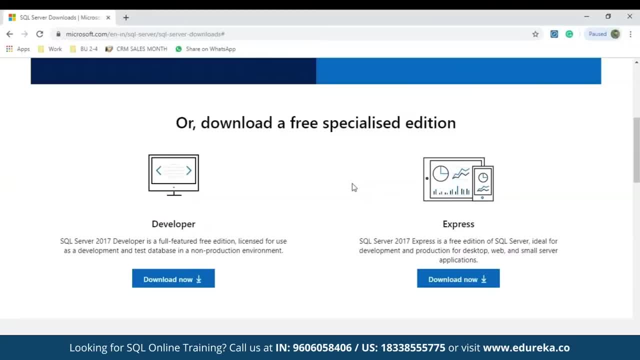 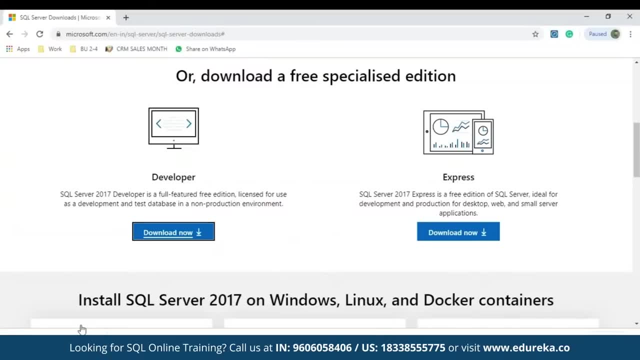 and the Enterprise Edition. So here I'll be downloading the developer edition. So to download, you just have to click on this option of download now. Now you can see that you know the application is getting downloaded. So once the application is downloaded, what you have to do 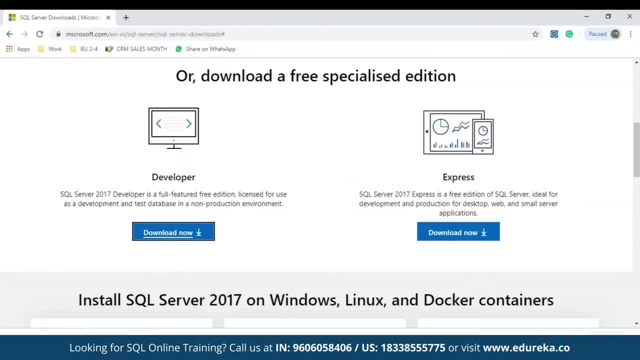 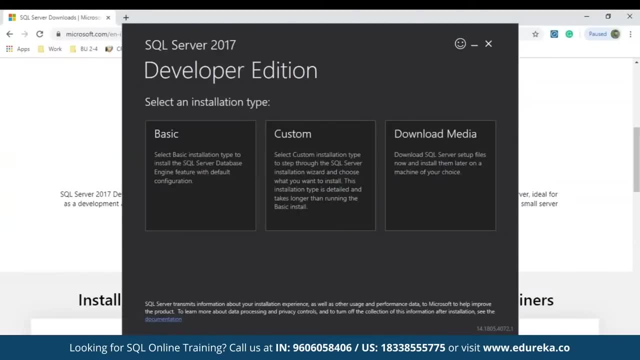 is you have to double click on this particular file and then you will see a window opening up. So let's just wait for that to happen. So, as you can see, our application is opening up now. once the application opens up, you see various types of installation types. that is, the basic type, the custom type. 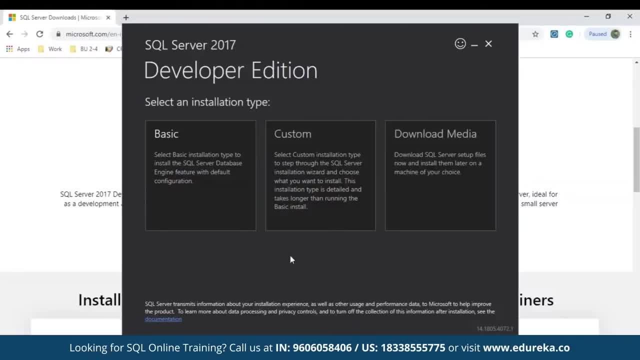 and the download media. So what I'll do is I'll just choose the basic type. So when you choose the basic type, you can select the basic installation type to install the sequel server database engine feature with the default configuration. Just remember, guys, when you're choosing the basic type, 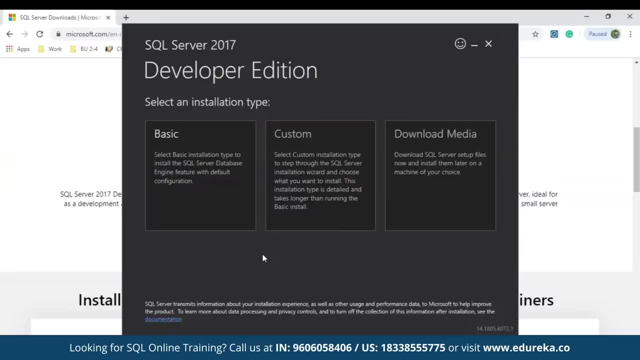 you're installing sequel server with the default configuration, moving on to custom type. So when you select the custom installation type to step through the sequel so installation wizard, you choose the features or I would say you choose the configuration based on your choice, right? So I would say, if you're using it on an Enterprise level, 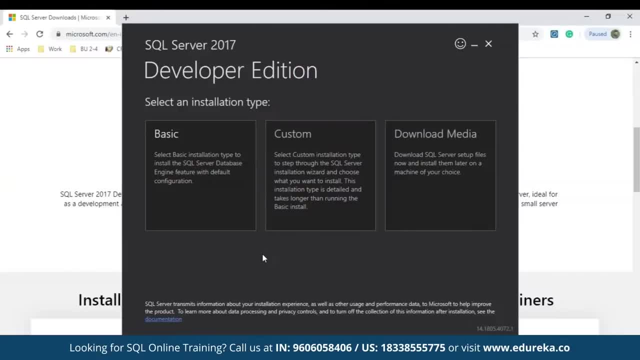 or maybe your complete companies using sequel server, then I would say you can go forward with the custom installation, because you may have few features or you may want few configurations, which must be same for the complete users, right? So that's when I would say you can go for the custom one. 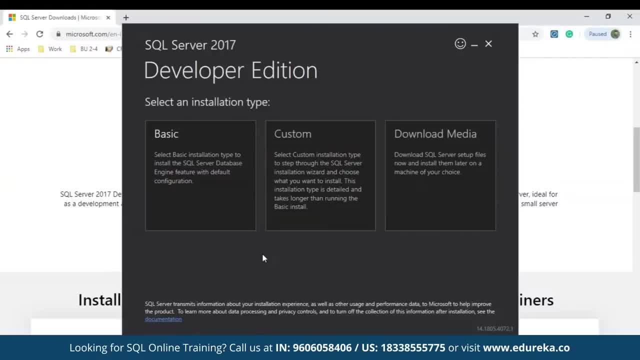 But if you're someone who is just using sequel server on locally on your machine and then you just want to get hands-on experience in that, I would say: go for the basic one, right? So on that note, I'll just choose the basic one. 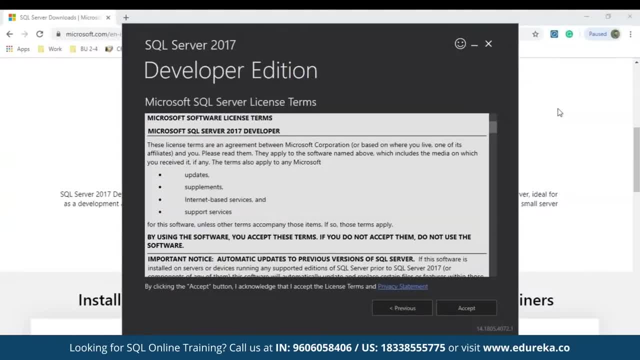 And then, once I choose the basic one, you can see that you know we get this page of sequel server license terms. So what you can do is you can just go through the license terms and then you can just click on accept button. 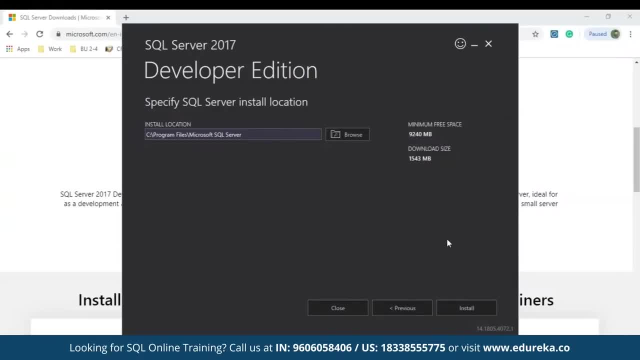 So I'll just directly click on the accept button. And once I click on the accept button, you have to next specify the sequel server installation directory, right? So that means where you want to install your sequel server. So I'll just let it be as it is. 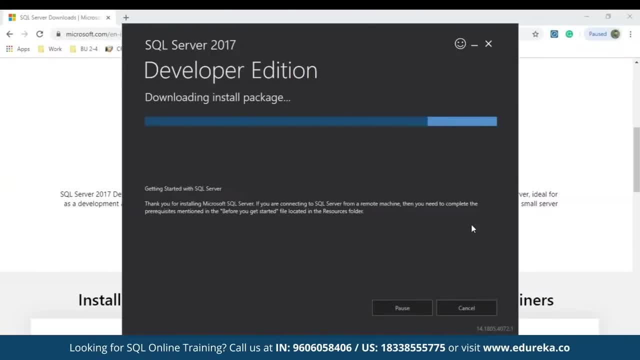 and then I'll click on install. Now, once you click on install, you will see that all the required packages and the libraries are getting downloaded. Now let's just wait for the installation to complete. So, as you can see, the computer requires a restart. 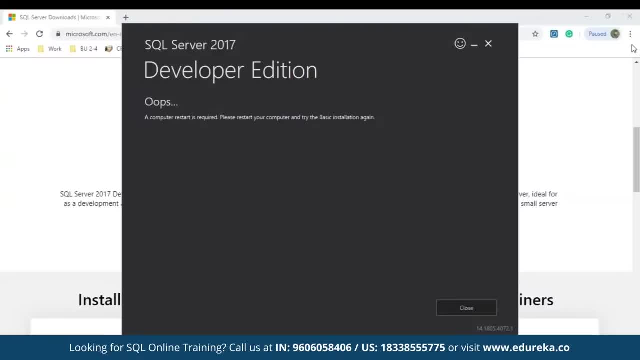 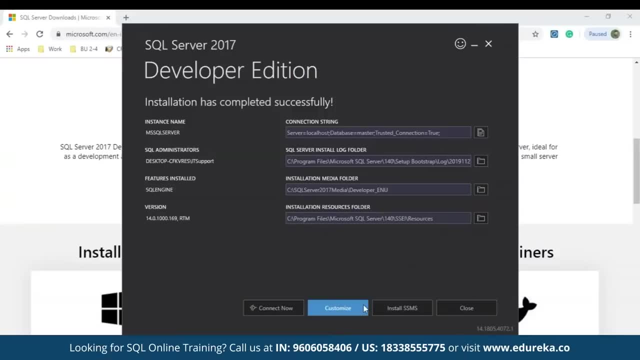 So let me just restart my computer, right? So let's just increase. start Now. once the installation has completed, what you next have to do is you have to go to this customize option pillow to basically configure your sequel server database, right? So I just click. 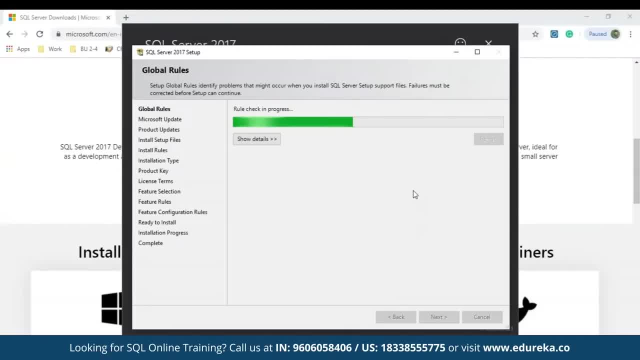 on this customize option. Now, once you click on the customize option, this is a screen that you will see. so, over here, What you just have to do is you just have to click on next, and once you click on next, you'll basically see that the files are getting installed, right. 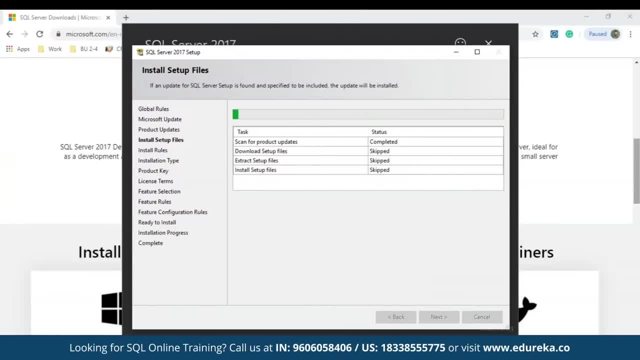 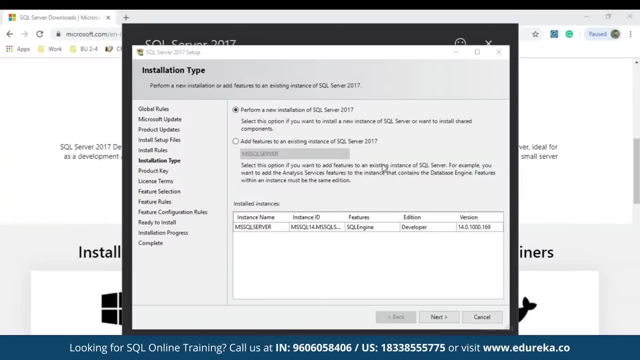 So let's just wait for that to happen, and then you keep clicking on. next, I'll tell you when you have to configure for something, So let's just wait for that to happen. All right Now. once the installation rules are also done, The next thing that you have to do is you have to choose. 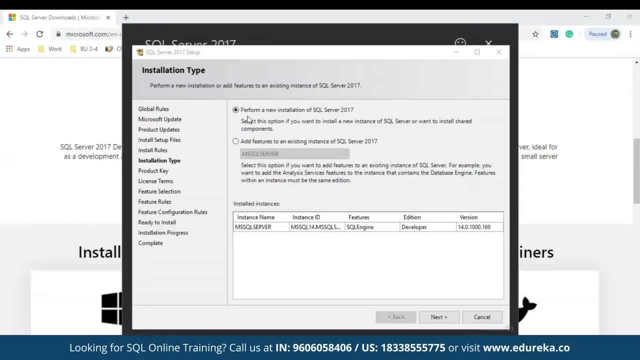 the installation type. So, since we are performing a new installation, we'll just choose this option of perform a new installation of sequel server 2017.. But, yes, if you had any pre-installed sequel versions, then you will choose the second option, right? 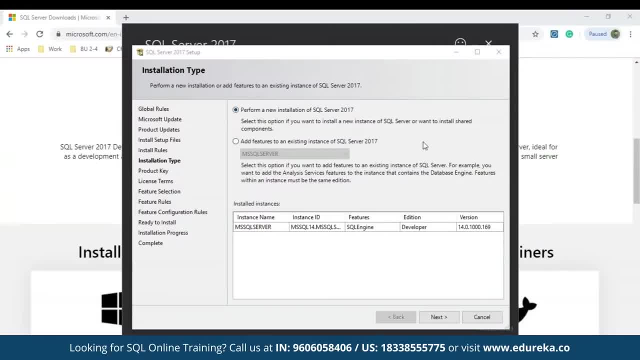 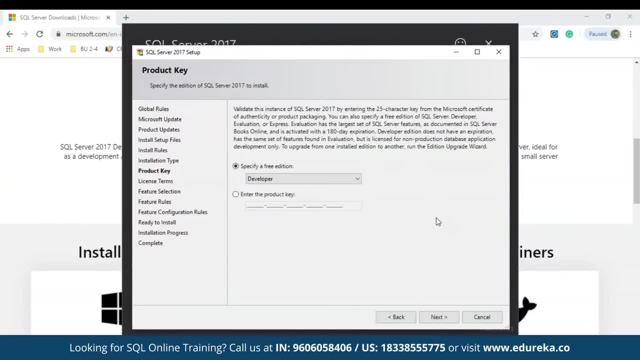 So I'll just choose this option of perform a new installation of sequel server 2017, and then I'll click on next. Now, in the next visit that opens up, you have to choose basically the type of addition that you are installed initially, that is, the developer Edition or the Enterprise. 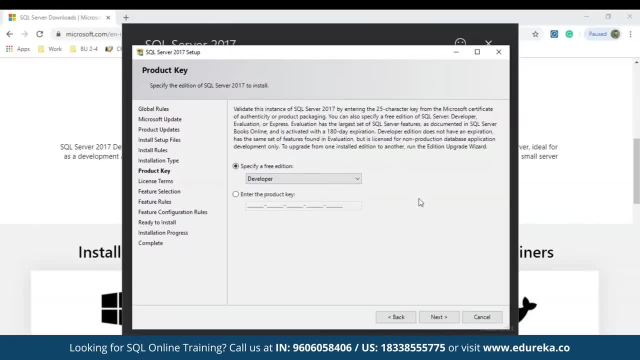 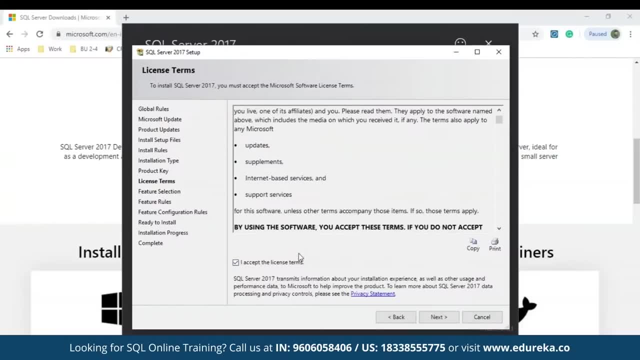 So, since I downloaded the developer Edition, I'll just choose developer and then what I'll do is I'll click on next Now. after that, you have to read this license terms and then just click on this radio button of I accept the license terms and then click on next now. 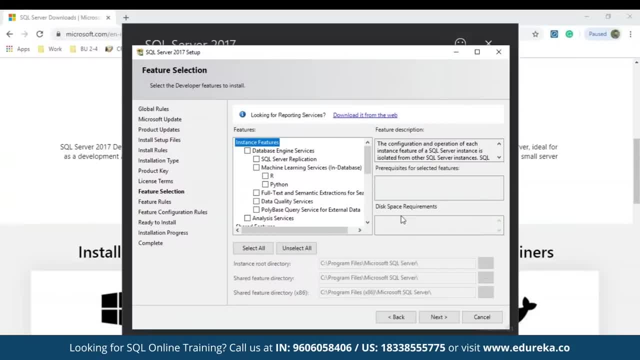 in the next visit that opens up. you have to choose the features which you wish to install. also, you can choose the instance root directory and then click on next. So what I'll do is I'll just choose the features, Let's say database engine. 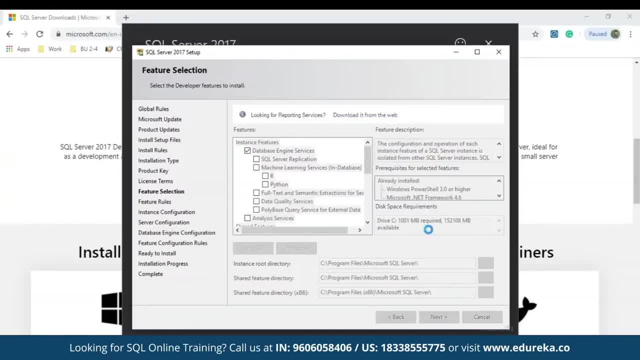 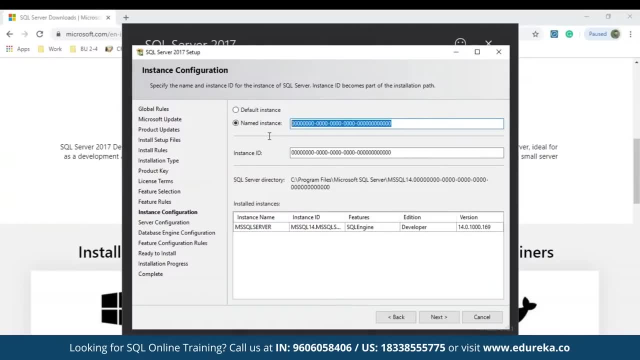 and then I'll let the root directory be the same, and then I'll click on next now, after that, What you have to do is you have to name your instance, and then this will automatically return an instance ID, right, So I'll just name my instance. 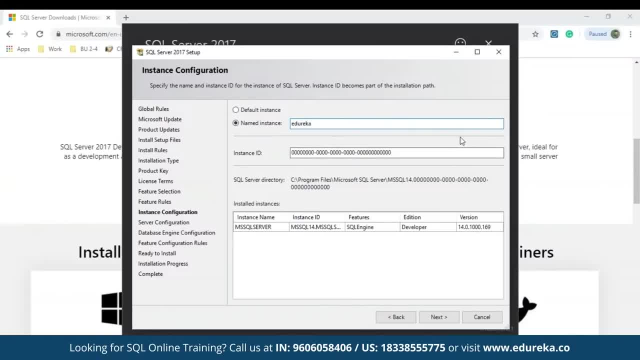 Let's say edureka, right, and once I mentioned my instance name, you'll see that you know automatically my instance ID will be edureka. So after that, what I'll do is I'll just click on next. Now in the server configuration wizard, just click on next. 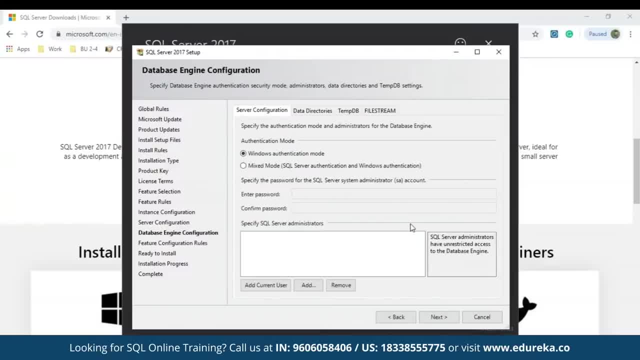 and then, once you click on next, you'll be redirected to this database engine configuration. So over here you have the Windows authentication mode and the mixed board. So over here, what I'll do is I'll just choose the mixed mode and then I can mention the password, right? 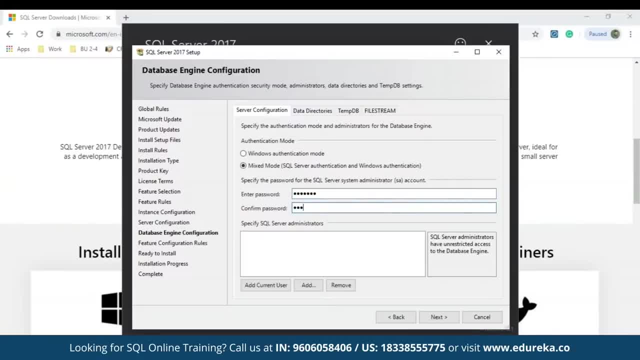 So I'll just mention the password and then I'll confirm the password, And then what I'll do is I'll just click on add current user and you'll see that you know, automatically a user has been added, So this particular user will be the admin after that, as you saw, 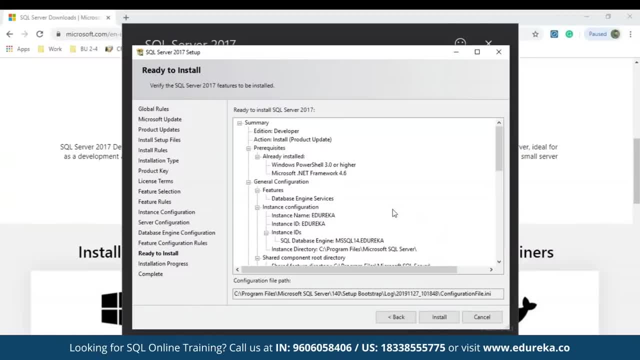 I just mentioned the password and then I'll click on next. Now, once we click on next, you can see the summary of the installation, like what are the properties or the features which will be installed. So you can just go through that and then what you can do is you can just directly click. 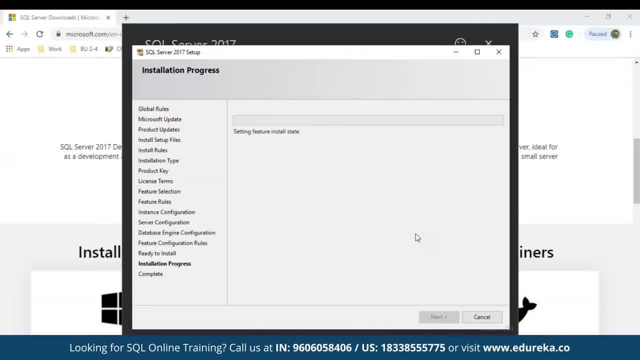 on install. So I'll just click on install over here And now. let's just wait for the installation to complete. Now, once the installation is complete, this is the wizard that you see. that means that you know our installation has completed, So I'll just click on close. 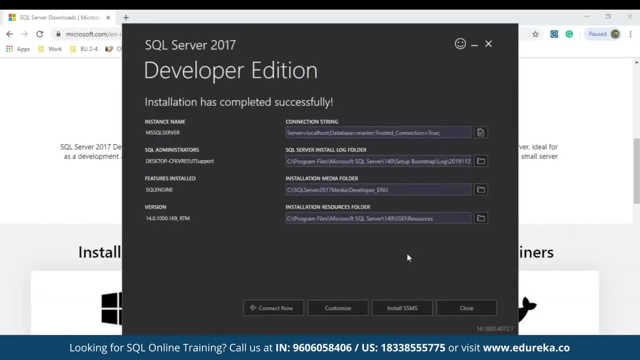 and then, with this, we finish our installation. Now the next step is to connect a sequel server using the sequel server management studio. So for that, what we'll do is we'll go back to this particular screen and then I'll click on install SSMS. 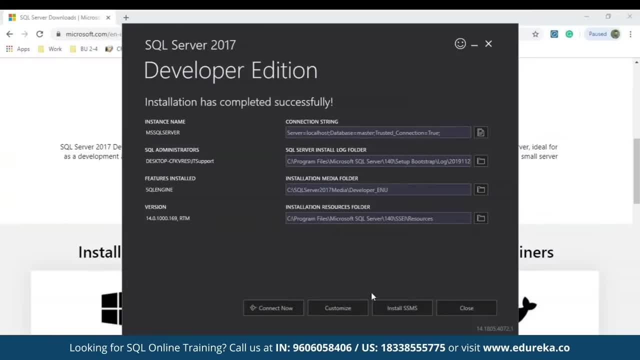 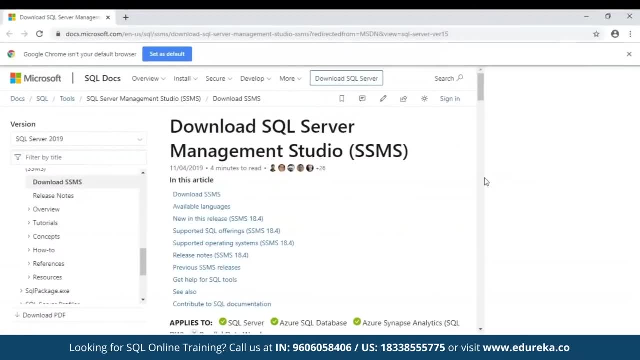 Now, once you click on install SSMS, you'll see that you know you'll be redirected to a web page, So let's just wait for that to happen. So, guys, this is a screen that you see once you click on install SSMS. 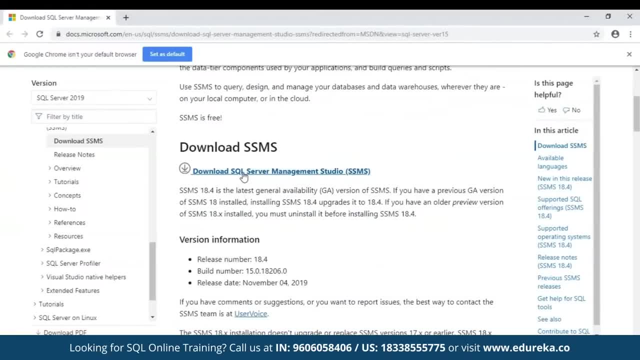 Now what you have to do is you have to just click on this download option. So I'll just click on this download sequel server management studio link And then, once I click on the link, you can see that you know the setup is getting downloaded right. 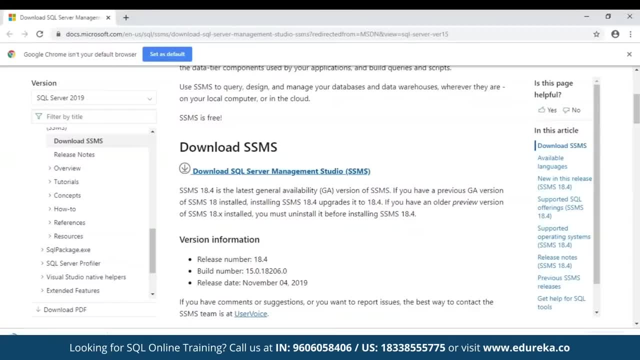 So let's just wait for that to happen again. All right Now, once the setup has been downloaded, just double click on this particular file And then you'll see this particular screen. So over here you can just choose the location or the installation directory. 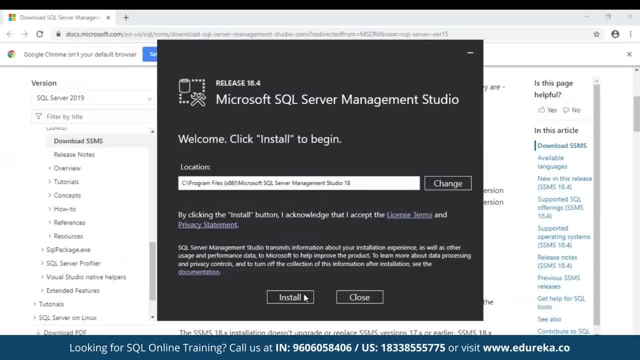 for your sequel server management studio. I'll let it be as it is, and then I'll just click on install. Now, once I click on install, you can see that you know a sequel server management studio is getting installed, So let's just wait for that to happen. 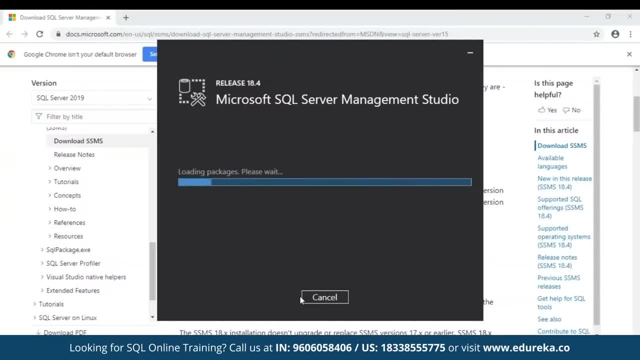 And once that is done, what we'll do is we'll basically access our database engine. So let's just wait for installation to complete. Now, once the installation is completed, you see that you know restart is required in order to do the complete setup. 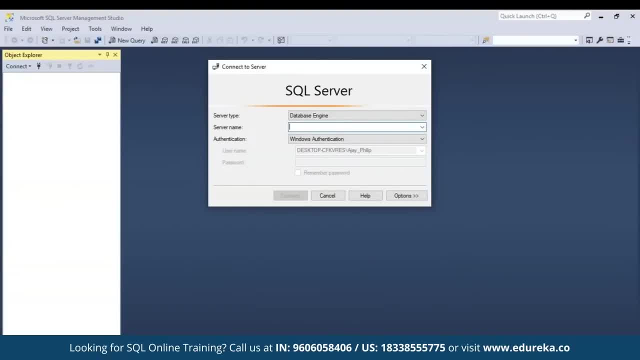 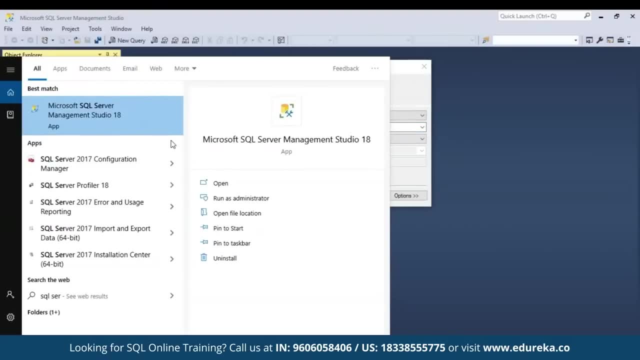 Now, once the sequel server management studio is installed, you just have to open your sequel server management studio from the Windows Explorer So we you can just type in sequel server and then you'll see this icon. So you just click on open. and once you click on open, 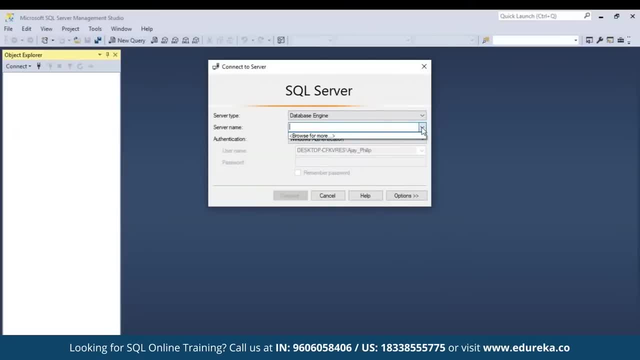 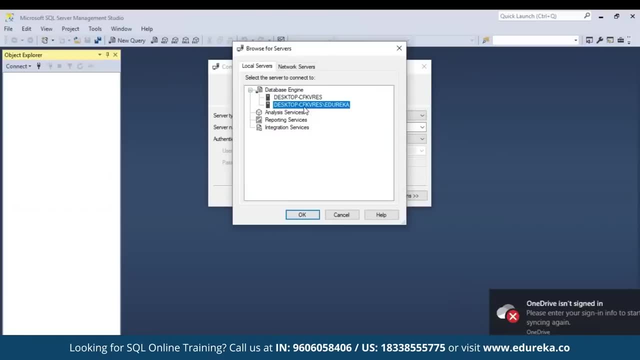 this is basically what you see now over here. What you have to do is you have to choose your server name. So you can just go for browse for more and just choose server name. And let's say, we choose our desktop ID: slash edureka, right. 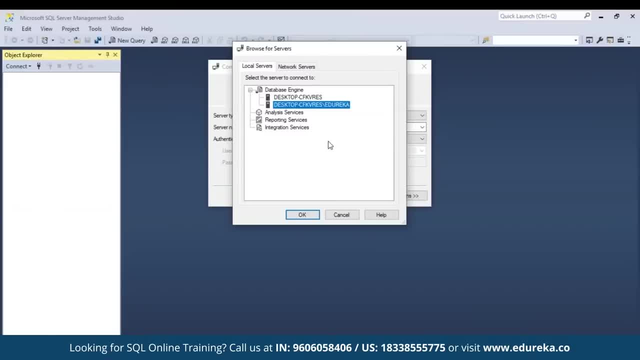 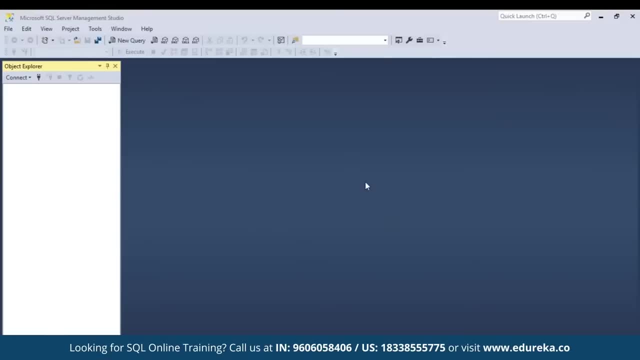 That is because that is the one that we chose, So we gave our instance ID to be edureka, if you remember. so I'll choose that and I'll click on OK and then I'll click on connect. now, once you log in, guys, this is the screen that you see now. 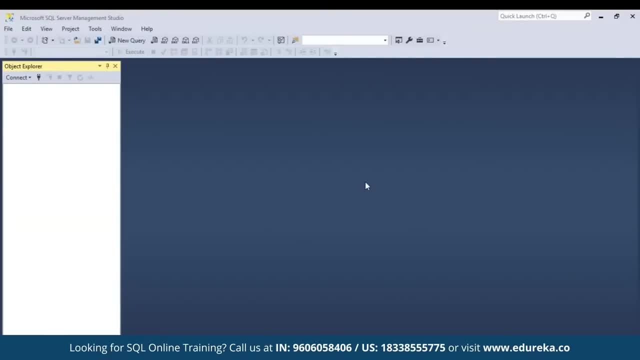 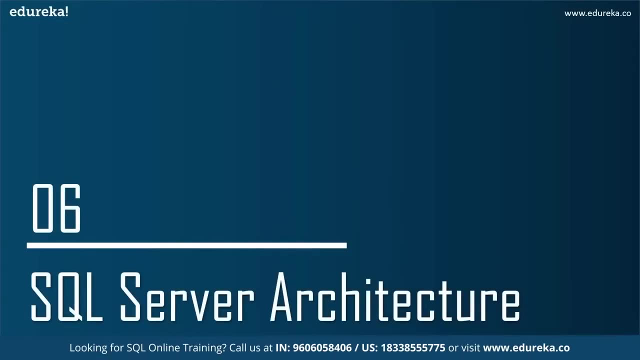 The next thing that you have to do is you have to basically start your query editor, right? So before we get into the query editor and start using the commands, let's understand. how does the sequel server architecture look like? so the sequel server architecture mainly has few components. 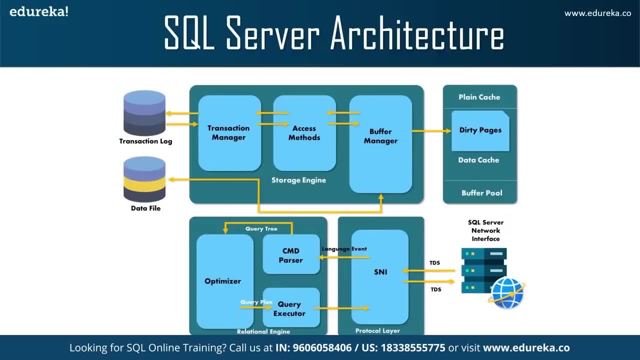 that you can see on my screen. So it has the server, It has the relational engine, the command parser, the optimizer, the query executor and the storage engine. coming to the server first, This is where the sequel services are installed and the database resides. moving on to relational engine, 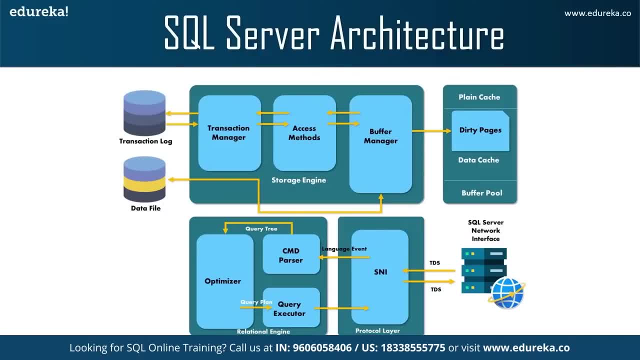 This contains the query, parser, optimizer and the executor, and the execution happens in the relational engine. moving on to command parser, Well, this checks the syntax of the query and converts the query to the machine language. moving forward with optimizer, this prepares the execution plan as the output by taking statistics query. 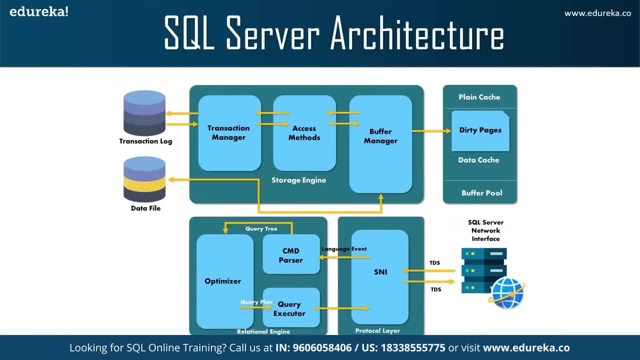 and the algebra tree as input, moving forward with the next component, that is, query executor. Well, this is the place where queries get executed step-by-step and the storage engine is responsible for storage and retrieval of data on the storage system, manipulation of data, managing and locking transactions. 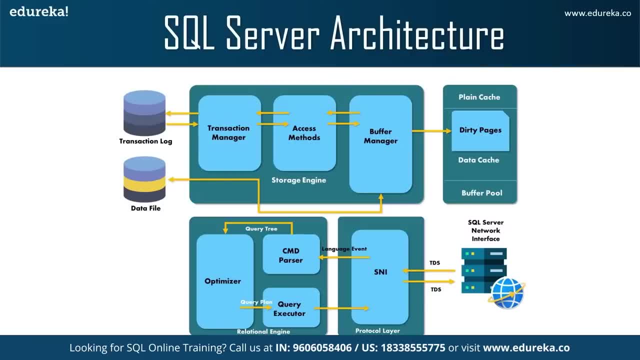 So you have a transaction log and then you have a data file. You also have a storage engine which has the transaction manager, the access methods and the buffer manager. after that We have the relational engine, where the relational engine has the optimizer and the command parser. 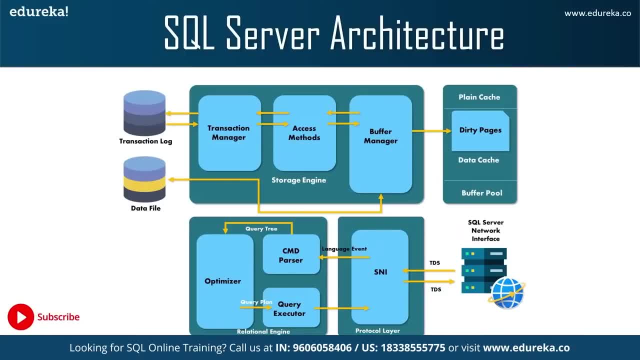 and the command parser is connected to the query tree, and similarly we also have the query executor, which executes the query, and the optimizer optimizes the query. Finally, we also have a protocol layer which has the SNI, and then this is connected to the sequel server network interface. 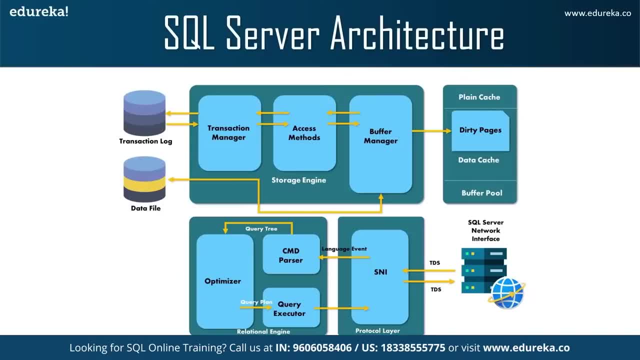 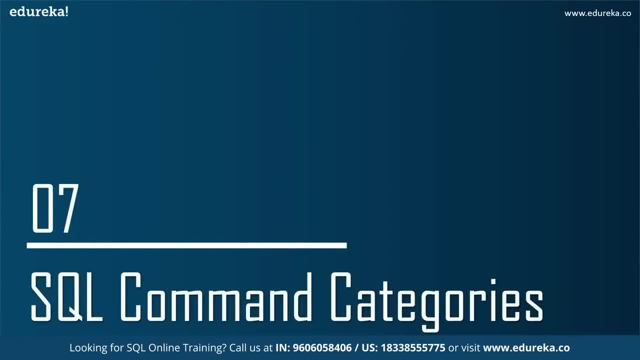 Well, guys, this was about the sequel server architecture on a high level. by now I hope that you've understood and got a good understanding of the sequel server. Now let's move forward and get into the sequel command categories, where there are mainly four command categories. 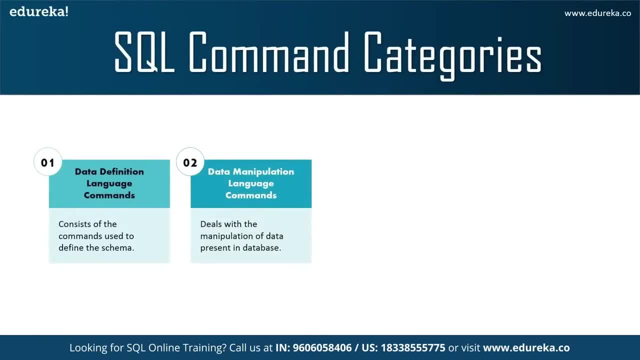 that we've got to consider, that is, the data definition language commands, the data manipulation language commands, the data control language commands and the transaction control language commands. coming to data definition language commands, Well, this consists of the commands that can be used to define the database schema moving. 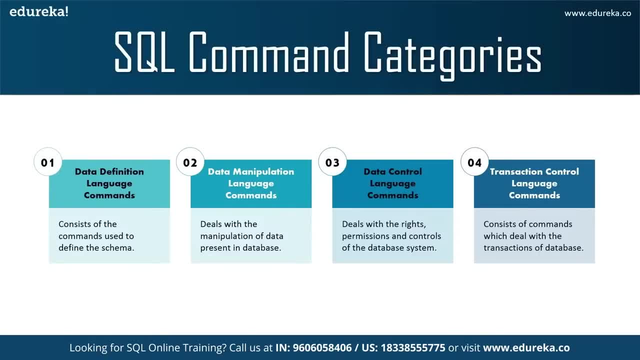 on to data manipulation language commands. Well, this deals with the manipulation of the data present in the database. coming to data control language commands: Well, this deals with the rights and permissions and the controls of the database system. and finally, coming to transaction control language commands, and this consists of the commands: 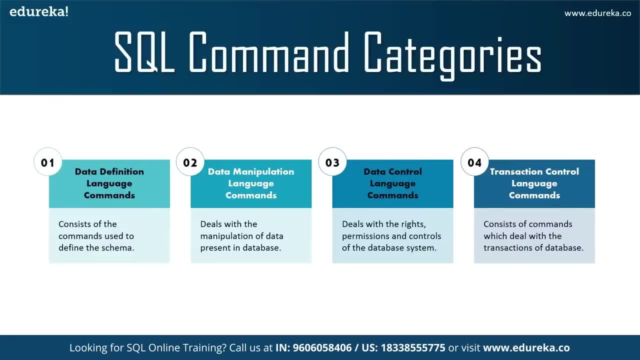 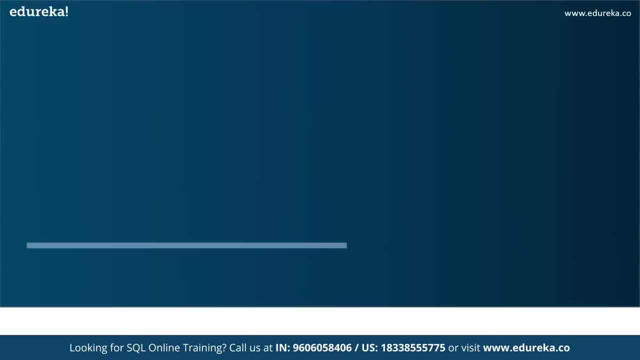 which deal with the transaction of the database. So I hope that you've understood. What are the sequel command categories? So before we move forward with the first command category, that is, the data definition language command category, So let me talk a little bit about the sequel server data types. 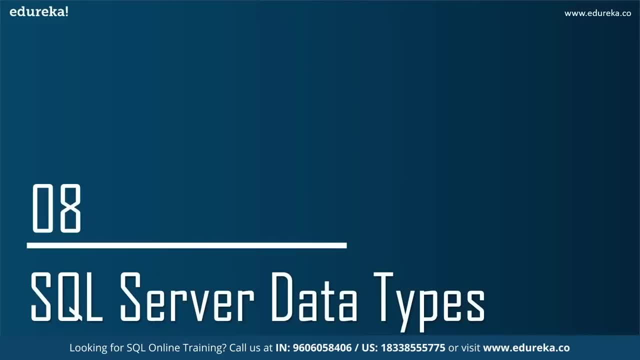 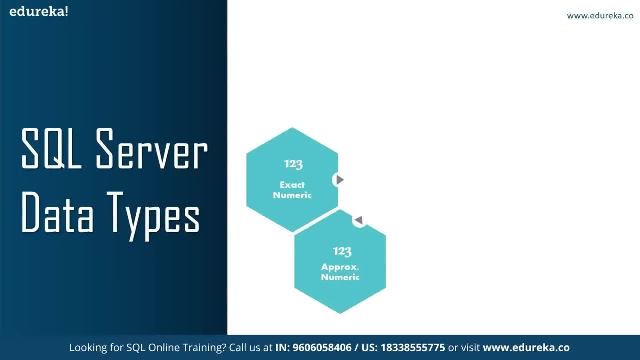 Well, there are various kinds of sequel server data types present. So when I say data types, I mean what kind of data can be stored in your databases so you can store exact numeric data types, the approximate numeric data types, the date and time values, the character strings, the Unicode character strings. 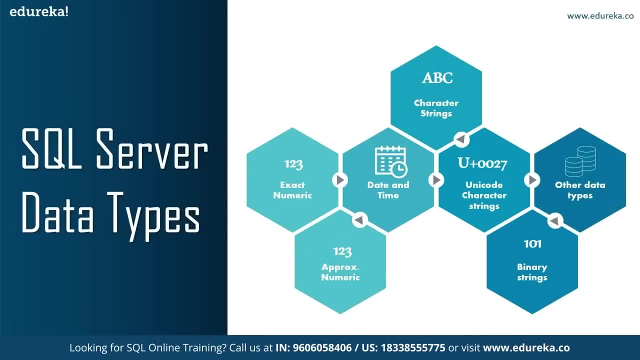 the binary strings and many other data types. So, talking about the exact numeric data type, Well, the exact numeric data type is used to basically store the numbers. So in this data type you have other data types, like the numeric, Like the tiny and small and big, int, and so on, moving. 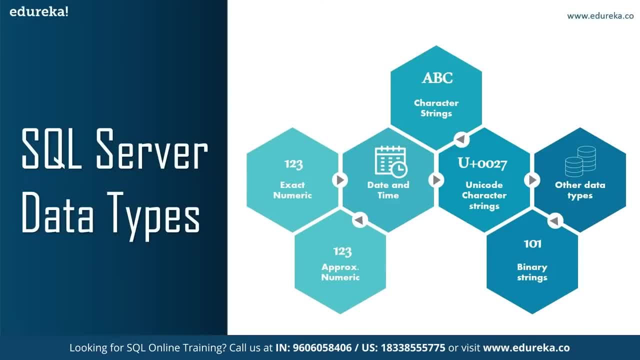 on to approximate numeric. Well, approximate numeric are used to store decimal or float value, So you have the float data type and the real data type coming to date and time. as the name suggests, this type of data type is used to store the date and time values in the database. 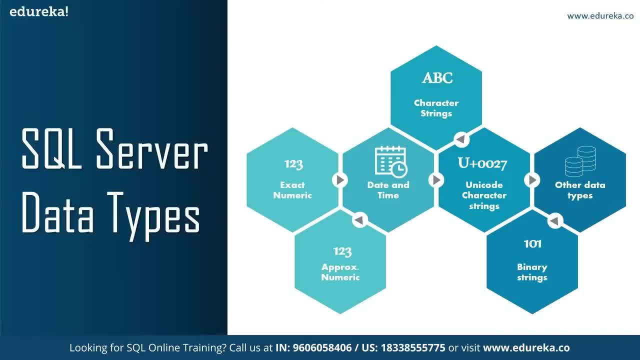 So we have dates, small date time, date time, date time 2, and so on. moving on to character strings, Well, this particular data type is used to store the character strings like care, varchar, text and so on. The Unicode character strings are used to store the end care. 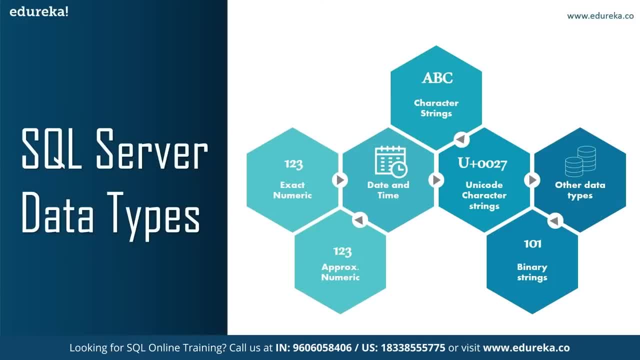 And then text after that, coming to binary strings: binary strings, as the name suggests. again, I used to store the binary values. So we have binary, where binary and image values in this particular data type, and in the other data type sections we have data types like the cursor, the row, version, hierarchy, ID, unique identifier. 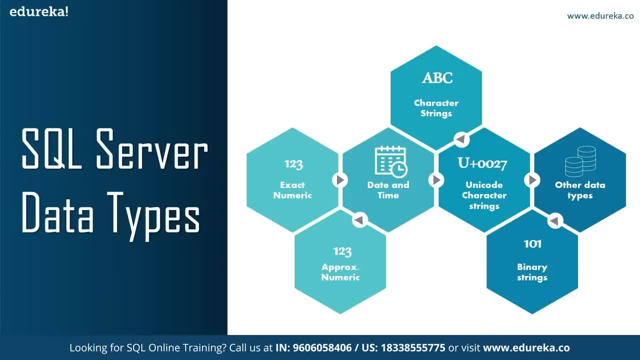 and so on. Well, I would say, once you get a hands-on practice on how to write queries and how to manipulate data in your database, You'll definitely understand which type of data type you need to use or you need to use to define your columns. 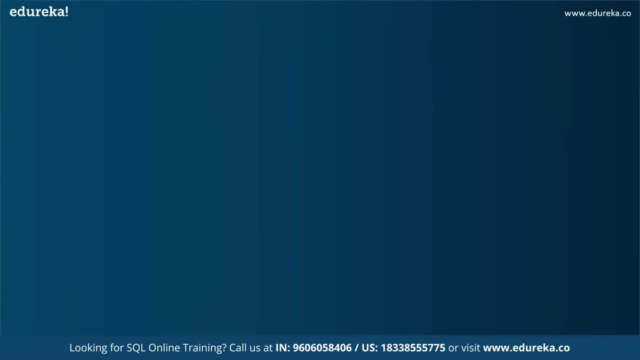 So I hope that you have understood. so, on that note, let's start with the first language command category, that is, the data definition language commands. So, to demonstrate the data definition language commands, what I'm going to do is I'm going to write few queries. 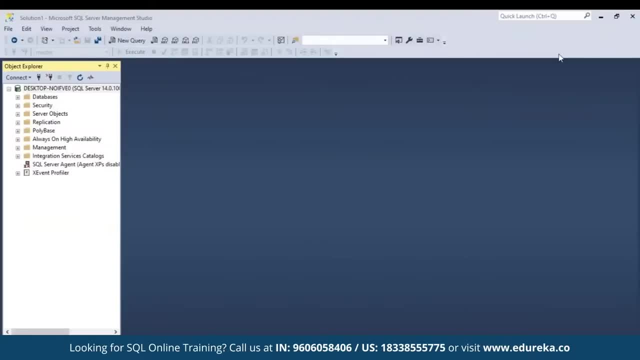 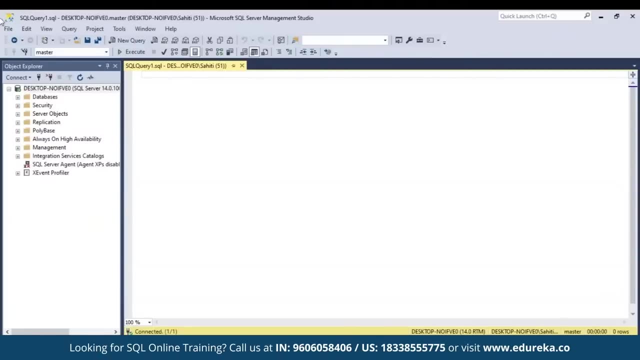 and then I'm going to explain how you can use that. So now what I'll do is I'll just add a query pane. So to do that, what I'll do is I'll just go to this new query option and then you'll see that you know, automatically a query pane. 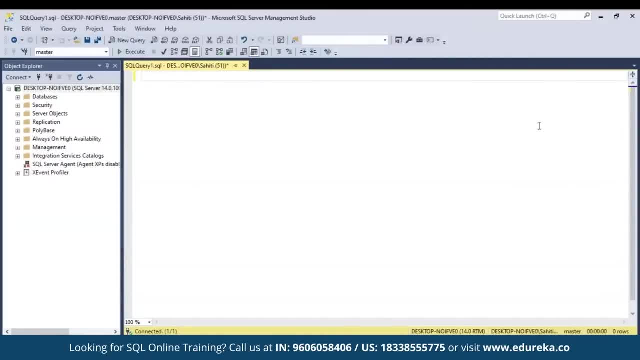 opens up. Let me just zoom in a little bit. So now that I've zoomed in, let's get started with the session. So initially, what I'll do is I'll just create a database. So to create a database, you'll type in a command: create database. 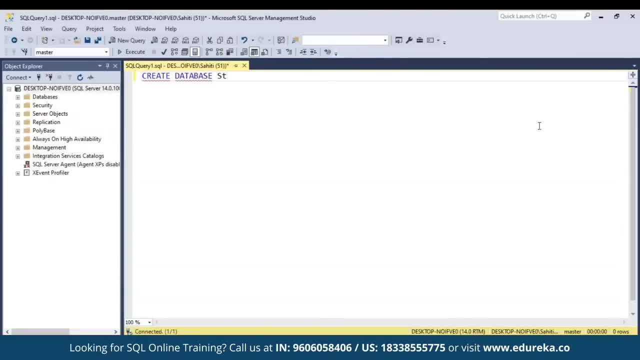 and then you'll mention the database name, right? So let's say, I mentioned the database name to be students. Now, after that, you just have to select this particular statement and click on execute. Now, once you click on execute, you clearly see that. 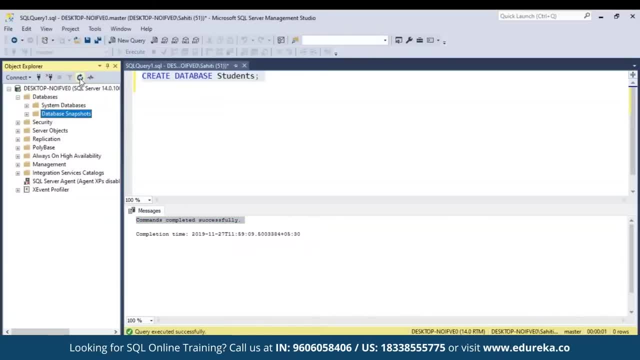 you know the commands have completed successfully, So our database has been created. if I just refresh this particular section and then I go to databases, You see that you know we've got a student's database right. So now to perform any action in a database. 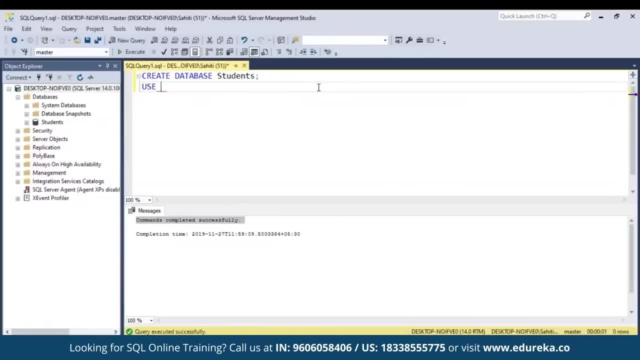 you have to first use that database. So for that you'll just type in use and then you'll mention the database name to be students, right. And then what you'll do is you just execute again, right. And once you execute again, 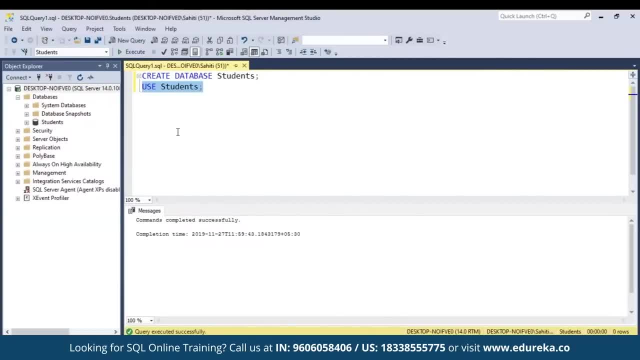 you'll see that you know the commands have been successful. So that means whatever actions that you're going to perform is going to happen under this particular database. Now, after that, what you can simply do is you can just create a table right. 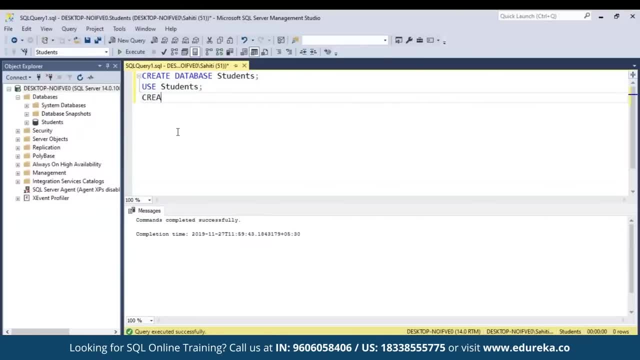 So to create a table again, you just have to use this command of create table right. So I'll just mention create table and then you can mention the tables name. So let's say we just mention it to be students info right. 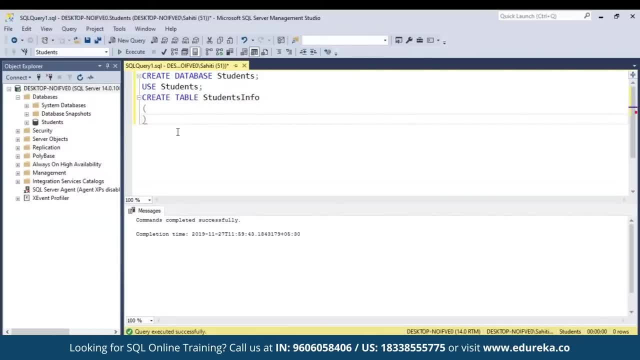 And then in brackets, what you have to do is you have to mention your column names and its data types. So the column names could be like student ID, Let's say it to be of int. right. next Let's say student name, Let's say varchar of 8,000.. 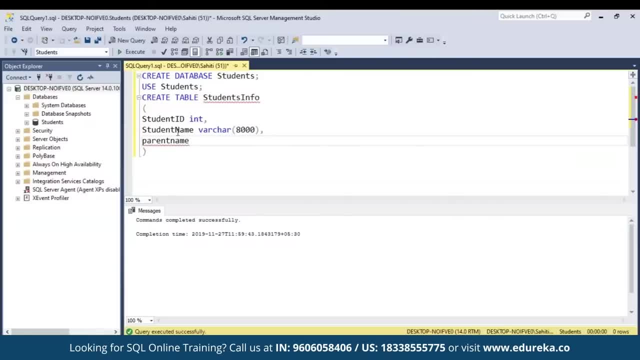 Similarly, we can have parent name Again of varchar, let's say 8,000.. After that you can have phone number: Let's say big int, because it's going to have a large value. After that we can have address of a student right. 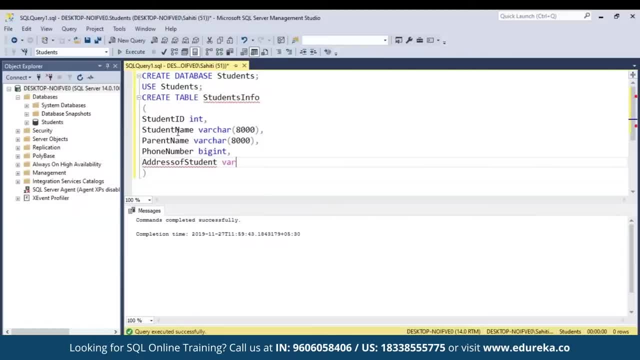 So I'll just mention address of a student, again varchar, Then I'll mention city, Let's say varchar of 8,000.. Then I'll mention country, again of varchar of 8,000.. After that you can just close this, and then, once you do, 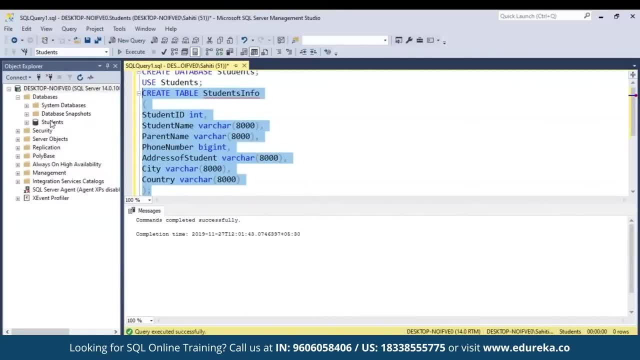 you can just execute this particular statements. So after the statement is executed, what you can do is you can just refresh this particular section. go to databases, go to students and in students you'll see that. you know if you go under the table section. 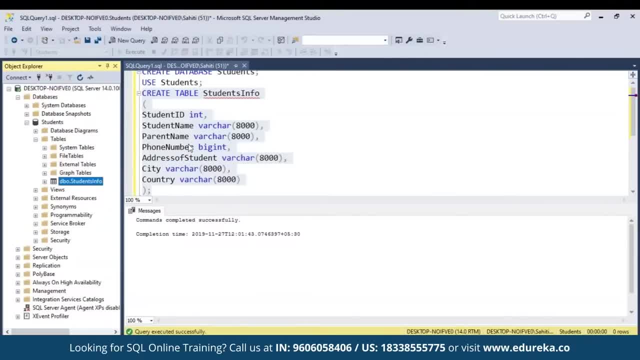 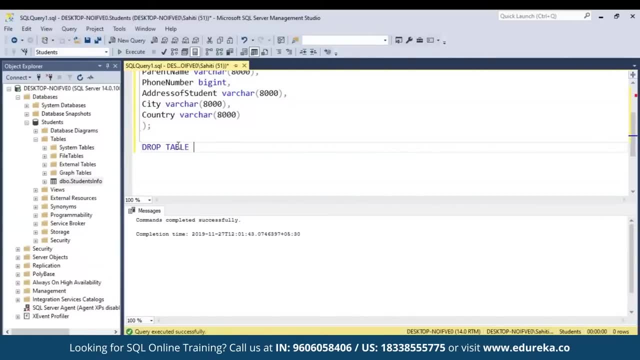 we find a table of students info. So that's how, guys, basically you can create a table also Now, for example, let's say you want to drop a table. now, dropping a table is also similar. You just have to use the command drop table. 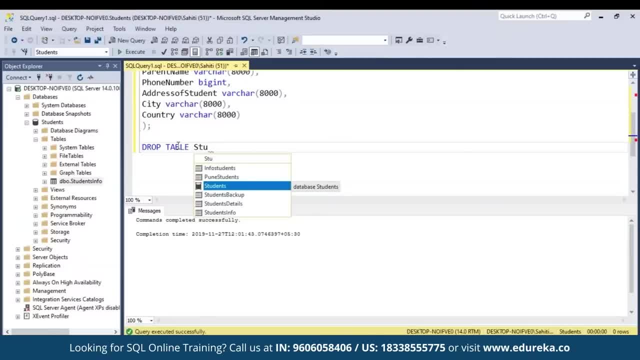 and then you mentioned the tables name. So it has students info, right. So I'll just mention students info, right, And then what I'll do is I'll just execute once I execute and then, if I refresh, you'll see that you know, table is gone. 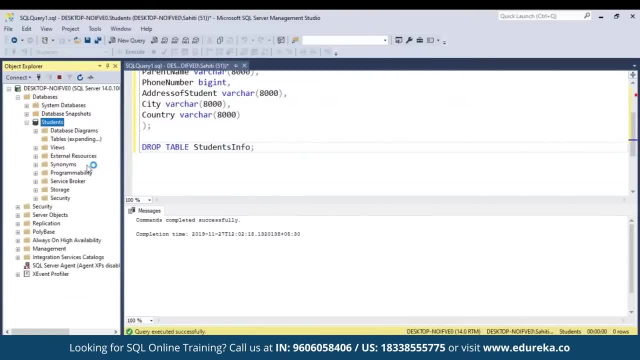 So let's just wait for it to happen. If I go to table section, you see that there is no table present. So that's how, basically, you can create a table and drop a table now. Similarly, you can also drop a database also. 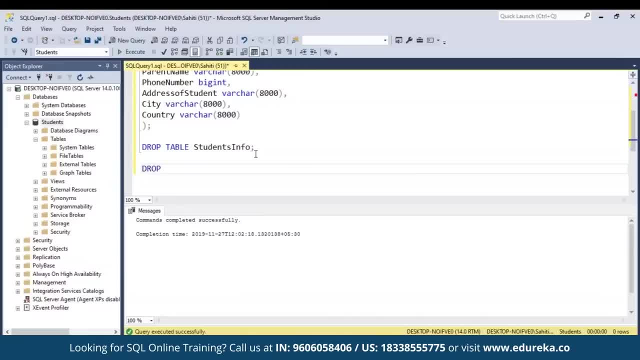 So to drop a database, what you have to simply do is you just mention drop database and then you mentioned the database name, which was students. So I'll just execute and then, once I execute, you see an error that you know we cannot drop the database. 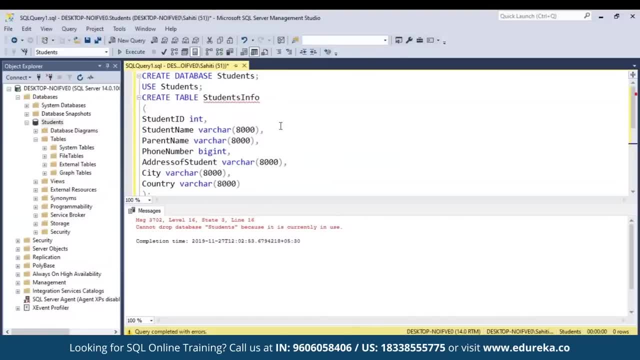 because it's in current use, right? So what you can do is you can just create another database, Let's say students one, and then we use students one and then you can go back and drop this database of students, right? So once you drop this database of students, 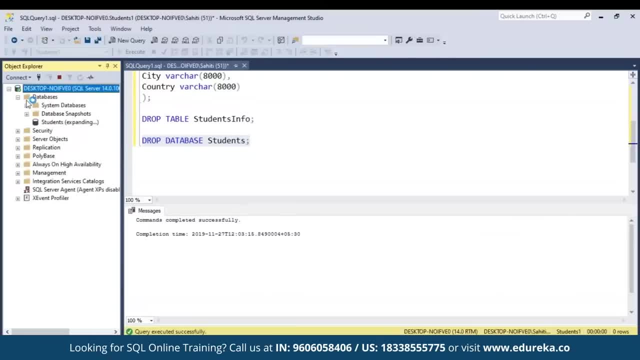 you'll see that. you know new database has been created, that is students one, and the students database has gone right. So let's just wait for that to happen, right? So, as you can see, we just have one database, that is students one, right. 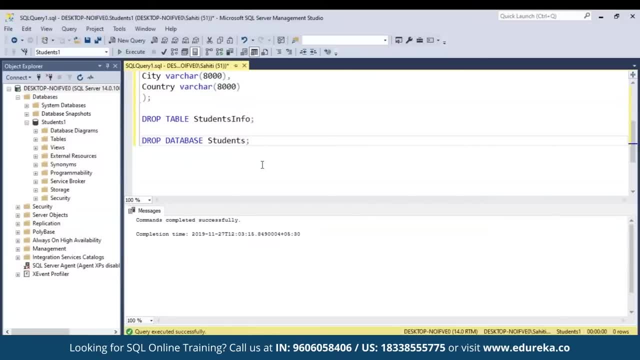 So that's how, guys, basically you can drop and create the databases and the tables. now the next command that you need to know in the DDL commands is the alter command. But before we start with the alter command, what I'll just do is I'll just use this particular database. 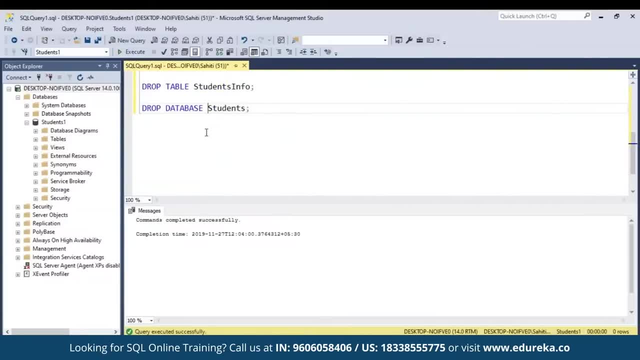 and then I'll just create back this table again, right? And then what I'll do is I'll just write the alter command. So, for example, let's say you want to add a column of blood, right? So what you'll do is you'll just mention alter table. 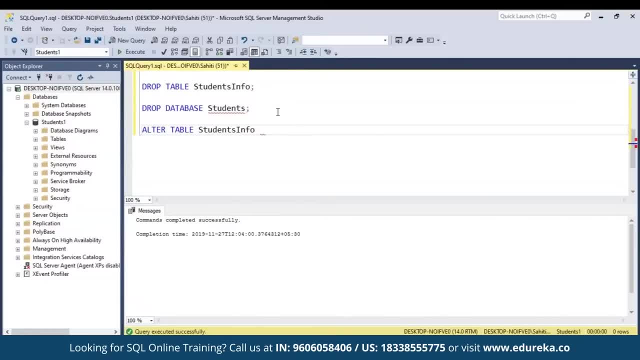 Then you'll mention the tables name, that the students info, and then you'll mention add blood group. So that is basically a column name that we want to add. and then we'll mention varchar of 8000 right and then I'll click on execute. once I click on execute, 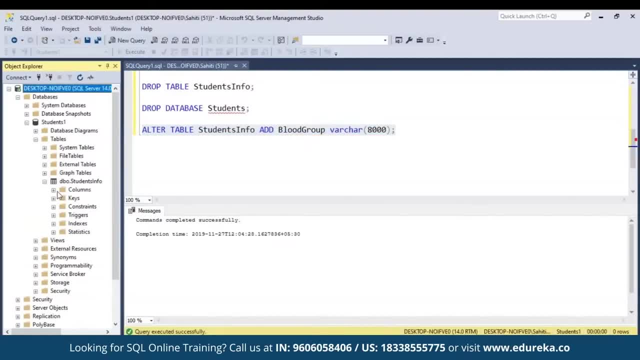 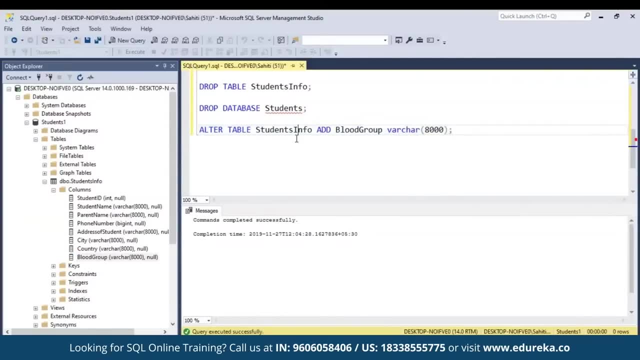 and go to tables, and then, once we go to this particular table and go to columns on the left hand side, you clearly see that our blood group column has been added. Similarly, you can drop the same column also. So what you'll do is you'll just copy paste this right. 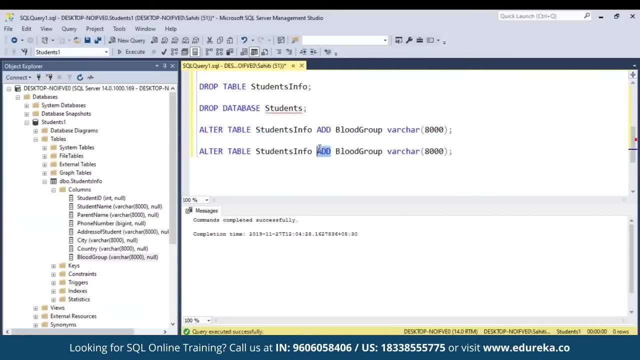 and then what you'll do is you'll just change the add function to drop function, Right? so you'll mention alter table and then you'll mention the tables name and then you'll mention drop and then you'll mention blood group, varchar, right? So if I just execute this, 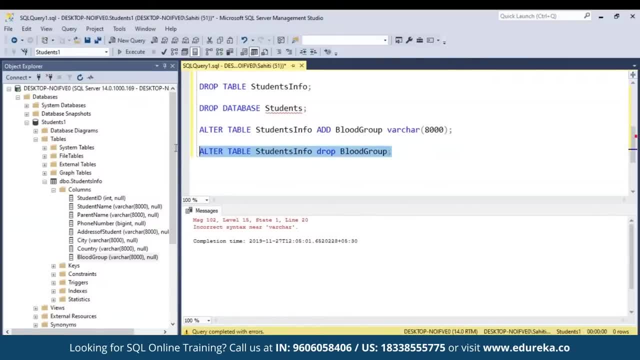 oh, I'm sorry. I have to remove this particular data type also because we're not creating the column right, So I'll just execute this particular statement again. All right, It says blood group is not a constraint. Now, This is one of the most common errors, as you know. 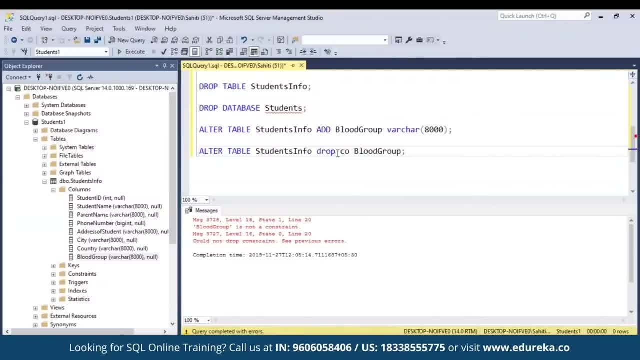 people just remove the command and then try to remove that column. But what you have to do is you have to mention that it's a column, right? So for that you'll mention alter table, table name and then you'll mention drop column and then the column name. after that you'll click on execute. 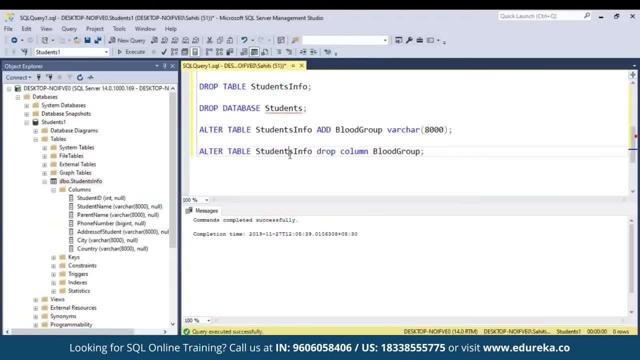 and then, once you click on execute and refresh, you see that our blood group column has gone. So that's how, basically, guys, you can add a column or you can delete a column. now, for example, let's say you want to add a column and then you want to change the data type also, right, 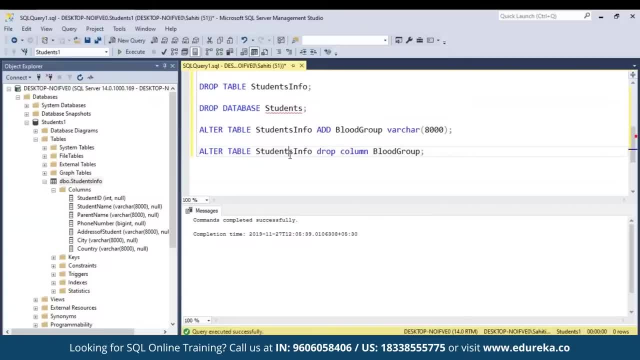 So you want to do both. you want to add a column and then you want to change the data type also. So what you'll do is you'll just mention alter table, We'll just copy paste this particular statement and then we'll mention all the table. students info. 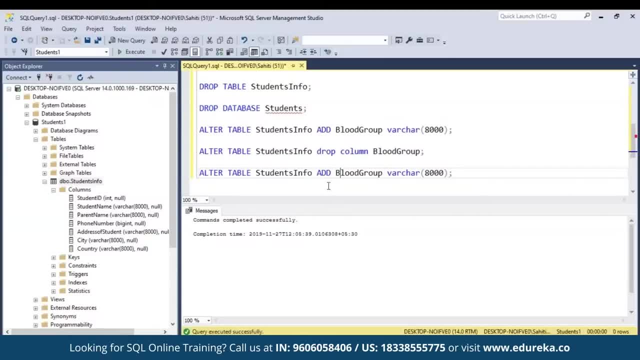 that is basically the table name. and then let's say we want to add a date of birth column, right? So I'll just mention DOB over here, Right? and let's say our data type to be date, right? And then I'll just execute. once I execute, you see that. 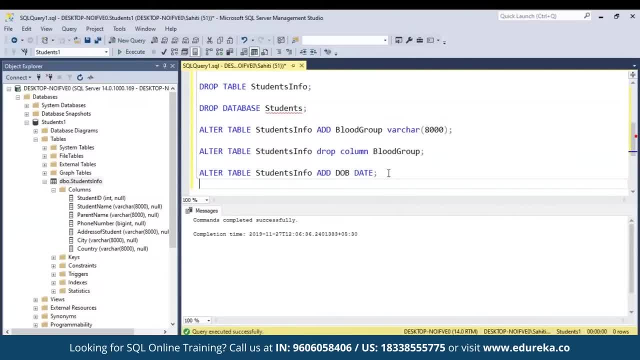 you know our column will be added. Now what I'll do is I want to change the data type, right, So to change the data type. what you do is we copy paste the statement again and then I'll just remove this particular part and I'll mention alter column. 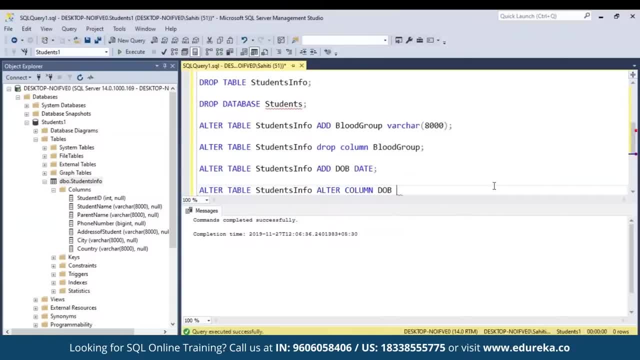 and then I'll mention column name- So that was date of birth- and then I'll mention the new data type, Right? So let's say I want it to be date time, right? So I'll just mention date time and close right. 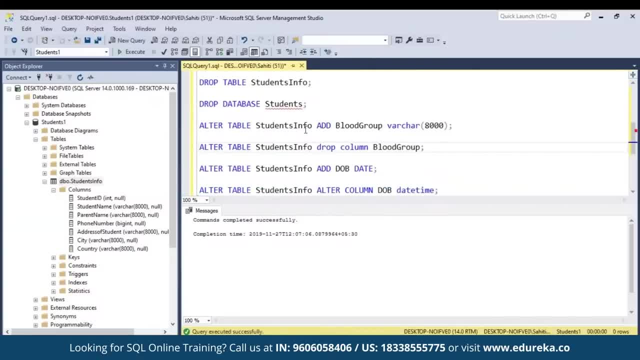 So that's how, basically, you can play around with DDL commands, guys. It's very easy and it's very interesting to learn with. so, guys, that was about the alter command. Now let's say, you know you want to truncate a table. 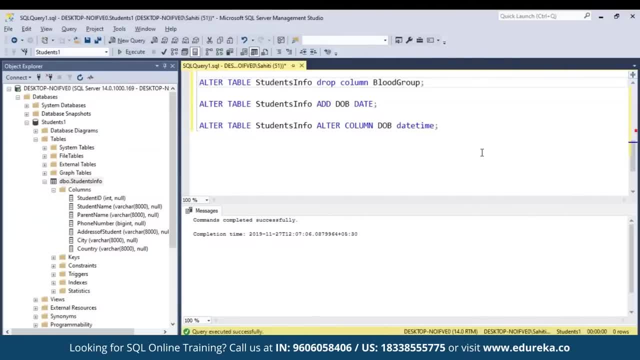 So when I say truncate the table, what I mean by that is that you know you want to delete the information present in the table, but the table itself is not deleted. But before that let's just include some information into the table. So to include information you have to mention- insert. 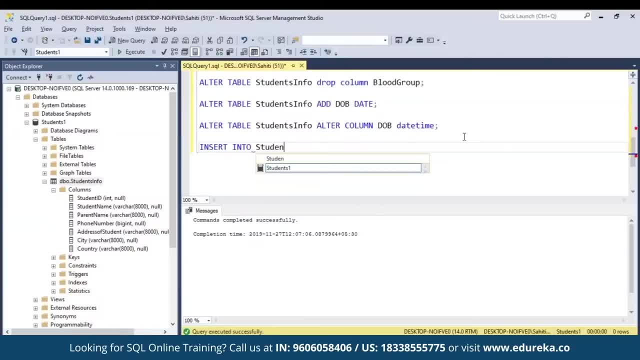 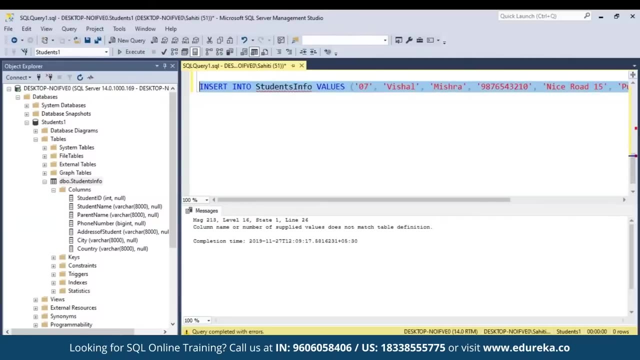 into. and then you'll mention tables name, right, So that students info, right. and then you'll mention values, and then let's say I mentioned few values, right, So I'll just mention, So I just execute this particular statement. Oh, it says column name. 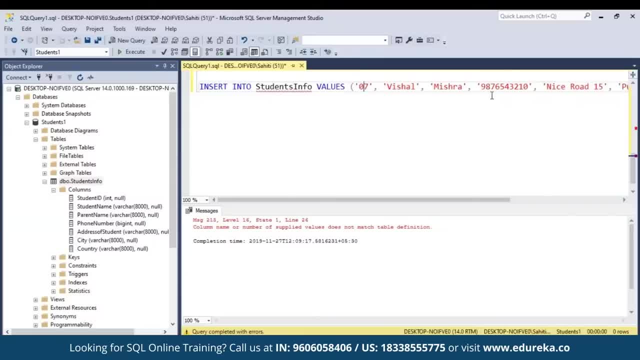 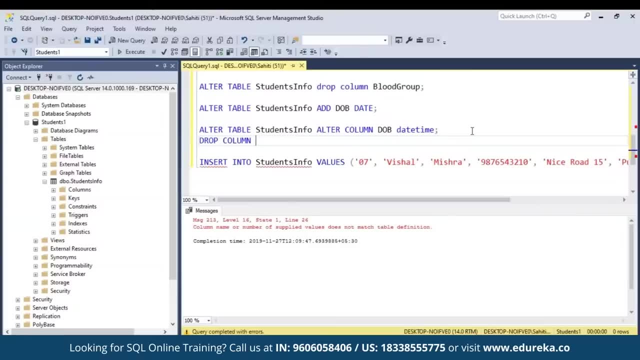 or number of does not match the table definition. We see this error because you know I forgot to drop the column of dob, So I'll just drop the column. So to drop the column, I'll just mention alter table. drop column and then I'll mention dob. right, 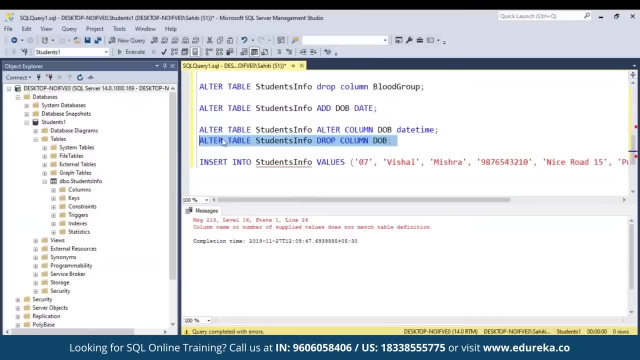 So let me just copy this particular section from here and then I'll execute the statement. and once I execute the statement, I'll execute the statement again, and then you will see that you know our values have been inserted now to truncate the table. What you have to do is you basically have 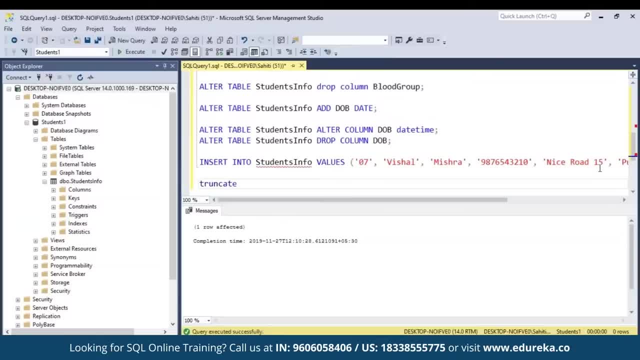 to use the syntax of truncate. So you'll just mention truncate and then you'll mention the table name. Our table name is students info, So I just mentioned students info and then I click on execute. Once I click on execute, we see that you know. 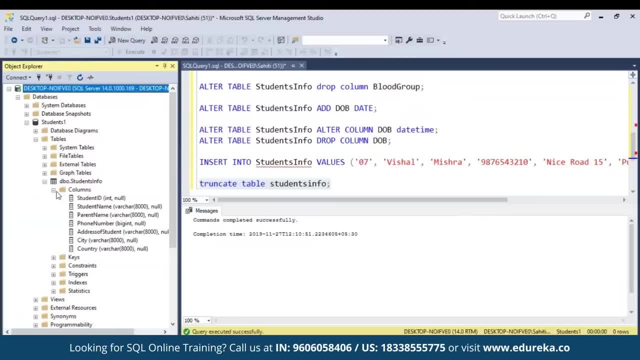 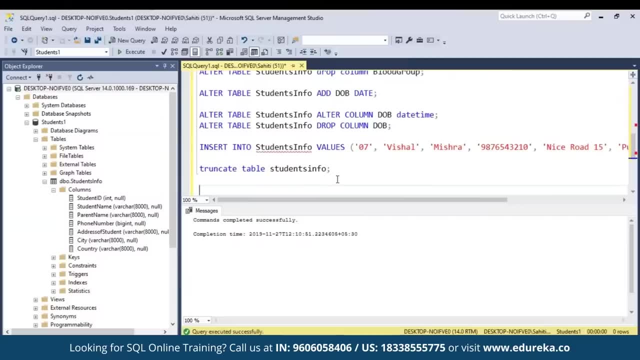 the commands have completed successfully. right initially Our columns have few values, but now our columns have no values over there. right apart from this, if you want to also rename a table or rename a database, you have to use the command of SP underscore rename. 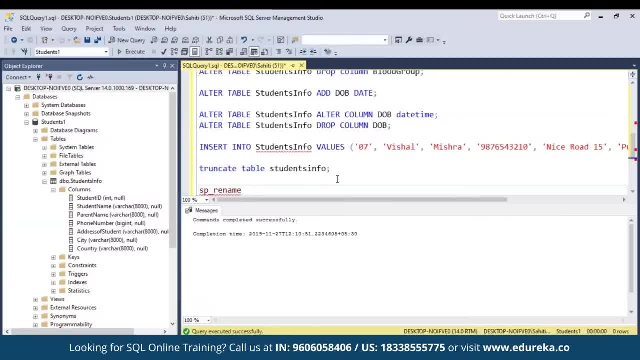 So this is something different from the other databases, as generally the rename command or the query is used, but in sequel server you have to use SP underscore rename, and then you'll mention students- one that is basically a database name- and then you'll mention students info and now you'll mention what you want to change it to right. 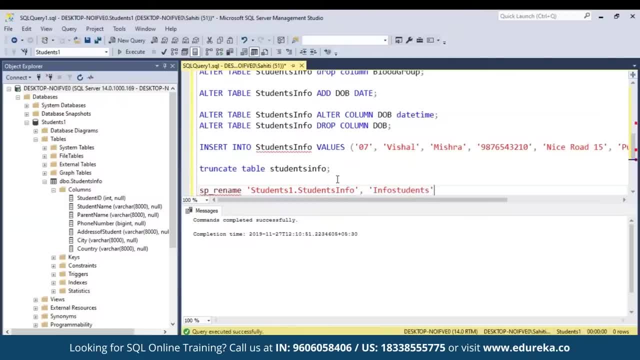 Let's say we want to change it to info students, Right, and then let's just execute. Okay, it says it cannot find, so I'll just remove this particular part and execute. and once I execute, you can see that you know our table name has changed. 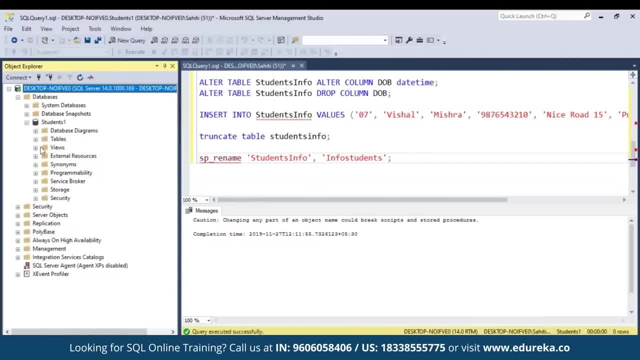 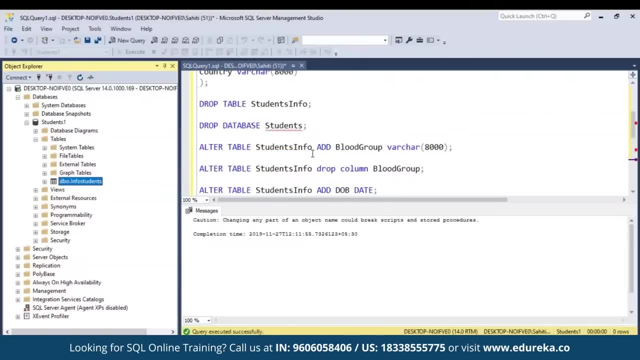 So what I'll do is I'll just refresh this left hand side and I'll go to students one. I'll go to tables over here and then you can see that you know it has changed to info students. So I hope I'm clear with the DDL commands, guys. 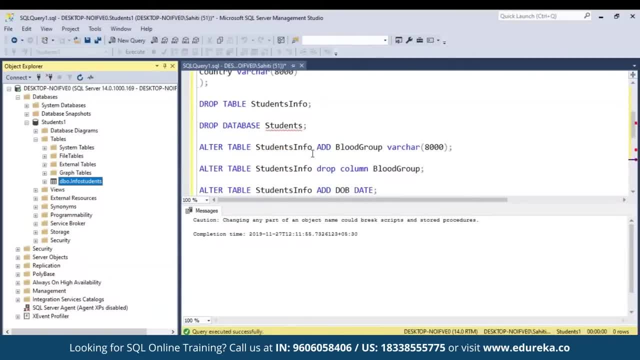 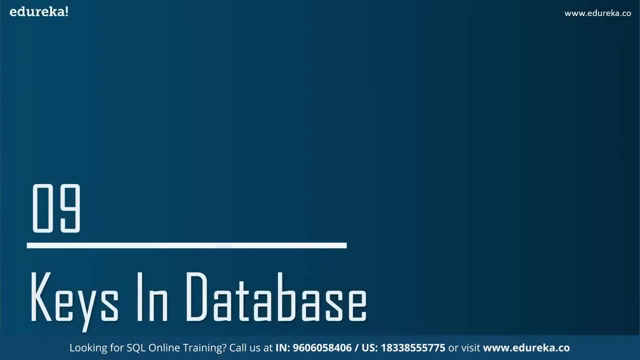 Well, these are few basic commands that you need to know before you start handling and manipulating databases. on that note, Let's take a look at the next topic for today's session, That is, keys in the database. Now, the different types of keys used in the database. 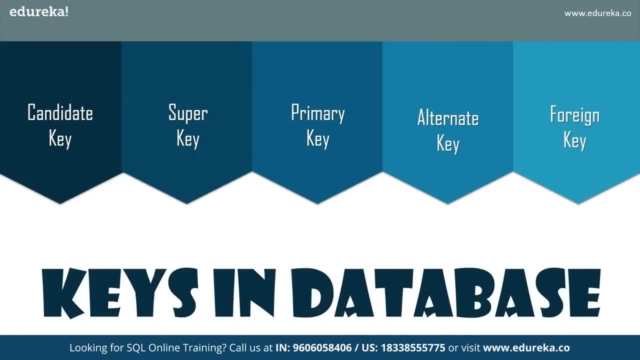 are the candidate key, the super key, the primary key, the alternate key and the foreign key. now coming to candidate key, candidate key is a set of attributes which can uniquely identify a table. So a table can have more than a single candidate key and out of the chosen candidate keys, a single key is chosen. 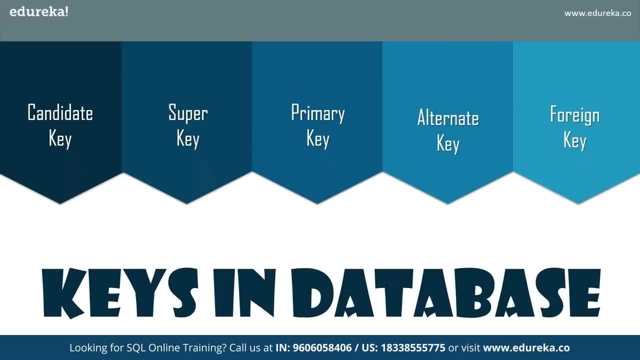 as the primary key. coming to super key, This is a set of attributes which can uniquely identify a tuple. So candidate key is unique keys and primary keys are super keys, but the vice-versa isn't true. coming to primary keys, The primary keys are used to uniquely identify every tuple. 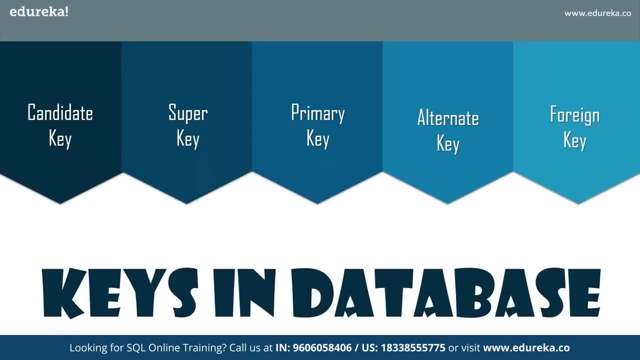 So a table can have only one primary key and that key will identify every tuple uniquely in the table. moving on to alternate key, The alternate keys are those candidate keys which are not chosen as the primary key. and finally, coming to the foreign key, The foreign key is an attribute. 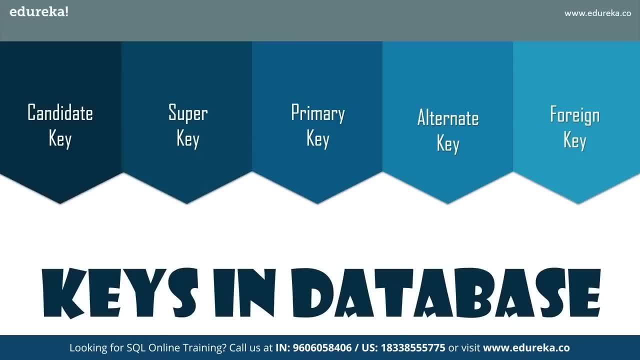 that can only take the values present as the values of some other attribute, and that is the foreign key to the attribute to which it refers. So, guys, these were the various types of keys in database. So it's completely based on your understanding or how you want to design your database model. 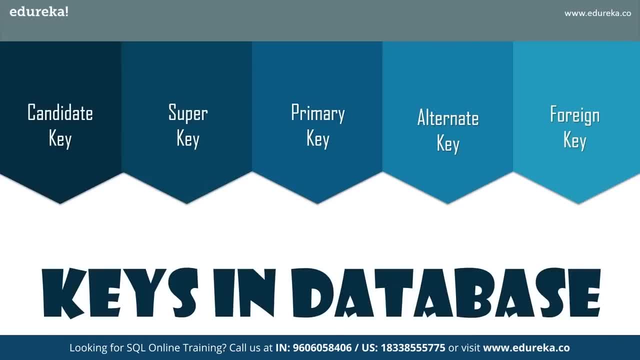 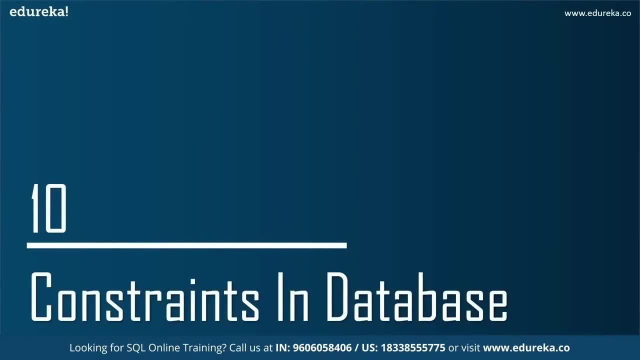 that which key should be primary key and which keys together can uniquely identify your table, and so on. apart from this, We also have few constraints which are very popular in the database. So next in the session, let's take a look at the popular constraints available. 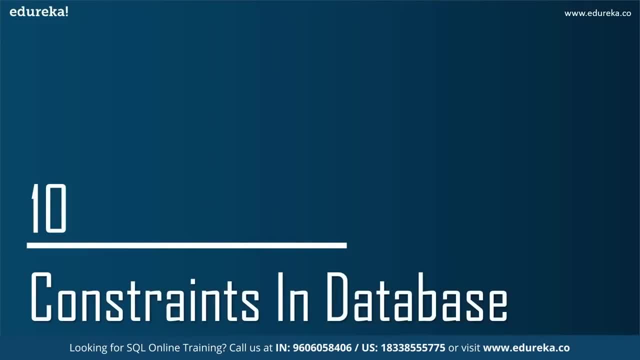 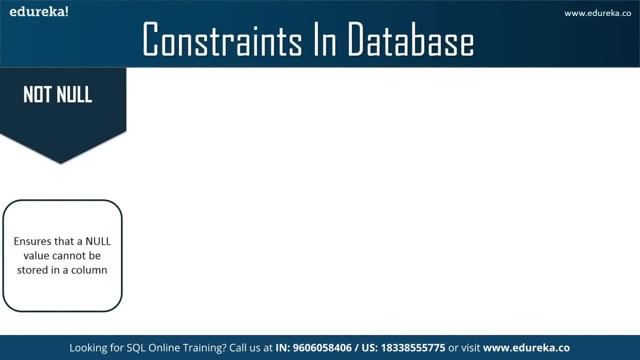 in the database. So the constraints used in the database are not null: unique, check, default and index. talk about not null first. the not null constraint ensures that a column cannot have a null value, right? So that is very simple. as the name suggests, It ensures that you know a column cannot have any null value. 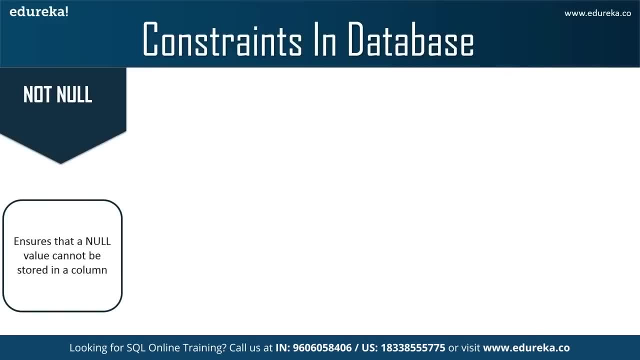 So if you just assign the constraint of not null to any particular column, then automatically you have to mention a value into that particular column. to enter that particular tuple into the database coming to you need the unique constraint. make sure that you know all the values in the column are different. 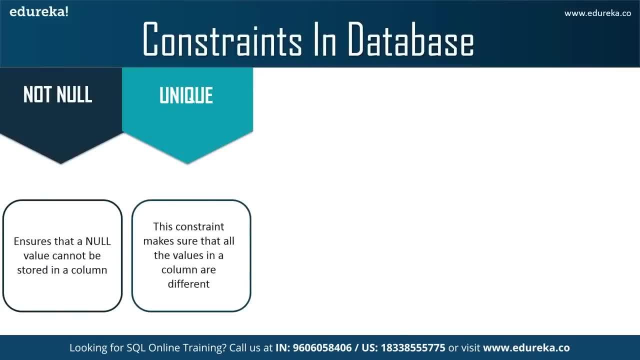 So, basically, when you mention a constraint unique to a specific column, then automatically what happens is that all the values present in the column are unique, So two or more values cannot be the same. coming to check constraint, this constraint ensures that all the values in a column satisfy a specific condition. 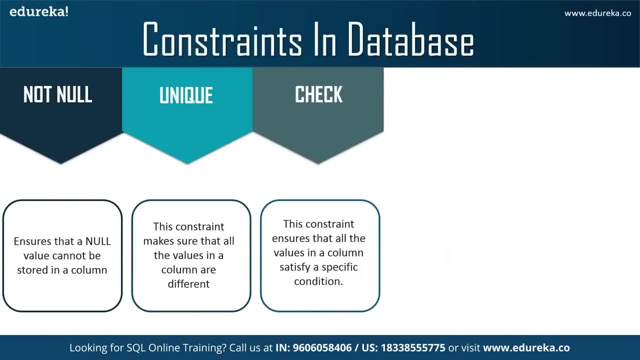 So, whenever you mention the check constant, you'll mention a condition and all the values which satisfy the condition can be present in that particular column. any value which doesn't satisfy and the condition cannot be present in that particular column. going on to default, Well, this constraint consists of set of default values. 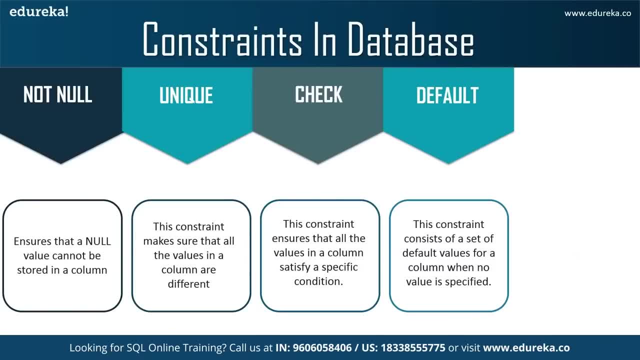 of a column when no values is specified right. For example, let's say, while entering values in a column you forget to mention a few. but yes, while creating the table or maybe while adding a constraint, you add the constraint of default for that particular table. 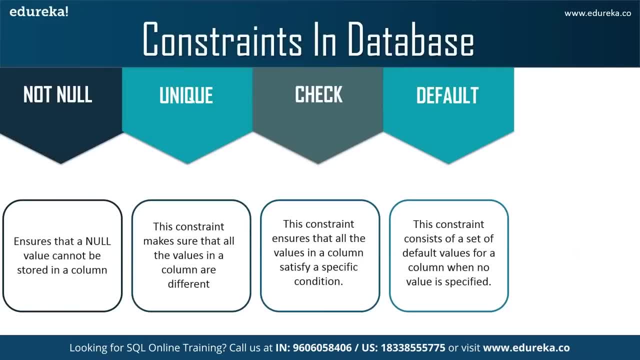 Let's say 10, so all the places where you do not mention any value 10 will be automatically added to that particular places. and finally, coming to the last type of constant, that is, index. this constant is used to create and retrieve data from the database very quickly. 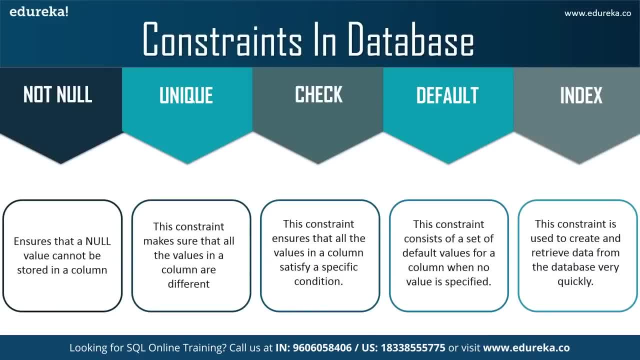 right. if you want to create and retrieve data from the database very quickly, then you have to use the index constraints. So now that I've explained your keys and constraints in database, let me just switch back to my sequel server management studio, And then what I'll do is I'll just execute few commands. 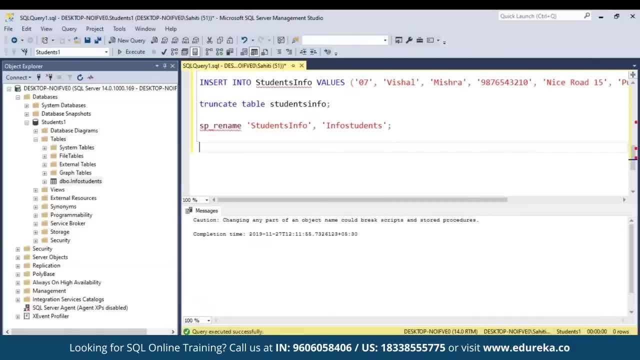 or queries based on this particular section. So let's get started. So what I'll do is I'll just copy this particular section from over here, right? And then let's say I just add a segment so that it's clear to us, and then I'll copy paste over here. 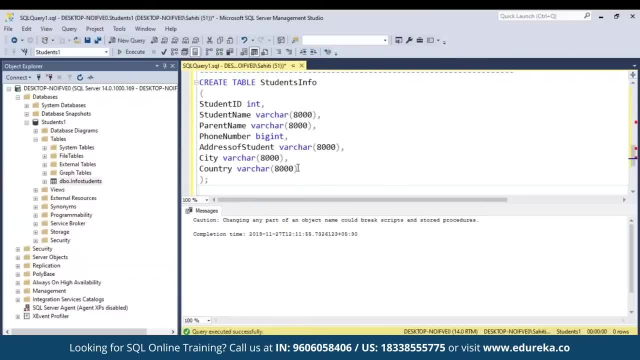 And now let's say we want to use the not null constraint. So, for example, let's say we want to make sure that you know the student name and the address of the student is definitely present, or maybe when the user is entering values. 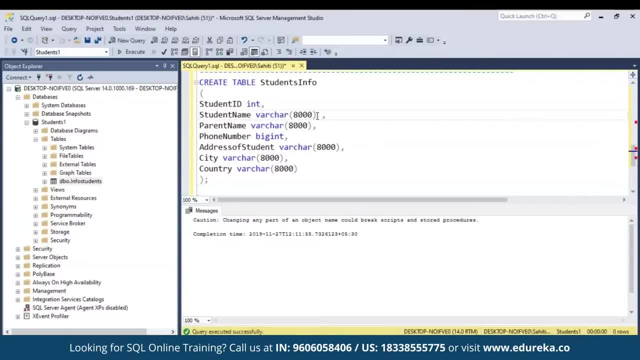 it's mandate for the user to enter the student name and the address of student, right? So then, what we'll do is we'll just mention: not no constraint over here, right? And again, I'll just mention: not null constraint over here. 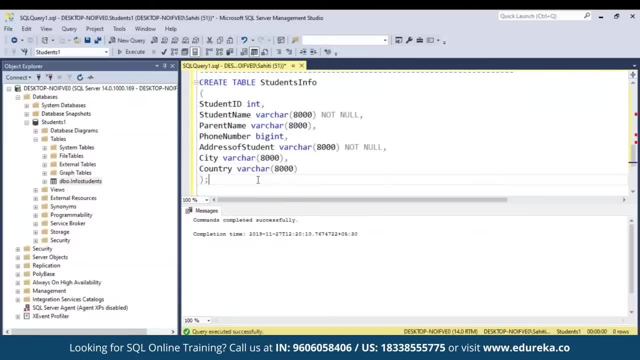 right, and then what I'll do is I'll just create this particular table right now. Once this table is created, what I'll do is I'll just copy paste this insert statement from over here. I'll paste this and let's say: you know, I just remove the address part, right? 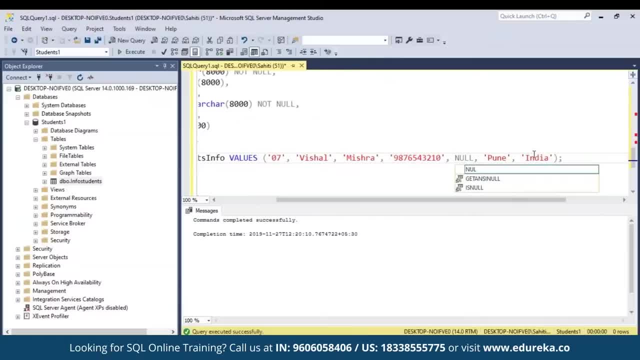 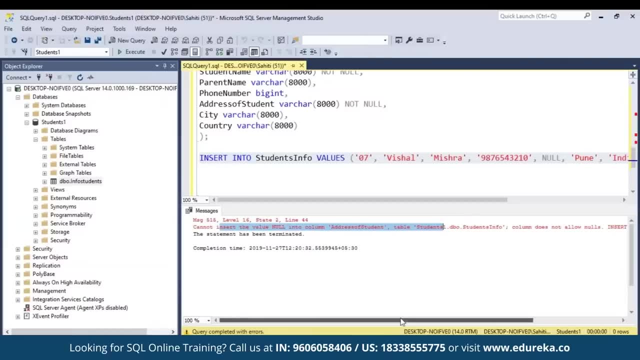 So I'll just remove this particular section and then I'll mention null and then I'll click on execute. when I click on execute, You can clearly see the error that you know cannot insert the value null into the column, because you know the column does not allow. now. 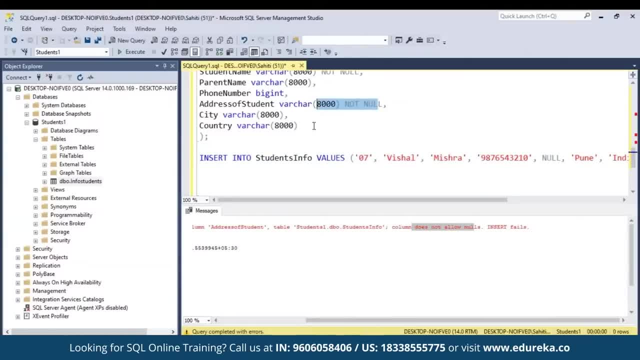 that is because we have given the not null constraint to the address column right. So that's how, basically, you can use the not null on create table Now. Similarly, if you want to use not null on the altar table, what you basically have to do is you just have. 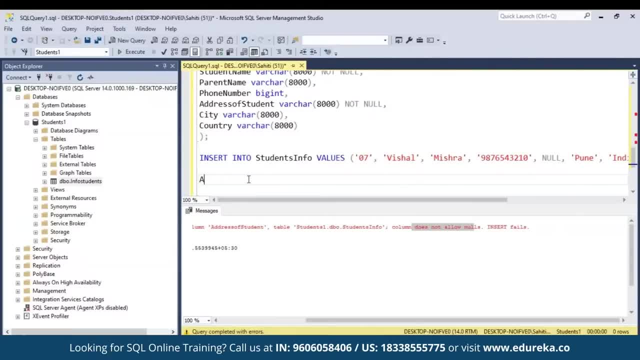 to mention the altar table statement and then at the end you have to mention not null. for example, let's say I want to mention altar table students info Right, and then I'll mention let's say all to call him, and then I'll mention phone number. 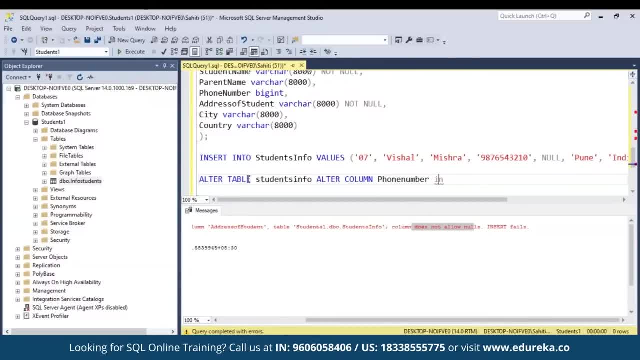 Right. and let's say I mentioned: ain't sorry, ain't not- null Right, and then I'll just click on execute and once I click on execute, you can see that you know the command has been successful. So, whatever happens, you cannot mention the null values. 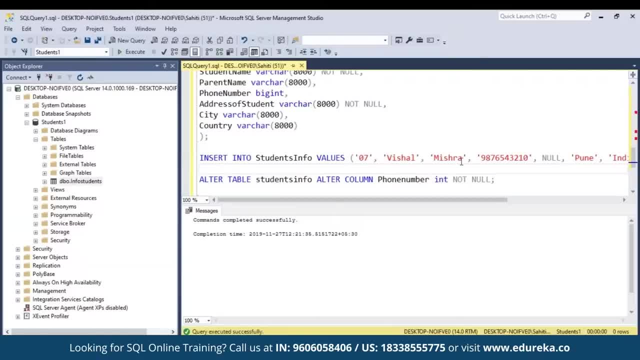 in the phone number column. So, guys, that's how basically you can use the not no constraint on the create and the altar table. Now let's move forward with the next constraint. that was the unique constraint. also, while working on the unique constant, Let's just check how to add the primary key. 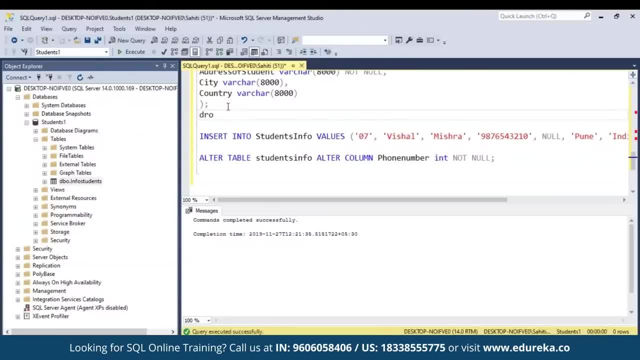 So what I'll do is I'll just drop this particular table. So I'll just mention: drop table, students, info, Right, I'll just execute right. and then what I'll do is I'll just copy paste this section, paste it over here. So what I'll do is I'll just mention the unique constraint. 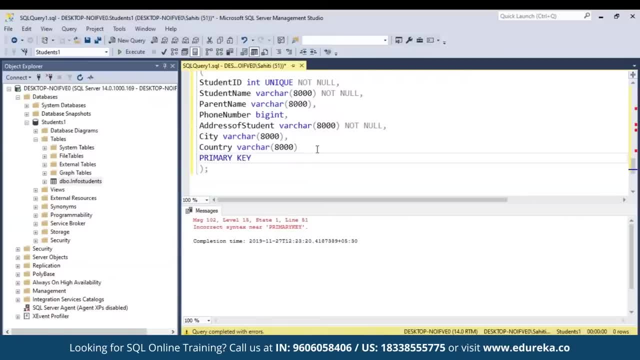 over here. And then what I do is I'll mention primary key And in brackets I'll mention student ID. right after that I'll just click on execute And once I click on execute you can see that you know the student ID will be unique. 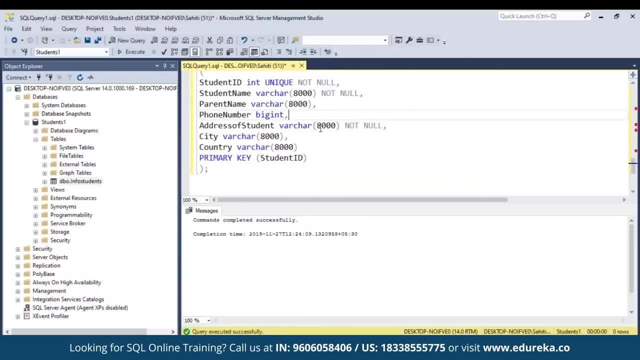 So every ID will be unique and since every ID will be unique, it will uniquely identify every tuple. so that could be the primary key. So that's how, basically, you can add the unique constraint for a single column. Now let's say you want to add unique constant. 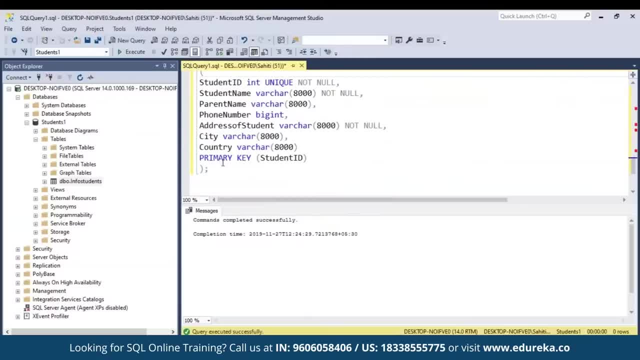 for multiple columns, right? So, similarly, what I'll do is I'll just drop this table again. I'll copy paste the section, paste it over here, remove the student ID and remove unique constraint from over here. And then what I'll do is I'll just mention constraint, right? 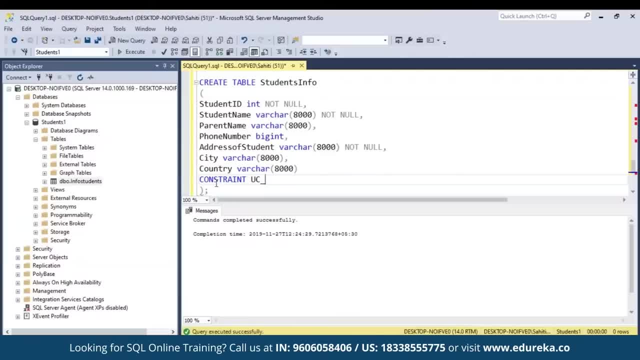 and then I'll mention the constraint name that I want to give. so it could be, you see, let's say, students info, and then I'll mention unique, and in the brackets I'll mention student ID. and let's say, we want the phone number also to be unique. 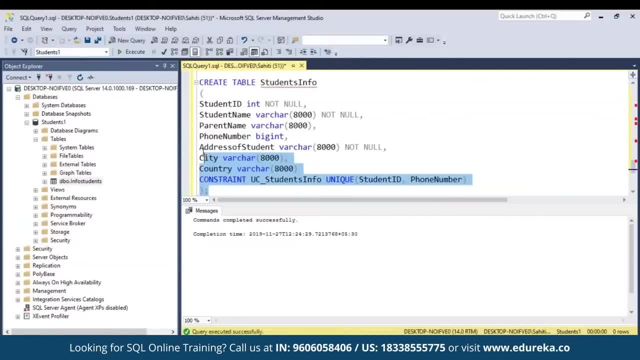 right. So we'll mention a phone number, right, and then what I'll do is I'll just execute again. So once I execute again, you can clearly see that you know we are. table has been created. So if I just refresh on the left hand side, 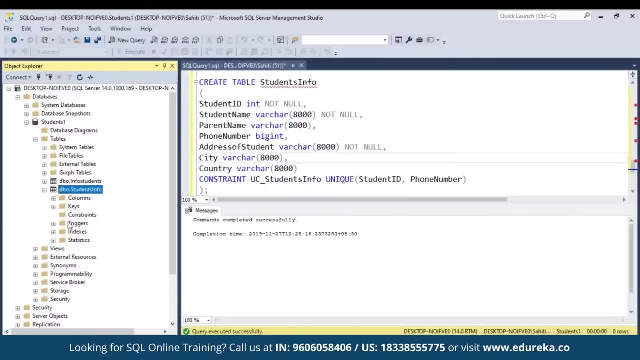 Right, and then what I'll do is I'll just go to the constraints part over here, or you can go see that. you know, if I go to the column section over here, you can see that our constraints are clearly visible on the left hand side over here. 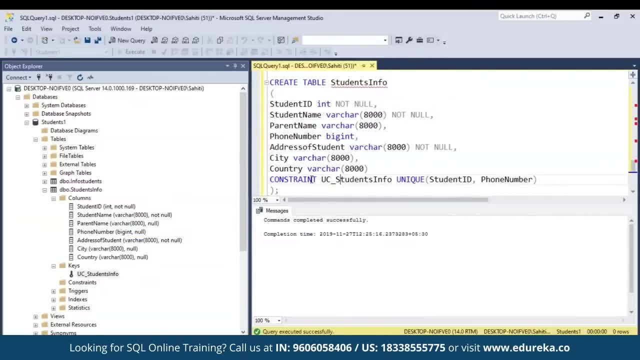 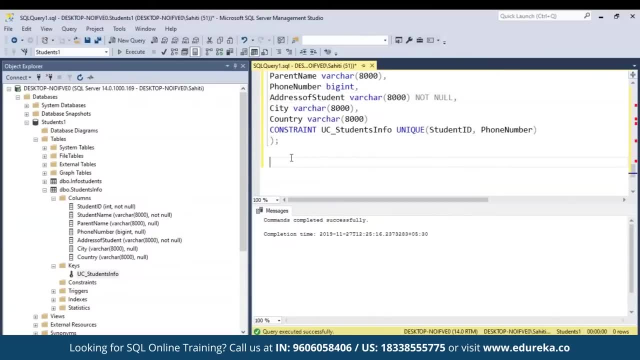 Also, if I go to the key section, we can see that in our students info, constant, which I just mentioned over here, is clearly present over here. So that's how, guys. basically, you can add unique constraint on multiple columns. Now, similarly, if you want to add unique constant, 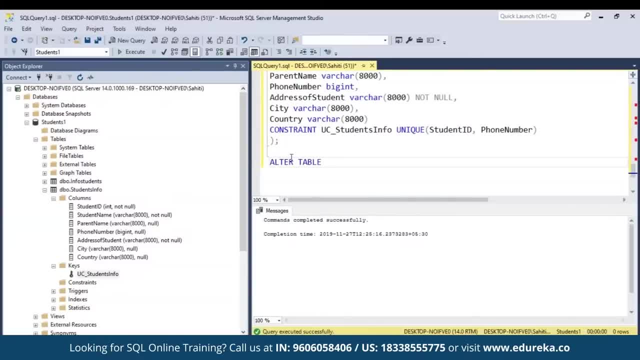 on an altar table. it's very simple: You just have to mention altar table and then what you do is you mentioned the tables name, as a we previously did, and then we'll mention add and we'll mention the constraint- that is unique Constraint- and over here will mention the column. 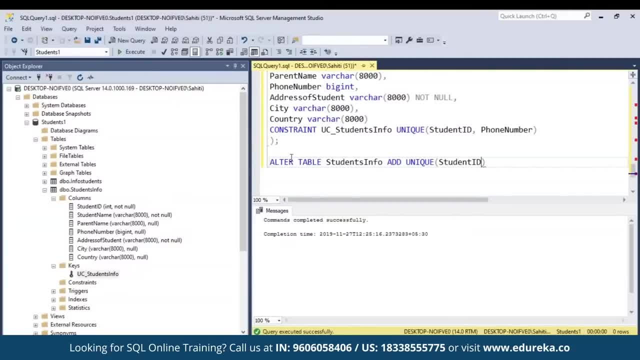 on which we want to add the unique Constraint. right, So I want to add it on my student ID, So I'll mention student ID and then I'll just execute: right, So that's how, basically, you can add a unique constraint on an altar table. 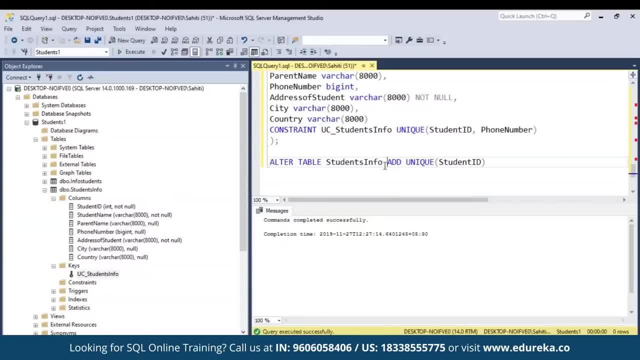 Also the. similarly, if you want to drop the constraint also, guys, you just have to mention all the table and then you'll mention students, info, and then what you'll do is you'll mention drop and then you'll mention constraint and then you'll mention the constraints name, right? 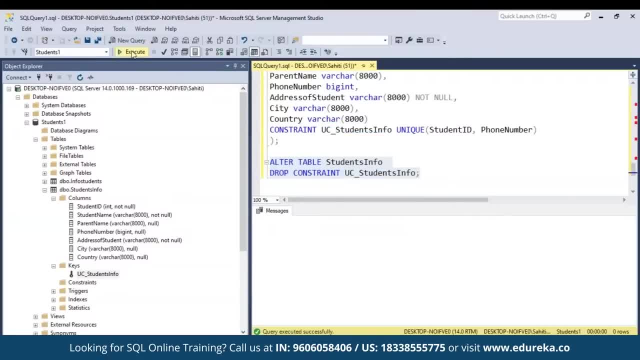 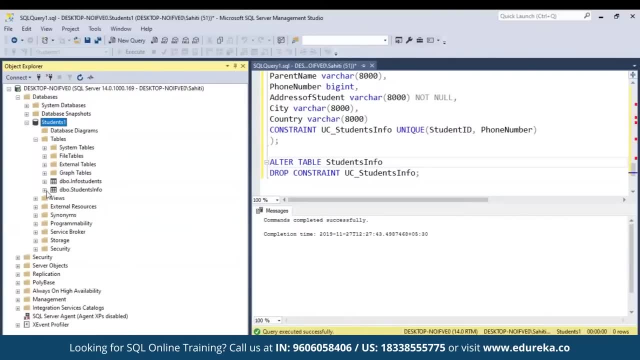 For example, let's say I'll mention this particular name and then I'll just execute the statement. Now, if I just refresh this left-hand side and let's just open again, So I'll go to tables, I'll go to students info and then, if I'll just refresh, 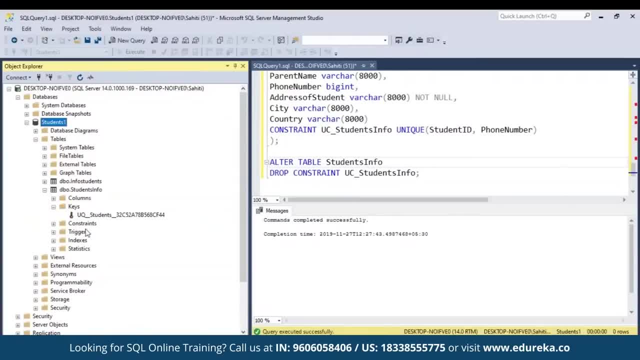 So go to tables, I'll go to students info And then, if I go to keys, we see that, you know, there's no UC students info constant present, but then this particular constant that we had just added before on the altar table statement, that is present. 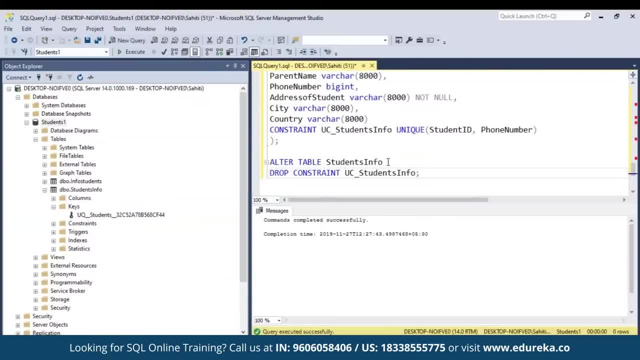 So that's how, basically, you can add the unique constraint. now let's move forward with the next type of constraint, that is, the check constraint. Well, the check constant, as I previously mentioned, is used to add a condition, right? So, for example, let's say: you know, 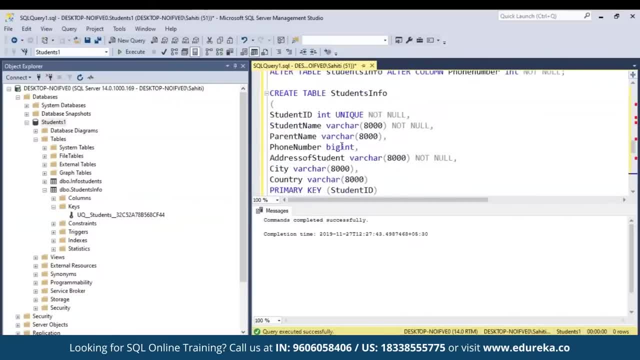 you want to add the check constant while creating the table itself. So to do that, what I'll do is I'll create a table, But before that, let me just drop this table again. And now, what we'll do is we'll just copy paste. 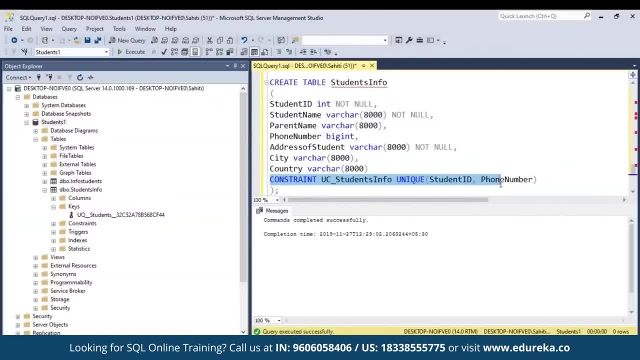 this particular section. put it over here, remove this part And let's say: you know we want our country to be India, So all the values which could be entered into the table must have the country value to be India, right? So we'll just mention check over here. 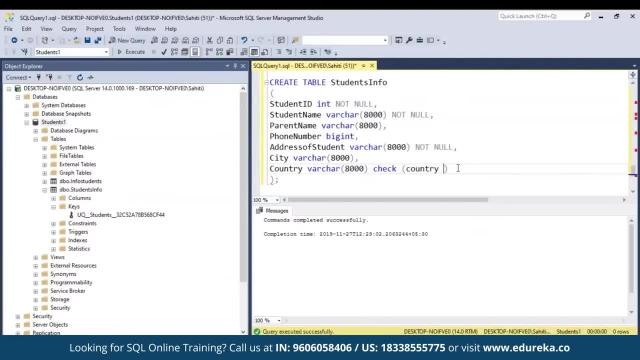 and then, in brackets, I'll mention country equal to, I'll mention India, right, And then what I'll do is I'll just execute this particular statement. So after that, let's say, if I want to insert a statement, So for that I'll just copy paste this particular section. 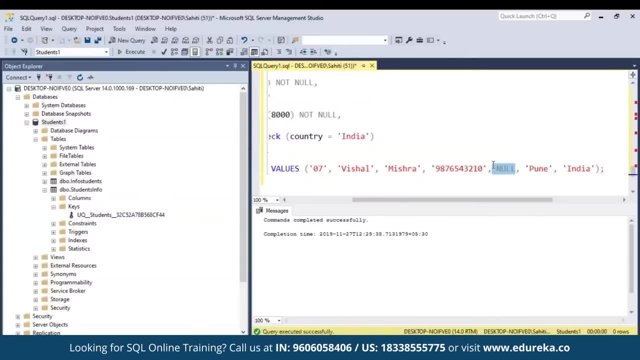 Let's say I put it over here, and over here Let's say I just mentioned any value like nice road, Right. and let's say we mention over here, Germany, right, And I'll just try to execute. and once, if I try to execute, 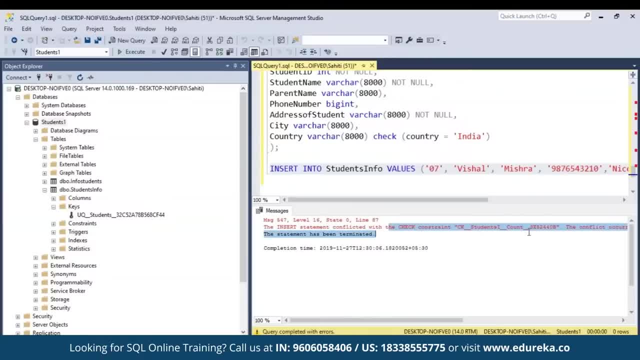 you can clearly see the error that you know. insert statement conflicted with the check constraint. the conflict occurred in the databases because you know the column country has to be India, right, And then we have mentioned Germany. So now what you can just do is you can just go back change. 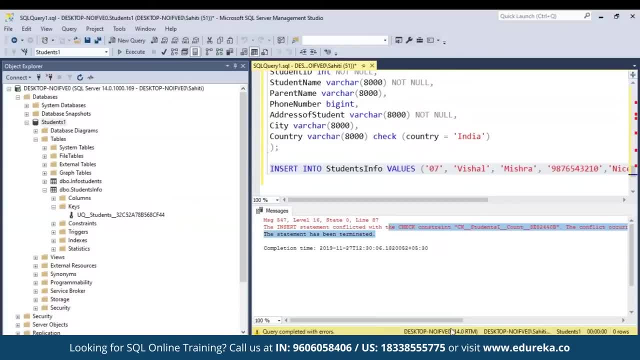 the country to India, and then you can insert the value. So that's how you can use the check constant on the create table. Now let's say you want to use the check constraint on the altar table, now similar to that of the unique constraint. 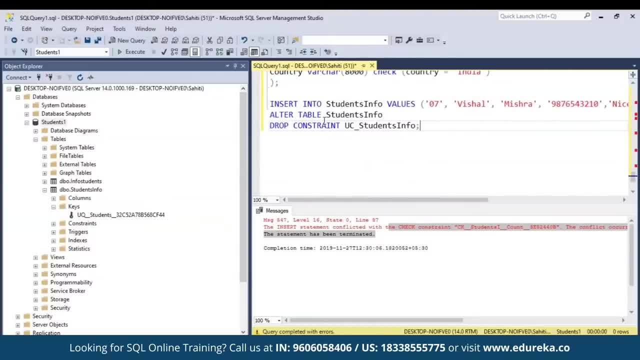 What you'll do is you'll just mention alter table and then you'll mention the tables name, and then what you'll do is you'll just mention add check And in brackets you'll mention country equal to India and then you'll execute. now, That's how, basically, you can add the check constraint. 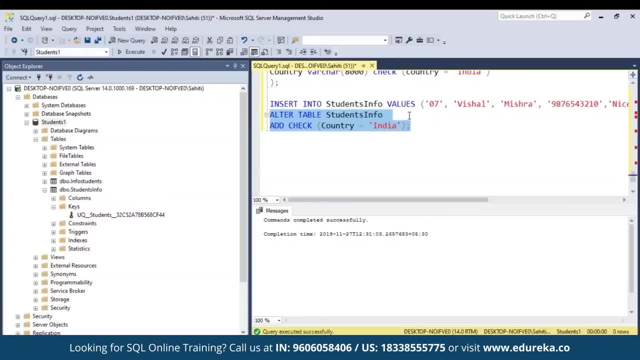 on the altar table. Similarly, if you want to give the name to the check constraint- but that's not necessary that you always give the name, But yes, if you're handling on an enterprise level and then you're handling a lot of databases, then giving a name must be. 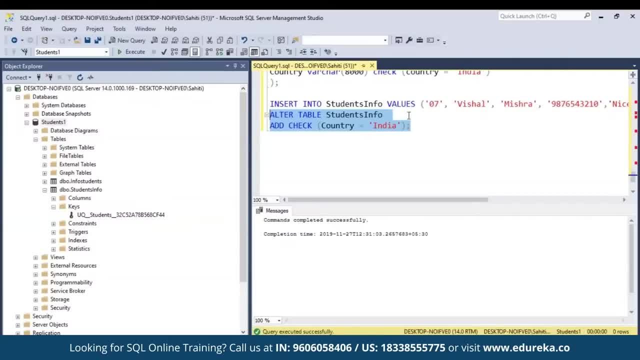 a priority right, so to add the name. what you simply do is you just use this alter table statement again, right, and then you'll mention the table name. and over here You have to add constraint, right, and then you'll mention the name. So let's say I mentioned the check. 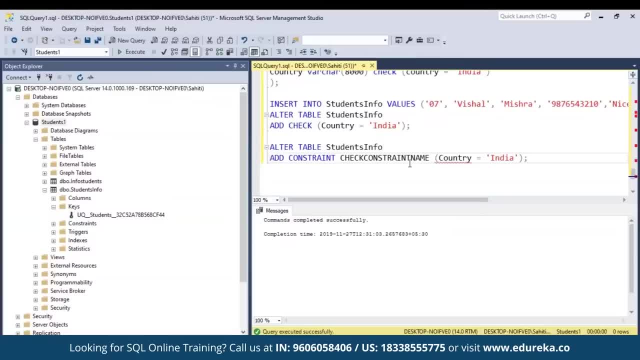 Let's say constraint name, right. and then what I'll do is I'll mention the check condition and that is India, right. So if I just execute the statement again, you'll see that you didn't completely works, and if I refresh on the left hand side, go to tables. 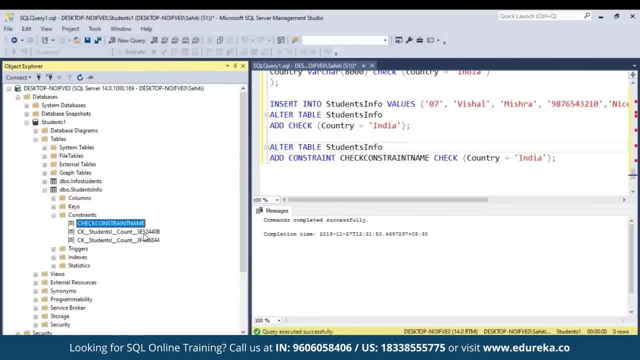 and go to students in for go to constraints. you'll see that in our constraint name has been added up right now. similarly, you can drop a constant will. dropping a constant is again Same. you have to use all to table students info and then you just mention drop constraint. 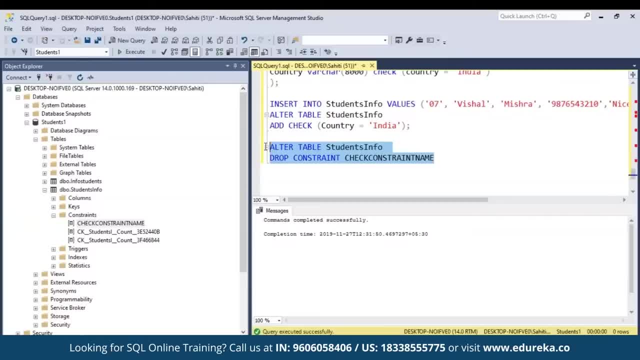 and I. you can just mention the drop constraint name. So I'll just execute this particular statement again and you'll see that in our constant has been dropped. So, guys, that was about the drop constraint. Now let's go forward with the default constraint. 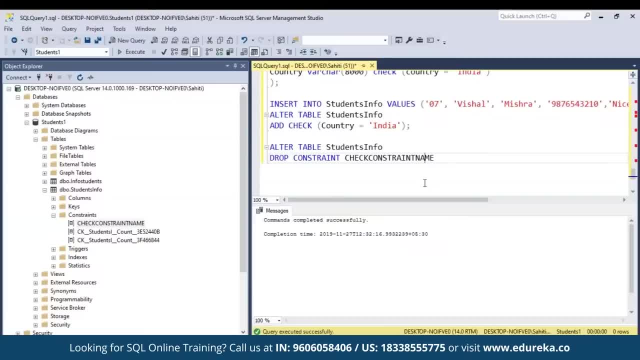 where the default constant, as I previously said, is used to add a default value. So what I'll do is I'll just drop this table again, right? And then what I'll do is I'll just copy paste the section, paste it over here. 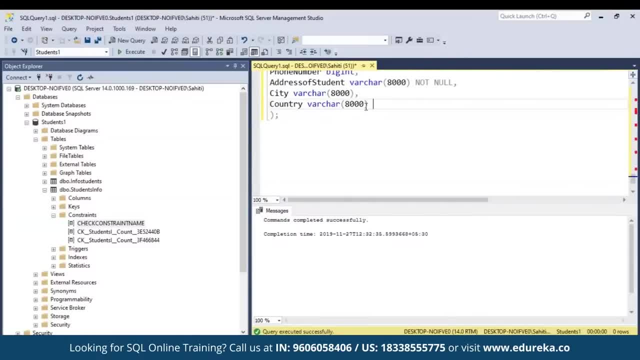 I'll just remove this particular section and then let's say our default country values: India, right? So I'll just mention default- Sorry, spelling mistake- and then I'll mention India. So basically, all the values which will be inserted into the table will have the default. 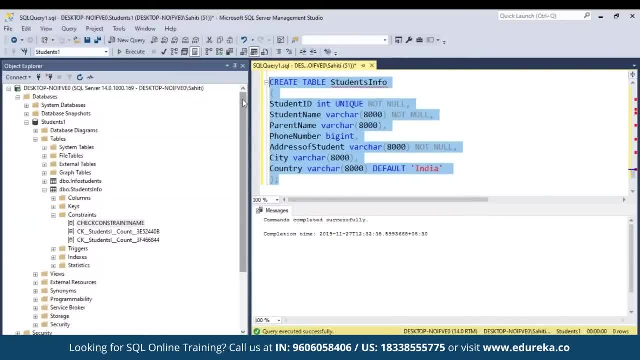 value India. So whenever there is no value that you enter- for example, let's say you are entering 10 values out of 10, 5 you've entered as Germany and 5 you've not entered any of them- Then all those other five will go, will get the values India. 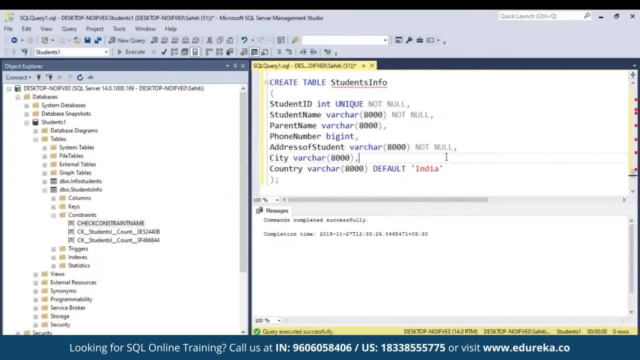 right, So I'll just execute this particular statement and then what you can just do is you can just check with the insert statement. So now, similarly, if you want to add the default constant with the alter table, you just have to again use all the table. students info. 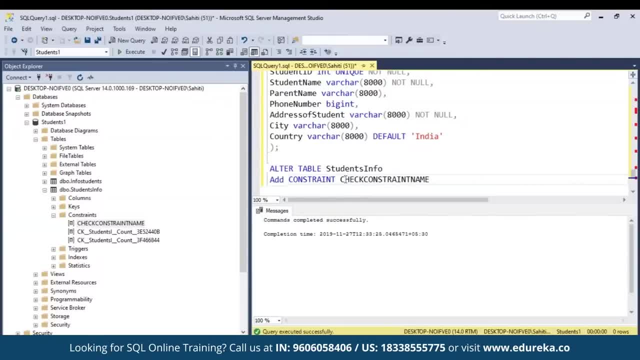 and then what you'll do is you'll just mention add constraint, and let's say you give the constant name to be, let's say, default, Let's say country Right, and then you'll mention the condition that is default, which will be India, and then you'll mention the column name. 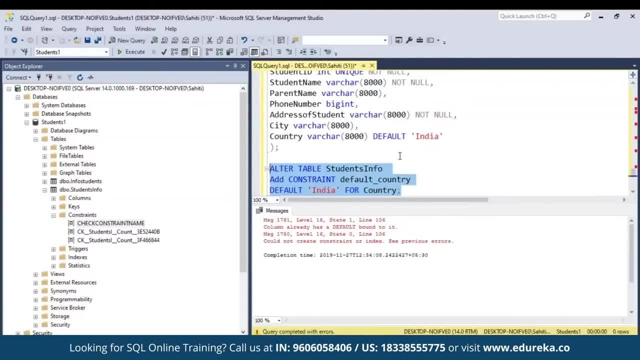 which is country, And then I'll click on execute. All right, it says that you know the column is already born. I'm sorry. So what we'll do is we'll add, let's say, City, and we'll just change it to City over here. 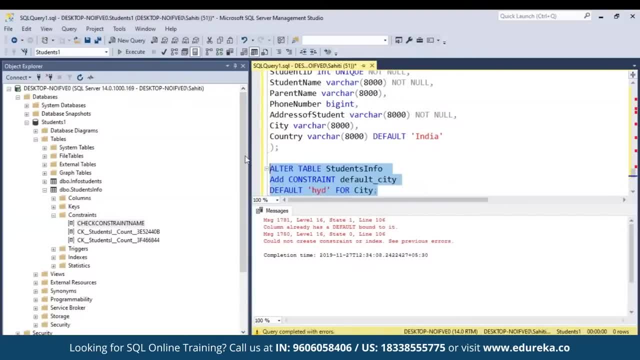 And let's say we change it to HYD right, and then I'll execute again. Once I execute, you can see that you know it's clearly working. Now to drop the default constraint. Also, it's very simple. You'll right click over here and just choose delete. 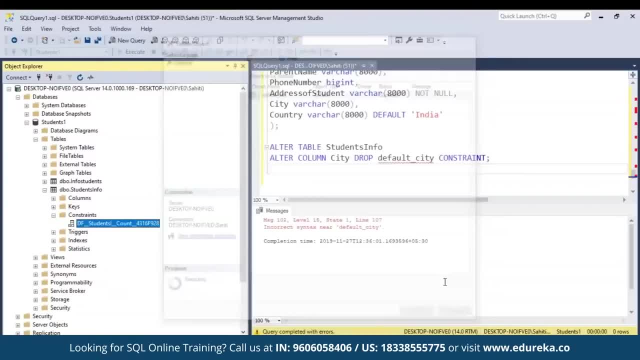 and then, once you choose delete, you can just choose the object name and click on OK, right? So once you click on OK, you'll automatically see that you know your default constraint has been dropped. now one more way to drop the default constant is by using the alter table. 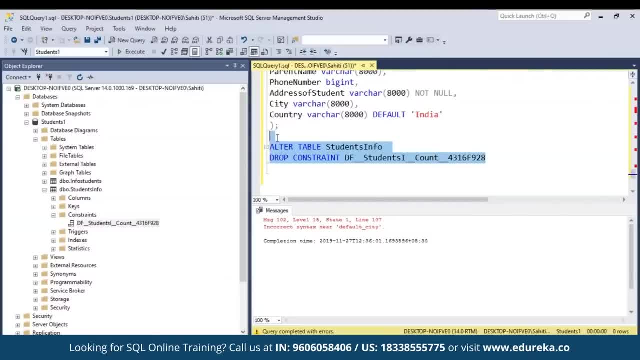 You just have to mention alter table students info and then mention drop constraint, and then you will just execute this particular statement, right? So that's how, basically, you can drop the constraint, guys. Now let's move forward with the next constraint. This is the index constraint. 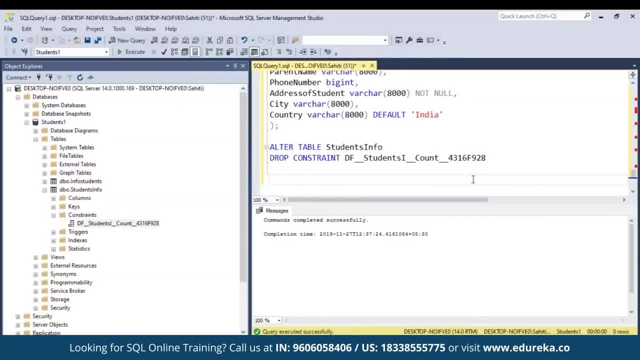 So the index constant, as I said, is used for the fast creation and retrieval of the database. So for that you'll mention create index and then let's say we mentioned the index name to be, let's say, student name, right, And then I'll mention on which table. 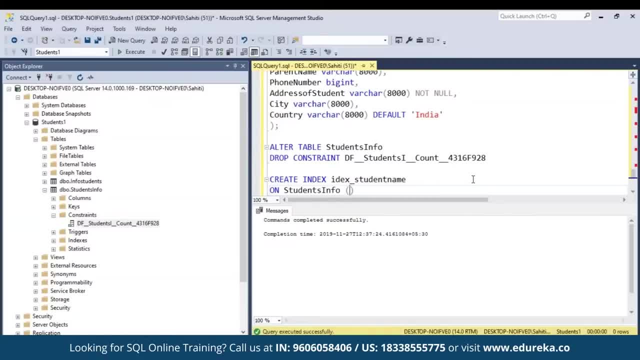 that is the students info table right, And then on which column. so we want student name from the students info table, right. So I'll just create this particular index, right, and then what I'll do is I'll just refresh this particular section. 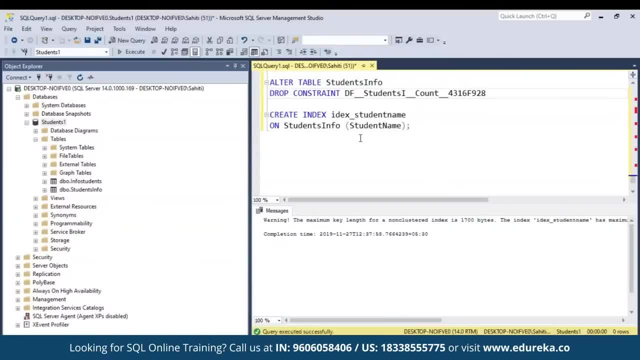 And over here what I can do is I can go and check on my left hand side. Now, if you want to delete your index constraint, what you'll do is drop index and then you'll mention the index name. So I'll just mention index name. 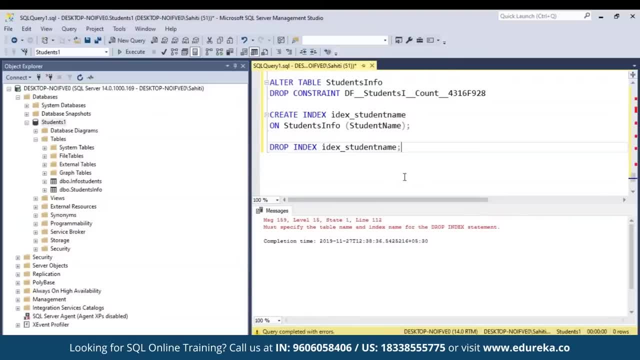 and then I'll click on execute. it says that you know, we must specify the table name and the index name. So I'll just mention the table name also. So I'll just mention table name dot. index name, right, And then I click on execute. 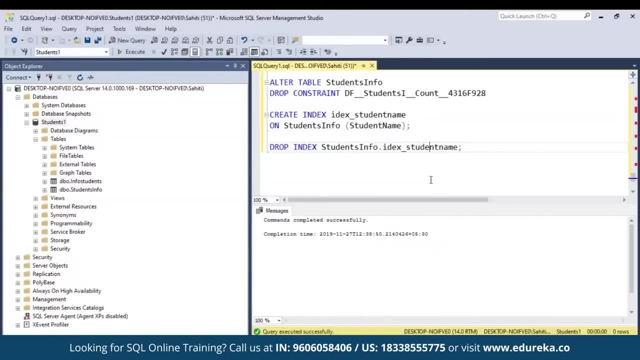 and then you can see that you know our index constraint has been dropped. So that's how, guys, basically you can create order and drop your constraints. I hope you've understood what are keys and constraints and how you can manipulate your data based on those keys. 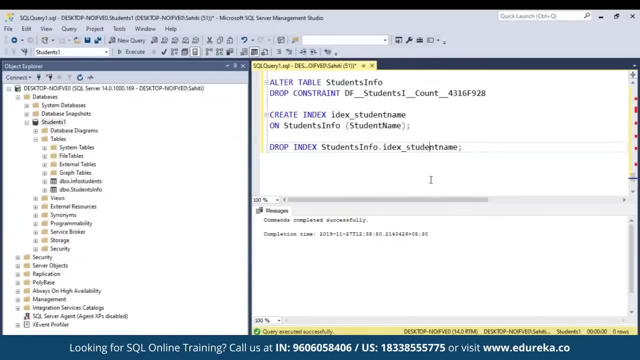 and constraints. right now, let's move forward in the session and go to the next sequel command category, That is, the data manipulation language commands. So the data manipulation language commands are used to manipulate or I would say, retrieve the data in the databases based on your requirement, right? 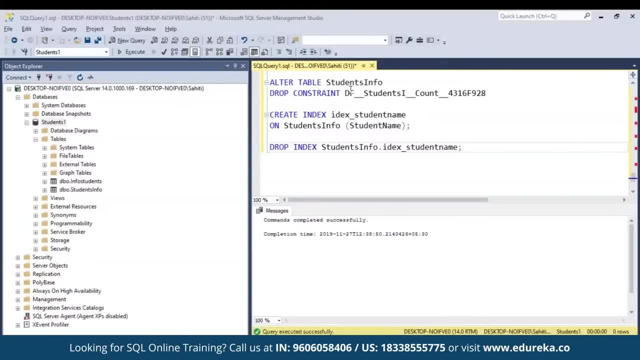 So to do that, what I'll do is I'll initially insert the values into the table And then what we can do is we can just manipulate the data. So what I'm going to do is I'm going to show you the use command, the insert command, update command, delete. 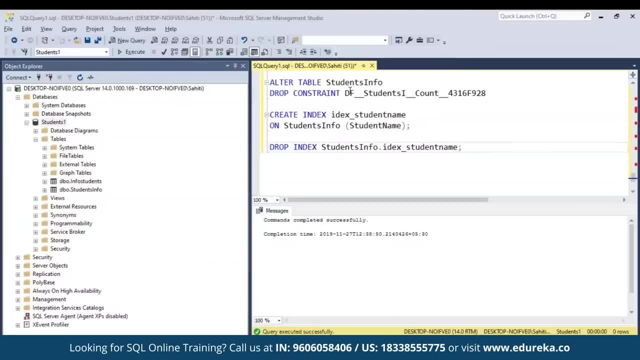 merge the select commands, the cube, the roll-up, offset, fetch, top and pivot, and apart from that, will also discuss the various kinds of operators which can be used. So, without any further due, let's get started. So initially, as I was talking about the use command, 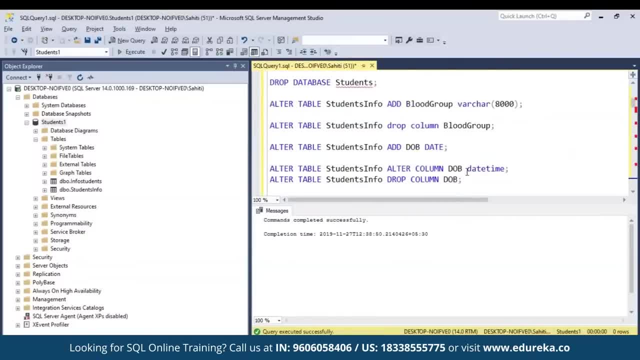 the use command is used to use a database, right, So to use a database, as I just mentioned previously. you just mentioned the command use and then you'll mention the database name. that is, students one. now, after that, what you have to do is if you want to insert values, 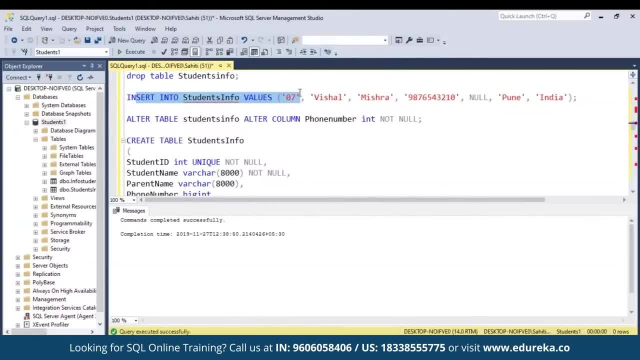 then you insert the values using the insert statement. So, as you can see on my screen, it's insert into, and then you mentioned the table name values and then you can mention the values required. So now what I'll do is I'll just drop this particular table. 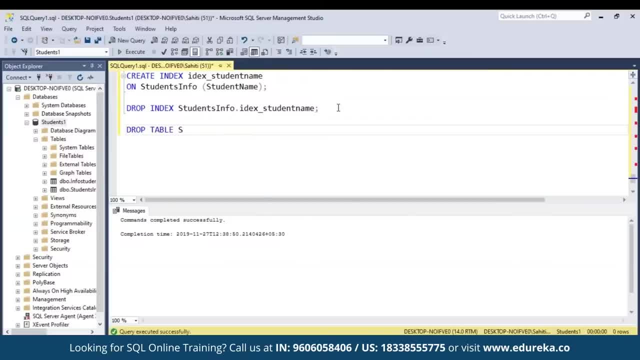 so that all the constraints are removed. right, So I'll just mention drop table students info And then again will create a table. right So I'll just copy paste from over here, Right? So once I just create this table, what I'll do? 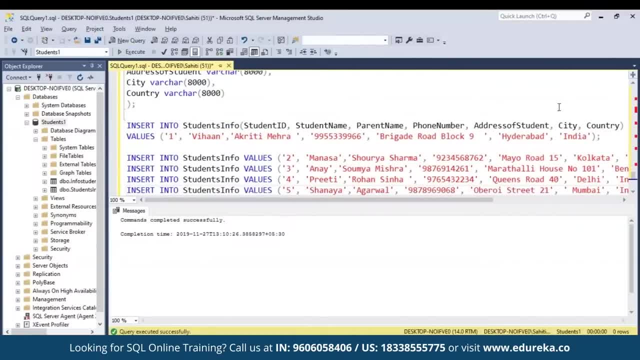 is. I'll just mention the insert commands, right, So as since I've already explained you the insert statement before, I'm not going to do that again. So the insert statement is simply used to insert the value. So there are mainly two ways through which you can insert the values into the table. 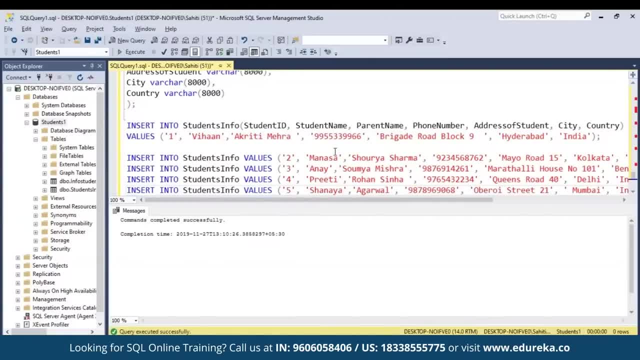 Either you mentioned the column names and then you mentioned the column values, else You can just mention the column values, right? So I'll mention insert into students info and these are the column names and then these are the specific values. Similarly, if you mentioned insert into values, 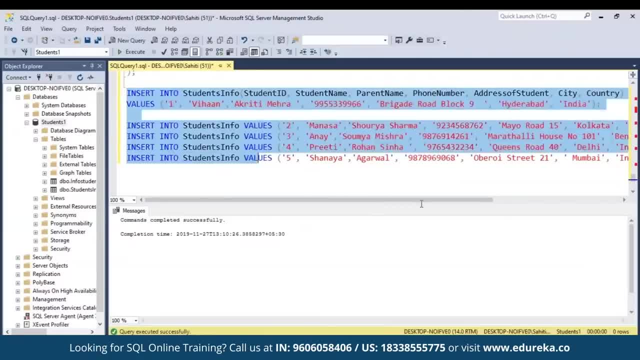 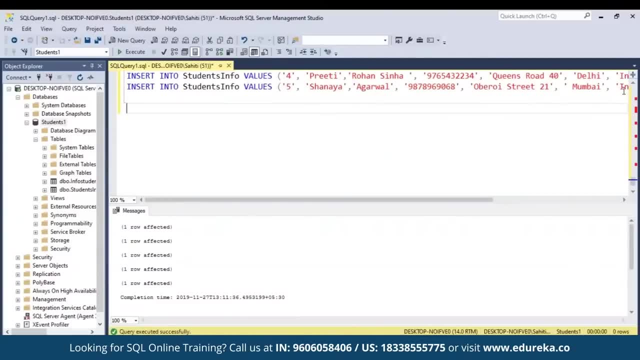 and then we can mention all the values which need to be inserted into the table right. So I'll select all of them and then I'll execute. and once I execute you can see that you know the table has values. So to check whether the values are inserted or not, 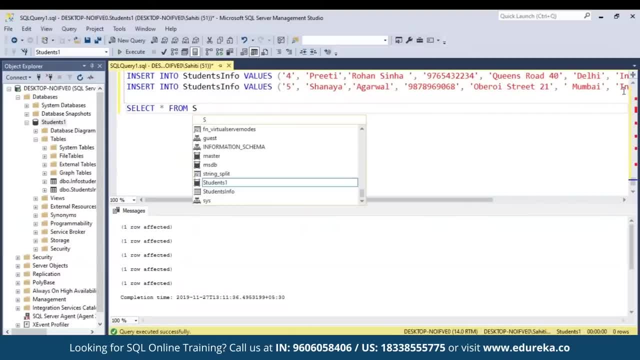 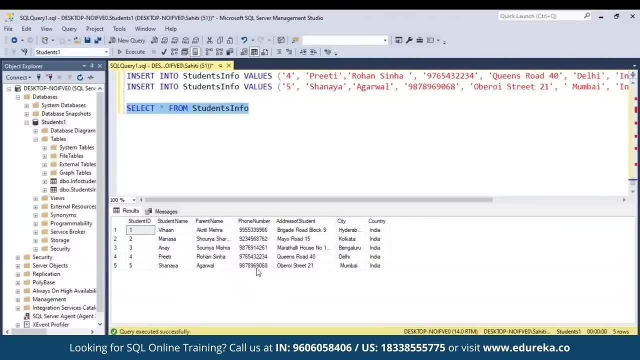 what you can simply do is you can just type in select staff from, let's say, students info, right? So we'll mention students info and then I'll execute. and once I execute you can see that you know all our values have been inserted. now let's say: you know. 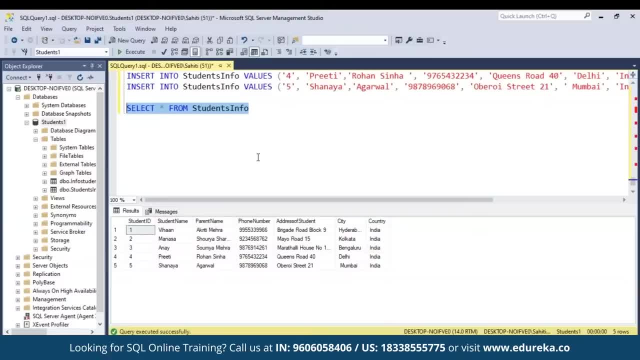 you want to update some data present in this particular database, right? For example, let's say, for student ID with student ID 1.. Let's say we want to set the student name to be Anna and then city to be M the bar right. 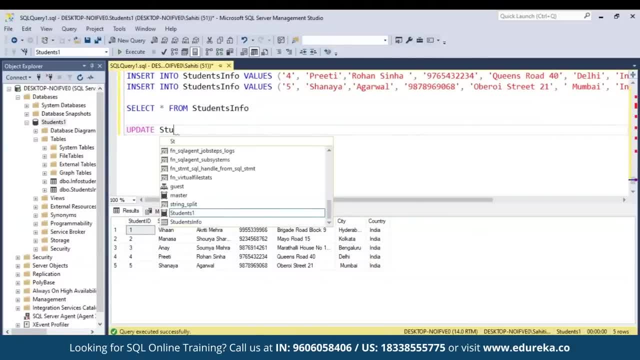 So what I'll do is I'll mention update, And then I'll mention students info, and then I'll mention set student name- that is basically a column name, right? And then I'll mention the value, that is, let's say, Ahana, right, and then also I'll mention City, don't forget. 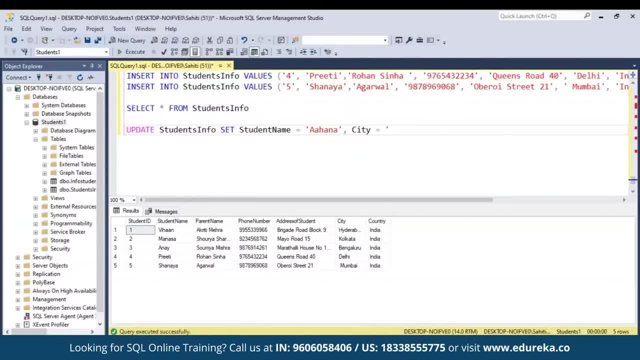 to put a comma over here, right. So I'll mention City equal to M, the bar right, and after that what I'll do is I'll mention the condition where student ID equal to 1- right, and then I'll just execute this particular state. 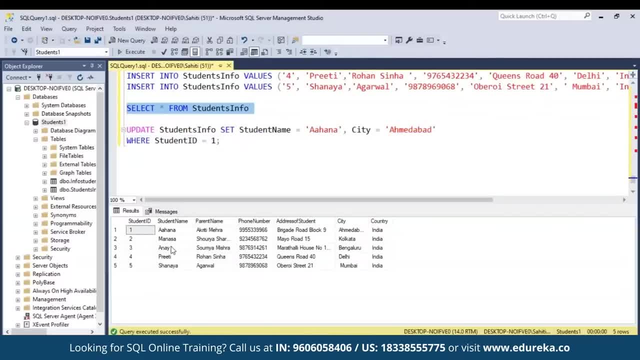 It meant. and once I execute the statement, let me execute this particular statement again, and then you can see that you know, the student name has changed to Anna and the city has changed to M the bar. So that's how, basically, you can update your data, guys. 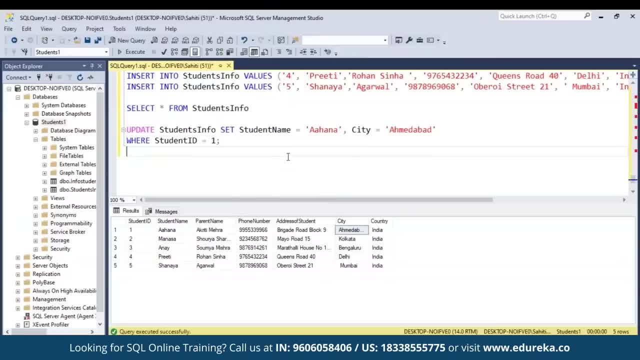 Now let's say you want to delete data from database. So to delete data, you'll just mention delete from, and then you'll mention students info where. and then let's say we want to delete the tuple with the student name Ahana, right? 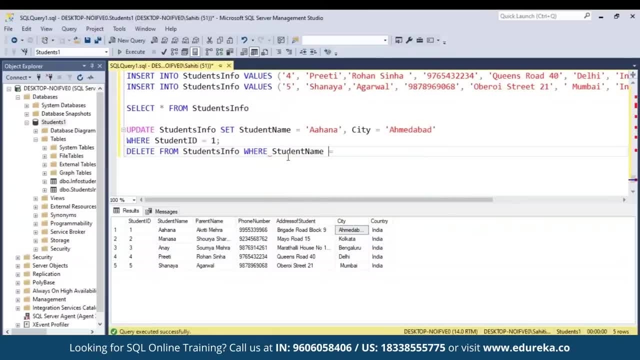 So I'll just mention student name equal to, and then I'll mention Ahana, and then, if I just execute this particular statement again, you see that you know our student ID with the student name Anna has been gone. So, guys, that's how, basically, you can insert update. 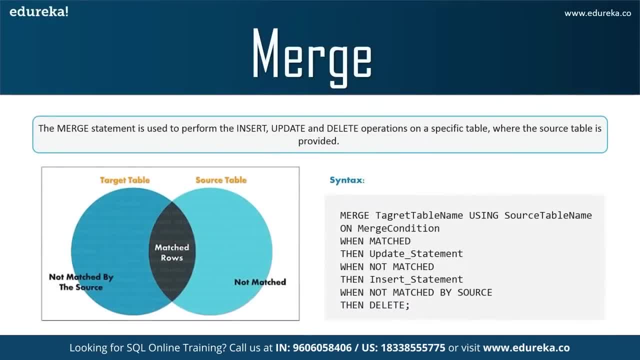 and delete values present in the database. Now, let's say you want to use the merge command. Well, the merge statement is used to perform the insert, update, delete operations on a specific table where the source table is provided. So when you have two tables, 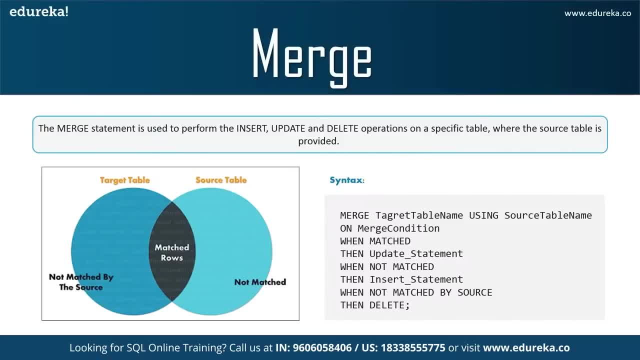 let's say table a and table B and then let's say: table a is the target table and table B is the source table, and then we have few match rows. So when we merge both these tables, we can see that. you know, we can perform the insert, update, delete operations. 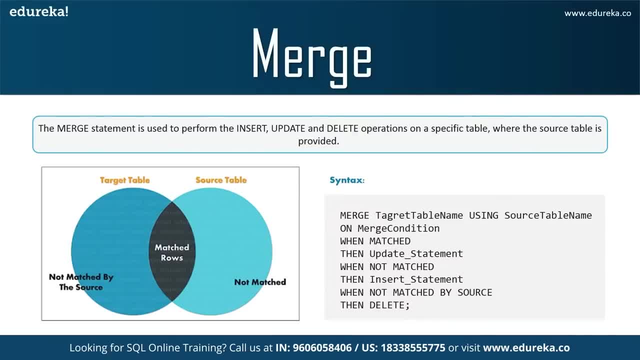 on the tables right. Well, the syntax to perform the merge operation is very simple. You just mentioned merge and then you mentioned the target table name, using the source table name, and then you mentioned the merge condition and then, if it matches, then you mention update statement. 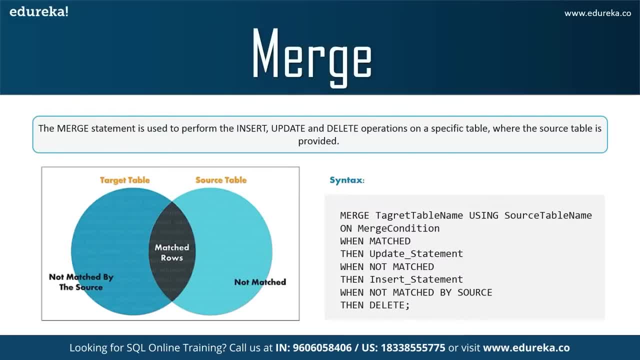 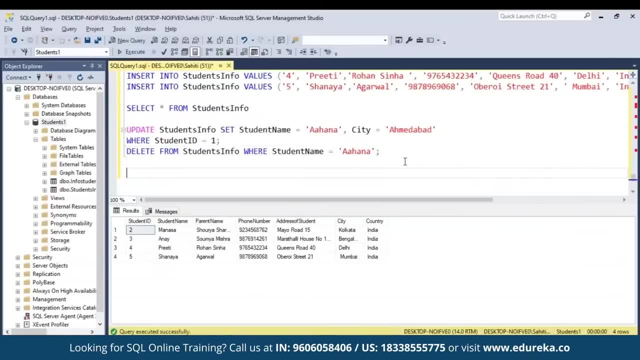 If it does not match, then you can mention the insert statement, and if it does not match by any source, then you mentioned the delete statement. So to understand the merge statement, let's just say we create two more tables, Right? So what I'll do is I'll just create table. 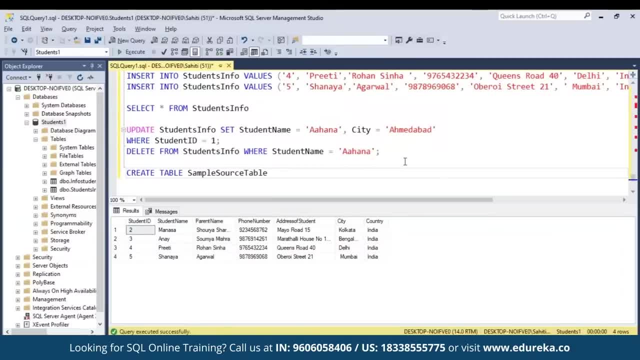 Let's say sample source table and let's say the columns to be, student ID Of in type- right, and then I'll mention student name of, let's say varchar8000, again right, and then we'll mention the marks column of in type. Now, similarly, I'll just create the target table also. 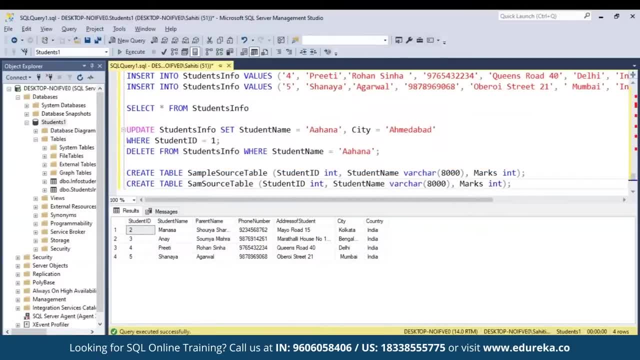 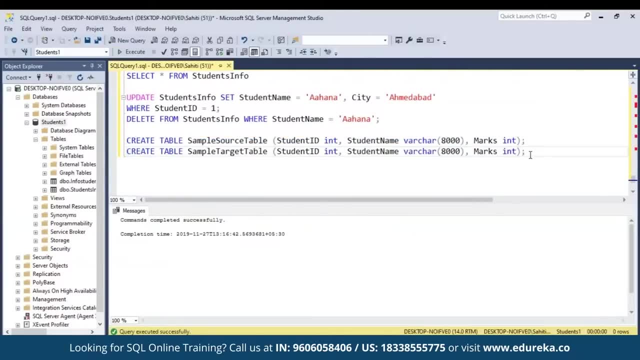 So before executing, I'll just change the name to Target, Right, so I'll just mention sample target table and then I just execute both these statements right now. after that, what I'll do is I'll just insert few values into the source table and the target table. 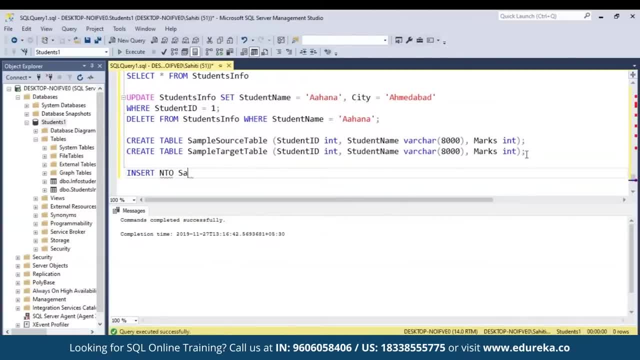 So I'll just mention insert into and then we'll mention sample source table, and then let's say we mentioned values and over here we mentioned, let's say first person with name Vahan, and let's say the marks: It has to be 87. similarly, 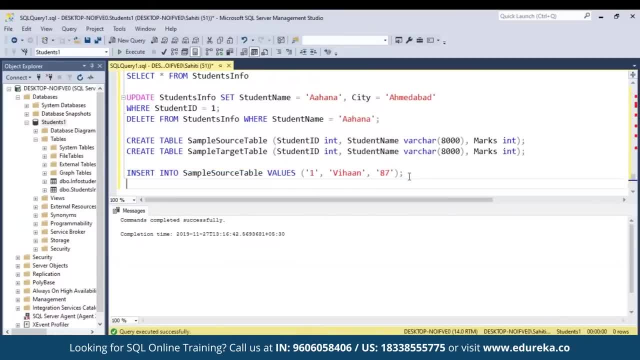 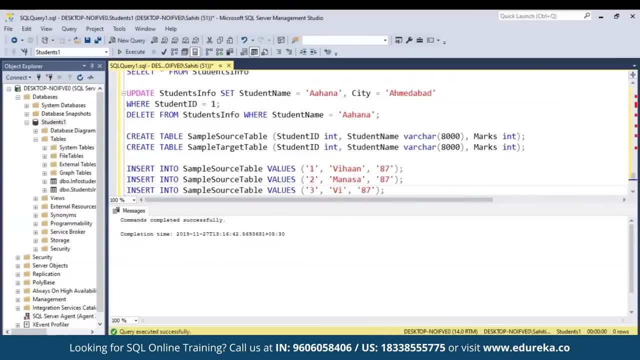 Let's just mention two more records, right? So I'll just copy paste, right? I'll just change this to two, three that we change the names and the marks Now. similarly, I'll just insert it to the target table also. So I'll just change the table name to be sample: target table. 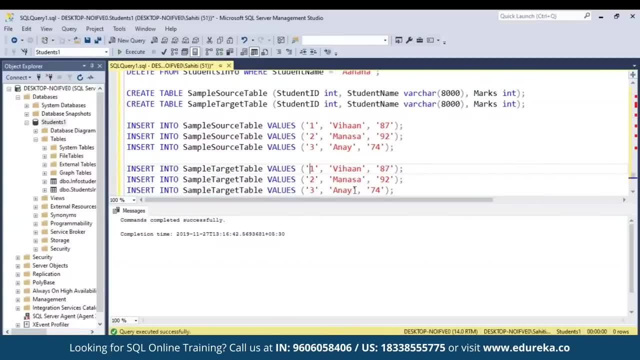 So I'll copy paste from over here And then I'll let the first record be the same. Let's say one behind an 87, and let's say we change it to 60.. Seven and please, sort of, and let's say we change it to 55.. 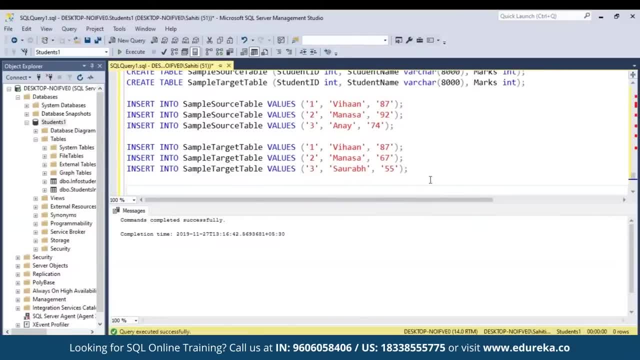 Now what I'm going to do is I'm going to merge both these tables, and that means I'm going to merge the sample target table and then I'm going to merge it by using the sample source table, right. So for that I'll mention the statement: merge sample target table. 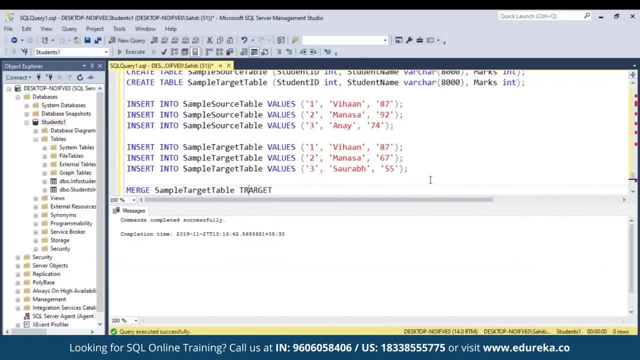 and then I'll mention Target- I'm sorry Using- and then we'll mention the source table, So it will be sample, So stable, and then I'll mention source on and in brackets I'll mention Target dot. Let's say we match it to student ID. 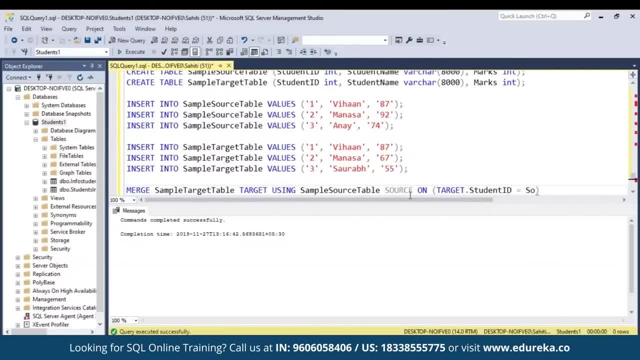 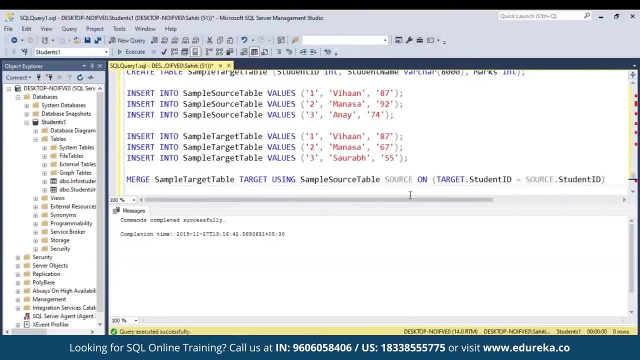 That is basically a condition: must match our source student ID, right? So we mentioned source dot student ID. So when it matches, what we want to do is, when matched and Target dot student, Let's say name is, you know, same as source dot student name. 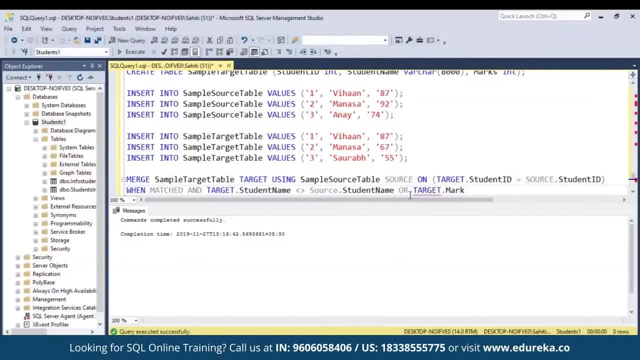 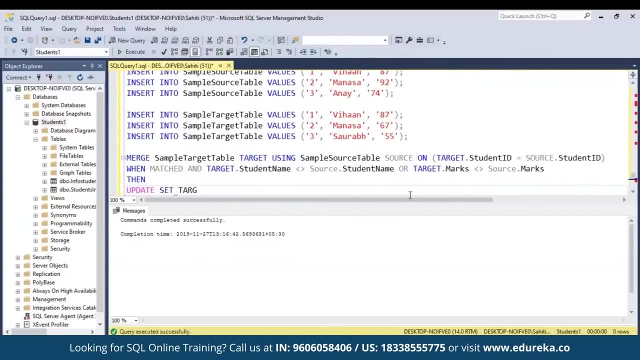 Right, or Target dot. you want marks is same as, let's say, source dot marks. right, Then we want it to update set. We want to update Target dot student name equal to- I'm sorry The target spelling is wrong- Source dot student name. 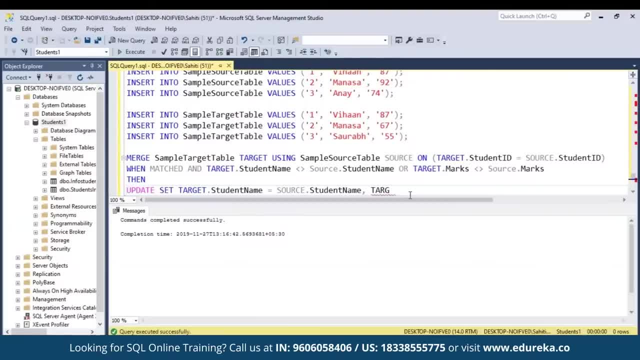 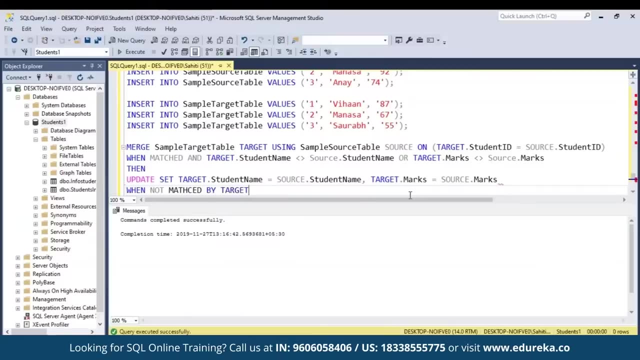 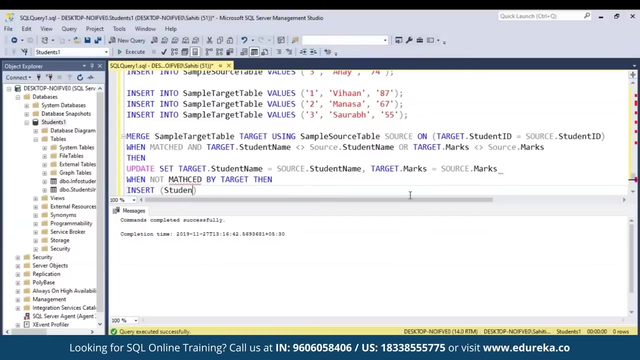 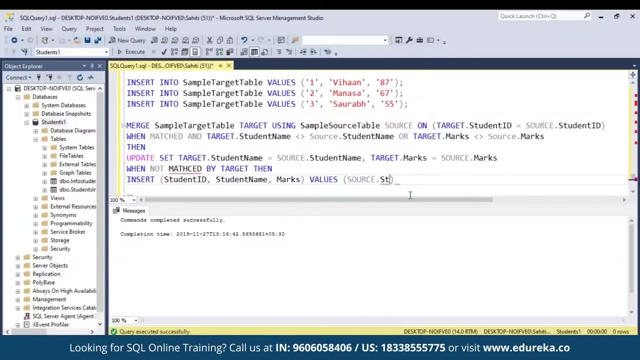 right comma. We also want to match the marks right: Target dot marks equal to source dot marks when not matched by Target, Then we want to insert right. So we'll mention insert and brackets will mention student ID comma. student Name marks right and will mention values. will mention source dot student ID. 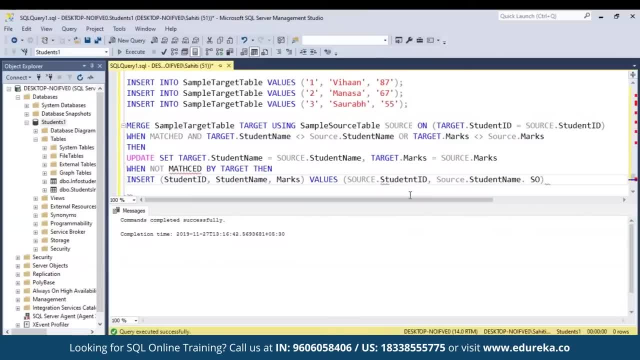 Similarly, source dot student name and source dot Marks right And after that when it doesn't match, right. So what we want to do is, when not matched, we want to delete right. So we'll just mention by source, then delete right. 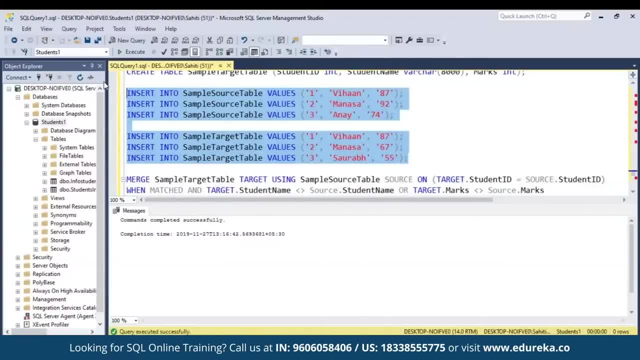 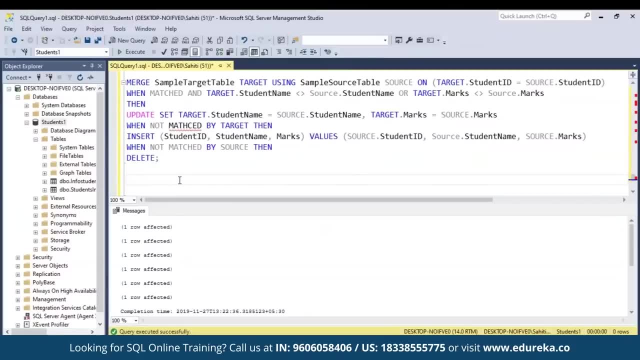 So I hope that you've understood right. So what I'll do is I'll initially insert the values into the sample source table and the target table, right, And then what I'll do is I'll just show you what are the values present. 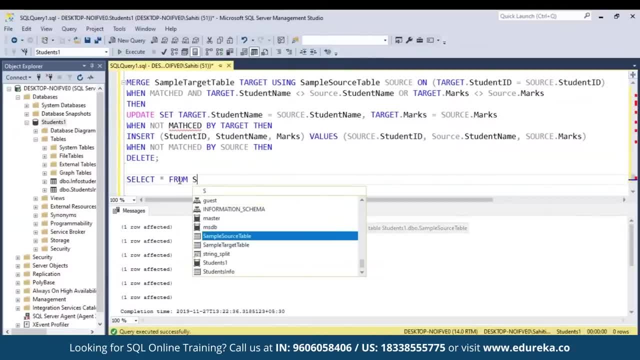 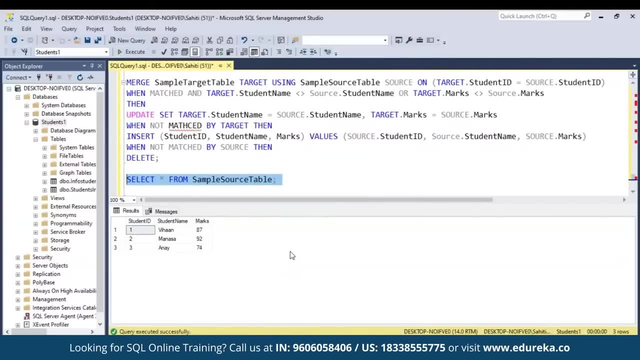 So I'll just mention select star from sample table. That is a sample source table. So you can see that. you know we have three tuples, that is, with vihan Mansa and any having 87, 92 and 74, and then when we have the sample. 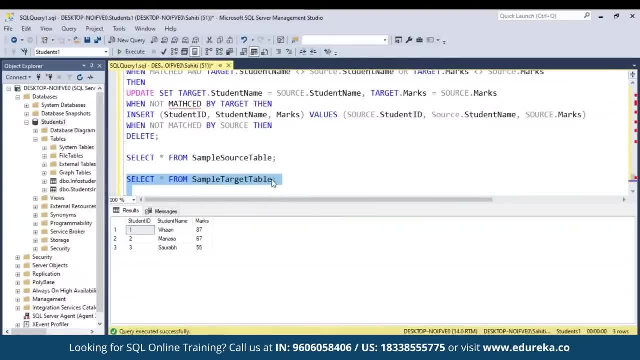 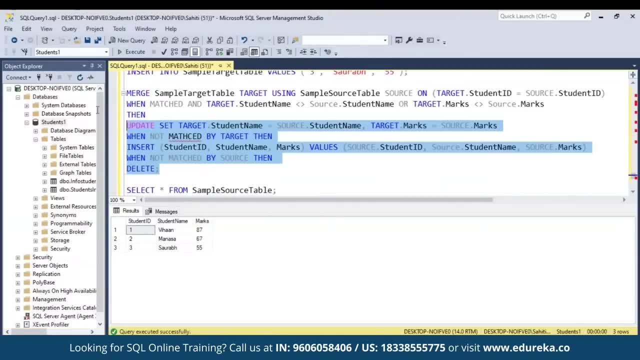 Target table. We have again three tuples with vihan Mansa and sort of having 87, 67 and 55 marks. So now what I'll do is I'll just include this merch statement. spelling mistake, right, So I'll just mention when not matched: 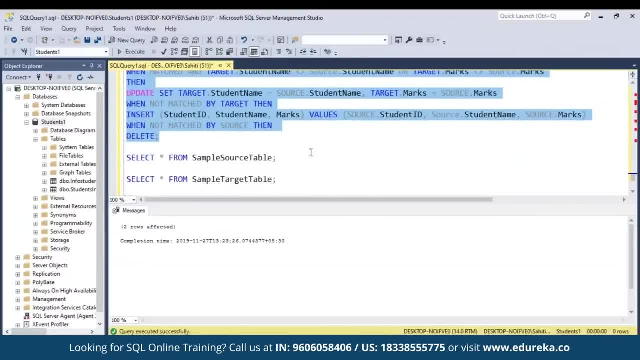 and then I'll just execute. so when I execute this particular statement, you see that you know two rows have been affected and then we see completion time right. So if we just again click on sample Target table, we see that you know. 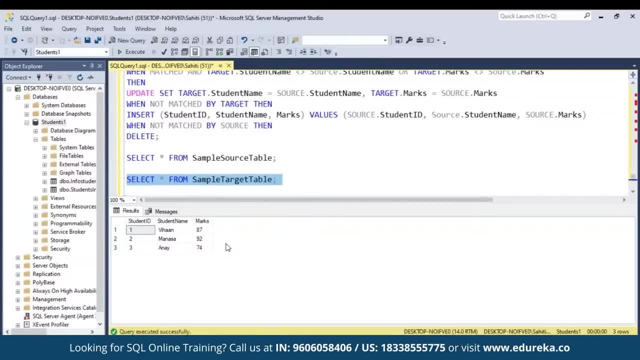 we have our Target table now having vihan as 87, Mansa as 92 and any as 74. initially our Target table had vihan as 87, Mansa 67 and saw the best 55, right. So that means our values have changed. 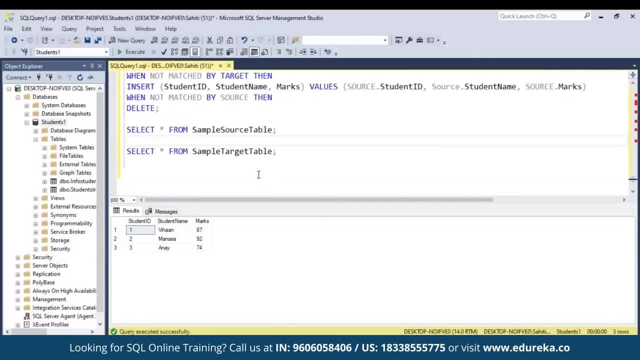 and our values have come from the source table. So that's how, guys. basically you can merge two or more tables. Well, that was about merging column, guys. now, since I was using a lot of select statement, let me show you a few actions which you can perform on the select statement. 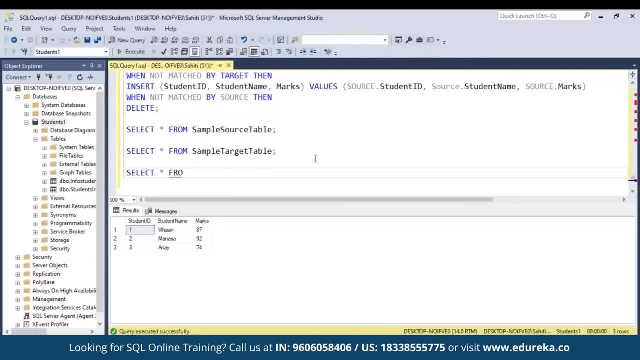 So, for example, let's say you want to select a few columns, right, You'll just mention select and then you'll mention the column name. So let's say I'll mention student ID and let's say we mentioned student name, right? 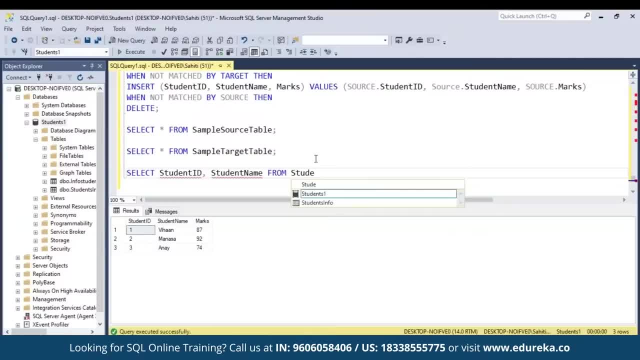 So it should. they should be a comma over here from students info, right? So if I just execute this particular statement, you see all the values of student ID and student name from the students info table Now. similarly, if you want to select all the columns, 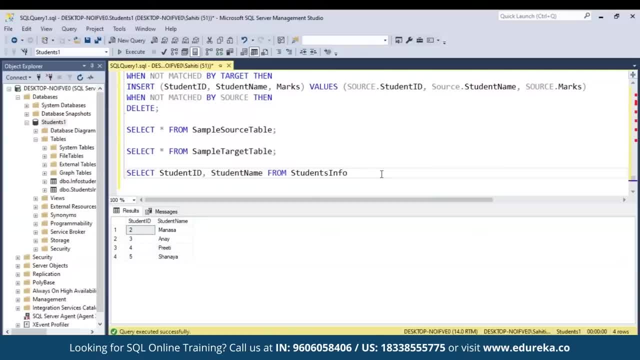 you'll just mention select star from the table name. So that's how you can use the select statement. Now let's say you want to select the top three records from the table, So you just mention select top three star and then you'll mention the table name. 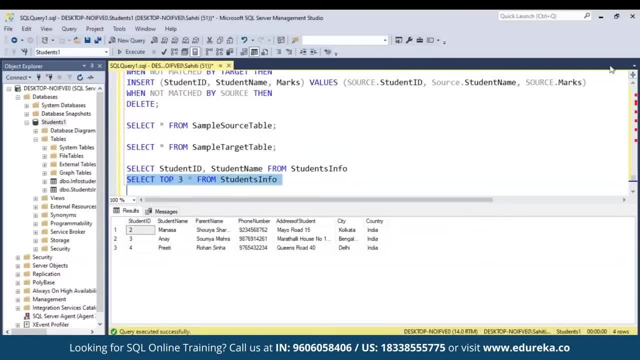 So that will be, let's say, students info and when I execute this particular statement. you see that you know we get the top three statements, that is, the values for the second student, third student and the fourth student, and now, similarly, you can also find: 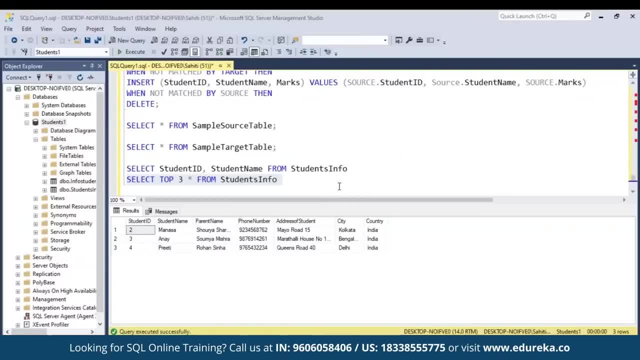 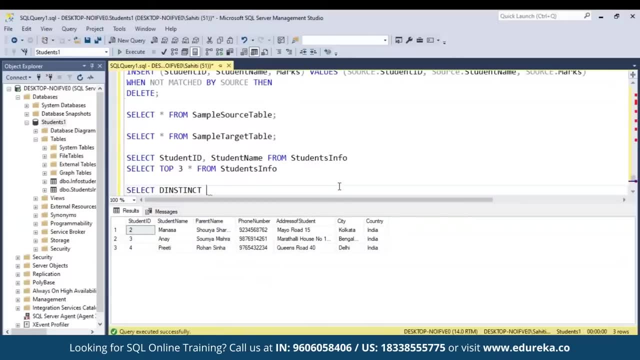 out the distinct values in a specific column Also. for example, let's say we want to find out the distinct cities present, right? So we'll just mention select distinct and you'll mention City from and you can mention students info, right. 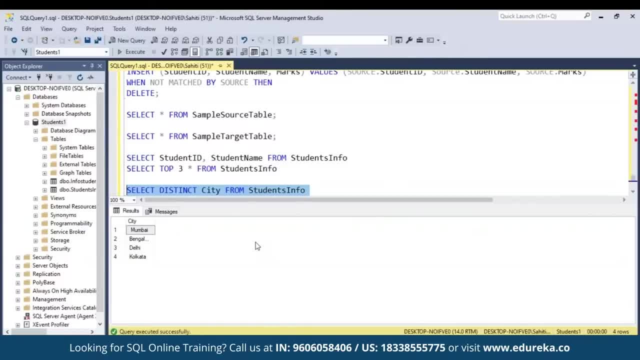 And then let's execute. if I execute, you can see that you know we have Mumbai, Bangalore, Delhi, Kolkata as the distinct cities present. now moving forward, Let's say you want to use the order by group by and the having clauses in the select statement. 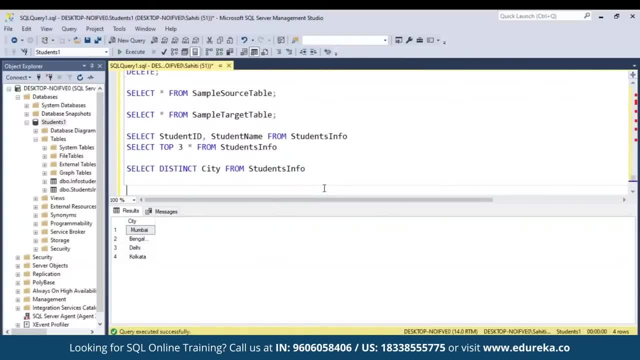 Well, to do that- It's really simple, guys. You just have to use those clauses. for example, let's say you want to select all the students from the students info table, sorted by the, let's say, parent name, So for that will mention select star from students info. 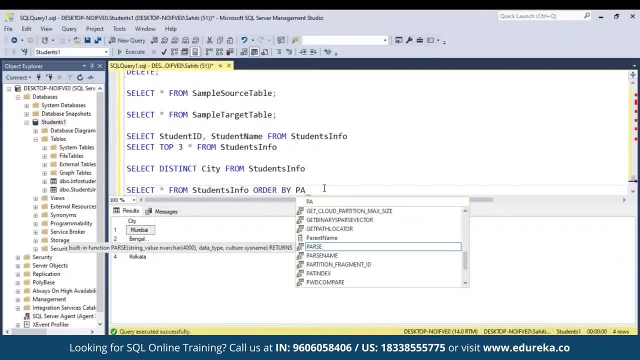 and then we'll mention order by parent name right and over here. if you do not mention anything, it will be ascending order by default. but let's say, if you want it in a descending order, you'll just mention the keyword descending right and then you'll click on execute. 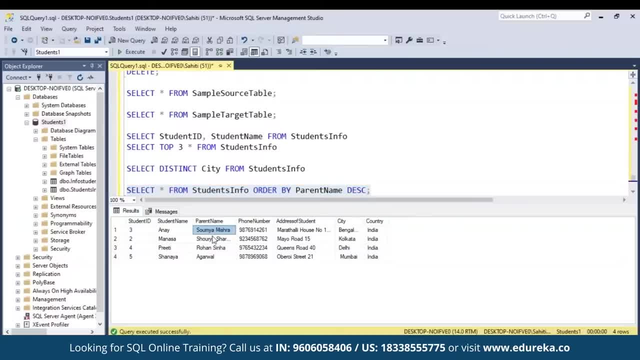 and you can clearly see that. you know, our students are sorted by the parents name, So it starts with S and then goes to a and then, if you just remove this particular section and then you execute again, you'll see that you know our fifth student. 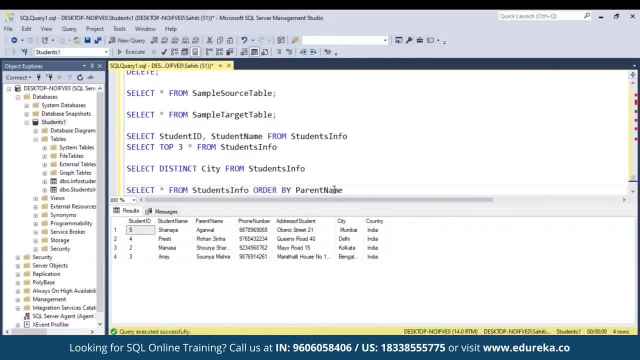 with the parent name Agarwal will be first on the list. But that's how you can use the order by statement. Now, This was just for one column. Now, let's say you want to saw the data present in the table with different columns, right? 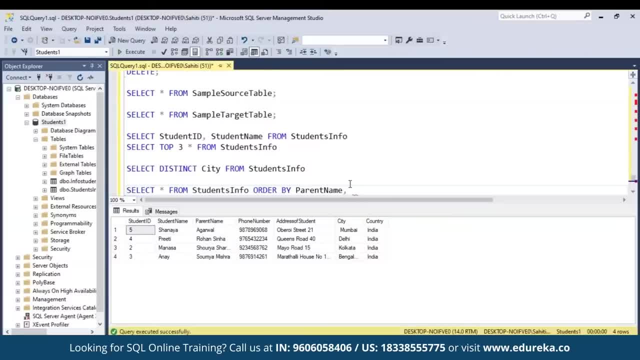 So let's say we want to sort the students from the students info table by parent name and also the student name. So we'll just mention student name and then what I'll do is I'll just execute, and when I execute you can see that you know. 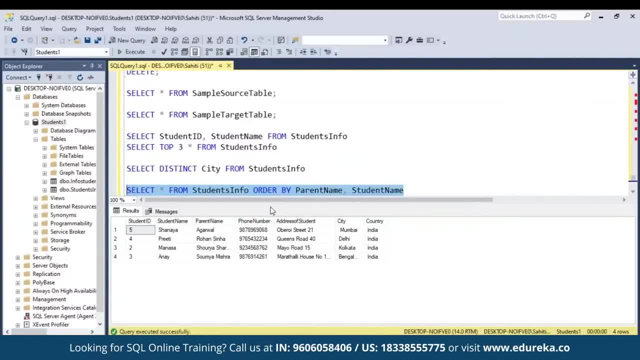 since we haven't mentioned anything whether it should be ascending or the descending order, automatically the parent name comes in the ascending order. So our fifth student comes first on the list and then the order follows similarly if you just replace this. So, for example, if you just put the student name first. 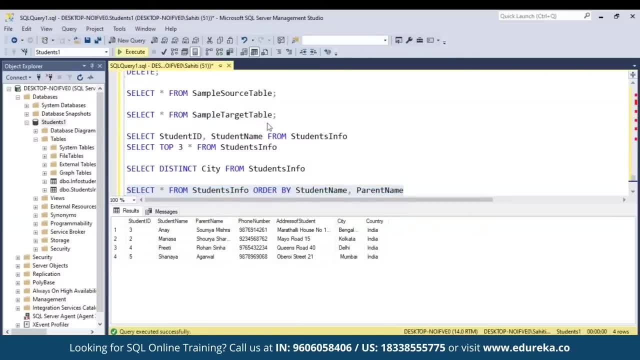 and then you mentioned the parent name, and then you execute the statement. you'll see that you know the results are different because our student name will be first sorted in the ascending order. now, apart from this, what you can also do is you can saw the data. 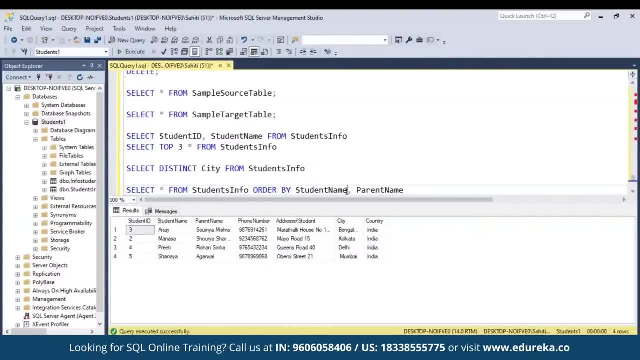 presented the table either in the ascending order or in the descending order for different different columns, right? So what I mean by that is that you know, student name can have the ascending order and the parent name can definitely have the descending order. So let's do the same. 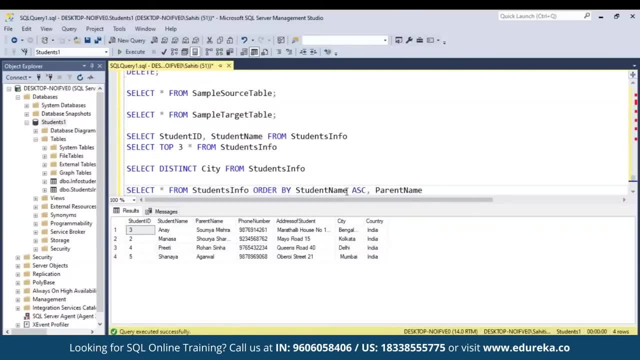 So I'll just mention ascending over here and over here I'll mention descending right, and then I'll execute. So once I execute you'll see that you know the student names are sorted in the ascending manner and the parent names are sorted in the descending manner. 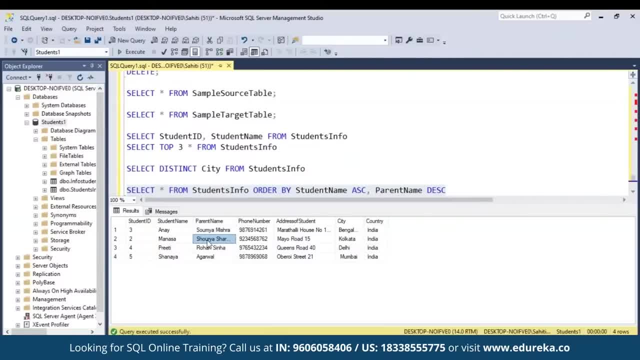 So that's how all the students in the student info can be sorted: by the parent name in the descending order and the student name in the ascending order. So, guys, that was about the select statement. Now this is one of the most popular statement, which is used by manipulating data in the databases. 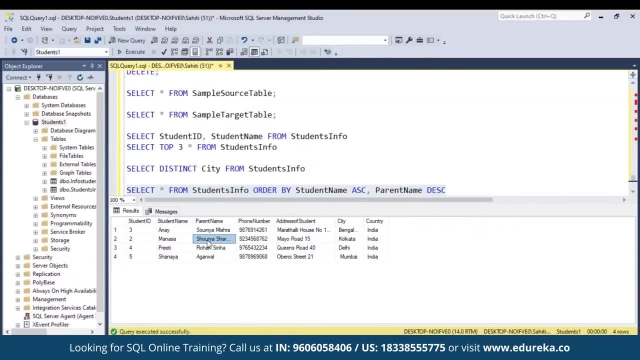 because you know this is one of the easiest way to retrieve data and this statement is used with lot of commands and other queries to retrieve data in the format The client wants. now, moving forward in the session, Let's say you know we want to list the number of students from each city. 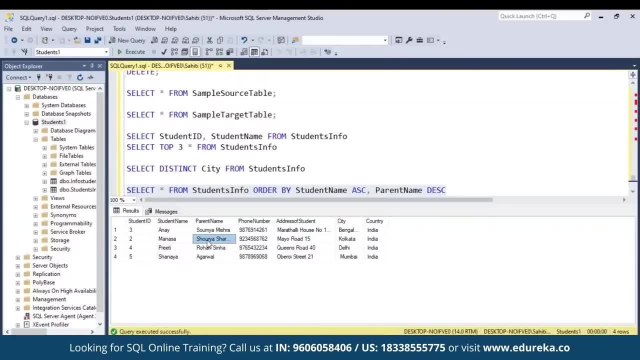 not to list the number of students from each city. What you have to do is you have to take care of the aggregate functions. So the aggregate functions are basically those functions which are used to calculate the sum, the average, the count and the range, the first and so on. 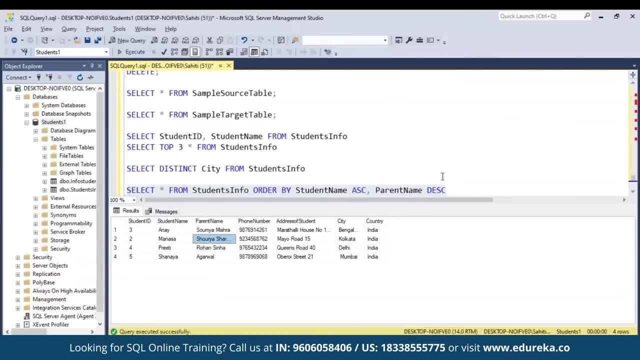 So don't worry, I'll be talking about them later in the session, But for now, if I just have to implement and show you, you can just mention select count and then you can mention, let's say, student ID, right, and then you can mention City from the table name. 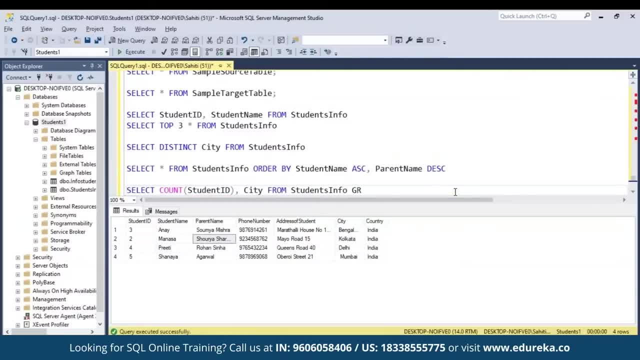 that a student's info, and then what you can do is you can simultaneously group them by City, right? So because we want to count the number of students from each city, We just group them by City and then we used to count function and then we execute the statement. 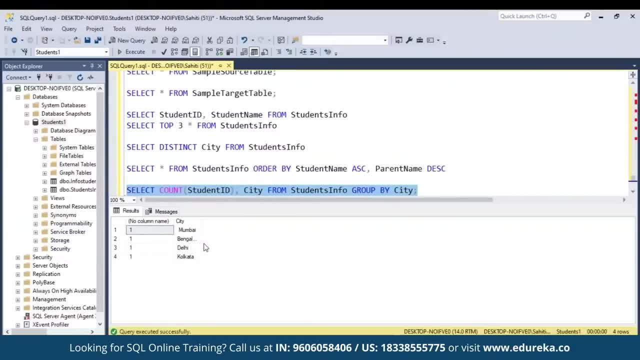 You see that you know Mumbai has one student, Bangalore has one, Delhi has one, in Kolkata has one. so, guys, that was about this particular query. Now, let's say you want to use the grouping sets. Well, grouping sets were introduced in sequel server 2008. 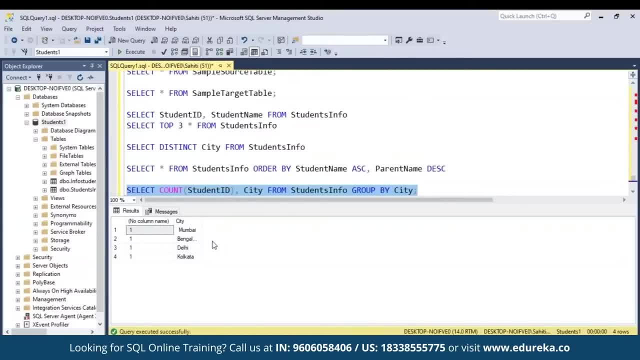 and we used to generate a result set that can be generated by Union, all of the multiple simple group by clauses. So the syntax is also very simple, guys. You just have to mention select and then you mentioned the column Names from the table: name group by and then grouping set. 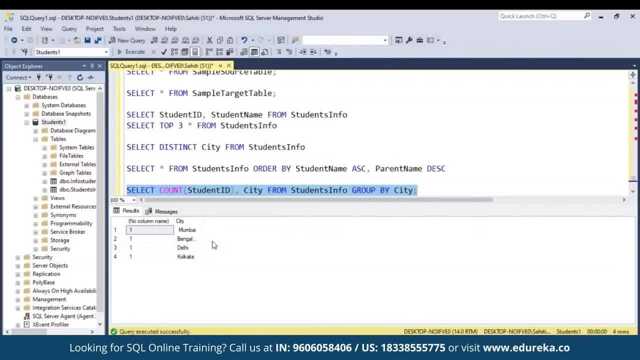 and then the brackets. you mentioned all those column names which have to come under the grouping sets. So, for example, let's say I'll just modify this particular query, right, So I'll just mention select and then I'll remove the count function. 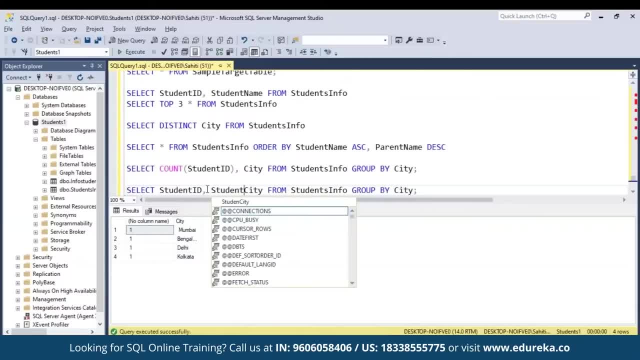 Let's say I mentioned select student ID and let's say I also mentioned student name, right, and then I count the number of cities from the students info table, and then I grew by, and then I again use the grouping sets. So I'll mention the grouping sets and in brackets are what I'll do. 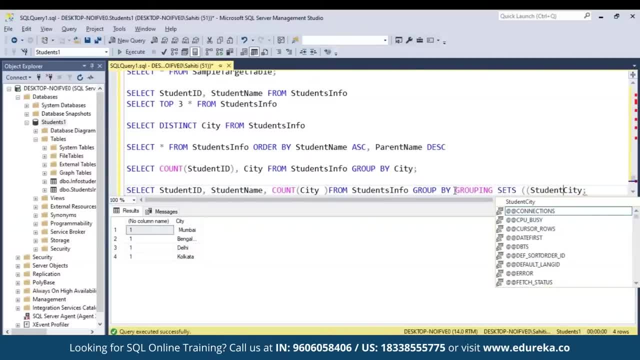 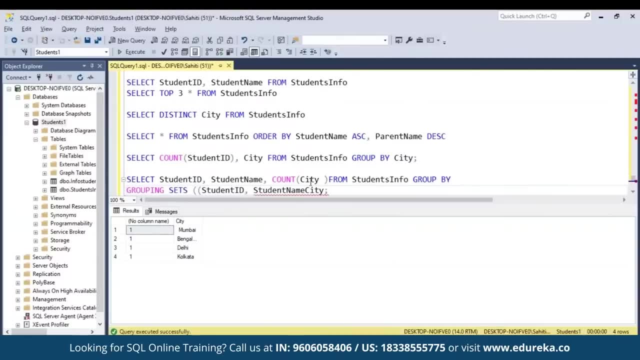 is. I'll mention the grouping sets right. So for example, let us first said we student ID, student name: Nice elect. We just press on enter, So that's clear. and also let's say: we have City. Now let's say in the other set, 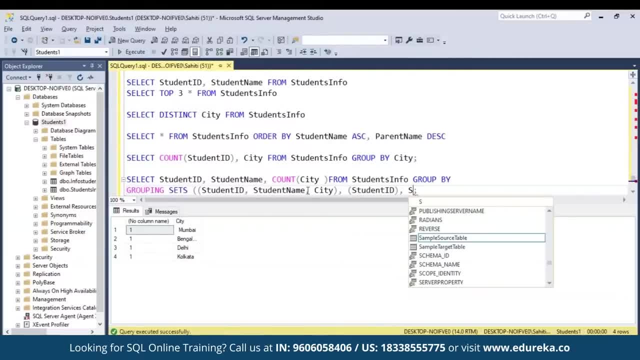 We just have student ID Right, and in the next one I just have student name right. So I'll just put in the bracket. and in the last one, let's say, we just have a city right. So these are ways sets that we have created right. 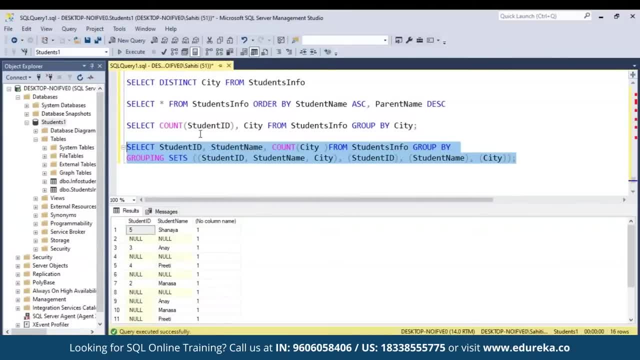 and now we can just execute this particular query. You can see that you know student ID, student name and no column name. that is basically account of City from students info and then it's grouped by basically these four sets, that is, student ID, student name, City in one set: student ID. 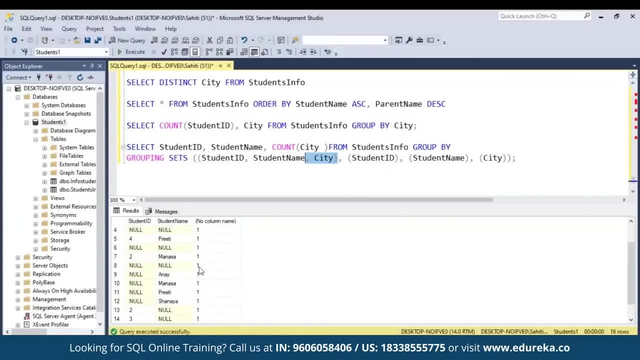 in the second set, the student name in the third set and the city in the fourth set. for example, let's say, for student ID which is null and student name is none, the count is one. So, guys, that's how you can use, the group by group. 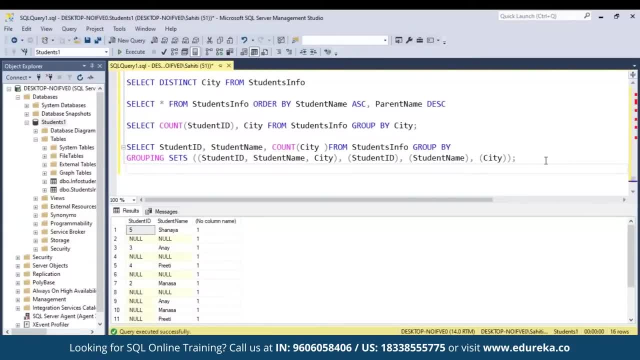 Clause and the grouping sets together. Now let's say you want to use the having Clause, while the having Clause is generally used in the scenario where the where keyword cannot be used, right? So if you observe, generally in the select statements we use the where keyword. so in the scenario, 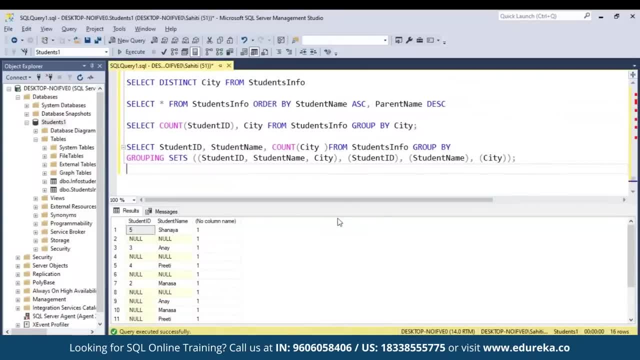 where the where keyword cannot be used, We use the having Clause. So let's say, you know. if you want to use the having Clause, let's say we want to count the number of students from a specific City and let's say: 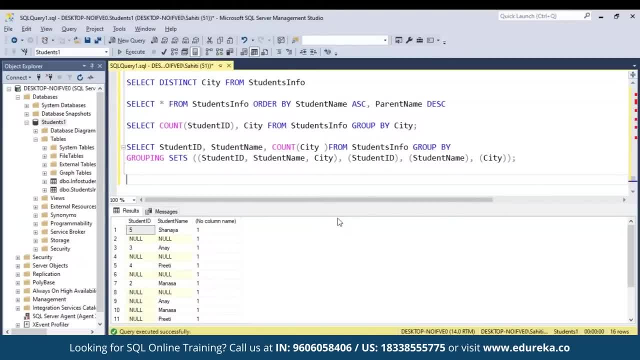 you know, their count should be one and should be ordered by, let's say, the student ID with descending order, right? So what we can do is we'll do select count And then I'll mention student ID, comma, City, and then I'll mention from, obviously, the table name, right? 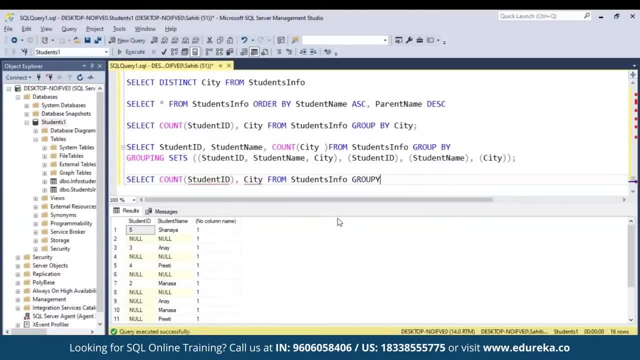 students info. and then I'll mention group by City having count, and then over here I'll mention student ID. again, equal to one, I'm sorry, equal to one has to come out, and then let's say we order by count. Let's say student ID. 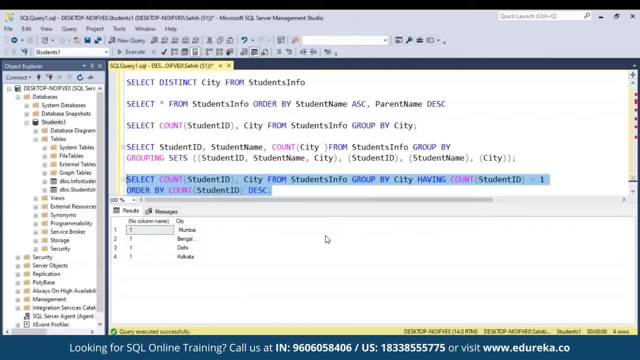 In the descending manner, right? So I'll just execute the statement. we can see that you know Mumbai, Bangalore, Delhi and Kolkata have come with their count having one. So that's how you can use the having Clause guys. Now let's say you want to create a backup of this table. 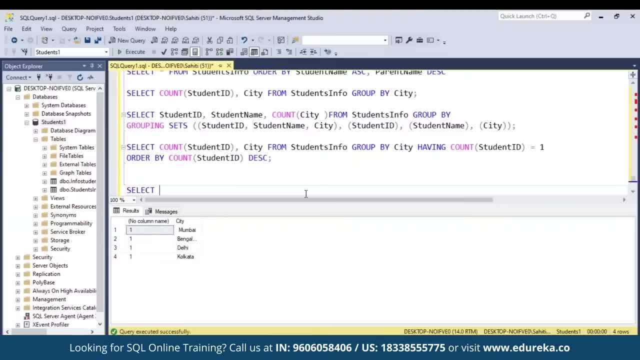 That is the students info table. So to do that, what you'll do is you'll just mention select star into and you'll mention the backup tables name. So let's say we mentioned students backup from and then I'll mention the table name, that is, students info. 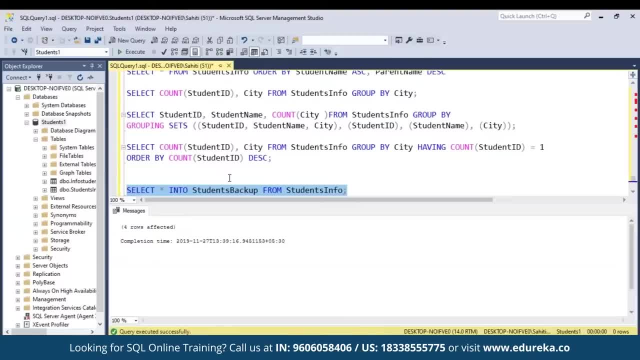 right, and then I'll just execute And then you'll see that you know, automatically the backup has been created. Now this is where we just included all the columns and the tuples from the students info table to the students backup table. Now let's say you just want to select only few columns. 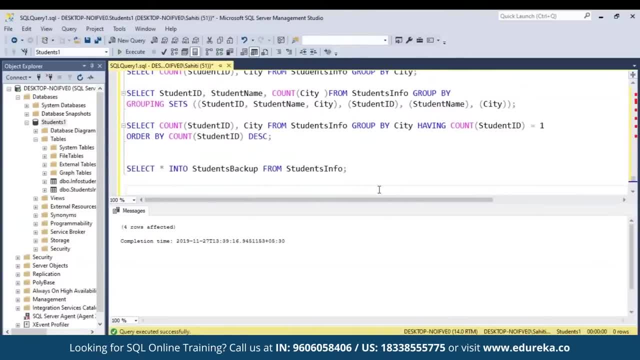 from the students info table. Well, to do that, what you'll do is you'll just mention few columns, that is, select, and then you'll mention ABC column from the table. apart from this, you can also mention conditions also. for example, let's say you want to retrieve only those students. 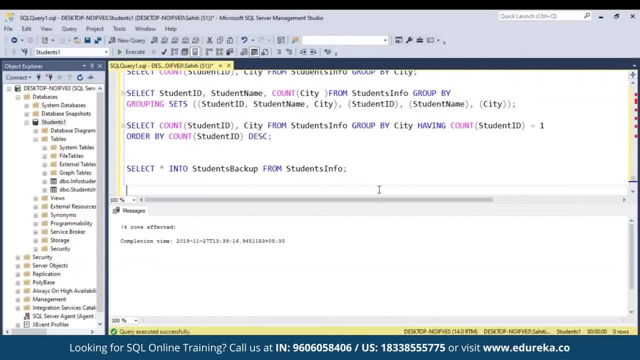 who are from the city Pune. So you'll just mention whatever column values that you want to retrieve, like select student ID, student name and so on, into the table. that is a table name from students info where the city will be Pune. So for your better understanding, let's just write that. 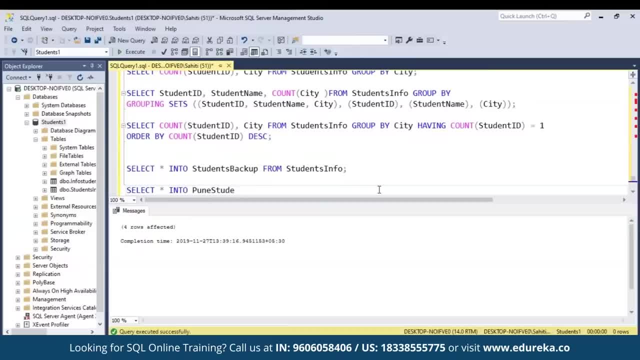 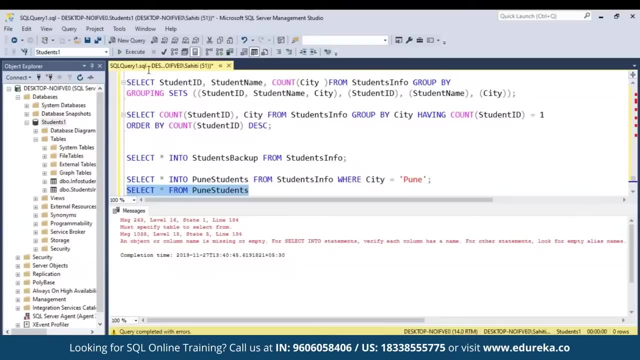 So select star into, let's say we mentioned Pune students from students info where city is equal to Pune, right, and then I'll just execute. So if I just execute this particular statement, you'll see that you know we have no values present because there was no student with the city Pune. 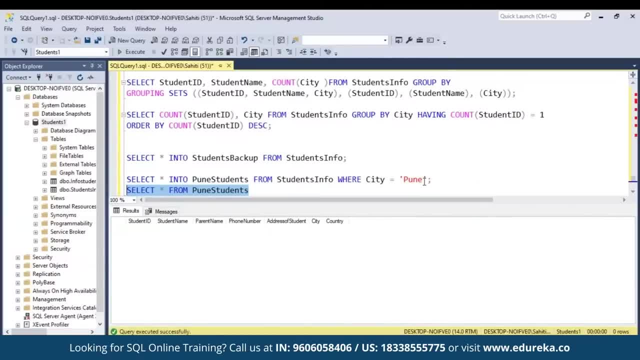 So now what you can do is you can just go back and change the city name and then maybe drop the table and create the table again. So that's how you can play around with the select statement, guys. Now let's move forward with the next DML command. 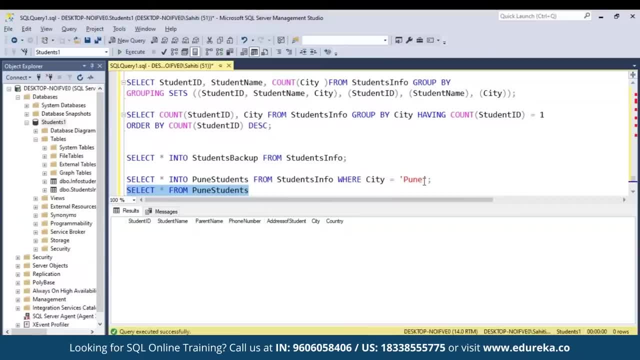 That is the cube command. Well, I would say that you know, the cube is an extension of the group by clause, So it basically allows you to generate the subtotals for all the combinations of the grouping columns specified in the group by clause. 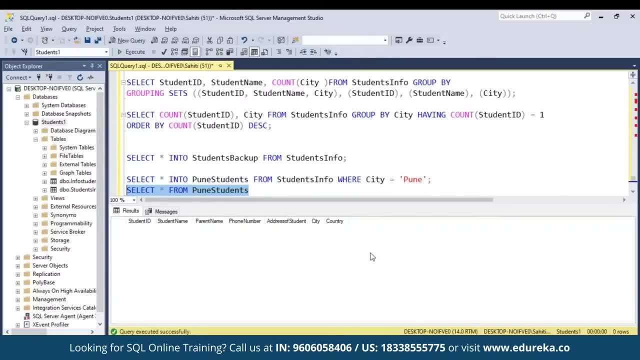 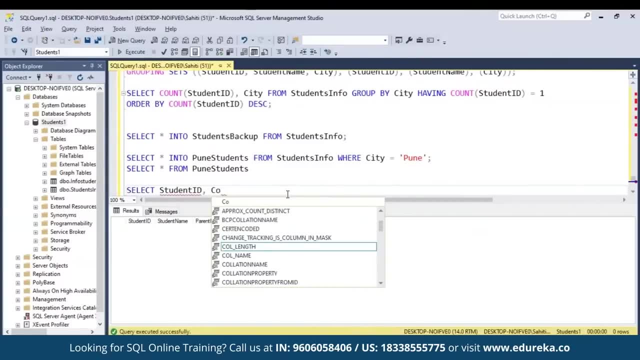 So, for example, let's say you know you want to use the cube statement, So what I'll do is I'll just mention select student ID, right, and let's say we also mentioned count, You mentioned City from students info, and then we mentioned group by, and then we mentioned Q. 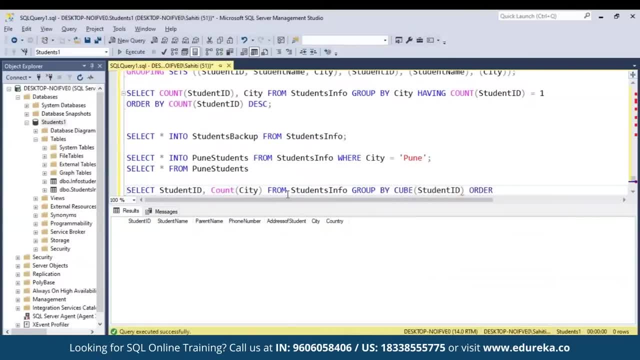 and I'll mention student ID order by student ID Right, and then I'll just execute. So when I execute you can see that you know we have four students, So each student belongs to a single city now, similarly to the cube statement. 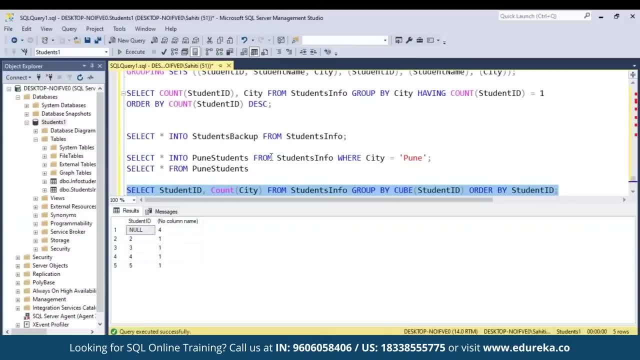 You can use the roll-up statement, So the roll-up is again also an extension of the group by clause, and this allows you to include the extra rows which represent the subtotals- So these are referred to as the super aggregated rows- along with the grand total row. 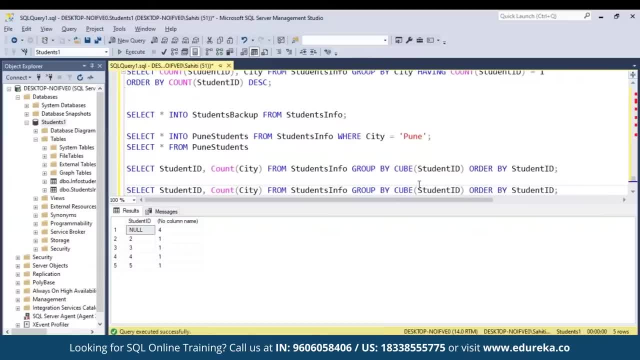 So, similarly to that of the cube clause, I'll just mention for the roll-up clause. So I'll mention select student ID count City from students info group by and then over here I'll mention roll-up and then I'll just remove this order by statement, right? 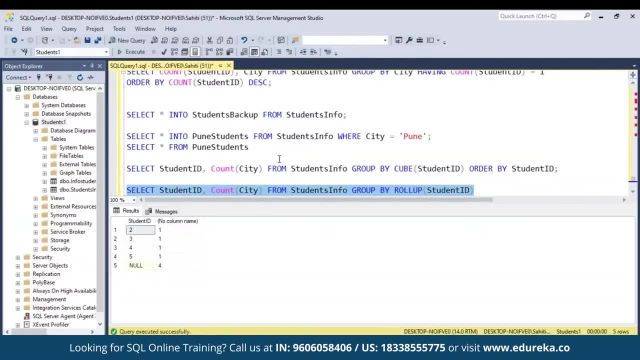 So you can just click on execute and then you'll see that you know the tunnel equal to 4 will come at the bottom of the table. So when you executed the cube statement, what you observe was that you know the super aggregated value. that was basically the subtotal. 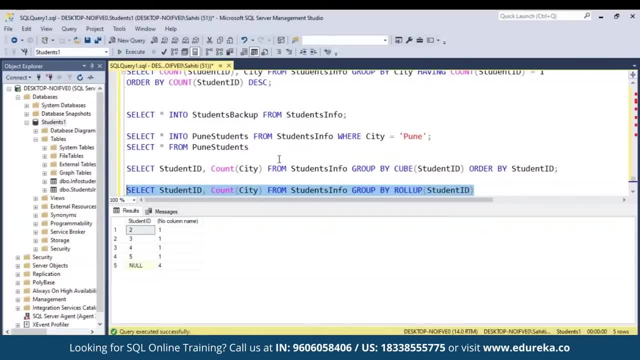 came in the first row, But when you execute the roll-up statement you see that you know it comes in the last row. So that was about the cube and the roll-up guys. now moving on to the next DML command, That is the offset clause. 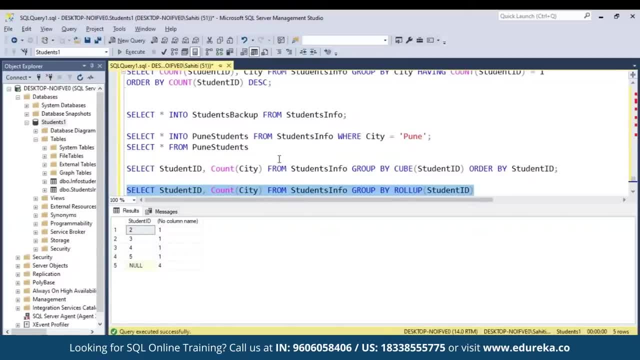 The offset clause is used with the select and order by statement to retrieve a range of records. It must be used with the order by clause, since it cannot be used on its own. Also, the range that you mentioned must be equal or greater than zero right. 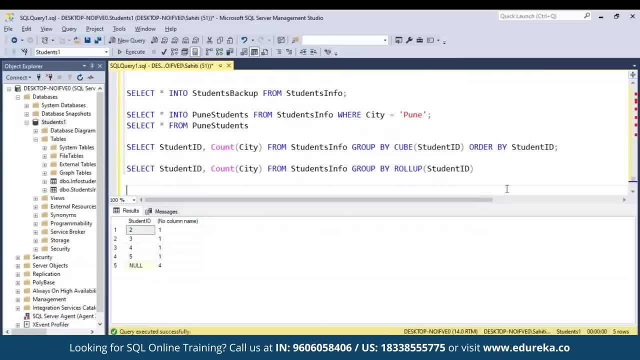 So if you mention a negative value, then it shows an error. So to demonstrate this, let's just create a table, right. So I'll just mention create table. Let's say offset marks, And then I'll mention marks int. So that will be our table column, right. 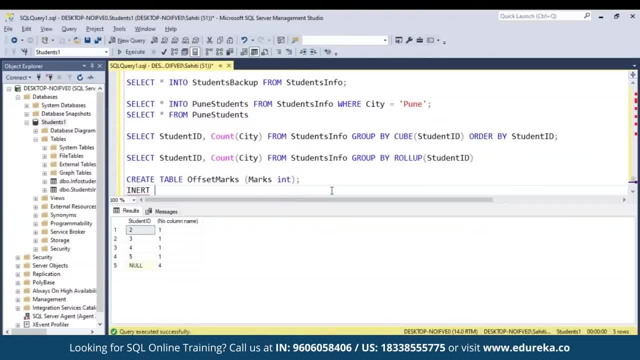 And then what I'll do is I'll just insert values into this, right, So I'll just mention insert into, and let's I'll mention offset marks, and let's say I mentioned a few random values, right? So initially I'll just execute this particular statement. 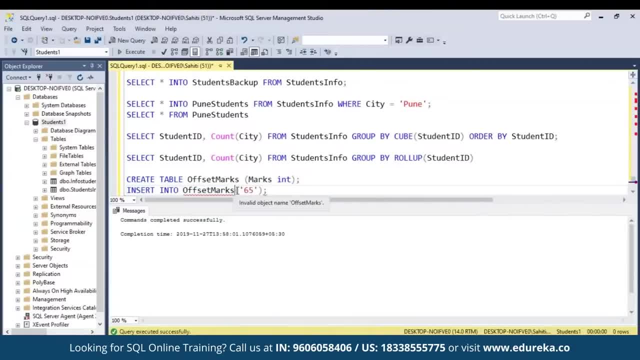 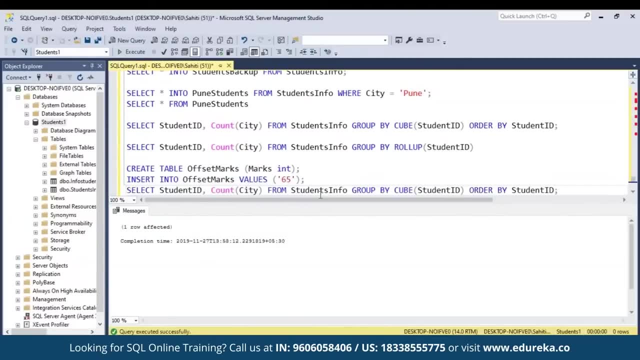 and after that, what I'll do is I'll just execute the statement before that. I forgot to mention values over here, right? So I'll mention values and execute this, and similarly I'll execute the other statements. So let me just copy paste and I'll just change the values over here. 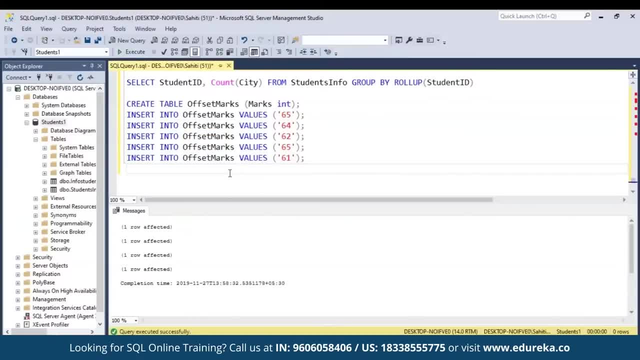 And then I'll execute again Now. after that, what I'll do is I'll use the offset statement, So I'll just mention select tar from. I'll mention the table name, that is, offset marks- order by marks, and then we want to mention offset one row. 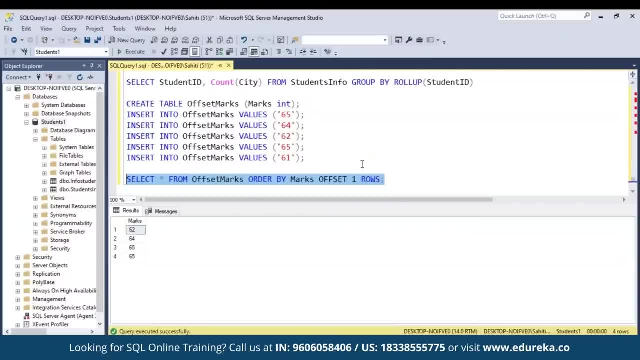 So that means our first value, which had 61. So when we use this order by marks, we see the table values to be sorted on 61, 62, 64, 65 and 65, and after that, when we say offset one marks, the first couple will be deleted. 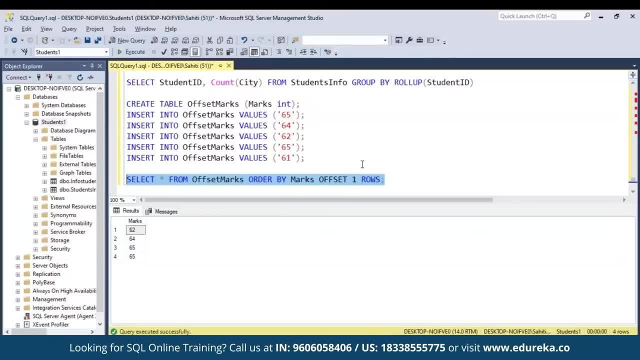 So that is the reason we get only 62, 64, 65 and 65.. So that's how we can use the offset statement, guys. Now let's move forward with the next one, That is, a fetch statement. Well, the fetch clause is used to return a set of number of rows. 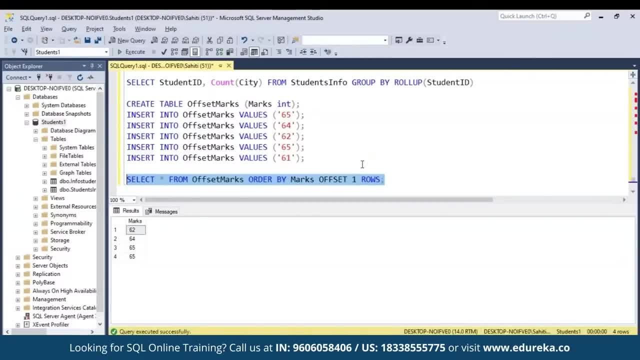 So it has to be used in conjunction with the offset clause, right. So to do that, what we'll do is we'll just mention select star from offset marks and then we'll mention order by, let's say, marks, right. and then what we'll do is we'll mention, let's say, 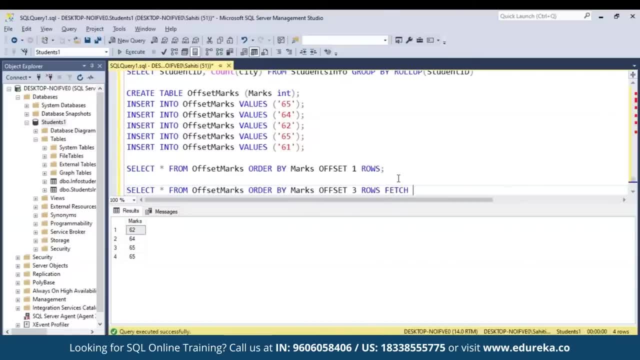 offset tree three rows and then fetch next two rows only, right. So we'll just fetch the next two rows after leaving the first three rows, right? So if I just execute this particular statement, we get the two rows, that is, 65 and 65.. 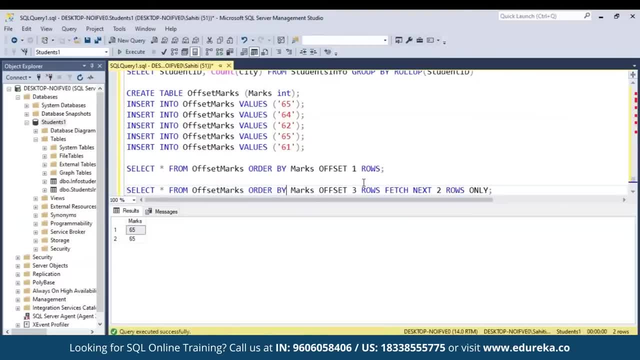 Now, similarly, you can also select the top three records from a table by using the top keyword, as I had mentioned previously also. So if we just mentioned selects top three star from offset marks, you'll get the top three doubles from the table. So, guys, that was about the offset clause and top class. 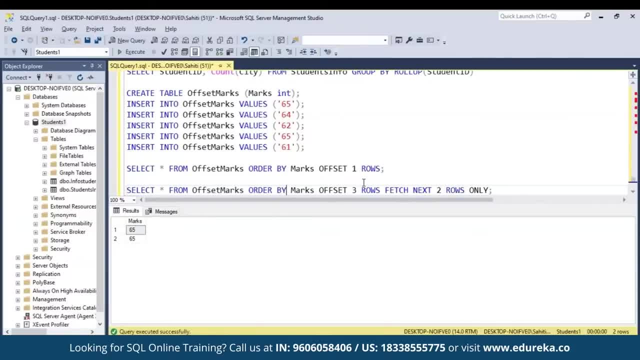 Now let's move forward with the next one, that is, the pivot. Well, the pivot is used to rotate the rows to column values and run aggregations, when required, on the remaining column values. Now, the syntax of pivot is also very simple, guys. 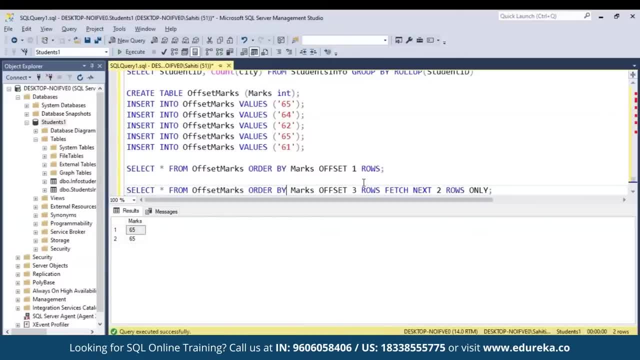 You just mentioned select non-pivoted column name, and then you've mentioned first pivoted column name as a column name, and then so on till the last pivoted column name as a column name from, and then you mentioned a select query which produces the data as a pivot. 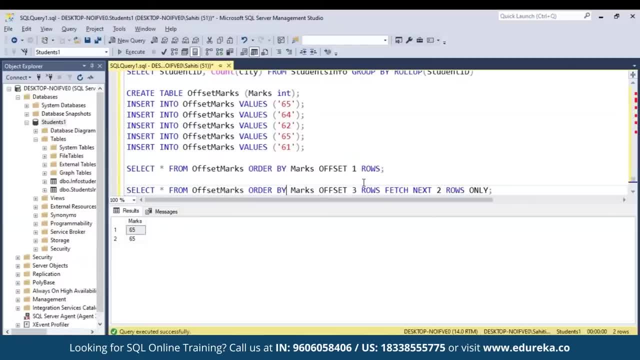 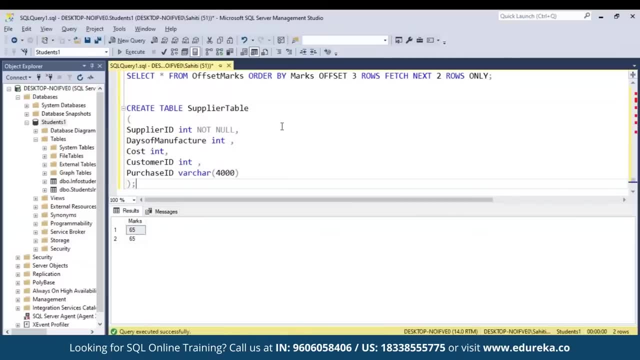 and then in the pivot section, you mentioned the aggregation function for the column name. So what I'll do is to give you a detailed understanding. I'll consider an example. So I'll just create a supplier table which has a supplier ID, the days of manufacture, the cost. 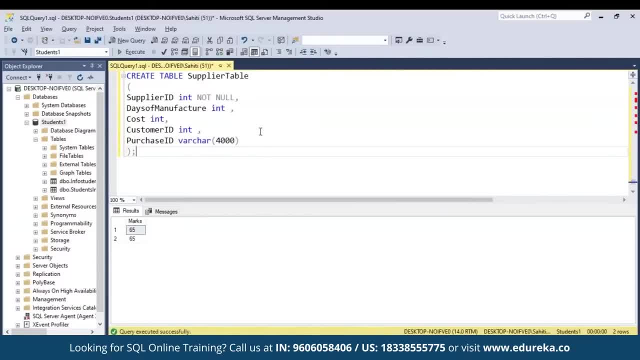 the customer ID and the purchase ID. right. our supplier ID should not be null, right. and then what I'll do is I'll just insert few values into it, Right? So let me just execute the statement first, right, after that I'll just go back. 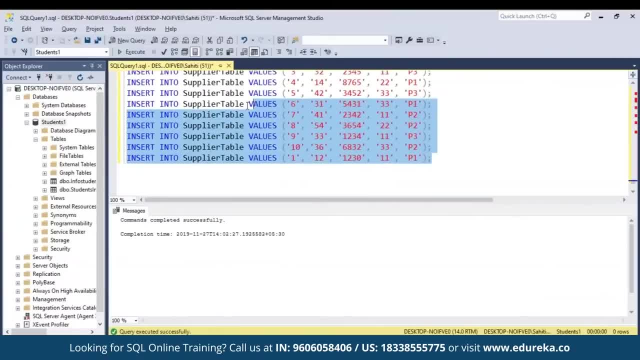 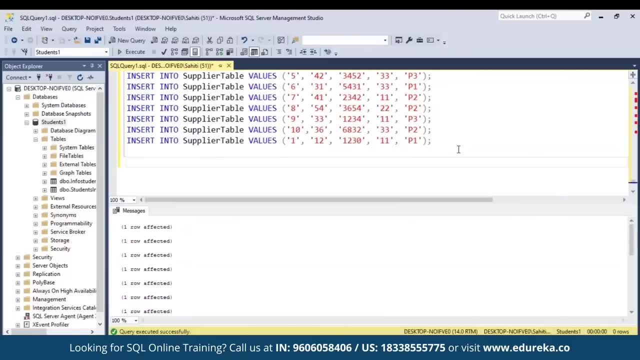 and then copy paste this section and then what I'll do is I'll just insert after the values have been inserted into the table. Now what I'll do is I'll just select the customer ID, the average cost, as the average cost of the customer from the supplier table. 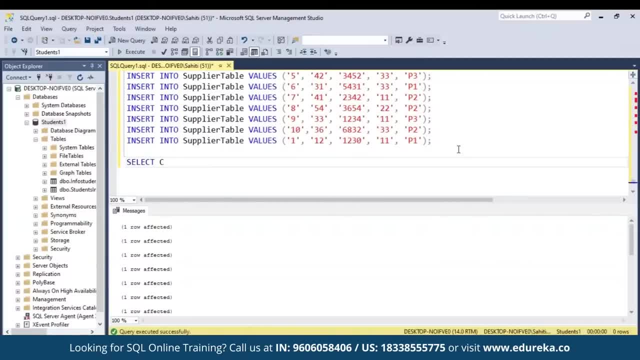 and then I'll group it with the customer ID, right. So for that I'll just type in the command select customer ID Comma average of cost as, and then I'll mention, let's say, average cost of customer from supplier. table group by, let's say, 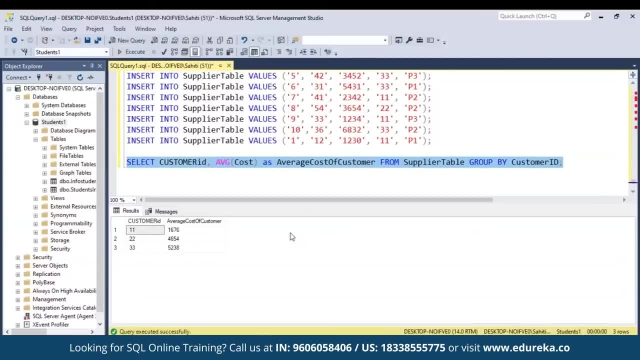 customer ID right and then I'll just execute the statement. So once I execute the statement, you see that you know we have the customer ID 11 and then the average cost of all the customers with the customer ID 11 is 1, 6, 7, 6. similarly, 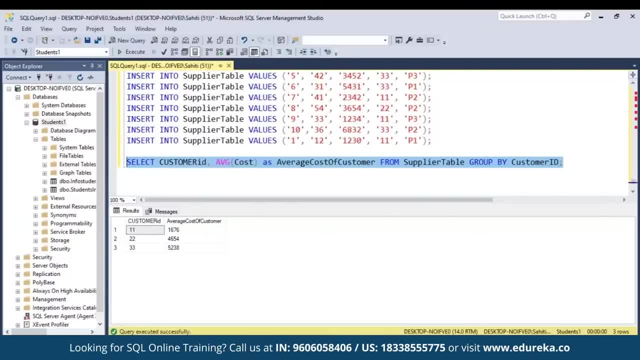 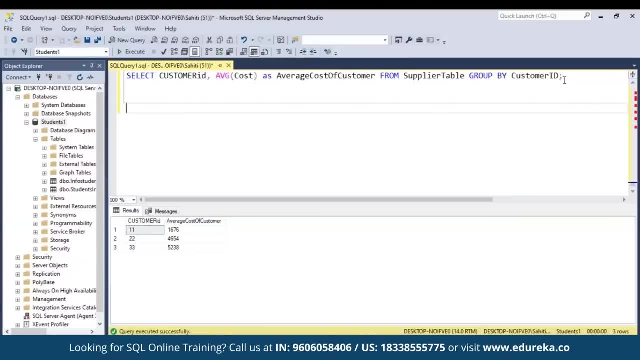 all the customers with the customer ID 22 have the average cost of customer as 4, 6, 5, 4 and similarly for the third one, that is, 33.. We have 5, 2, 3, 8. right now what we're going to do. 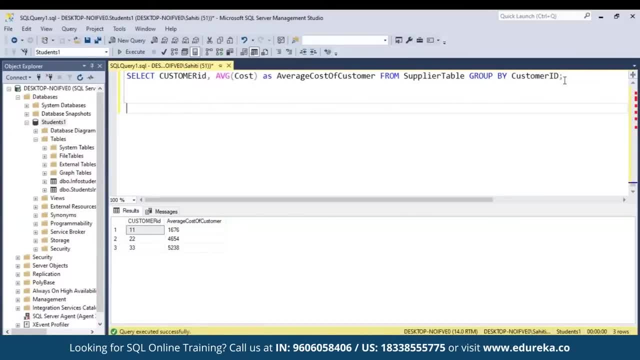 is we're going to create a sequel pivot table with one row and three columns. So over here, if you observe, we had three rows. Now what we'll do is we'll just create the pivot table with one row and three columns, right? 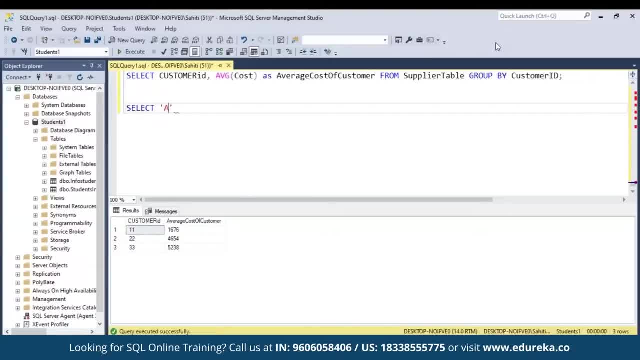 So for that we'll just type in the command select, Let's say average cost of customer, as, let's say, we just change it to cost according to customers, right? And then we mentioned one, one To two and three, three, and then we mentioned from. 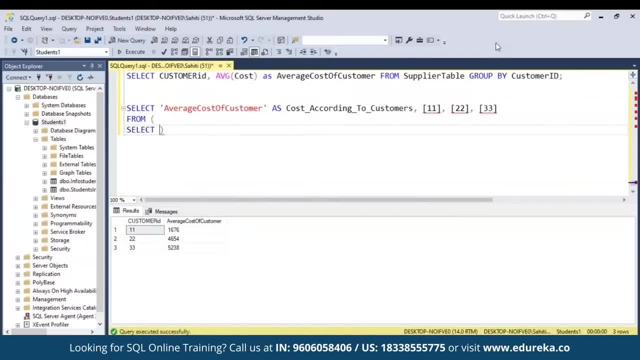 and in the inner section we mentioned select customer ID right, and then we mentioned cost from supplier table as, let's say, source table, and then what we'll mention is: we'll mention pivot and in brackets will mention average cost for customer ID And in brackets will mention 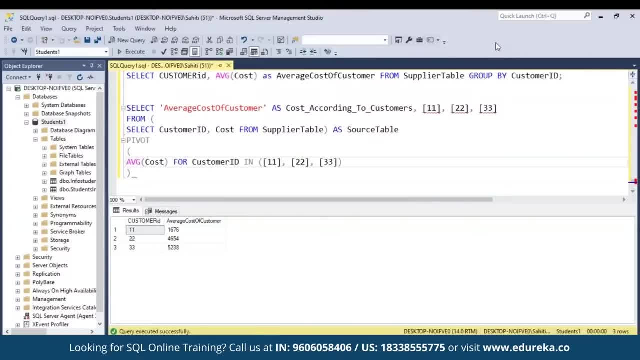 1, 1, 2, 2, 3, 3 as pivot table right. So I'll just mention pivot table right And then I'll just close, right. So I've just mentioned select average cost of customer as customer according to the customers: 1, 1, 2, 2, 3, 3.. 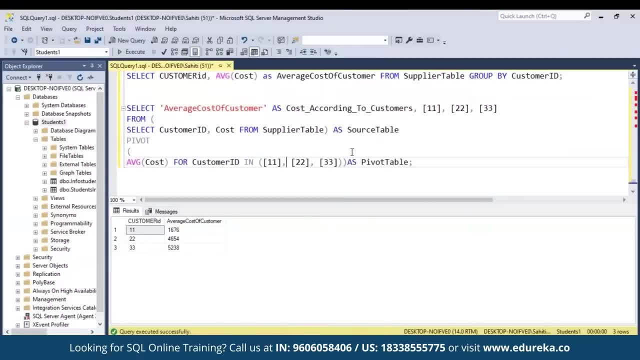 So we have one row and three columns. We want to select customer ID and cost from the supplier table, a source table, and then continue right, And so I'll just execute. So once I execute you can see that you know the average cost of customers has been named. 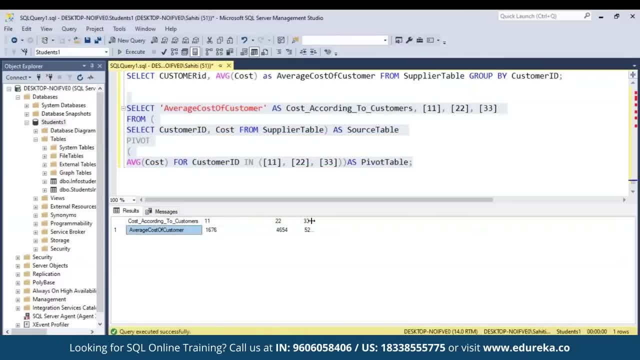 as customer, according to the customers, and we have 1, 1, 2, 2, 3, 3.. So we are. if I just drag, you can see that. you know the average has been put over here. So basically, in our previous table. 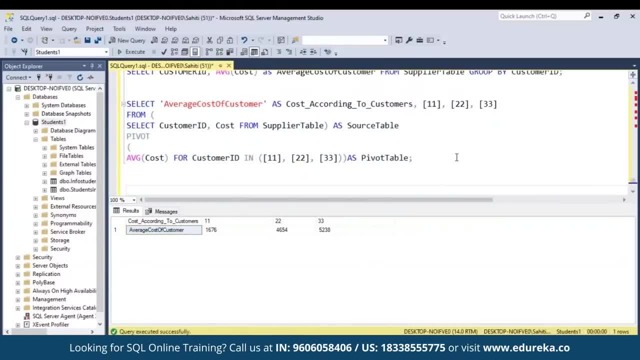 which were rows, have now become the columns. So that's how, guys. you can create a sequel pivot table Now. Similarly, you can unpivot it also. for example, let's say I create a table, sample table, and in that I mentioned supplier ID is the int. 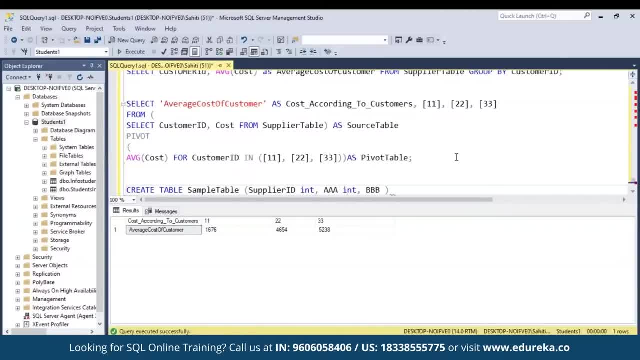 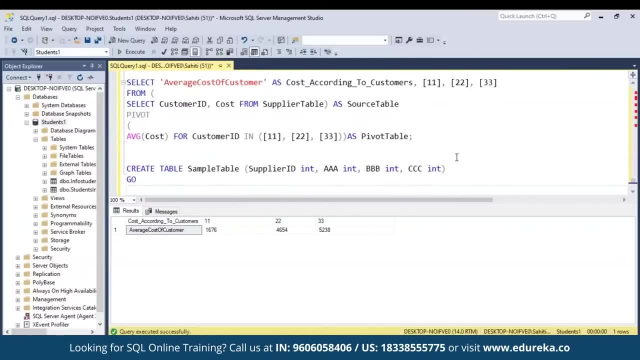 aaa of in type, Let's say BBB of in type and CCC of in type, right, and then I just type on go. and then I mentioned insert into, let's say, sample table. and then I mentioned values right in brackets. I'll just mention, let's say 1, 3, 5, 6, right. 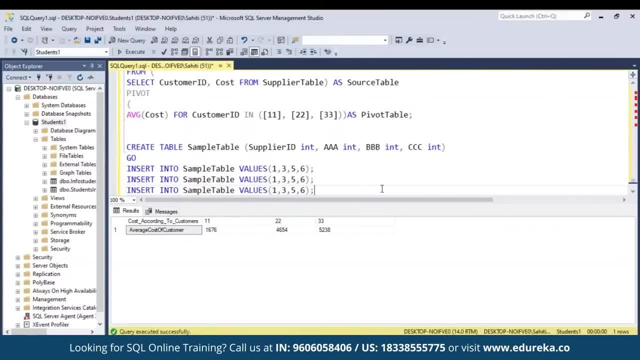 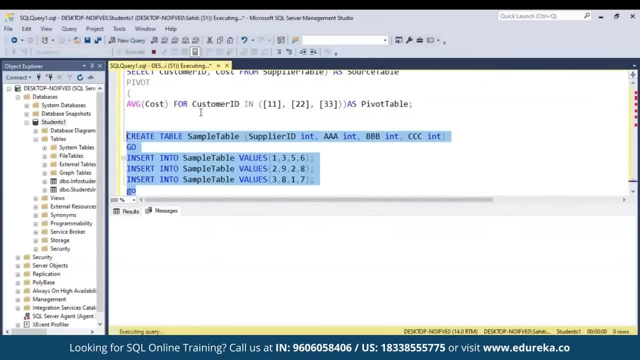 Similarly, I'll just mention the other values also. So let me just copy paste, All right, and then I'll click on go. So I'll just execute the statement, right and now what I'll do is I'll just show you the value. 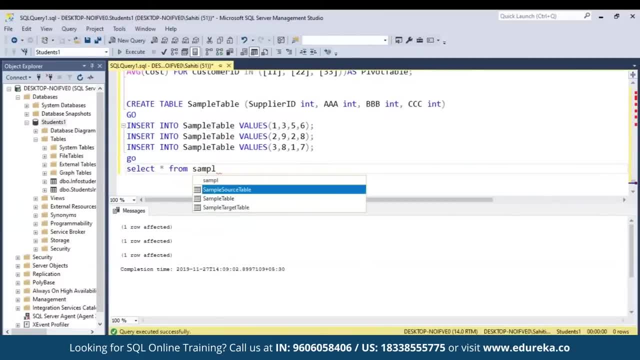 So I'll just mention select star from sample table, right, And I'll just execute this once. I execute this so you can see that. you know we have three rows in four columns, right? So we have the supplier ID and then we have a BB and CC. 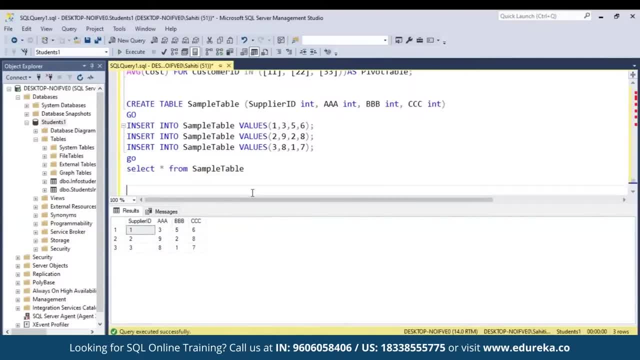 Now what we'll do is we'll unpivot it. So to unpivot it, what you have to do is you have to mention select- let's say supplier ID, that is basically a column names- and then we'll mention customers and let's say products. 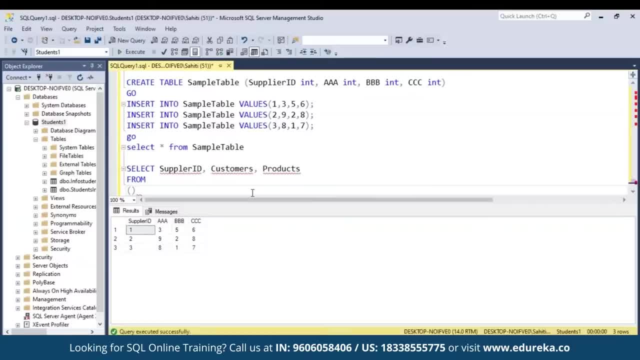 From, and in brackets again I'll mention select supplier ID and then I'll mention AAA, BBB and CCC and I'll mention from sample table, right. So I'll just give a space, give sample table And then I'll mention unpivot Right and over here. 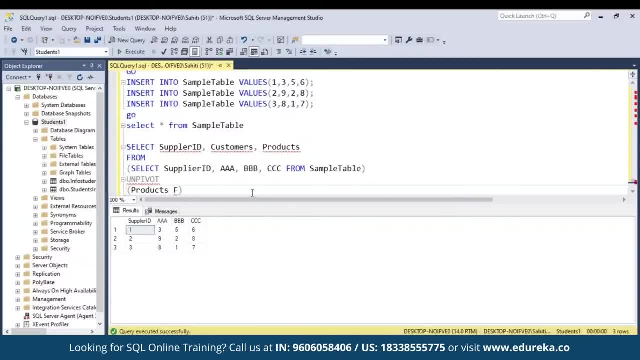 I'll mention products for customers in and in brackets. again, I'll just mention the values, that is, AAA, BBB and CCC, as, let's say, example Right, and then I'll just put on go Right, and then I'll click on execute. once I click on execute. 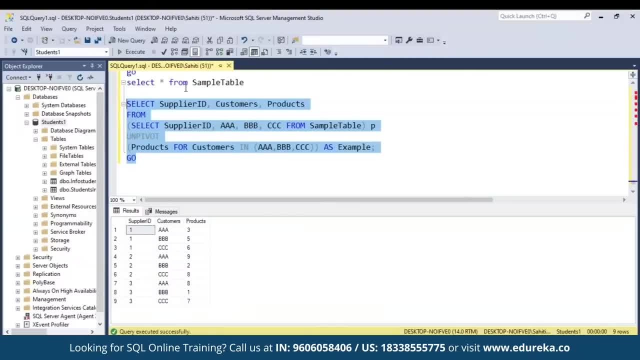 You can see that you know what we had as four columns and three rows has now been converted right. So for every customer that is AAA, the products show three. the values that we have entered previously are shown. For example, let's say a, which had value 398. 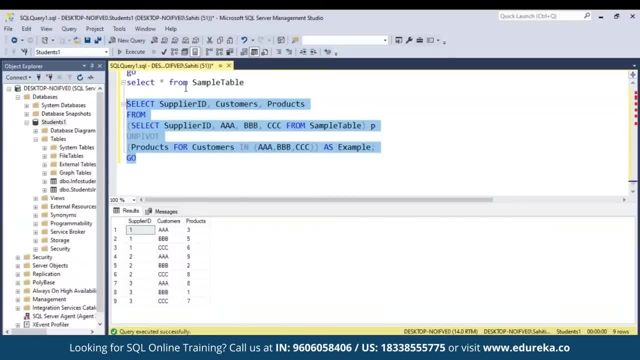 are now put into three different rows. similarly goes for BBB and CCC. So that's how you can unpivot the table also, guys. Well, that was about a little bit section of the DML commands. Now, if you want to know in depth about sequel, pivot and unpivot. 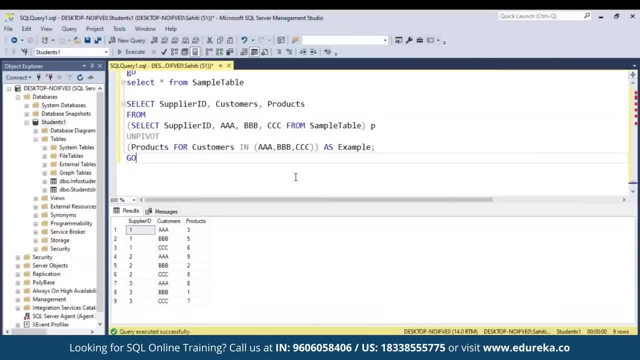 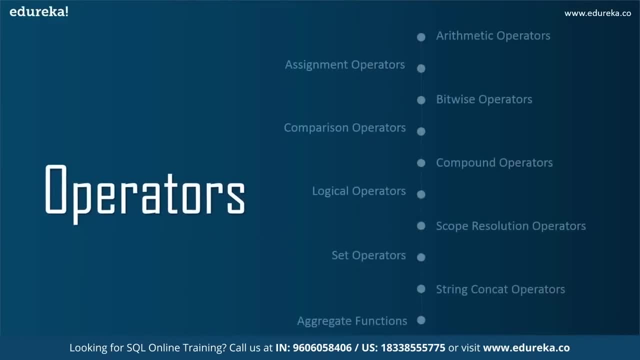 I'll leave a blog link in the description box below and you can refer to that. Well, guys, that was about this part of the section. Now let's move forward with the next part of the session, that is, operators. Now, I would say operators is a very important part. 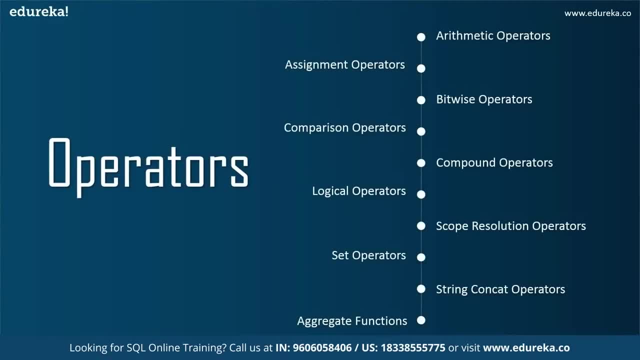 of the session, because operators play a very important role to handle and manipulate data, I would say different ways to retrieve the data right. So the different operators present in the sequel server are the arithmetic operators, the assignment operators, the bitwise operators, the comparison operators, the compound operators, the logical, the scope resolution operators. 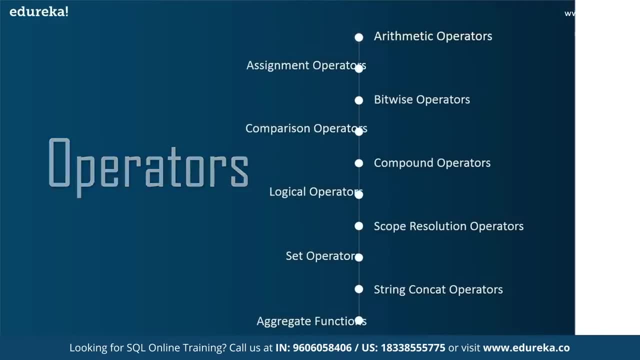 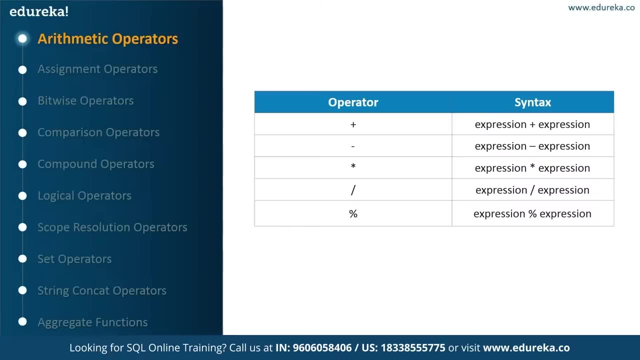 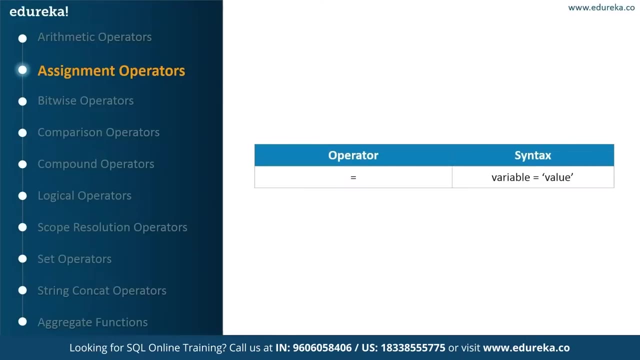 the set operators, the string, concat and the aggregate functions. So, talking about the arithmetic operators, first will the arithmetic operators have the addition, subtraction, multiplication, division and the model. I sign right so you can just add, subtract, multiply, divide or find the reminder. coming to assignment, The assignment operators are used to assign a value. 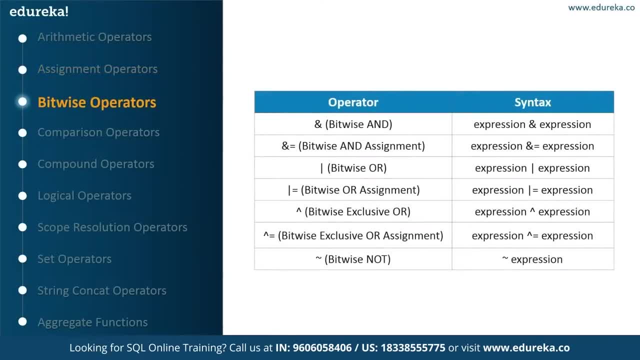 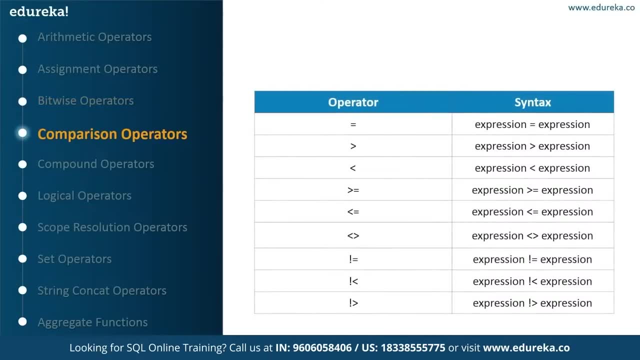 to the variable. coming to the bitwise operators, The bitwise operators are used to perform the bitwise and or an exclusive or operations. moving on to the next operators, that is, the comparison operators, Well, the comparison operators are the relational operators which are used to perform comparison operations like greater than less, than equal to greater. 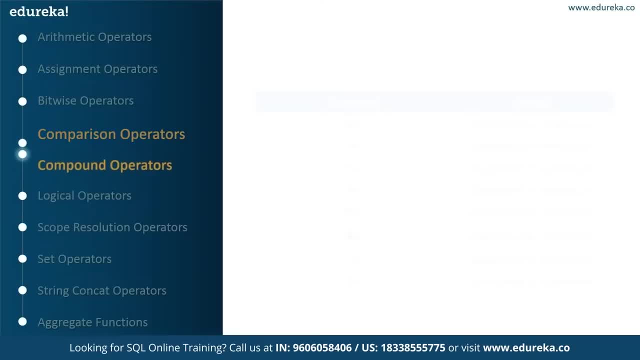 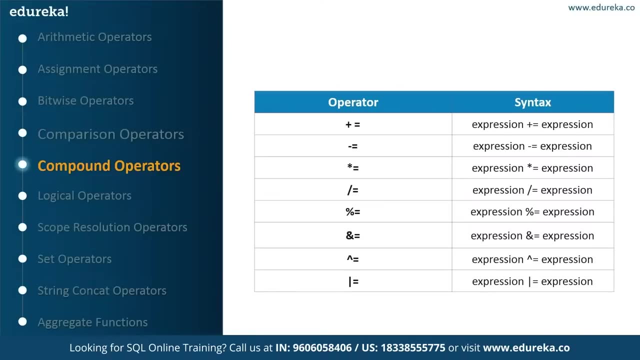 than equal to, not equal to, less than equal to, and so on. moving on to the compound operators, for the compound operators are used to perform the compound operations of addition, subtraction, multiplication, division, moduli and function or function, and this or function coming to logical operators, with the logical operators are used. 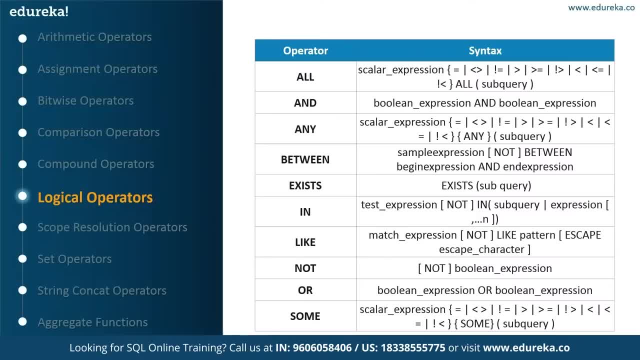 to perform logical operations between the data. So these are generally used in the nested queries. So the different kinds of logical operators are, as you can see on my screen, like all and any between exists In, like, not, or, and some right. I'm not going to go into the depth of each one of them. 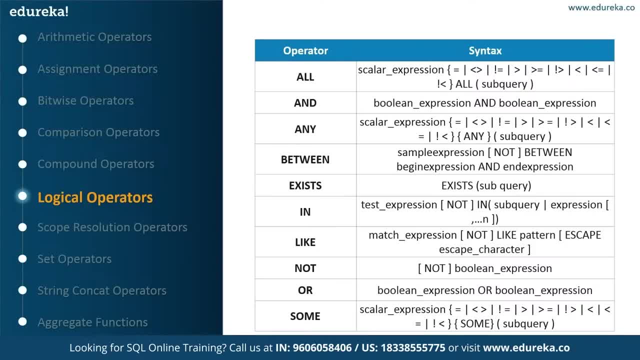 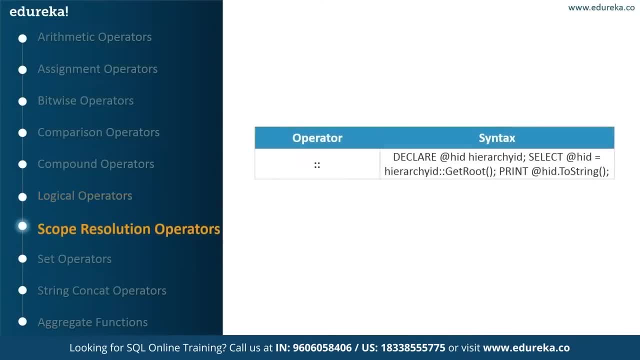 because you know it's completely based on your understanding of how which operator will benefit you better. But I would say the more you practice, the more you will have an understanding about the different operators. moving on to the next type of operator, that is, the scope resolution operator. 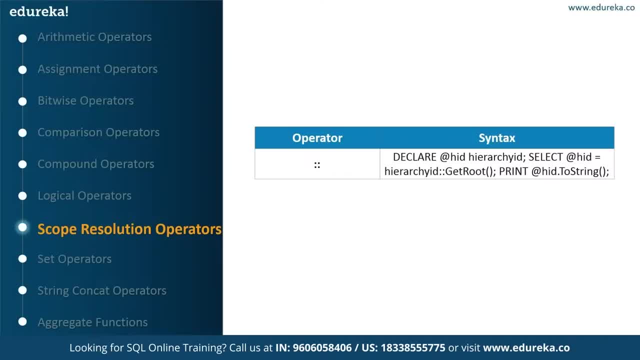 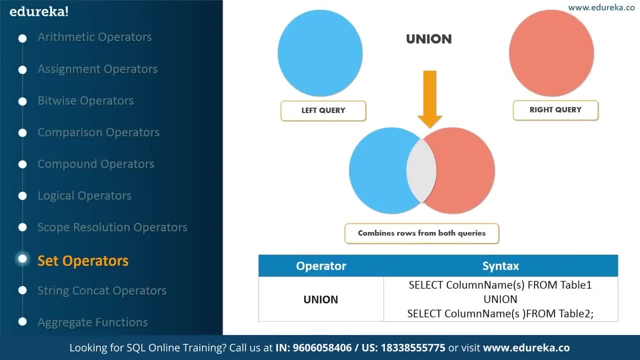 Well, this operator is used to define the scope and after the scope resolution operators, we have the set operators. So in the set operators we have the union operator, the intersect operator and the minus operator, So the union operators used to combine the rows. 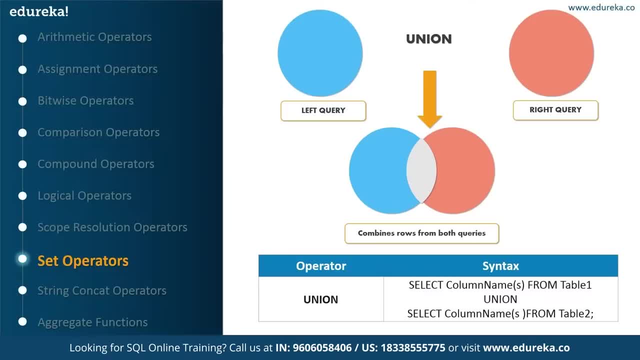 from both the query. So when you have a left query and right query and you perform Union operator and then you apply the Union operator, then automatically you will see that you know it will combine rows from both the queries. coming on to the intersect operator. 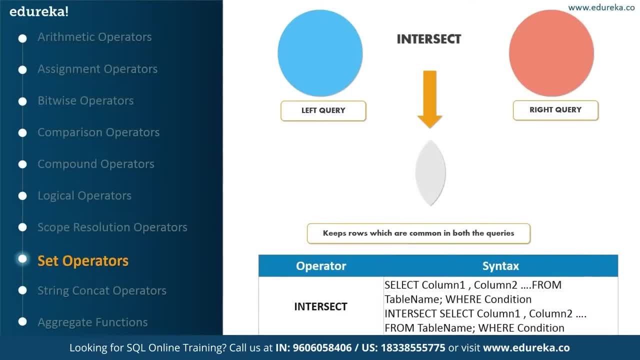 But the intersect operators is used to keep the rows which are common in both the queries right. So, for example, they could be few common queries in both the left query and the right query. then when you apply the intersect operator, only those queries will be taken into account. 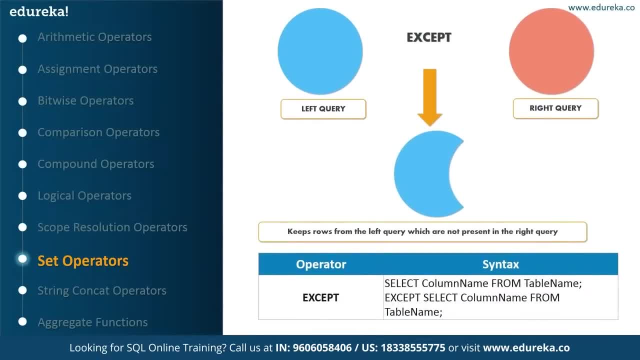 and finally, coming to the minus operator. the minus or the except operators used to keep the rows from the left query which are not present in the right query, and the vice versa right. So when you have two queries or the two tables, let's say left query and the right query. 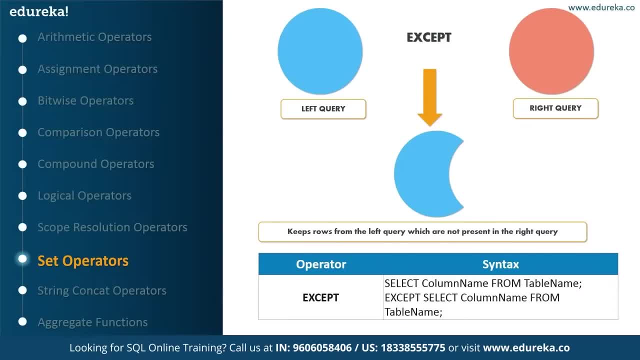 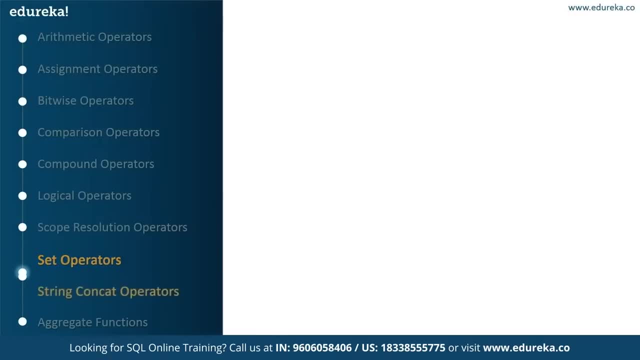 when you say a minus B, then it keeps all the rows from the left query which are not present in the right query. And if you say B minus a, then it keeps all the rows from the right query which are not present in the left query right. 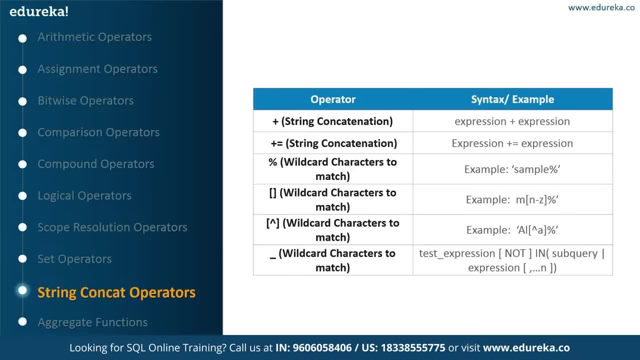 Now coming to string concat operators. Well, the string concat operators are used to perform various actions on the string, like you know: string concatenation, then wildcard characters to be matched, wildcard characters which match just a single value, or maybe multiple values, and so on. and finally coming, 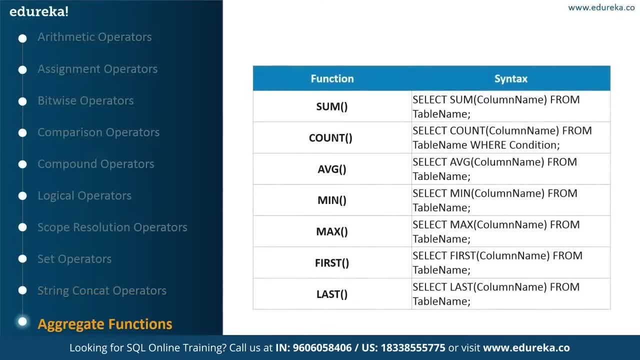 to aggregate functions, as I previously spoke about in the session. aggregate functions are used to find the sum, average, count, min, max, first and last values. So all of these operators are very simple to use, guys. for your better understanding, Let me give you a few examples. 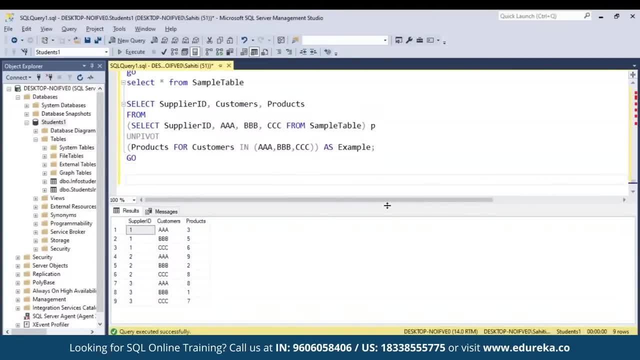 but I would say, the more you practice, the more will you benefit, right? For example, let's say you want to use the arithmetic operator. additions can just mention: select 40 plus, let's say 60, and then you can just exit execute. once you execute, you see the output as hundred. similarly, 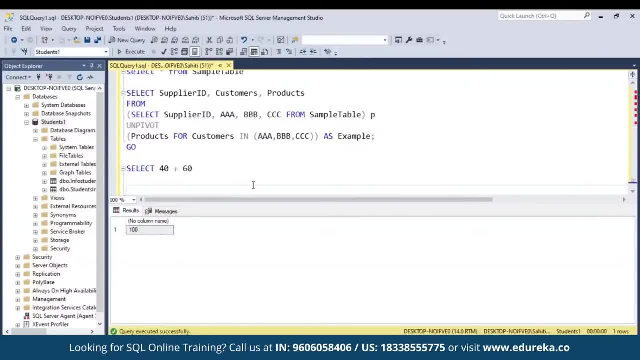 for example, let's say you want to use the comparison operators, Let's say greater than, equal to right. So for that you will mention select star from. let's say we choose a table offset marks where marks is greater than or equal to. and then you mention, let's say, 62. 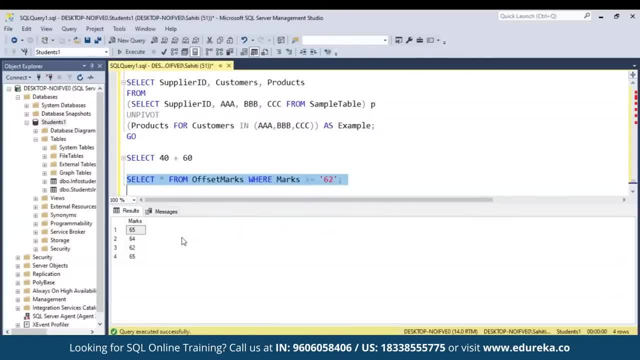 and after that you'll just execute. so you can see that you know, we'll get all those tuples which have marks which are greater than or equal to 62.. Now, similarly you can also use the compound operators also. for example, let's say: let's just declare two variables. 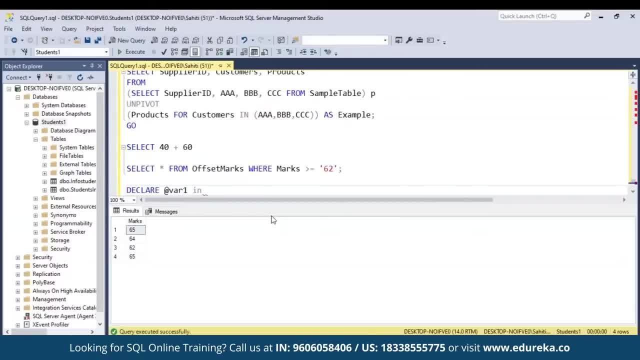 So I'll just declare, let's say, at the rate where one of n type let's say to be of 30, right. and then what I'll do is I'll just set it to be divided by, let's say, 16, right. 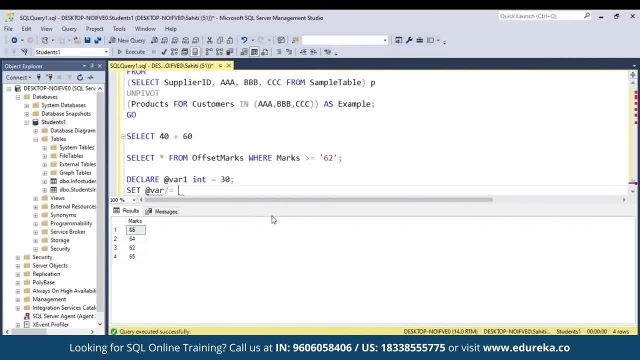 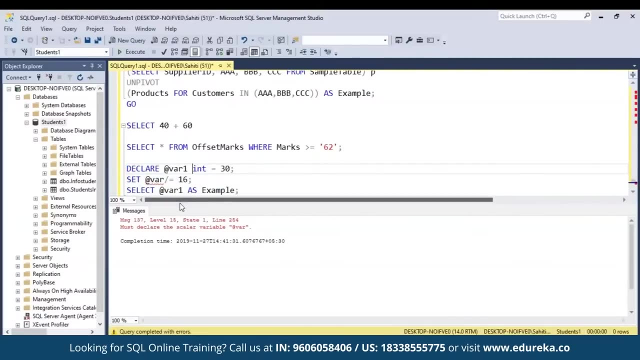 So for that I'll just use this compound operator and then equal to 16, right, and then I'll mention select at the rate where one, as example, Right, and then what I'll do is I'll just execute. or it says that we must declare it first. 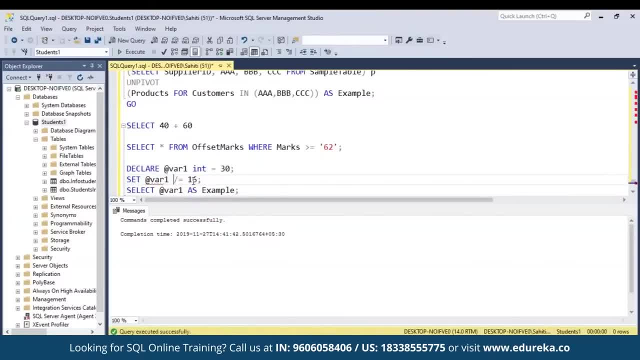 I'll just declare it first, and then what I'll do is: I'll just mention by one right, I'll just set as 16. I'll just execute it again. And when I execute it again, you see, the example is one- that is because you know. 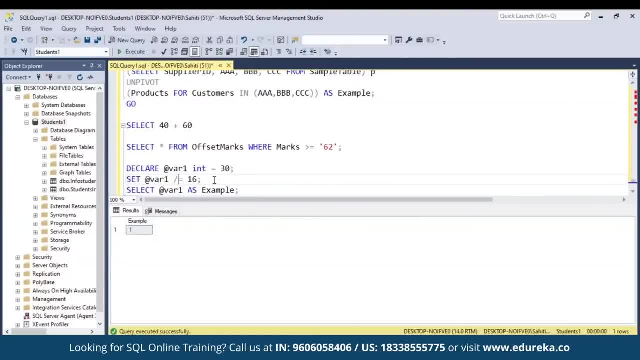 when we divide 16 by 30, our quotient is one. So, similarly, if you use the modular symbol over here, then you'll see the reminder right. So I'll just execute it again and then you see that reminder to be 14.. So that's how you can use. 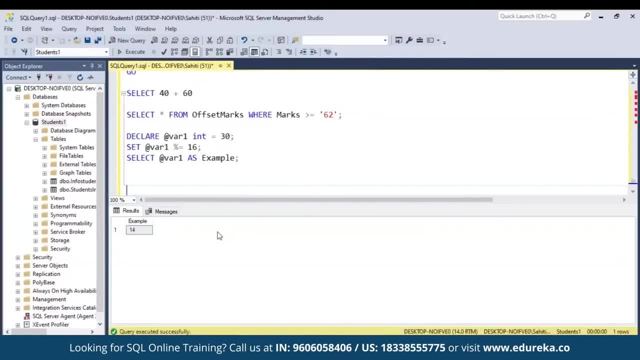 the compound operators. Now, let's say, if you want to use the logical operators- right, for example, let's say, if you want to find out the marks between 62 and 65, what you'll do is you'll just mention select star from. 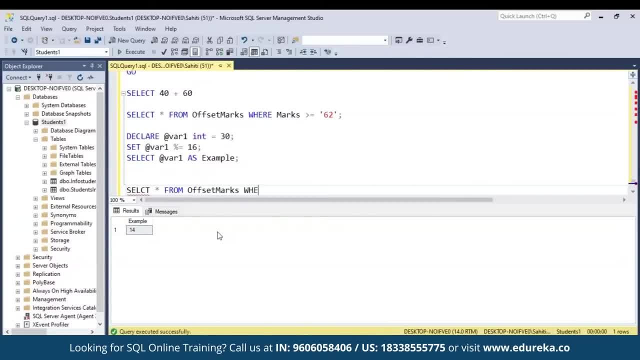 and then you'll mention offset marks, where, and then you'll mention marks, which is a column name, and then you'll mention between, and then you'll mention 62, and, which is again a logical operator, and you'll mention 65, right, Okay, my bad. 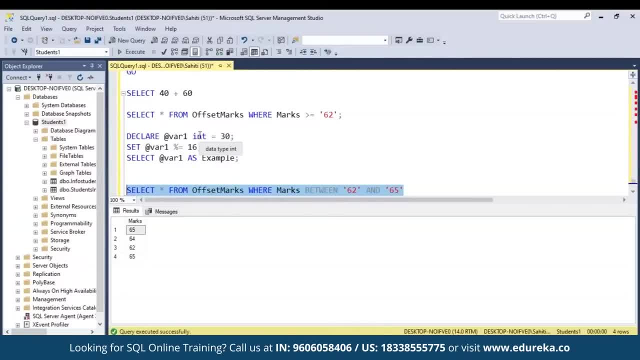 This has to be select, and then I click on execute. So we get all the marks between 62 and 65. now, for example, let's say we want to find out those marks which are greater than 62 or marks which are equal to 67.. 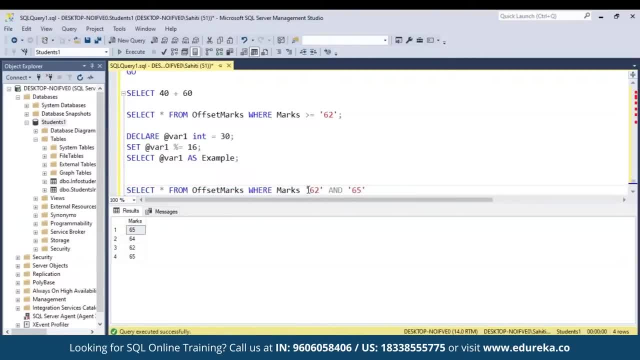 So what we'll do is we'll just change this statement, So select star from offset where marks- and then we'll use a comparison operators- are greater than 62 and or. I would say, or marks equal to what did I say? It was 67. 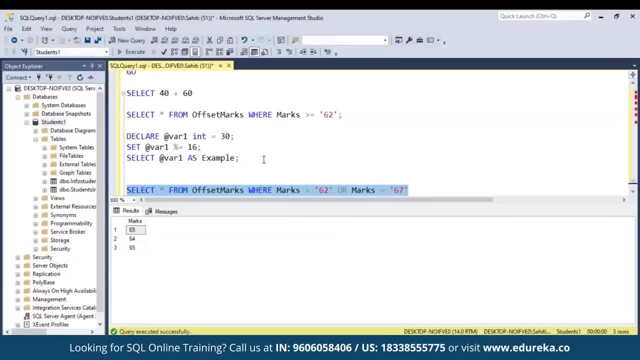 and then I'll execute Again. and then you see that you know, marks greater than 62 are just 64 and 65. So we get that. and since there are no marks which are equal to 67, we do not get that now. 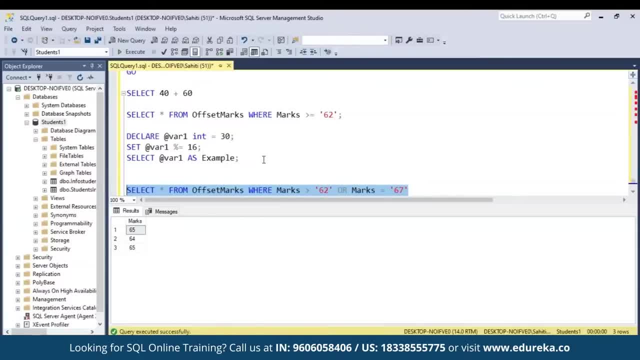 Let's move forward with the next one, That is, the like operator. So the like operator is one of the most popular question asked in your interviews. Now, this is since people often get confused between how to use the like operators right. So for that, I'll just show you a few example. 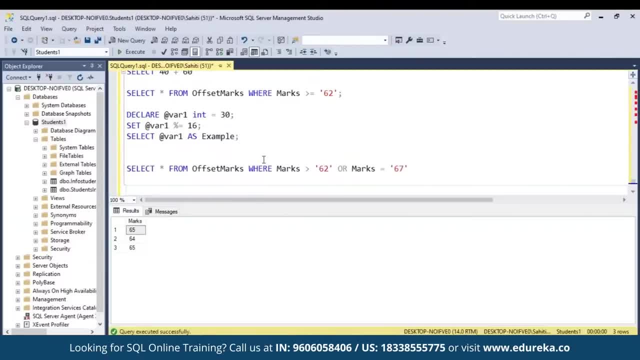 So let's say: you know we want to find out all those students name starts with. let's say s we'll just mention select staff from, and then we'll use students info right where I'll mention student name like, and then what I'll do is I'll mention s right. 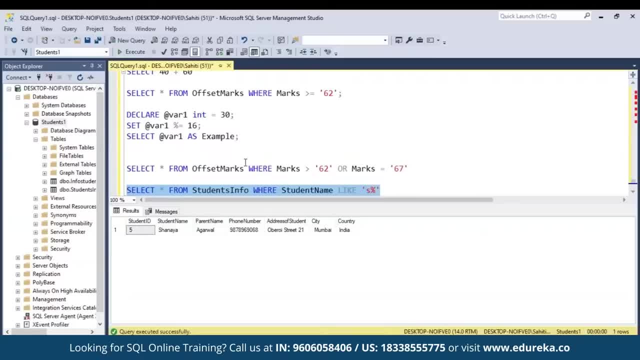 and then I'll mention the percentage symbol. So when I execute, we see that you know only one student with the name Shania, because her name starts with s, is in the result set. Well, that was about this query, guys. Now, for example, let's say you know. 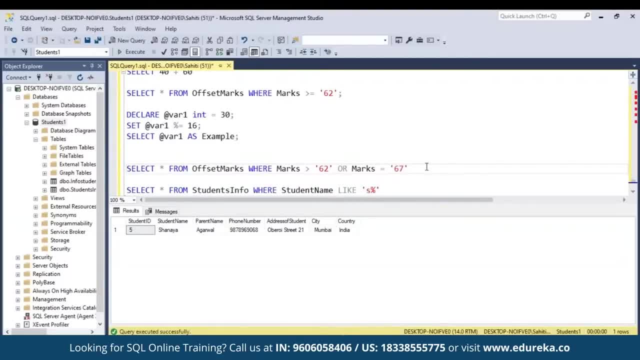 you want to find out the student name whose name starts with M and the name has six letters, right? So what I'll do is I'll just mention select star from student name like, and then I'll mention M, and then I'll mention five underscores. 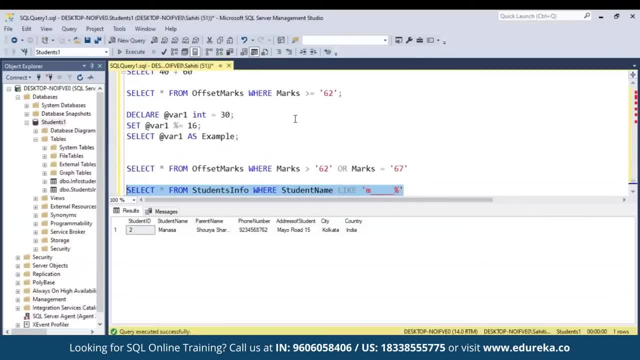 and then mention a percentage symbol right and then I'll click on execute. when I click on execute We again see only one query, because man says name starts with M and has around six letters, including M itself. So the five underscores were, for the rest, five letters. 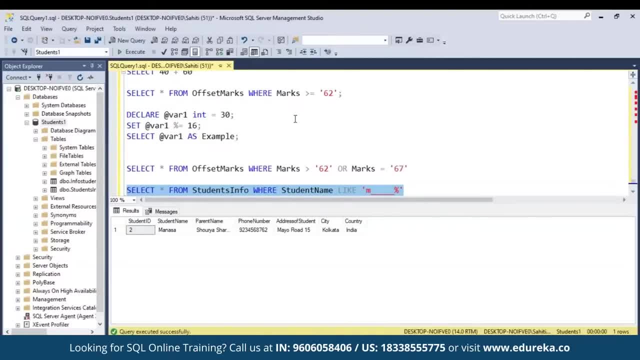 and M was the starting letter and percentage symbol represents anything can be there after that right. So that was about this particular query. Now let's say we want to find out all those tuples whose student name starts with M and then ends with a right. 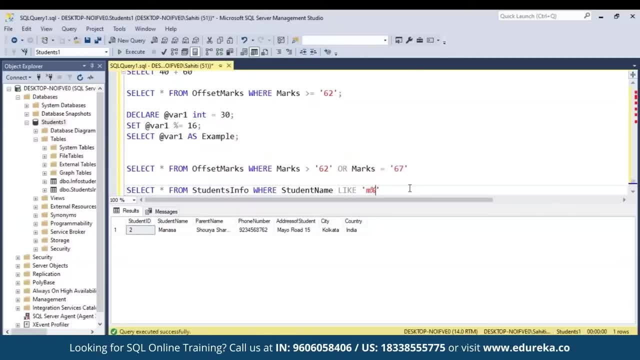 So I'll just change this particular query only. I'll just remove the underscore and then put a percentage symbol and mention a. what I mean by this particular statement is basically that you know the student name should start with M, should end with a and any number of letters can be present in between. 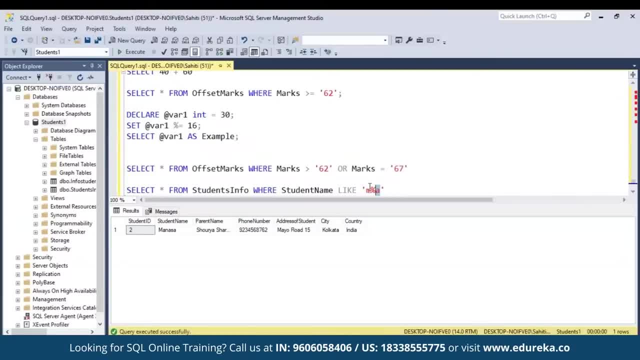 Well, that was about this particular query, guys. Now, let's say you want to use the scope resolution operator to access the get root member of the hierarchy ID type. Well, to do that, what I'll do is I'll just declare a variable. 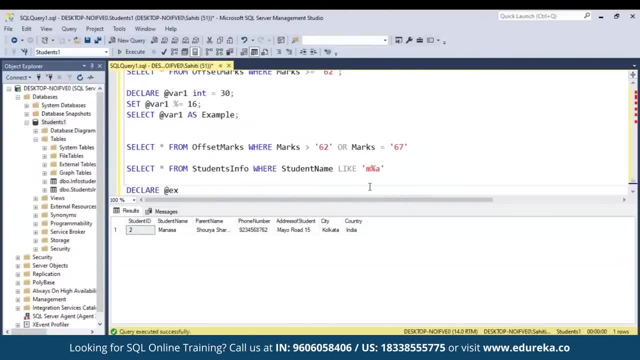 So let's just declare at the rate example ID of hierarchy ID type, and then what I'll do is I'll select this particular ID, right? So I'll just mention: select at the rate example ID equal to hierarchy ID and then I'll mention the scope resolution operator. 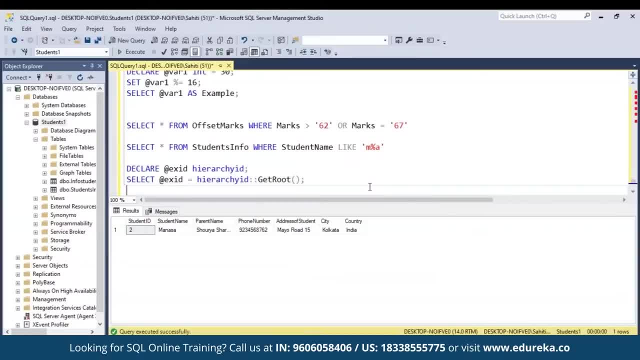 and then I'll mention get root. after that I'll just print at the rate example ID that is basically available to string. So basically I'm just converting it to string, right, and then what I'll do is I just execute this particular set of statements. 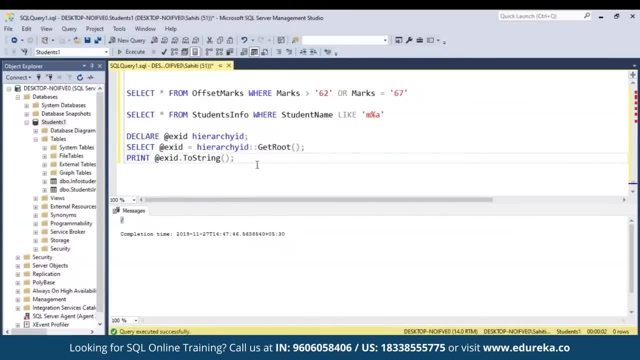 And then, once I execute the set of statements, you see this output. right, So that's how you can use the scope resolution operator also, guys, well, that was about this particular operator. Now let's say you want to use the string concatenation operators. 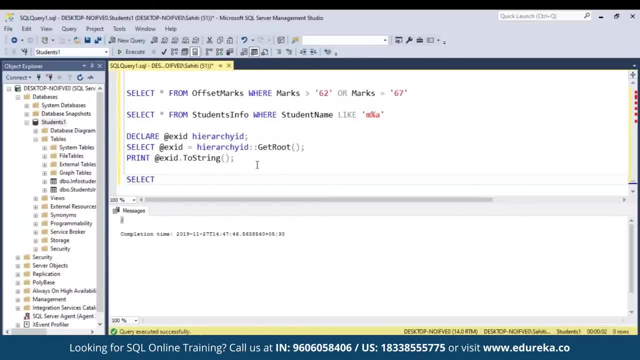 well, to use the string concatenation operator. Let me just consider the example of select. Let's say we take student name, right, So I'll just mention Student name, right, And then I'll put a plus mark over here. That is, I'm using the string concatenation operator, right? 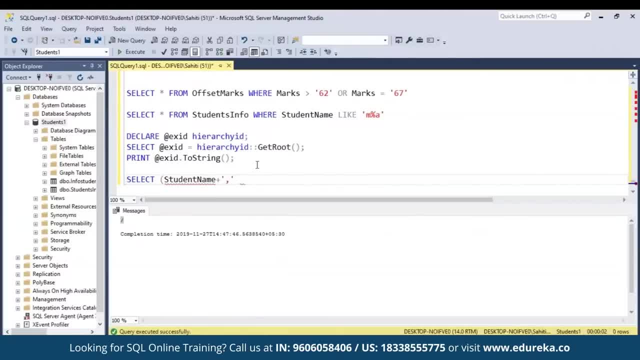 And then what I'll do is I'll just use single quotes, right, I'll put comma, and then I'll put a plus sign again and then choose parent name, right, And then I'll just use the aliases function. that is, I'm combining these two columns. 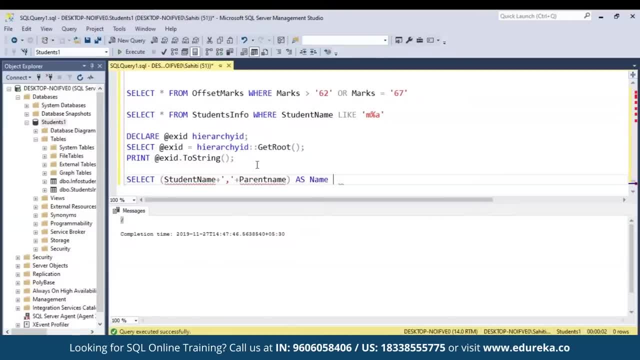 and putting it as another column and let's say I just mention it to be named from students info, Right, and then I execute. So, as you can see the output, you can clearly see that you know we've got a name column which has the concatenated values of the student name. 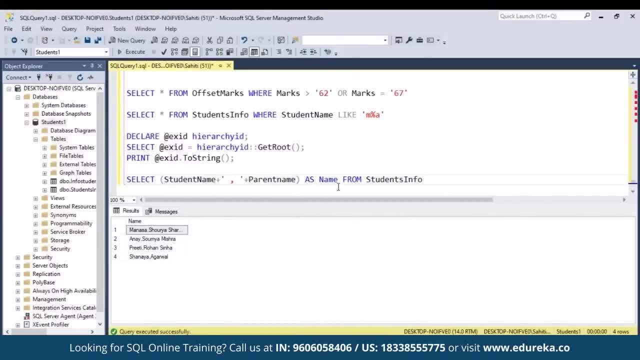 and the parent name. So if you want to give a space, then you have to mention spaces over here right, And then you click on execute again and then you can clearly see that you know the space is visible. So that's how you can use the string concatenation operators. 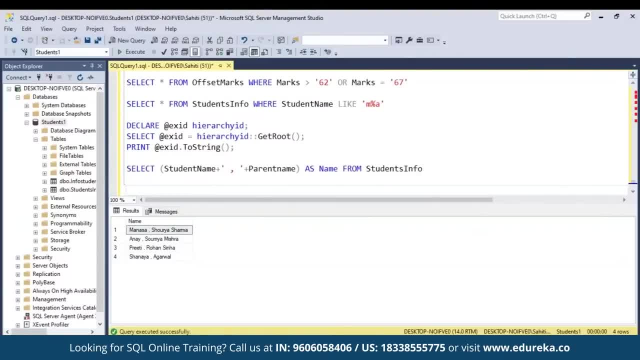 guys. Now let's say you want to move forward with the aggregate functions, but aggregate functions were used before, also when we were doing the order by and the group by clauses for your better understanding. Let's say, if you want to just calculate the average of all the marks, you'll just mention select. 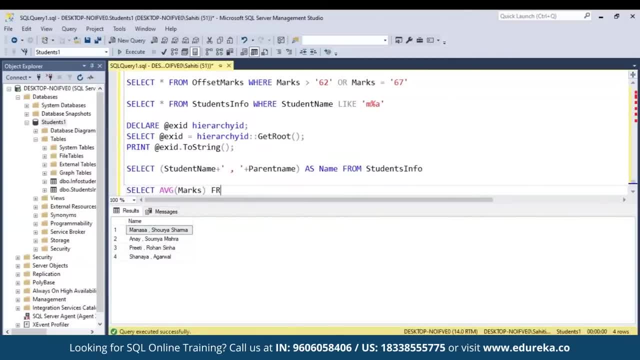 and then you'll choose average marks, right, So that's basically a column name, and then you'll mention the table name, that is, offset marks, and then you click on execute. So once you click on execute, we get our average of all the marks present. 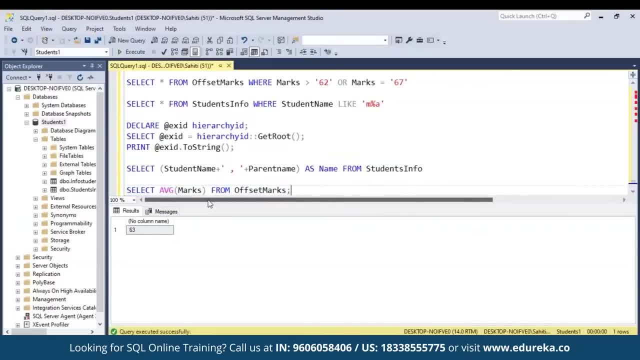 So that's how you can use the aggregate functions also, guys. Now let's move forward with the set operators. Well, as I explained before, the set operators consists of Union, intersect and the except operations. So what I'll do is I'll just consider another table. 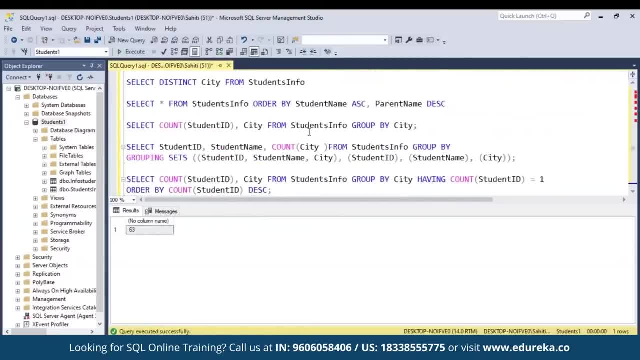 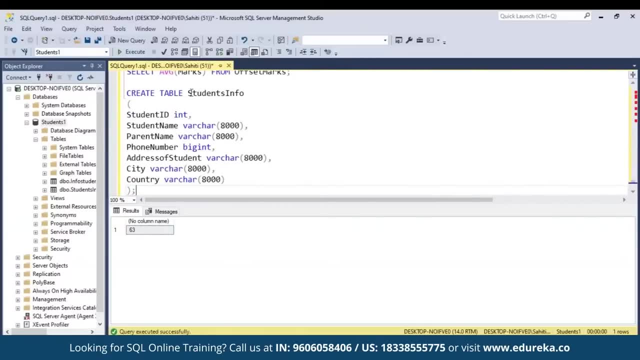 but it's similar to that of our students table, So I'll just create one more table. So let me just scroll up right and I'll just copy this particular section. Come down, paste it over here, change it to, let's say, students details. 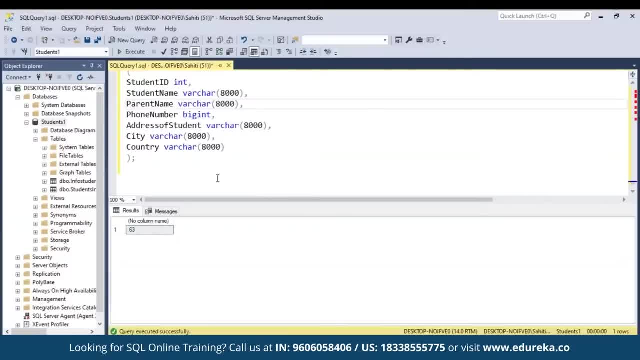 Right, and then I'll also insert few values, right. So let me just copy paste from over here so that it's faster. So I'll just execute this particular statement now and now, once a table has been created, I'll just execute these three statements again. 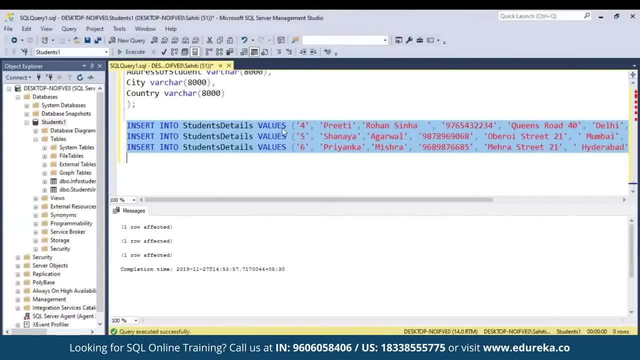 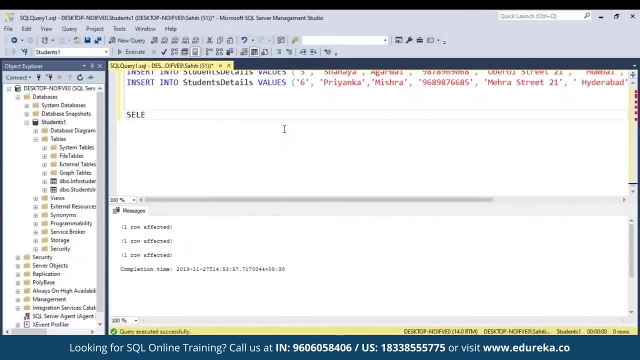 And now there are two tables- students info and students details- and both of them have few values. now let's just perform the Union operation, the intersect operation and the except operation. So I'll just mention select star from students info and then I'll mention Union. 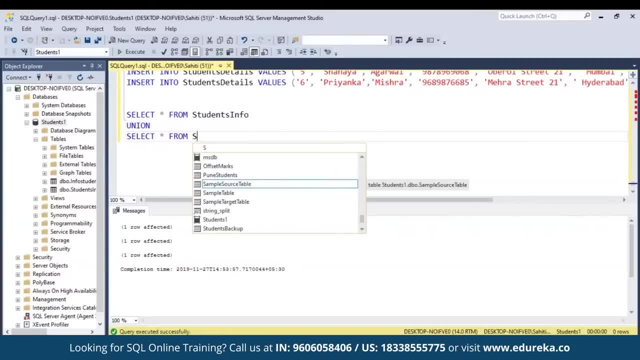 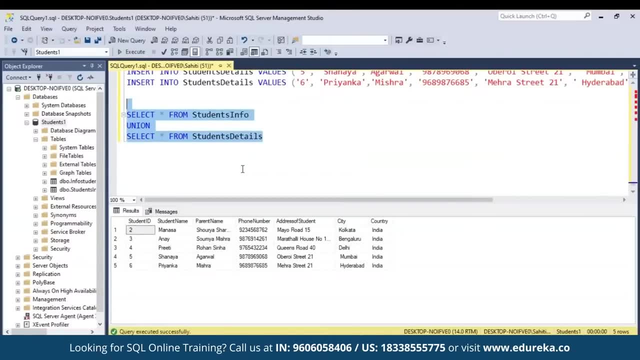 and let's say, we mentioned select staff from the table to, that is students details, right? So I'll just search for students details, right, And let's just execute now. Once we execute, you can clearly see that you know all our table values have been inserted. 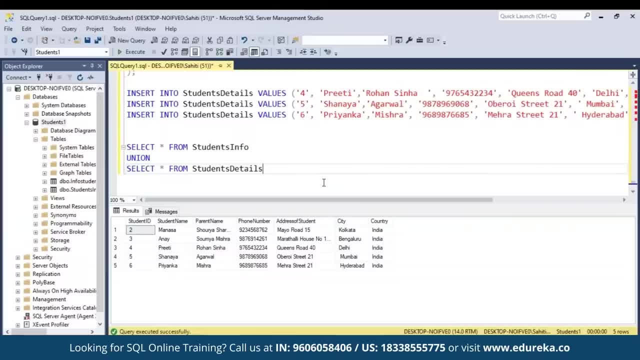 So we had few values in at first table and a few values in a second table, So all the values got combined into a third table. right now in similarly features do the intersect option. So I'll just mention intersect and then we can see the common values in both the tables. 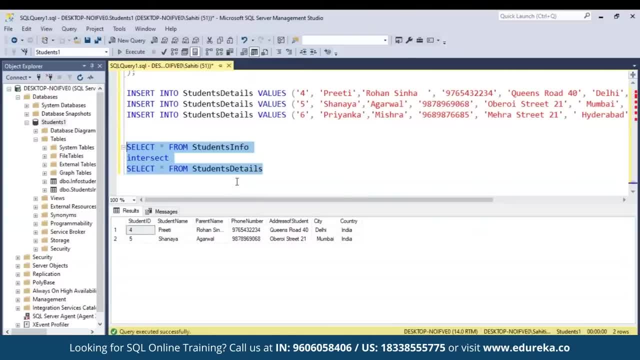 I'll just mention intersect and execute and we can see that you know. the fourth and the fifth record are common in both the tables. when I type in students info except students details, all the tuples which are present in students info and not present in student details are given as output. 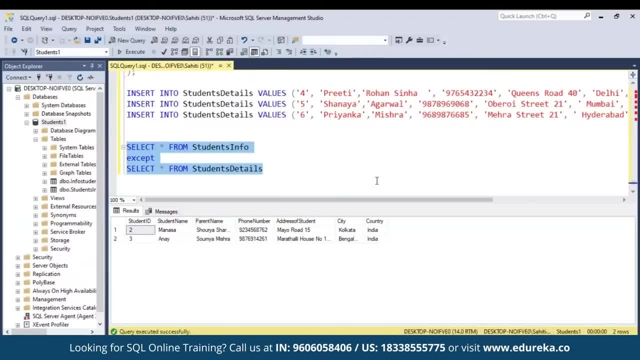 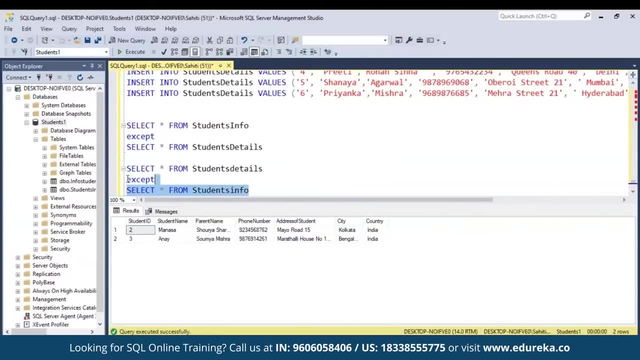 and similarly, if I just do the reverse- right, So if I just change it to students details- except students info, so let me just do that- and then I'll just do it to info over here- You'll see the opposite output, right. So that's how, basically, guys, you can use the set operators. 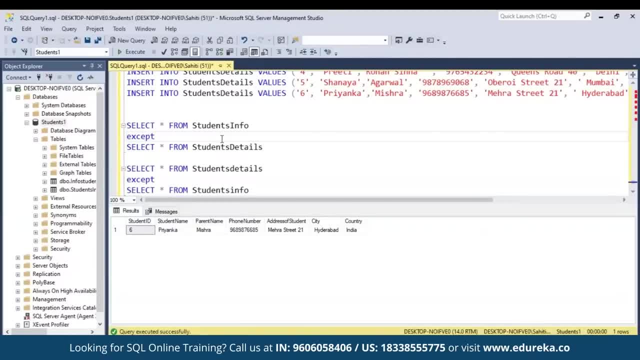 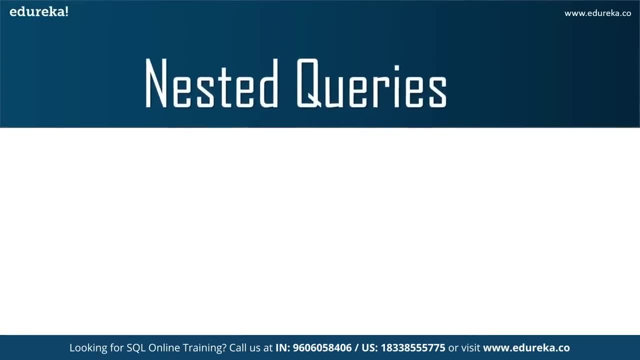 I hope that you've understood how to use the different kinds of operators to manipulate and retrieve and handle your databases. Now let's move forward with the next part of the session, that is, nested queries. Now, nested queries are also one of the most popular concepts that you need to know. 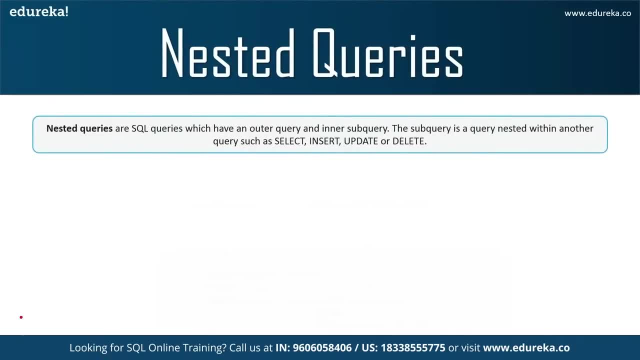 because, you know, nested queries are sequel queries which have an outer query and an inner subquery. So the subquery is a query nested within another query, such as the select, insert, update and the delete statements. So this was about the nested query guys. So, as you can see on my screen, 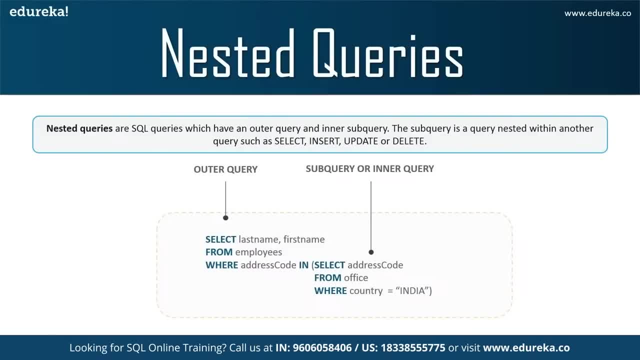 we have an outer query and then we can have a subquery. So what will happen is that, you know, the first, the subquery or the inner query, will be executed and whatever output comes, that output will be the input to the outer query and then we get the final output. 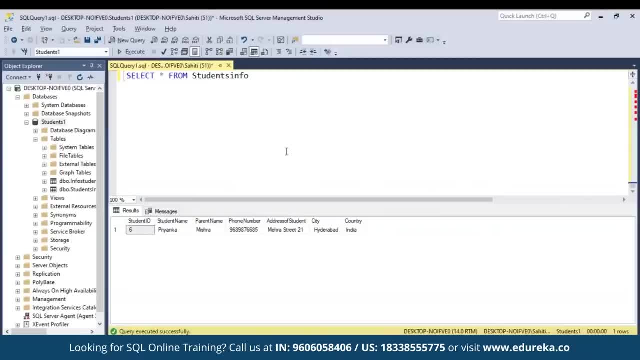 that was about the nested queries guys. So for your better understanding, if I have to give you an example, we can just write a query, like you know, select student name and, let's say, parent name from we mentioned students info right, and then I'll mention where address of student in. 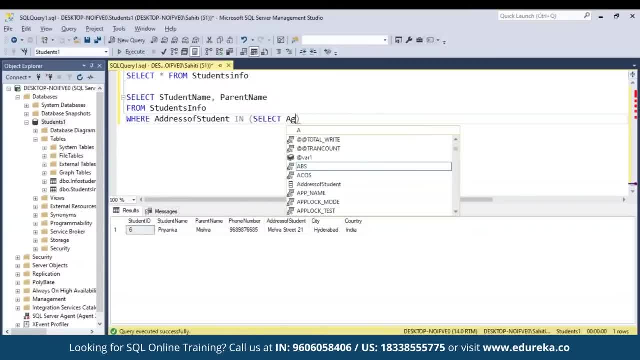 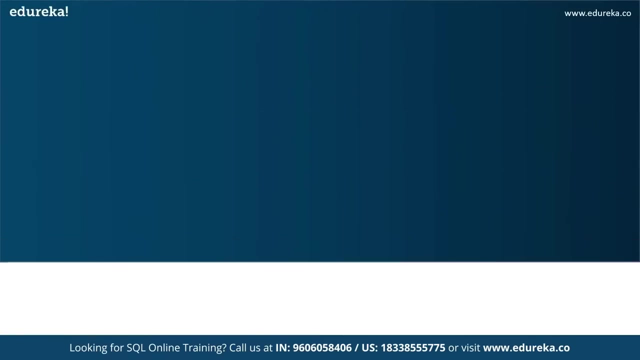 and then we can have an inner query which says select address of student from students backup that we had initially created, where, let's say, country is equal to India. right and now we can just execute this particular query and then we get the output. So that's how you can type the nested queries, guys. 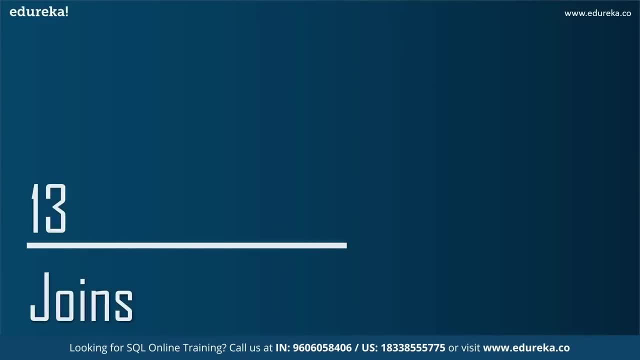 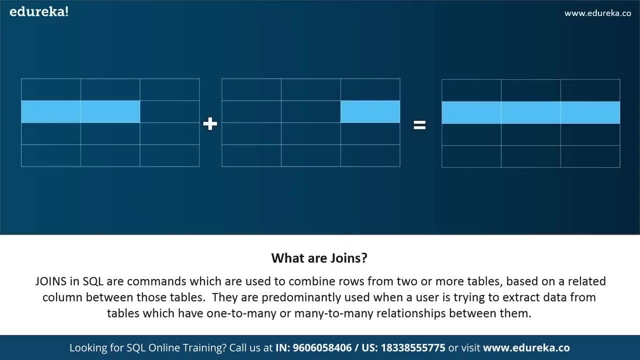 Now let's move forward with the next part for today's session, that is, joints. now, joints in sequel are commands which are used to combine rows from two or more tables based on a related column between those tables. So they are predominantly used when a user is trying. 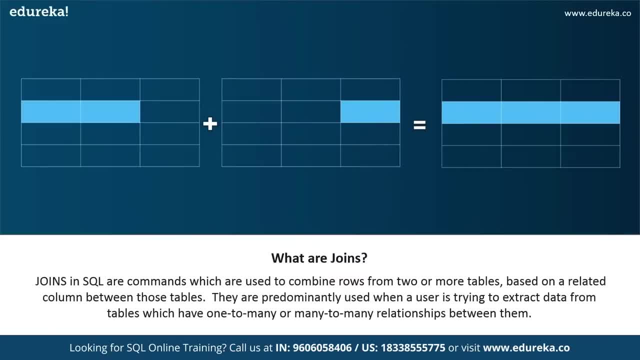 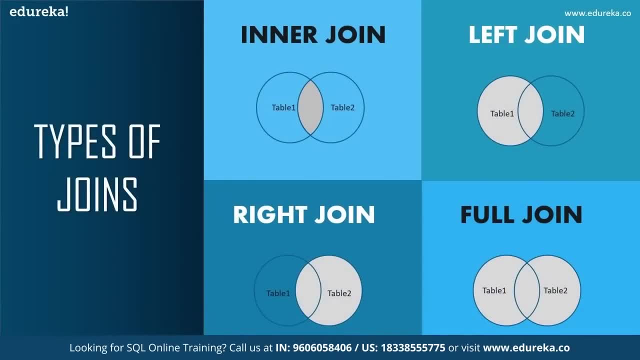 to extract data from the tables which have one too many or many too many relationships between them. Now, there are mainly four types of joints that you have to understand, guys. That is, the inner joint, the left joint, the right joint and the full joint. now, the inner joint returns the records. 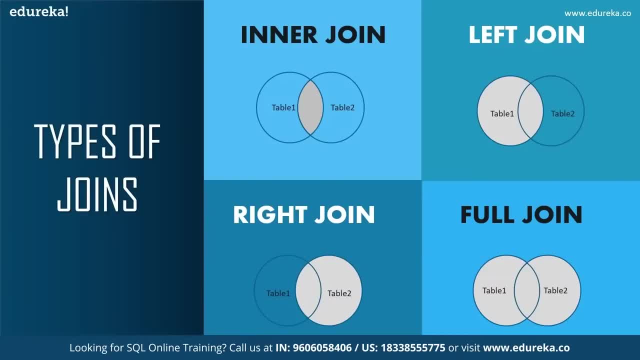 which have matching values in both the tables. the left joint returns the records from the left table and also those records which satisfy the condition from the right table. The right joint returns the records from the right table and also those records which satisfy the condition from the left table. 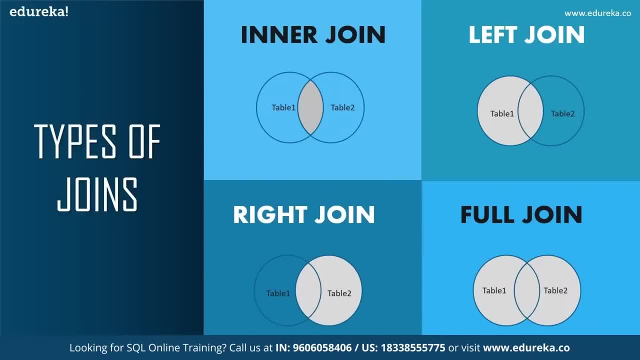 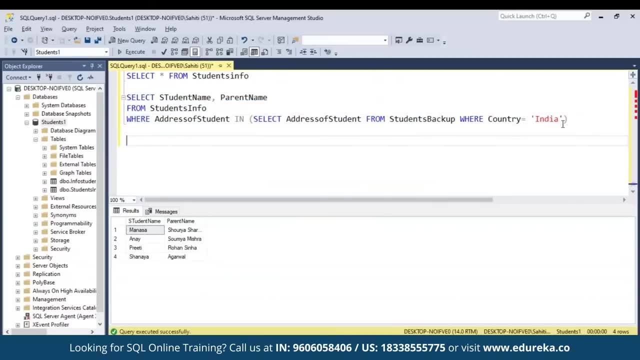 and finally, coming to the full joint. the full joint returns the records which either have a match in the left or the right table. So, for your better understanding, what I'll do is, I'll just consider an example. So, apart from the students info table, 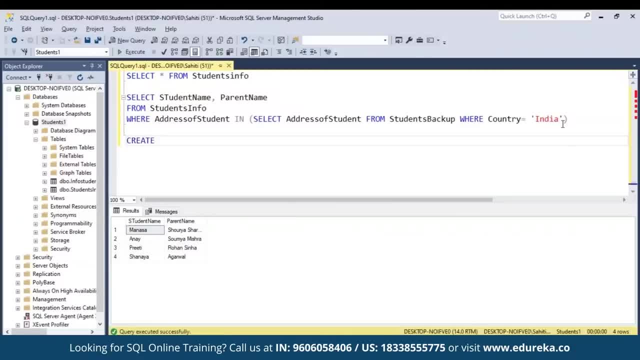 let's just consider the subjects table, right? So for that I'll just create the subjects table. So let me just type in create table subjects. and let's say we have subject ID of in type, right, and let's say we have student ID of in type. then we have subject name of, let's say, varchar type. 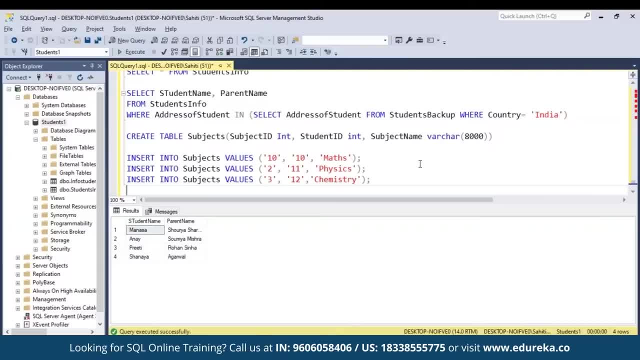 and after that let me just insert few values. So I'll just mention: insert into subjects value 10, 10 maths and 211 physics and 312 chemistry. So I'll just execute these statements now. once the statements are executed, let's apply the joint functions. 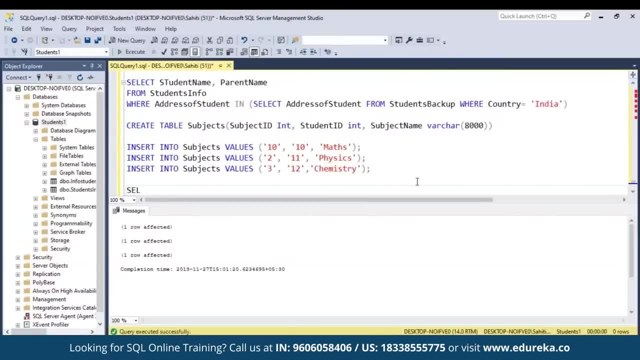 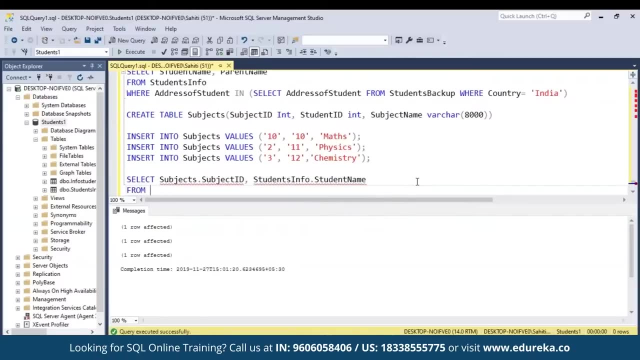 So let's say we want to apply the inner joint right. So we'll just mention select subjects dot, subject ID and let's say students info dot. and we want the student name right from both these table from, we want from subjects table. that is a table a. 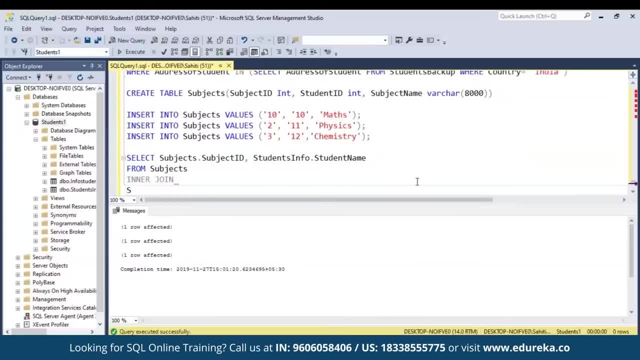 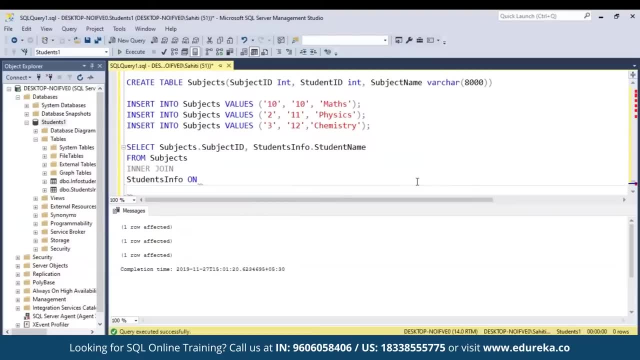 and then we'll mention in a joint that is a joint condition. and then we'll mention the second table name, that is, students info, and will mention on and after that will mention the condition that the subjects Dot- student ID must match students info, dot- student ID right. 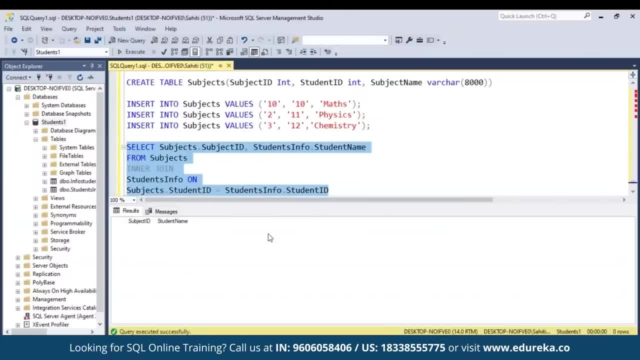 and then we'll just execute this particular statement. and once you execute the statement PC that you know there are no common values present. So that is the reason we do not get any values. Well guys, that was about the inner joint. Now let's say we want to apply for the left joint right. 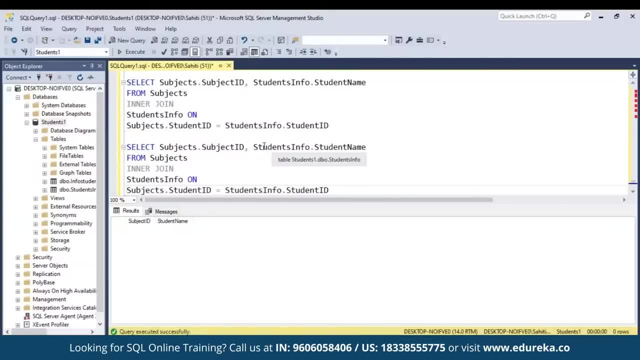 So what I'll do is I'll just select students info dot, student name, and let's say we also select the subject ID from the subjects table and let's say our first table is students info. Right, So that is what we are considering over here. 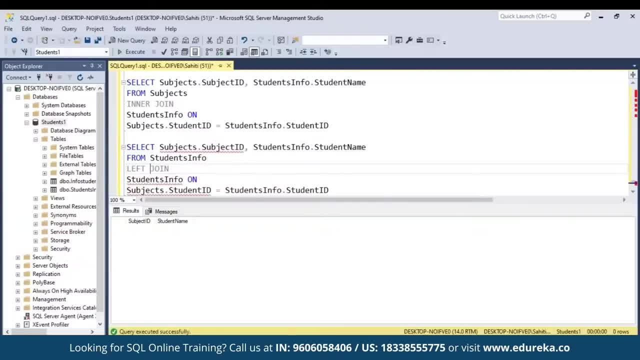 and over here I'll mention left joint and after that what I'll do is I'll mention the other table name that the subjects, and then I'll mention on, and then what I'll do is I'll just match the students info: dot. student ID equal to subjects: dot. subject ID. 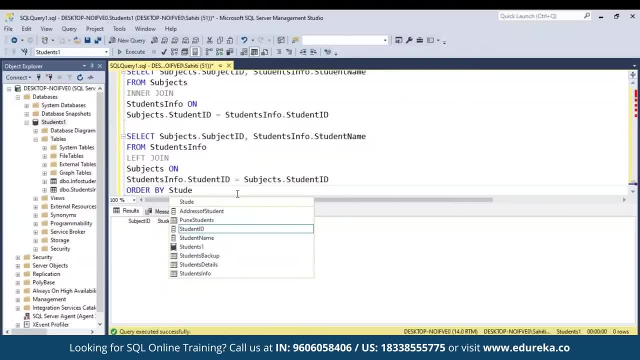 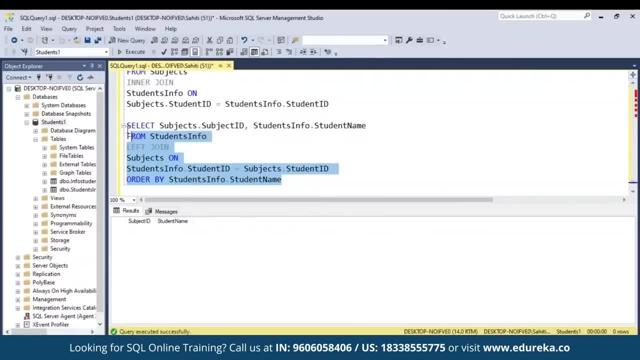 and then let's say we order it by the student name, right? So I'll just mention students info, Let's say student name. Right now I'll just execute this particular The statement and then we can see that. you know, we get all the values from the left table. 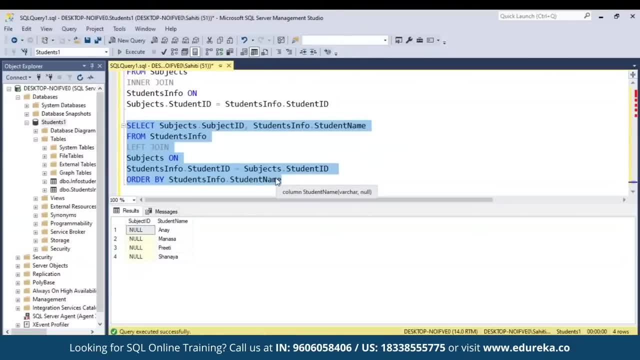 That is, the students info table and then also those records which master condition from the right table. Similarly, if I apply the right joint over here, you'll see all the records from the right table and also those records which satisfy the condition from the left table. 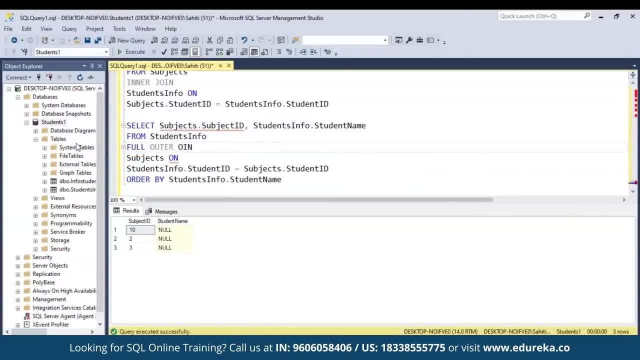 Now, finally, let's apply the final type of joints, that is, the full outer joint, And then let me just execute. and once I execute, we see that you know, we get all those records which have either a match in the left table or the right table. 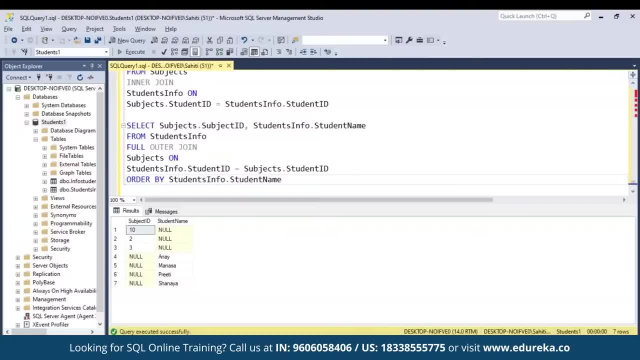 So, guys, this was, in short, about the different types of joints in sequel. Now, if you want to learn in depth more about the sequel joints, you can refer to my session on sequel joints. with that, guys, we come to an end to the joints part of this particular session. 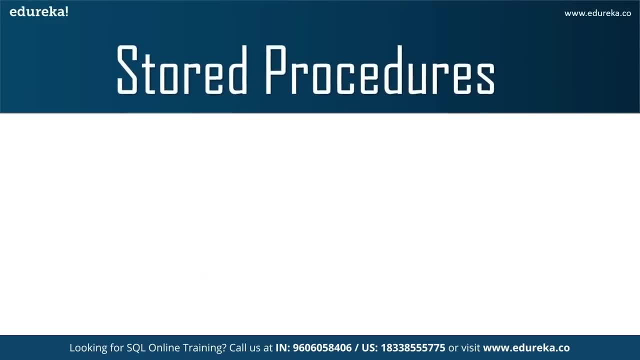 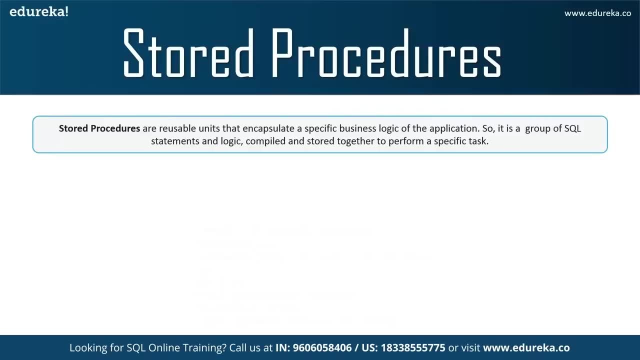 Now let's move forward to the stored procedures. I am sure that you know, you might have an understanding of what stored procedures are. stored procedures are those reusable units that can encapsulate a specific business logic of the application. So it is a group of SQL statements. 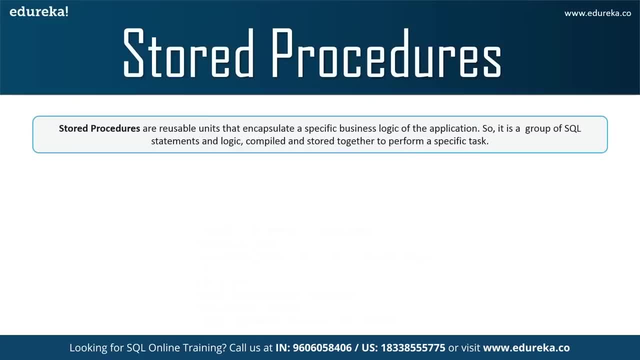 and logic compiled and stored together to perform a specific task. the syntax of stored procedures is, as you can see on my screen, right, So you just have to mention create or replace a procedure and then you mentioned the procedure name and after that you'll mention the parameters name. 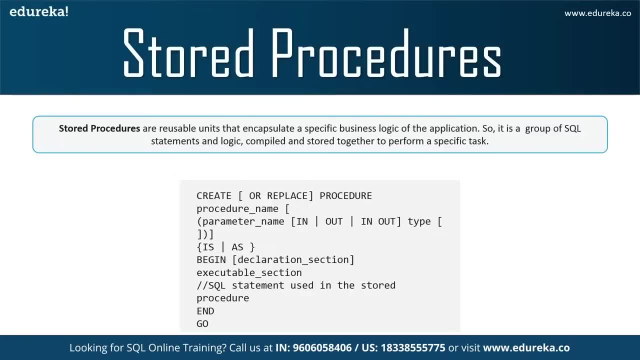 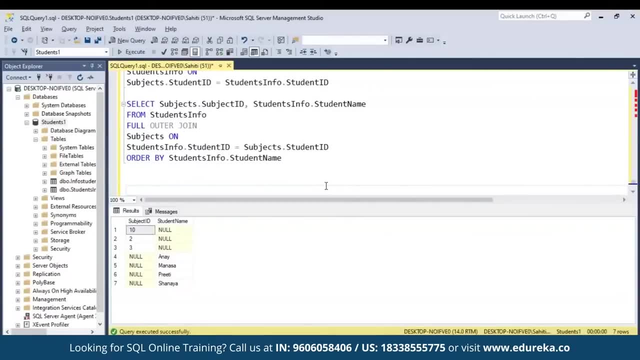 and then you'll use the aliases is or as, and then you say begin, right. and when you say begin, you declare the section and then, finally, you end the procedure. So demonstrate this. Let me just create a procedure for you. So let's say we create procedure. 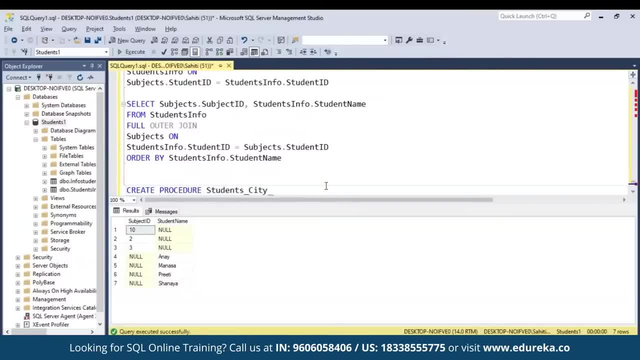 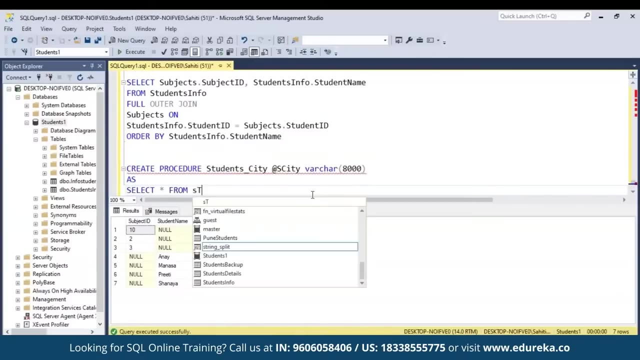 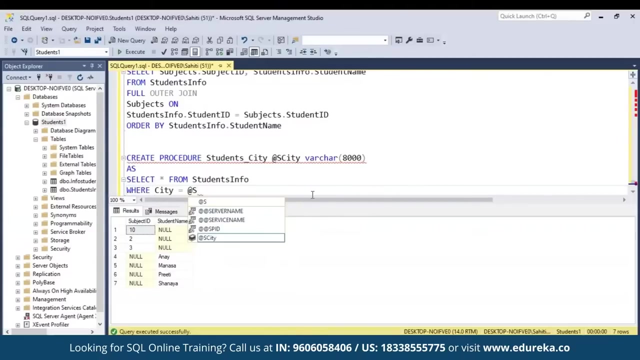 Let's say students City right, and then we choose the parameter name, The name to be a city, and let's say to be of varchar type, a thousand right, and after that we choose as, and then we select from students info And then we can mention where city equal to add the rate. 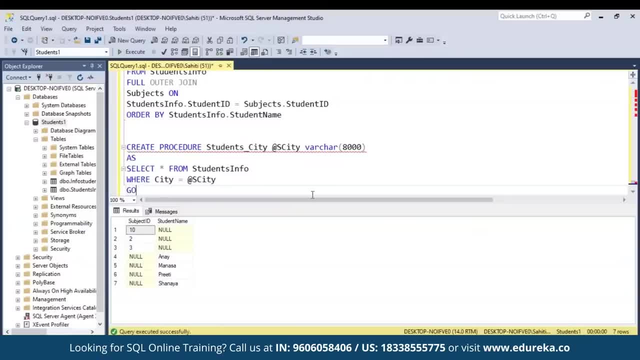 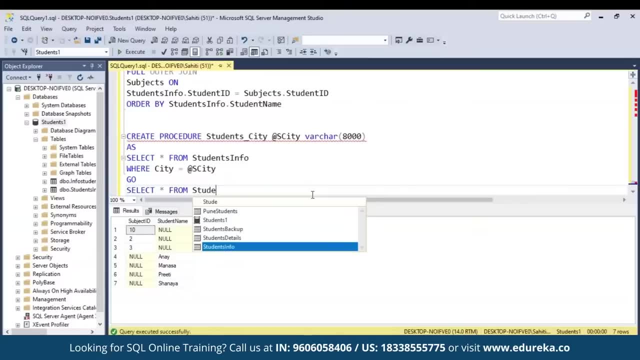 and then we mention it to add rate as a city. Then we create go and after that we mentioned select star from students info again. Now, once it is created, what you can do is you can just execute the statement simultaneously also. So for that you'll just use in the command execute right. 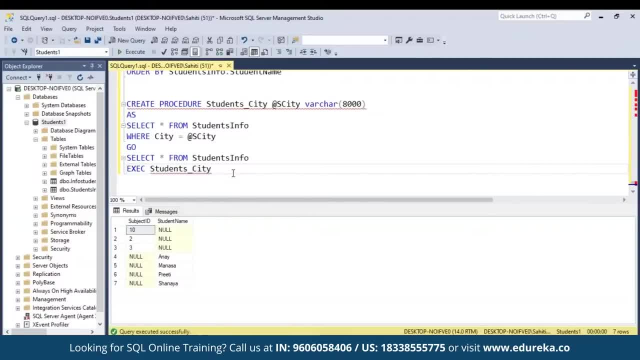 to execute students, City, right, and then you'll mention at the rate as City, because that is the type of the variable that you've created, and let's say it to be of Hyderabad, right, and then you'll click on execute. So once you click on execute, you can see that you know. 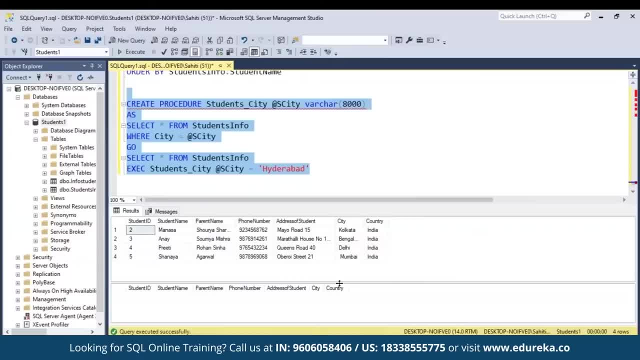 you select all the students from the students info and you see that you know there's no student from Hyderabad, example. So if you mentioned Kolkata over here, right, so I'll just mention Kolkata, right, and then if I execute it again, you can see that you know. 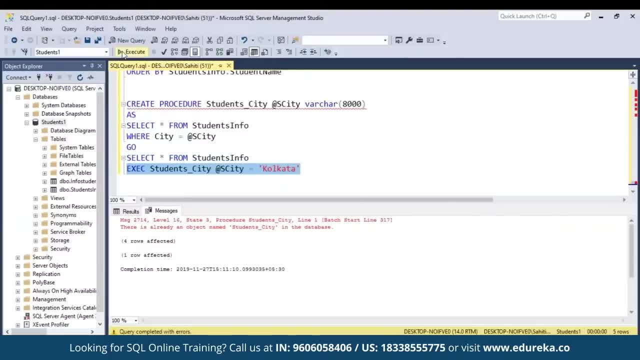 we get an error that you know there's already an object named student City, So I'll just execute this particular section and we see that we get only those tuples whose City has Kolkata value. So that's how, guys who you can use stored procedures. 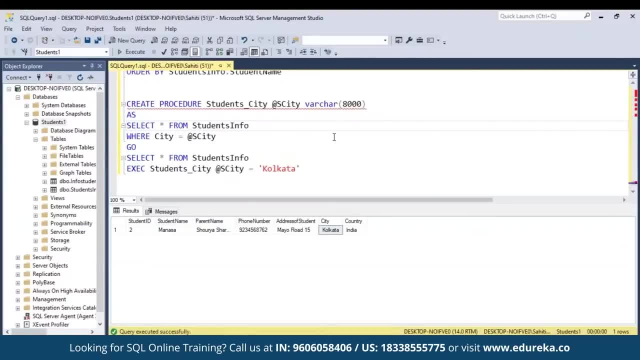 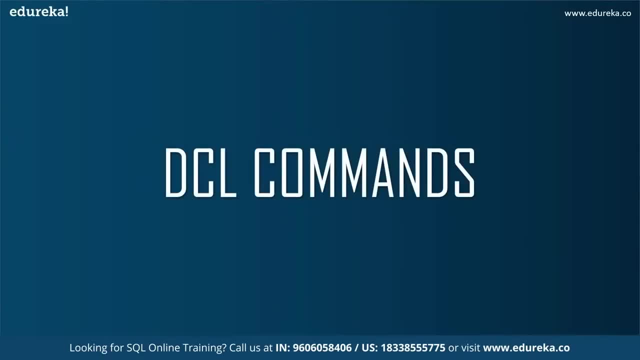 You just write the code once and then you can keep using it again and again, like any other programming languages. So, guys, that was about the stored procedures, and with this we come to an end to the DML commands. Now let's move forward with the next. 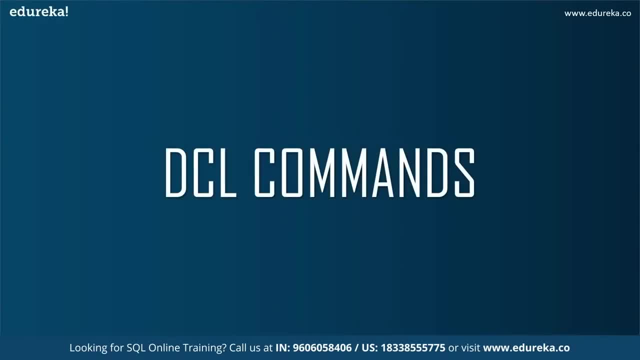 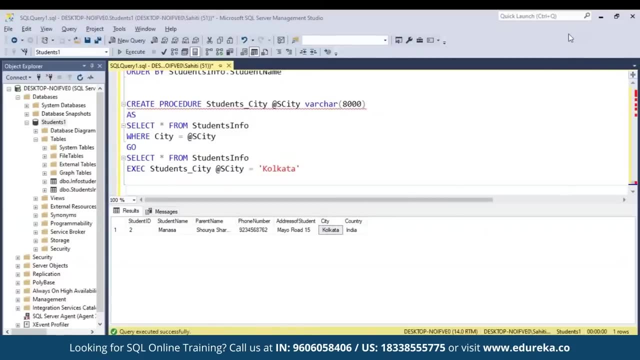 Section of commands, that is, the DCL commands. So, as I mentioned before, the DCL commands are used to grant or revoke privileges to a user. So, for example, let's say you want to create a user, so to create a user, what you can do is you can just mention create login sample. 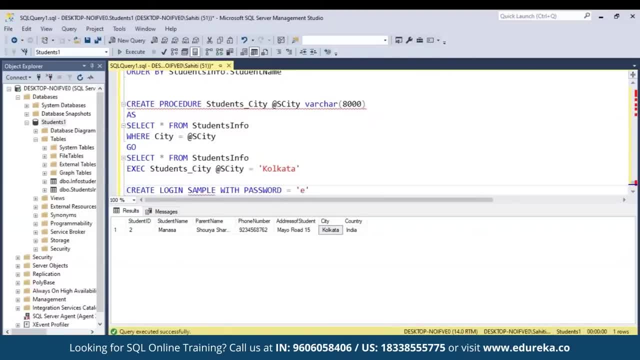 with. we mentioned the password to be edureka. So this will basically create a user, So I'll just execute the statement. Okay, it says that you know the sample user already exists. I'll just mention it as the sample one right, and then I'll click on execute. 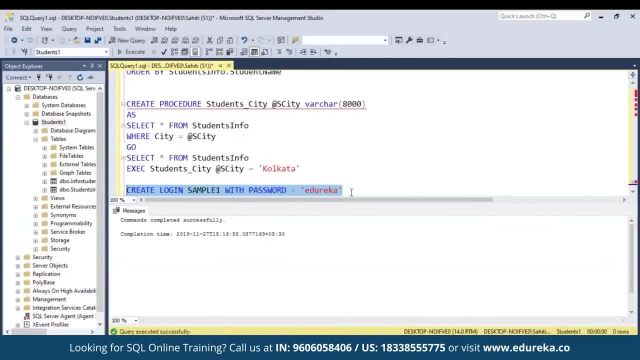 and once I click on execute, you can see that you know my user who's with the name, sample one and password. edureka has been created. Now what you can do is you can just use this user to perform various actions, rather than only using the admin login. 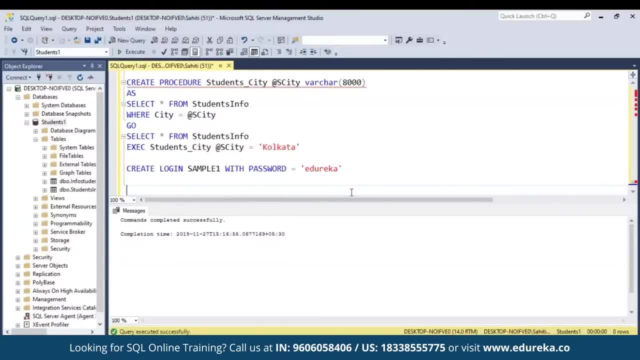 So this is how you can create a login, sample one, with the password edureka. now to create a user. What you'll mention is: you'll mention create, and then you'll mention user edureka Right and for login, and then you'll mention sample one. 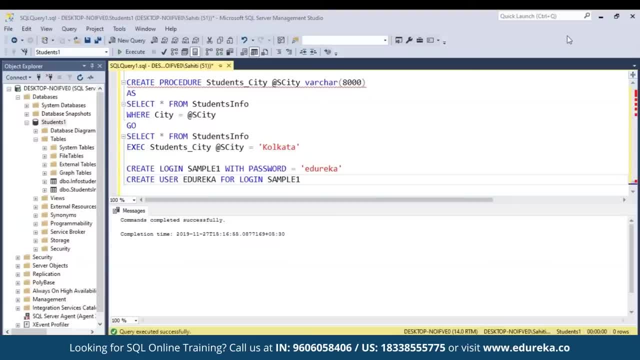 So to create a user, what you initially have to do is you have to create a login for that particular user, and then you go forward and create a user, right? So I've created a login and then I'll just create this user. So I'll execute this. 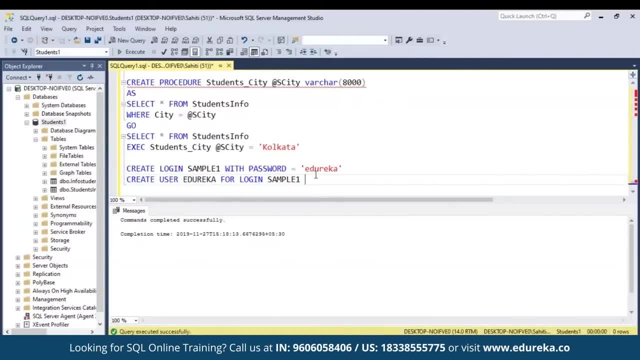 and now this particular user can be used rather than just using the admin login credentials. Now, what you can do is now you can grant and revoke any kind of privileges to a specific user. Now, for example, let's say you want to grant few privileges. 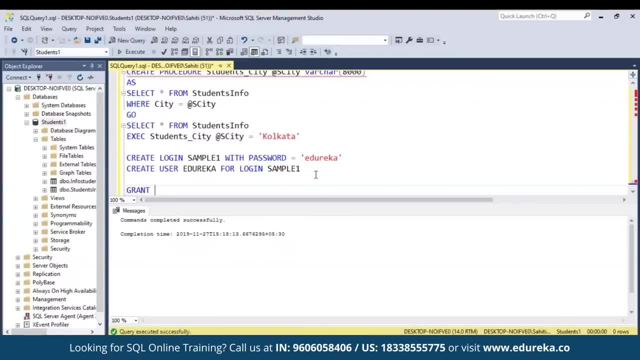 for this user, edureka, right. So for that you will type in grant, Select on, and then you'll mention the table name, Let's say students info, right? and then what I'll do is I'll mention two and then I'll mention the username, that is, edureka. 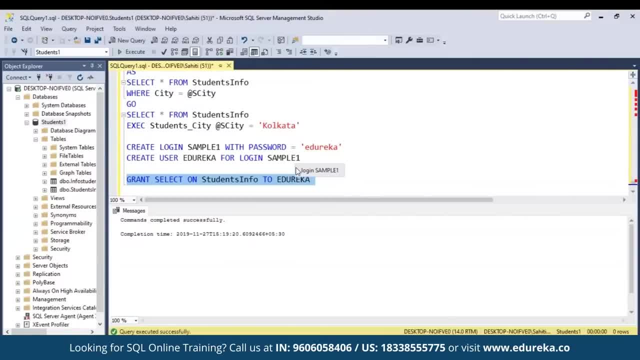 So I'm just granting this privileges to this particular user now. Similarly, I can also revoke back the granted privileges. So I'll just go back and choose revoke- So I just mentioned the work over here, and then I can just go back and execute, right. 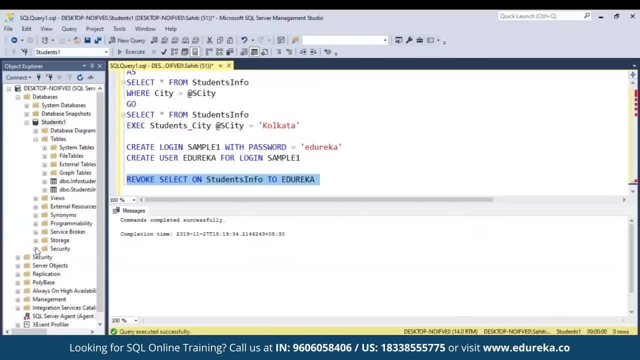 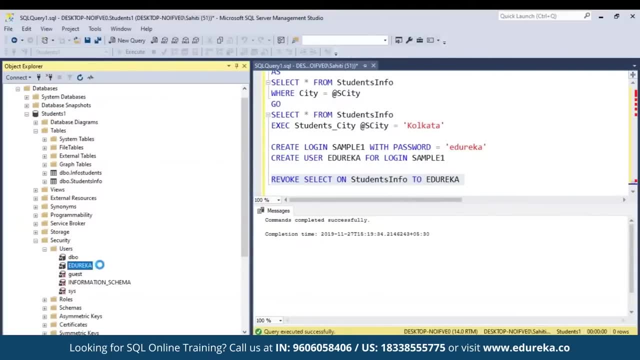 So once I execute, you can see that you know no privileges are there. also, if you want to check, you can go to security, You can go to users over here on the left hand side and then you can choose edureka. and then, once you choose edureka, 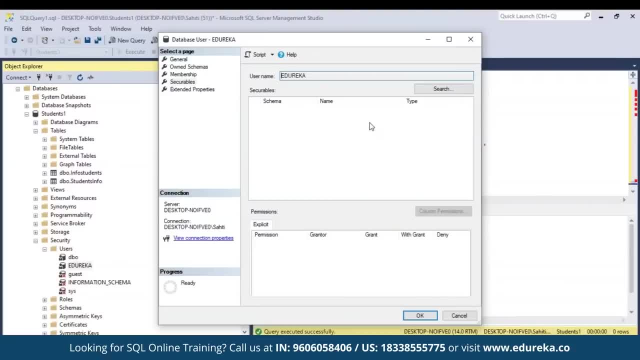 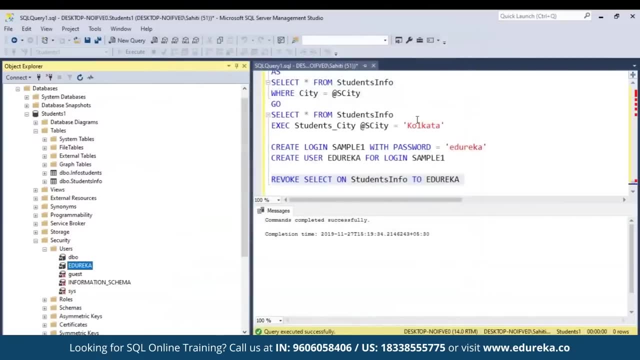 when you double click on that particular user, you can see all kinds of permissions granted to this particular user. So since none are granted, you can't see anything presently. But yes, if you grant some, then you can definitely see over here. So, guys, that was about the DCL commands. 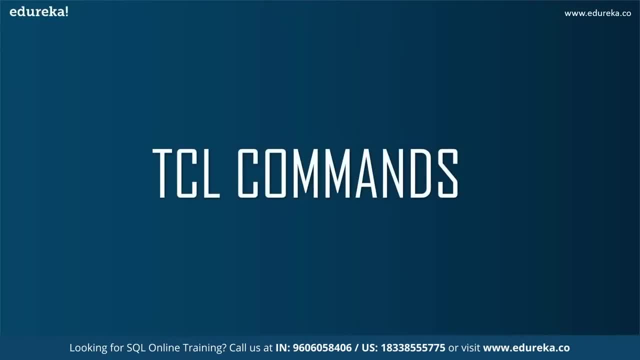 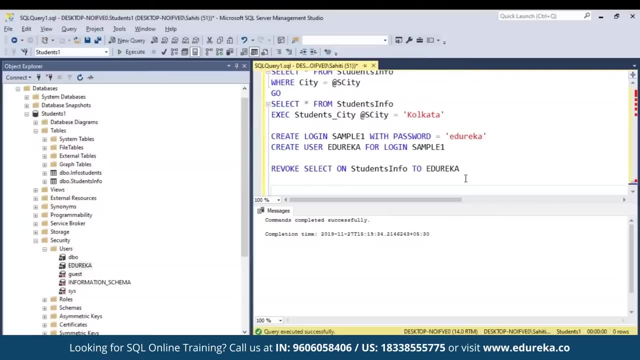 Now let's move forward with the next section for today's session, That is, the TCL commands, or the transaction control language commands. Well, these commands are used to handle the transactions in your database. to demonstrate this, what I'll do is I'll just create a table. 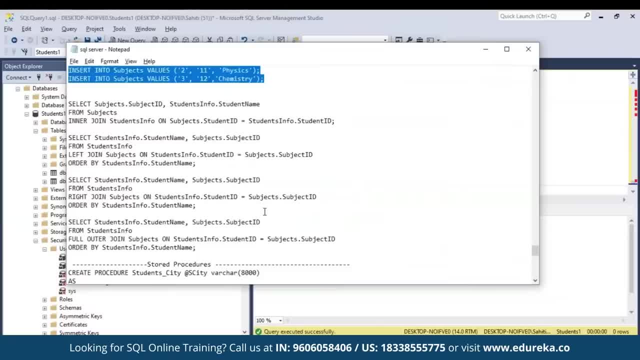 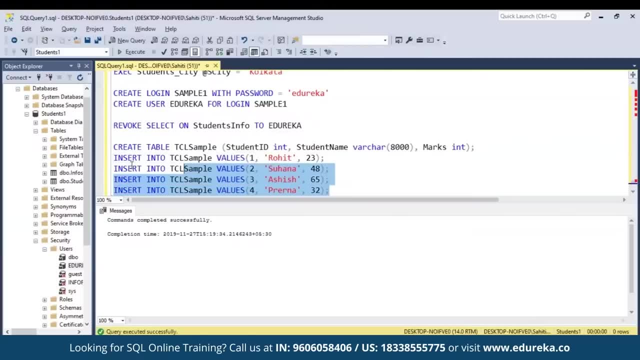 So I'll just create a table and insert few values. So let me just copy paste the same. I've just created a table as TCL sample with the student ID, student name and marks columns, and then these are the values which will be inserted, right? 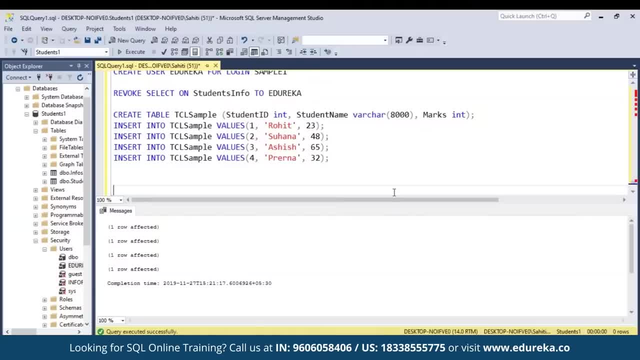 So I'll just click on execute now, Once these values are inserted. now let's just start a transaction. right? So to start a transaction, what I'll do is, I just mentioned begin, try. So that's a try-catch block which I'll come to later in the session. 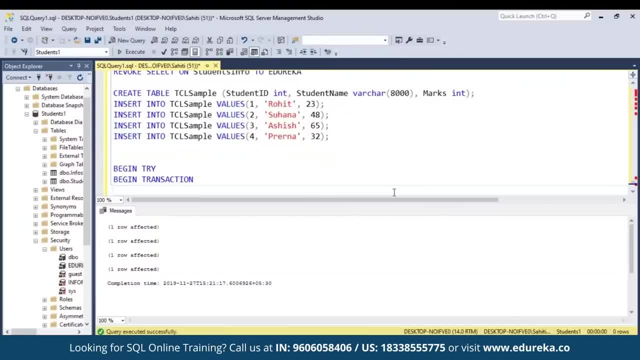 So don't worry. after that I'll mention begin transaction right and then I'll mention insert into TCL sample- That's a table name. and then I'll mention values, and let's say we mentioned few values, Let's say five, and then I mentioned the name. 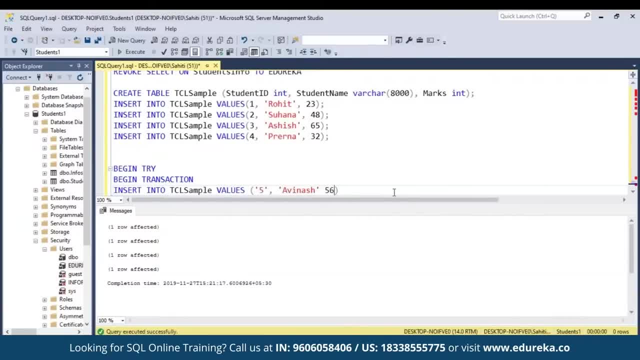 and let's say we've mentioned other values, right? So I'll just mention 56. this need not be in code, So I'll just remove that, right, and after that what I'll do is I'll just mention update TCL sample. That's a table name. 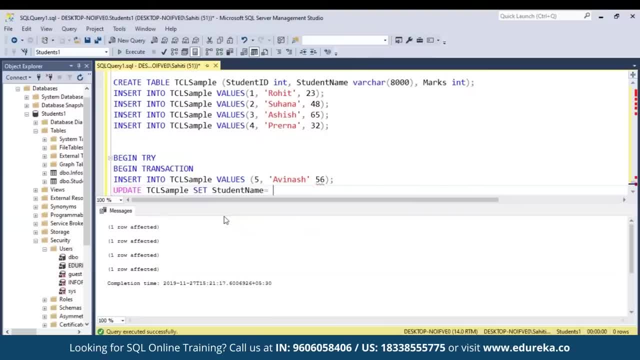 and then animation. set student name equal to. let's say, we mentioned the student name to be Akash, where our student ID is five. Also, you want to update our TCL sample table again and set our marks equal to 67, where our student ID is five. 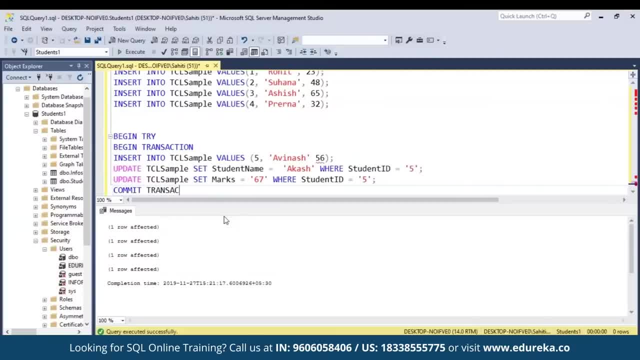 Right after that we want to come at this transaction and then print that transaction completed, right. So I'll just promote a print on the screen and then I'll end my try block right and begin my catch block. now, and over here I'll mention rollback transaction. 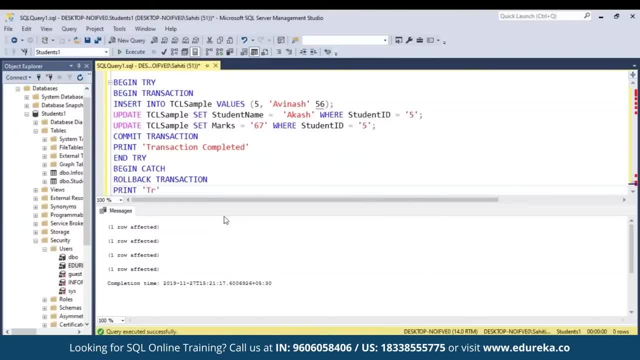 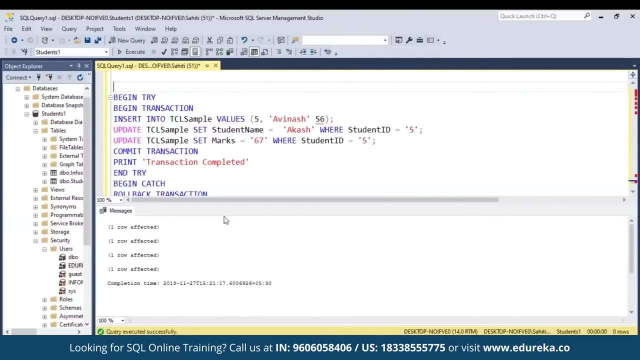 and over here I'll mention again print transaction Unsuccessful and rolled back. after that I'll end my catch block. So if you observe over here, what I've done is I've just started my try catch block and then I've pick in my transaction after that. 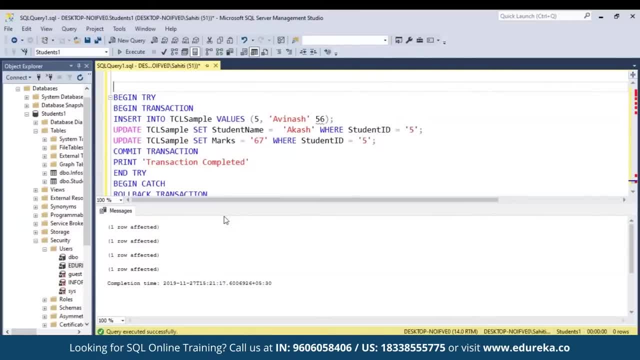 I've inserted a value into the table now. after that, I want to value to be updated, right? So I want to set the student name to be Akash, with the student ID is five, and this marks to be 67 with the student ID is five after that. 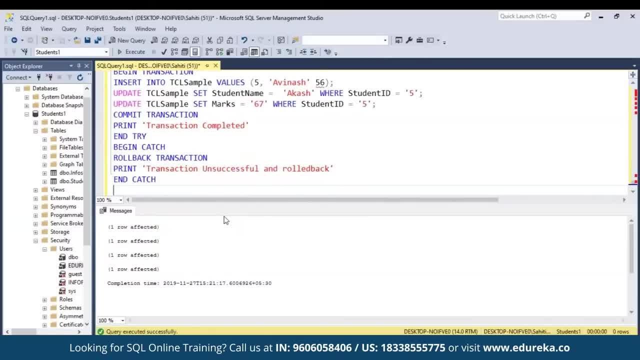 I want to commit the transaction and print transaction completed and then only if there is no error, the try block will end. But if there's any error found or any exception found in the catch block will be executed, where it will print transaction and successful and rollback. 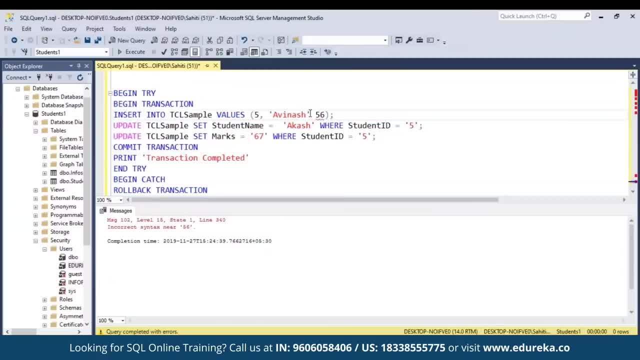 So what I'll do is I'll just execute the statement. Okay, I'm sorry, I missed a comma over here. right And now let me just re-execute the statement again, And once I execute the statement, you see an output that you know: transaction completed. 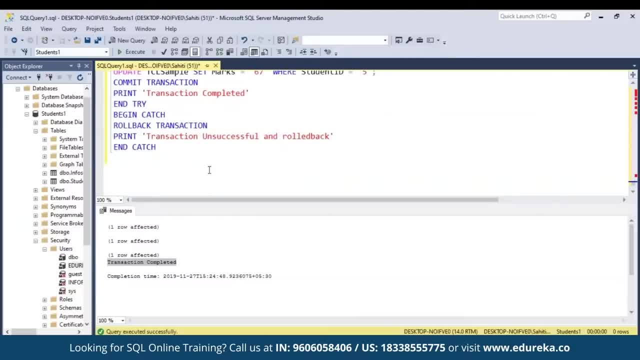 That means that you know we have inserted this value into the table and then we have also updated the values, right? So I'll just show you that. so let me just type in select star from TCL, sample right. So when I execute you can see that you know. 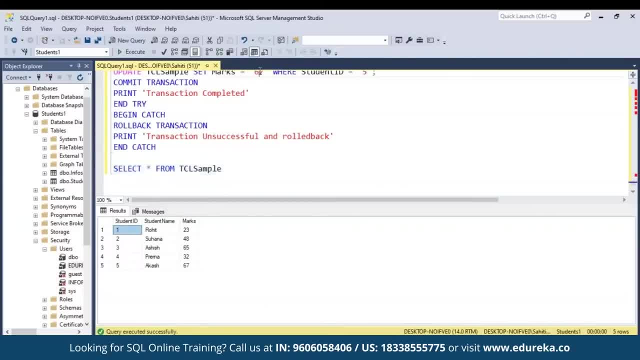 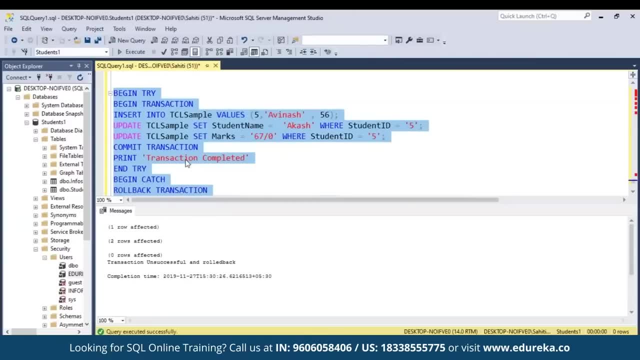 we have our fifth student with the name Akash and the marks to be 67. Now let's say you know you set the marks to 67 by 0 and then let's just execute the section again. Now, once I execute the section again, 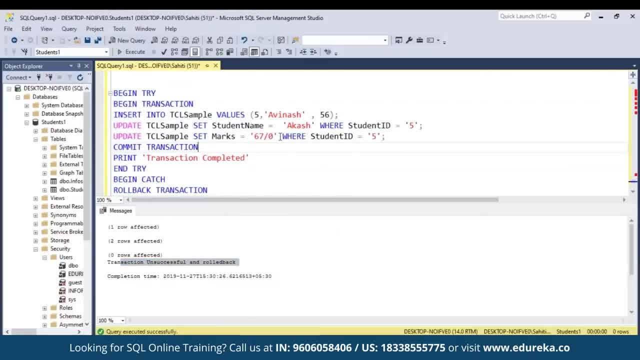 you clearly see an output that you know: transaction unsuccessful and rollback. that is because you know we cannot set our marks as 67 by 0, as we have, given that you know marks column is an int column and then an int column cannot have this particular kind. 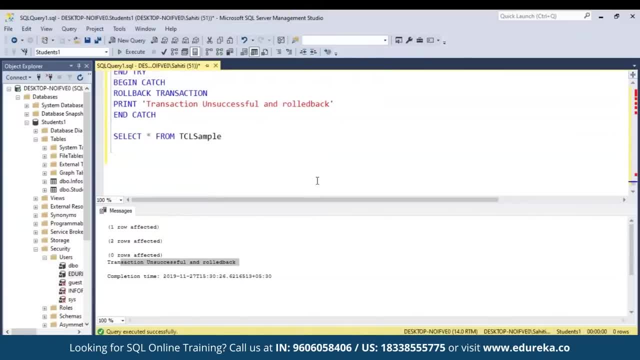 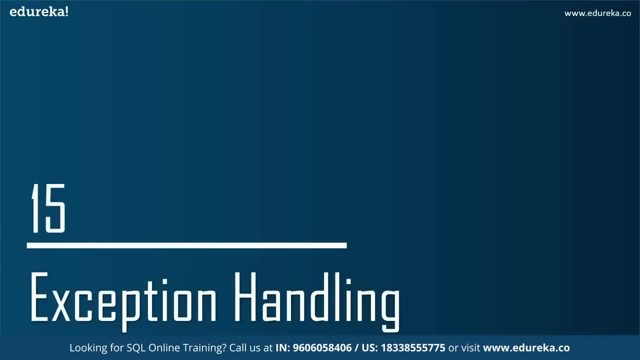 of value. So that's how, guys, the transaction control language commands works right. with this we come to an end to the different sequel command categories that you need to understand about. now let's move forward with the final topic for today's session, That is, exception handling. 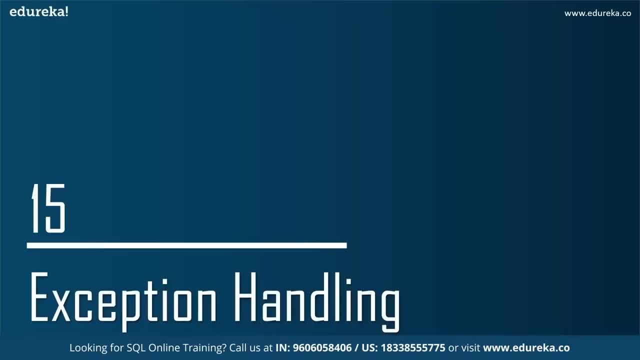 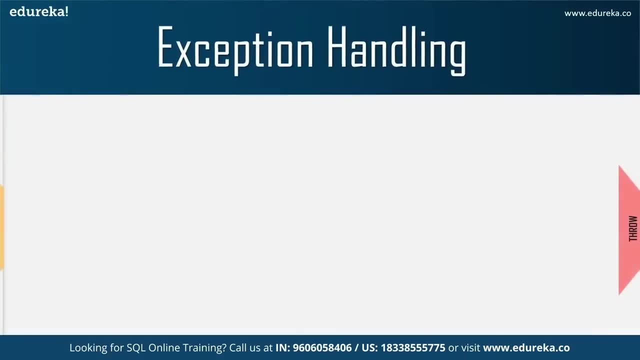 Well, exception handling in sequel server is almost similar to that of the other programming languages. It's the same as you handle exceptions in all the other programming languages. You have a true blog and then you also have a try-catch block. So talking about the true block first, 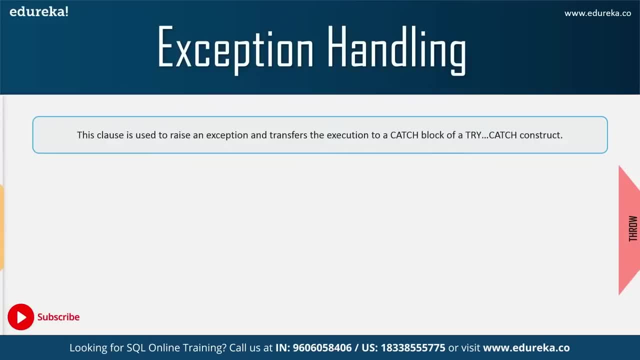 or I would say the true clause. this clause is used to raise an exception that transfers the execution to a catch block of the try-and-catch construct. If you want to see the syntax, the syntax is as you can see on my screen. you mentioned throw. 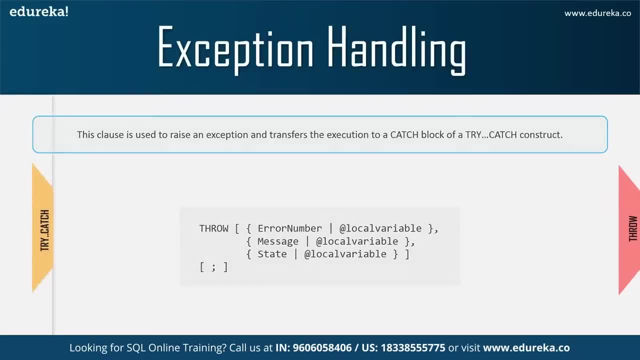 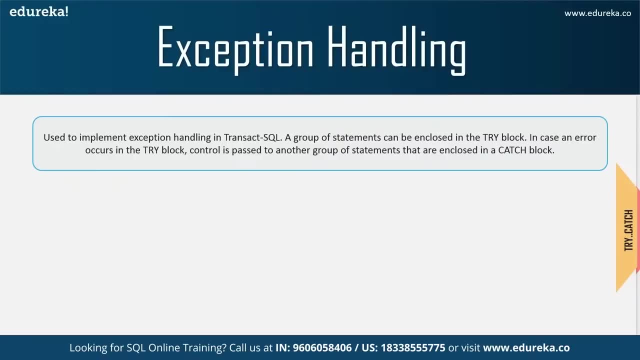 and then you mentioned the error number, and then you can mention local variable message and so on. Coming to the try-catch block, The try-catch block is used to implement exception handling in transact sequel, So a group of statements can be enclosed in a try block. 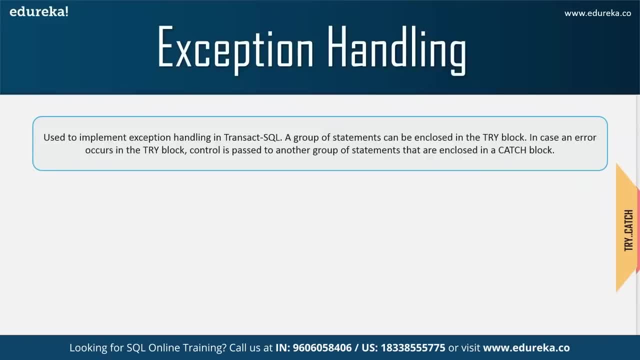 So in case an error occurs in the try block, the control is then passed to another group of statements that are enclosed in the catch block, as we just saw in the transaction control language commands. So the syntax is as you can see on my screen. it starts with begin try. 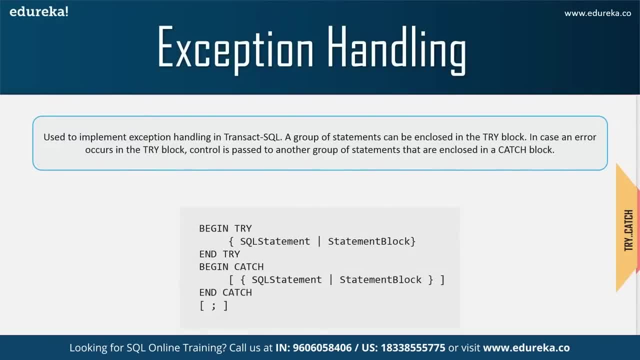 then we mentioned few sequel statements, then we mentioned and try, then we mentioned begin, catch, and then we again mention few sequel statements, and then we mentioned and catch. So that's how you can do exception handling guys. So for your understanding, let me just give you a quick example. 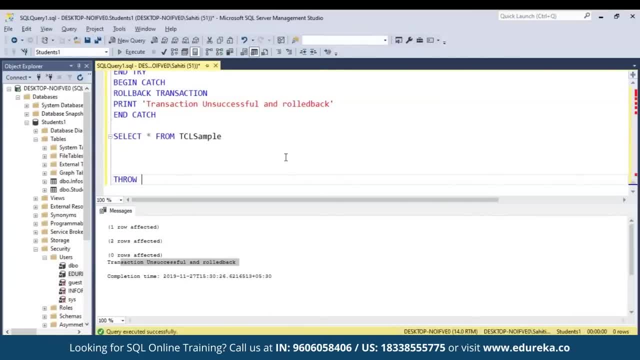 So let's say, if you want to use the throw clause, you'll mention throw. and then I said you'll mention the error number, right? So let's say I'll mention 5100 and let's say I mentioned it as record does not exist. 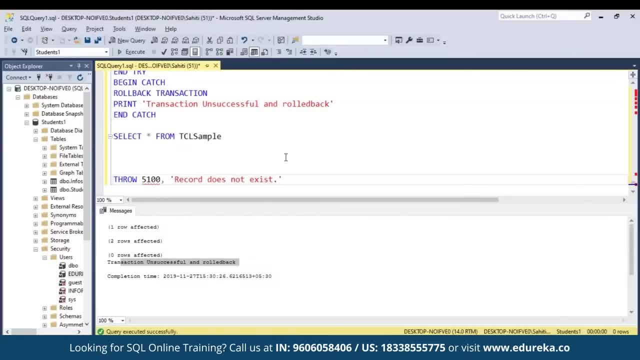 Right, and then what we can just do is we'll put a comma and then put on one, and then when I execute this particular statement, you can clearly see that you know message 51,000. and then you can see that you know state line is one. 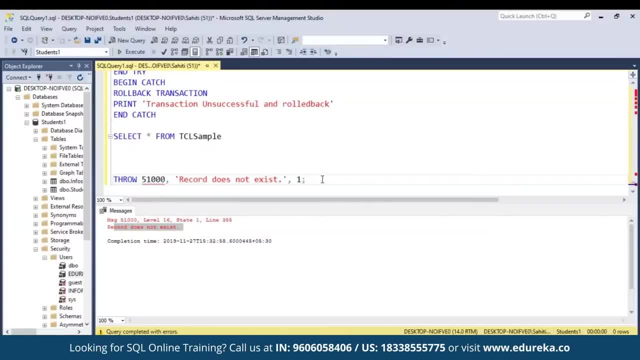 and the messages record does not exist right. So that's how you can use the flow clause now. Similarly, you can use the try and catch block, as you saw before. So for that you'll just type in begin, try, right, and let's say we select phone number. 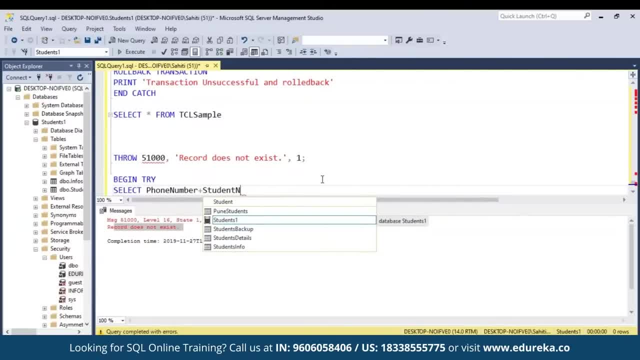 Plus student name, Right? So if you remember, our student name was of varchar type and a phone number was of begin type, right? So we cannot concatenate both of them, So I'll just mention phone number: concatenates to the name from students info. 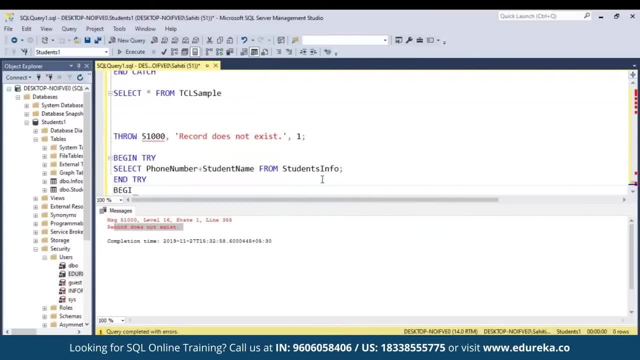 And then what I want to do is I want to do and try. then I'll begin the catch block, right, and then I'll mention print not possible, right, And let's say I'll just mention and catch right, and then we can just execute the statement. 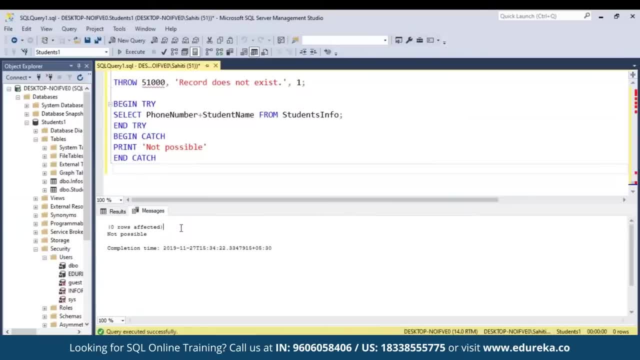 So when I execute this particular statement you see that you know no column name. but if I go to messages you can clearly see that you know. the message shows not possible, right, So that means a try block did not get executed. 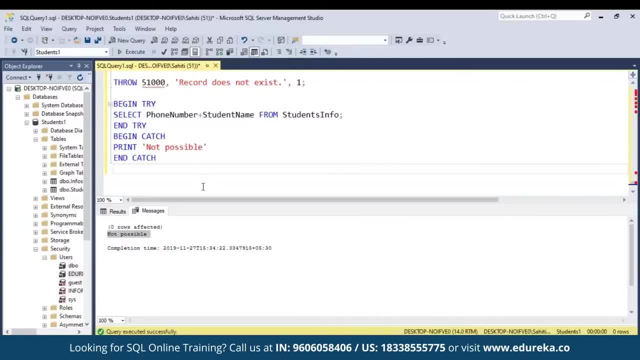 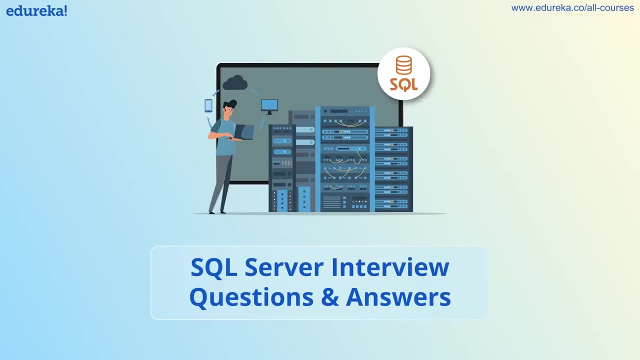 Only a catch block got executed and shows the exception of not possible. that indicates the user that you know we cannot add these two columns, So that's how you can perform exception handling in Microsoft's equal server guys. Let's look at the first question for today's session. 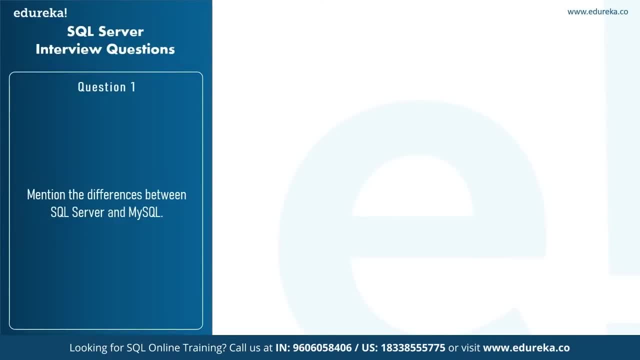 that is mentioned, the differences between sequel server and my sequel. Now, This is one of the most popular questions as, as you know, both of them are relational database management systems. So, if you have to give the differences between sequel server and my sequel, 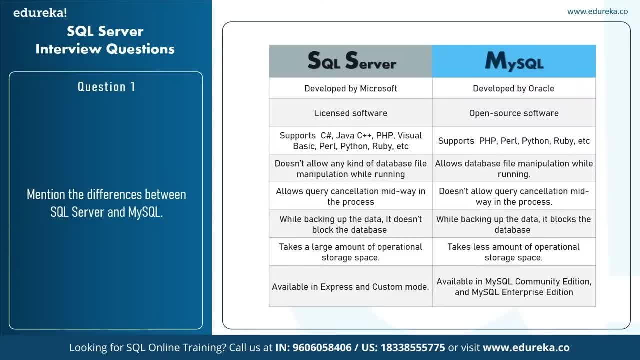 then I would say sequel server is developed by Microsoft and my sequel was developed by Oracle. sequel server is a licensed product, So you do not have the free edition for it, and my sequel is an open-source software, right? So if you want to know how to install both of them, 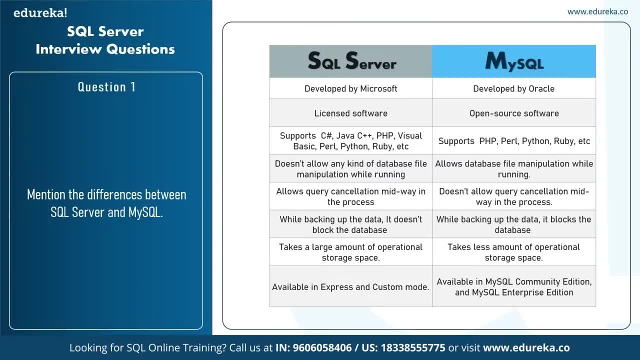 I'll leave the links in the description box below, But let me tell you over here that you know you can easily install my sequel in very few steps. But when it comes to sequel server you have to enable few ports and name pipes and then you have to follow a proper step. 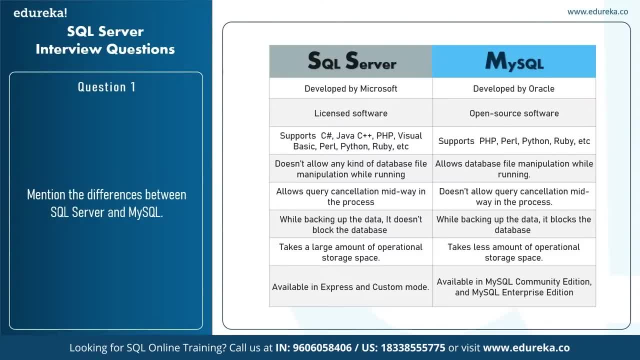 to configure the databases. So I would say, if you have to compare the installation step between both of them, then I would say installing my sequel is very easy, comparative to that of sequel server. coming to the next difference: sequel server support, See hash Java, C++, PHP, Visual Basic, Pearl, Python. 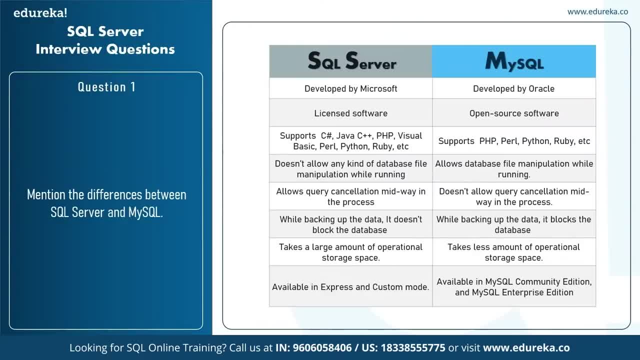 and Ruby. coming to my sequel, my sequel also supports various programming languages, like you know: PHP, Pearl, Python, Ruby and so on, right? So both of them offer quite good amount of support to build various kinds of applications using different technologies. coming to the next difference, 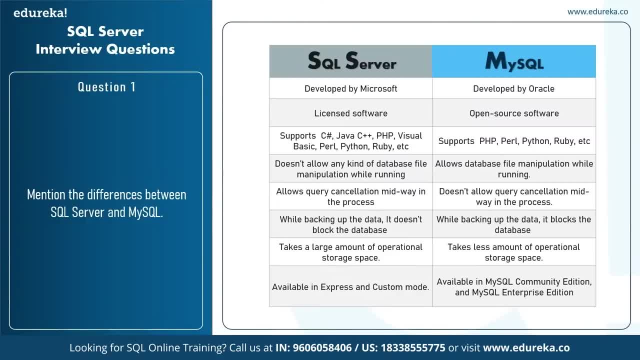 I would say sequel server doesn't allow any kind of database file manipulation while running the database, whereas my sequel allows database file manipulations while running. sequel server allows query cancellation midway in the process, but this is not the scenario in my sequel, as my sequel does not allow query cancellation midway. 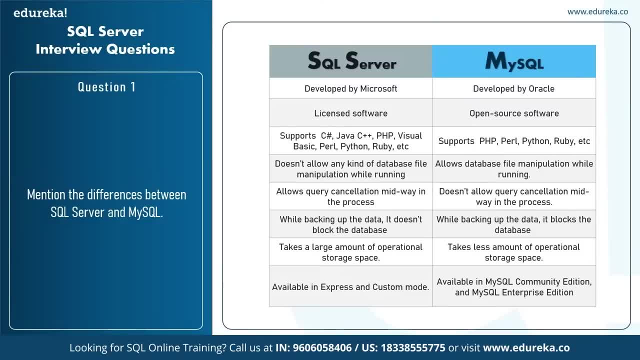 in the process. moving on to the next difference, while backing up the data, sequel server doesn't block the database, But when it comes to my sequel, it blocks the database. right, and coming to the next difference, you can see that you know, sequel server takes a large amount. 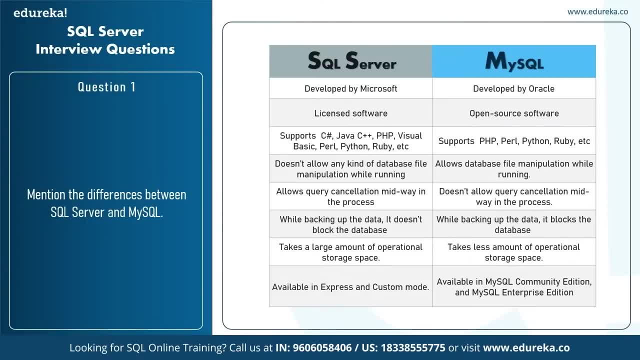 of operation storage space, Whereas that's not the scenario in my sequel, as it takes a less amount of operation storage space. coming to the last difference that you know, sequel servers available in the Express in the custom mode and my sequel is available in the my sequel Community Edition. 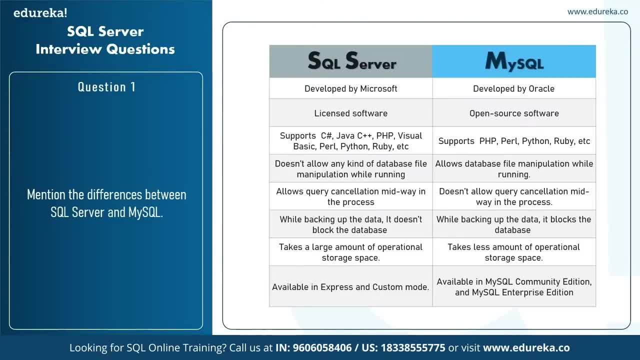 and the Enterprise Edition. So, guys, these are few differences between sequel server and my sequel. apart from that, also, you can answer the interview by talking about your personal experience while using sequel server and my sequel. right, you might have created databases in both of them and maybe you have manipulated data using both of them, right? 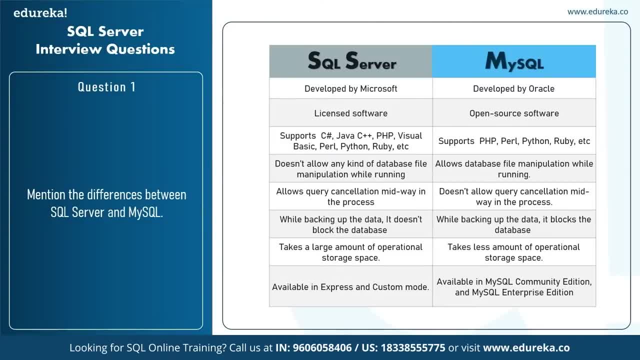 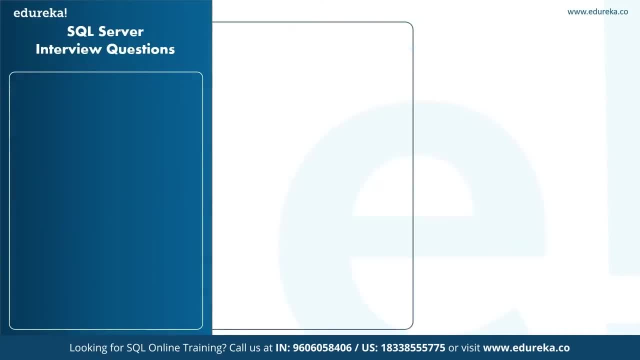 So you can talk. you know what happens when you want to do a specific set of actions in my sequel and sequel server. So with this we come to an end to the first question. Now let's move forward with the second question. 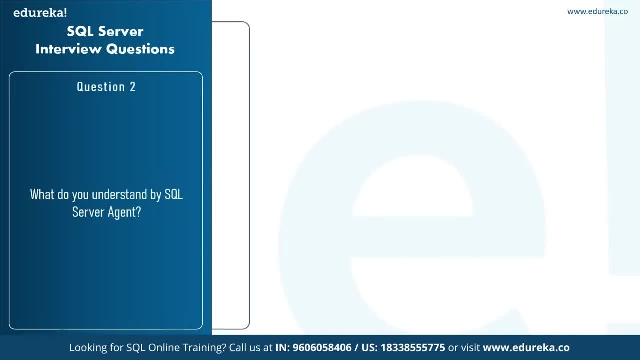 That is what do you understand by sequel server agent. Now, sequel server agent is one of the most popular component of sequel server, right? So basically, if you have to explain sequel server, then you can just say that you know. sequel server agent is a Windows service which is used to schedule. 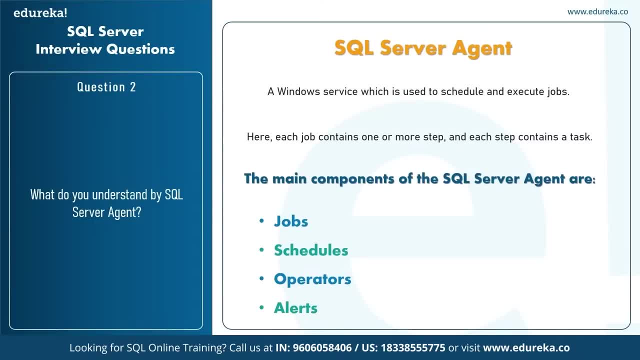 and execute the jobs. So here each job contains one or more steps, and each step can contain a task. So what happens is that the sequel server agent uses the sequel server to store the job information and run a job on a schedule. now the main components: 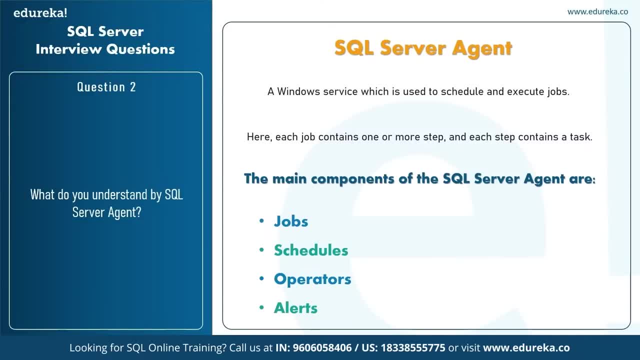 of sequel server agent are basically jobs, schedules, operators and alerts. So if you have to explain with an example over here, you can just consider the example. like you know, if an Enterprise wishes to take the backup of the company servers at 9 pm, 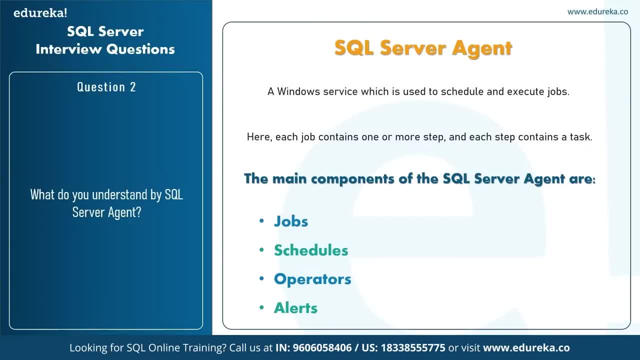 On every Friday. Now what you can do is you can just automate this task and let the task happen at the scheduled time, But in a scenario when a backup encounters and error, the sequel server agent records the events and notifies the corresponding team. So that's how you can use the sequel server agent, guys. 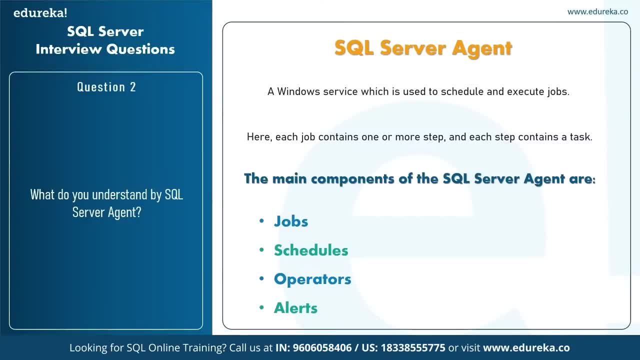 Well, this was one of the simple usage. you can do it in a very complicated way also. So I would just say that you know, sequel server agent is one of the most important concept, or you can say, the most important component that you need to understand about Microsoft sequel server. 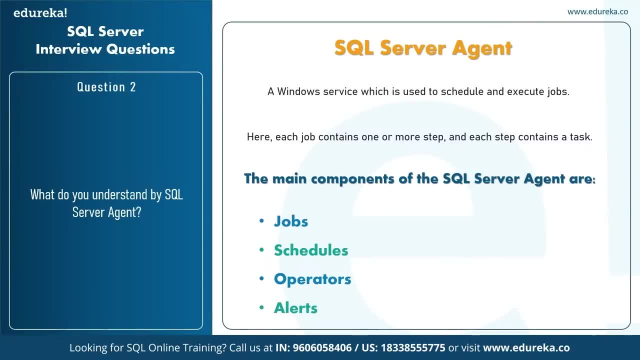 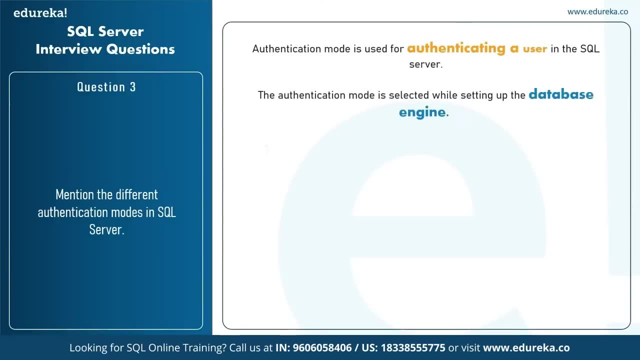 So, moving on in this tutorial on Microsoft sequel server, Let's look at the next question that is mentioned: the different authentication modes in sequel server. now, before I tell you the different authentication modes in sequel server, Let me tell you that the authentication mode is used. 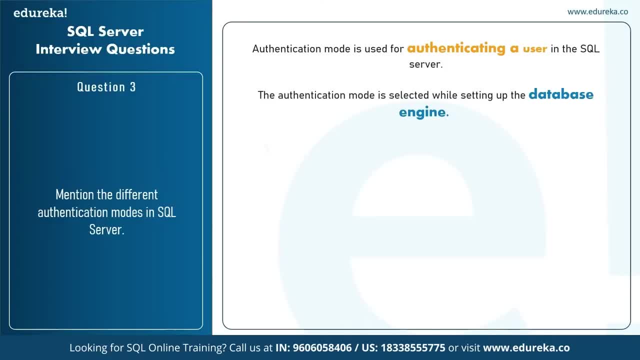 for authenticating a user in the sequel server. So the authentication mode is selected while setting up the database engine. and the different authentication modes offered by sequel server are basically the Windows authentication mode and the mixed mode. Now the Windows authentication mode is used to connect the server through a Windows account. 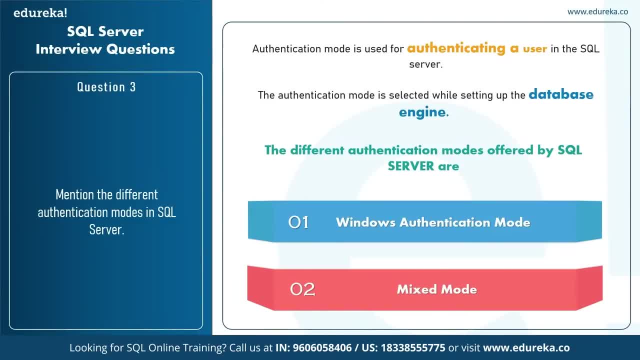 So what basically happens over here is that you know the server takes the computers username and password for authentication purposes and also the sequel server authentication mode is disabled in this mode. coming to mixed mode, The mix mode is used to connect with an instance of sequel server using either the sequel server authentication. 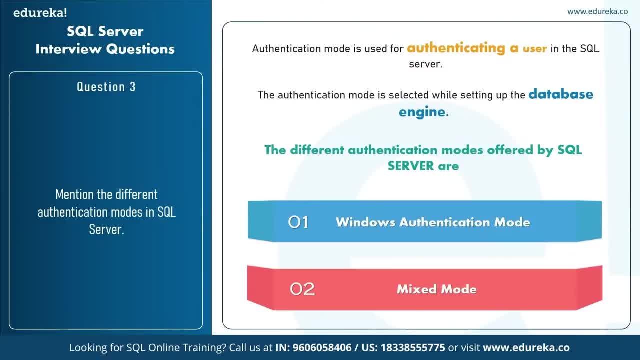 or the Windows authentication. So in this mode, basically, there's a username and the password set by the user for the database, and then when you want to log into your sequel server, you have to mention those username and passwords. So, guys, these were two authentication modes. 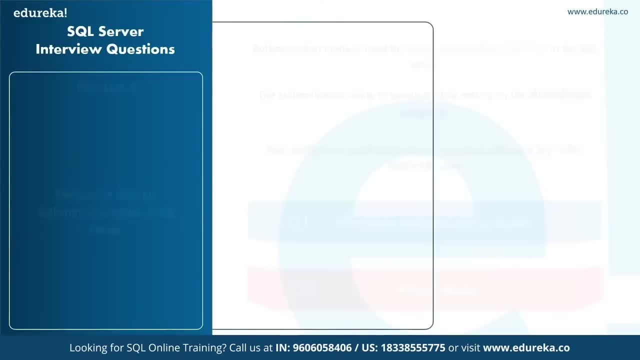 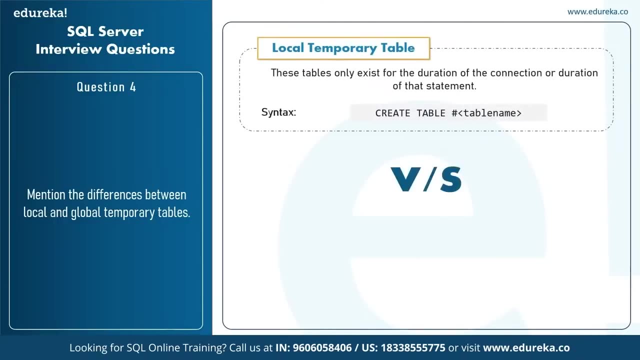 that is, the Windows mode and the mixed mode. Now let's move forward with the next question that is mentioned: the differences between local and global temporary tables. Now, the local tables are basically those tables which only exists for the duration of the connection or the duration of that particular statement. 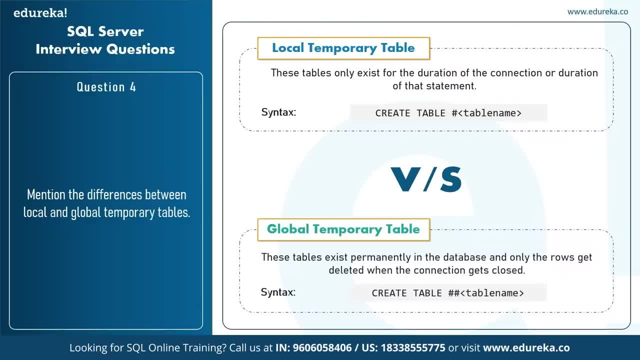 which is executing. But when it comes to global temporary tables, the global temporary tables exists permanently in the databases and only the rows get deleted when the connection gets closed, right. So over here you have to remember that. you know, the structure does not get deleted, only the rows get deleted. 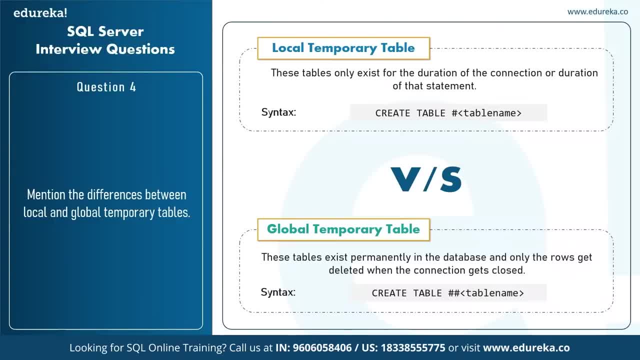 So if you have to talk about the syntax between both of them, then I would say the local temporary variable. You can write a syntax, as you know, create table and then put a hash mark and mention the table name. coming to global temporary tables, The only difference in syntax is that you know. 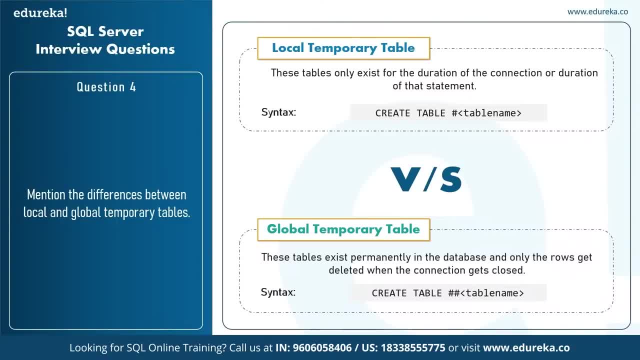 you have to mention two hashes, So you'll mention create table hash, and then again and hash, and then you'll mention the table name. So, guys, these were the differences between local temporary table and global temporary table. Now let's move forward with the next question. 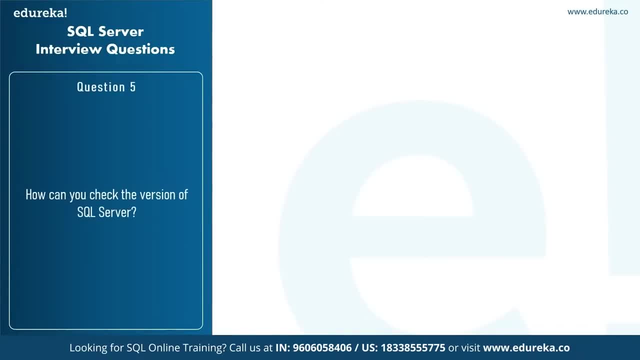 That is, how can you check the version of SQL Server? Now, I would say you could be asked this question just to check whether you have a good hand on the commands or not. So to check the version of SQL Server, you just have to mention the command. 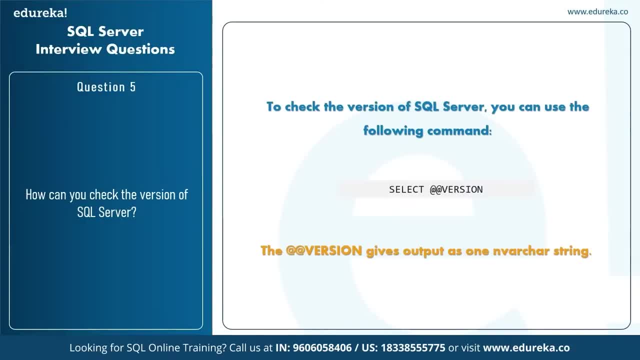 that you can see on my screen, that is, select and then add the rate at the rate version. Now this particular command will basically give you the version of the SQL Server that's installed onto your system, and this gives an output as one nvarchar string. 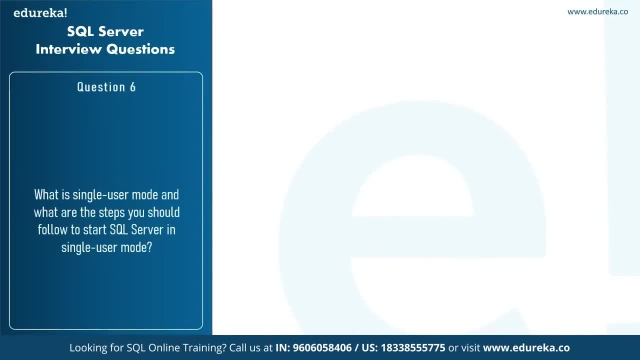 Now let's move forward with the next question, That is, what is single user mode and what are the steps you should follow to start SQL Server in a single user mode? now, as the name suggests, the single user mode, This particular mode, is basically used. 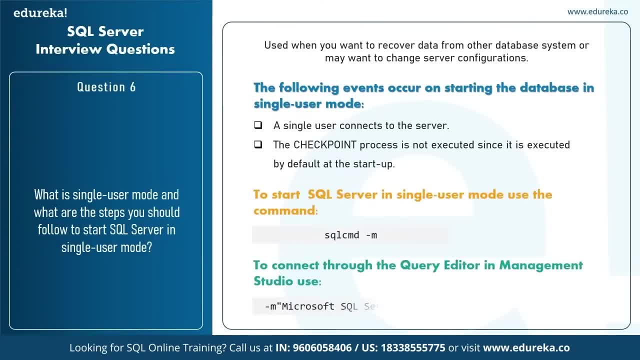 when you only want a single user to be active on your SQL Server. So single user mode is a mode where only single user connects to the server. Now you might be wondering: when do we use it? right now? Let me tell you that you know. 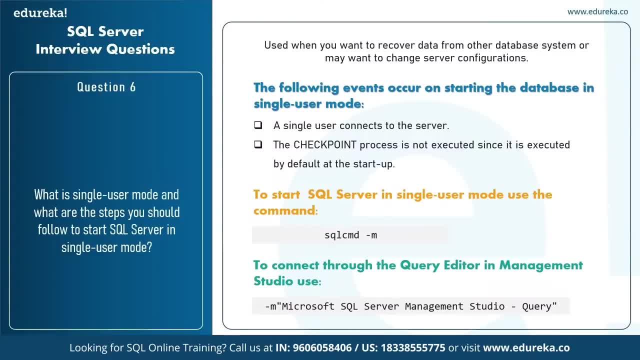 it may often happen that you would want to start an instance of a SQL Server in the single user mode and you would want to do this either when you want to recover the data from other database system, or maybe you want to change the server configurations. So basically, there are two scenarios. 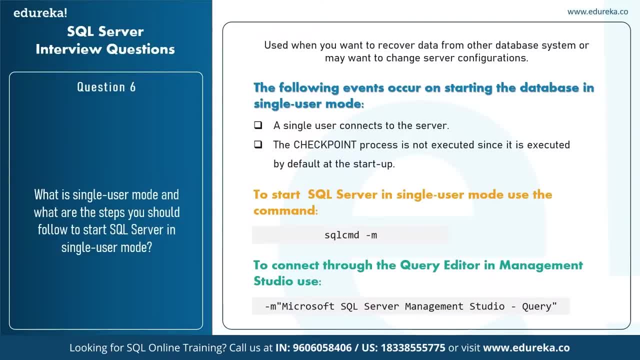 where you would want to use the single user mode. that is, either you want to recover data from the other database system or you would want to change the server configurations. So when you start the SQL Server in single user mode, then any member of the computers 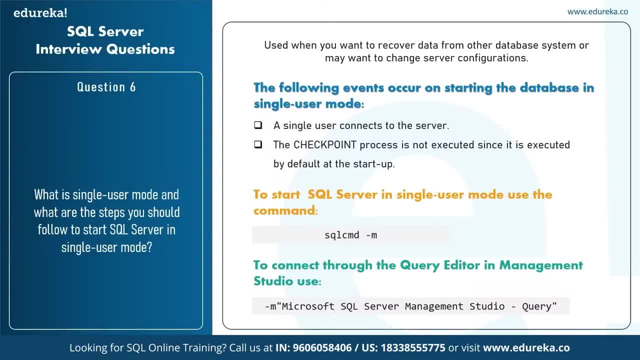 local administrators group gets connected to the instance of SQL Server as the system admin. Now, once you start the SQL Server in a single user mode, what happens is that you know a single user connects to the server and the checkpoint process is not executed, since it is executed by default at the starter. also know 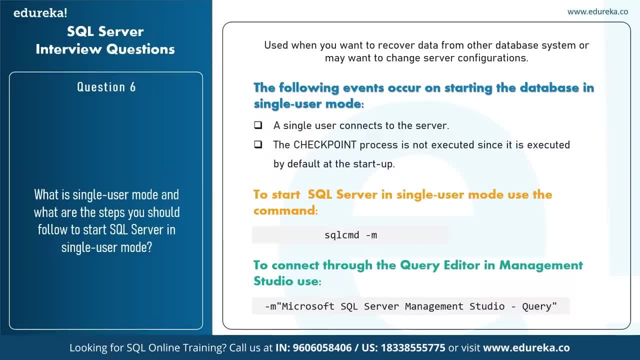 that you know you have to stop the SQL Server agent service before connecting to an instance of the SQL Server in the single user mode. Now, this is a little bit of an extra information that you can give to an interviewer, but I would say it would be nice. 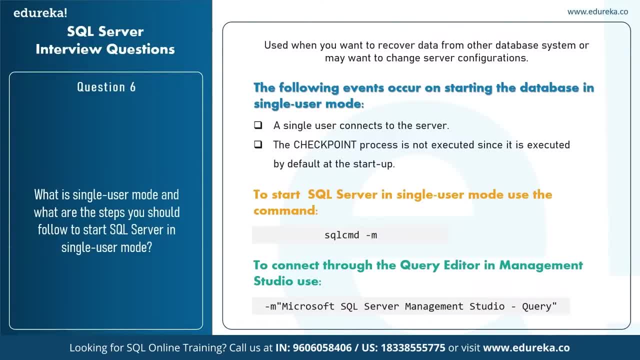 if you answer like that, now to start the SQL Server in single user mode You basically have to use the command of SQL command, hyphen M, right? So you just type in SQL CMD, hyphen M, and then you can start the SQL Server in the single user mode. 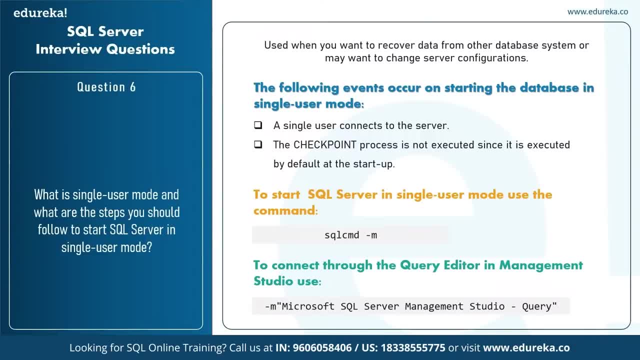 now to connect to a query editor in the management studio use. you can just mention hyphen M and then you can mention the Microsoft SQL Server management studio query. that query is completely on your basis, that how you want to connect. but these are the two ways to which you can start the SQL Server. 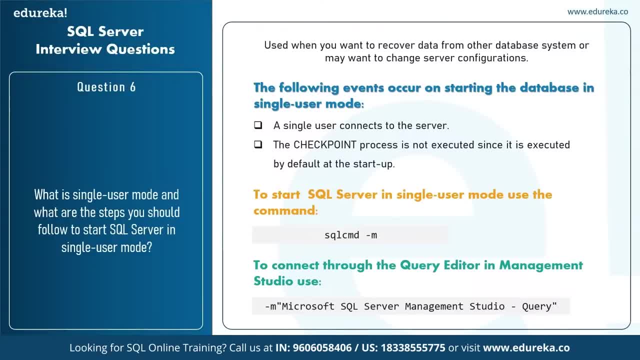 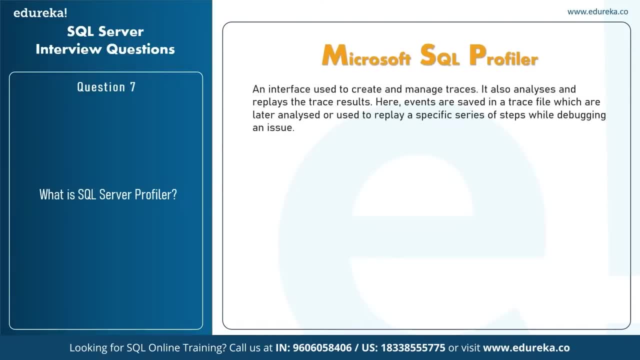 We're in a single user mode. So, guys, that was about this question. Now let's move forward with the next question, That is, what is the SQL Server profiler? The Microsoft SQL Server profiler is an interface used to create and manage traces. 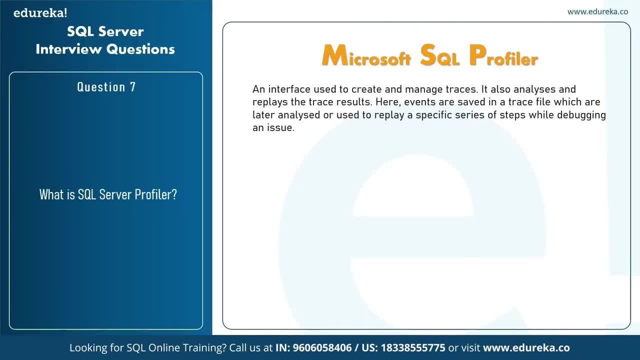 So basically what it does is that you know it analyzes and replace the trace results. So here the events are saved in a trace file which are later analyzed or are used to replay a specific series of steps while debugging an issue. Now you can use the SQL Server profiler for activities. 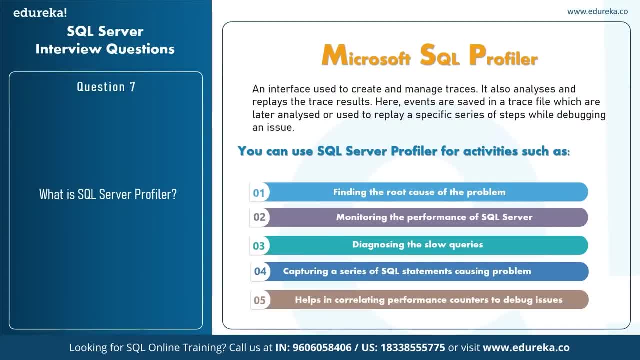 as you can see on my screen. like you know, finding the root cause of the problem, monitoring the performance of SQL Server to handle workloads, diagnosing the slow queries capturing the series of SQL statements causing a problem. to further replicate the problem on the test server. 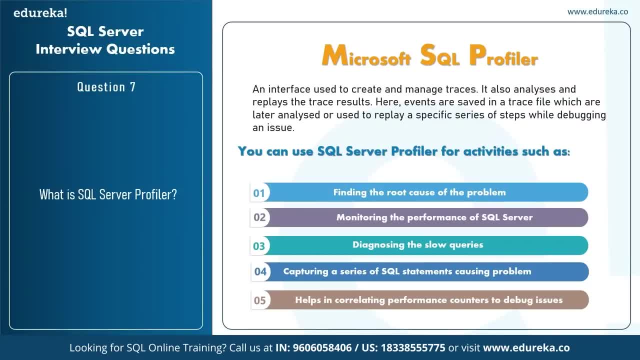 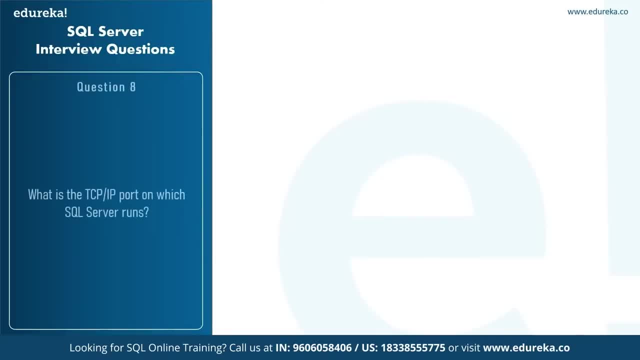 while debugging the issue and also correlate the performance counters to debug the issues easily. So, guys, this was about SQL Server profiler. Now let's move forward with the next question, That is, what is a TCP IP port on which SQL Server runs? Now, this is one of the most interesting question. 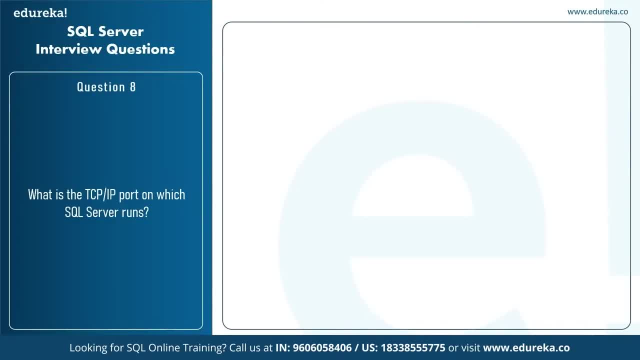 that is asked in interviews, because you know it's a number that you have to guess exactly and then your answer cannot be wrong, right? So well, the answer to this particular question is that you know the TCP IP port on with SQL Server runs is 1433, right. 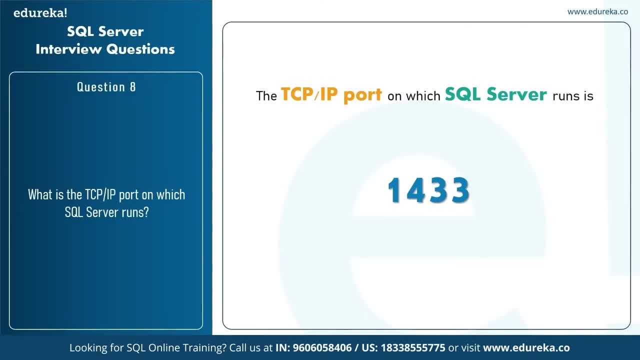 So that's 1433 that you have to keep in your minds. Now let's move forward with the next question, That is, what are sub queries in SQL Server? and then can you mention few properties of it? So if I have to explain you what a sub query is, a sub query? 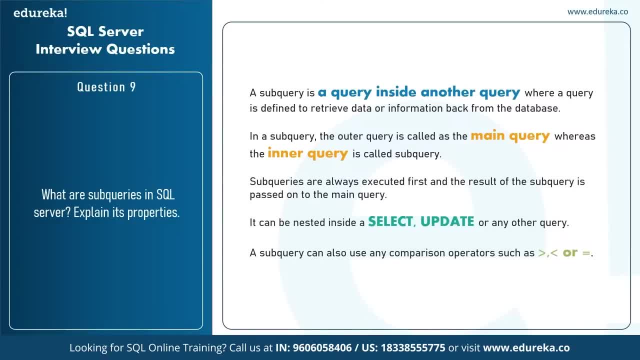 is a query inside another query where a query is defined to retrieve data or information back from the database. So in a sub query the outer query is called the main query whereas the inner query is called the sub query. sub queries are always executed first and the result of the sub query is passed to the main query. 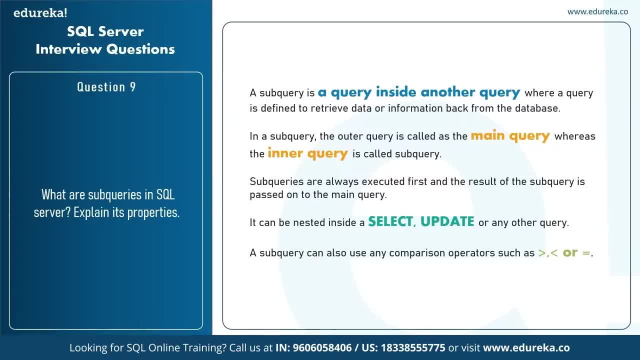 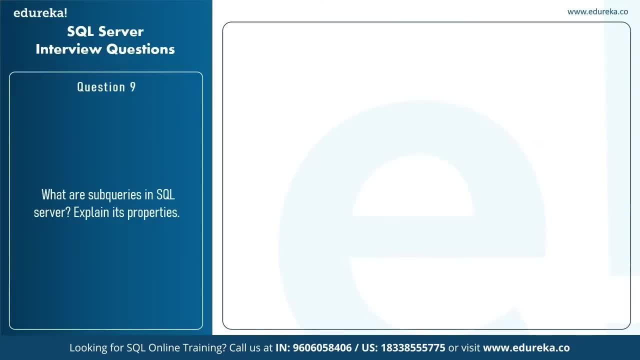 Now sub queries can be nested inside a select statement, update statement or any other query. a sub query can also use comparison operators, like you know: greater than, less than or equal to now. if you have to mention few properties of sub queries, then you can say that you know. 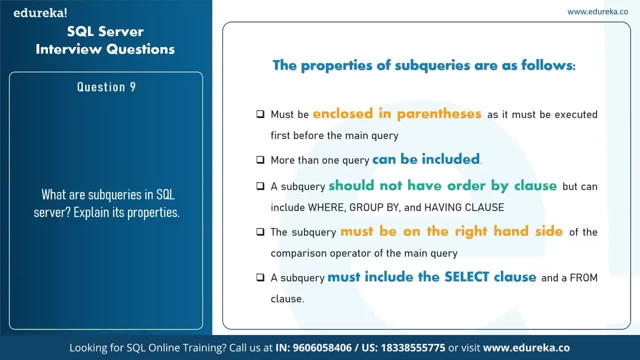 it must be enclosed in parentheses as it must be executed first before the main query. more than one query can be included and a sub query should not have the order by clause but can definitely include the where group by and the having clauses. the sub query must be. 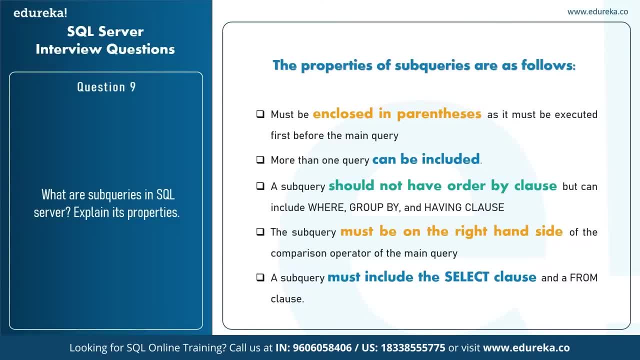 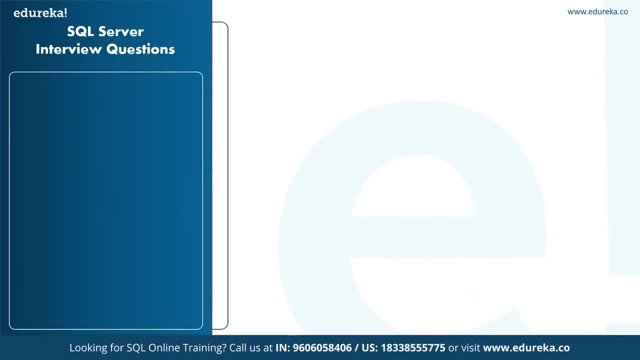 on the right hand side of the comparison operator of the main query and must include a select clause and a from clause. So, guys, these are a few properties of sub queries. Now let's move forward with the next question, That is, how do you start single user mode? 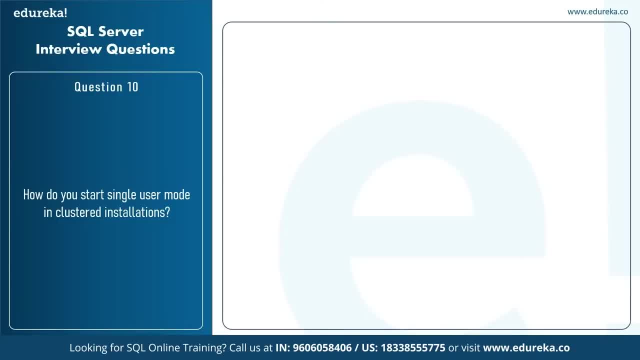 in clustered installations- now in clustered installations to SQL Server basically uses the DLL available connections and thus blocks any other connection to the server. now in this state, if you try to bring the SQL Server agent resources online, then it may fail the SQL resources to a different node as it could be configured to a group. 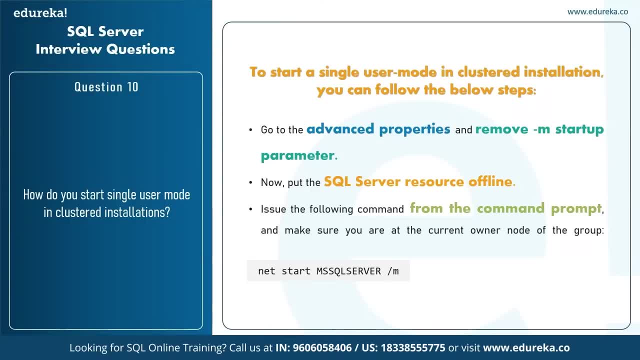 So to start a single user mode in clustered installations, you have to follow the steps that you can see on my screen. You have to first go to the advanced properties and then remove the hyphen M startup parameter. after that you have to put the SQL Server resource offline. 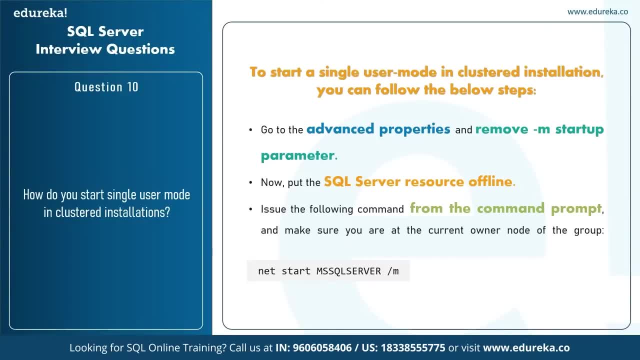 and then issue the command from the command prompt and make sure that you know you're at the current owner node of the group. So the command is basically net start MS SQL Server, slash M. after that you have to verify from the cluster administrator or failover cluster management console. 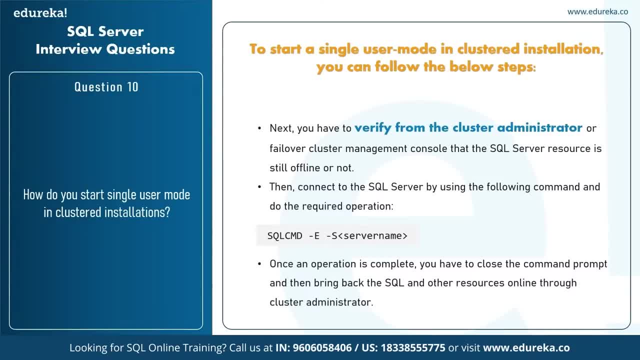 that a SQL Server resource is still offline or not, and then you have to connect the SQL Server by using the command SQL CMD, hyphen E, hyphen S, and then do the required operations. Once an operation is complete, you have to close the command prompt and then bring back the SQL Server. 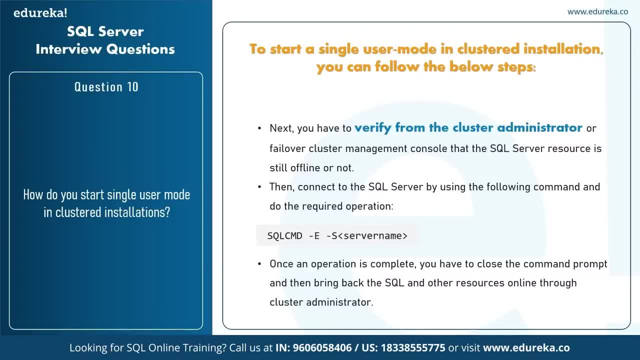 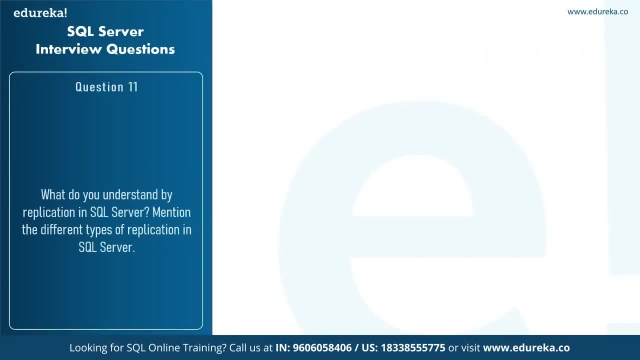 and other resources online through cluster administrator. So, guys, these are few steps that you have to follow to start single user mode in clustered installations. Now, moving on to the next question, That is, what do you understand by replication in SQL Server And what are the different types of replication? 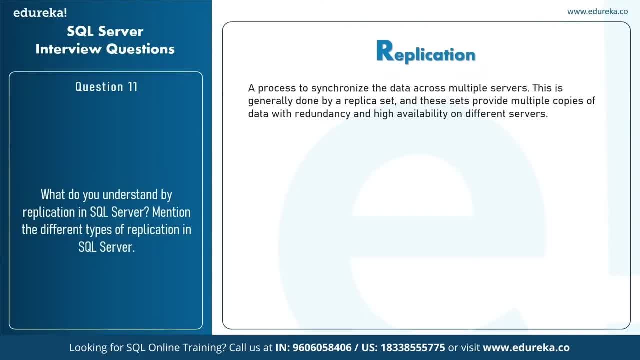 that are present in SQL Server. now, replication in Microsoft SQL Server is a process to synchronize the data across multiple servers. Now this is generally done by the replica set, and these sets provide multiple copies of data with redundancy and high availability on different servers. not only this. 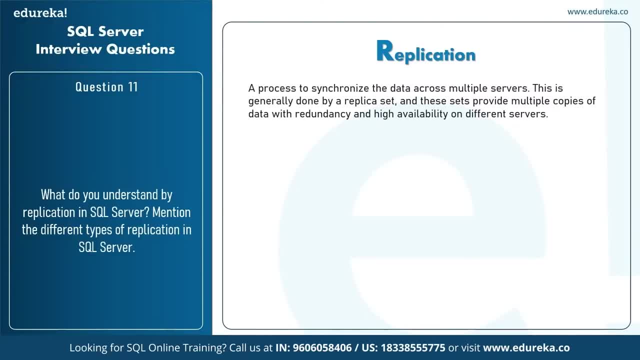 but replication also provides a mechanism to recover from the failures. So it basically removes the dependencies from single server to protect the loss of data from that particular server. Now the different types of replication available in SQL Server are merge replication, transactional replication and snapshot replication. 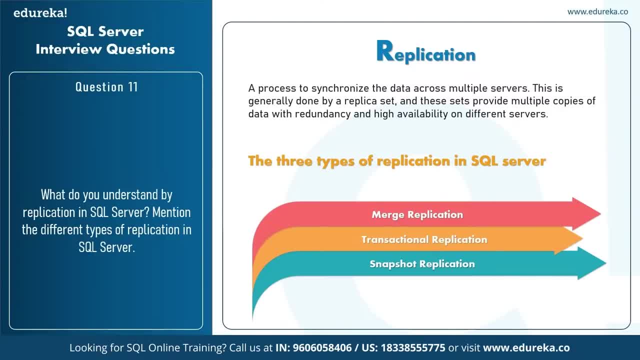 Now the merge. replication basically groups the data from various sources to a single centralized database and is used in the server to the client information. coming to transactional replication, This particular application is basically a process of distributing data from publisher to subscriber and is used in the server to server environments. moving 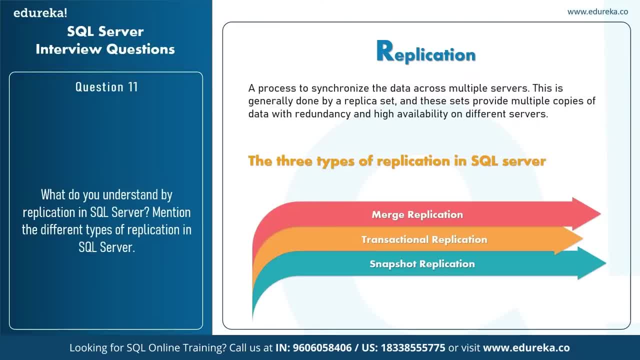 on to the final replication, That is, a snapshot replication. The snapshot replication basically distributes data exactly as it appears at a specific moment and is used for replicating data with changes in frequently. So, guys, that was about replication and its type. Now let's move forward with the next question. 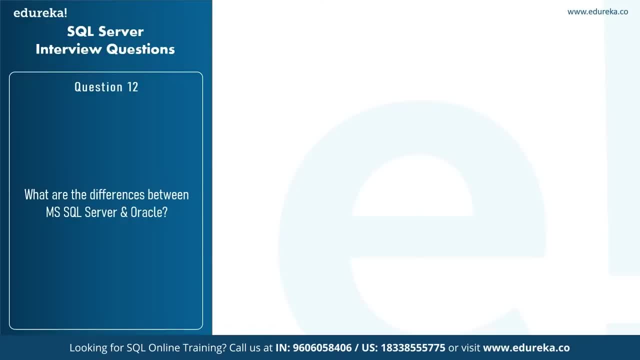 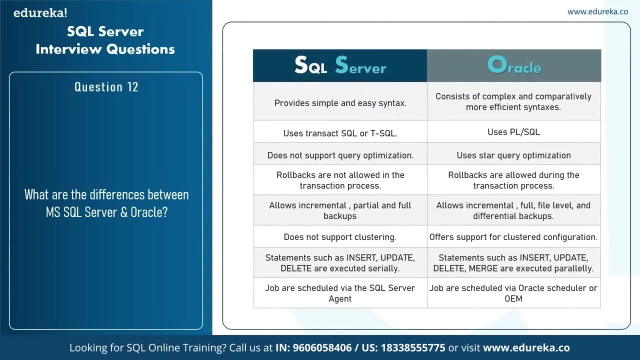 That is, what are the differences in between Microsoft SQL Server and Oracle? now, if you have to mention the differences between Microsoft SQL Server and Oracle, then MS SQL Server basically provides simple and easy syntax, whereas Oracle consists of complex and comparatively more efficient syntaxes. the MS SQL Server. 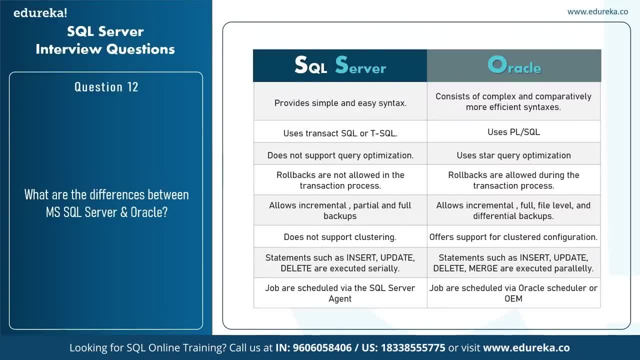 uses basically the transact SQL or the T SQL, but as Oracle uses the PL SQL. moving on to the next difference, that is, you know, SQL Server does not support query optimization, but Oracle supports query optimization and uses the star query optimization. moving on to the next difference: in SQL Server, rollbacks are not allowed. 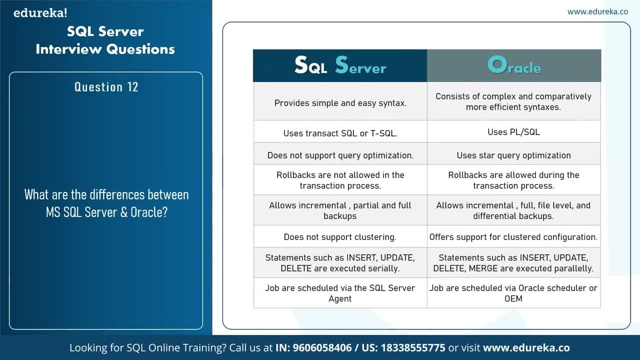 in the transaction processes, but in Oracle, rollbacks are definitely allowed during the transaction processes. SQL Server allows incremental, partial and full backups, Whereas Oracle allows incremental, full file level and differential backups. SQL Server does not support clustering, whereas Oracle offers support for clustered configurations in SQL Server. statements such as insert, update, delete. 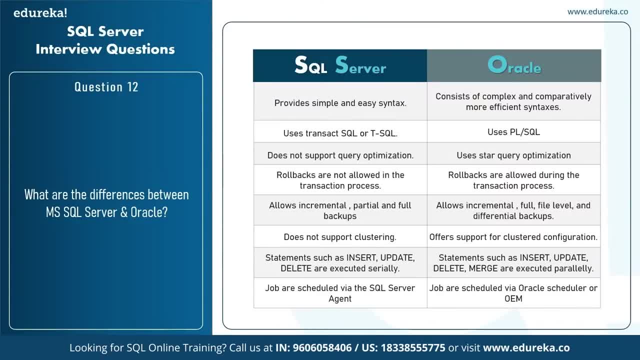 are executed serially, whereas in Oracle, statements such as insert, update, delete and merge are executed parallely. and finally, coming to the last difference, jobs are scheduled via the SQL Server agent and SQL Server, whereas jobs are scheduled via the Oracle scheduler or the OEM in Oracle. 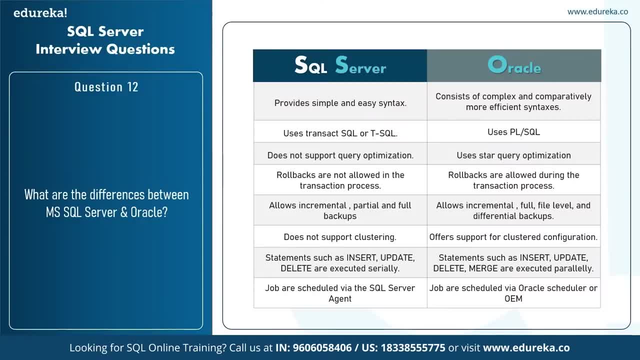 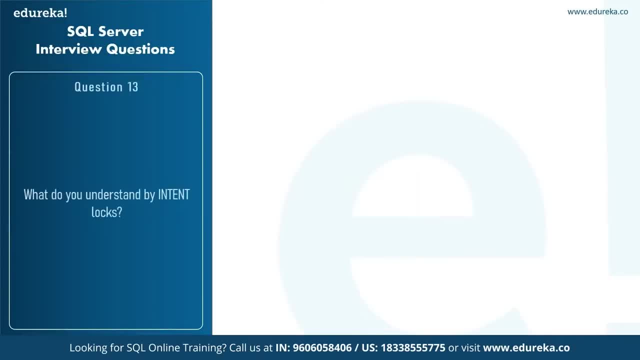 So, guys, these are a few differences between SQL Server and Oracle, So, as I said before, you can also talk about your personal experience while using both of them. Now let's move forward with the next question, That is, what do you understand by intent logs? now, 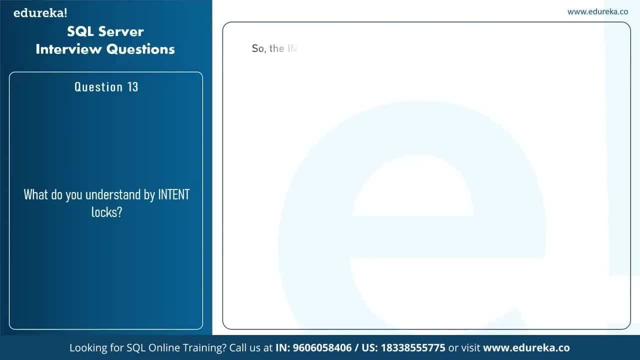 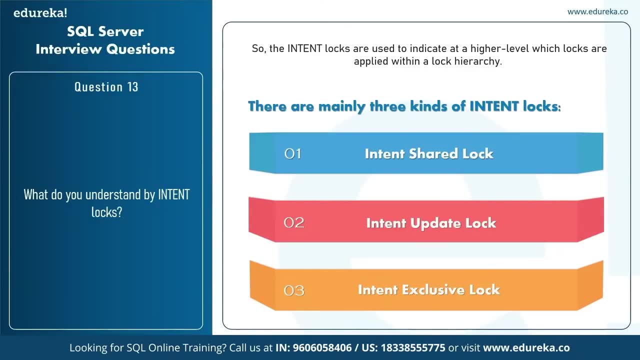 Microsoft SQL Server uses a log hierarchy whenever the data is read or something is changed in the data. So whenever a row is read, the SQL Server acquires a shared log, and whenever you change a row, the SQL Server acquires an exclusive log. So these logs are basically incompatible with each other. 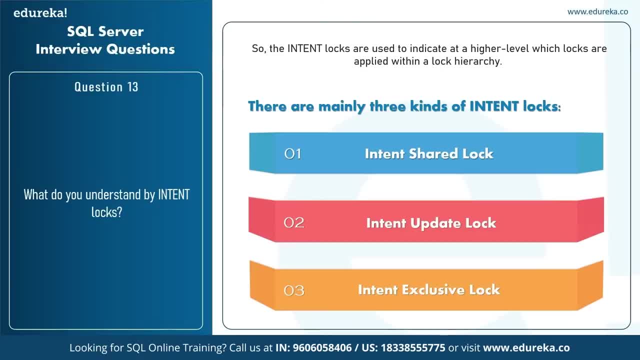 and this is where the intent logs come into the picture. So the intent logs are basically used to indicate at a higher level which logs are applied within a lock hierarchy. Now there are mainly three kinds of intense logs, that is, the intent shared lock, the intent update log. 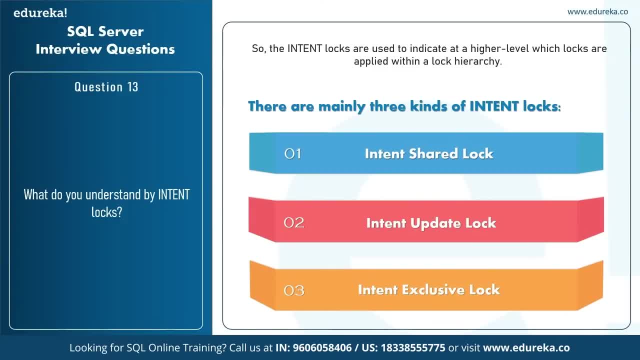 and the intent exclusive log. now, as the name suggests, the intention log is basically used when you have a shared lock at the row level. coming to intent update lock, the intent update log is used when you have an update lock at the row level. and finally, coming to intent exclusive lock, 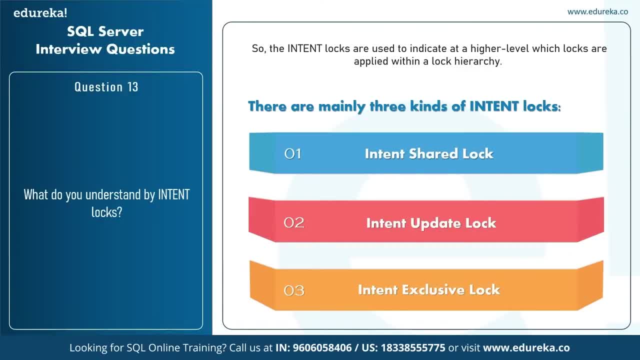 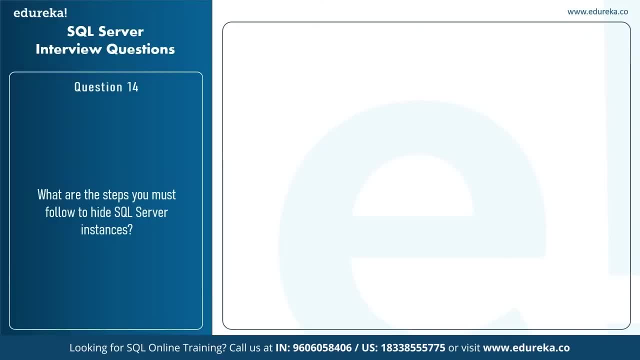 This particular lock is used when you have an exclusive lock at the row level. Now let's move forward with the next question, That is, what are the steps you must follow to hide SQL Server instances? now, the steps that you must follow to hide SQL Server instances are: 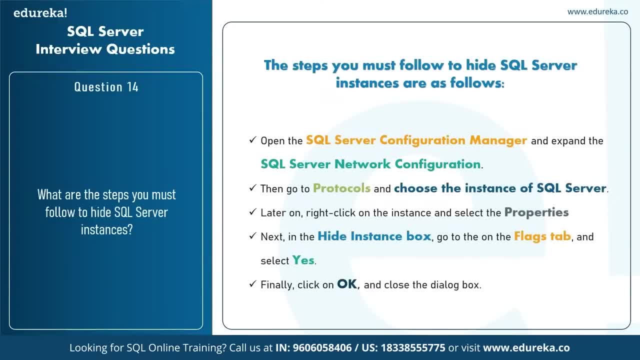 as you can see on my screen, initially have to open the SQL Server Configuration Manager and then you have to go to the SQL Server Network configuration. after that, in the SQL Server Network configuration, go to protocols and choose the instance of the SQL Server. later on you just have to right click on the instance. 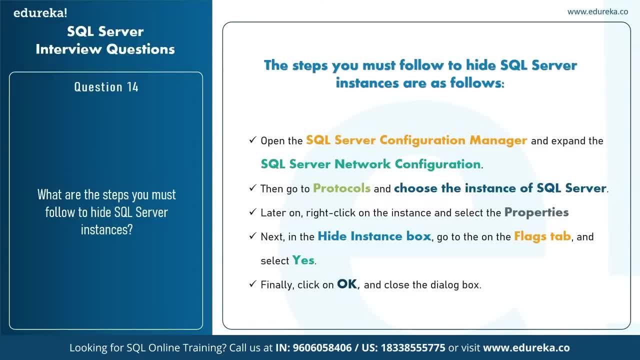 and select the properties. after that You'll see a dialog box which opens up. So go to the flags tab in that particular dialog box and then you see an option of hide instance over there. So over there you just have to go to that particular option. 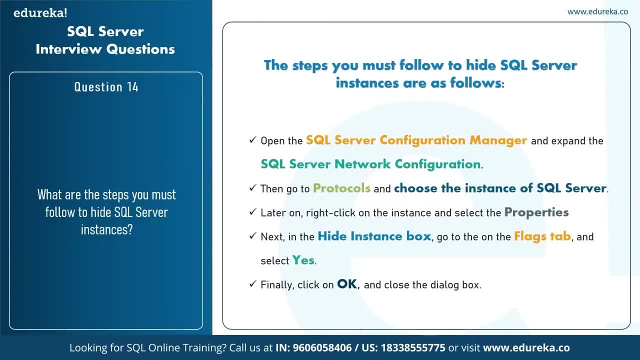 of hide instance and just say yes and then open the drop-down and choose Yes. So once you choose yes, you just have to finally click on OK and then, automatically, your instance will be hidden. So, guys, these were the steps to hide the instance. 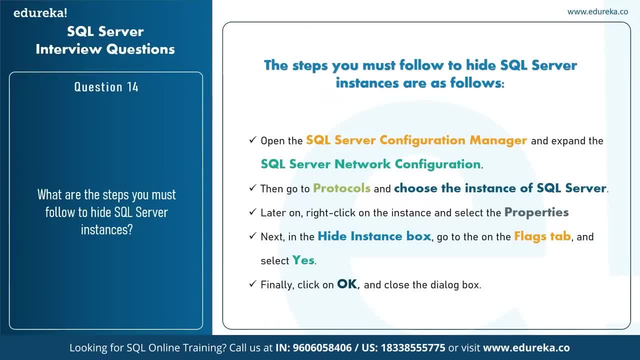 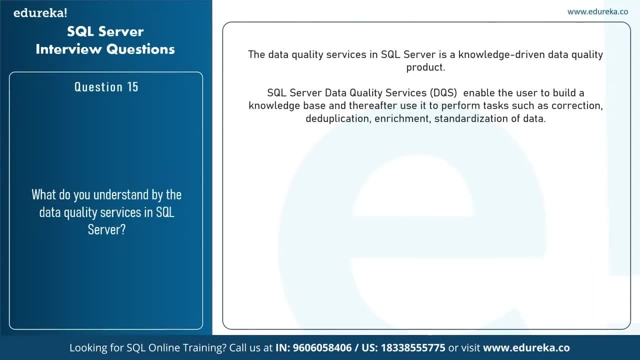 in SQL Server. next in this tutorial on SQL Server, Let's move forward with the next question, That is, what do you understand by data quality services in SQL Server? So the data quality services in SQL Server is basically a knowledge-driven data quality product, right? 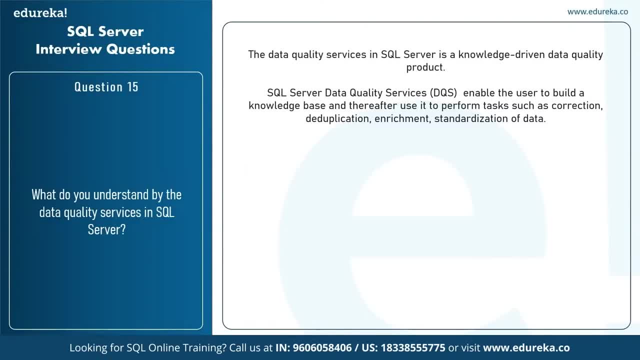 So the SQL Server data quality services enable the user to build a knowledge base and thereafter use it to perform tasks such as correction, deduplication, enrichment and standardization of data. Apart from this, the data quality services also provide profiling and enable you to perform data cleaning with help. 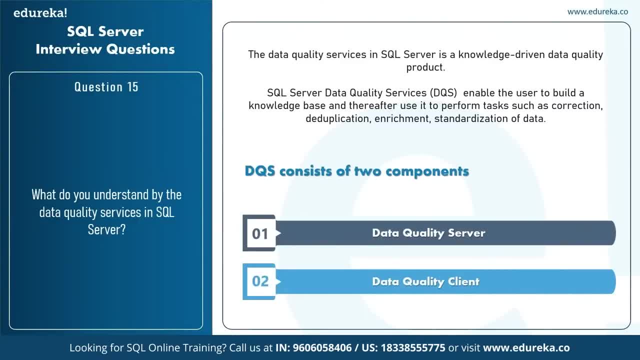 of cloud-based data services, Now the DQS services, or the data quality services, basically consists of two components, that is, the data quality server and the data quality client. now talking about the server first. So the data quality server is basically a SQL Server instance feature consisting of three SQL Server catalogs. 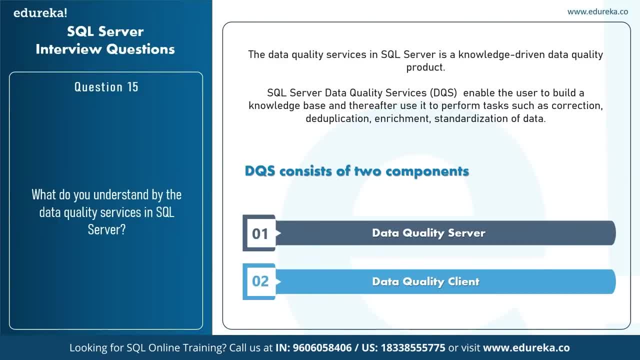 with data quality functionality and storage. coming to data quality client, It is also a SQL Server feature which users can use to perform computer-assisted data quality analysis and manage the data quality interactively, right? So, guys, that was about the data quality services. 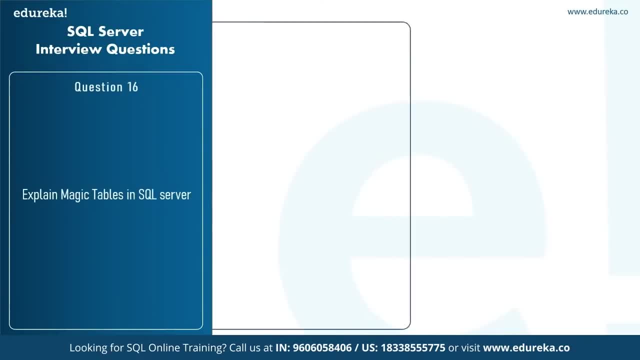 Now let's move forward with the next question, That is, explain magic tables in SQL Server. Now, magic tables are tables which are automatically created in SQL Server and are used to internally store the inserted updated values for DML operations such as select, delete, insert, update. 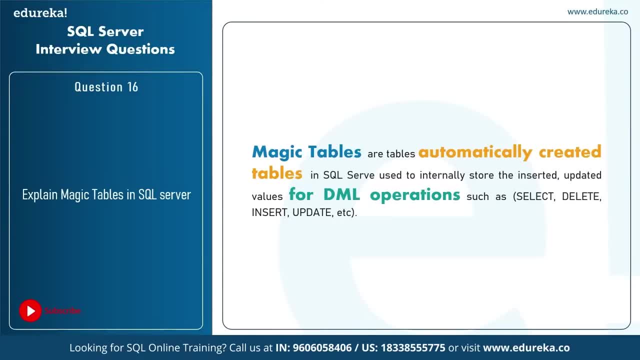 and so on, right? So basically, guys, magic tables are just automatically created, tables in SQL Server used to basically store values, you know, maybe inserted, updated or deleted, and you can understand that. you know magic tables are used on a temporary basis. Now let's move forward with the next question. 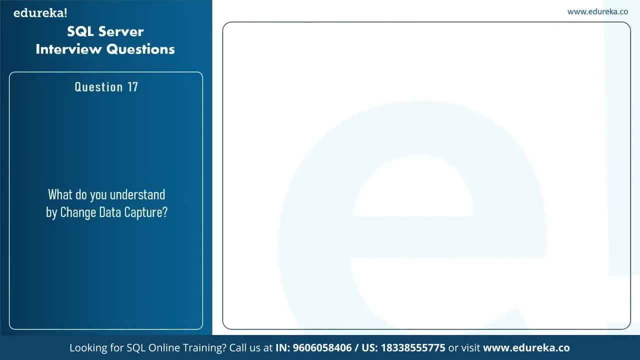 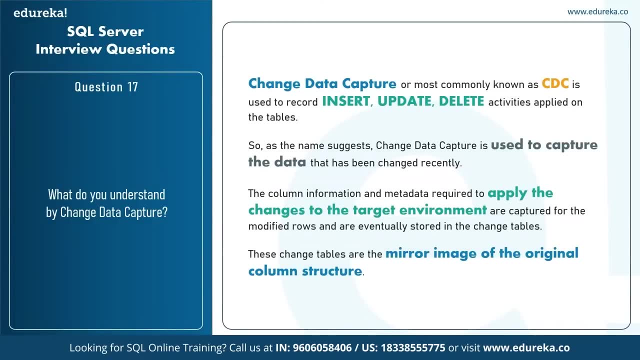 That is what do you understand by change data capture. So change data capture, or most commonly known as CDC, is used to record insert, update, delete activities applied on the tables. So, as the name suggests, the change data capture is used to capture the data that has been changed recently. 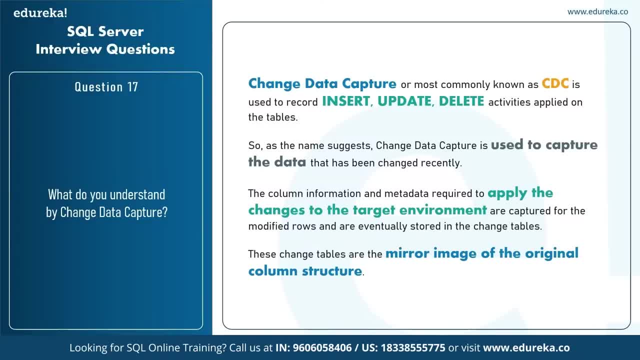 So the column information and the metadata required to apply the changes to the target information are captured for the modified rows and are eventually stored in the change tables. So these change tables are the mirror images of the original column structure. So, guys, that was about change data structure. 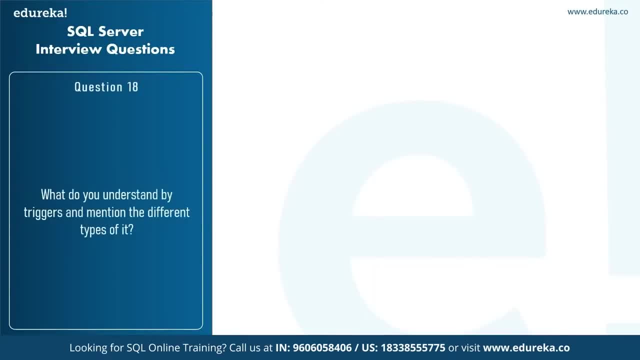 Now let's move forward with the next question, That is, what do you understand by triggers and mention the different types of it? So if you have to explain triggers, then triggers are used to execute batches of sequel code whenever insert, delete or update commands are executed against the table. 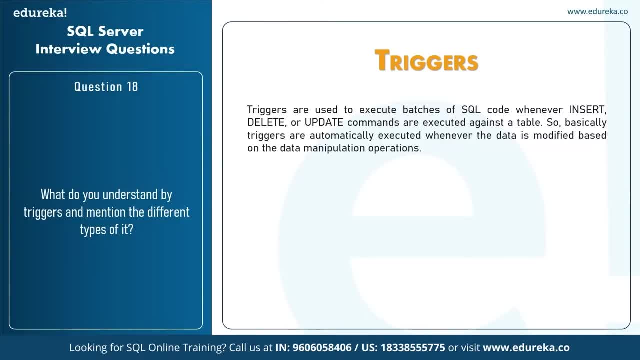 So basically, triggers are automatically executed whenever the data is modified based on the data manipulation operations, or you can just understand that you know triggers are triggered when there's an event happening. So the different types of triggers are basically insert, update, delete and instead of so guys, that was about triggers. 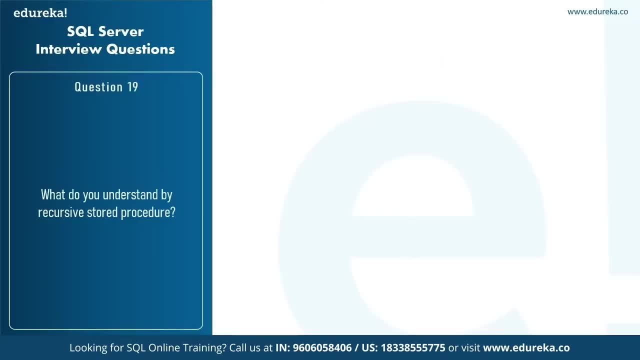 Now let's move forward with the next question, That is, what do you understand by recursive stored procedures? So recursive stored procedure is basically a problem-solving method through which you can arrive at the solution again and again and again, Right? So in programming also, we see recursive functions, right? 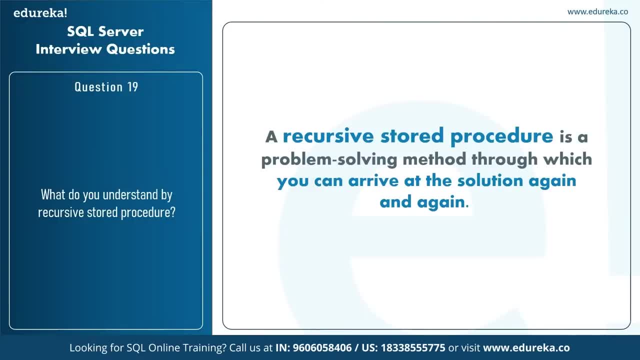 So you can just keep calling back the function and with the help of that, you can keep getting solution again and again, and again. right? So that's the same in sequel, Also because of stored procedures is basically a method through which you can arrive at the solution again and again. 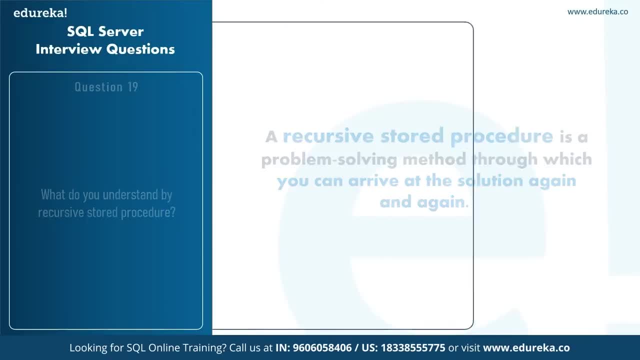 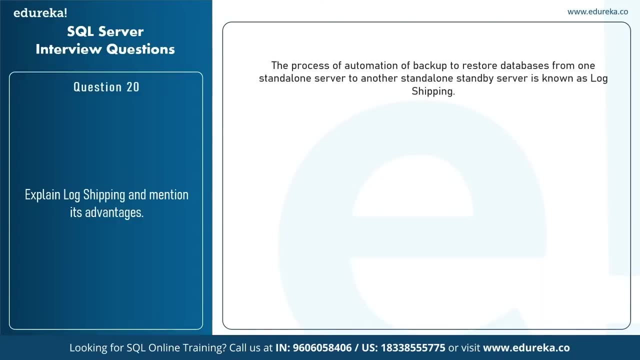 So that was about recursive stored procedures, guys, Let's move forward with the next question. That is explained: lock shipping and its advantages. Now, lock shipping is basically the process of automation of backup to restore databases from one standalone server to another standalone standby server. so you can understand lock shipping. 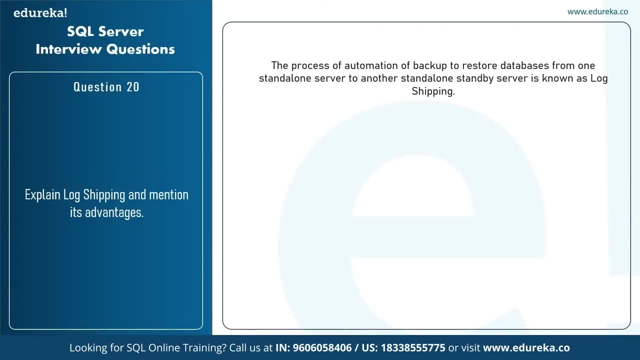 as one of those disaster recovery solutions, as it makes sure that you know, even if one server face, the standby server will have the same data as that of the server itself. So the advantages of lock shipping are as you can see in my screen. it needs low maintenance. 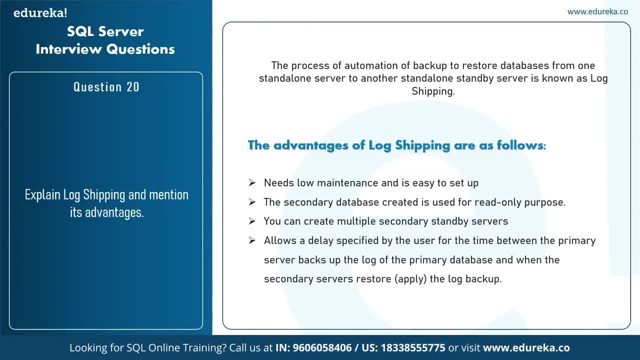 and it's easy to set up. the secondary database created is used for read-only purposes only, and you can also create multiple secondary standby servers. Not only this, but it also allows a delay specified by the user for the time between the primary servers. backup the log. 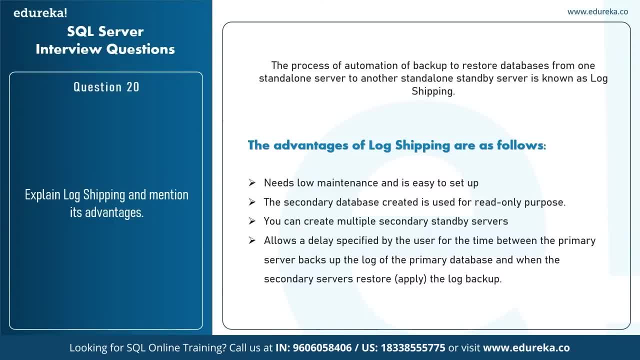 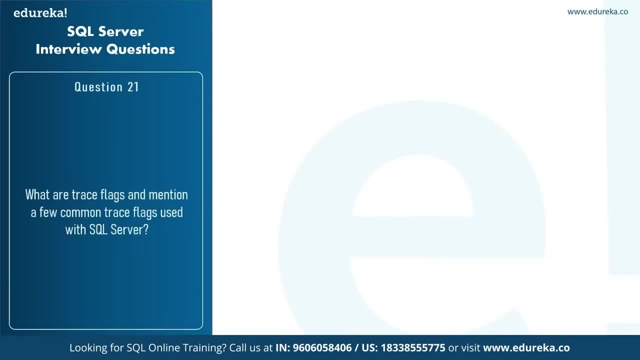 of the primary database and when the secondary servers restore or apply the log back up. So, guys, these are few advantages of lock shipping. Now let's move forward with the next question, That is, what are trace flags, and mention a few common trace flags. 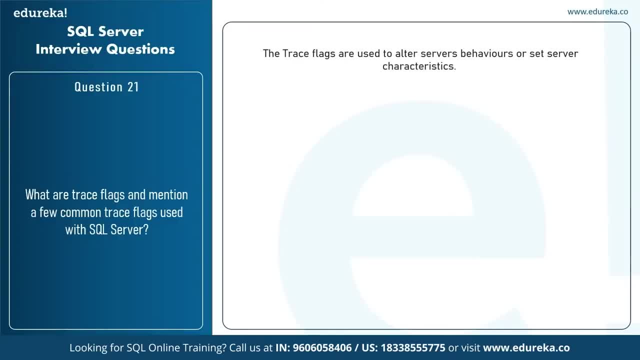 that you might have faced. So the trace flags are basically those flags which are used to alter server behaviors or set server characteristics. now, few common trace flags that all of us use or encounter, basically 1, 2, 0, 4, 1, 2 0, 5, 1, triple 2.. 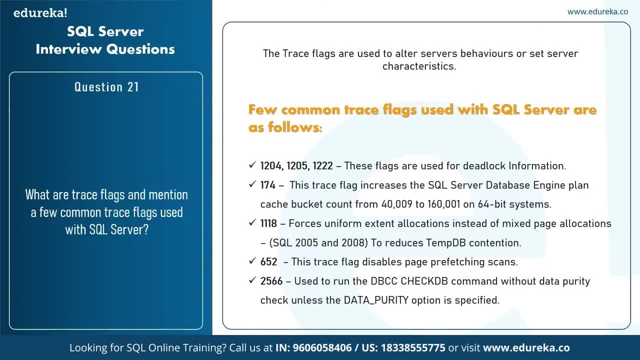 So all the three of them are used for deadlock information. The 174 trace flag is used to increase the sequel server database engine plan cache back account from 40,000 9 to 1 lakh 60,000 1 on 64-bit systems. 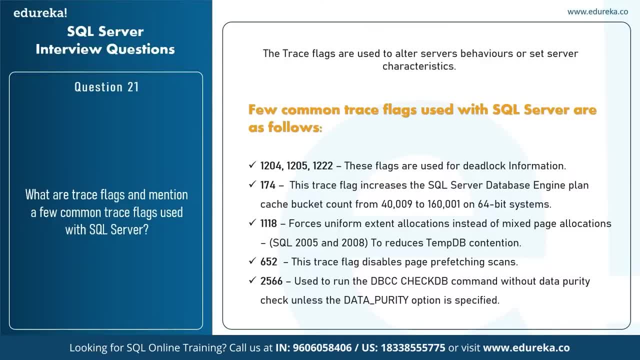 coming to triple 1- 8.. So triple 1: 8 forces uniform extent allocations instead of mixed page allocations. moving on to the next one, that is 652. now, 652 is basically used to disable the page prefetching scans, and 2, 5, double 6 is used to basically run the DB CC check. 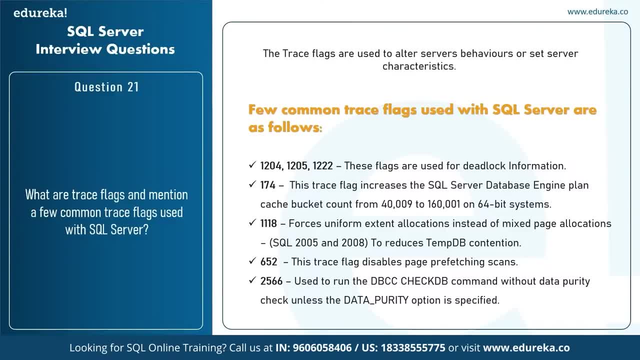 DB command without the data purity check unless the data purity option is specified. So if these are few trace flags that I have encountered or I've used, that, this answer is not something that you know. you have to give only these face flags. There are hundreds of trace flags present. 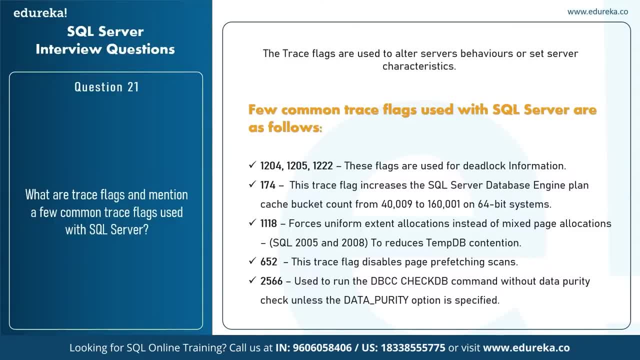 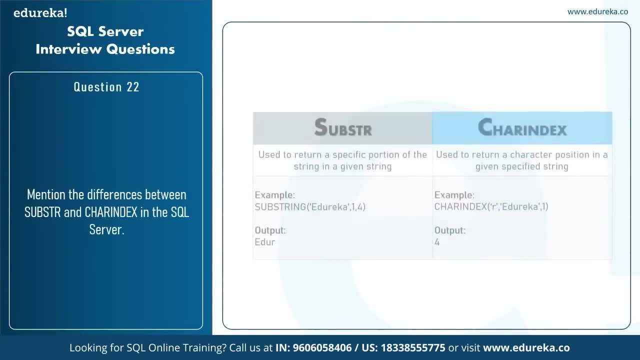 So whatever you have encountered, or maybe whatever you have used, you can mention that right now. let's move forward with the next one that is mentioned: the differences between substring and character index and sequel server. substring is basically used to return a specific portion of the string. 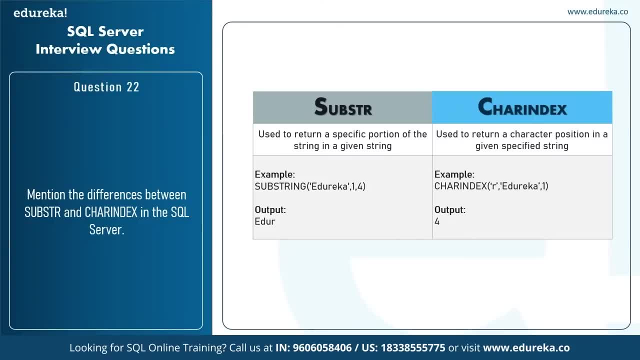 in a given string, But whereas the character index is used to return a character position in a given specified string right. So, for example, if you have substring at Eureka 1 comma 4, so what the syntax mentioned is that you know. 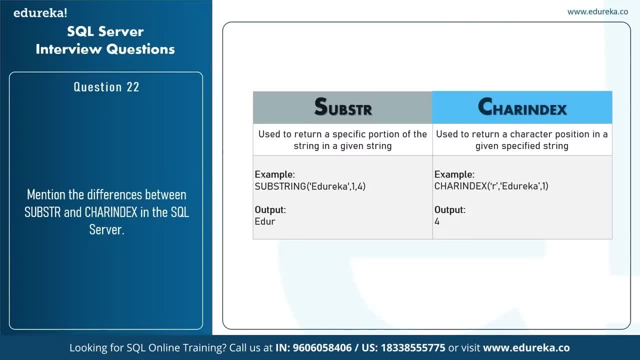 Eureka is our string. 1 is a starting value from where the characters have to be extracted, and 4 is the range till where the characters have to be extracted. So if you count a direct on your fingers, we have seven letters right. 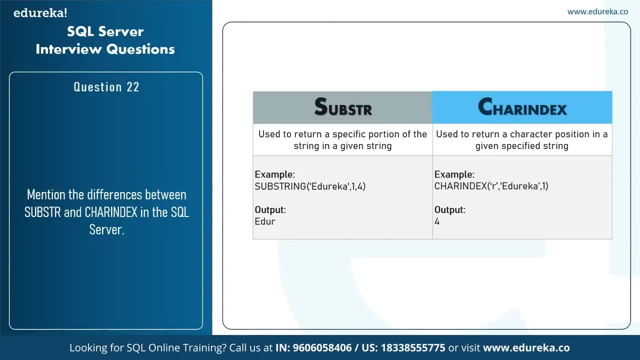 So we've mentioned 1 to 4.. So our output should be: edu are right, So it starts with E. That's a first letter, then D, second one, you third one and our fourth one. but when it comes to character index, character index. 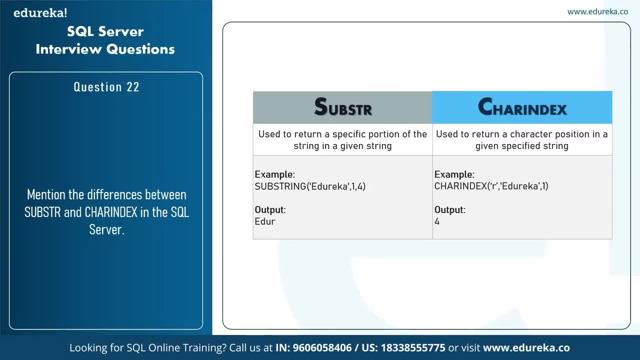 as I mentioned before, is used to return a character position in the given string right. So, for example, if you mention an example, character index are comma Eureka. comma 1 R is basically the character for which we want to find out the position. 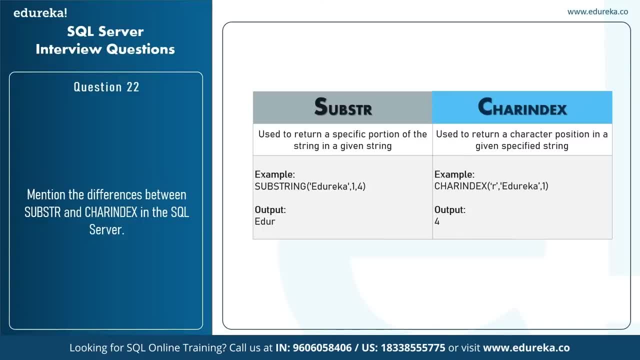 It is a guy's a string and one is the starting range of the string. So if you again count a direct on your fingers, then you see R is at the fourth position. So we see output us for. so, guys, these were the differences between some string. 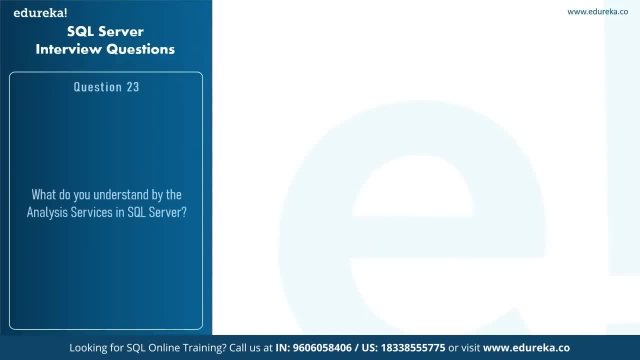 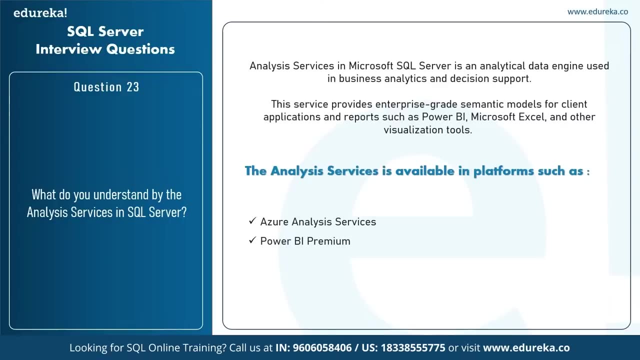 and character index in SQL Server. Now let's move forward with the next question, That is, what do you understand by analysis services in SQL Server? So analysis services in Microsoft SQL Server is an analytical data engine used in business analytics and decision support. 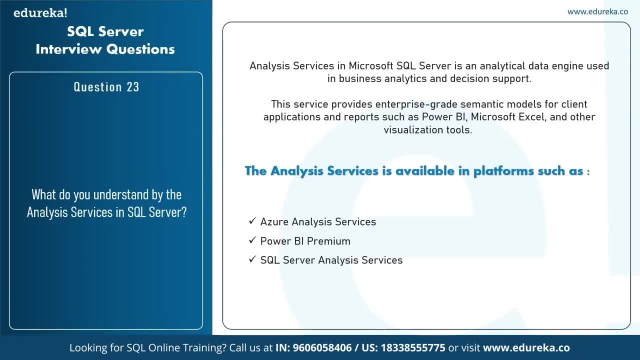 So this service basically provides Enterprise grade semantic models for client applications and reports such as Power BI, Microsoft Excel and other visualization tools. So the analysis Services is basically available in platforms like you know: Power Analysis Services, Power BI Premium and SQL Server analysis Services. 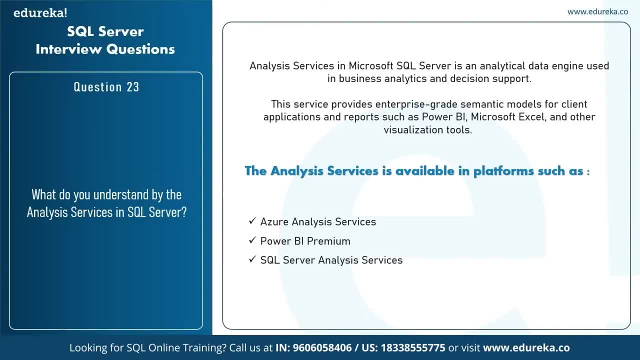 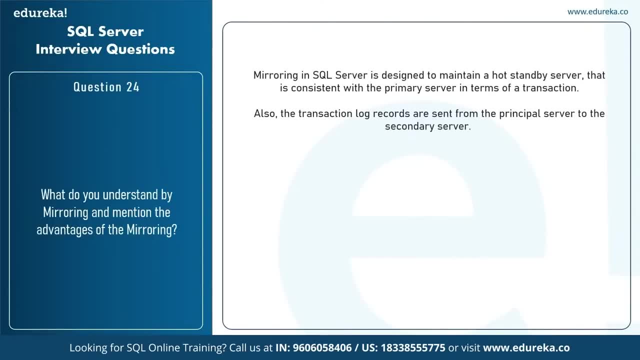 So, guys, that was about analysis Services in SQL Server. Now let's move forward with the next question. That is: what do you understand by mirroring and mention few advantages of it? So mirroring in SQL Server is basically designed to maintain a hot standby server. 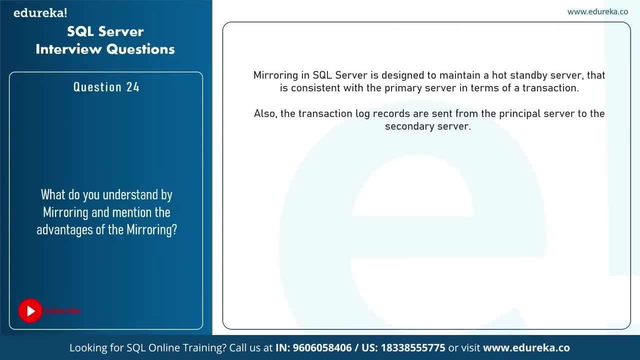 that is consistent with the primary server in terms of the transaction. Also, the transaction log records are sent from the principal server to the secondary server. Now, the advantages of mirroring are: as you can see on my screen. It consists of an automatic failover mechanism. 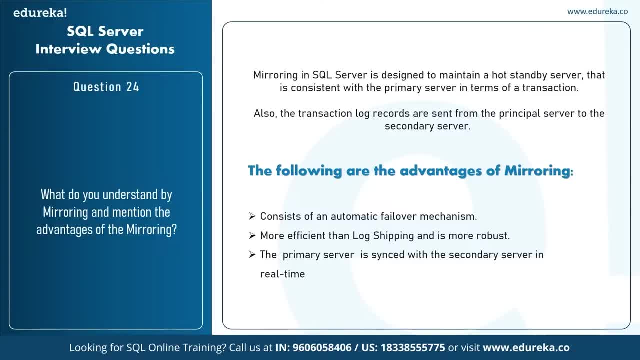 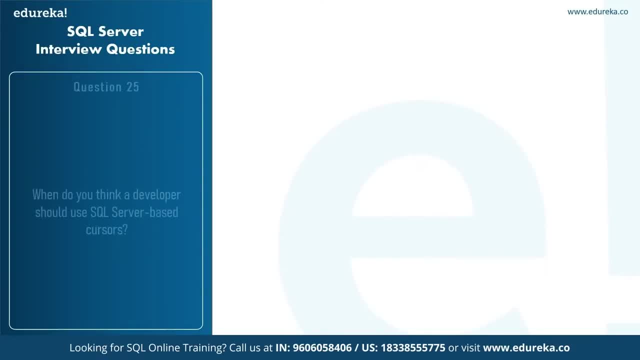 It is more efficient than the log shipping and is more robust, and the primary server is synced with the secondary server in real time. So, guys, that was about mirroring. now let's move forward with the next question, That is, when do you think a developer should use? 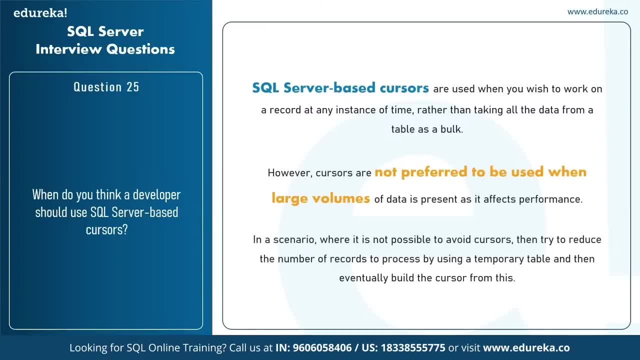 SQL Server based cursors. So SQL Server based cursors are used when you wish to work on a record at an instance of time rather than taking all the data from a table as a bulk. However, cursors are not preferred to be used when large volumes of data. 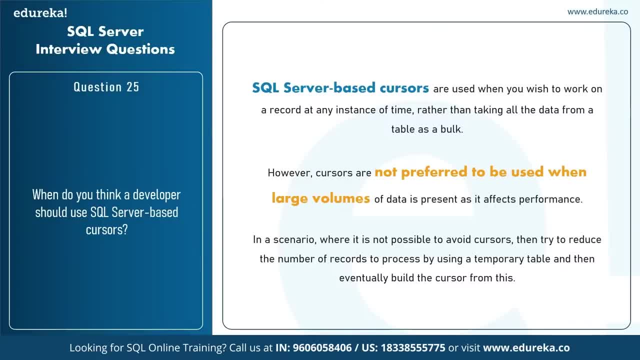 is present as it affects the performance. So in a scenario where it is not possible to avoid the cursors, then I would suggest try to reduce the number of records to process by using a temporary table and then eventually build the cursor from this. So I think, guys, this is one of the most practical questions. 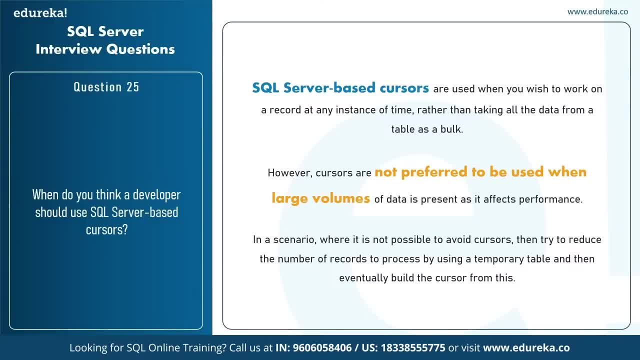 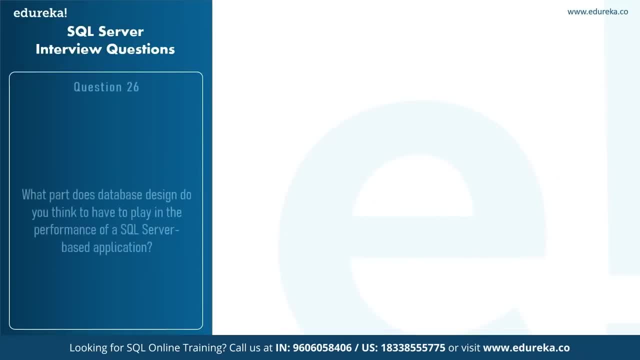 that could be asked, where the interview checks whether you have practical knowledge of where SQL can be used and how you can use different commands or different functionalities based on the scenarios. Now let's move forward with the next question, That is, what part of database design do you think? 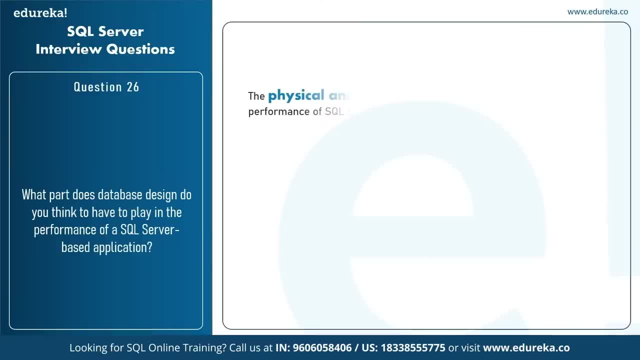 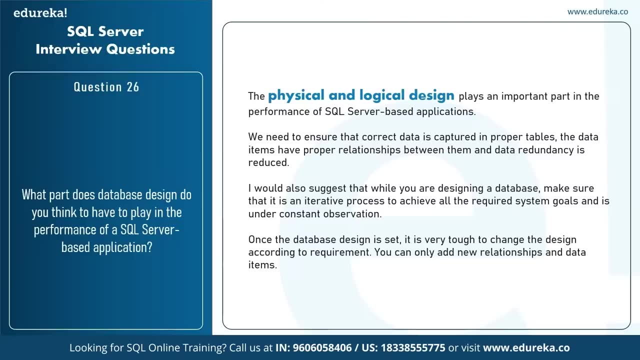 affects the performance of a SQL Server based application. Well, I would say the physical and the logical design plays an important role in the performance of SQL Server based applications and we need to ensure that the correct data is captured in the proper tables. The data items have proper relationships between them. 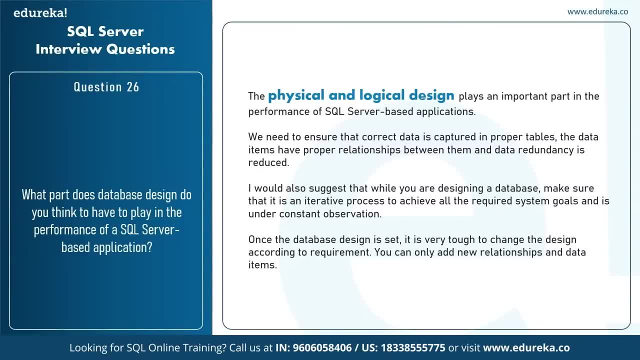 and the data redundancy is reduced. I would also suggest that you know, while you're designing a database, make sure that it is an interactive process to achieve all the required system goals and is under constant observation to make sure you know all the client requirements are added. 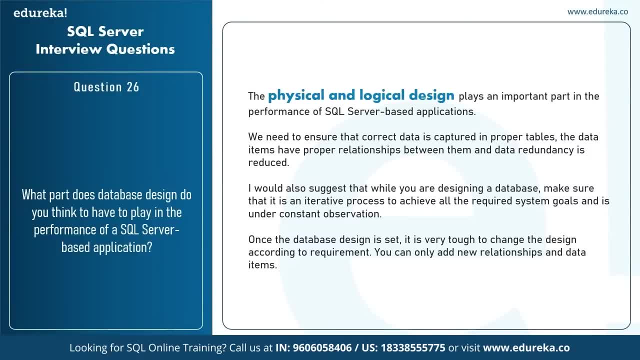 and the database satisfies the requirement. now I'm saying this because you know, once the database design is set, it's very tough to change the database design according to the requirements that come later on. So you cannot change the basic entities of the databases. 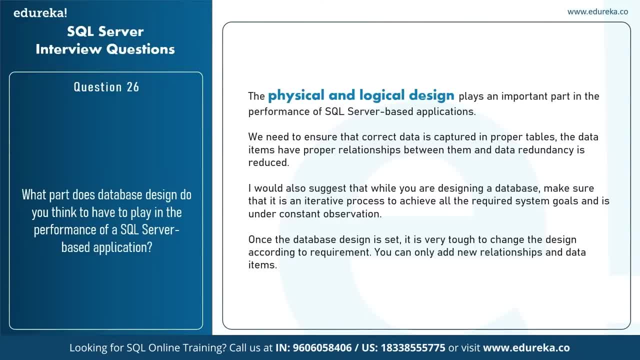 but you can only add new relationships and data items. So I would say, if something affects the performance of a SQL Server based application, then I would say the physical and the logical design of the database affects the most. now let's move forward with the next question. 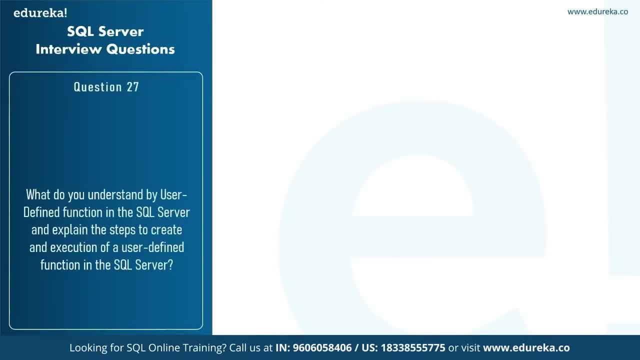 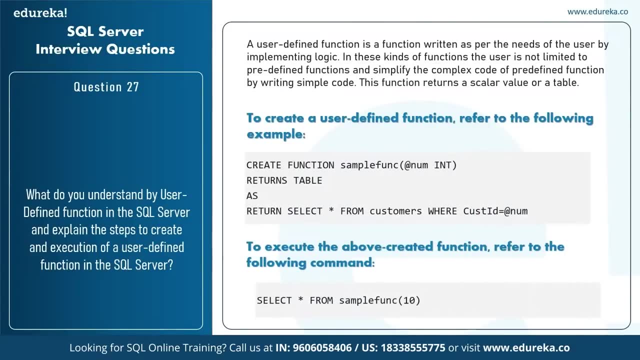 That is, what do you understand by user-defined functions in SQL Server? And then, what are the steps to create and execute the user-defined function in a SQL Server? Well, a user-defined function, as the name suggests, is a function written as per the needs of the user. 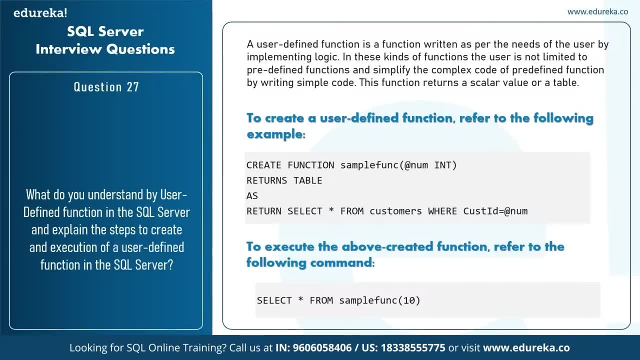 by implementing a specific logic. now, in these kinds of function, The user is not limited to any predefined functions and simplifies the complex code of a predefined function by writing a simple code. apart from this, Let me also tell you that you know the user-defined function returns a scalar value or a table. 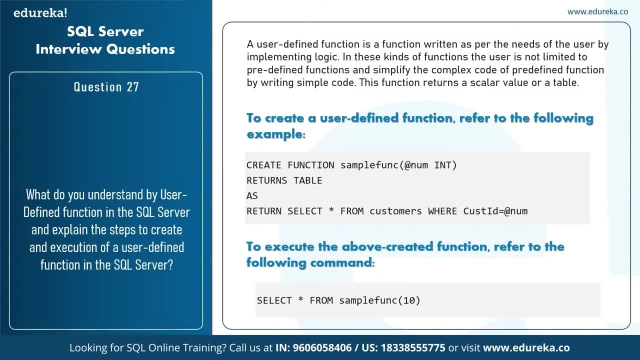 not to create a user-defined function. You can refer to the example that you can see on my screen. I've just created a function, sample, funk, and then in the brackets I've put either it, num, int, So basically it's an integer and then it returns a table as return: select star. 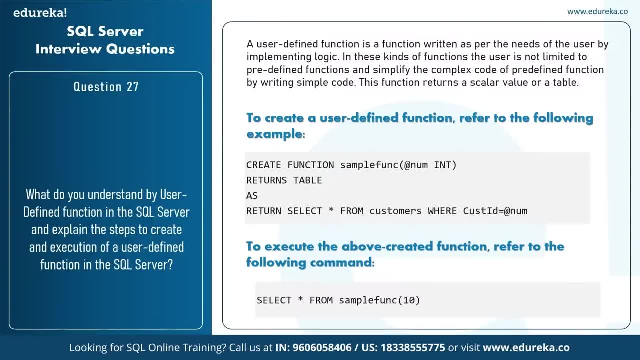 from customers with customer ID equal to- at right now, bread. We're trying to basically return all the customer IDs from a customer table and store it in the table Now. after that, to execute the function that we are just created, You just have to mention the command select star. 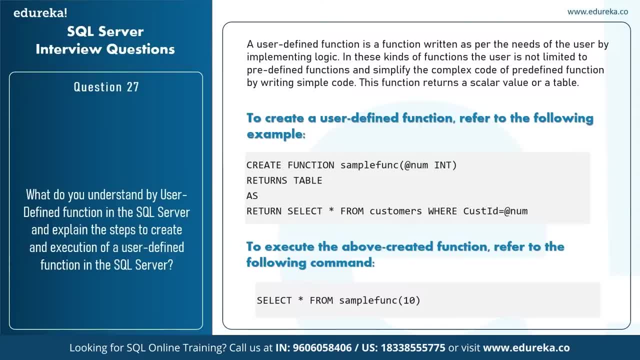 from sample funk. that is basically the functions name and in brackets you'll mention the customer ID. So, for example, I'd mentioned 10 over here. So that's how, guys, you can create a user-defined function and also execute it. Now let's move forward with the next question. 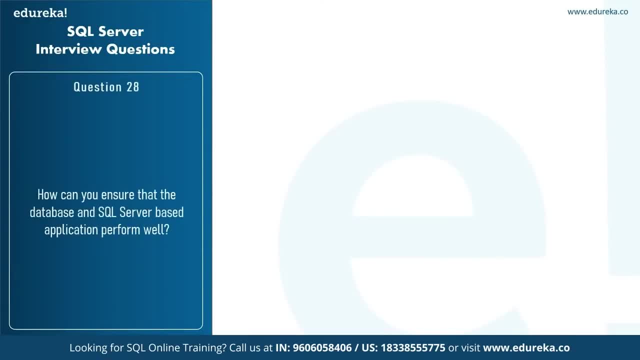 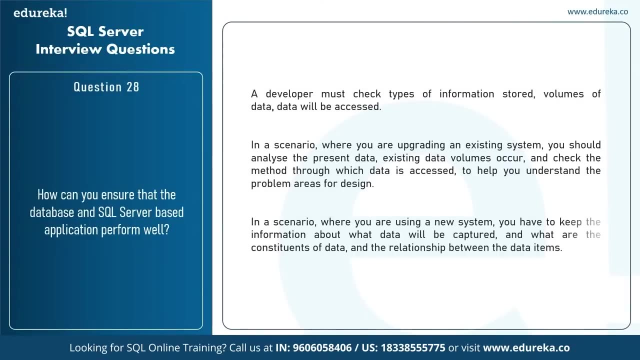 That is, how can you ensure that the database and sequel server-based applications perform well? Well, I would say, to ensure that the database and the sequel server-based applications perform well, a developer must check the types of information stored, the volumes of data and what data will be accessed. 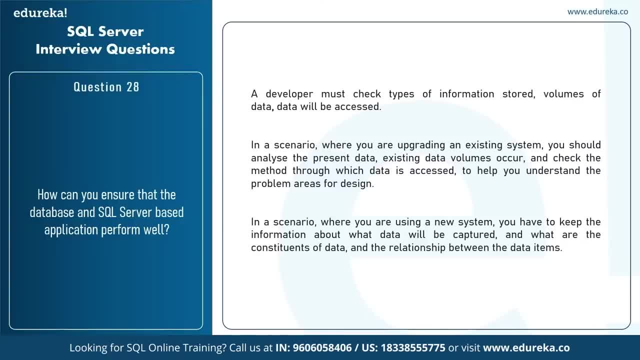 So, in a scenario where you're upgrading an existing system, you should analyze the present data- the existing data volumes occur- and then check the method through which the data is To help you understand the problem areas for the design. but, on the other hand, 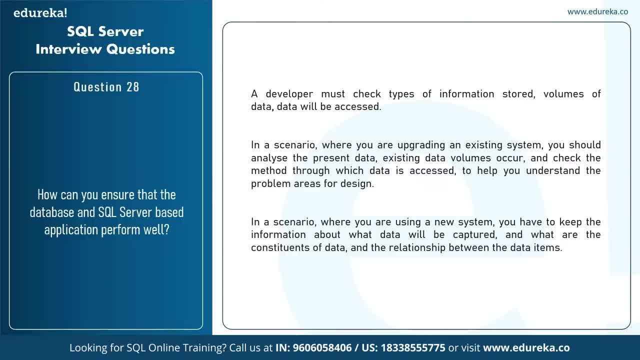 if you're creating a new system, then you have to keep the information about what data will be captured, What are the constituents of data and the relationship between the data items. So like that, the developer can make sure that you know the database and sequel server-based applications. 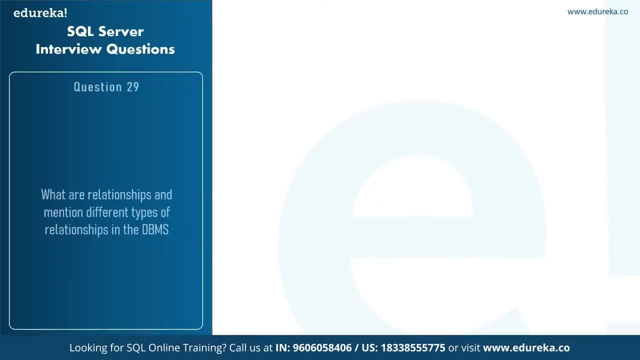 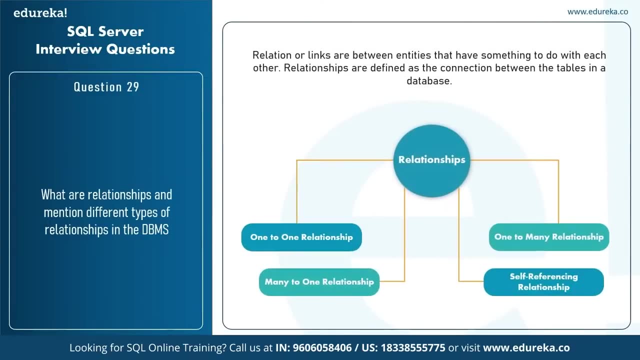 can perform well. Now let's move forward with the next question, That is, what are relationships in databases and what are the different types of it? Well, I would say a relationship in database management system is a scenario where two entities are related to each other. 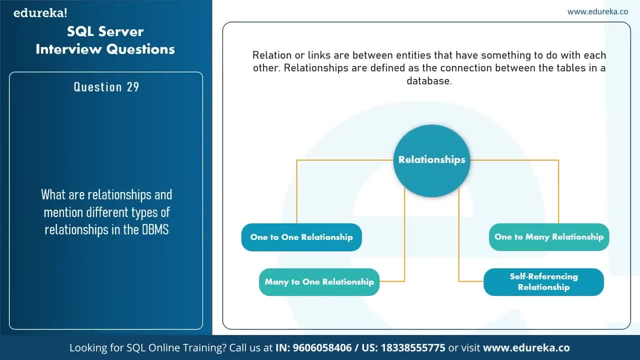 So, basically, if you have two tables, table A and table B, then the table consisting of the foreign key references to that of the primary key of the other table. So the different types of relationships in DBMS or database management systems are one-to-one relationship, one-to-many relationship, many-to-many relationship. 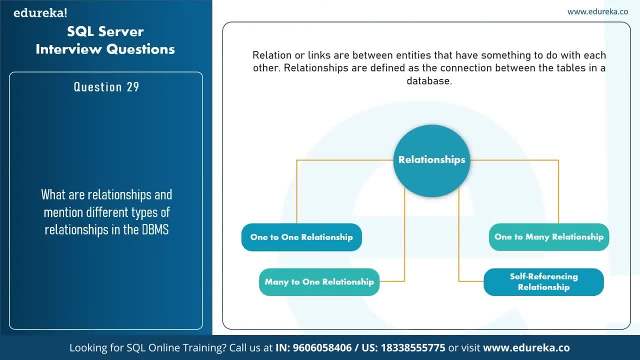 and self-referencing relationship coming to one-to-one relationship. So this is basically used when a single row in table A is related to single row in table B coming to one-to-many relationship. This is used when a single row in table A is related to many rows in table B coming 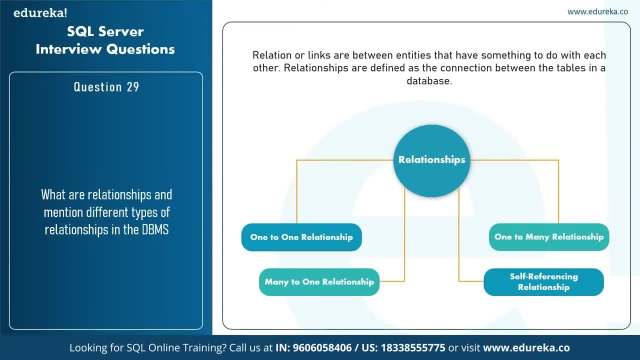 to many-to-many relationship. This is used when you have many rows in table A related to many rows in table B. and finally, coming to self-referencing relationship, This is used when a record in table A is related to the same table itself. 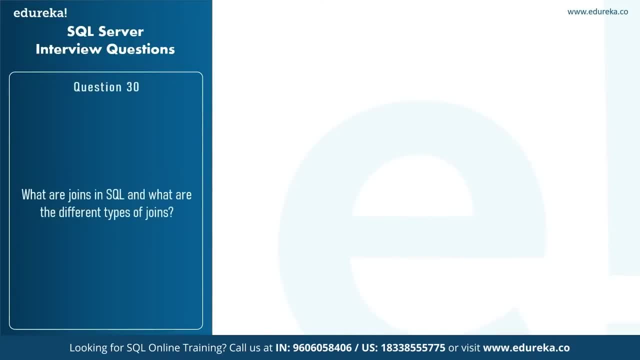 Now let's move forward with the next question, That is, what are joints in sequel and what are the different types of joints? a joint clause is basically used to combine rows from two or more tables based on a related column between them, and it is used to merge two tables. 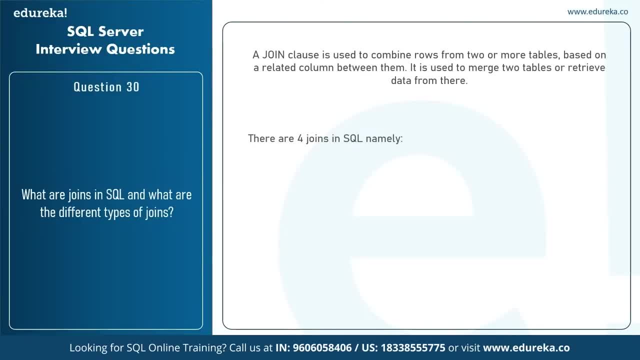 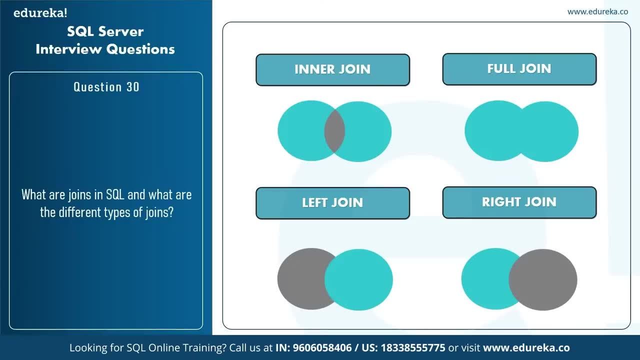 or retrieve data from there. So there are mainly four types of joints. is equal: the inner joint, the right joint, the left joint and the full joint right. So I'm not going to go into depth of them. So if you want to know how to use sequel joints, 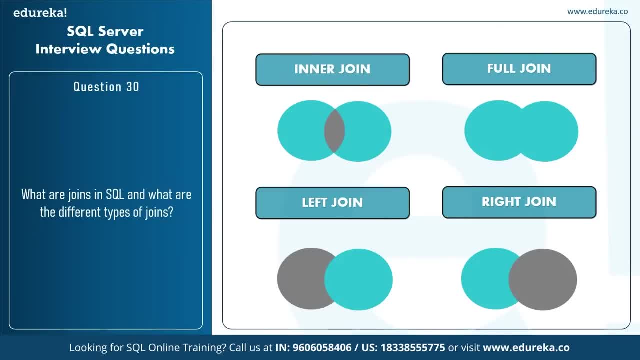 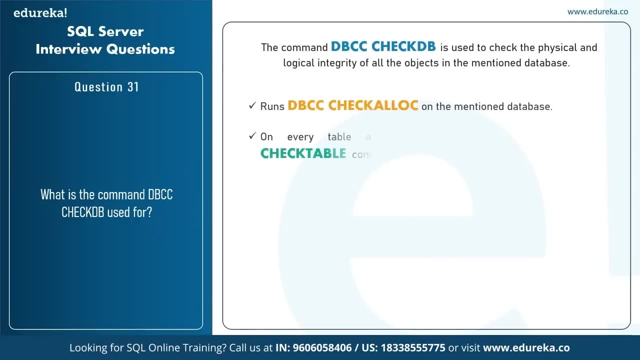 you can refer to my session on sequel joints. on that note, Let's move forward with the session and let's look into the next question, That is, what is the command DB, CC, check DB used for? so the command DB, CC, check DB is used to basically check. 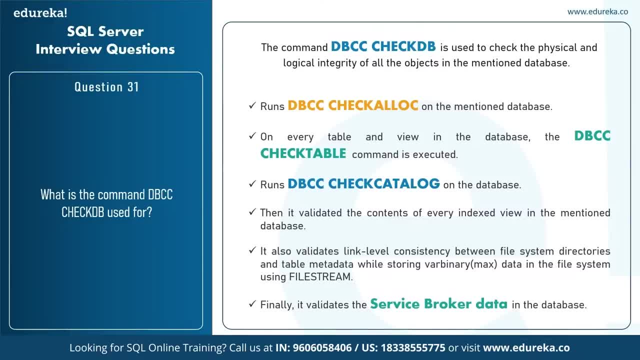 the physical and the logical Integrity of all the objects in the mentioned database. So to do that, it basically performs the operations that you can see on my screen. It runs the DB CC check a log on the mentioned database and on every table and view in the database. 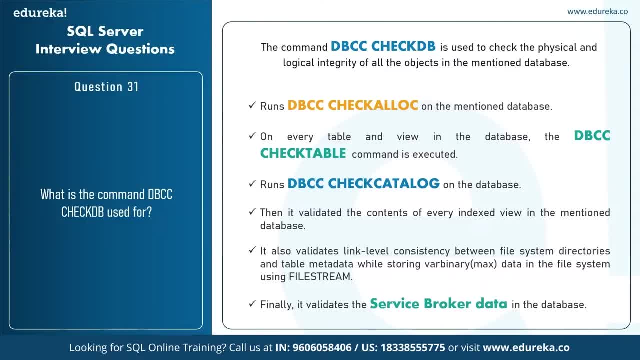 The TV CC check table command is executed. It also runs the DB CC check catalog on the database and then it validates the contents of every index view in the mentioned database. after that It also validates the link level consistency between file system direct crease and table metadata. 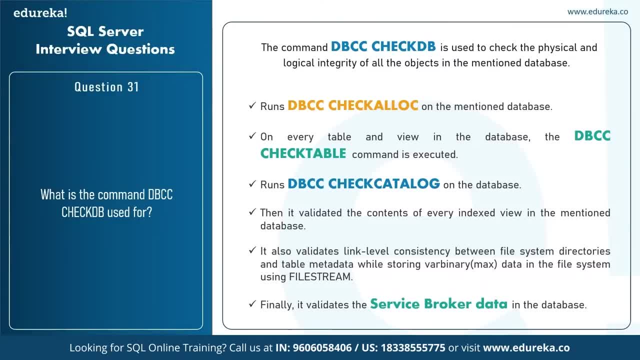 while storing where binary Max data in the file system using file stream. Finally, it validates the service broker data in the database. So, if you observe clearly, you just have to execute the DB CC check DB command and automatically the DB CC check a log, the check table. 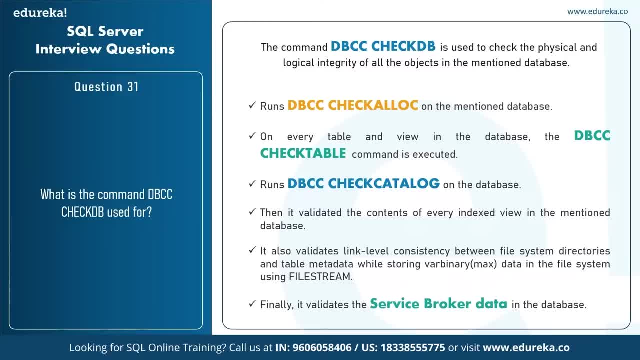 and the check catalog command gets executed. also know that DB CC supported on databases that contain memory optimized tables, but does not provide repair operations. So basically, this implies that you must regularly backup databases and test those backups. So, guys, that was about the DB CC check DB command. 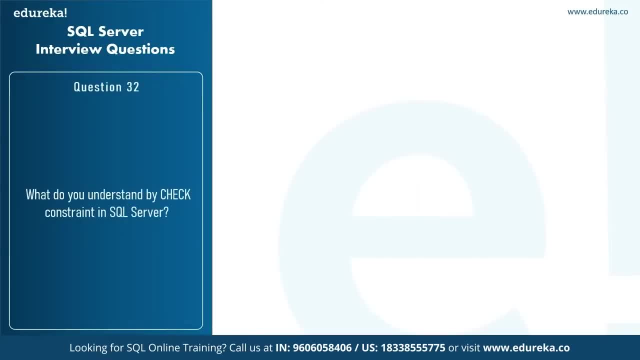 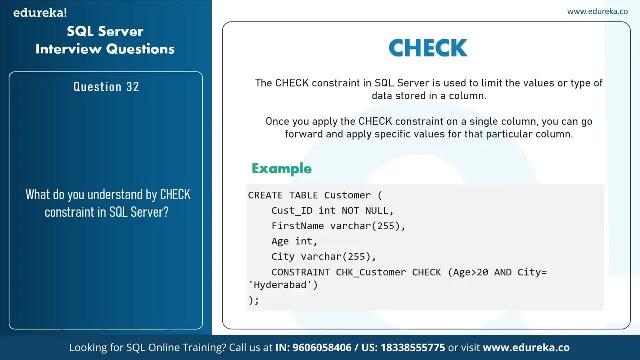 Now let's move forward with the next question, That is, what do you understand by check constraint in sequel server? So the check constraint in sequel server is basically used to limit the values or the type of data stored in a column. Now, once you apply the check constraint on a single column, 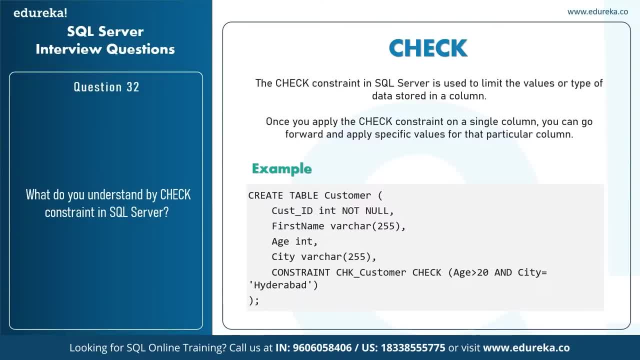 you can go forward and apply specific values for that particular column. See the example on my screen. I've created a table customers with few columns like customer ID, first name, age and City, and then I've applied the check constraint and then I've given the name to be check underscore: customer. 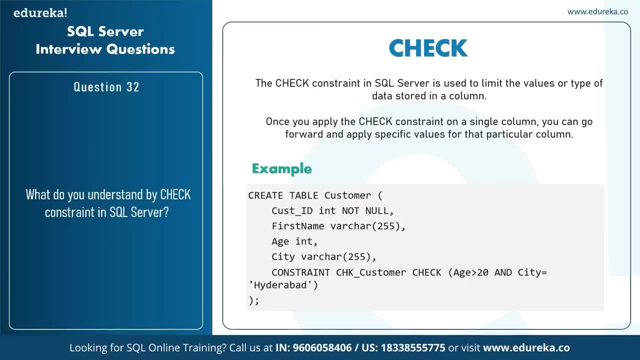 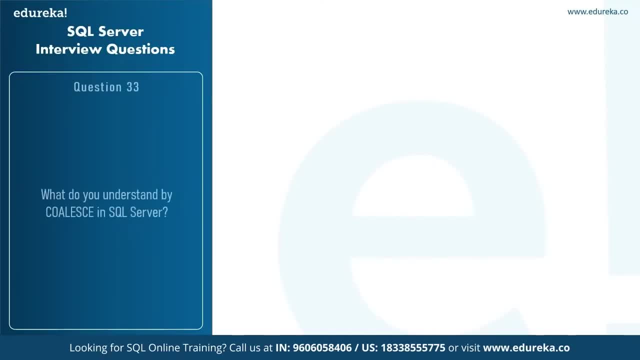 and the condition that I've applied is basically: 8 should be greater than 20 and City should be Hyderabad. So, guys, that is basically how you can use the check constraint. Now let's move forward with the next question. That is, what do you understand by? coil is in sequel server? 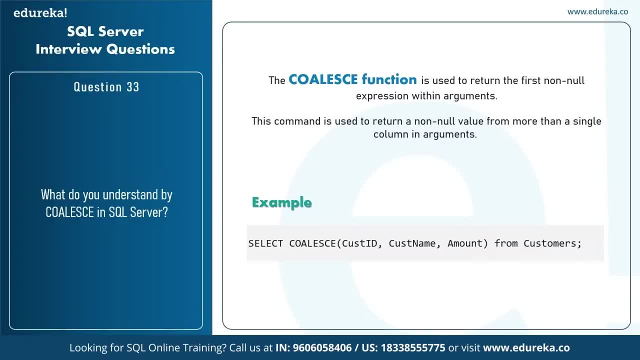 and the coil is function is used to basically return the first normal expression within the arguments. So the coil is command is basically used to return a non-null value from more than a single column in arguments. So to use the coil is command, You can refer to the example that you can see on my screen. 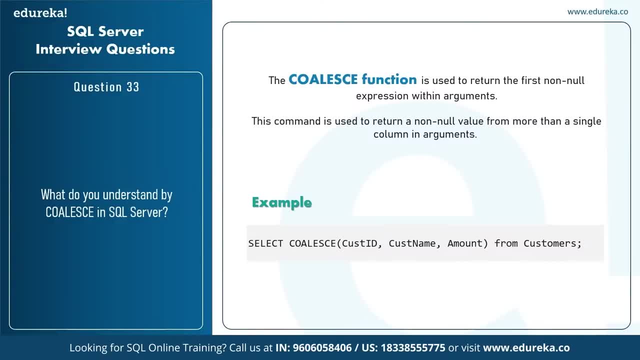 that is, select coil is. and then I've mentioned customer ID, customer name amount from customers, right? So basically customers was a table and customer ID, customer name amount are basically a column names, right? So I'm basically trying to return the first normal expressions. 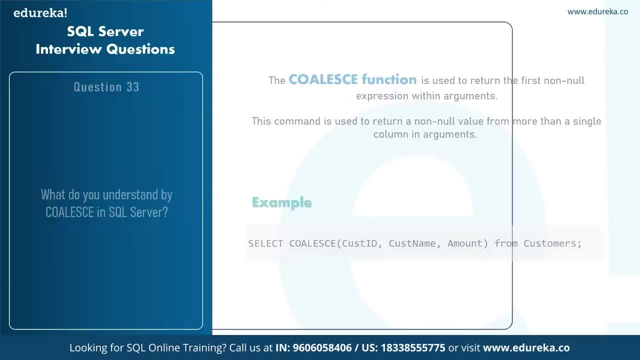 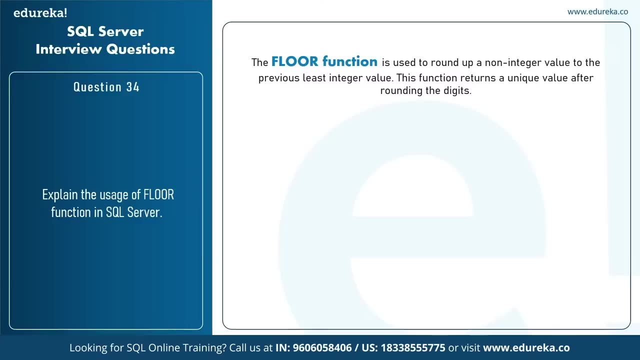 from customer ID, customer name and amount. now let's move forward with the next question. that is explained- the usage of floor function in sequel server- that the floor function is used to round up a non-integer value to the previous least integer value. This function returns a unique value after rounding. 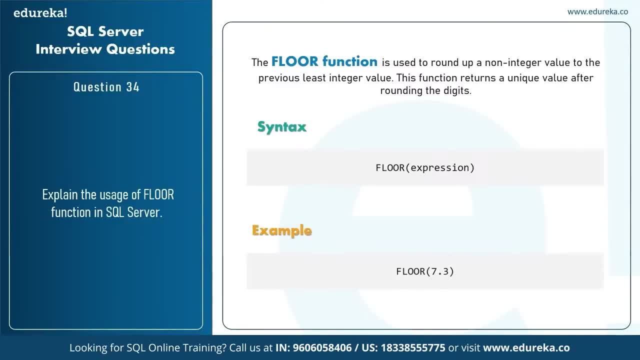 of the digits down. the syntax, as you can see in my screen, is basically floor, and then you mentioned the expression and if you also want to know how to use it, you can see the example on my screen. I've just mentioned floor and then I've mentioned, in brackets, 7.3.. 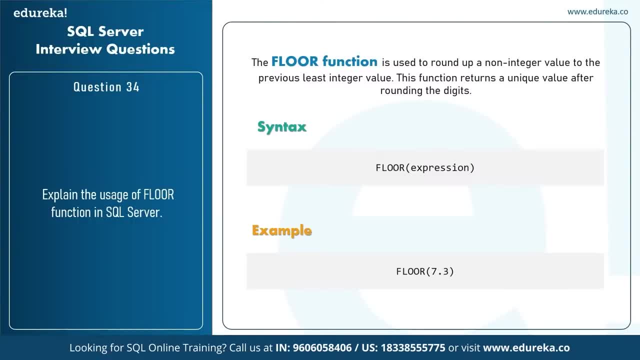 So it will basically round of the value to 7.. So, guys, that was about the floor function. Now let's move forward with the next question. That is, what is the command used to check locks in Microsoft's equal server, So to check locks in a database? 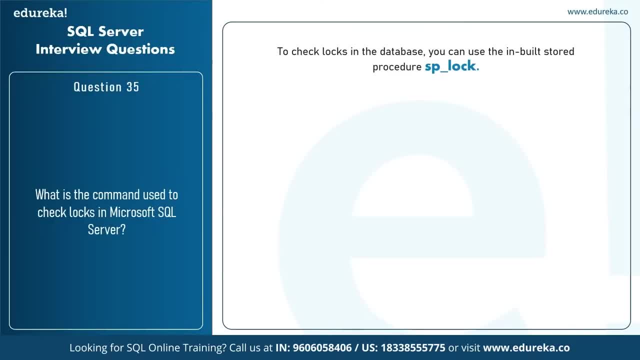 you have to use an inbuilt stored procedure, that is SP underscore lock. So the syntax is again as you can see on my screen. It's SP Log and then you mentioned at the rate SP ID equal to 1 and session ID 1. you can go forward. 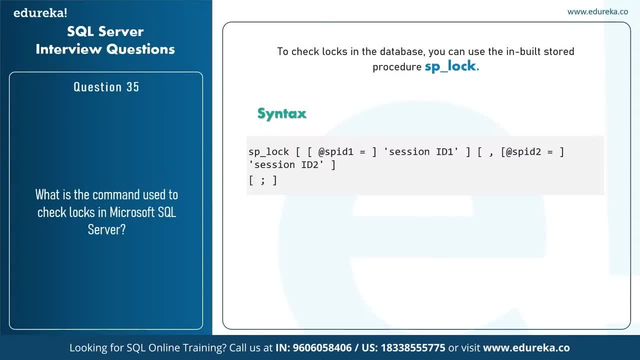 and mention the session ID 2 and so on. right, You can also go forward and explain the command to the interviewer by giving them an example, right? So, for example, if you want to list all the locks currently held in an instance of a database engine, 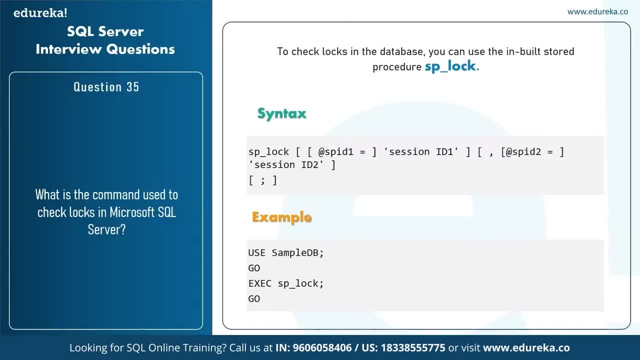 you can use the command SP underscore lock. as you can see on my screen, I've mentioned you sample database. that is basically my database name, and then I've mentioned go, execute SP underscore lock and then go again over there. So that is basically how I want. 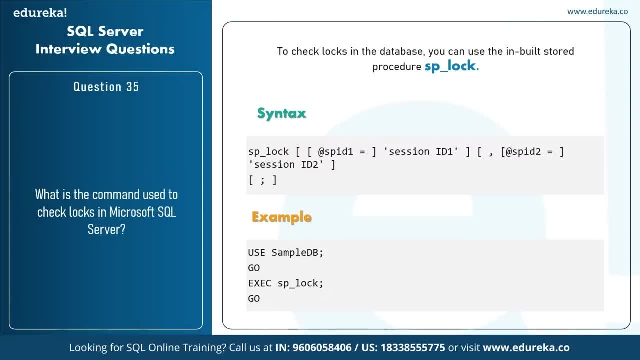 to list all the locks currently held in an instance of the database engine. Now let's move forward with the next question that is mentioned: the three ways to get a count on the number of records in a table. Now, the three ways through which you can get a count. 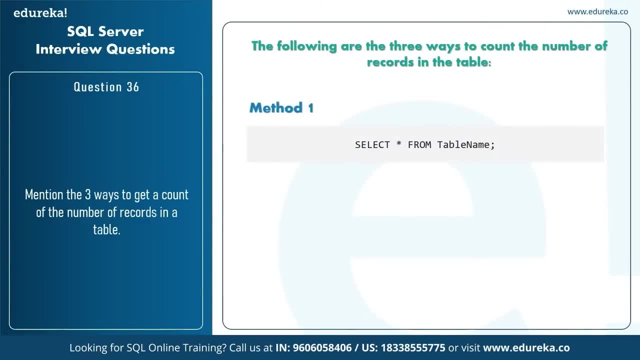 of the number of records in a table or, as you can see on my screen, you can initially write a query. like you know, select star from table name. This will basically retrieve all the data from the table, right So, and over there you can clearly get a count. 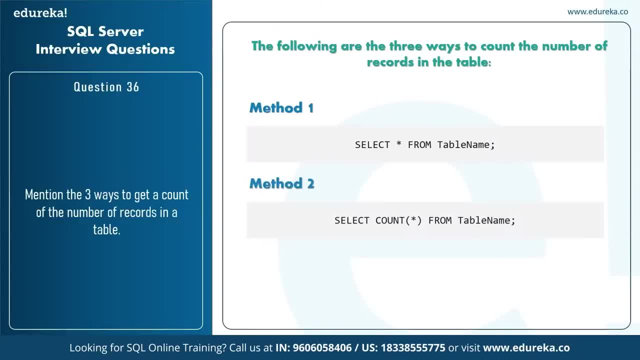 of the number of records in the table. The second way is basically you use the count function, right? So for that you'll write a query like as you can see on the screen, that is, select count and in brackets you'll mention star from table name, right? 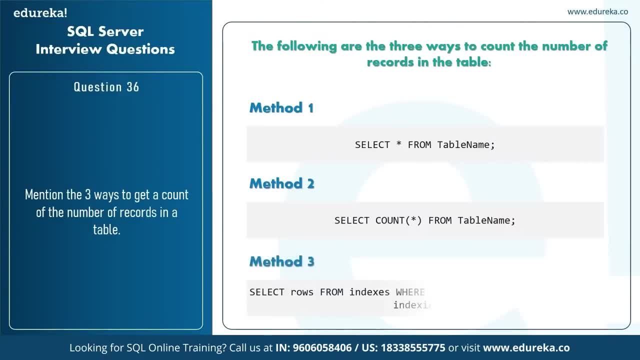 So you'll basically count all the row values and then you'll mention- and the third one is basically select rows from indexes where ID equal to object, underscore ID- You mentioned the table name- and index ID- is less than two right? So, guys, these are the three ways. 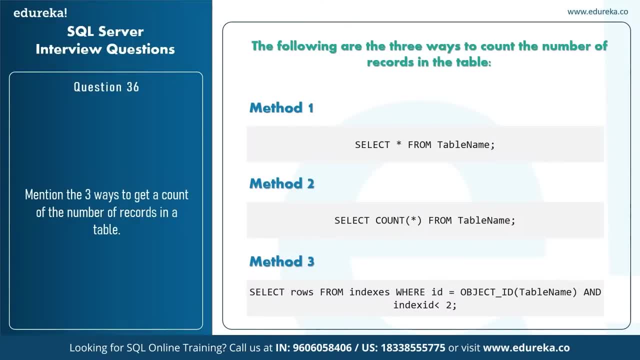 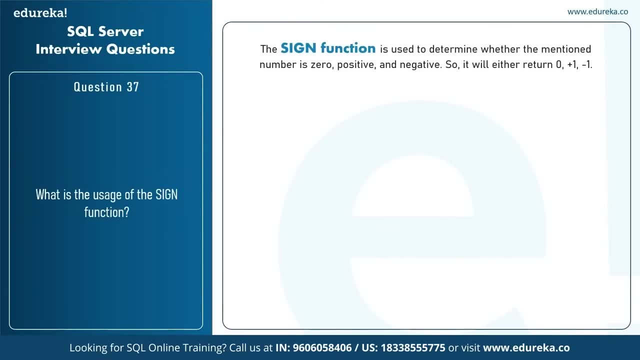 through which you can get a count of the number of records in a table. Now let's move forward with the next question, That is, what is the usage of the sine function? Now, the sine function is basically used to determine whether the mentioned number 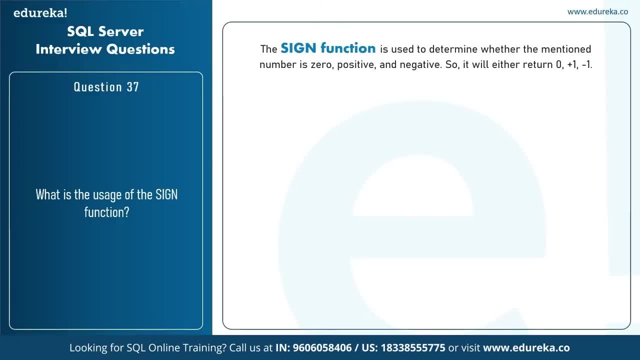 is either 0 positive or negative, So it will either return 0 plus 1 or minus 1.. So the syntax is as you can see on my screen: It's just sign and in brackets you mentioned the number. and if you want to see the example, 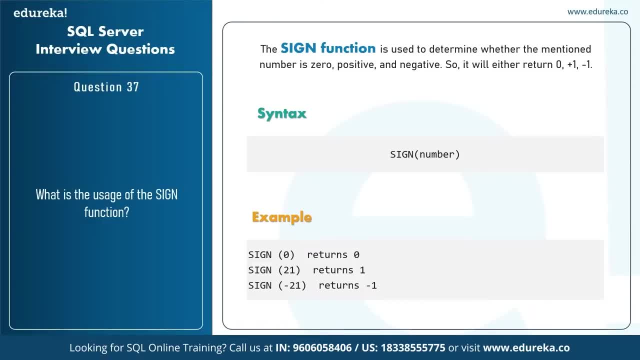 the example is again on my screen. like you know, if you mentioned sign 0, then it will return 0. if you mentioned sign, let's say 21, then it will return 1, and if you mentioned sign, let's say minus 21, it will return minus 1.. 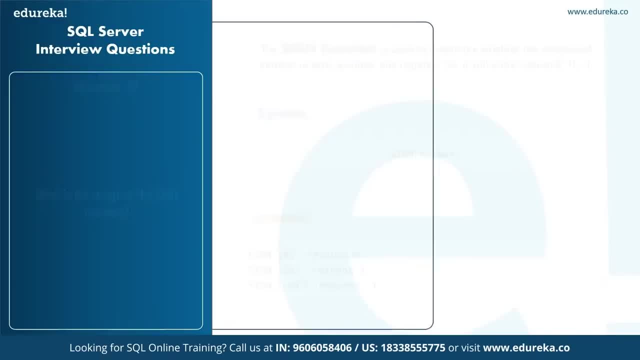 So, guys, that was about the sine function. Now let's move forward with the next question, That is, write a sequel query to find the first weekday of the month. now, to find the first weekday of the month, You can write a query like as you can see on my screen: 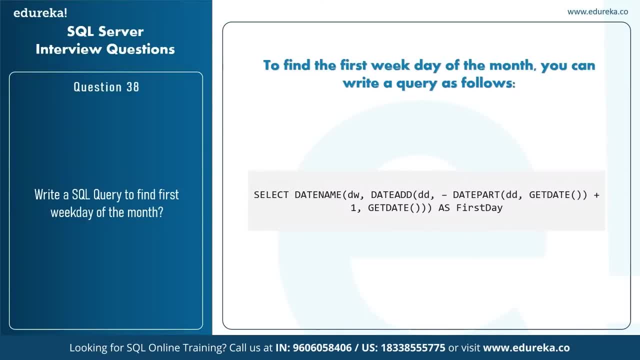 that is select date name and in brackets you'll mention the W comma date add. in the brackets again You'll mention DD comma date part and then in brackets again will mention DD comma- get date. that is basically used to get the current date plus 1 comma. 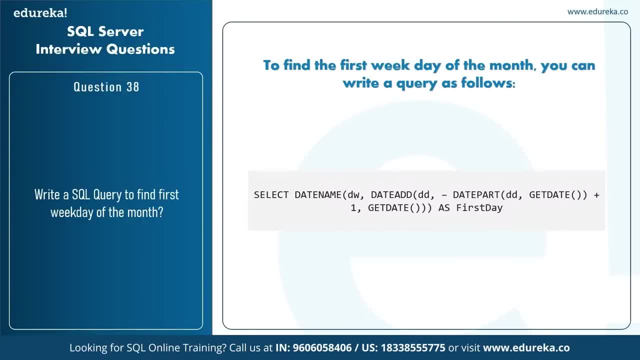 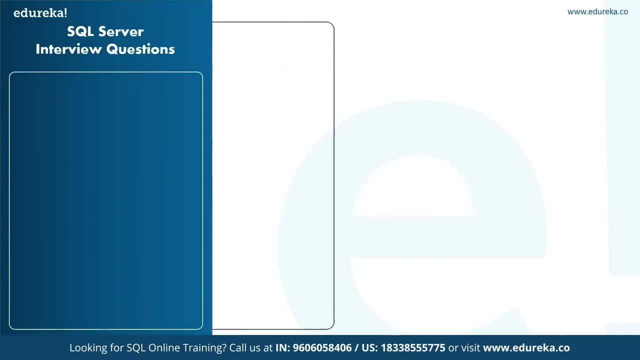 get date as first day, right. So that's how you basically get the weekday of the month, now date at date. part get date are all predefined functions that you can use. now Let's move forward with the next question that is mentioned: the command used to rename the database. 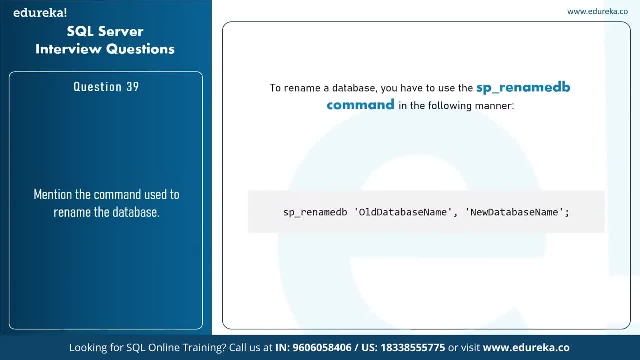 Now the command used to rename the database is SP- underscore- rename DB. So to know how to use this command, you can look at my screen. You basically have to mention SP- underscore- rename DB and then you have to mention the old database name and then the new database name. 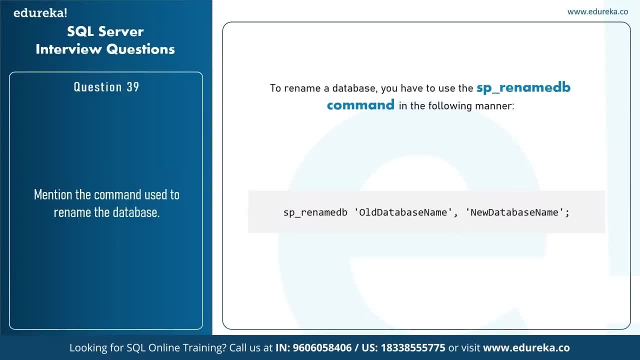 So, for example, if you have customers initially and then you want to change it to customers information, You mentioned SP underscore, rename DB, customers and the customer information. So that's how I use- you can rename the database. Now let's move forward with the next question. 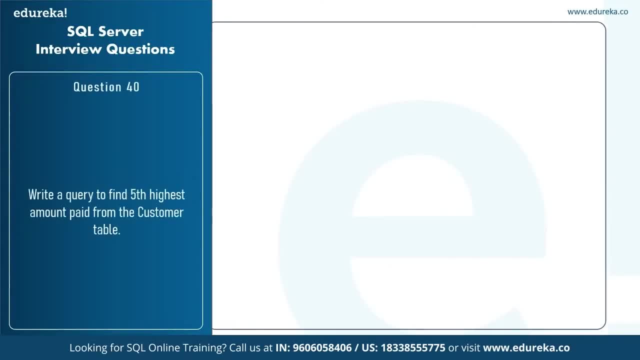 that is, write a query to find the fifth highest amount paid from the customers table. now to find the fifth highest amount paid from the customers table, You can write a query, as you can see on my screen. that is, select top one amount from and then in a brackets, 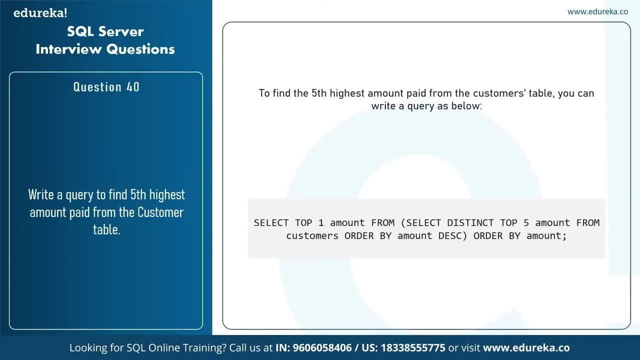 you'll mention, select distinct top five amount from customers order by amount in a descending order and then close the inner brackets and then come out of the brackets and mention order by amount. So basically in a query we're basically trying to find out the top. 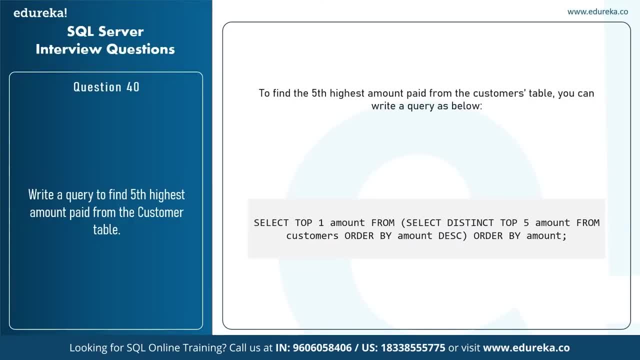 by distinct amounts paid by the customers in the customer table and then we'll order it by descending order, and when the output comes to the main query or the outer query, in the outer query it is ordered by the amount and then it is in a descending order already. 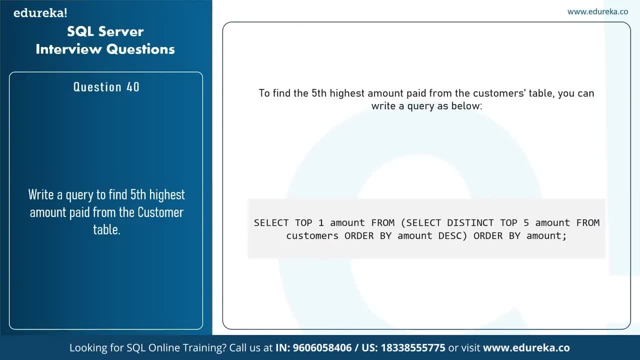 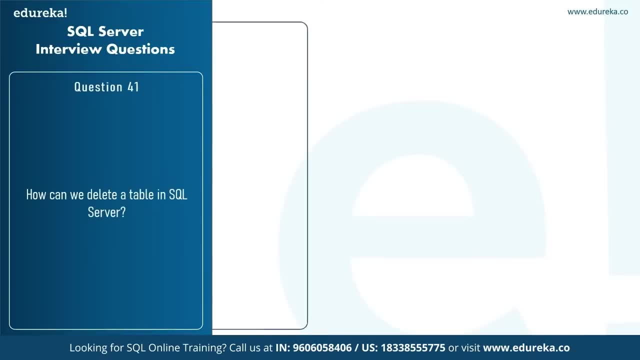 So you just pick up the first amount. So, guys, that's how you can write a query to find the fifth highest amount paid from the customers table. Now let's move forward with the next question and understand how can we delete a table in SQL Server. 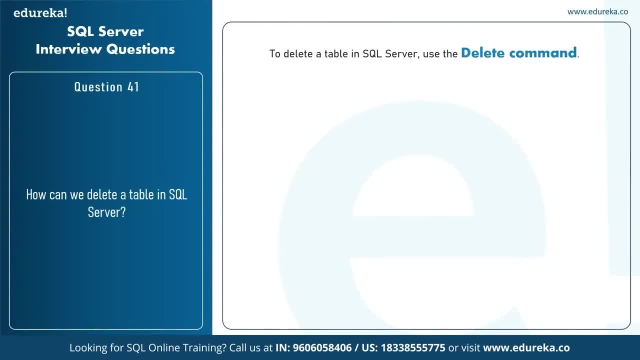 Well, to delete the table in SQL Server You basically have to use the delete command. So the syntax is as you can see on the screen. you just mentioned delete and the table name. So, for example, if you have to delete the customers table, 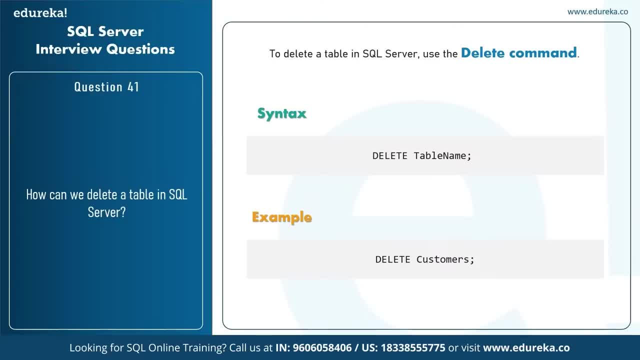 then you mentioned delete customers. So, guys, that was about how you can delete a table in SQL Server. Now let's move forward with the next question, That is, what is the purpose of update statistics and scope identity function. The update statistics function is basically used. 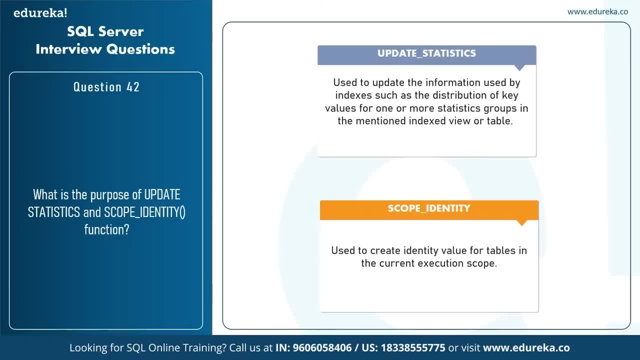 to update the information used by the indexes, such as the distribution of key values for one or more statistics groups is mentioned in the index view, or the table coming to scope identity function. The scope identity function is used to create identity values for tables in the current execution scope. 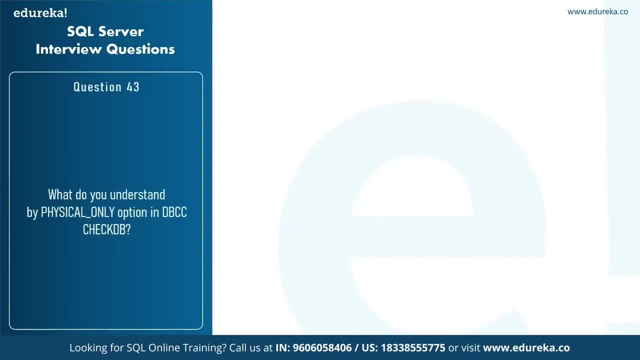 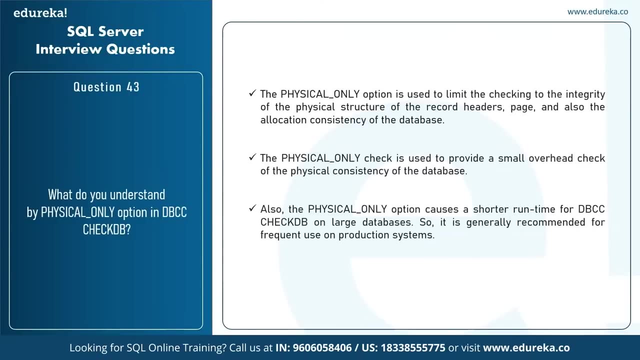 Now let's move forward with the next question, That is, what do you understand by physical only option and DVCC check TV command? Well, the physical only option is used to limit the checking to the Integrity of physical structure of the record headers page and also the allocation consistency of the database. 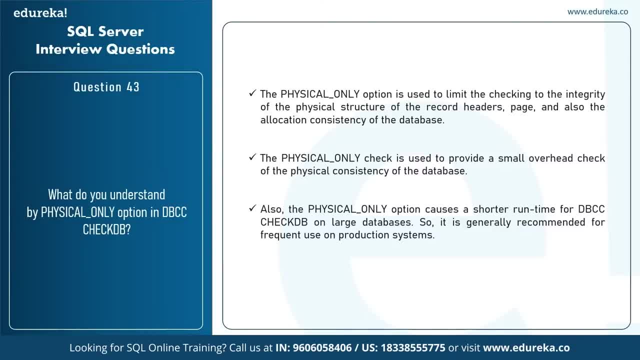 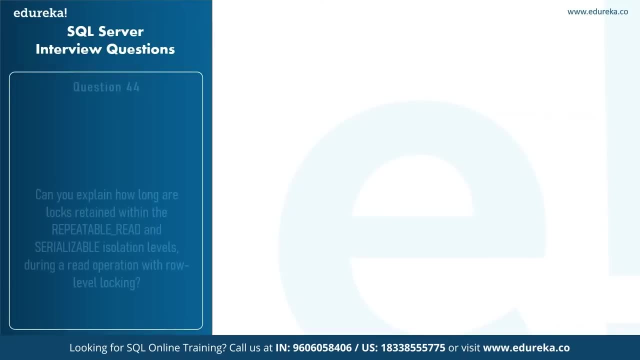 The physical only check is used to provide a small overhead check of the physical consistency of the database, and this option also causes a shorter run time for DVCC check TV on large databases, So it's generally recommended for frequent use on production systems. Now let's move forward with the next question. 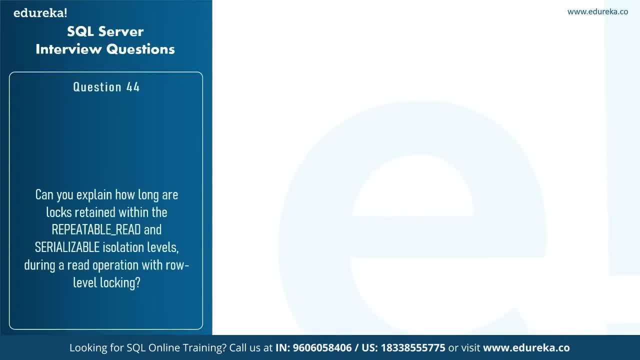 That is, can you explain how long are the locks retained with repeatable read and serializable isolation levels during the read operation? with low level locking, well, with repeatable read and serializable isolation levels, The locks are held during the transaction. answer to this particular question is that you know. 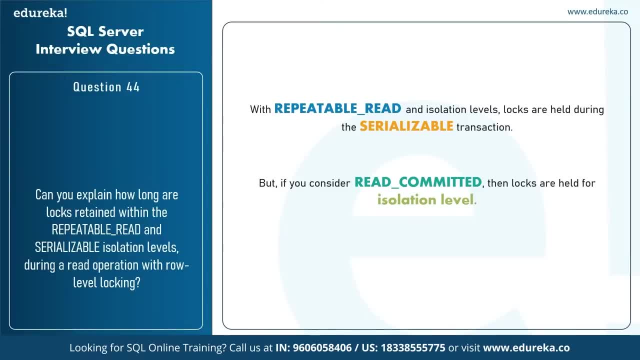 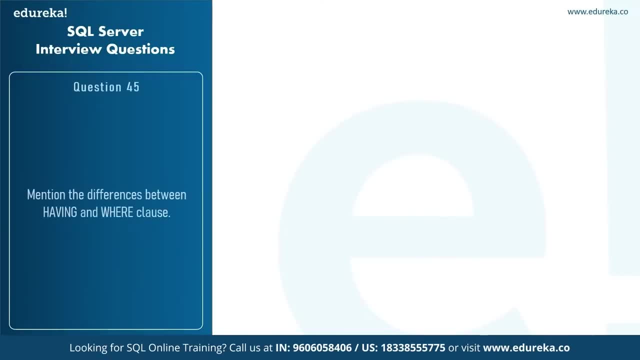 the locks are held during the transaction, But if you consider the read committed, then the locks are held for the isolation level. So, guys, that was about this question. Now let's move forward with the next question that is mentioned: the differences between having and where Claus, while the having Claus is basically used only. 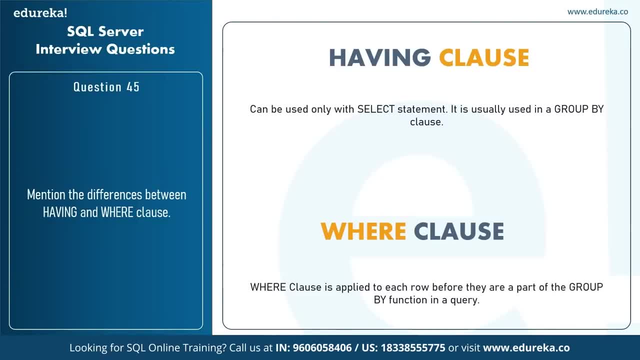 with the select statement, Whereas the where Claus is used in a group by Claus. the having Claus is used with a group by function in a query, whereas the where Claus is applied to each row before They're a part of the group by function in a query. also know 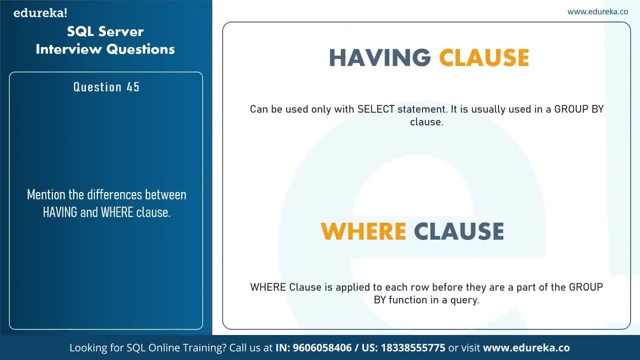 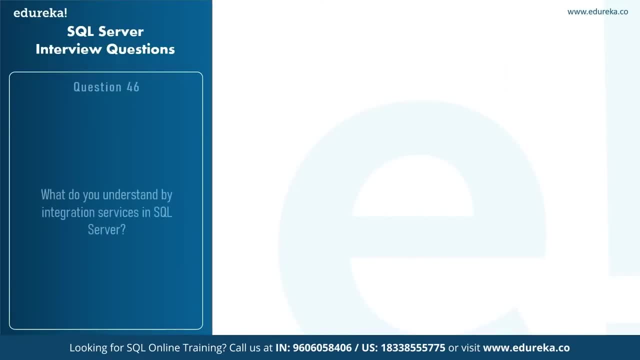 that you know. whenever group by function is not used, having behaves like a where Claus right. So, guys, these were the differences between having and where Claus is. now let's move forward with the next question, That is, what do you understand by integration services in SQL Server? 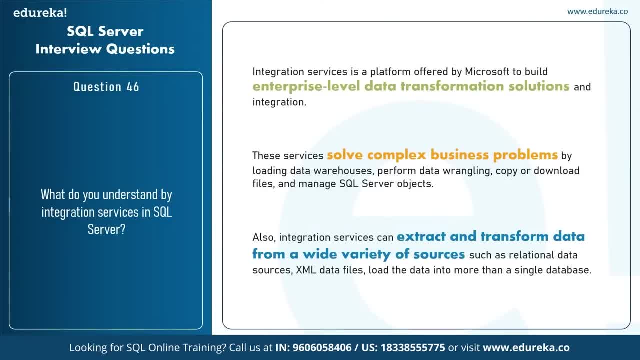 Well, integration Services is a platform offered by Microsoft to build Enterprise level data transformation solutions and integration. now the services solve complex business problems by loading data warehouses, perform data wrangling, copy or download files and manage SQL Server objects. Also, integration Services can explain how to extract and transform data from a wide variety. 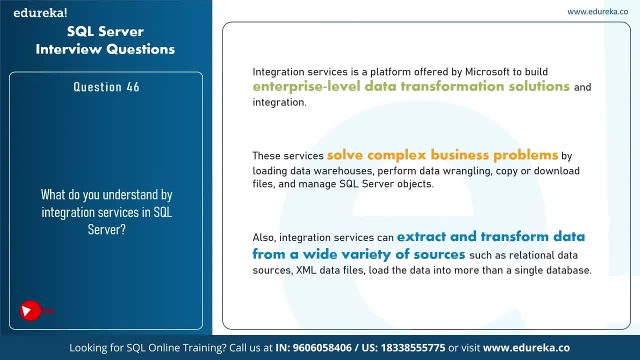 of sources such as relational data sources, XML data files, load the data into more than a single database. So, basically, you can use the integration services to create solutions without coding, or maybe code complex task program, the extensive integration object model to create objects. not only this, but the integration Services include a good set of built-in. 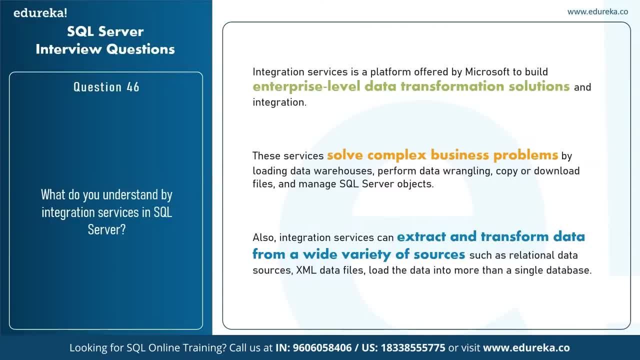 tasks and transformations and graphical tools used for building packages, and also contain the catalog database to store, run and manage packages. So, guys, that was about integration Services in SQL Server. Now let's move forward with the next question, That is: what do you understand by hot fixes? 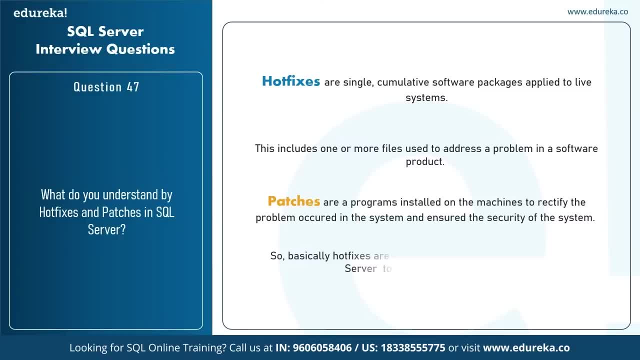 and patches in SQL Server. So hot fixes are single cumulative software packages applied to life systems. So basically this includes one or more files used to address a problem in a software product. The patches are a program installed on the machines to rectify the problem occurred in the system. 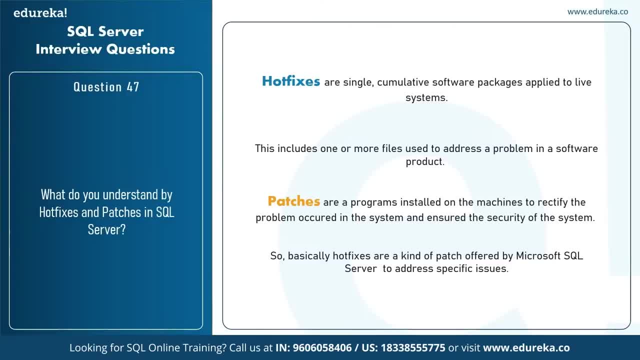 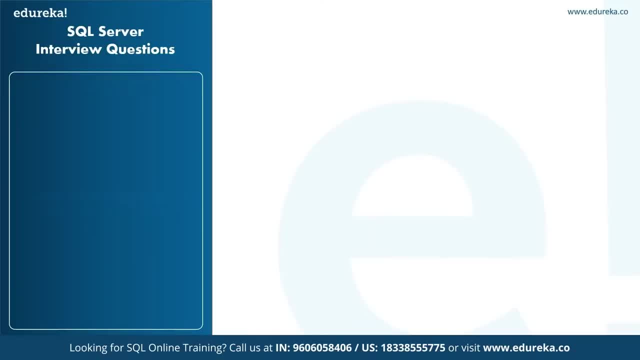 and ensure the security of that particular system. So, basically, hot fixes are a kind of patch offered by Microsoft SQL Server to address specific issues. Now let's move forward with the next question, That is, can you name a few encryption mechanisms in SQL Server? 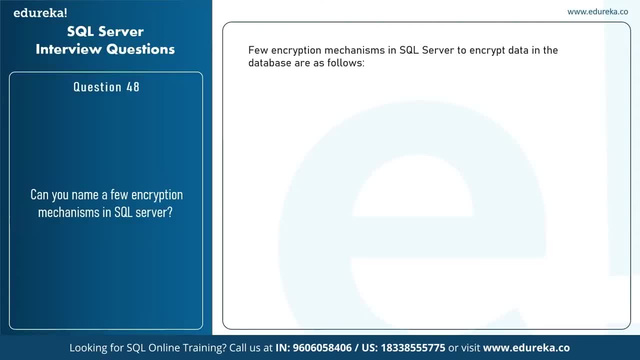 Well, few encryption mechanisms in SQL Server to encrypt the data and database are, as you can see on my screen, that is transparent data encryption: symmetric keys, asymmetric keys, transact SQL functions and certificates- right. So these are few encryption mechanisms through which you can protect your data. 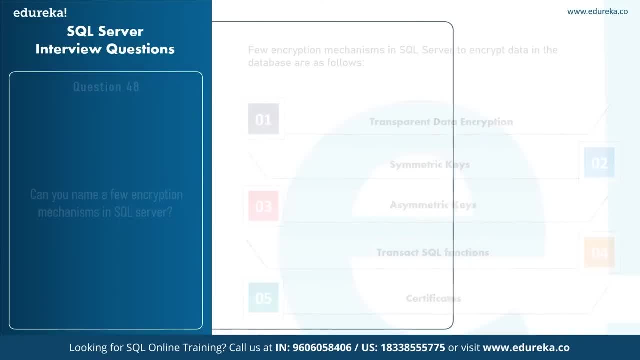 or you can encrypt the data in a database. Now let's move forward with the next question, That is, what are the options which was me sent to allow the usage of optimistic models? but the options that must be set to allow the usage of optimistic models are the read underscore committed. 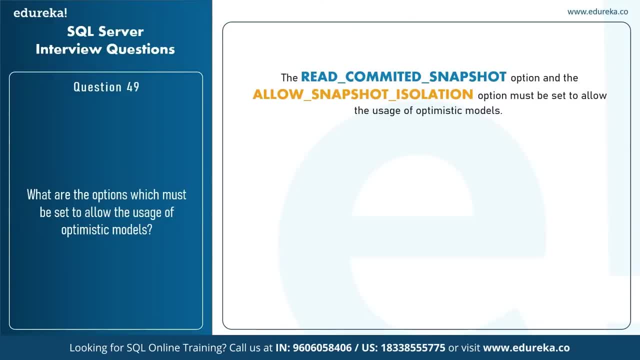 underscore snapshot option and allow underscore snapshot, underscore isolation option: right. So basically these two options are used, that is, the read committed snapshot and the allow snapshot isolation option. So the read committed snapshot option is basically used to read the committed optimistic model and the allow snapshot isolation is used. 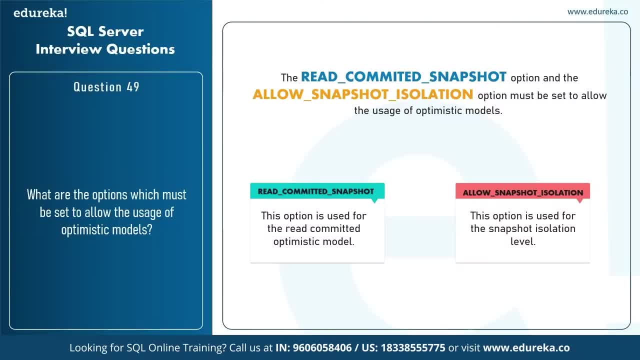 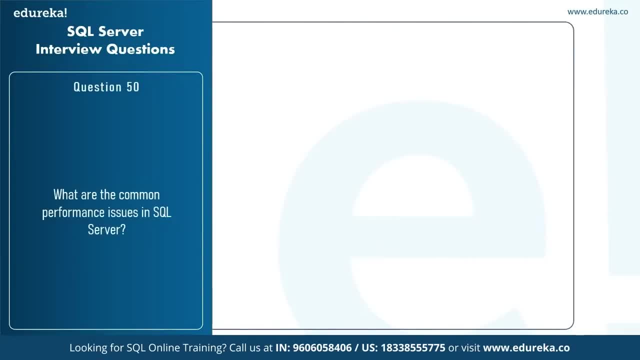 for the snapshot isolation levels, right. So, guys, these are the two options that you must keep in mind. Now let's move forward with the final question for this particular session, That is, what are the common performance issues in SQL Server? Now, this is one of the most practical questions. 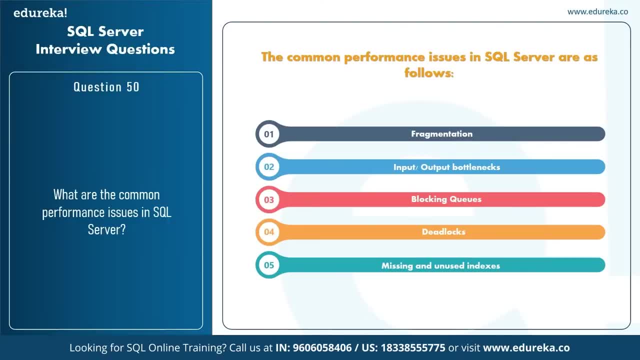 I would say that could be asked because you know it's completely on your experience basis, on how much you have used the databases and how many issues at your face. So the most common performance issues in SQL Server are fragmentation, input, output bottlenecks, blocking, queues, deadlocks and unused indexes. 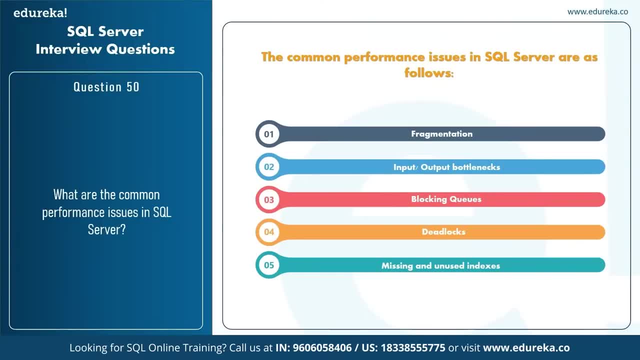 So these are few common performance issues that I had seen, but if you think you've also seen in the other issues, you can definitely go forward and mention it. So I would say in this particular question also: please explain with examples, on which scenarios did you see the performance issues? 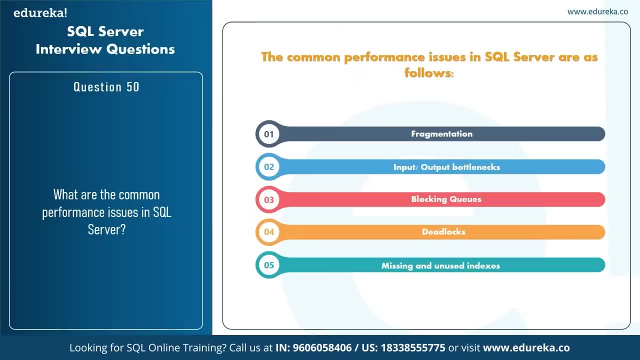 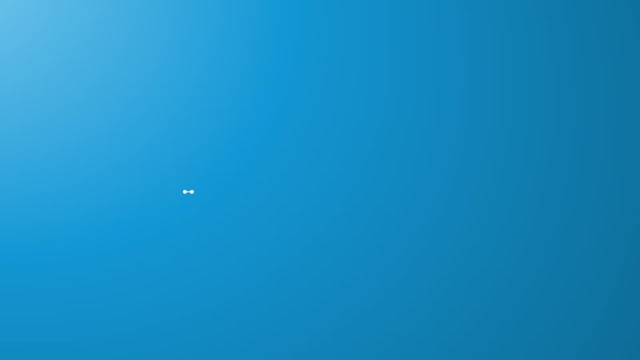 and how did you resolve it? So on that note, guys, we come to an end to this particular session. I hope you found this session interesting and informative. So thank you and have a great day. I hope you have enjoyed listening to this video. 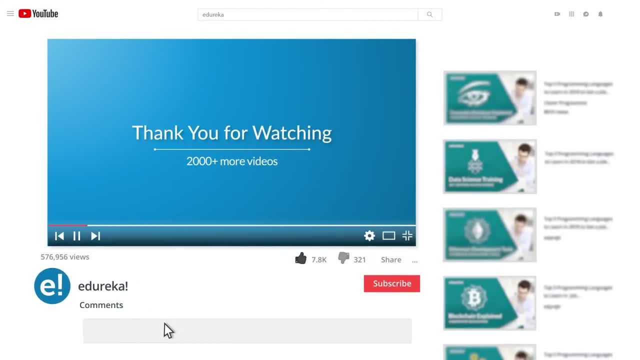 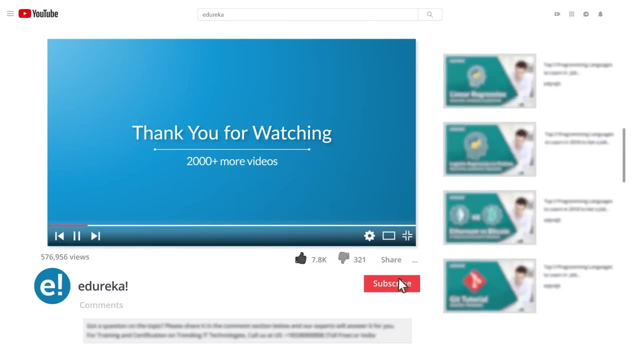 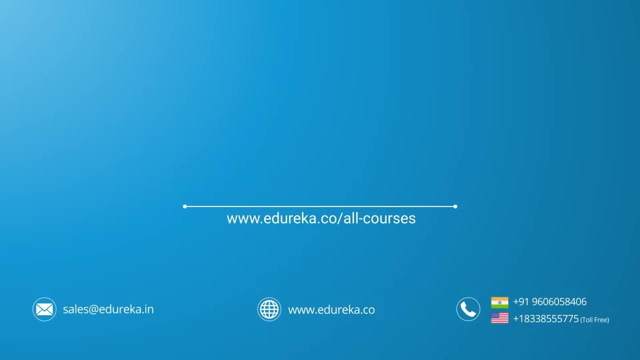 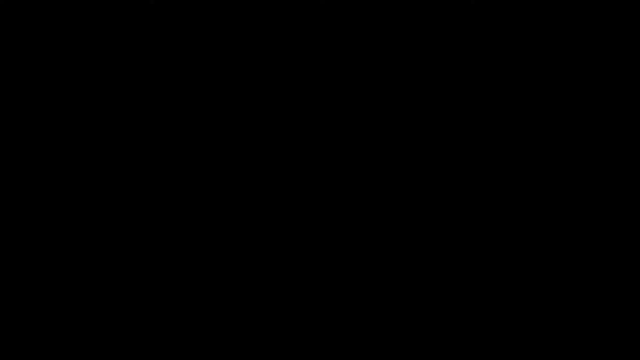 Please be kind enough to like it and you can comment any of your doubts and queries and we will reply them at the earliest. Do look out for more videos in our playlist and subscribe to Edureka channel to learn more. Happy learning, Thank you.